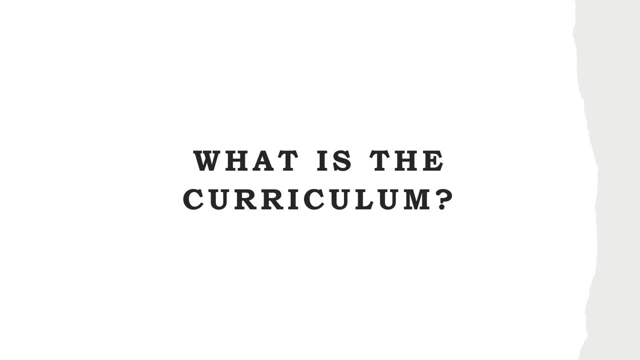 size and growth of Extended Reality over the years. In module 2, we will start to learn about a game engine called Unity 3D, which will be using to design and develop our Augmented Reality applications. Then, in module 3, we will be starting with a programming language- C sharp- that we will be using to code our 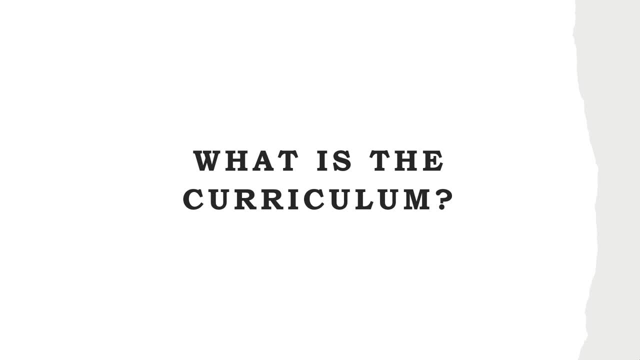 Augmented Reality applications, in which we will be learning about the basics of programming with C, sharp and many other fundamental concepts. Then, in module 4, we will start with developing our AR applications. We will learn about Marker-based AR in depth, including its architecture and. 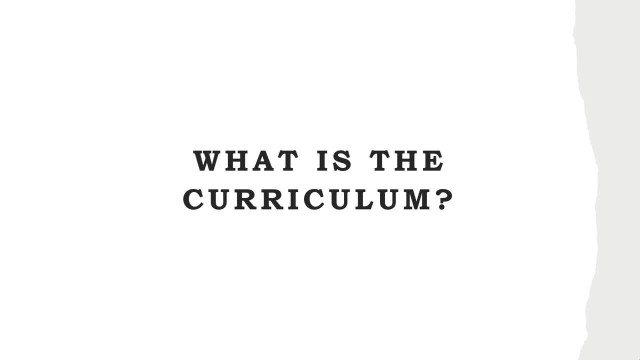 how Marker-based AR really works. Then we will be learning about the SDKs and start developing applications with an AR SDK called Vuforia Engine. After the completion of this module, we will be moving forward with module 5, in which we will be developing 3 AR applications, which includes AR Card Customizer, AR Business Card. 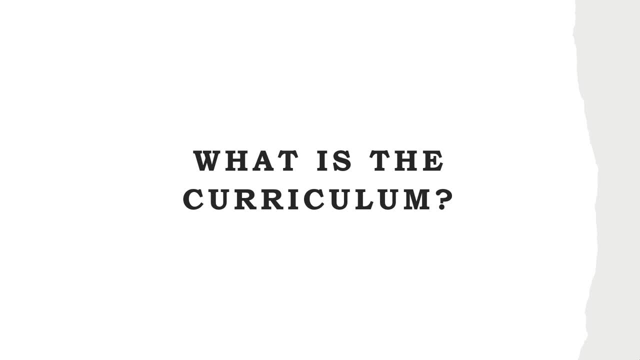 and AR Encyclopedia. After we learned to develop AR applications, we will move on to module 6, which is a bonus section, where we will be learning to develop our AR Encyclopedia. We will be using our own AR filters for Instagram and Facebook, and then in module 7, which is: 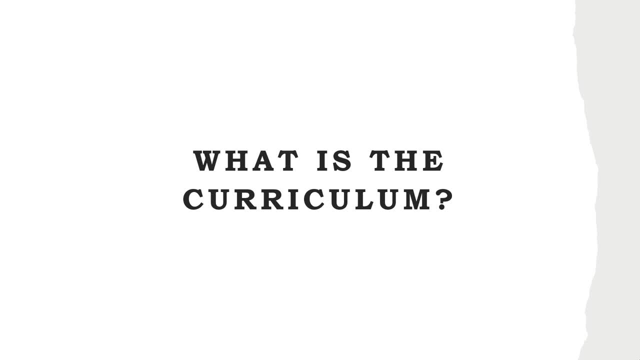 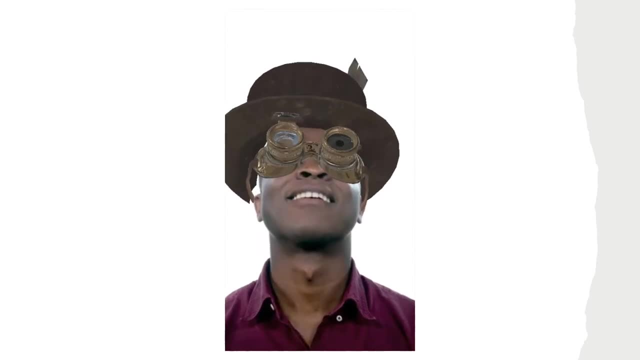 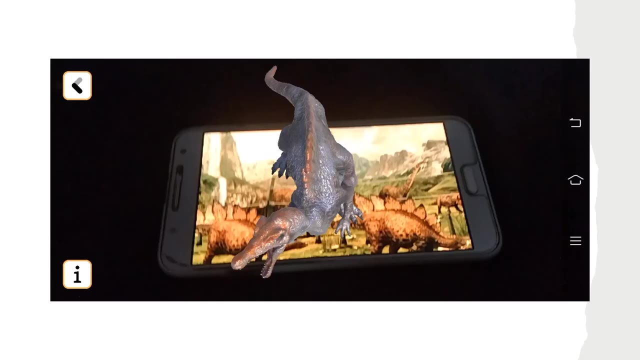 also a bonus module. We will end this course by creating our very own 3D AR Filter. Here I present to you some of the AR applications and filters we will be building throughout the course. So this is an AR filter which we will be building and this is an AR application. 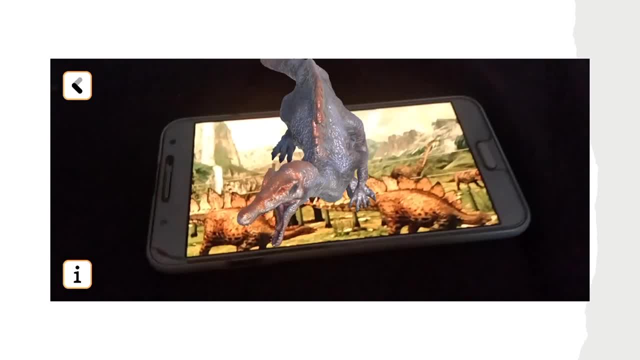 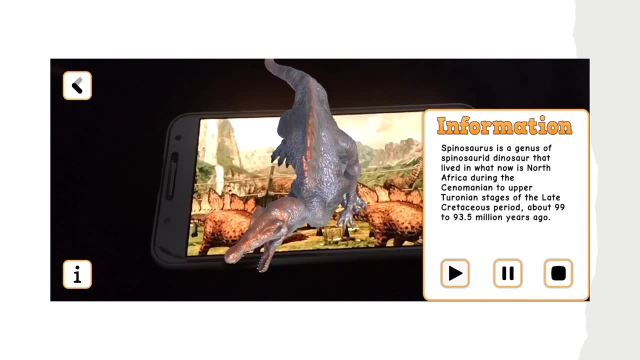 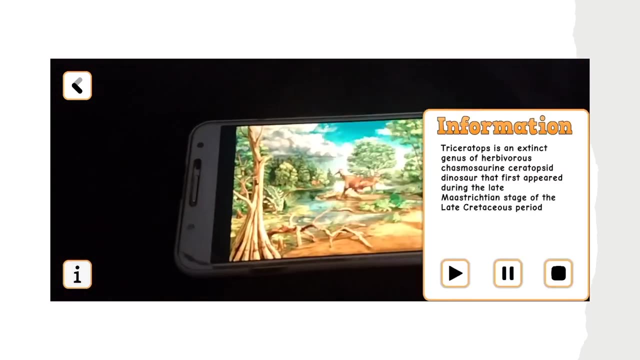 which we will be building. All right, This is an AR Encyclopedia, All right, app. but these are not only the one which we will be building. during the course, we'll be developing two more applications like ar car customizer and another one is ar business card. so who can? 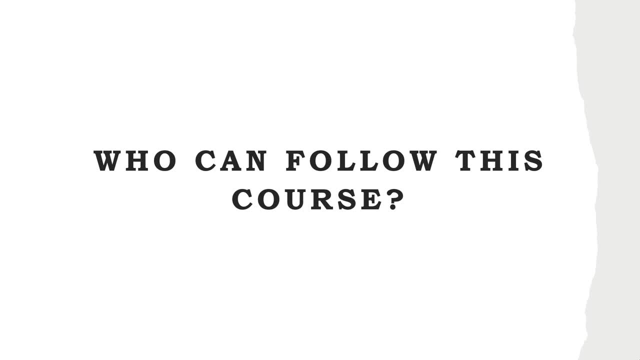 follow this course. this course is made for beginners, so you don't need any working knowledge of augmented reality to follow this course. i'll be teaching you everything from the very basics. so if you don't know about augmented reality, don't worry, you'll be learning to develop. 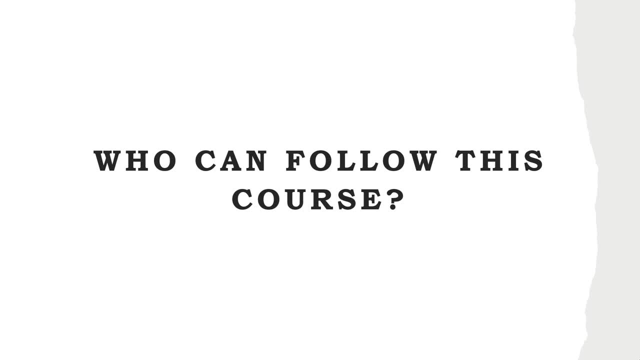 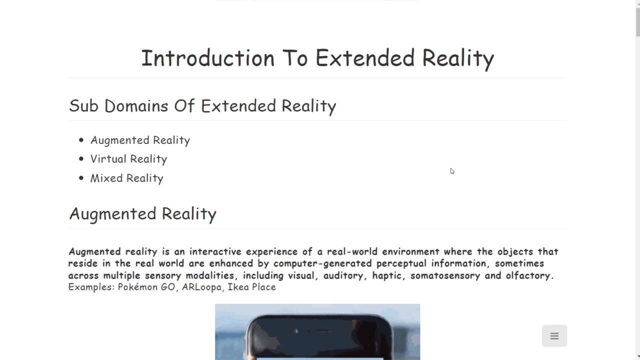 augmented reality applications from scratch. you can get more detailed information about the course from the website wwwarcoursenetlifyapp. thank you, hello folks, welcome to this lecture. this is the first lecture of our course augmented reality for everyone. in this course we are going to get 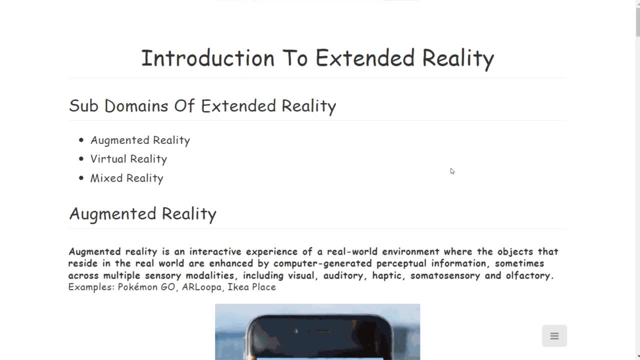 an idea of what exactly is extended reality, what comes under the hood of extended reality, that is, we are going to learn about augmented reality, virtual reality, mixed reality. we are going to learn about the mixed reality continuum. all right, then we will end this part of the lecture by understanding the growth. 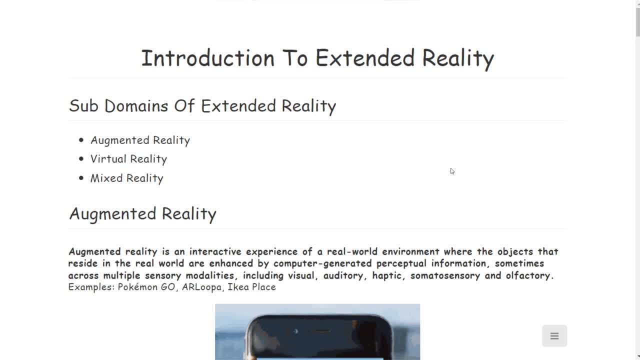 of you know the growth of extended reality over the years and what we are projecting by the year 2025. all right, so, without any further ado, let's understand. all right, see extended reality. now try to understand extended reality in this way. it is the extension. all right, it is the. 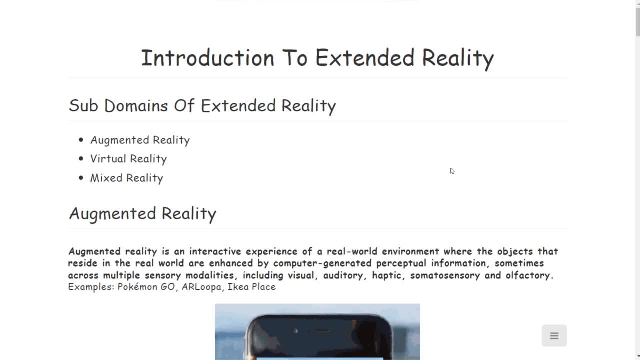 extension of our current reality. all right, you can see that it is the a virtual. all right, it is a virtual extension of our current reality. all right, you can understand extended reality, uh, like this. all right, there isn't any specific. all right, there isn't any specific definition that would you know. 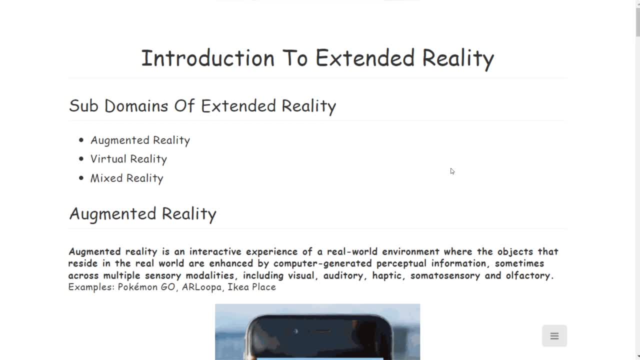 uh, do justice to this, uh, whole domain, all right, but how i like to explain extended reality is: it is the extension of our current reality. that and, uh, it is the virtual extension of it is the virtual extension of our current reality. you can say: extended reality is the hood, all right, means it is the roof and that roof has. 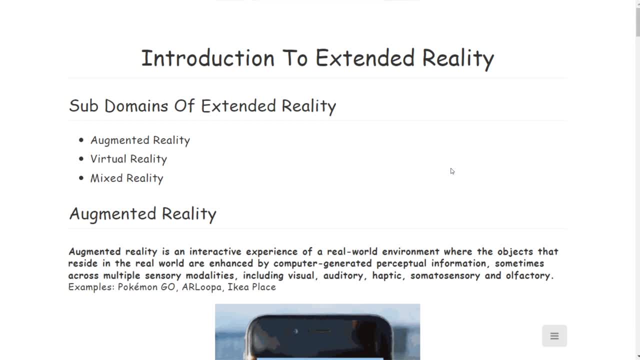 three children. all right. those three children are named as augmented reality, virtual reality and mixed reality. all right. so extended reality is the main hood and it contains three other domains: augmented reality, virtual reality and mixed reality. all right. extended reality is a parent domain. all right, now, as we have understood what exactly, uh, is extended reality? right? what are the? 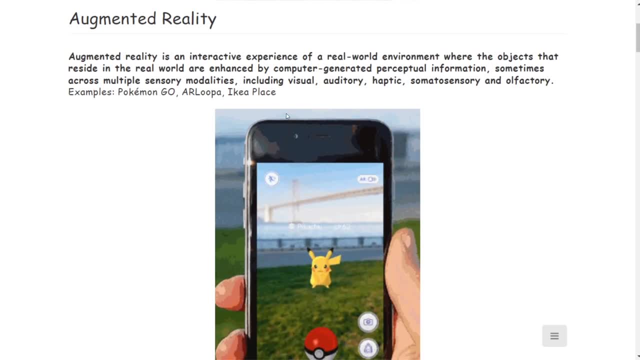 subdomains of extended reality. let's you know, let's understand what is augmented reality. all right, you see, you might have, all right, you might have, uh, experienced augmented reality in your life, but you it might happen that you didn't knew that it was augmented reality, like you know, when 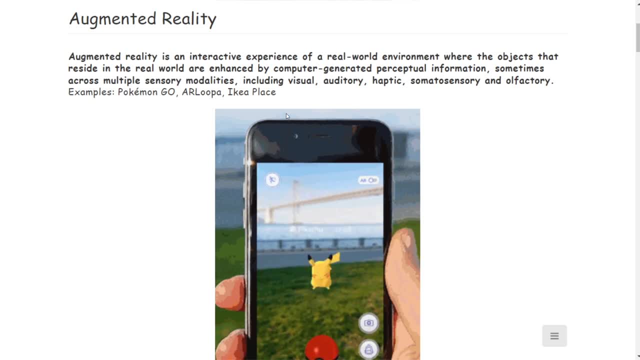 you used to play, uh, pokemon go when i, i guess it released in 2016. at that point of time, i was very excited to play that game. all right, just because i could- uh, you know, the spawn the pokemon. all right, i could bring the pokemon into the real world, all right, it had a ar feature that could you know by. 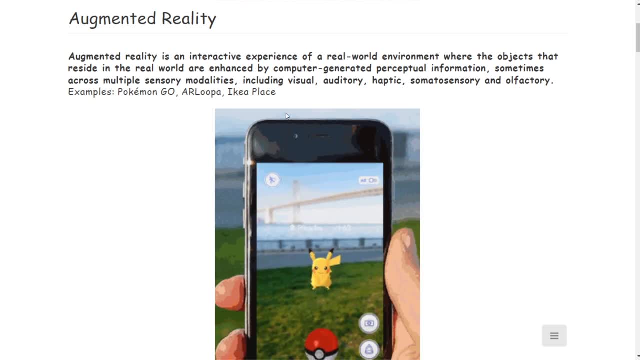 pressing the ar camera, we could bring the pokemon into our real world. all right, i was very excited about that feature. all uh. the reason why i didn't uh what? i wasn't able to play the game because, you know uh, i wasn't able to roam around for free, like it had gps enabled, right. so i the only reason why i played the game. 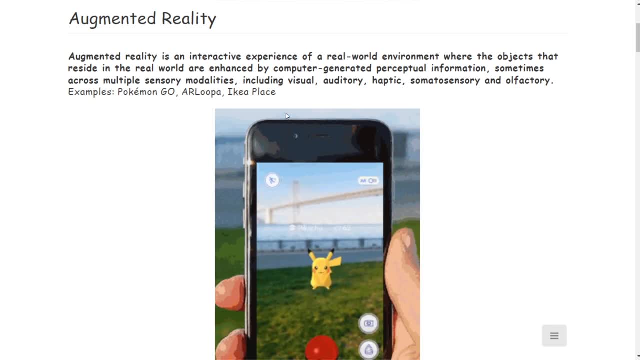 was because of its ar feature, and at that point of time i didn't knew what exactly augmented reality was. i didn't even knew how this thing worked. all right, at that point of time i just started with programming, all right. so, uh, we have. we all have used augmented reality at some point in our life. 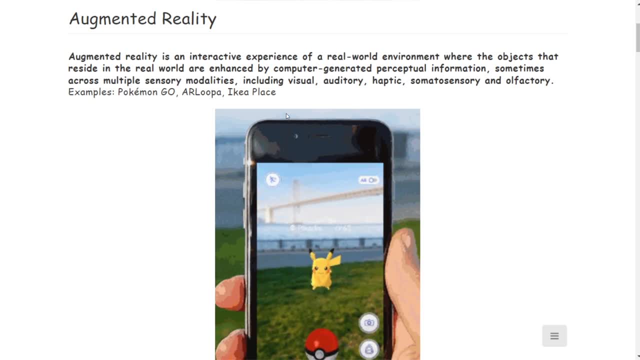 and didn't knew exactly what it was right. so one example you already got all right: the one with pokemon go. now, people used to think, uh, that pokemon go is one of the biggest big breakthrough in augmented reality, but it is not. the truth is this? because, see, if if i, if you, look in after this course. 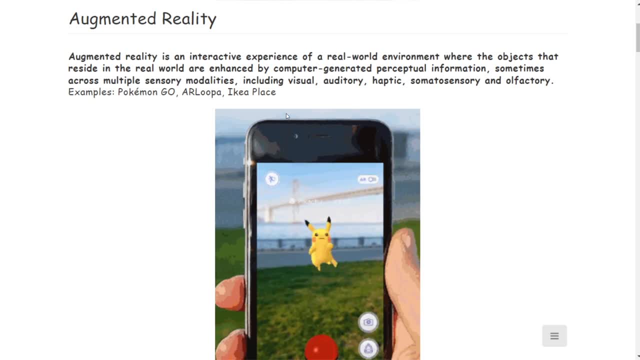 all right after this course, if you look into that now, creating the mechanism. all right, that is the pokeball throwing mechanism to the uh, pokemon, it uh. that mechanism is very simple to make. all right, that mechanism is very simple to develop. it's just we are throwing it through a projectile. 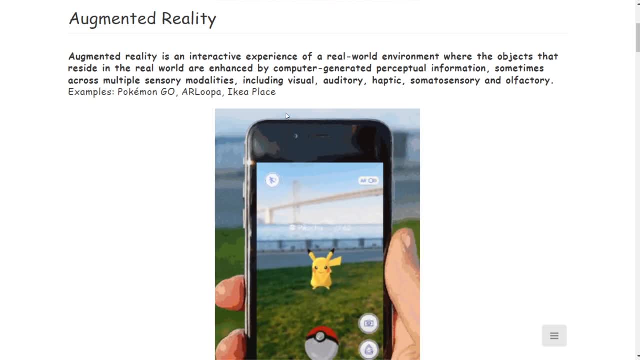 uh understand it like this: all right, basically, augmented reality is nothing. augmented reality is nothing. but you know uh bringing all right, that is, uh augmenting. or you know putting the digital objects all right in, in our case the digital objects like uh in pokemon go pikachu. 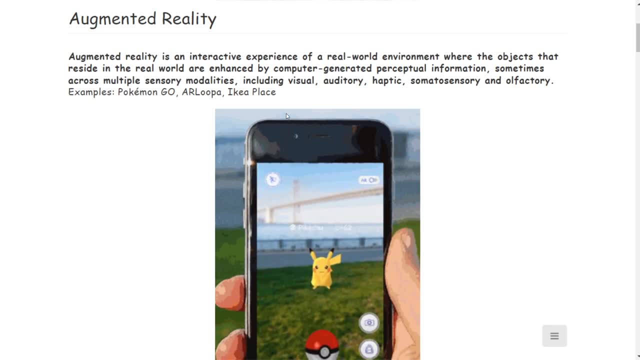 is a digital object, right? so we are taking the digital object, all right, and placing it into our real world. that is what augmented reality is how we are placing it. we are placing it through our. don't worry, we are going to understand, all right, how all these thing works. all right, how. 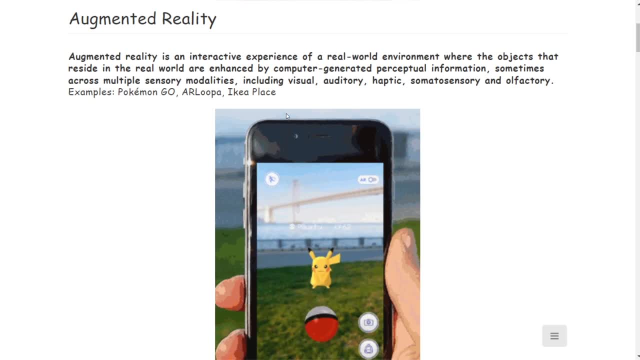 augmented reality actually works right? how? what is the architecture in our future videos? but for now, understand it like this way that we augmented reality is basically the augmentation, or you can say the placement, of digital object in real world, like, for example: take your favorite cartoon, all right. for a long time back, my favorite cartoon cartoon was doremon. all right, i used to watch it. 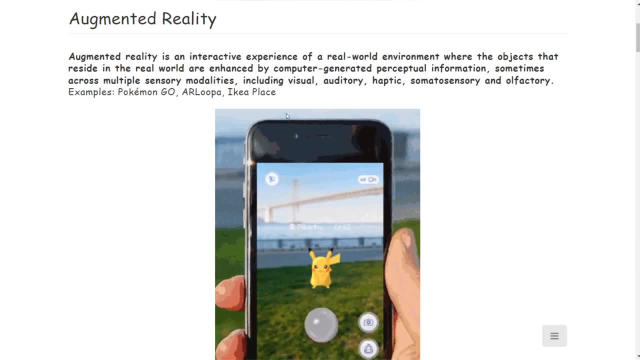 like all day, i love that cartoon when i was like in class third or fourth. so at that time, uh, if i knew about augmented reality, i would have surely tried that. he, uh, i would have tried augmenting doremon into into my room. all right, i would have tried that. so 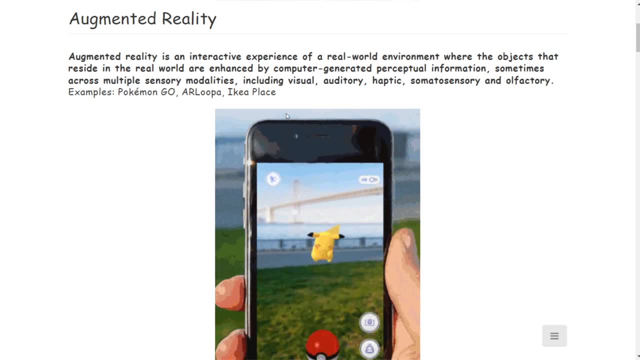 just think of it this way: you are actually bringing your favorite digital uh character all right into your real world. so that is what augmented reality is. that is basically what augmented reality all right, it is basically the placement of digital object into the real world like all right. and now, as i have, 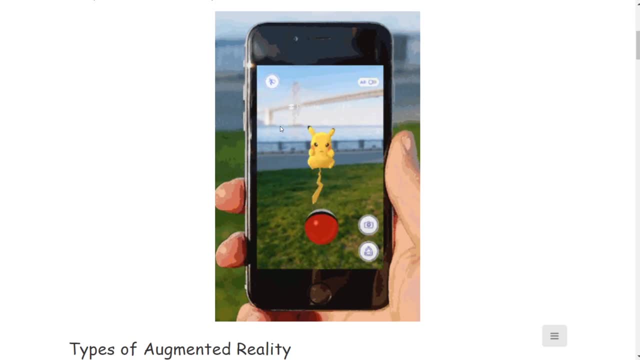 told you, as i have told you now, you, you might know. all right, you, you, you, right now, you are aware of what exact, uh, how you know, pokemon go uses augmented reality. right now, what i wanted to do is, after finishing this lecture, install that game and try it out. try it out by yourself, see how. 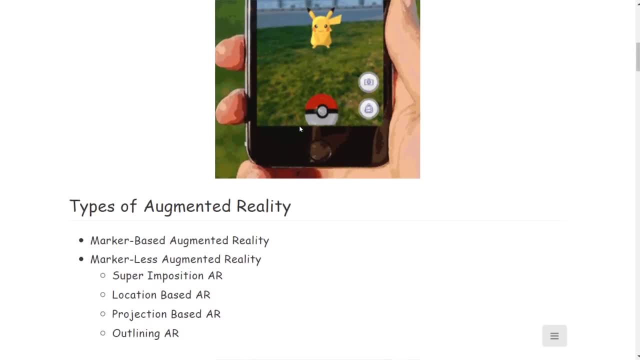 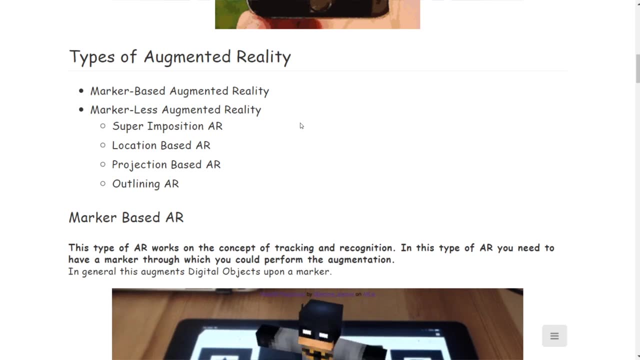 exactly the ar feature is working all right. it would be really fun, believe me. now there are, uh, mainly all right. there are many majorly two types of games that are available right now. the first type of augmented reality: marker based augmented reality, marker less augmented reality- all right, in markerless. there are four other types of augmented reality. that is super imposition. 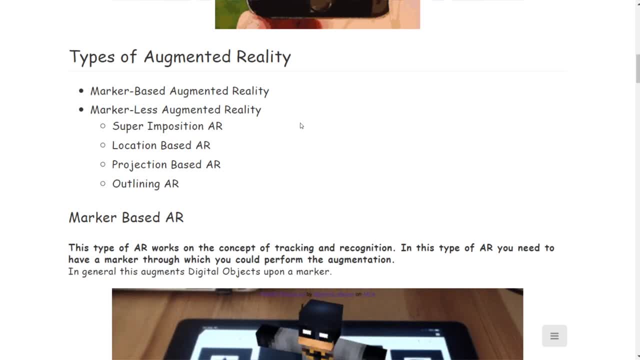 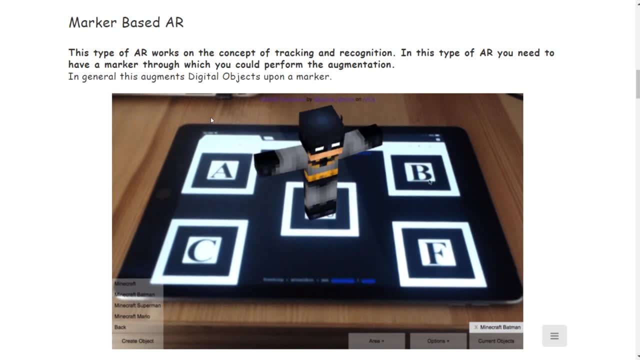 location based projection and outlining. all right, don't worry, i'm going to uh make you understand what exactly are these? all right, so let's start with marker based. see the meaning of this already. the meaning of marker based is in its name only. marker based ar means the augment, that or the 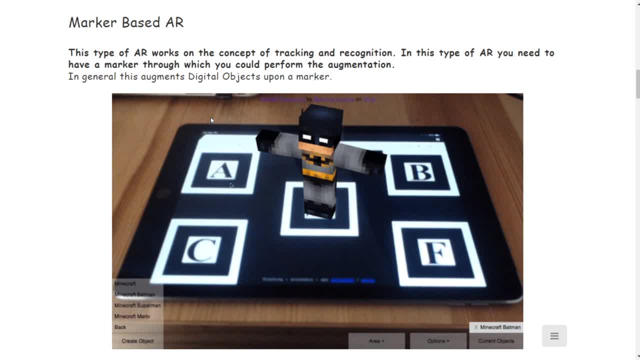 augmented reality feature works only if- uh, there is a marker, all right, only if it. there is a marker to help augment the object, all right. that is what augmented marker based augmented reality is basically now. this type of ar basically works on the concept of tracking and recognition, all right. 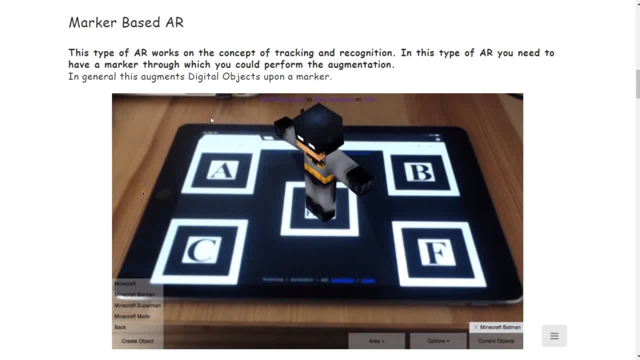 it first tracks the marker means it first recognizes the marker and then tracks it, tracks it all the way long. all right, so that is how this marker based ar works. all right, basically, in this type of ar- now you would be- you will be needing, all right, you will. 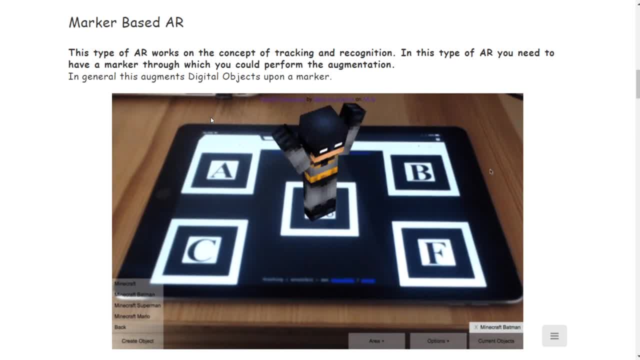 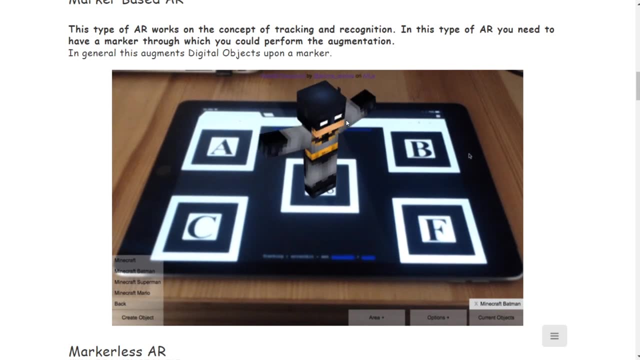 be needing a marker to augment, all right. you will be needing a marker, uh, to help augment, uh, the digital object in the into the world, all right. like like in here, all right. like in this, you can see that this, uh, lego batman, all right. or you can see this: minecraft. 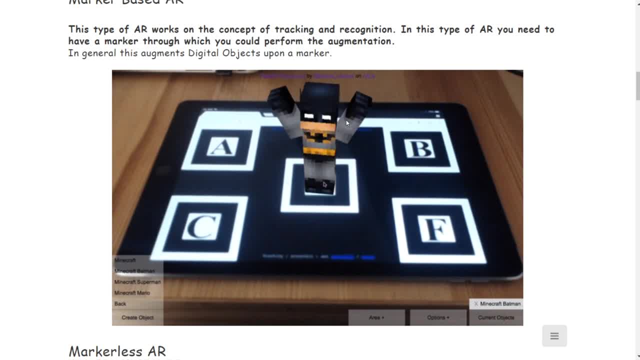 blocked batman, all right, is being augmented. this, uh, this particular minecraft shaped man is being, uh, what can i say? is being augmented on top of, uh, a marker. all right, here you can see, it is being augmented on top of a marker. so this is what marker based augmented reality to augment. 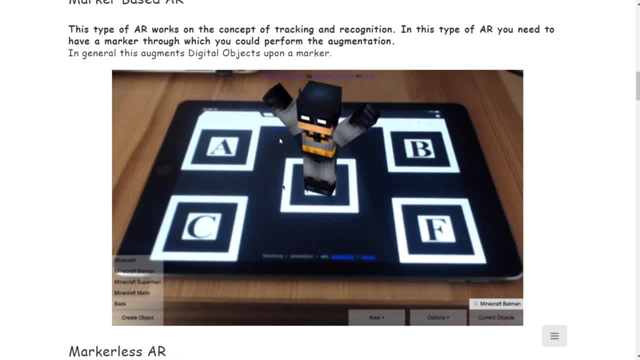 this kind of uh. to augment digital object, we would be needing a marker, all right. so that is what marker based augmented reality is all right, and in this course we will be developing marker based ar, all right. so if you are not clear with the concept right now, that's totally fine, all right. 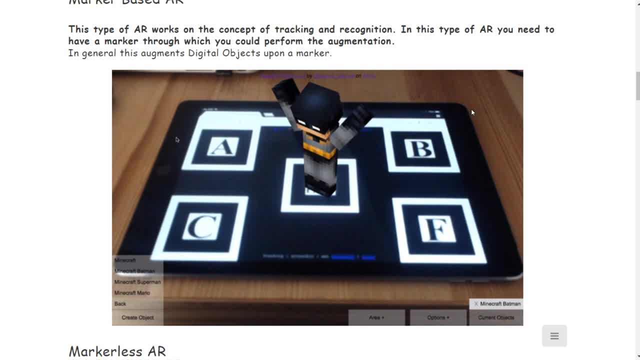 uh, you, you would be. when you will be developing, uh, a marker based ar app by yourself, you'll be very clear that, how exactly that those things work. all right, but for now, in simple words, uh, marker based ar is something all right that would be needing. all right, in which we will be, we'll be needing. it is mandatory to have a marker. all right, it is. 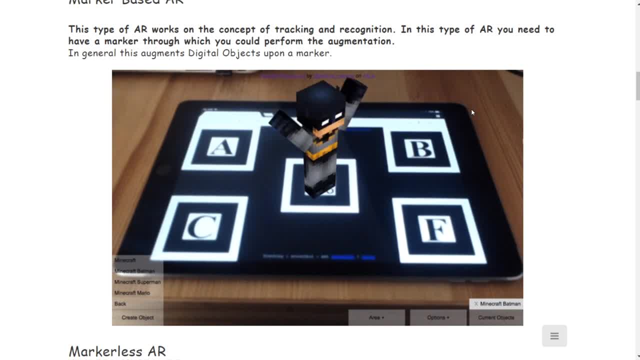 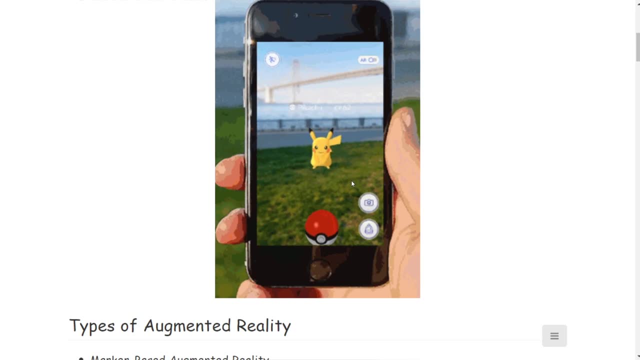 mandatory to have a marker to augment the digital object on top of it, or or else you won't be able to, you know, or else you won't be able to augment it. all right. so that is what marker based augmented reality is all. right now. uh, pokemon go is not an example of marker based augmented reality, all. 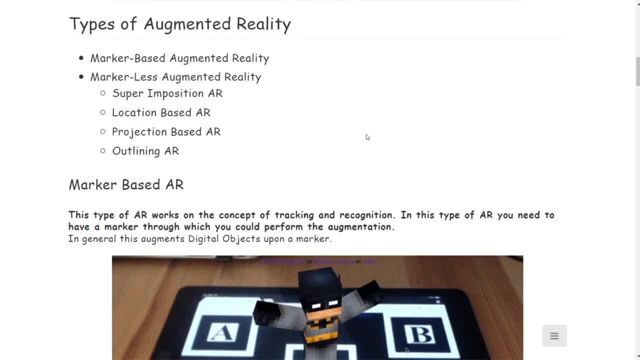 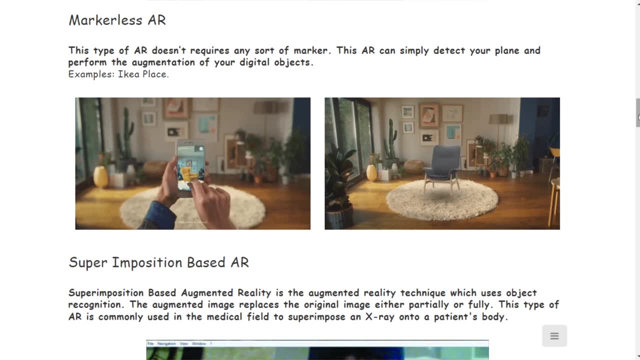 right, i would tell you: uh, what example is it for? all right now, let's understand what is uh. marker less ar. all right now, as we have understood about marker based ar, markerless ar is the total opposite. all right, the difference between them is all right. the difference between them is marker based ar. 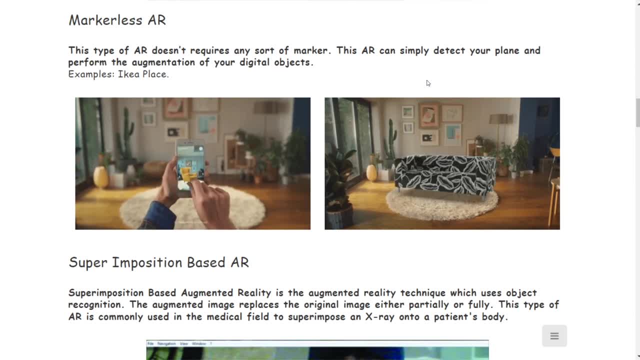 that is, it needs some you know, point. or you can say some something to: all right, it needs something to augment, all right, it needs. and that thing is a marker. so marker-based augmented reality needs a marker to augment, but markerless AR doesn't. now there are some algorithms all right, like 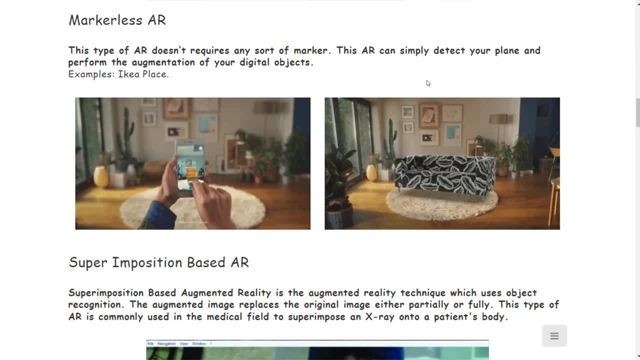 simultaneous localization and mapping is an algorithm that is used. all right, that is used to map the whole, you know, the whole environment around us and then place the objects in there. all right, so markerless AR doesn't need all right, markerless AR doesn't need any sort of marker. 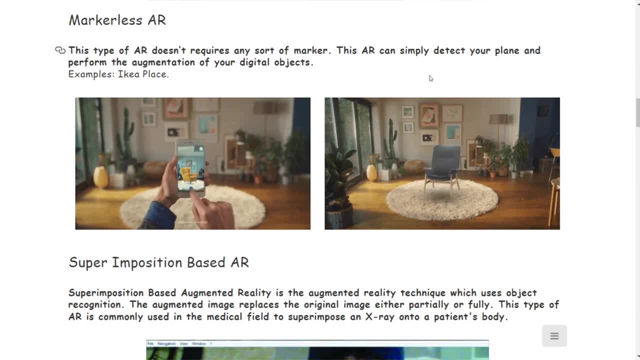 what it does? it will scan the. let's say, if I am trying to augment some object in my room, what will it do? it will scan the surface, it will scan the walls. all right, it would create- you can say it creates- a virtual, you know visualization of itself and then you know it will place. all right, 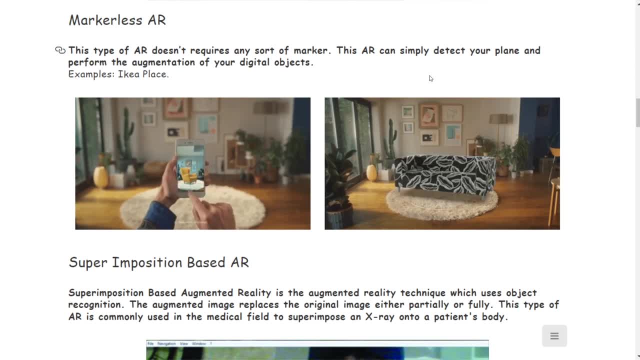 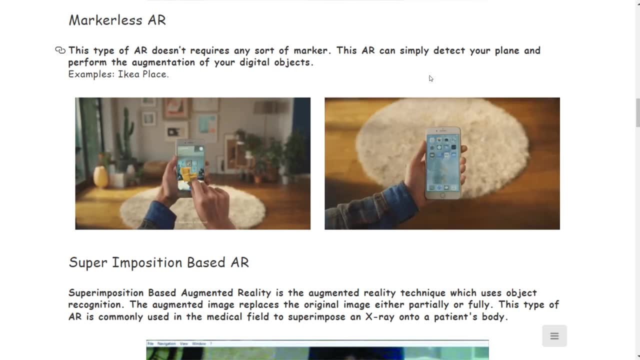 it will place the object right in there. all right, so it would first scan the room. all right, it will first scan the room. after scanning, it will place the object, all right. now, how it will scan, there is an algorithm. it's it's a very widely used algorithm. it is also used in robotics, but it 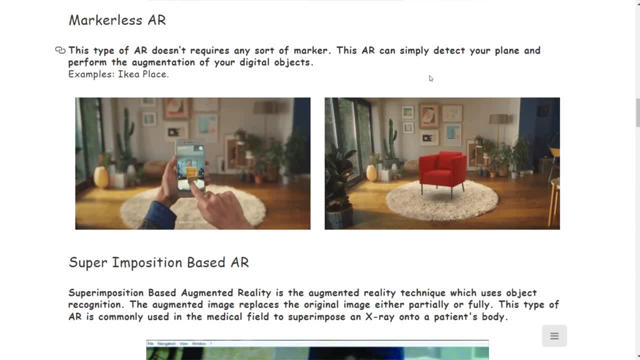 is also used in virtual reality, augmented reality and virtual reality. it is known as SLAM, that is, simultaneous localization and mapping. all right, so that's how we, you know, build markerless AR features. all right. so markerless AR is is very simple. it will this AR, will you know, simply detect your. 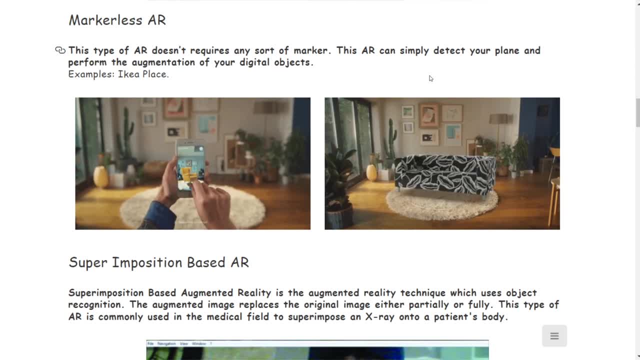 room, or means the plane, the vertical and horizontal surfaces of your room- all right, that is, the planes- and perform the augment, augmentation on those particular planes of those objects. all right means it will augment the digital objects on on top of those planes that your AR app has detected. 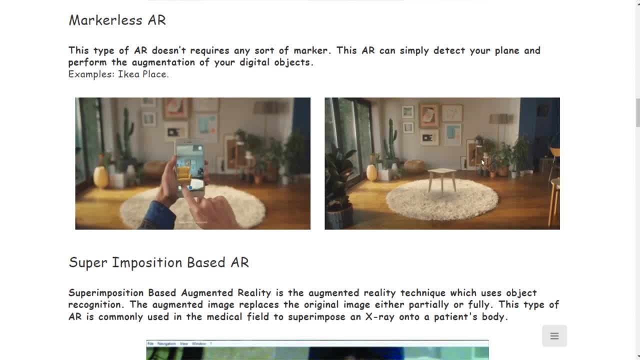 right now. for example, in this you can see this IKEA place app. all right, this is the demo of IKEA place. basically, this is a very famous, you know, uh, furniture app that you know makes use of markerless augmented reality to help you decorate your room. all rights like if I, let's say if i want. 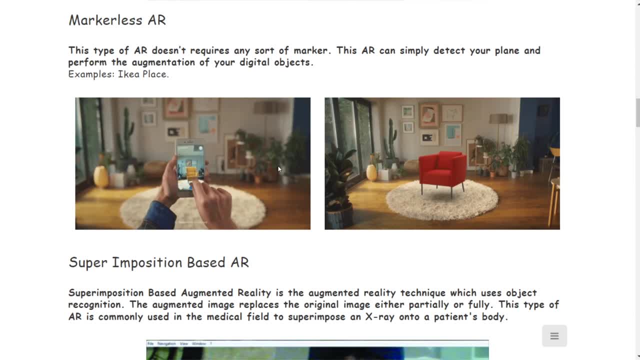 to buy a sofa. all right, like you can see it in here, what i'm doing is i'm installing the Ikea place app. i'm searching for some sofa in there. i i like that sofa very much, but i don't know, will, uh, that sofa, will you know, fit my home or not? fit might, in the sense it will look good in my. 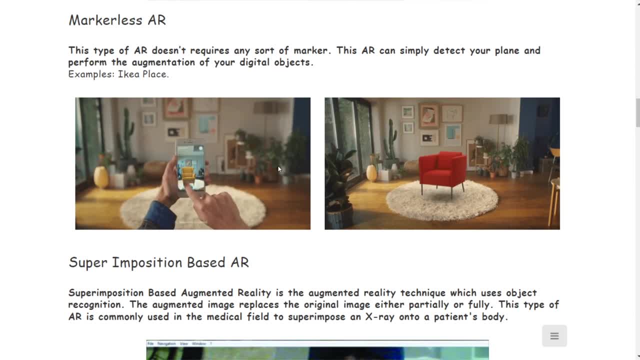 room or not, something like that. alright. now what I can do is I can make use of Markerless augmented reality, scan my room and then place the object in there, alright. and then through my mobile I can see that if the sofa is adjusting at my place or not. alright, and based on that, 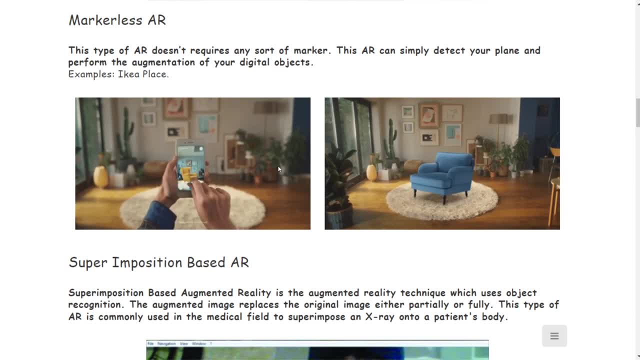 I can buy the sofa. so that is how Markerless, that is what Markerless AR alright. now there are multiple use cases of Markerless, AR alright. and decoration alright means this: putting furnitures and all this is one alright is one industry focused alright it is interior design. 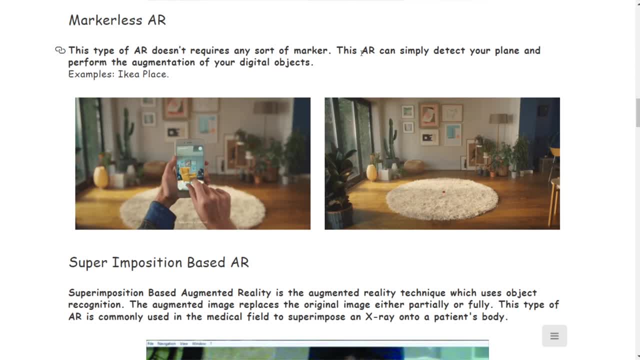 is another industry. alright, in where mixed reality? alright, in where mixed reality and augmented reality are widely used, alright, like for decorating the homes and all those things, alright. so I hope Markerless and Markerless AR is clear. So basically, Markerless AR is nothing. Markerless AR needs a marker to perform the augmentation. 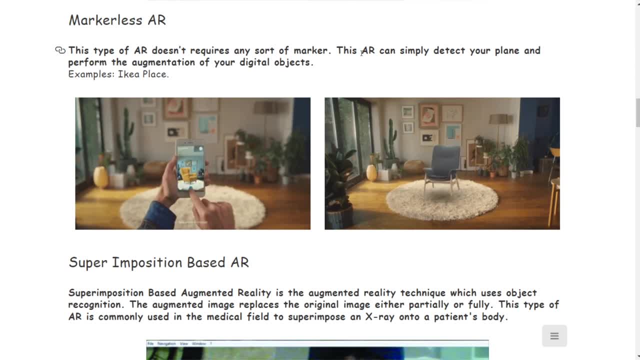 of digital objects on top of the marker, whereas Markerless AR doesn't need any marker. alright, what it will do? it will scan the surface and then augment the digital objects on top of the surface. alright, so that is what. that is the basic difference and that is what 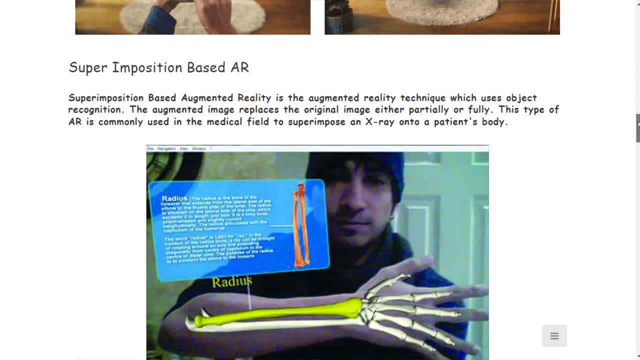 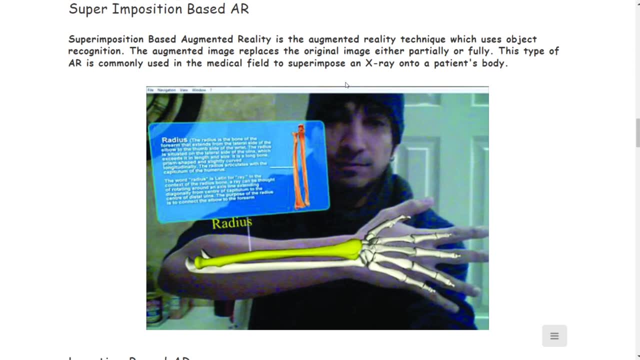 they do. alright, now let's get into the concept of Superimposition-based AR. alright, see Superimposition-based augmented reality. alright is basically a technique that you know uses object recognition. now in this diagram. alright, in this diagram you can. 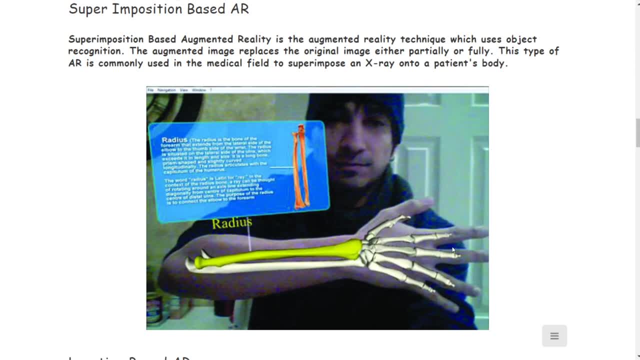 see there is a person's hand. alright, there is a person's hand and on top of that hand, we, what we are, what this app is doing is, you know, displaying, displaying a skeleton of the hand on top of the person's hand. alright, so that is what Superimposition-based AR is. 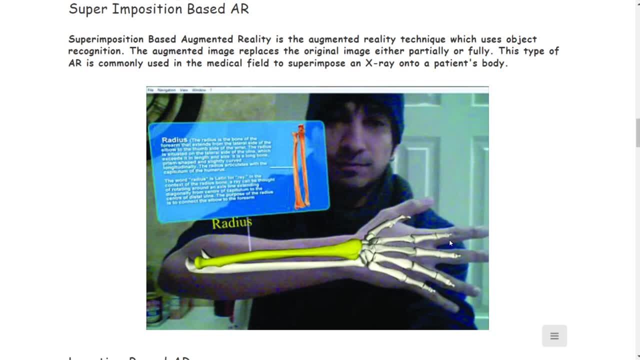 it superimposes it- alright. It superimposes that means it put- alright. it puts an digital object on top of a real object- alright, and that works with the help of object recognition- alright. so that is what Superimposition-based AR is. it's very simple, alright. it's very simple now, alright. 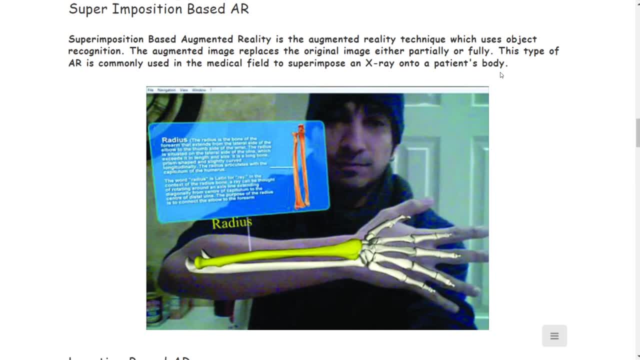 see what is happening in here. basically, with this photo, alright, you can see that we are able to, you know, augment a skeleton, skeleton of hand on top of another person's hand. alright, so what is happening? the algorithm- alright, that is, the AR app- is recognizing the hand. 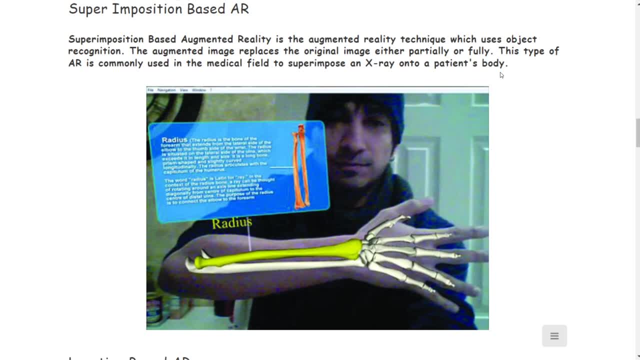 then putting alright. or you can say then superimposing, alright, superimposing the skeleton on top of that hand, alright, that is what it is doing. that is what Superimposition-based AR is. alright, very simple, alright. 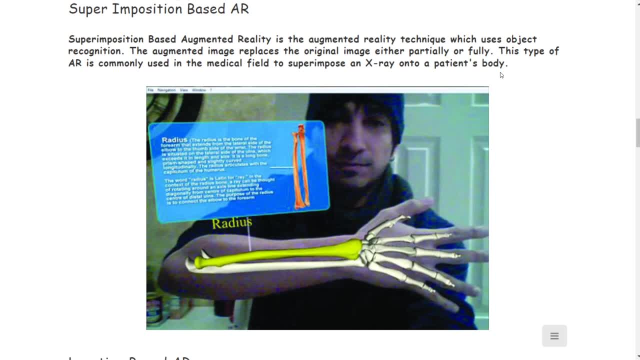 Now, This type of AR right is very helpful. alright, in medical industry. alright, like you can say, you can superimpose an x-ray alright on a patient's body and look into it real. 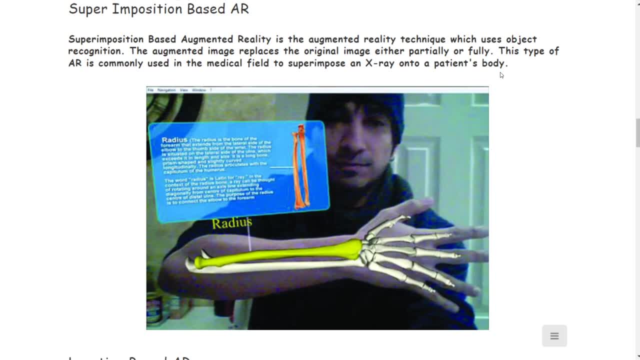 time in 3D. so how cool that would be and how efficient that would be. right, that would make the doctor's job more easier, right? so that is how we use Superimposition-based AR. alright, and Superimposition-based AR are used in, you know, in many different ways. 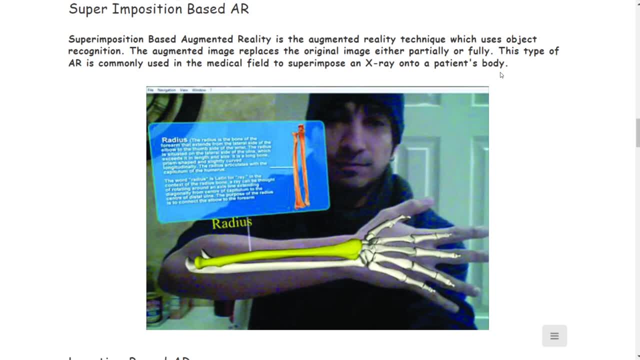 so you can do your research on that, alright, even if you, if you like, you can uh try developing something with superimposition ar also all right, so you can totally do that. that would be real fun, all right. so that is what superimposition. 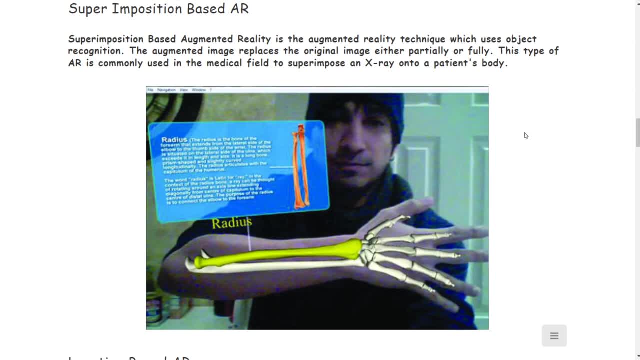 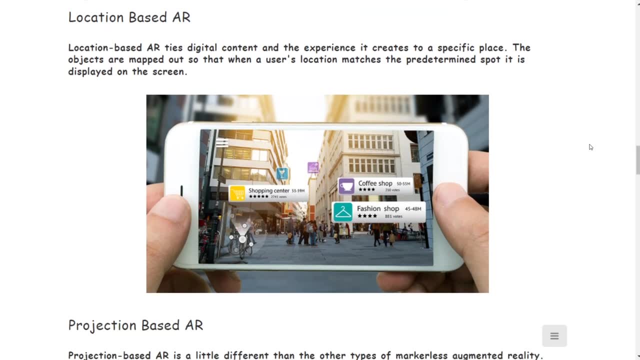 based ar is. so i hope you are clear with the very fundamental concepts right now. after this, we are going to get into this location based ar. all right, see location based ar. now, uh, let me tell you uh, you, you, uh. i'm sure you know about uh gps, right, you know about, uh- what can i say? google maps. 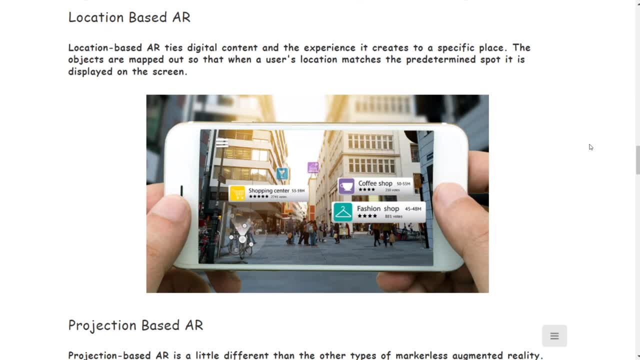 right. so you can say this is google maps in augmented reality. all right, like in google maps, when you search for a place, what it does it? it gives you the address of that place. all that means it marks the uh road. it will highlight the road through which you can go. go how much time will? 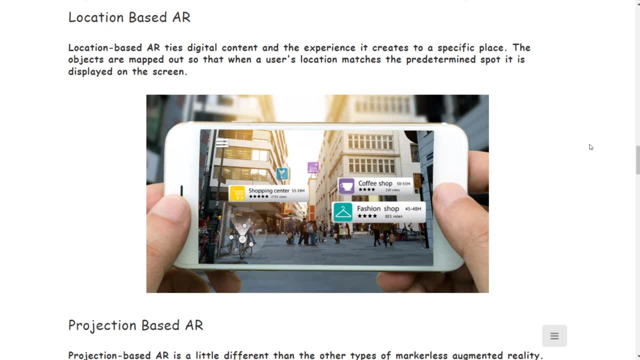 it take to get to that place. it will label the places. uh, that will come uh while you are going in there. right, it will label those places, you, but what you are doing in there, you are uh, seeing all those in a 2d screen. all right, what location based ar does, is it's also, you know, does the things. 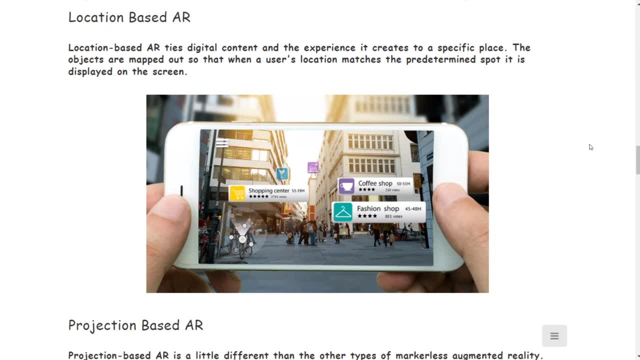 almost same, but in augmented reality. it would give you the live feed, all right, in 3d. it will give you the live feed in 3d, like you will. if you are going somewhere, you, uh, if you turn around, you would be seeing a nameplate- all right- hovering over a building. all right, that would, uh, give you an idea. 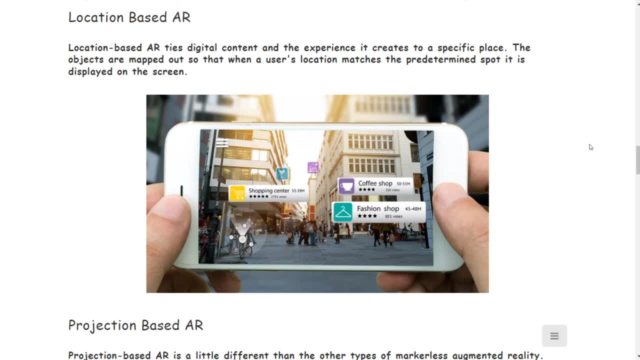 yeah, this is the building, what i'm looking for. all right, then you can go in there. so this type of ar experience makes it more easier. all right to you know, use us like locate places. all right, so that is what location based ar is. location based ar basically, you know, ties, digital content and 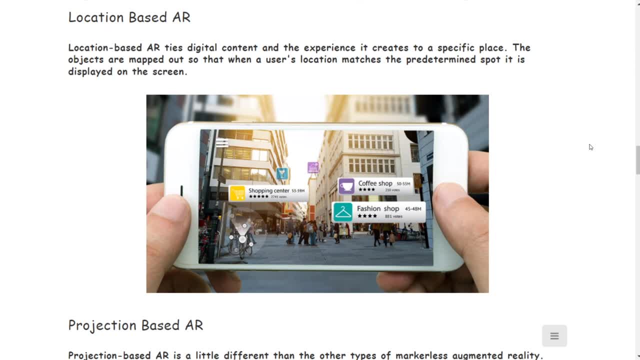 the experience it creates to a specific place. all right, the objects are mapped out so that when a user's location matches the predetermined spot, it is displayed on the screen. all right, so that's what i told you just just now. all right, this is the definition. this is. i gave you the very simple uh explanation. 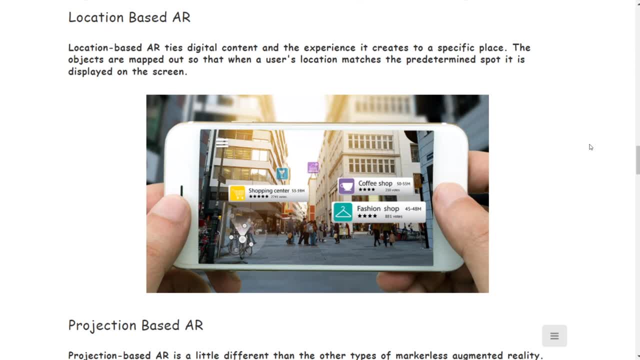 of the same definition written in here. all right, so location based ar is just like google maps, but in ar. all right and more efficient, more better. all right, in a more better way. of course, now you guys might be thinking why we are going to. you know, uh, held our phone in, held our phone in hand and 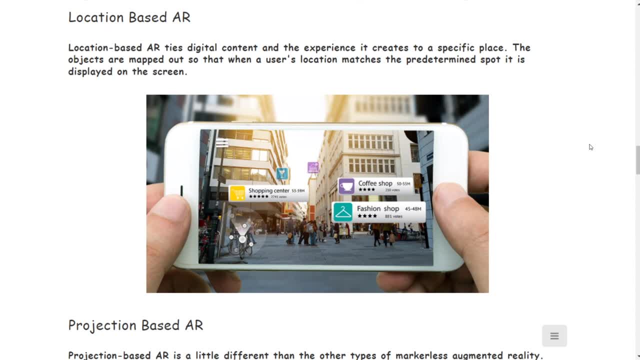 start looking for places. all right, it's going to be very hectic. i totally understand that. all right, and that's not how we are going to. you know, use location based ar. currently, there are multiple ar glasses that are being released. all right, like geo glass is releasing their own ar headset. 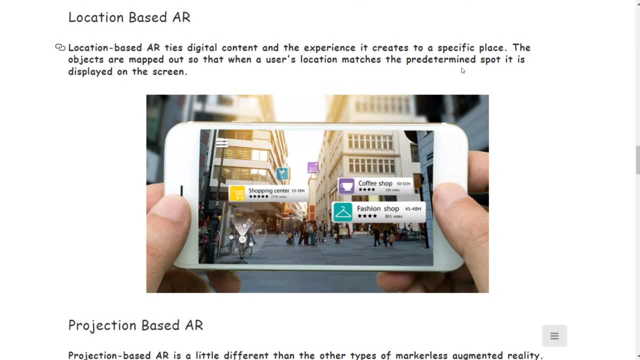 then qualcomm, all right, qualcomm is releasing their own ar headset. all right, so many people, many industries, all right, are working on their own ar headset and they are using location based ar and ima headset, then a magic leap is there. so when those glasses will release now, after a few years, 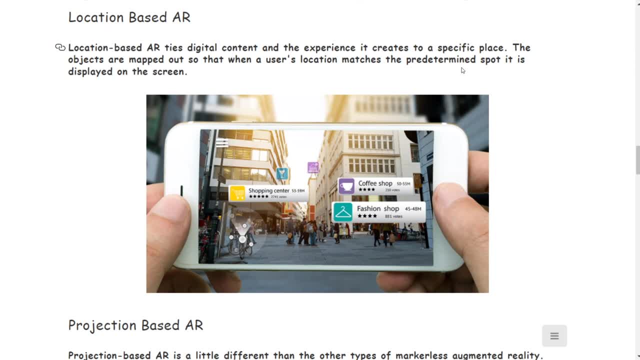 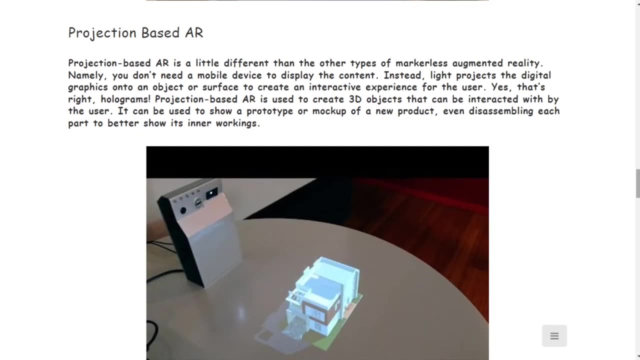 all right. or maybe in this year only, you will be seeing location based ar. all right, it would be gps, but in ar. so how cool that experience would be right. so that is how these things will work, so i hope this- uh, the concept of location based ar is clear all right. now here comes projection based ar. 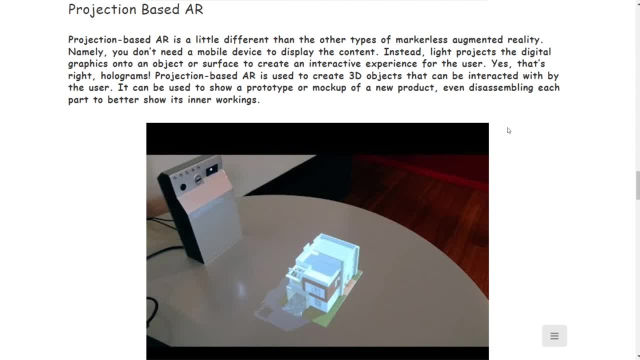 now let me make it simpler for you, all right, nice, so i'm starting with location based ar. uh, right, and you know, projection based ar is another name of holograms. all right, i know you guys might uh have an idea about what exactly a hologram is, right, it basically projects. all right, it is. 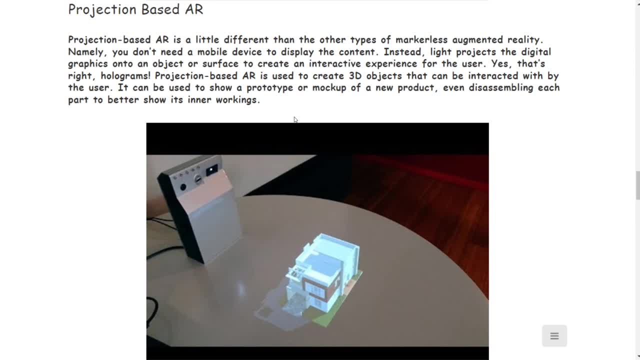 projecting with, uh, you know, a projector. roll uh into. uh, it means into the means. uh, what? let me? let me explain it in a simple way. what it is doing- it is like normal AR- is we are in normal AR. we are using our phone to augment. all right, we are using our. 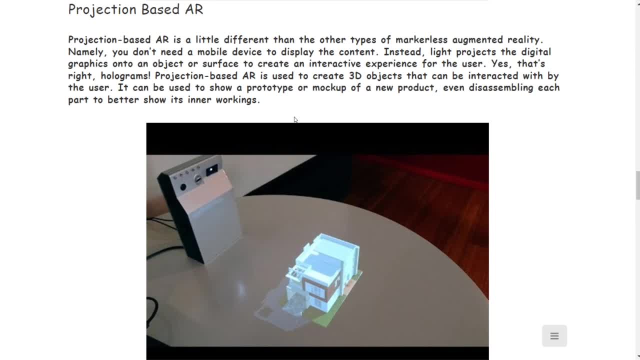 phone to augment, but in projection based AR we are using some other device to project. all right. to project the digital object into the real world, all right. that gives a more immersive experience. in that case, you are not. you are not going to need a phone, all right, you are just having some. 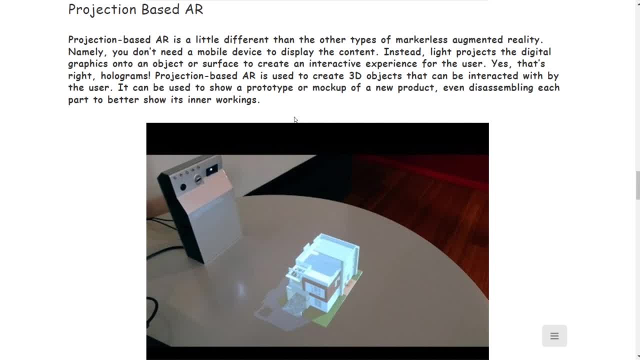 project and it is projecting- all right, it is projecting the 3D object in the real world. people are working on this kind of technology, all right, although right now it hasn't been that successful, all right, but people are working on that and I'm sure this is something that we are. 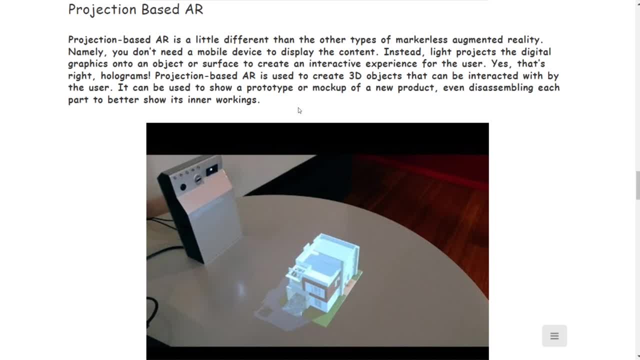 going to get in future. all right, and people are really working like working hard on this kind of AR. all right, it would be like really cool, like you would be the Tony Stark, all right, of real world. so yeah, augmented reality, virtual reality, mixed reality, has the potential to bring all the 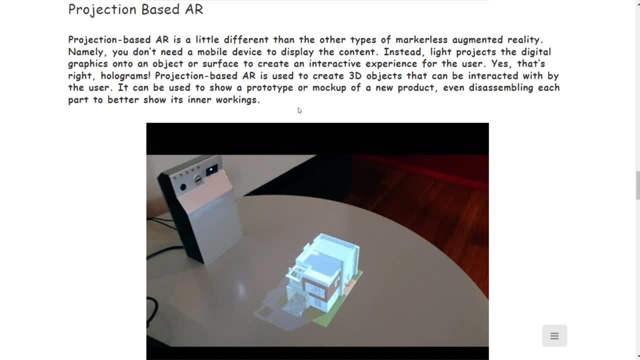 things that you see in the Iron Man movie. of course, not the arc reactor, but all the digital things like the Jarvis. all right, artificial intelligence is also having the potential. so if we combine these technologies now, we can have something like Jarvis. so understand it this way, all right. augmented reality, virtual reality and mixed reality is the future of our world. all right. 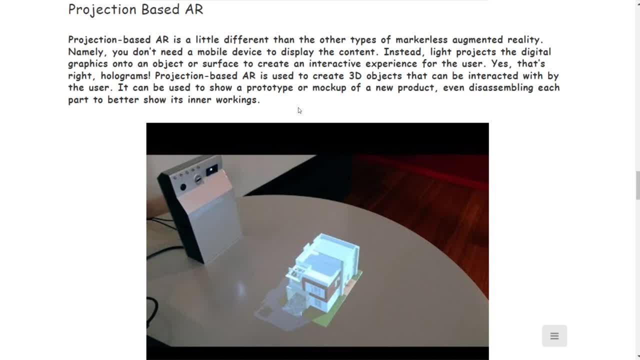 maybe within five to ten years, you won't be even using your phone. you will be having slim glasses, all right. you will be having slim glasses through which you will be able to augment the digital objects. all right, and that is going to be true because we have those glasses now. all right. yes, they are. they are bulky, like if I. 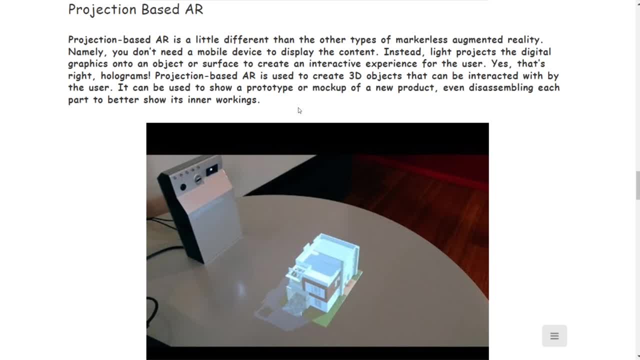 take an example: there's a Microsoft HoloLens. all right if you, if you have used that before, you would get the same experience like a Tony Stark, right? similarly, then the, the, the, the the other AR glasses is being released, like GeoGlass is releasing their own, then Qualcomm is releasing their own, so within five to ten years, 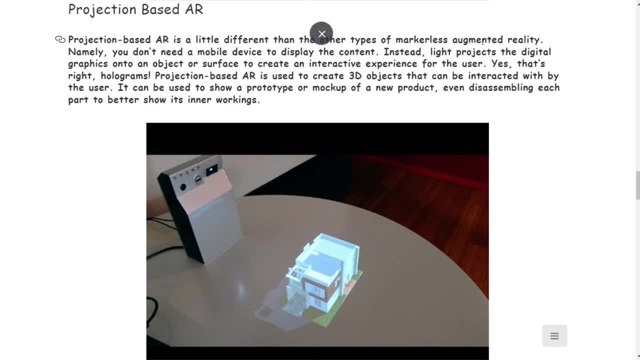 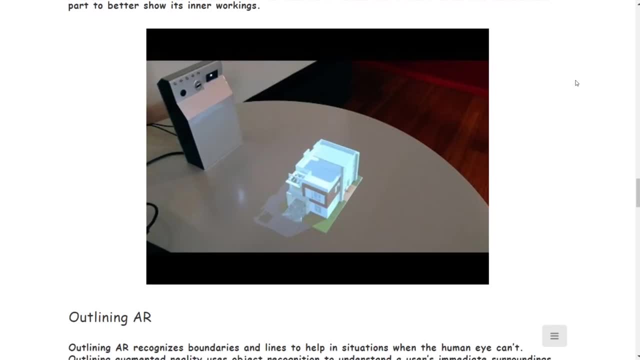 all right. you won't be using your phone to communicate or, you know, do things. you'll be using your AR glasses to do all the things. all right, there's Snapchat's lens, all right. so a lot of things are there that you can do, all right. so now, as we have, as we have understood, the very 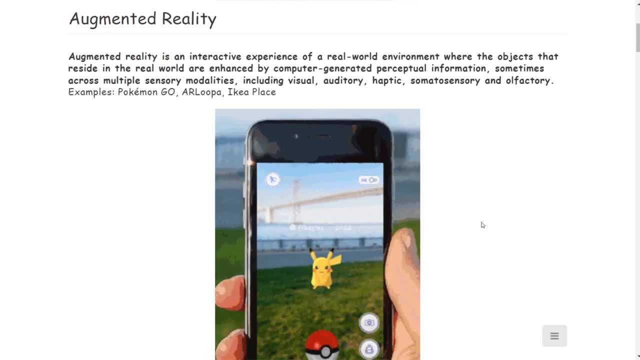 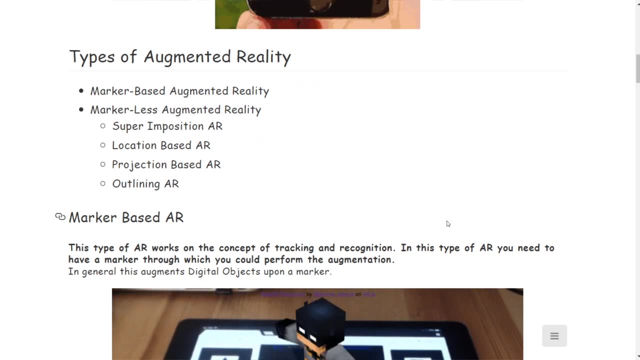 basic concept. you know the concept of extended reality, or we have understood the basics of our augmented reality. we have understood markup based AR, markerless AR, superimposition, location based and projection based, and the last one we have in the. you know the topic of augmented reality. 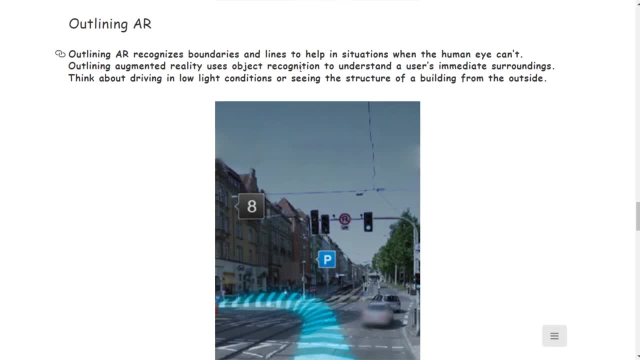 is outlining AR. alright. now, what exactly is it? all right, outlining? AR is mostly used in cars, allright, you might not be seeing them more often. all right, although I guess even Tesla is AR in their cars, all right, so basically, outlining and it will outline the direction. all right, it will outline the, it will map the world and then outline. 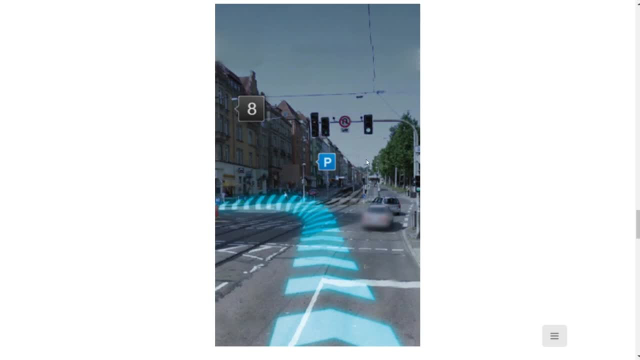 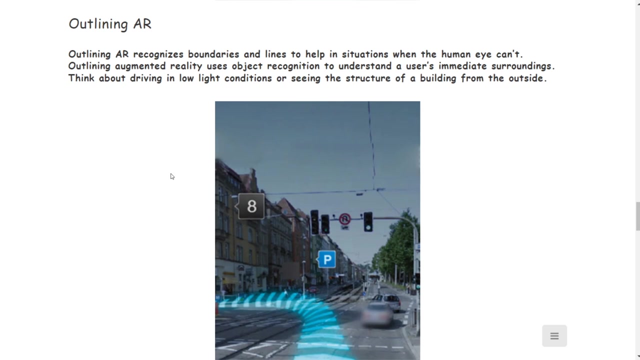 the direction. all right with. these are trails, here you can see, right here you can see. so they will outline those trails and help you. you know, go through all the paths. all right, it would recognize the boundaries. all right, it would recognize the lines. it would help in many situations. all right, when. 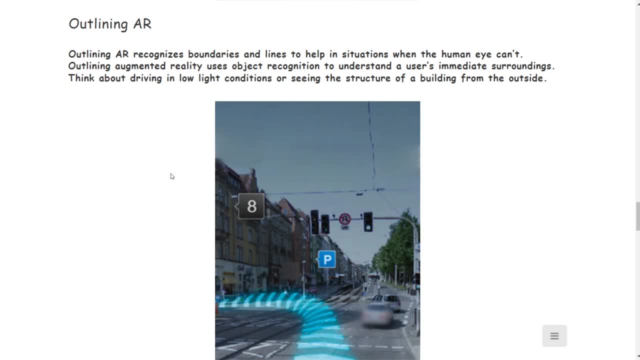 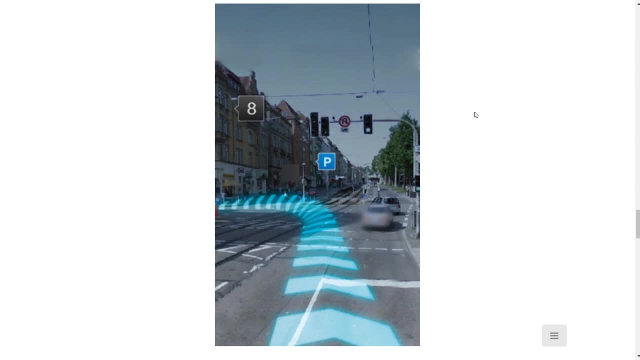 human, aware human, I can't, all right. so augment augmented reality is the future. all that augmented reality, mixed reality and virtual reality- is the future. so this is how outlining AR is used. all right, even. yes, if Tesla is working on implementing augmented reality, all right, then why can't we? right, we are. 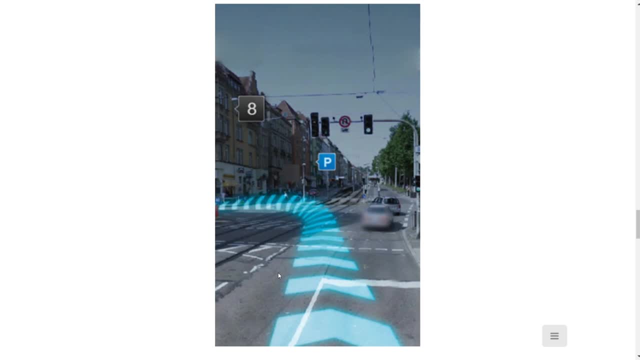 developers. we can do that, of course we can do that. so you can see people are working on implementing AR in their car, right? you can see people are working on implementing AR in their car, right? and how cool is that right? so that is what outlining AR is all right now, as we've 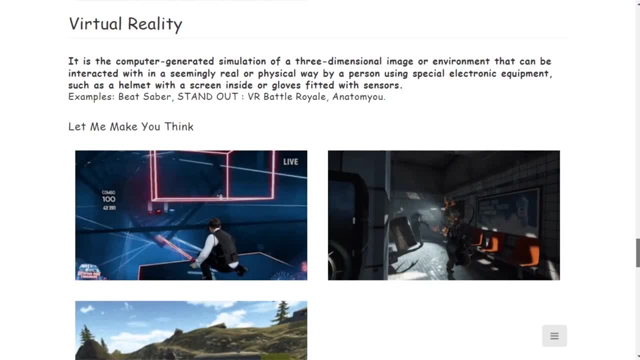 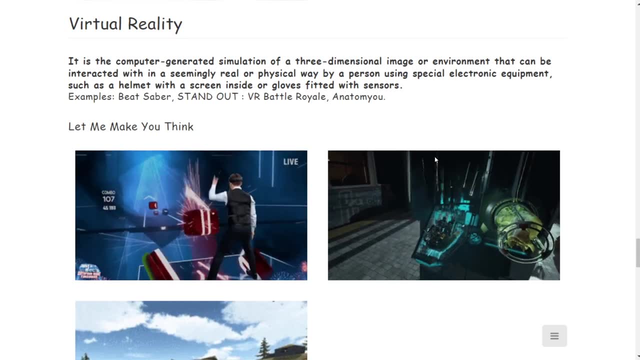 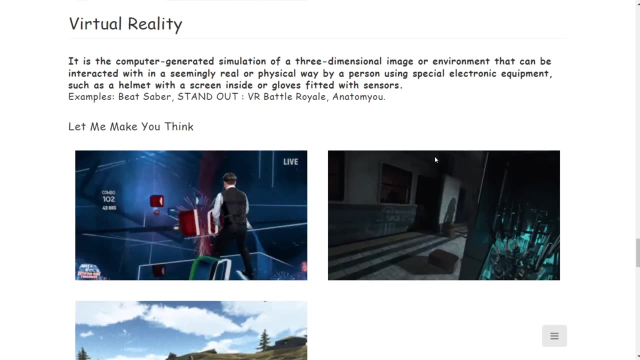 understood the fundamental concepts of augmented reality, let's get into the virtual reality, all right. virtual reality is the total opposite of augmented reality. in augmented reality, what? what did we do in augmented reality? we were augmenting, all right. or you can say, putting the digital objects in the 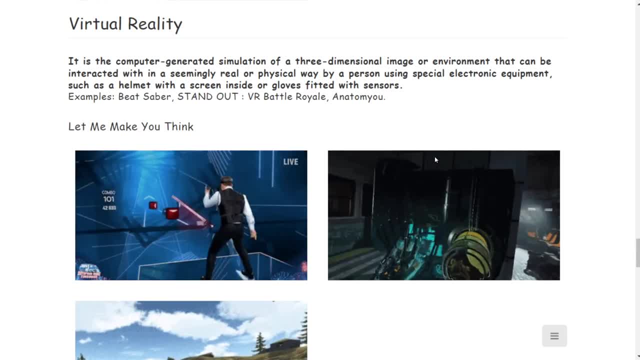 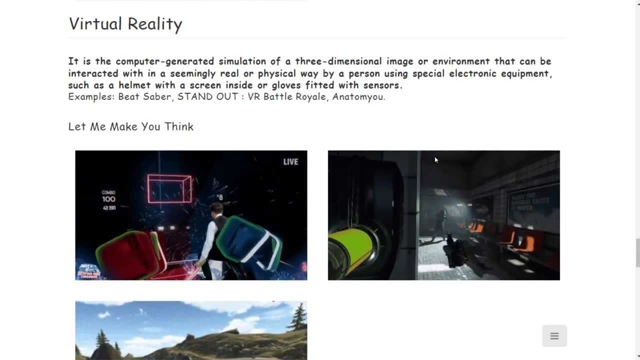 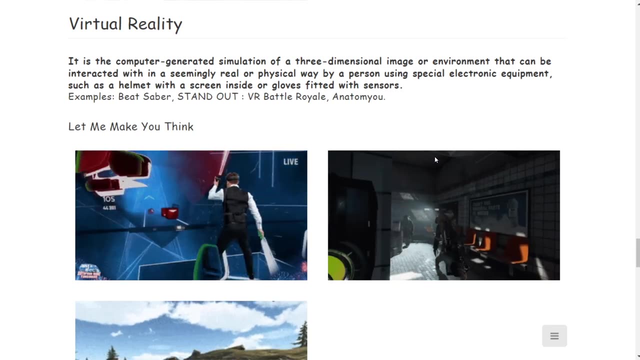 real world, but in virtual reality we are taking, all right, we are taking the person itself to the virtual world, all right. or you can say we are teleporting the person to the virtual world, right? that is what virtual reality is, and it gives a very good sense of immersiveness. all right, for example. all right. see, even I don't. 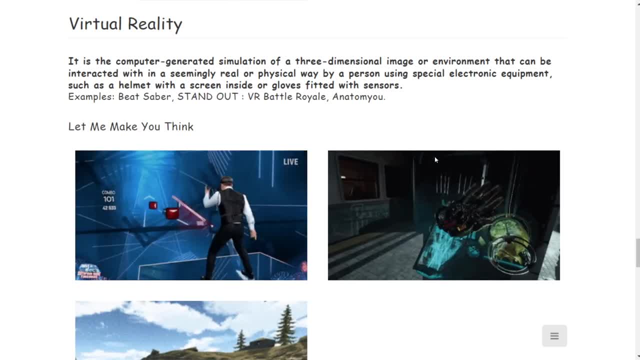 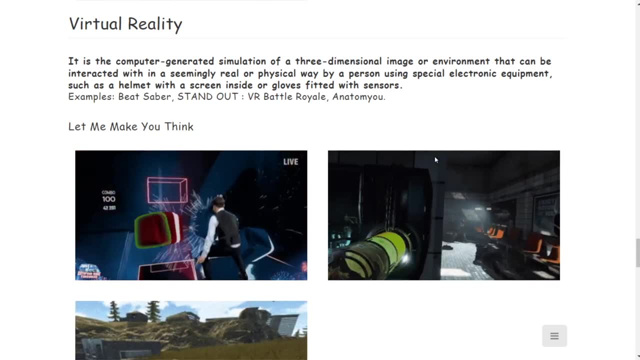 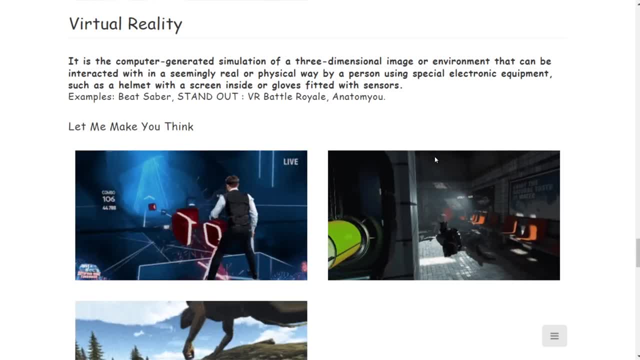 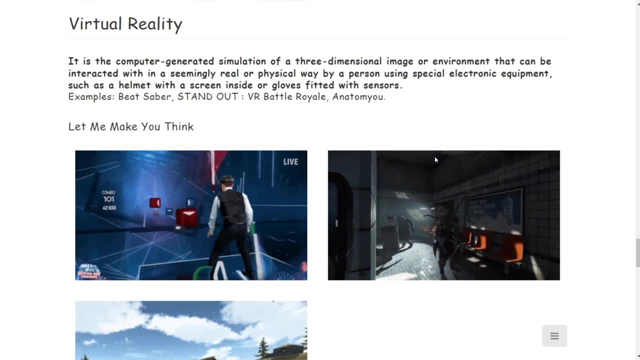 I have used. at some part of my life I have used virtual reality headset. yeah, of course, not at my home, but when I used to go to some game parlor, all right, they had a virtual reality experience of it. I am, I have used, I know how that feels. 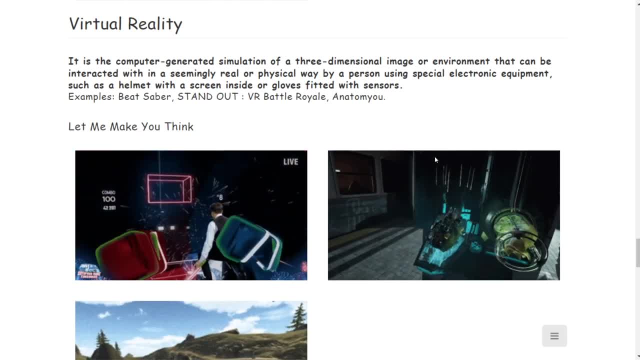 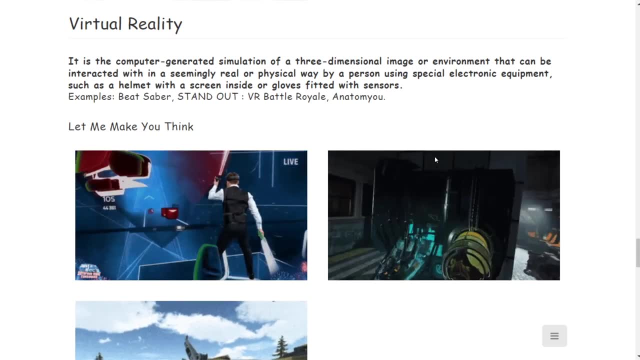 all right, and I'm glad that I can explain it to you. that try to understand it like this. all right, let's say you, you are playing a game. all right, take any of your favorite game. all right, one of my favorite game is, you know, Gpfi. all right, although I don't play games much in. 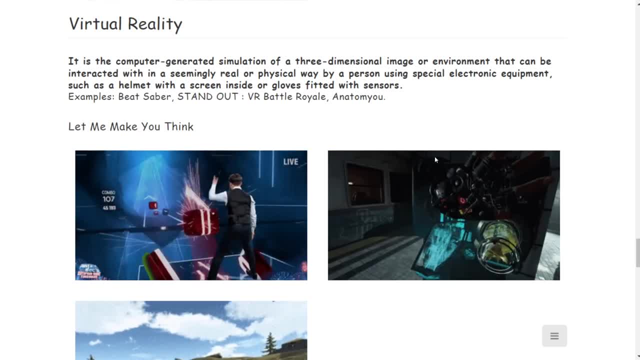 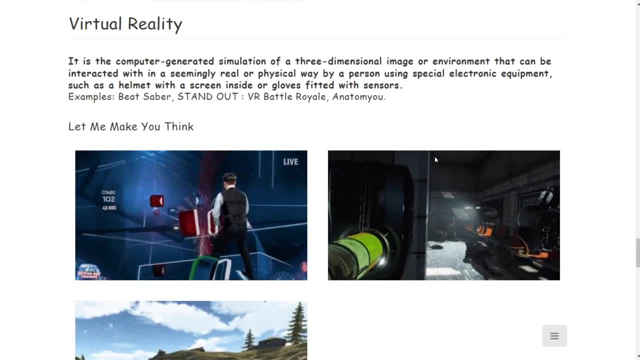 nowadays. but if i, if i had to say, one of my favorite games is gta 5 and gps, android, all right, so what i'm going to do is i'm i'm going to close my eyes and you know, think of, uh, think of, think of. 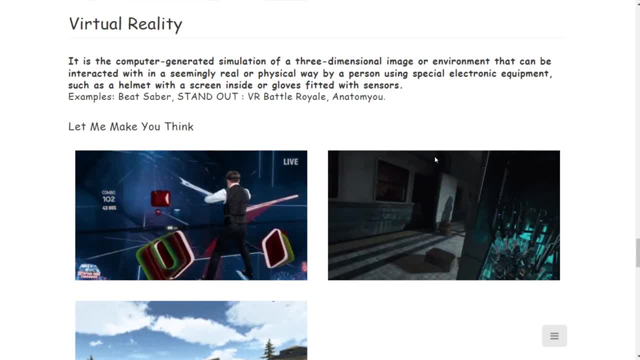 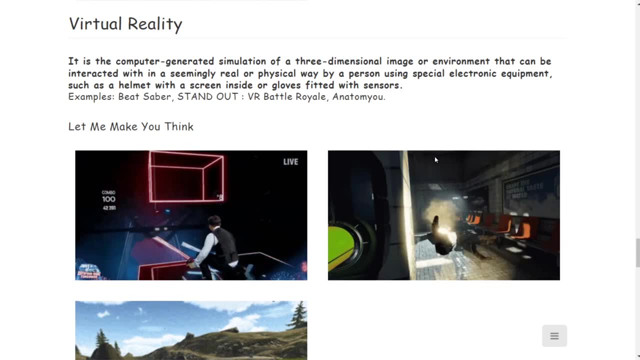 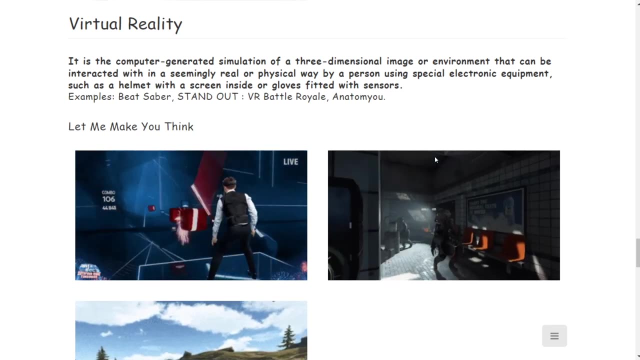 a character in there. all right, think of a character in there and try to, you know, close my eyes and try to experience, all right, all that thing by myself. all right, and the level of immersiveness you will get there now, of like while thinking or while imagining you are in, uh, in there in real. 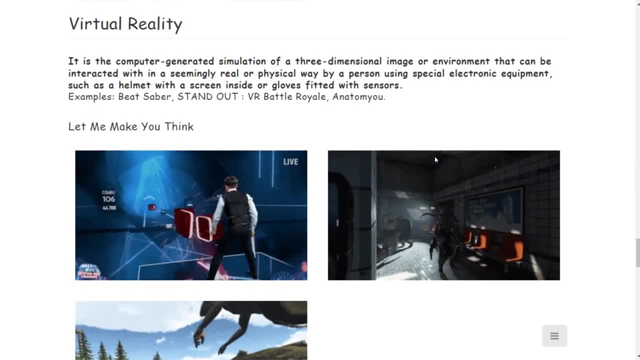 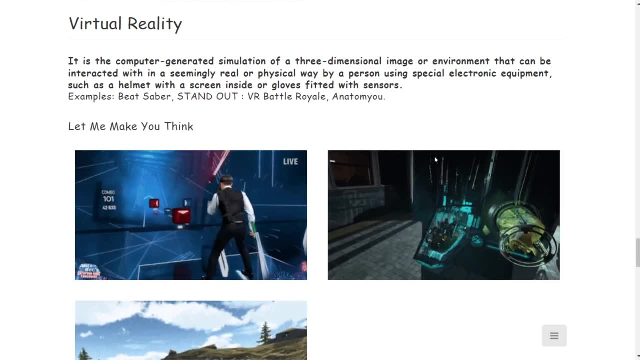 time in the game and playing all the things, doing all the things that the game's character can do, will give you- uh, you know- a sense of immersiveness. and using virtual reality, that sense of immersiveness increases by 100. all right, because at that point of time you are actually in there. 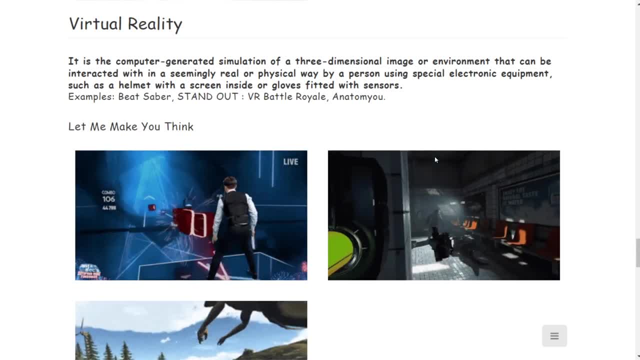 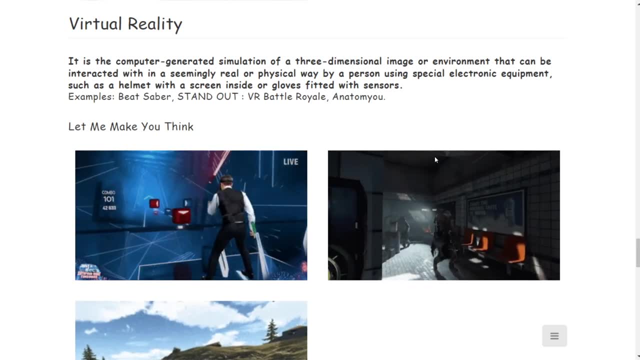 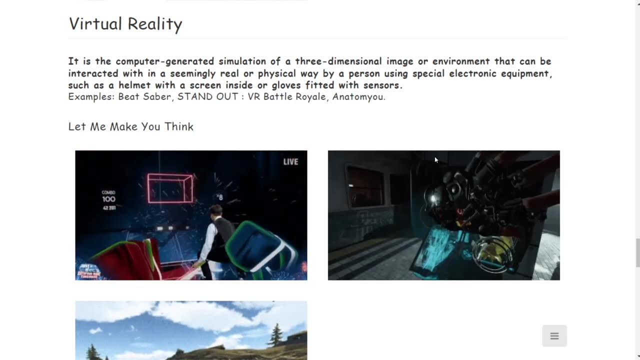 you are actually controlling the person available inside the game. right, you are actually able to control the. you are actually able to control the. you are actually able to control the. you know you are actually able to control the character available inside the game. so virtual reality is nothing, but you know, it is the technology that you know teleports. uh, you to. 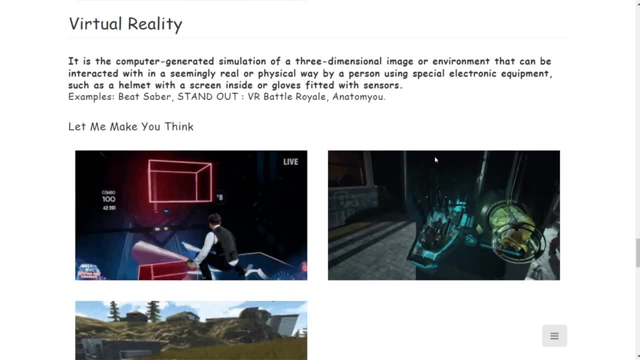 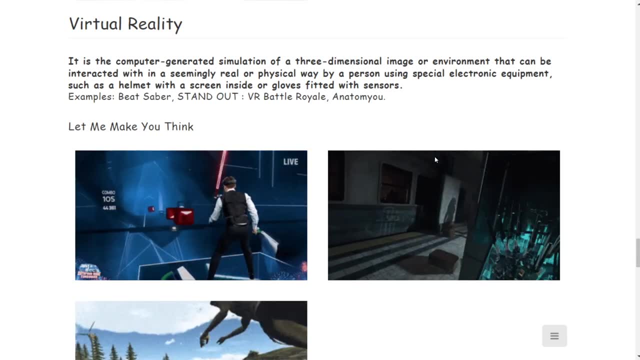 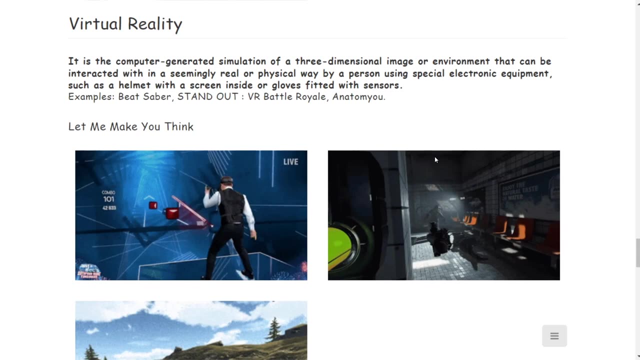 a virtual world, all right. so that is what exactly it is now. there are, you know, multiple games and educational applications available, right? for example, uh, anatomy- all right, it teaches you about the human anatomy. all right, so that that is an educational app? all right. then there there is beach saber, one of the very famous 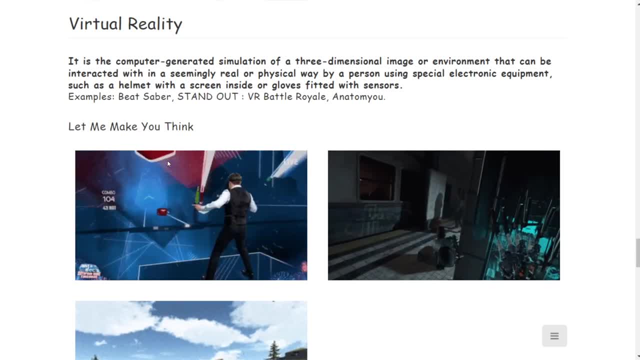 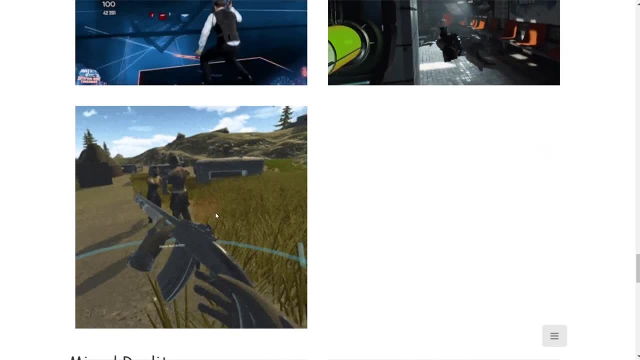 game like uh, in the. in the first image you can see this is a gameplay of a beach saber, all right. in the second image, this is a gameplay of half-life alex, all right. in the third image, there is a battle royale game. yeah, there is also a battle royale game in virtual reality, so you can see. 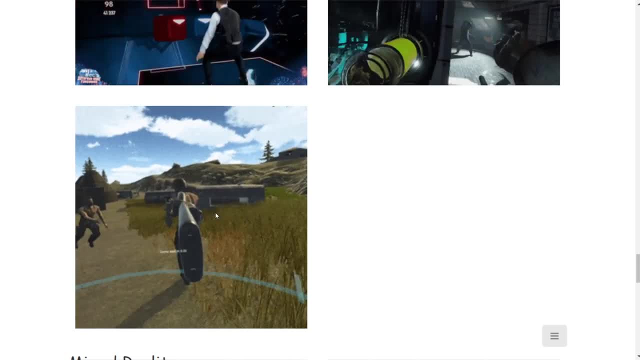 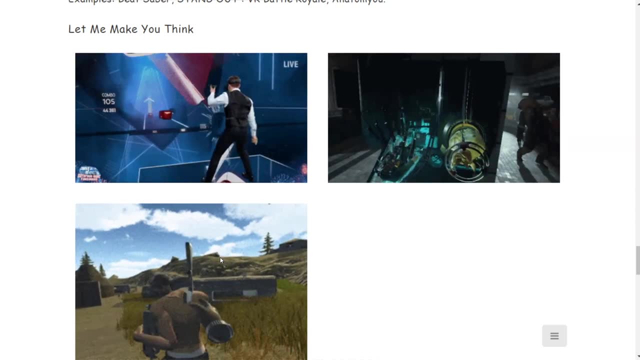 the level of immersiveness, the level of realism you will be getting. this is called, uh, what can i say? uh, standout. vr battle royale, all right. so this is a game where you can see the level of creativity, all right. so, uh, you have the interaction of the真的是, the interacting condition of the. 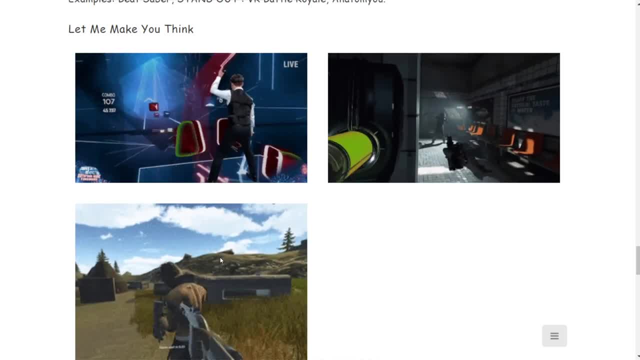 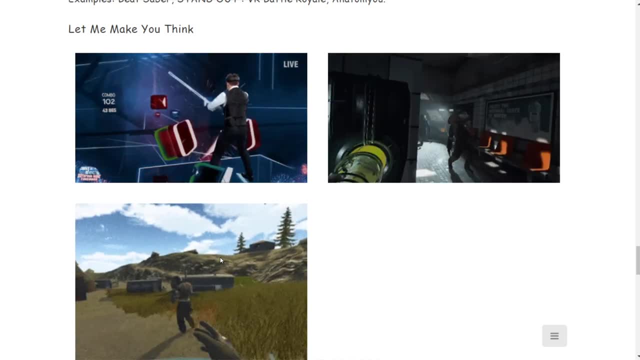 game. you can be in just a space and it can be used in like as African influence, um environment, you can say, or whatever, uh, so vr can be used in nature as well as. so the vr can be used in multiple sectors. it can be used in healthcare, it can be used in military training. 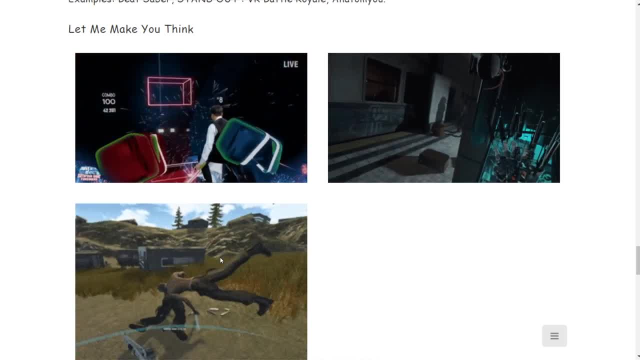 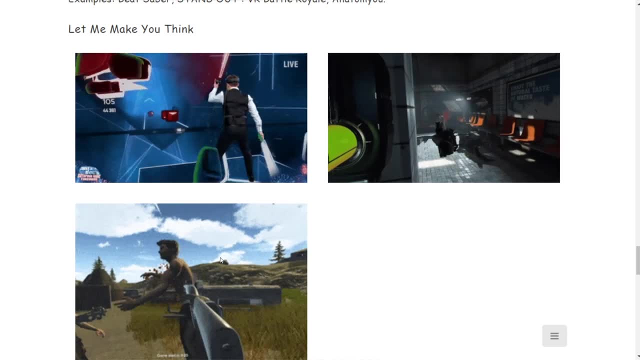 all right, it can be used in flight training. it can be used in manufacturing. all right, you. LIT can be used in education. it can be used in gaming. so the you know what can i say? the level, all right, you know cost is decreasing, like previously in India already. I'm talking. 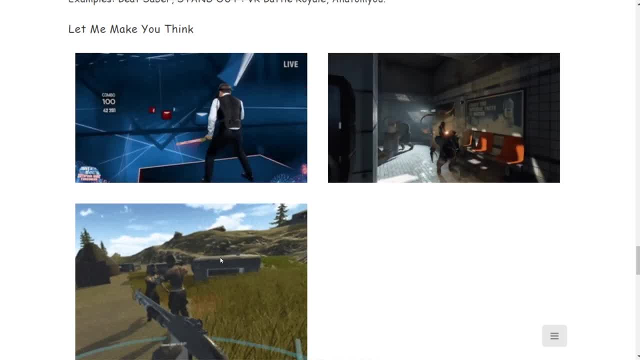 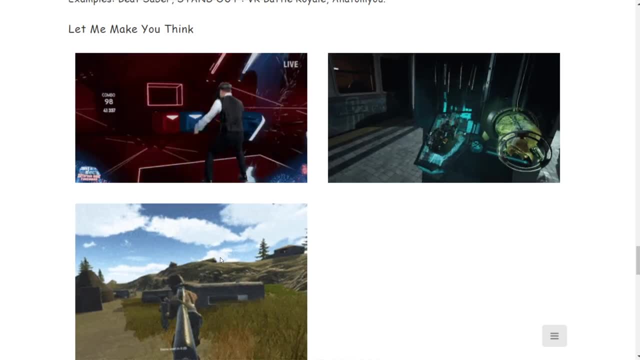 about in India. in India, previously oculus quest- all right, it's the VR headset. it used to cost around 80 to 90 thousand, I guess, all right. and now oculus quest 2 costs around 30 to 40 thousand. all right, so you can see how. 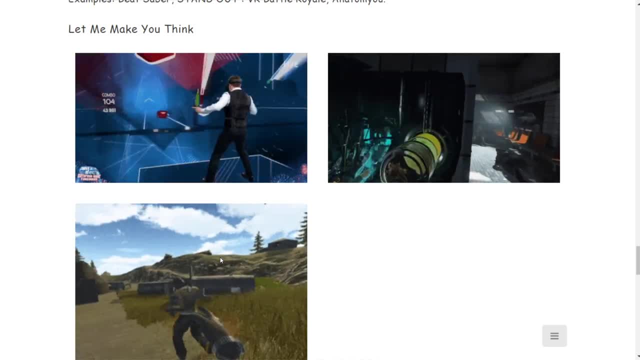 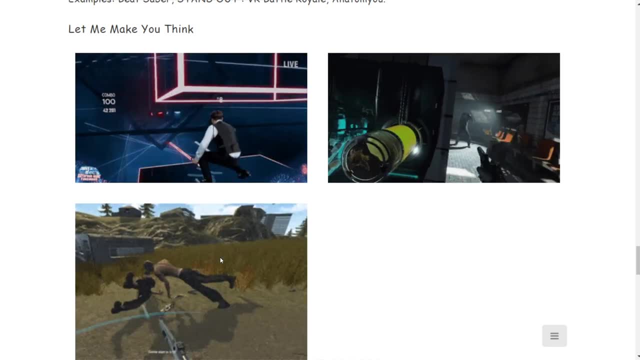 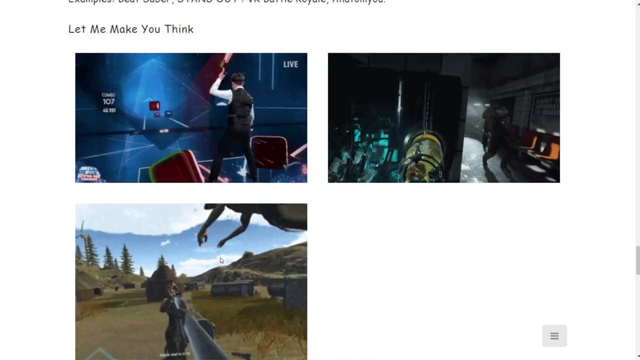 drastically has the price. has you know the price had decreased by half? all right, so the price of VR headset are decreasing, all right, and also the quality and the technology is improving and increasing, all right. so just a few more years and you'll be getting VR headsets, maybe in 10,000 or 20,000. so 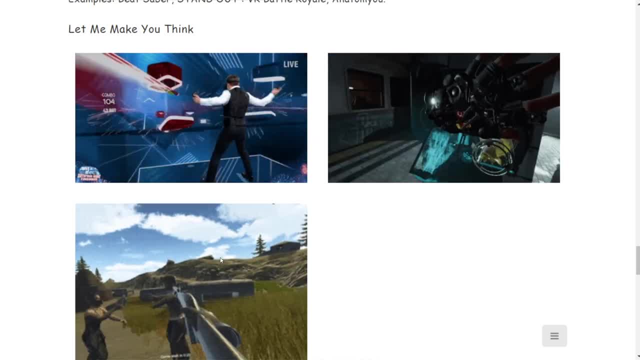 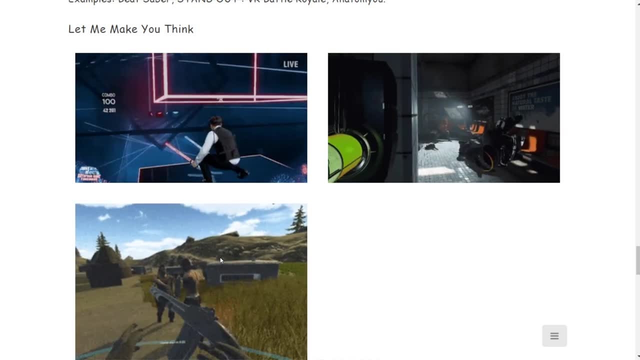 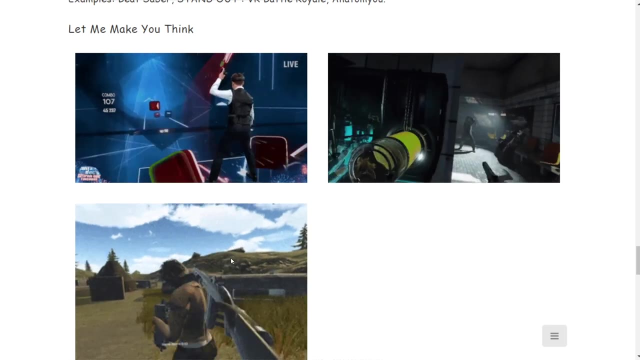 things are. you know things are happening real quick and mixed reality is actually. mixed reality is going to help us a lot. if I talk about in the manufacturing industry, all right. if I talk about the military training industry, all right. and as we have understood about the virtual reality, augmented reality, it's our high time to go to mixed. 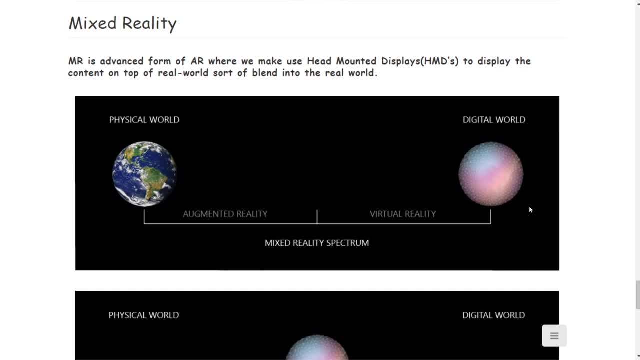 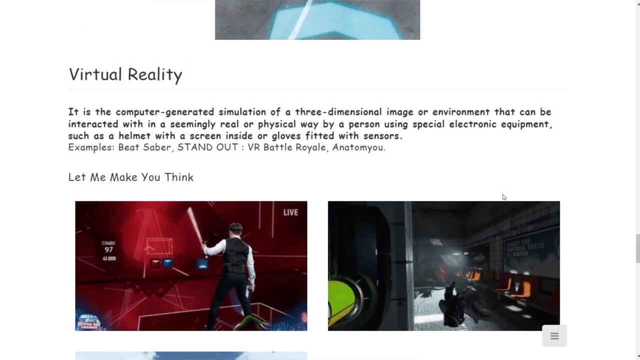 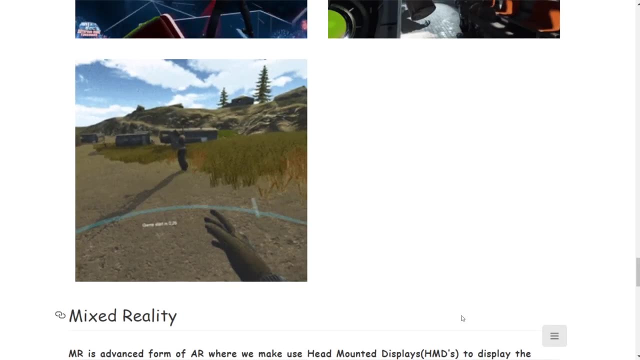 reality. all right. now let me tell you all right also one thing: I forgot to tell you: that if you are using virtual VR now, you'd be needing an headset. that headset is called head mounted display- all right, so you make sure you know that this term. all right, or you can say in abbreviated form, it: 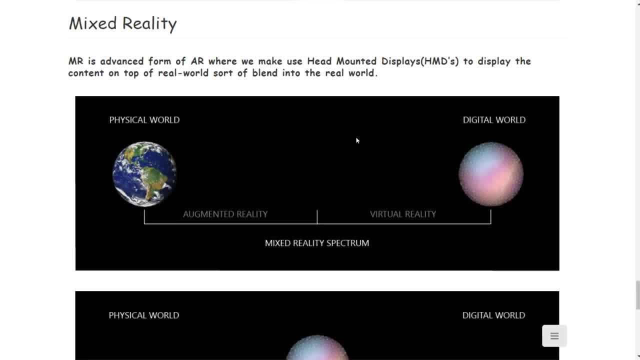 is also called HMD, all right. or head mounted display. now see, mixed reality is reality, all right. mixed reality, you can mix reality- now is the. you can say it is the brother, all right, this is the brother or the twin brother, you can say, or you can say, just just the brother of augmented reality, all right, why? because 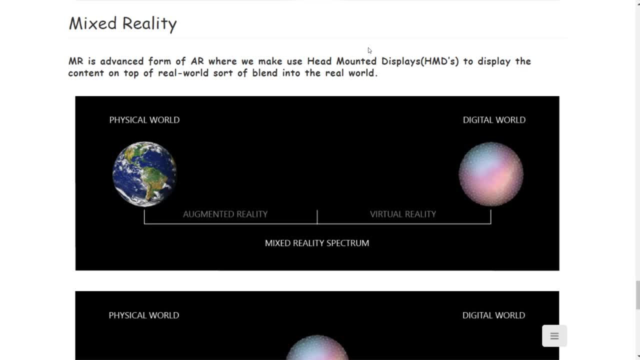 see, it is. let me, let me simplify this term to you. mixed reality is just like augmented reality. but yeah, there's a but. but it is more advanced, all right, it has more capabilities than normal augmented reality, why? all right, see, there is something called, all right, mixed reality, continuum, or you can say mixed reality. 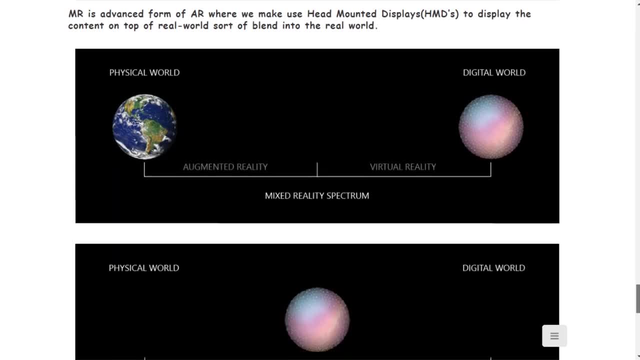 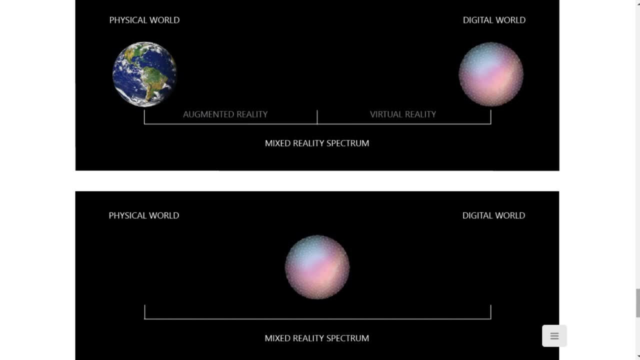 spectrum. what does that mean? it means that now you know the merge, all right, the merge of augmented reality & virtual reality, or you can say the real world and virtual world, or digital world. all right, we combine them. you can, you know, go virtual and real at the same time. all right with, with mixed reality. so mixed reality has a larger 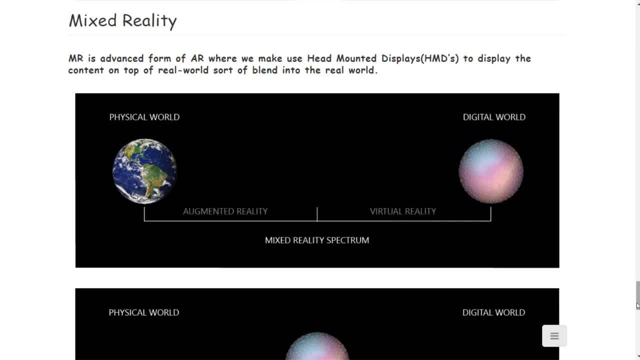 potential. if we talk about the uh like training industry, all right, like in manufacturing industry, mixed reality can help you know to recognize those uh items, all right. it can help you through the manufacturing process in healthcare, all right, it can help you, you know, operate a patient, all right. 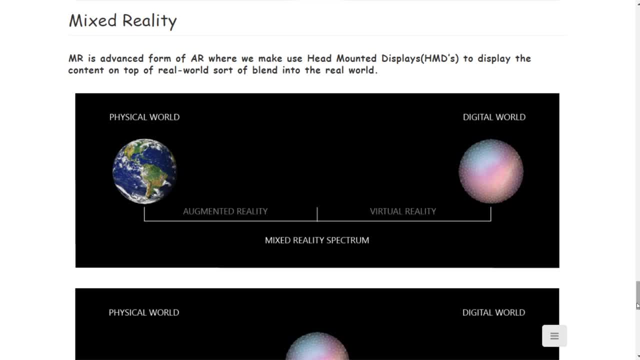 it can guide you through all the things you don't even need to, you know, distract yourself, uh, to any other computers or, uh, you know, digital objects available in the. in the icu, all right, you can say. or in the patient's ward, all right, where? uh, basically? 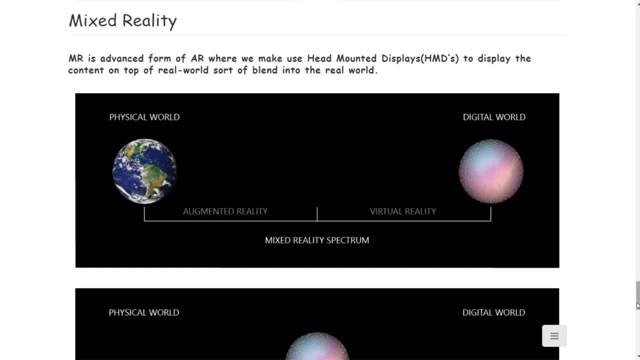 the operation is happening. all right, you don't even have to move from the patient, you can stay in there. uh, monitor all the things, all right, in your mr headset. all right, monitor all the you know how- let's say, heart rate or blood pressure or any- any data through your mr headset only. 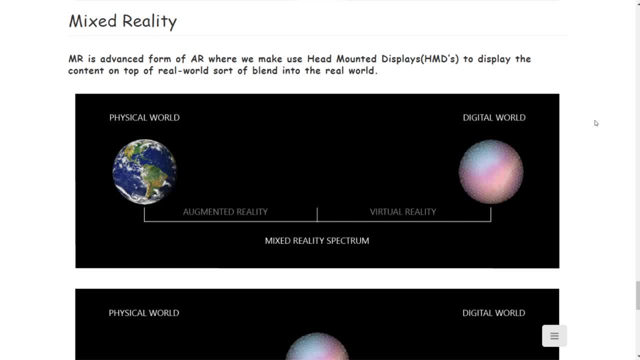 all right. so this is how it can help in, uh, you know, medical industry. then, uh, military training. recently, i guess i just read somewhere uh a byte: in 2018, all right. in 2018, uh, military, all right. i guess us military uh reached microsoft and offered around, you know, 400 to 500 billion dollars to. 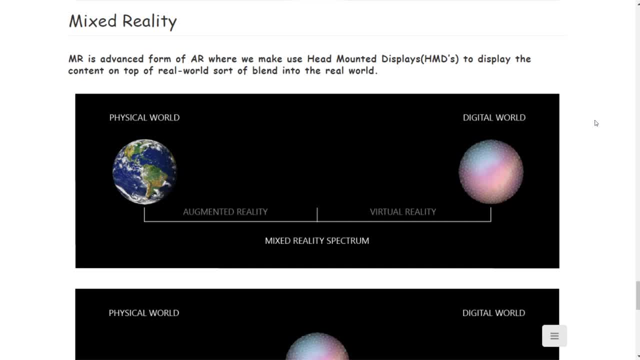 build mixed reality headsets for them. all right for training military. all right for training the military. so you can, you can, you know, you can just think how powerful these headsets are. all right, it can help in training. so mixed diet can help you. uh, anywhere like, for example, in india, there's a 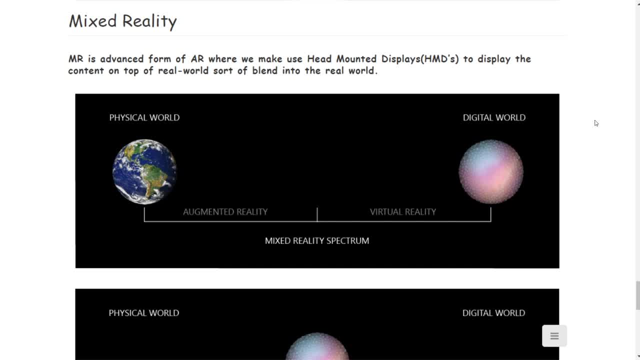 startup called ajner lens. all right, what they are doing, they are, uh, creating headsets for government which are being, you know, used to train military. all right, they are creating headsets for government which are being, you know, you know, being, you know, used to train military as well. uh, which was used to train military themselves. and they started thaterma when i pointed this question. we actually started this subject, you know, assa, at the first time that we did as a third, cuando, uh, whatever, the common sense realized that. you know, on such, have a parlé to. 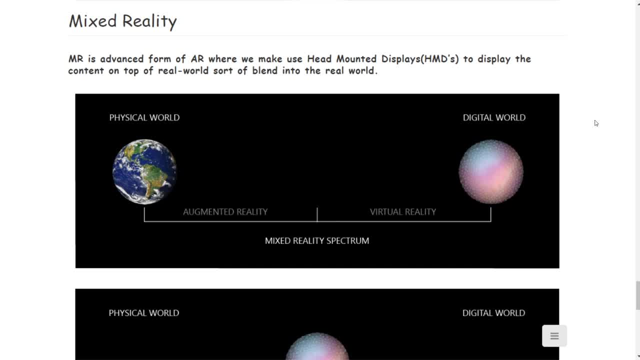 Indian military. so it is being used to train navy seals. it is being used to train numerous people out here in India. so you can see how mixed reality is exactly helping. so mixed reality, I would say mixed reality is future. extended reality is the future of our world. it is the future of our world. 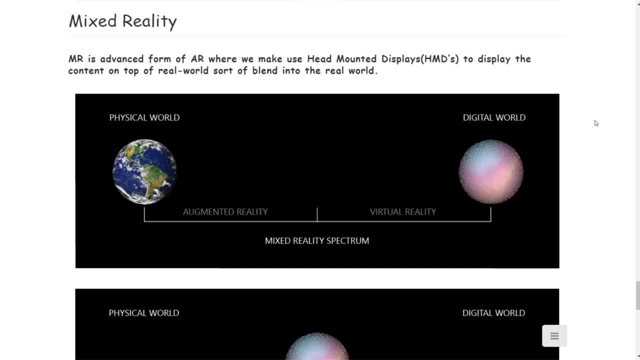 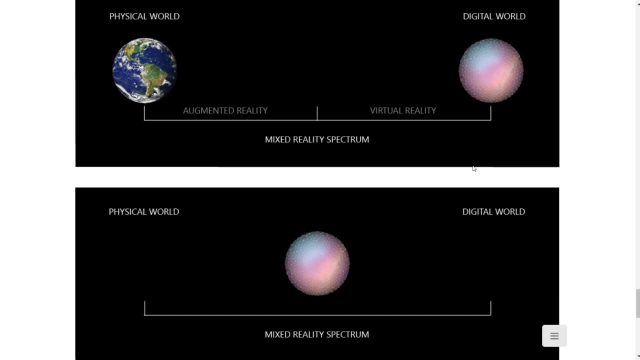 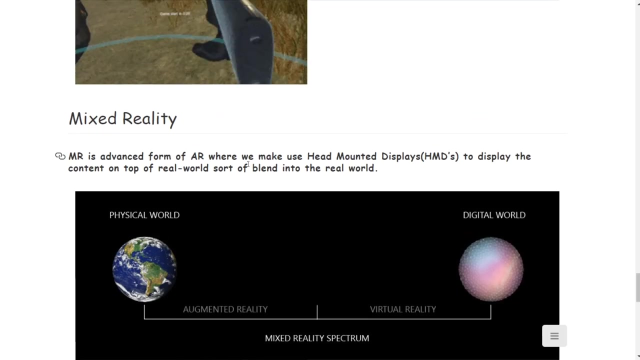 so mixed reality is nothing, but you know, it is the advanced form of augmented reality. alright, it contains both. it means it can go both virtual and real. alright, so that's what mixed reality is, alright. and you have already understood about the mixed reality spectrum. that is the combination- alright, that is the combination of physical and digital world. alright, so that is what mixed reality is, alright. and also, this image is taken from Microsoft's website, so yeah, 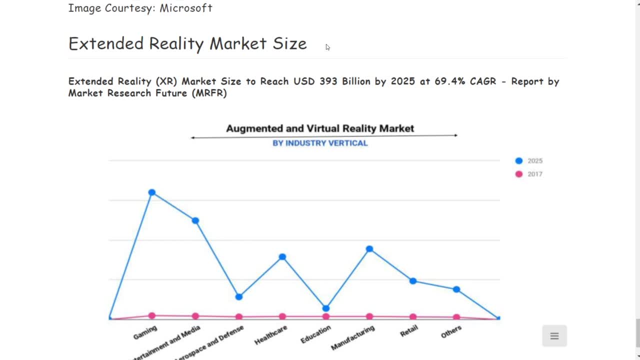 now, as we have understood, alright about all the things, alright about mixed reality, augmented reality, virtual reality, let's, you know, let's get our heads into the growth of XR, alright, or you could say the growth of market, of extended reality. alright, see the extended reality, market size, alright, is going to reach alright around, you know. 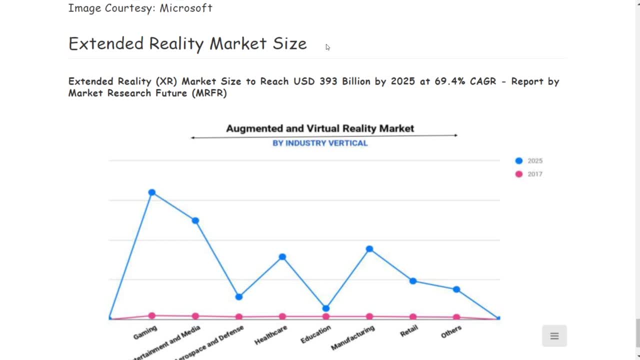 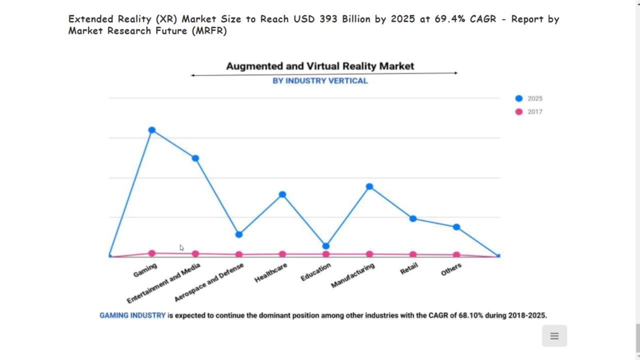 393 billion dollars by, you know, 2025, at a growth rate of 69.4% CAGR. alright, it is a report by market research future. alright. now you can see that in 2017, the growth was the growth was. so less alright means there wasn't any awareness of augmented and virtual reality, but you can see by 2025, what will be the growth. alright, you can read this chart by yourself. alright, so 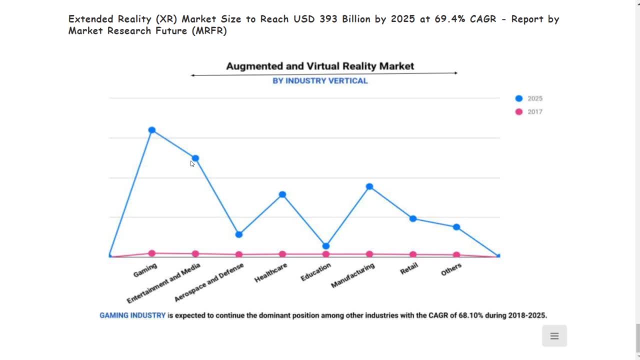 you can see how, how it is impacted. now I want to tell you that this chart- alright, this chart is- you know, this chart is not stable. alright, right now, in 2022 only, the market has reached more than 200 billion dollars. alright, so you can see, you can see how, how the growth is actually. it can even happen by 2023,, alright, by 2023, it can even reach 393 billion dollars. 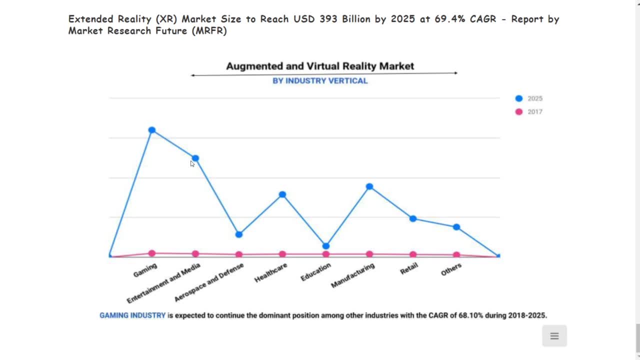 by 2025, so, alright, so make sure you know you go through all these notes. alright, all the notes will be available in the website, so make sure you go through that. so, yeah, that's it for this lecture. thank you. 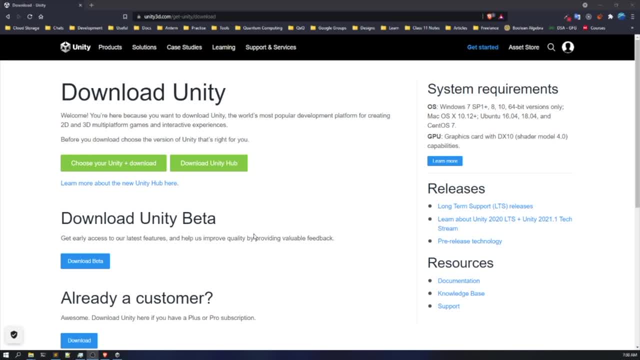 Hey folks, welcome to our module 2, and in this module I am going to tell you how to install Unity and after that I am going to show you, or tell you, how to use Unity. alright, what are its interfaces and all those things? alright, so 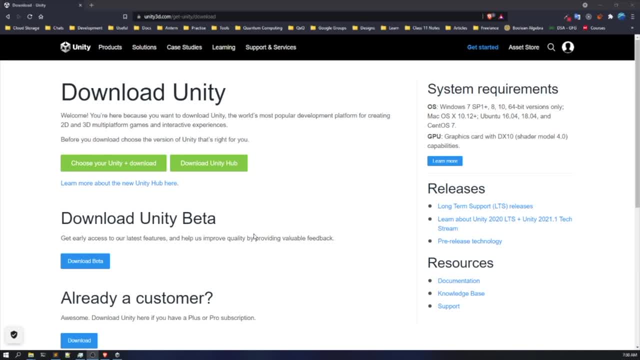 sit tight on your seat and watch the video. alright, if you want, you can grab some popcorns also. so, yeah, yeah, first of all, what is Unity? before downloading, we must know, yeah, what is Unity? if we don't know about that, then how could we work with that? so we need to know what is Unity. see, Unity is an engine. alright, it's sort of a tool. it's not sort of a tool. 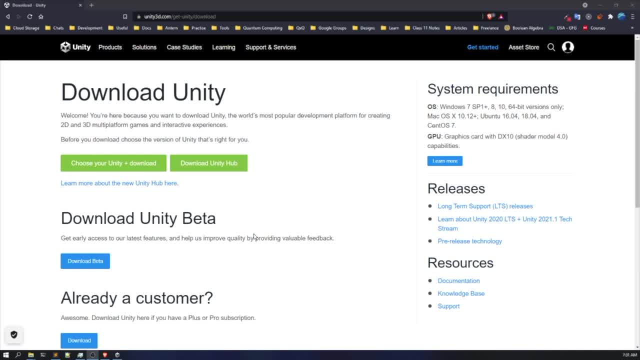 a tool. it's a definitely a tool. it's a tool for developing games, for developing simulations, for developing arvr applications. all right, uh, you can even make your own simulations. like you can develop your own um robot, inside of unity, you can develop your own uh, let's say, uh, self-driving car. 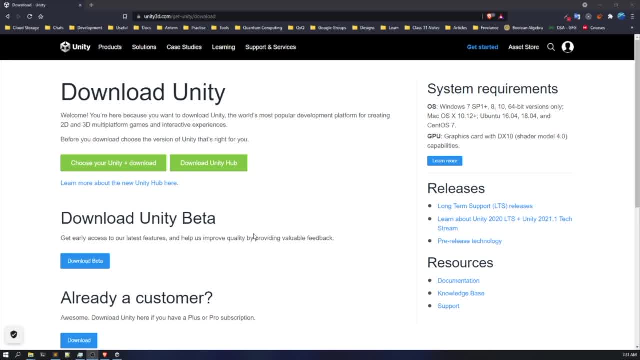 you can implement your own self-driving car inside of unity. yeah, that's possible. that is 3d simulation. so, uh, and one of the most like most, one of the best things about our unity is it is multi, it can, it works on me. unit, uh, linux, it works on mac os. it all works on. 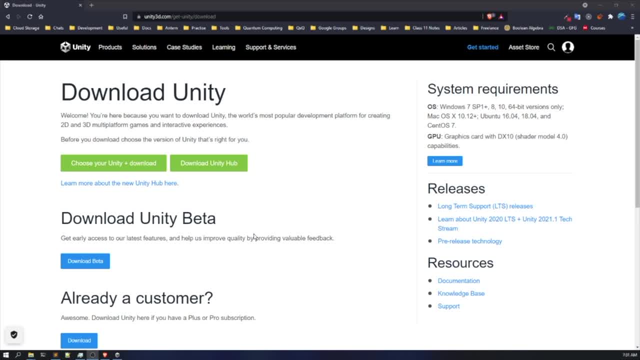 um, windows, all right. and also you can build- uh, actually, you can actually build applications, all right. uh, you can build your games, your apps for multiple platform: windows, mac os, linux, then android, ios, playstation. then i guess it also has a feature for, uh, xbox also. i'm not sure about that. 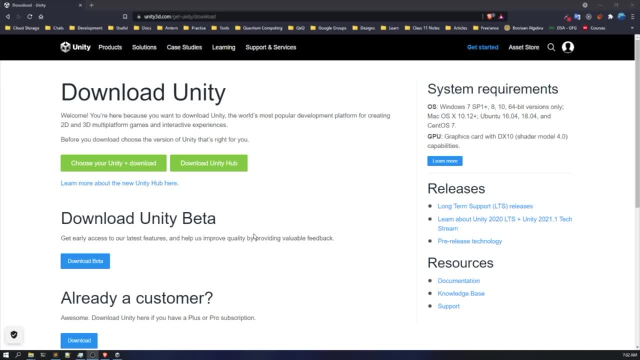 i haven't researched about it. then there's also uh lumen lumino is. then there's uh web gl. so, yeah, multiple things are available, all right. so, yeah, that's what unity is. unity is a very good tool for developing these things. now, what you need to do? uh, you have to go to this page, all right. 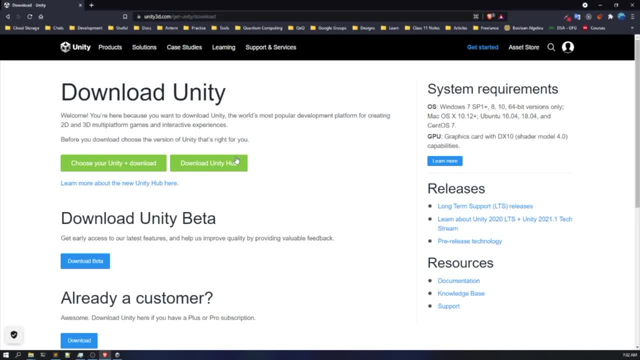 i'll be providing the link down below right and, uh, click on this. all right, just just click on this. download unity hub, all right. after you have downloaded, install it. all right. these processes are very simple. i need not to show you. i'm pretty sure about that. now, what do we do after you've? 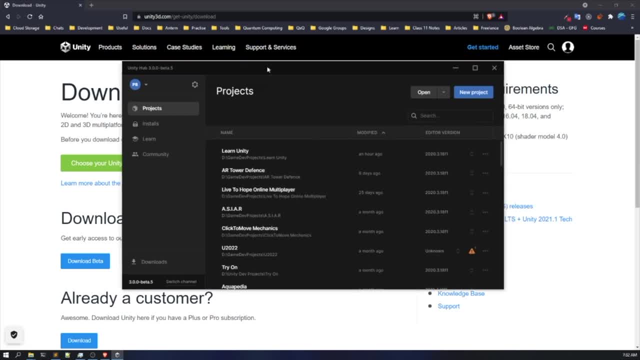 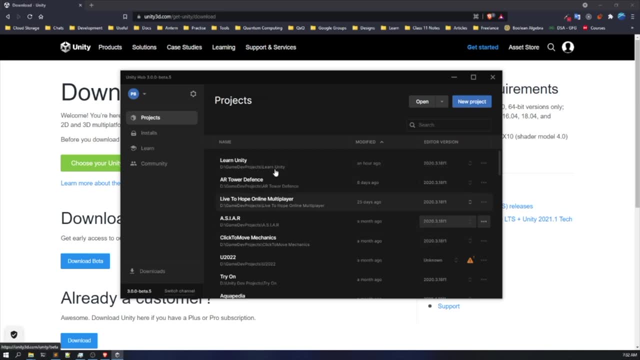 installed on it, open your unity hub. it will. it might not look something like this. all right, because this is a beta version on it. uh, it's a beta version of it, all right, so let's go ahead and it's in. currently in beta testing, all right. it does have some bug, like recently i ph. 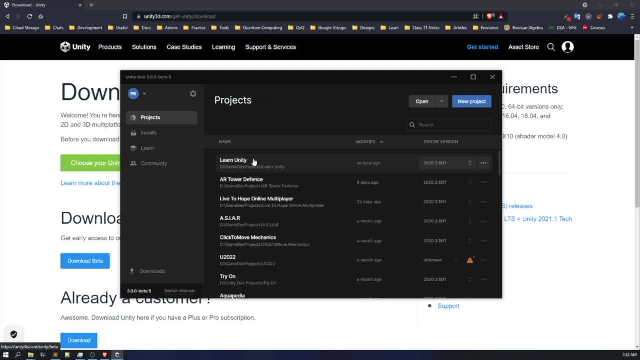 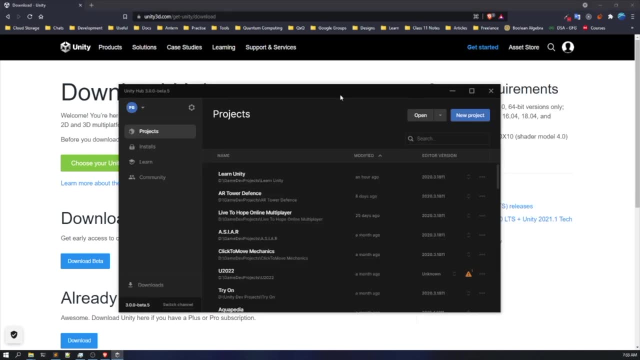 phased one, that it wasn't grabbing my license, but i had to restart it and it like worked really well, so yeah, so basically, uh, it might uh seem a bit white, all right, the interface might be white, but components are uh same. so when you first open your unity, all right, log in. log into your account. activate your license. 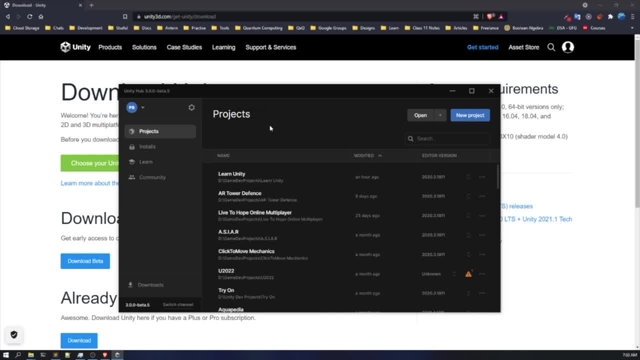 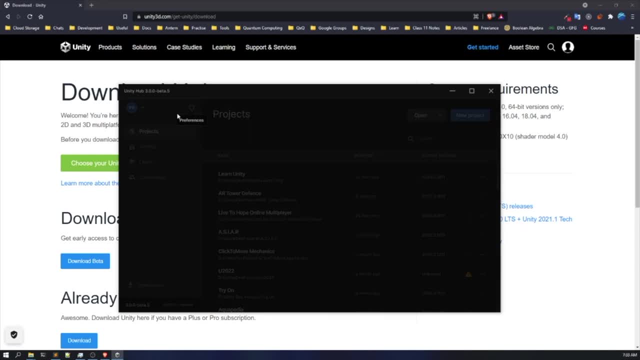 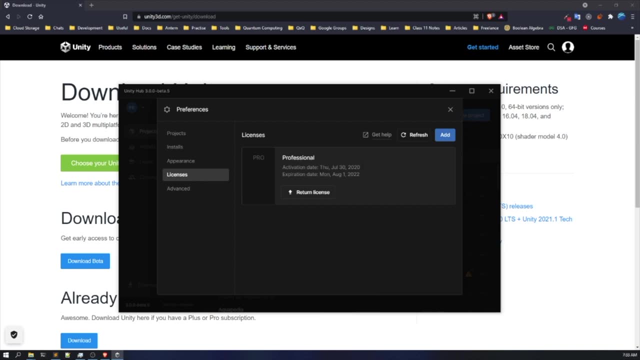 it will only show you like it will by default. uh show you how to activate your license. all right, you just need- and if it doesn't, uh go to this- click on this like preferences option. all right, uh go to these licenses. all right, i have a professional license. i got it through student. 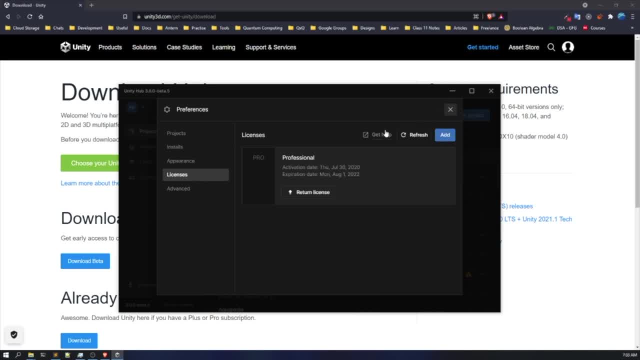 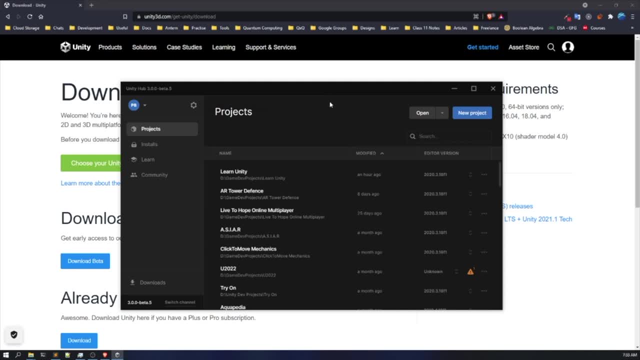 plan and click on add and, uh, choose any license you want. all, right, now let me show you one thing right? um, this is the basic of our wholeufenyardre plaster, of all right, the basic interface of our whole unity hub. right through this we have to run our unity. this is the project. 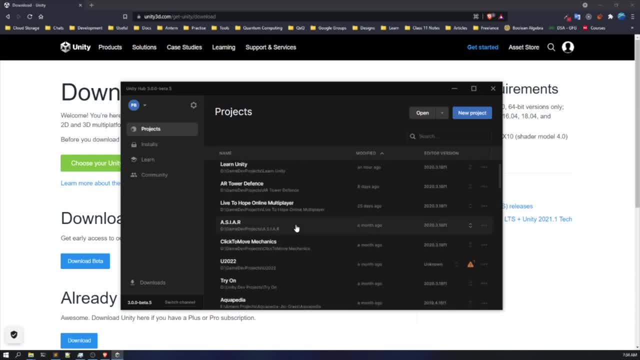 uh section. all right, in this project section, multiple project of yours will be like. put it in here. like will be listed down here: uh, as you will be installing uh unity for the first time, it won't show any uh of the projects. it will be totally empty. these are my projects, all right. 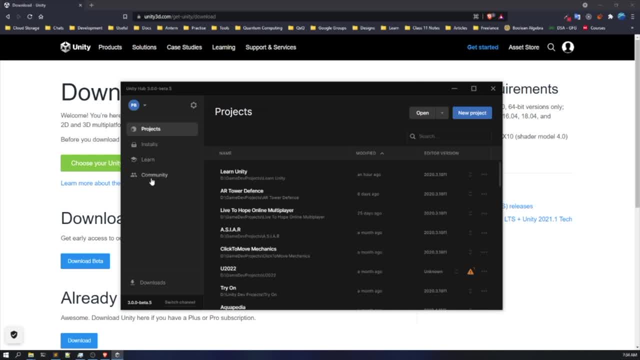 tabs also. I'm sure you would explore this learn and community tab, but for now, let's go to this install tab. so in to install our own unity version. all right, now, this is my unity versions. all right, these are my unity version that I am having that is going to 2020, 2019, 2018. all right, these are my unity versions. I. 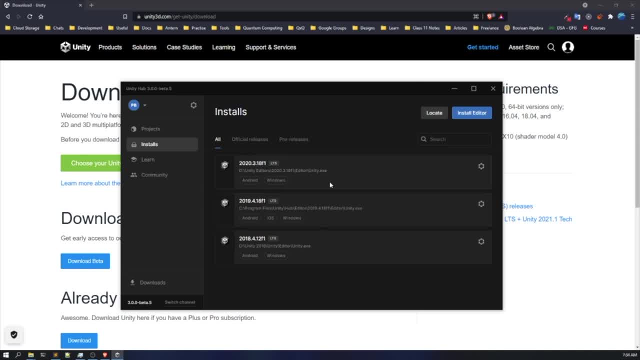 have installed those. I work with these, mostly these two version, more often. all right, now this this panel would be empty. all right, this panel would would be empty if you haven't installed any, if you haven't installed any of your unity versions till now. so to install one, just click on install editor. all right after. 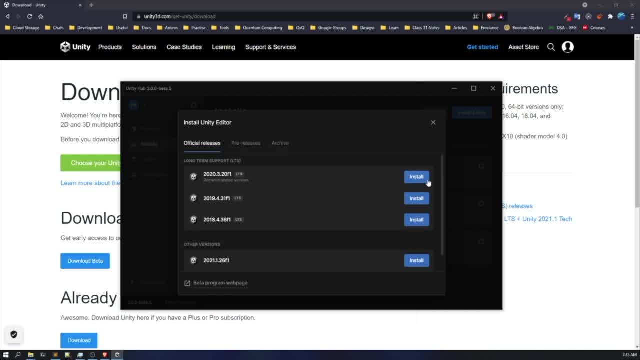 that it will prompt up a menu. already there are multiple versions in here. all right there. multiple versions in here. I'd recommend go for 2020, all right, even unity recommends this as of now, and also always download the LTS version. why LTS is limited time support and it's it's the most. 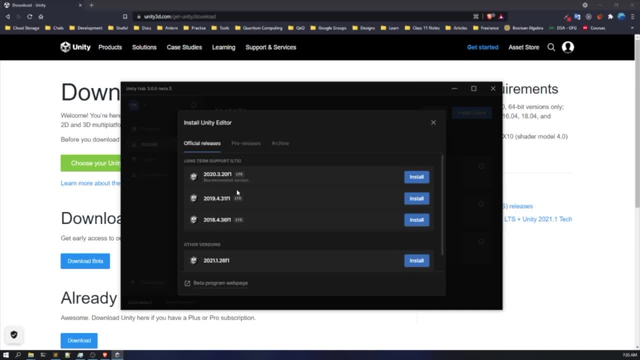 stable version. all right. it's the most stable version that we would have, so always download a stable version, and we'd also if doing our development in unity 2020 only so I would recommend download it all right to then click on install now. you can either install this: all right, any- actually any- ID or code. 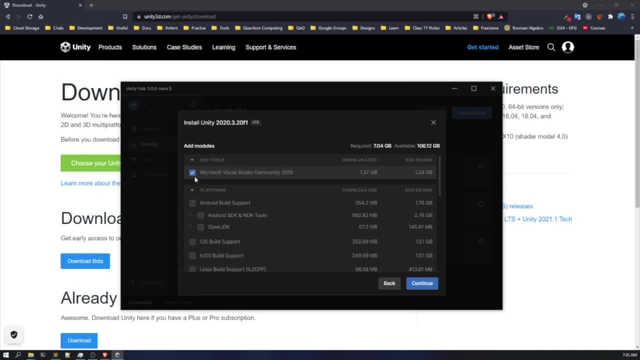 editor would work, but maybe you won't get the code completion on that. auto complete what I would suggest: downloading it all right, so download this too. all right, if you are Linux you might not get this option. then you have to use any other code later only. but another thing I would want you to do this: 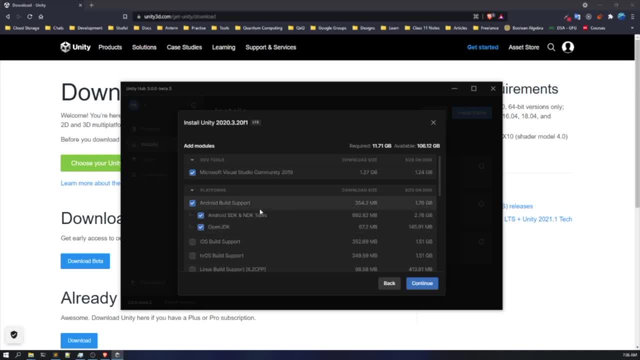 is: click on this Android build support and SDK and indica tools and open JDK, all right, and remove this checkmark from the documentation. we don't. we can access it from web. all right, and there are other like build versions too. you can also look, take a look at these and download them. then click on continue all. 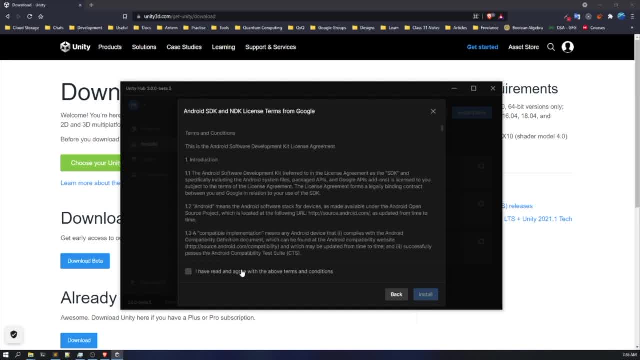 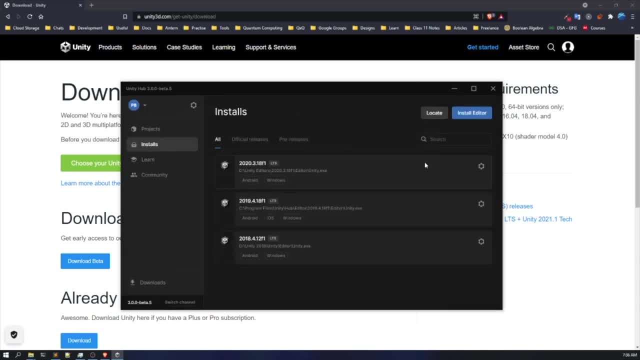 right. click on this. I have agree and all those terms and things. click on this alright, and then click on install- all right, and it would start installing your editor right and after. it gets installed or it just downloads and it will show if any of you in any of your data is installing or 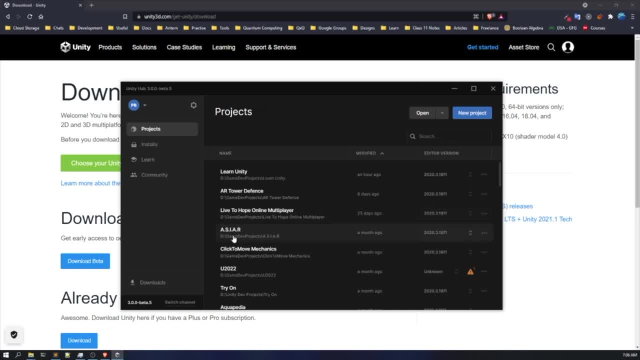 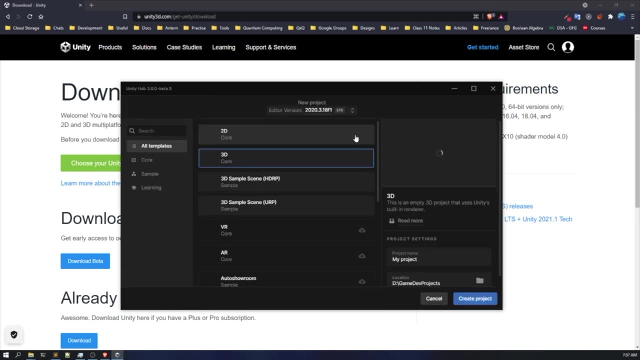 not. and now, if we want to create our own project, click on this new project option. let's sorry, it's taking a bit of time. I it's, it's a it's a bit buggy, so, yeah, I'm really sorry about this thing. yeah, so, as you can see, here are multiple templates. 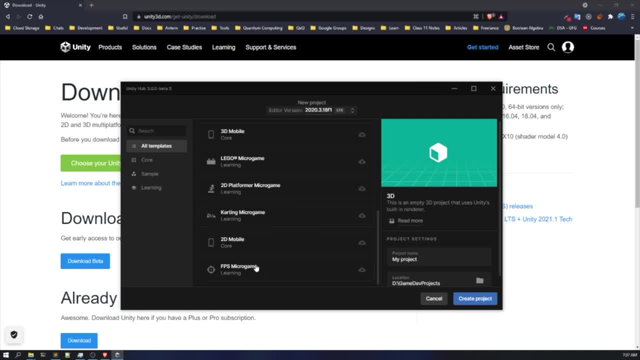 available right, and multiple templates are available there. if this micro game 2d mobile carting, micro game, Lego 3d mobile auto show, alright, but for now we have to work with these two only. all right, not even the 2d one, we have to. 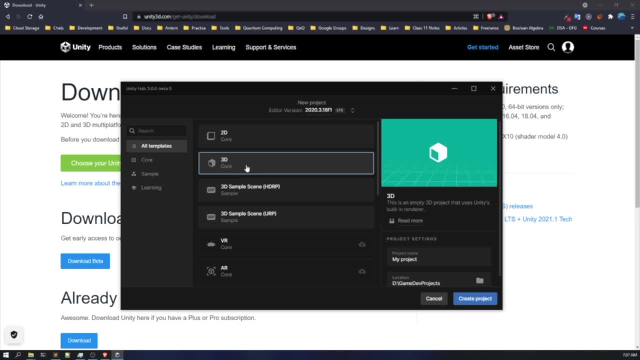 work with the 3d only, all right. so what we have to do- see there are multiple options like another- is this 3d sample scene, HDR, P and URP. so basically what this does is this: basically gives you a more better graph, is more optimized. 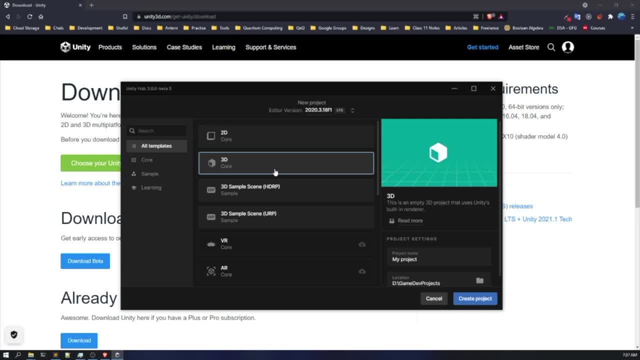 graphics, all right, URP better, best works for best works for us, like computer systems, and the URP best works for mobile phones- all right. so yeah, and then you need to name your project. all right, name your project in here. I want to name my project, let's say, learn. 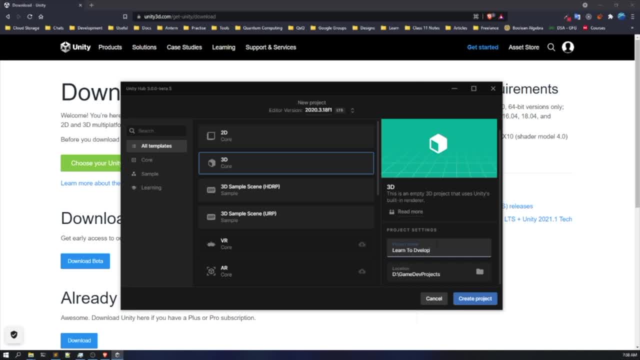 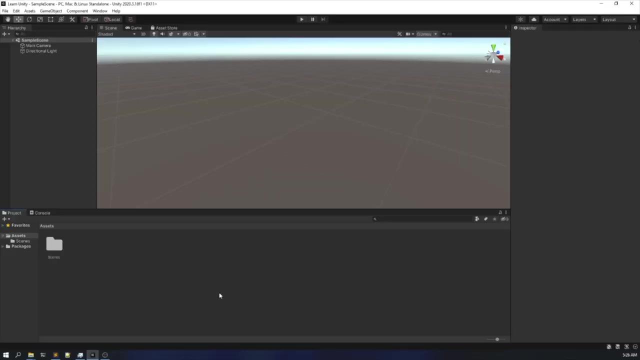 to develop. all right, I'm sorry for the spelling mistake- all right, and then you can simply create project and your project will start creating. all right, so we are. that's it. this is the base procedure, and I have also shown you how to install unity. so, yeah, thank you. so hey, folks, welcome to this video and in 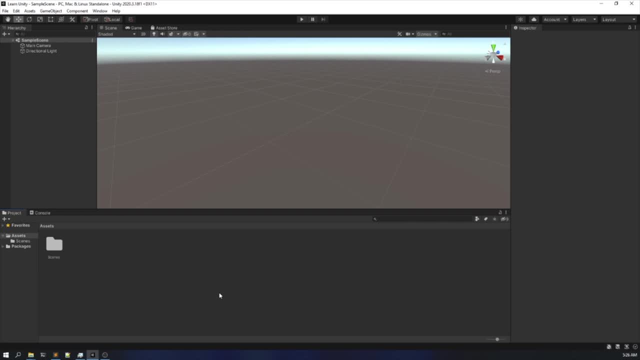 today's. this is the second part of module 2. all right, in the first part of the module, I gave you an introduction to unity and also told you how to install unity and create your first project with it. all right, but now in today's video, we'll be covering rest of the topics, all the rest of the. 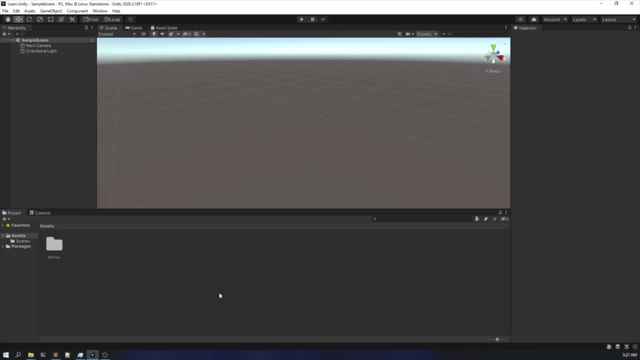 important topics that are left. all right, so without any further delay, let's get started. so our first topic to cover is navigating through interface. all right, so we'd be navigating through our interface, learning about what, how, like, what are the different components of our interfaces? all right, so first we have to 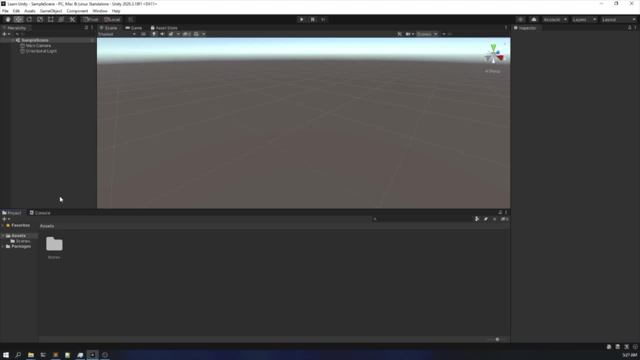 start with our project window. all right, so the part here you are seeing, all right, like the folders here are. this panel is particularly known as the project panel. all right, this panel. in this panel we can create multiple. all right, you can kill multiple as many as folders we can. we can add our own 3d. 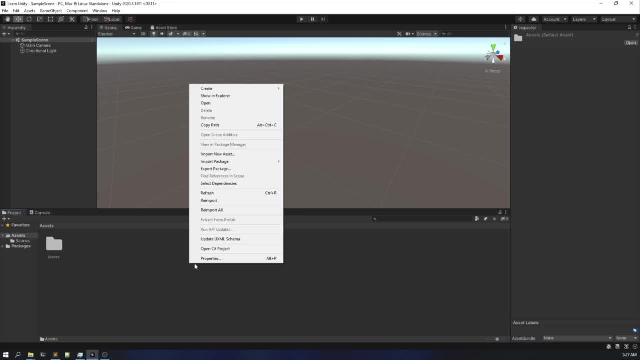 models and all those right. so just to create your own folder in here in the project project panel, just right click in the panel, go to this create option and click on a folder, all right. so I want to create a folder named materials, all right, where I would be storing my materials, right? so this is my, my. 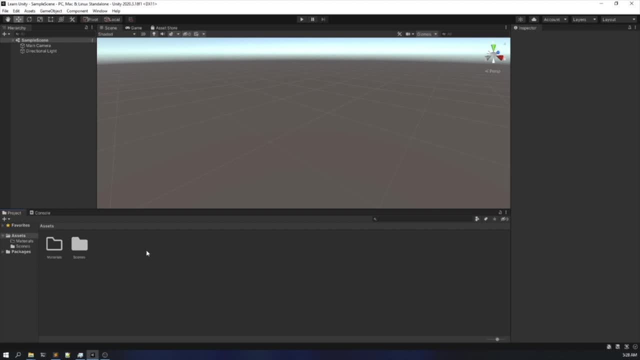 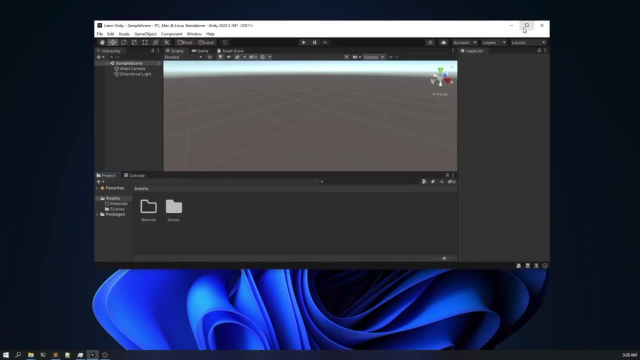 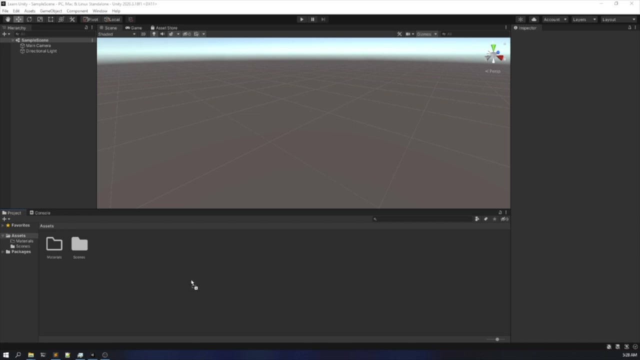 material folder. right now in the project panel, I can even add numerous amount of assets, right, like if I. if I show you, just just wait, I'll be adding an audio file in it. all right, so this is a bird and beach file? all right, I'm going to add this audio file in it. just wait for a. 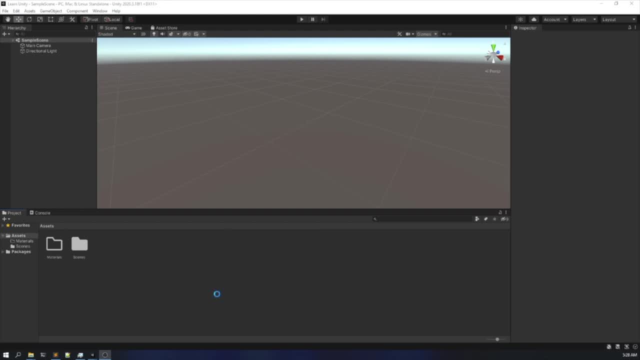 few seconds and the file will be imported. it does take some time, all right, because currently I'm also recording, so it took some amount of time, but it's usually fast. so here I have just what I did. I just dragged and dropped that particular audio in here, all right. 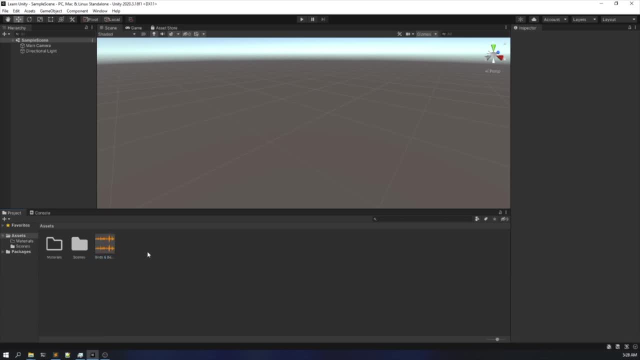 you click in here, you can even play that audio, but I don't want to play it right now. so yeah, so we learned about our project window. now why do we develop a little? while we develop our own games, our own application, we face multiple bugs, we face multiple errors, right, don't we? we do so, we do. where can 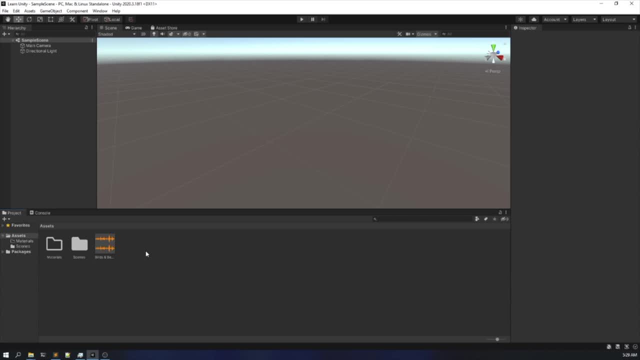 we see those errors? where can we look for those errors? right, so unity has provided us something known as the console window. all right, it's just right here. all right, us are like. only after the project: if you don't have this console panel or console window, just go in this top section named. 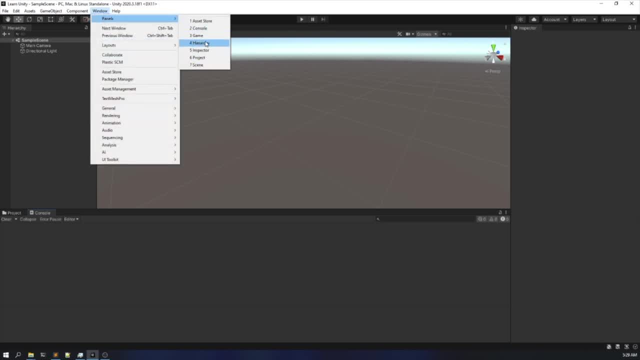 window, click on this, click on panels and just select that panel that is not available in this in your workspace, right? so currently it's and empty. right, and it's empty. I will show you how an error will look like. but yeah, in here you will get all the errors and warnings and particular debug texts in here, right? 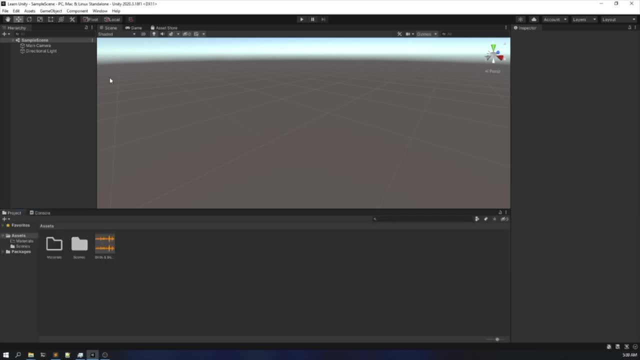 so this is our console window. now here comes our another window or panel, that is the hierarchy panel. so what is the hierarchy panel? all right, see, there are multiple objects in this the scene. all right, don't worry, I will make you make you understand what the same is. but currently, uh, currently, there are like two objects, that is a one. 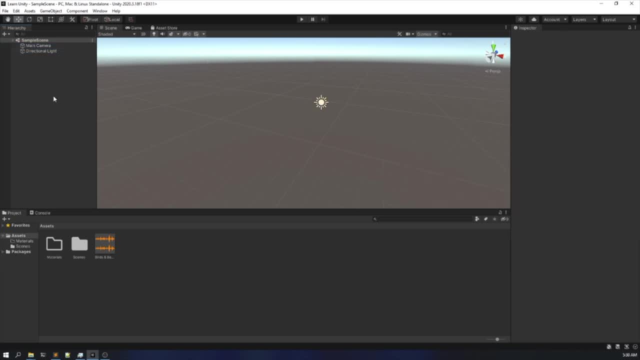 light object, another is a main camera object, right? so hierarchy panel, what it does is it lists down. all right, with the help of hierarchy panel, we can just right click and create our another object, right, i would show you how to create one. but hierarchy is basically, uh, the structuring of 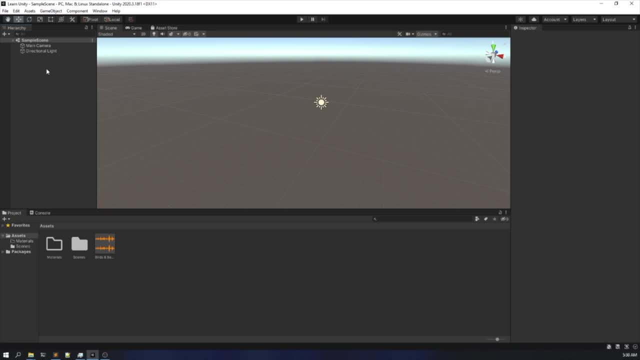 or like the objects. it is a panel where you would be able to see what objects are available. uh, inside of the scene, all right. and through the hierarchy panel you can create your objects, you can modify them and all those things, all right. modifying is done by another panel, actually. 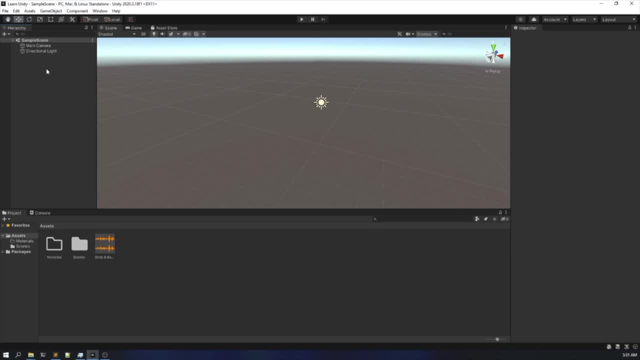 i would show you right now, after the hierarchy: all right, so this is what our hierarchy panel does, right? so we understood what our hierarchy panel does. now, here comes our inspector panel. all right, so what is this inspector panel, man? what is so this inspector panel is basically used for? 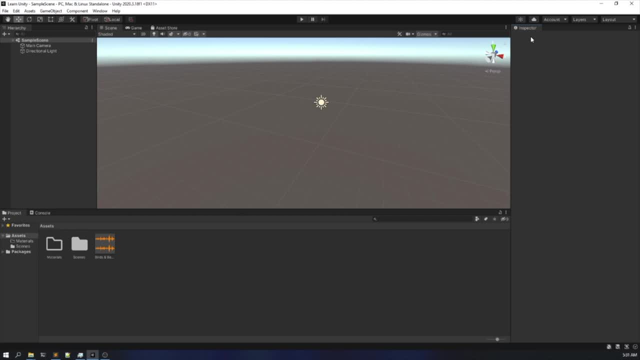 what can i say? it is basically used for modifying the components. all right, it displays the properties of the object. all right, like if i click on the main camera right. so here you can see here multiple, multiple uh components. here there are multiple options are there we can manipulate. 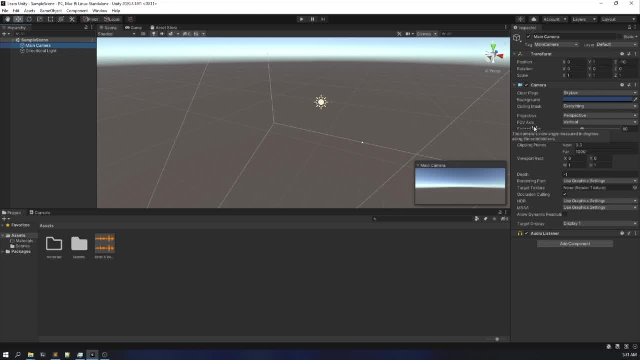 those of these options and, uh, like we can manipulate this and make the camera component look our own way, all right, we can uh edit these components. right. so inspector panel gives you an inspection of that object. right, it gives. uh, it helps you to edit those options inside the object. all right, now, as we have. 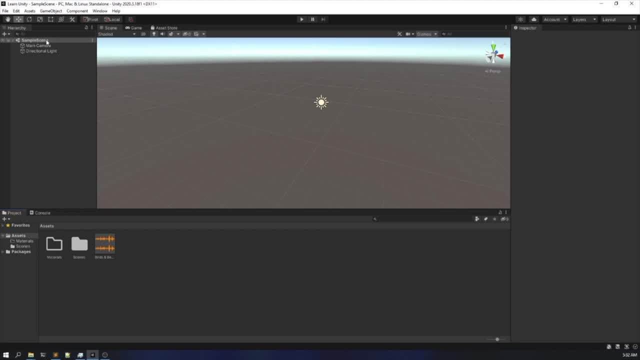 so tell us what, uh, which panels have we looked? we have looked into the project panel, the console panel, the inspector panel and the inspector panel and the hierarchy panel. now it's our time to look into the scene panel. all right, see scene. the scene panel is nothing but a whole different, like it's. 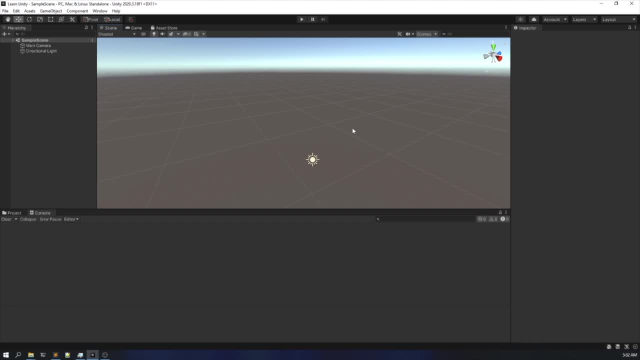 a. it's a workspace, all right, it's a. it's a workspace where we can actually put our models in right, like our 3d objects. in there we can put our 3d of your engine like main camera. main camera is inside the scene, main camera is inside this. 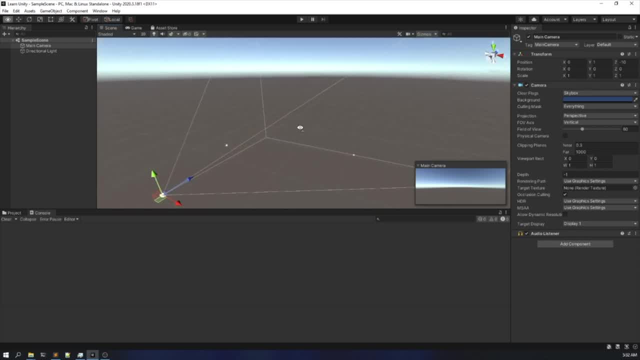 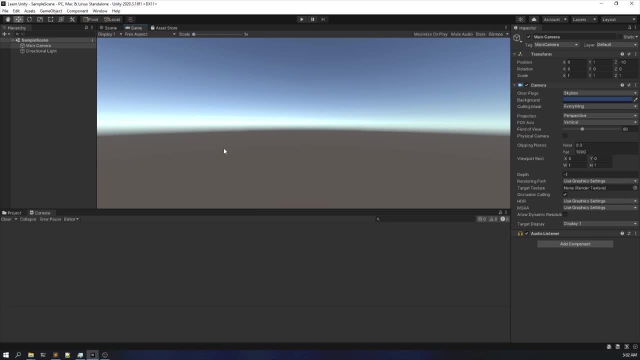 whole scene. right, it's in this 3d workspace. so scene is the 3d workspace right now. after that there is another panel. that is this game panel right now. what is this game panel? see, this scene is for navigating through. all right, we can manipulate these objects like like this. all right, we can. I would show you. 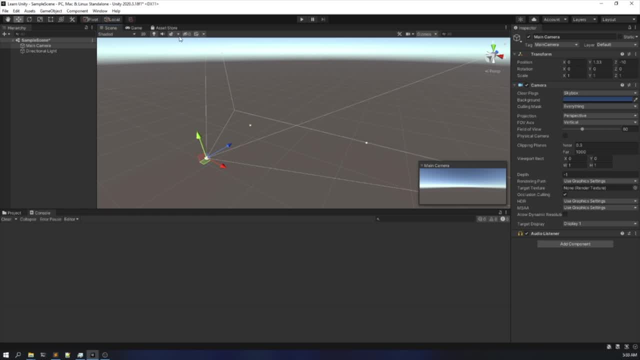 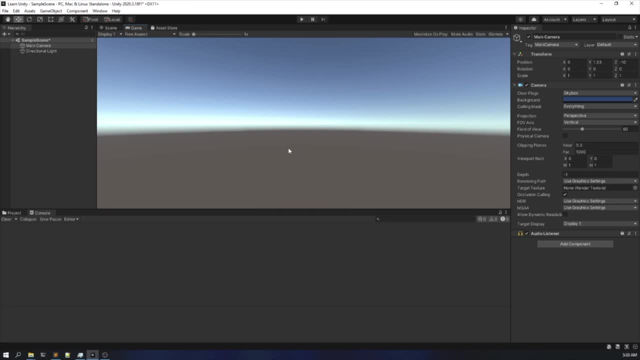 what are these? but we can manipulate these, we can put our 3d objects in there, but game game is the rendering part. all right, like after our like. let's say, I have made a 2d game for now. all right, but I now I want to test it out, I want to play it. so what I will do is I would. 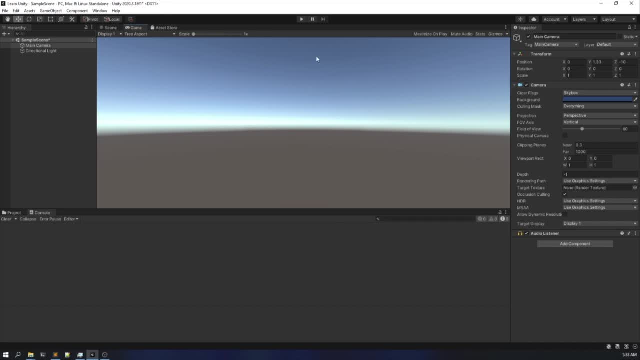 play that particular game and or in this screen. all right, in this particular screen or in this particular panel, the game will start showing, right, so yeah, now here comes, Oh, another thing. here you can see three buttons. all right, these are the play buttons. this one is the play button. this one is the pause button. this 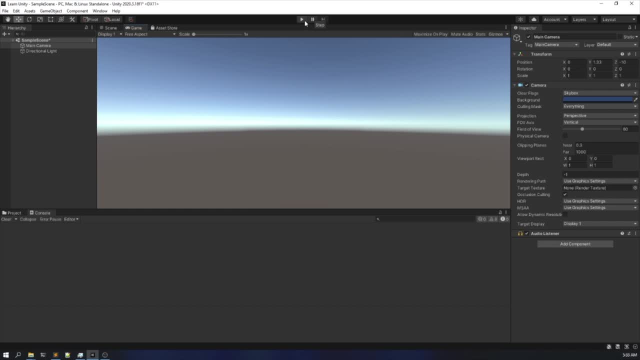 one is the step button, right? so what this play button does is just plays the scene, all right, that is, starts the rendering. this is like the pause button: it will pause while you are like like rendering it and the step now the statements it will like. after we have paused, you can click on this step button. 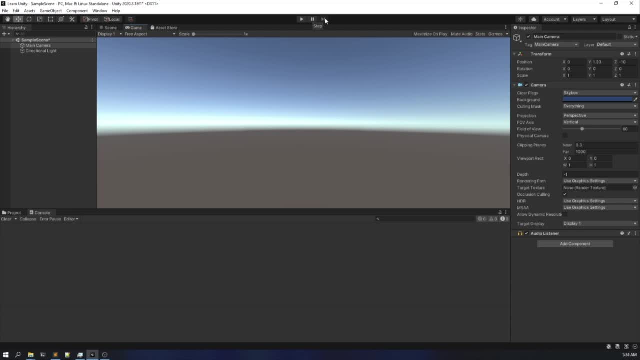 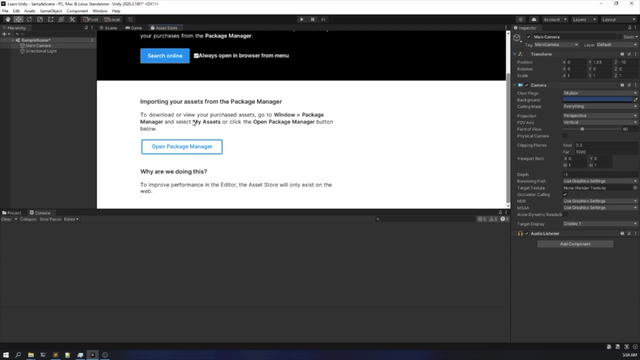 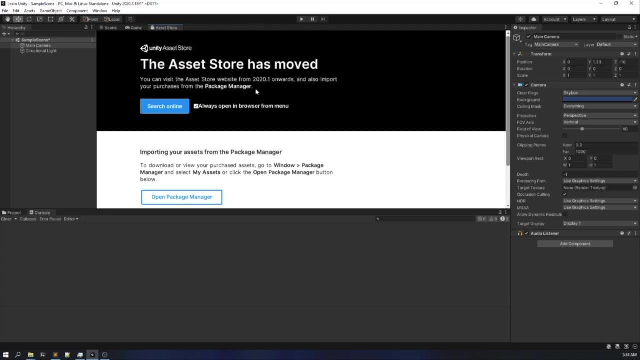 it will like move one by one. all right, I'll show you those. all right, I will show you these. now here comes another panel. this is the asset store panel. all right, now one thing to notice here you can see. it has told that they have moved, like the asset store, to the web. all right, and I 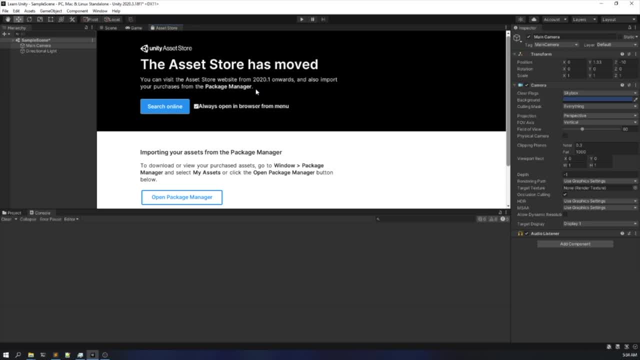 don't know why they did so, but actually I prefer that more because in my system the unity asset store used to lag all right inside of unity, so I think that was a good idea. but the main difference, all right that you would notice as a beginner in unity 2019 and 2020 is that in 2019 the asset store is 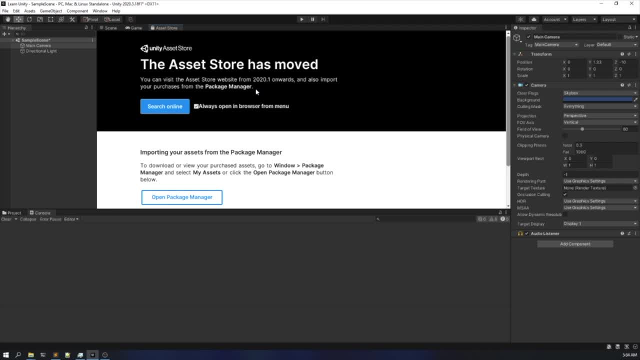 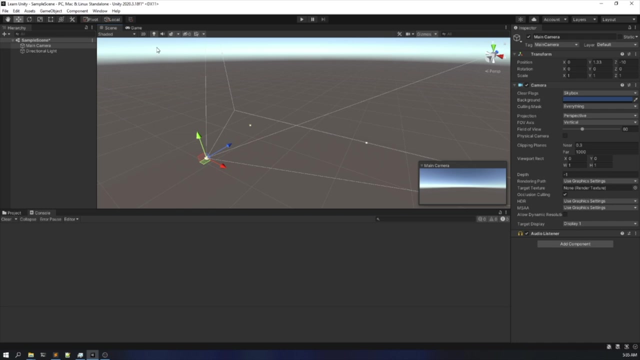 already integrated in your like whole unity and in 2020. the asset store is on the web browser. all right, so you can access it on from the web browser. all right, so we don't need this panel as of now, so I will just right click on it and close that, all right. one more thing I would like to show you is 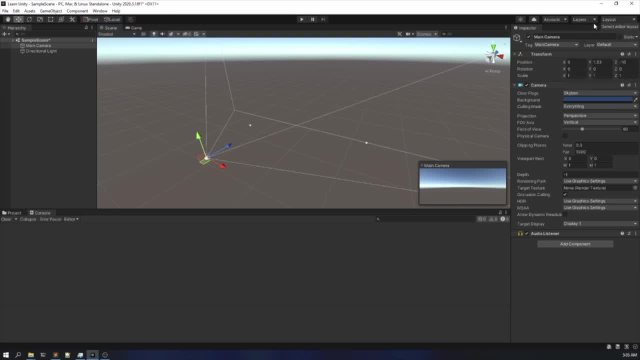 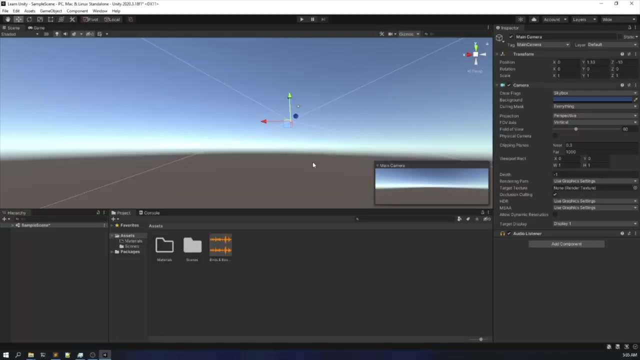 there are multiple layouts available in unity. all right, that's just like go to the right of your screen and click on this layout. there are multiple layouts. all right, you can try any one of these and one of my very favorite. all right, just just wait for it. yeah, one of my very favorite layout is this one. why? 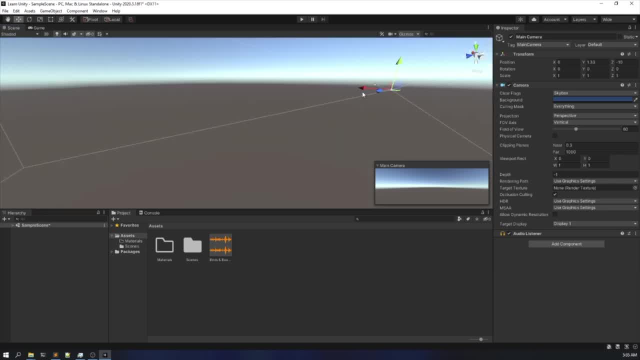 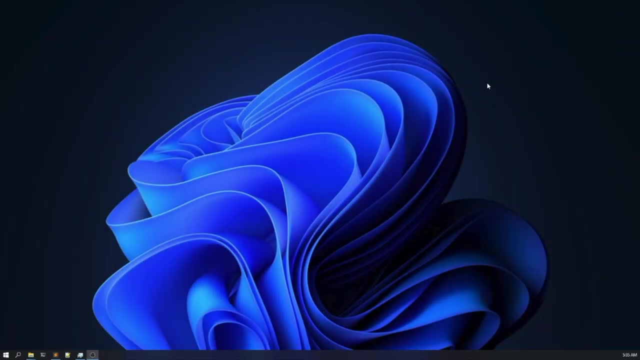 because this gives are like more broader view. all right, this gives a more broader view of this scene. all right, it gives them. it gives more free space to work on. so I like this one the most, but for now let's go to the default. all right, we'll be working on the in the. 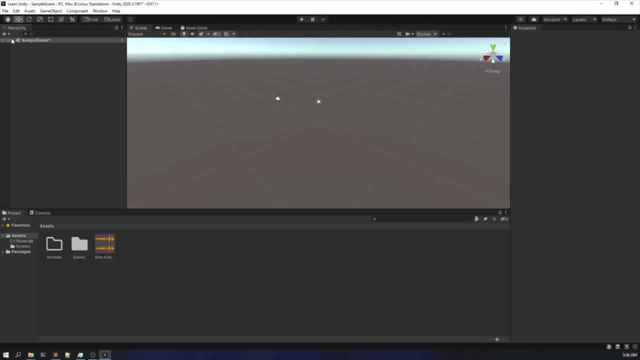 default only as of now. so, yeah, so let me save this. yeah, so we have understood that, the very basic interface. now let's go and look at the tools. all right, the tools that we have. so first of all we need, but before that, looking into the tools, we have to understand our game objects, all. 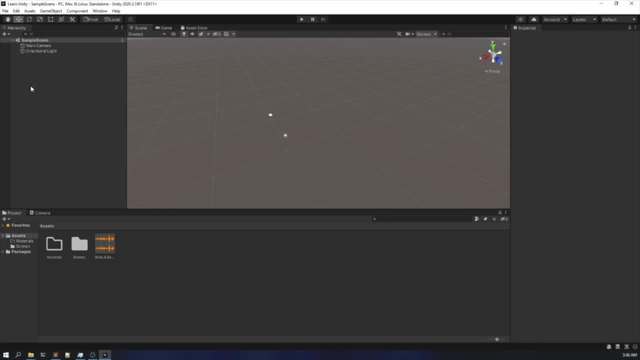 right. so see, we have got into another section, that is game objects. and what are game objects? so see, game objects are digital objects, all right. game objects are those digital objects that we can use digitally. all right, game objects can be anything, all right, I mean anything. it can be 3D. 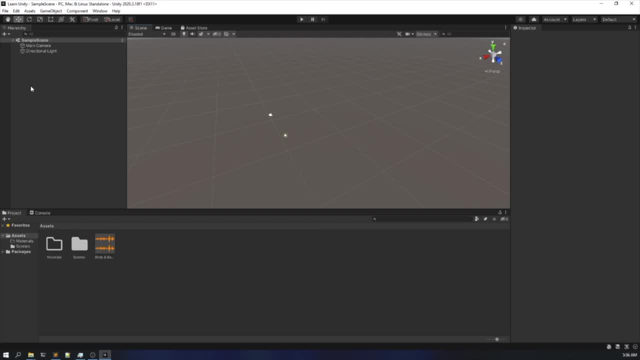 game object or 2D game object? all right. so what are game object? basically, game objects are virtual objects, nothing else, right? so like, like an example, this main camera, it's a game object, all right, it's, it's a game, a game object. now, this directional light? all right, this is a game object, right? so yes, similarly we. 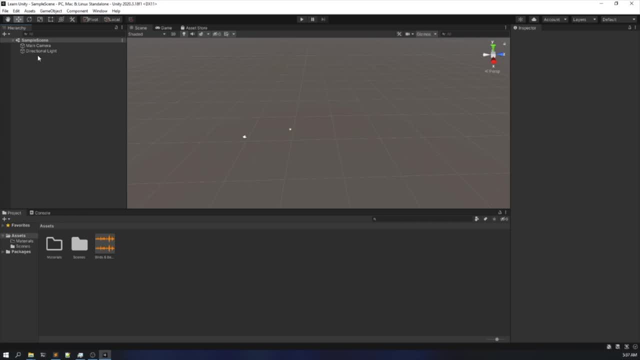 can create our own game objects, for example, right designed of a game you can decorate with games like this. so we can create objects like: just just uh, go to this hierarchy right, click in here, uh, click on this 3d object, all right, click on this: um cube right. so we have created our own cube right. so now. 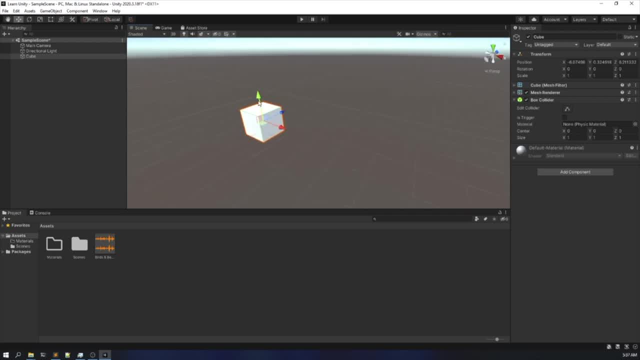 here you can see, there are multiple anchors. right, there are multiple anchors. i will tell you what are these: in the in the top, here you can see, here is a toolbar. right, here is a toolbar. so what does this toolbar does? first, first of all, uh, first and foremost, there is a tool named hand tool. this, uh. 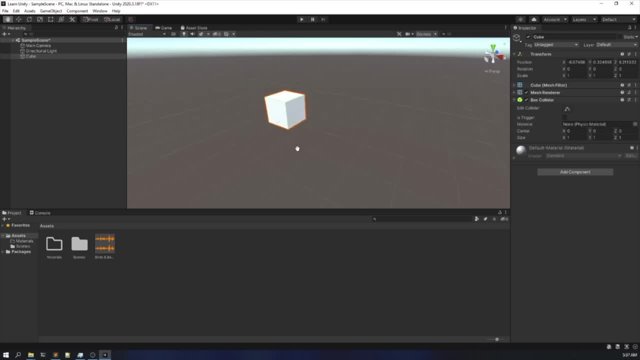 is uh used to like, uh, grab the screen and navigate through it, grab the scene and navigate, just just for that now. after that, after that, we have move tool. this move tool gives you some certain anchors, right, uh, where you can hook on. all right, you can hook uh. with those anchors, you can move your game. 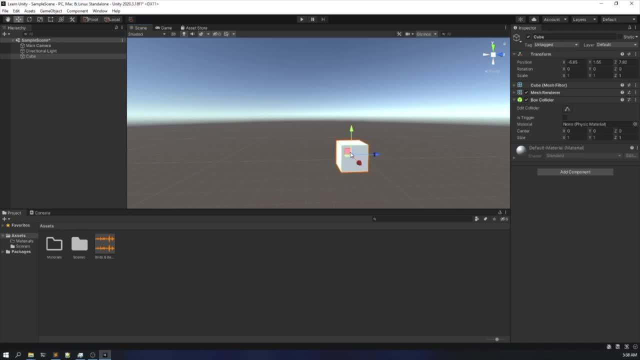 object throughout the screen, right? so that's what it does. after that, we have a rotate tool, like: if you want to rotate your object, i can. i can do that. it gives rotational accesses through which i can do that. right, isn't it like really fun. now, after that rotate tool, there's another tool that is a. 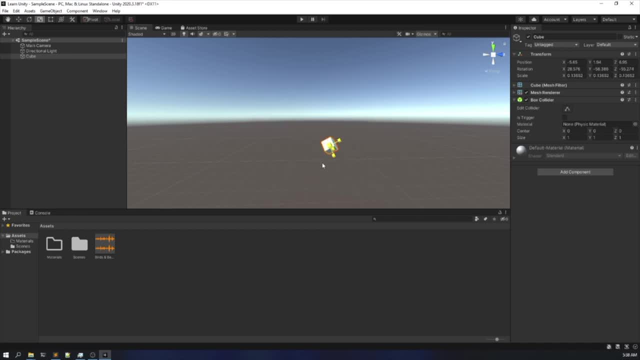 scale tool. it helps us to scale the screen and navigate through the screen and navigate through the object. scale the object. all right, like you can, i can scale it in any, any uh axis. i'm scaling it at any axis. right after that we have a rectangle tool or rec tool. all right, what? 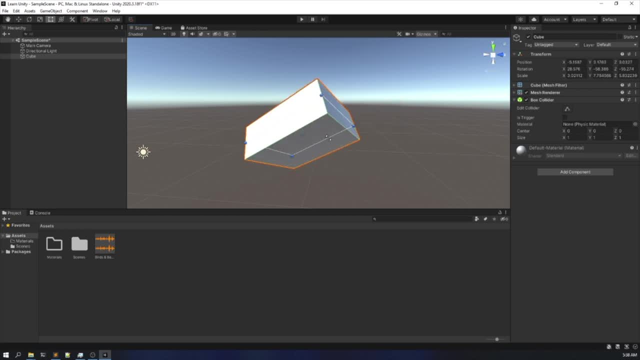 is this? it just like helps you to resize the object in a rectangular manner, nothing else. now then we have a universal tool. uh, i guess this is called. uh, oh, this doesn't have a name actually, but i will call it universal tool. all right, so it is a combination of all the tools we discussed previously. all right, except the hand. 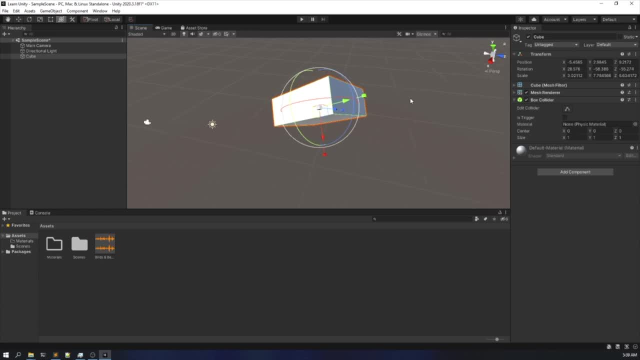 tool and if you would see, uh, i am able to use the hand tool. uh, even when i am like not uh selecting it or like externally selecting it, it's automatically getting selected. so the basic shortcut for that is, sorry, to click the uh middle mouse button right. so 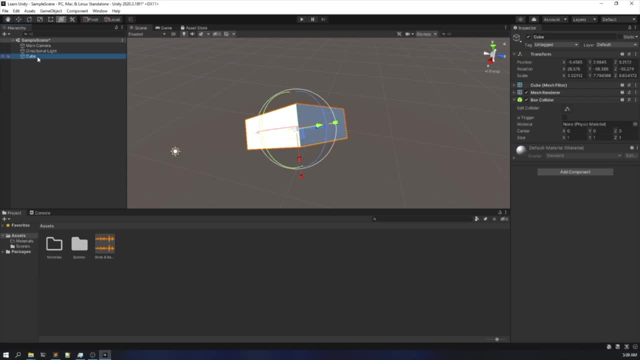 i'm really sorry about that, uh. so, yeah, uh, we have created our own cube. we learned about game object, right, we learned about game objects. now, our- uh, just just wait, i want to like reset all the things now. i want, uh, to play with it, right, i want to manipulate it. i want to manipulate this game object. how to do that? 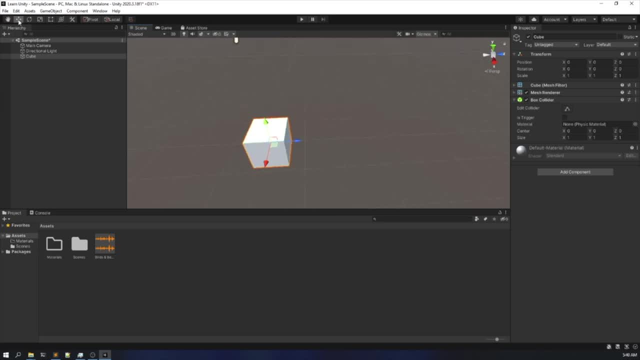 first of all, i can use these, uh, these several tools, these fancy tools available, or i can uh go to my like simple methods, like uh, as i previously told that, in the inspector menu. inspector menu gives us the properties of the game object, so we, with the inspector menu, we can edit those. 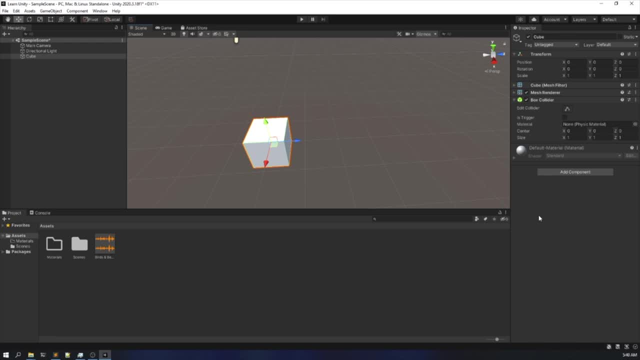 properties too. right, we can. so how do we do that? first of all, let's say i want to edit the transform. all right. so what are the transforms, man? what are transforms like? see, i am moving this right, i'm moving this like this, i'm i'm able to rotate it also. so what is that? the? the things are like. 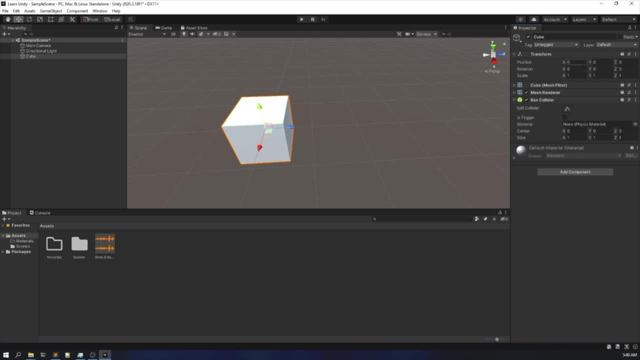 moving at a particular direction. we can also do the same thing through this, like inspector, meaning like here you can see there are three parameters, like: first of all, see the transform here. first of all see the transform. here comes the position. so what does? what does it does? it changes the position, like i want to be it, at 10 of x axis. 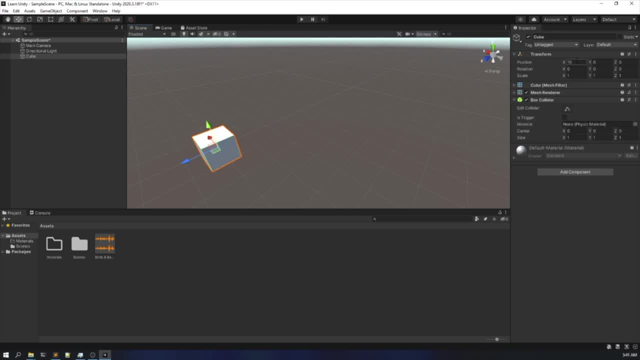 right, so it has got to 10. then, uh yeah, you can simply manipulate your position from this, but for now i want it to be in zero. right now, rotational values: all right, let's say i, i, i want my cube to be rotated 45 degrees at x, 90 degrees at y, and let's 45 degrees at z. so i rotated my 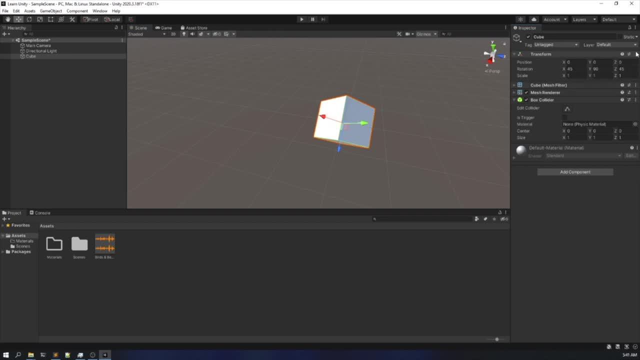 cube, right, i did, rotated it. now one thing you'd be seeing like: let's say, you messed up with all these uh parameters. now you want to reset it. how would you do that? just click on this, three little dots. click on reset. as simple as that, nothing much. all right, you're going to. 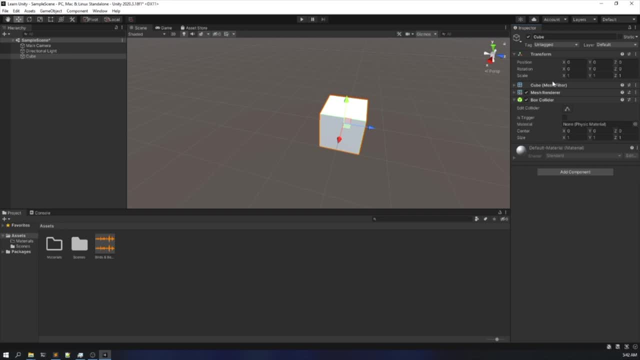 also scale it. all right now, this is your homework. you have to try this scale portion by yourself. all right, you have to try the scale portion by yourself now. here are some other other parameters too. all right now, this is a cube mesh filter. all right, uh, then there's a mesh renderer. i want to 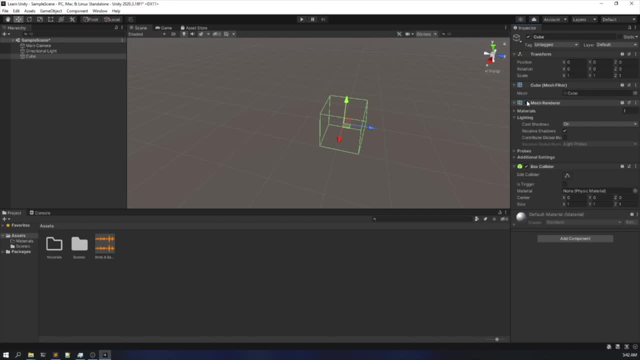 show you something. if i, if i remove this mesh renderer, you won't see any sort of mesh. all right, what are these green lines? these green lines are the box collider. if i, if i remove it, you won't see any sort of mesh. all right, what are these green lines? these green lines are the 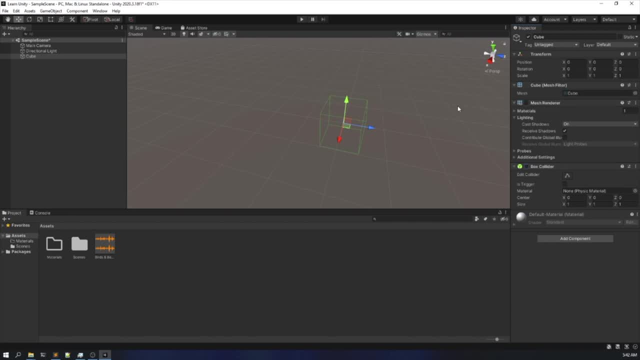 you. you would see the very light green, right, very light green. now these other light greens are this, this of cube mesh filters. but this box, collider lines are also getting attached to it. now here is the mesh. render mission is basically the mesh of the cube, nothing else. all right. so 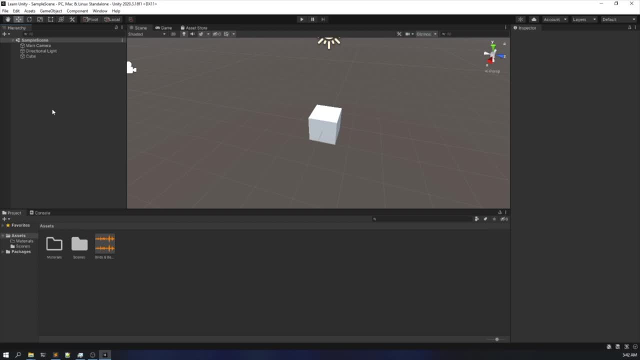 till now, we have learned manipulating our cube. we have learned, uh uh, navigate our interfaces. all right, we have learned about game objects, right? so yeah, we have learned this much by now. now let's talk about materials. what are materials? see, of course you want, uh, your like game objects to be colorful, right, you want your game objects to be. 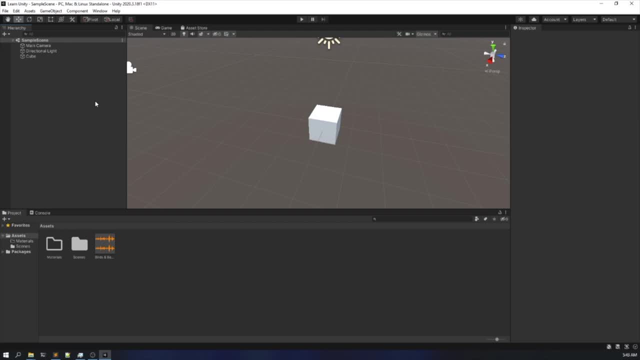 like texturified, like they should have some sort of skin. even humans does have skin. why won't a game object that's like that's really bad right. so our game objects also wants materials like just humans. we want our skin. similarly, the game objects also want. 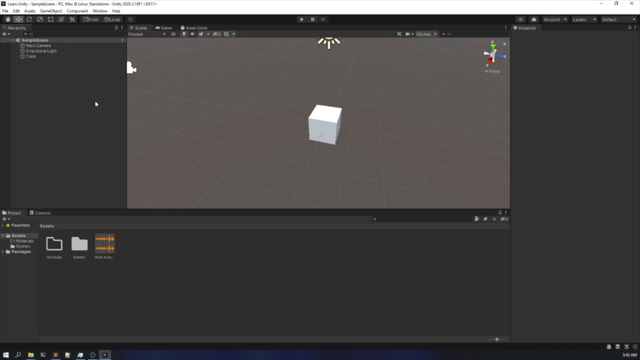 their skin. so the skin is known as materials in this terminology, in technical terminology. all right, so just just as you can see, I previously created a folder right. go to that folder right click, click on create. find the material I found it in here. click on it. let's name it. I want to. 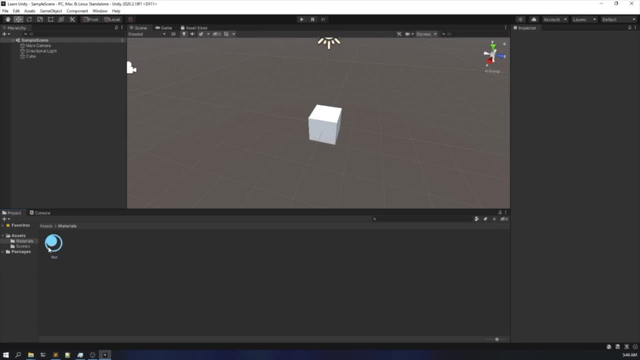 name it red. right, I want my material to be red now. what now? what now? I want to change the color. all right, see, simply click on this material and here you can see that you are the properties of those one. that material is available in this vector now. after that, click on this white box. all right, this. 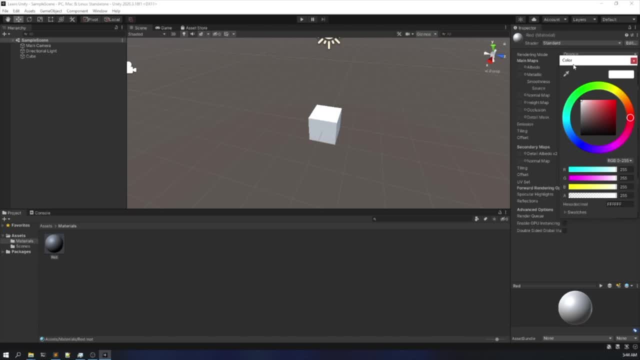 is us at the right of albedo. click on this, all right, and select a color, let's say. let's say I want it to be red, yeah, so that's sort of a bit pink also, but well, that would work for me. so now let's say it's not green. get rid of the color of this material, man. I have like I. 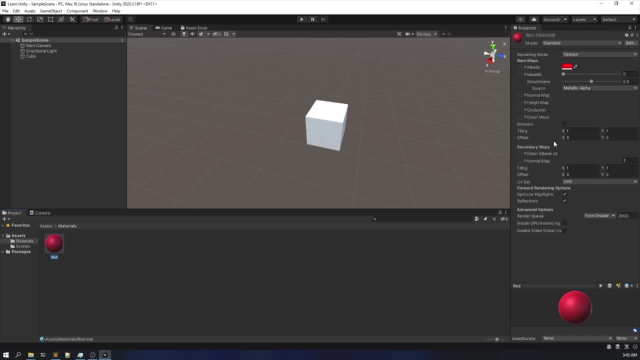 have edited the color. I have put, put something color in it, but why isn't it reflecting in the cube? why isn't it showing on the queue the cube angry, that with the color there's a cube angry? no, it is not. of course not. so we. we have to. 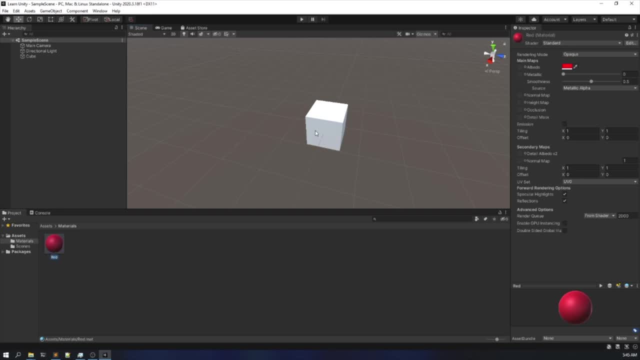 apply this material in the cube. right, we have to apply it. so how would you do? two simple ways: click on this q circle, click on this cube, drag and drop this material inside its inspector. voila, you got the material. now our cube is happy, just like us humans. the cube has also got its skin. another way is just drag. 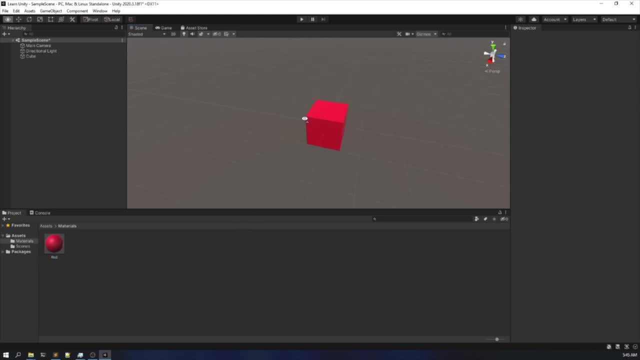 uh, drag this and put, drop it in the scene view without also using the inspector. this can also be done, right? so our cube is now really happy because we have provided him a skill, right voila. so now we learned about materials. now one more thing. if you want to add textures, it is really 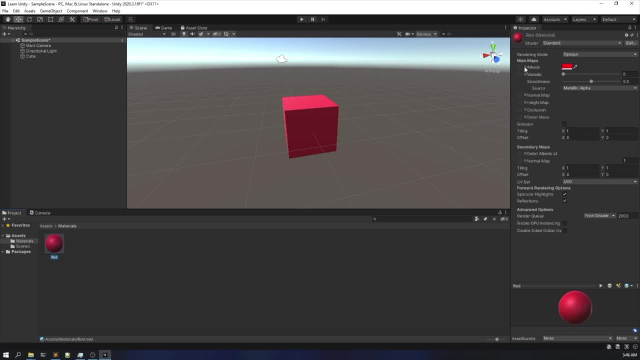 easy click on this, like albedo. here, you are seeing a blank box and after that there's a zero sort of click on this. all right, now let's say what, what sort of material i want i want. all right, let's see, um, and no, no, not not this, not this, of course, not this. uh, let's say this: yeah, this, this looks. 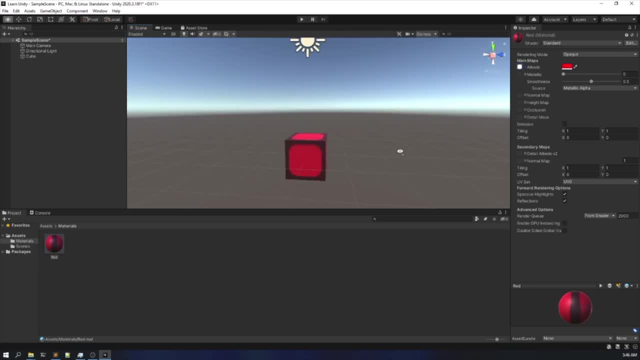 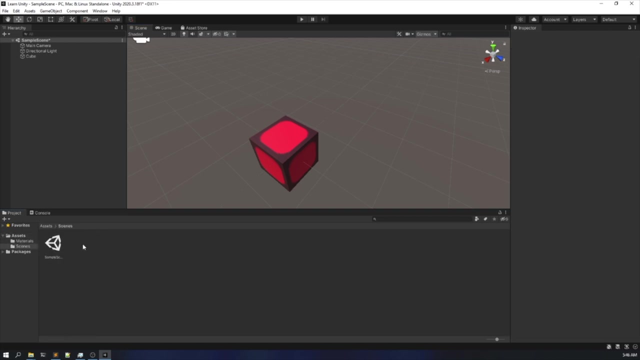 a bit, a bit good, right? so, yeah, we gave our cube a texture also. see, now our cube is more than happy. so we successfully made our cube happy and also learned about materials and texturing. find those all right. now, how to create a scene- all right, see what are scenes? scenes are nothing but. 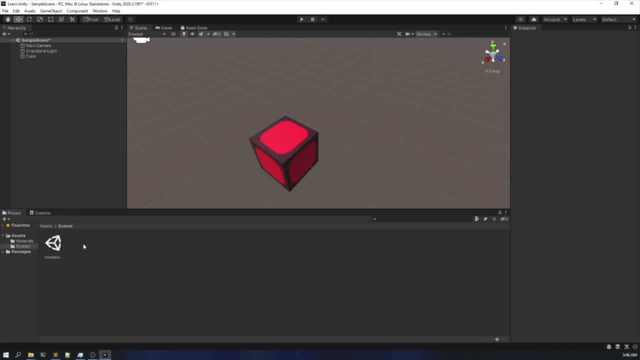 different environments. right, they are different environments like. this is a sample scene. i want to name it. let's say, i want to name it where? where is the rename? yeah, i want to name it a main scene. all right, main scene. this is the scene i want to name. 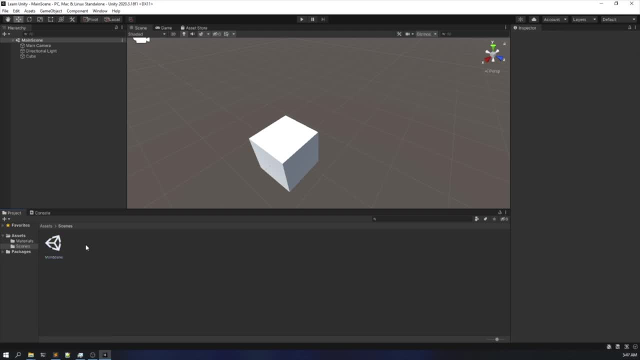 right, this is my main scene, so this is a scene, all right. and where did the material go? that's weird. first, i guess this is the bug of unity, but this is really weird. i guess it happened because i didn't saved it. i'm not sure, but yeah, but we managed to get it back. 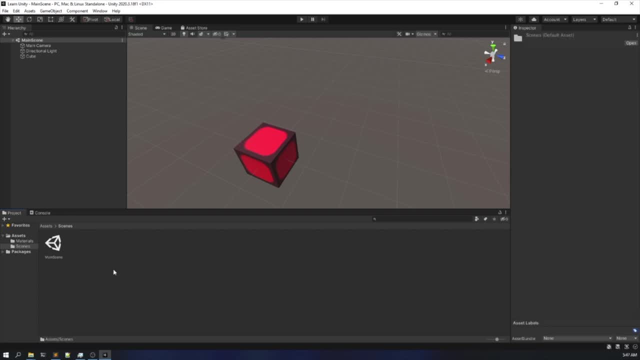 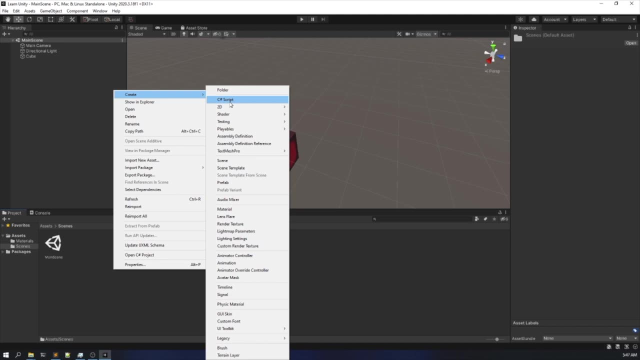 now scene is at a separate environment so that we can create another scene. all right, i would also like uh while uh getting into v4. yeah, i will be. i will also be showing how to navigate through different scenes. all right, so don't worry about anything. how to navigate and. 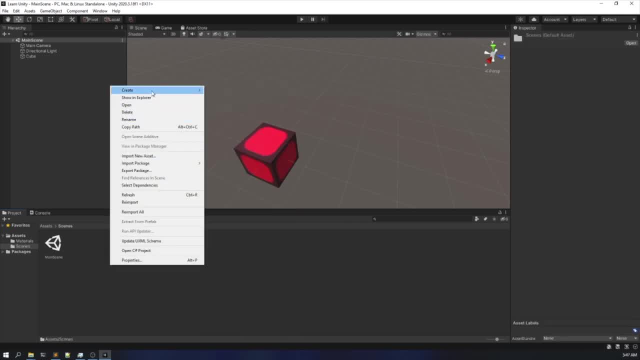 all those things. so i just want i just have to click right, then create. then here's our the scene. man, oh yeah, got this scene now. and to create a new scene, that is test scene. see, i got another scene with, uh, main camera and directional light by default. all right, but 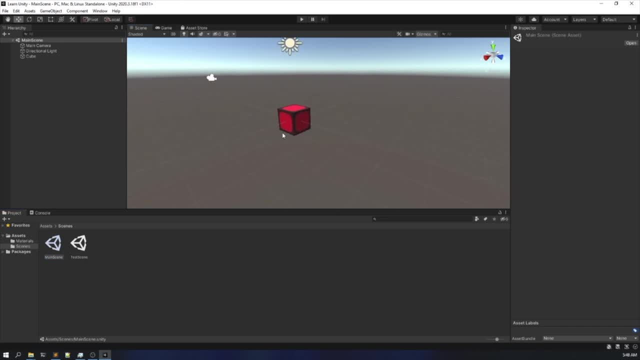 currently, i want to be in the main scene, right so so we successfully created our queue and also managed to make it happy by giving it a skin. now let's learn a bit- uh, a bit, about project structure, right? what is a project structure? what is it? a project structure is a way of structuring. 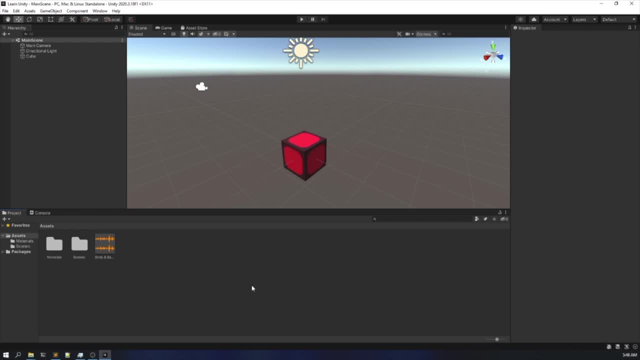 your project, all right, nothing else. see why. uh see, this is not something like many people teaches you all right, this, this, uh, this thing you gain by. you gain by experience. but today i'll be teaching you, all right, see, maintaining your project on it. maintaining your project is: 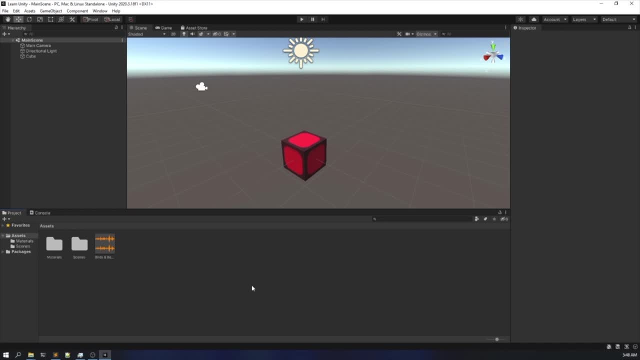 really important, like when i was a beginner even. uh, i remember when i was a beginner i i used to like make my whole project very much cluttered, right, i used to make everything cluttered out and that actually caused a real problem for me. like later on, all right, because 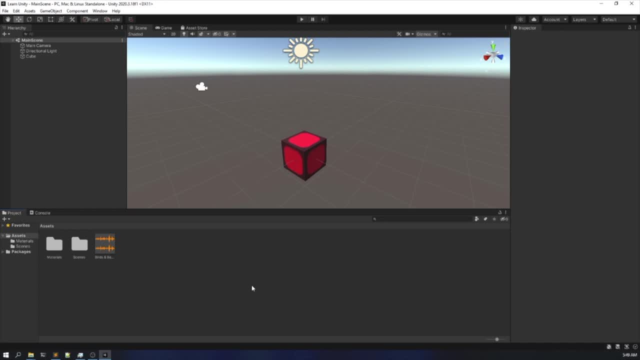 managing those were really like hectic. so with after like, after working with unity, i learned that, uh, it is really important to manage your project. so how do i manage? i create separate folders, all right, for separate type of file, all right. like for materials, like for skins, i created this. 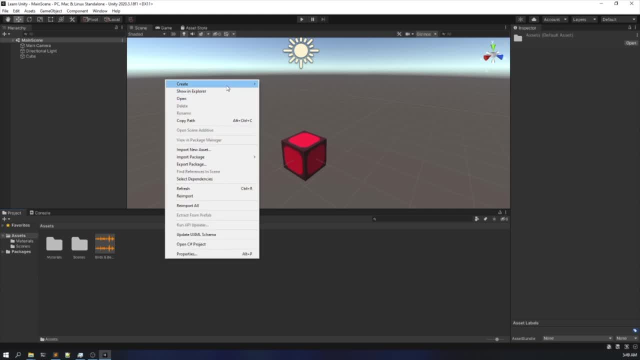 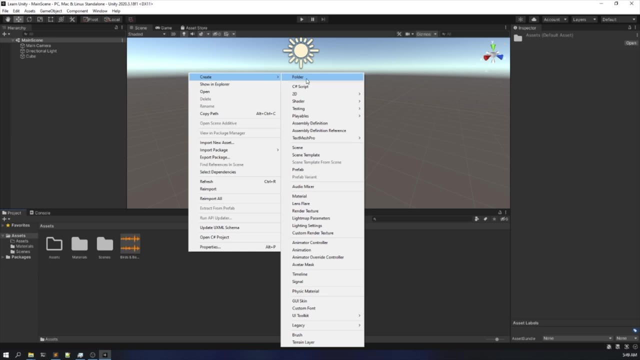 particular uh folder named materials. all right to add some sort of assets. all right, some sort of assets. i would name another folder named assets where i'll be storing my assets, like 3d model, like 3d images. right like to store audio. i'd be creating another folder that is audio folder. 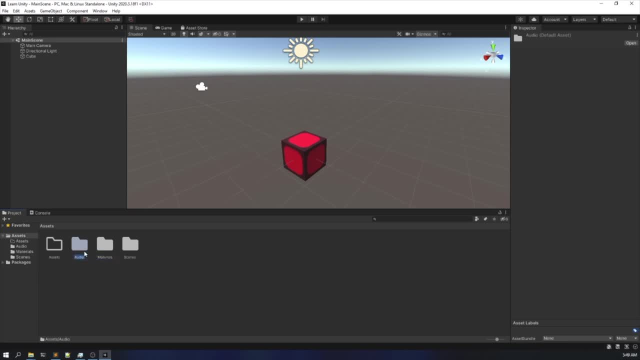 all right, so i create separate types of folders, like i create a file where i will store all my assets. all right, so i create separate types of folders and, as you'll see, all right, so there's that's types of folders. all right for separate types of files, right? so similarly, throughout this video. 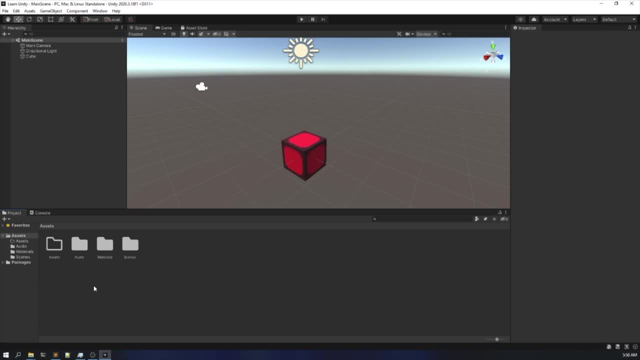 would be saying: how am i creating folder for each type of file, right? so i recommend to stay along with the video till the end, right? so till now we have learned about navigating through our interface. about game objects, about manipulating those, all right. about materials, all right, like. 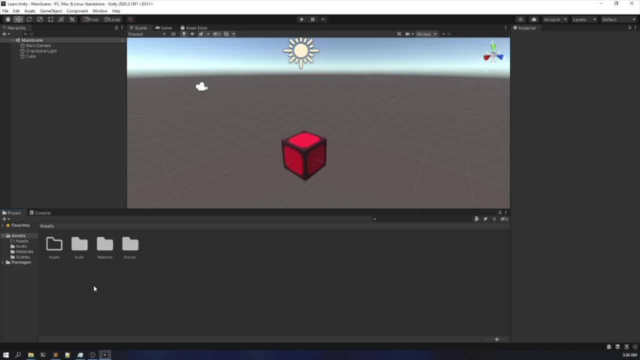 the skins. then we have learned about the scenes. what are scenes right? uh, then we have learned about our project structure. isn't it cool? like within a half an hour, we have done so much. so, yeah, so we learned about structuring our project. all right. now some more parts are left. 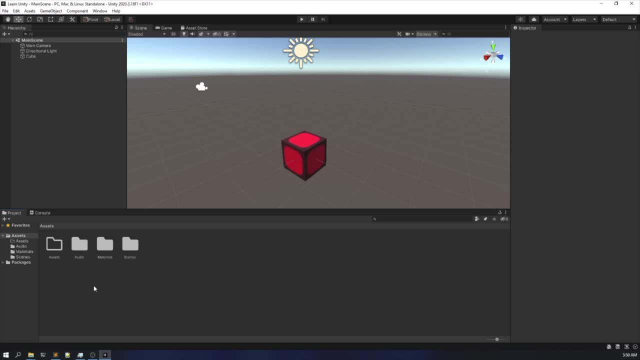 like creating our own c-sharp script. all right, then we will be learning to modify our own components, then prefabs, uh, then physics and collision, then we will be learning about audio and then, at last, we wrap up this module after designing our interfaces, all right, so, yeah, let's, let's do it, let's get the energy back and let's do it so to to keep the scripts. 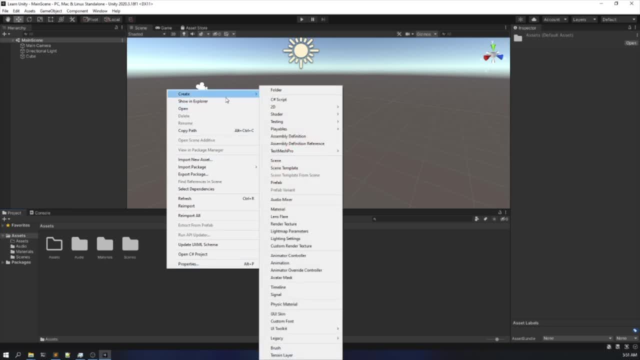 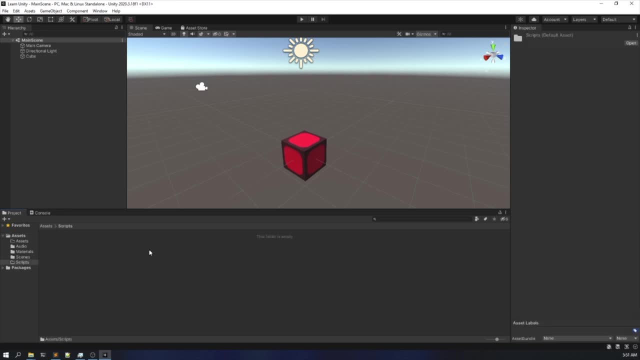 all right, to keep the scripts. uh, what i want to do? i want to create another folder, name scripts folder. all right, it would be containing all the scripts in here. just then, right click, click, click, shisha. all right, i want to name it a test script. all right, now, as you can see in here, there's a like a buffering going on. this buffering is: 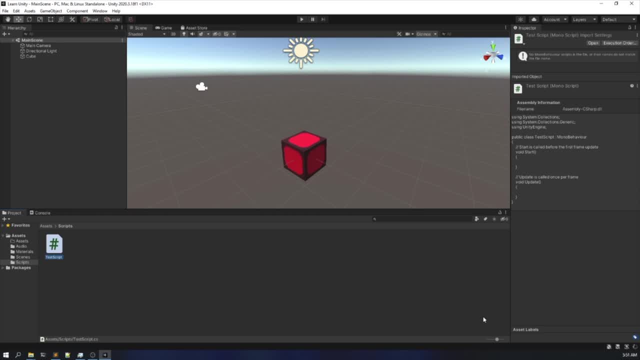 basically, uh, the shows that, uh, our script is getting compiled right, so just wait for a few seconds and it would be done. actually, my system, like my system, has got really slow and because of that it's taking a lot of time, but i guess we can manage with that, right. 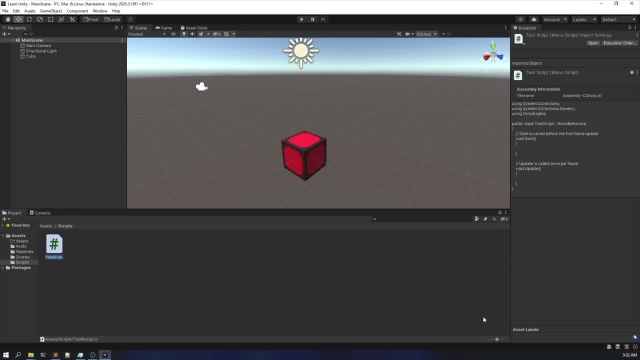 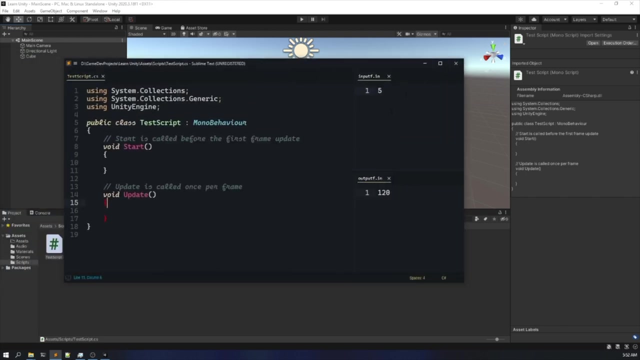 so yeah, voila, our test script is created. now i would be using my own text editor. all right, i'm dragging and dropped it into the one. um, just wait, just just, uh, just wait, uh. so yeah, now let me drag and drop it in here. all right, now? see, don't look. 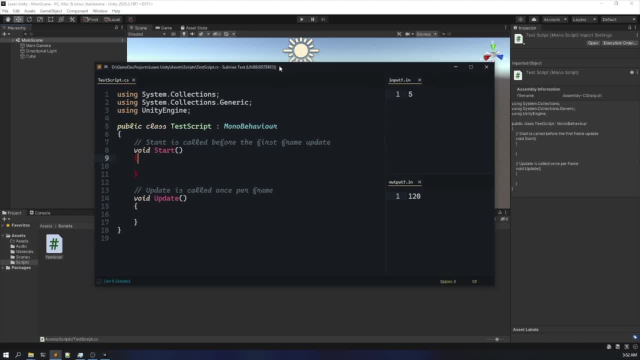 into these windows, all right? um, i have set up my sublime text for competitive programming, so don't look into this, but let's understand. what are these? all right, see if? uh, don't worry, i'll be explaining all these things. all right, what is like public class? what is like what is void then what is using? 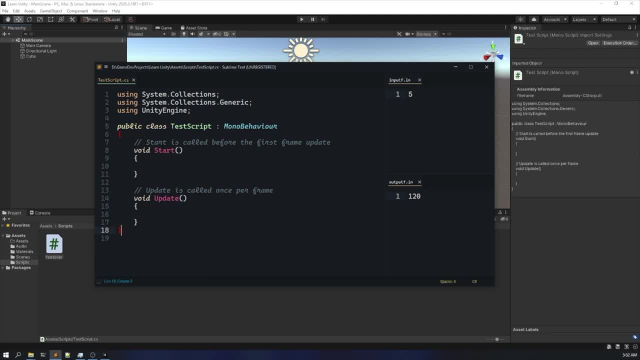 so i'll be under, make you understand all these things, all right. if you don't understand something in here, don't worry, i am there for you. all right, i am your instructor. i am always there for you. if you have any doubt, join our community. all right, join our community. ask your doubts in there. you. 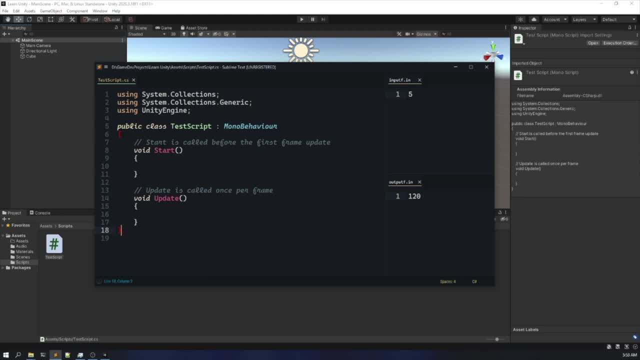 would. i promise you would get instant doubt support in there. all right, so yeah, as you can see in here. all right, just wait, let me uh make the font a bit bigger. yeah, so first of all, we are uh including all these system packages like unity packages, all right, 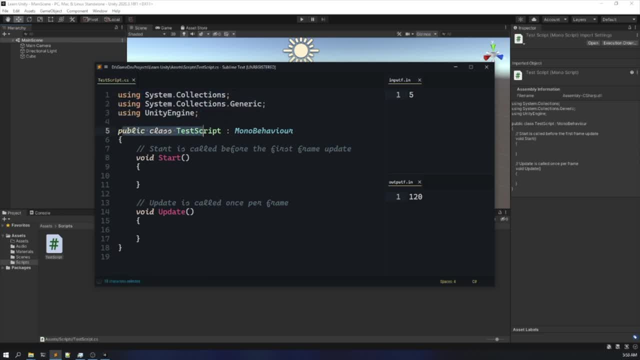 these are packages we are including. now we have created a class of transcript. all right, that is inheriting another class. all right, that is mono behavior class. all right, there's the mono behavior class. now, inside that mono behavior class, see, remember, this mono behavior class consists of: 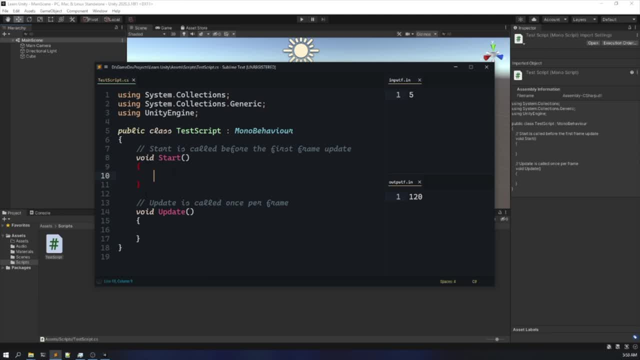 these functions, all right. so it is important to inherit this mono behavior class now. if you don't understand what inheritance is, don't worry, i am there now. this is uh with the void uh start function. this is the update function. what happens in start is so the first time? all right, the first time i'm playing. 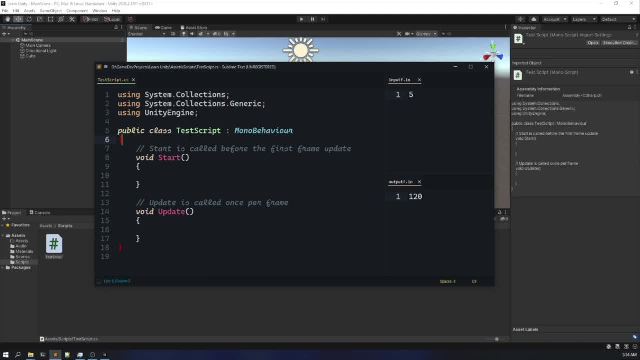 my unity, like playing, uh, the particular scene. all right, it will show at first, like the first frame. it will do some function that i will define. all right, and what the update does is what it does. it basically updates, uh, every frame, like it will do that function. it will do that. 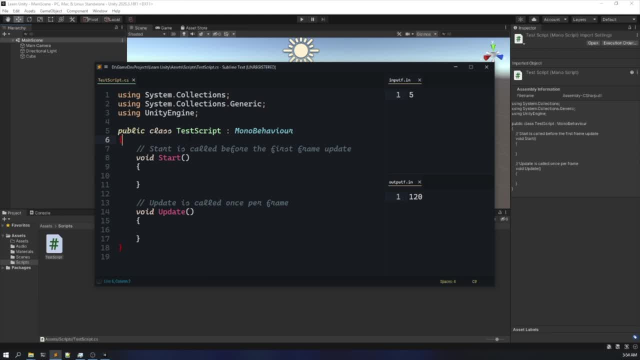 particular function in each and every frame, all right, and it will be called once, like if, if it the frame is one, uh, the update function will be called once the frame is two, again one. so yeah, so update function is called once. now, let's, let's try it out, right, try it out so. 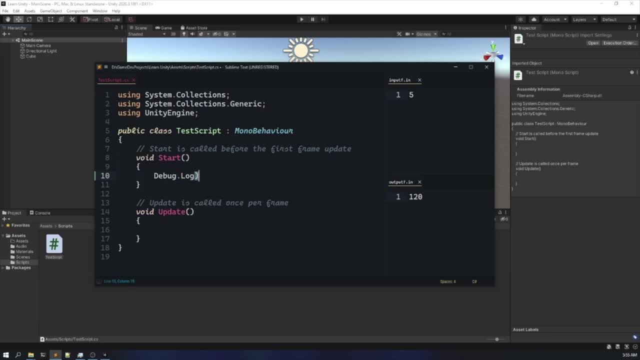 to uh print something. i'll try to print something that has to print something in like unity or like in the console. we do debuglog and let's name it, start function right and also remember to put the semicolon. i all i sometimes forget and this gives us right. 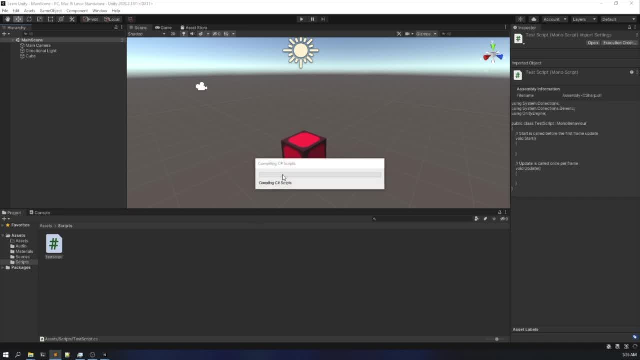 right, so it's compiling the script. all right, just just wait for it. all right, it will. it will compile the script and then we are good to go. i will also show you how to execute a script. all right, um, just just to wait. uh yeah, we are good to go, right, so, yeah, now let's play. all right, how to. 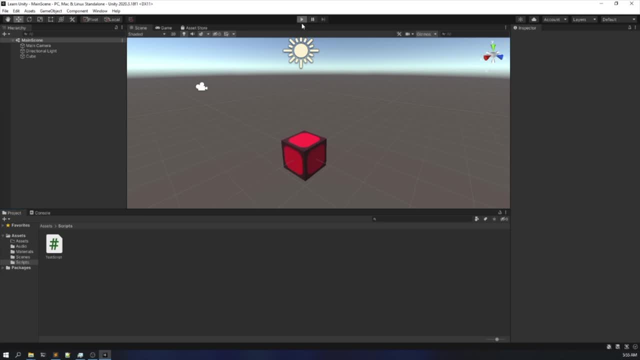 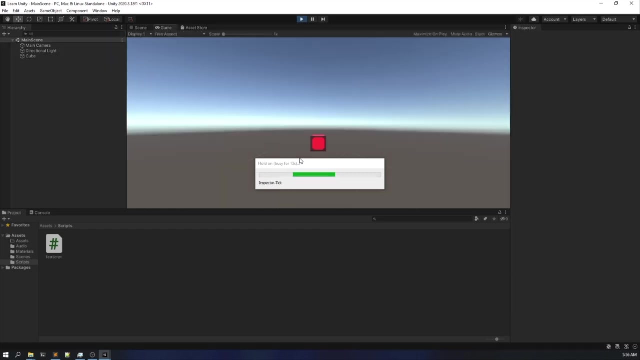 play. click on this play button. all right, just wait, this would take some time, all right? uh, all right, it is telling us to hold on and we will hold on. like unity is really good. it notifies us everything. so, yeah, as you can see, we have got into our games in and started playing it. let's go to. 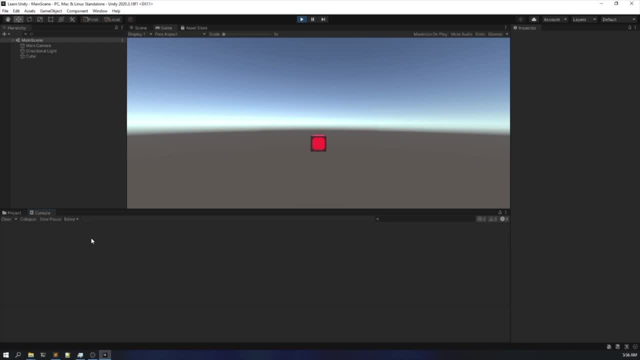 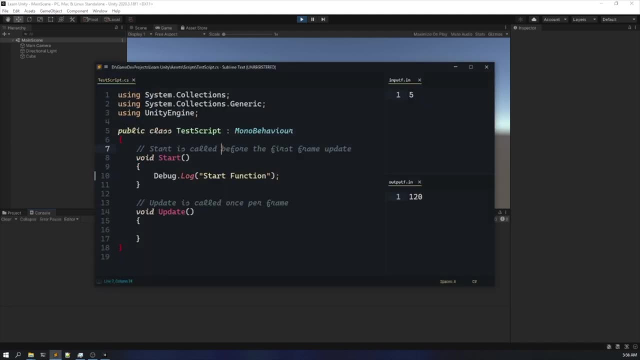 the console. oh my god, why isn't it printing? have i, have i done something wrong, like, have i coded something wrong? let's check the script again. no, nothing is wrong in here. i guess everything is okay. yeah, it looks good to me. but why didn't it actually work? let me show you. so i got out of. 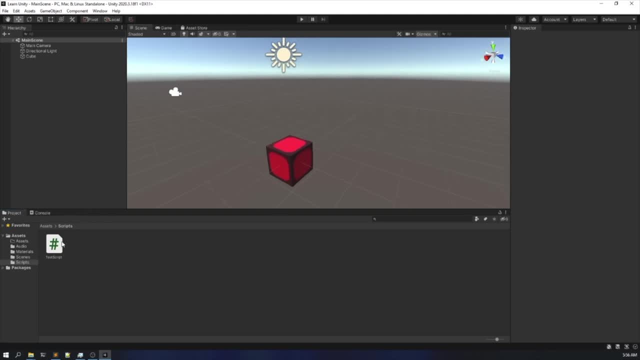 my play screen. all right, go to the scene. yeah, see, the script is in here. all right, it is in here in the project, but we haven't executed it right. we haven't executed it. so how to execute? pick an object: all right, i want this cube object. then just drag and drop the script. all right, drag and drop in it. 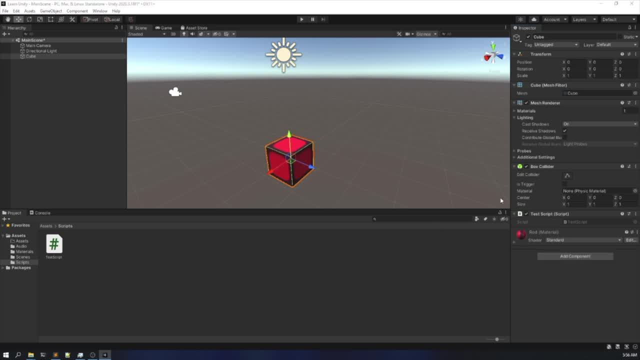 there's another option, all right, that is click on add component. all right, and type the script name. all right, like test script. so here you got the test script right. so similarly, there are two ways to add on. you can also drag and drop in here also, all right, that's another option. now another got. 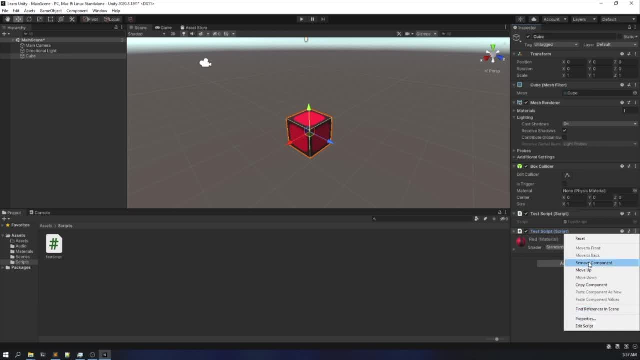 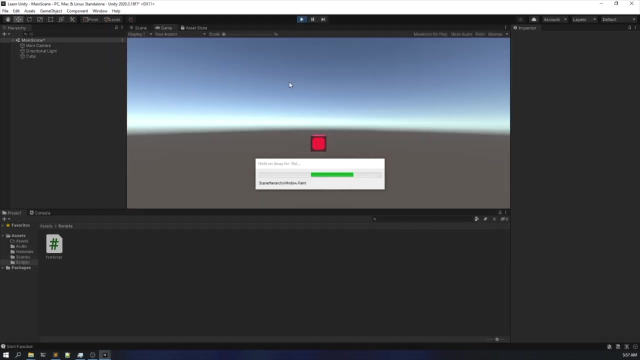 added here, but i don't want it, so i will remove it. all right. so let's play it now. let's try playing it now. just wait, hold on. our unity is telling us to hold on. it is entering the play mode, so now let's see what has happened in our console. cool, now you can see in the console. 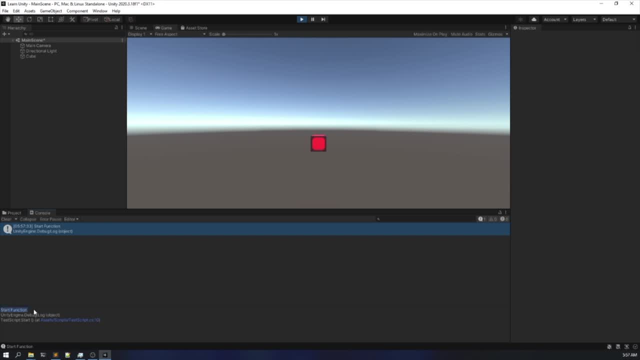 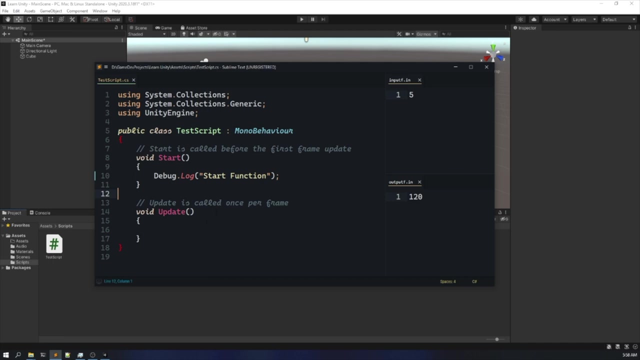 there are different changes on the actual console. let's see what is happening in the console. right is something written. it is written: start function. that's what we wrote in the debuglog. right, that's what we wrote. so what happens? the start function works in first frame right now. this is the update. 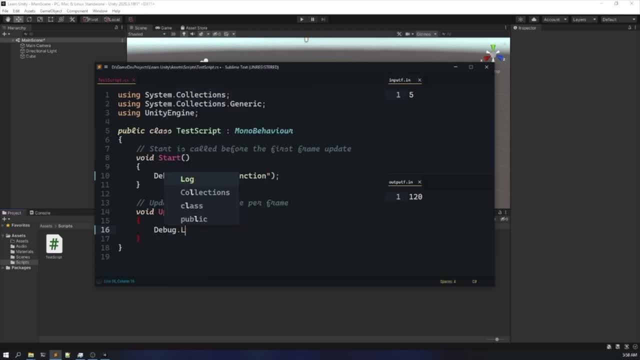 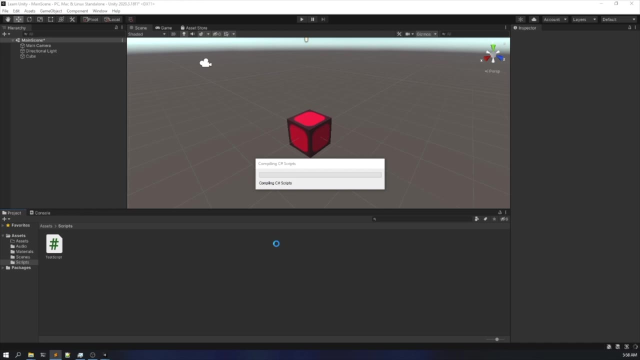 function. all right. now we want to check the update function too, right, just wait. right, so yeah, so i have saved it. it will take some time to compile it. let it do its compilation. we won't bother him. all right, unit is good. it does everything for us, all right, so let's- uh, let's- hold on it's. 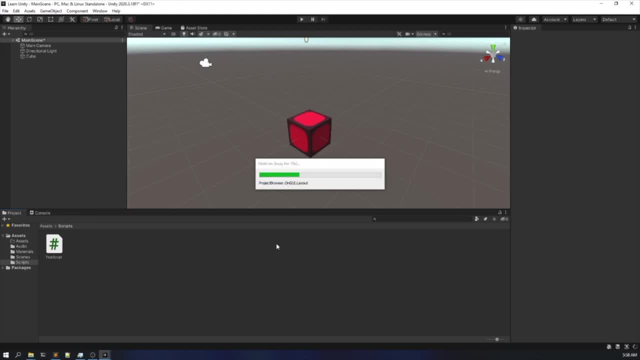 just wait, it will take some time to compile it. all right, so let's save it. all right, so let's take some time. oh cool, so it got uh like compiled and let's play it. let's see what happens. just wait, uh, now let's. are you ready to see the console window? 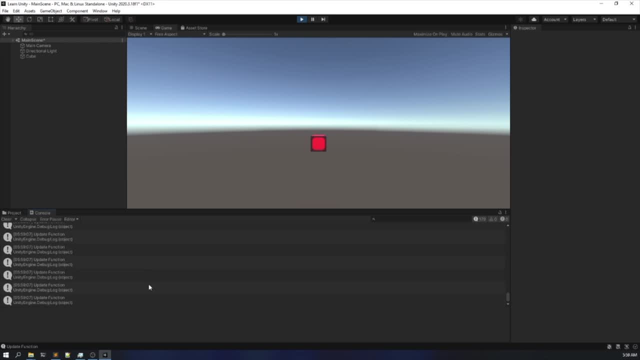 are you ready to see the console window? are you guys ready? let's see it. oh my god, what's it doing? it's continuously like putting giving the function update function like each frame. it is doing this on each frame. see, it continuously updates the function in each frame. so actually i think you got a very basic idea of what this 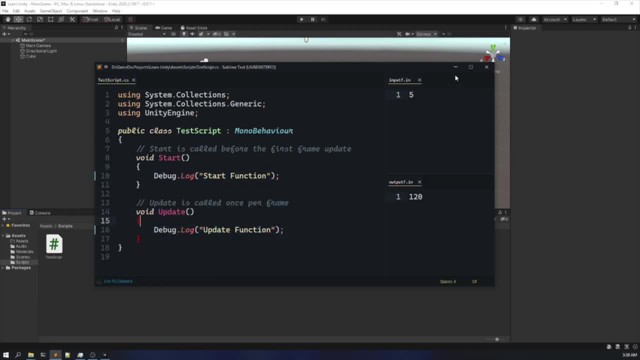 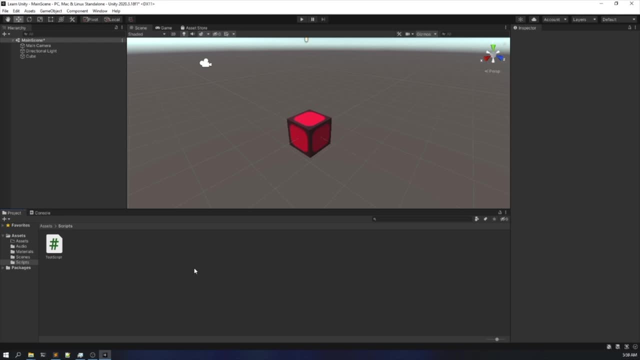 this function is doing right. i guess you got that very basic idea, so for now, uh, this is the like. you learned how to uh basically learn unity- sorry, i'm not the only teaching unity. basically, you learned how to uh create your own script, all right, and understood the functions in. 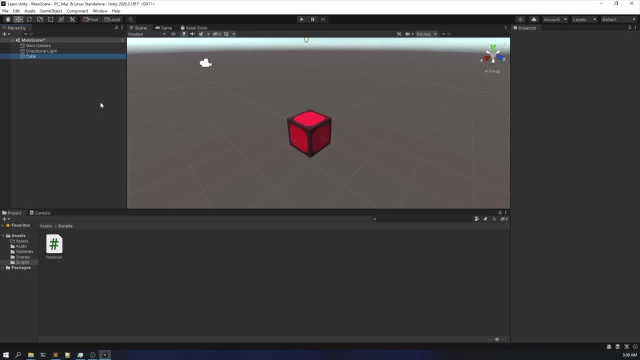 there, all right. now there's another section known as modifying components. we already learned how to modify components, all right, so yeah, now here comes prefabs. what are prefabs? prefabs? you can do this, can say: these are the collections. all right, these are collection. let me create another folder. i will. 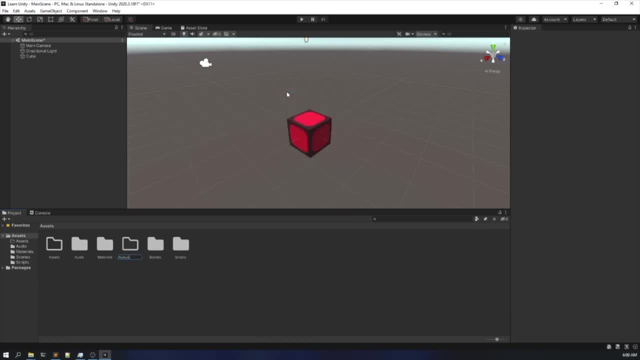 also show you how to create a prefab. so what is a prefab man? a prefab basically helps us to create a collection, right like it. it is sort of a storage particular thing, right see? uh, let's say right now, let's, let's take a scenario, all right. let's take a scenario, you are developing a game, all right. 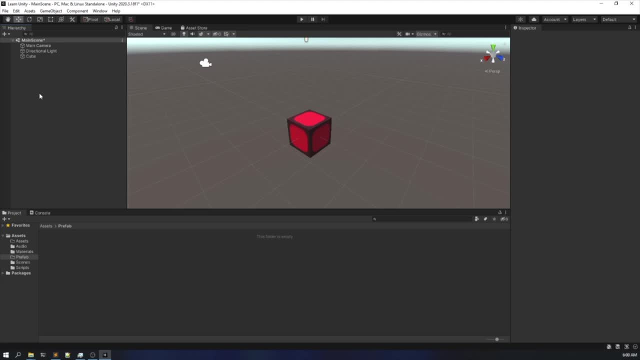 so that's a first person shooter game. all right. you have implemented it, uh, on one scene, all right. now you have created your own first level. now you want to go to a second level and you want that same particular fps player- all right, same particular fps player in this, in another scene. 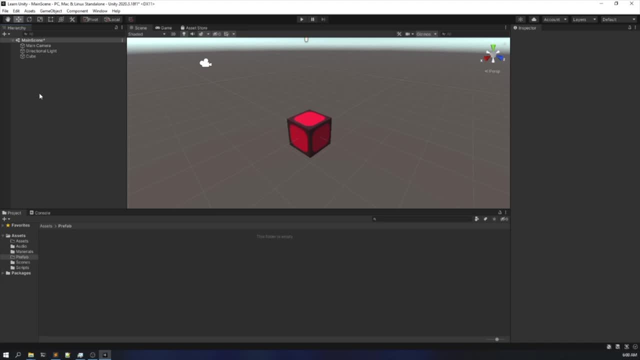 that you are going to create. that is, in another level, what you would do. you have one way, all right. one way is to like create, like assemble all the components that you made previously. again, all right, and that would consume your time, all right, and of course, that isn't a. 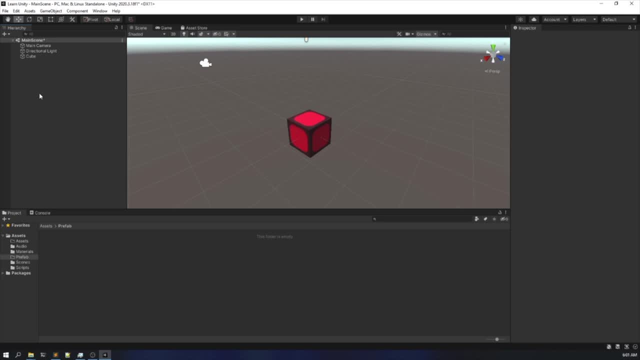 good thing. another way is to create a prefab, so prefab creates an another, like a package of that particular object. right, it's, it's a package of that particular object. it helps to create a like a package, like: if i, a cube, has certain properties, all right, i need the same cube on this. 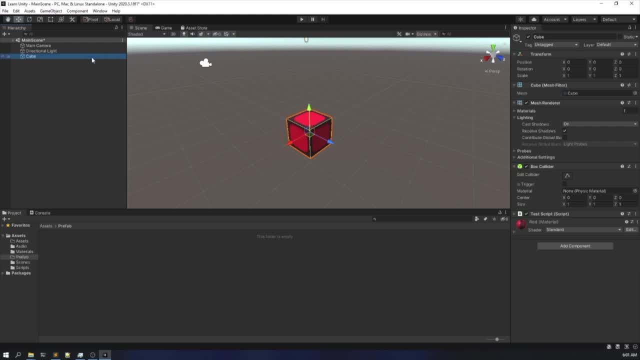 next, next scene. right, i need the same cube on the next scene. then one way is to recreate it. another way is to create a prefab and just use that prefab. now how to create a prefab: click on this cube, all right, click on this cube, drag it and bring it in this project section. 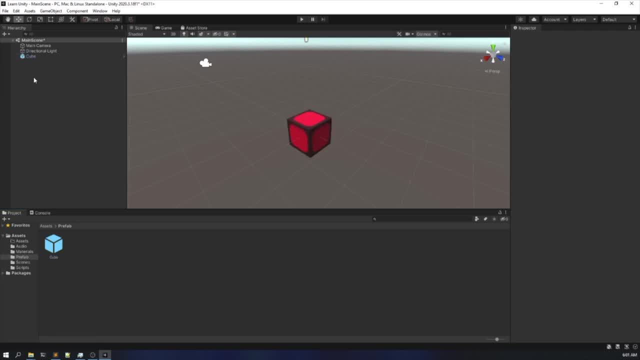 put it in there and voila, your prefab is created. now here you can see, the cube has turned like this. this thing has turned blue. this is the indication that it is a prefab. now let's create another scene and let's see. does it does? uh, oh, i, i have already won. does this work on this? on this, another scene. 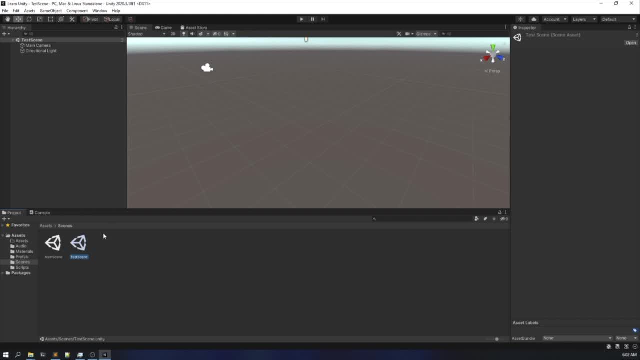 i want to save it. right, i definitely want to save it. uh. so yeah, let's go to this. uh, where is it prefab? all right, now let's drag and drop it in here. wow, i got it in here. just reset the transform. yeah, i got it in here. let's, let's try playing it. let's say the functionality works or not. 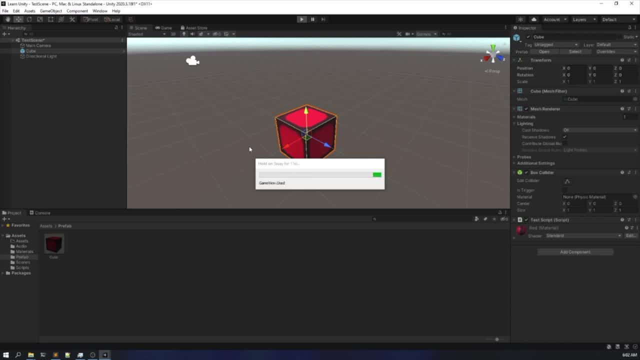 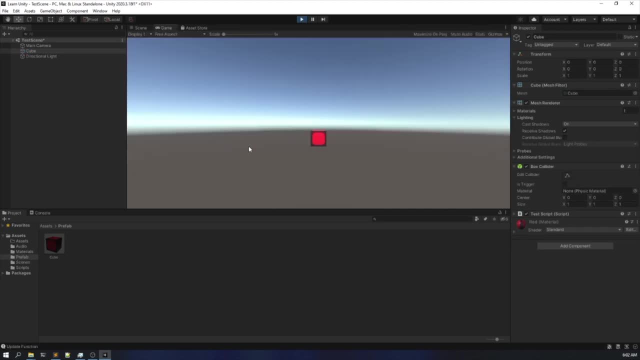 just wait for a few seconds to run. um, it is doing its job. uh, so yeah, now let's look at in the console. wow, the same thing that was working on the previous scene is the same thing is working in here. so yeah, one more thing i forgot to tell you. i just okay, it just came up in my mind. 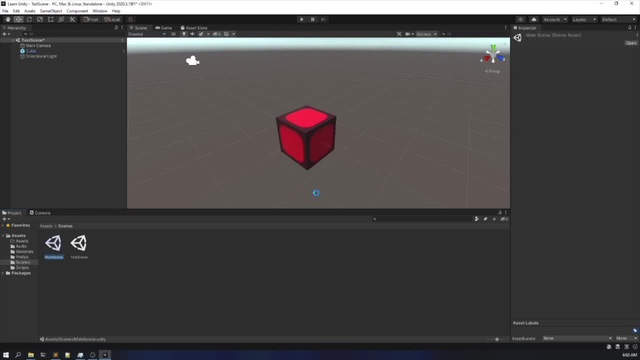 just all, let me like go back to my main scene. uh, wait, let me lower down the desktop volume. yeah, so now? so now, what? all right, so what? now? it's uh what we have to do. uh see, now i would be telling you something really important. all right, uh, i forgot to say that. 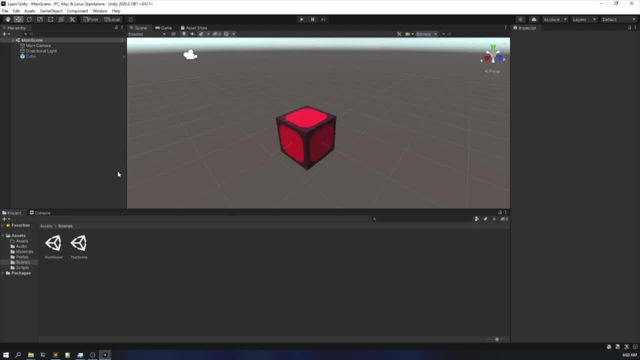 I forgot to tell you that previously an object all right. an object can have its child object, all right, like you can branch the objects like if I, if I want to want the cube to be a child of main camera, I would just click on the cube, drag and drop it in here and see, my cube is now the. 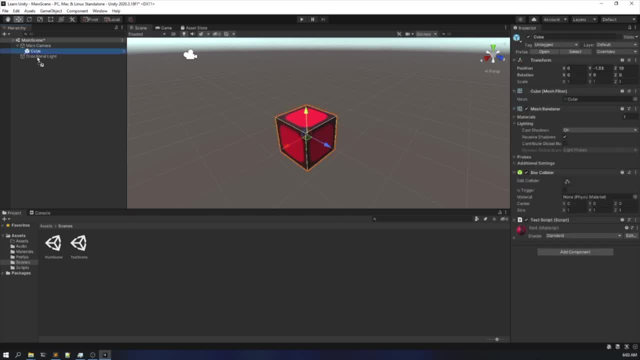 child of the main camera. right and main camera is the parent. similarly, I can also create empty, empty objects. that is, click on create and create empty. all right, I won't change its name, I will just reset its transform and put this cube underneath of that game object. all right now. 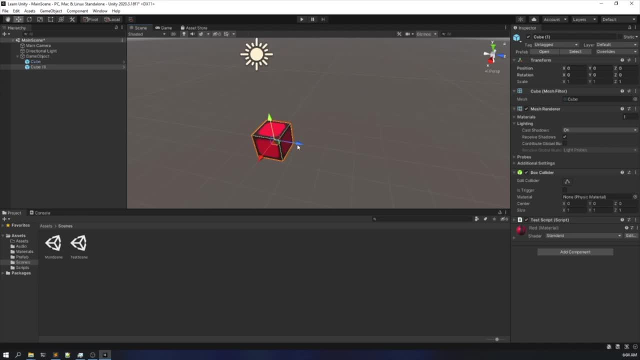 I can make multiple childs of this cube. all right, I just ctrl d. all right to duplicate ctrl d. so, yeah, again ctrl d, again ctrl d. so similarly, like this, I am able to like: oh wait, yeah, I'm able to create multiple child objects inside another empty game object. right, so you can do those things. similarly, nothing much different. 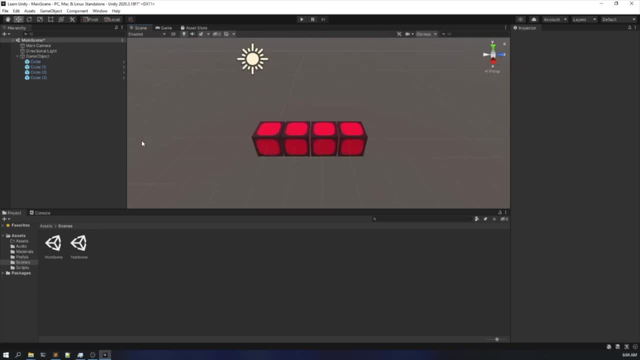 right. so till now we have learned a lot of things. all right. we have learned also modifying our own components. we have learned about prefab. now three more important sections are left. that is, physics and collision. all right, physics and collision. another one is audio: how to work with. 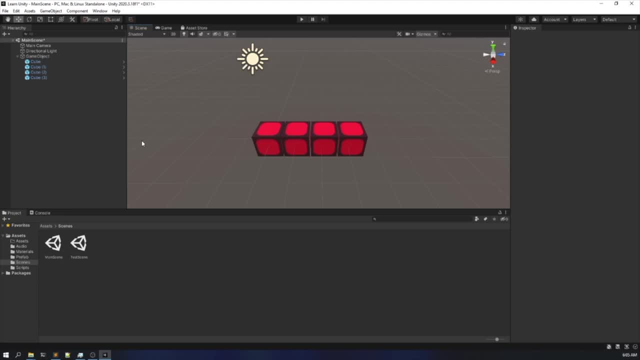 audio files. all right, audio is really simple. all right. then we have the last but not the least: designing our interfaces. all right, and at last of that, I would also be showing you another thing, all right. so yeah, let's move on with the next section. so, let's move on with the next section. 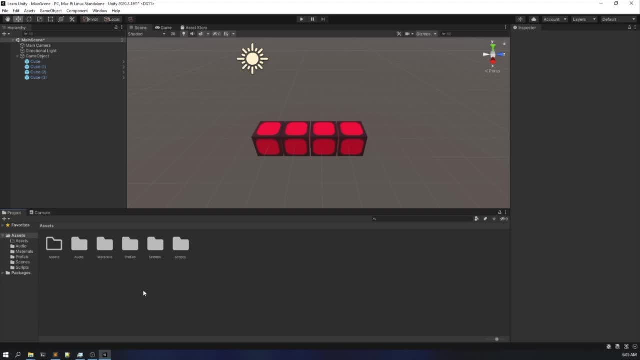 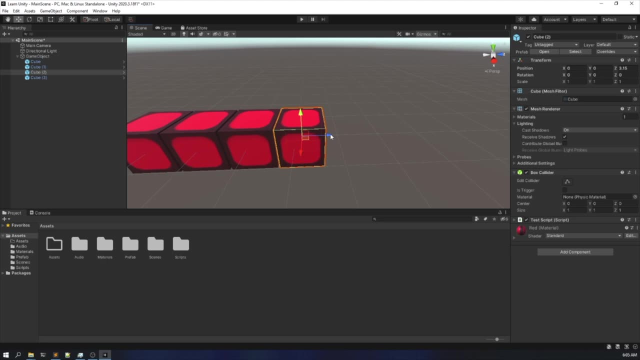 physics and collision. what is a collision man? what is it? see, collision is nothing. all right. collision is nothing but the hit, or like the hit, of an object for on another object, all right. it is like see these two objects are colliding with each other. all right, these two objects are colliding. 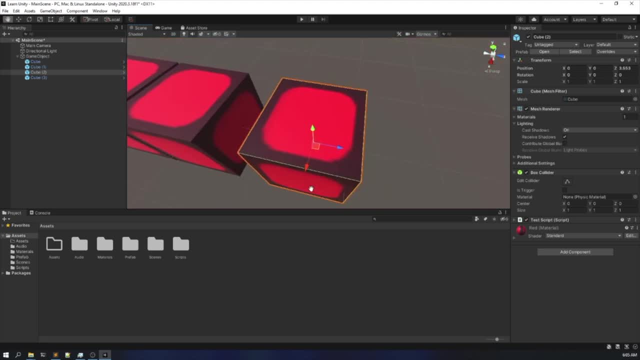 collision is basically the like, interfering of two object with one another, right? so? so that's what collision is all right. now, if I, if I had to say: you all right. game like this, this whole unity engine is a replica of our real world physics. I will be showing you how. all right, just just wait. 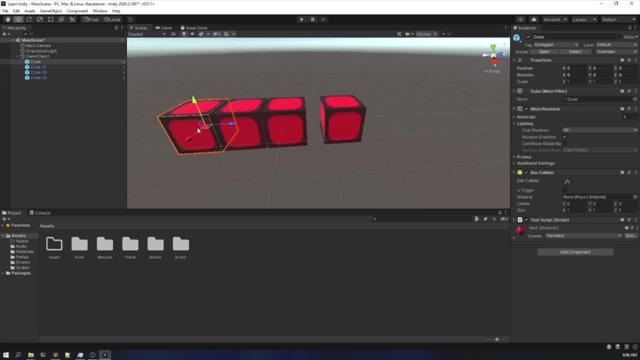 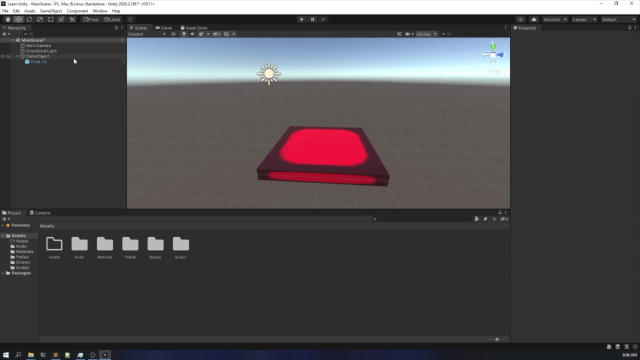 all right. first of all, I would be deleting all those other game objects. just wait, uh. first I need to uh set up my environment to show you how right uh, oh, no, no, y let b, let y be 0.4, right, and the z be 4 or 1 b, 4, right. so this is how it is all, right now. 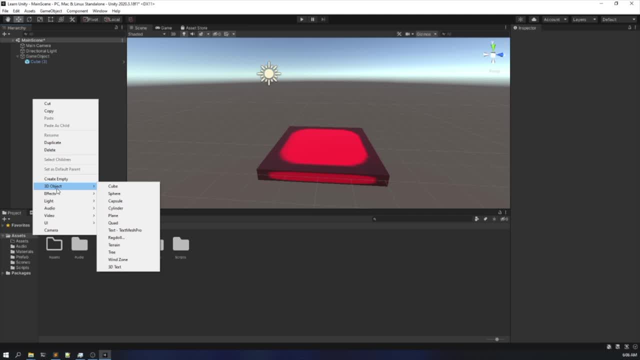 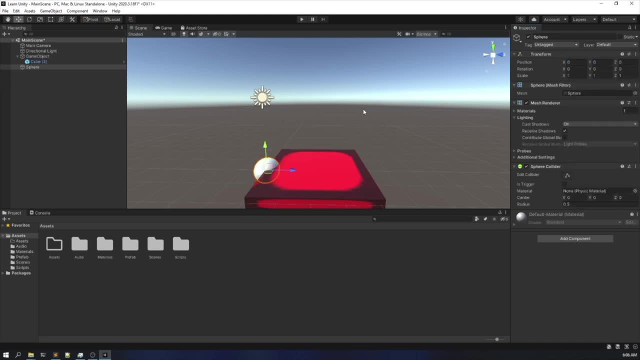 let's take another 3d object, that is a spear. we would call it a ball right. it is a ball for, uh, for us it is a ball right, just wait. so, so yeah, this is a ball right. now I want to implement a real world physics. 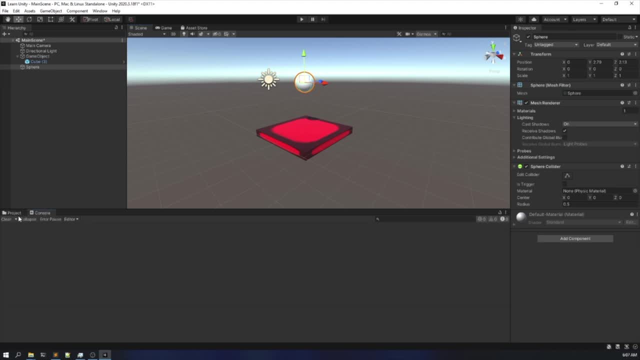 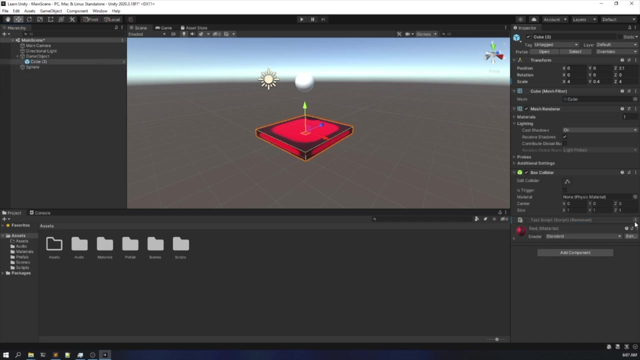 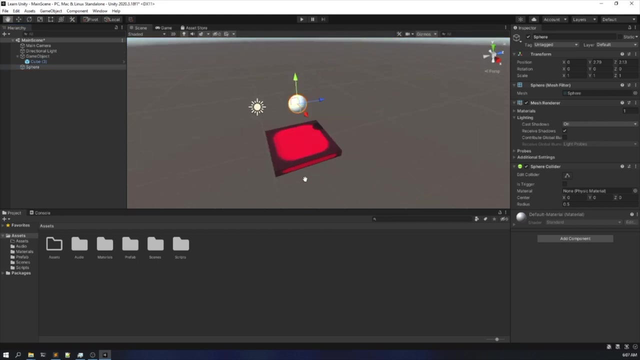 so as of now, all right, let me, let me first, uh, de-attach the script. all right now, or else it would be working continuously. I don't want the script to be interfere, to interfere, all right, just wait. oh, let me apply to a prefab. so our 3d, uh, our script has been removed. all right, like here. one thing: 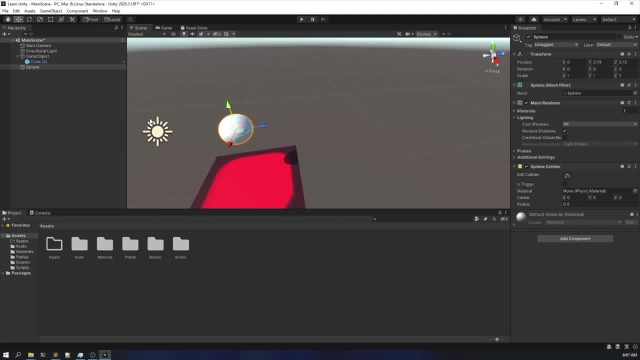 you can see of it. here's a shadow. that's because of the lightning. all right, you can play with the light lighting later, all right, so let's play it now. so in real world, what happens in real world? if we have a plane and if we throw a ball from the top of the plane, it will play a. 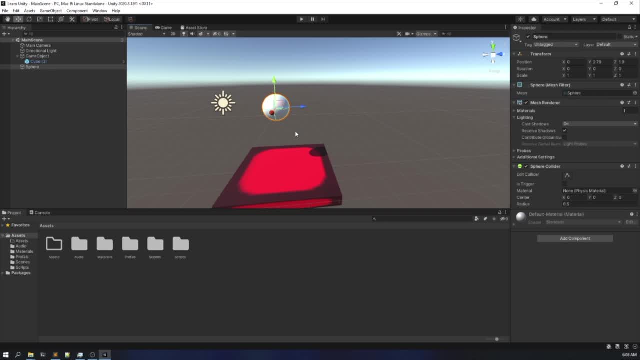 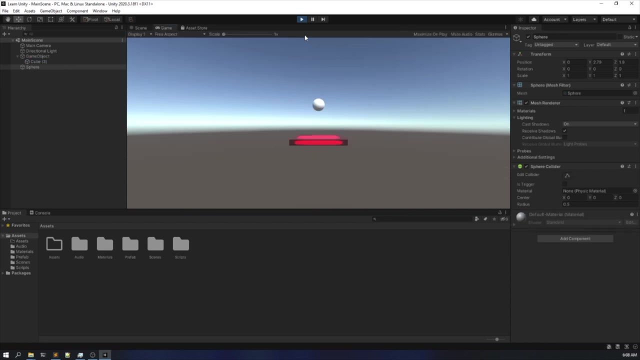 ball for us. what happens in real world if we have a plane and if we throw a ball for us, what happens? that from the top, it will fall down. right, it will fall down and bounce. let's check that it happens in here or not. just wait. keep patience, alright, keep patience. oh my god, why isn't it falling? 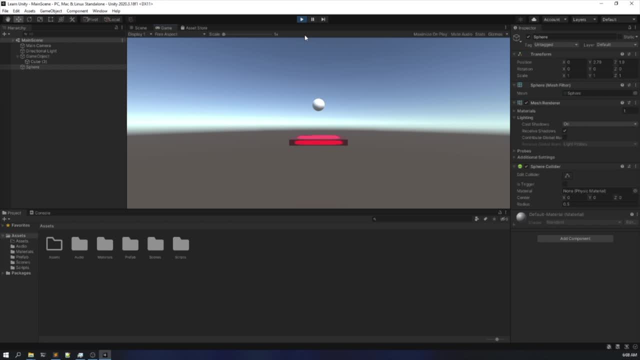 it should fall right. it should because I recently told that unit engine is a replica of our real-world physics. but you have to implement those physics right. you have to implement those. how. how would we implement those? unity is really really caring about us, and what unity developers did they already? 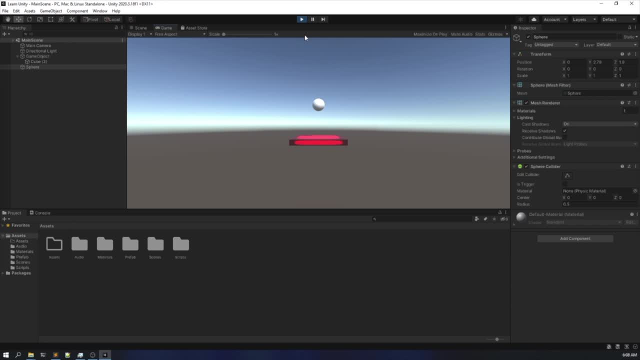 created those physics objects for us, those physics components that will help us replicate the real-world situation. all right, now, how do we do that? so see, we are. first of all, we are in the game scene. all right, we are in the game scene. I'd be editing this whole thing while. 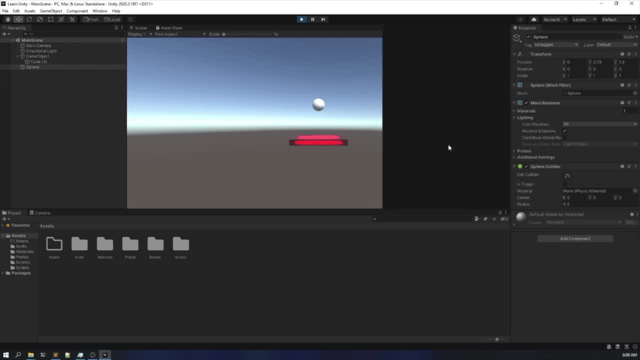 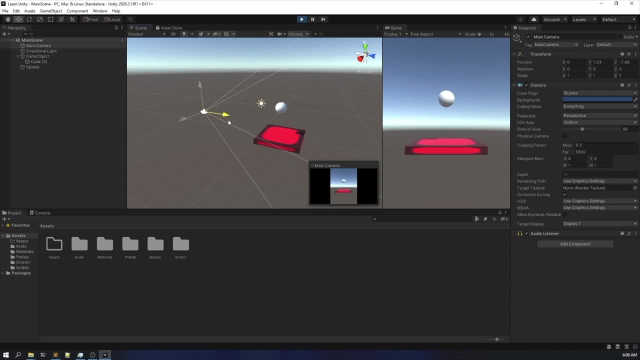 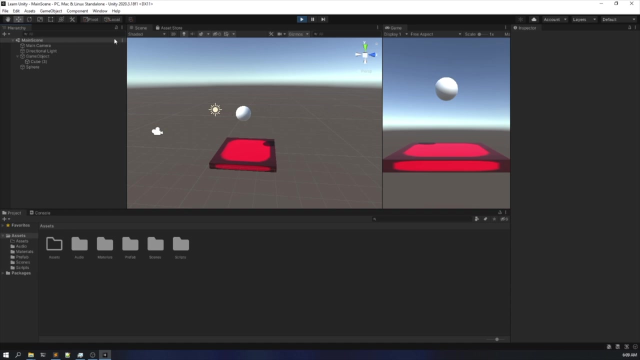 being in the game scene, all right. so just put it aside in here. all right, because we need the view, only, nothing else. one more thing I would like to say that after I get out of the, this game view object will get reset it because the won't be saved during the game view. remember that, alright. so now I 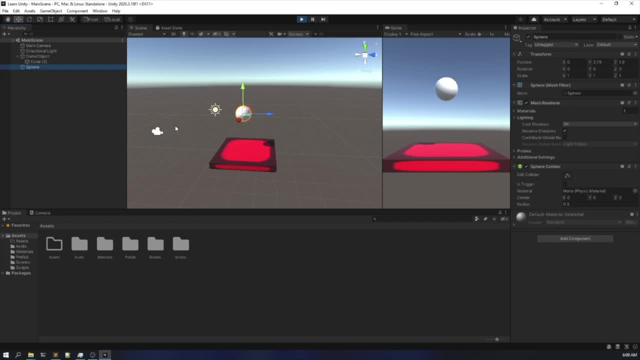 want this ball to fall due to gravity? all right, I want this ball to fall. how do I do that? so for there, click on this. add component. alright, there's something known as a rigid body. alright, click on this rigid body and see the effect. cool, isn't it like? after I added this rigid body, it's: the ball starts falling. no, it. 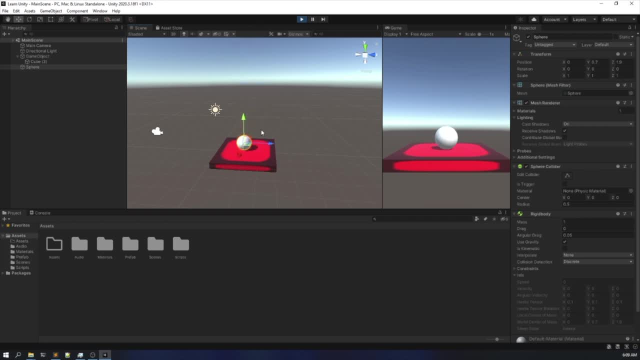 isn't bouncing right, see, to make it bounce. there's another, uh, sort of physics. all right, we need to create a physics material and all those things, but we won't be doing that in here. but as of now, you understood that, uh, we were able to add the gravity, like we would be able to add make the. 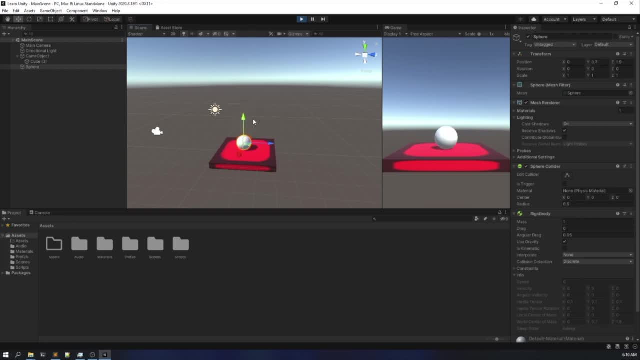 ball. uh, physical like we are, we are able to add physics to the ball right now, in the rigid body component. you can play with the values in here, all right, like the mass value, the drag, the angular drag. you can like click on this, use gravity, let me. let me show you one thing if i click on this. 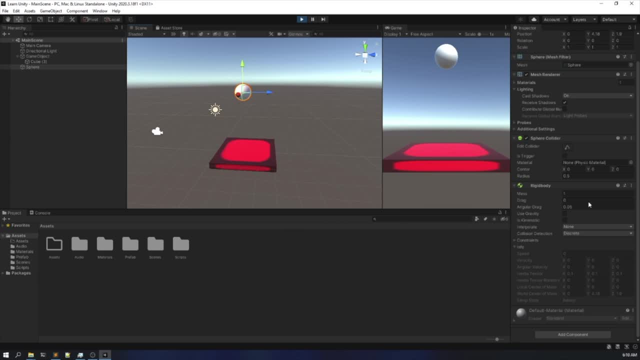 uh, see, it isn't falling because it is not using gravity. so see, cool, isn't it great. now here's another option: collision detection, all right, uh, before explaining this collision detection thing, all right, i would be telling you how this collision is happening. how is it? is there any sort of magic? before that i 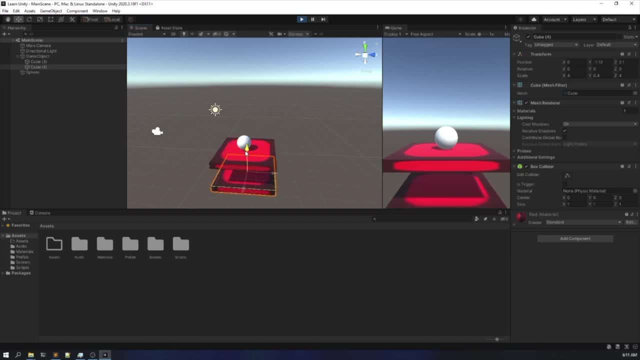 need to replicate this object. all right, because i don't want the ball to fall. all right, i literally don't want it to fall. so here you can see. here are some options. box collider: all right, this box basically provides the collision platforms. all right, it provides the platform like, uh, like in. 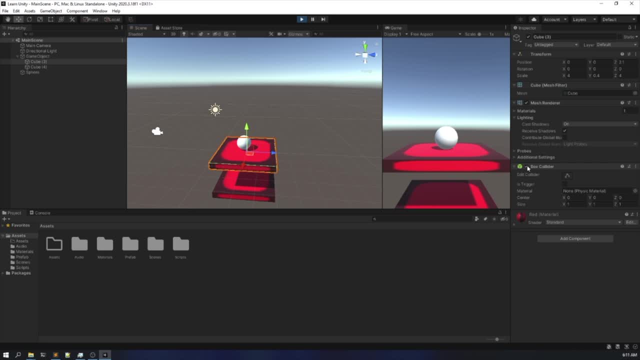 the ground. we are moving, all right, we aren't falling like we are falling. we aren't falling through that, uh, whole road, right, we aren't like. penetrating that road and going to the bottom of that road are like: does that, does that thing happen, doesn't right. similarly, in terms of games, 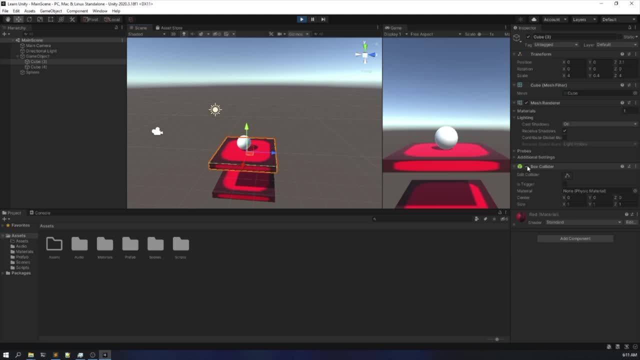 platforms: right, those platform has some colliders. all right, those are both box collider. so here, if i click on this box creator, you can see: all right, you, uh, you just saw that. the ball caught it through that because there aren't any collision. i like there aren't any collision happening to. 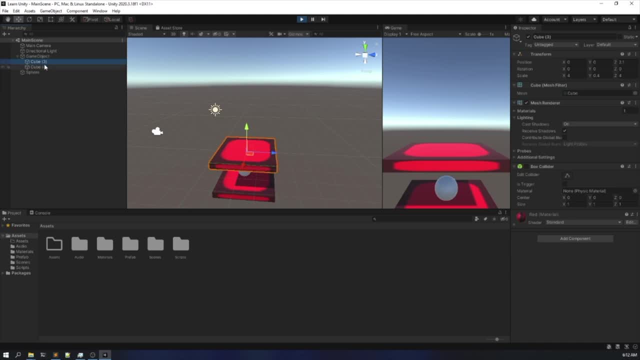 stop that ball right in there, because we have disabled the uh box collider, right. so box collider actually helps us to uh like these colliders. they're multiple colliders, so if i types of colliders, actually box color is one of which type. like there is peer collider, all right. 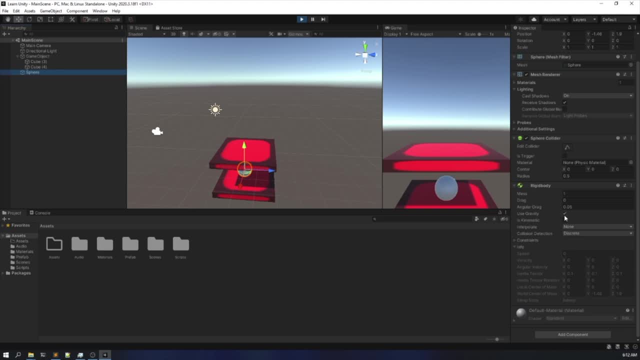 so box collider is? uh. basically helps us to pro uh to provide collision to that particular platform. right, just just wait, uh, so yeah, so uh, this is how everything is happening. right, cool, isn't it? so we have understood about colliders. one more thing: they're like: there are many multiple. you can have multiple uneven shapes. 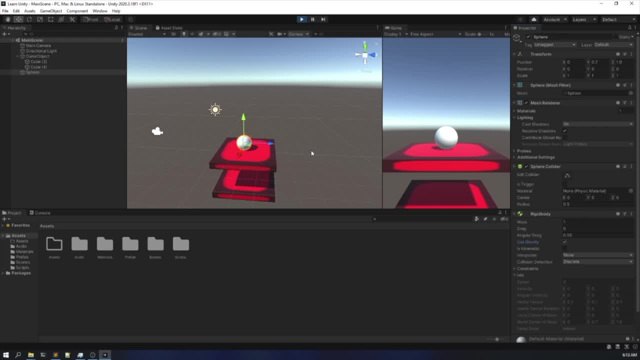 right, like, like a terrain, all right, like a road. they are like. a road is uneven, all right. a desert, it is uneven, it doesn't have a flat surface, it is totally uneven. there are uh highs and lows, right, so this is how everything is happening, right? so for that type of for like, if you want, uh want to provide collider to that platform, 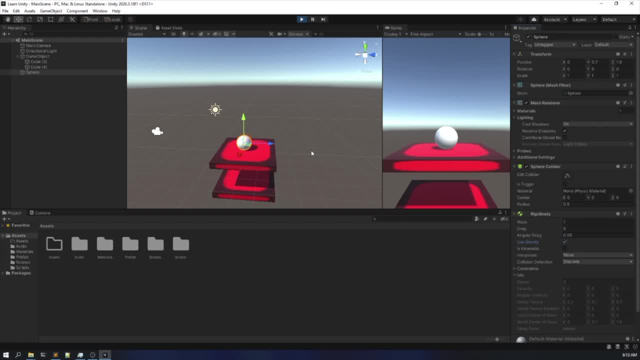 we can't use box collider in there, right, because then it will be totally plain: we want, we don't, we won't be able to use it. so there's another collider name: mesh collider. all right, it is in the component only. all right, i want you to try that collider out. all right, by yourself. just. 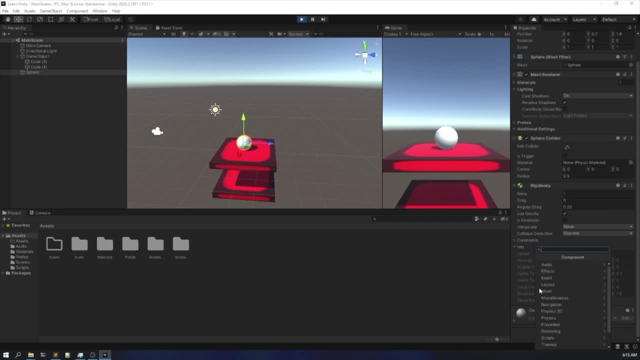 flow to app component. click on mesh collider and you can use it. now the problem with mesh collider is, uh, it is a bit more cpu intensive. all right, then this box collider or spear collider or any other collider. the reason being there is it does more calculations than box and spear collider because, uh, the mesh collider. 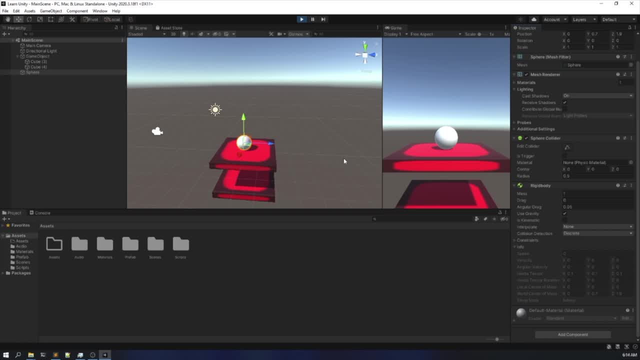 what it does it? it gets the accurate shape based on that particular terrain or the particular model, right, isn't it? so so what? uh, they get that particular shape. so it does more calculation now in the rigid body. i was going to show you something known as collision detection. what is? 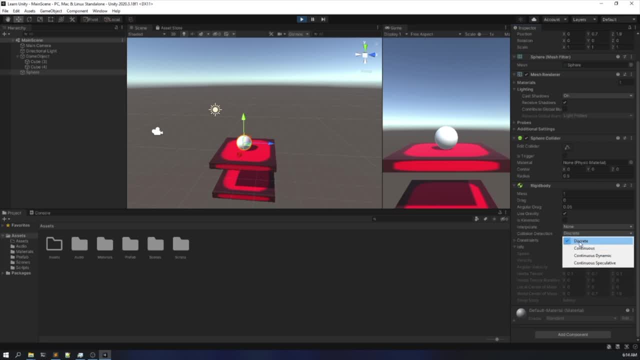 that the multiple option. all right, we'll be looking into two main of these: discrete and continuous. now, there's a huge difference between those. all right, see what is the difference? discrete is performant, all right. discrete, uh, gives a lot of performance. it is like in in: performance wise it is better than continuous. 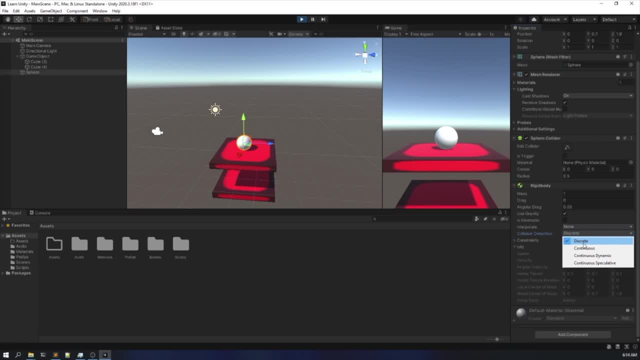 all right, but the problem, the problem there is. it uh does like it doesn't do accurate calculations, it doesn't like it can. if you, if you throw it from a really high, like at a really high position, it will penetrate through this whole uh collider all right through this whole platform. 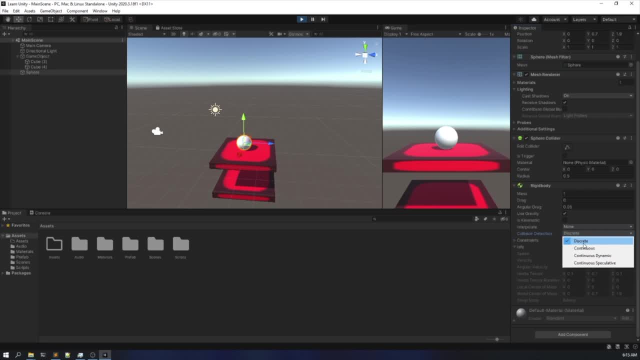 but continuous. continuous is uh is better than discrete. all right, because, uh, with the use of continuous there are very less chances that it will penetrate through, because it does more calculations than discrete. but the problem is: continuous is cpu intensive. so that's the difference, major differences. all right, so we also learned about the very basic physics. right, we learned about the very 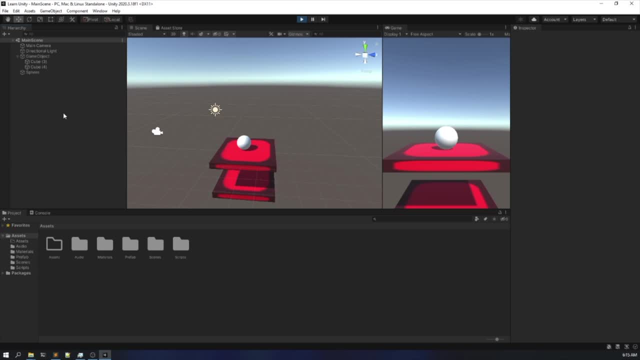 the very basic points, from the very basic points, from the very basic point of view. here we will now go to the next step. that is all right, and that is our time now. it's our time, it's up-to-date, it's our time to learn. uh, this audio right. so for that, first of all, to play that. 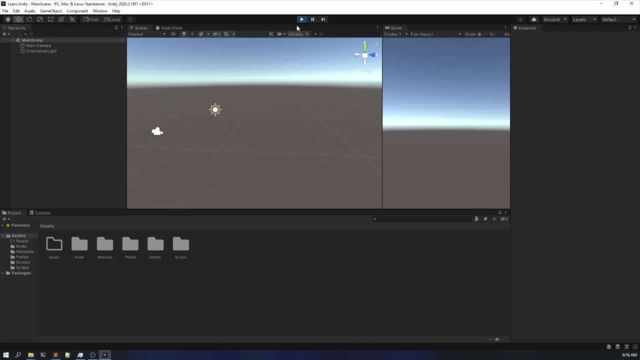 audio. all right, first of all, to play that audio. oh my god, i deleted everything, uh. so, yeah, all right, i will be getting those objects back, because i did that with, uh, our whole environment. so we are now. i want to create an audio object. how do i do that? go to this, uh, click on this. 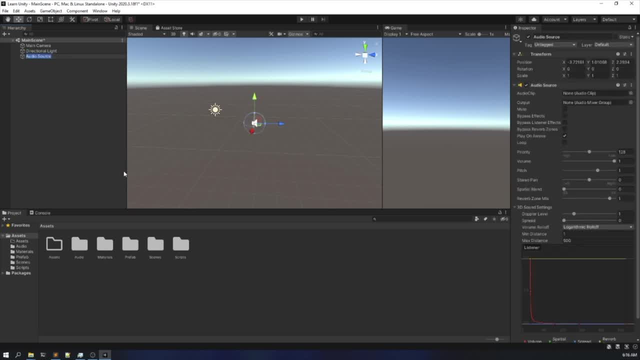 go to this thing. all right, click on audio source. all right, so we created a simple audio source, right, we created it. now, here are some particular options in there. all right, click on this, select the audio and, uh, let's, let's play it. all right, just wait, this is a. uh, this audio is the. 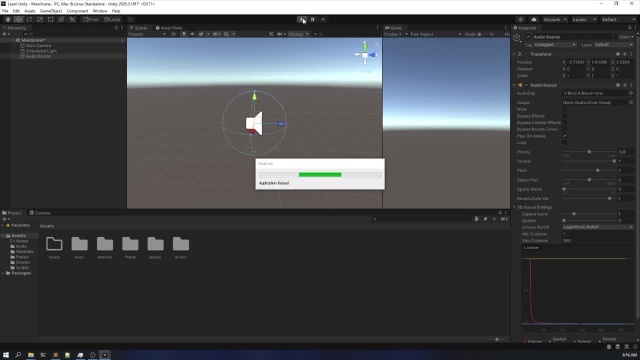 birds and beach audio all right. like we, birds chirping are in the big uh beach, all that audio thing. are you able to listen it? i'm sure that you are able to listen, so audio is playing right. so, uh, the audio is playing in here. right, the audio is playing. that's cool, isn't it? so we implemented. 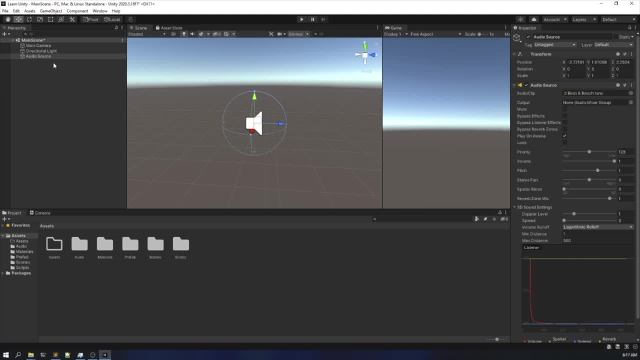 our own audio source. all right, now, uh, soon in our pre uh, in our future lectures. all right, we'll also be learning how to control our audio sources through scripts. all right, but for now, if we look into these like uh properties, there's a uh option for mute. now, i won't. 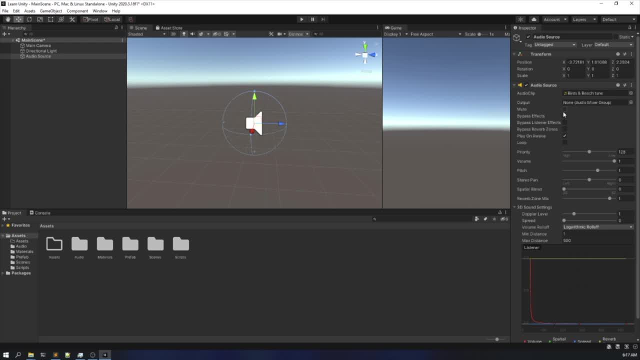 be actually explaining all the things in here. you have to explore it by yourself. like: uh, you can explore these bypass effects, bypass listener effects, bypass reverb zones, all right. now, these- this loop is basically uh- will loop the audio. all right, because without loop initiated, all right. 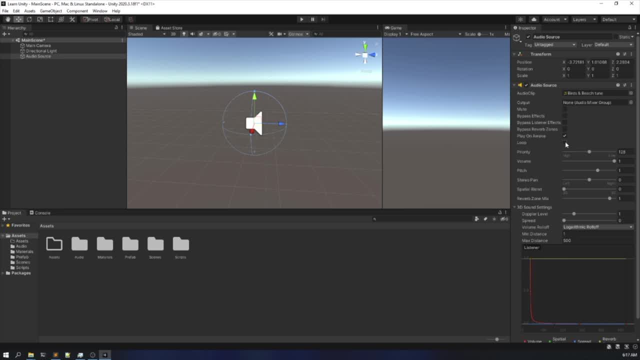 without click. checked on loop. uh, what will happen? your audio will only play once, but with loop, it will play all the time. all right. now here's another option, that is play on awake. all right, uh, play, play on awake. what it does, is it like when you? 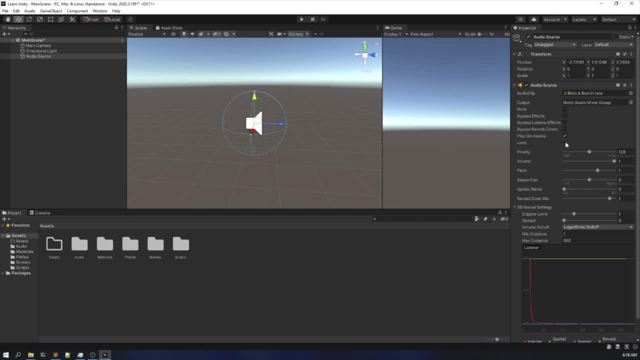 play your game. all right, it will start the audio at that time only if i, if i uh like remove it and then start playing it. uh, just wait. so, uh, it has started playing, but you uh won't be seeing anything, like you won't be hearing anything. 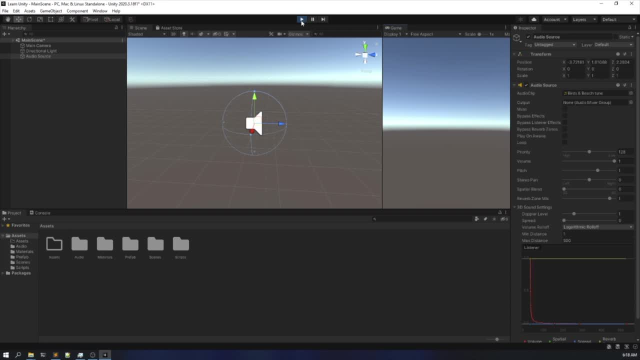 play on awake is disabled. now to play that audio i need to add some trigger or some sort of script to play that audio. all right, so play when on awake. what it does it basically uh, plays the audio whenever you start. now here's another thing. that is volume. all right, now, this is the volume it uh. 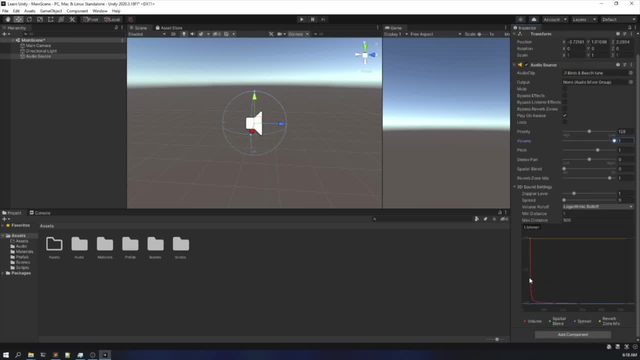 varies from zero to one. all right, now there are multiple other audio editing uh feature. you can check them out by yourself. all right, you can do some research on them. all right, so till now we have- also we uh have- completed most of our topics. all right, we have completed most of our topics now. now, the last but not the least. 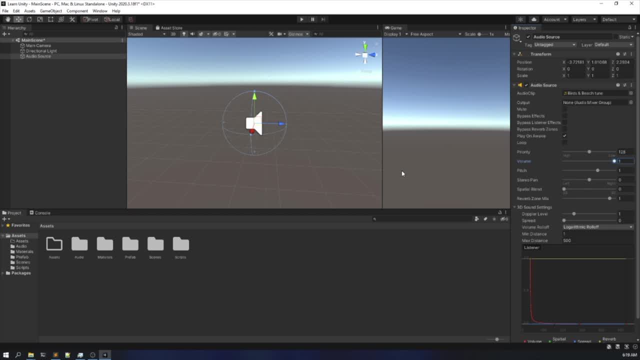 creating our own user interfaces. how do we do that? all right, see, i'll be creating a very simple user interface. all right, nothing too complicated. all right, nothing too like, nothing of like very complicated user interface. a very simple one, just to show you, all right, how to create one. 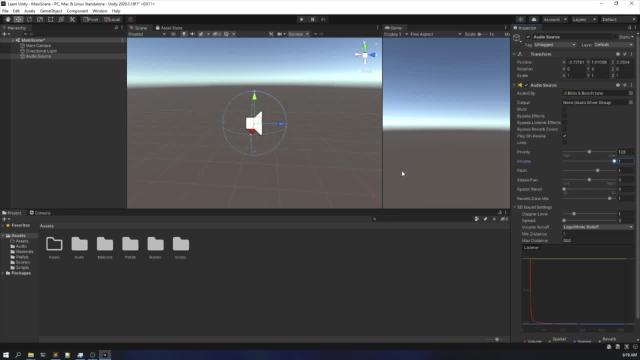 all right, but we will be creating uh beautiful interfaces during uh like during the making of our uh course, like the uh projects. all right, so just let me delete this particular thing because i don't need it now. all right, so let's save it now. how to design our own interfaces. all right, let me dock this game view in here. 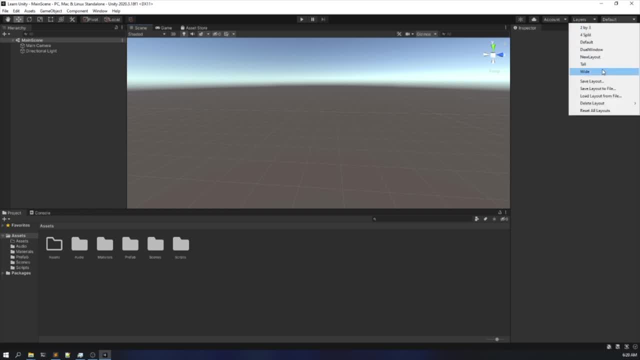 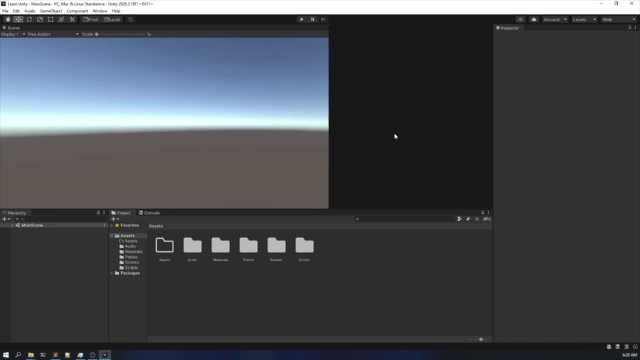 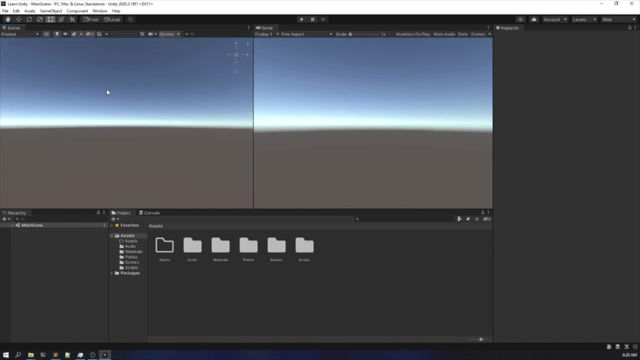 and for that. first of all, i want to go to my wide view, right, because it helps me a lot. all right, so, first of all, click on this 2d option here you can see. all right, this will give you a 2d view. all right, this would give you a 2d boost. i got the 2d view. all right, i would like. 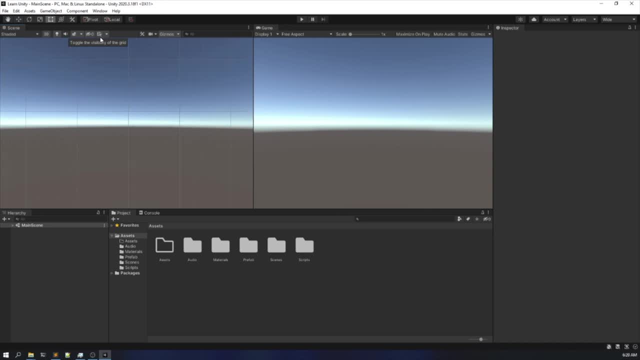 to say here that this is this white thing. the reason, because this will give you a grid and it's really helpful. now, uh, first of all, we have to uh right click and click on the ui option, then create a canvas. all right, what is this canvas? right, what is this canvas? basically, this canvas is. 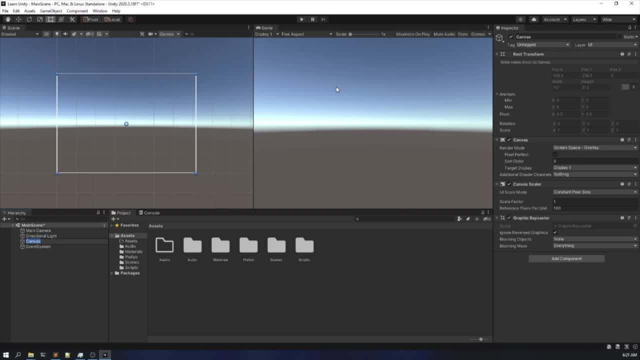 basically the like: uh, the basic framework, all right, the basic wireframe of the, or you could say the frame for handling the user interfaces, right? so click on this canvas. all right, here are some options. what i would like you to do is, uh, first of all, uh, click on render mode. all right, keep its screen space overlay as of now. 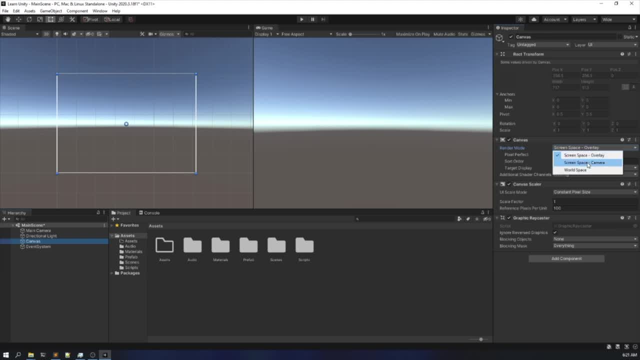 there are multiple options and definitely we'll be looking forward to uh these in our future lectures. all right, and this world space is going to be really useful during the like, during our making of those projects. right now, here are some options. all right now, go to this canvas scalar. 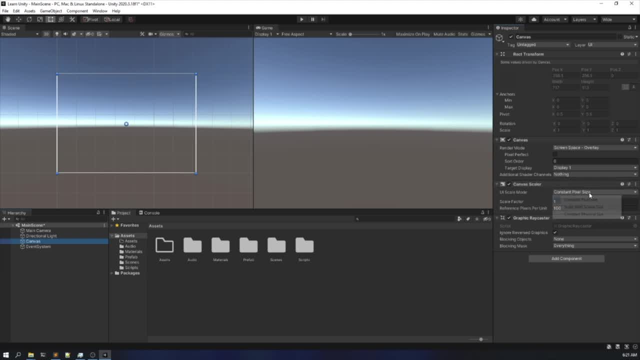 thing. all right. now, ui scale mode, constant pixel size. do to scale with screen size. all right, and give it a default resolution for me as of now. uh, this, uh, 800 by 600. you can see that it is now. uh, it is now uh, 800 by 600. 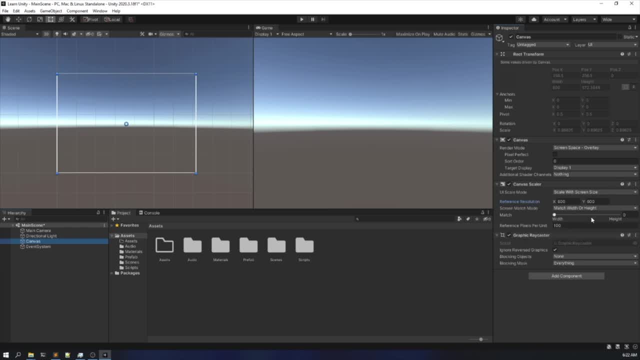 is okay and leave all those parameters same. all right, uh, for now, this is what i need. now our canvas is ready. right, our, our canvas is ready. now i want to like get the display of my laptop in here, like the resolution of my laptop in here. okay, uh, very well, sorry, my mouse is like. 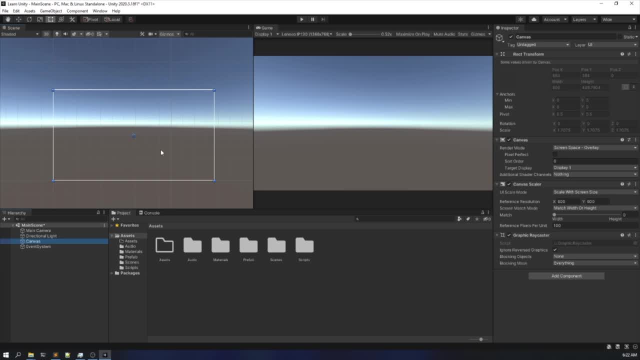 sometimes, creating the problem of navigation like the mouse is like creating the problem of navigation like the mouse button- middle mouse button. so as we've created a canvas, all right now we need to, uh, create a background image for it. so how do we do that? so click on canvas, click on ui. 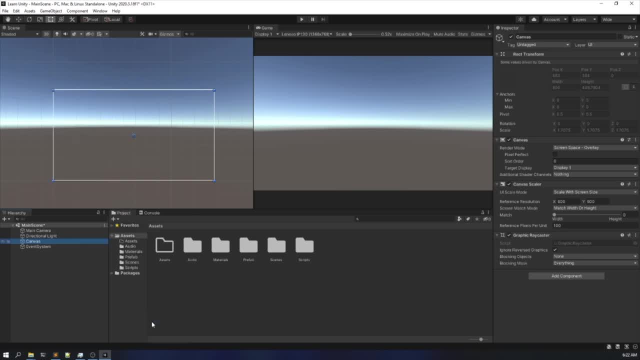 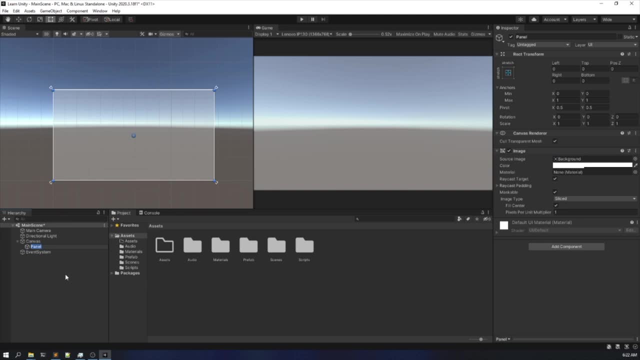 then there's something known as panel. all right, click on this panel right. see, you got a sort of background. all right, now i need to color the background right. first of all. i name it a background image, right? although i haven't imported any image, so i will take coloring it all right. first of all, how to do that. 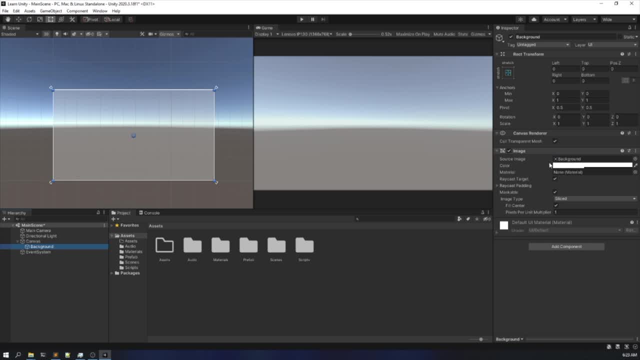 uh, click on this panel, all right. uh, click on this image section. all right, here. from here, you can select the image you want, all right. so already one is selected, i don't want to change it. click on this color option and here we'll be seeing that this, this thing, is transparent. how to make it opaque? 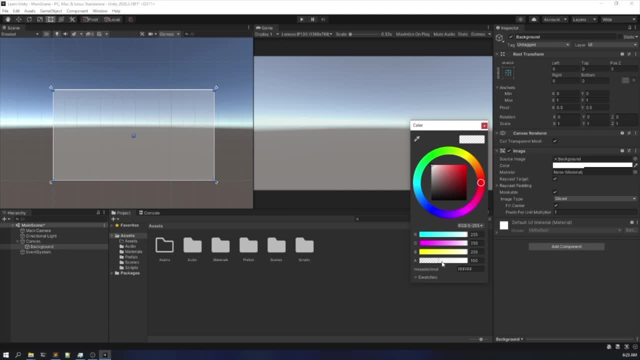 see, here's an option known as a, also known as alpha. so just just click it in here and like, make it 255, like, make it too full. i want an yellowish orange color. so this is the color i wanted and i got right. so now this is my background. i'll be scaling the 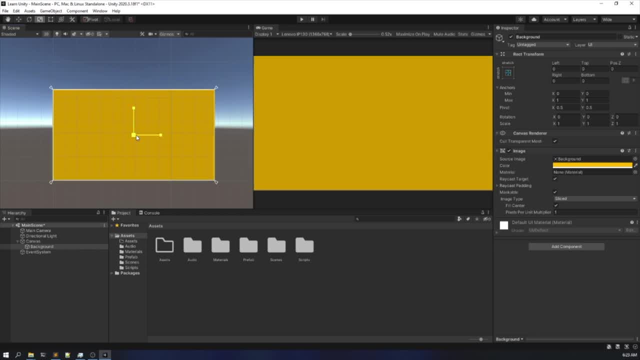 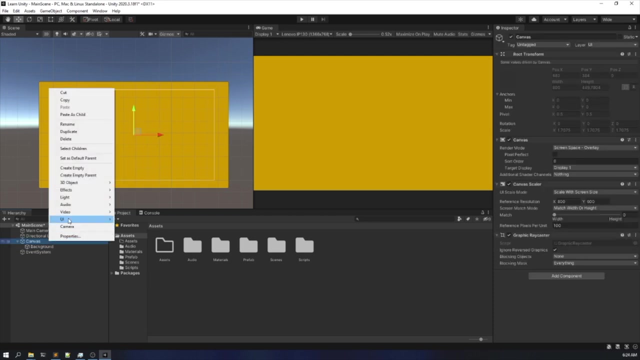 background a bit. how do i do so? uh, choose the scale tool, click on the middle option and just scale it right now, as we are. uh, have created our own background. now what we want- we want is to create a heading text for it. how do we do that? how do we so? click on ui, then i. there are two options: text and text mesh pro. 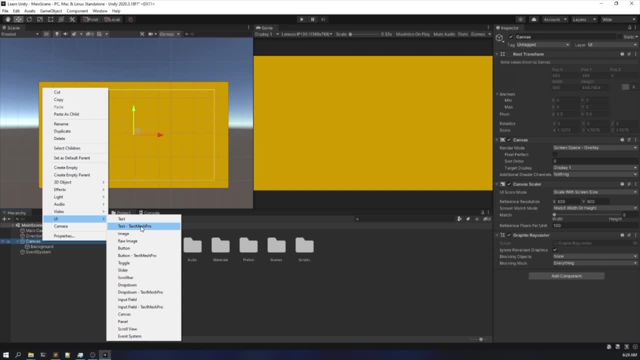 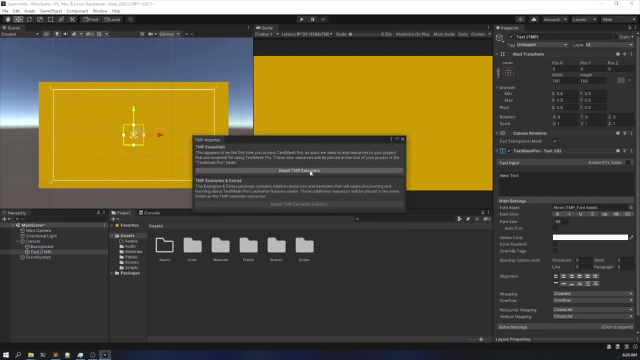 alright, i haven't imported text mesh pro, although text mesh pro is the better option to go for. all right, because it pro and the quality of the text in text mesh pro is really good. all right, just wait. yeah, uh, i'll be uh importing the uh text message essentials. all right, it will take some amount of. 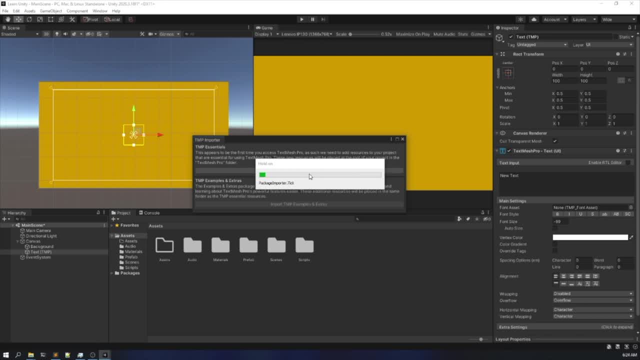 time. all right, don't worry. all right, let it. uh, let's take the time it want, all right. all right, because that is importing all those assets, so it's important for it to be important, clearly, just wait. so yeah, it is getting imported. uh, just, it would take some amount of time. 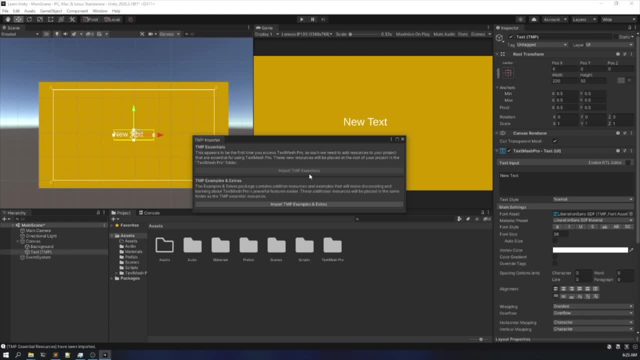 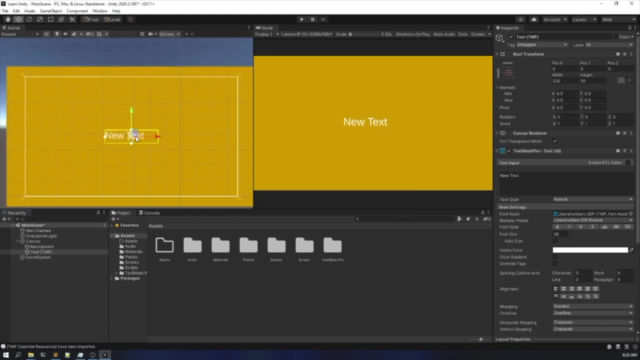 actually, i guess i should have like imported it previously only, but, uh, if i did so, you wouldn't have like caught how to do that. so here, we got our text in here, right? we got our text in here, all right. now we want, uh, to edit the text. 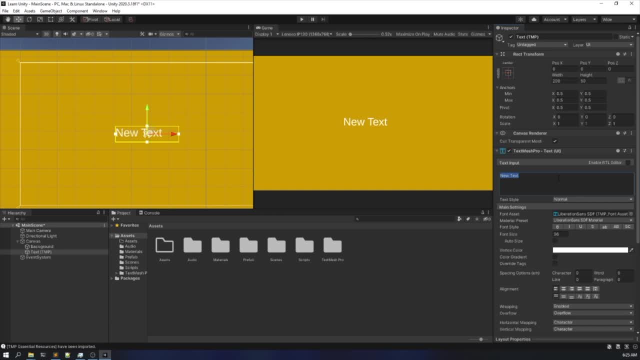 and let's, let's, let's name something. all right, let's name it, uh, our new ui. all right, i know, this is like a very bad name. now i want the textile to be like something like h1- right, but it's giving a color, no, no, let's leave it. let's, let's keep it normal only and click on bold right. we can even. 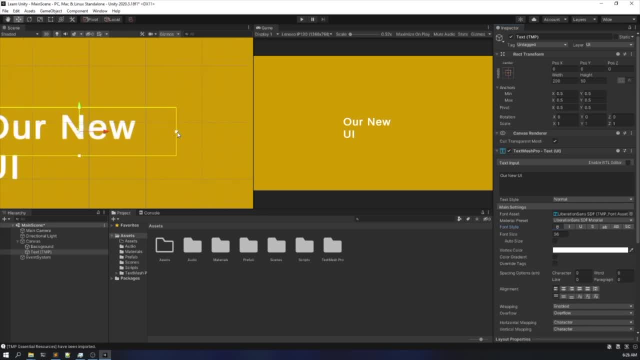 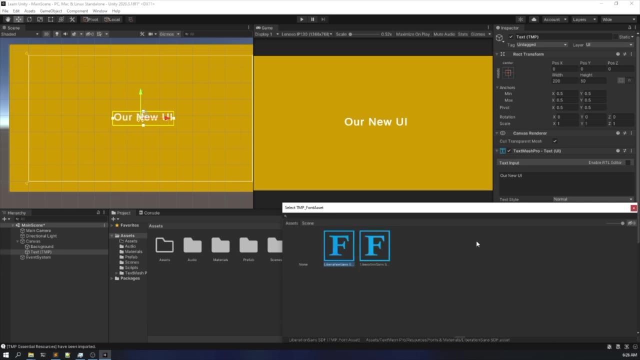 resize it how, uh like, zoom it in here and you will find these anchors. all right, do this, do this right? other thing we want is to center our text. so we did that. all right, so you can. uh, we also have some other forms, all right? uh, okay, we don't have one. oh, i, sorry. i. 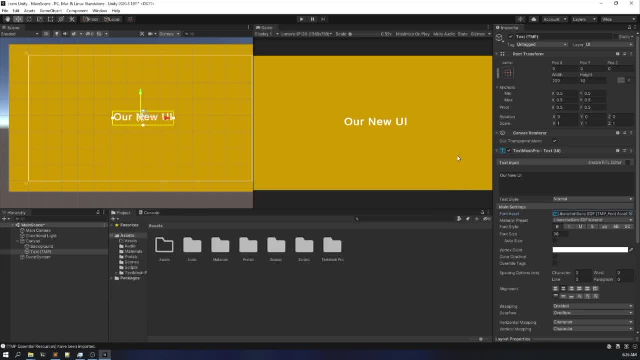 forgot to import that. uh. a extra package came with uh. test my flow, but no worries, we don't need that as of now. now, here you can see, here is that direct transform option. click on alt, all right click on alt. click on uh. so, as you can see, if you just open it, all right. 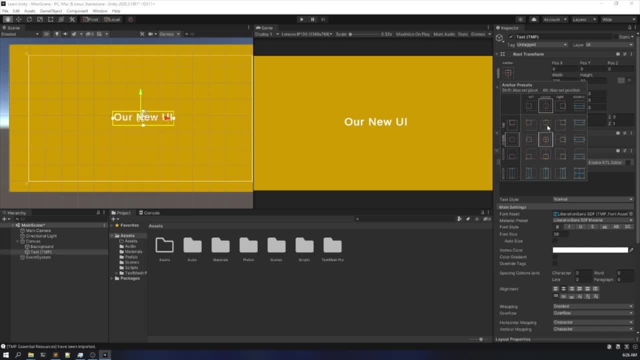 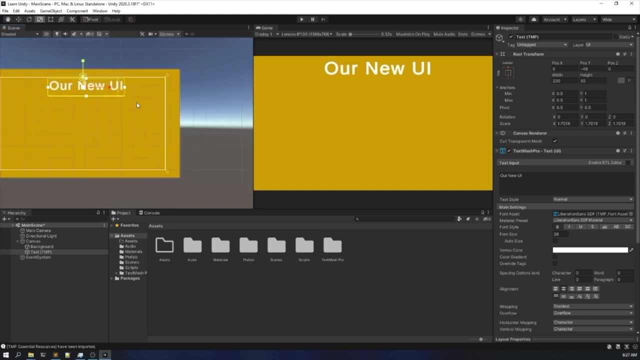 and click on alt. there are multiple options here. i want you to click on this top one. see our text automatically got in there. now i want to reposition it and voila, we got our text. or just yeah, we got our text to where we want and this is our ui. all right, our new ui. or let's say: 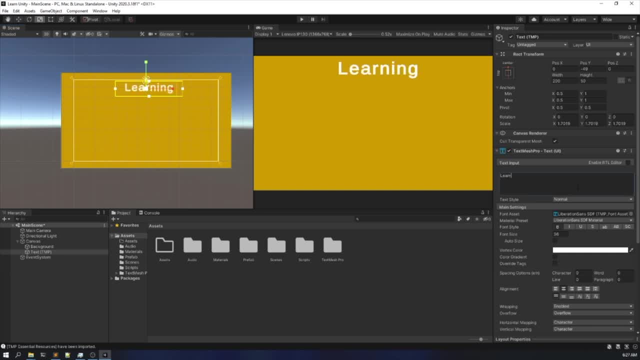 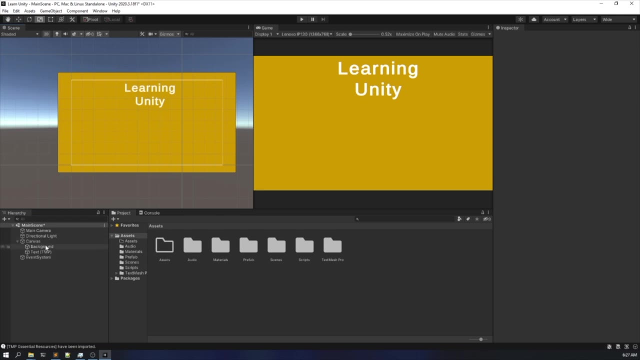 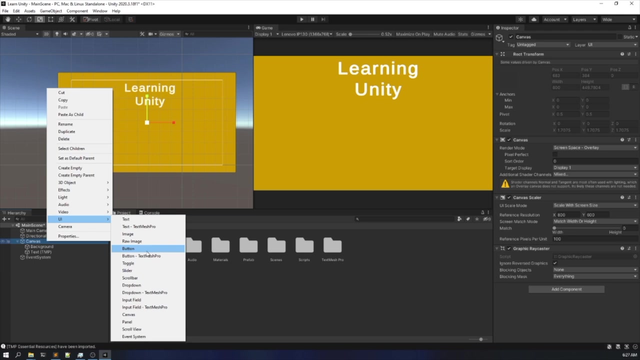 uh, let's name it- to learning unity, right? so this is our new ui. cool, isn't it? now we want to add- uh, some buttons. right, we want to add some buttons. how would we do that? click on canvas, click on ui. here is an option known as button and button text mesh pro. i would i want you to go for. 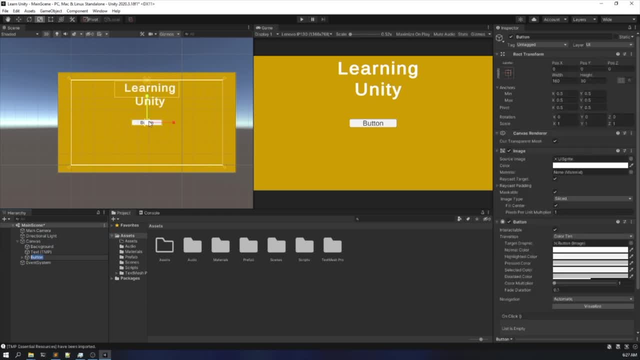 button text: mesh pro. it's better. believe me, it's a lot better. all right, now we can even add some functionalities. all right, first of all, i want to like put a transform to it. i wanted to be, wanted to be in center. only, let's name it as a play button. all right, let's name it a play button. 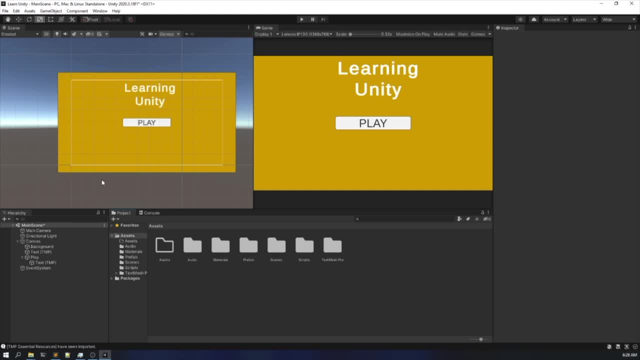 name it play see in future, or we. today, we are learning just how to implement our own ui. all right, in future, in future lectures, we will be learning uh like how to navigate through, uh our scenes, how to like add functionalities to our button right. so for now, this is what i want. 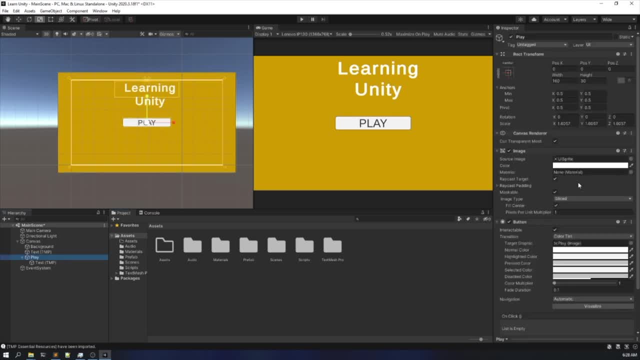 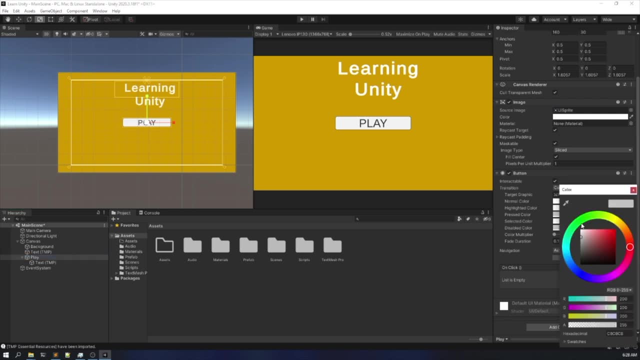 so we created our play button. all right, even, uh, i can change the color. all right, there are some many things all right, like if i, if i click on this praised color, i want to make it green when it gets pressed right now, if i play this, if i play this, just wait it. 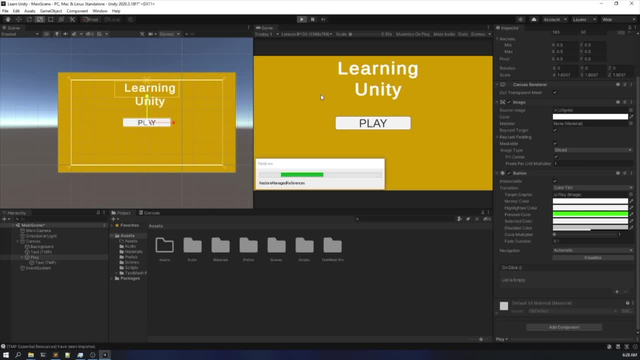 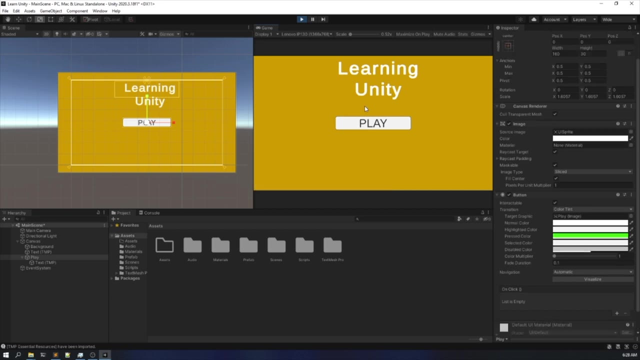 would take some amount of time, because unity takes time, all right, so, uh, just just wait. it's entering the play mode. cool now, if i click on this. see when i'm clicking or clicking on it. uh, it is uh getting green now if i, if i select the highlight color and 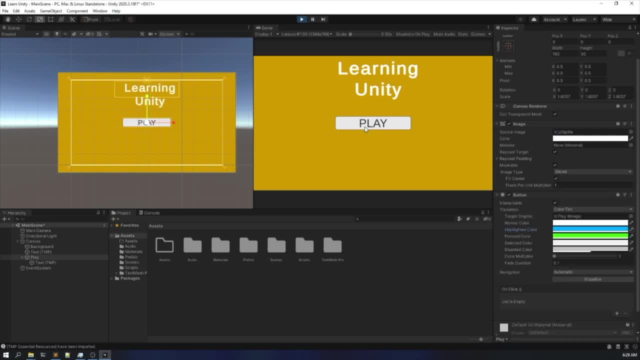 like: make it a blue, let's see what happens. oh well, nothing happened. uh, let's, let's check out the selected color. let's make it sort of like yellow. wow now, oh, i don't know why it didn't work. so when i'm hovering on it, it is highlighting the color as 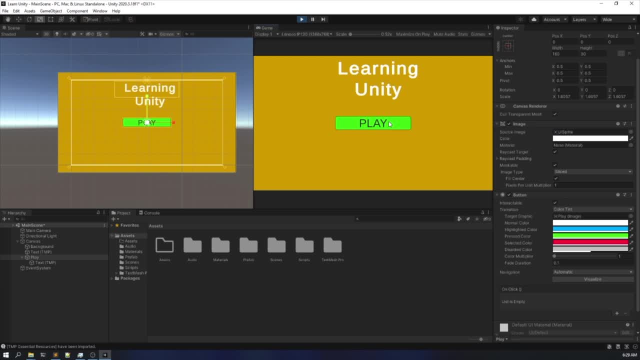 blue when i'm pressing it. that is the pressed color. it is green after it is selected. it got pink right, so isn't it really cool, all right. similarly, we can add some functionalities all right, like there's an option on click. all right, if i want, i can select the color and then i can. 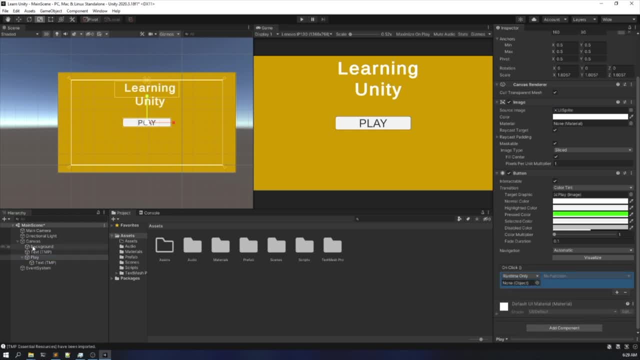 like add some particular function, like for now, let's say, i want to disable the text. all right, so what i will do, i would drag and drop this text. first of all, let me show you from again. this is an on click parameter. click on this add, then take the text in here. all right now, in here. 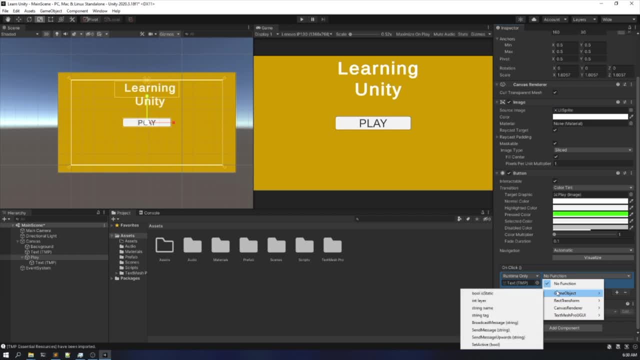 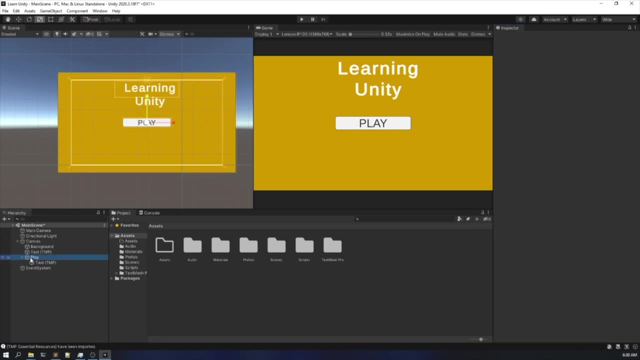 there is written: no function. click in here. go to game object: uh. click on set active. all right, and just don't check that button out. all right, we have. we can create another button something like this: all right, name it, uh, active. first of all, i would name it active. 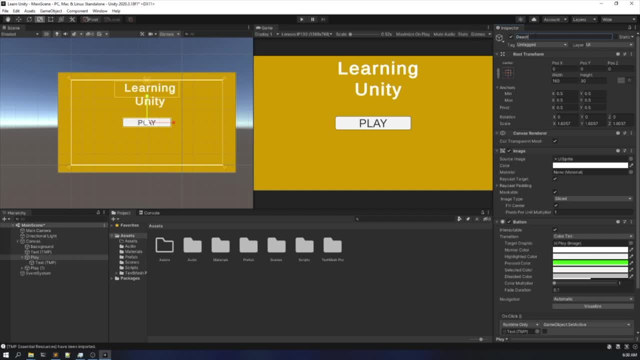 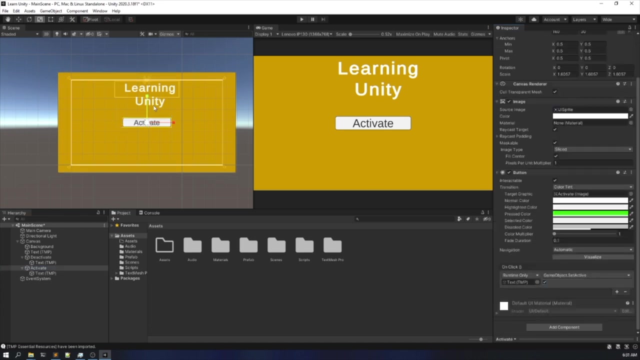 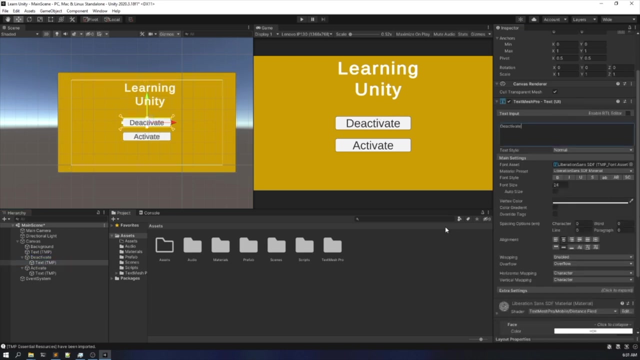 sorry, deactivate, deactivate, deactivate, and this one is activate. all right, i just want to like wait, this is going to like activate, like activate the whole thing. all right, just wait, let me drag and draw. drag it down in here, all right, uh, cool, isn't it? now, let's, let's try this out. what happens? let's. 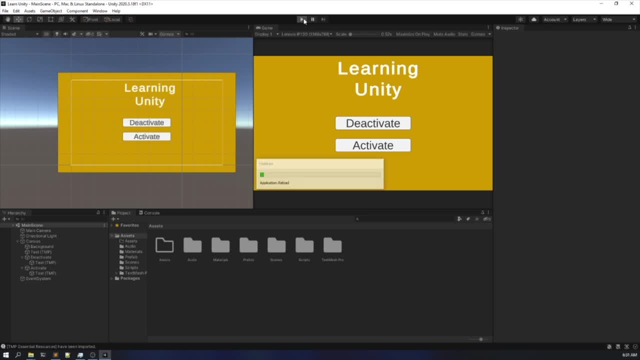 see, just wait. it would take some amount of time, but it will. uh, it will get done, all right, so just wait. cool, now, if i want to like, deactivate on it. i don't want this learning unity, i want to hide it. click on deactivate. see, it got deactivated, but i but i want it back. see, it came back. see. 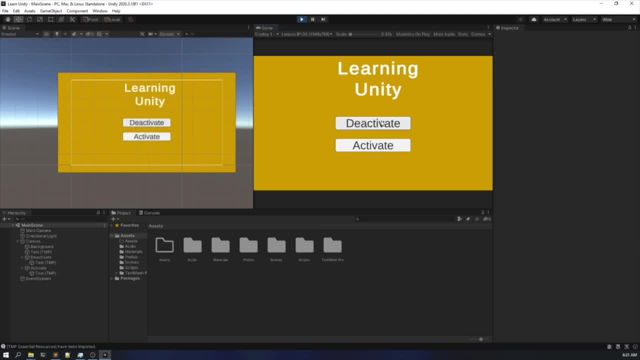 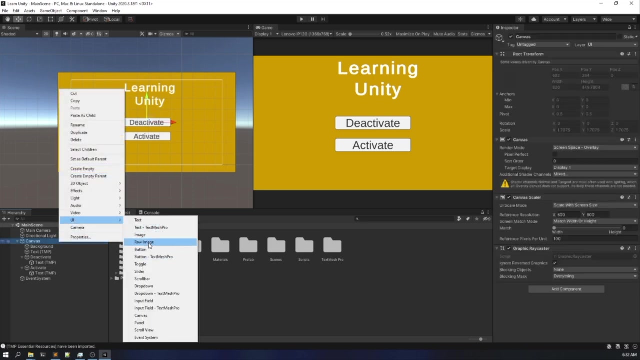 i'm making my button do some activity, so i'm going to activate it and then i'm going to go back and do some activity. so we also learned how to uh design our own interfaces. if you want to add some sort of image, you can just click in here ui, then uh draw image. all right. 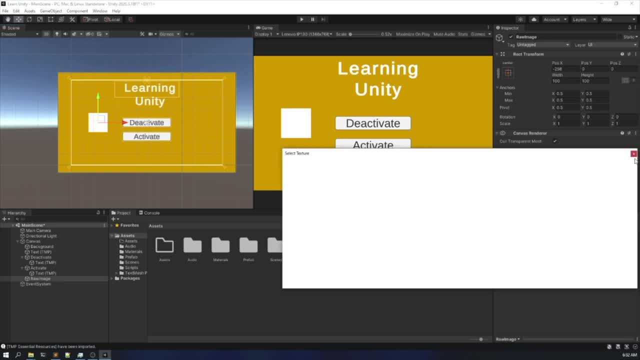 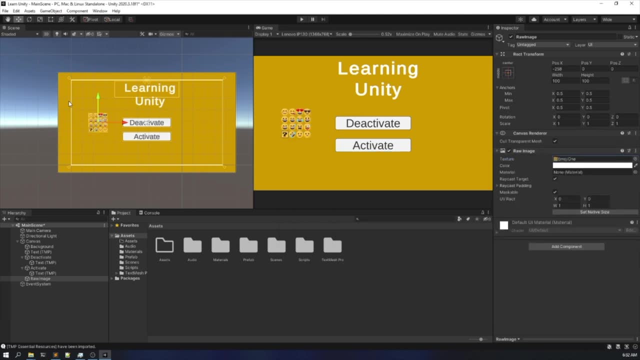 i, i don't know, i have any image for this all, just, oh, i do. uh, let's say i want, uh, i want this emoji one. right, i want this one to be in there and i can also resize it. um, sorry, it got resized wrongly. i'm in the wrong manner. so yeah, see. 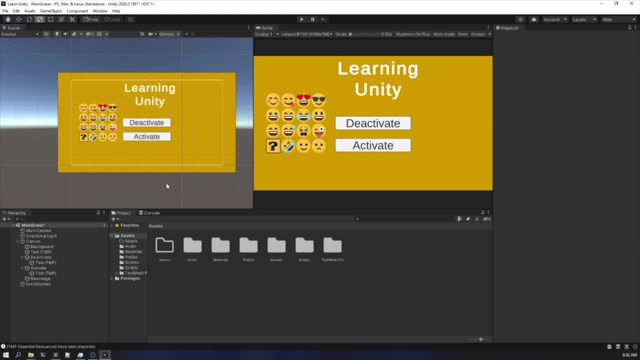 isn't this the ui looking good? actually it isn't looking good, but yeah, for now it's, it's okay, it's fine, right. so we also learned how we learned. uh, today we learned a lot of things in unity, right? so see you in the next lecture, thank you. so, hey, folks. 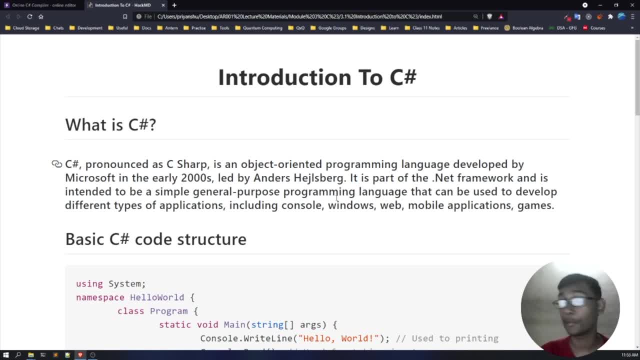 uh, welcome to our first lecture of module three. in this module, i'm going to introduce you to uh c sharp. so without any further ado, let's get started. so what is c sharp? right, see, c sharp. uh, first of all, one of the most important thing i'm going to tell you right now is 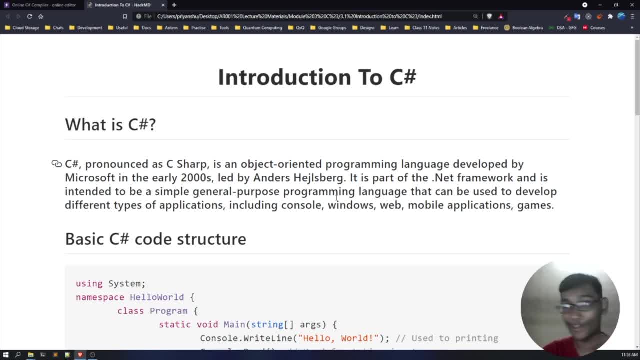 pronounce c sharp as c sharp, only not c hash, like i have seen many people. they like, uh, they don't know that how it is pronounced, or they even sarcastically tell that it is c hash. guys, it's not c hash, it's c sharp, right, uh, so yeah. so see, c sharp is an object-oriented general. 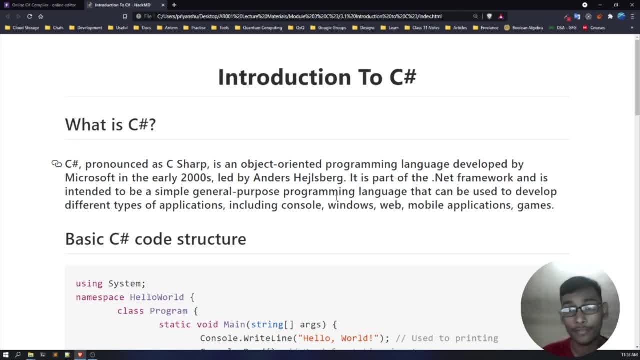 purpose programming language. all right, it was developed by microsoft uh in the early 2000s, right uh. the development team was led by uh anders hillsberg and it is a part of the dotnet framework. it can be used to develop different types of uh softwares, like console applications, windows. 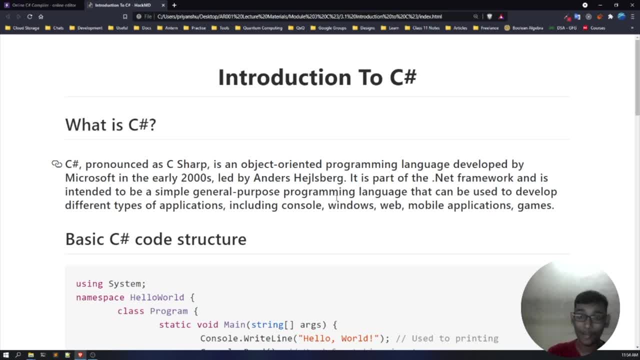 applications, uh, then web applications, mobile applications, and so on and so forth. so that's all. so the c sharp is just a cork. so this is what it's made out of: the code package with a, some things like csh and c meet and all the home versions and the program models and 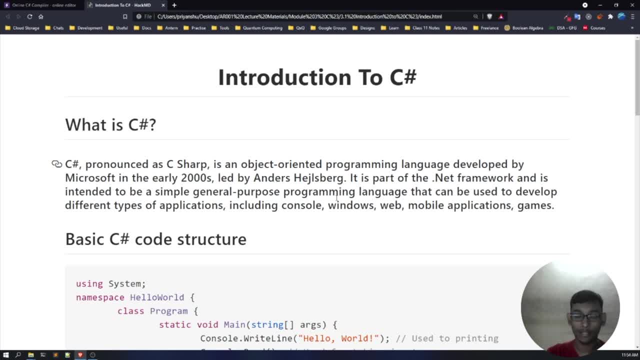 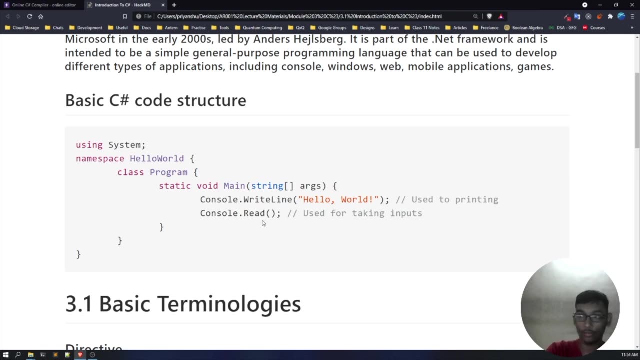 so this is what they are. all this is what it's like to do. so now let's get into the coding part. all right, so this is the coding part. so the coding of this process is very basic. right, so this is the code structure of the game. all right, so this is some of the things that we 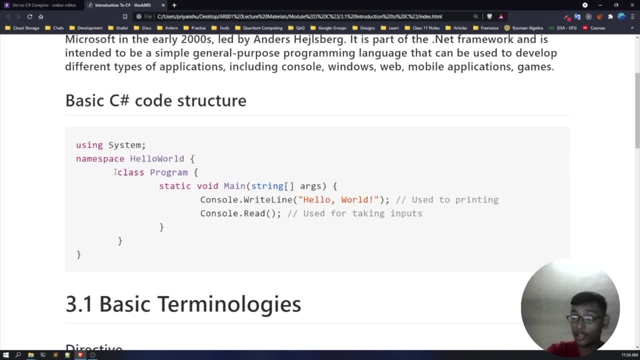 need to know to get into this part of the game, and that's not a lot, but this is a good way to do it. so let's get into the coding part, all right. so this is a very basic code structure, all right. so使用 hello world, then class program, then static void main, then console dot write line. then. 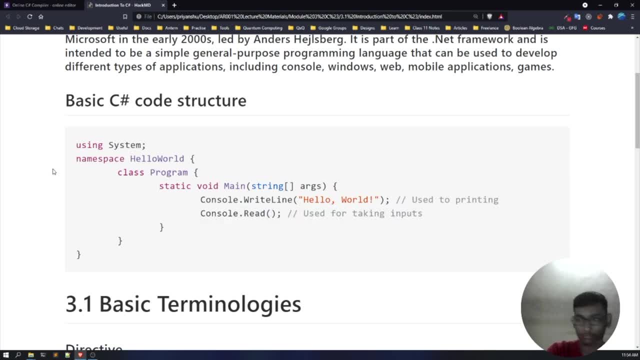 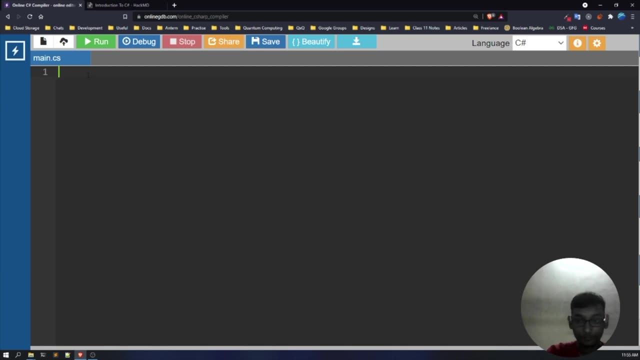 console dot. read right, so don't worry. uh the. if you are not able to understand what are these, don't worry, i am there right now. i'll be coding this, all right, and after that i'll be make you understand what is this? all right, so here's my c-sharp compiler. right, this is my c-sharp compiler. 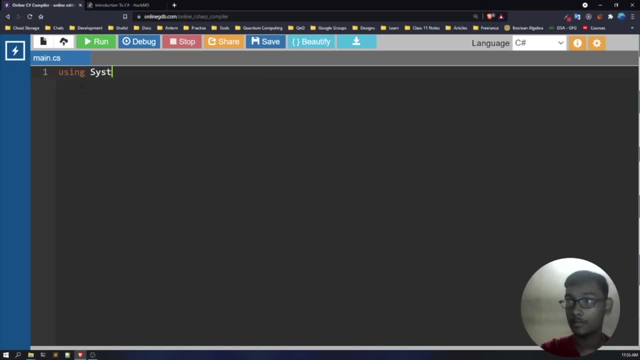 so i'm going to write using system name space: hello world, right class. uh, let's say, program um public static void main. uh string args. then console dot right line: hello viewers. sorry, then console dot read right. um, that's it. now let's uh run this program. let's see what happens. 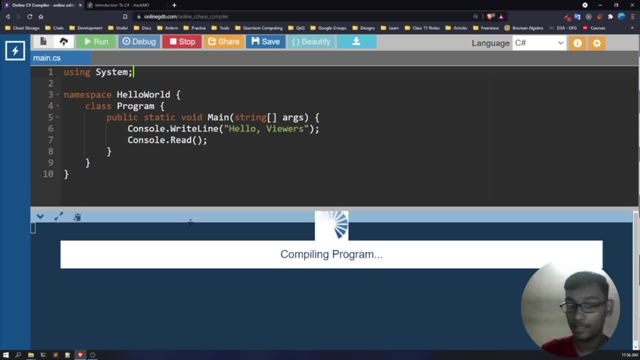 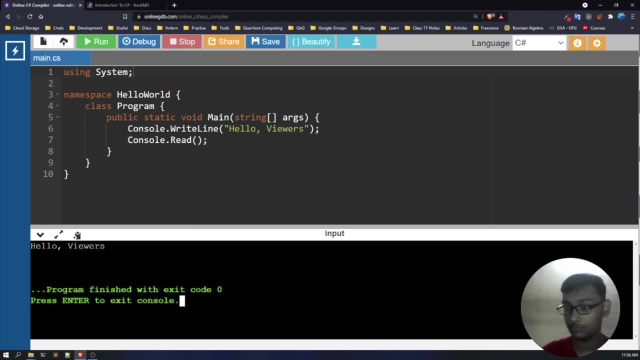 um, wait, it's compiling the program. cool, now, if i click enter, the program will be finished. so what did just happen, man, it printed something, right. it printed something in the console. can you see it in here? it's it's printing something right. it's printing, definitely it's printing. so let's understand how is. 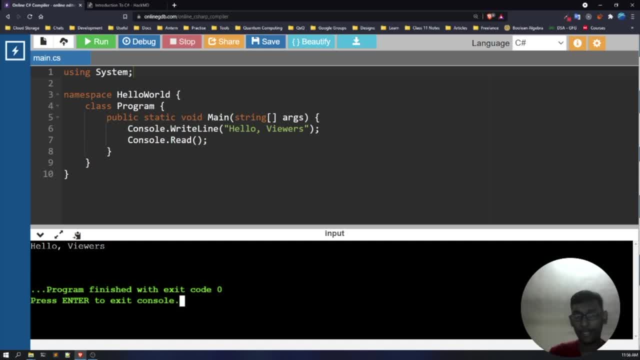 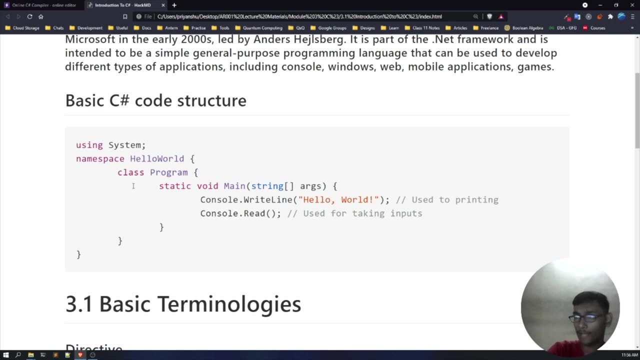 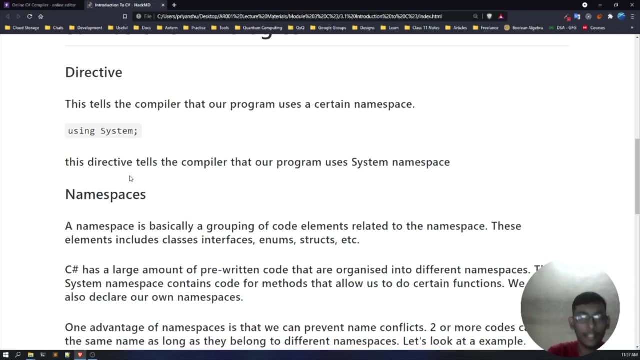 this working? what are these gibberish right? let's understand. so, by the way, congratulations, you coded your first program, so let's get back to the notes. so yeah, first of all, let's let's know what a directive is right. what is a directive? see, a directive basically tells our program: all right, so not the. 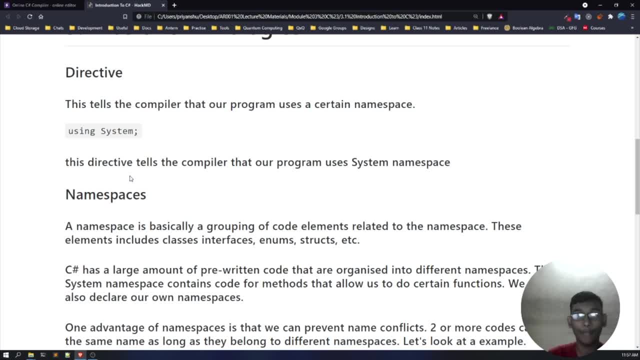 program. directive basically tells our compiler what is the compiler. compiler compiles the program, all right. we haven't set up any sort of local compiler because we are using our own online IDE for coding, all right. so directives basically directs our compiler, all right, our compiler that our program is using this namespaces. our program is using 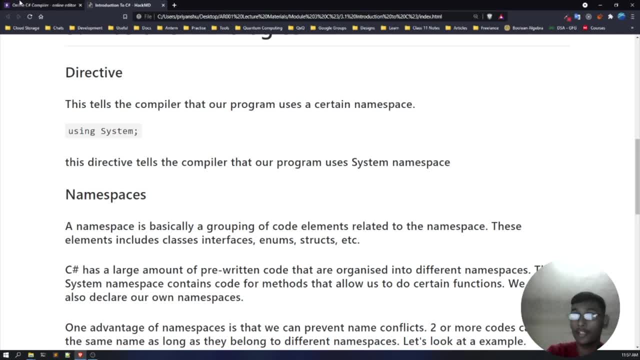 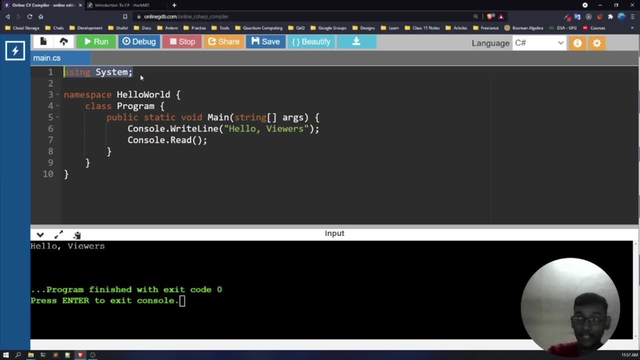 this, certain namespaces, all right. so what is a directive? right, see, this using system, this, this using system is a directive. this using system is a directive, all right. similarly, there are others also, like system collections and all those things. all right, like you watched in the that unity video right in. 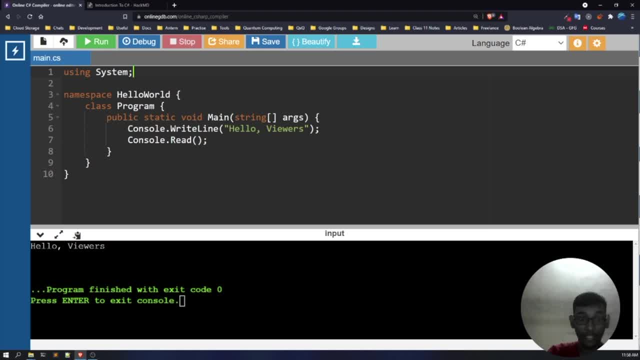 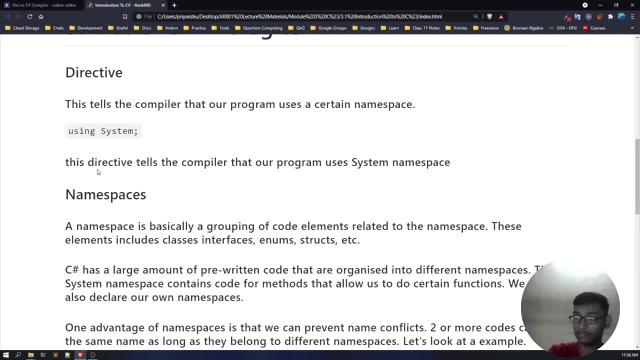 that unity tutorial, that there was a using unity engine, right? so yeah, there are multiple namespaces, sorry, multiple directives. so yeah, this directive is basically this: using system directive tells us all, right, this using system directive tells us that our program is using this system namespace correct. it is telling that our to our compiler to. 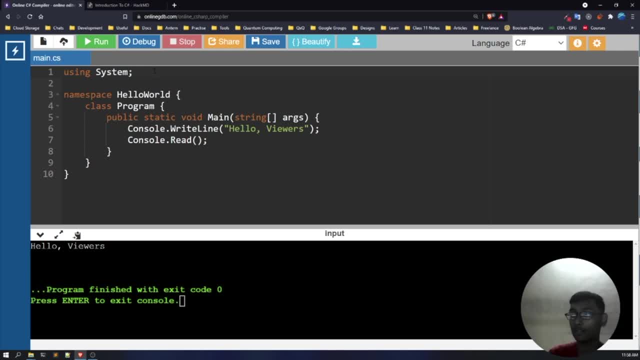 it is telling to over compiler that, hey, compiler, I am your C sharp program. this is the system. to our compiler. that a compiler, I am your csh program. this person created me, so i'm using this uh system name namespace. are you okay with that? and that compiler? 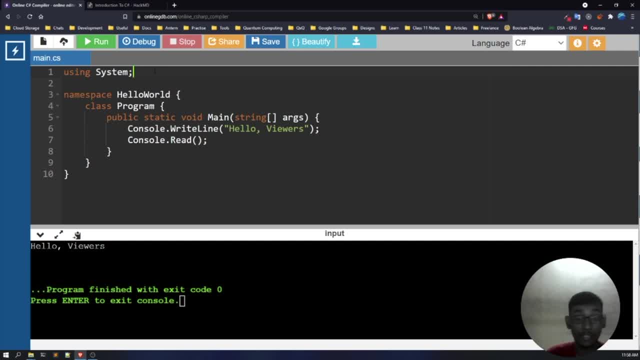 replied: yes, i'm totally okay with that, because this uh using system is already predefined in my compiler code base, right? so i am totally okay with that. we can run the program. so yeah, compiler happy, our code happy, the other code are happy, right? so yeah, now, as i told you about namespaces, right, see? 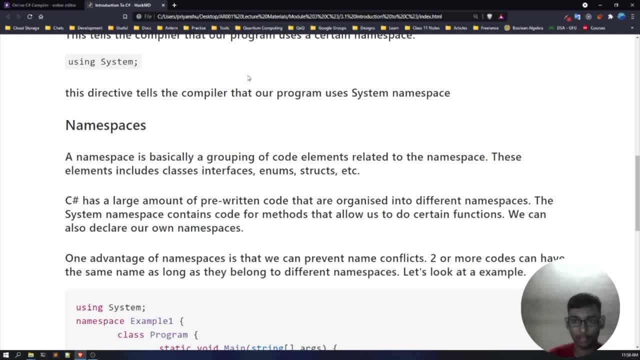 namespaces, now, they are basically a collection, all right, they are collection. collection of whom? namespaces are, collection of whom? i just told that namespaces are a collection, but collection of whom? see, namespaces are basically a collection of other code properties, you can say: or other code structures, right, or other code elements, all right, so these, uh, code elements. 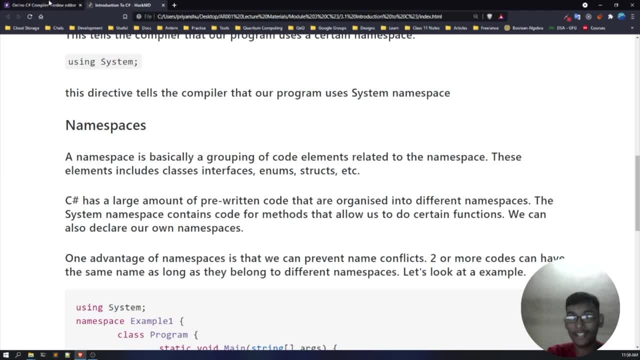 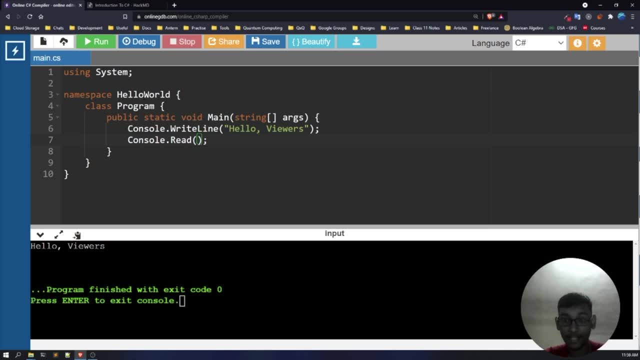 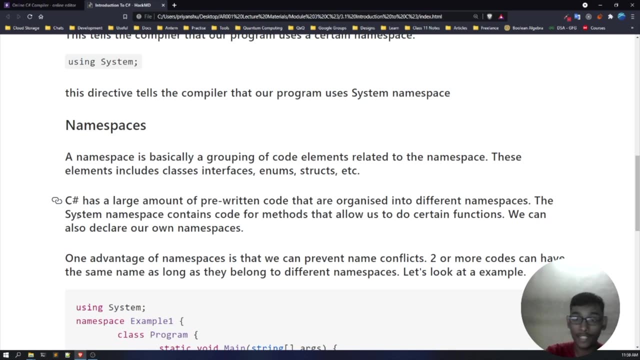 can include classes like see. currently, we only created our own namespace. this is our hello world namespace. it is containing a class, right, it is containing a class. it is containing a program class. so we certainly created our own namespace, right? we certainly created our own name space. so 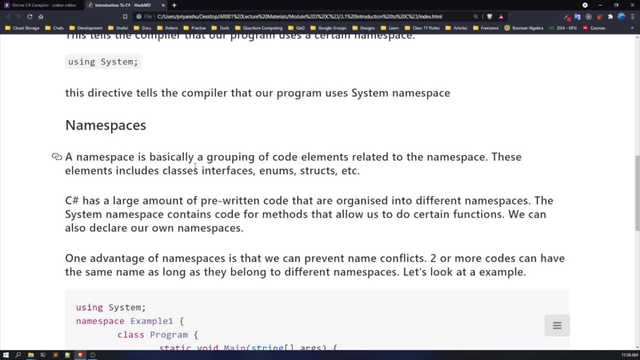 yeah, now we understood what our namespaces. all right. what our namespace says is: see and uh, if i have to repeat, namespaces are a collection of code elements. all right, it is basically a collection of code elements. it contains other classes, other interfaces, other, uh enums, other structure, uh structs. all right, so namespaces are a collection of those things. 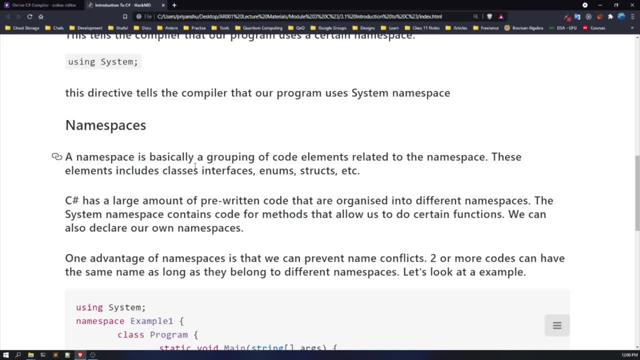 all right, see c sharp. our c sharp is a programming language, right? uh? c sharp has a large amount of code- all right, c sharp has a large amount of pre-written code that, like the team who developed c sharp, they already wrote code for us. all right, useful codes for us that we are using. all right, that we are. 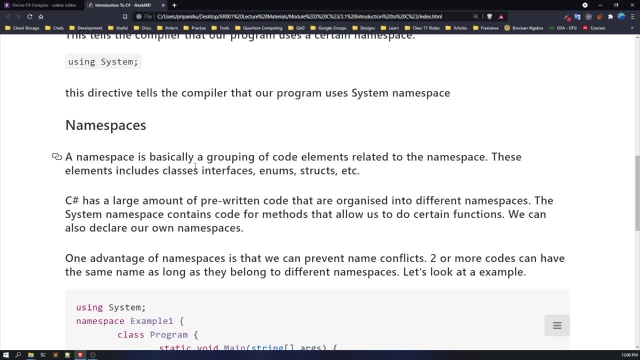 using. but can you, can you tell that if the programmers, if the programmers took all the those programs and just put, uh, put it in only one file, wouldn't it be cluttered up? like there are multiple hundreds, like hundreds, thousands code files, wouldn't it be cluttered up? and now, if i 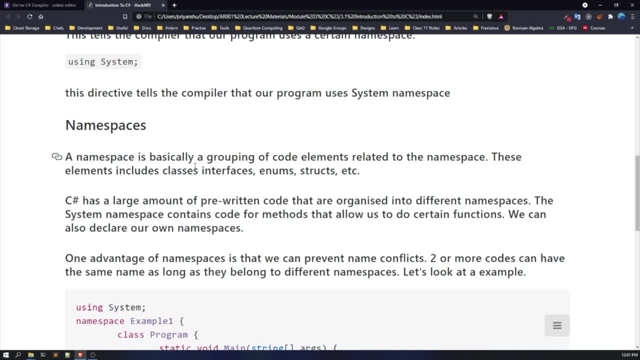 had to find one file, then wouldn't it be cluttered up? so what they did? they divided those pre-written code into different name spaces. all right, see, using system is not all, is not the only namespace available. all right, there are many other. all right, so yeah, so our code, the like. 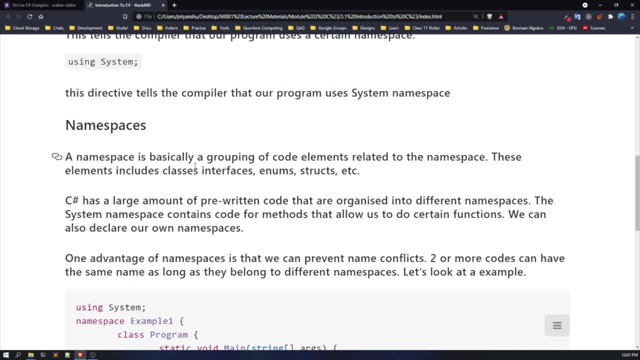 the C sharp, the developers who wrote C sharp, they- they actually divided all those code. all right, though. divided all those code into different namespaces, alright, the system namespace- all right, the system namespace that is available. it actually contains the codes. all right, codes for methods. that allows us to do. 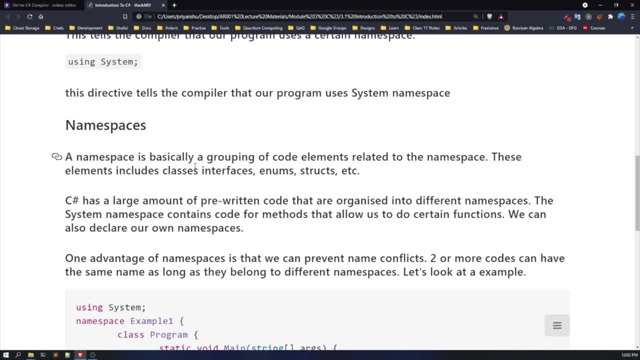 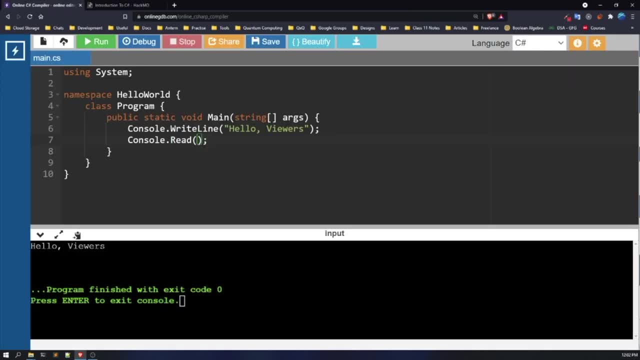 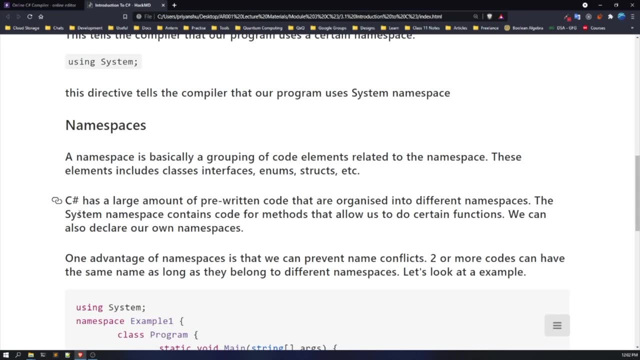 certain functions all right, like if we want to print, we can do that. so. or I already told that we can actually declare our own namespace. we even did. we even did: declared our own namespace. all right, we can copy this and create our another namespace. all right, I would show you how to do that and you know what are. 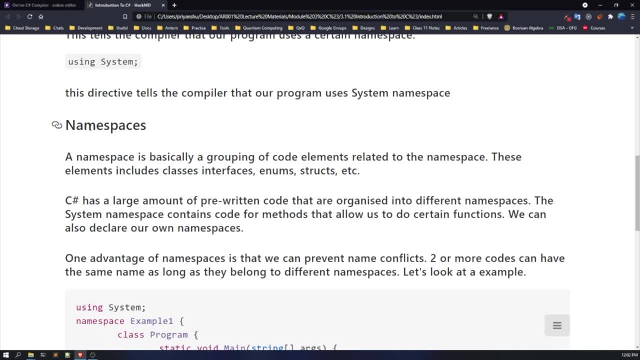 the advantages of using namespaces, right see. first of all, one more thing: if you are creating two or three or n numbers of namespaces, it is really important for you to name it differently. all right, the namings should not be same. so then, if the first name is: 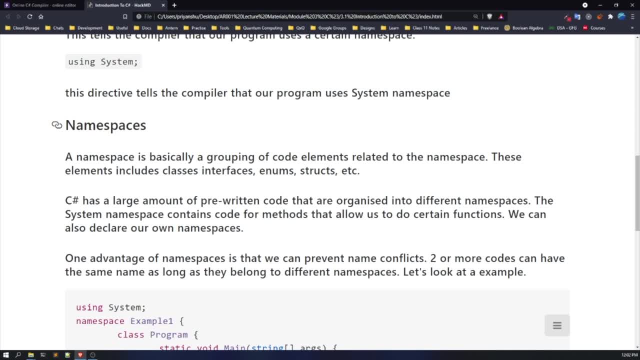 hello world, or I mean your first namespace name is hello world. the second namespace name should be hello Priyanshu or any other name, right, or your name. so remember that and one of the major things of like helpful things of namespaces are namespaces are two different environment. you could say all right in namespace one, see namespaces. 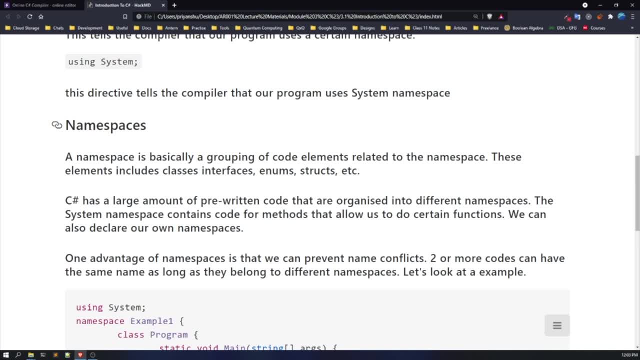 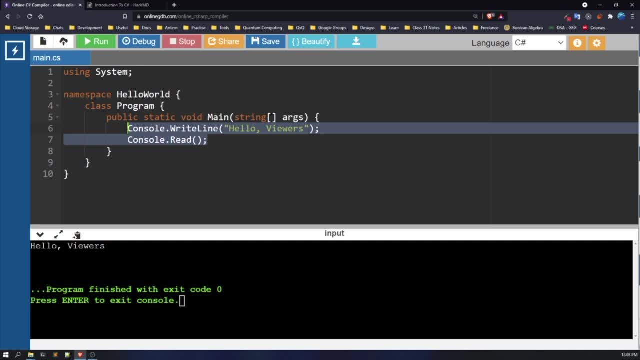 basically help us to prevent the conflicts, name conflicts like: see if we, if I show you here, all right, if I, if I create, if I, let's say, if I created a same type of variable. I know that you won't understand this as of now, all right, you won't understand this, all right, I'm. 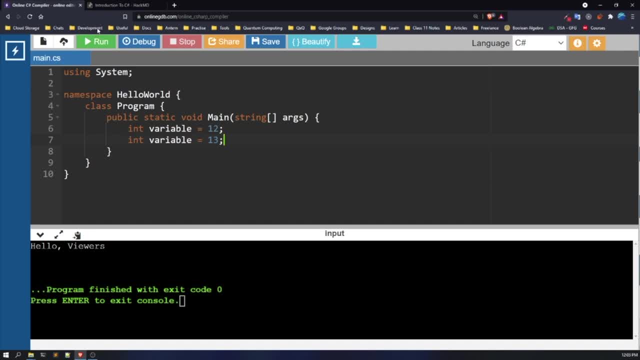 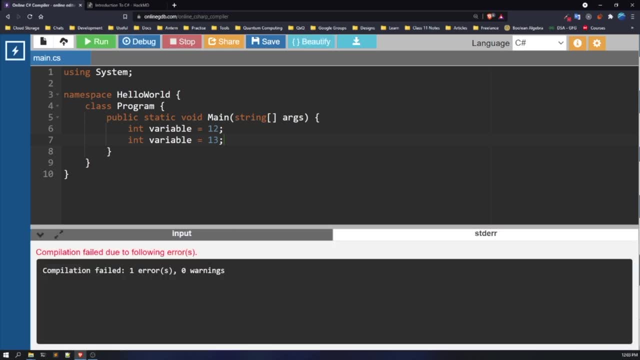 pretty sure about that, but don't worry. all right, don't worry, I'm going to cover about variables, comments and all those things. now let's play it. let's just play, see, see, it is giving us error. you know why it is giving us error: it is giving 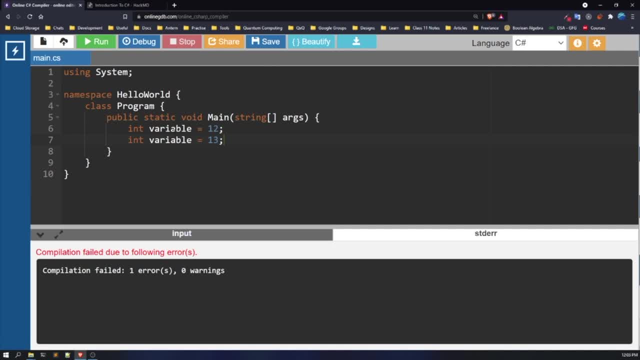 us error. the reason is that we are using at the same name, the same name, all right. so in you in C sharp, we can't use the same name. all right, we can't use. so it's really important to give different names, but. but, but if I had to show you, all right, 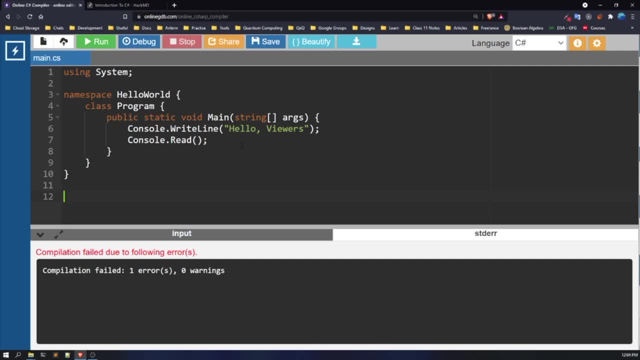 we can declare, we can give the same names in second namespace. all that, like this, is one of our namespace, right? so namespace hello Priyanshu. all right, this is a another. this is another name. says: I'm creating so class program. can you see? I'm givin the same name in here, right? the same name in here, now, now. 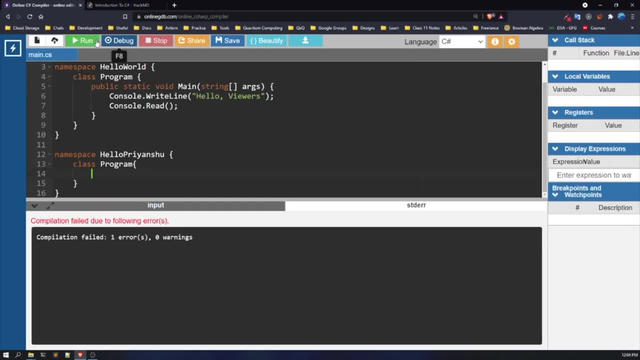 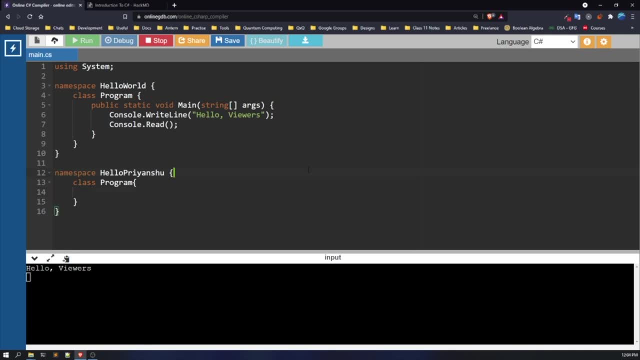 let's, let's try running it. man, let's try running it. see it didn't return. does any sort of era? didn't work because name spaces you can't think of. namespaces are different environments. actually they have the in there. if namespace one has program and namespace two has program the same names, then it won't conflict it. 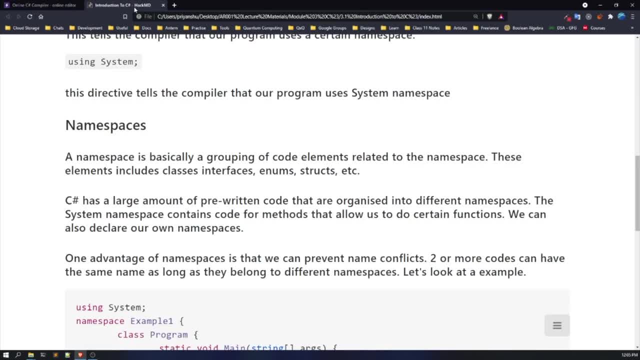 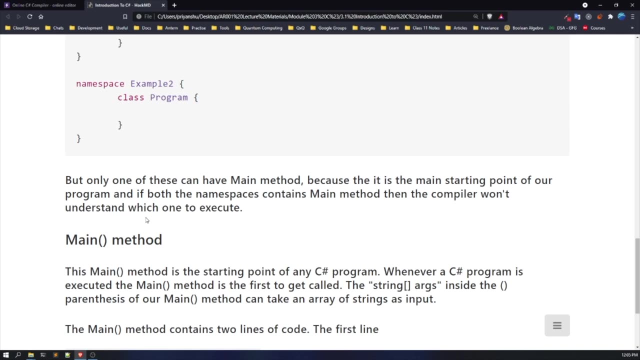 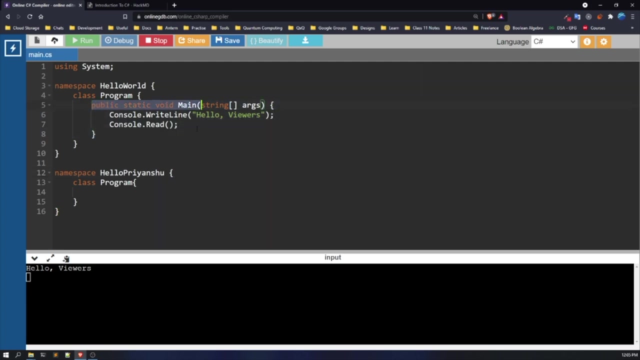 won't create any problem. so, yeah, I hope you understand, right, I hope you understood this thing now. we looked into the example, right, we looked into the example who? oh yeah, one more thing: I forgot to tell you that that this, this main method. alright, see, this main method, the main method you could see, this is 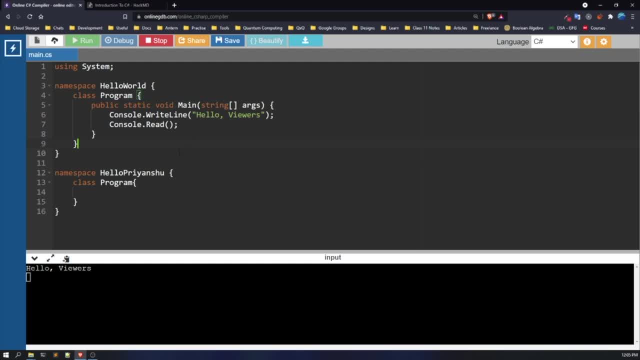 the starting point. alright, this is the starting point of our program. the main method is basically the starting point of a program. it's where our program starts. alright, if I, if I give the same thing, alright, let me copy this and put it in here. if I give the same thing in here, where it didn't got printed, 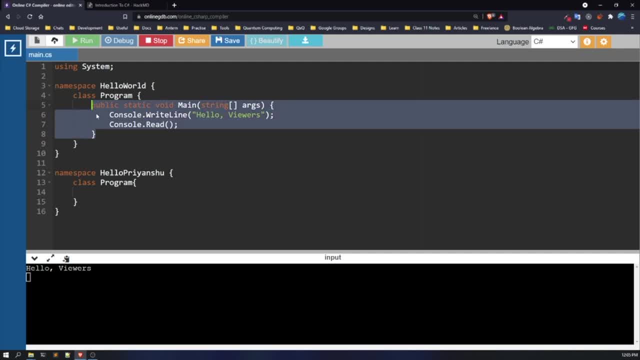 so, oh, why is it happening? wait, copy paste. all right, it isn't pasting, I don't know. oh, I got to know I didn't ended the program, right, sorry, I'm really sorry about that. I was like, oh god, now let's, let's try running this, and I'm sure you 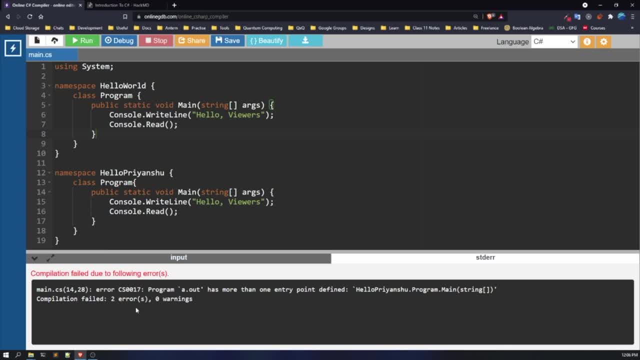 would get a see. it is giving us error. see visiting program. a dot out has more than one entry point defined. do you know what it means? it means that there are two entry points and main method is the entry point. so in our program, in a particular file, there should be only one method. alright, there should be only one. 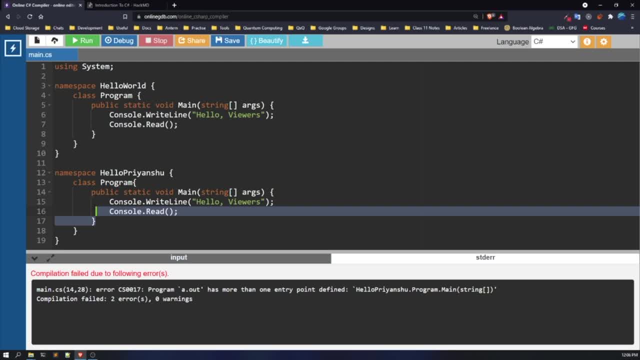 main method, because it is the starting point of our program, right? because if we have, if we give two main methods in two separate namespaces, then our compiler will be like: hey man, which, which main method should I go for? I'm confused, and because of that, and because of that, 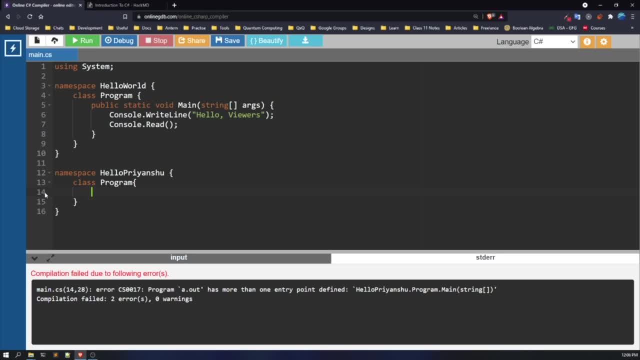 you. you are very rude to me. you gave me two main method. I'm really angry about that, so I will what I will give you. I will give you error and you won't be able to run your program, so our compiler will tell this. so to make our compiler 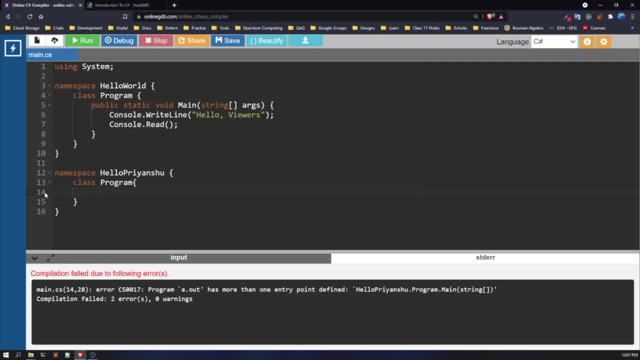 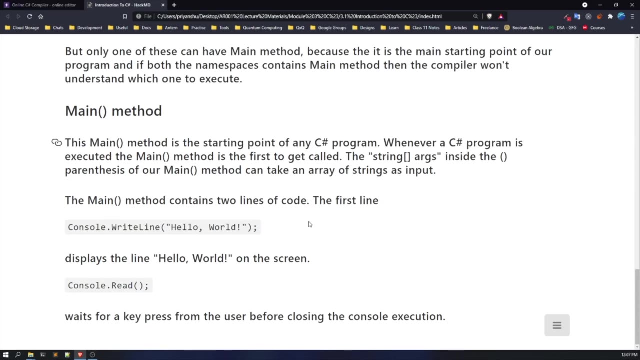 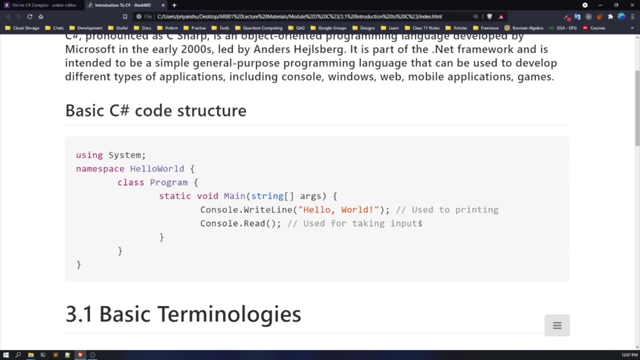 happy to make our compiler work fine. to make our program work fine, we need to provide only one main method in our, but in our, any in any of our namespace, all right, no, no, no, no, yeah, oh, ok, ok, I also forgot to tell you about these this: to write my bad, my bad. so what see you? 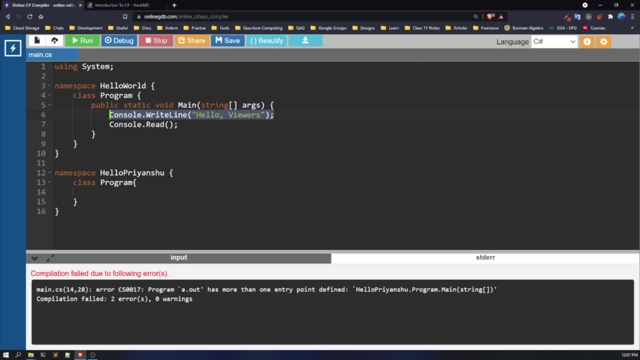 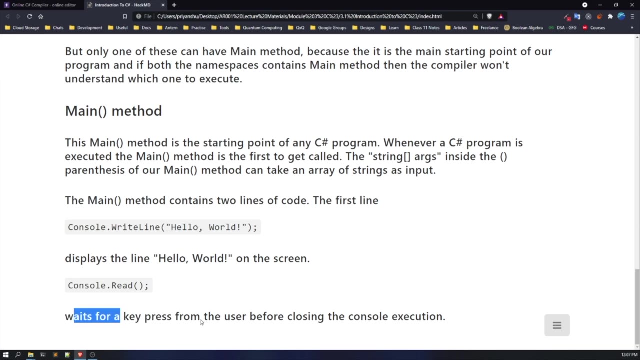 have already seen that what this console dot write line does this console dot write line basically print, all right. oh, this console dot write line prints a statement. but what? what this console dot read the read does? all right, i have written it in here. see, the console dot read: all right, it basically waits. 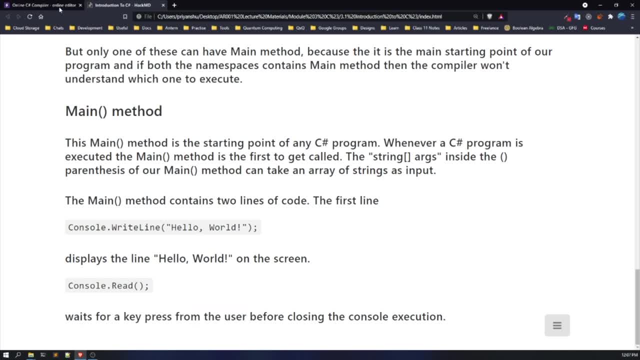 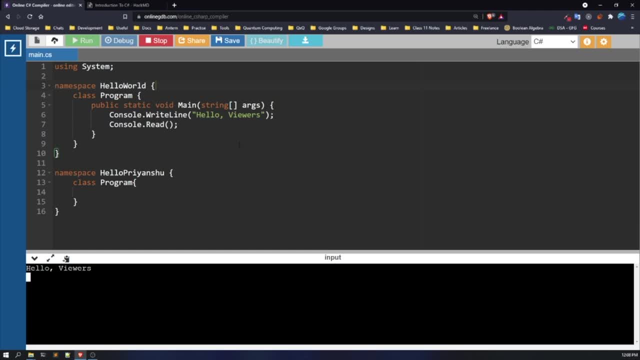 for a key press from the user before causing the console execution. like if i, if i execute, it all right, if i, if i let's say, execute, i will show you all right, i will show you. now, if i, let's say, i try doing something like editing this program, can you see you can't edit the source code when. 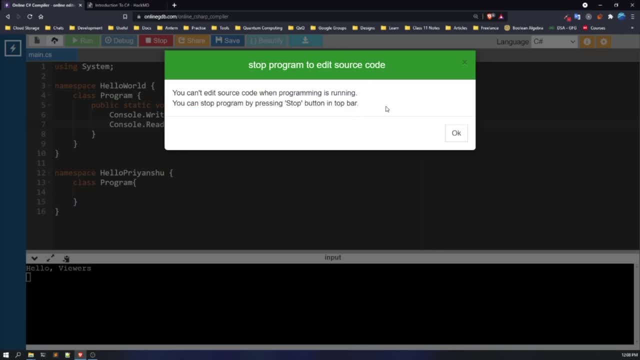 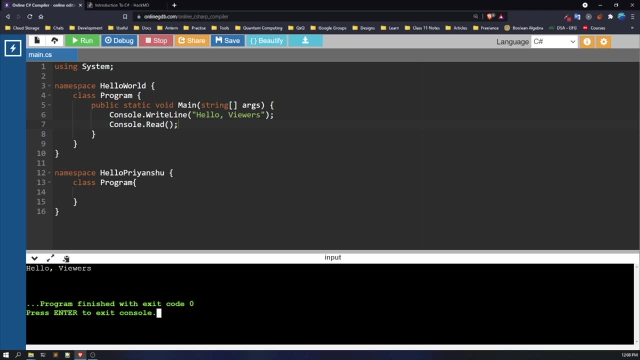 program is running. you can, you can't edit the source code. when program is running means our program is running. it hasn't ended. if i press enter, see our program ended. now if i, if i had to comment this down- i know you don't know about comments, don't worry- or let's say, i remove this. 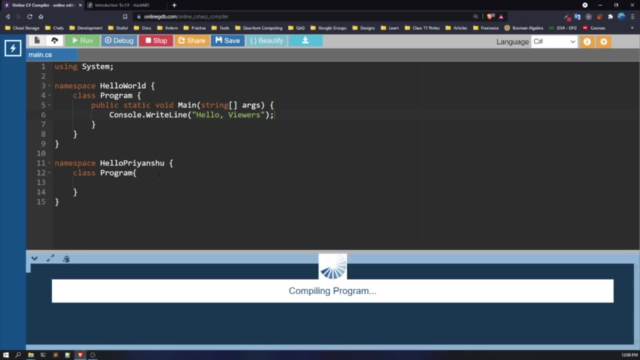 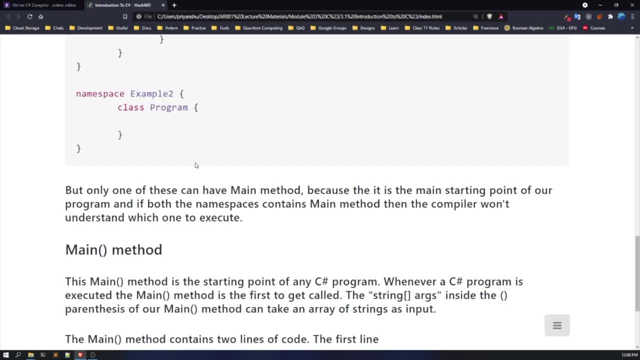 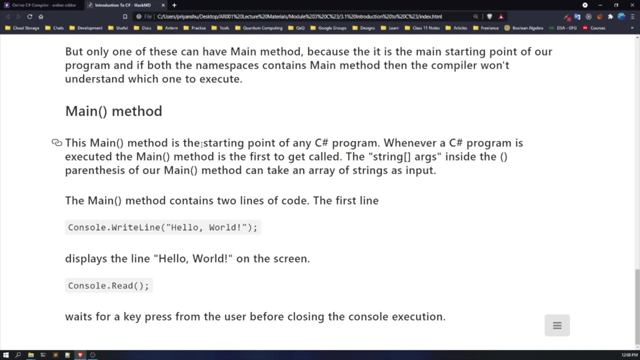 i'll remove this particular code line. all right, if i remove this. see, i didn't even need to press it, just exited. so that's what our console dot read does. all right, so let's, let's get- uh get- an idea about our main method. all right, so what is it? 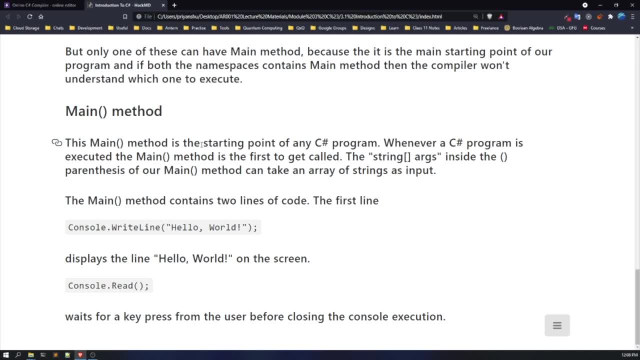 so see the main method in here. the main method is basically the starting point- all right, the starting point- of any of any of our c sharp program. all right, yeah, so our the main method, the main method in here. the main method here is our entry point or the starting point of our c. 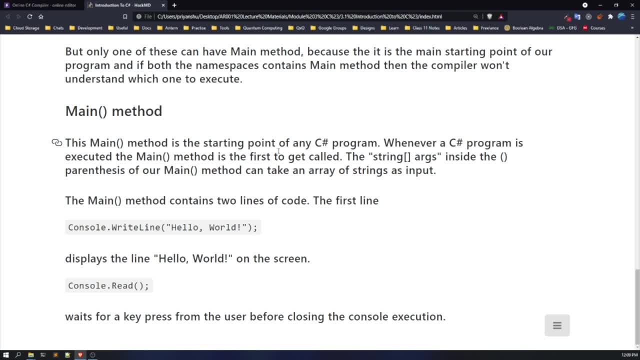 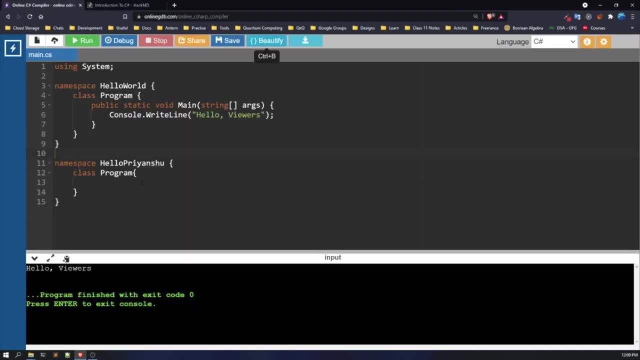 sharp program, right? uh, whenever, whenever we run a program, all right, why did? why did, when we saw the example where we like, added another, added another public static void, mean in in our second namespace, why didn't it ran? it didn't run because there should be only one entry point of the program. i already 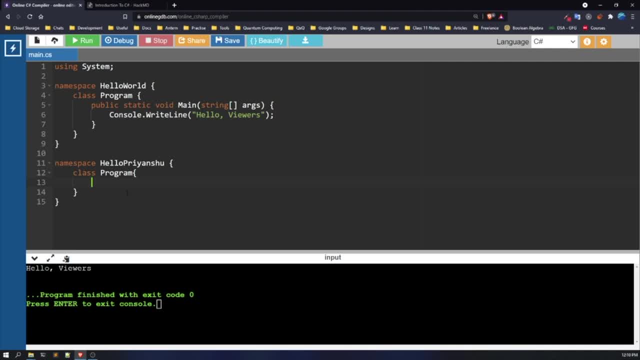 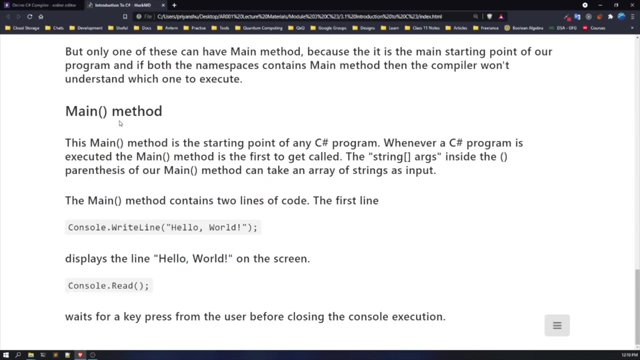 told you what would the compiler will feel if you give, uh, two entry points. right, the compiler will be angry. it will be an insult for him, i guess. so so, yeah, there should only be one entry point, all right, one main method. and also one thing: that these entry points are called first, all right than any other methods. 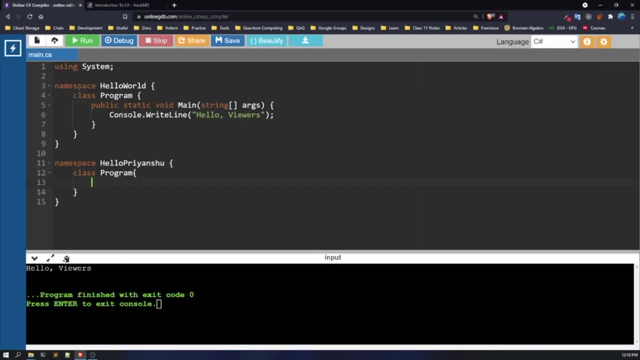 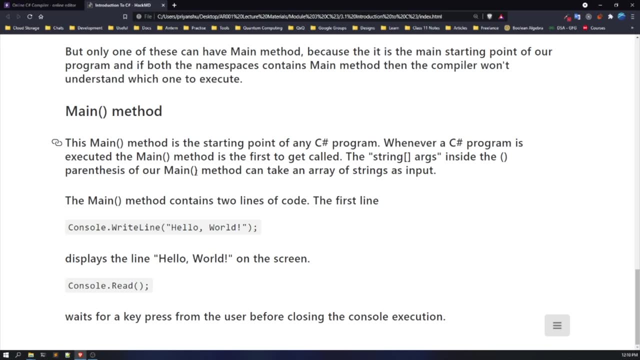 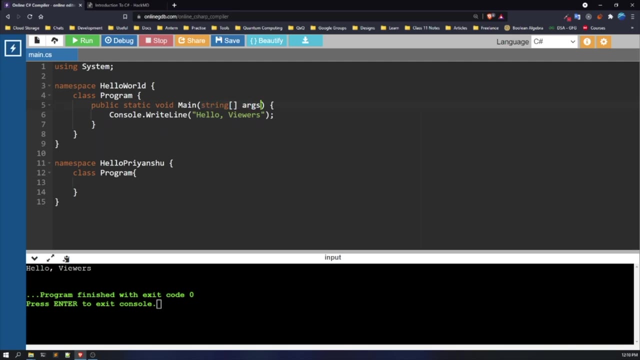 like, if you define any other methods, they won't be called first. the first thing that will be called is this main method, all right, i hope you understand. so yeah, there's another parameter, this string args. all right, if you don't know what a string is, man, don't worry, i am there now. i am there for you, i am. 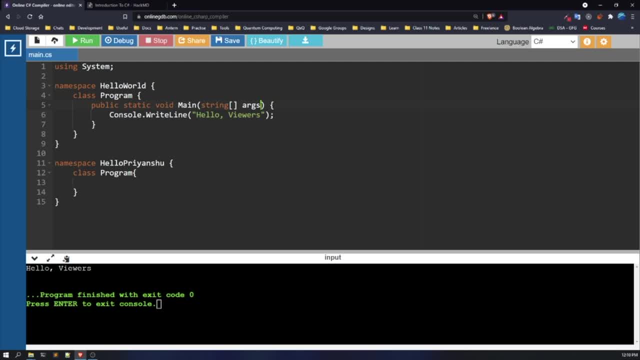 there for you to make you understand it is. i will make you understand this. uh, why? what is this string? args- all right. what is this string? right, this is an array. all right, this is a collection. it can take a collection of strings. all right, it can take a collection of string. if you're not able to. 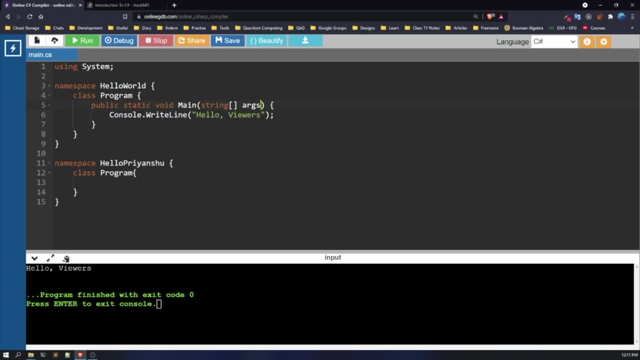 understand what is this, don't worry. next lecture is there, all right. next lecture is there for you. after that lecture, you will understand what it is, what it does, all right, and i will recapchulate it, recapchulate this particular portion in that, don't worry. so basically, it can take this this: 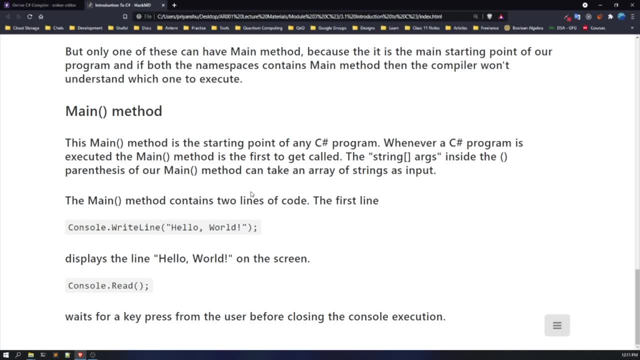 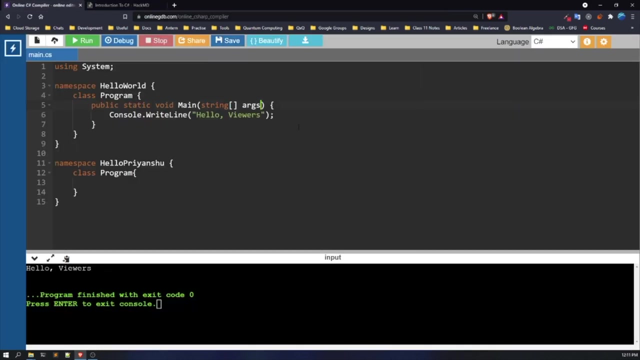 string method can take- sorry, the string argument can take multiple, multiple amounts of string data. right, and i already told you what this consolewrite line is and what this consoleread is. all right, so for the for today, for this lecture, our first first lecture is completed. all right, so our module three first lecture is done, all right. 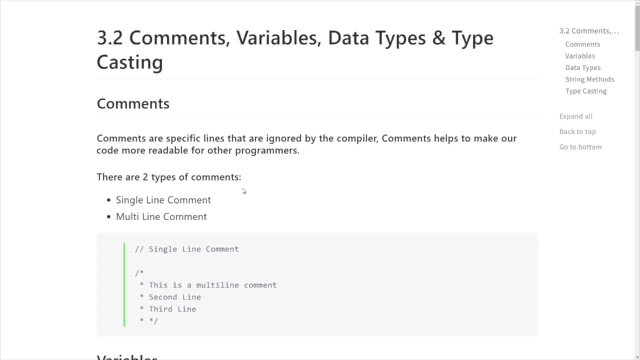 see ya, bye, bye, see you in the next lecture, thank you. so, hey, folks, uh, this is module 3.2, and in this module we are going to learn about comments, variables, data types and typecasting, all right, and in our previous module- that is 3.1- we learned about, uh, c-sharp, we learned the. 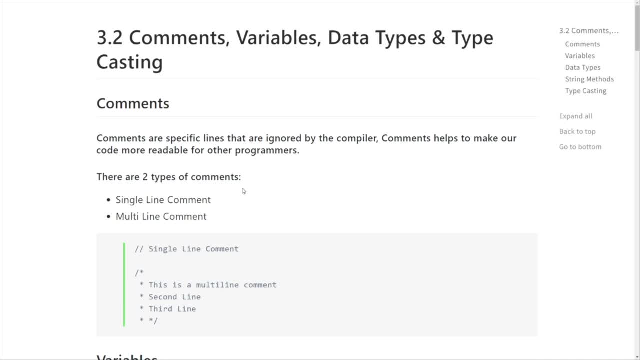 basic structure of c-sharp, all the very basics of means. what is the that using a system? what is, uh like? we learned a lot of things, all right. what is console dot right, line, right. so in this module we are going to learn about uh comments. then we are going to. 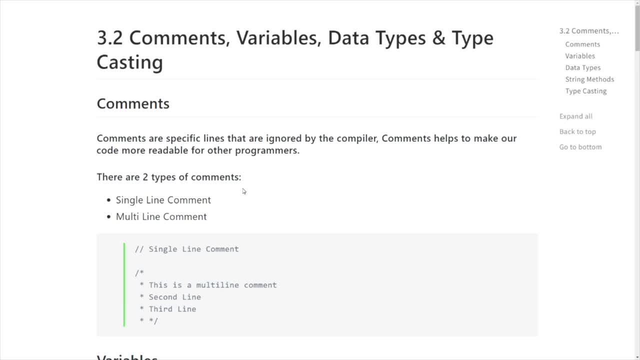 move on to variables, then data types and, last but not the least, and one of the important concept, that is, typecasting. all right, so, without any further ado, let's get started. so what are comments? all right, see, comments are basically, uh, some sort of statement, or you could say, some sort of 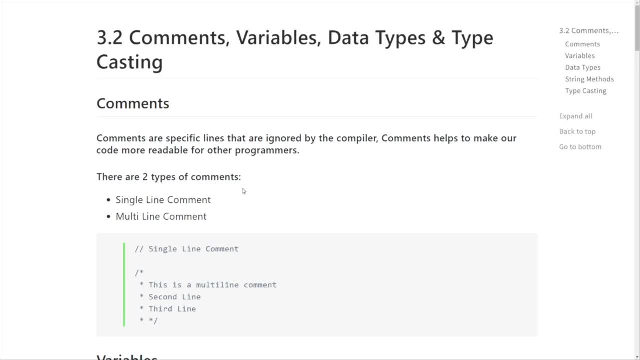 keywords or something like that. all right, it is some sort of specific lines that is ignored, all right, that is ignored by the compiler, all right. you already know what a compiler is. a compiler is: uh is a tool that uh converts the code to a binary form. right, that that is. or you can say: 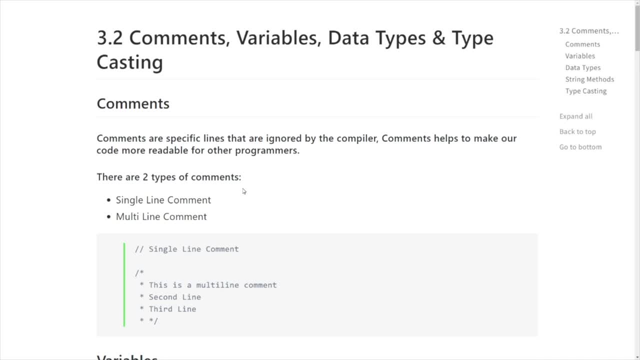 machine understandable code, right, uh, why it does that? it does that because, uh, machines cannot understand english, all right, it can't understand our words. machines can only understand binaries. that is zero and one, all right, so, yeah, uh. so what comments does is comments, uh, the comments, basically. all right, these comments. 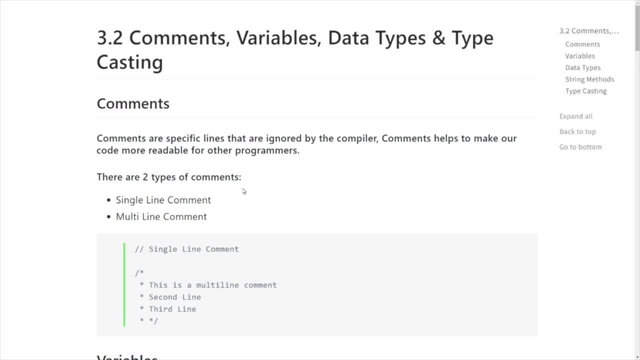 are basically ignored by the compiler. they, they won't run that particular line. all right, they, they will just ignore that that. yeah, it is a comment, all right, why should we run that? it's a you, it's a useless thing. all right for a compiler, for a compiler. 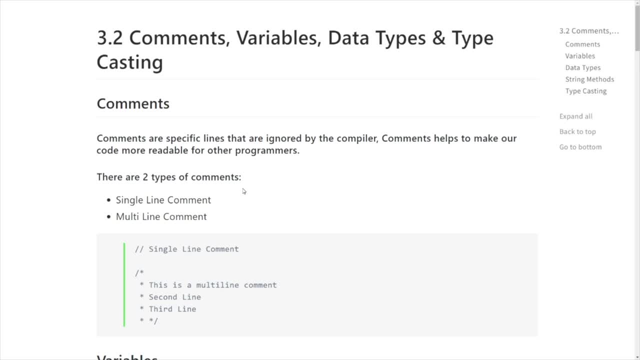 it is a useless thing. they won't run it because, uh, nothing will come out of that, right? so a comment is basically: uh, a comment is basically some, some sort of lines, all right, some sort of specific lines that are ignored by the compiler, all right. and how comments are useful, all right. 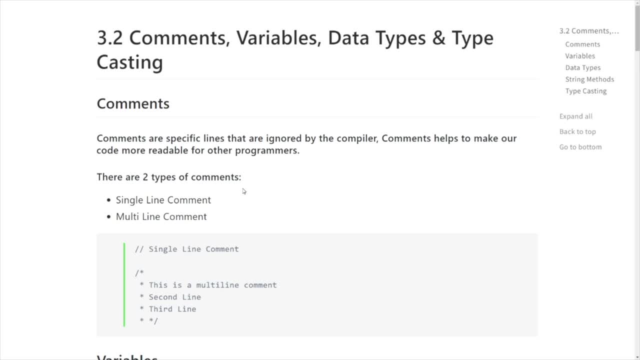 how comments are useful: see comments are useful in a in a way. all right, it is. uh, you have to make your comments useful, see comments are useful. see, uh, as a programmer, all right, we have to make our code understandable. all right, uh, because, let's say, i'm working on some project. 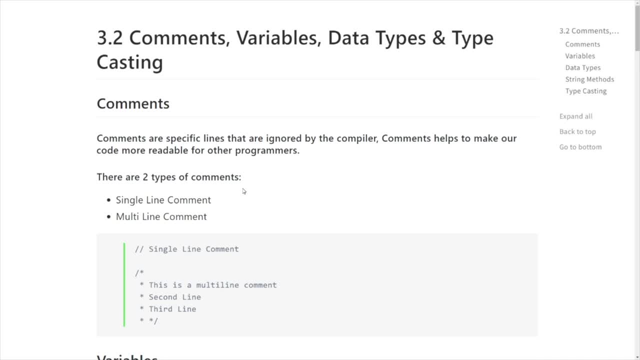 right now. all right, i'm working on some project and in that project, all right, uh, the code is of thousand lines, or two thousand lines, or let's say even, uh, hundred, two hundred lines. all right. now, uh, the code is being passed to another developer. he has to work on it, all right, without any proper 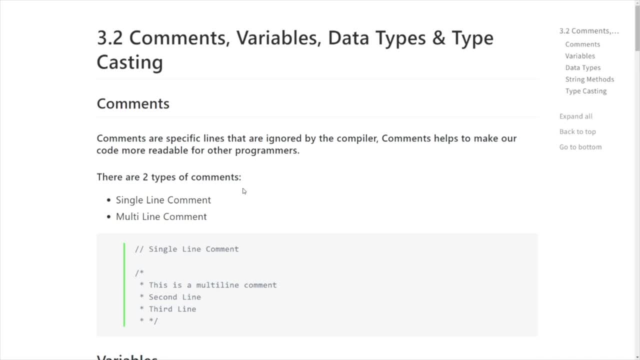 we can't. uh the the coder? all right, the new developer can't understand what that program is doing. all right, we have to, like, put a lot of time to understand the whole code. but we can make that thing easier. right, we can make that thing very simpler. we can comment. all right, we can. 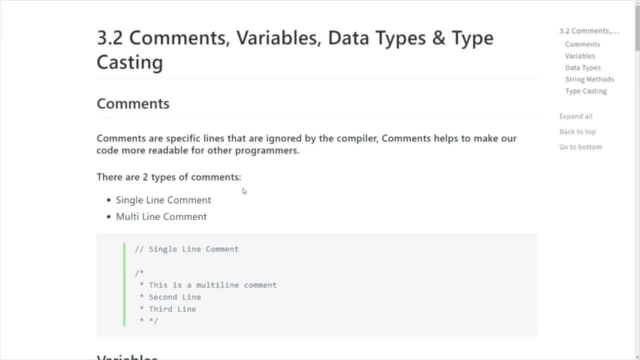 comment the lines. we can comment the lines. right, we can, means we can uh sort of create small, all right, small documents, or you could say small, small lines or small paragraphs. spot for that particular code. like let's say: uh, currently we are developing a ar app and in there we have to. 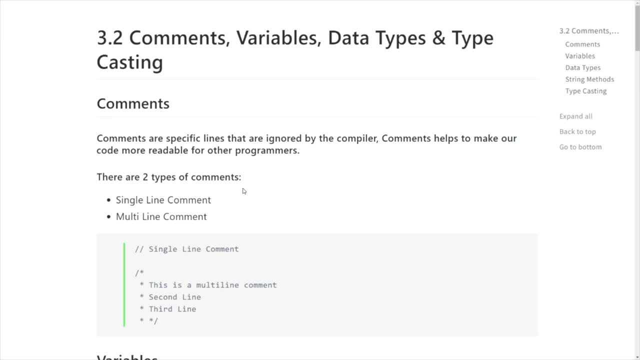 rotate. all right, we have to rotate that 3d model. right, we have to rotate that 3d model. so i i have written some code for that and in the top of that, all right, in the top of that code, what i did, i wrote a comment. all right, i wrote a comment that. 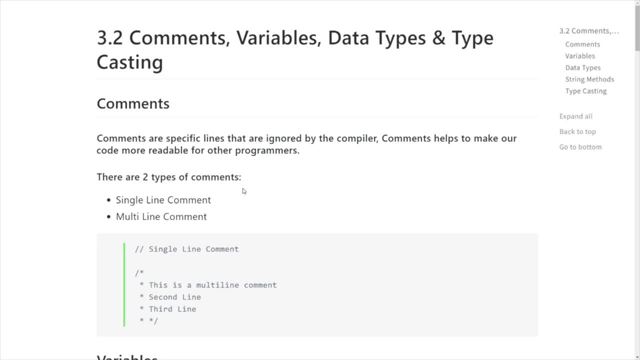 code. all right, this particular code is rotating the 3d game object. all right, it is. it is rotating the object, all right. so if I am passing the code to another developer, then he won't have any problem understanding the code. all right, he won't have any problem. so that's why comments are useful. all right, now let's. 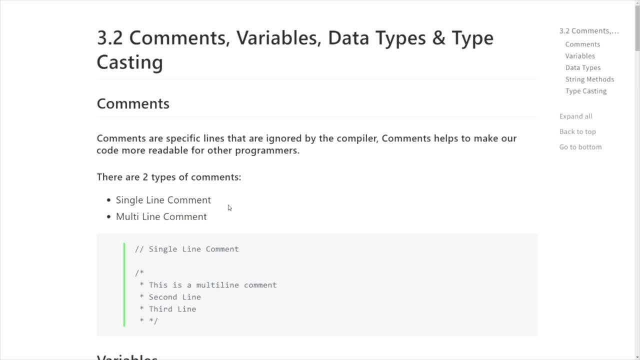 let's try this out. and also, there are actually two types of comment: all right, single line comment and multi-line comment. so what is a single line? all right, single line comments works for only single lines, like if the line is one, then it will be within line one only, or it will, if you are not understanding. 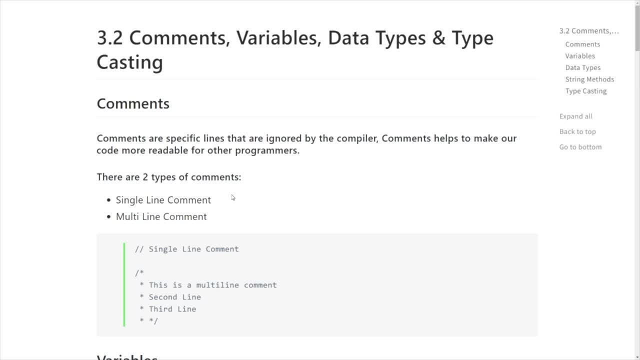 that, don't worry, you are going to do the practically all right. so single line comments are basically: they stay in one line already. all right, if you, if you go to the next line, that comment won't work. all right, that comment won't extend, actually. but this is not the case of with multi-line comment, all right. 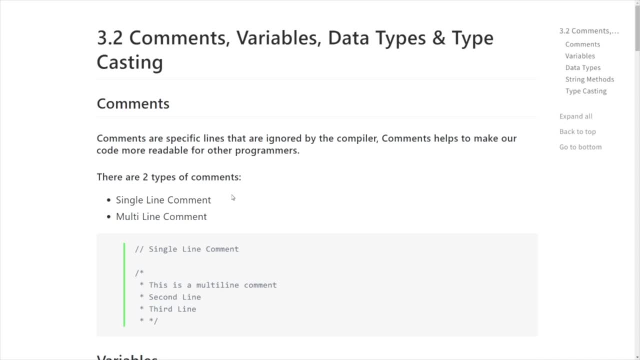 multi-line comment can help us in documenting also. so multi-line comments starts from a particular point. or let's say we are starting that multi-line comment from line number three, all right, and we are writing some multi lines, all right. we are letting some text within that comment, all right, in separate, separate. 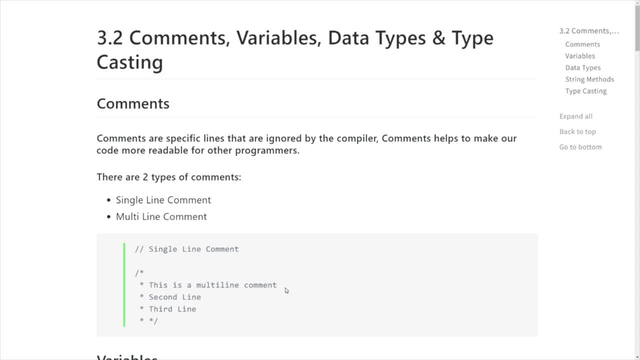 lines, like you can see right in here. all right, right, like you can see right in here, we have taken three lines to write some content, and in the in the fifth line. all right, we are ending it in the fifth line, we are ending it, so that's. 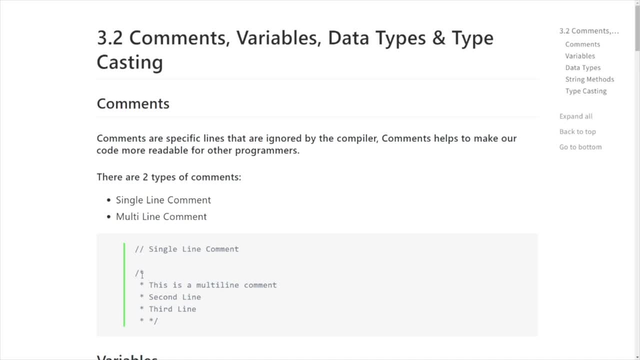 how we start a single multi-line comment, all right. so to start a single line comment, we have to give double forward slash, all right. and to write a multi line comment, all right. there are two things: a starting point and an ending point, all right. the starting point is like forward slash star, it is the start. 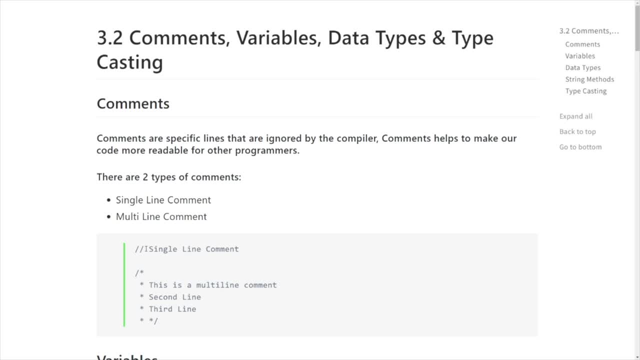 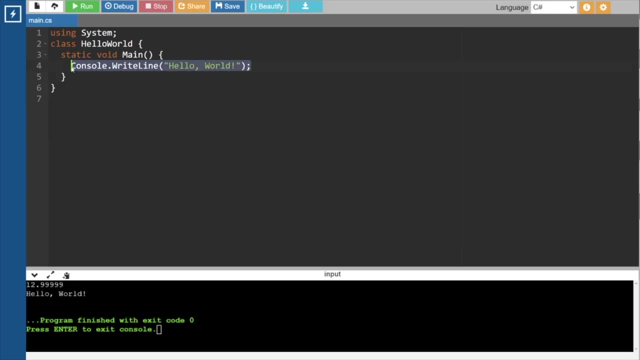 of the comment and to end that comment, what we have to do is start backward slash. all right, I hope you understand, right? so let's try this thing out right before going to variable. let's try this thing out. all right, so this is our code. all right? so first of all, let's write some sort of code. all right, let's write. 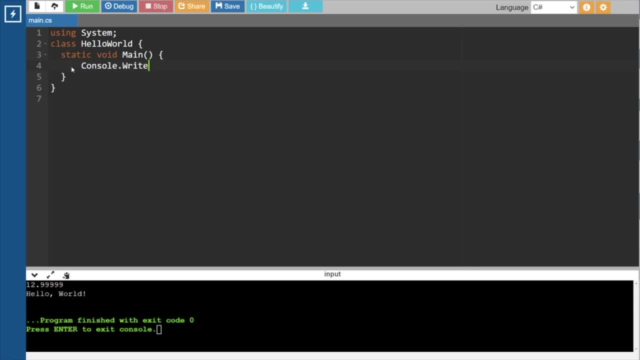 console dot- write line comments. all right, so this is our code right now. let's try to run it. let's run. run this program. see, it is printing comments, right. let's let's try to give the single line comment notation. all right, see after I have given to forward. 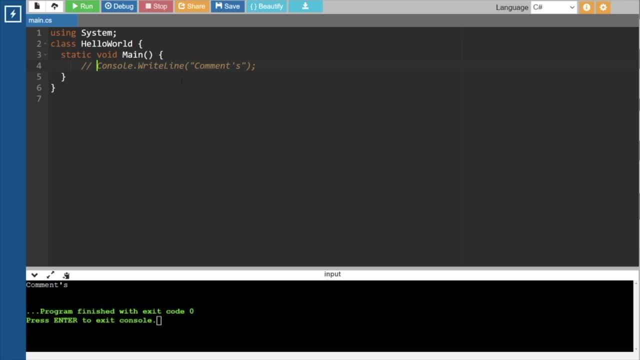 slash, you can see the whole line has gone brown. what does this indicate? this indicates that this is a commented line. all right, this is a commenting, commented line, although the color will will be different in your editor if you are using some other kind of editor. all right, because this is the theme of it. 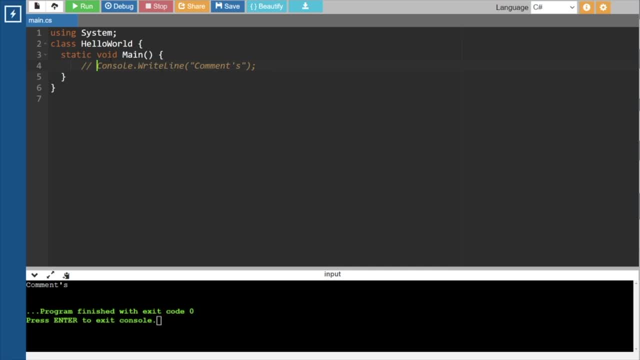 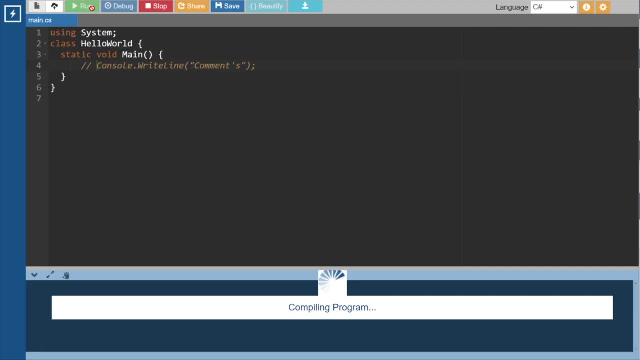 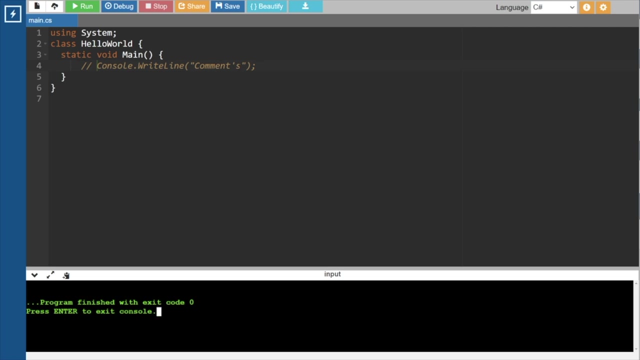 but don't worry about the color, but it is highlighted, all right, when it is highlighted you are, you will understand that your code is committed, commented. so let's run. run it. all right, let's run it. see, it is not printing anything because it is not reading the line it. the compiler is just ignoring this particular line, all. 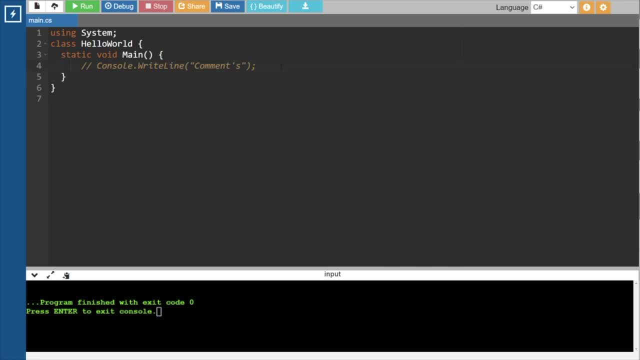 right now, let's try out something. another thing. can we add another line of code in the same same single line comment, can we? so let's try it out. why not try to try it out? right, let's try it out and see. so line two: all right, so 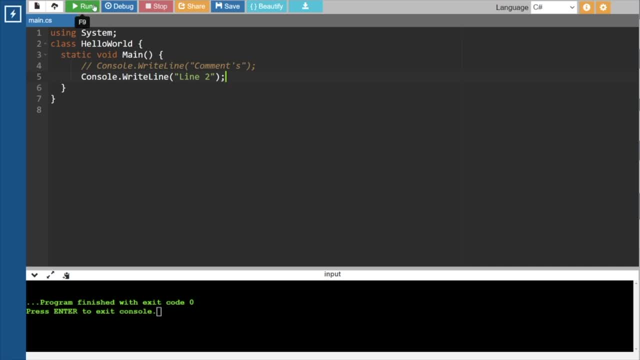 let's try it out. let's see that the single line comment is also ignoring the next one, or not? oh no, it is not ignoring the next line. okay, do you know what? what is the reason? the reason it? it works for only one line. all right, if we. 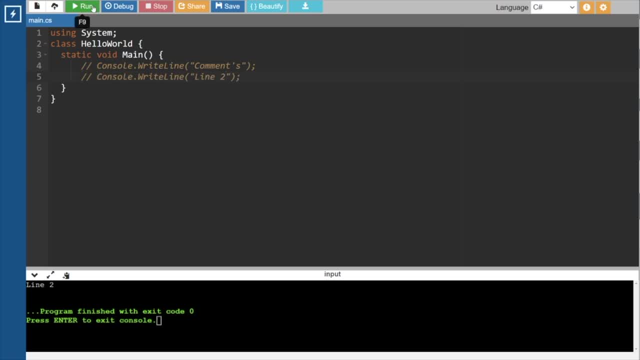 if we give another set of forward slashes in line to comment, that means in the consolewrite, line, line two, then again it would perform its function all right. but it is also like it's it is. the task is also tedious to give every time. uh, the double slashes, right, double forward slashes. so there's another thing. all right. 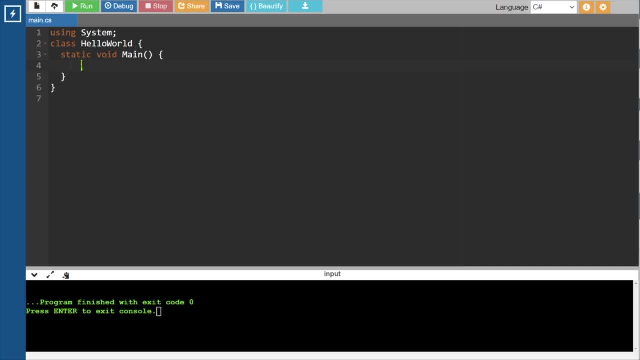 let's say we want to give uh. let's say we want to uh write multi-line comment, all right. or you could say we want to uh like write multi-line things, right. so first of all, let's give console dot right line comments, all right, console dot right line. 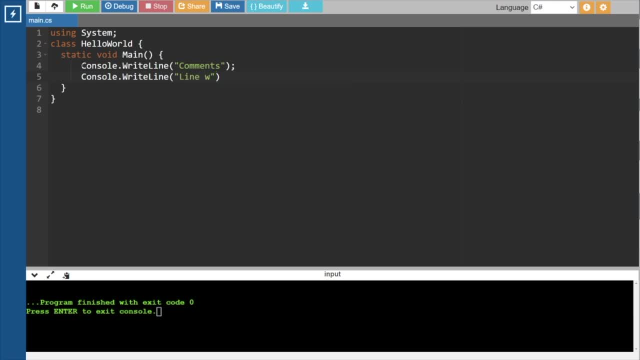 line two: all right, uh, line two again. uh, console dot. uh right, line line three: all right. so let's try it out. all right, let's try it out. uh, let's run it see, uh, the code is running. but we don't want the code to run, we want to comment it, all right. 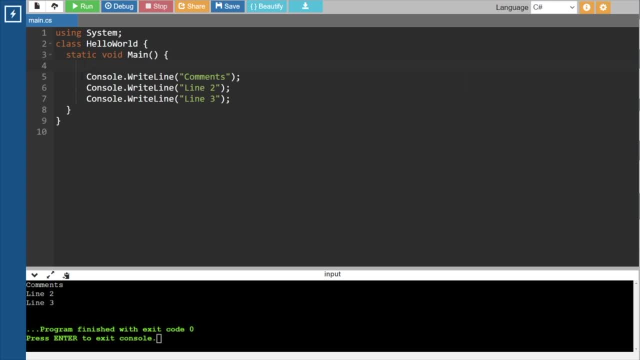 we want the compiler to ignore it. so how would we do that? all right, so simply give forward, slash and star. all right, see, uh, as you can see here, just as I have give as soon as I uh gave this comment, uh, comment notation, multi-line comment: uh, starting point. all right, you. 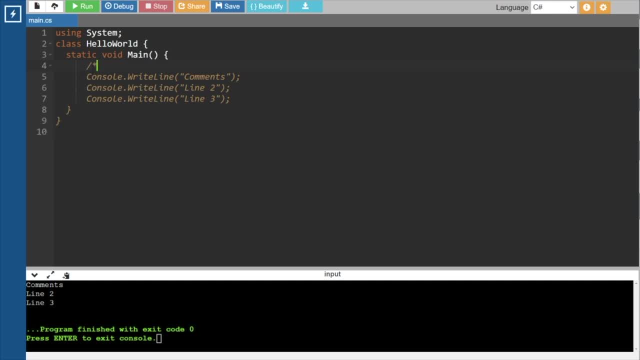 can see it has highlighted, all right, or made the colors brown from where it started. all right, uh, now we have to end it. how would we do that? so it's. it's again as simple as that. just star forward, slash, all right, and you can see the uh commented portion is only brown. 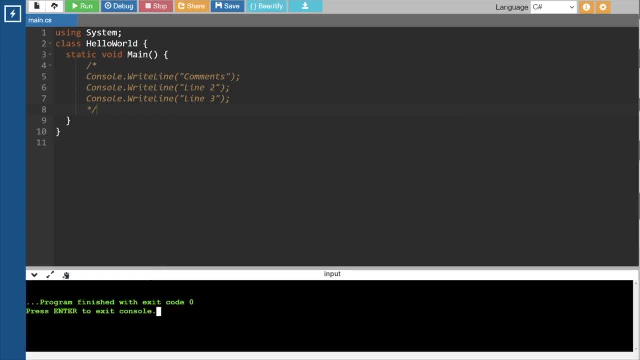 right, let's run it. see, uh, the compiler is ignoring the codes. it is as simple as that. so I hope you understood. what are comments? all right? comments are basically, uh, some set of lines, all right, that are ignored by the compiler. that's it, all right. so now, as we have understood, 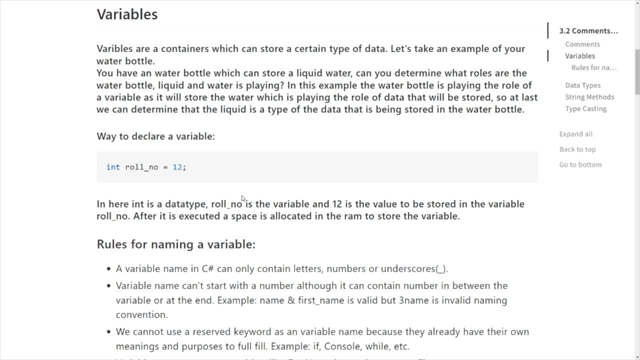 the comments. let's- uh, let's- go for variables. all right, see, variables are, uh, you can see, variables are used to store some value. all right, variables, in a programming language, are used to store some value. right, so to see, I won't be using any technical terms to make you understand about. 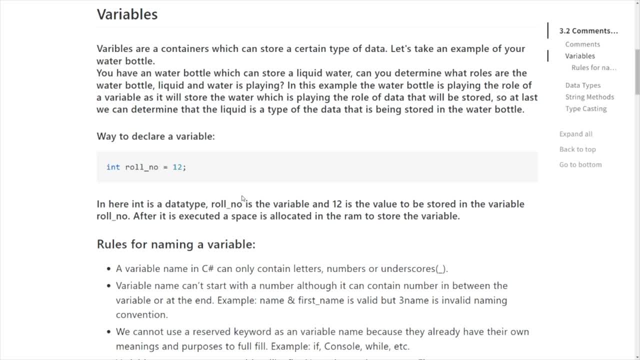 variables, all right. uh, I would be using a layman's term, all right, or you can say the simple term to make you understand about variables: all right. so, first of all, first of all, think the variable as some sort of container. all right, a container that can store something. all right, let's say: 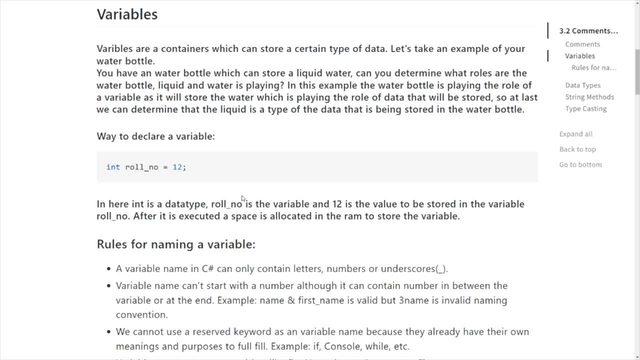 let's take a common container. all right. let's say, let's say a water bottle. all right, take a. taken water bottle. all right, taken water bottle. it is a variable, all right. for now, think your variable as a water bottle, all right. and you are storing, all right, something in it. all right, what thing? what is? 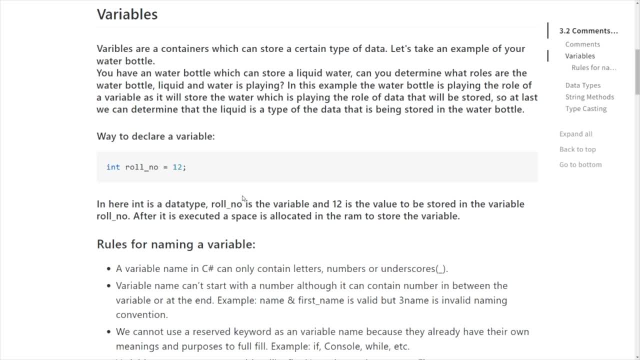 that thing that you are storing in that water bottle. it is all right. it is a liquid, all right. in a water bottle you will store some, some kind of liquid. doesn't matter what kind of liquid, it is all right. it can be a orange juice or chocolate milkshake or a simple water, right, all it is a. 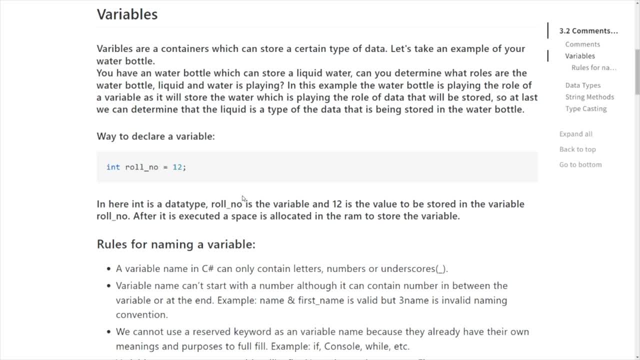 liquid, all right, doesn't matter what what liquid it is, but it is a liquid right in the water bottle. you are storing some kind of liquid, all right. and what liquid are you storing? all right? what is the liquid means? is it water, is it an orange juice or is it a chocolate milkshake? so i want to store a chocolate milkshake in the 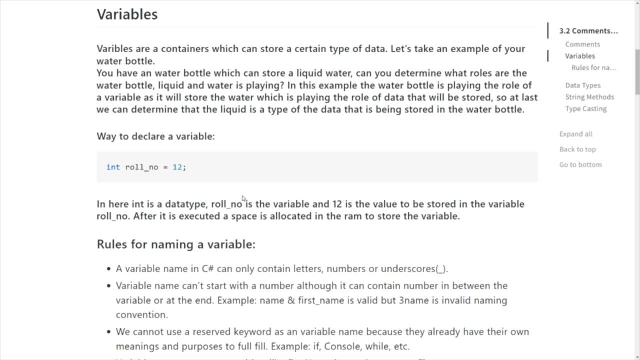 water bottle, right, or even a simple water. i can store water in the water bottle, so you can, you can imagine all right, you can. you can interpret this, uh, in technical terms, how see the water bottle is acting like a variable, or you can say a container, because 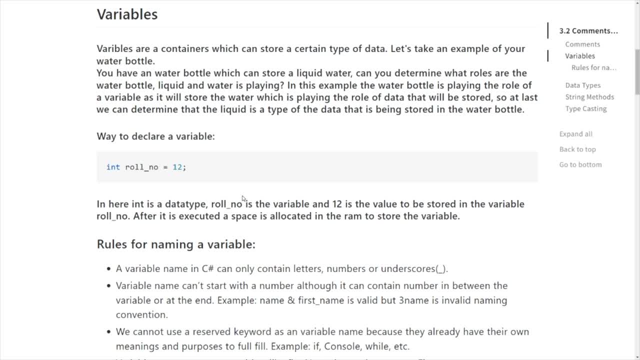 variables are containers. variables are meant to store some value, right. variables are meant to store some value, all right. so variables are container and in our example, a variable is our water bottle- all right, water bottle is our variable, all right. and the uh, and we are storing some sort of liquid in here. the liquid is the type, all right, liquid is the type of the data we are. 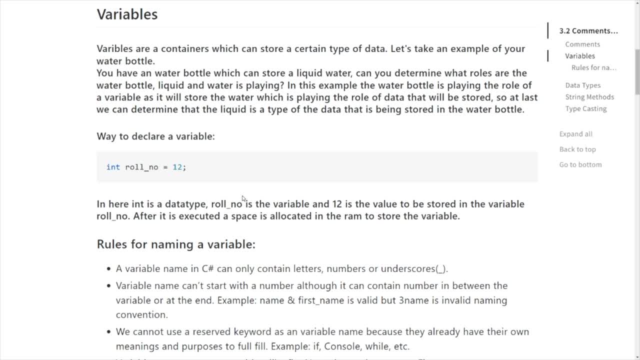 storing. all right, see, water comes in the type of liquid, right. we all know that chocolate milkshake also comes under the type liquid, because it is liquid, of course. uh, then orange juice also comes under the type of liquid, right. so we are storing some kind of liquid in here and we are storing some. 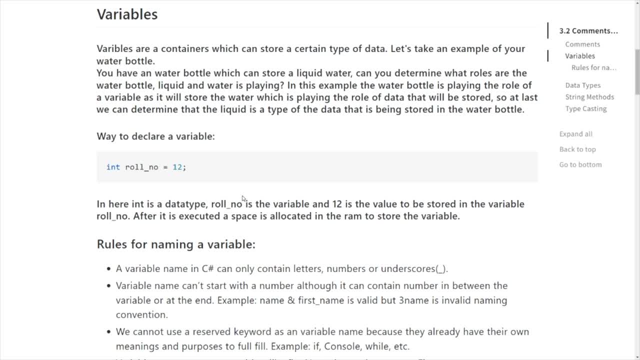 kind of liquid. so that is a type. or you can also say data type. right, we can also say data type. right, it is the data type, right? so water bottle is our variable, uh, liquid is our data type. and and the type of liquid you are storing? all right, the type of liquid you are storing, that is. 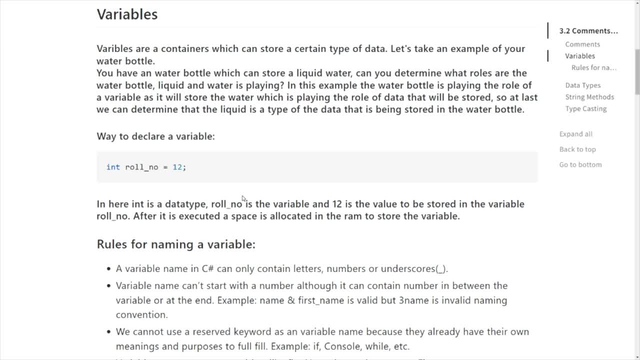 water, or, let's say, chocolate, milkshake. that is the data. all right, that is the data we are storing in our variable, all right? or you can say in our water bottle. so we are taking our water bottle, all right, we are taking some sort of liquid. all right, some sort of liquid is the uh, chocolate. 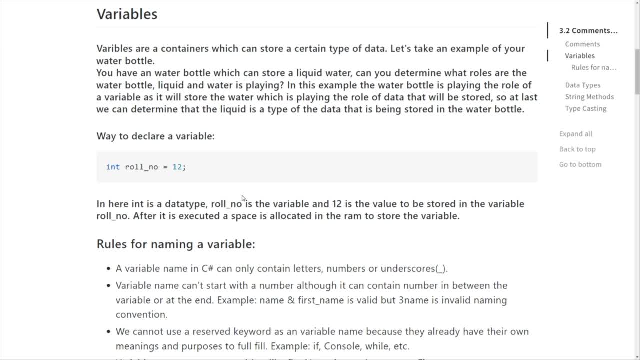 milkshake. i am storing my chocolate milkshake in the water bottle, all right, and the type of the chocolate milkshake is liquid, all right. so i hope you understand. so variables are basically containers. they are containers, but in computer programming. all right, they are containers in computer programming, right? so let's uh, to make you and make, make it more understandable, let me show. 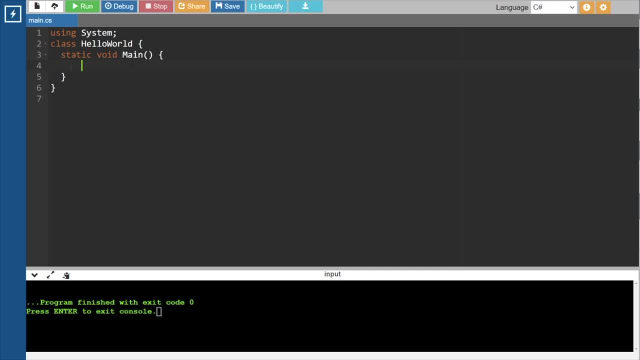 you all right. see, this won't execute. of course, this will give you error, but let me tell you: all right. so this is the type. all right, liquid is the type. water bottle, water bottle: right, water bottle is our uh container. all right, water bottle is our container and the data we are storing in it. all right. the 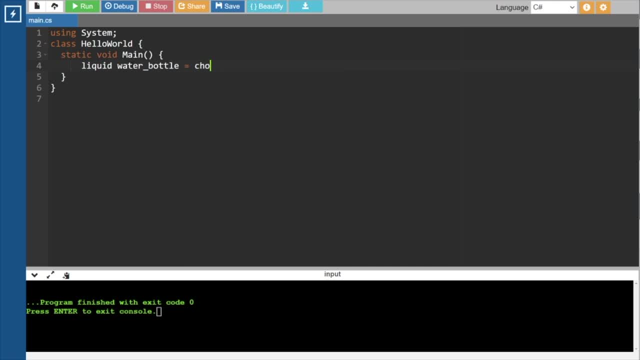 data we are storing in is: is chocolate milkshake, right? so yeah, here you can see. this liquid is the data type, all right, this liquid is the type, this water bottle is the container and this choco milkshake, all right, is our data. this choco milkshake is our. 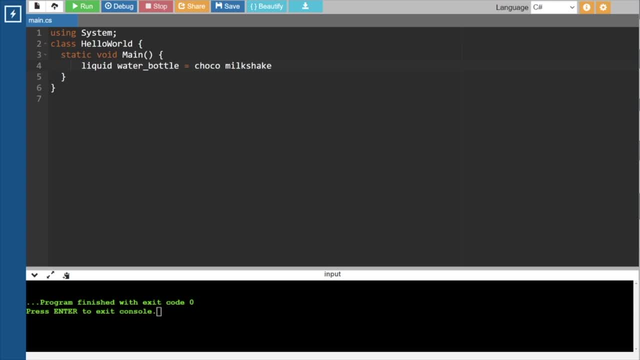 data. all right, and this is how. all right, this is how we initialize. all right, or create a variable in our c sharp programming. all right, this is how we create variable in many other programming languages too, like java, c, plus, plus. so let's uh write a comment for it. all right, that is data type. 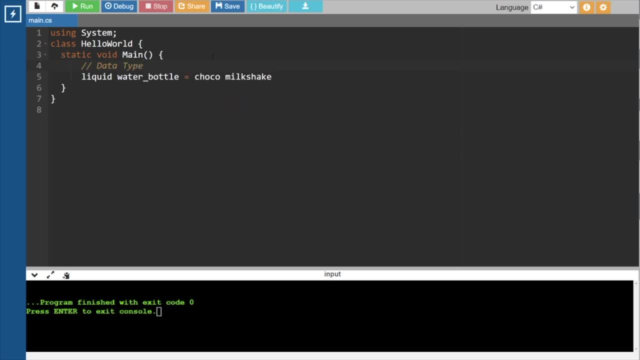 data type, then we have to uh, give the variable name right variable name, then we have to initialize the data to it. so this is how it works, right. or you can say: if i remove this data only, let's say: type: variable equals data. as simple as that, nothing too complicated. all right, so we are. 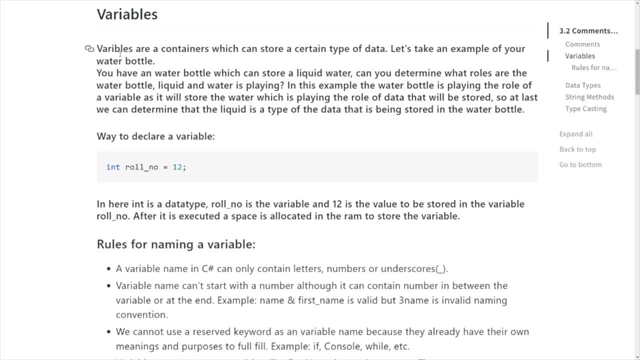 storing chocolate milkshake in our water bottle. all right, and what type of, uh, chocolate milkshake it is? it is a liquid. all right, it is a liquid, so that's it right. this is what variable is a container? nothing else. so i already show you how to like what is the way of declaring a container. 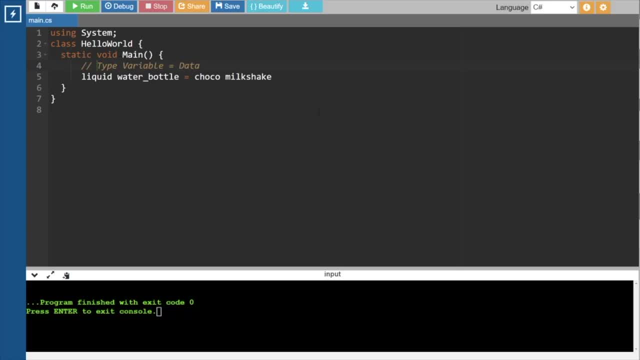 right now, let's try it out. all right, let's. let's try, uh, actually initializing a variable. right, let's try out initializing a variable in in computing terms. all right, not in layman's term. so it's simple. first we have to give the type, or you can say data type. then we have to write the. 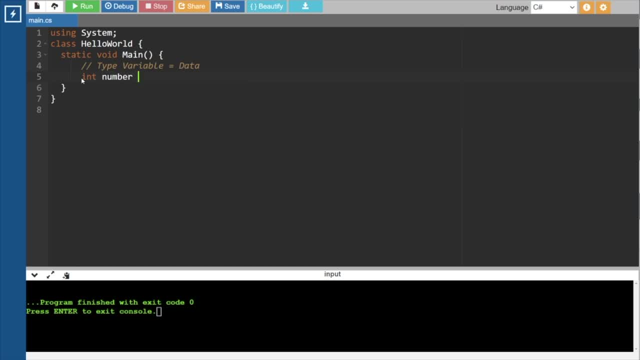 name of the variable. all right, let's say data type, and then we have to write the name of the variable. let's say i want to store a number, all right, then we have to uh use the equals operator, also known as assignment operator. all right, and we have to assign. all right, we have to put some sort of data. 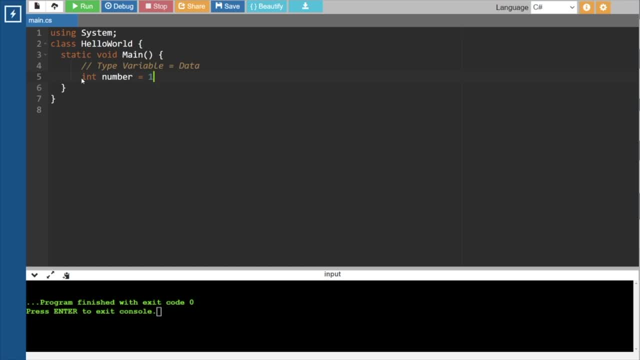 in our case. in this case, the data will be numbers, so i'm trying going to put 12 in here, all right, and let's say it works or not. so i'm going. what i'm going to do is i'm going to print it out, right, i am simply going to. 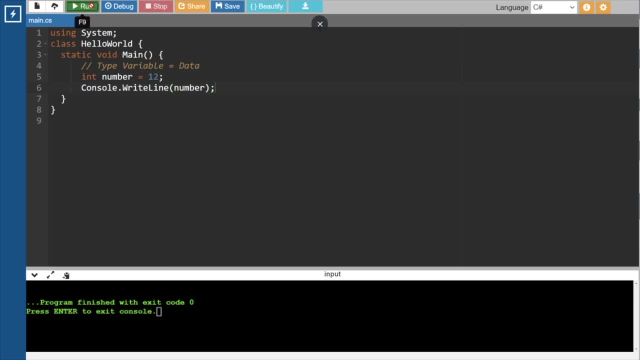 print this thing out. let's see what happens. yeah, so it has printed our number that we stored in a variable, right? so we created a variable that is storing the value, right? so that's great. it's a good start, actually. so we learned what is a variable. all right, we 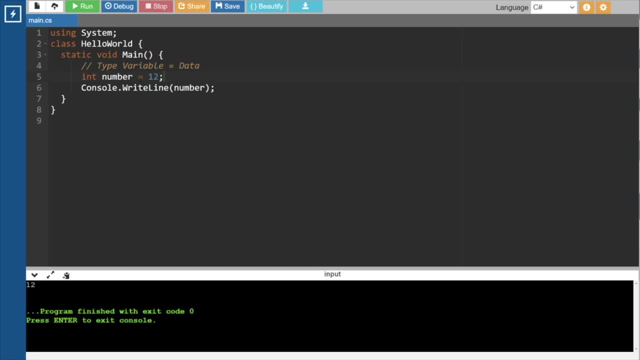 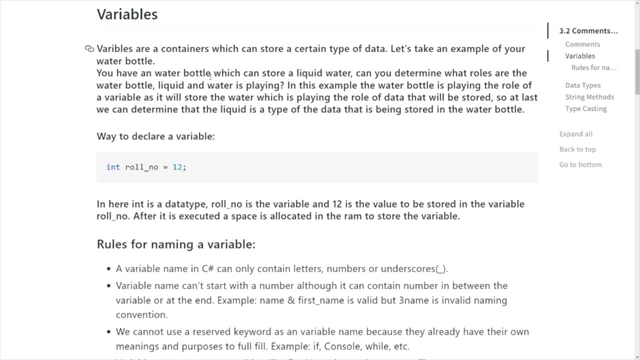 learned what is a variable, how to create a variable. one more thing i would like to say is now you, many of you, might have a question- that we are creating a variable, right, like: uh, where do we store our water bottle? all right, we can. we store our water bottle in our backpack, all right, or? 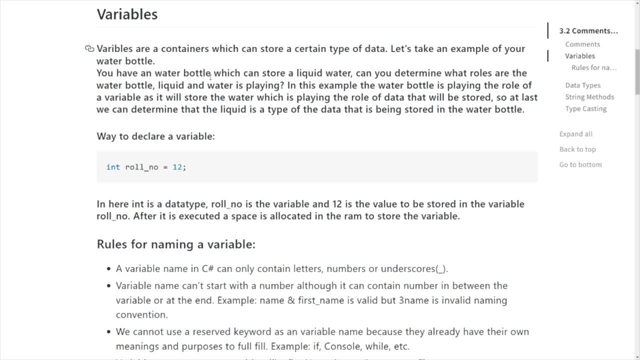 in in some place at our house. right, that's right, right. so where do we store this variable? all right, where this variable gets stored, see, uh, in our systems we have random access memory. all right, that is ram, all right, and, uh, this some sort of all right, when we create a variable, some sort of memory is allocated, all. 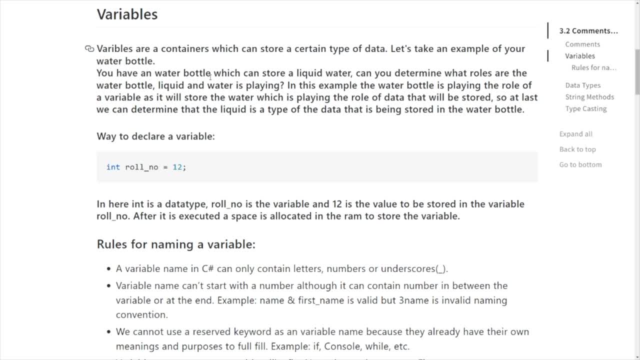 right what memory like, how much memory is allocated in the ram. we will see in the later sections. we'll learn about data type, all right, but it uh, it allocates all right, or you can say, makes some space for the variables to store in in the ram. so our variables and values are stored. 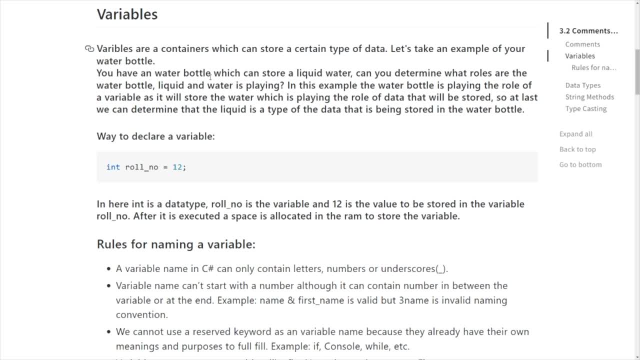 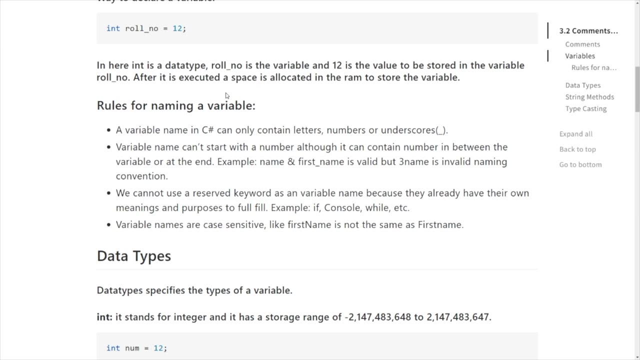 in the ram, all right. so i hope you understand. all right, i hope you understand the concept of variable, all right. if you are confused in some point, you can comment it down, all right. so, uh, now, uh, it is, uh, there's a dialogue that uh, with great. 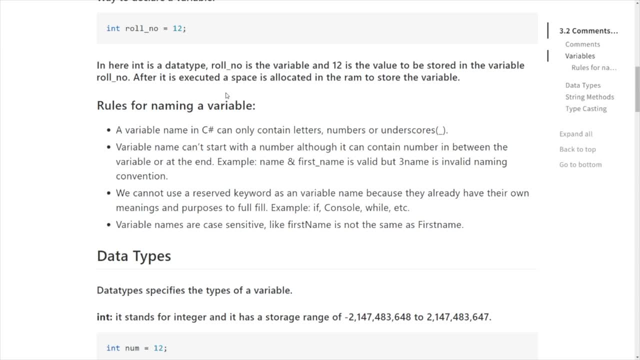 power comes great responsibility right. similarly, with variables, there also comes rules, all right, and we have to maintain those rules. the very first rule- all right, the very first rule- is that a variable name in c sharp can only contain a variable name in c sharp can only contain. 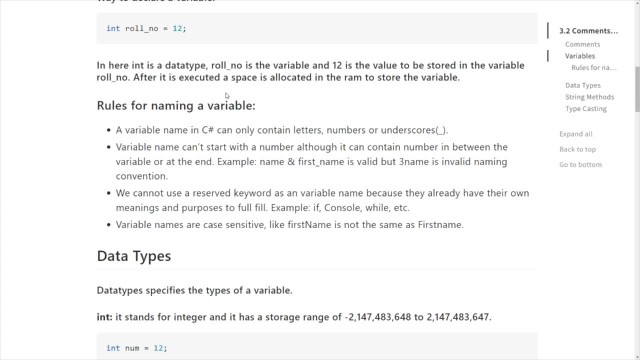 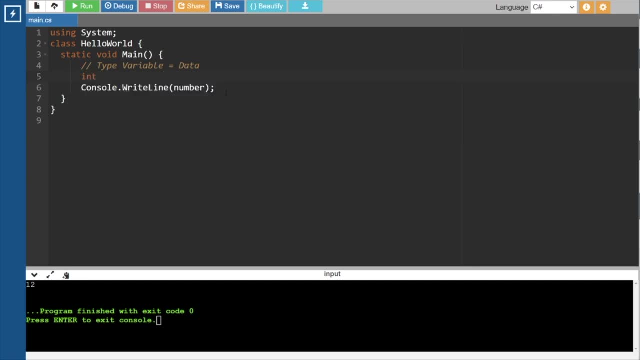 numbers, uh, letters, numbers or underscore. all right, what that means is all right, we can't create a variable, all right? uh, let me, let me show you: actually, int dollar num equals 12. all right, let's uh try to print it out and you will see what happens. all right, 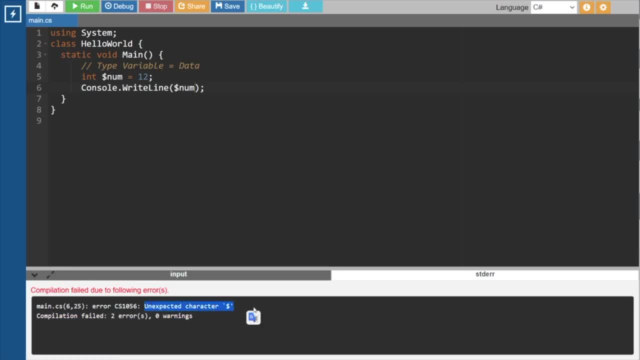 see, it is giving us an error that is unexpected. see, it is giving us an error that is unexpected because the reason is: c sharp doesn't allow a variable to have dollar in in its variable naming. all right, these are called naming conventions, but we can have underscores. all right, we already have letters. right, we already have letter, we can. 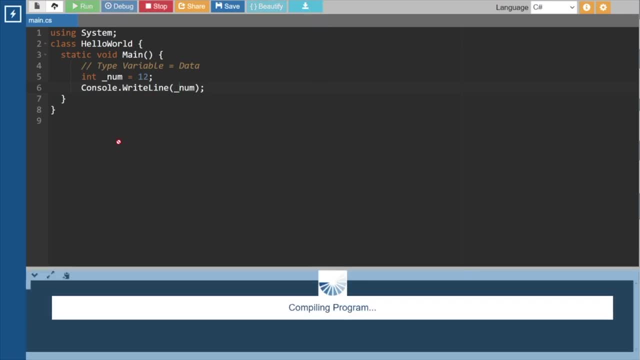 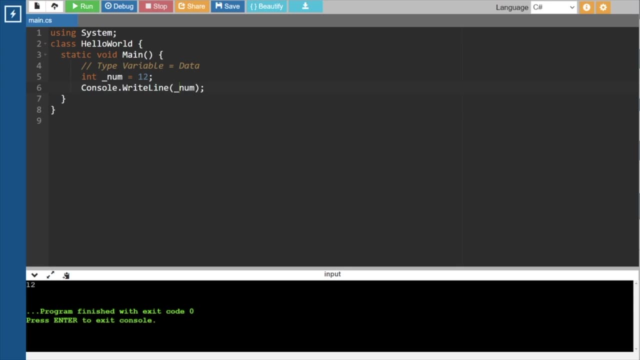 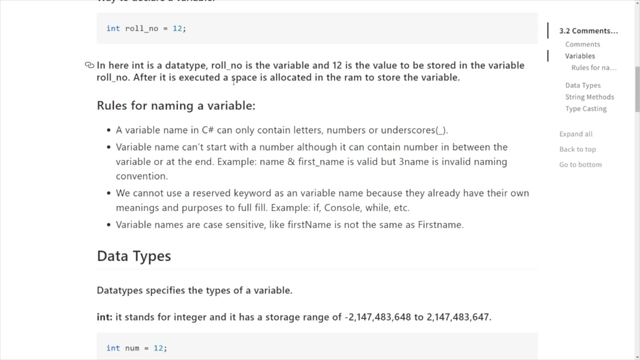 have underscore, all right. we can have underscore two, all right. so yeah, of course we can also have numbers. now here comes another rule regarding it all right. here comes another rule regarding it all right. so variable name- all right. variable name can't start with a number. see, here it is written. 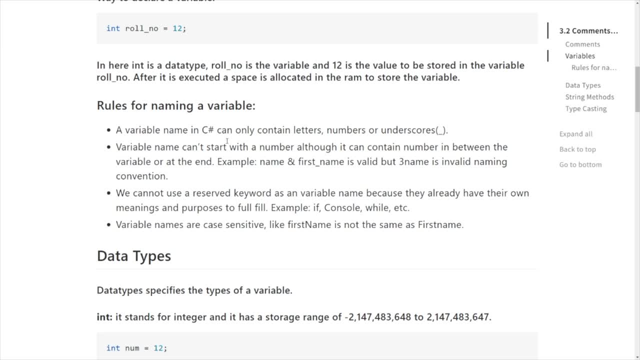 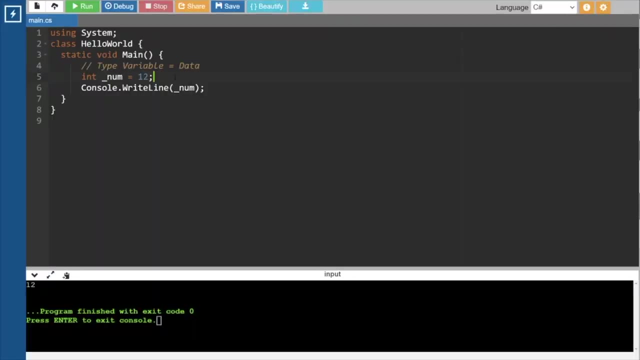 that we cannot start a variable name with a number. that is it. we cannot write a variable name as three abc or two name like that. all right, let's try it out and see. all right, let's try it out and see if that works or not. right, so two num, let's try it out. 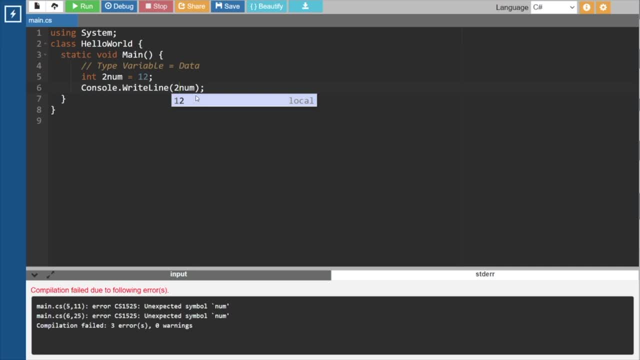 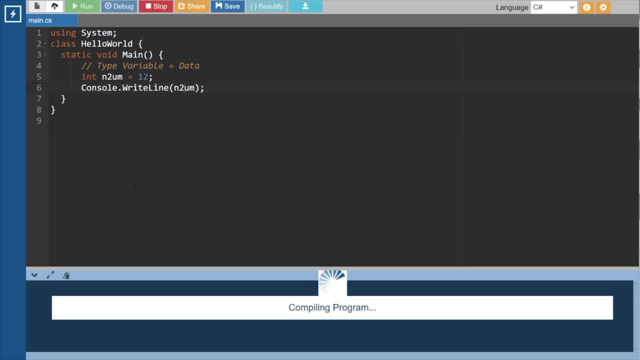 see it is uh giving us an error. that is unexpected symbol, but but we can have uh numbers in between, all right. we can have numbers in between of variable names all right, like n to um. i know it's it's weird, but we can have like this. we can have numbers like this, all right. similarly, we can also. 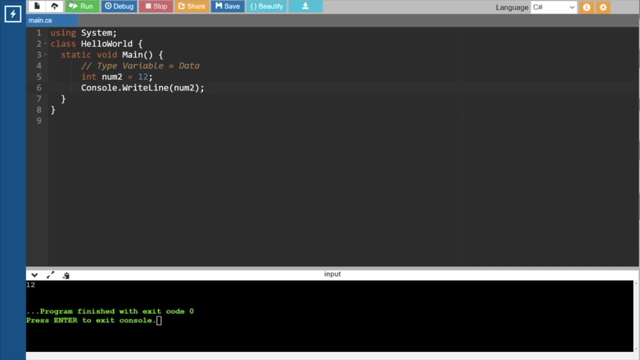 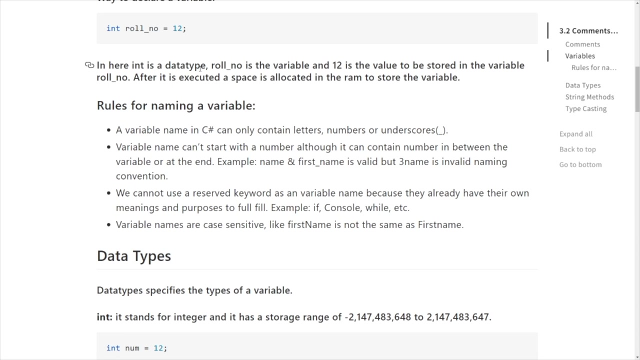 add numbers to the end of the variable. all right, we can also put numbers to the end of the variable. see, it is working perfectly fine, right? so we learnt about two rules: that, uh, we can only add letters, numbers and under underscores during any uh, naming convention, already during the naming of. 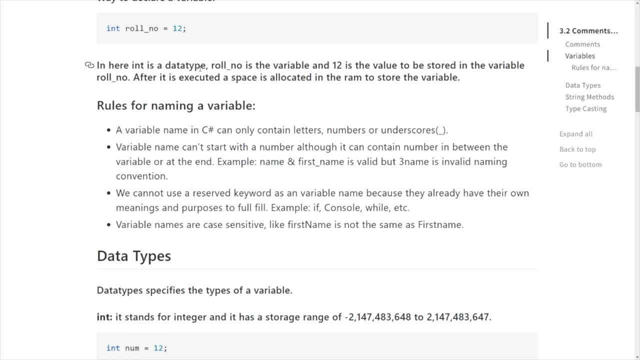 any variable, and also a variable can't start with a number, all right, although it can have. all right, it can have number in between the name of the variable or at the end of the variable, right. so the next rule, all right, the next rule we have is that we cannot use a reserved keyword. 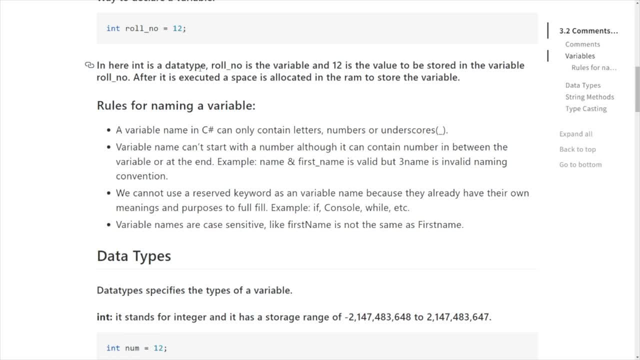 we cannot use a reserved keyword as a variable name, because they already have their own meanings and purposes to fulfill right now. what does this mean? see, there are multiple keywords, all right. or you can say reserved keywords in, uh, in our sisha program, just like we saw previously. like using 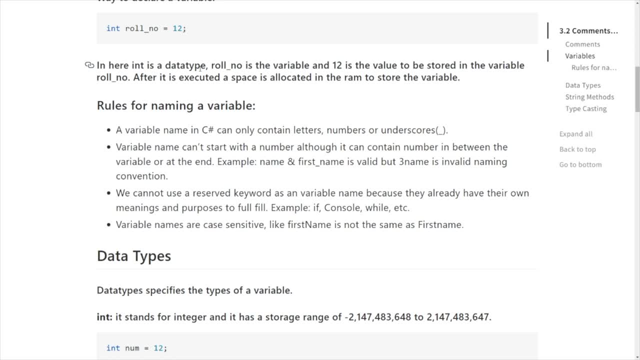 all right using system. they are reserved keywords. all right using is a reserved keyword. class is a reserved keyword. all right int. all right int is a reserved keyword. if is a reserved keyword, all right console. it is a reserve keyword. so we cannot use any sort of reserved keyword. 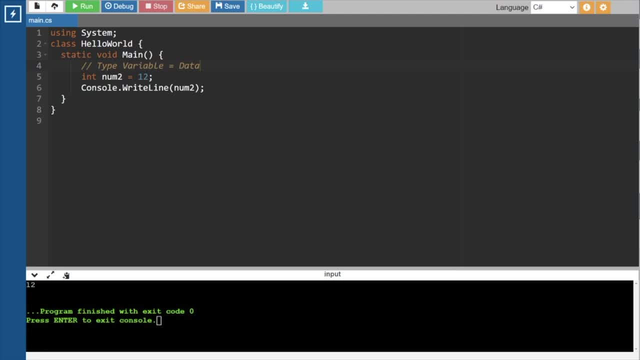 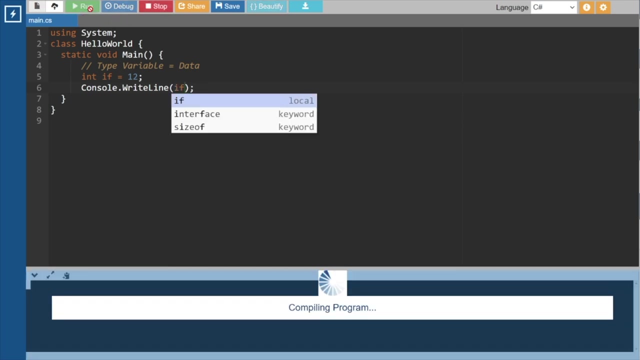 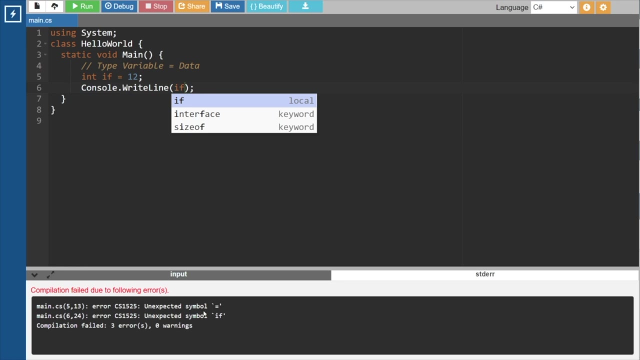 during a variable naming convention, right? so let's try it out, all right, let's, uh, let's give it a variable name as if. all right, and just let's try it out. what happens. let's see what happens. wow, it has given some error, right, it is giving unexpected symbol. equals then unexpected symbol. if it would, it will give, because 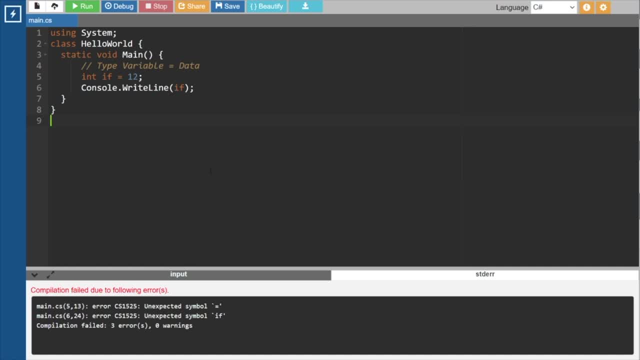 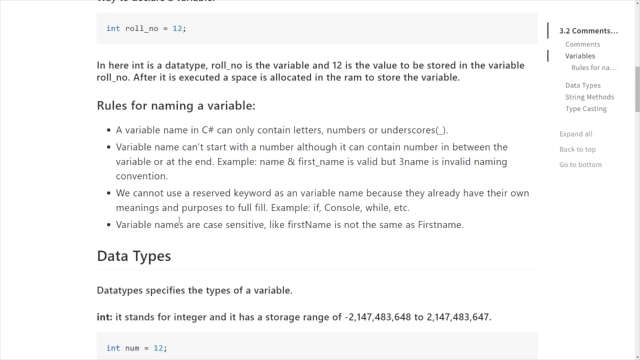 this is not the syntax of f, right. that's why it is giving the error. unexpected symbol equals all right, so yeah, so you, uh, you learned that we cannot use any sort of uh, reserved keywords as variable names. all right, similarly, uh. another thing is: variable names are case sensitive. all right, what? 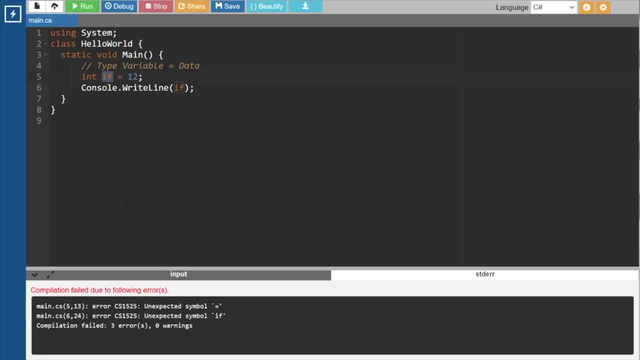 does this mean? see, uh, it means that if you write a variable like this, all right, let's say uh. if you uh write a variable like this, name equals priyanshu. all right, see, uh, this is a string data type. all right, i would uh tell you what is this, but don't worry, for now i'm just showing an example, and uh. 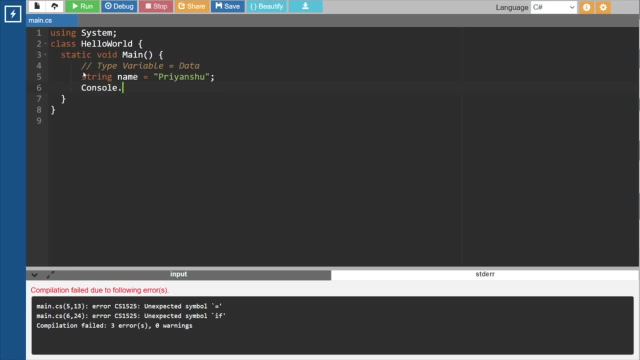 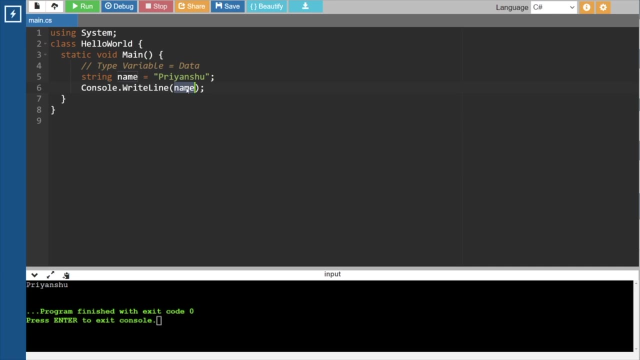 let's try to print it out. all right, so let's try to print it out and let's see what happens. right, so you can see that it has printed my name right. but let's say, if i write uh the name in capital letters, all in caps, all right, all in caps, can you? can you, uh, can, can you tell that? will it uh? 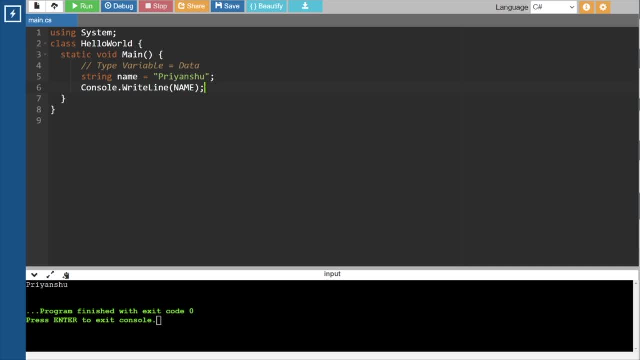 execute the program. execute in the sense, of course it will execute, but will it give any sort of error? or just print priyanshu as it is written right now? all right, so will it just take time? all right, just take a few seconds and think about it. all right, think about it, will it all right? 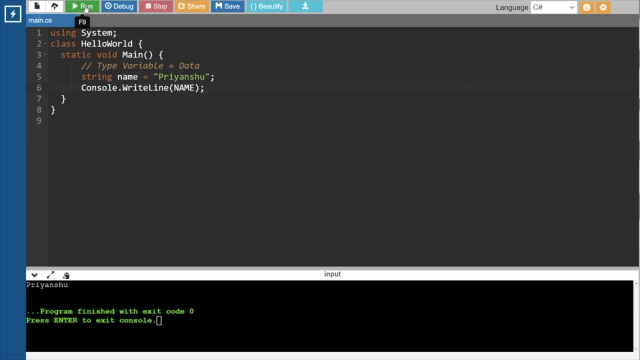 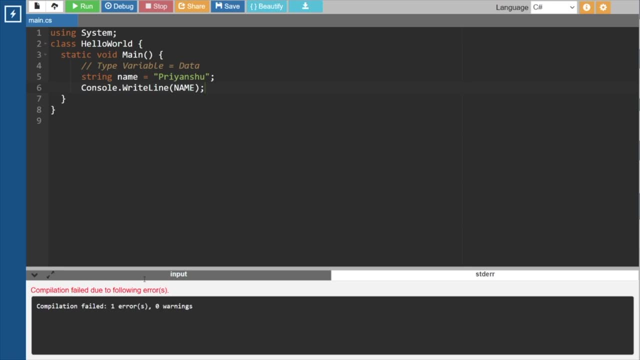 pause the video and think about it. so let's, let's run it now. all right? see, it is giving us an error. it is giving us us an error why? because there is no variable defined as n a, m e, that is, capital letters, n a m e. there's a variable defined. 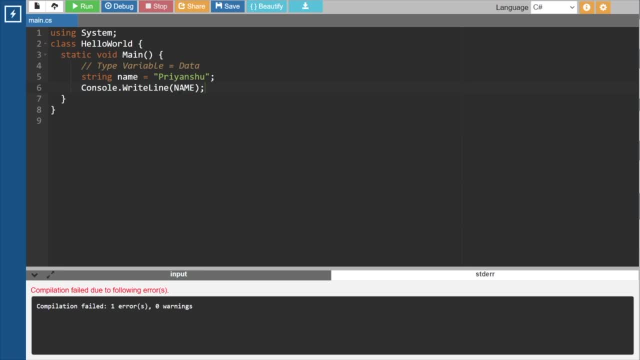 as n, a, m, e, as small letters. all right, this variable is in small letters and we wrote it in capital letters, so both of them are totally different. all right, both of them are totally different. so uh always remember that the variable names, that is, uh the type, or you could say: 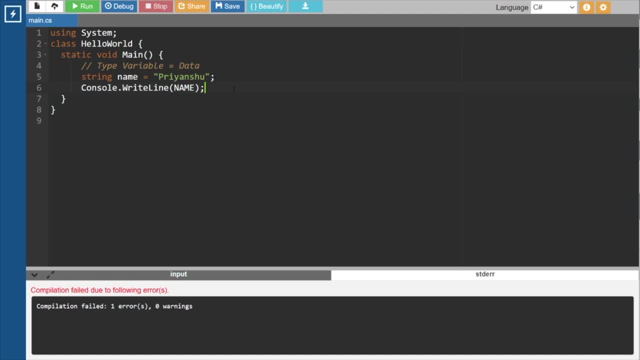 not exactly the type uh. just check that. if the variable name is in caps or uh in small letters, all right, because these are uh case sensitives, all right, these variables are case sensitives, all right. so we can't have like if we write a name in small letters and we are trying to print. 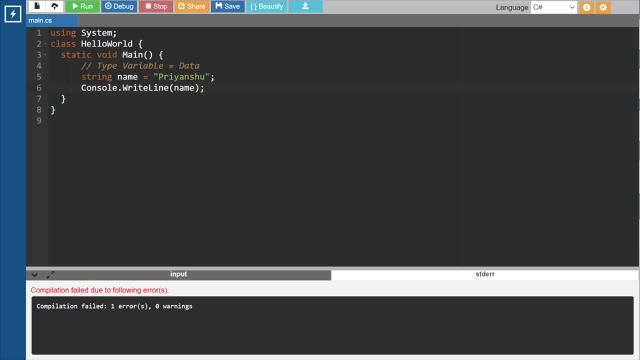 that name in capital letters means uh. in capital letters is uh means that we are uh trying to write that name variable in the consolewrite line in capital letters. it won't execute, because it would, then it would search for another set of variables. all right, it would search for another variable whose, whose uh text is in a capital letter, and 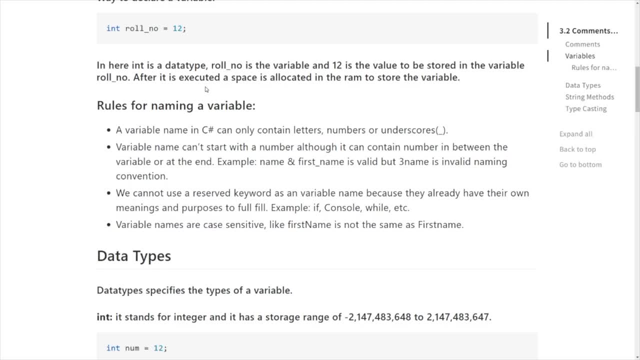 is written name, all right. so i hope you understand that we can't have uh like variables means we can have variables, but uh, they are case sensitive. all right. like uh, because the see in this example this first name, all right, this first name. you can see that the first is written in a small letter, the n. 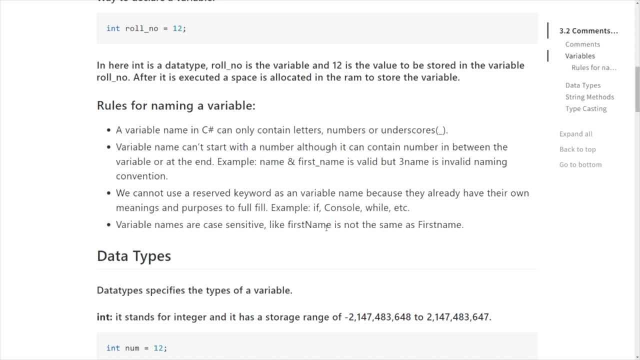 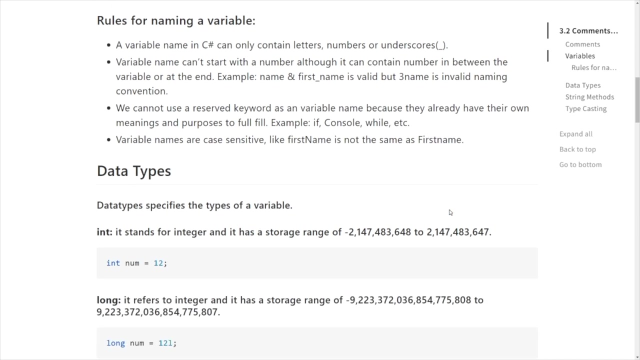 is written in capital letters, capital letters and a, m, e is written in small letters, but in in another, is in another uh text, it is uh, the f is caps, but but the other letters are in a small letter, all right, are in small. so this, this name and this name are not same, all right, both are totally different, all right. 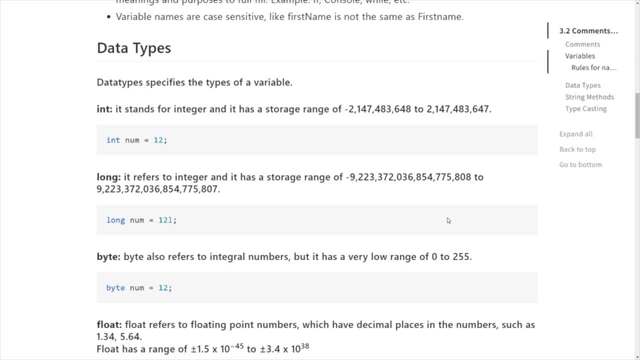 now, as we have learned about variable its rules. all right, now it's our time to get into the data types. all right, see, it is a very important concept. all right, data types is a very important concept. so, uh, try to understand it. all right, if you are not able to understand. 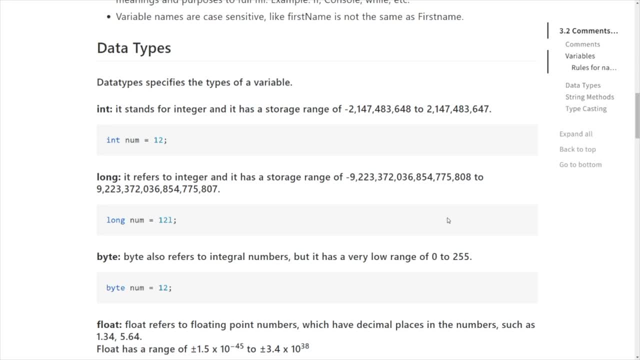 something. all right, you can comment it down, and also i would suggest re-watching this particular portion. all right, re-watching the particular portion you have not understood. then also, you have, you haven't understood, you can comment it down and i would uh like to help you, all right. so, yeah, data types. right, see, uh, i already told you about an example. 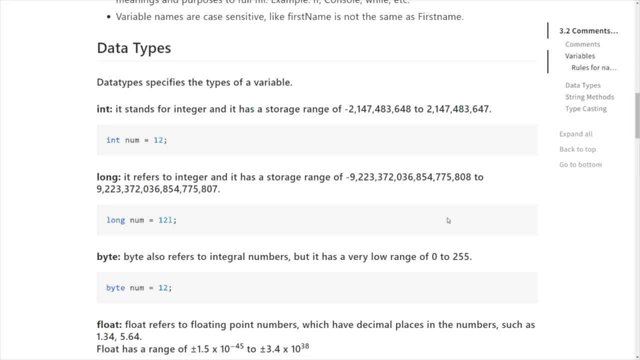 right previously, the water bottle example- that the liquid is the data type or you can say the type of the value, right? similarly, data types are also the same thing. they they specify the type of a variable. already specify the type of the variable, all right. the type of value it can. 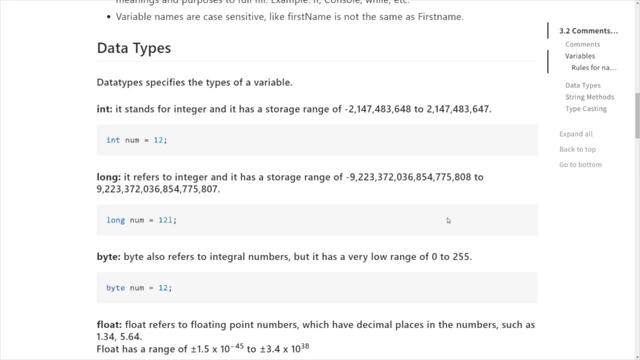 store, right. so the very first data type we have is int. all right, so basically the int. int is basically a short for integer. all right, uh, and it has a range. all right, it has a range of minus two, one, four, seven, four, eight, three, six, four, eight, two, two, one, four, seven, four, eight, three, six, four, seven. 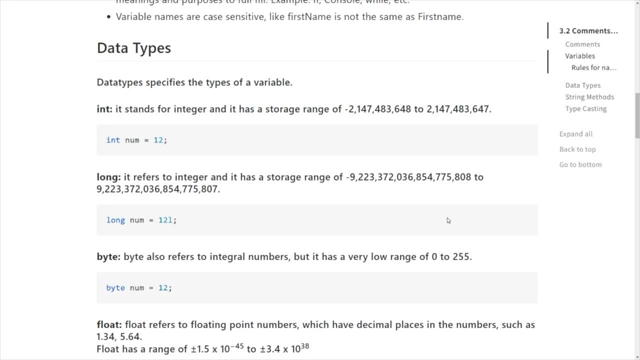 all right. what this means? that it has a range of this to this. all right, it has a range of this to this. if we exceed that value, all right. let's say, if i write two, one, four, seven, four, eight, three, six, four, seven, then it would return a error. all right, let's try it out all. 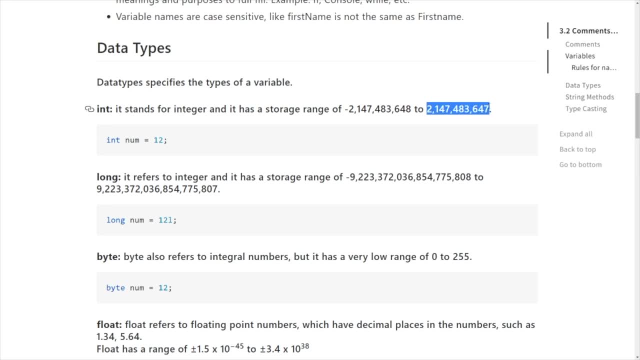 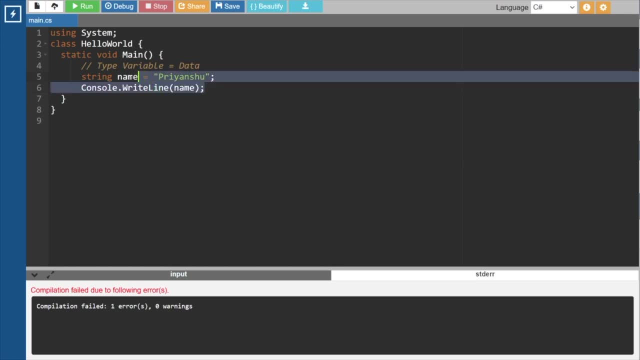 right, let's copy this value first. all right, um, let's copy this value first and let's try it out in our code editor. all right, let's copy this value first and let's try it out in our code editor, all right. so, um, yeah, int val equals all right, so, um, now let's try to print it out. console dot right. 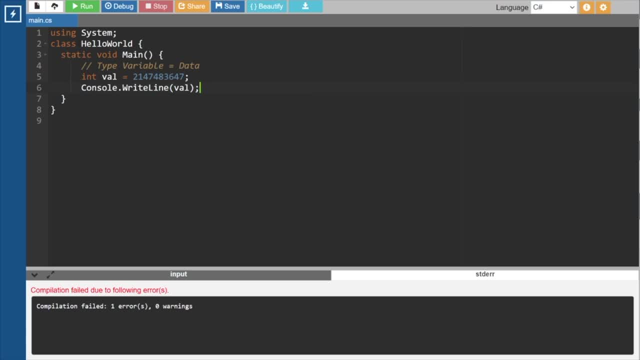 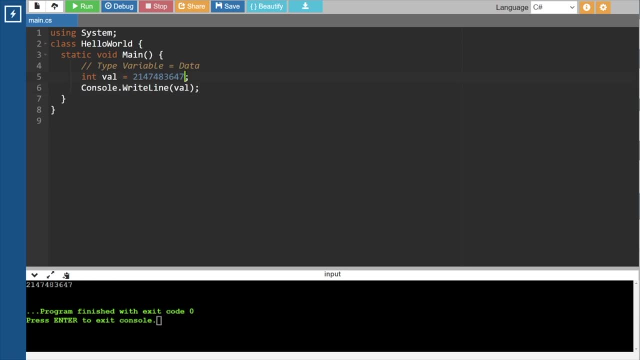 line val. all right, let's run. run the program and see it is printing. right, it is printing the exact value, but but for now, let's, let's change it to 2147483648. can you tell me, will it print or will it like give us some error? 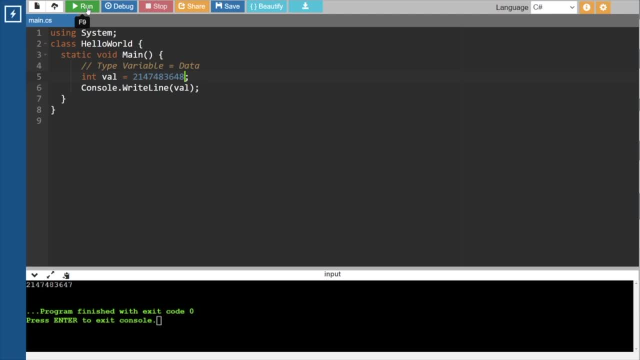 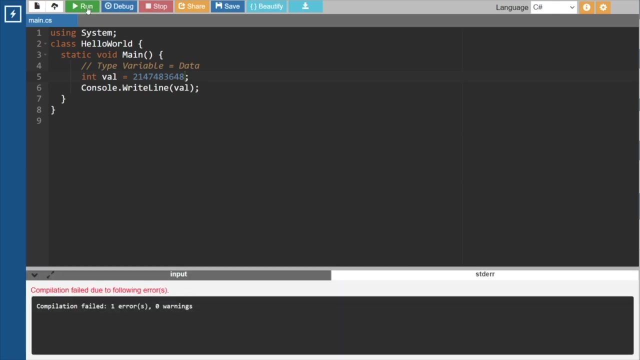 pause the video and think about it. all right, think about it and just tell me that will it print the value? all right, just pause the video and think about it. so let's run the program and let's see, my god, it is giving us some sort of error. why it is giving that error? because the range is 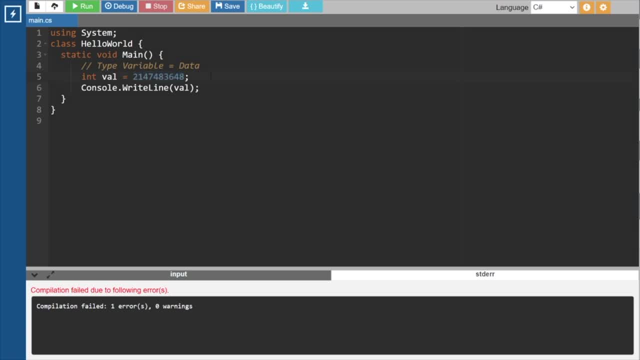 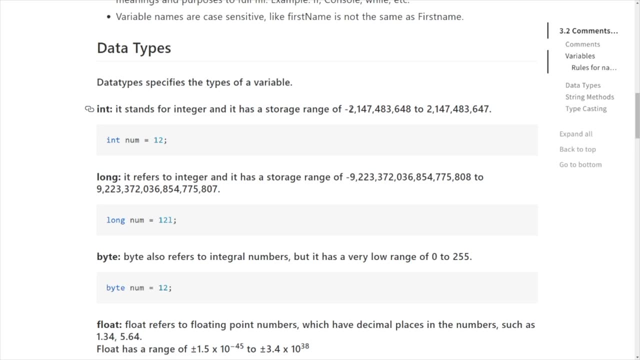 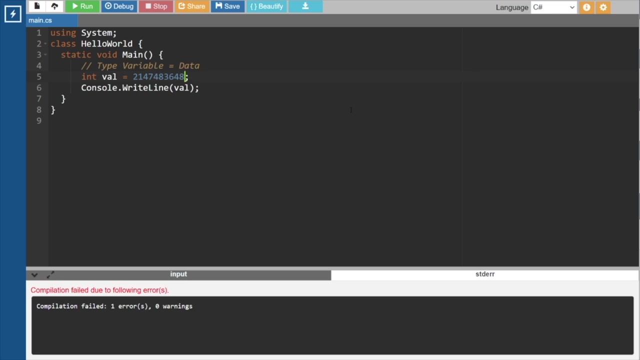 exceeded. all right, means we have exceeded the range of integer, like here. you have seen that the max means the negative range is 2147483648, right, and the positive range is up to 2147483647, but in there we wrote 2147483648, so it is having a plus one value. all right, it is exceeding the range. that's why it is. 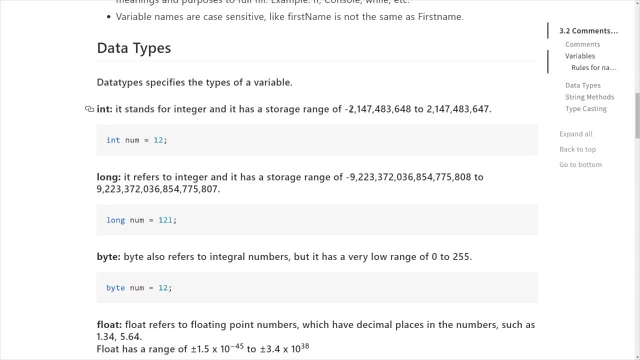 giving error. so ranges basically tells us that how much value, all right. how much value the a particular data type can store, all right. and we also learned how to use integer. that is int, as long, all right it is. you can say it is a big brother of int, all right, uh, it also store. 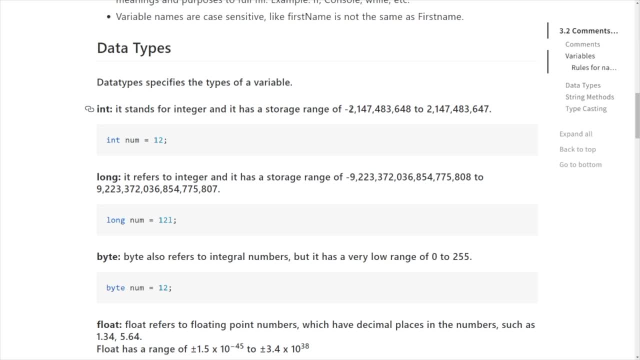 integer value, all right. that is, for uh means non-decimal value. we could say, or you can also say, integer value, all right, so it has a more higher range, all right, this long, all right. this long has a more higher range than int, all right. so when you need more values to store, all right. 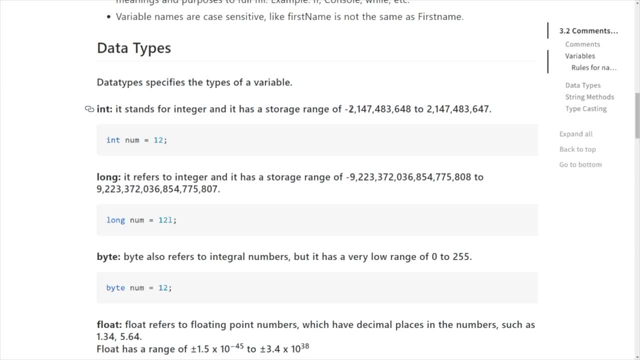 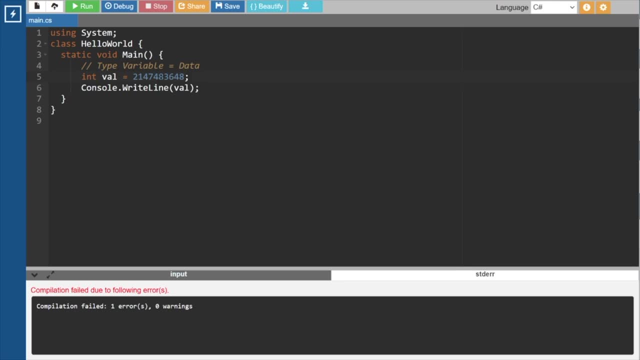 that is, higher range of values to store, then you should go for long. all right, like, let's try out the same example. right, we like. here we see that we put some uh using int, it exceeded it, uh, its range. right, because the range was up to 2147483648. right, but let's try the same thing out with. 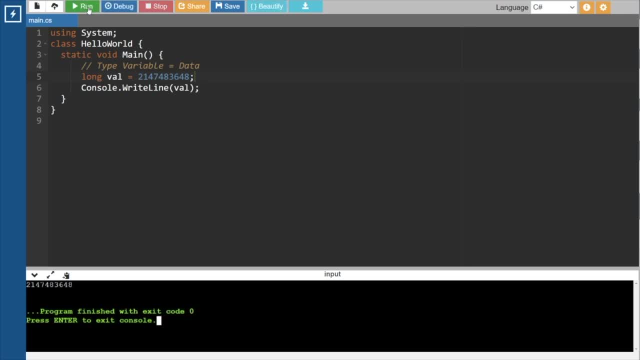 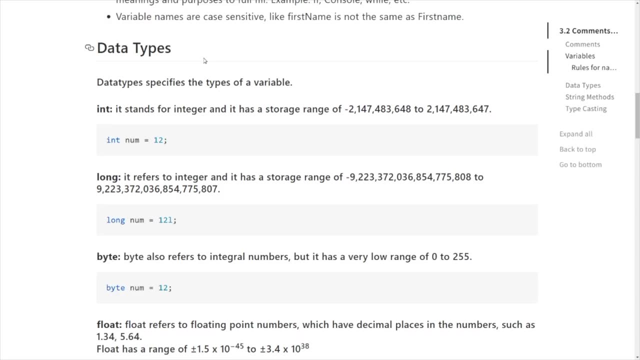 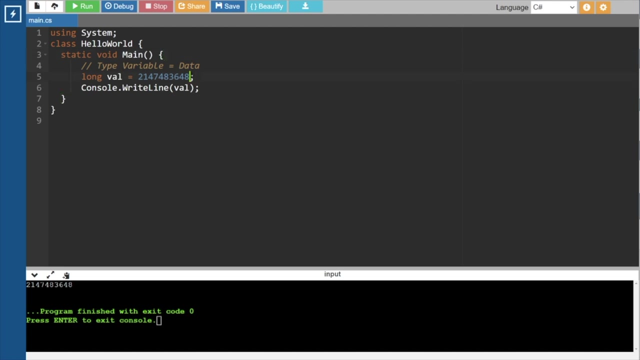 long will it exceed? let's see it won't. it won't exceed. do you know the reason? the basic reason behind it is because the range of long is much, much bigger than of, uh, integer. all right, it is really. the range is very much bigger than integer, right? uh? another thing, all right, as you can see in here. basically, uh, we can. 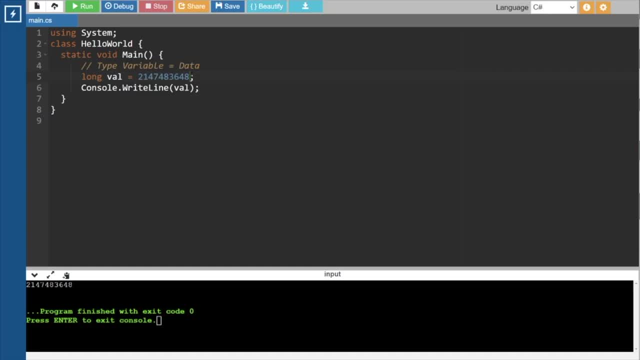 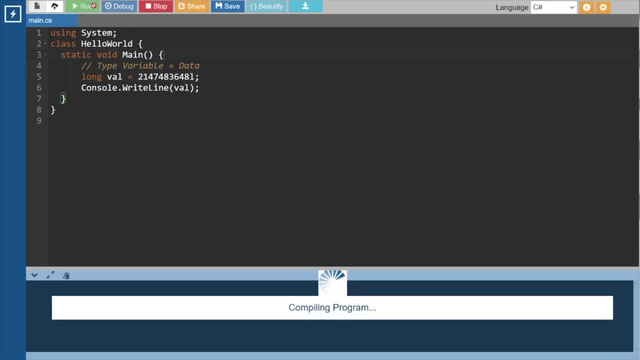 also add a suffix. all right, we can also add a suffix l. all right, we can also add a suffix l in here. and it is not mandatory. all right, it is not mandatory, but it is uh recommended to add the suffix l. all right, it is recommended to add the suffix l, all right. so, uh, yeah, now, as we have understood about uh long, all right, as we. 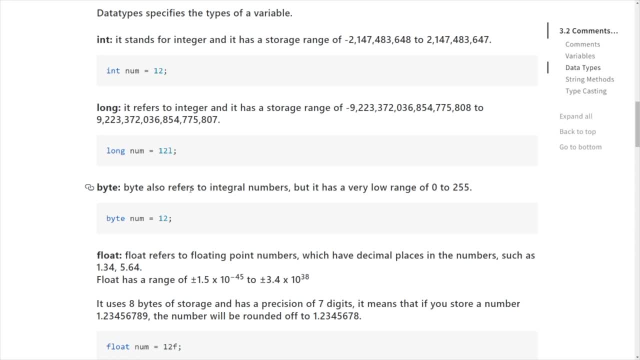 have understood about uh long. all right, it is now a time. all right, it is now time to understand about. it is now a time, all right, it is now time to understand about. it is now time to understand about byte. so we are going to learn about uh byte. 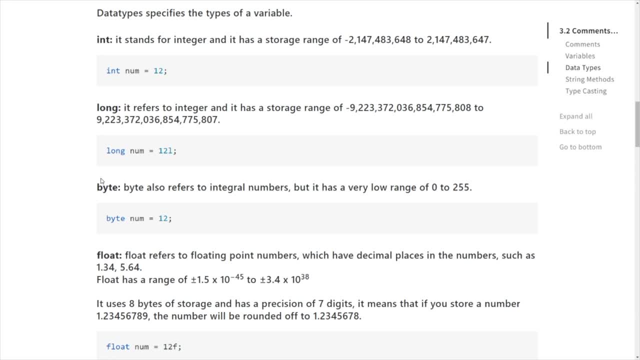 byte, so we are going to learn about uh byte, byte, so we are going to learn about uh byte, right. so another thing: uh, before going into right. so another thing, uh, before going into right. so another thing: uh, before going into byte. all right, another thing i would like to. 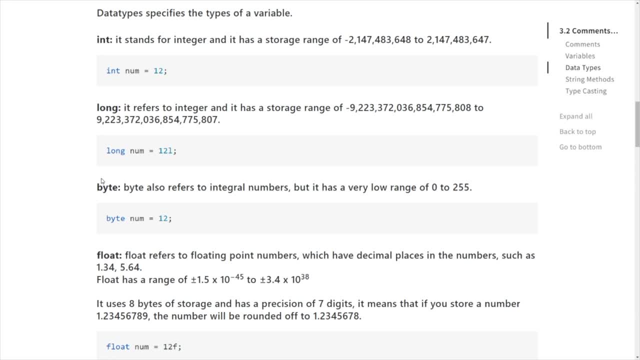 byte all right. another thing i would like to byte all right. another thing i would like to suggest is: whenever you are writing all right. suggest is whenever you are writing all right. suggest is whenever you are writing. all right means this suffix l all right in the long. 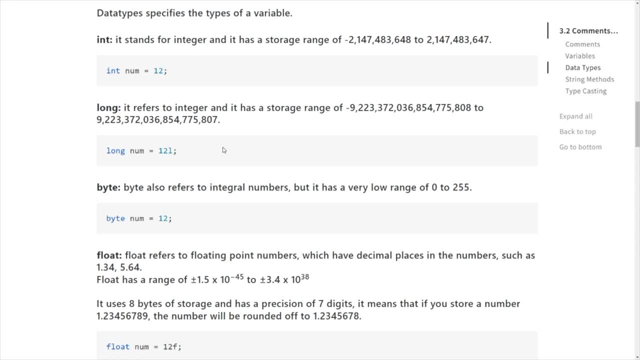 means this suffix l all right in the long. means this suffix l all right in the long? whenever you are writing this, always remember, whenever you are writing this, always remember, whenever you are writing this, always remember that to use capital- all right capital l. that to use capital- all right capital l. 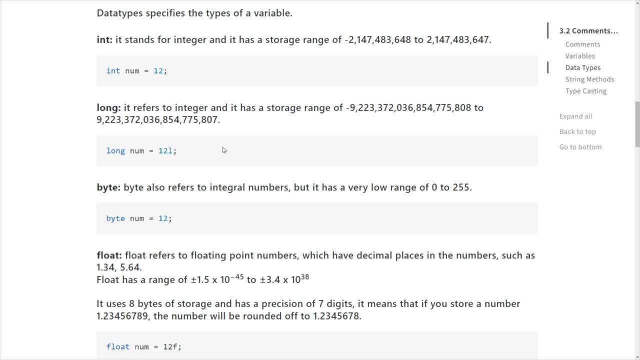 that to use capital, all right, capital l. there's a very uh specific reason for that. there's a very uh specific reason for that. there's a very uh specific reason for that: because many people, what many people does is because many people. what many people does is. 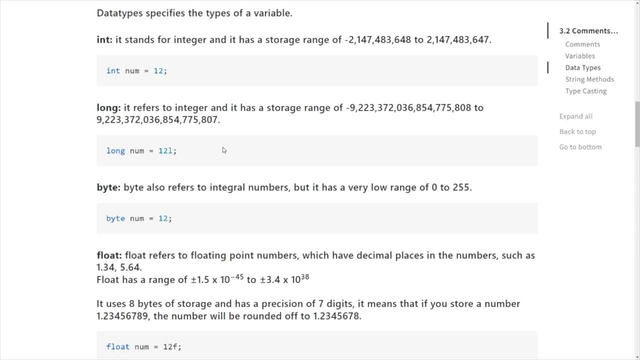 because many people, what many people does is they, they. they gets confused with a small letter l and gets confused with a small letter l and gets confused with a small letter l and one, one, one. it's sometimes uh confusing- and even c. it's sometimes uh confusing and even c. 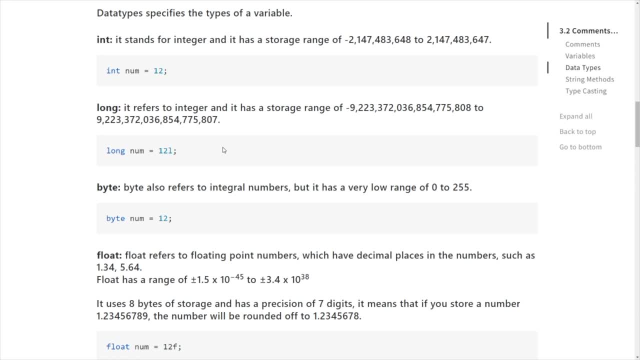 it's sometimes uh confusing. and even c sharp, uh sharp, uh sharp. uh. recommends to use a capital letter. l recommends to use a capital letter. l recommends to use a capital letter. l all right to use capital letter. l all right to use capital letter. l. all right to use capital letter. l in spite of small letter. l all right. 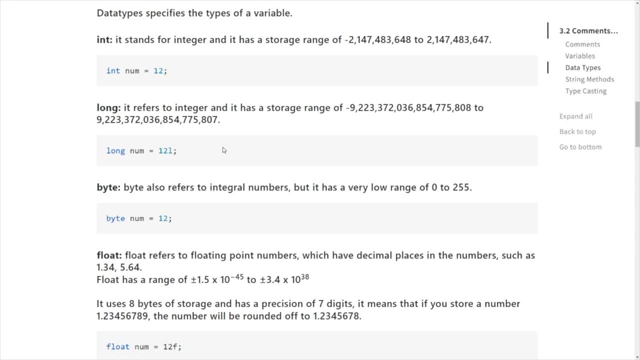 in spite of small letter l, all right. in spite of small letter l, all right, although it will give a warning if you, if, although it will give a warning if you, if, although it will give a warning if you, if you use small letter l, but uh there. 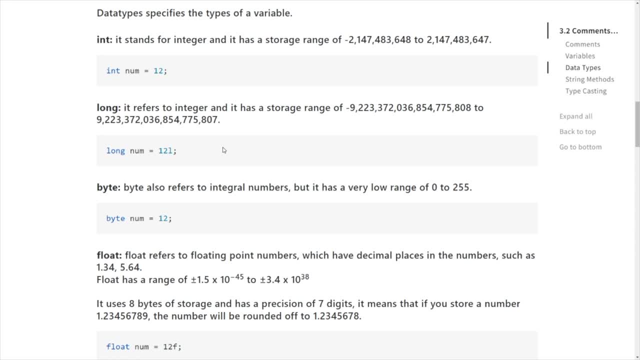 you use small letter l, but uh, there, you use small letter l, but uh, there won't be much uh issues with that. but it won't be much uh issues with that. but it won't be much uh issues with that. but it is recommended to use capital letter l. 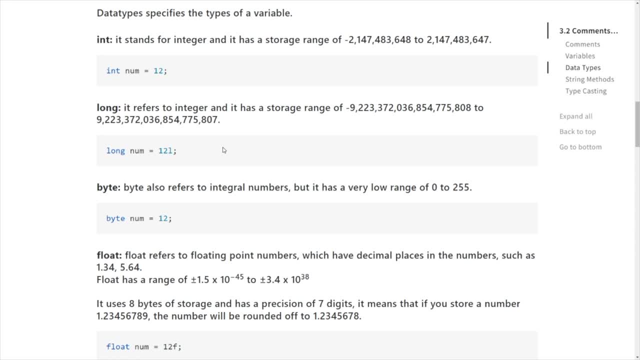 is recommended to use capital letter l is recommended to use capital letter l in spite of, in spite of, in spite of small letter l in the suffix of long. all small letter l in the suffix of long. all small letter l in the suffix of long. all right long data type. 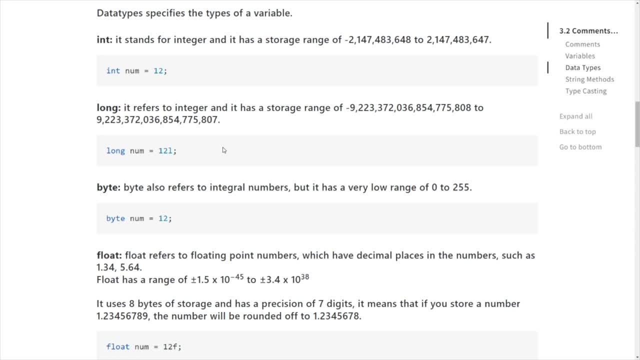 right long data type, right long data type. so, uh, let's get into the byte all right. so, uh, let's get into the byte all right. so, uh, let's get into the byte, all right. byte data type. byte data type. byte data type: see byte is also uh. 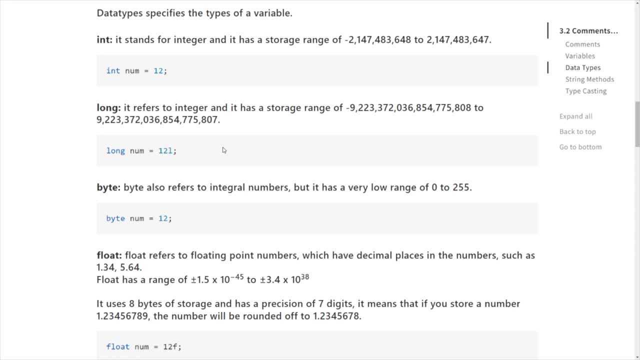 see, byte is also. uh see, byte is also. uh so, uh sort of integer only all right, it so, uh sort of integer, only all right, it so uh sort of integer, only all right, it also stores, uh, also stores, uh also stores, uh integers, but integers, but integers, but the byte, all right, bytes range is: 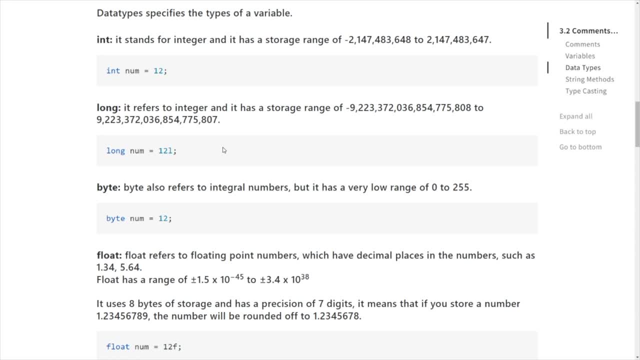 the byte all right bytes range is the byte all right bytes range is really low. all right byte has a really really low. all right byte has a really really low. all right byte has a really low range, low range, low range, all right, all right. all right byte has a really 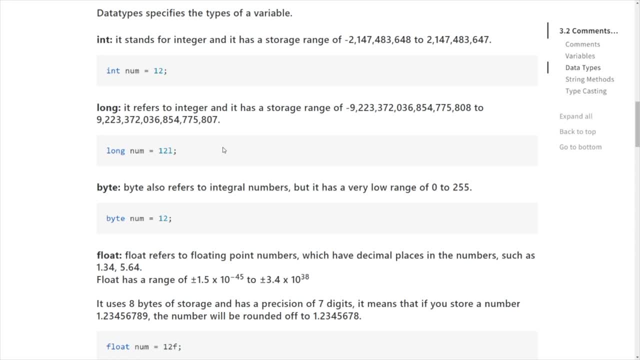 byte has a really byte has a really low range, low range, low range. so, uh, the range of it is from 0 to 255. so, uh, the range of it is from 0 to 255. so, uh, the range of it is from 0 to 255. all right, it is, it is the range of. 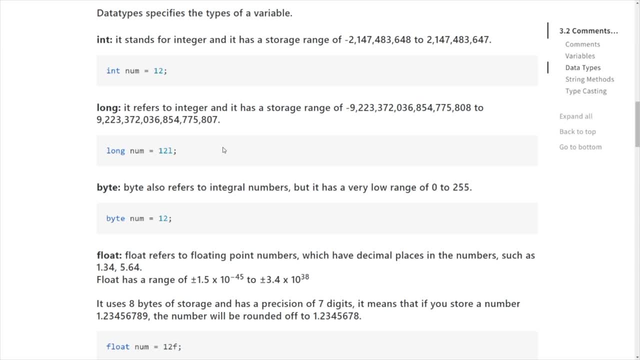 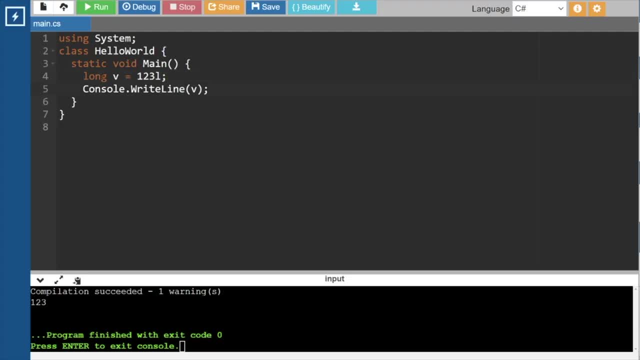 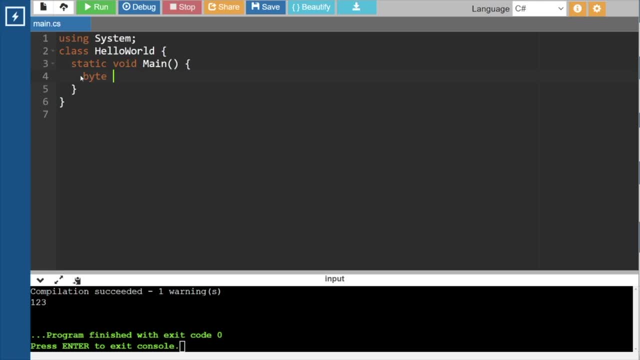 that is, that is, byte all right, byte all right, byte, all right, byte, byte, byte, all right now. if we give value, uh, byte, all right now. if we give value, uh, byte, all right now. if we give value, uh, exceeding all right, if we give value exceeding all right, if we give value. 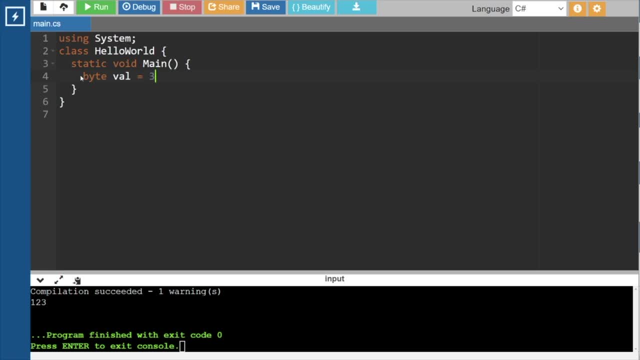 exceeding. all right, if we give value exceeding, exceeding, exceeding 255, that is, let's say 300, 255, that is, let's say 300, 255, that is, let's say 300. all right, and then try to print console. all right, and then try to print console. 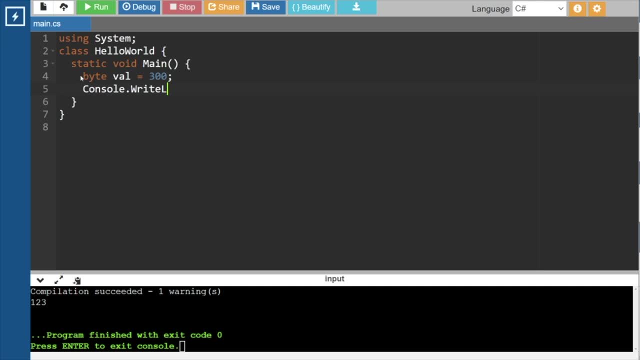 all right, and then try to print console: dot, dot, dot, right line, right line, right line, all right, all right, all right. val, val, val. so let's see what it does, all right. so let's see what it does, all right. so let's see what it does. all right, let's see what it basically. 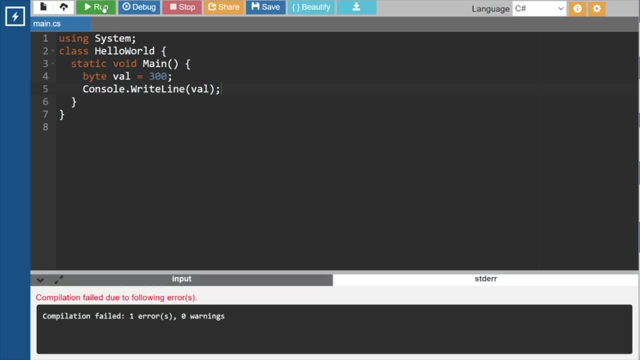 let's see what it basically. let's see what it basically does, does, does. let's see, all right, so it is giving us. let's see, all right, so it is giving us. let's see, all right, so it is giving us some sort of error. why it is giving error. 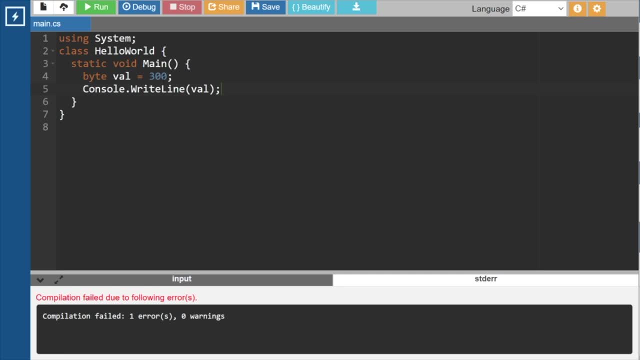 some sort of error. why it is giving error, some sort of error. why it is giving error? all right why it is giving it. it is all right why it is giving it. it is all right. why it is giving it. it is giving us error. because giving us error? because 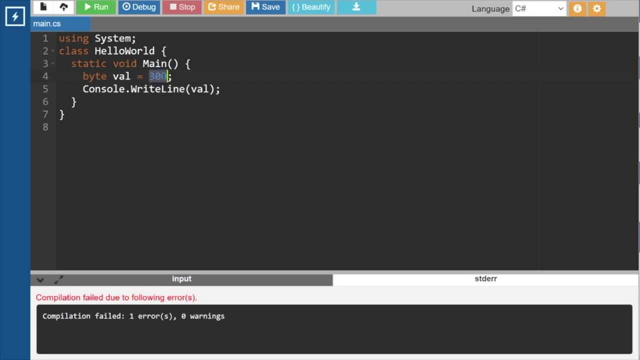 giving us error because we exceeded the limit. all right now if we exceeded the limit. all right now if we exceeded the limit, all right now. if we give something, we give something, we give something under the limit- all right, that is uh. under the limit- all right, that is uh. 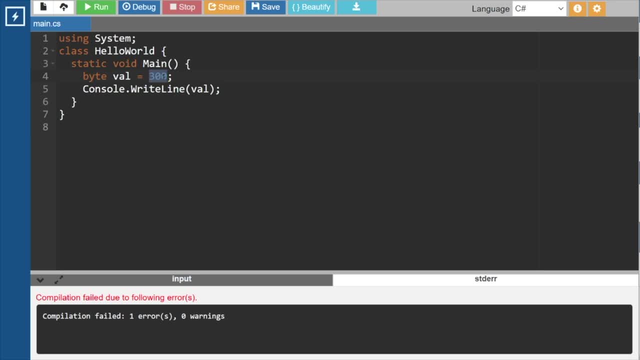 under the limit. all right. that is, uh between the uh, between the uh between the uh. zero to 255. all right, let's say we give zero to 255. all right, let's say we give zero to 255. all right, let's say we give 255 only. 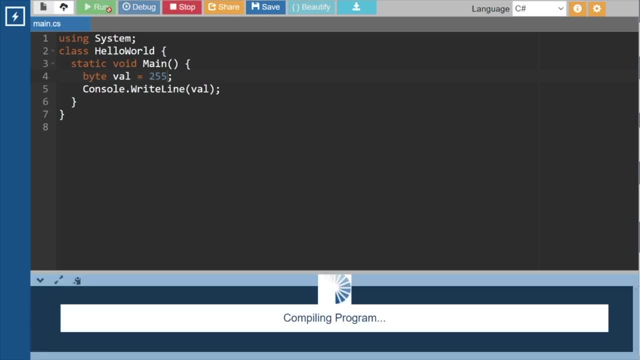 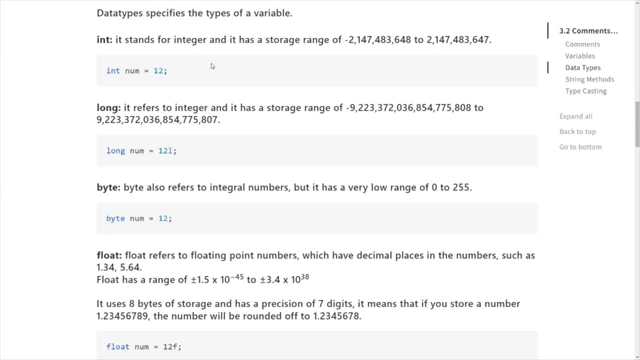 255, only 255, only. all right, if we give this, see it is working perfectly fine. see it is working perfectly fine. see it is working perfectly fine. so, yeah, that's what byte is. it has a low. so yeah, that's what byte is, it has a low. 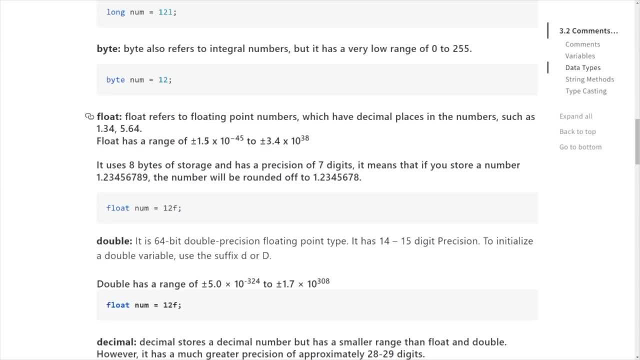 so yeah, that's what byte is. it has a low range, range range, but it is an integer data type, all but it is an integer data type, all but it is an integer data type. all right, similarly right, similarly right, similarly, we also have other data types- all. 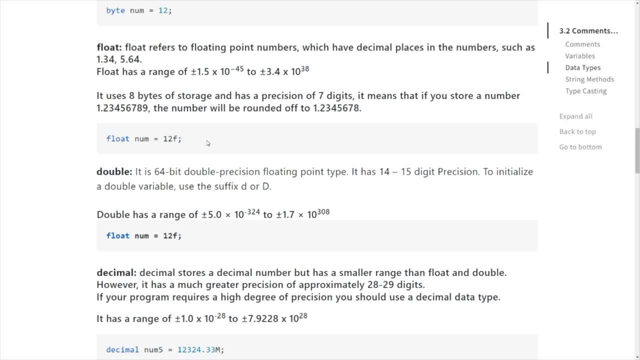 we also have other data types. all we also have other data types. all, right now we are going getting into the right. now we are going getting into the right now we are going getting into the floating the point data type so you can floating the point data type so you can. 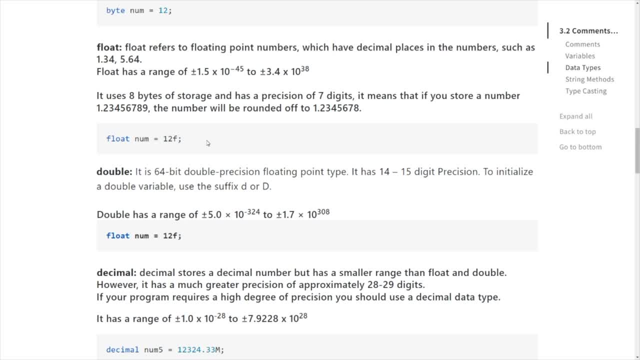 floating the point data type, so you can say decimal data type. right, that say decimal data type. right, that say decimal data type. right, that these are the data types that has. these are the data types that has. these are the data types that has decimal decimal places. decimal decimal places. 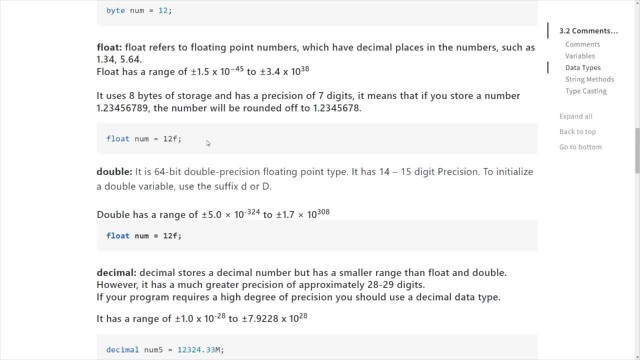 decimal, decimal places, all right, these data types has decimal, all right. these data types has decimal, all right. these data types has decimal places, places, places. so the very first uh data type, we we so the very first uh data type, we we so the very first uh data type, we we will be learning in. 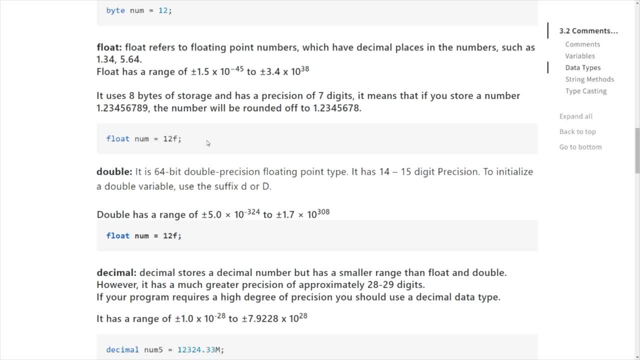 will be learning in. will be learning in in decimal places. uh, all right, uh, that is in decimal places. uh, all right, uh, that is in decimal places. uh, all right, uh, that is floating point numbers. or you can say floating point numbers, or you can say floating point numbers, or you can say float. all right, so float is a data type. 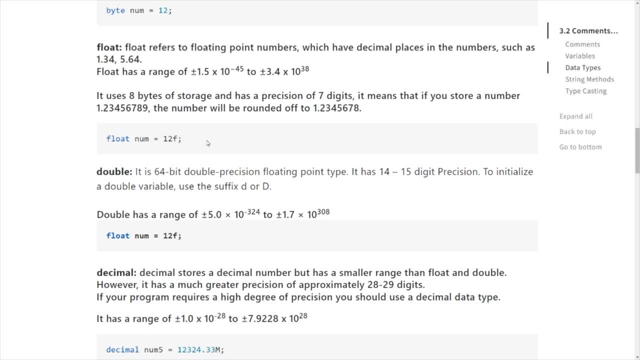 float- all right, so float is a data type. float- all right, so float is a data type- all right. which can have dating decimals: all right. which can have dating decimals: all right. which can have dating decimals, means which have decimals, means which have decimals, means which have decimals, places in numbers: all right, if you want. 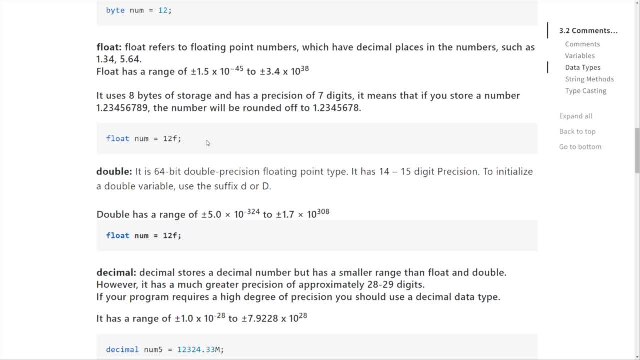 places in numbers. all right if you want places in numbers, all right. if you want to store to store, to store the uh some value in points, we can't the uh some value in points. we can't the uh some value in points. we can't store that in integer, of course. 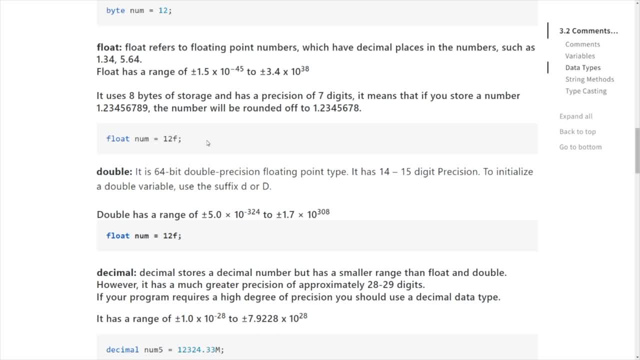 store that in integer, of course. store that in integer, of course. right? so we have to use some sort of data, right? so we have to use some sort of data, right? so we have to use some sort of data. type meant for it, so type meant for it, so. 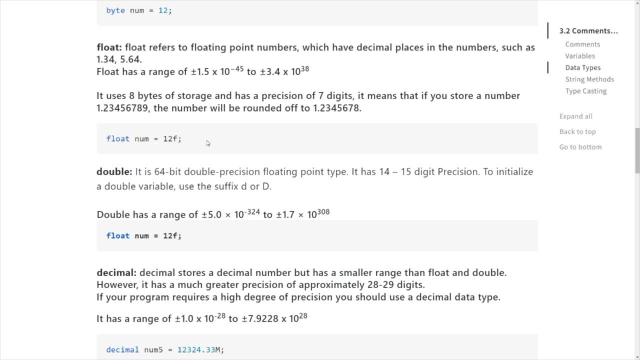 type meant for it. so similarly, there are three data types. all similarly. there are three data types, all similarly. there are three data types. all right, meant for uh storing. right meant for uh storing. right meant for uh storing. uh decimal placed uh values- that is float. uh decimal placed uh values. that is float. 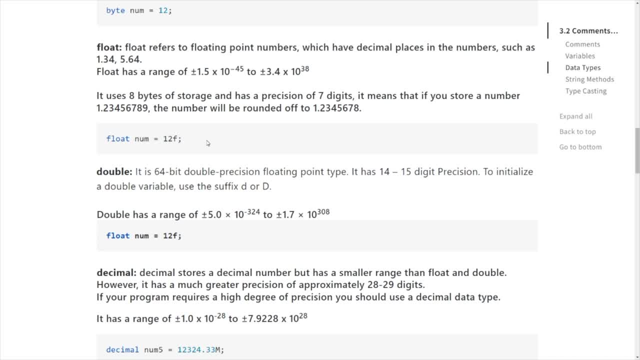 uh, decimal placed, uh, values, that is float. double and decimal all right. so the double and decimal all right. so the double and decimal all right. so the very first thing we are learning is very first thing we are learning is very first thing we are learning is float. 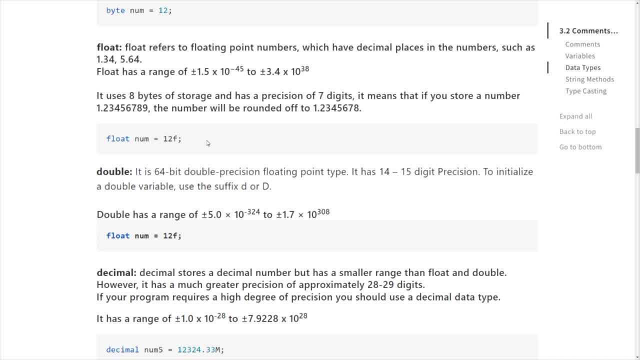 float, float, all right. so floating point, uh, all right. so floating point, uh, all right. so floating point, uh, basically float refers all right to basically float, refers all right to basically float, refers all right to floating point numbers: all right, and floating point numbers: all right, and floating point numbers: all right. and they have decimal places in the numbers. 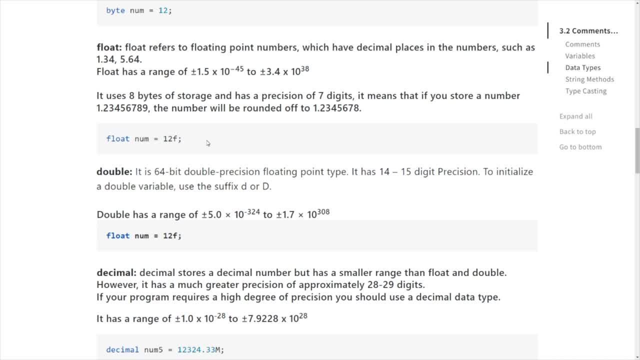 they have decimal places in the numbers. they have decimal places in the numbers, all right, just like 1.34 then 5.64, all right. just like 1.34 then 5.64, all right. just like 1.34 then 5.64, all right. these numbers have decimals. 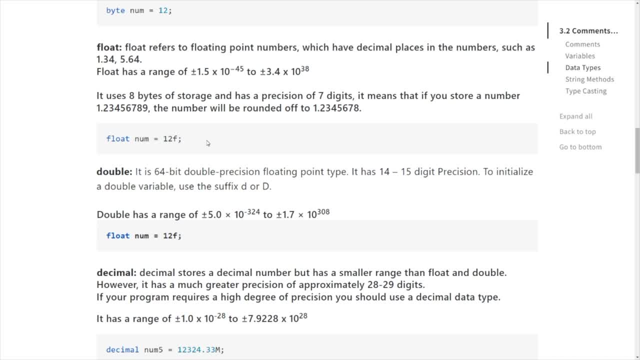 all right. these numbers have decimals- all right, these numbers have decimals, decimal places in them, decimal places in them, decimal places in them. and if we talk about the range, all right, and if we talk about the range, all right. and if we talk about the range, all right. the the float has a range of plus, minus. 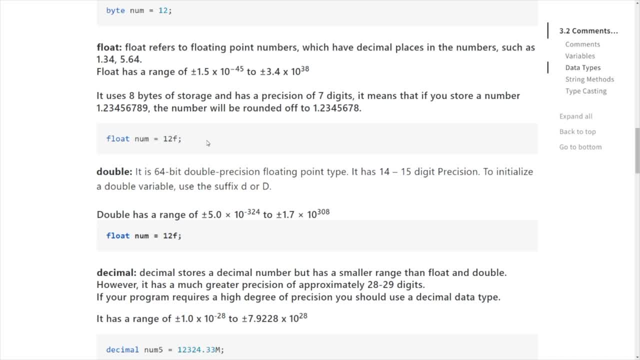 the the float has a range of plus, minus the the float has a range of plus minus 1.5 into 10 to the power minus 45, 1.5 into 10. to the power minus 45, 1.5 into 10. to the power minus 45. all right, 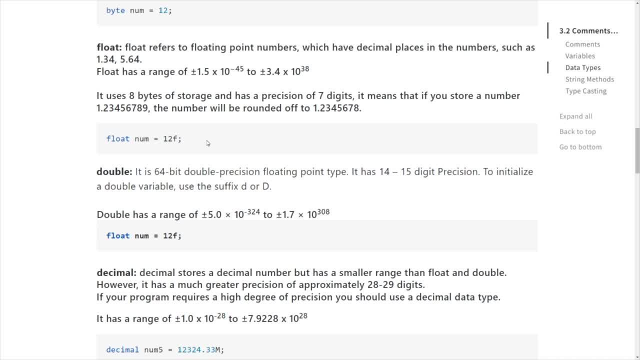 all right, all right. two uh plus minus 3.4 into two uh plus minus 3.4 into two uh plus minus 3.4 into 10 to the power 38. all right, so this is 10 to the power 38. all right, so this is. 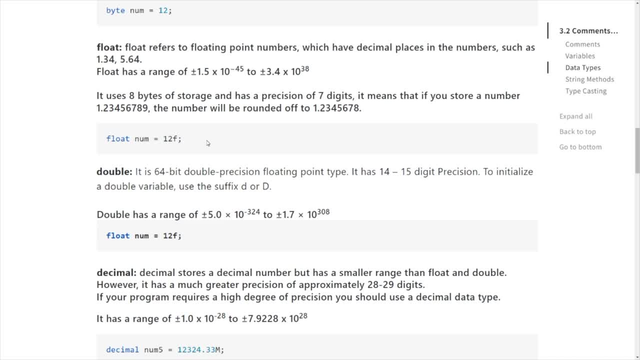 10 to the power 38, all right, so this is the range of float, the range of float, the range of float, all right, and also float uh uh uses, all right, and also float uh uh uses, all right, and also float uh uh uses eight bytes of storage. all right, and it. 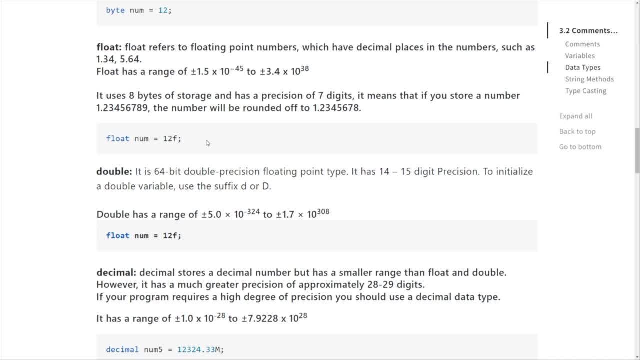 eight bytes of storage, all right. and it eight bytes of storage, all right, and it has a precision of about, has a precision of about, has a precision of about seven digits, all right. so basically, seven digits, all right. so, basically, seven digits, all right. so basically, um, um, 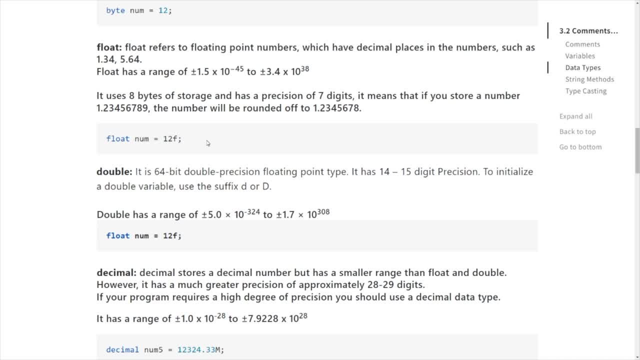 um, it has a precision of seven digits. all it has a precision of seven digits. all it has a precision of seven digits, all right. what that means is it means that, right. what that means is it means that, right. what that means is it means that if you are storing a number like one, 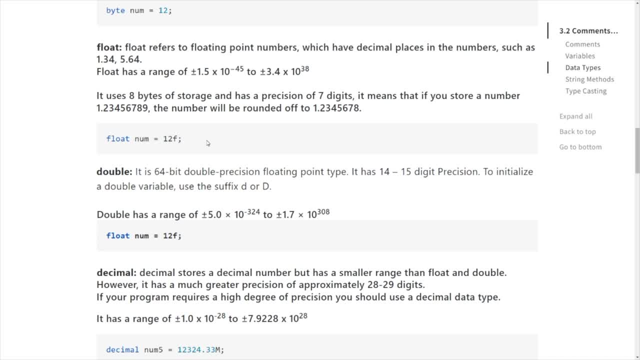 if you are storing a number like one. if you are storing a number like one: point two, three, four, five, six, seven. point two, three, four, five, six, seven. point two, three, four, five, six, seven, eight, nine, eight, nine, eight, nine- all right, if you are storing a numbers, 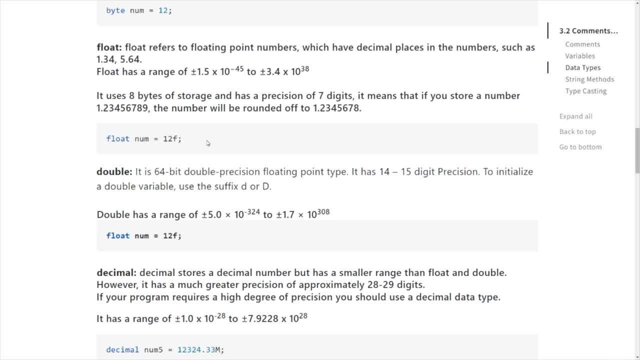 all right if you are storing a numbers. all right if you are storing a numbers like this, like this, like this, so it will be rounded off. all right it, so it will be rounded off. all right it, so it will be rounded off. all right, it would be rounded off. 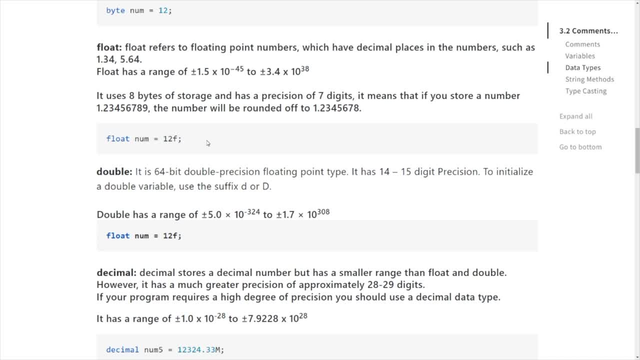 would be rounded off, would be rounded off to to to one point two, three, four, five. one point two, three, four, five. one point two, three, four, five, six, seven, eight, six, seven, eight, six, seven, eight. all right, so it would be rounded off to. all right, so it would be rounded off to: 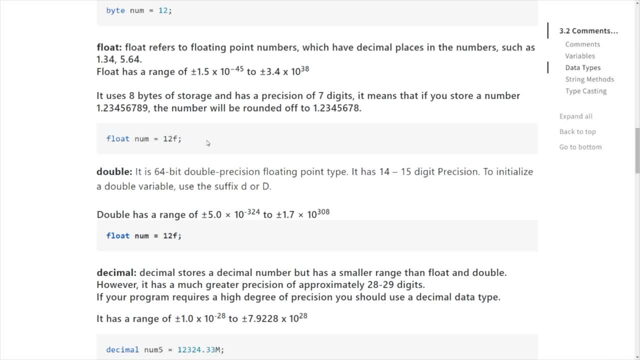 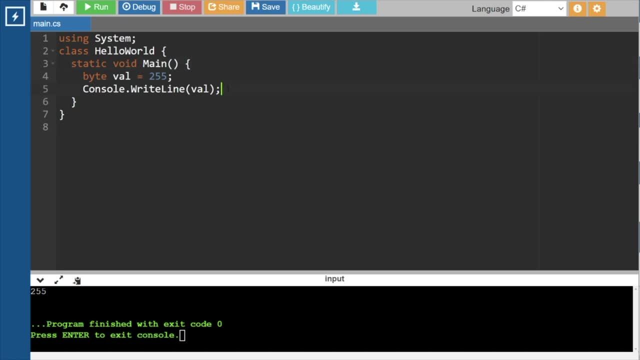 all right, so it would be rounded off to this, all right, so let's this all right. so let's this all right. so let's learn how to initialize this float. learn how to initialize this float. learn how to initialize this float: variable, variable, variable, right, let's learn to do so. 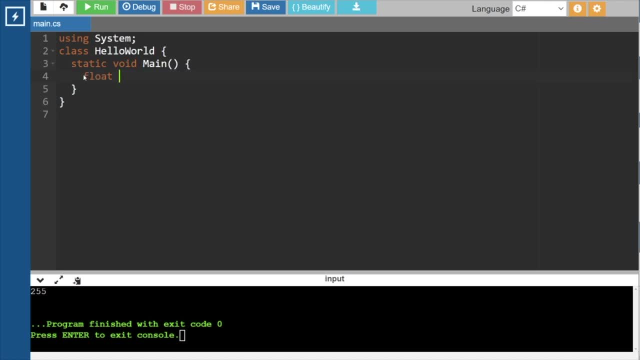 right, let's learn to do so. right, let's learn to do so. so float: all right. so float: all right. so float, all right, float float. float value equals, value equals, value equals- all right, float value equals- all right. float value equals- all right, float, value equals. let's give some sort of uh. 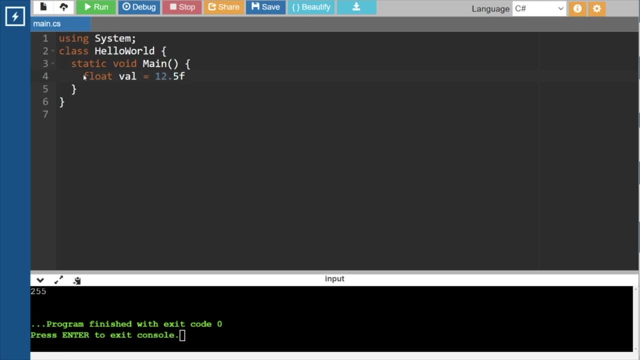 let's give some sort of uh, let's give some sort of uh. decimal value that is 12.5, decimal value, that is 12.5, decimal value that is 12.5, and also add a suffix, and also add a suffix, and also add a suffix f. all right, then, what the suffix? 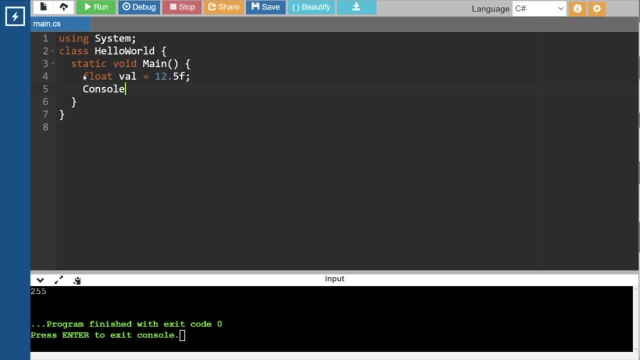 f. all right, then. what the suffix f? all right, then, what the suffix uh f does. is it tells that it is a uh f does? is it tells that it is a uh f does? is it tells that it is a floating point value? floating point value. floating point value. now, by default. all right, by default, the. 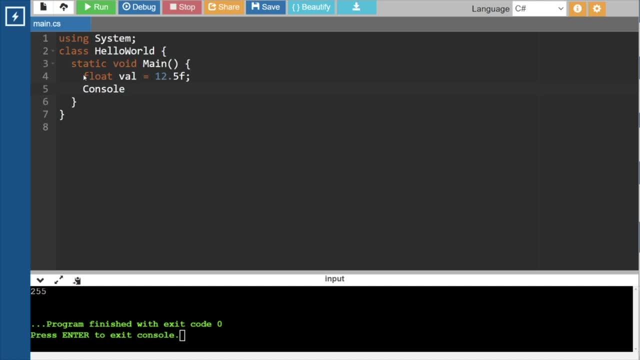 now by default, all right, by default. the now by default, all right, by default. the val, the decimal values: all right, the val, the decimal values- all right. the val, the decimal values- all right. the decimal values are in double. decimal values are in double. decimal values are in double, all right, are in the format of double. so 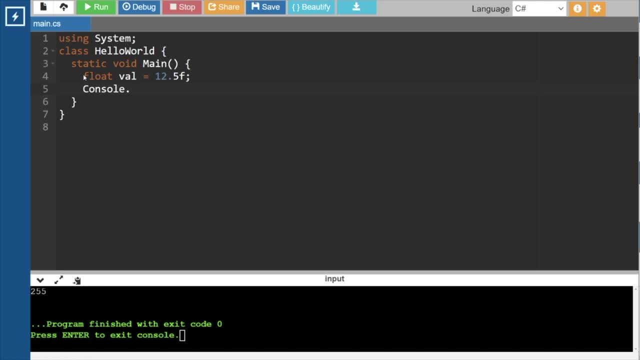 all right are in the format of double. so all right are in the format of double. so it is always recommended to, it is always recommended to, it is always recommended to give f in the uh back of give f in the uh back of give f in the uh back of float, uh, float numbers. all right. 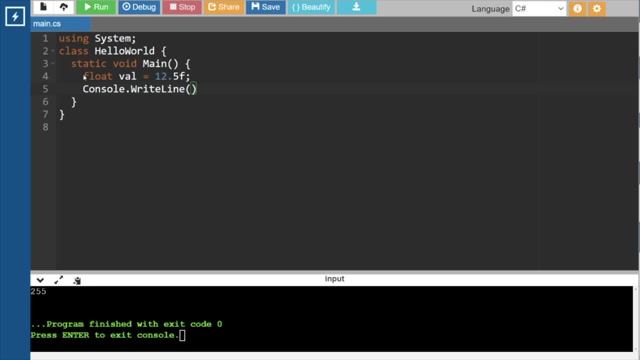 float- uh float numbers. all right, float uh float numbers. all right, floating point numbers. so well, let's try and print it out. all so well, let's try and print it out. all. so well, let's try and print it out. all right, see, it is printing 12.5. now let's try it. 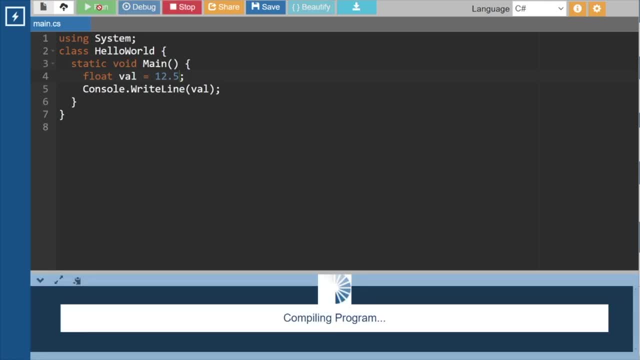 see it is printing 12.5 now, let's try it. see it is printing 12.5 now, let's try it. try it out without the f suffix. all try it out without the f suffix. all try it out without the f suffix, all right. 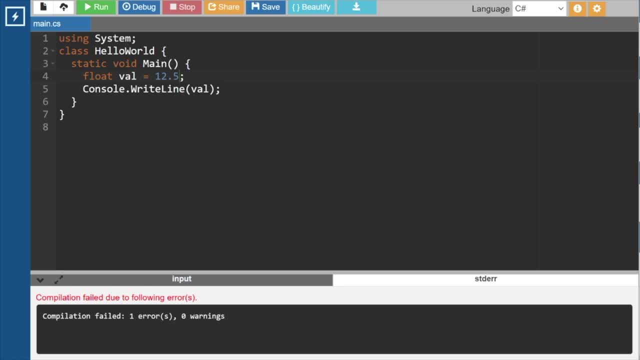 right, right. let's see what happens it is giving us. let's see what happens it is giving us. let's see what happens it is giving us error. the uh error, the uh error, the uh. the reason is because the the b means. the reason is because the the b means. 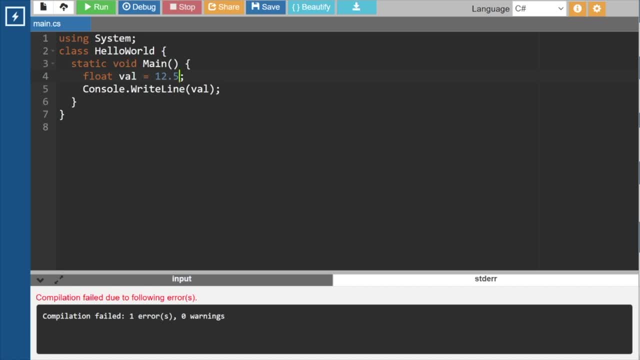 the reason is because the the b means these decimal values. all right by these decimal values. all right by these decimal values, all right by default. these decimal values by default, default, these decimal values by default, default, these decimal values by default are in, are in, are in, uh, double, all right, are in the type of 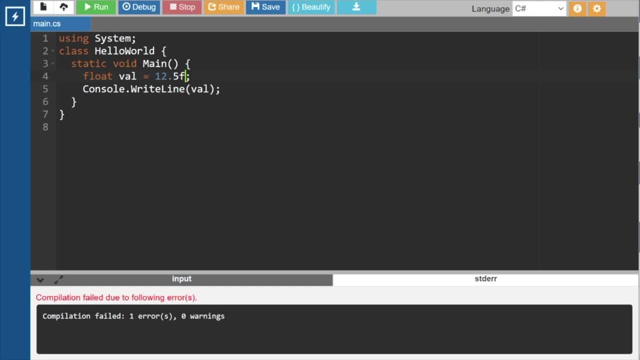 uh double, all right. are in the type of: uh double, all right are in the type of double. so it is always double, so it is always double. so it is always recommended, recommended, recommended to to to uh you, uh add, uh you, uh add, uh you, uh add. f suffix. 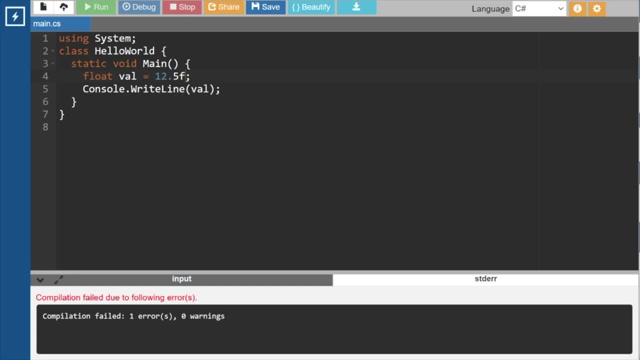 f suffix, f suffix at the last of, at the last of, at the last of float variables: right float variables, right float variables, right. so that's what, so, that's what, so that's what it is all right, so as simple as that. it is all right, so as simple as that. 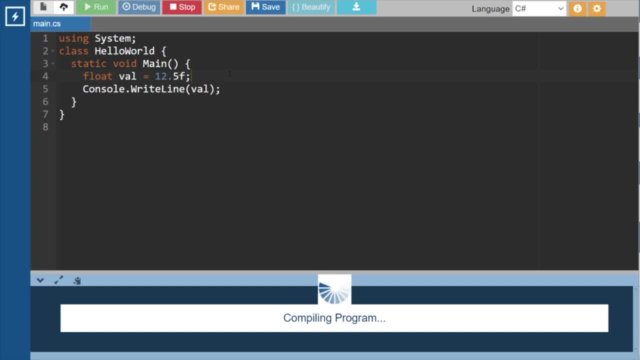 it is all right. so as simple as that. so yeah, so yeah, so yeah. let's uh, let's see all right. let's uh, let's see all right, let's uh, let's see all right, let's see other data types too. that is: let's see other data types too. that is. 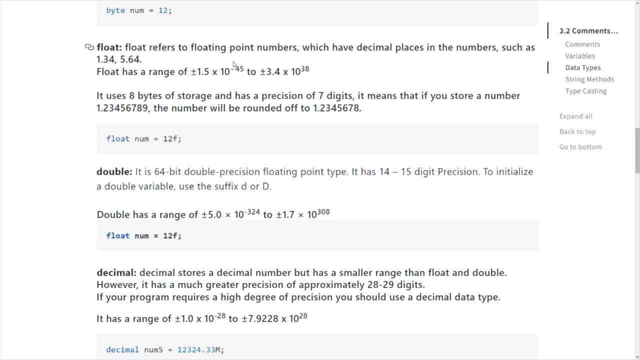 let's see other data types too. that is double, all right. let's see double, all right. let's see double, all right. let's see double. so, double, so, double. so, as we have learned about float all as we have learned about float all as we have learned about float, all right. 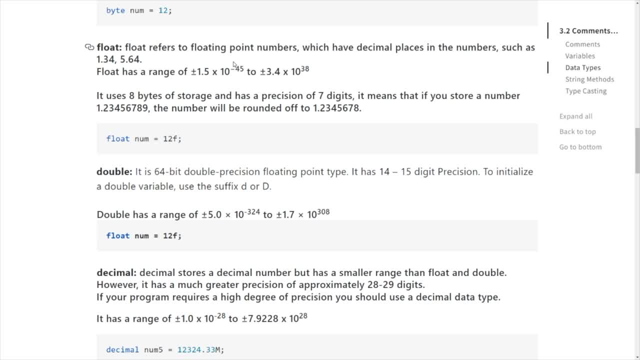 right, right. it is, uh a really great data type to be. it is, uh, a really great data type to be. it is, uh, a really great data type to be used. all right, used, all right, used, all right. another is a double all right, uh, it has. another is a double all right, uh, it has. 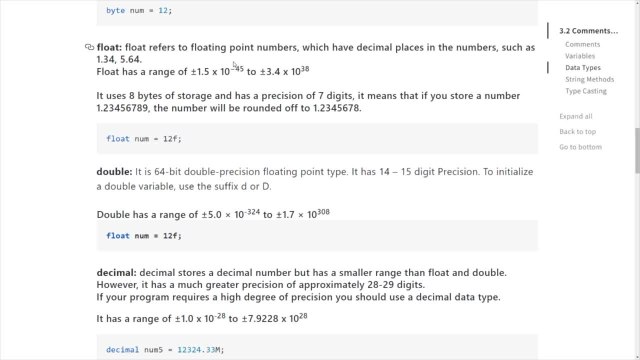 another is a double. all right, uh, it has a higher range, a higher range, a higher range. all right, this double has a higher range. all right, this double has a higher range. all right, this double has a higher range. and uh and uh and uh. a good precision, all right, a good. 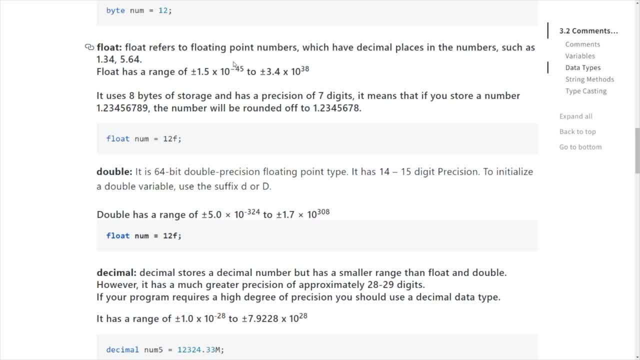 a good precision, all right. a good, a good precision, all right, a good precision, precision, precision. so double all right. what is a double all, so double all right. what is a double all, so double all right. what is a double all right? see, double is also a data type. 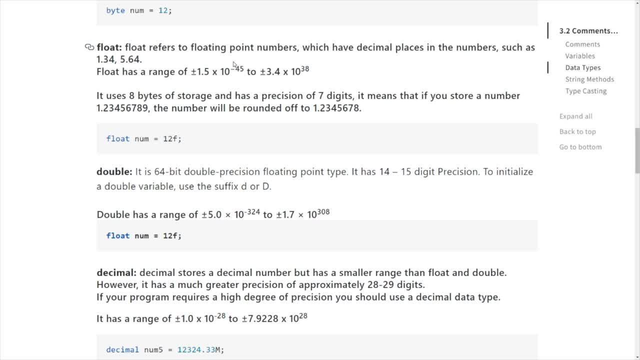 right, see, double is also a data type. right, see, double is also a data type. and and and it is a 64-bit. all right, it is a 64-bit. all right, it is a 64-bit. it is a 64-bit. all right, it is a 64-bit. double precision floating point type. 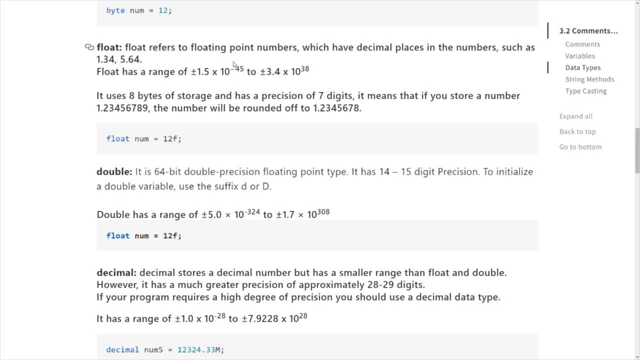 double precision floating point type. double precision floating point type. all right, all right, all right. and uh, it has a precision of 14 to 15. and uh, it has a precision of 14 to 15. and uh, it has a precision of 14 to 15 digit. all right. 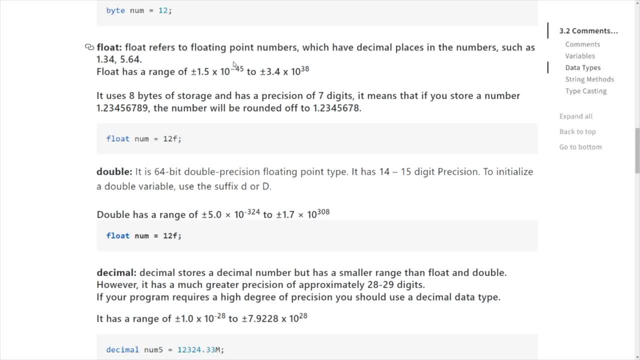 digit. all right digit, all right it. it has a good precision of around 14 it. it has a good precision of around 14 it. it has a good precision of around 14 to 15 digit to 15 digit to 15 digit and also all right also to initialize a. 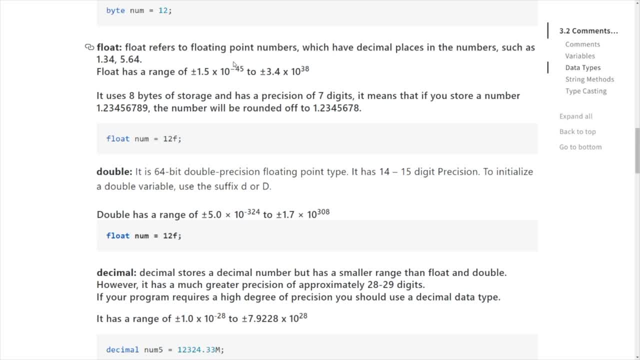 and also all right also to initialize a and also all right also to initialize a double variable, double variable, double variable. we have to use the suffix small d. we have to use the suffix small d. we have to use the suffix small d or capital d, all right. similarly, in: 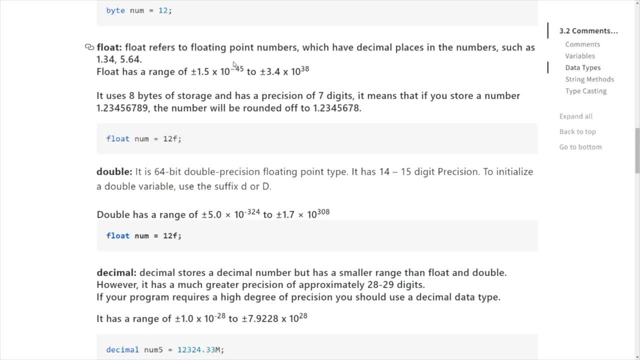 or capital d, all right, similarly in or capital d: all right, similarly in float also. we can use capital f, but i use float also. we can use capital f, but i use float also. we can use capital f, but i use smaller, smaller, smaller, all right, okay, uh, so here in the example: 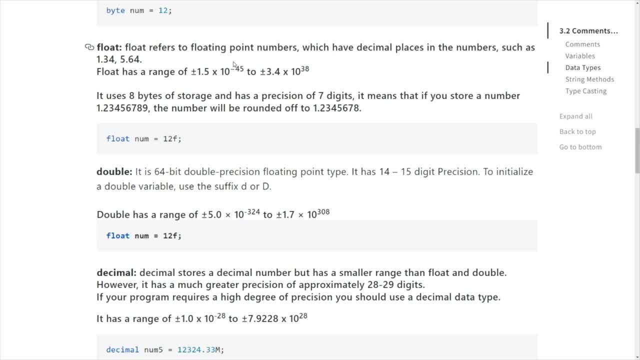 all right, okay, uh. so here in the example: all right, okay, uh. so here in the example, i guess, i guess, i guess i did a mistake, uh, i would fix this issue. i did a mistake, uh, i would fix this issue. i did a mistake, uh, i would fix this issue. all right here. you can see in the 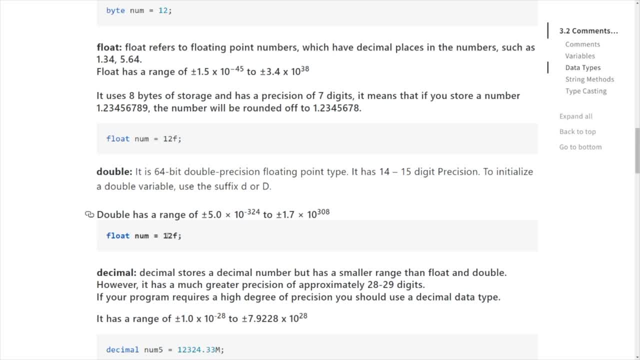 all right here. you can see in the all right here. you can see in the example i gave example. i gave example. i gave: float num equals 12f, but don't worry. in float num equals 12f, but don't worry. in float num equals 12f, but don't worry, in the in the final node that would be. 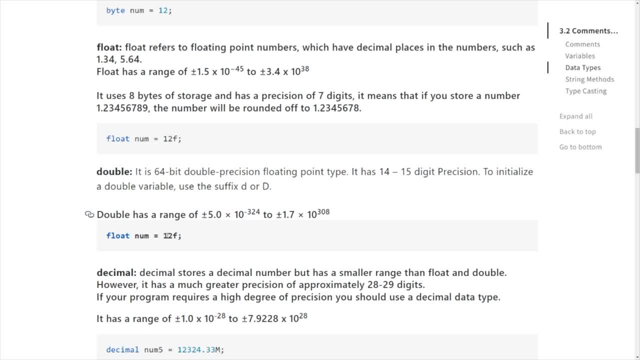 the in the final node, that would be that you would be getting all right, i that you would be getting all right, i that you would be getting all right, i would be, would be would be: i'll be fixing this issue all right, but i'll be fixing this issue all right, but. 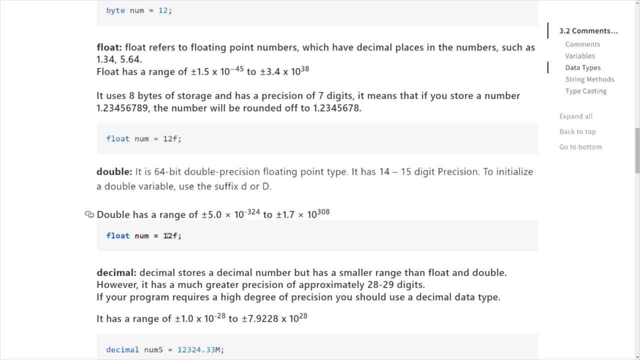 i'll be fixing this issue, all right, but for now, uh, i will show you the actual. for now, uh, i will show you the actual. for now, uh, i will show you the actual example. all right, i will show you that example. all right, i will show you that. 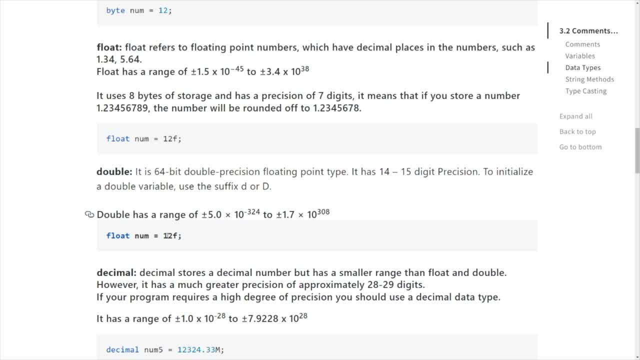 example. all right, i will show you that example. i'm really sorry about this example. i'm really sorry about this example. i'm really sorry about this mistake, mistake, mistake. but uh, in the actual uh note this issue. but uh, in the actual uh note this issue. but uh, in the actual uh note this issue will be fixed. 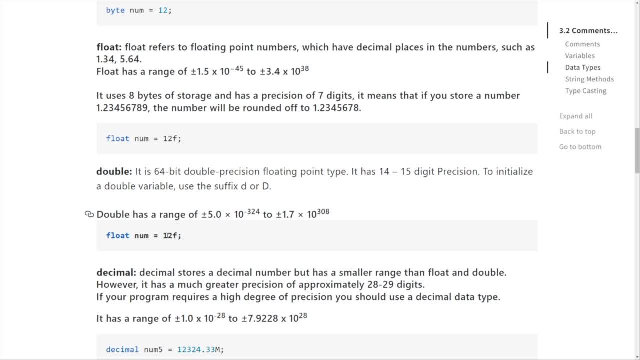 will be fixed. will be fixed. all right, uh. so the range all right. so all right, uh. so the range all right. so all right, uh. so the range all right. so double has a range of uh. double has a range of uh. double has a range of uh plus my uh plus minus 5.0. 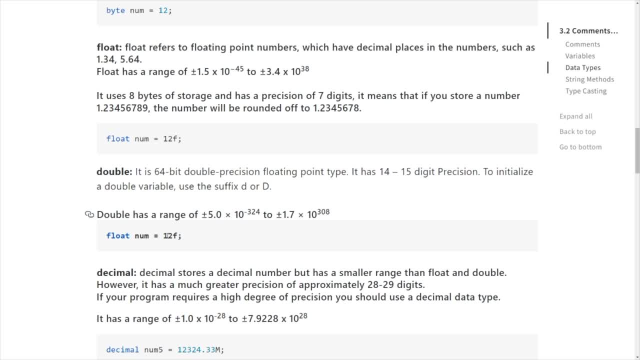 plus my uh plus minus 5.0. plus my uh plus minus 5.0 into 10 to the power, minus 324 into 10 to the power, minus 324 into 10 to the power, minus 324. 2 plus minus 1.7 into 10 to the power. 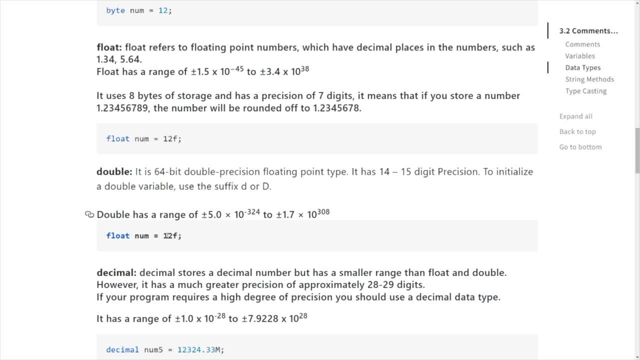 2 plus minus 1.7 into 10 to the power. 2 plus minus 1.7 into 10 to the power 308- all right, so let's try it out. let's 308- all right, so let's try it out, let's. 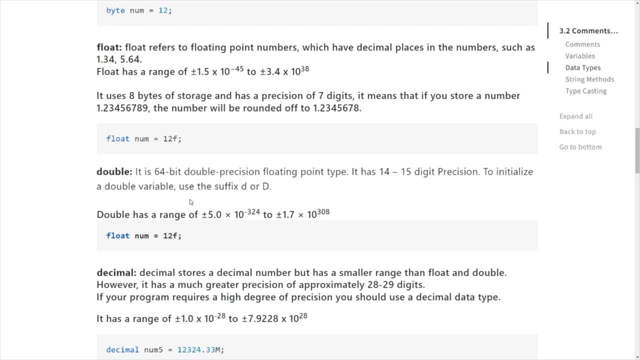 308. all right, so let's try it out. let's try this, try this. try this double. all right, try this double out. double, all right, try this, double out, double. all right, try this double out. so n let's get to the uh. so n let's get to the uh. 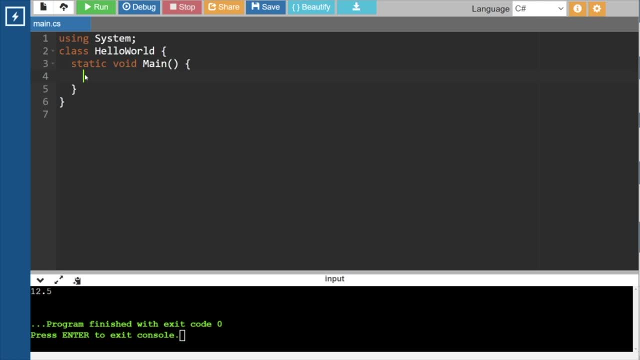 so n let's get to the uh editor, of course all right, and let's editor, of course all right, and let's editor, of course all right, and let's write, write, write, double, all right, double, all right, double, all right. num equals num equals num equals 12.5, all right. 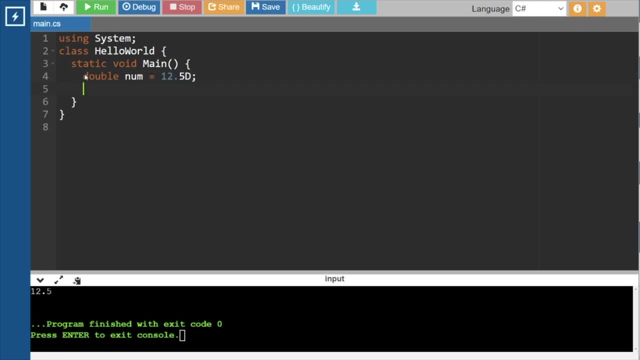 12.5, all right. 12.5, all right, d okay, d okay, d okay. and then console, and then console, and then console, dot log, dot log, dot log. oh sorry, not consolelog. i'm always, oh sorry, not consolelog. i'm always, oh sorry, not consolelog. i'm always writing this. 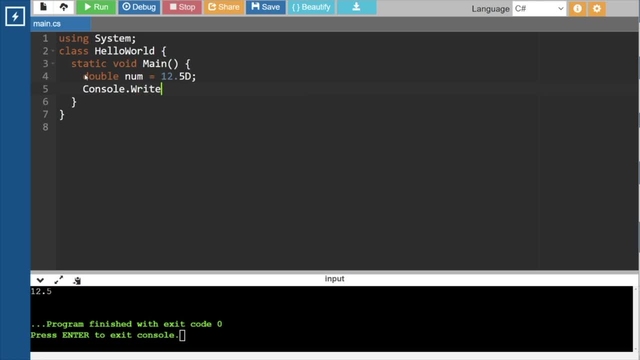 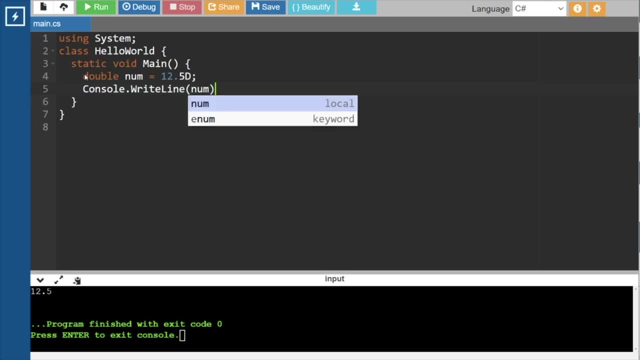 we do debuglog, so it's like: uh it, we do debuglog, so it's like: uh it, it is habituated to me, it is habituated to me, it is habituated to me, so, um, yeah, so, um, yeah, so, um, yeah. so let's try and print it out, all right. 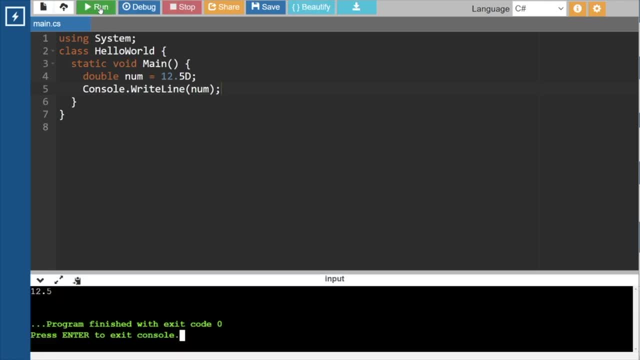 so let's try and print it out. all right. so let's try and print it out. all right, let's say: if it gives any sort of errors, let's say: if it gives any sort of errors, let's say if it gives any sort of errors or runs seamlessly, so we can see that it. 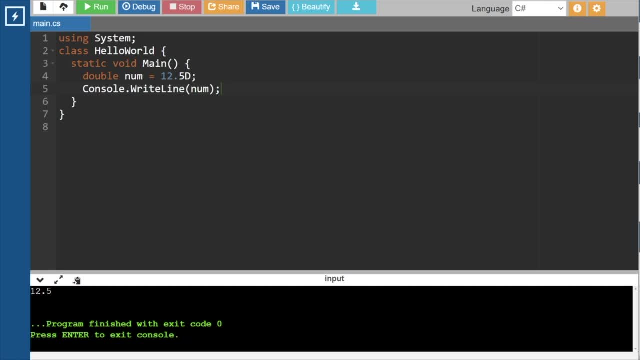 or runs seamlessly, so we can see that it. or runs seamlessly, so we can see that it has rams ran. has rams ran? has rams ran seamlessly? all right, so we have learned seamlessly. all right, so we have learned seamlessly. all right, so we have learned about double data type. all right, we have. 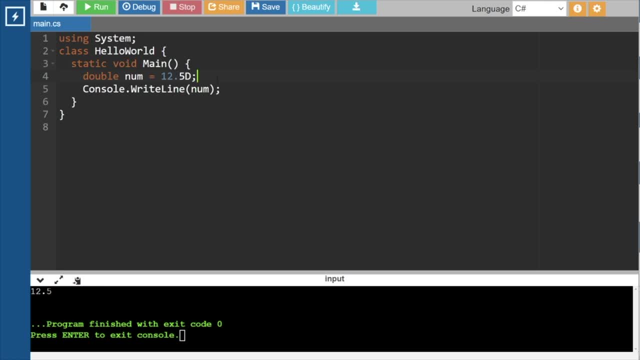 about double data type. all right, we have about double data type, all right. we have learned about float. we have learned, learned about float. we have learned, learned about float. we have learned about into. we have learned about long. we about into. we have learned about long. we about into. we have learned about long. we have learned about. 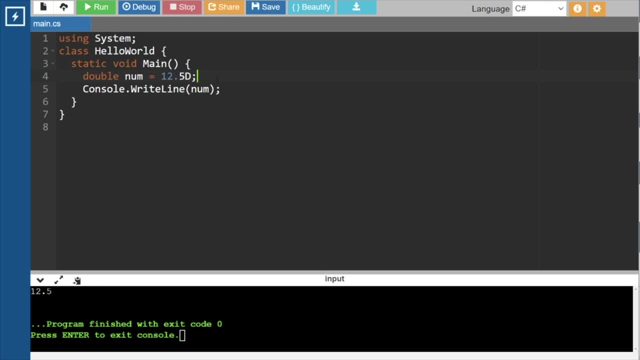 have learned about. have learned about byte. we have learned about float. we have byte. we have learned about float. we have byte. we have learned about float. we have learned about, learned about. learned about double. now it's our time, all right, it is double. now it's our time, all right, it is. 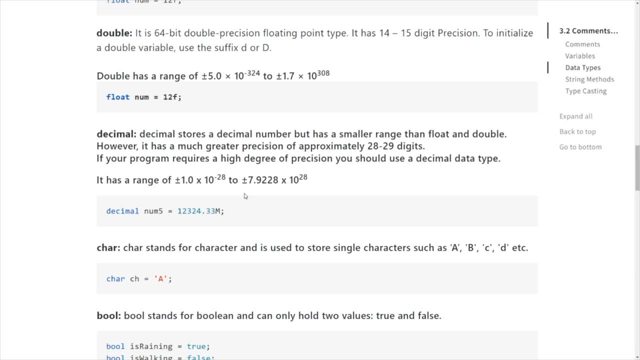 double. now it's our time. all right, it is now. it is our time. now it is our time. all right, it is our time to understand this decimal, to understand this decimal, to understand this decimal. all right, let's understand this decimal. all right, let's understand this decimal. 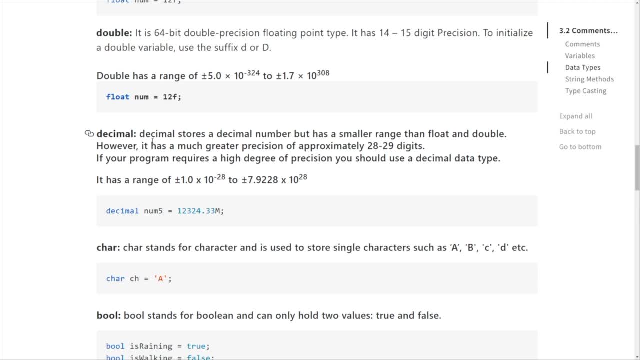 all right, let's understand this. decimal data type, data type, data type: all right, see. decimal is another floating- all right, see. decimal is another floating- all right, see. decimal is another floating point. data type: all right. where you can point data type, all right. where you can point data type, all right. where you can uh store decimal values, all right, even. 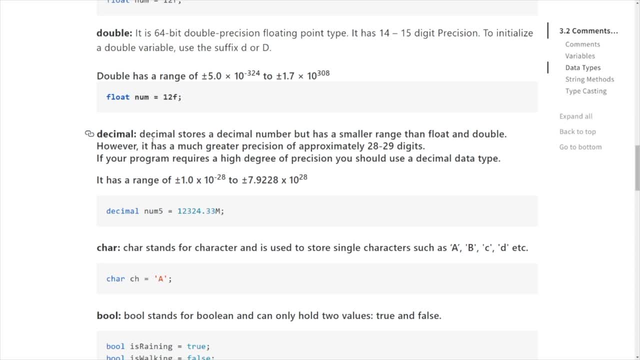 uh store decimal values, all right, even uh store decimal values, all right. even the name suggests the name suggests the name suggests it so, but all right. but this date it so, but all right. but this date it so, but all right, but this date, this decimal, all right, this. 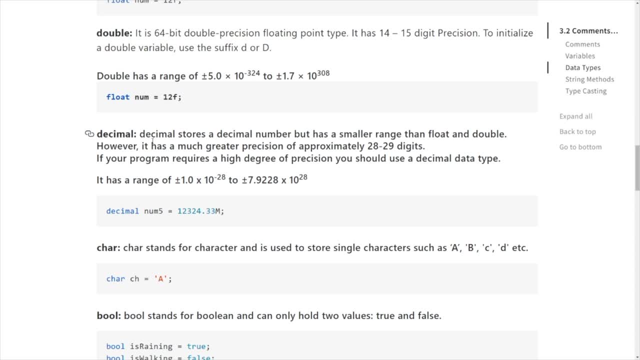 this decimal, all right. this, this decimal, all right. this decimal uh has much greater precision. decimal uh has much greater precision. decimal uh has much greater precision. all right then. all right then. all right then. any other, all right. that is a float or any other? all right, that is a float or. 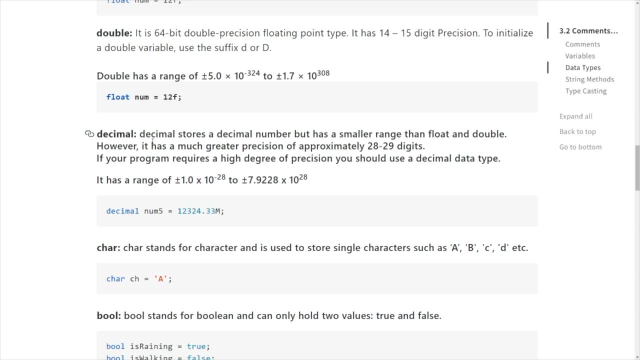 any other, all right, that is a float or double, all right. double, all right, double, all right. the precision of uh float and double is the precision of uh float and double is the precision of uh float and double is lower than, lower than, lower than decimal. all right, so the decimal has. 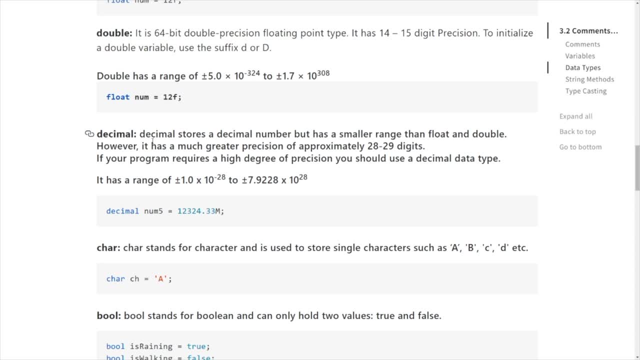 decimal. all right, so the decimal has decimal. all right, so the decimal has better precision. all right. it has a better precision- all right. it has a better precision- all right. it has a greater precision. that is of greater precision. that is of greater precision. that is of approximately 28 to 29 digits, all right. 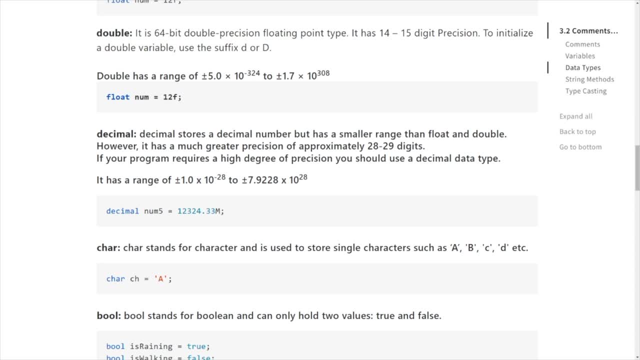 approximately 28 to 29 digits, all right. approximately 28 to 29 digits, all right. approximately 28 to 29. approximately 28 to 29 digits, all right. approximately 28 to 29 digits, all right. so this double uh, this decimal data type. so this double uh, this decimal data type. 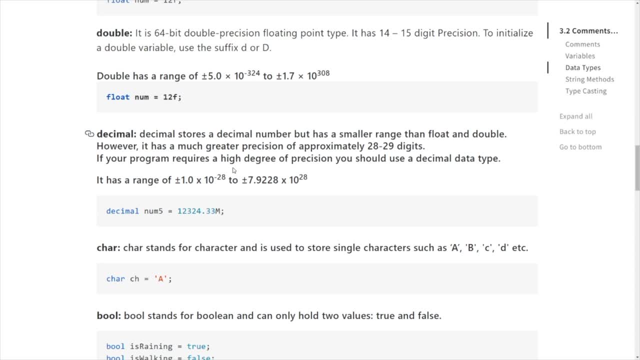 so this double, uh, this decimal data type, all right, has an all right, has an all right, has an? uh greater precision of approximately 28, uh, greater precision of approximately 28, uh, greater precision of approximately 28 to 29 digits, all right, and to 29 digits, all right, and 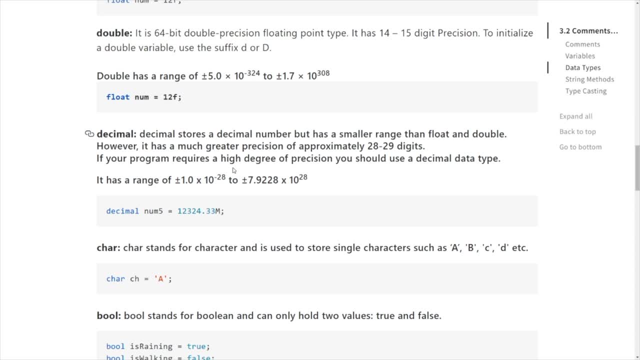 to 29 digits. all right, and it is recommended, all right, it is always. it is recommended. all right. it is always it is recommended. all right, it is always recommended to use the recommended. to use the recommended to use the decimal data type. all right, in spite of. 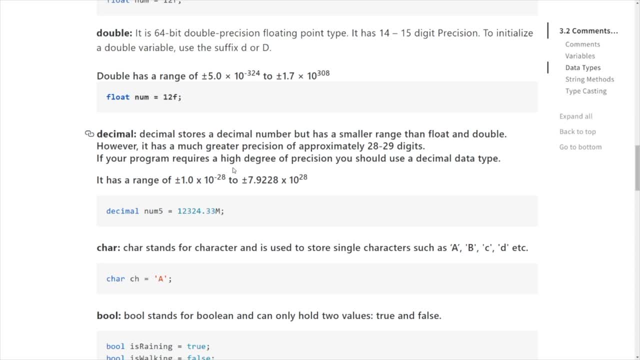 decimal data type. all right in spite of decimal data type. all right in spite of double or double, or double or float. if you want a greater precision float. if you want a greater precision, float. if you want a greater precision, all right, if you want a greater precision. 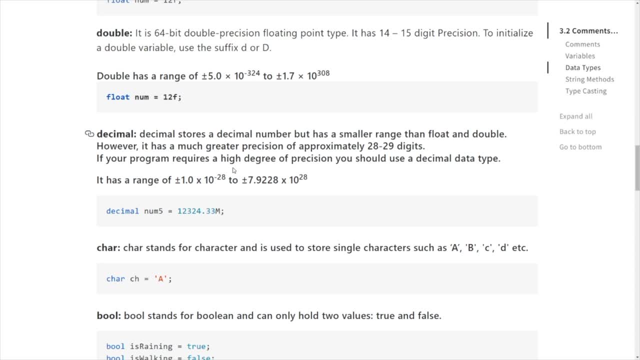 all right, if you want a greater precision, all right, if you want a greater precision, then you should use decimal. all right, then you should use decimal. all right, then you should use decimal. all right, but the range, but the range of decimal, but the range, but the range of decimal. 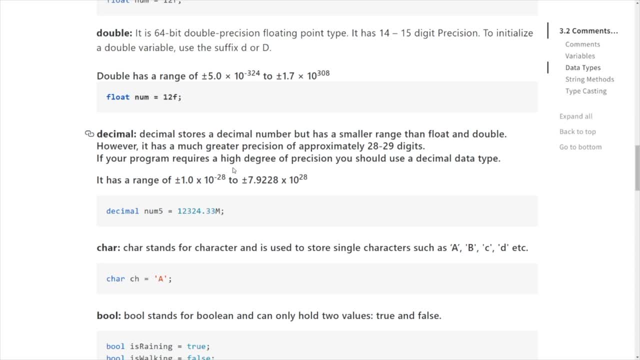 but the range, but the range of decimal data type, data type data type is uh lower than is uh lower than is uh lower than that of double and float. all right, so that of double and float, all right, so that of double and float, all right. so it has basically a range of uh. 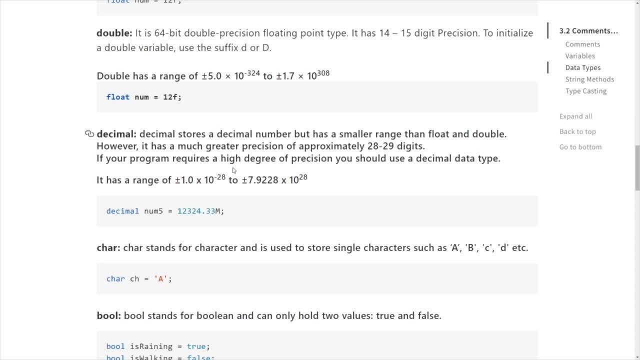 it has basically a range of uh. it has basically a range of uh plus plus minus 1.0 into 10 to the power plus plus minus 1.0 into 10 to the power plus plus minus 1.0 into 10 to the power minus 28. 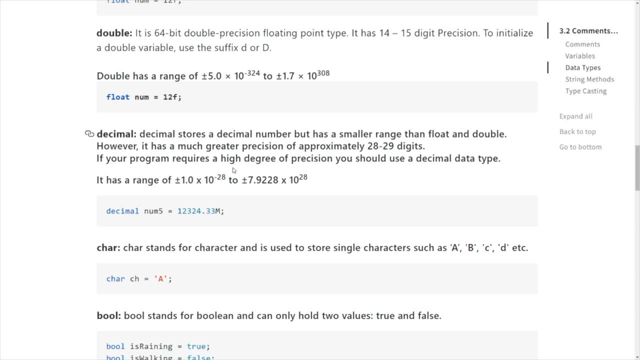 minus 28 minus 28: 2 uh plus minus 7.9228. 2 uh plus minus 7.9228. 2 uh plus minus 7.9228. into 10 to the power 28. so this is the into 10 to the power 28. so this is the. 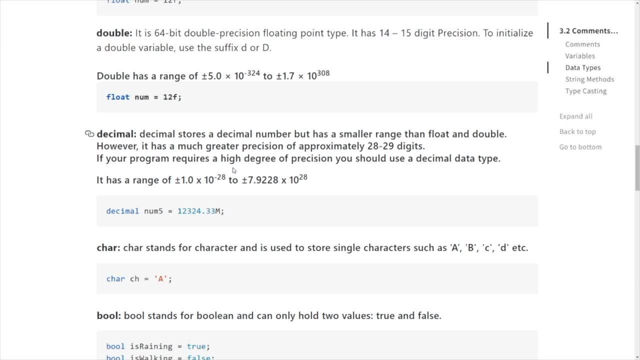 into 10 to the power 28. so this is the range. all right, this is range. all right. this is range, all right. this is the range of decimal data type. all right, the range of decimal data type. all right, the range of decimal data type, all right. similarly, let's um try it out: all right. 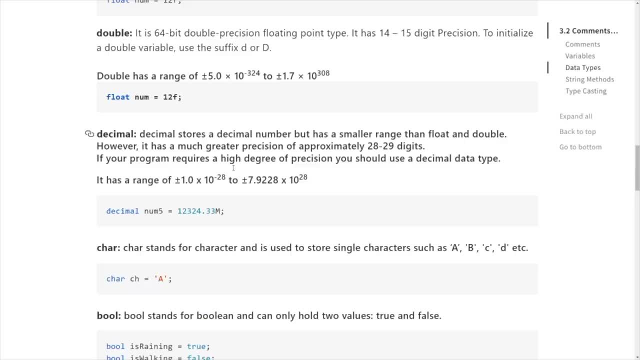 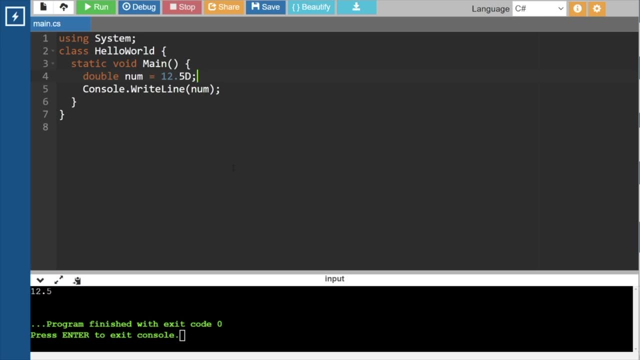 similarly, let's um try it out, all right. similarly, let's um try it out, all right, let's try it out. let's try it out. let's try it out in our code editor, all right. so, uh, in our code editor, all right. so, uh, in our code editor, all right. so, uh, it's very simple. i already included uh. 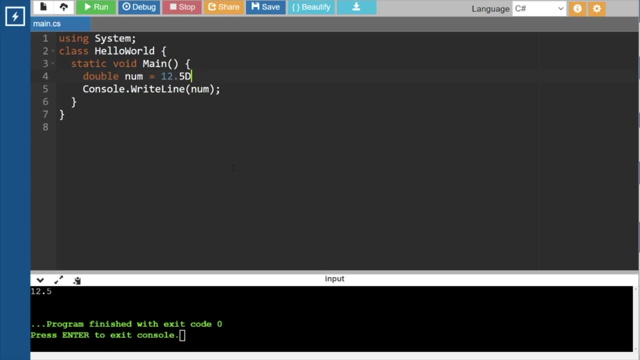 it's very simple. i already included, uh. it's very simple. i already included, uh- the definition right and also the the definition right and also the the definition right and also the example- all right, nothing too, uh too. example. all right, nothing too, uh too example. all right, nothing too, uh. too complicated in here. 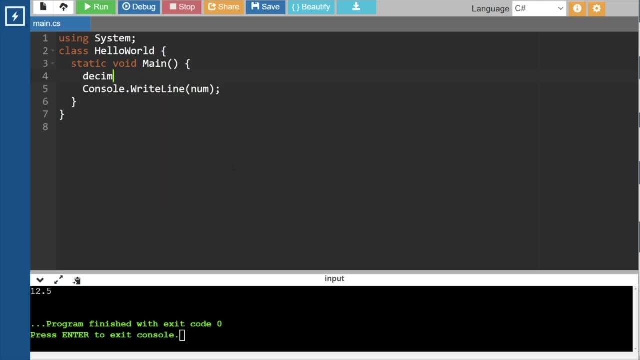 complicated in here. complicated in here. so decimal, so decimal, so decimal, decimal, decimal, decimal, num, num. num equals 25.5, 25.5, 25.5, d, d, d. sorry, the suffix will be m, not d. i'm really sorry, the suffix will be m, not d. i'm really. 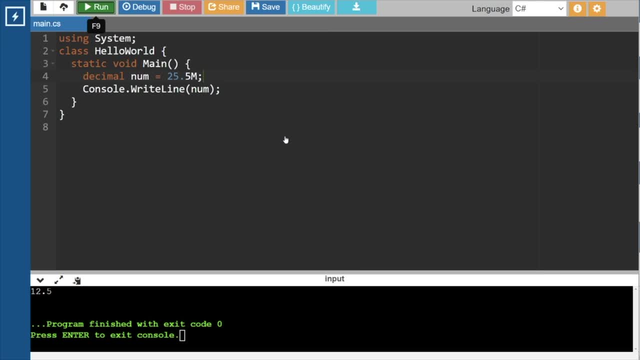 sorry, the suffix will be m, not d. i'm really sorry about that. so the suffix will be sorry about that. so the suffix will be sorry about that. so the suffix will be m. all right, so the suffix for decimal is m. all right, so the suffix for decimal is: 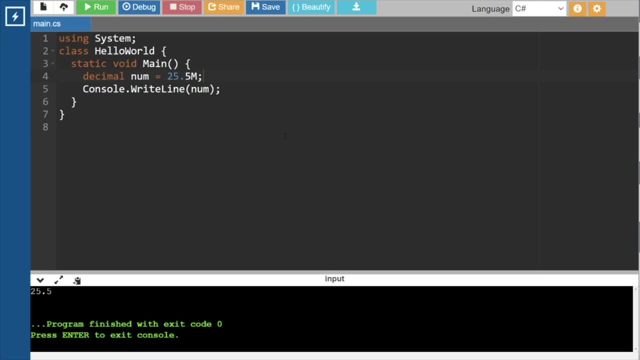 m. all right, so the suffix for decimal is f: m. all right, so the suffix for decimal is f. so this is how we write a. so this is how we write a. so this is how we write a. initialize a decimal data type. all right. initialize a decimal data type, all right. 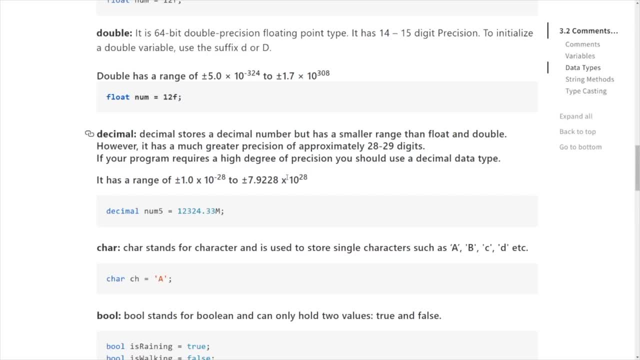 initialize a decimal data type. all right, this is how we do it. this is how we do it. this is how we do it, so so. so, now, as we have learned about uh decimal, now, as we have learned about uh decimal, now, as we have learned about uh decimal data type, now it's our 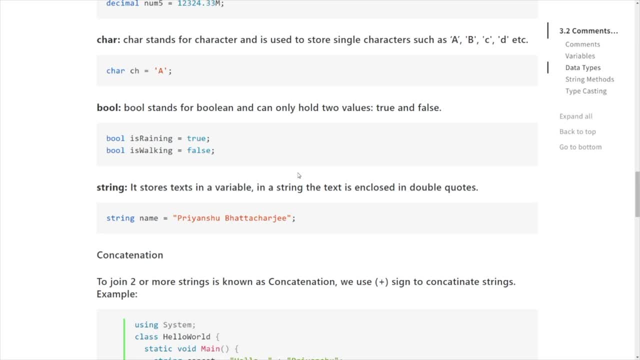 data type. now it's our data type. now it's our time to learn about three other data types. time to learn about three other data types. time to learn about three other data types? all right, that is all right. that is all right. that is cad, bool and string. these are very important. 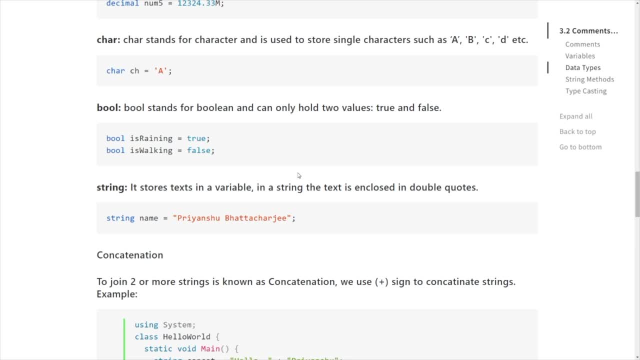 cad, bool and string. these are very important. cad, bool and string. these are very important data types. all right, all of the data type data types. all right, all of the data type data types. all right, all of the data type that i'm teaching you. all right, all of. 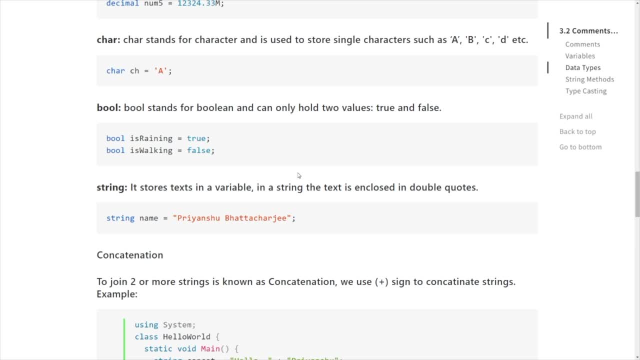 that i'm teaching you all right, all of that i'm teaching you all right. all of them are very important for you to them, are very important for you to them, are very important for you to understand, understand, understand, all right, so, all right, so, all right. so care, all right, care. data type: what does? 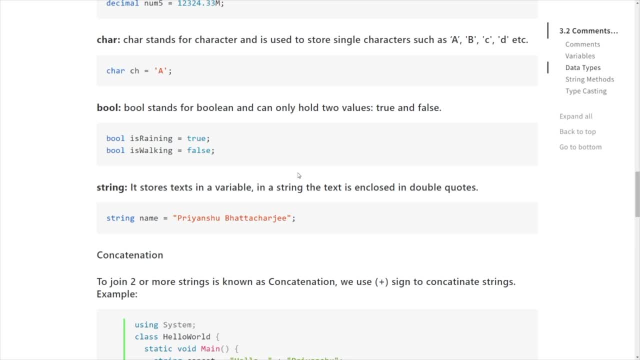 care all right, care data type. what does care? all right, care data type. what does care all right. what is care actually care, care, all right. what is care actually care, care, all right. what is care actually care is a care basically stands for character is a care basically stands for character. 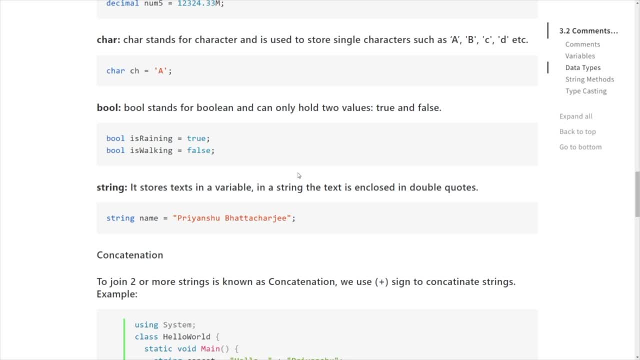 is a care, basically stands for character: all right, or you can say all right, or you can say all right, or you can say letter: all right, a particular letter, all letter, all right. a particular letter: all letter, all right, a particular letter, all right, right, right. so like, like, uh, like a is a particular. 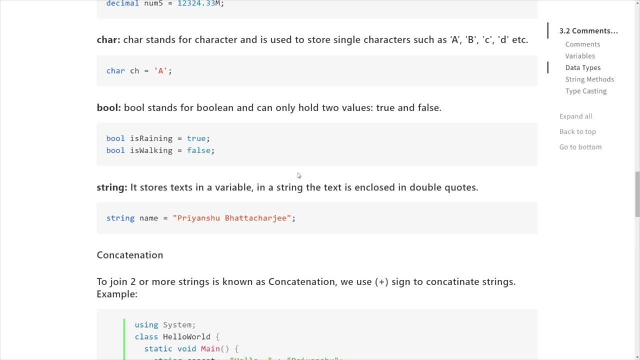 so like like uh, like a is a particular. so like like, uh, like a is a particular letter, or a character letter, or a character letter, or a character like b, like c, like d, all right. like b, like c, like d, all right. like b, like c, like d, all right. so these are characters, all right, these. 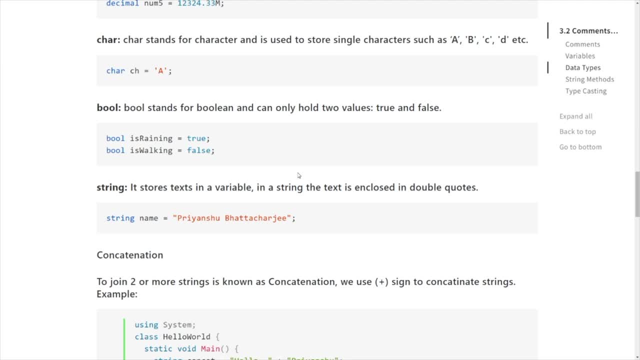 so these are characters. all right, these, so these are characters, all right, these are characters, are characters, are characters. similarly, if you say you have to all similarly, if you say you have to all similarly, if you say you have to, all right. if you want to define any sort of 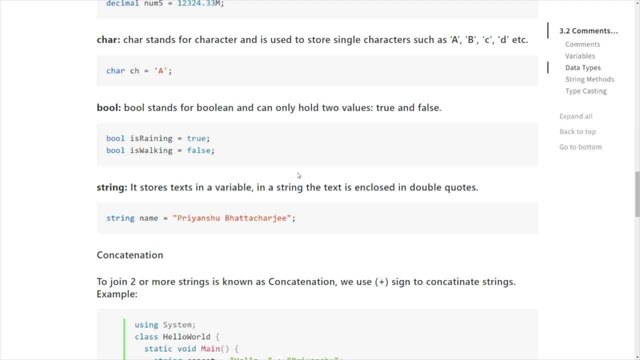 right, if you want to define any sort of right, if you want to define any sort of character in a in a, character in a in a character in a in a our program. how would we do that? all our program? how would we do that? all our program? how would we do that? all right, how would we? 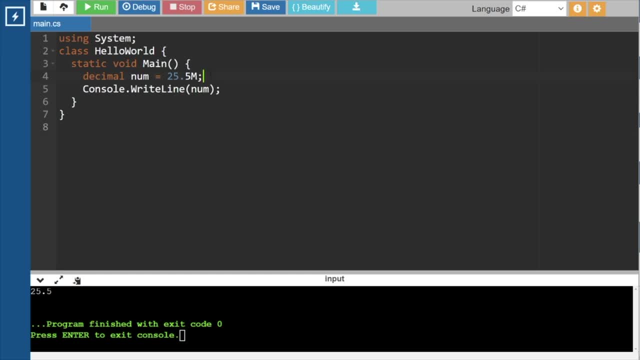 right, how would we do that? all right, how would we right, how would we do that? it's pretty simple, all right, it's do that. it's pretty simple. all right, it's do that. it's pretty simple. all right, it's pretty simple, pretty simple, pretty simple. just write care, all right. uh, also, i'm just write care, all right. uh also, i'm just write care, all right. uh, also, i'm not changing the variable name. i'm going not changing the variable name. i'm going not changing the variable name. i'm going to keep it numb only. to keep it numb only. 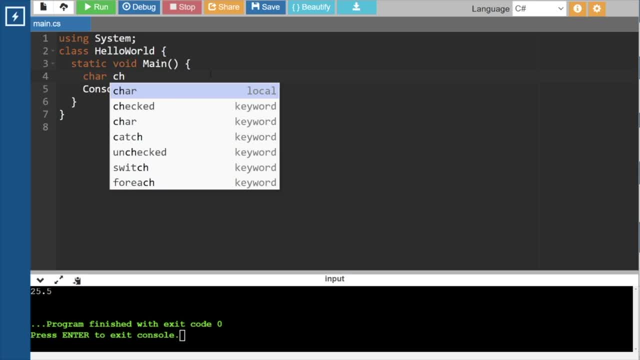 to keep it numb, only all right. or let's say: change it, let's all right. or let's say change it, let's all right. or let's say change it, let's change it all right, change it all right. and let's say: i want to store a character. 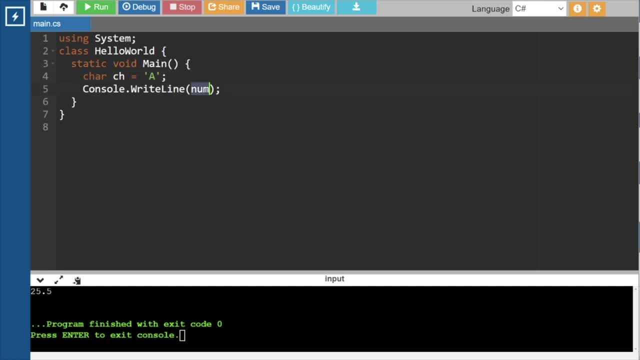 and let's say i want to store a character. and let's say i want to store a character all right, called a all right, all right, called a all right, all right, called a all right. and if i put ch, all right, uh, and if i put ch, all right, uh. 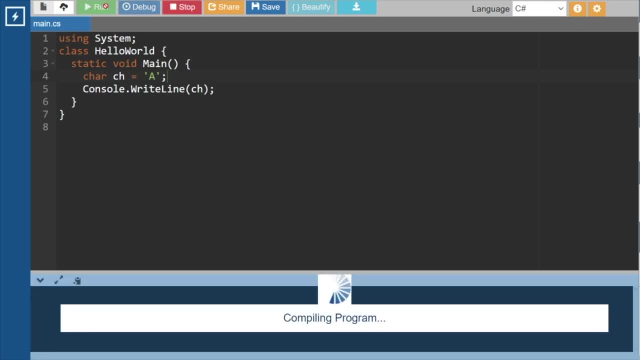 and if i put ch all right, uh, now i want to print it all right. so now i want to print it all right, so now i want to print it all right. so let's see it gets print on printed, or let's see it gets print on printed, or? 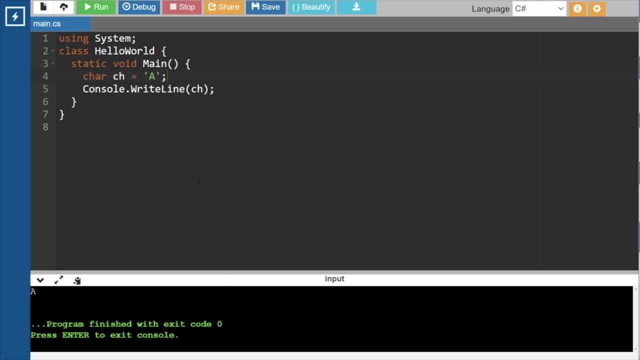 let's see, it gets print on printed or not. so here it is being printed. one more not so. here it is being printed, one more not so here it is being printed. one more thing: there are some details that you thing. there are some details that you thing there are some details that you should look out for. 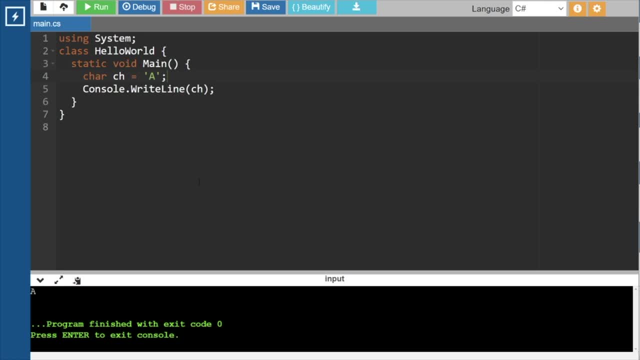 should look out for. should look out for first of all, all right. if you are a first of all, all right. if you are a first of all, all right. if you are a character, all right. a character data character, all right. a character data character, all right. a character data type can only store. 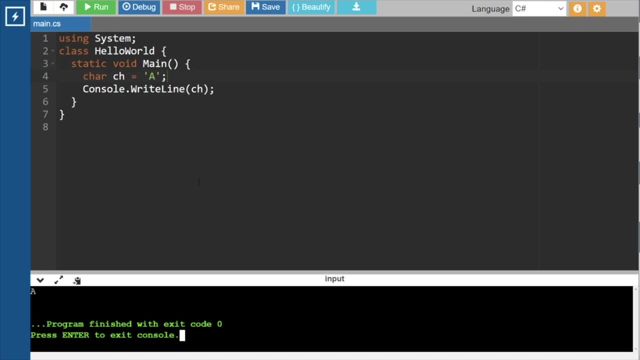 type can only store. type can only store only one letter, all right. it can't store only one letter, all right. it can't store only one letter, all right. it can't store a- b, all right, a, b, c. it can only store. a- b, all right. a, b, c. it can only store. 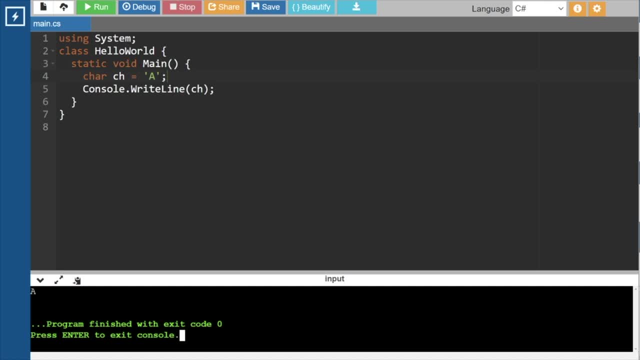 a, b, all right. a, b, c. it can only store one letter, all right. another thing: you- one letter, all right. another thing: you, one letter, all right. another thing you have to uh put in your mind is that have to uh put in your mind is that have to uh put in your mind is that whenever we write a character, we have to 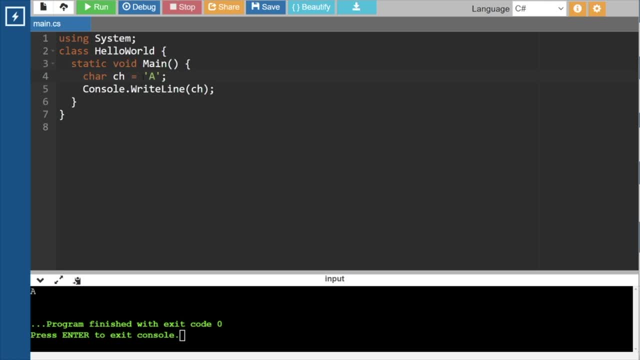 whenever we write a character, we have to, whenever we write a character, we have to enclose that particular uh letter, enclose that particular uh letter, enclose that particular uh letter in single brackets, like just like we did in single brackets. like just like we did in single brackets, like just like we did in here. all right, so similarly, let's try. 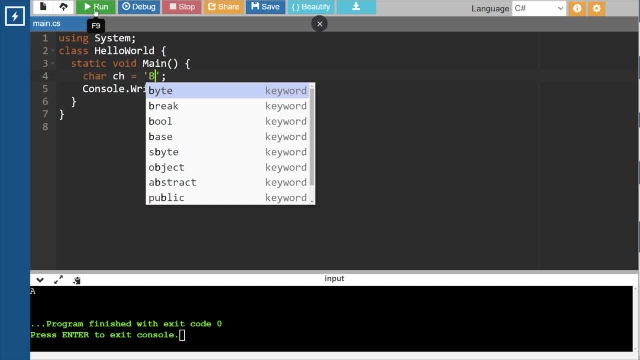 in here: all right. so similarly, let's try in here: all right. so similarly, let's try: another out that is b, another out that is b, another out, that is b all right, and all right and all right, and let's, let's, let's run this program, all right. 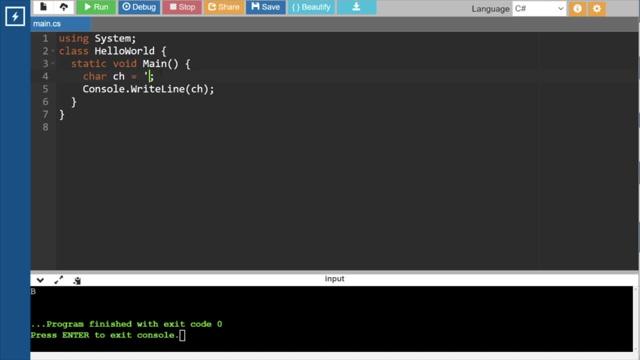 run this program. all right, run this program all right. see it is printing b all right now. see it is printing b all right now. see it is printing b all right now. what if all right if we? what if we try? what if all right if we? what if we try? 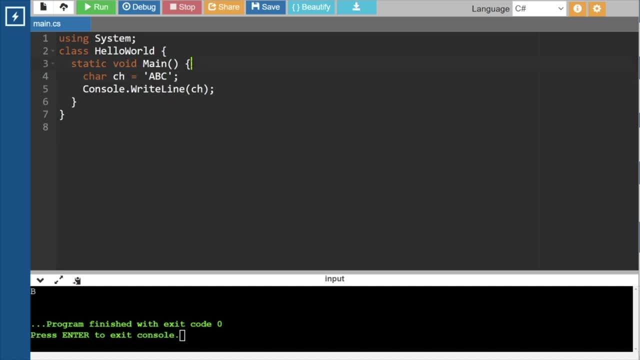 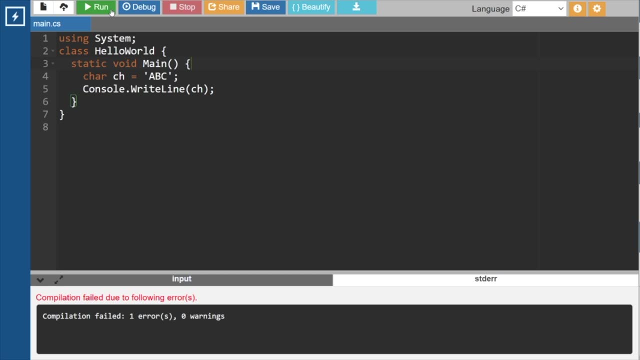 what if? all right, if we, what if we try to add, to add, to add multiple, all right, add multiple, uh, multiple, uh, multiple, uh letters in it. so here you can see, it is letters in it. so here you can see, it is letters in it. so here you can see, it is giving us error because, of course, this: 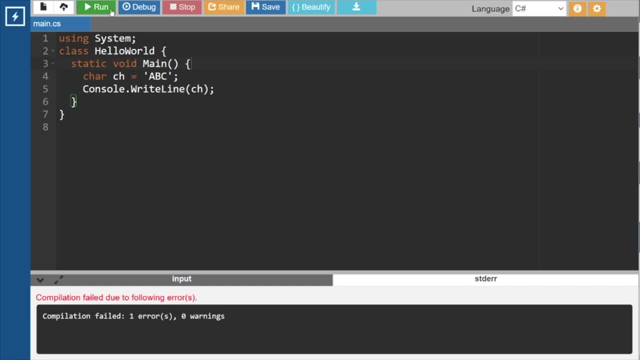 giving us error because of course this giving us error, because of course this is a single, this can only store a single, is a single, this can only store a single, is a single, this can only store a single character. it can only store us character, it can only store us. 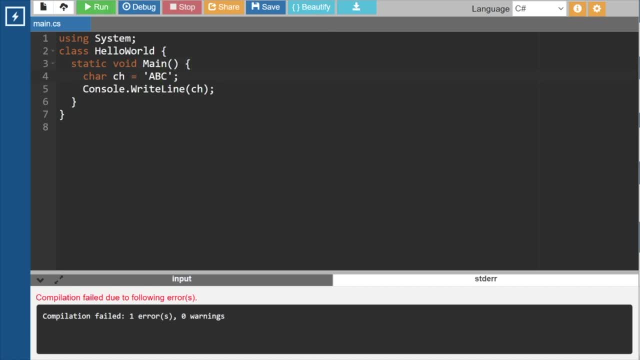 character. it can only store us, uh like only one, only one, uh like only one, only one, uh like only one, only one character all right. so that's, we are character all right. so that's, we are character all right. so that's, we are giving it to it. that is only one. 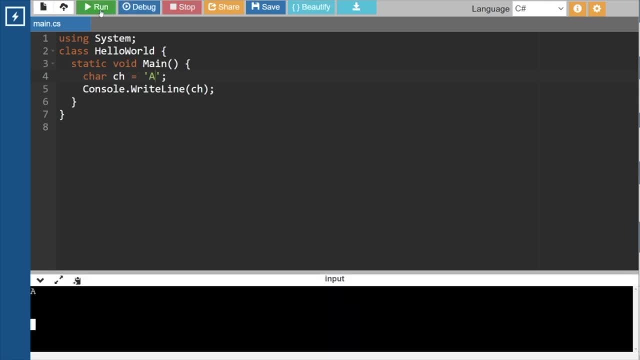 giving it to it, that is only one. giving it to it, that is only one character. so remember character. so remember character. so remember uh. if you, if you want to store only a uh, if you, if you want to store only a uh, if you, if you want to store only a single character, then always go for. 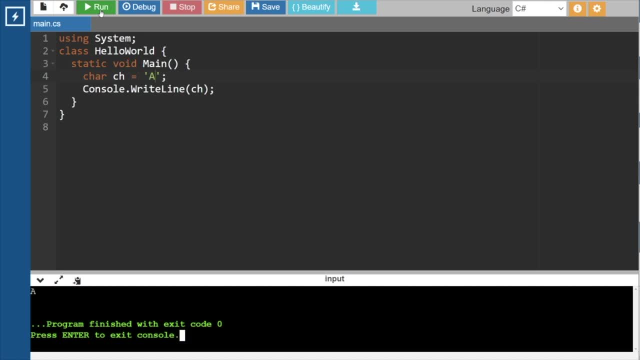 single character, then always go for single character, then always go for care. all right care, all right care, all right now, now, now, our next. all right, uh, let's see what is our next. all right, uh, let's see what is our next. all right, uh, let's see what is our next, yeah. 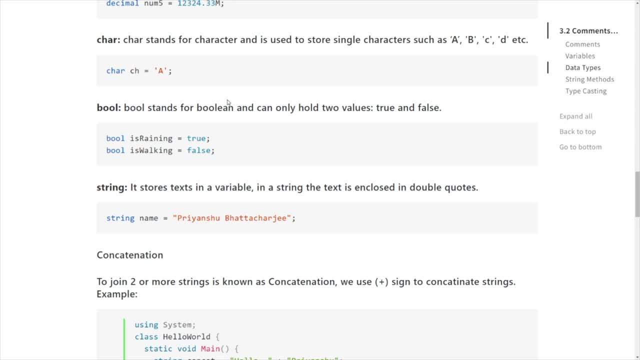 our next. yeah, our next. yeah, our next topic is bool. all right, see, our next topic is bool. all right, see, our next topic is bool. all right, see. bool, uh, bool, uh, bool. uh is stands for boolean. all right, it is the. is stands for boolean. all right, it is the. 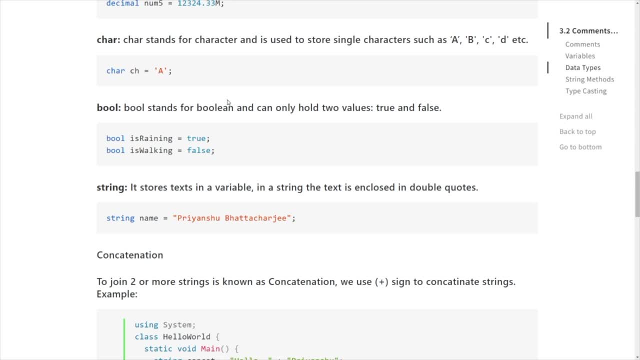 is stands for boolean. all right, it is the short for boolean, short for boolean, short for boolean. so bool data types. uh can only contain so bool data types. uh can only contain so bool data types. uh can only contain true or false. all right, true or false, all right. 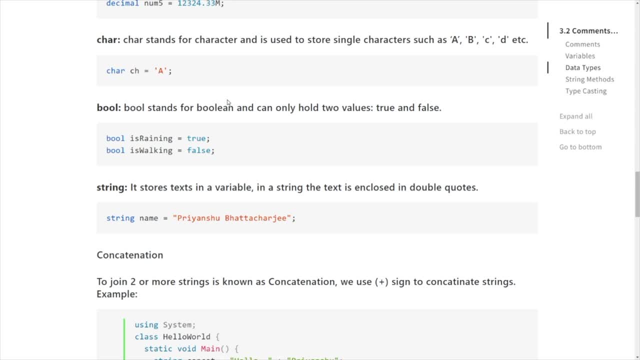 true or false, all right. true means on all right. true means it. true means on all right. true means it. true means on all right. true means it is executable. all right true means uh is executable. all right true means uh is executable. all right true means uh, it will work it. true means on. 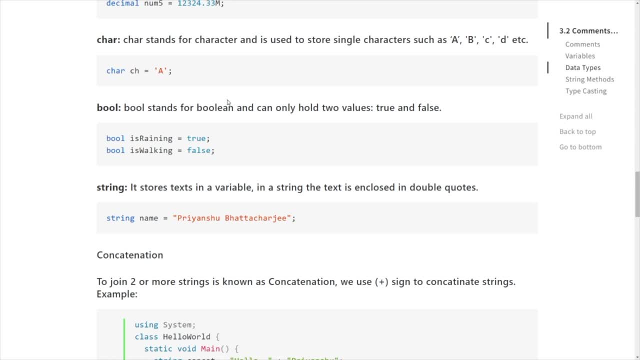 it will work it. true means on, it will work it. true means on and false means, and false means and false means off. all right, you can say it is off off. all right, you can say it is off off. all right, you can say it is off, right, right. so if, if you take an example, 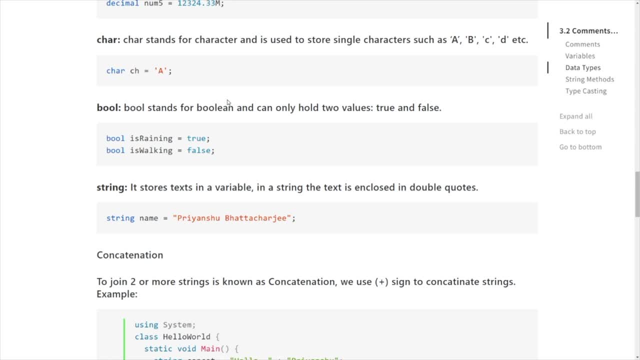 right, right. so if, if you take an example, right, right. so if, if you take an example of a circuit, all right. or you can say, turn on the light, all right, the value of that particular switch is becoming true, all right. or you can say: the value of that particular switch is becoming on and because the the value is true. 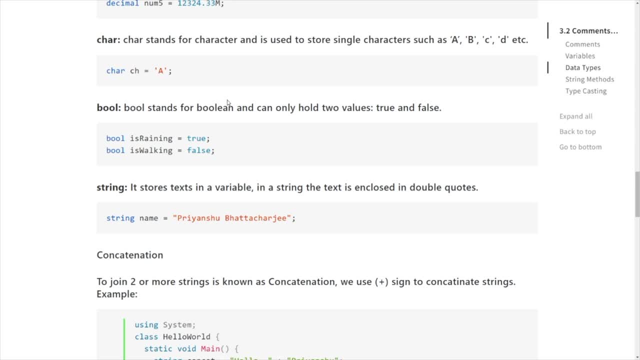 all right, because the value is true. the current is flowing, all right. the current is flowing through the circuit and lighting and putting the lights on, all right, and and it is putting the putting the lights on. similarly, if you turn off the switch, all right. similarly, if you turn off the switch. 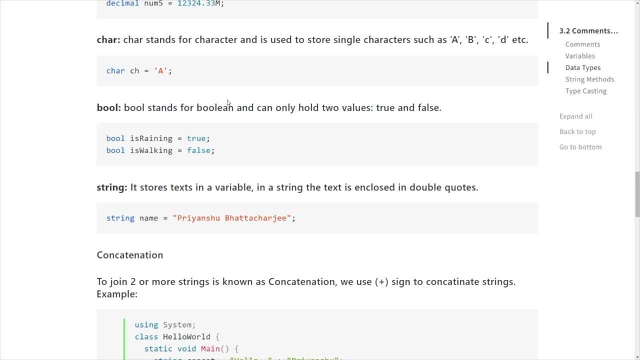 then the value of the switch will be false and no current will pass through it. all right, it will just terminate. so that's what true and false is in terms of programming. similarly, how would, how can we basically, how can we basically initialize it? i have also given you example, all right, and i will. 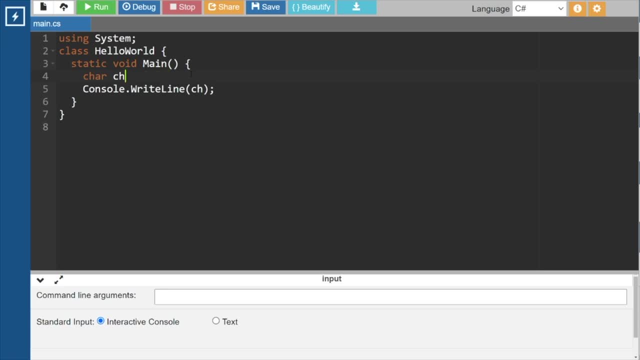 also show you how to do that. all right. so bool is uh running. so am i running? no, i'm sitting right, i'm, i'm, i'm sitting right. so if i print it now, all right, if i print it now, let's see what happens. see, it is uh printing us, true. 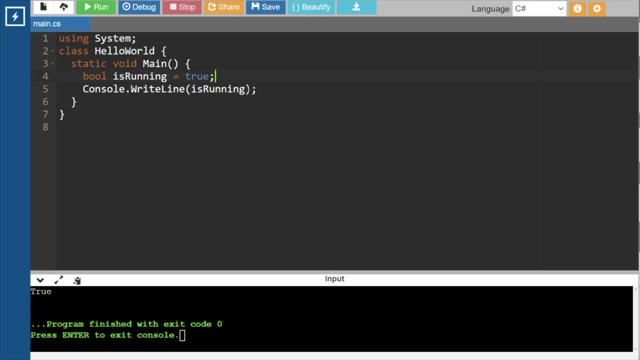 that the value is true. right, that the value is true. now, if i, if i turn it false, that is, yeah, i am running- then let's say what happened. it is printing false. see we? uh, we will understand the use of true and false. all right, there's true and false in further lectures. all right, because we'll. 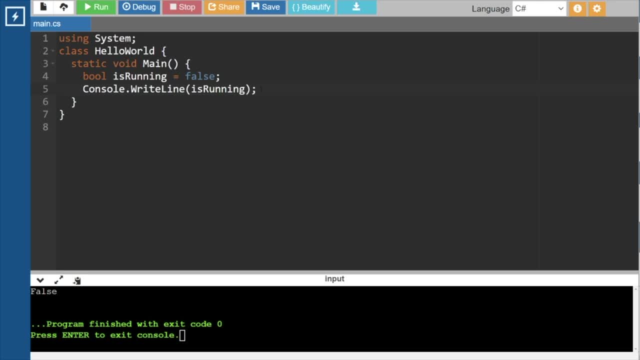 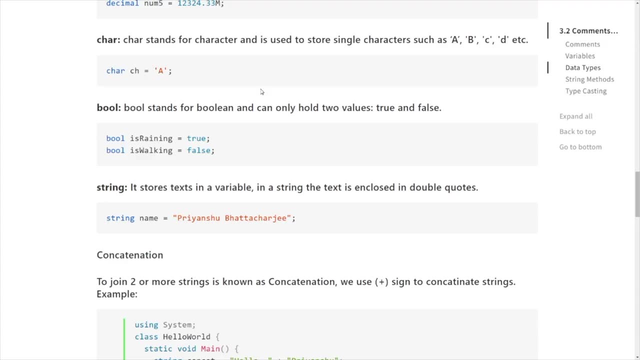 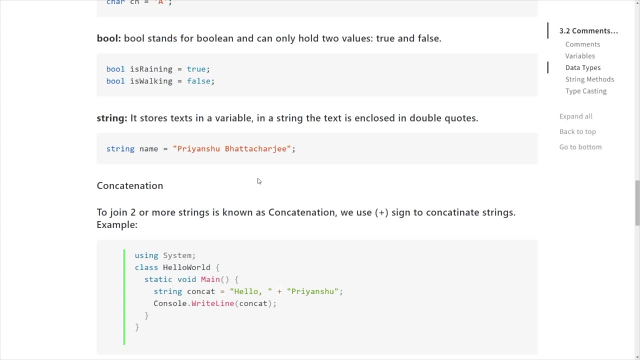 be using this often, uh, especially in the if else, all right. so if i print it now, all right, it will be in the if else and the development. so you, at that time you will understand the use case of bool and how important is it. all right now. similarly, we have another all right string now. 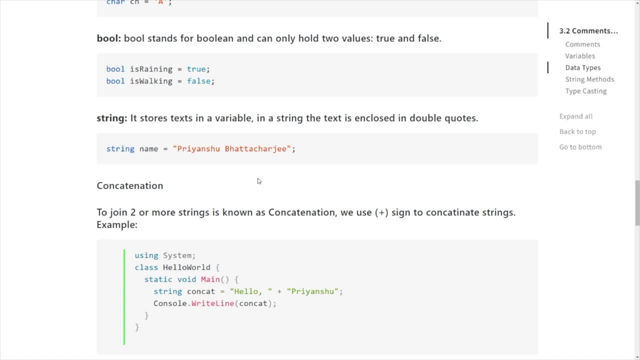 previously. uh, you might think that it is also similar to cal and it is somewhat true. all right, see a string. all right, a string is basically collection of characters. all right. the thing that we can't do in characters is that we can't do a string in a collection of characters, all right. 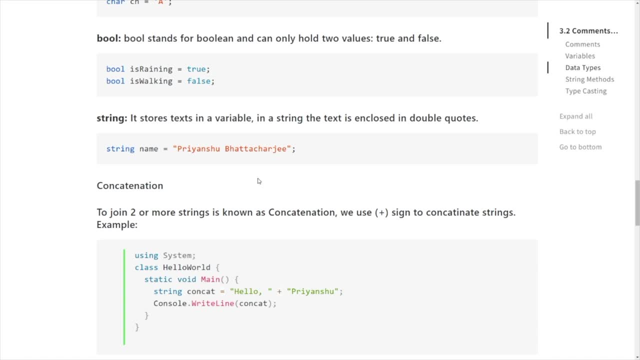 string data type. we can do that in string data type. all right, string is a collection. you can say it is a collection of characters. all right, every letter in here is a character. p is a character, r is a character. all right, and we are able to contain it, all right. you can say: uh, we are able. 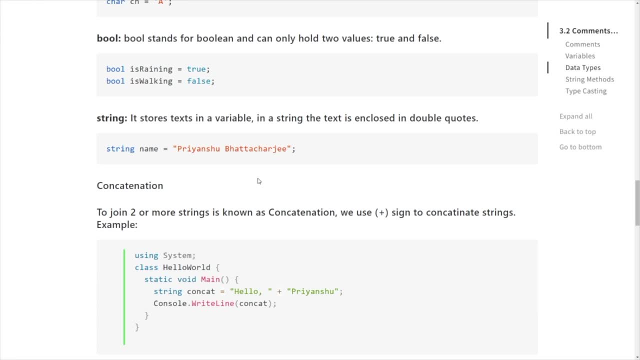 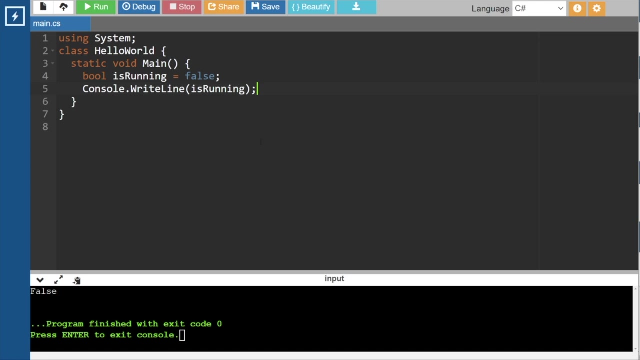 to unite them in a single variable. all right. that we can't do in character, because it can only store a single letter, right, so that's the thing that we can do in a single variable. all right, so that's what a string is. string can store multiple characters in a single variable, all right. 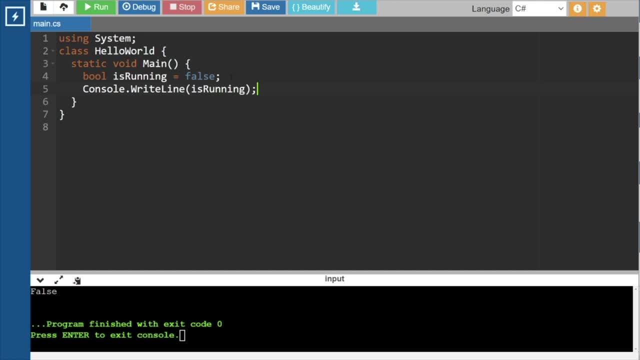 because it is a collection of characters. all right, let's try out. string. name equals you can write your own name. all right, my name is priyanshu, all right, so oh, also, i forgot to give the semicolon. this happens a lot. uh, and then name. let's try it out. 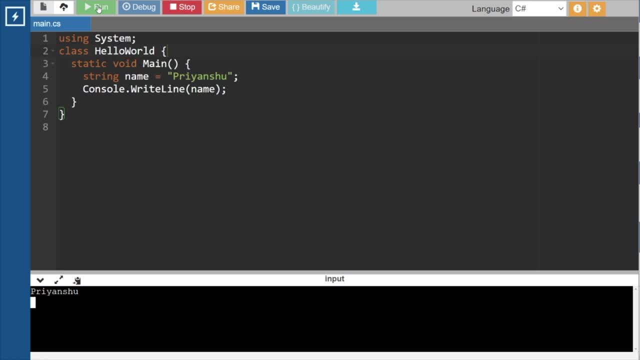 and see what happens. see, it is printing priyanshu. it is not giving us any sort of error, just like the cal date when we try to store abc. right. so string can store multiple characters, because it is, it can store a collection of characters, all right. so another thing: all right, that is. 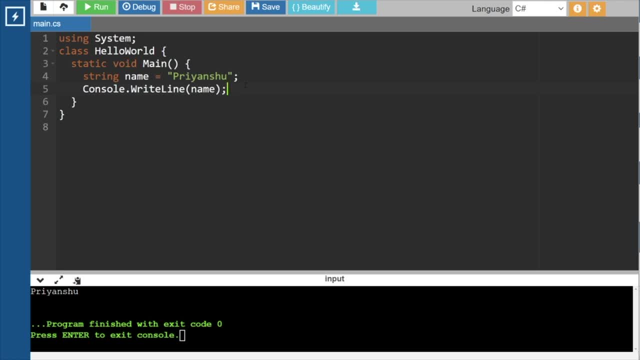 noticeable in here is: uh, whenever you are writing a string, all right. whenever you are using a string, you cannot use a string in a string. you cannot use a string in a string. you cannot use a string in a string. uh, single quotes, all right. you, you should only use double quotes, all right. so whenever, 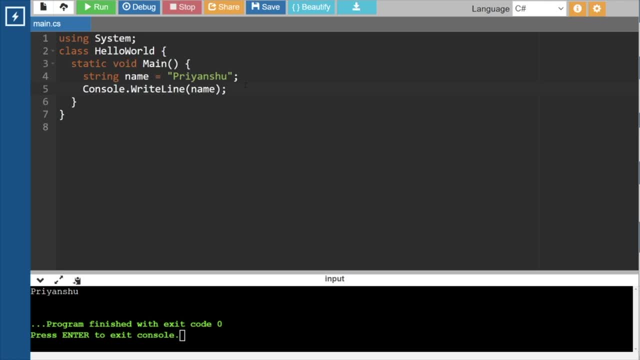 initializing a string, remember to uh enclose the characters, or you can say the let. uh means the word: all right, the word that you are uh assigning in the string, string type variable. all right, remember to enclose them in double quotes, all right, just like we did in here. all right, so. 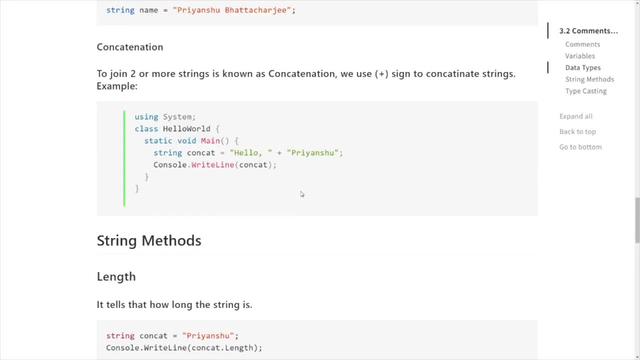 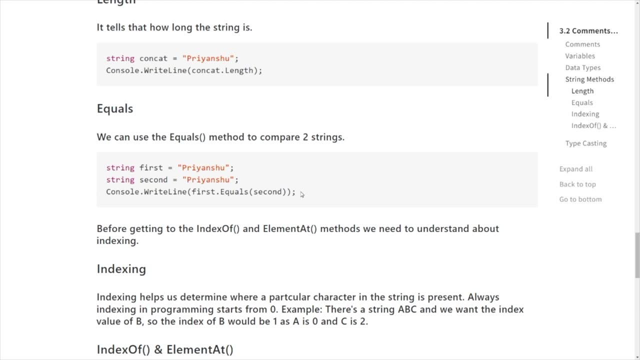 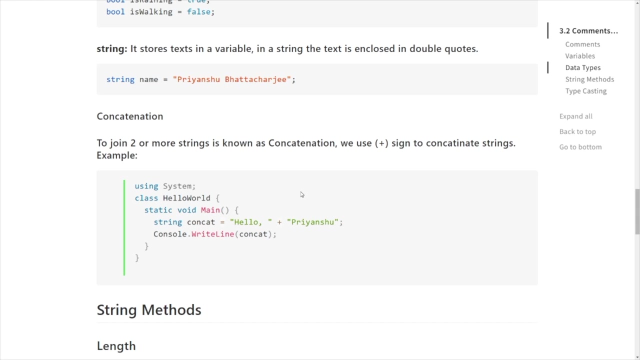 yeah, now it is our time. all right, it is our very time to understand, or you can say learn. all right, it is our very time to learn, uh, about strings in depth. all right, because strings is one of the most important concepts. all right in in programming, so let's understand it, all right. the 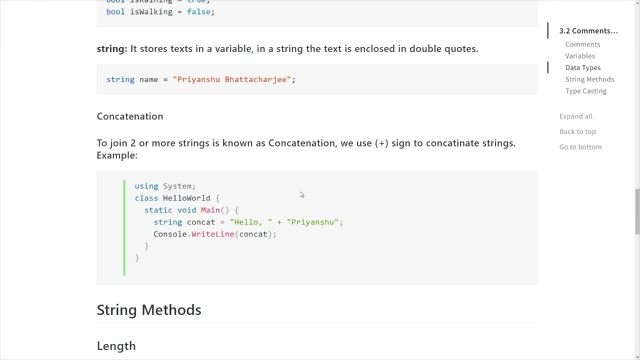 very first thing we are going to learn is concatenation. all right, what is concatenation? all right, see, concatenation is, uh, nothing too much uh of a complicated concept thing. all right, it is a really simple thing. all right, see, concatenation, uh, is basically the joining. all right, uh, it is basically the joining of two strings. all right, concatenation means it. 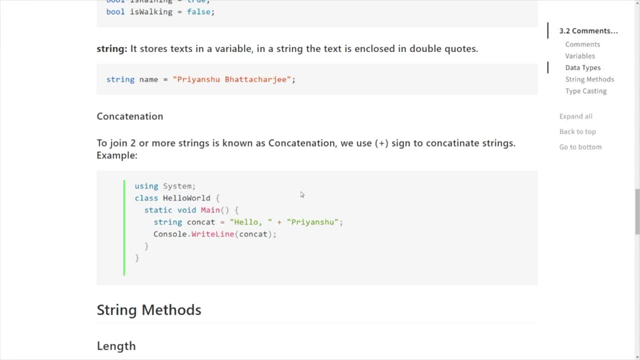 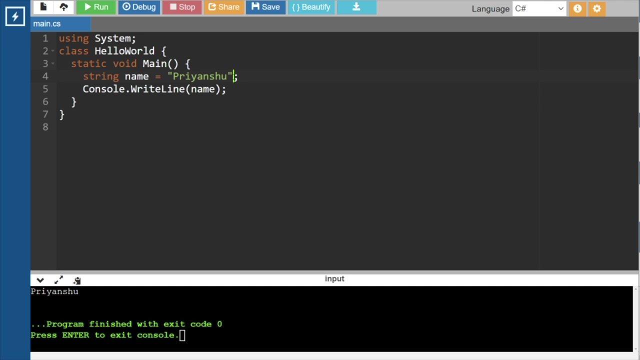 is the joining of two particular strings. all right, that is what concatenation is. so let's try it out practically right. let's try it out in our code editor, all right. so see, here we have the name, right. i'm not going to edit anything in it, just i'm going to add some another instructions. 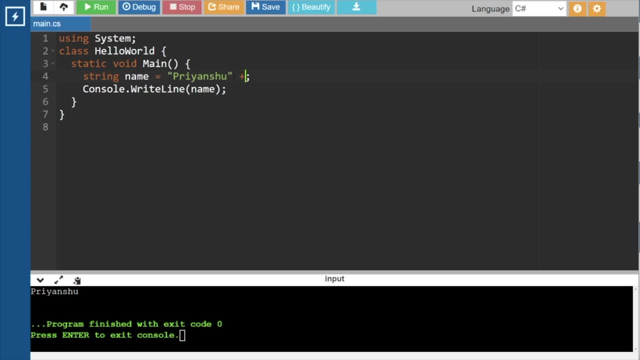 to it. all right, so add a plus in it. all right, add a plus and all right. and then add the title. all right, that is bhattacharji. all right, this is my title, right? also, i would like to give a space uh before bhattacharji, because then it would add some space to it. then, let's, let's try to print it. 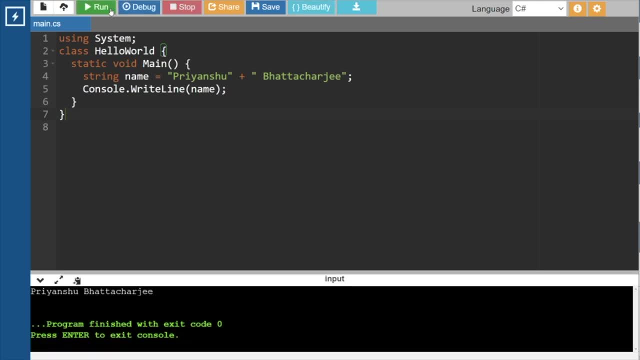 all right, see, we, i'm able to print my full name and we have successfully concatenated. all right, see. uh, you might think that, hey, man, this add is used for adding two numbers. right, we can use this add to add two numbers. right, we can use this add to add two numbers. this addition operator. 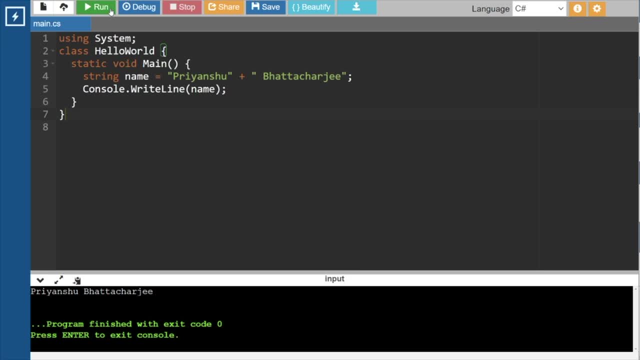 but if we talk about in terms of strings, all right, if you talk about in terms of strings, then we can use this add to add two numbers, all right, so we can use this add to add. then this uh add operator becomes a concatenation operator. all right, means it is used to. 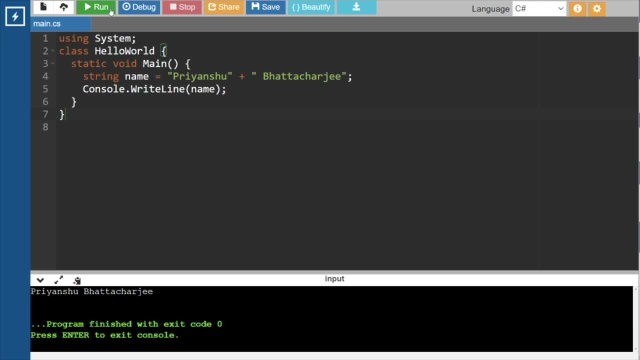 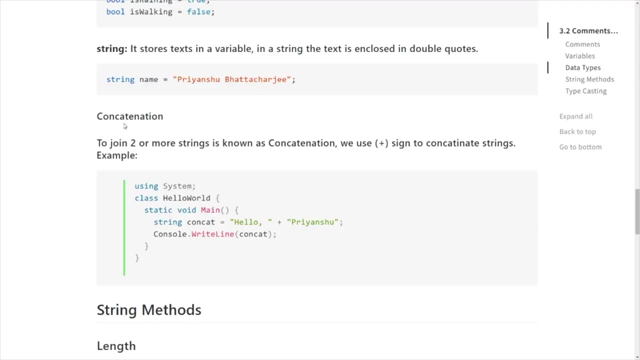 concatenate two strings into one. all right, uh, this is what this addition, uh operator does in terms of strings. all right, as simple as that. all right, so, yeah, now, as we have understood about concatenation, concatenation is nothing but but the joining. all right, the joining of two different strings. 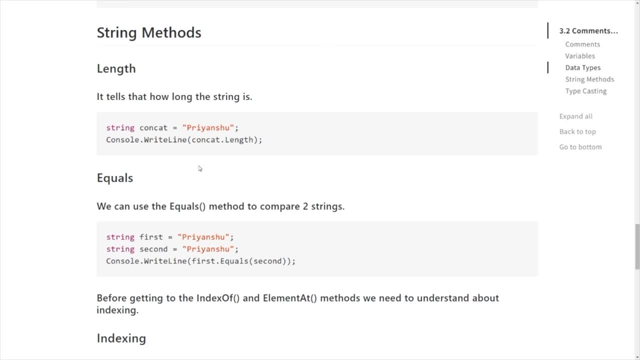 all right. now here comes some very important string methods. all right, it is, uh, it is very important to understand. all right, so let's see, see, uh, this length method. all right, it basically tells us what is the length of the string. all right, basically tells us what is the length of the string. let's try it out. all right, let's simply try it out, let's. 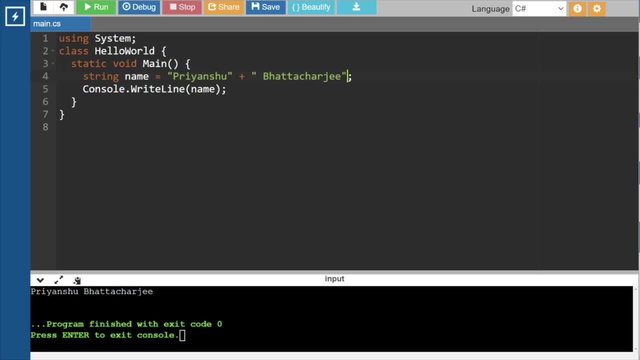 uh see, we are going to uh do it with a very simple string. all right that, a string that doesn't has a lot of characters. all right, so let's take abc. all right, see this. we all know that this, this particular string, has three characters. right, this particular thing has three characters. 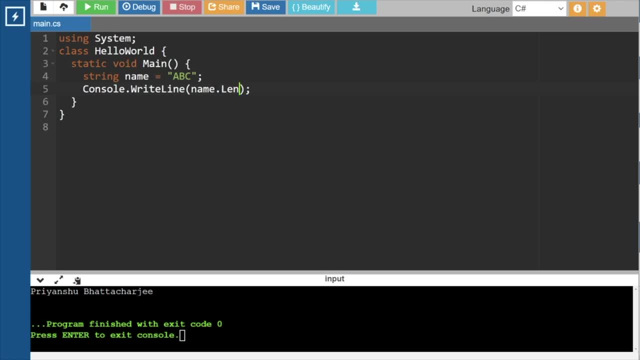 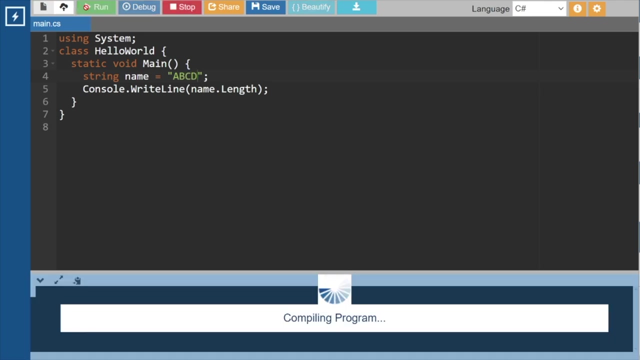 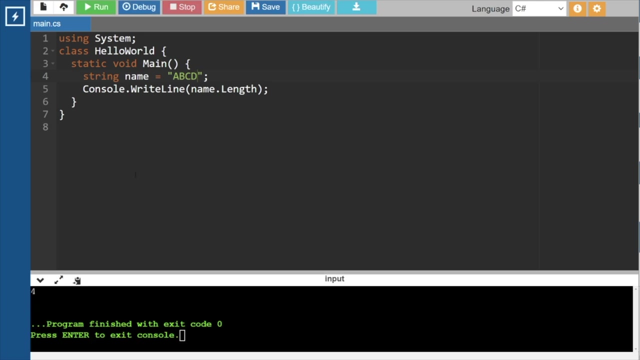 so let's try to print the length of it and let's see what happens. wow, it has given three. now let's add another. all right, let's add another character in it and let's see what it what it does. so, as you can see it in here, that it has printed four. so our length means the string's length is. 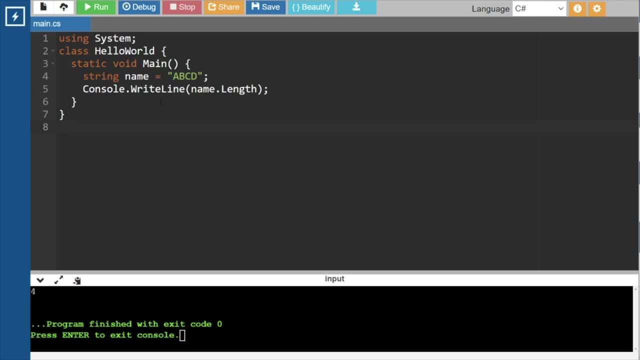 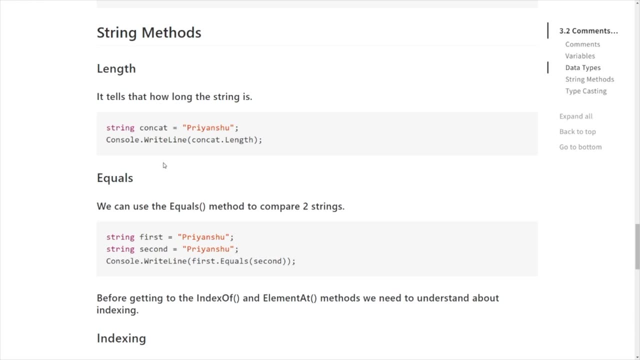 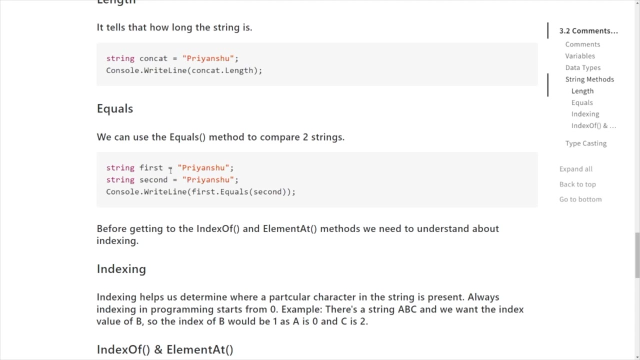 four, of course, so that's what the length does. all right, and this is going to be really helpful in our further sections. all right, even in the development. so always remember to go through these notes. all right, after watching a particular lecture. all right, so always go through these notes. 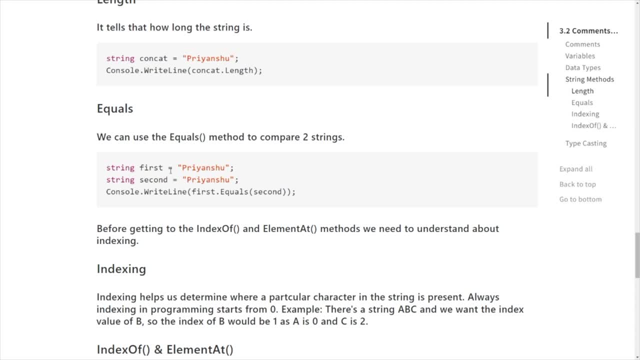 to clear your concepts again. all right, or you can say: revision of your concept. now here's another function. all right, that is equals. all right, what this equals does see, uh, this equals will just compare one string to another. all right, it will just compare one string to another. nothing, uh, too much in here. all right, it would just compare one string to another. 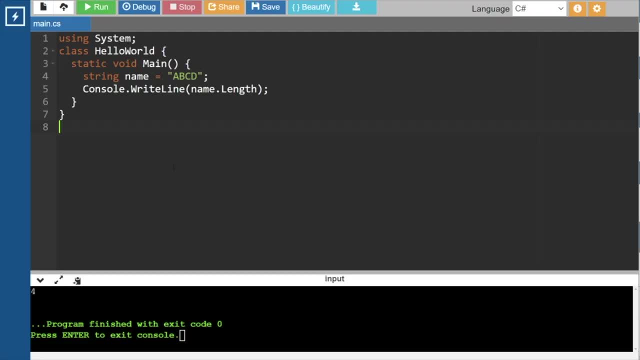 all right, so let's try it out in here, right? uh, i give it. uh, let's uh write another string, all right. string name: uh: two, all right, equals: uh, let's say dcba. right, and let's try to use this function. all right, how to use this function? first of all, select, all right, select a. 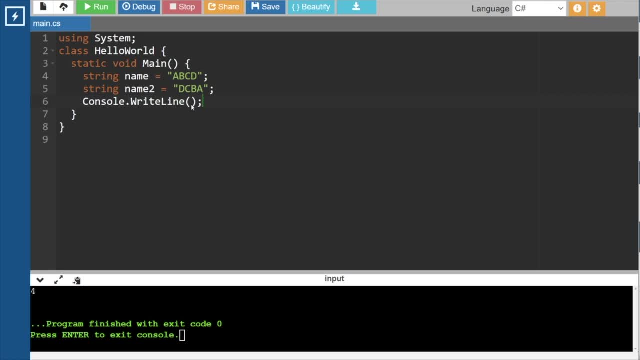 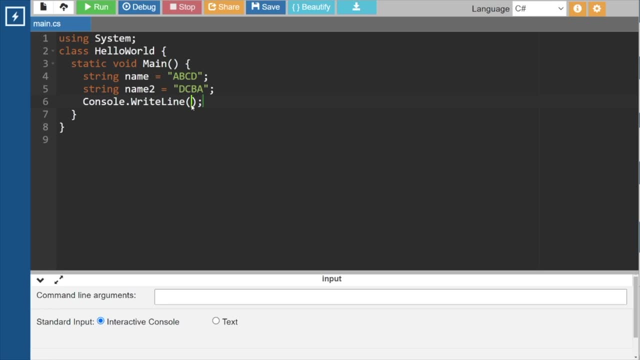 variable. all right that you want uh to compare to, all right. so i'm going to select name as my parent variable. all right, i want to compare name two with name with name, all right. so then you have to give name dot equals, all right. and then, within the 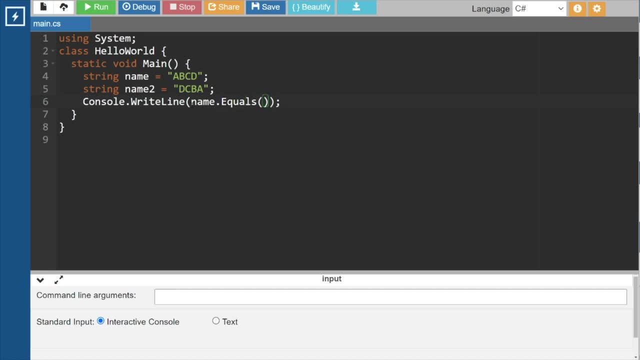 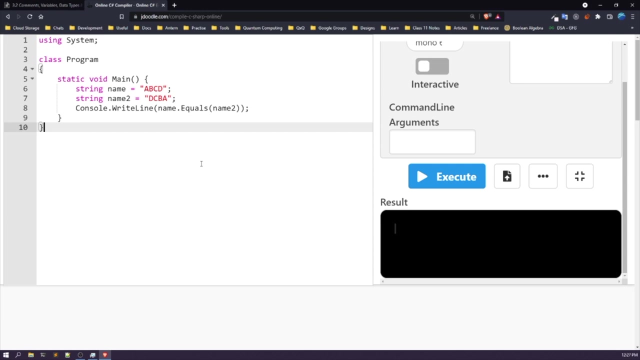 parenthesis: all right, within the parenthesis of equals, we have to pass the second variable, that is name two. all right, and then simply print it out. as simple as that. all right, guys. uh, sorry, i had to change the ide. all right, the code editor i was using that is gdb compiler. uh, it had some server. 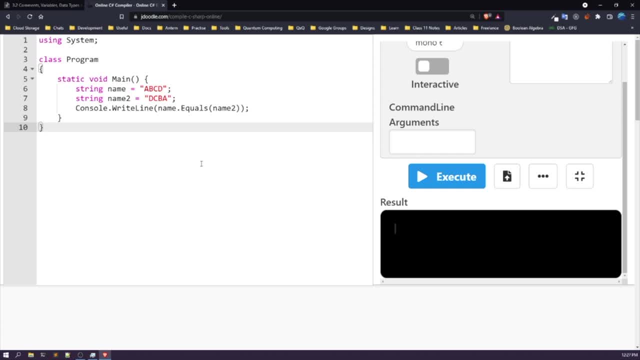 issues, all right. so now i'm using jdoodle. all right, and let's try to run this program again, but in jdoodle. all right, and let's see, uh, what will be the output. so here you can see, false. why is it false? because, of course, of course, dcba is not equals to abcd. both are different. 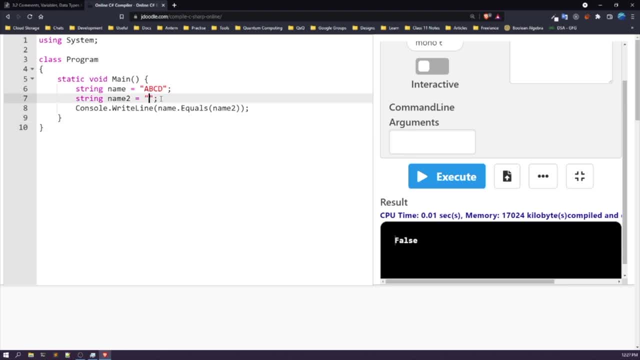 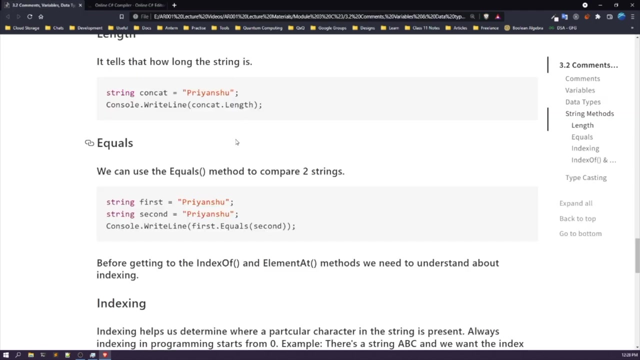 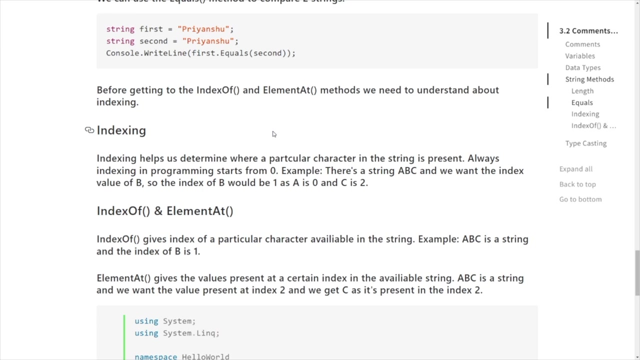 all right now. if we, if we try to give abcd again, all right, let's say what will be its output. see, it is giving true. why? why is it giving true? it is giving us true because abcd is equals to abcd. both are same right. so, yeah, of course. now, all right, we are going to see two more methods. 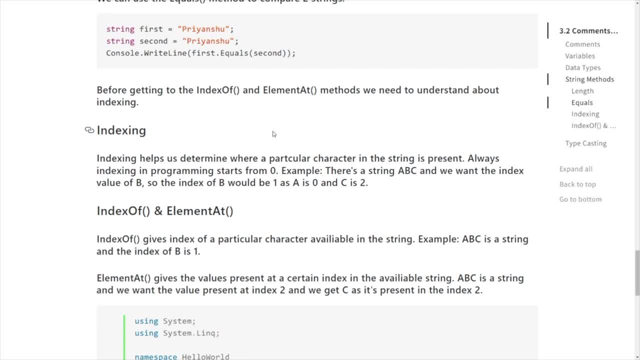 or you can say two more methods of abcd, and we are going to see two more methods of abcd: functions of strings, that is, index of and element at. but before that, all right, we have to be aware of the concept of indexing. all right, where, uh, where, this concept comes in picture? what is this? 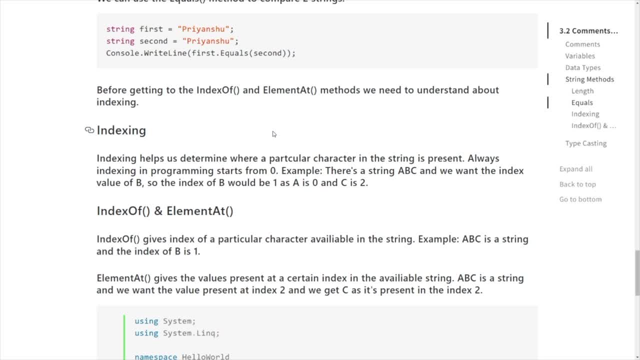 what is that? all right. so yeah see, indexing is basically tells the placement. all right, it basically tells the placement, or you can say where the particular character is present in the string. all right, like it is. it works sort of like this. so we are going to see two more methods of abcd. 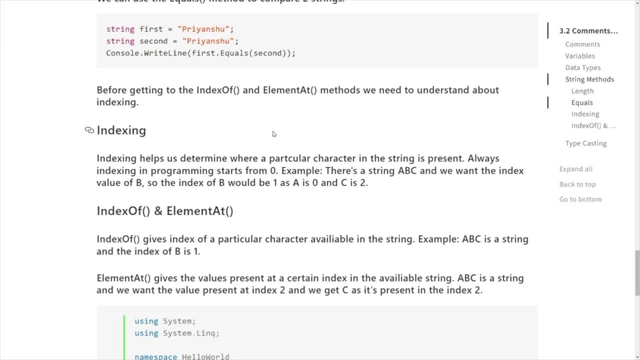 look sort of like a location in in the particular string. all right now in programming. all right, in programming, indexing always starts from zero. all right, so remember the first character. all right, the very first character of the string. all right, the very first character of the string will always. 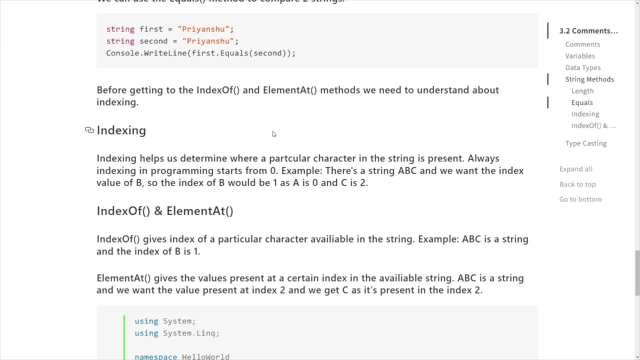 be zero, all right will always be zero. now, if we take- uh, take- an example of abc, all right, and we want- all right, we want the indexing of abcd, all right. so we are going to see two more methods of indexing, all right, we want the indexing of abcd, all right. so basically, the index of b would be one. 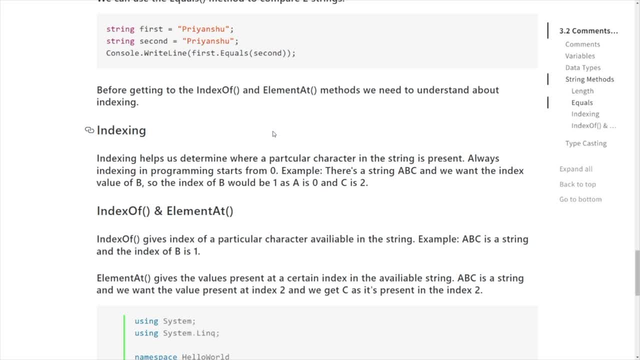 how i? i already told you that the starting point- all right, it is- the indexing always starts from zeroth position. all right, the indexing always starts from zeroth position. so a would be zero, b would be one and c would be two. so the b's b's address is one. the a's address is: 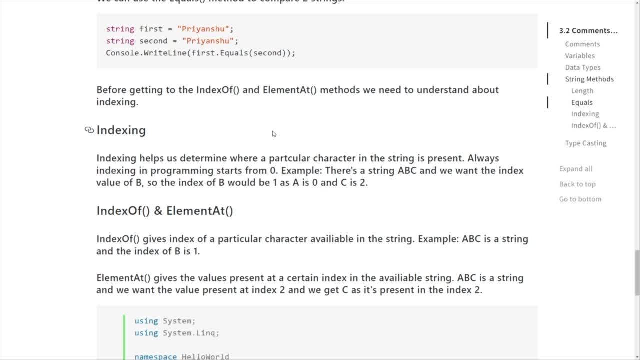 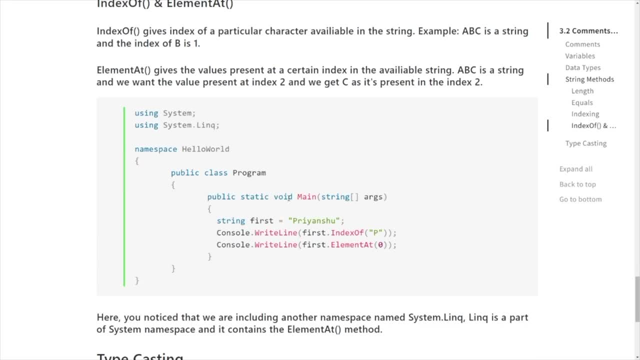 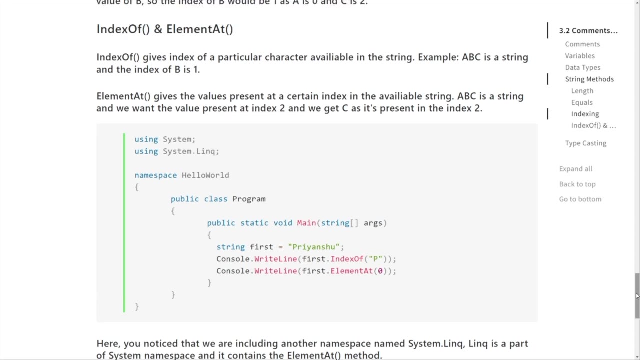 zero and c's address is two. that's what indexing is. it tells us the index or you can say the location. now, there are two. uh, two certain functions, all right, there are two certain functions available. all right, there are two certain functions available for uh, getting the. 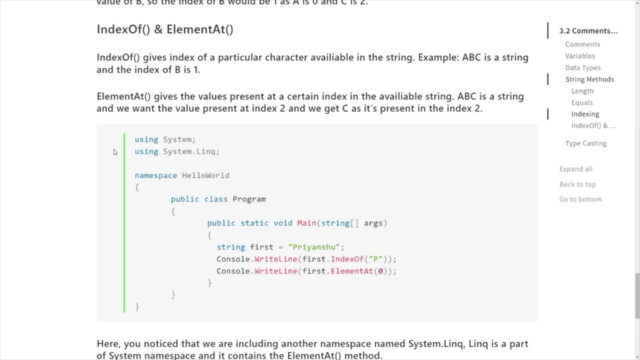 index and uh, getting the index and the element present at the index. all right, see the in what index office does. all right, in the index of function. we have just um pass. all right, we have to pass a particular uh means a particular character present in the string. 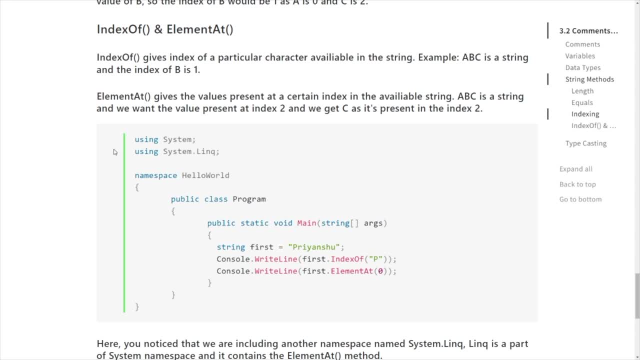 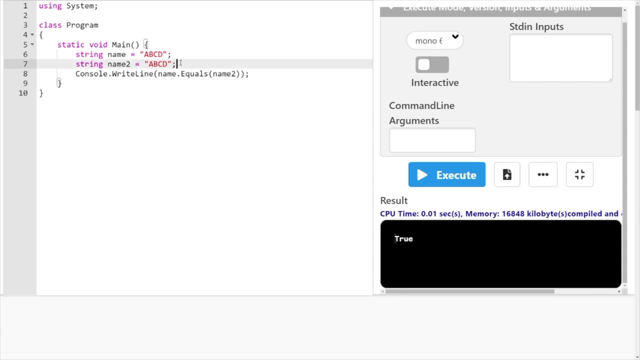 all right, and it would return. or you could say, it would give us the index, all right, the index position of the particular character. all right, let's, let's try it out. right, let's try it out. it would be as simple as that. nothing, nothing too much complicated in here, all right so. 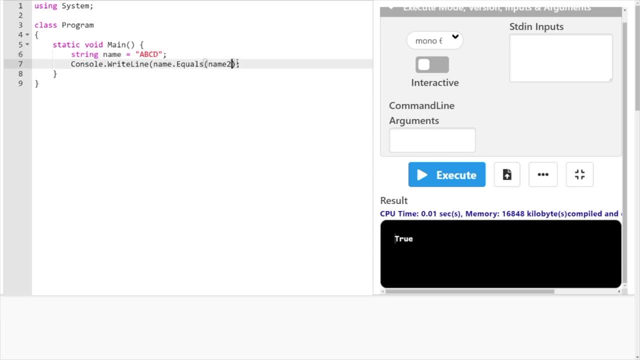 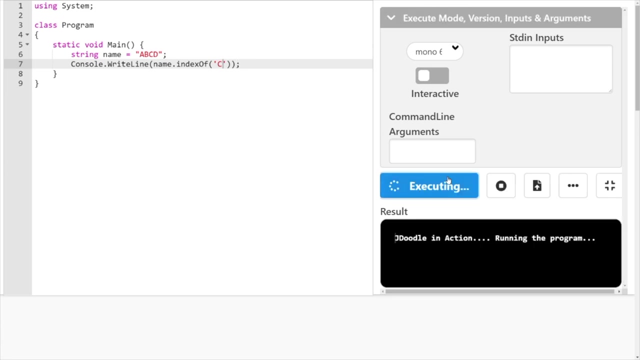 now if i, if i had to remove this weight? yeah, so what we have to do is we have to just write index, all right, index of. and then, uh, let's say, i want the index. all right, i want the index of c. how would i do that? all right, before this. pause the video and try. uh, okay, it's giving us error. 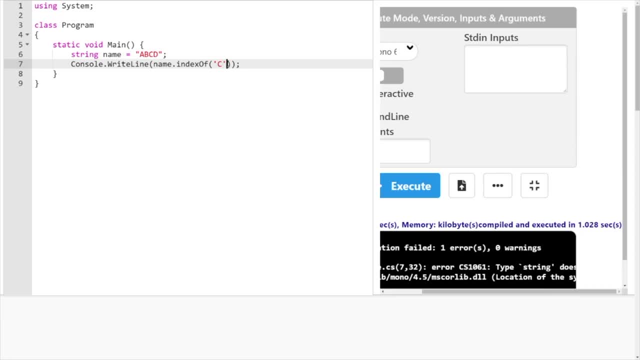 oh, i understood why it is giving error. actually, i use single quote, uh, single quotes. i'm really sorry about that, although, uh, the quiz is still on. so you have to guess, all right, you have to guess or not even guess. try to, uh, try to calculate, all right, try to interpret by yourself. 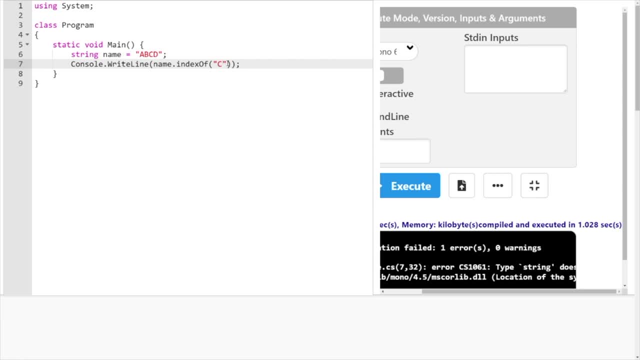 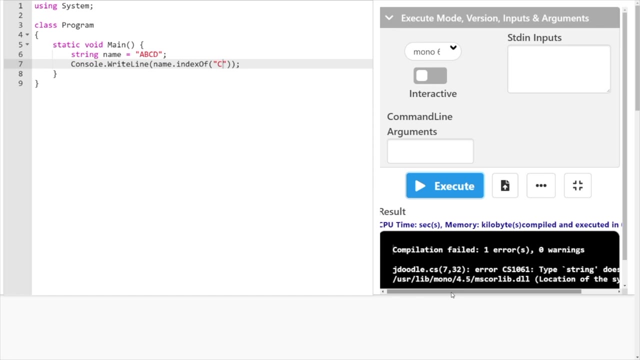 that? what will be the output of this? all right, because we are trying to get the index. all right, we are trying to get the index of c. all right, index value of c from that string. that is meaning a, b, c, d. all right, now let's execute it. all right, so it is again giving me errors. i'm not. 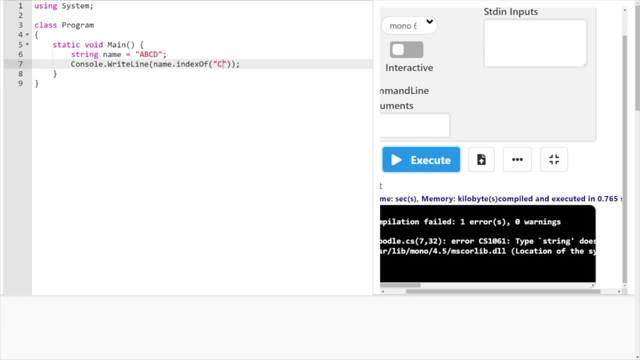 sure why wait. a definition for index of no instruction type code string. all right, wait, oh sorry. yeah, as i told, uh, case sensitivity, i uh i actually used a small letter, i that's uh. that's why i was like confused why it is giving error. it would uh the cap the first. 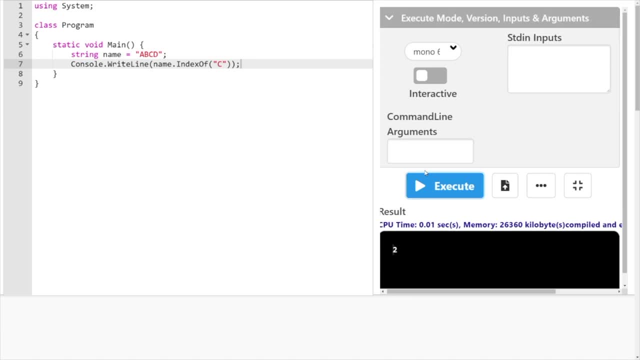 letter will be in caps. all right, so the index? all right. so the index of c is two. how, if we talk about a, the index of a is zero because it is the starting point, so of course it would be zero. then index of b is, uh, one. all right, index of b is one and the index of c is two. all right. 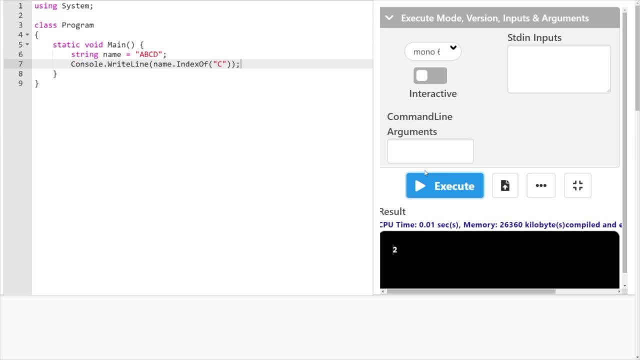 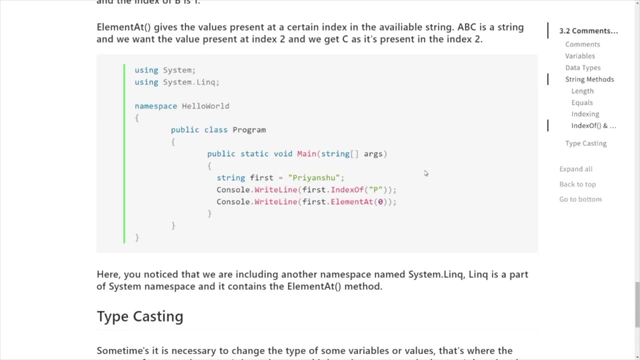 similarly after this, all right. similarly after this, there's another. all right, that is element of all right. let's see. let's see, sorry element at, i'm really sorry about that. so uh, it got a rhyming. so uh, yeah, so the uh, this is the element at function. what it basically does is see, we have 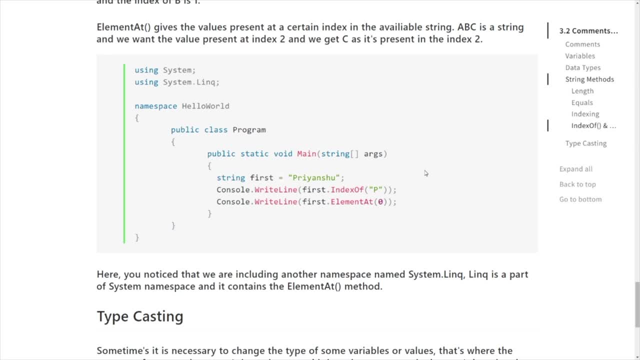 to pass. all right, we have to pass some sort of index value. all right, we have to pass an index value in it and, and after we got the function, we have to pass the value in it and we have to pass. pass the index value. let's say, i pass, uh, from the a, from a, b, c, d, i pass two. all right, then it would. 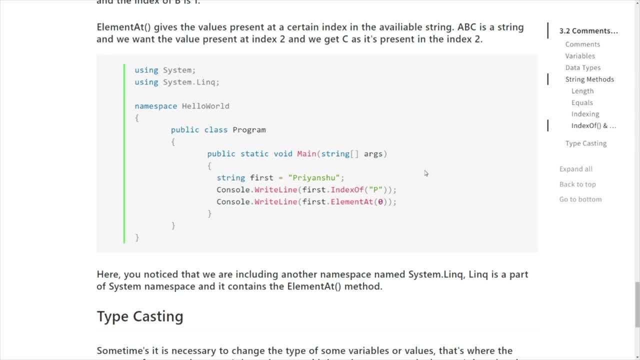 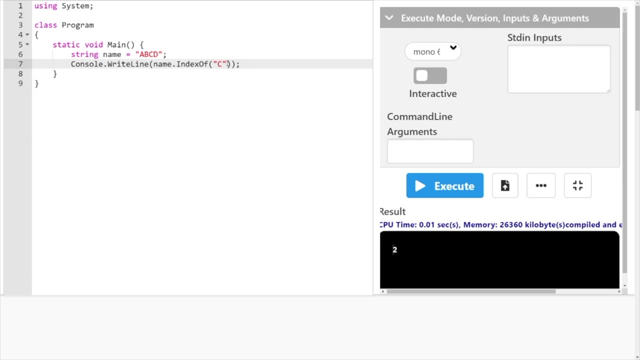 return c because the at index two uh c is present. right, let's try it out. all right, let's try it out and you will. uh, you will also notice something. all right, now i will tell you what element at all right, and we have to put the index value. that is, let's say, i want. 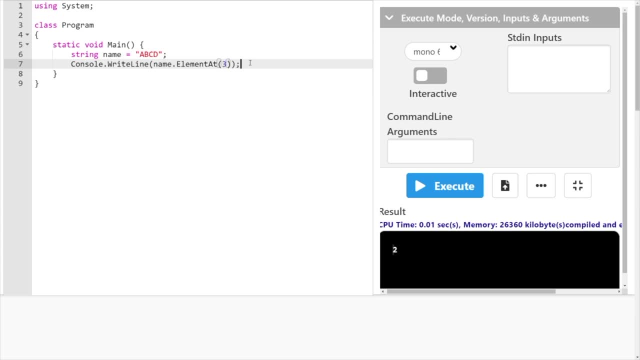 the value present at index three. all right, let's see, see it is giving. it is giving some sort of error. what error? why is it giving that error? see the reason that is giving error. because basically in you can see that it is giving some sort of error. so let's say i want the value present at index. 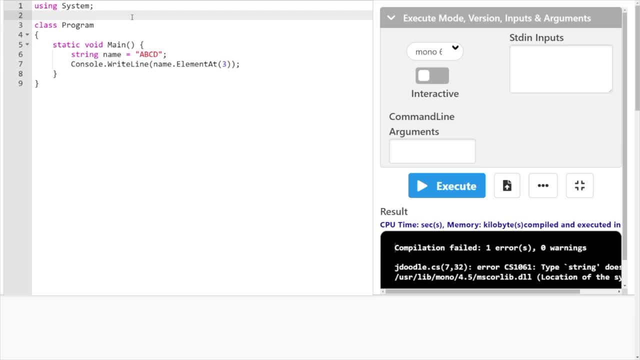 the system. in the system namespace there is no dot element at function available right now. to use this function we have to include another namespace that is using system dot link. all right, and then if we run it, all right. and then if we run it, see, we got the element present at index 3, that is D, already now. if I, if I, 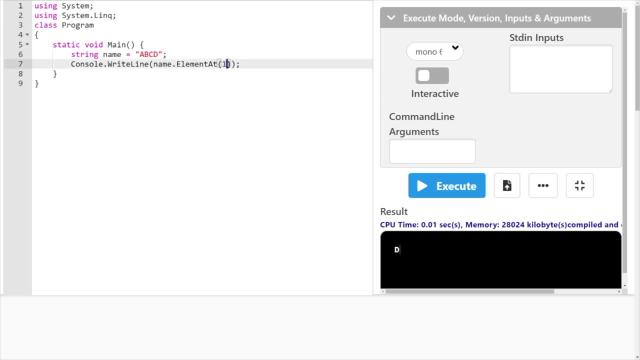 want element present at, let's say, 1. can you guess what we are in the index 1, which element is present? pause the video and think of all right. pause the video and think and tell in the comments: all right, let's try it out, let's see Wow. 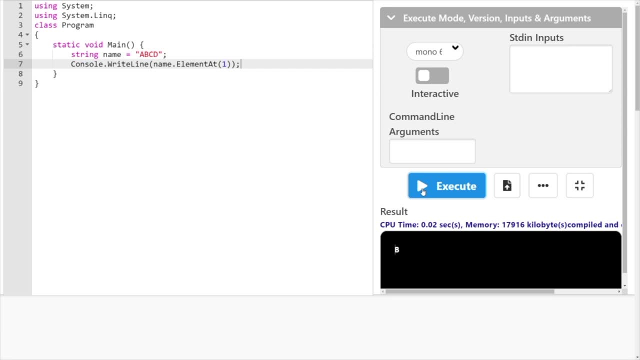 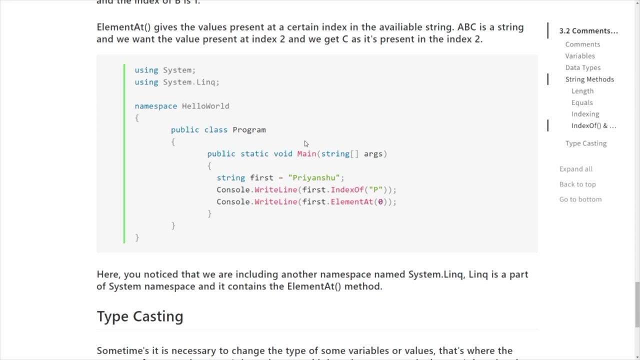 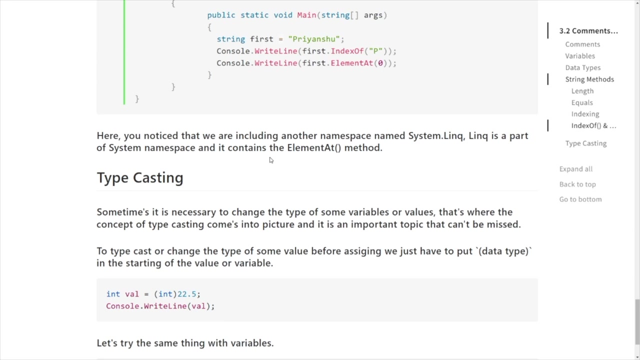 it is correct at doe, at index 1, element B is present, that is, ad ad 0. alright, add index 0. a is present. at index 1, B is present, right, so it is as simple as that. all right now. I already told you about system linked, all right, so we used a. 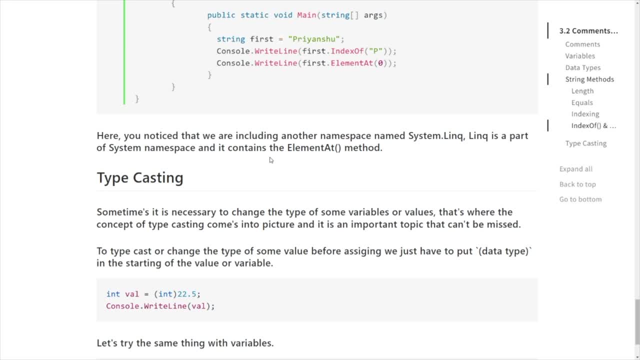 system dot link. all right, it is. it is another namespace already. next is basically a part of system namespace only. all right, and it contains the element act method. nothing too complicated, all right. so till now we have learned a lot, all right. we have learned a lot about data types. we have learned a lot about comments. we have learned a lot about variables. 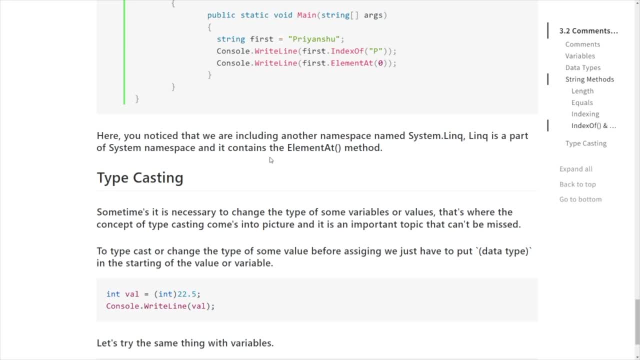 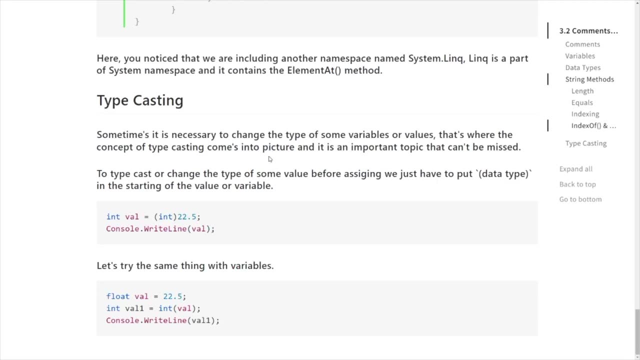 right, and the lecture has almost crossed one hour point. all right, so now this is our last. all right, this is our last topic of today. all right, last but not the least, because there are many other topics available, that is, operators, loops, conditionals and etc. so now this concept, all. 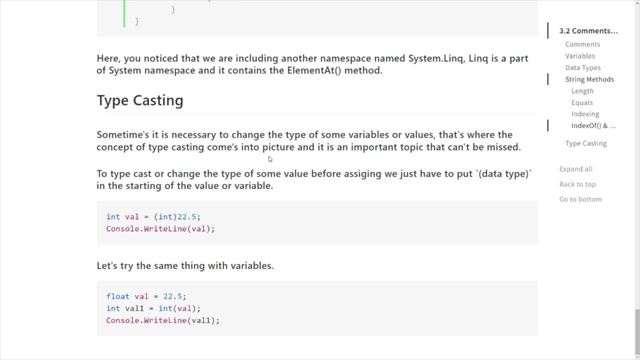 right now. i also have a homework for you that you guys have to do. all right, i won't show you how to do it. all right, i won't show you how to do it, but you have to do it by yourself. all right, because after this typecasting, i'm pretty sure that you would be able to solve some like a problem. uh, 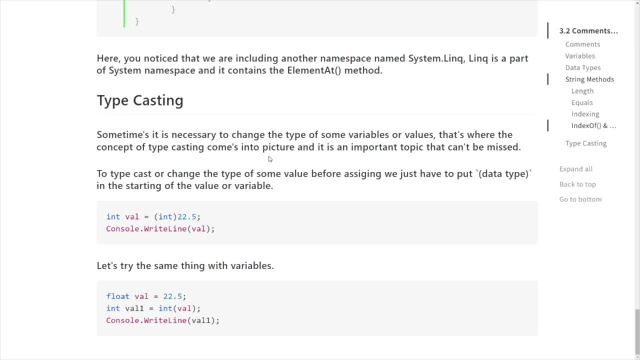 only one problem means i would only give you one problem, and i think you will be, i think you will be able to solve it all right. so see, sometimes all right, sometimes it is really necessary for us, all right to change the value all right, before assigning means to change. 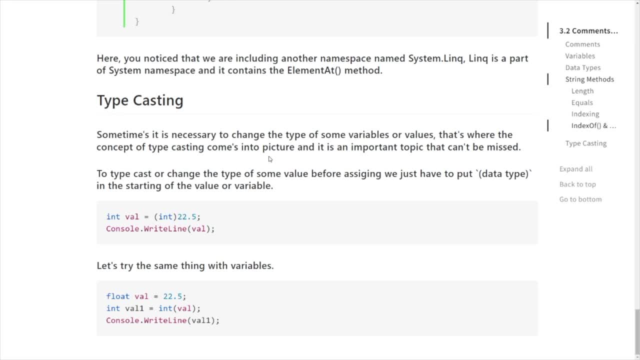 not the value but the type of the value, before assigning all right. uh, let's say, if we, if we want to assign, all right, if we want to assign a floating point value to a integer, of course, of course it will give us an error. right, of course it will give us an error because of course we 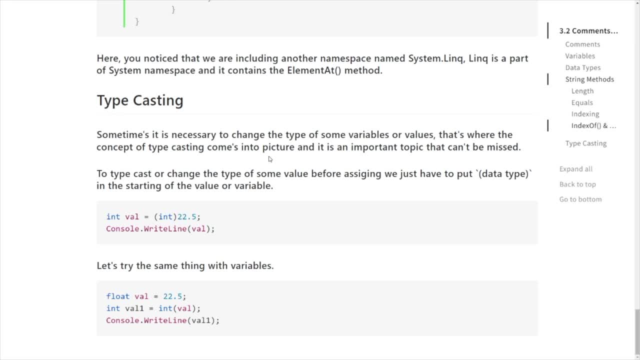 can't store store a floating point value, all right, we can't store a floating point value in, all right, we can't store a floating point value in our integer right, in our integer right. so we we have to convert it. all right, we have to cast it. we have to convert that type, that type value, right, that float type. 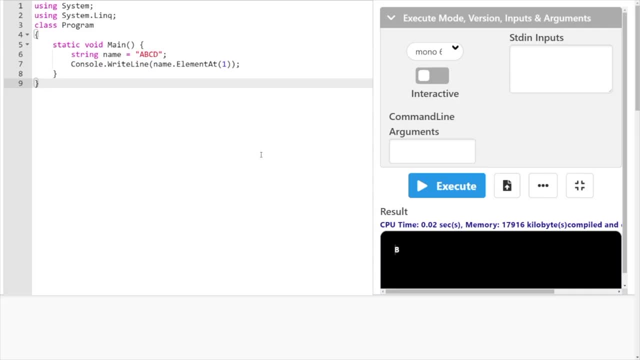 value. so let's try it out. all right, so typecasting is basically changing the type of the value before assigning. as simple as that, all right. so let's take another thing, that is int val. all right, int val equals 23.2. all right, f. of course we have to add f suffix if we are going to add floating. 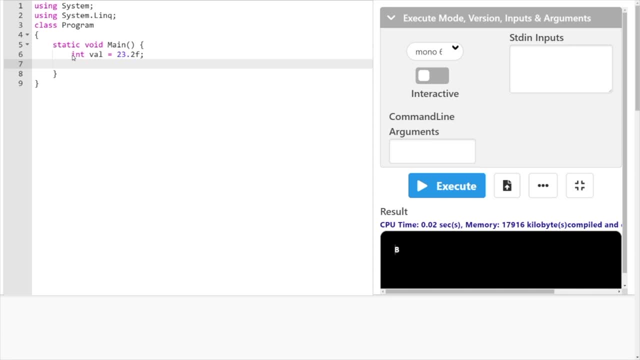 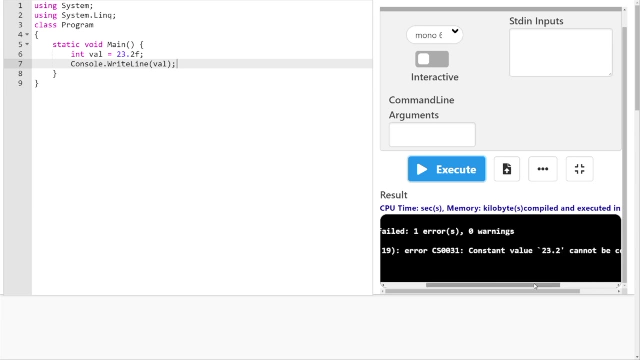 float type value. all right, and let's try it print it out. all right, let's see it. uh, it works or not. so, val, all right, let's see it works or not. oh, my god, it has. it has given us some some error. right, constant value cannot be converted to a int. right, because of course it can't be converted, because 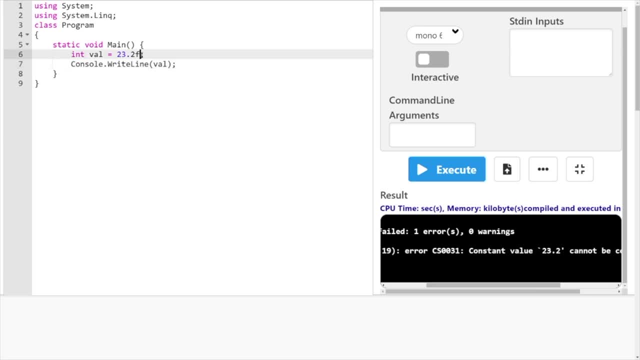 because, uh, the compiler cannot convert it by itself. we have to give some sort of instruction to convert it, right? so how would we do that? as simple as that. we have to convert it to int, right? so before, uh, assigning the value- all right, like you have assigned this value before that- give a parenthesis, all right, all right, and give the data. 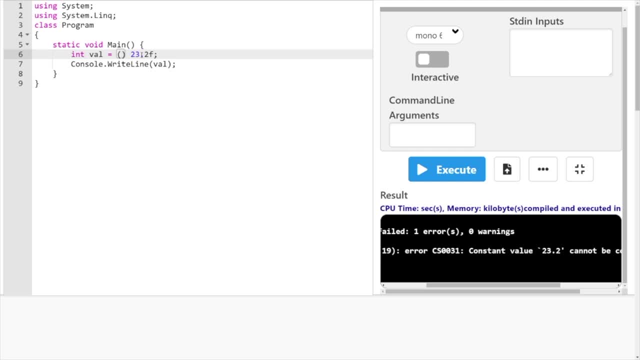 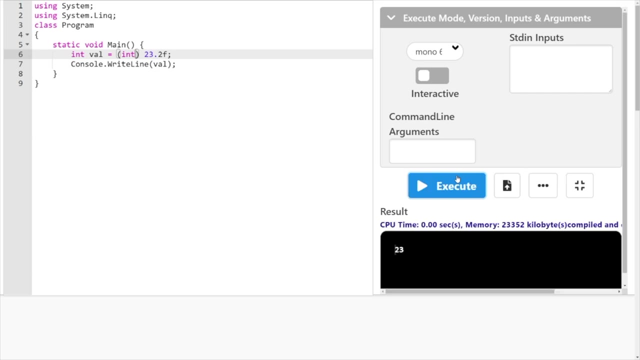 type you want to convert the value to. so it will currently: uh, this value is in float. all right, this value is in float. we want to convert it to int to store in the in data int variable. right, so it has stored. basically, what is happening is it is removing that uh value from the point. all right. 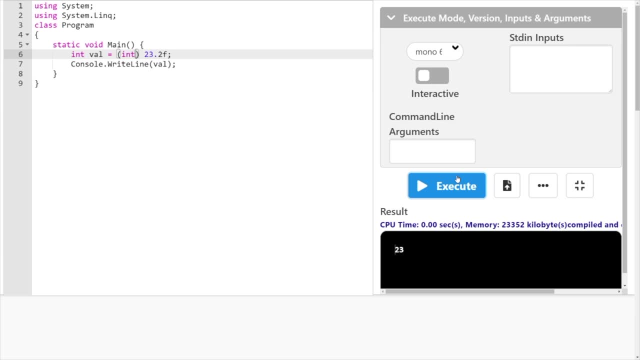 from the decimal. it is removing that value, all right, and it is storing the exact value, all right. so this is what type casting is now all right now. another thing i would like to show you is: we can also do this with the variable, also all right, let's, let's um, create um. 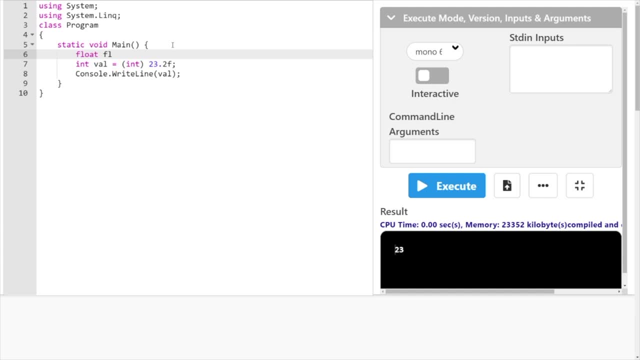 a variable. all right, that is float fl. i have given any name i i could have imagined, all right. so let's give 23 point. or let's say 24.5 f, all right. so let's give that, all right. and what i will do is i will remove that value and instead of that value i'm going to put the. 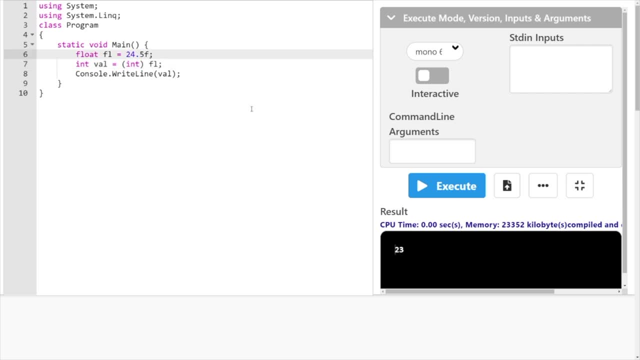 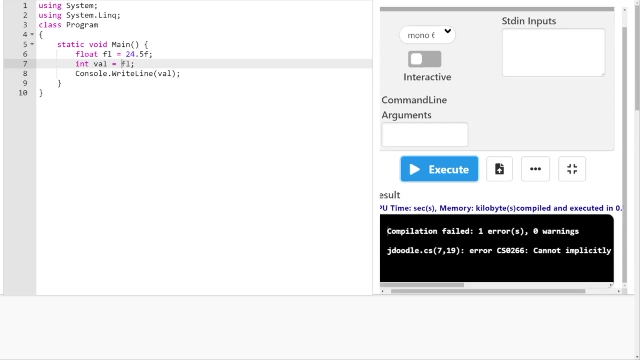 variable. all right, i'm going to put the variable and let's let's remove this int. also, first try converting and then let's see what will be the output. all right, i'm trying to assign a float value in the integer. see it is giving all right. cannot implicitly convert type float to int all. 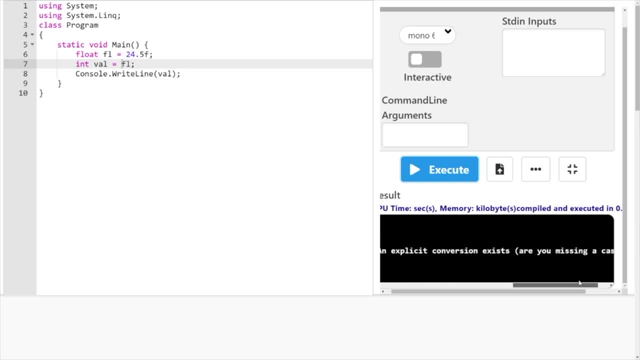 right. an expl, an explicit conversion exists. are you missing a cast? see, the compiler is so kind that it is also telling us what. what can help us fixing it all right? so what thing can help us fixing it all right? so what thing can help us fixing it all right? so what thing can? 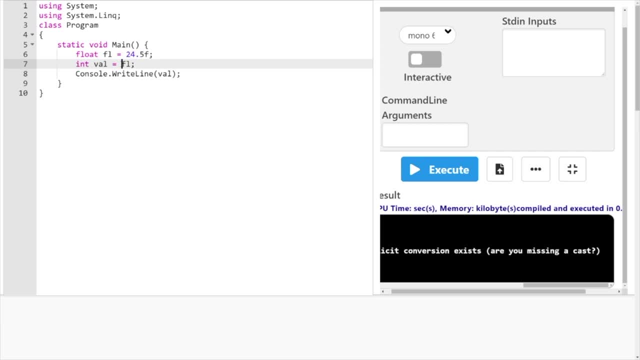 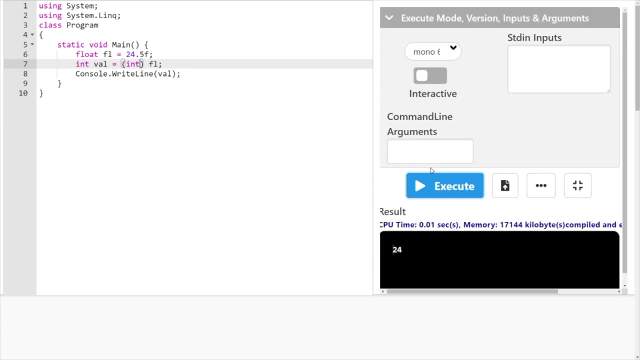 help us fixing it right. so let's do it. so. open the brackets, all right. open the brackets and we are going to typecast it. that is int. all right. we are going to typecast it to int. all right, and let's say it works or not. let's see. wow, congratulations, it has worked. it has worked. 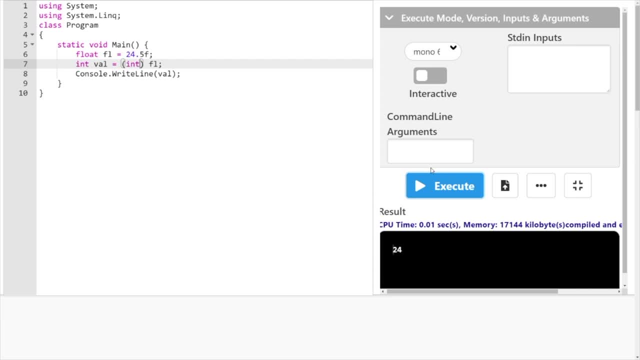 right, we, we have successfully make. uh, the floating point worked. right, we are, we have successfully typecast it now. now, here's the task for you. all right, here's the task for you. you have to convert an integer to float. all right, you have to convert an integer to float. this is your task. 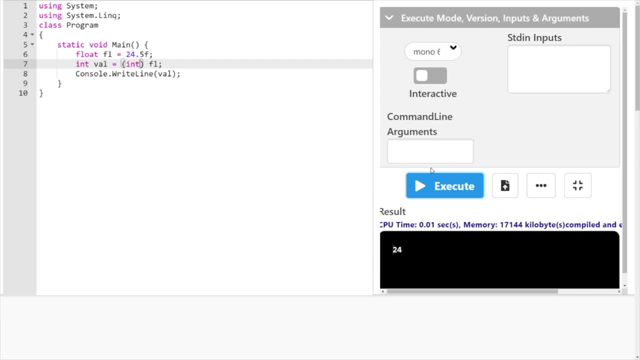 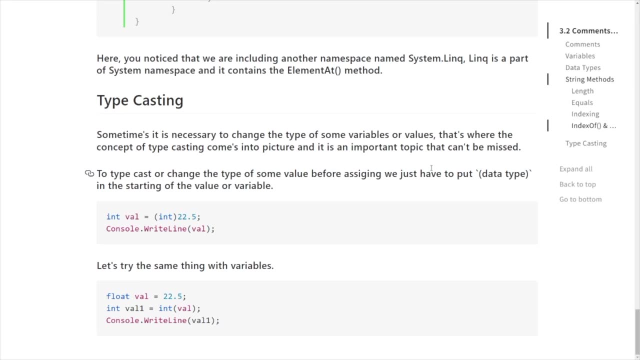 all right after. after watching the video, you can. you can surely complete it all right, it is as simple as that. it is not that complicated task, right? so for today, all right, for for today's lecture for module 3.2. we have come successfully completed this lecture, all right. 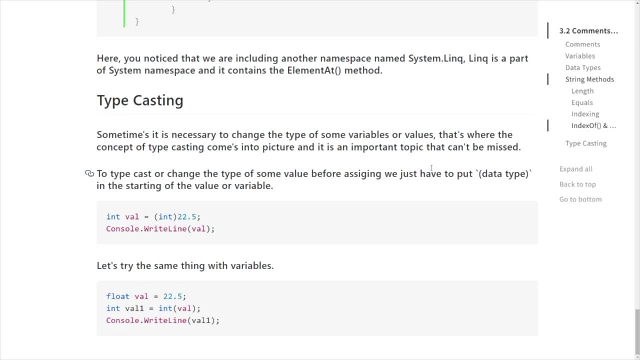 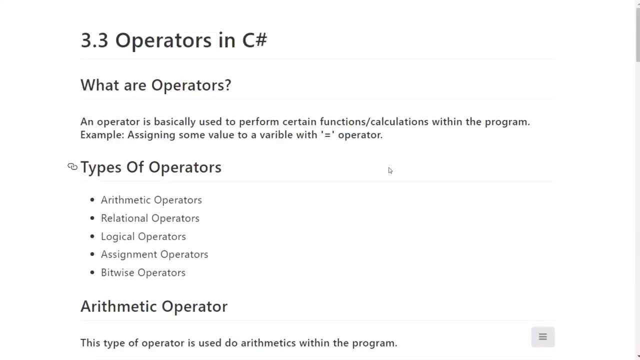 and in the next lecture we are going to learn about operators. all right, uh, it is really important to learn about the operators, so next lecture is on operators. all right, hey guys, welcome to this lecture. and in today's lecture we are going to learn about operators in shisha. all right, 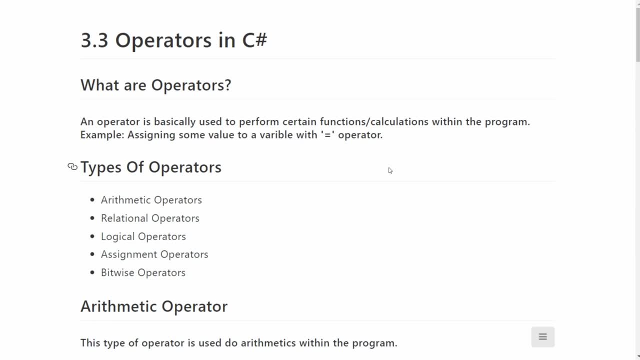 this uh particular topic is very important for us because whenever we'll be uh coding any solution- or let's say we'll be solving any sort of problems- all right, or maybe coding our own uh mechanisms in augmented and virtual reality- we will be needing operators on a highly basis. 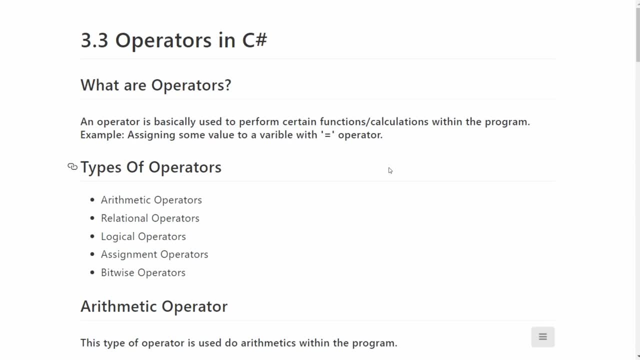 because this is the very fundamental concept. all right, all the operations that we perform within a program happens only because of operators. all right because, for example, whenever we are, uh, assigning some value to a variable, right, when we, whenever we are assigning some value to a variable, the assignment that is the equal. 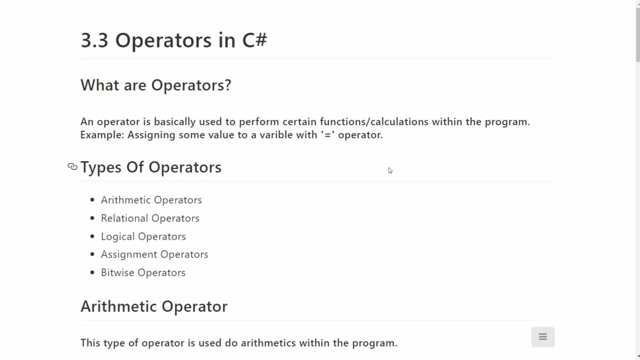 right, the equals to option, uh, or the equals to sign is called assignment operator. yeah, that is also operator. or let's say, for another example, we let's say we are multiplying- all right, we are multiplying a particular speed. all right to time, dot delta time- all right, i'm just taking it as an. 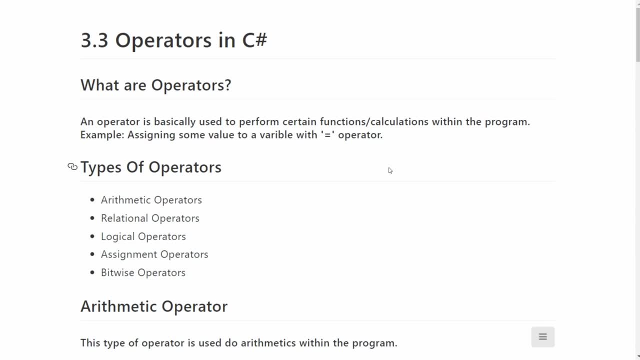 example, we will be covering time dot delta time in future videos, whenever when we will be uh learning to code in unity and uh we'll be developing our ar applications. all right, but for uh time being, just understand this: uh, there's some function that is time dot delta time and we are multiplying uh the speed variable. 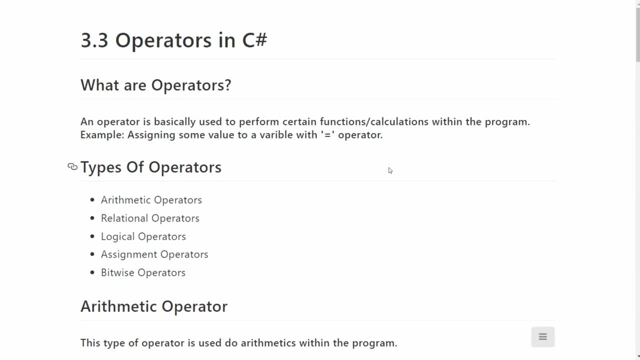 all right. the speed variable with the time dot, delta time- all right. and the you know, the, as uh means the multiplication sign. all right, that would be putting in there. that is also an operator. all right, so operators are everywhere in program, so it is very important for us to understand the concepts of operators. all right, so basically what? 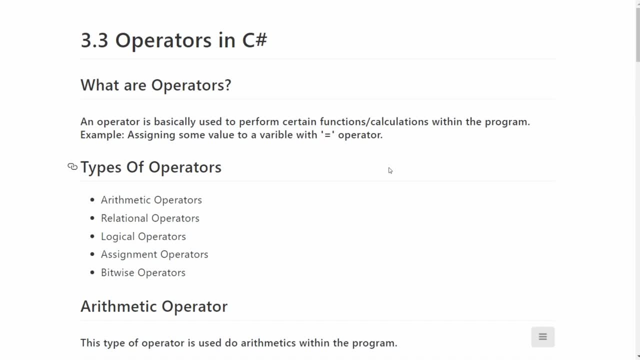 are operators. see, an operator is basically used to perform some certain functions or calculations within the program. all right, for an example, assigning some values to a variable, all right. just like an equals to operator. or, as i said, a multiplication operator is there to multiply, right. so similarly, we use operators for multiple tasks, all right. and in today's 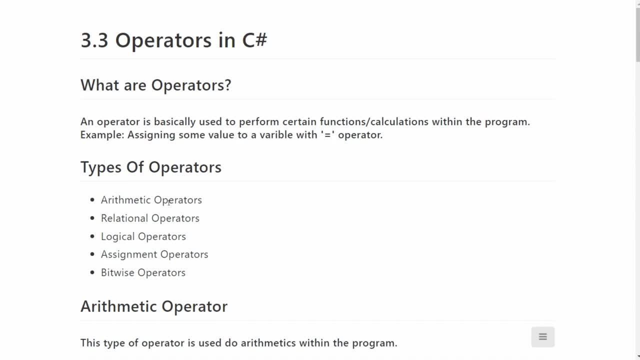 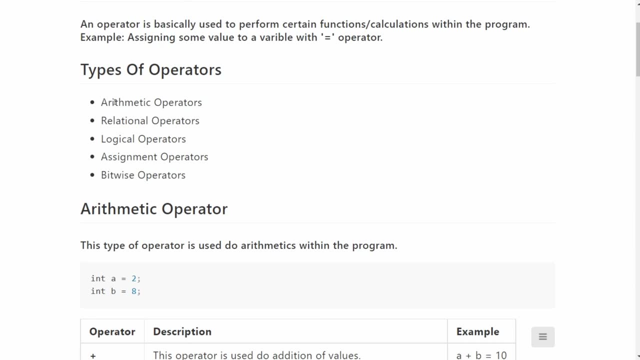 lecture. we are going to see that now there are multiple types of operators. all right, there are multiple types of operators. there are majorly five that are arithmetic operators, relational operators, logical operators, assignment operators and bitwise operators in this lecture. all right, uh, we are going to learn about four, the four of these operators. all right, that is arithmetic, relational. 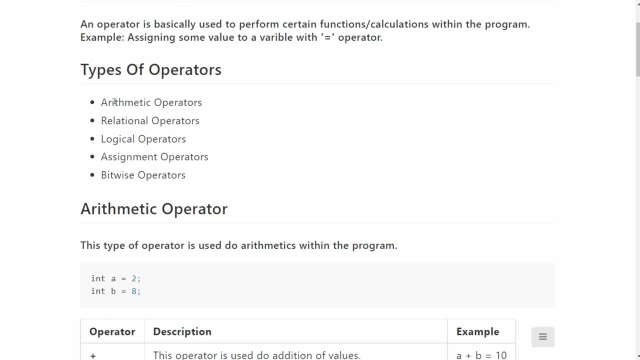 logical and assignment. all right, we won't be needing bitwise operators as of now, so that's why i am not teaching it. but, uh, if you want, i can bring a whole lecture video on bitwise operators. all right, because, uh, to understand bitwise operators, you need to understand binary operations. all right, how? 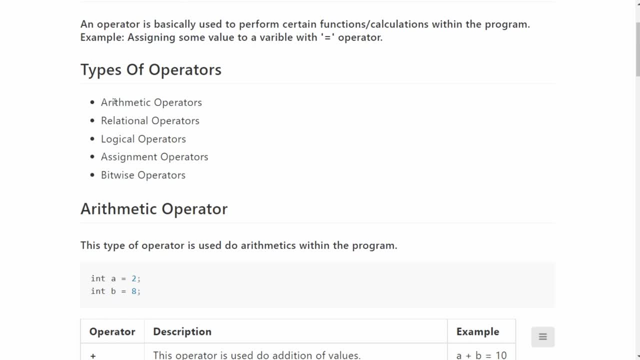 how we perform binary calculations, because bitwise operators shift those binaries right. so that's why i'm not including this uh, bitwise operator concept, uh in, you know, in this lecture. so in this lecture we are going to learn about only four of these, and uh, all right, so 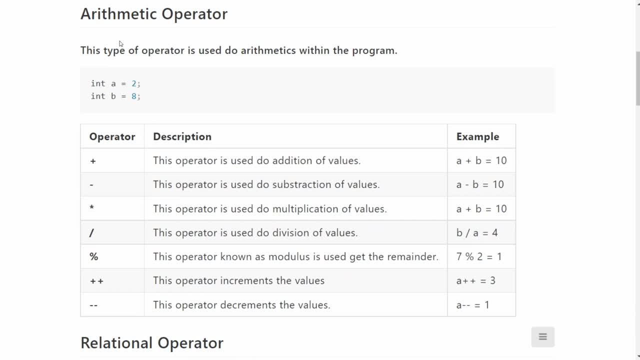 let's start with, uh, our very first operator, arithmetic. all right, so see the use. all right, the use of this operator is operator is only available in its name. arithmetic means we use these operators to perform some sort of calculation. all right, we use this operators to perform some. 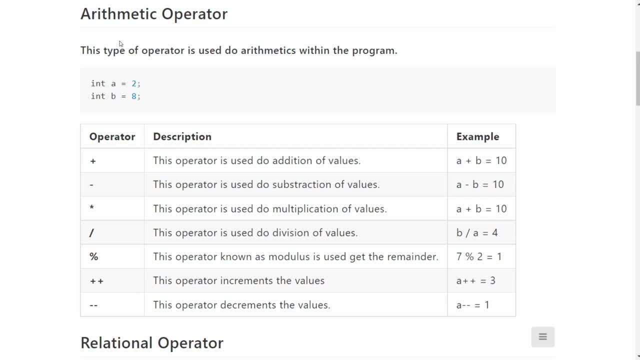 sort of calculation. the calculation can be anything. it can be division, it can be multiplication, it can be subtraction. all right, and we are going to look into that. so here are all the operators listed in. uh, you know, in a table that is, this is the plus operator. it is used for addition of values. you can: 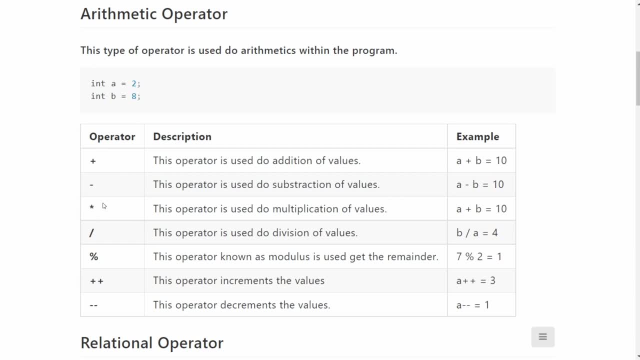 do it like this: a plus b equals 10.. similarly, there is subtraction, then there is multiplication, right, then there is a division. all right, you might- uh, this might seem a bit unfamiliar- all right, means, of course, there's a percentage sign, all right. but uh, in terms of programming, we don't call it a. 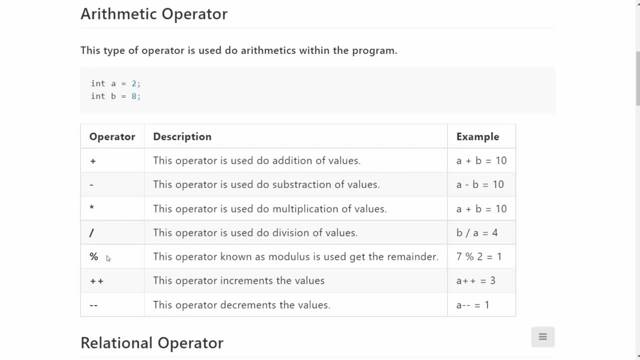 all right in terms of programming. we don't call it a percentage, we call it a modular operator. all right, we call it a modular operator. all right, or modulus. what this operator does is: this operator gives you the remainder. all right, it gives you the remainder of any division. 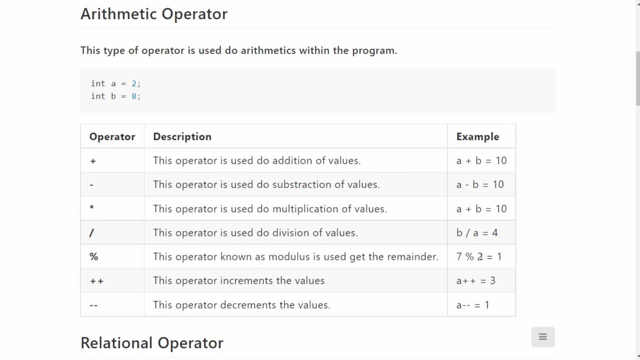 right, like, for an example: divide seven by two, all right, uh, there will always be a remainder of one, all right. so that's how it gives us the remainder of: uh. you know a particular calculation right, and here, uh, in the last two, these are unary operators, the. what these basically does now this: 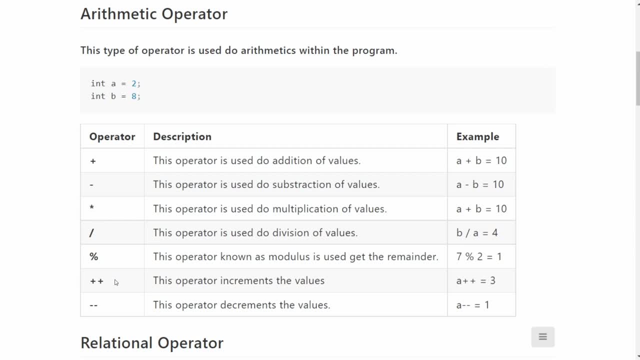 plus plus sign increments value- all right, increments value with one. let me, uh, make you understand this: plus plus sign all right will be incrementing the value as one, and this negative means negative, negative, that is, double negative. this will decrement the value. all right, this will decrement the value. that's it now to you know. understand it more. 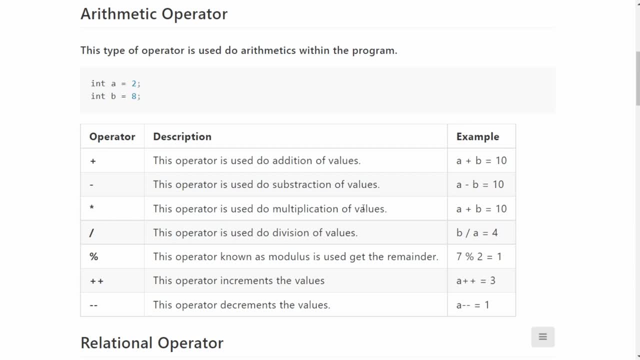 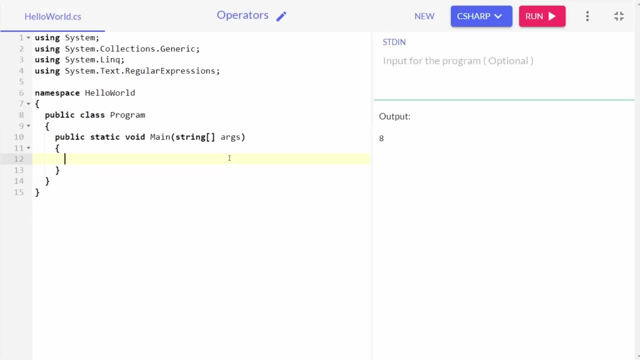 all right, understand it more wisely, more carefully. let's do one thing, let's uh do a practical on it, right? so i'm going to open, uh, just uh, give me a second, all right. okay, here is the editor, so i'm just going to open it, all right, and. 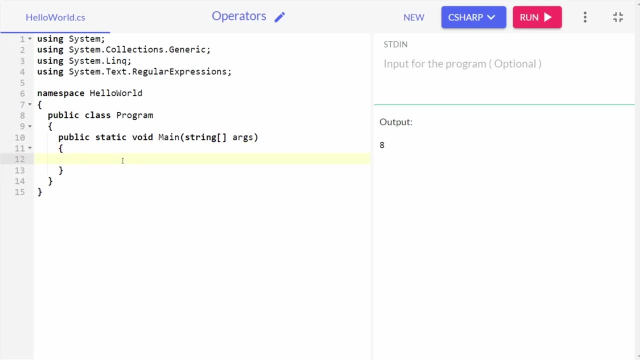 uh, what i uh first, the very first thing. all right, what i wanted to do is declare two variables. all right, that is the uh first variable. i would like to be, you know, um, let's say eight, and uh, you know the second variable, let's uh be it four. all right, now i'm going to perform the calculations, uh, you. 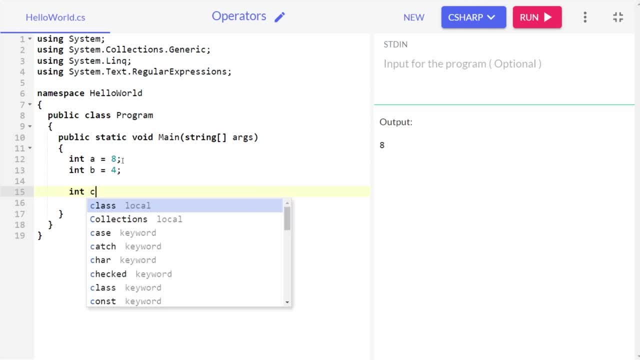 can see, there are two ways to perform the calculation. you can create another variable, that's the int c equals a plus b, all right. another way around is you just directly print it. all right, just directly print it. that is a console dot right line a plus b, all right. both will do the same task, but the difference between them is in here. 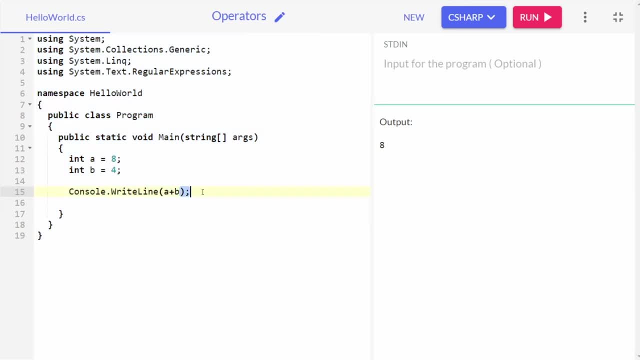 you are just printing. you aren't. uh means in this particular line. you are just printing, all right, you are just printing the uh, adding uh additive value. but when you are assigning a variable and then uh doing addition in it, just like i, uh like, just like this, all right, what you are doing is you? 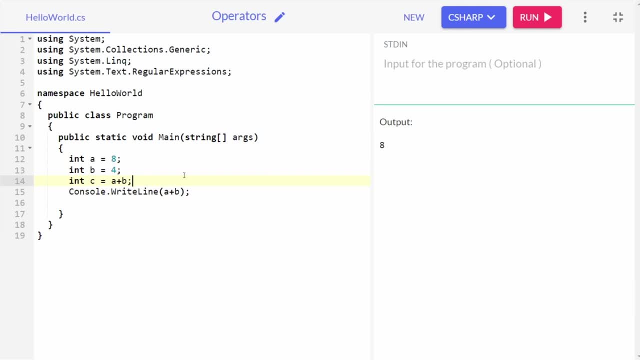 adding all of the add of b, lucky number. addition of a plus b, that is, addition of a and b in another variable, c. all right, you can surely do that, let me, uh, let's do it that way. all right, that would be better. so here you can see. all right, here you can see that we are performing the addition. now let's. 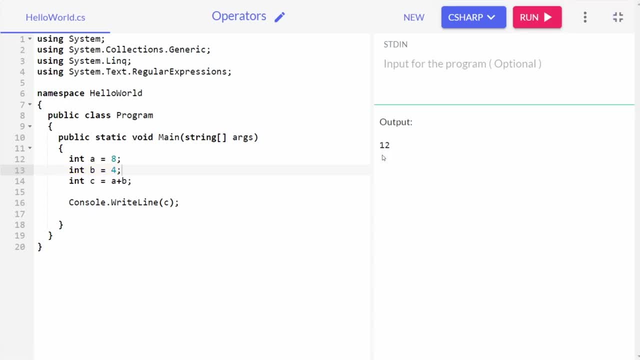 see it's: uh, is it even working? let's start out: yeah, it's, it's perfectly working. what is the addition of 8 plus 4? it is 12 and we got it right now. now for today, let's say: uh, we are out of that. 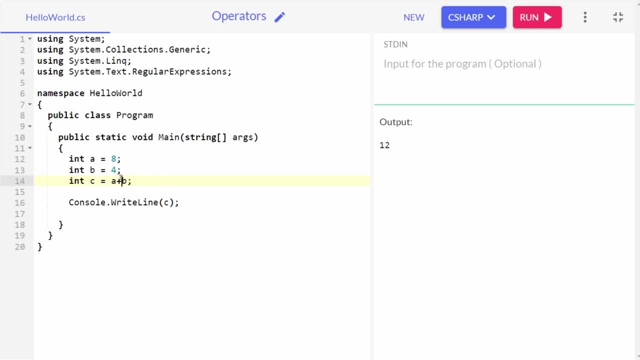 Right Now let's try out. you know subtraction, So to do the subtraction it's very simple: Remove the addition operator and put that minus operator All right. Or you can say in your keyboard there would be a dash: Put that All right, It is called a minus operator And you can see: 8 minus 4 is 4.. Right Now, let's do another thing. All right, Let's multiply it. All right, Let's see. 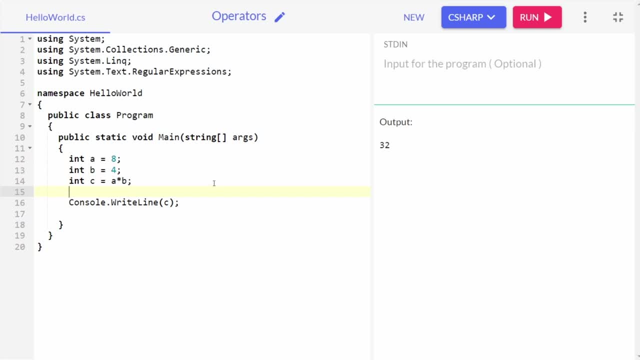 See 8, 4 is 32.. So multiplication is also working. Now let's try out division. Before doing the division operator, I want you to pause the video and do the calculation by yourself, without using any program. Let's see if you get it correctly or not. See: Yeah, 4, 2 is 8.. So the outcome is 2.. Right, So that's how it works, All right. 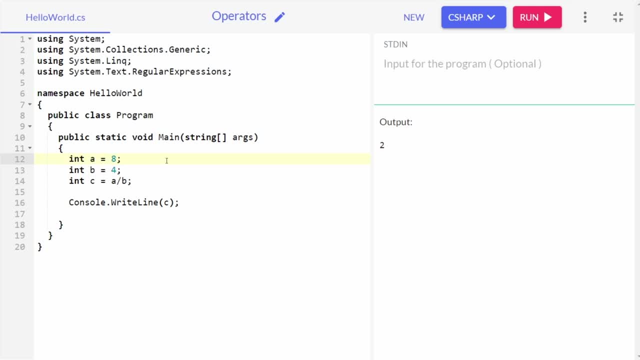 So till now we have seen, We have seen 4 operators. Which one is I mean? which are those? Addition, subtraction, multiplication and division? Now let's see, All right, Let's see the remainder operator. All right, Can you guess what would be the remainder of, like, what would be the output of this particular calculation? Just give it a thought, All right, Do it manually, All right, And then again continue with the video. 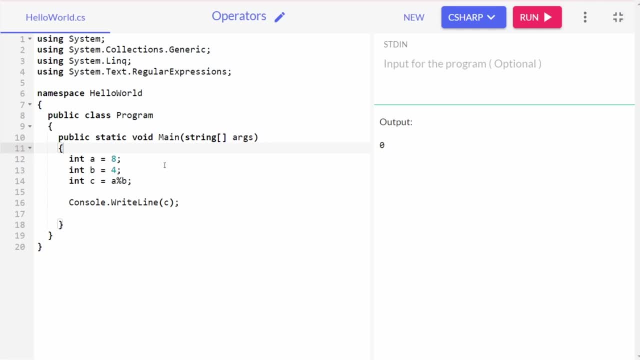 It's 0 because when we divide 8 with 4.. All right, It's completely being divided. All right, The division is being completed. So remainder is 0.. Now let's say, if I give, let's say for now I remove 8 and give 9.. Let's see, The output is 1 because there's a remainder remaining. All right, The division is not being completed. 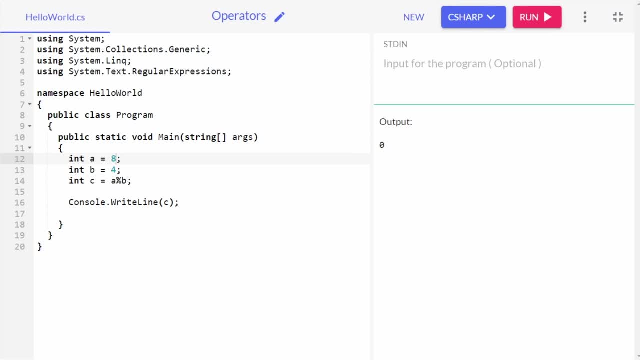 So let's see the remainder operator Evaluate the value. Thank you, This should do. this is a very simple and a simple example of how this remainder operation works. All right, It's fairly simple. So we saw about, you know, addition, subtraction, multiplication, division and remainder. 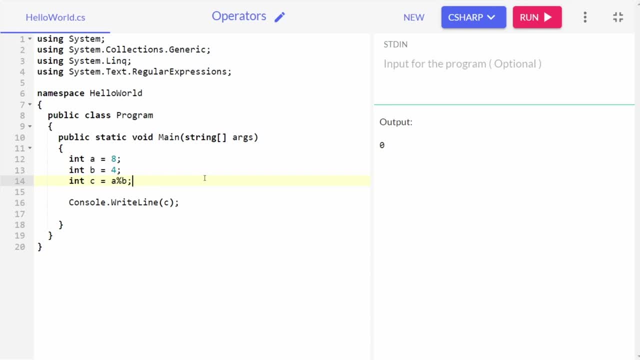 Now there remains two more operator, All right, And those are called Un udah And those are called un embodd, two ways of using increment and decrement variables. all right, means: increment and decrement, unary operators, all right, so understand it like this. so now the basic: see to understand unary. 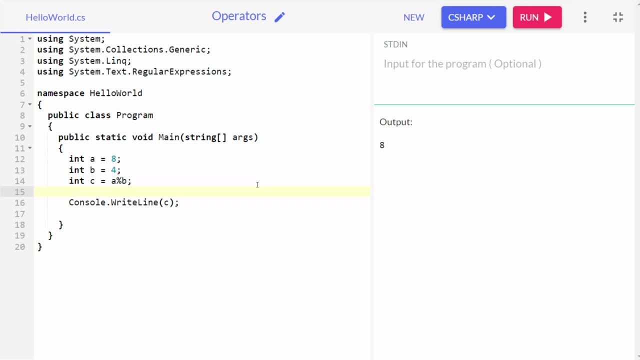 operator all right. first of all, we have to understand what it does see, unary means these increment and decrement operators. now they increment the number or decrement the number. all right means it will, uh like. if i let me show you by example on: all right, let's remove this. 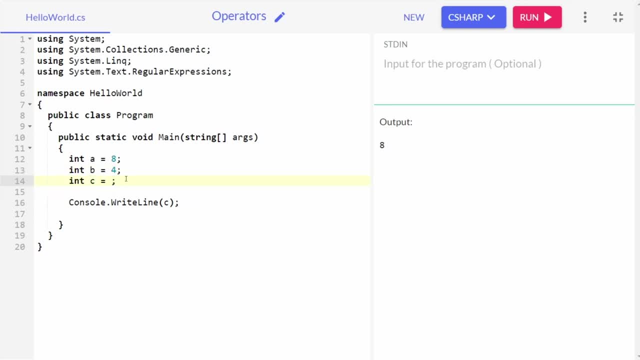 particular, uh, particular calculation from here. all right, let's, uh, let's, let's perform this increment operator on. let's say b. all right, let's give b plus plus, let's see what happens. all right, let's just see what happens. so here you can see. all right, let. let me show you again. 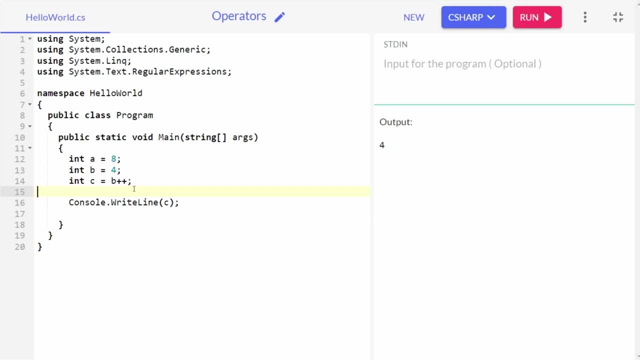 here you can see, the operation is not working means uh, i, i, i promised you guys, right, that, uh, this particular plus plus operator will increment the value. right, let me tell you one thing: it is incrementing now. there's a whole round of concept behind it. all right, but before that, let me show you by incrementing: incrementing the value actually. 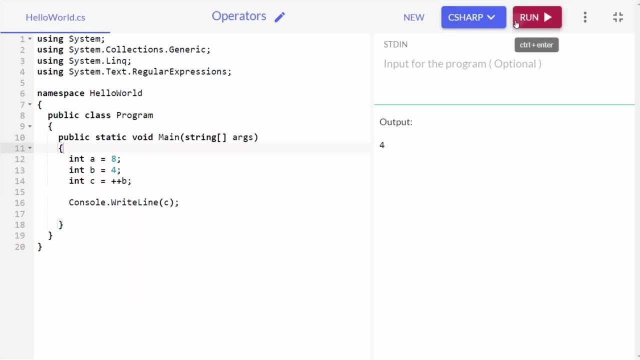 so give plus plus b, all right, let's see if this works. yeah, it works, but why didn't the first one work? see, let me uh, let me wrap your head around it. first of all, the plus plus sign. all right, let me uh make a comment right in here, all right, 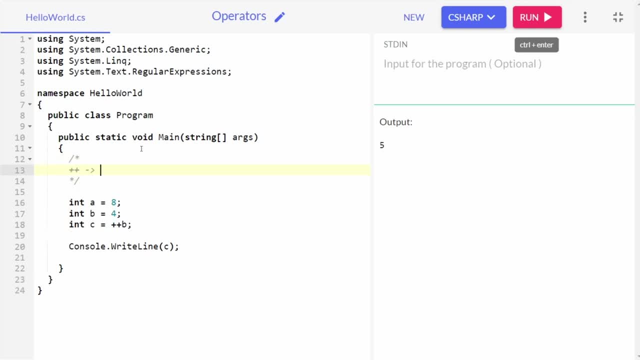 see. first of all, understand all right. this plus- plus operator is always used for incrementing, all right, and this minus- minus operator is always used for decrementing, all right. increment means increasing the number by one, all right means this operator will always increment a number by one, and decrement means this operator will always decrement the number. 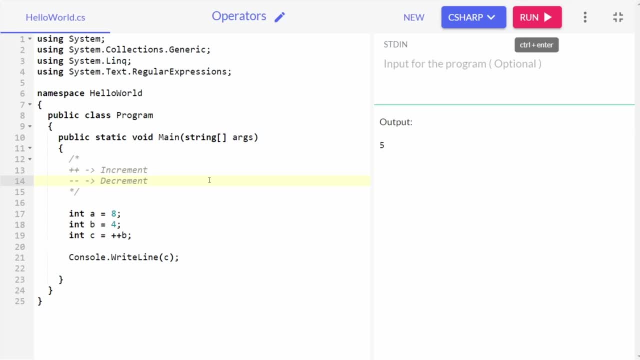 by one. all right, that is, subtract one from the previous value. let me show you something like this. see, the our value was four, right, our value was four. and now it, as it has decremented by one, it is three, right? so that's how increment and decrement. 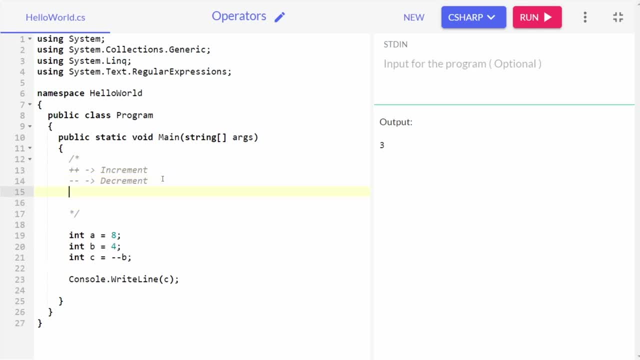 works. all right now the uh. there's a underlying concept, all right. there's the underlying concept behind increment and decrement operator. all right, that is, post increment, pre-increment- all right, and post decrement and pre-decrement- all right. now, what are those? first of all, let's uh, let's. 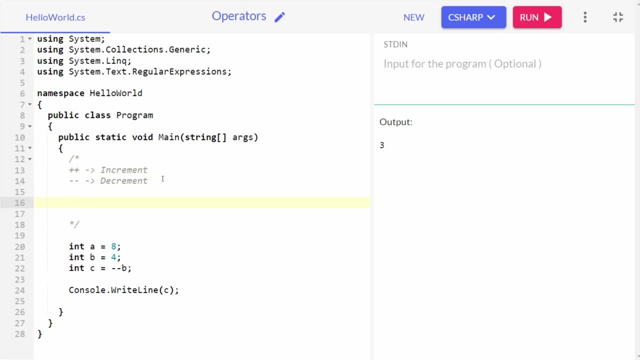 wrap our head around: pre increment: all right, that is the pre and post increment. so first write it: pre increment, all right. so what this does, all right. pre means first. all right means that it will perform the task first, then anything else, all right. understand this way. pre increment is that is it will be. 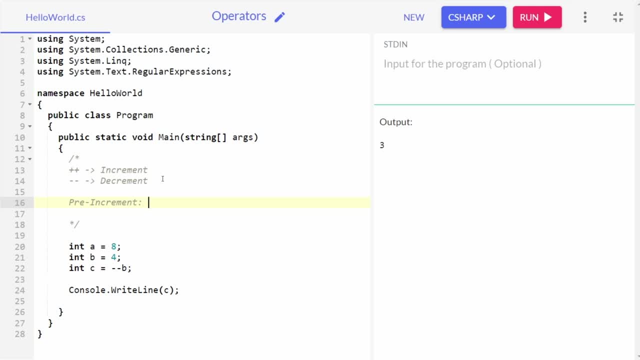 performing? all right, it could. performing the operation first means in our case the operation is incrementing, so it will perform the incrementation first. all right, and how do we write it? fairly simple, plus, plus. first of all, we would be giving this a symbol plus, plus and then write the variable name. all right, 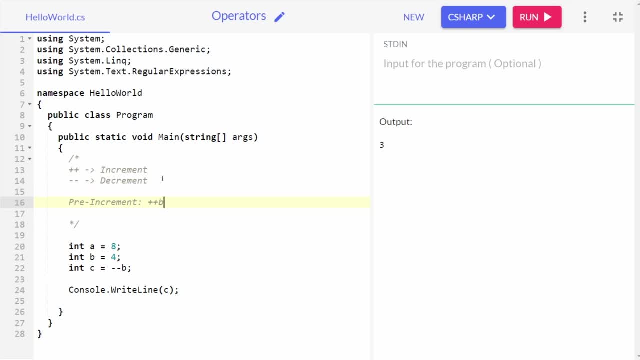 so that's how pre increment work. all right, and post increment is, after all, right, after performing the operation. all right. now, I know this might get a bit confusing, and, and we write it like this: all right, that is B plus plus post increment. now see, let me clear this mess up. pre increment, pre. 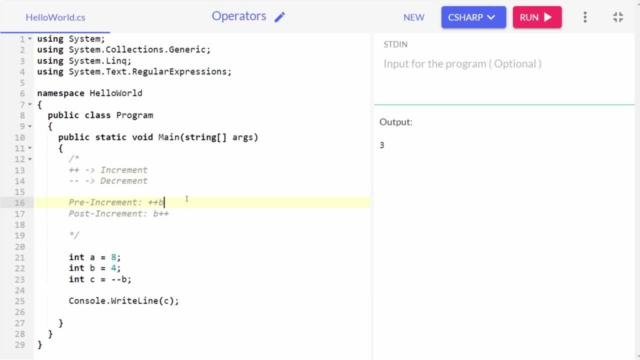 increment. what is doing first? it is all right. first it is incrementing the value, then assigning, and post incrementing or post increment. what is it doing is, first it is, you know, assigning, then incrementing, all right in case of this variable. that's why. that's why previously the B plus plus didn't work. 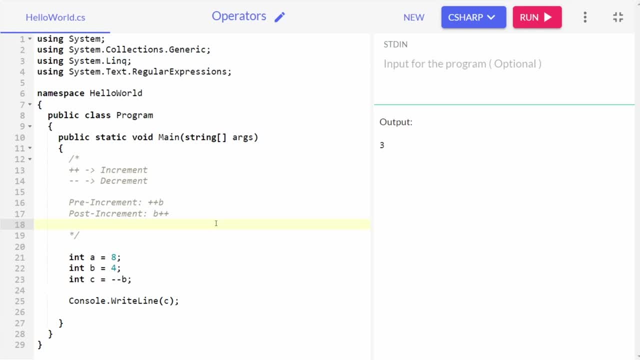 that's the reason, because it or it has already- first it has already- assigned the value of B to the variable C. after assigning it, then it is incrementing. all right, that's the difference between pre and post. that's the difference. all right, nothing else. or else, in both the cases, value is being incremented, just the. 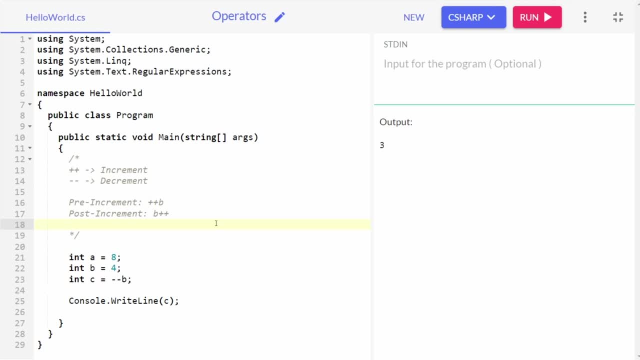 difference is one is doing doing it first, then assigning it, and another one what the other one is doing. it is first assigning it, then incrementing it. that's, that's the difference. all right, so that's how this thing works. all right, now let's try it again. let's, let's try pre decrement. all right, that is plus. 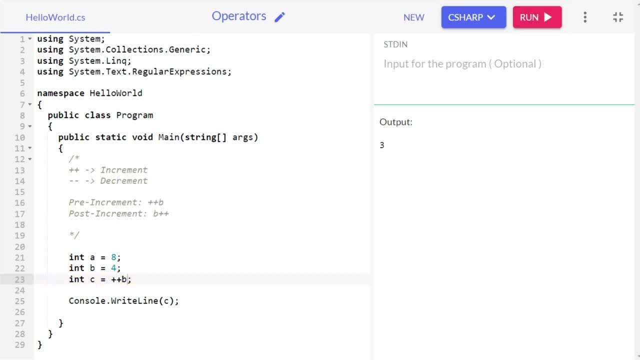 plus B. all right, now just guess the output. all right, let's, let's not get B, let's, let's get a. all right, guess the output. what will be the output? it would be nine. right, because? why? because, first of all, it is incrementing, then assigning. 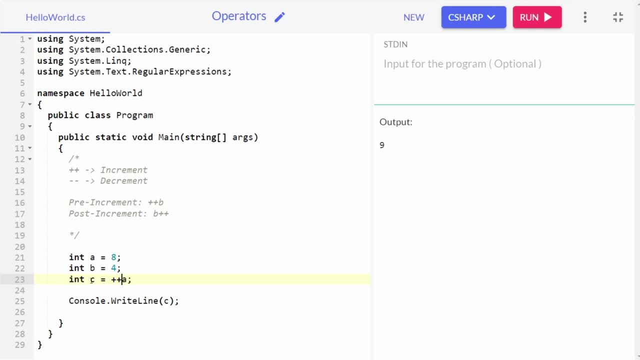 the value: increment, increase, incrementing by how much? is incrementing by one? all right, now let's again try out a plus, plus. let's see how that works. so see it doesn't. it is not showing that it has incremented, but but our particular. all right, this particular value has been incremented. right now, I know you might 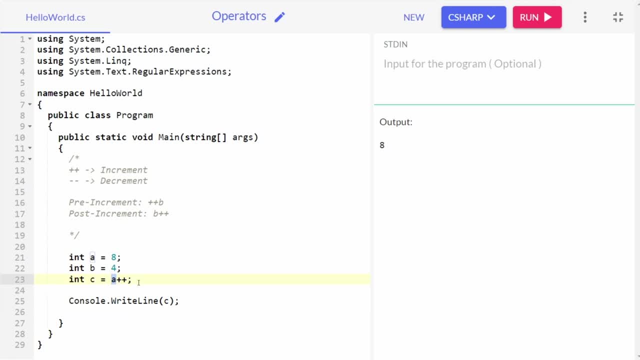 not be believing me already, might think: what? what is the proof? all right, and your question is right, it's totally right, all right. so let me first, you know, let's comment out this line- let me show you the proof, all right, let me show you if, if this, this particular function, is even incrementing it or not. let's see. 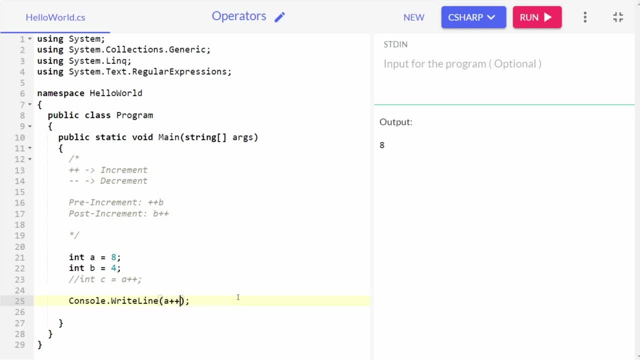 all right, let's see. so give a go to console dot write line and write a plus plus, let's see. so here you can also see that it is not showing all right, that it is incremented right. I know it might be confusing. now let me show you the proof. all right, let me show you the proof. all right, let me show you. 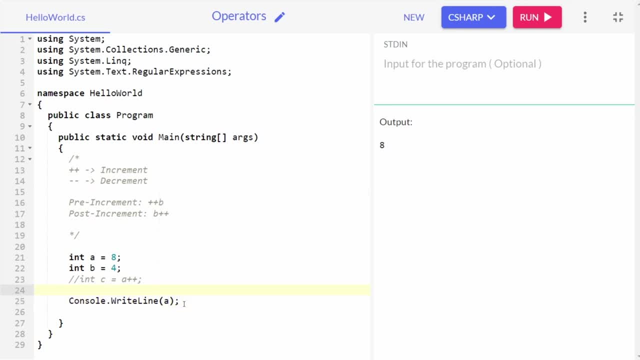 another way around here is the variable. I wrote this variable in here. all right, and again, do a plus plus in here, or I don't assign it to any variable. let's do a plus plus and let's see- yeah, it worked, how. how see, it is not assigning any. 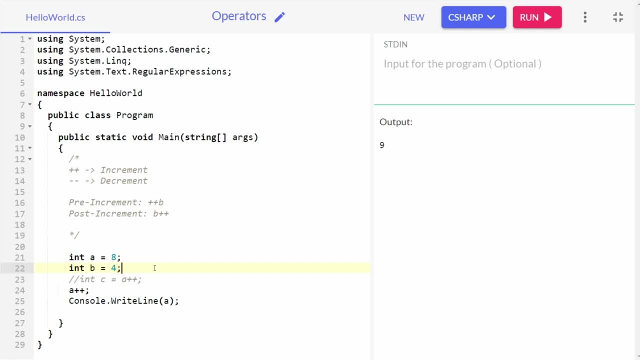 variable. we aren't printing any variable. we are printing a variable, but we have. we haven't assigned this increment, all right, we haven't assigned this increment to any other variable, all right, just like we did in the variable. see, we didn't do that, all right, did we? we didn't, so it just incremented the. 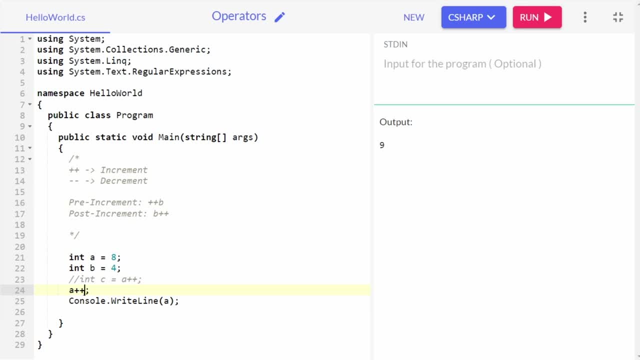 value it didn't assigned itself, so it it is not stored now it as it has incremented the value. that's why we are getting 9. so here you can see that this particular thing is working right. it's totally working fine. so the major decree- sorry, the major are, you know, difference. 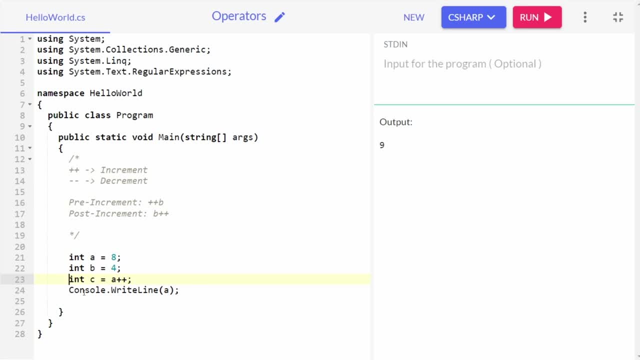 between pre increment and post increment is that one works first and the other one works last, something like that. all right of means this: that is the pre one, all right. the pre increment will increment the value first, then assign it, and the post increment- post increment- will first of first of all assign in. 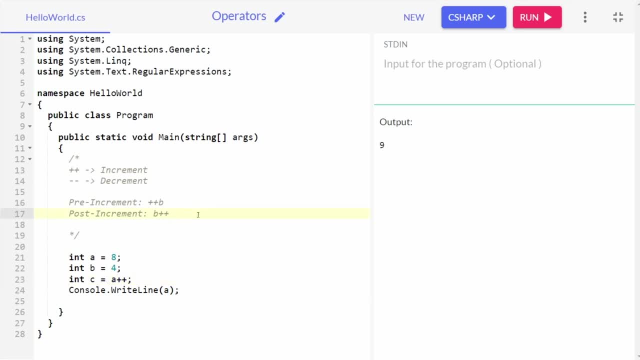 then increment. that's the difference, all right. so same or the same concept goes around the decrement, all right, that is pre decrement. that would be, you know, minus minus B, and post decrement would be B minus minus, right. so let's, let's try this one, two right. first of all, let's try minus minus B, all right. so our 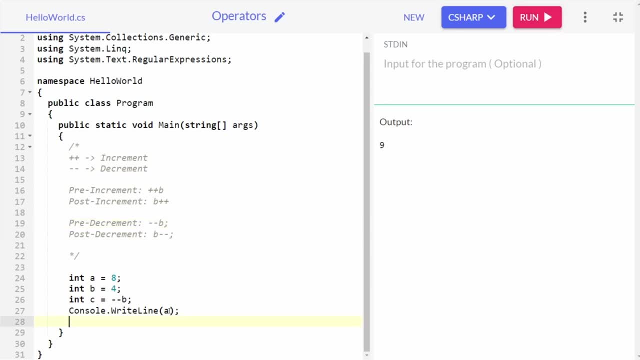 current value for B is, you know, C, and let's print the C right. see, we are getting three, because first it is being decremented, then assigned. now let's again try, all right, let's again try B minus minus in here and let's see if that works or not. no, it's not working, because the value is: 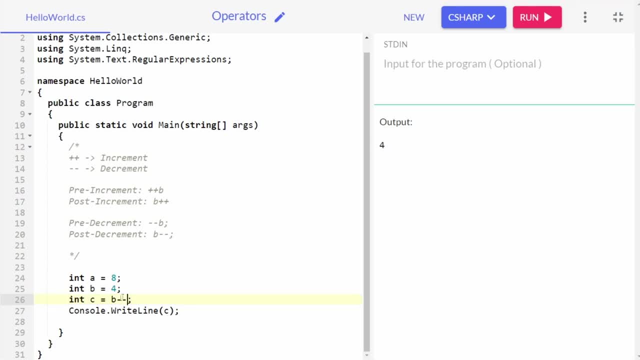 already assigned and we are printing that assigned value now to check whether act in in real. all right, in real if it is being decremented or not. okay, I guess I ran it by mistake. so let's go and give B minus minus and since it is B, all right, and let's remove the C and let's put B in here. 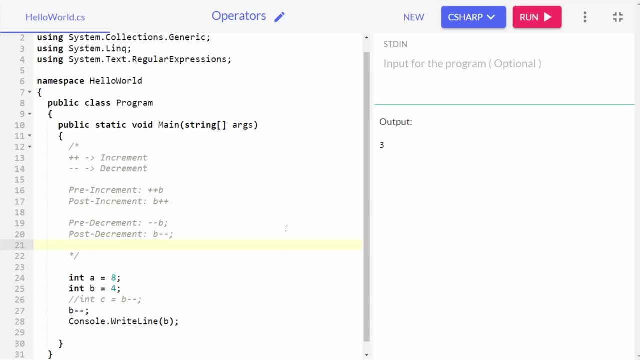 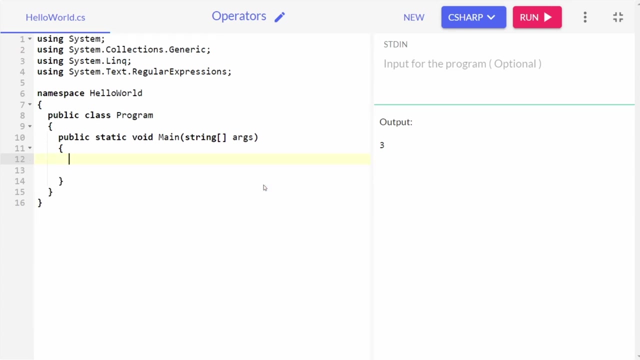 let's see if works. yeah, it worked. it did work. so you can see that this post decrement also work. so that is what we pre and post. dec мо lte is all it very simple, all right, nothing too complicated. so I'm going to erase this program all. 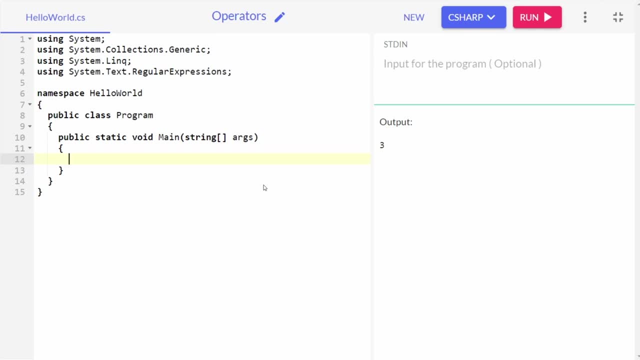 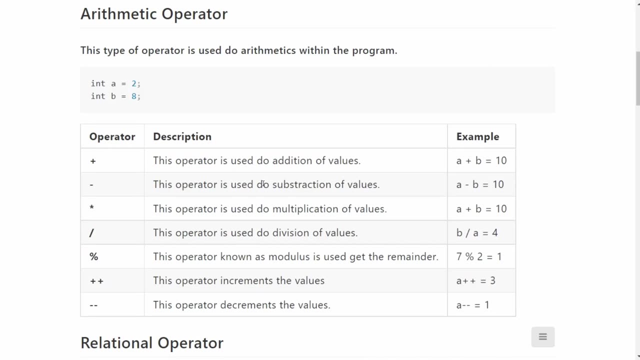 right, I'm going to use this program and go towards our next set of operators. all right, so this concept of operators. alright, addition operator is for addition. subtraction operator is for subtraction. this asterisk is for, you know, multiplication. this slash is for division. 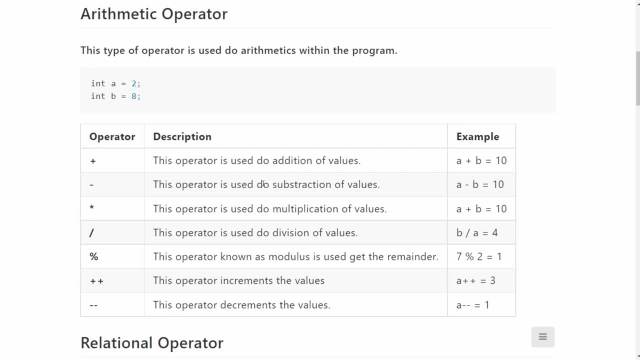 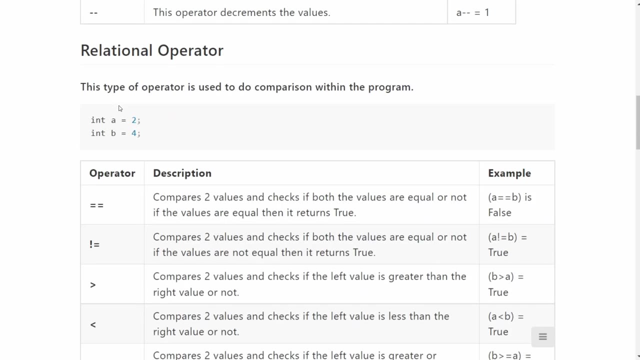 this module, or you can say: percentage operator is for remainder, alright. this plus plus operator is for incrementing and this minus minus operator is for decrementing- alright. so I hope you understand how arithmetic operator works right now. here comes our relational operator. 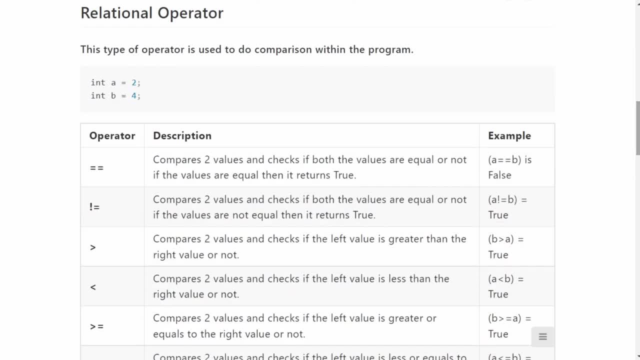 alright, see again. the meaning of this operator is already told in, is already listed in its name relation it tries to you know. tell us that if there is any relation between the two values right now in this operator there are, you know how many types are there? 6. 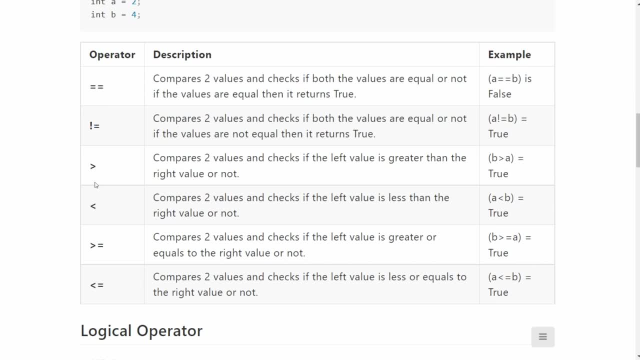 total 6 types are there, that is, equals, equals, not equals, greater than less than greater than equals, less than equal. if you are, you know, I know most. everyone means everyone of you have experience with maths, right? I know every single person of you and you. 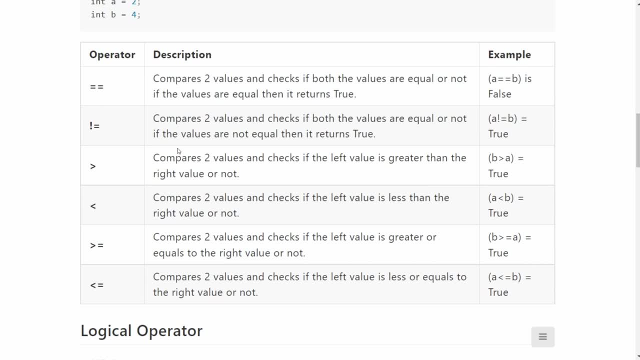 already know what greater than equals does, less than equals does, right. so let me make this thing clear to you. alright, see, If. alright, if the condition is correct, then it will return true. if the condition is correct, then it will return true. if the condition is false, then sorry. if the if. 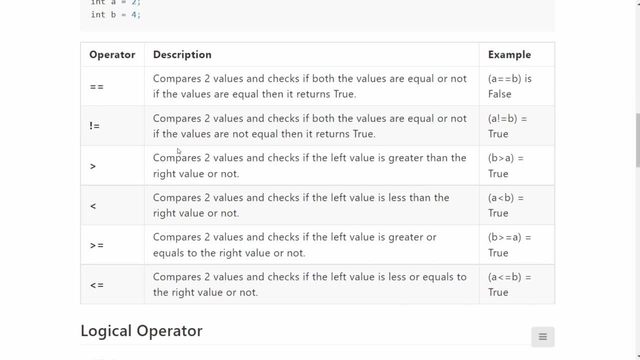 the condition is not correct, alright. or the condition is wrong, alright. or let's say the condition is not matching. then it will return false. alright, and these operators: alright. these operators are wide, very widely used. alright, these operators are very widely. 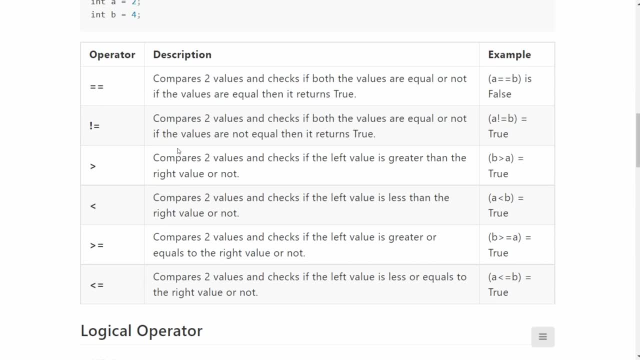 used. They are widely used in if-else operations, alright, if-else for loop operations, so we'll be learning those too, so don't worry. alright, the main focus currently for us is to understand. alright is to understand how these operators work. so for that, let me open my. you know, 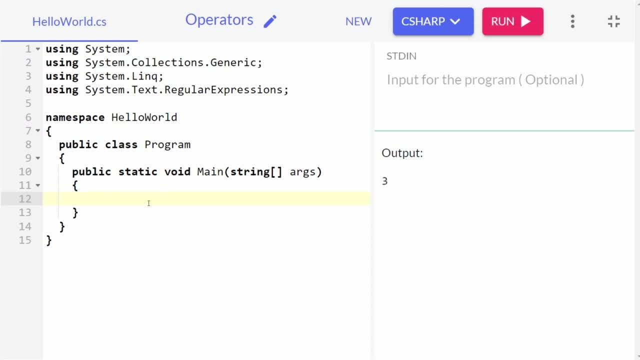 let me open this particular you know this editor and let's see how our relationship. let me open this particular you know this editor and let's see how our relationship works. So let's give it a comment, alright. relational operators. see, there are total six operators. 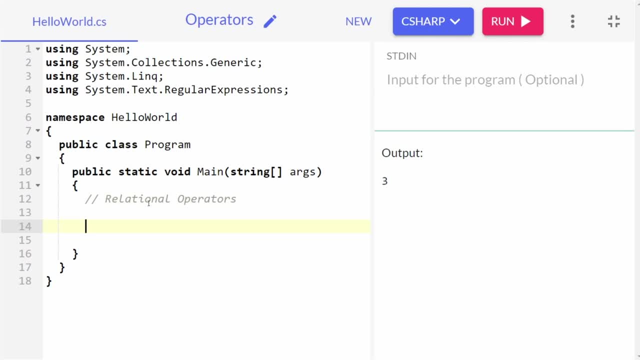 you know who are those and let me show you what do they do. alright, let me show you. So take two variables: that is int a, let's say it 12, and let's take another variable, that is, you know, int b, and let's assign it 10.. 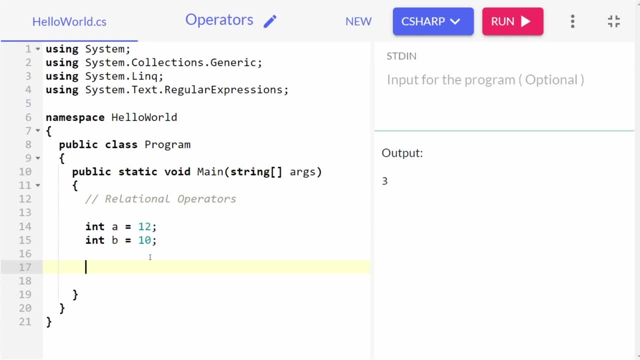 Alright, now. alright, now, do one thing right: console dot write line. write line: alright, and the very first operator is equals, equals operators. now let's see what it will return. let's see it's returning false. why? why see, understand the concept behind equals. 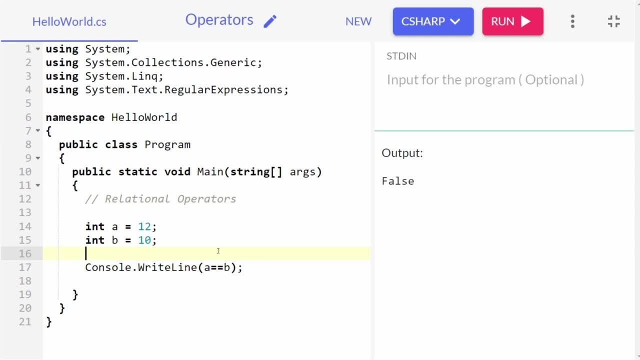 equals. this is this operator: alright. this operator compares two values: alright, and if both the values are same, alright. if both the values are same, then it will return true, and if both the values are not same, then it will return false. alright. so these. 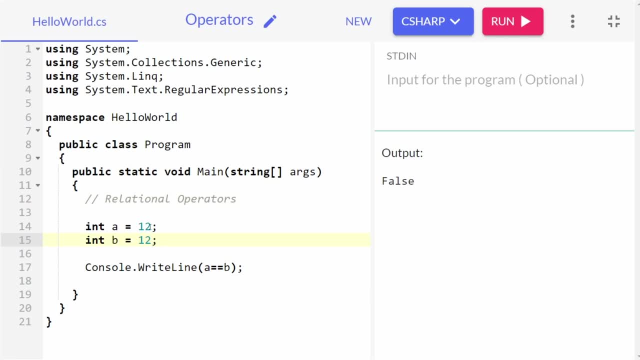 equal, equal to operator is used for comparison now, as I've changed the value of b to 12, and also the value of a is 12, now let's see what it returns. see, it is returning true because the condition is true. 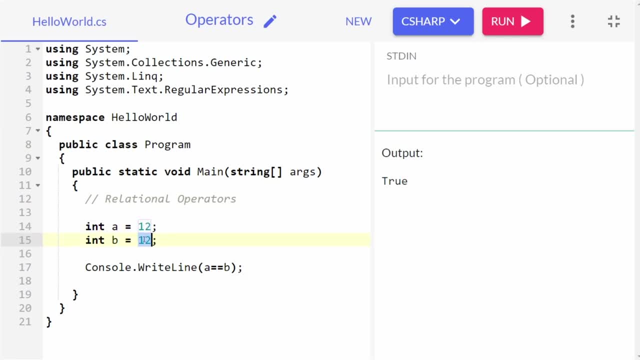 The condition means a and b Is, means a and b is. yes, it is true. It's true That that's: a and b are equal, all right. a is also 12, b is also 12. so that's what? uh, you know, equals, equals. 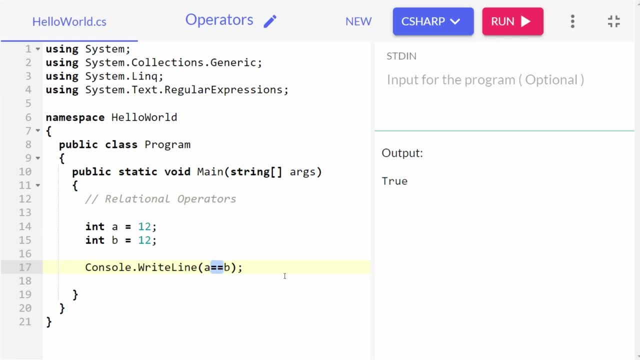 operators does. now, the second one for us was not equals. all right, it's the total opposite. it will check if the value is equals to or not equals. now let me show you all right: a not equals to b. now can you guess what will be the output? all right, pause the video and think. 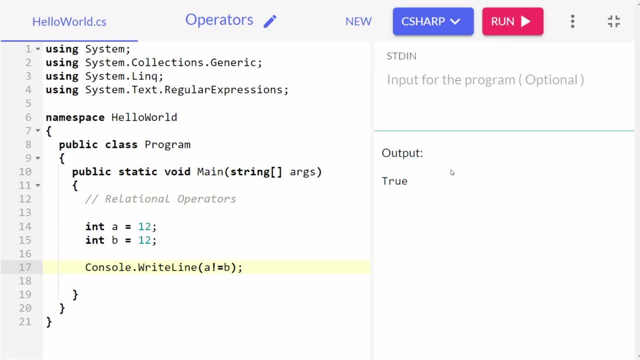 for a few seconds and, uh, you know, try to answer it by yourself. what will be the output? so let's see, it is returning as false. why? because the- it is the, the conditionally is also- is only telling us: not equals to. we don't want it to be equal, all right, it means if it, if both the values are not. 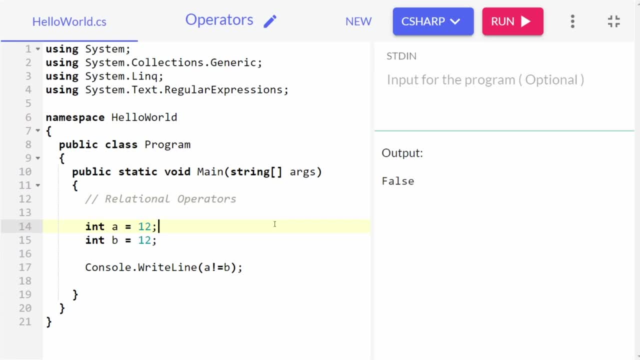 equal to each other, then only i will return true, and if they are equal, i will not. i will return false. now let's try to change the value to you know. change the value of b to 10. now let's see it is returning true. now we understood about equals, equals operator. we understood, you know. 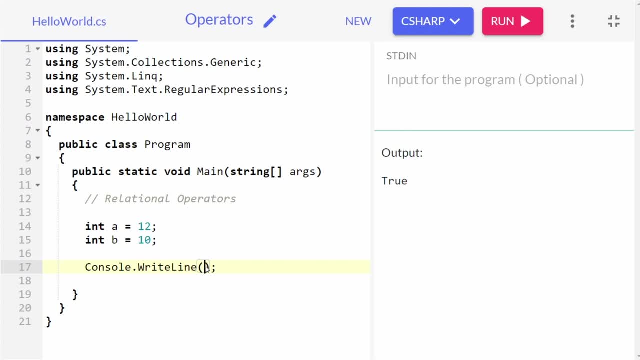 we understood about: uh, not equals operator. what's next? next is greater than all right. next is greater than and less than operator. now let me show you. all right, let's see a, all right. a greater than b, of course, you all know it. will, you know, return false because, uh, sorry, it will. 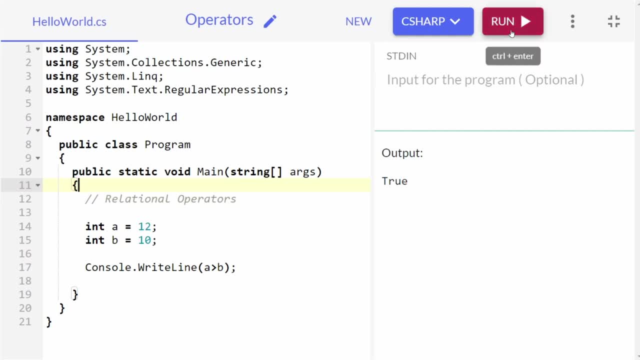 return true because, of course, a is greater than b, a is 12, 10, b is 10. now, let's see, yeah, it is returning true now. now you know, let's uh, let's uh, let's give it 13. all right, let's change the. 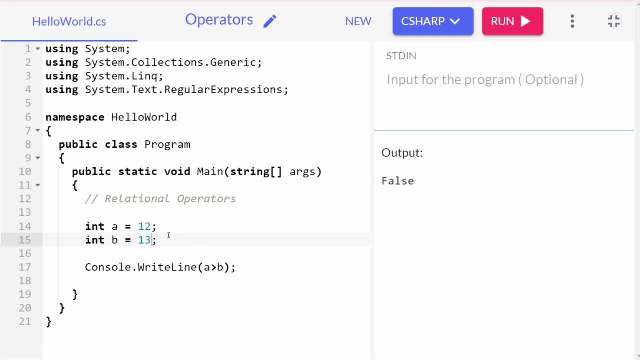 value of b to 13. let's see, it is returning false. right? it is returning false because of course, bro, uh, a is not bigger than 30 means 12 is of course not bigger than 13, right? that's where it is returning false. so now, let's, let's back it up to 10. 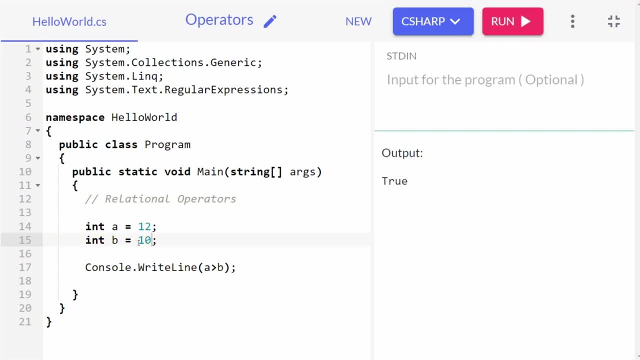 and let's try it again. yeah, it is returning true, because 10 is less than 12 and 12 is greater than. all right, 12 is greater than 10.. so same again. let's try out: a less than b. all right, of course, the the condition has to be true. all right means: uh, this condition is telling us the. 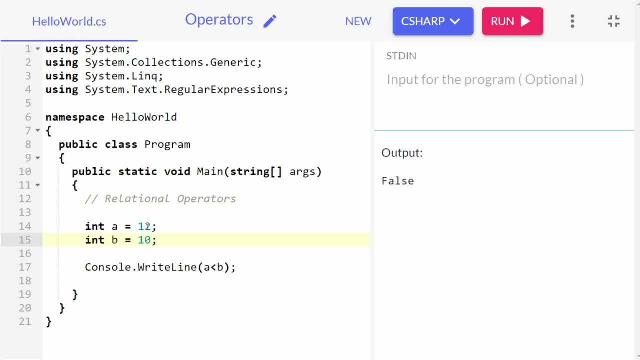 truth: a is not less than b. a is not less than b. that is false. that that's why the output is false. how can 12 be less than 10? it cannot be right, so that's why it's returning false. now let's say, if i change the value of a to, let's say, 5- sorry, yeah, let's change it to 5 and let's see the output. 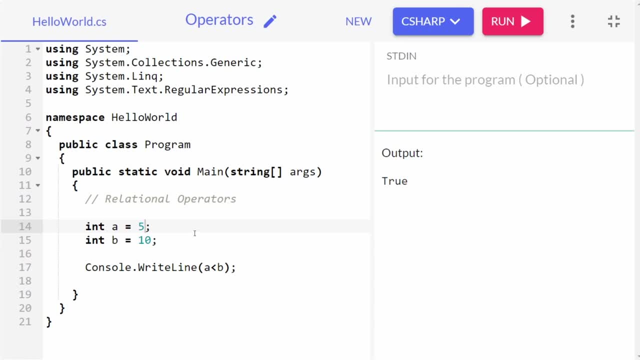 now it's returning. true, because it is returning to, because the value of a is, of course, less than b, because the value of a is 5, the value of b is 10 and 5 is less than 10.. so that's how this, you know. 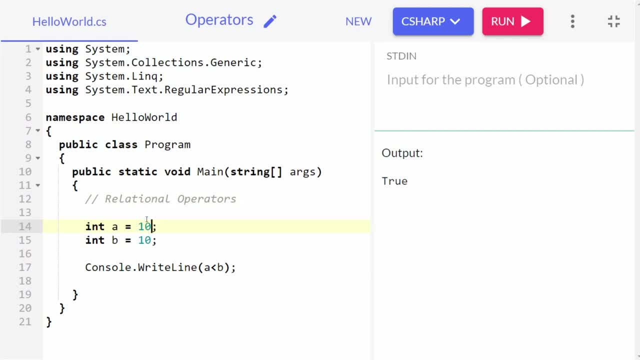 you know this thing works. now let's say: all right, let's give both the values you know, equality. that is, let's make a to 10, b to 10. right now, let's see it's returning as false. it is returning as false because there isn't any option, right, because? uh, you see that that means for these type of no uh. 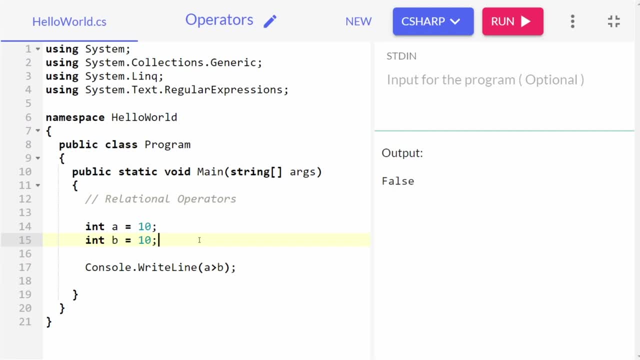 for these type of values. now, uh, less than equals and greater than equals comes in right. so we are going to see those uh operators now. so till now, what we did till now we learned about, uh, you know, arithmetic operators. all right. now we are going through relational operators and 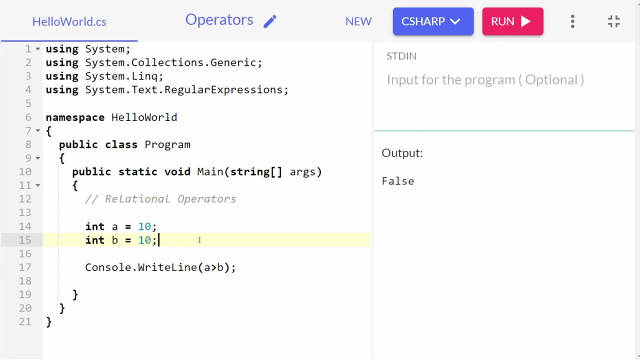 in relational operators, we learned about equals, equals, not equals, greater than or less than now, uh, here comes two more operators, all right, here comes two more operators less than equals, greater than equals- all right now let's see. first of all, you know, let's uh, reset its value, let's a b12 and bb10. right now, in here, it's very simple: you just have to give. 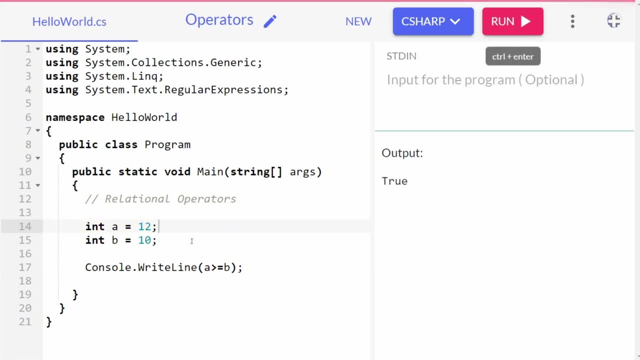 a greater than equals b. now let's uh try and run it. here you can see. here you can see, it is returning us. true, there's no difference, right? you might be thinking: oh god, what am i showing? what am i showing? it's just like the, you know the previous one, just like the previous greater than. 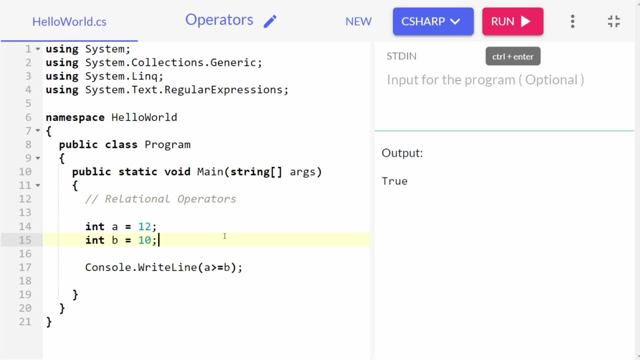 equals sign. sorry, greater than sign. no, there's a difference. you just have to wait, so here you can. it's returning true. yes, of course it will return true, because 12 is greater than 10. now, let's, let's make it to 10. all right, let's make it up to 10, let's see. oh my god, it's again returning. 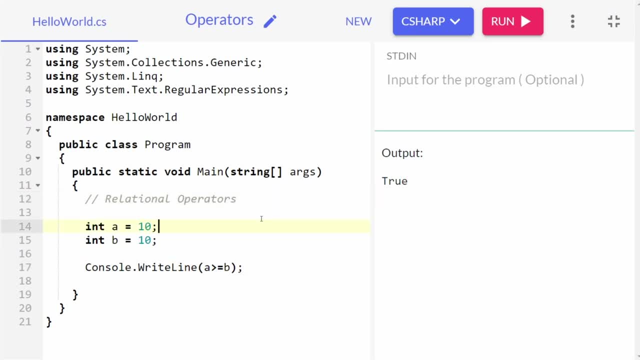 false. why? that's because here's an equals to sign it. the condition is telling: all right, if the number is greater than equals to some other number, then only return true, and if the condition means if that condition is not matching, then return false. now, let's, let's try giving 9. now let's see, say it is giving us false right now, let's again, let's try less than. 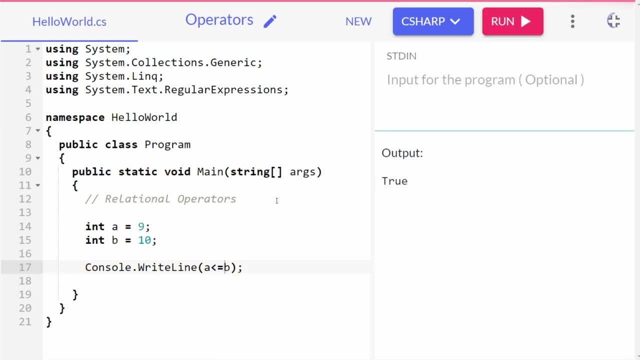 equals. it's returning us true because you know, uh, 9 is less than 10. now again, let's give you know, 10 to a. let's see again: you, you, you, you. you is returning as true because 10 is equals to 10. right now, let's give 12 to. 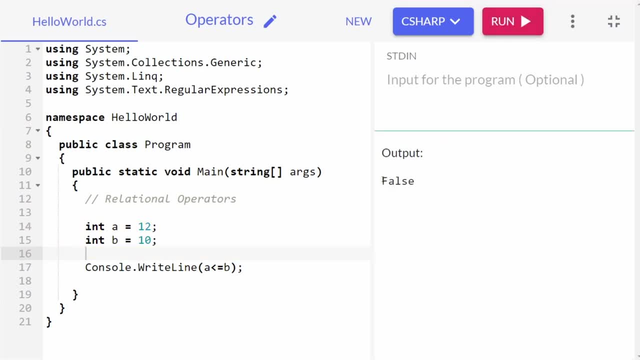 a. let's see, it is a returning false. alright, because then the condition is not matching. now condition is not matching. it is: 12 is nor less than nor equals to you know what? nor less than nor equals to 10. so that's how this whole relational operators works. I hope the concept behind relational operators 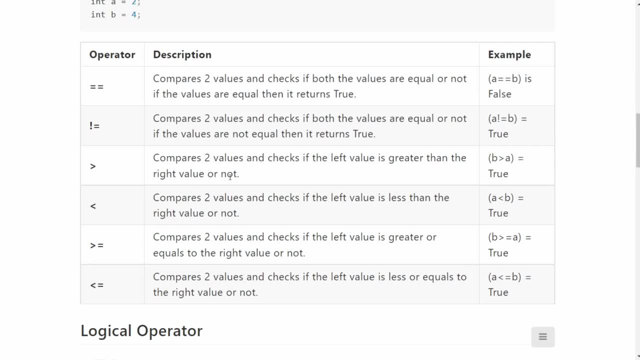 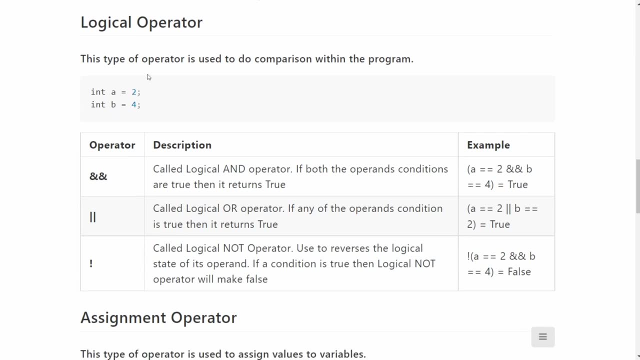 is clear. all right, now, as we are very clear around relational operator, let's understand the concept of logical operator. all right, see, logical operators are you know? they are very simple to understand. all right, very simple. some people don't understand it, but some people do understand it. but some people. 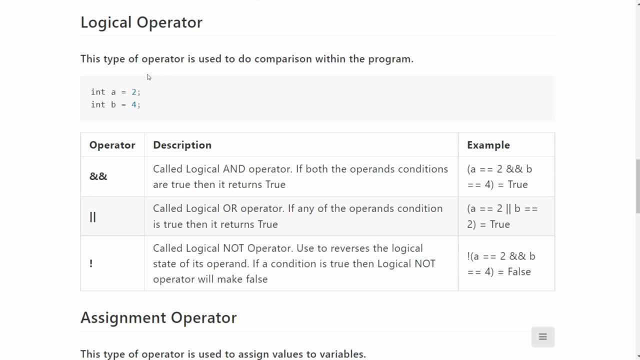 like exaggerated. I've seen like some people are exaggerated- exaggerated but currently in the beginning stage- and operator- and you know these or operators are very simple, very simple to understand. now, logical operator, what are they? all right, these type of operators, now all right is used to. you know what? 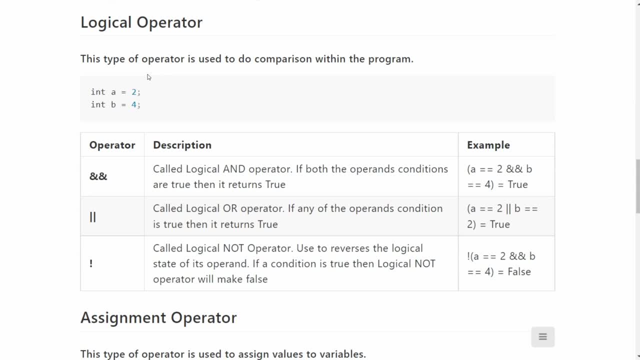 can I say? what can I say? I'm not getting the right word. these two operators now put, put some condition between, like you know, another two condition. all right, I know it might get a bit confusing. I will show you how to you know how this works, right? but for now, understand, all right it. 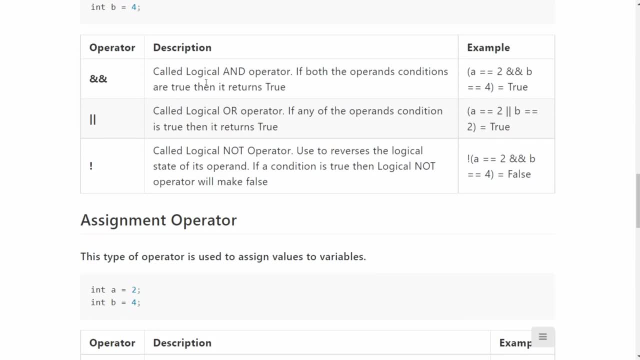 performs logical calculations. all right, understand it like this. it performs logical calculation. now, here you can see: two and all right, that is logical. and two ampersand signs. all right, what this means. we call it as an and operator. what this means is in this example. here you can see, there are two conditions, that is, a equals equals two. 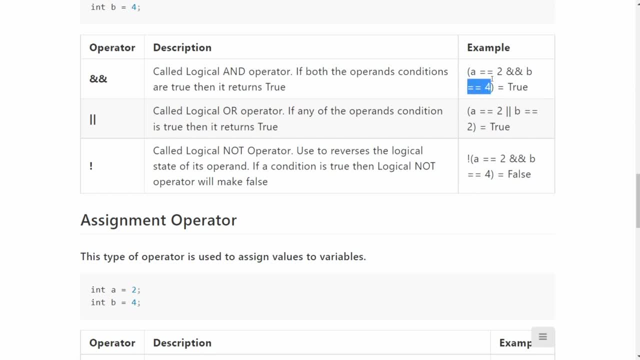 and another condition is: b equals equals four, all right if both the conditions are returning true. all right. if both, that is, a equals equals two is true and b equals equals four, is true, then only it will return true. let's say any of the condition in here. let's say let's, for example: 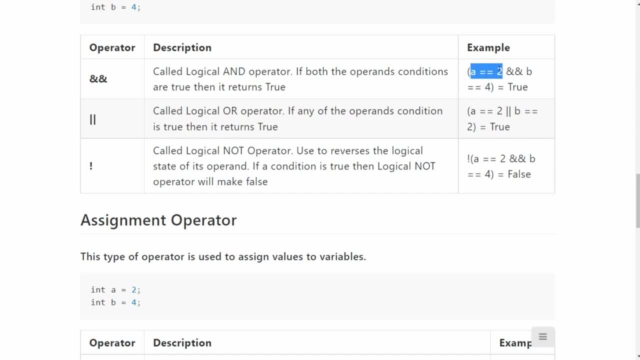 let's say: b equals equals four is false, but a equals equals two is true. all right. for example, then it will return false. that's how the and operators works, all right. so, as we have understood the and operator, let's you know, let's try to code it. 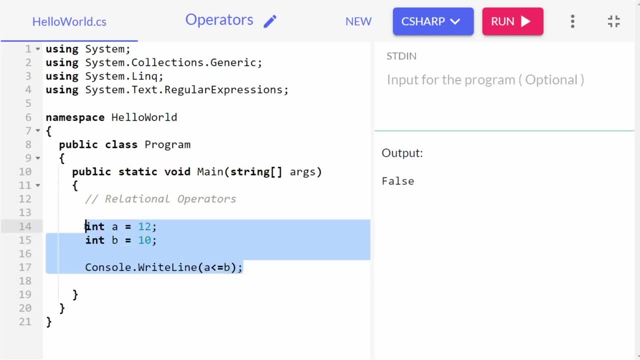 you right, let's see how this thing works. so first of all i wanted to remove this whole code, all right. now again write in here logical operator. all right, cool, now here. assign two values, that is, int. a equals, you know, 10 and b. sorry, int and. 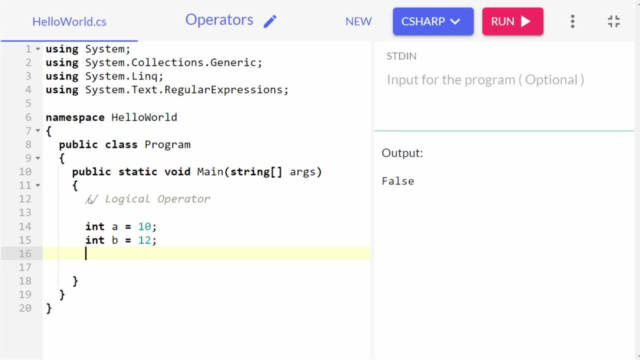 b equals. again, you know, let's say 12, all right. and now, you know, go to console dot right line and in here in here, what you have to do is first of all first write one condition, that is: a equals equals 10. all right, we are comparing the value of a. 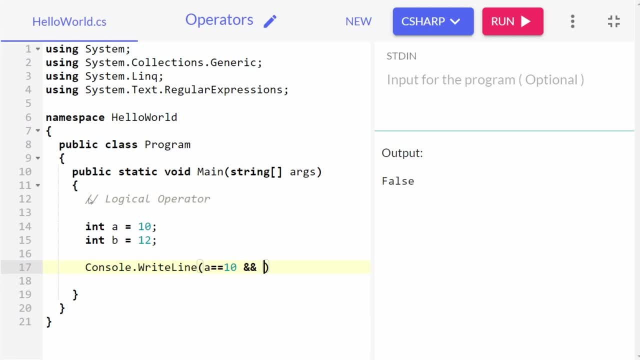 to another value, 10. all right, now here comes the and operations. now let's again do the same thing for b, that is, b equals equals 12. now let's try and run it. it is returning us true, because both in here, both the conditions are true. now, let's, let's. 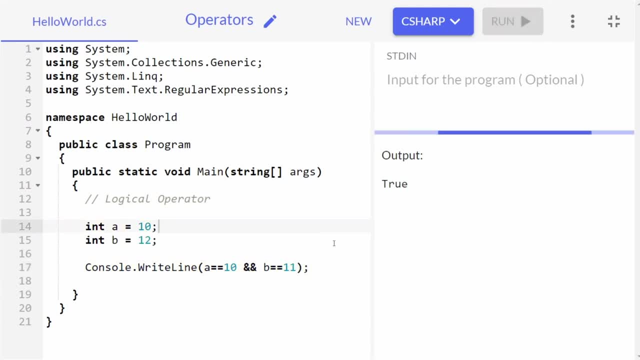 change one value, that is, let's change the value of b to 11, let's see. so it is returning false. so here the concept of you know, and operator is very clear. that to to means to get the and operator return true. we have to make sure that both the conditions all right, both the conditions. 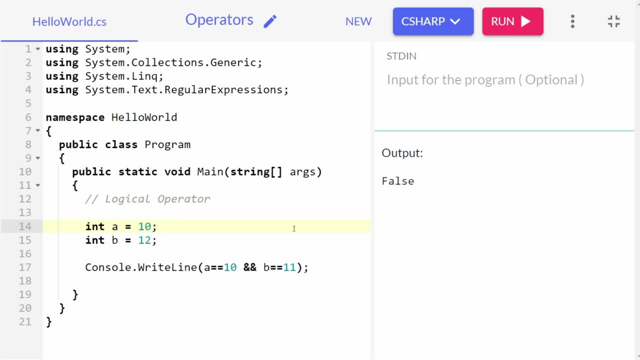 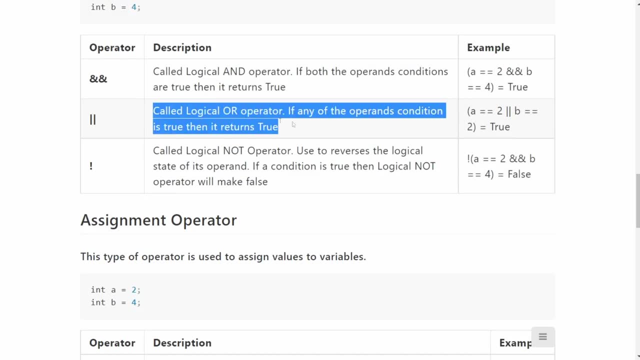 which are, you know, using the and operator should be true, all right. so that's what the purpose of. and operator is. now, another operator is or operator. all right, it's like if this doesn't works, then we will work with these, all right. so basically, what it means is, let's say there are two. 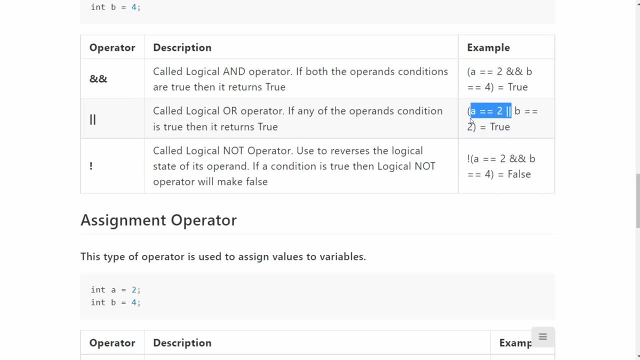 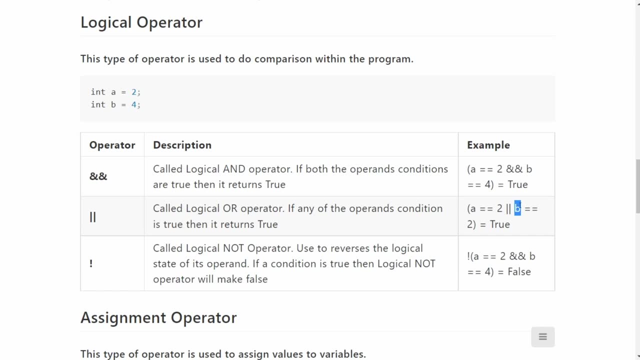 values: a equals, equals to b equals equals to all right. that is in our case, all right. in here b equals four right. that means in here b all right for b. it is false. the condition b is false because of course b is not equals to four. all right means b is four. of course, sorry, i'm i just you know. 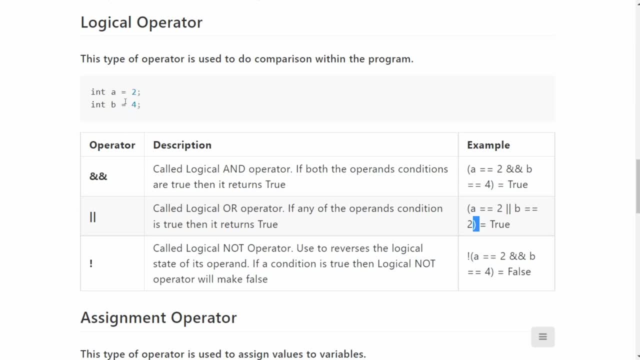 confused you, i i think so. let's understand it this way. see, b is b, right in here is four, and we are comparing b with another value, two, right, and of course two is not equal to four. all right, it is not so for this particular condition. it will be false now for this. all right. 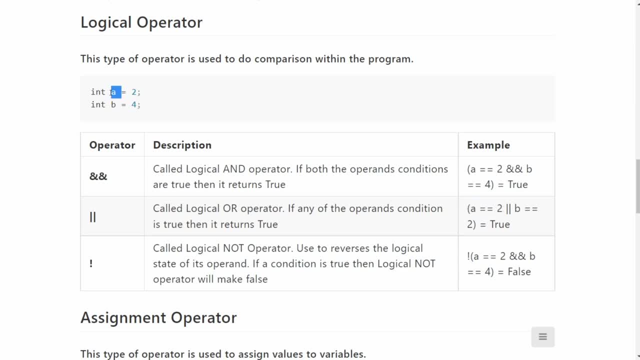 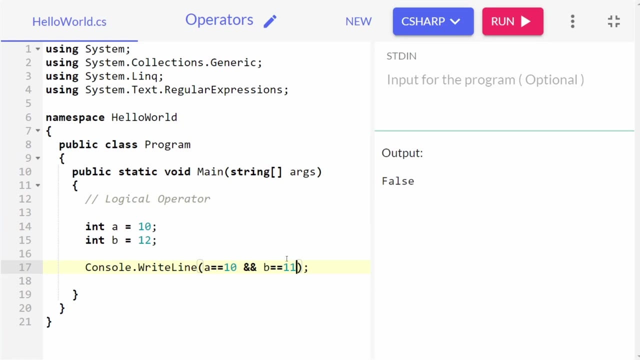 that is a equals equals two. in here the value of a is two, and two equals equals two. that is this. but for this condition it will return true. so as one condition is true, it is going to return us true. all right, so let me show you so here you can see. i already have it assigned. that is a equals equals 10. that 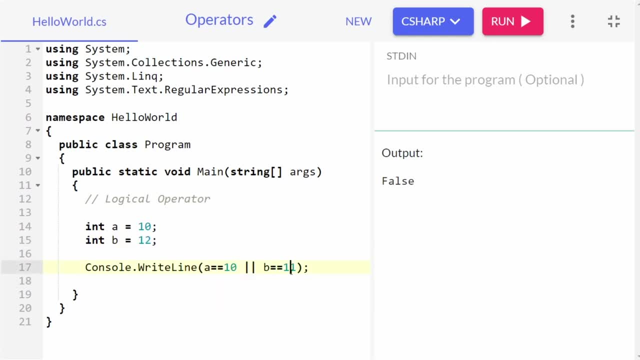 is 10 equals equals 10, it will be true, and b equals b equals equals 11, but in our case, b is 12 and and we are comparing it with 11.. let's see, it is returning us true. all right, now let's do this. 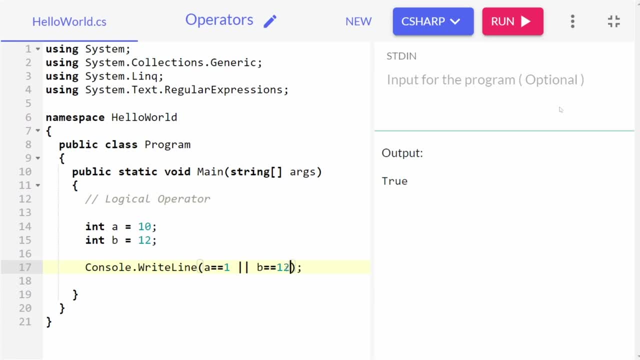 the other way around. let's change it to 10 and let's um, you know, let's change the b to 12.. again, it is returning us true, because you know, one of the condition is continuously matching. now let's say: change, you know, change, uh, both the. let's make both the condition and false and let's see: 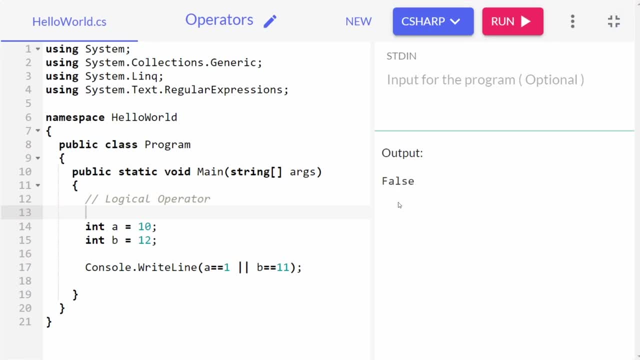 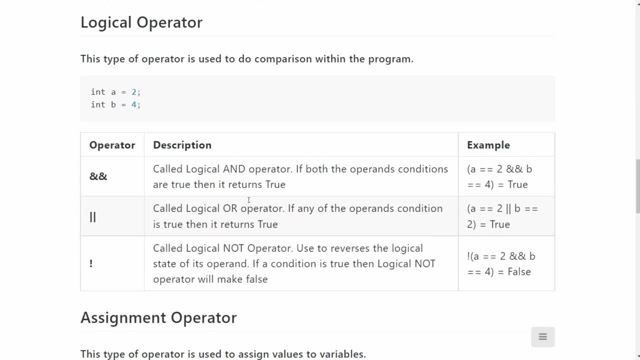 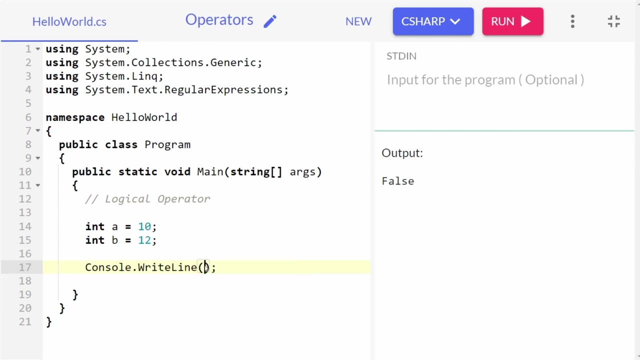 here. you can see it is getting us, it is giving us false right. so that's how this thing works. that's how or operator works. now this, not operator. now it's totally different. all right, now, let me show you not operator, and it will, uh, it will, you know, reverse, or you can say inverse. 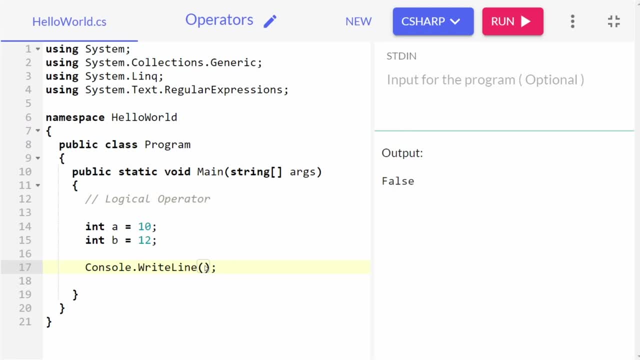 all right, invert the result. all right, it will invert the result now. for example, let's give a equals- equals, you know- or 10. all right, the output for this will be true. right, the output for this will be true now if we all right. patch this particular uh condition means uh, wrap this condition with the you know. 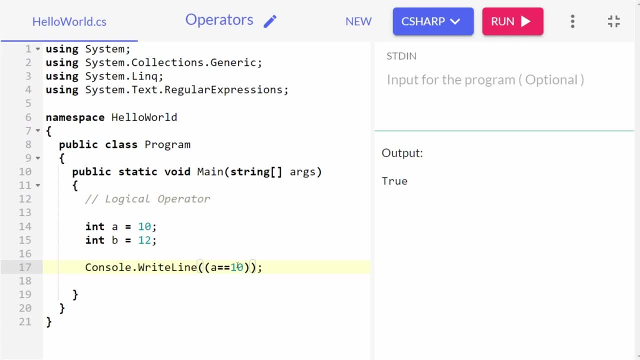 round brackets and put you know, and put uh uh- what is this called except exclamation mark, or you know, not, all right, not operator- in front of that uh uh condition and then run it here. you can see that it is. although the condition is true, it is. 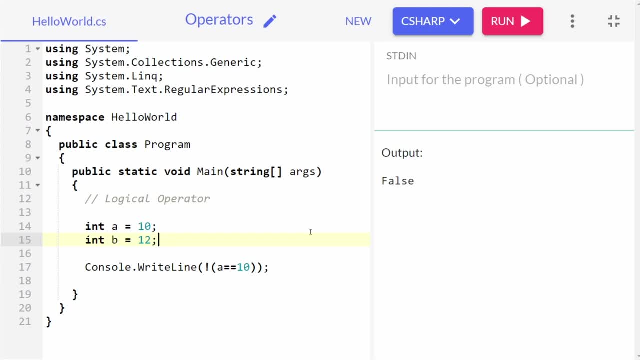 uh returning us false. why? because this this particular not operator, now it is uh inverting the result. now, if, if it is, you know, if it is resulting to, you know, false, it will return us to. all right. so that's how this not operator works, all right. so till now, we have uh, we have learned about uh. 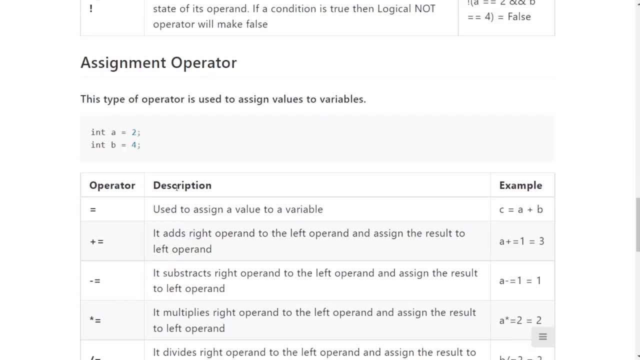 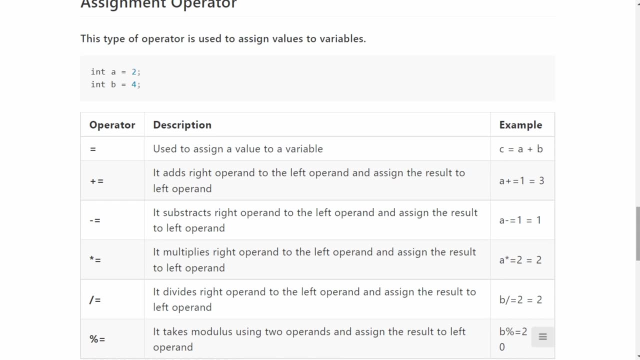 arithmetic operator, relational operator and logical operator. now here comes the last one that we are going to learn. all right, this one is assignment operator. all right, see, assignment operators are, you know, going to be very useful to us. all right, they are really going to be very useful to us. and, uh, you got to be like you know. 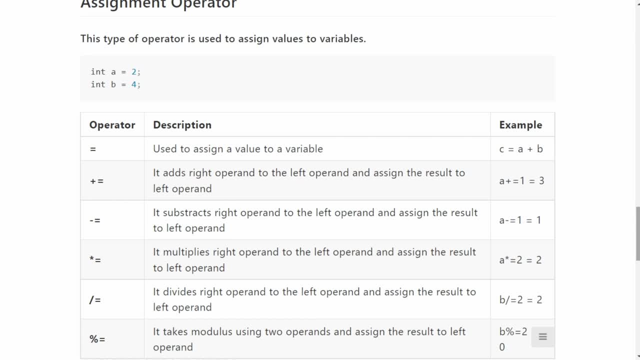 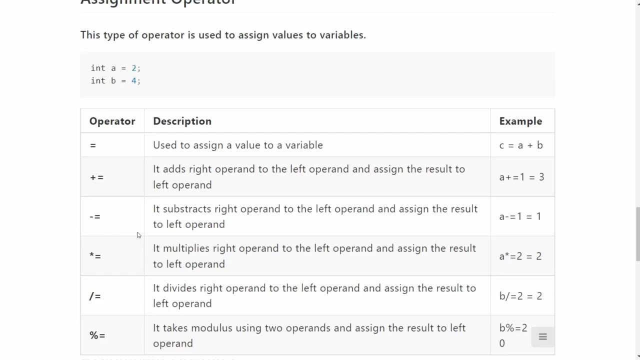 very uh like. you need to understand how these things work. all right, uh, understand it carefully, because sometimes- not because of these operations- it might like, especially in this case, this uh, these uh, three for uh for case of these three. it gets a bit confusing, all right, so don't worry, i'm. 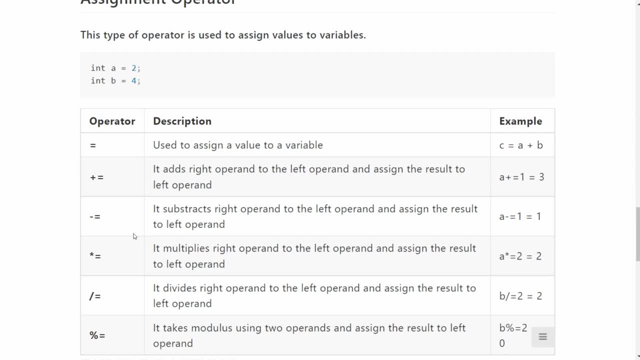 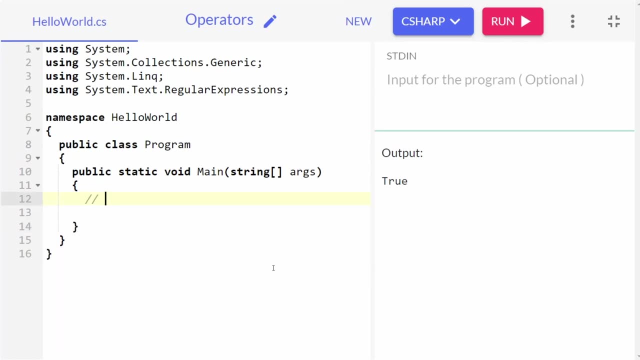 going to you know, uh, understand, uh, make you understand this concept brick by brick, all right. so let's remove this. all right, let's remove this again, comment it and uh, let's give it a name, that is assignment. all right, assignment operator- all right, very cool, very great. now create a variable int. a equals you. 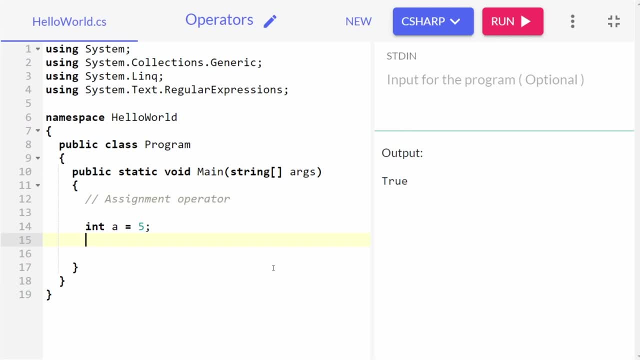 know, let's, uh, let's give it five. all right. now, here we'll used our very first operator, which one equals operator. all right, how? see? equals is an assignment operator. it's in its name only see equals is assigning a value to a. all right, equals is assigning a value to a. that's how it is working, right. 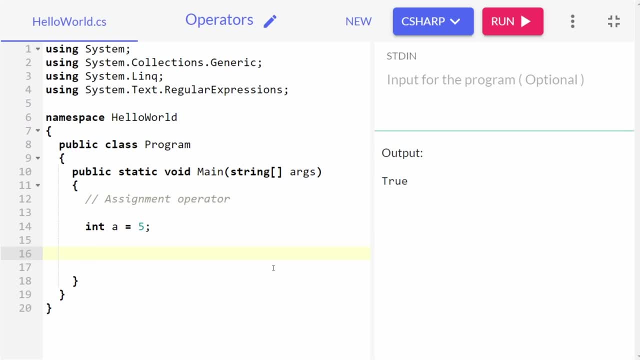 that's how it is working. so equals is an assignment operator. we learned about our very first operator. right means not very first, but we learned about our first operator in assignment operator category. all right. now next operator is plus equals. all right, see, i hope you remember we. 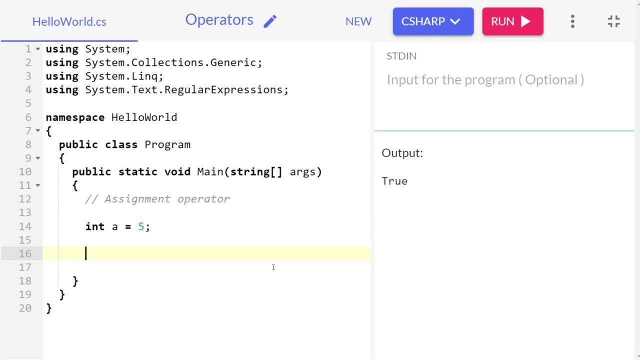 learned about uh- increment and decrement operator, uh plus plus equals operators- also does the same thing. all right, but it you know it is more modifiable. all right, it is more modifiable. it also increments the value. all right, it also increments the value, but we can determine how much. 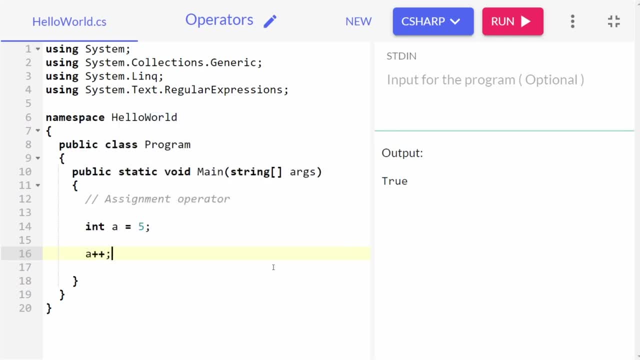 to increment. all right, like in the previous one, we are giving, you know, uh, a plus, plus, and it was only incrementing the value. all right, it was only incrementing the value by one. we weren't able to. you know, change it means if we want how to do like, if we use this, we won't be able to increment the. 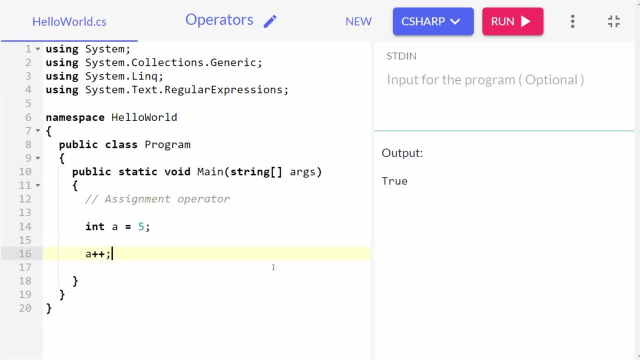 value with 2, all right. it will only be incremented with 1, all right. but with the plus equals operator, what we can do is a. a plus equals 2.. all right, and now let's, let's print it a. let's see, it is 7, because 5 plus 2 equals 7. right now, you know, there's a more abbreviated 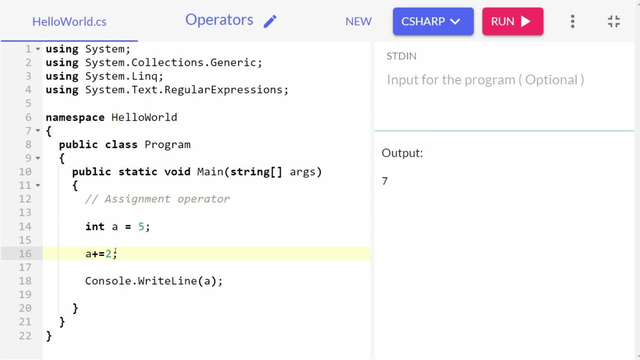 not abbreviated. there's a more expanded version of it. all right, let me show you. a plus equals 1, all right, a plus equals 1, okay, so plus equals 2. or it also has a d- uh, you know big version. that is a equals a plus 2, all. 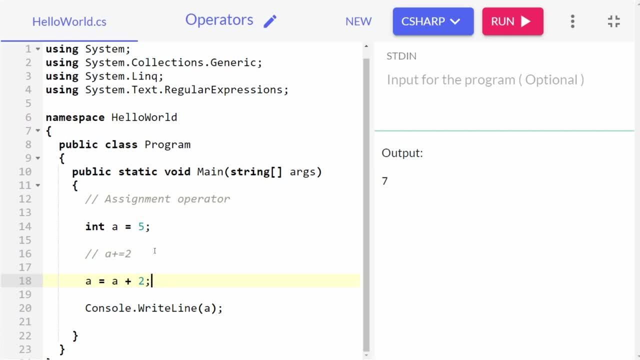 right. so basically this: this would help you to understand how exactly it is working. all right, how this operator is working. so pay attention carefully what is happening. first of all, it is performing the addition of a, that is 5 plus 2. then it is assigning the addition to a to the variable a all. 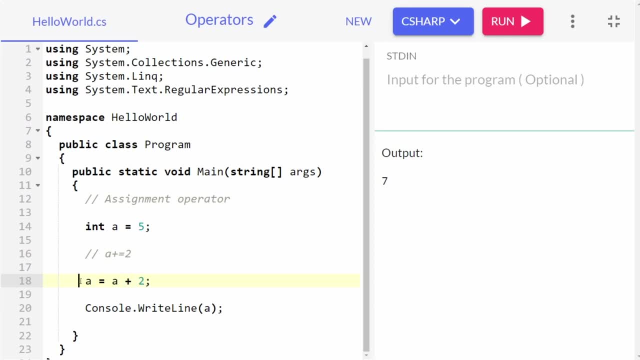 right, it is performing the addition on a, then it is assigning that addition to the variable a. that's how it is working. all right, so that's how this plus equals operator works. all right. now the next in our you know the first, uh, first let's understand what we learned we. 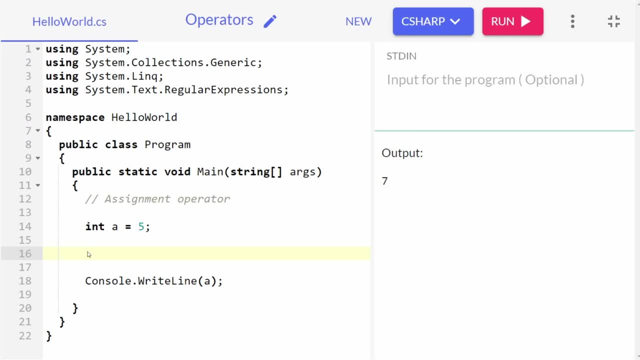 learned about uh assignment, that is equals operator. now, uh, we learnt about plus equals operator, all right. now here comes minus equals operator. This is the decrementing operator, but is modifiable. all right, That is a minus equals 2.. Let's try it out. 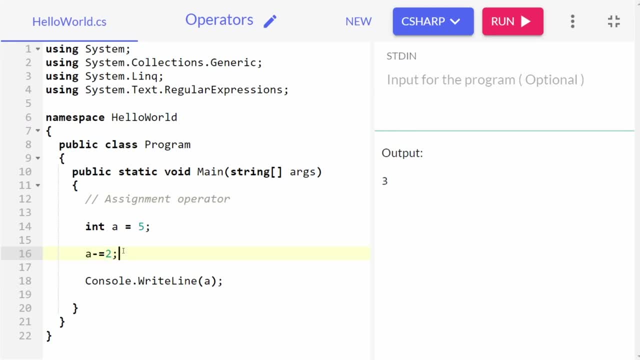 See 5 minus 2, 3,. all right, Now you know, let's expand it. That is a equals a minus 2.. Again, it's doing the same thing, right? Just it is more expanded version. 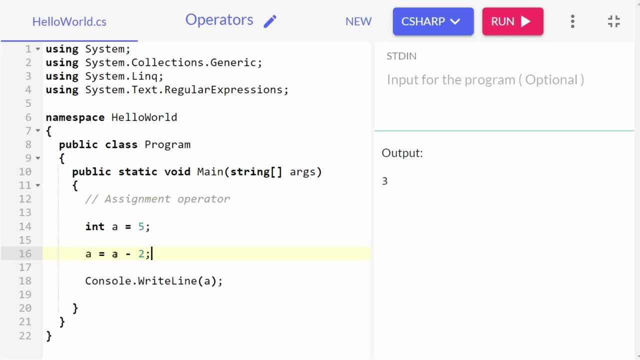 What it's doing. It is first performing the calculation, That is, it is first, you know, decrementing the value by 2. Then it is assigning it. all right, So that's how it is working. Now we learned about the three operators. 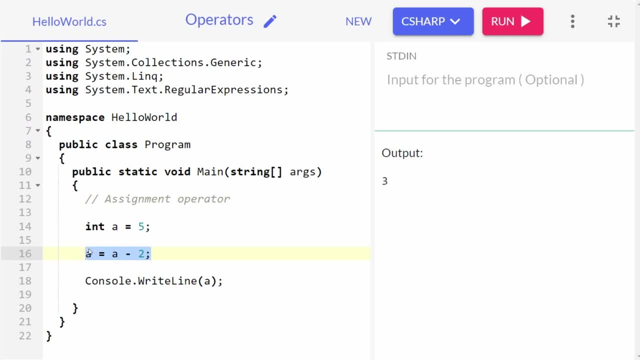 That is assignment plus equals. all right, That is equals plus equals and minus equals. Now here comes multiply equals Now with the first two operators, your, I guess your concept might be, but let's say, if it isn't clear, I will show it to you, all right. 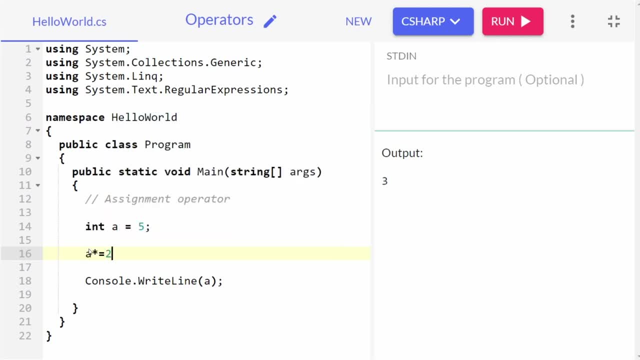 The syntax is something like this: a asterisk equals 2,. all right, So what will happen? It will multiply 5 by 2,, 5 with 2,. sorry, Let's try it out. See, it is multiplying it. 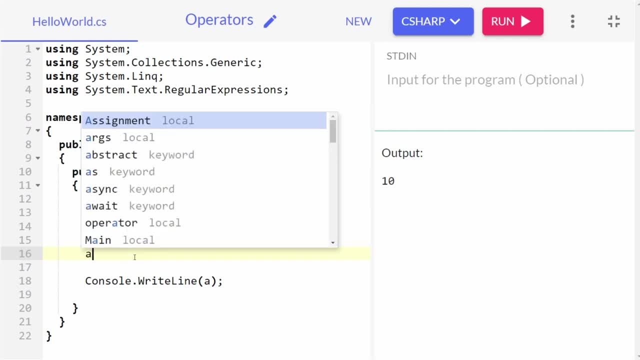 Now, if we look into the underlying- all right means the underlying logic- it will be like this: a equals a into 2, all right. And you know, 5 into 2 is 10.. And then it is assigning: 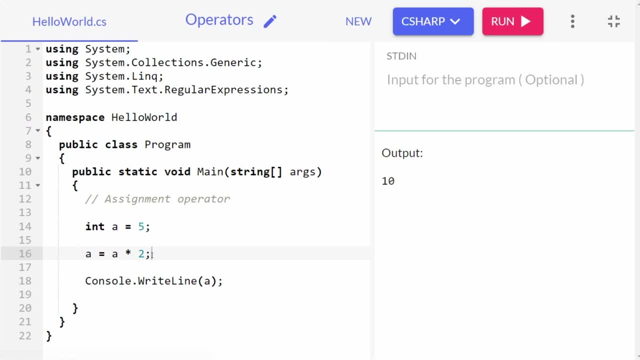 So that's the underlying logic behind it all. right Now, as we understood this. also, there's another one, that is: divide equals a divide equals 2.. So basically, it will divide 5 with 2.. Now, of course, I don't want to divide 5 with 2,. 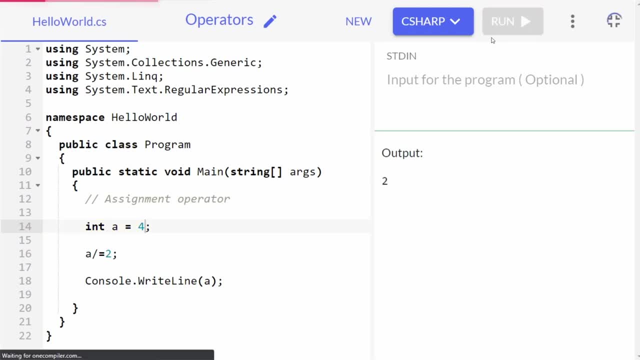 so I'm going to change the value to 4,. all right, Let's see for the simplicity here. you can see: 4 divided by 2 is 2, all right, Now let's you know, let's simplify it- a equals a divided by 2.. 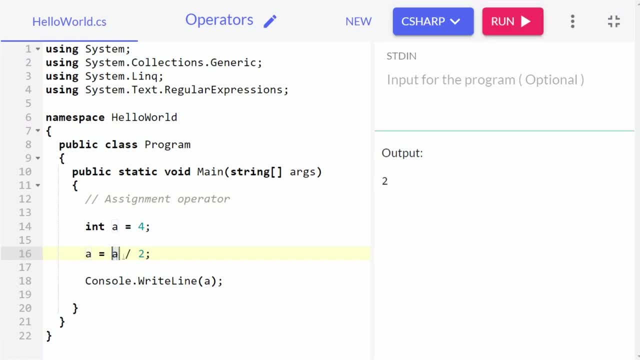 It's doing the same thing, right. First it is dividing, then it is assigning. as simple as that. all right, That's how this thing works. Now again, the last one remains, that is, modulo equals. let's see. 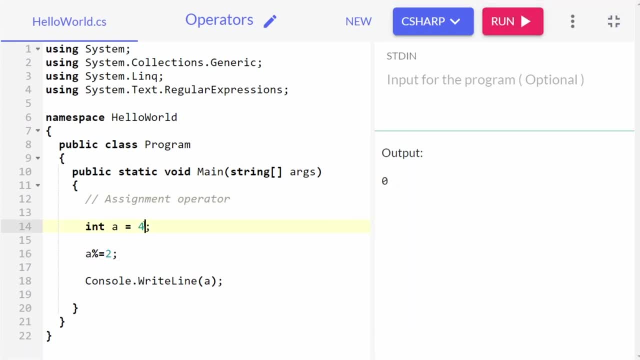 It is returning 0 because of course there are no. you know, it's a complete division if we divide 4 by 2, right, Now, let's try it out with 5.. Now, let's see, Is returning also 1 because it is not performing a complete division, right. 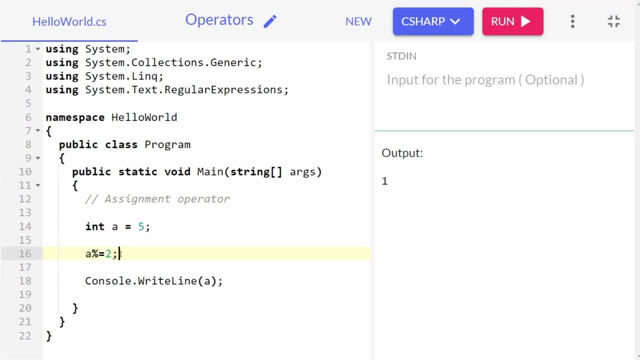 So that's how this, you know, this whole thing works all right. So let me show you the abbreviated version of it. also: a equals a modulo 2,. all right, Now, you know, let's remove this particular line and let's see if our you know. 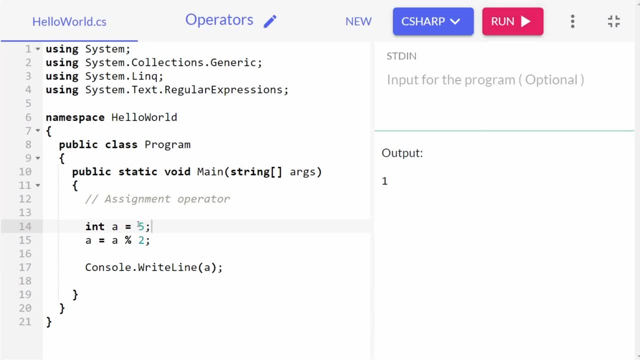 our idea works or not. See it is working right Now. let's change this value. Now let's see So. here you can clearly see all right, Here you can clearly see we are able to do all the actions, all right in the assignment operator. 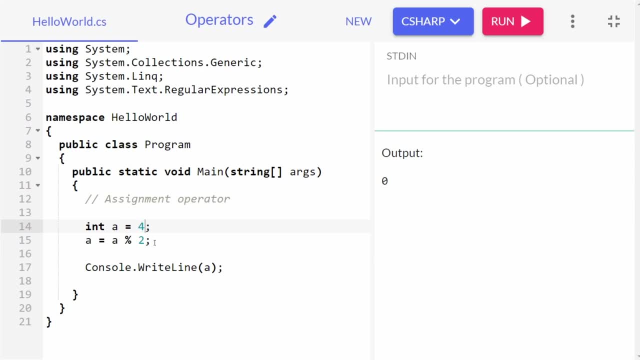 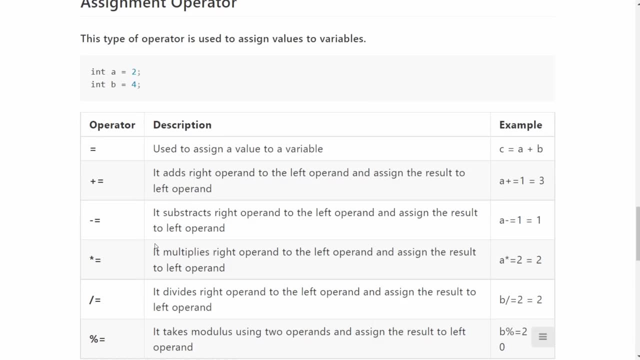 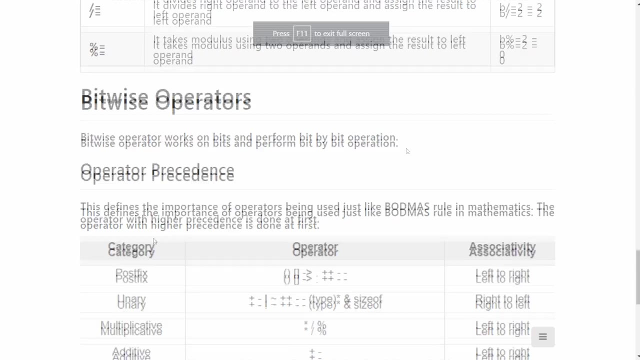 And I hope it is clear how everything under you know, under the hood, is working right. So let's get to our next topic, all right, And that is bitwise operators. I'm just going to tell you the over Like overall idea behind. 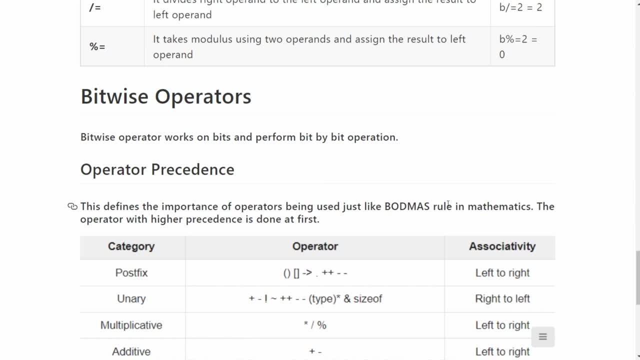 So you know, let's see See, bitwise operator works on bits and perform bit by bit operation. all right. Now in here, bit is binary, all right. So before see, the thing is you have to understand binary operations, all right. 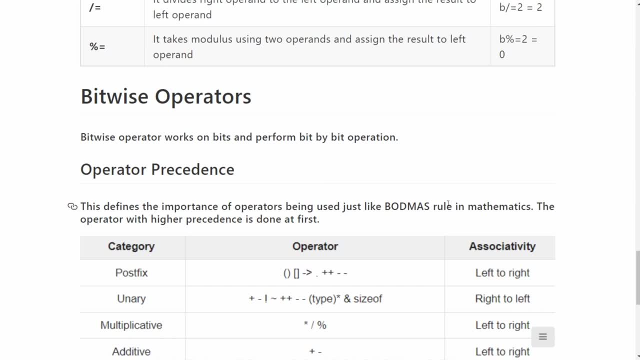 You have to understand binary hexadecimal octal operations before getting into bitwise operators. all right, Because bitwise operators works on binary And that's why bitwise operators are fast, all right. So remember that, Remember this thing, and I would like see, I would like you guys, all right, 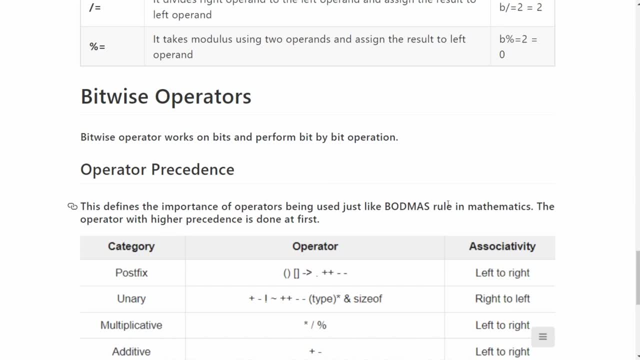 After you are completed with the C-sharp topic, I would really like you guys to do your research and learn about. all right, Do your research and learn about bitwise operators more, because it is one hell of an interesting topic. all right, All right. 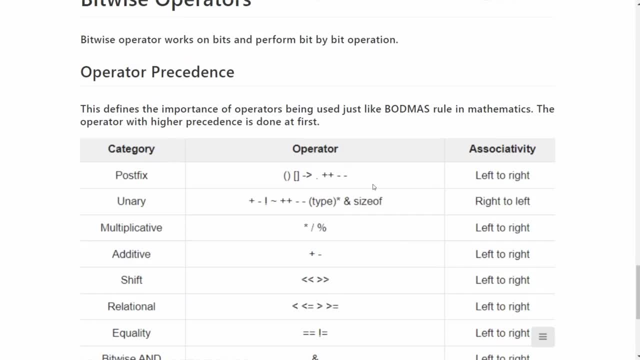 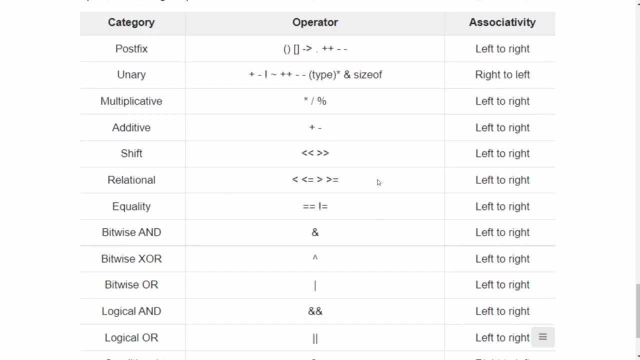 So do that. Now. here comes another topic: operator precedence. all right, See, operator precedence is, you know, a very interesting topic. It's like the Baudemars rule in maths. all right, It's like the Baudemars rule in maths. 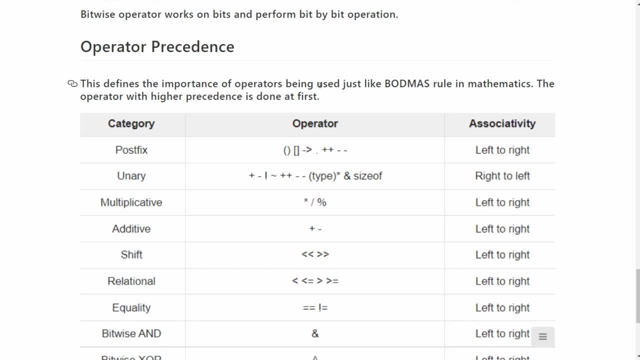 What Baudemars rule tells us? all right, First of all, it is in Baudemars rule, the associativity, or you know the importance, all right, The importance is from left to right. all right, The importance of operators, like in the Baudemars rule, the importance of all those operators start from left to right. all right, 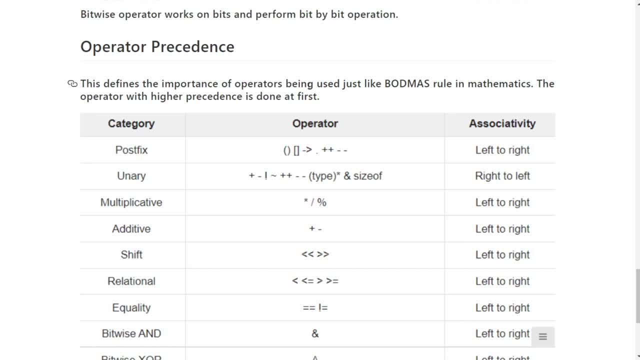 Bracket of, you know, division, subtraction, multiplication. sorry, bracket, you know, bracket of division, multiplication, addition, subtraction, right? So that's how it is, Means bracket has the very high importance And subtraction has very low importance. all right. 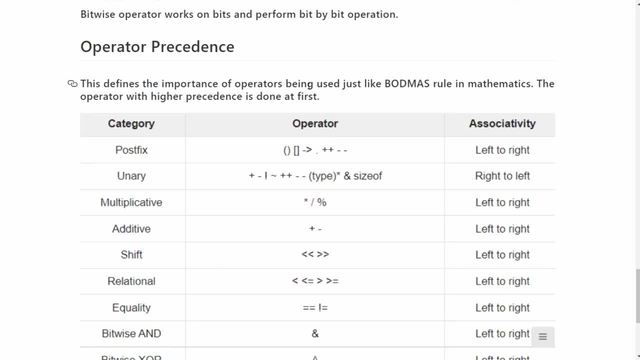 And you know, as bracket, all right, As bracket has very high importance: the, you know, the calculations inside a bracket is performed first, Then other calculations are performed. So these all right, You know these all right. 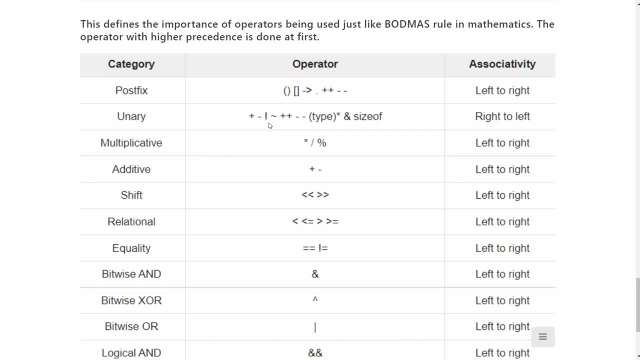 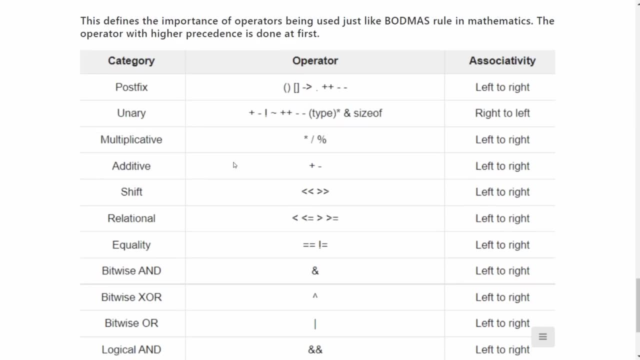 These. this is the whole concept of bracket Operator precedence. So I would like you to go through this chart. all right, It's very important to have understanding of this chart. It's just that it is telling us all right. 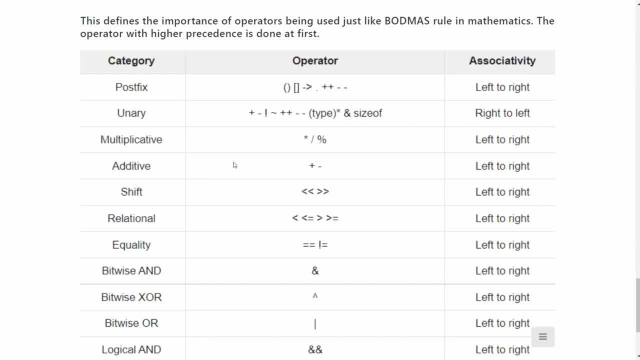 About the precedence of operator. all right, That is how important an operator is And how much important is it from its next operator. So it is telling us that, all right, And I want you guys to you know, have understanding of this, all right. 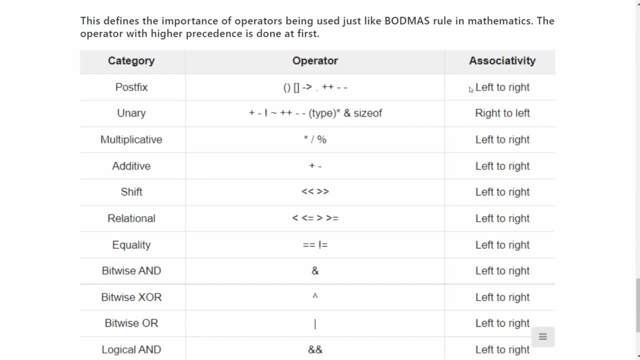 So that's it for Thank you, Thank you, Thank you, lecture, and i hope, uh, you guys are liking this whole series, so make sure to press the subscribe button and more lectures are coming. all right, thank you. in this lecture, we are going to learn. 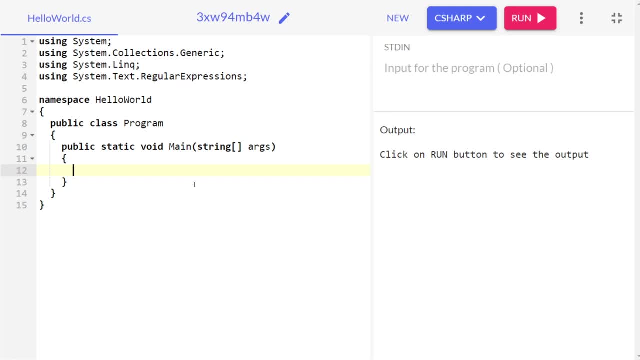 about conditional statements. all right, conditional statements in c: sharp uh. the reason why we are learning is we. we need to know how we, you know, uh- drive our program. all right means we, how we drive our program to a certain direction, all right. and how do we uh drive a program to a? 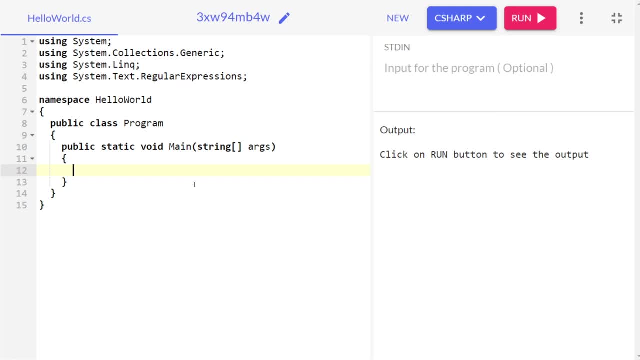 certain direction. it's by applying conditions. all right, it's uh, you know. it's just like that, like when you know: uh, i guess you guys remember when parents used us to know: uh tell us that we will buy you a thing if you bring 90 percent, uh, 90 percent marks in uh your exams. like it's. 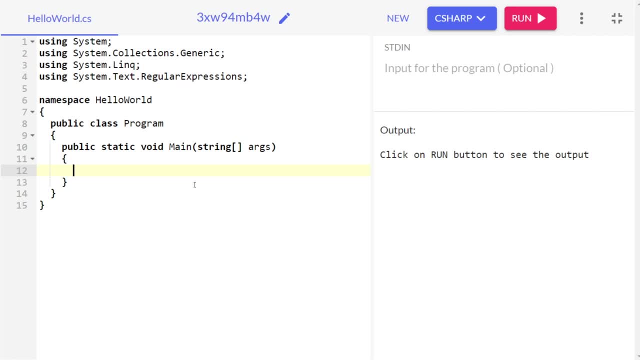 you study harder to get that thing. so that's how conditional works. all right, we give some condition, all right, and uh, it works upon that condition. that's what conditional are. all right, basically conditional uh statements. now they help us to execute. all right, it helps us to execute. 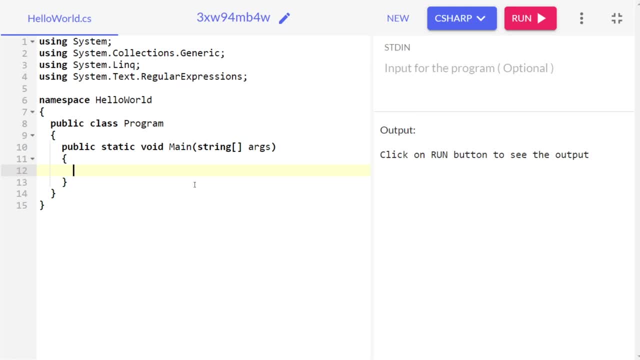 some sort of programs? all right, some programs. uh, with respect to the conditions assigned to it, all right now. if the condition is true, all right. if the condition is true, then you know, uh, a condition will get executed, and if the condition is false, it won't get executed. all right, so. 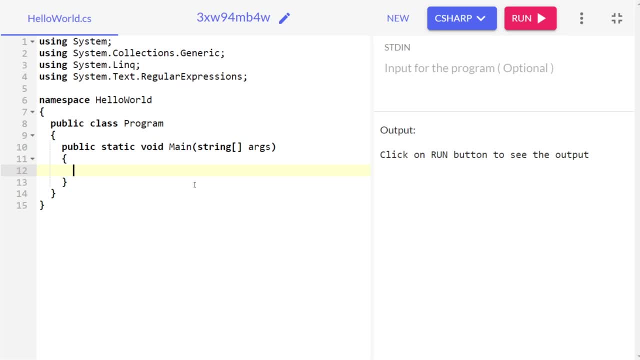 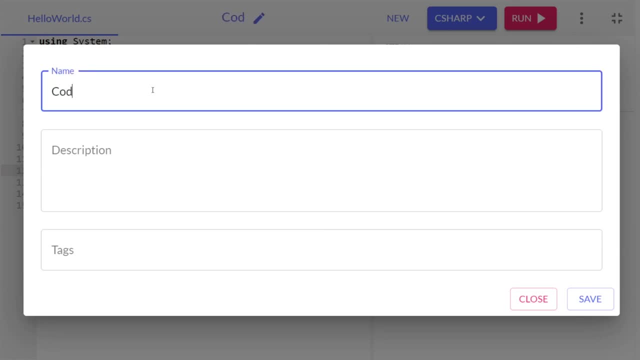 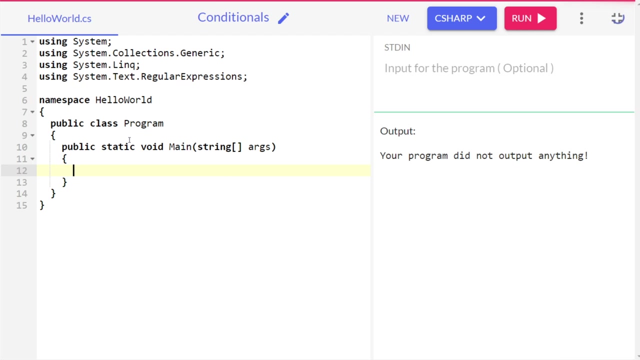 that's what conditional is, all right. so now, uh, first of all, uh, just let me rename this editor to you know, uh, conditionals, um conditionals, all right. so, yeah, see, there are, uh, you know there are three, or you can say four uh conditional statements out there. now let me. 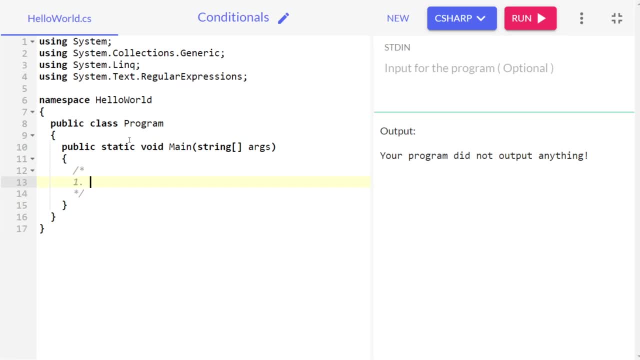 write them down, all right. the very first one is if else, all right, or you can say if and else. the next one is if else, if and else, all right. the third one is in line. if we are going to learn about that, don't worry, uh. and the fourth one is switch statements- all right, or you can. 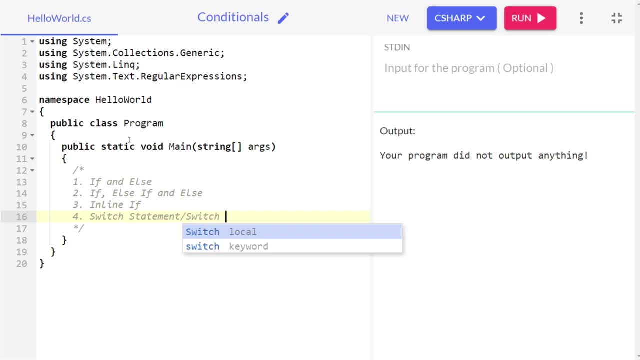 say, uh switch, uh case, all right statements. so, uh there, these are the four types of conditionals we have, all right. so now, as we are clear with the like what conditionals are right, we should, you know, get going with our very first. you know, our very first statement, that is, if and else. 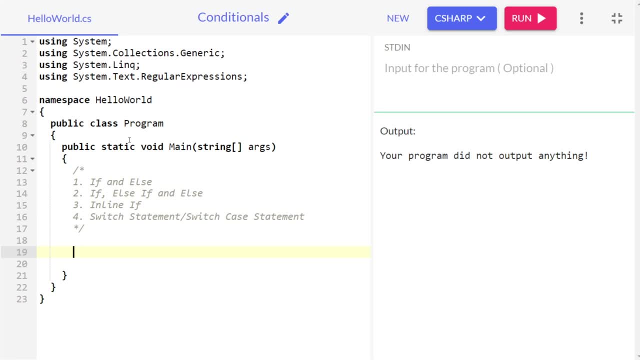 statements. all right, see if and all statements. now, it helps us, you know. it helps us to execute some condition already to use. it helps us to uh execute some statement under some condition. all right, it's like that, it's. it's like you know. uh, let's say for an example: um, it's raining outside, all right for an example. 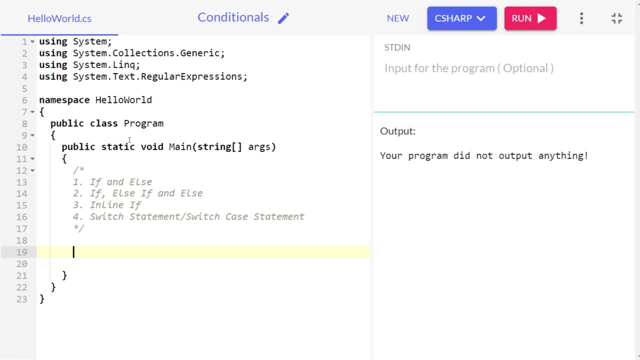 uh, it's raining outside. or uh, let's say, uh, how can i, you know, represent it? um, yeah, let's say it is, it is raining outside, all right, and you, you want to take an umbrella. why you want to take an? uh, see, the very first thing you are. 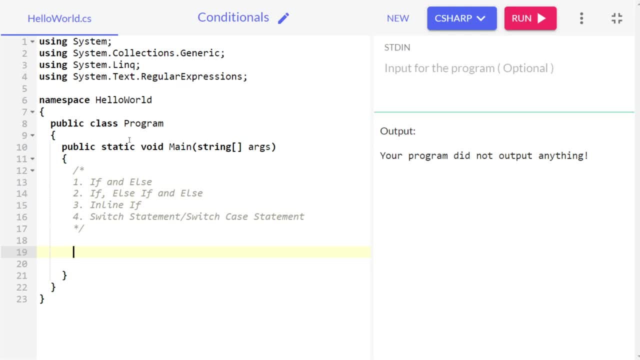 going out, all right, you see, while going out, you see that their rain is falling right and you are very sure, as it is raining, you want to take a condition. sorry, you want to take an umbrella with right because, uh, it is raining and if you, you know, uh, get wet in, uh, due to the rain, uh, it will. 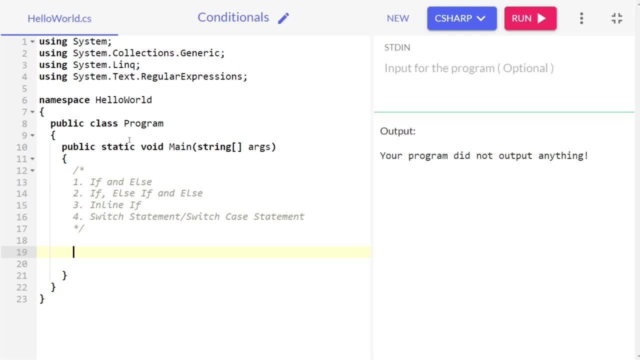 you know, uh, it will give you fever, all right, you won't be well, all right, so you want to prevent it. all right, and because of that you are getting an umbrella so that you don't get wet, right. so in here, can you all right. can you guess what is the condition in here? all right in this case. 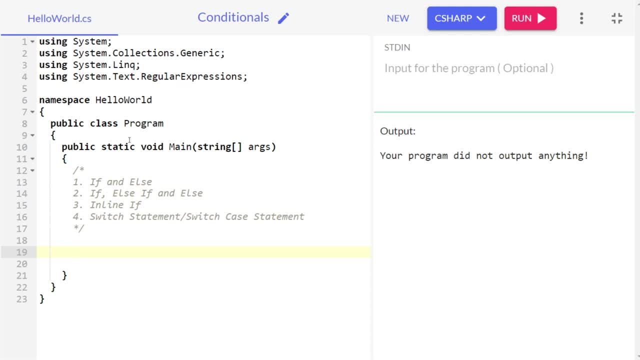 the condition is rain, all right, how? let me tell you see, as it is raining, you are taking the umbrella. what if it didn't rain? you won't be taking and taking an umbrella. all right, because of course, dude, it is not raining. why would we need an umbrella? we can walk freely, right. so the 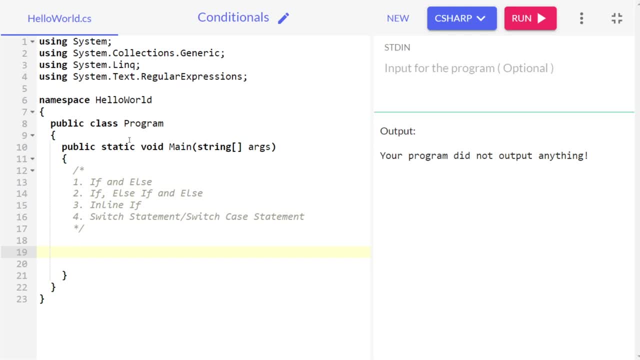 condition in here is rain, and the statements that are being executed is: will uh, is that the person will take uh umbrella or he will not take the umbrella? all right, so that's how it is working. now to uh, you know, to implement. all right, let me show or tell you about the syntax, how we, you know, represent. 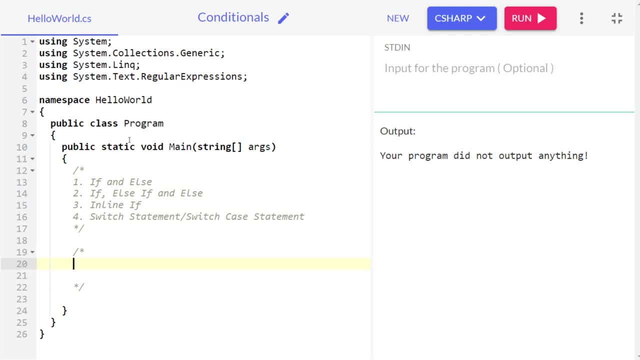 the syntax of if and else, i would uh like i would implement the example i told you. all right, i will do that right now. just give give me a few seconds. first, let me make you, uh, you know, go through with the condition. the first thing is, uh, we have to give a, you know, first thing is we have to write. 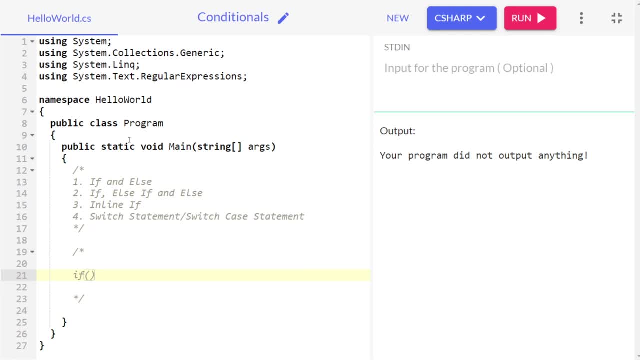 if all right, and within that, if a condition goes all right, a condition will go on and after that, all right. within the f block, some sort of you know uh statement will be there. statement in the set, some sort of program you have written or some sort of you know uh. 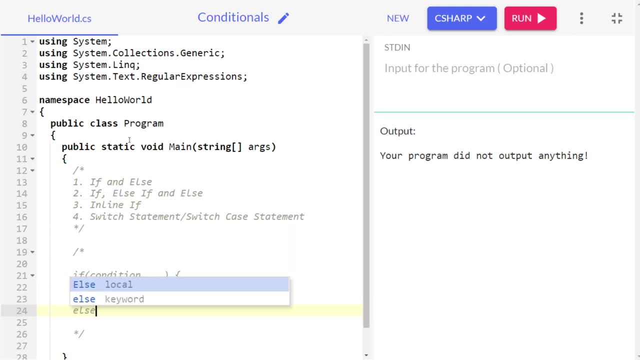 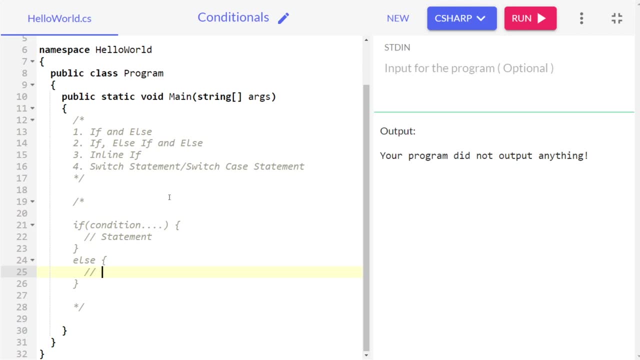 command you have written, that would go on all right. and let's say: if the condition, all right, if the condition is, you know, if the condition is not satisfying or the condition is wrong, then another set of all right, uh, another set of statement will work on right. 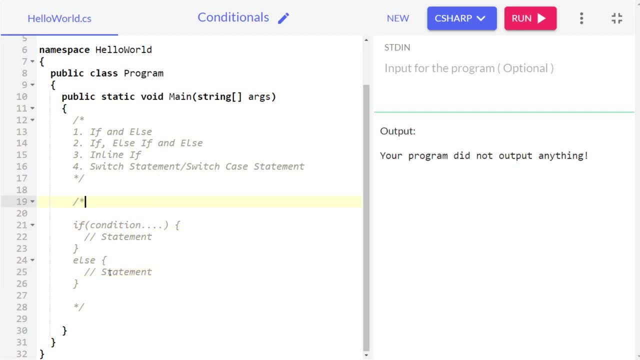 so if the condition is not true, then means, uh, if this particular kind uh statement condition is not true, then this uh else block will execute. now, to understand it very you know uh very carefully, let's code it. first of all, create a bool variable that is is raining and, you know, set it to false as. 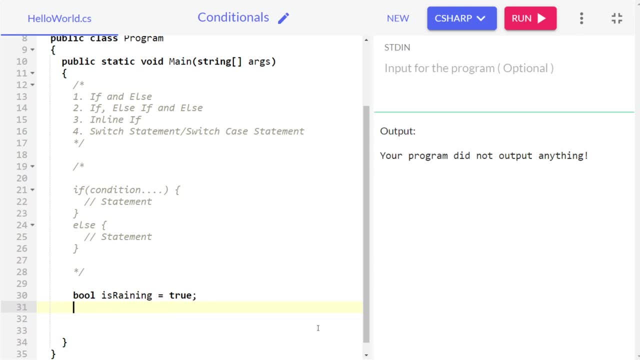 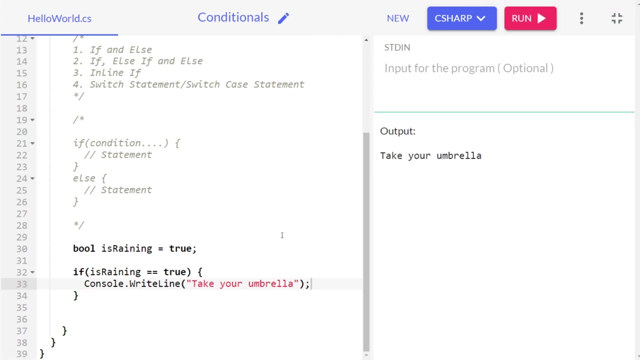 of now. or let's say, set it to you know, true, all right, that would be better. now, if is raining equals, uh, true, what i want to do is i want to print. i want to uh print that. take your umbrella right, let's see if it is working or not. yeah, it is working as it is raining, all right, as it is rainy. 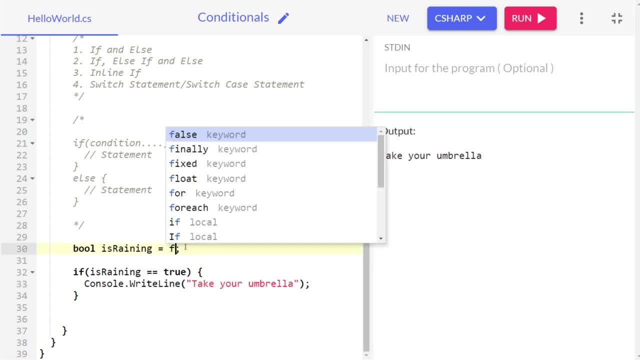 that's why we are taking our umbrella. let's say: what will, uh, what will be the outcome if we, you know uh, say false, see, it is telling us that progr-, your program did, did not output anything. what does it mean? it means that this, if condition? uh, like you know, here our condition is only that. 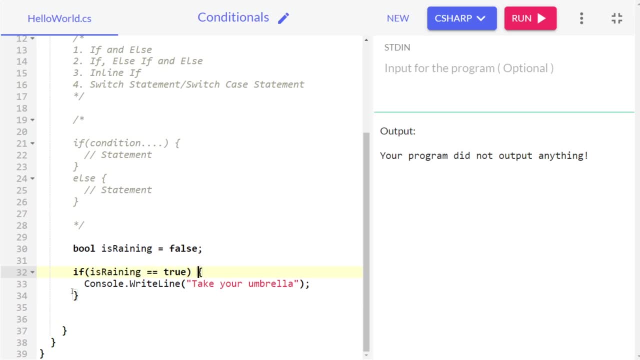 if it is raining, all right. if is raining equals true, then only execute this particular block of code, all right. or else means we haven't specified. let's if, if this is raining, training equals equals to condition, doesn't execute, all right. let's say: if it returns. 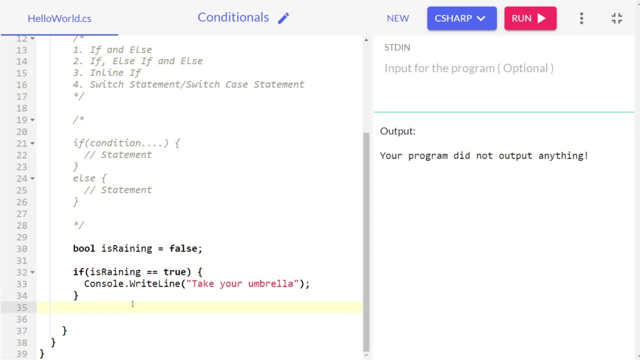 false, then what? all right. then another block of code, will you know, show its. you know what can I say? show its magic. that is else block, all right. what else block does is, if any of the condition becomes false, all right. if any of the you know previous condition becomes, 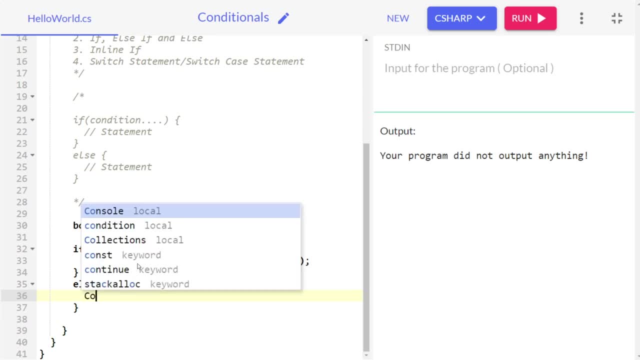 false, it will go to the else block, all right. and in the else block we can write: okay, just all right. in the else block we can write: don't take your umbrella right. so now let's see as is. as it is not raining, that is is. raining equals false. so what is happening? our code. 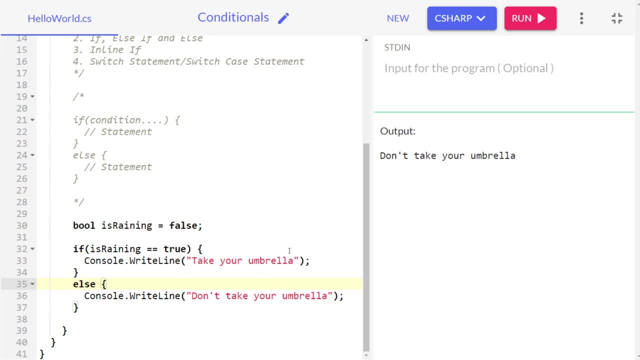 is telling: don't take your umbrella, all right. So that's how. So if an else statement works, it helps us to drive a program to certain directions, all right. so it's like that. it's just like the example I give you, like the raining example. 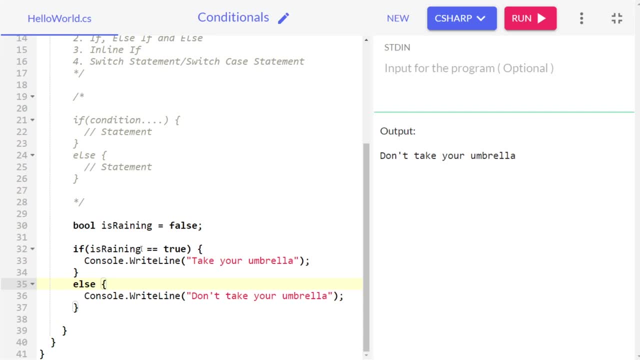 and you know the parents are like. you know the parents are giving us some, you know some sort of gift, like promising us to give some gift and they are telling they will only give the gift if we bring 90% marks in our exam. So it's something. 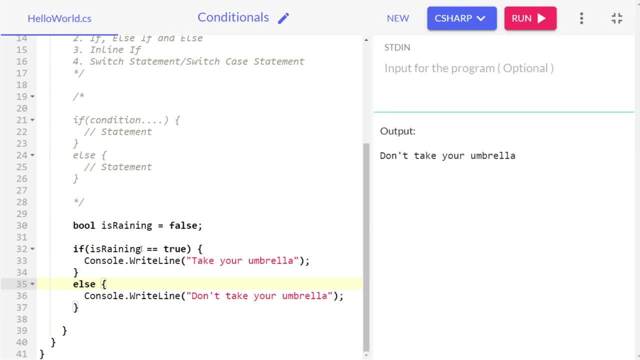 It is totally like that. all right, it's, it's how we drive our code. all right, it's how we actually, you know, drive our code. that's how this whole thing works. all right, so that is what it is now our next. all right, as this one is done, right, this one, let's mark it done. 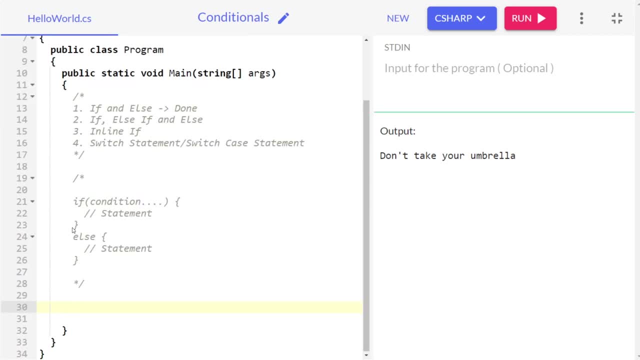 if and else is done. we are clear with if and else statement Now. Now. So the next one, all right. the next one for us is if else, if and else statement. right Now, see, it is also similar. all right, it is also similar to if and else statement, just. 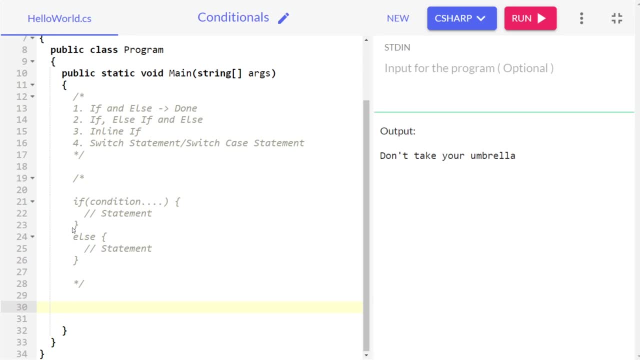 here comes another block, that is else, if, else. if is also, like you know, if statement, but let's say If and else. if statement doesn't execute, it will go to the else if statement, and if else, if statement also doesn't execute, then it will go to the else statement. all right, 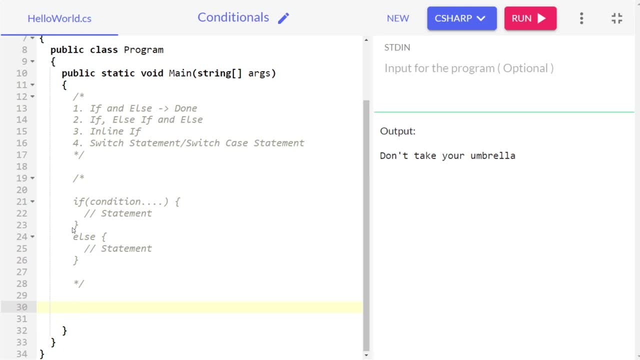 These kind of statements comes in real like, comes really handy when, whenever we are writing, let's say, solving some problem, or let's say making our own AR application in where we have to put some conditions right, So this kind of statement comes really handy, all right, and they are used more oftenly, all. 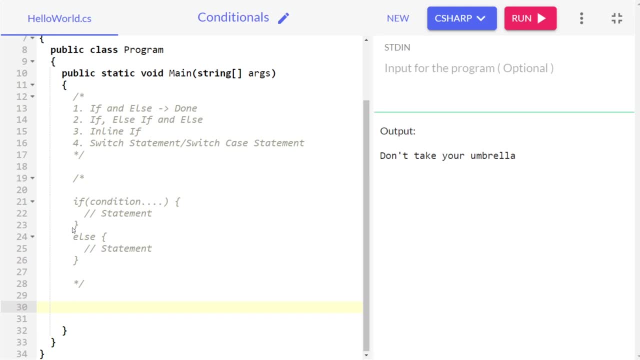 right. They are used oftenly, so make sure understand it. all right. the syntax is, you know, very similar to the previous one. you like, just in between if and else block, all right, you have to write another block, all right. that is else if and in here a condition goes on, all right, and. 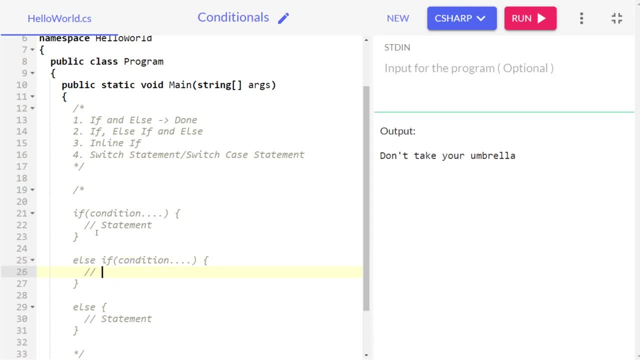 within that condition, we have to write, and you know, block, and it would contain a statement: all right. So it's like that. now let's. let's say, let's take an example of voter voting age: all right, let's implement it. let's take age, let's. currently, my age is 17. all right, as of now, my age is. 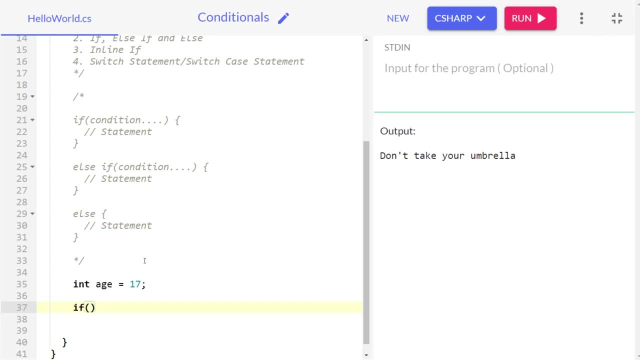 17.. Now for the very first condition I'm going to give is all right. the very first condition I'm going to give is: if- sorry, if age no is greater than equals age 18, then only, all, right, then, only I am eligible to vote in India. right, then, only I am eligible. 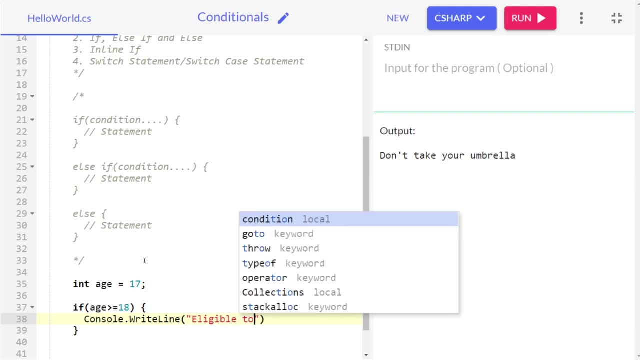 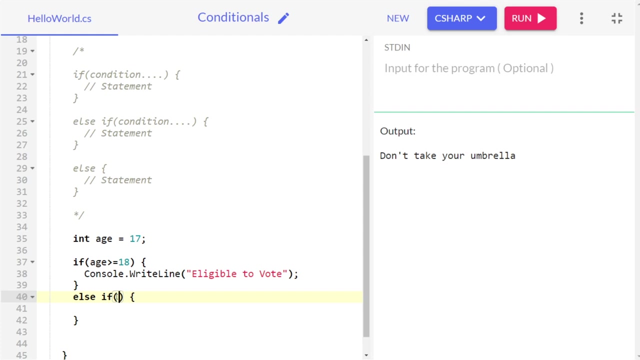 to vote. Let's say: what if? all right. else, if our age is less than 18, all right. let's give another condition: all right, If our age is less than 18, and all right. And age greater than let, greater than zero, of course, a child, all right. who? who are like? 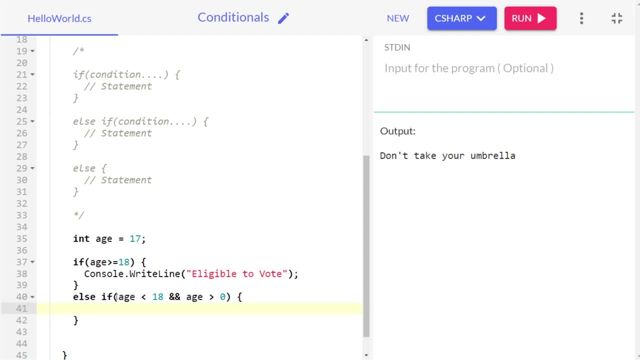 who's not even born, he won't be able to- you know, vote, of course that's. you know that's ridiculous right. so console dot right line and give not eligible to vote, all right, so yeah, And in the else block we give console dot right line, give invalid age- all right, invalid. 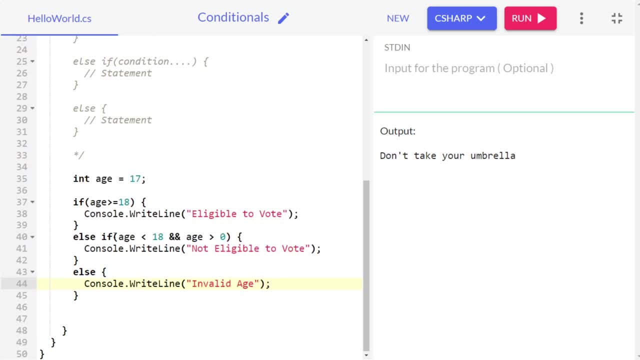 age. now, what does this means? all right, let's first give it to you know, let's give the age 19. all right, let's see which one will get executed. See, the first condition is being executed. That means the if block is being executed. why? because, of course, of course, the age, the 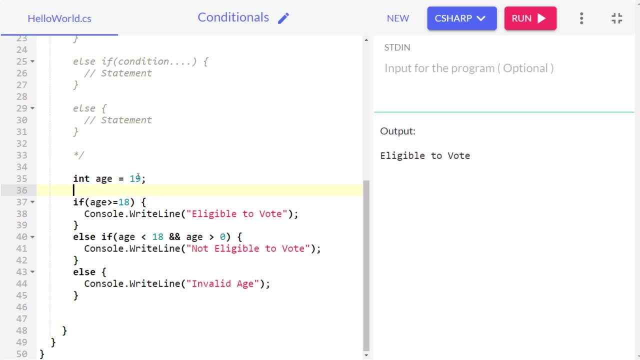 age we specified is greater than all right. greater than equals 18, it is greater than 18 right. that's why we're eligible to vote. now, let's let's try out 17 right. we are not eligible to vote, of course, because we see I am not 18. in India, the minimum voting age 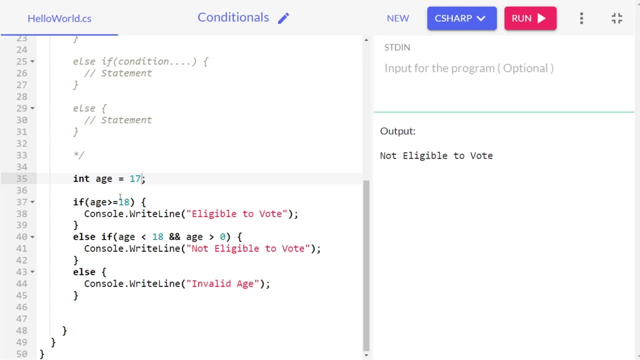 is 18.. I am not 18, so how I, how will I vote if I am not 18.. So 17 is like, if you are 17, you can't vote right now. let's try out. you know 4? let's let's. 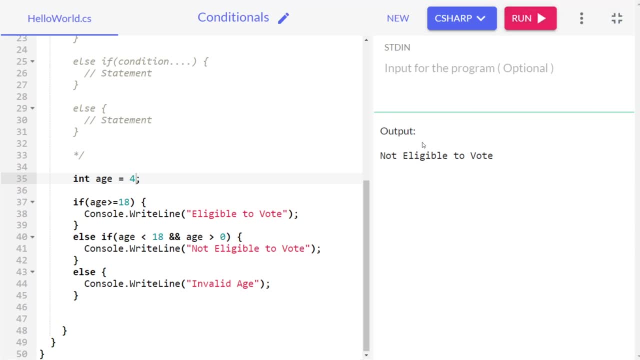 see if a 4 year old can vote or not. no, the 4 year old cannot, can't vote. now let's see if a zero, all right. if a zero year old kid can vote or not. Invalid age- All right. A zero is not an age, right. so here is the thing: if else, if and else. that's how we use. 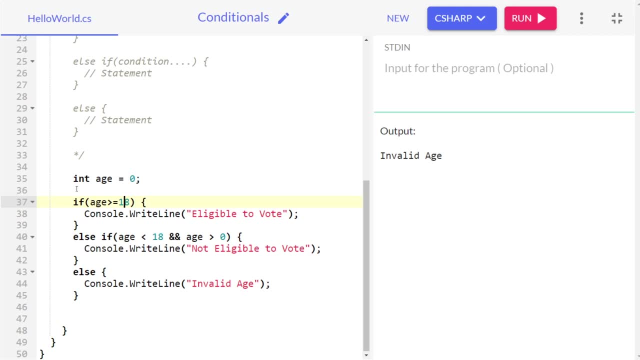 it. all right, that's how we use it and you, you, you are going to use more oftenly when you will start coding your own AR, AR applications or games- right, or even like when you will you do go in competitive programming or solve problems- you are going to use these statements. 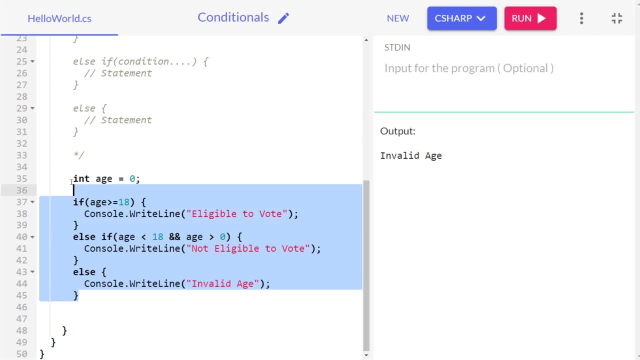 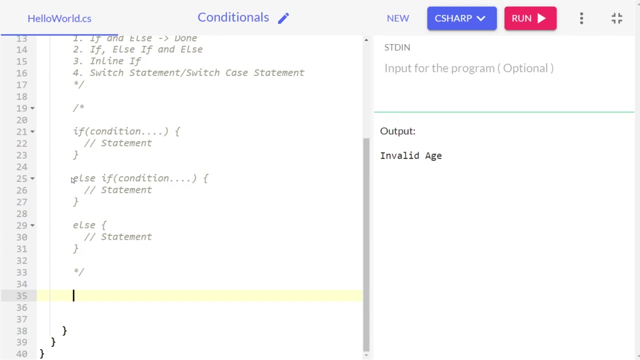 oftenly. All right. So you know we use these statements. all right. so I hope you know the concept, the concept of you know. this is clear. now we are going to, you know, do a bit of problem solving in here, all right. So for us there is a question, all right, for us there is a question, let me write it down. 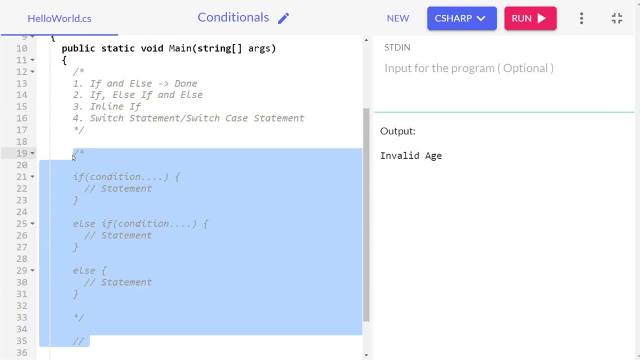 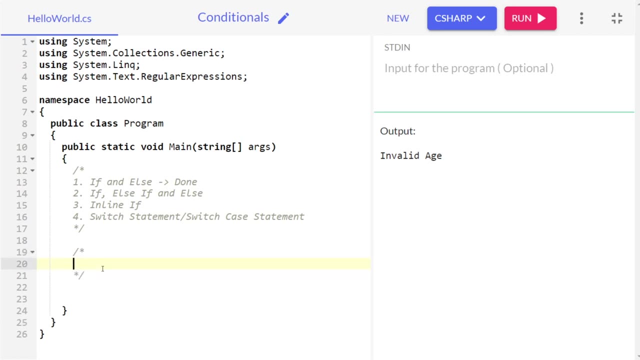 here. first of all, let me remove all this, you know, this statement. now. let me, you know, write this question in here. All right, All right, write a program to take certain numbers and if the numbers are, if the number is divisible, just wait. if the number is divisible by two, then we have to print divisible by two. 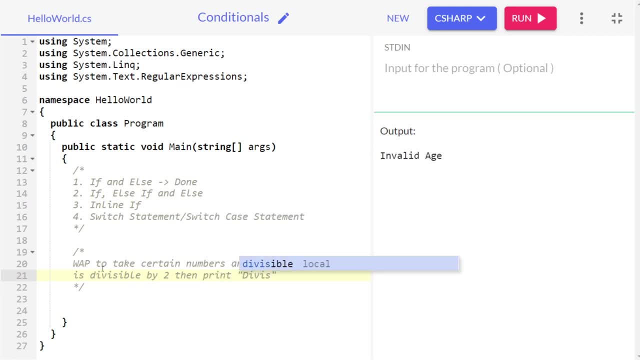 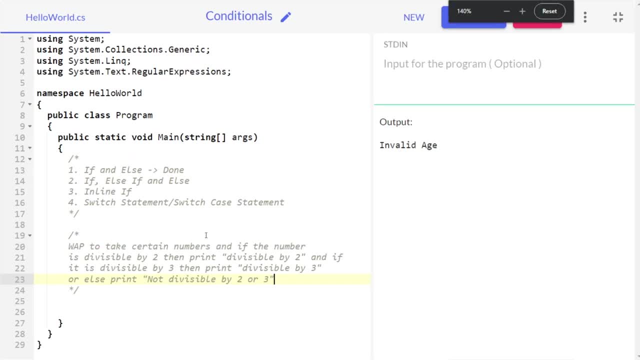 three, alright. so this is a very simple program. alright, you learned about operators. alright, now you know how to perform. you know how to perform remainder operation. right now, let's understand the logic. first, alright, to check. all right, if the program is fully divisible, alright, see, understand this. if a program to know if a number is fully divided, we have to make sure that the remainder is zero. if the remainder is zero, then only alright, then only we say that that particular division is, you know, is valid. alright means it is fully divided. that's when we call like, for example, four divided by two. in this case, 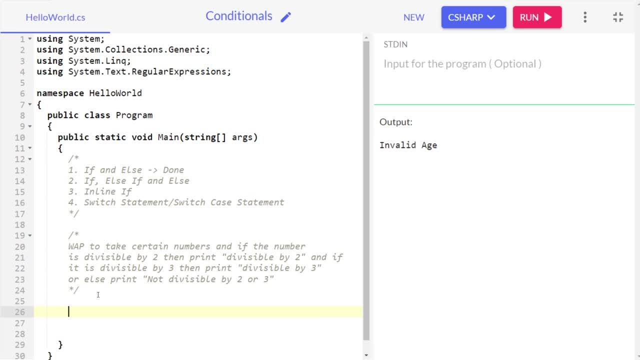 the remainder, alright, in this case the remainder is zero, right. but let's say again, let's take an example: five, let's divide five, divided by two. in this case, there will be one as a remainder and we can't call it divisible by five, so divisible by two, right? so make sure that. keep this in mind, alright, keep this in. 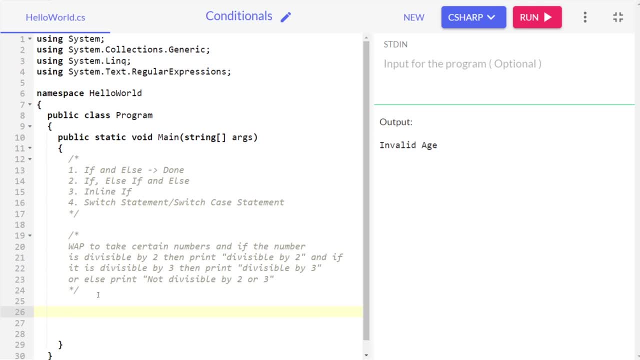 mind any pro, any number that is. you know that whose remainder is coming zero of, like it's coming zero after the division. it is divided that first by a specific number. alright, so make sure you know that now you already know which, which one is the division operator: this one already, this amp or this percentage? 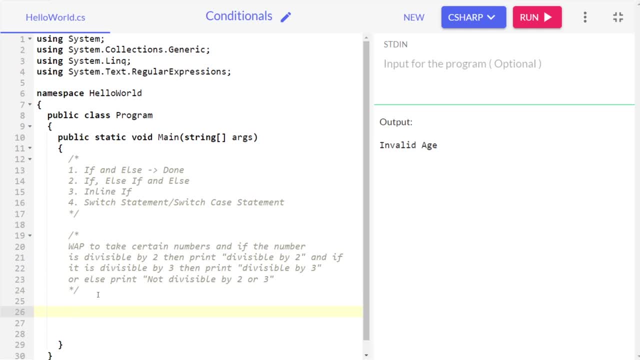 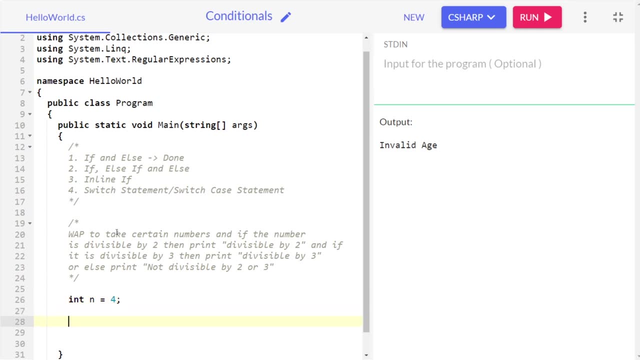 operator, or you can some module operator, alright, and to perform the division. it's very simple. let me show you. first of all, you take a value that is int n. let's, as of now, let's give you know, let's give it four now, if n per. 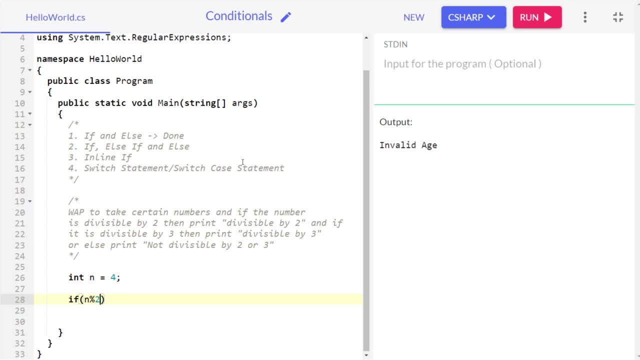 percentage two, alright, that is. we are how this working. we are taking out the remainder- alright, remainder- by dividing n with two. we are trying to take out the remainder, then we are checking, alright, then we are checking if the resultant alright remainder is equals, equals, zero or not. if it is zero, then we are going. 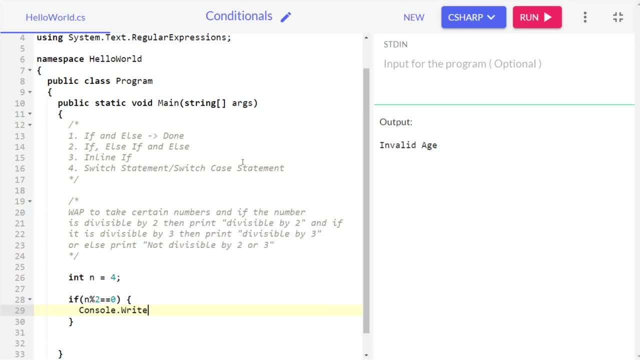 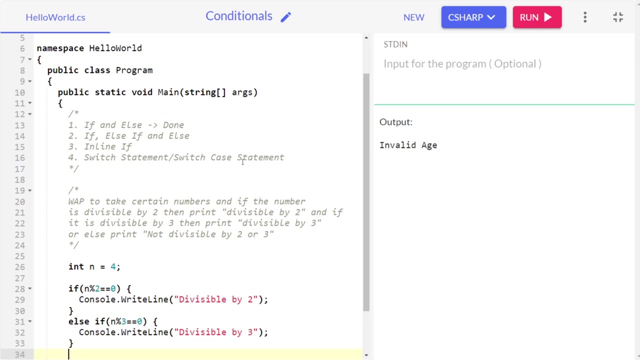 to, you know, print console dot, right line, right line. divisible by to, similarly, similarly, we are going to do the same thing with three, that is, in, divided in module of three equals equals zero. if that works, that then it is divisible, divisible by, you know, three by three o'clock. now, if, if 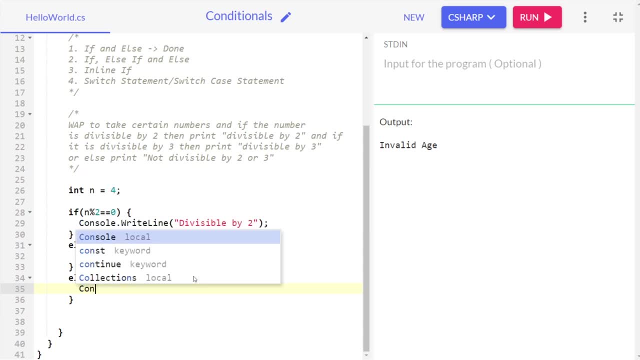 none of the condition works already. none of the condition will. then I want to to print out, not divisible by no, by both 2 and 3. all right, so now let's check this out. all right, let's check this out and how these things works. see, as 4 is divided, as the remainder, all right. 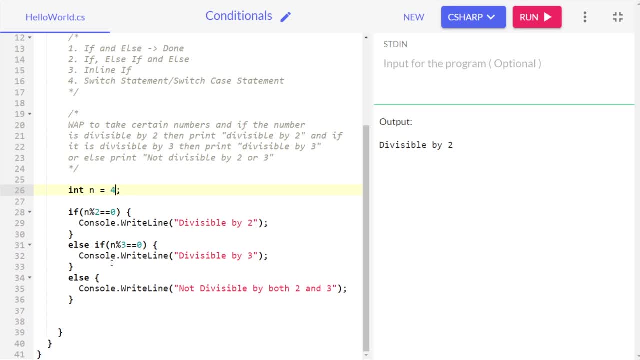 as the remainder of 4 divided by 2 is 0 and it is matching the condition. that's why it is returning divisible by 2. now let's try. try out 9. all right, it is returning as divisible by 3. the reason is: 9 is divisible by 3. when we divide 9 by 3, the remainder comes 0 and as the remainder remainder. 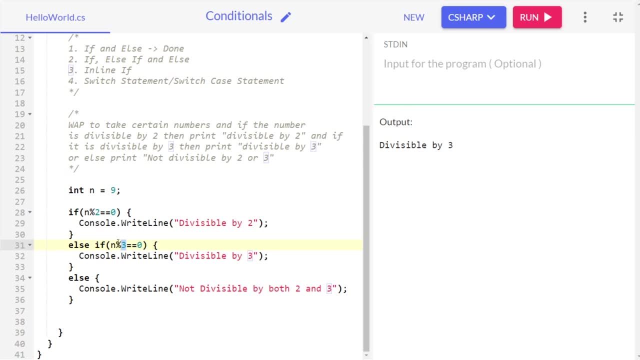 of the resultant division is 0 and it is equals equals 0. that's why it is returning divisible by 3. all right, it's as simple as that. now you know. now let's, let's give 1. it is not divisible by 2, not divisible by 3, all right. so that's why in the else block it is returning. 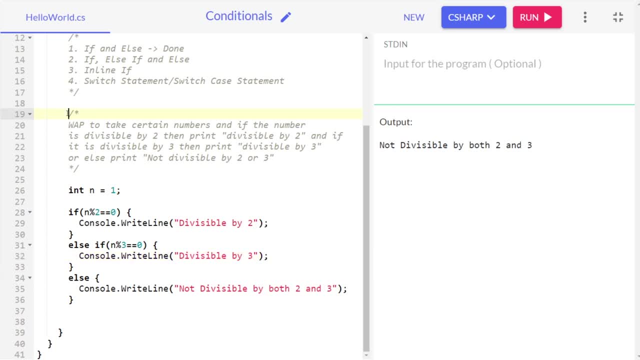 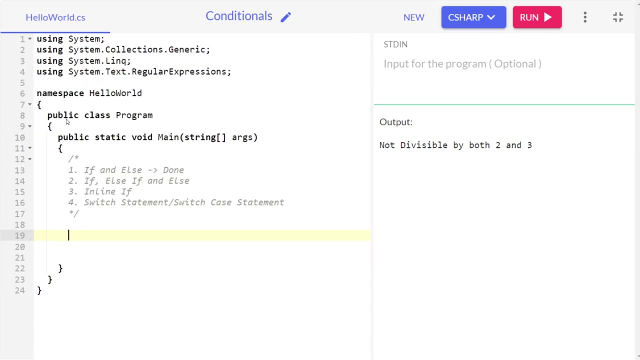 us not divisible by both 2 and 3. so i hope you understand how we exactly use if and else. you know, if else, if and else statements, all right, and i hope it is you know clear. so yeah, let's you know we can conclude. all right, we can conclude that if else, if and else statement is also done. 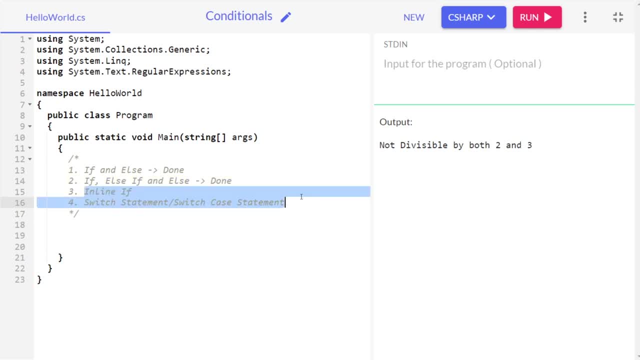 all right. now here comes two other statements. all right, very important. all right means actually: uh see, you are going to use inline if, if you want to assign, you know it doesn't have extra conditions in there. like only one single condition means only one actually. let's, let's you. 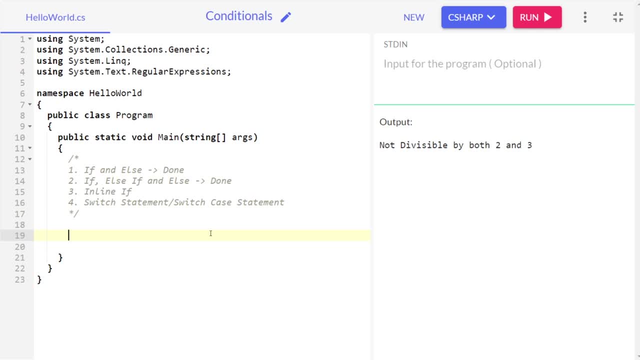 know, write the program first. all right, let's understand the program first, then you will understand what i'm trying to say. all right, so you can. uh, you saw the. you know the syntax of if else statement it's a bit big. right, it's a bit big. 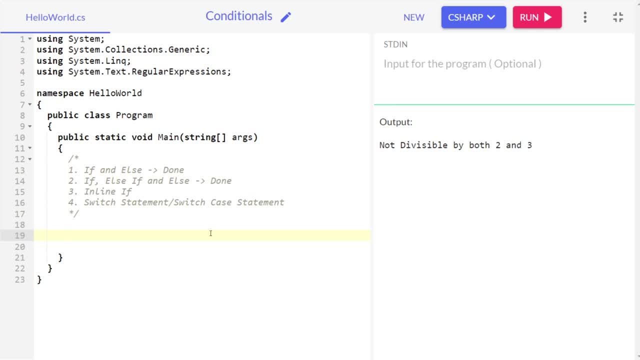 now inline. if now is, uh is basically now inline. if it basically the shorter version of if and else, all right, it's the shorter version, uh, of if and else and it is, you know, mostly used. uh, you know it is mostly used, or you can say it is more convenient to use when you assign, assign some. 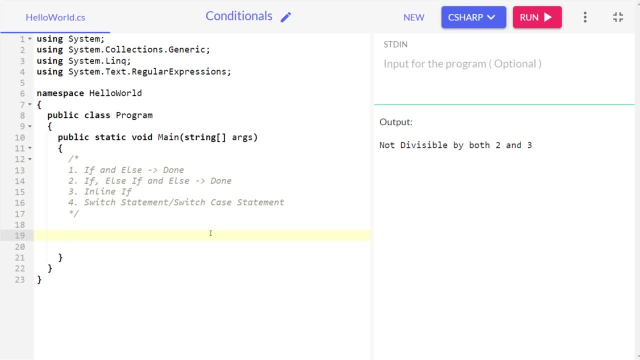 to a variable depending on you know some condition. all right, it's, so, you, it's more convenient to use in there, all right, rather than using it any. uh for taking any input or something like that. all right, so it's uh. it's uh, it's very convenient to use those statements while, uh, you. 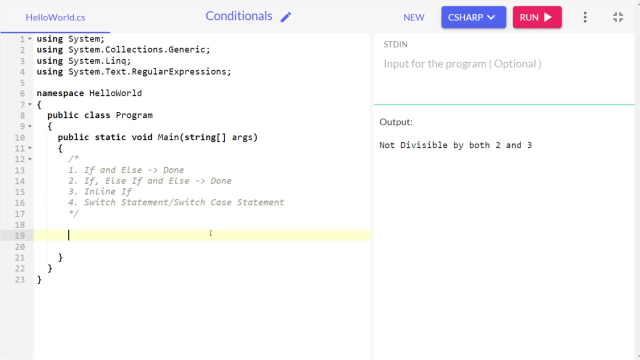 know being in the variable. so make sure you keep this in mind. right now, if i, if i talk about the syntax, the syntax is, you know, pretty simpler. all right, first of all, here's the condition. all right, after that there's a question mark. all right, then here's a value. 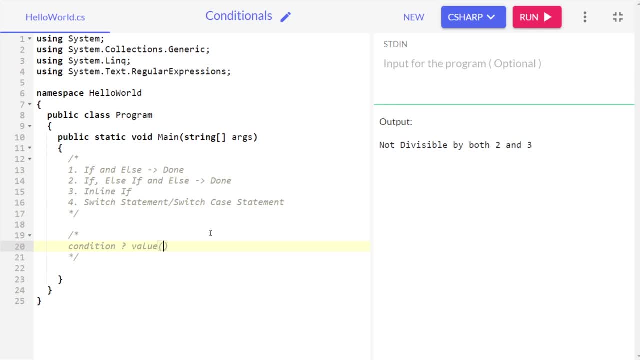 all right, and it will be assigned all right only if the condition is true. and then here comes a colon: all right, and this value will be assigned if the condition is false. it's just like if and else statement: right, let's say: you know, let's try it out, let's try it out, let's create a string. 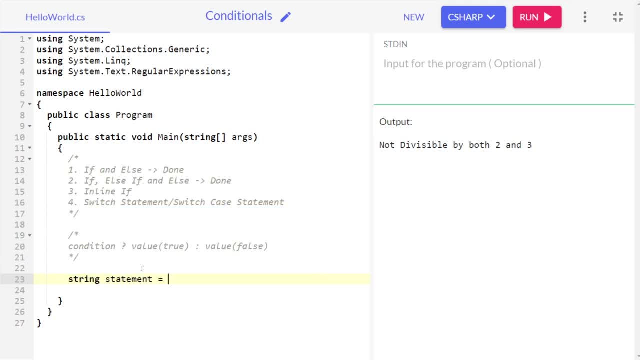 variable. all right, let's say string statement and let's give give a condition, that is 4 greater than 2. all right, now let's give the question mark and let's write 4 is greater than 2. all right, else else what we can do is 2 is greater. 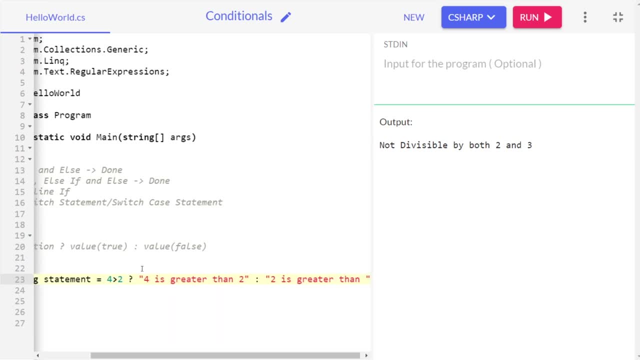 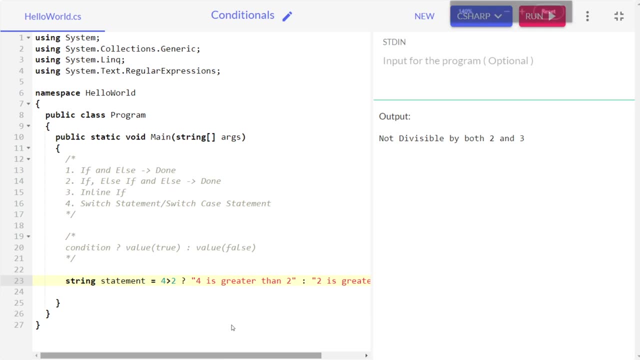 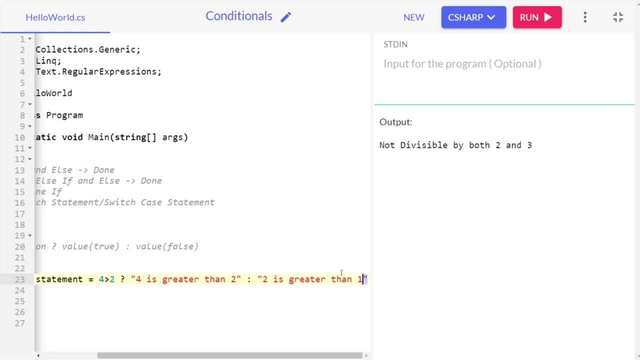 than uh let's say 1 or uh, just uh, give me a second, just give me a second, let's, you know, let's uh change this whole statement. all right, change it will uh actually confuse you a lot. let's change this whole statement. uh, let's say: if 4 is greater than 2, then uh, you can say: 4 is assigned, all right else. 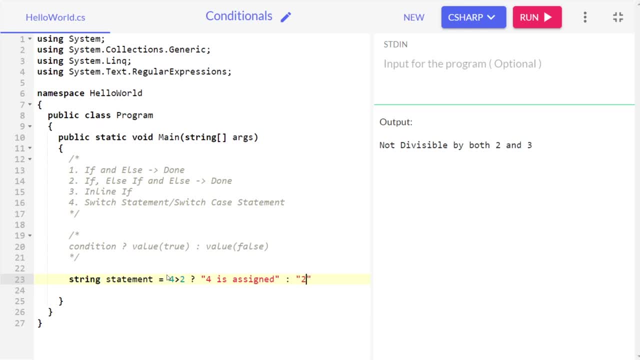 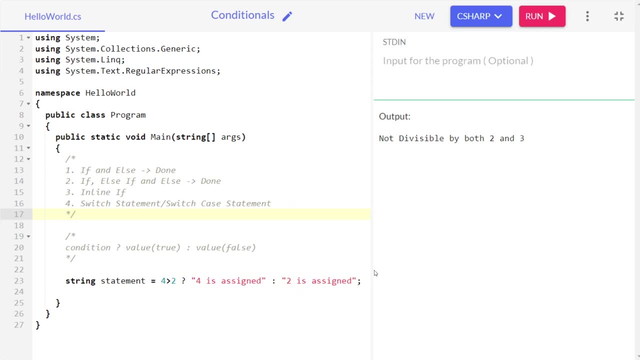 you can write: 2 is assigned. all right, let's make this simpler. so here you can see that what i'm i'm trying to say right now. also, let's print the statement to see if everything is working right or not. all right, now let's try it out. 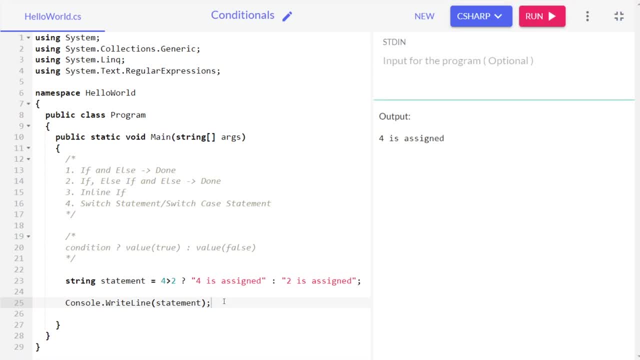 see, it is telling us 4 is assigned because this condition is true. and if this condition is true, then only the first one, first one statement, will be assigned. all right, so let's try it out: if the condition is false, then the second one will be assigned. let's change this sign. 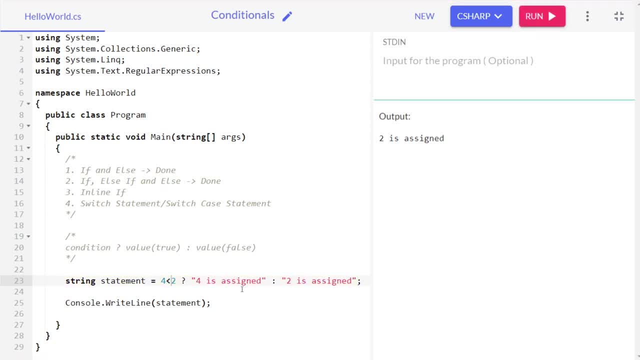 a greater than sign to you know less than sign. let's see, see, as this condition is false. that's why it didn't assign the first statement. it uh, rather uh. than assigning the first statement, it assigned the second statement. so that's how it works. all right, so it's just like if and else. 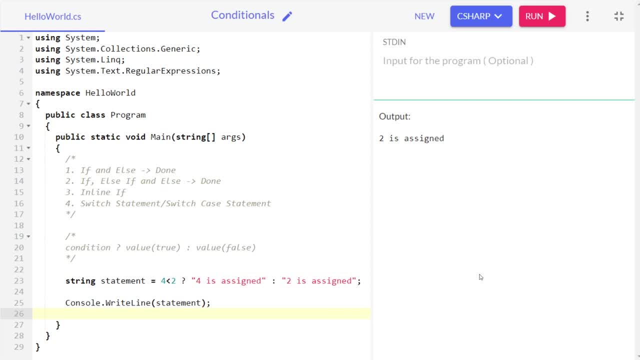 statement. all right, just in, you know, uh- abbreviated form, so i hope you are clear- with in line f: all right, this, uh, this statement is very simpler to understand. now let's mark it as done. and uh, here comes our last one, that is, switch case statements. all right, see, switch case. now it's, like you know, pressing some. 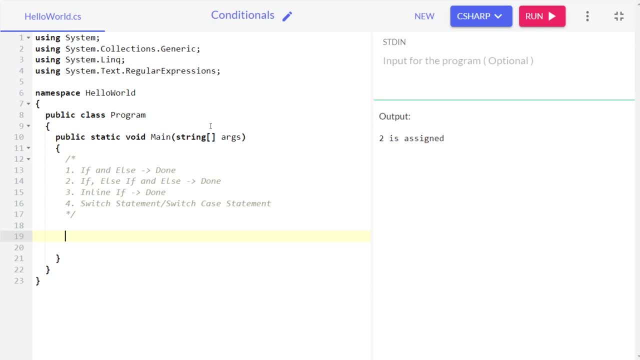 switch. if you press a switch, a certain perform will, um, a certain you know, certain function will performed will be performed. and if you press another switch, um, another set of functions will be performed. right, it's something like that. all right, now you can uh say: all right, see, let me, you know, make it simpler for you, the uh, i can say: 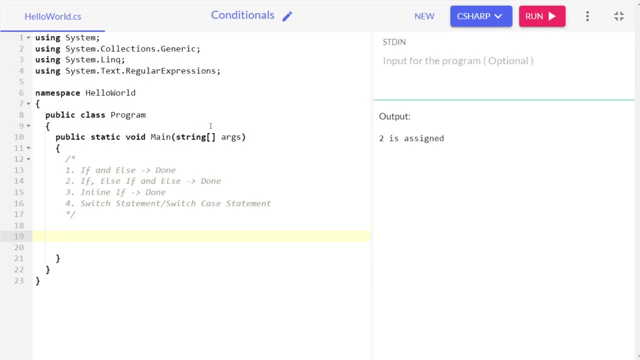 that, you know. the switch statement is, uh, you know, very similar to an if statement. all right, just that. all right, just that it does not, you know, work with a range of value. all right, it's simple as that. it. it's just that it doesn't needs any, uh, range of value doesn't work with that, all right. 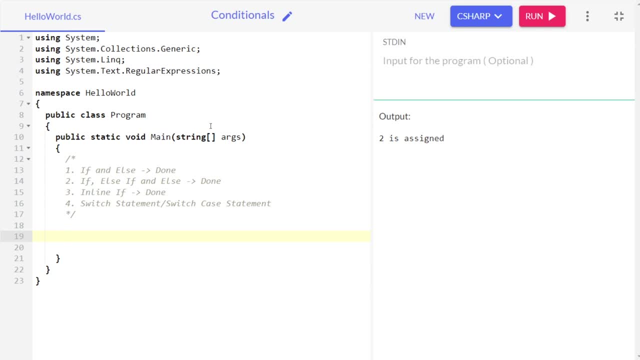 it's, it's uh, a switch case statement. now, it requires, you know um a case, all right, it requires a case, all right, which, uh, which you know is based on a single value. all right, it will be based on a single value and uh, depending on the value of the variable. all right, it will be, it will switch you. 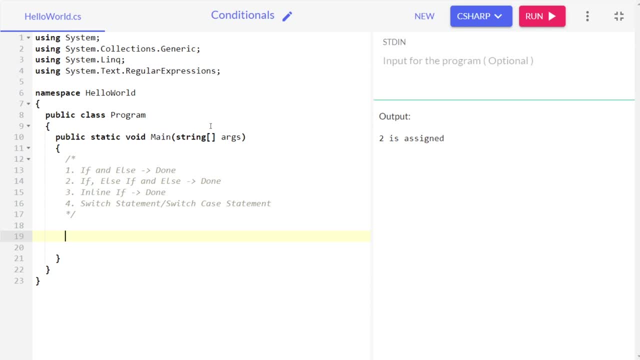 know, uh, it will turn, it will switch to some statement. all right, and the program will execute the correct block. all right, i know it. this definition, you know this. this wordings might get a bit confusing. all right, i totally understand. all right, even if i was uh in in your place, i would also have got. 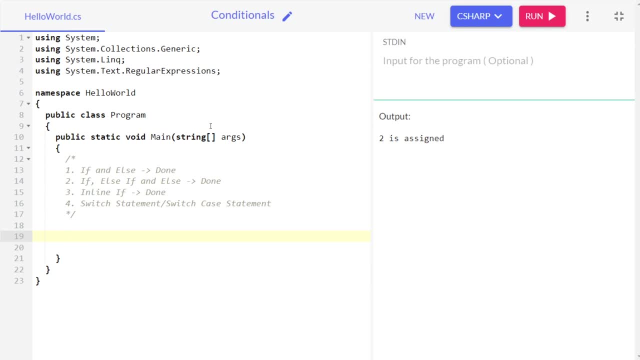 you know, confused. now, to remove our confusion. all right, to remove our confusion, let's code it. all right, let's code it first of all. let's understand the syntax. all right, it's very important for us to understand the syntax. all right, see the very first thing. all right, that. 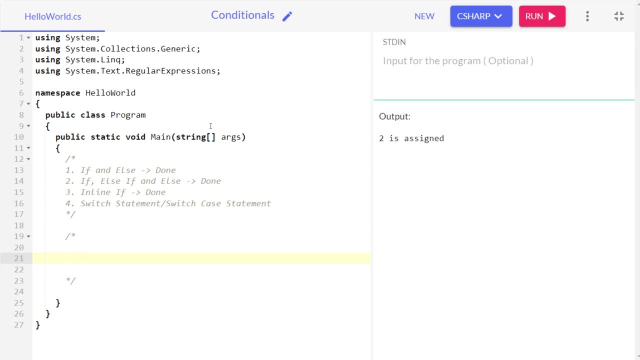 comes to us. the very first thing that comes to us is: which one can you guess? switch? all right, in inside that switch, you know, inside that uh switch, uh statement: we pass a variable, all right. we pass a variable that would work as our choice, all right. and then we 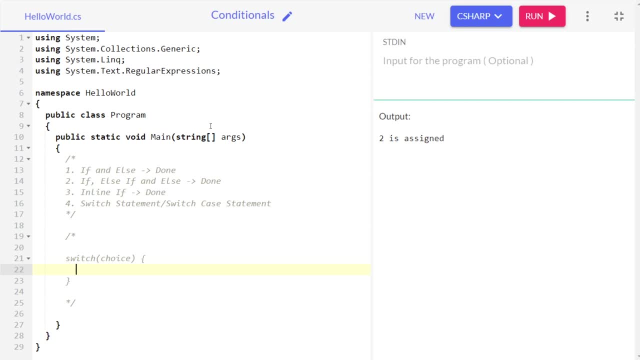 start, you know two curly brackets, brackets, and then we write a statement: is no case, uh, wait, case, all right. and in that we pass some value and we give a colon, all right, and we say that, bro, do something, all right, do something. and now see, this choice, now this choice will work as this value. now, if this choice, all right, if the value of this 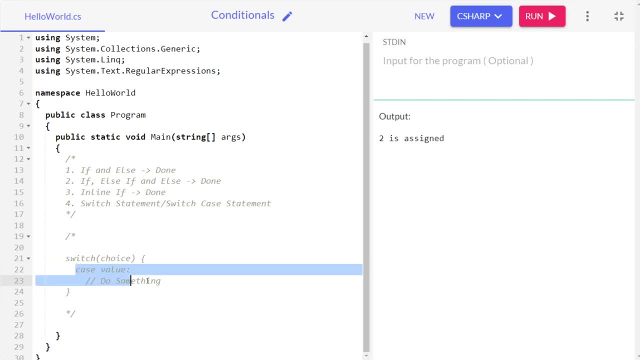 choice is similar to this value, then this switch case statement will work all right. and then we, you know, uh, give another statement, that is a break statement, all right, i would tell you what that, uh, what is that? all right, and what happens if we don't put that in there? now, here comes another case, all. 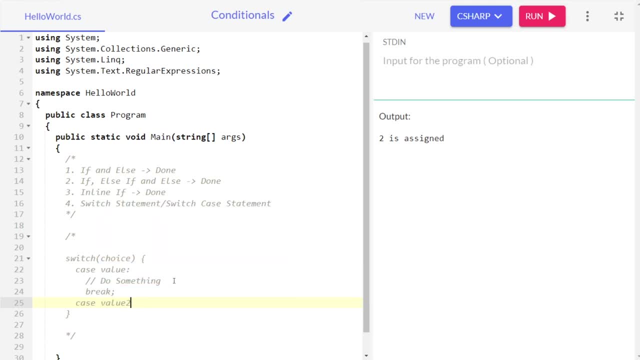 right. that is, let's give another value to all right and let's again say: bro, do something, all right, do something now. again break now. after that, here comes default statement: all right, default is basically this: default statement will occur if all right. this default statement will occur if none of the 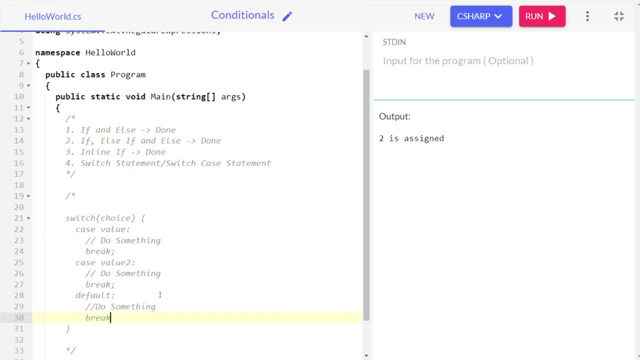 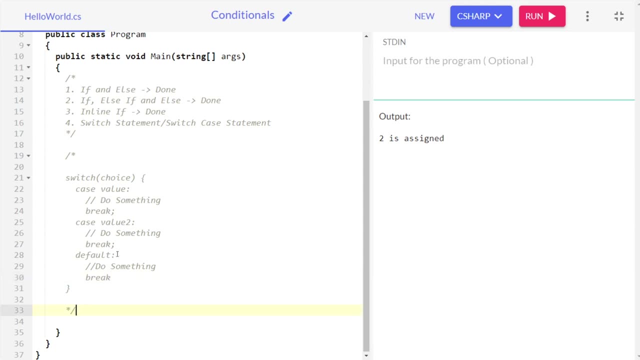 you know, none of the value works all right means none of the case works all right. so this is the basic syntax, right? this is the basic syntax of switch case. now there's no need, you know, there's no need to get confused. all right, there's no need to. uh. 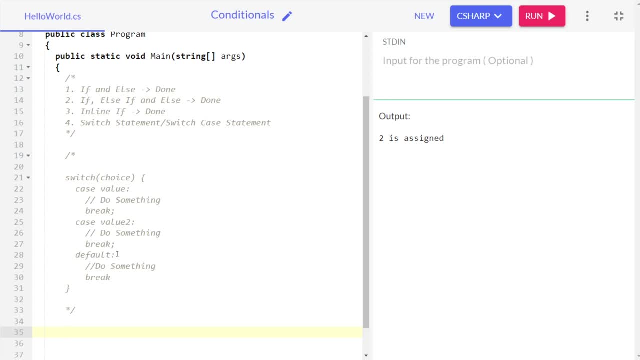 be confused. let's you know, let's create a, a simple, very simple grading system, right, like, uh, let me make you understand the logic in here, basically what it will do now. it will tell us: all right, we have to tell that, uh, which grade we got? all right, and then, based on that grade, it will tell: 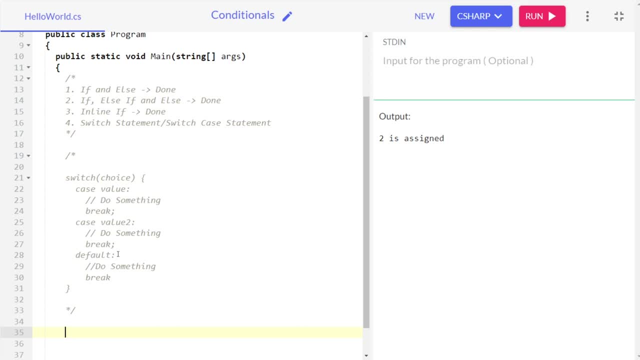 us that the grade is good or not all right. if it is good, if it is bad, it will tell us that all right. so that is what we are going to do now. so let's see what we are going to do now. so let's see what we are going to do now. so the first thing, i want you to create a variable. all right, that is. 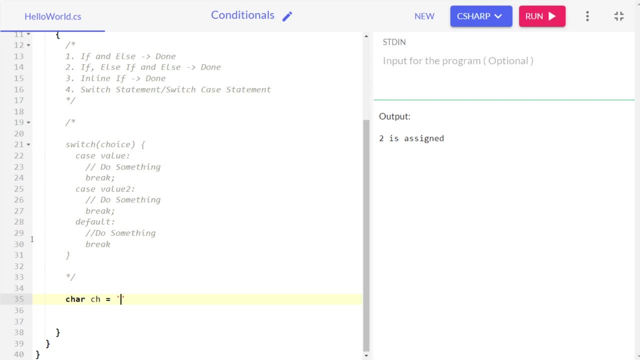 char ch and assign it like, let's say, for now let's assign it some, you know, value eight. right now here what you have to do is write the switch statement in here, pass the ch variable. it will be work as our choice variable. that i told you about, right, and in here, write case, all right. 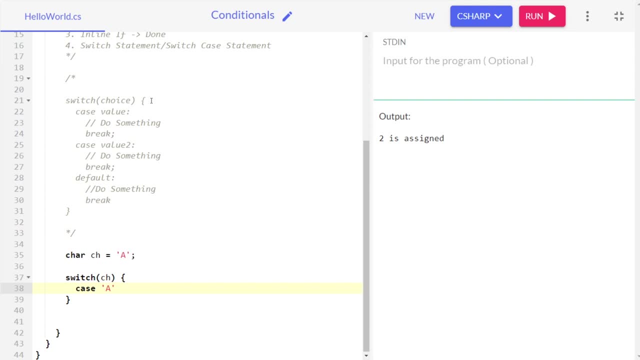 and in that case give a single- uh, you know single- colons and write all right. then, if you want, you can indent it. then you know, console dot right line. what i have to do, as the grade is a, i'm going to say very good, right, very good, because you know the grade is. 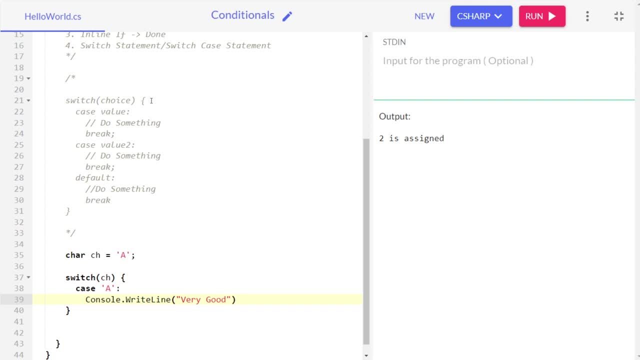 really impressive, right. so now, after that, after that, let's give another case that has case b. now again write console dot right line. we'll just go into right. good, all right, b is also grade b is also no bad, all right. so, as we have defined two grades, all right, you can, you, can you. 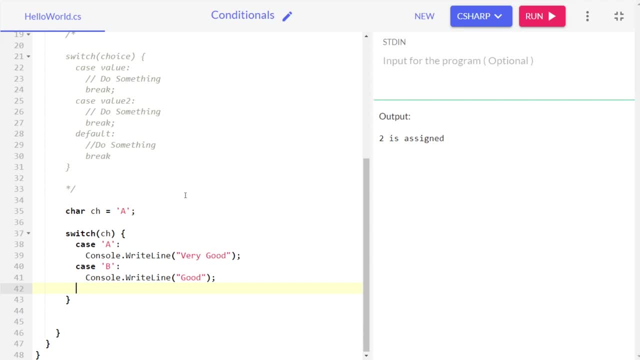 know, give more such grades in there, all right, you can add c grade, you can add d grade, all right. you can add e grade. you can add f grade, all right. but for now, for this example, uh, this, this one is enough, you all right. so see, now let's give default, all right. one thing: you would notice that i haven't, uh, you? 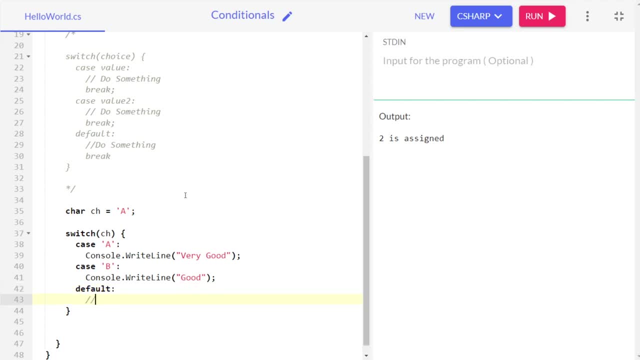 know, uh, gave the you know break statement. all right, i would show you why i'm actually wait. let me write the break statement first because, uh, what will happen? it will be more easier to make you understand how, how this break statement is working. let's give the break to every you know. 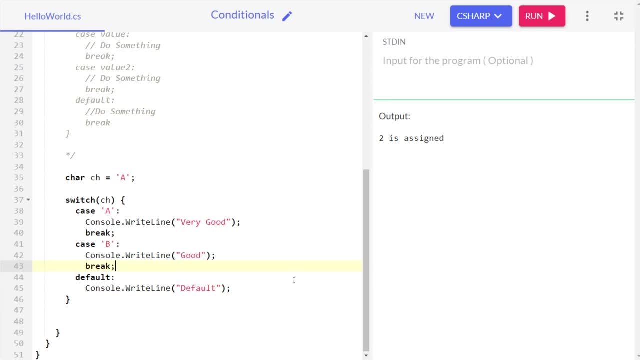 every particular step. or you can say case: all right, now let's uh try and run it. see as uh the, you know, as uh grade is a. it is returning us: very good, now try with b. it is telling us: good, now let's try with c. it is telling us: default big. why default? because, uh, we haven't defined it. we haven't defined it. 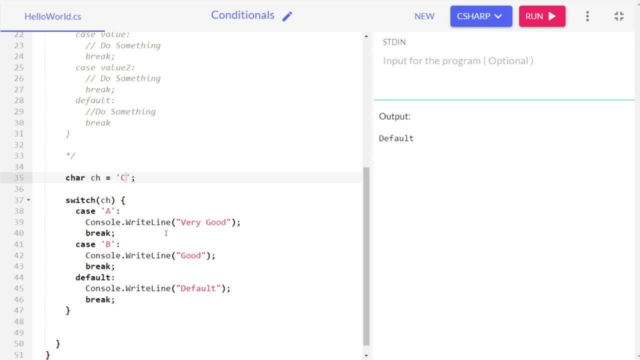 all right, case c: we haven't defined case c. that's why it is going to the default block. all right. it's also, you know, very similar to if and else statement. there's just a, you know, bit of difference. now let's try and remove this, break statements from there. all right, let me show you what is it. 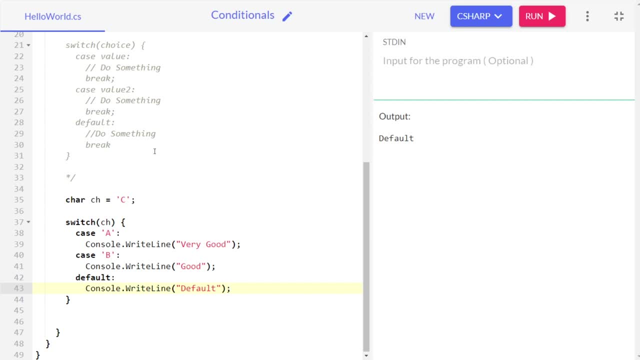 exactly doing now let's, let's start with a grade. so here you can see. it is giving us all right. it is giving us some error. all right cannot fall through from one case label, case a, to another. all right in general, all right in c sharp. it is giving us error in java if 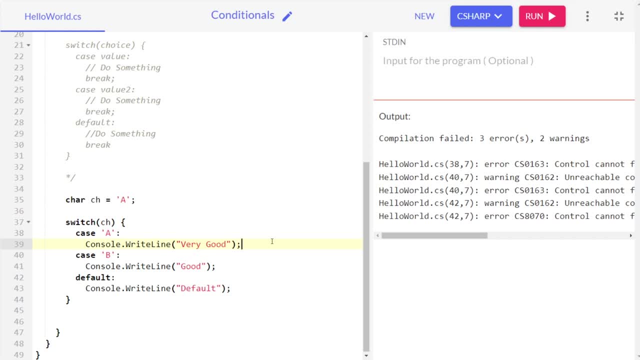 you would code in java or any other language, you will find that, uh, they are skipping like uh, after they are, as i've stated, a case a. they printed the case a, then, without the break statement, they are going to case b, and then they are going to case b, and then they are going to case b and then they are. 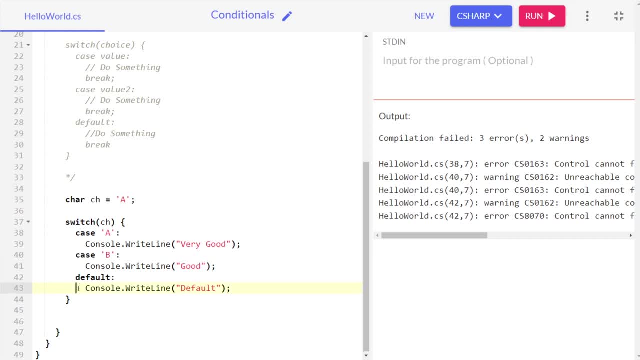 going to case b and without the break statement in case b they are going to default. so that's why we use break statement in here. of course, in c sharp it's giving error, but in java all right. in java, if you don't give break statement, it will print like: uh, every other statement in there, all right. so 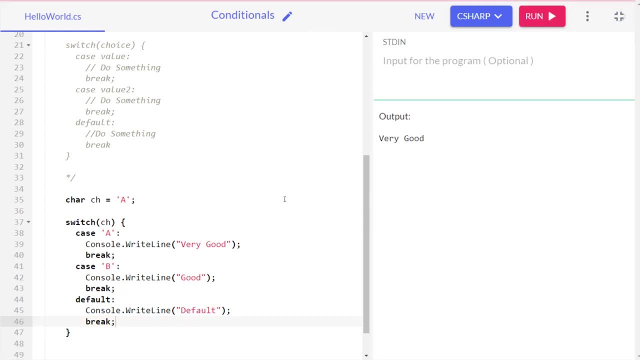 that's why i hope you understood the reason why we give break statements, right? so yeah, so make sure, all right, so make sure you understand, all right, you understand this concept uh very carefully. all right, because, uh, this concept is, you know, going to be uh very, very, very, very useful. all right, and always remember this break statement. 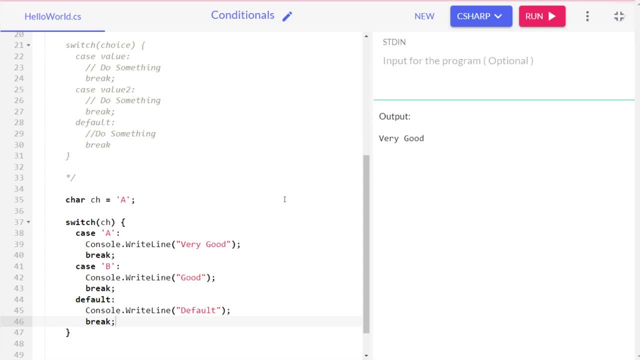 now it, it, it is a jump statement. all right, big statement is a jump statement. basically, break is the execution of after some condition is met. all right, you can understand that it like that, all right. so break statement is just: uh, breaks the work, work, the work of the work, of the work of the. 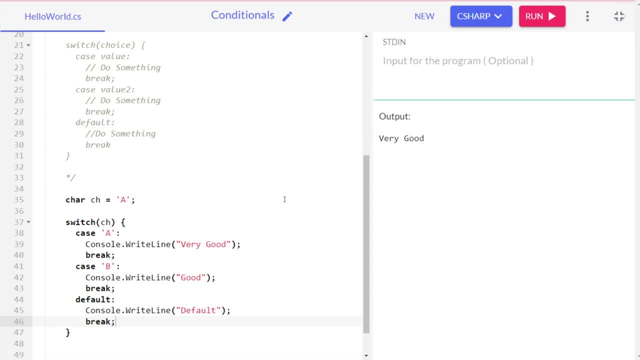 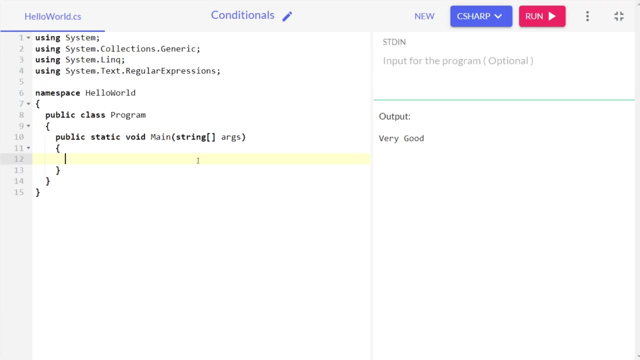 work like breaks the working of the statement. right, so this is it for, uh, this lecture. all right, see you in the next lecture. thank you, have a good day, guys. welcome to this lecture, and in this lecture we are going to learn about loops, all right? uh see, this is a very important concept. 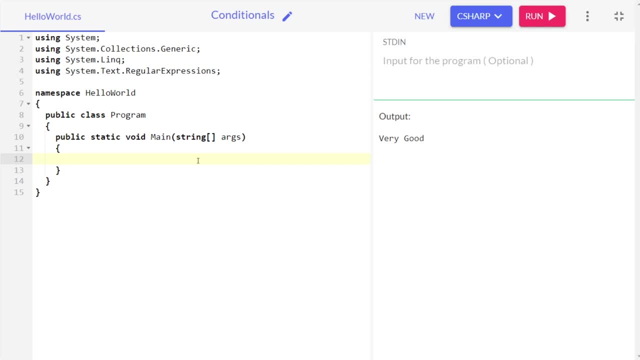 all right, because we are going to uh, use loops a lot. all right, we are going to use a loop like loops a lot, because whenever you will be developing something- all right, you won't be like uh, like every. you don't want to do everything manually, right, you can loop. 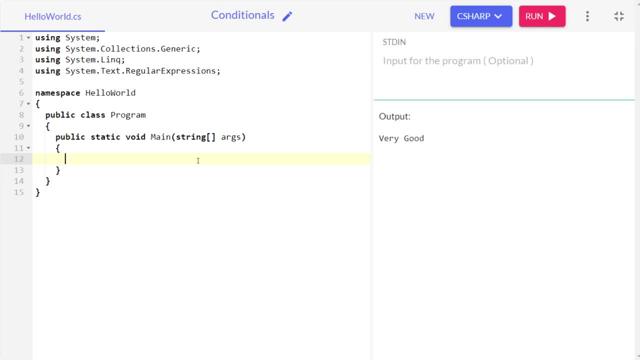 through it, all right. for example, if you are, um, what can i say? let's say uh. if you're, let's say you, uh like, created an array. all right, you created an array. i know you, you might, you, you don't know the meaning of array as of now, all right, but that's totally okay. i would uh like in in the 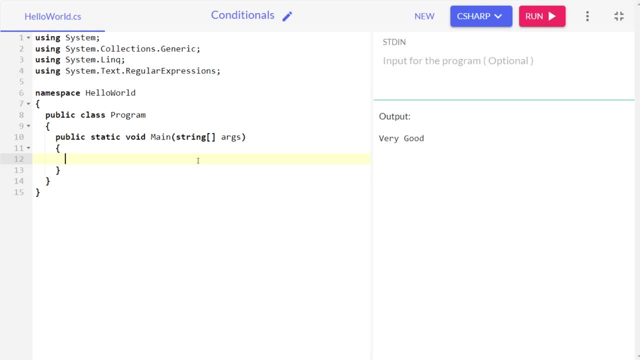 next lecture only we are going to discuss arrays, all right, and for arrays we are going to uh need loops, all right, we have to understand the loops to like work with arrays, right. so see, we can use loops in multiple ways, like, for example: uh, let's say, uh, we want to apply some materials, all right. 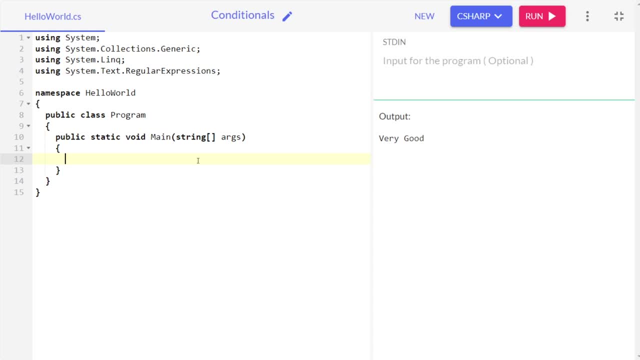 so i i'm taking an example. all right, in terms of uh, ar like the application we are going to make during, uh, like after we learn euphoria, right? so, all right, the basic understanding of uh, the basic concept of looping is to loop through something. all right, loop through something, loop, uh see the formal definition. all right for loop. 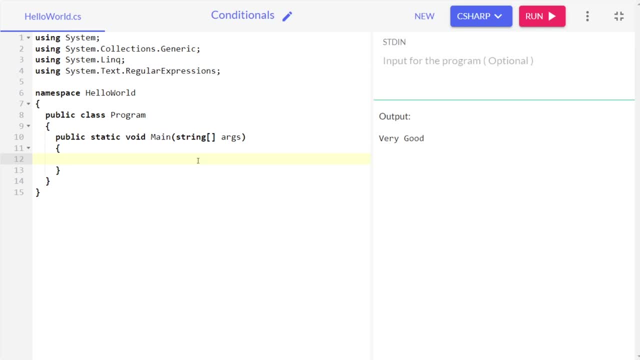 would be. loops are basically a way to, you know, iterate over something for finite or infinite number of times. all right, so let's say, for an example: all right, let's say for an example, do you remember? uh, i'm not sure if this happened with you, uh, but this happened with me a long time. 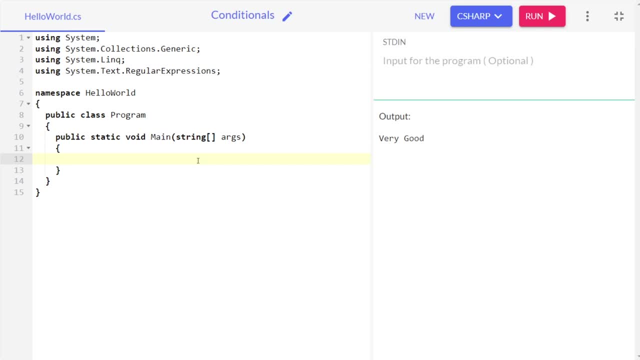 back. i was in, like you know, in class fifth and at that point of time, uh, i was in, uh, like i. i learned my first programming language. all right, that was q basic, all right. in class fifth i learned my first programming language and, uh, you know, uh, i got punishment at at that time i was like, uh, like you. 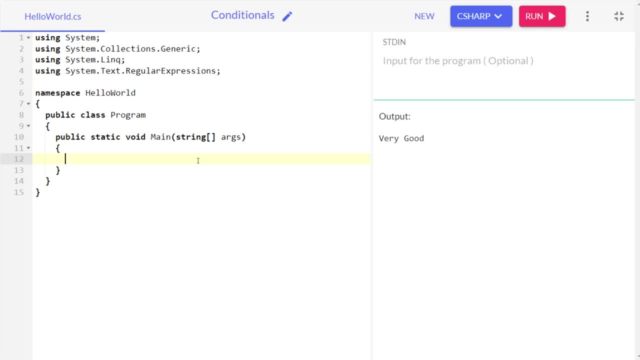 can i say, a very naughty kid. i used to, like you know, uh disturb my friends and because of that, uh, what i got was uh they- the teacher punished me- told me that you have to write. uh, something i exactly don't remember, i think it was: uh, i'm sorry, you have to write, i'm sorry, a hundred times. 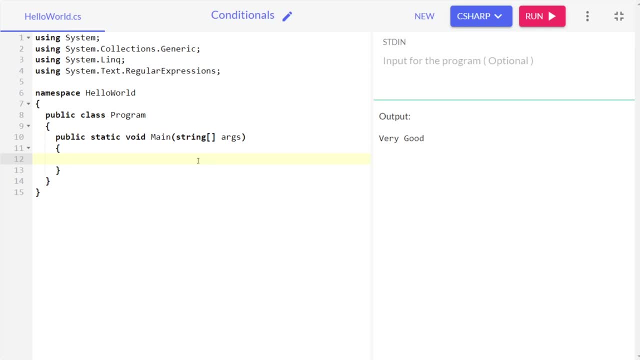 all right, and uh, you know, at that point of time, uh, i knew how to use for loops, right? i i understood, let's, why not see? the teacher is no, teacher is trying to tell us that. you know, uh, you have to write, i'm sorry, a hundred times. right, and you know, teacher just wants it a hundred times she. 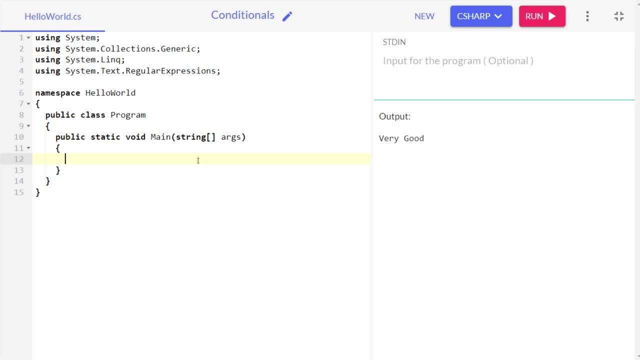 didn't told me how to write, like i have to write it manually or i can you know, use some dynamic way, like you, using a for loop to iterate over, iterate over for hundred times and uh, print, right, uh, print, i'm sorry, right. so what i did is all right. what i did, i basically i uh use the technique of for loop. 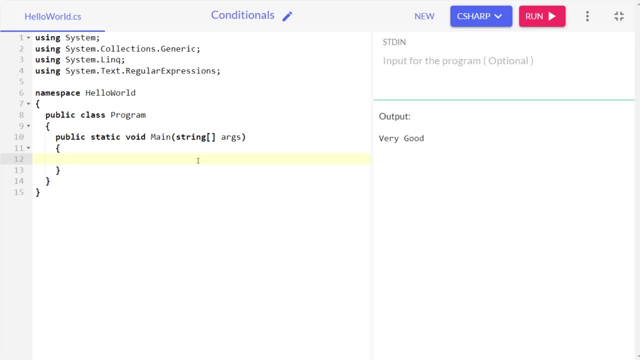 all right to, you know, iterate hundred times. i use the technique of for loop to iterate hundred times and print, i'm sorry, a hundred times. all right, it like it, completed in four to five lines and after i shown it to the teacher, the teacher, you know, scolded me a lot. all right, and then. 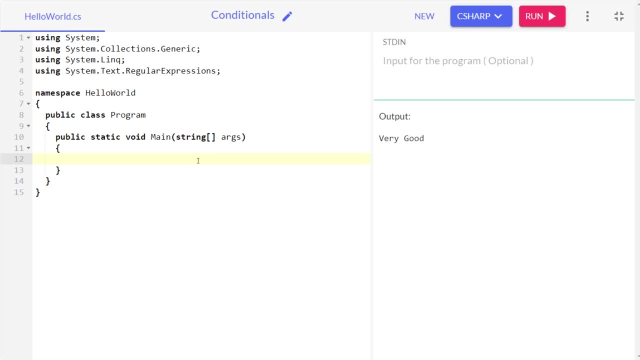 gave me uh, then told me that you have to write- i'm sorry, two hundred times, uh, for you know, manually. and after that i never tried, tried this with any teacher, all right. after that, actually, i never got punishment from class six, so it never happened. so, uh, in class fifth, this incident was, you know, was- a very funny. 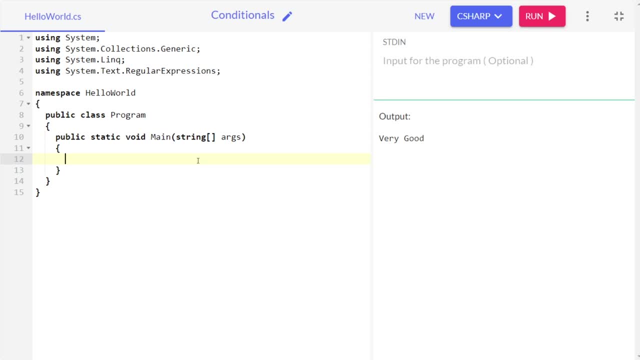 incident for me, because that was the first time i actually used for loop to save myself from, you know, writing the whole thing. so that's the concept of loops. all right, loop actually helps us to, you know, reduce uh or most of the work, right, like, for example, uh, right now i can give you. 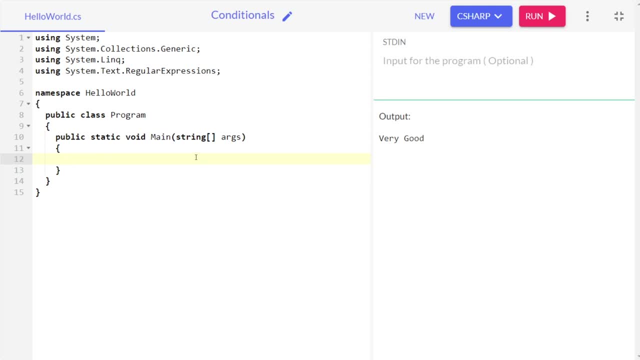 all right, hey brother, uh, write, you know hello world a hundred times. all right, so you, right now you don't know the concept of loops, but you are a very obedient student. uh and uh, you will start writing like a console dot. uh, right line. all right, hello world. right, you will be writing that. uh. 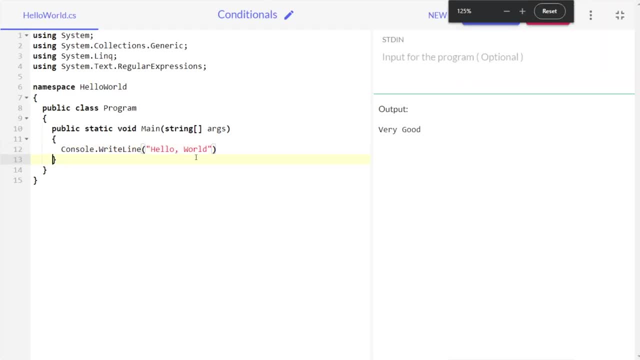 a hundred times. right, you would be writing that a hundred times, all right, and that that's going to take a lot of time. right, that's going to take a lot of time. so what we can do is we can use, you know, a loop. all right, we, you can use a loop to actually do it for us a hundred times. all right, so that it uh the computer. 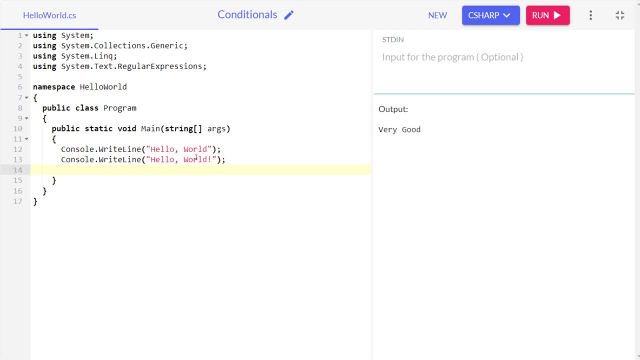 will only perform the- you know the function. we don't have to do anything. currently we are doing it manually. but with a, with a loop, we can, uh like, make our computer do the you know, write the hello world. all right, so i will show you how to do that. 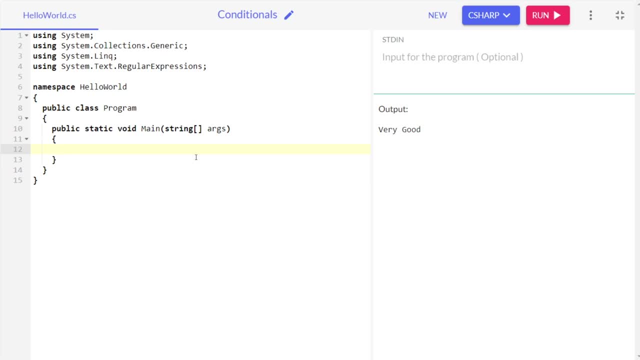 but before that, let's understand what a loop. so loop, basically, are a way to iterate over something for finite or infinite amount of time. all right, so you know. first, uh, let's understand how many types of loops are there. all right, see, there are um three types of loopholes. all right, that is. 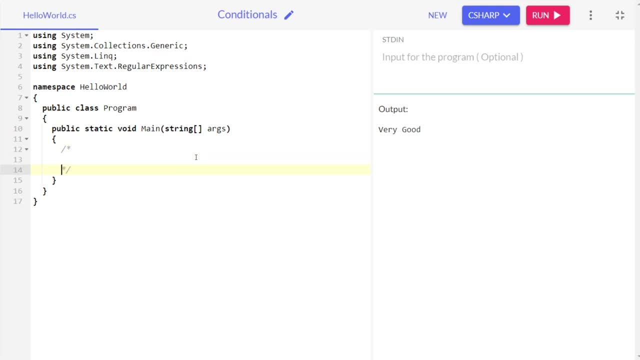 let's first write it down in here. all right. the first type, all right. the very common used is for loop, all right. then another one is while loop and the third one is very least used- all right. uh, actually i really don't use this loop anymore, like i don't need it. all right, but 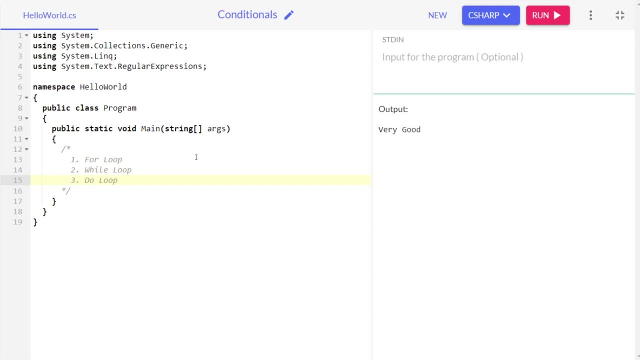 you have to. you have to have an idea about do while loop right, so make, uh. that's why i'm teaching it right now, although i don't think you will also be using do while loop in your career yet. uh, but you know, whenever developing applications, i never used dual, but it never came handy to me whereas i 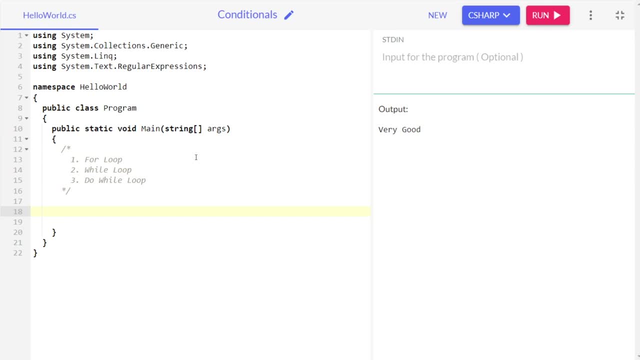 used for loop and while loop a lot right. so that's why i'm going to teach you all the three loops today. all right, and we are going to start with uh fall. all right, see, remember, the concept of looping is simple. all right, concept of looping is simple. it just tells that we are, you know, uh repeating. 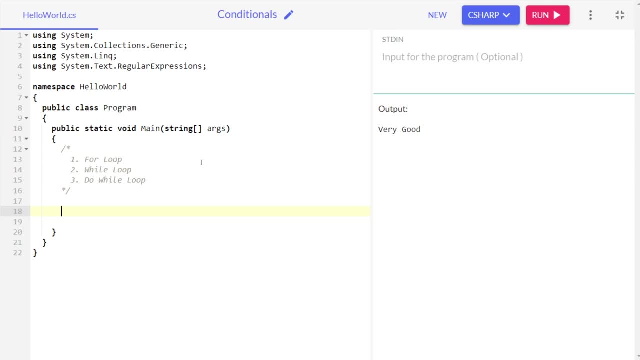 all right, looping means repeating. all right, we are looping. totally means repeating ourselves over something right. so that's the concept of looping. but there are three different ways to loop. all right, that is, one is for loop, another one is while loop and the one is do while. all right, and i would. 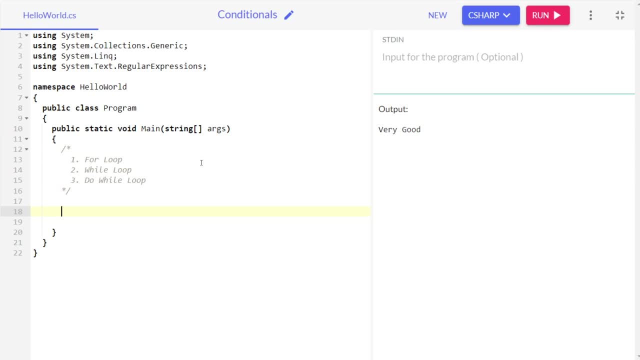 tell you, all right, when to use for loop and when to use while loop. all right, so make sure to you know. listen to this lecture carefully. so, first of all, let's understand the syntax of for loop. the syntax of for loop is very simple, all right. so the first is we have to write for. 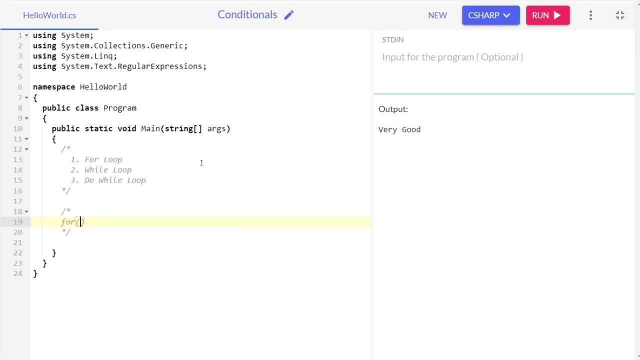 all right inside the, for we have to give brackets, and the first, all right. the first would be, you know, first statement we have to write is start. then we have to give a semicolon, then we have to give a condition, all right. condition that for uh, how many steps we want to run, means for for how many. 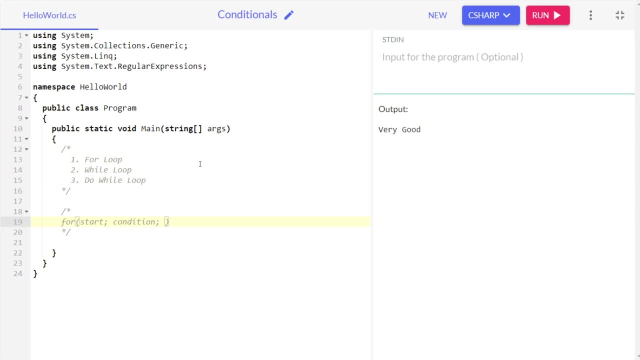 times we want to run right now. the next would be all right. the last one would be steps. all right, that is how many steps we want to take. step means how many, you know? uh, let's just say, if we give step as two, then uh, let's say we are trying to uh print. 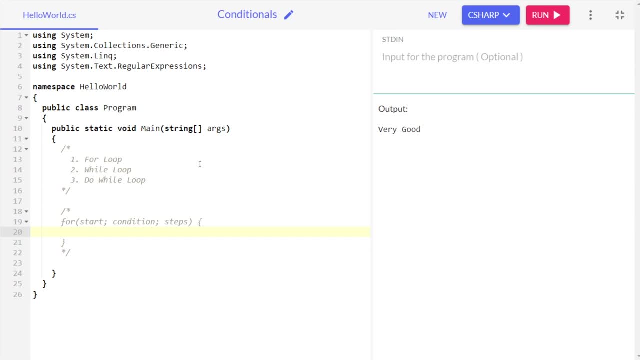 numbers from one to ten, right? so let's say, if we give step as two, then it would only, uh, like you know, if we start from zero, then zero plus uh two. let's say it would uh give us two, then four, then some. uh like it would give us like this: all right, then inside that we would be printing. 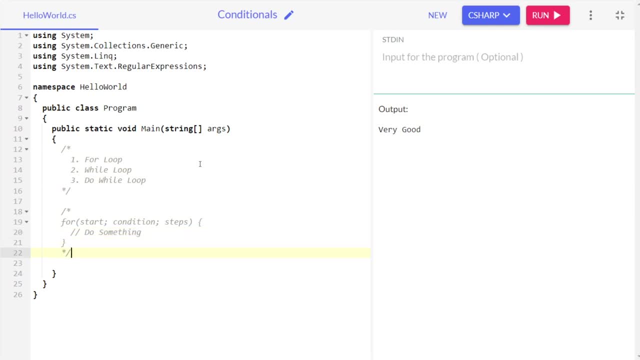 uh like it would be instructing the program to do something, all right. so this is basically the syntax of follow, all right now. i told you- you know my story of uh- how i was punished. right now, let's try to implement that. punish. uh like, let's try to implement that all right. so for you have to. 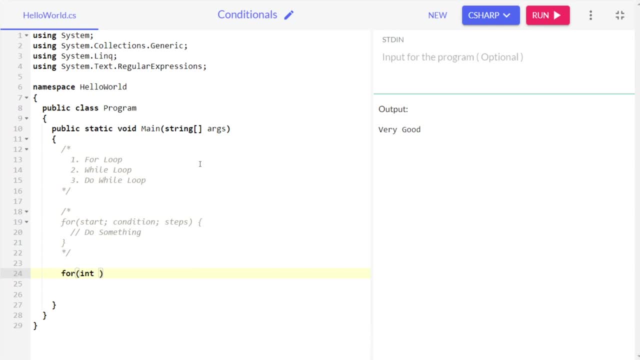 declare a variable, right, so i'm going to declare a variable within the follow only. so, for i equals zero. yeah, it's uh, and remember that i'm starting the value of i from zero. all right, then i want to go till i less than equals 100. i want to go till 100. then i have to give how many steps i want to. 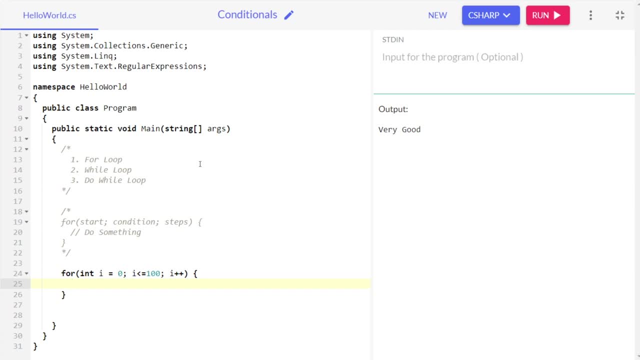 increment, all right, how many steps i want to go with. so i plus plus means one, all right, every step will be incremented by one. now, if we, if we want to, you know, uh, let's say, if we want to increment every step by two, what we can do is plus, sorry, plus equals two, all right, but for now, 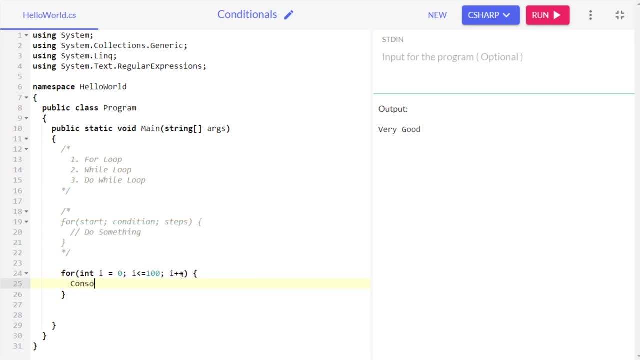 plus, plus is totally fine with us. so now what you can write. console dot right line: hello world, all right. so teacher told us let student write hello world instead instead of i'm sorry, all right. so now let's see if, uh, it is printed hundred times or not. all right, 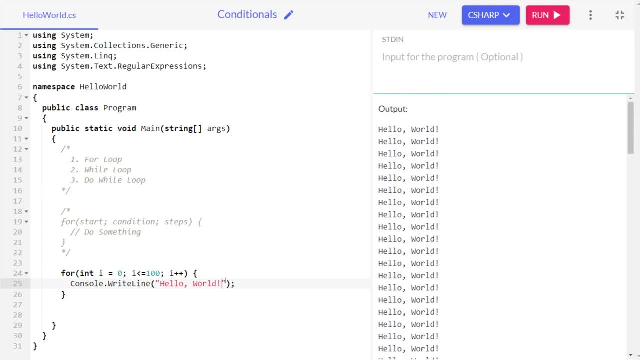 so you know there's not really a way to. you know we are not able to count it right. so let's uh give a plus sign and, you know, add the i in here. let's see now, yeah, so here you can see that it's starting from zero and uh, it is going from hundred, going up to hundred. now, here you can see. 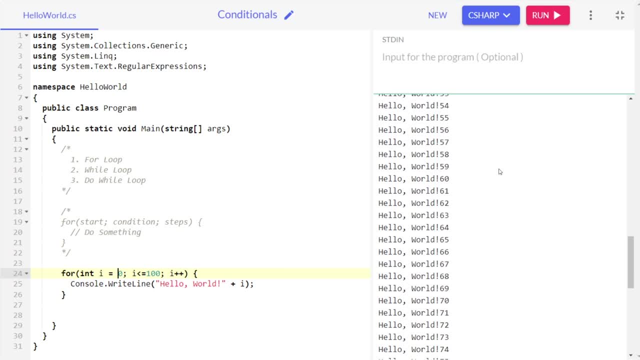 as it is starting from zero, the total number will be 101. all right, because if one is starting from here, then zero is another extra one, so it will be hundred and one times all right. so to fix that we can actually start the loop from one or, what we can do is we can, you know, mark it? uh, like give the. 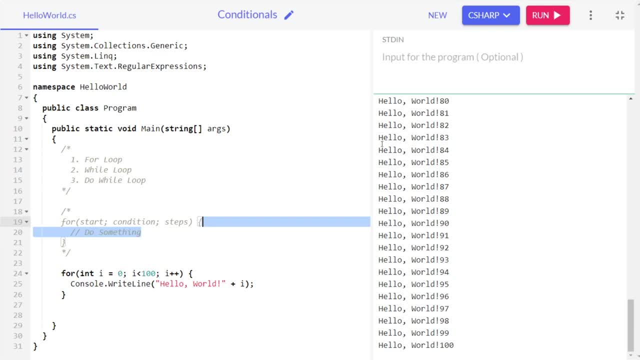 condition as i less than zero, then what will happen? it would start from zero and, uh, end up to 99, so it would be total hundred, uh, it will be total hundred times. we looped. all right, so that's how we, you know, work with for loops. so for loop is a way to loop through, all right, some sort of 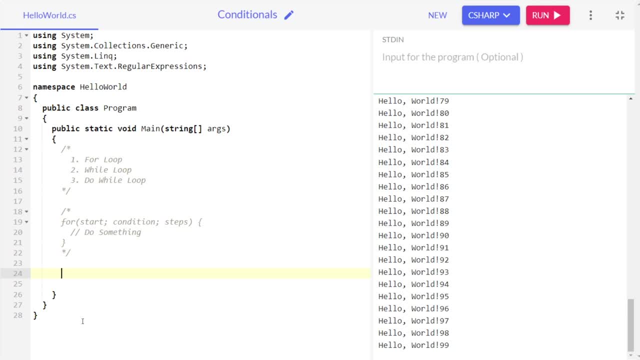 you know, uh, some sort of condition. now, always remember, we use all right, we use for loop. all right, we use for loop when we know exactly how many, uh, how many iterations do we want, like right. so for, in this example, we knew all right, in this example, we knew that we are going to need 100. all right, we. 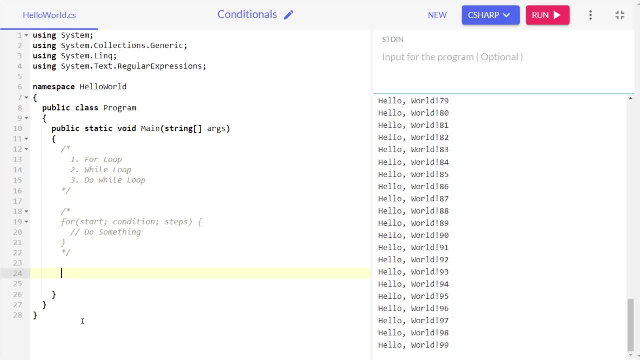 are going to need 100 iterations. so that's what we did. we uh go. we did 100 iterations in the program to print hello world. so that's when we use for loop. all right, so now, as we have understood the concept of for loop, let's you know, let's try uh writing some program through, like, let's try solving some. 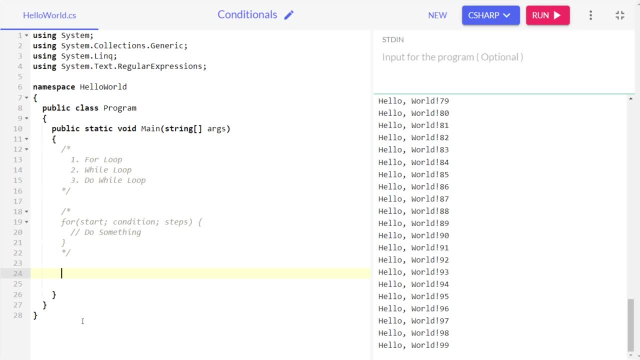 program program. right, i want you, you guys, to try it first, all right, so pause the, you know, pause this particular video after i give you the question and try it by yourself. then uh come to this video and see the solution, all right, so i'm writing a comment in here. let's uh write a program to print. 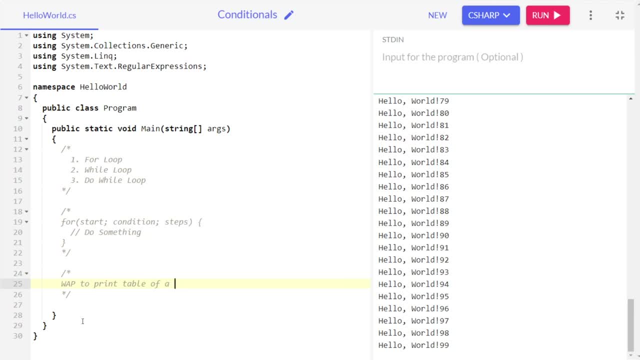 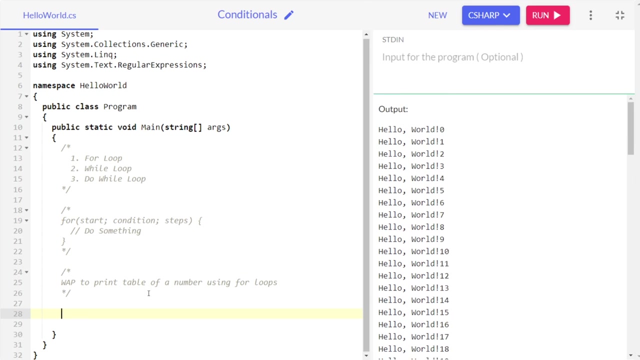 table of a number using for loops, all right. so what you have to do is you have to code a solution, all right, which will be able to print table tape. uh, all right, it will be able to print table of that number, all right. so make sure you do that. and uh, right now pause the video. 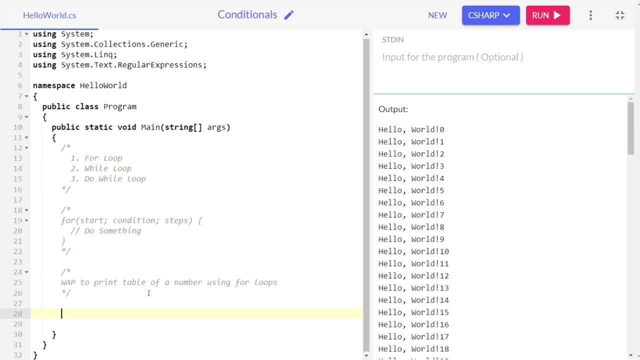 and try it by yourself. it's okay if you are not able to do it, all right, it just needs some more practice. after uh, practicing, you will be very familiar with the concept of all right, so let's try it out now. all right, so for i'm going to implement it. so for see, first of all, the very 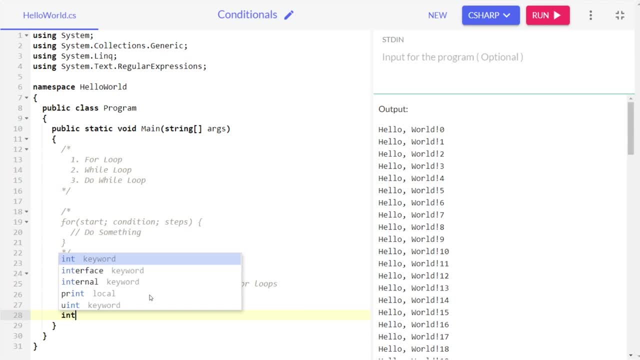 first thing i want you to is to declare a variable. all right, that is int n. all right, this would be the number. all right, that is, i want to create a table of two, all right. so now, what i want is for int i, because i want to start from zero, all right, and i want to end up till 12, all right, and i plus plus. 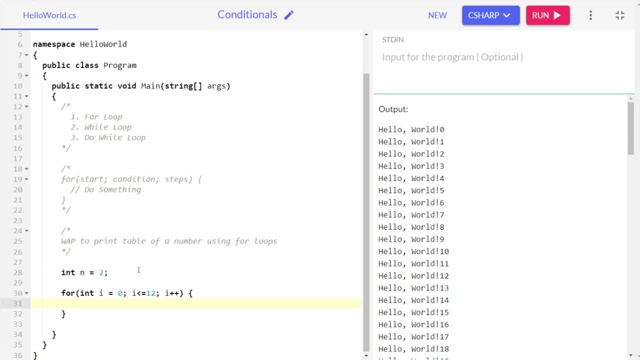 why? because we aren't skipping any step, we are just incrementing by one. all right, we are just. we just want one step each. all right. now create another variable. all right, that is int, let's, uh, you know, let's name it f. all right, and uh, what you have to do is: 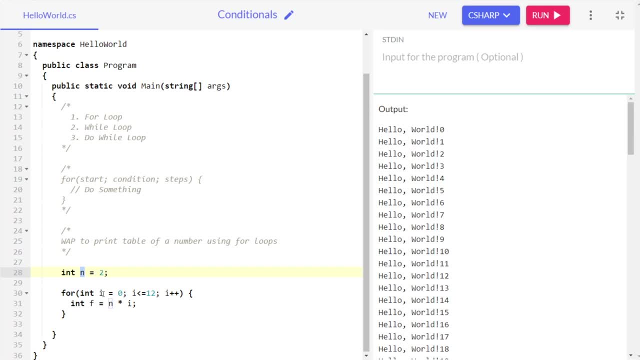 multiply, all right, this value of n. all right with. i see, remember how this is working. first of all, in the first iteration, the first iteration, two is multiplied by zero and the outcome is zero. in the second iteration, all right how it is reaching to a second iteration. it is: 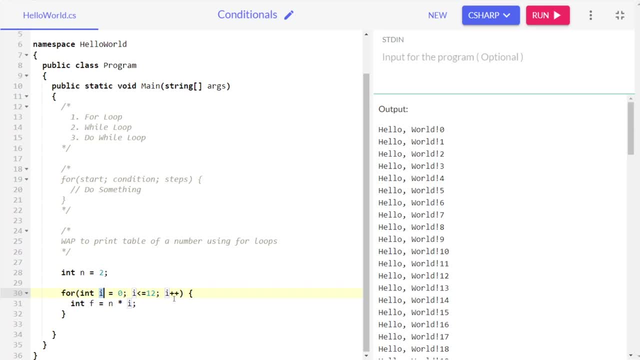 reaching to the second iteration by incrementing this i by one. all right. so now in the second iteration, i will be one, all right, i will be one, and two will be multiplied by one. and in the again, in the third iteration, it will be incremented and it will be go to two. all right, then again two. 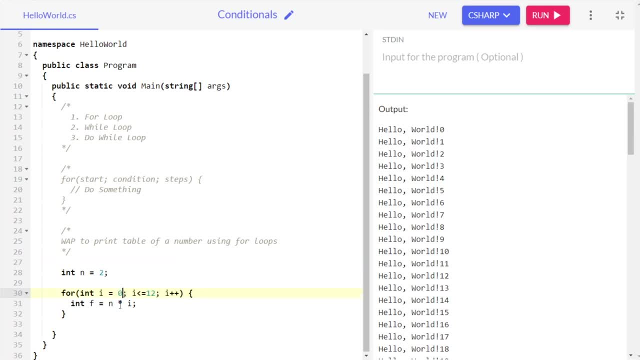 will be multiplied by two, so it will be working like this. all right, so i hope you understand how, how this program will be working. all right, then console dot, right line and uh, print the value. all right, and also make sure, uh, you know, write it like this. so just wait in. let n plus give an asterisk. 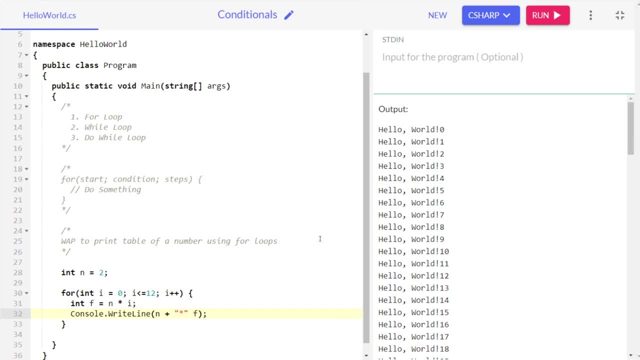 in here, all right, and uh, plus i, it's. it's just a. you know, i'm just maintaining a decrement here, all right means i'm just actually let's leave this thing. all right, try this one later on. first of all, let me show you if it is printing the table of two or not. 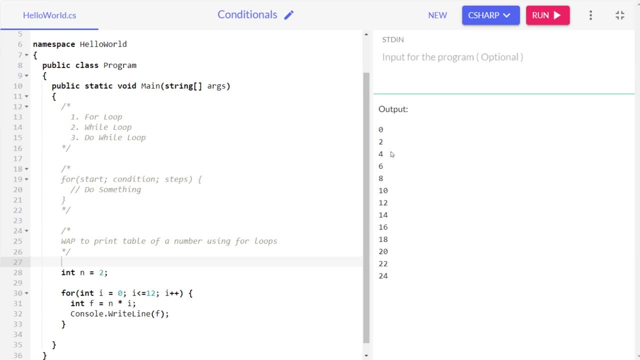 yeah, it is of course printing. so two zeros are zero, two ones are two. two to the four, two three the six, two four is the eight, two five is the ten. two six are twelve, and so on. it is going up to two twelve twos are twenty four. right, so we have successfully printed the table of two. now let's. 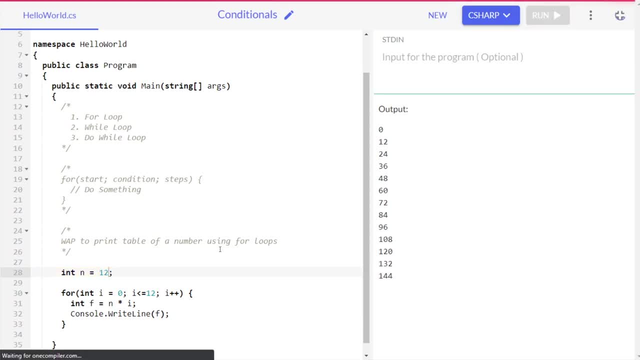 uh, you know, print the table of twelve, let's see if it is able to do it or not. see, twelve ones are twelve, twelve, twos are twenty four, twelve three, thirty six, and it is going up to twelve twelve hundred and forty four. so that's how it is working, all right. 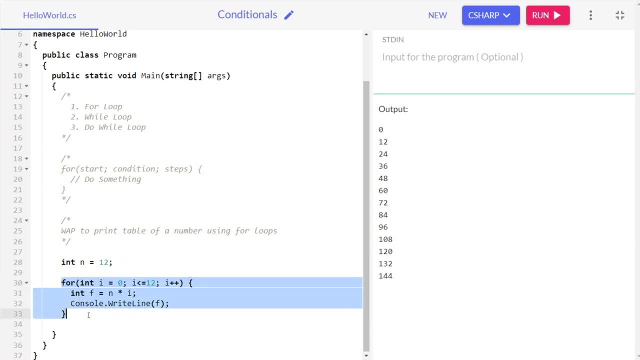 that's how a for loop is working. first it is remember. it is iterating till the condition is met. all right, and for us the condition is 12.. we exactly know how many times we want to iterate. we know that we want to iterate it 12 times. that's how we set. 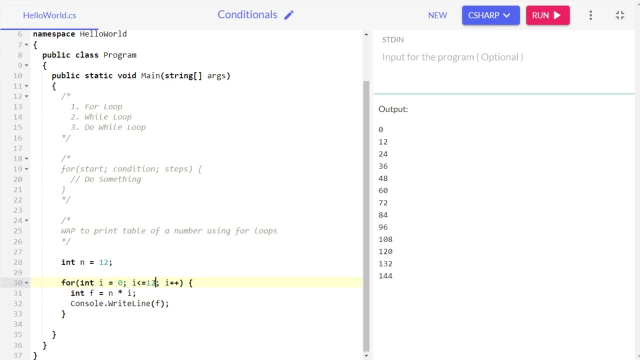 uh, that's how we actually set up. you know the condition, so that you it iterates uh, up to 12, all right, now, for each iteration it is incrementing the value of i. that is, uh, in the first iteration the value of i is 0 and you know, 12 is multiplied by 0 and it is printed. 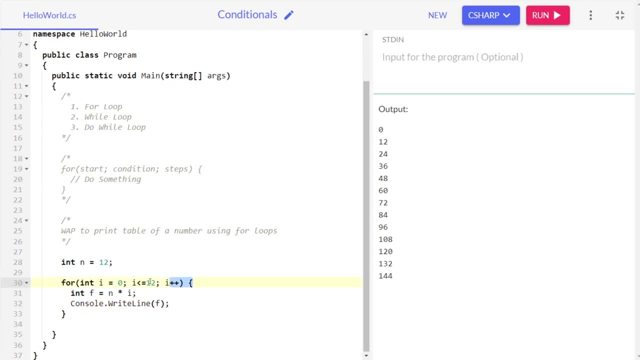 and in the second iteration, when it goes to a second iteration, the value of i is incremented. all right, the value of i is incremented, and this zero is changed, uh, to one. all right, so. and then, uh, in that iteration, 12 into 1 equals 12, right, so? that's how this whole thing is working, all right. 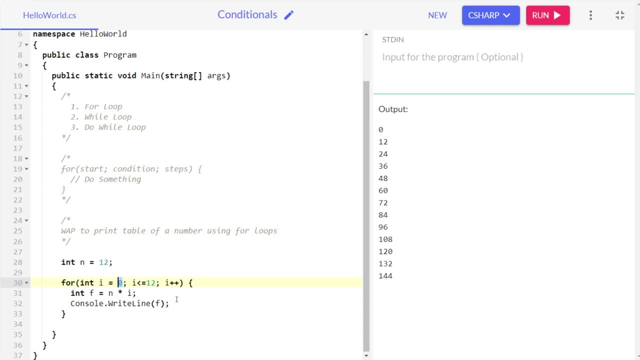 so i hope you understand how this worked right now. i hope you know for loop is uh, the concept of follow-up is cleared, because right now i'm going going to go to a while loop. so make sure, if you are not- uh, you know, not clear with uh, the concept of for loop, make sure you uh. 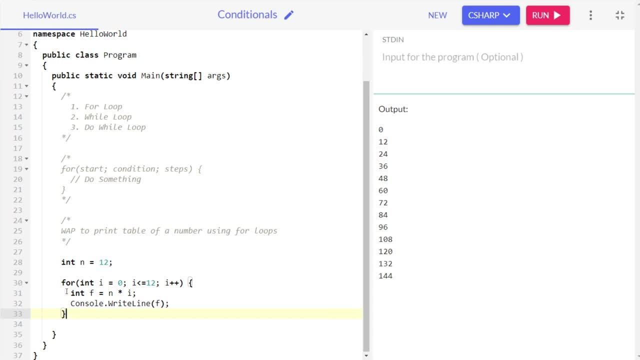 practice it a little bit. all right, watch the uh portion of for loop, all right, the one i taught right now. so watch that again. practice for loop, all right. then only go to while loop, all right, so make sure you do that. so now let's- uh, you know, remove this whole uh syntax thing and let's mark for loop as: 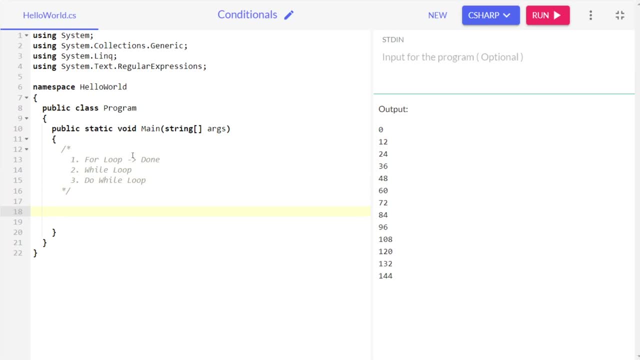 done, all right. now here we uh, go to the follow, all right. so what is follow? why loop? sorry, what is y loop? yeah, see, you can say, while loop is a brother, all right, brother of follow, all right, it is also used for looping all right. but the thing is all. 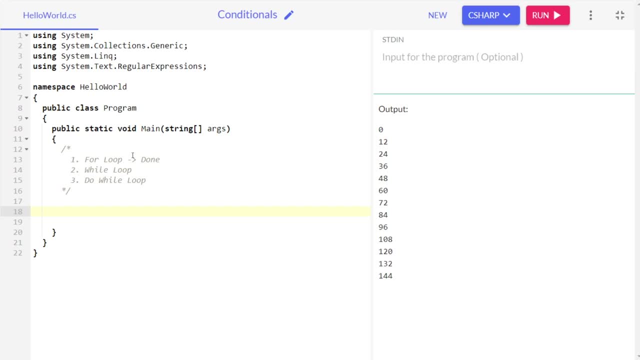 right. while loop, all right. while loop runs, all right. while loop runs runs till the condition is false. all right, it will run till the condition is false. and this proves one of our concept that for loop is only used. for loop is only used when all right. for loop is only used if we don't know how many iterations we want. all right, that's when for loop 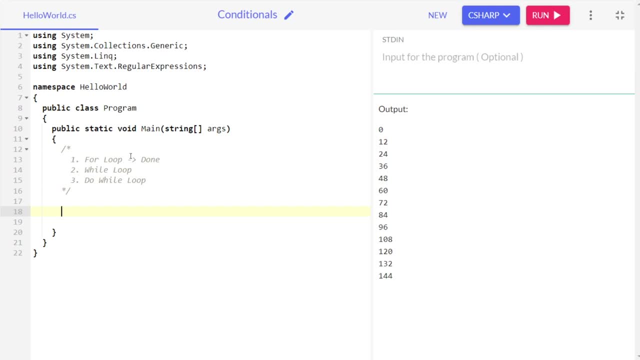 is used. all right, as simple as that, all right, so now let's- uh, you know, learn about the syntax. so let me comment this out. all right, so this is the basic syntax. we have to, you know, first, uh, declare, uh, a variable. all right, it's better to declare. 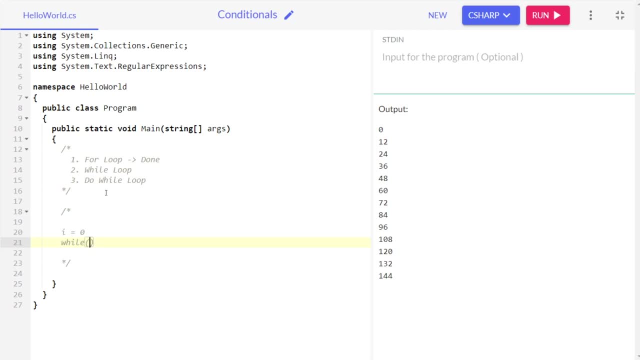 a variable at first. then you know, uh, write the while, all right, and in here the condition will go on, all right. actually, this, you know, this variable is not a part of the sentence, but i'm showing you because you would be needing it. all right, then curly braces, and inside that you have to, you know. 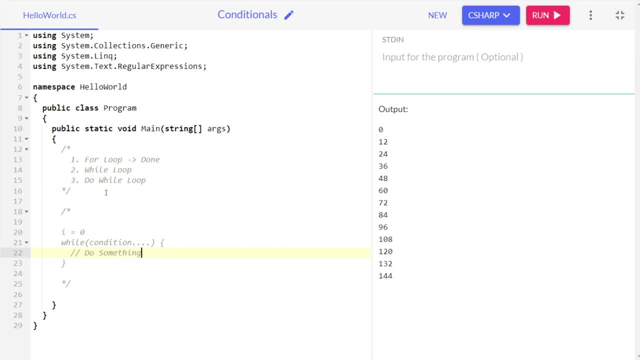 uh, right, do something. all right. so that's, that is what the syntax of fall while lupus, all right. now, you know, uh, i told you about the whole hello world example. let's, you know, try to implement it. so, first of all, i want to want you to declare a variable, all right, int i equals, you know, zero. it should start from zero. 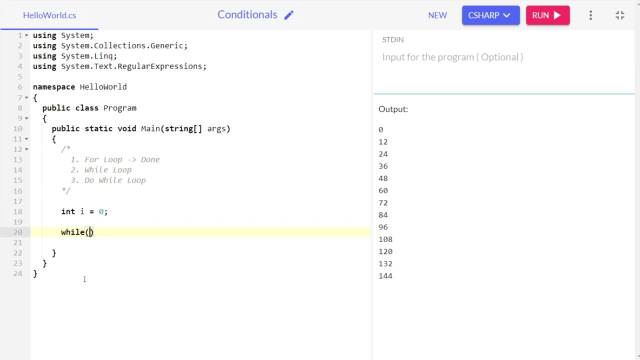 all right, and give it a condition. while, all right, while i is less than equals 100, all right, i is less than equals 100. i want to print hello world. all right, i want to print hello world. now, one more thing, all right, in for loop. remember how we were incrementing the value, right, do you? 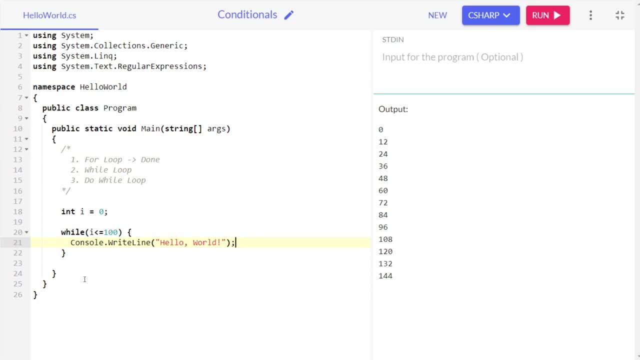 remember that how we were incrementing the value by i plus plus. similarly in here also. we have to do something, and we have to do that. after all, our statement is done. all right, that is for now. our only statement is concert or heart, right line and you. 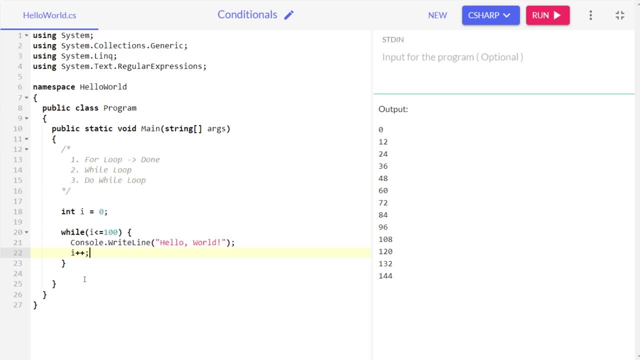 at the end we are going to write i plus plus. all right, now i will. i will let you know what will happen if you don't give i plus plus. but for now, all right. for now let's see what happens if we give. it all right, let's see the basic example. 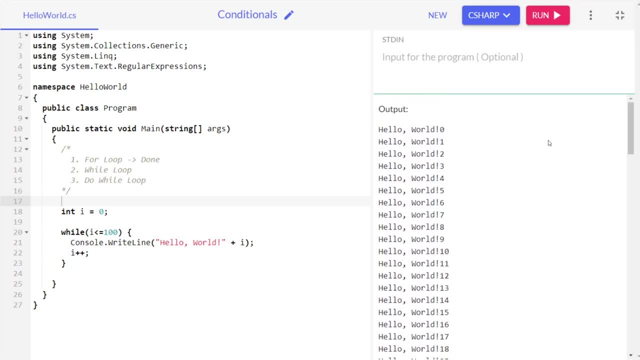 see, it is, you know, printing hello world till 100. all right, it is printing hello world till 100 and it is stopping when the condition is becoming false. all right, it is stopping like say, like see, when it reached 100, when it reached 100 after when. 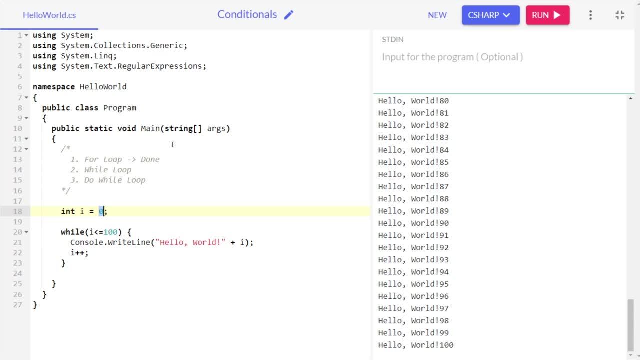 it was go. it was going to 101. as the condition is not meeting, as 101 is greater than 100, it stopped looping, all right. so that's how it is working. so let's understand. first of all, we declared a variable, declared a basic, you know, a basic variable. all right, we declared a variable i. 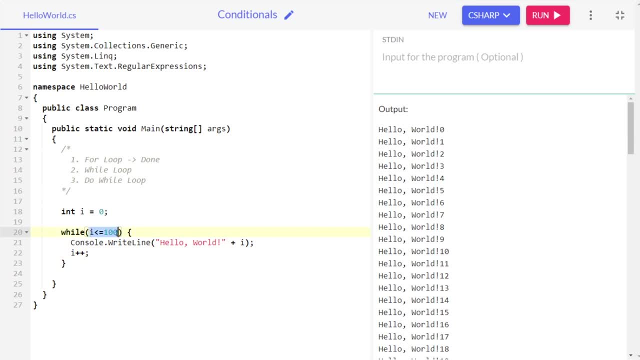 then we created a while loop. in the while loop we declared a variable, i. then we created a while loop. there's a condition i less than equals 100. now this condition will be like: what can i say? this condition is responsible, all right, for executing this particular line, concert or right line, all. 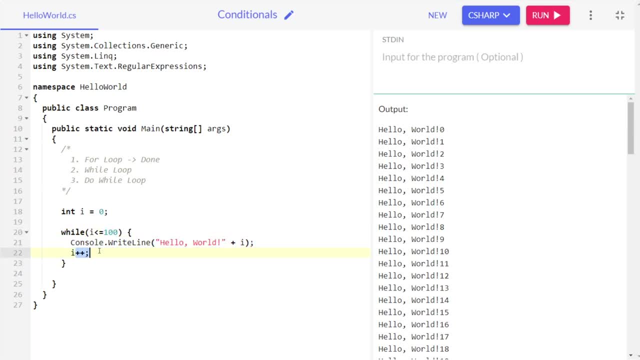 right, and then we are going i plus plus, that is, incrementing the value of i by one. all right, that's what we are doing. let's say, if we, you know, let's say, if we remove this, i plus plus, let's see what will happen. see it, uh, you know, this, uh particular website in a sort of, crashed for for a moment, like it. 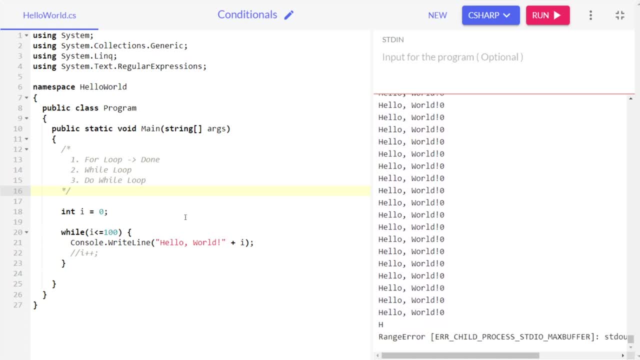 you know it not exactly crashed, but you know, uh, what can i say? it uh freezed, all right, freeze for a moment, all right. and here you can see the value. uh, you can't. everything in here is zero, all right, everything in here is zero. and at the end, here's a error that you can see the value of: i plus plus. 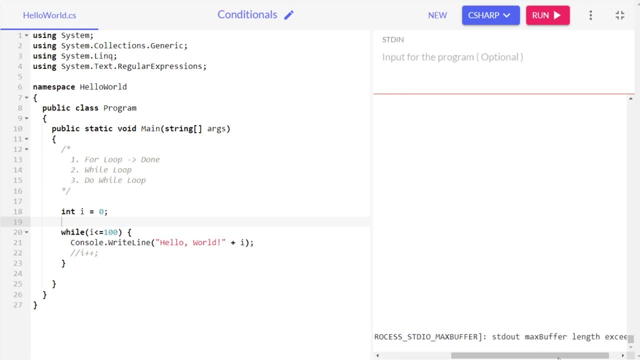 that, uh, range error, all right, range error: max buffer length exceeded. that's because, all right, that's because we ran into an infinite loop. all right means it. it is a never ending loop, it won't end ever, all right, that's why? uh, that's because we didn't give i plus plus. the reason is what? 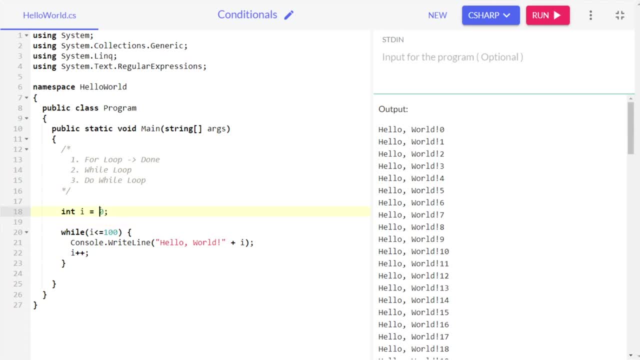 role is i plus plus. playing is it is incrementing the value of i, all right, like for the first order, first iteration, it performed this particular thing. then we are incrementing to one, all right same. then Y is the second, I mean then one, all right, then one is the second iteration. in the second iteration means the second. 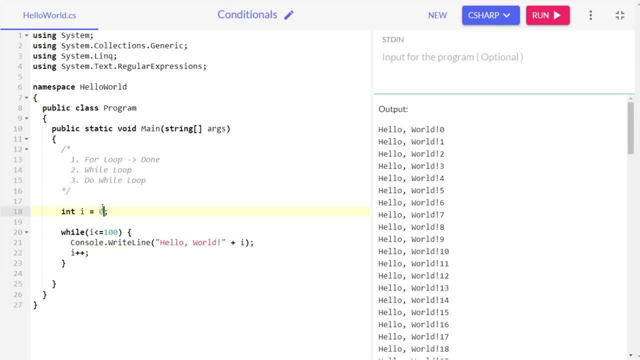 iteration completed. we incremented the value of I. now one has gone to two. so like this, all right, like this, we are working on the for loop, all right. so if you don't give the I plus plus, then what will happen? then what will happen if we don't give the I plus plus? then it will run into a infinite loop, all right. and 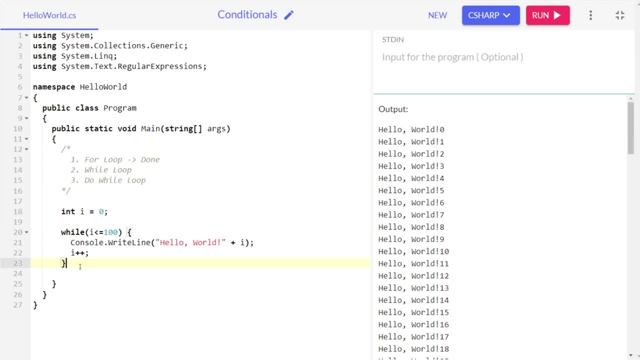 of course we don't want that. so that's how our while loop works, all right. so I hope you are clear with the concept of while loop. all right, and also one more thing. we can. you know we can write this: I plus plus 2. I plus equals 1, I plus. 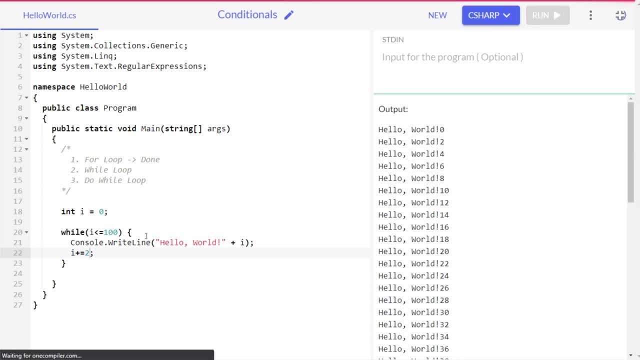 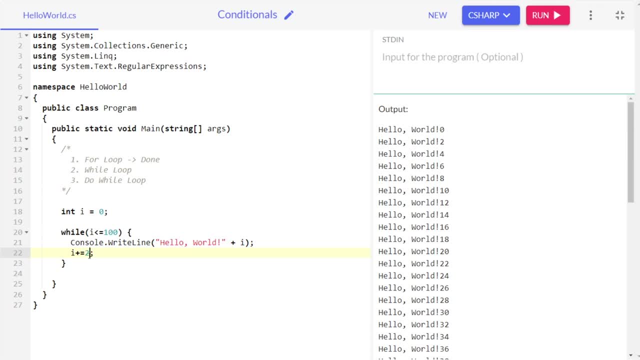 number of times of hundred. so that's how it is working. all right, so that's how we. you know code, you know for loop. all right now, let's all right. remember the program which I taught you like to print out a table of a sort and number. right, we are going to do the same thing with with while. all right, so. 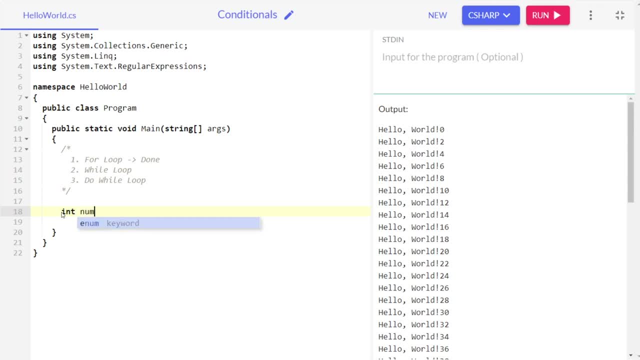 the very first thing I want you to understand is write a variable, all right, and that would be containing the number. then, right, all right, write a variable I. it would be the counter. counter variable means the I that we are taught you. all right, it would be incrementing the value after each successful statement, right so? 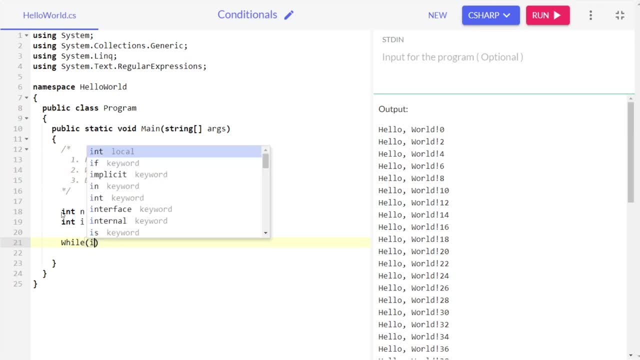 now go to while I- all right, just wait while I all right- is less than equals 12, all right, what I want, I want is to multiply, all right, multiply. multiply the number n with I, all right, then after that, I want to print it. all right, I want to print it. console dot. 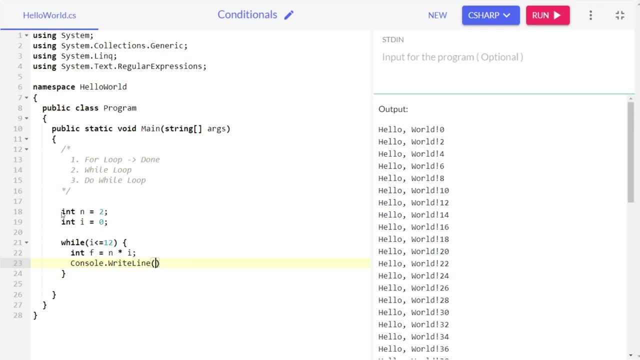 write line. all right, that's myFe GR, which is the thing, what I want. I want it to be move modelans in here. so I want to vote so that I can calculate the square root. so I wanna calculate square root, so I say I want to print it and then after: 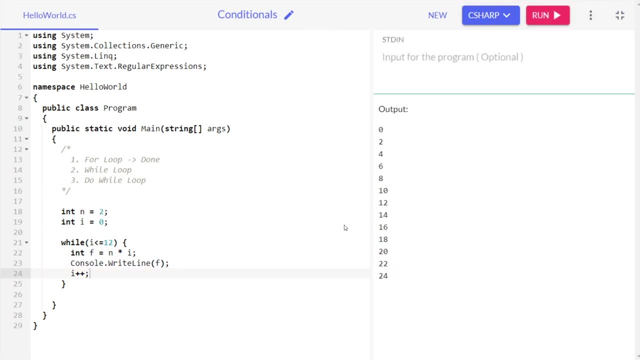 printing Hill. staying true value, I am going to increment the value. all right, I am going to increment the value by 1. so now let's see, cool. so we got the same output that we got for. all right, that's how it is working, all right, you all, i guess you also know how, when, when to use which right. so we use for loop when we exactly. 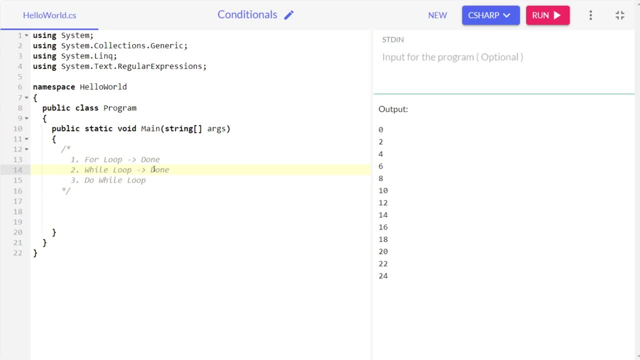 know how many iterations we want and we use for. sorry did i? oh sorry, sorry, i guess i messed it up. so again, we use for loop when we know how many iterations we want. we use while loop when we don't know, all right, when we exactly don't know how many iterations we want. so that's when we 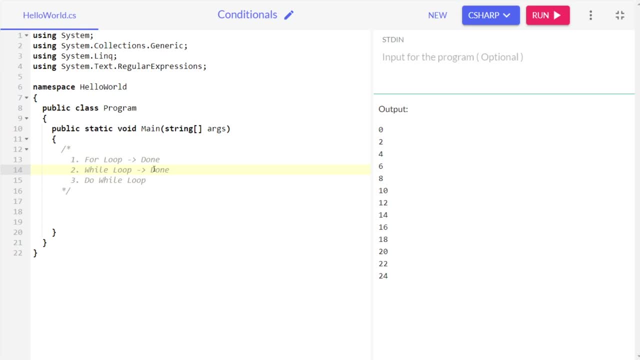 use for loop, all right. and a for loop statement stops working when the condition- no, when the condition- gets to false, all right. so always remember that. now here comes our last looping statement- all right, and the least used ones, all right. this is known as do while loop- all right. 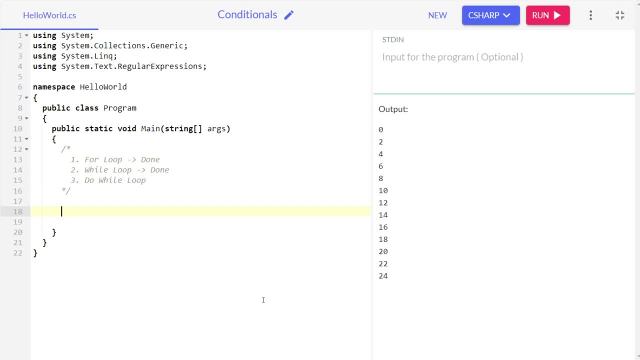 it's a see, do while loop now is, you know, very similar, you? all right, it is very similar to uh, what can i say? uh, while loop, all right, it is very similar to while loop. just there's a one difference. all right in while loop, if the condition is false from the 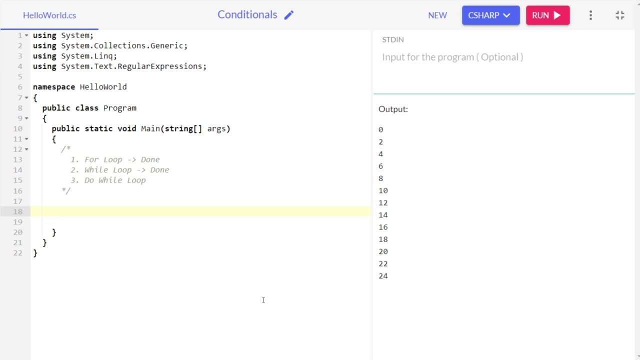 starting point now, it won't even execute a single statement, but in do while loop, even if the condition is false, all right, it will all right. even if the condition is false, it will execute once. all right, it will at least execute once, all right. so let me first, uh, make you familiar with the concept of do while loop. 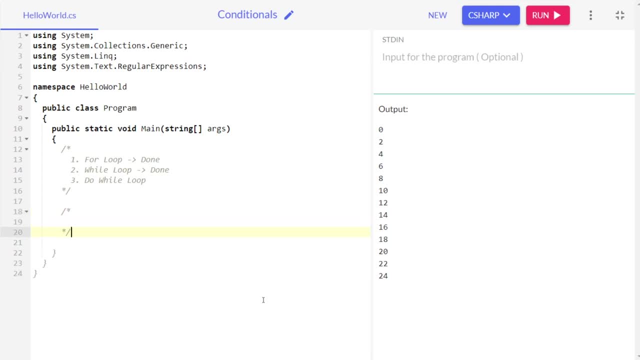 means the syntax of develop actually. so i hope you are familiar with the concept of: you know, do while loop. so do first of all you need to write, do then curly braces. all right, inside the curly braces you have to, you know, go for, uh, writing the you know particular code. you want to write, do while loop. 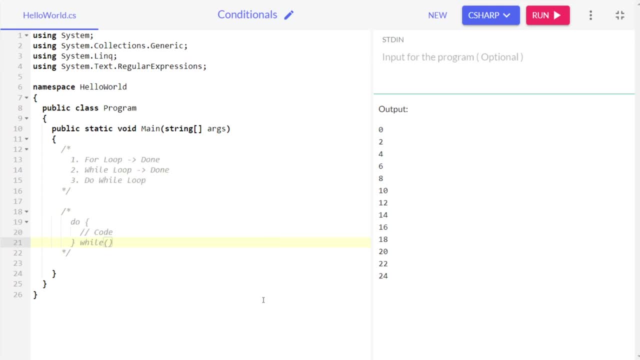 to give, then you have to give a while statement in here. then the condition in here to uh to be executed, all right. so that's what the syntax is. it's a bit weird syntax, right, i know, i know. so now what you have to do is define i variable. all right, see, we are going to uh, you know, write the. 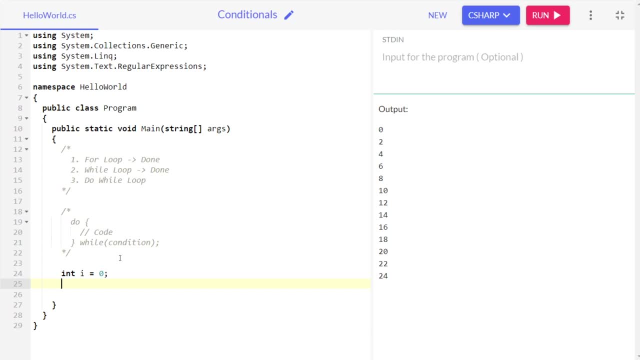 example we did last time, that is the hello world one. so then write, do, write, do. all right, then console, dot, write, line hello world. then i'm going to increment the count. all right means increment the value of i, i plus by i plus plus, or you can also do: i plus equals one. all right, then in the 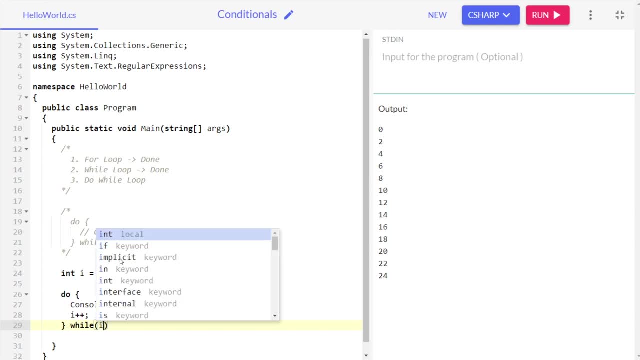 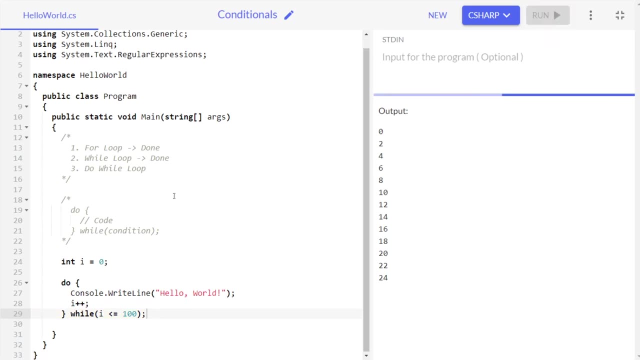 while. all right, i'm going to give the condition i less than equals no hundred, and then semicolon. now let's try to run it. so here you can see. we actually got the hello, hello world. now, to verify that, if we actually ran hundred times or not, i'm going to, you know, uh, add i to the equation. so now, here you can see. 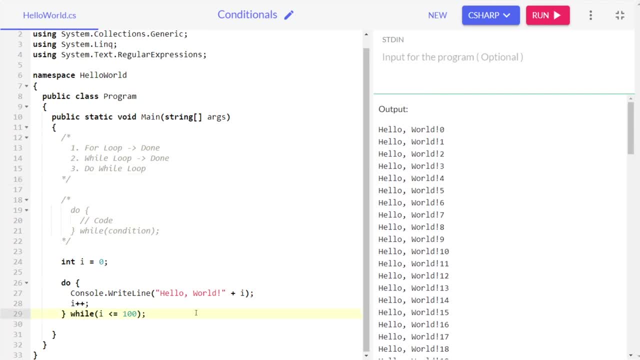 it has ran hundred times now. You know what I told you just a few seconds ago: that even if the condition is false from the starting point, do while loop will at least execute once. All right, So you know? let's, let's verify it. 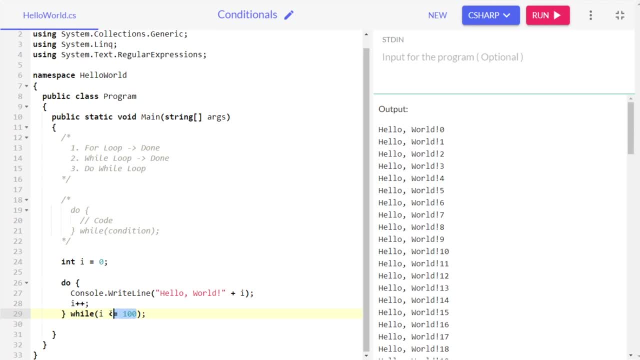 Let's verify it. Let's give if the condition is greater than equals 100.. All right If the value of I is greater than equals 100.. And of course the condition is false. So here you can see, you can see with me, All right. 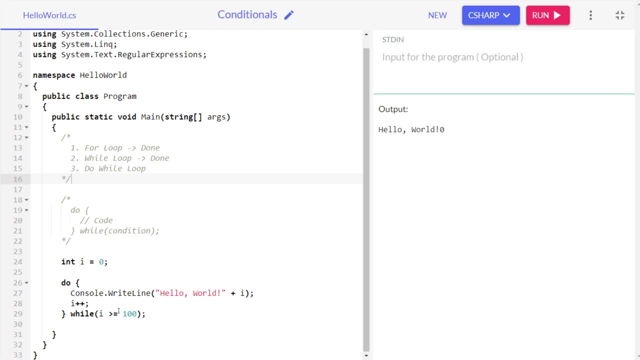 Even though the condition is false, it at least executed once. All right. So that's what? All right, That's what I do. That's what a difference between do while and while loop is All right. And see, you won't be using this do while loop much. 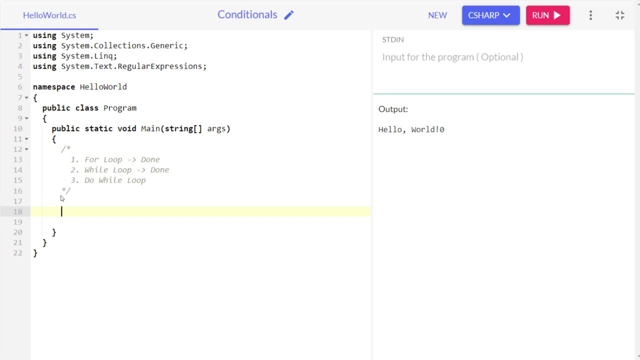 I'm very sure of that because, even like I've been like using Unity engine for almost four years- Yeah, So it's been almost. I started in 2019 and it's been almost four years I've been using Unity engine and it's been more like almost two years. 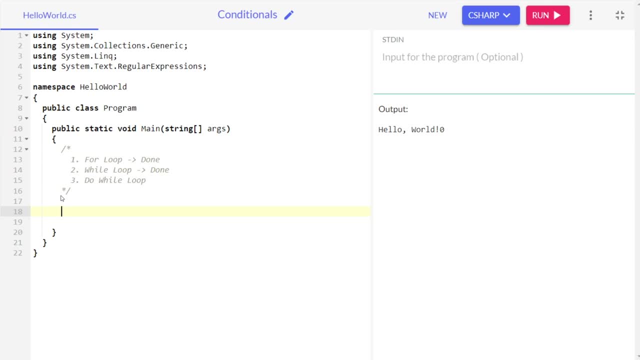 All right. I guess two to three years I've been doing augmented reality development, All right. So here's the thing. All right, I have never used do while loop. All right, I have never used do while loop while developing games or AR applications. 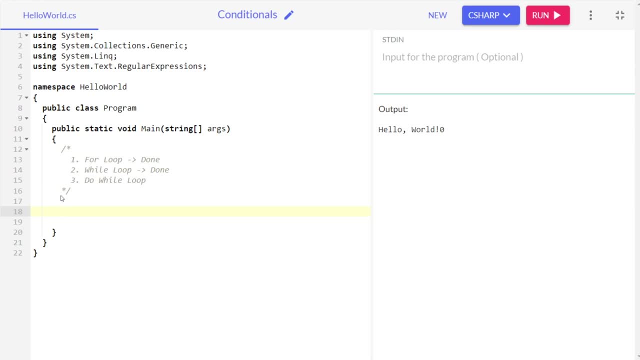 So Maybe in your case you might face, you know, some moment where you have used, where you should use or can use do while loop. So it's totally, totally OK, All right, But in my case I never used do while loop in my development journey. 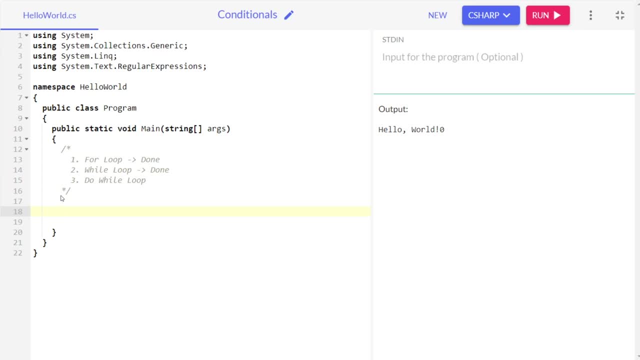 So yeah, that's it. Now. here's something you know last. All right, Here's the last concept we are going to learn in this: conditionals. Oh, sorry, Not in this. I guess I forgot to change the name. 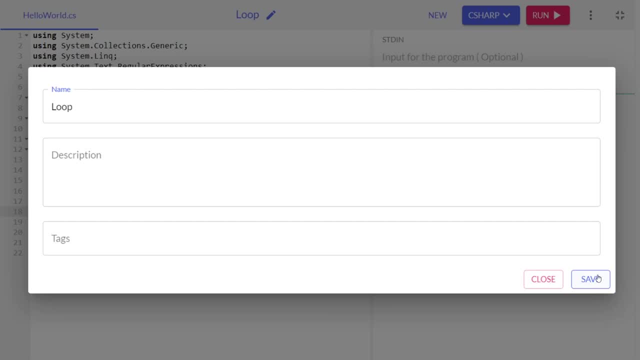 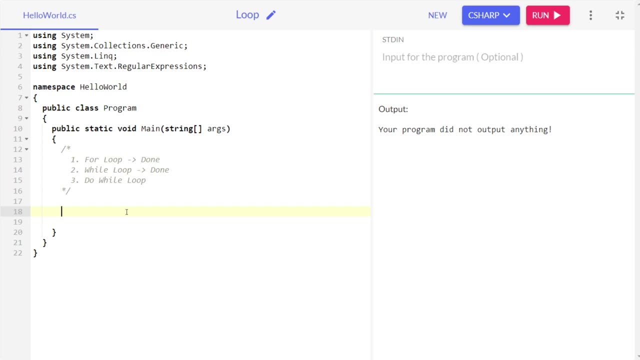 Sorry, I'm very, very sorry, So I'm going to change the name. So in this looping- All right, In this loop concepts, we are going to learn this last thing, that is, jump statements. All right, There are multiple jump statements. 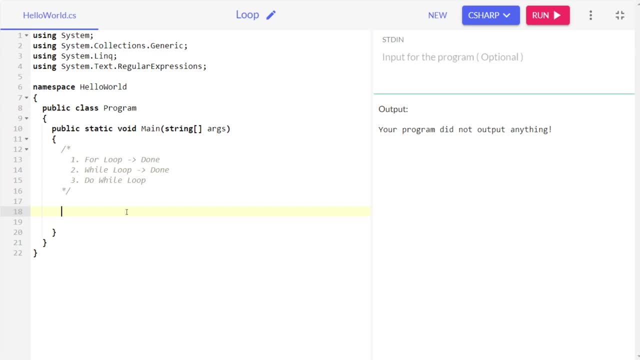 C sharp like there's go to, there's break, There's a continue statement, Then there is return statement- All right, Then there is throw statement, But in this particular lecture we're going to learn about only two of them. That is continue. 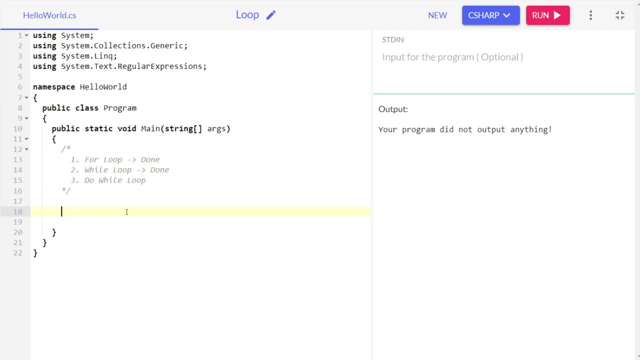 Continue and break statement. All right. So they're very simple. All right Jump statements. Basically now they are a statement. All right, Jump statements are basically a statement that instructs the flow of a programmer. that instructs the program to deviate from its normal flow sequence and jump to another line of code. 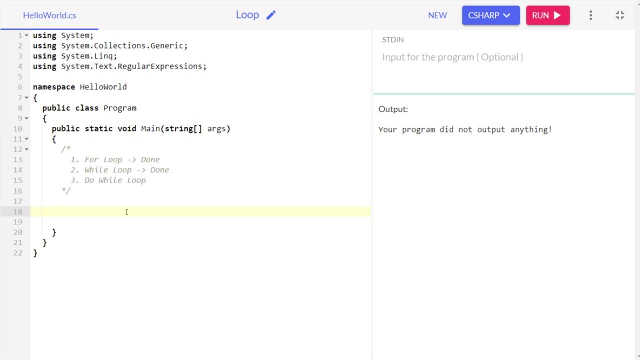 All right. So jump statements are commonly used in loops and other control flow statements. All right, You will also, you know, use this in a switch case statements, often in, if else, statements. All right, So let's see what are these. 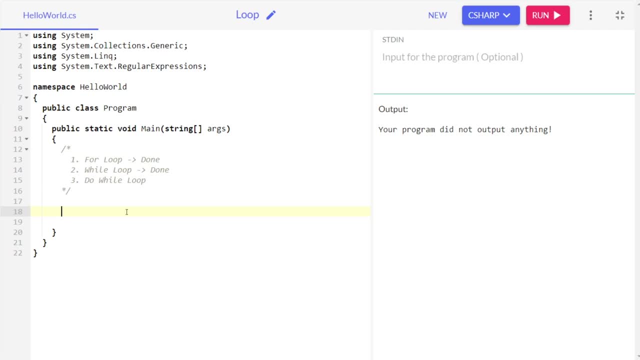 So, first of all, let me show you, Let me tell you, which statements we're going to learn today. All right, That is break. All right, We're going to learn about break and continue. All right, We're going to learn about break and continue. 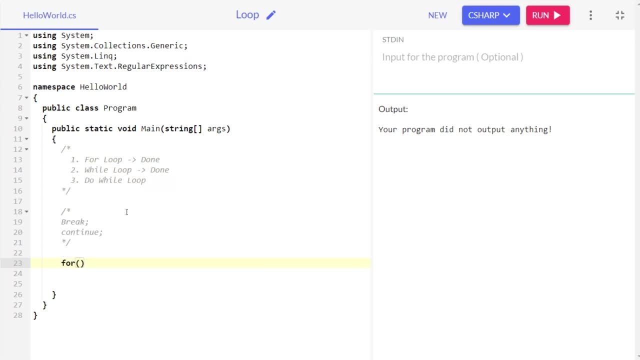 So let's implement it. So I'm going to use for loop for this. All right, You can try out with while loop. do while loop anything you want, All right. So I'm going to create a for loop. All right, I'm going to iterate. you know, iterate this for loop over up to 10.. 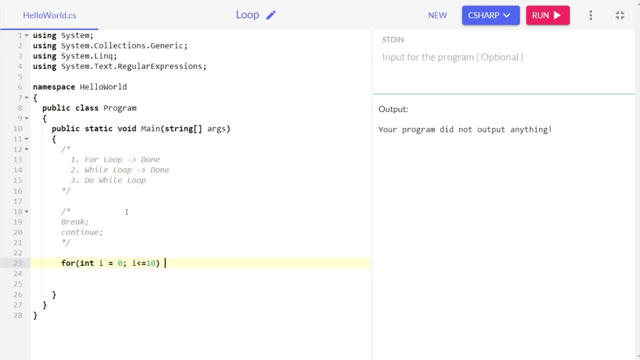 All right, I'm going to iterate this for loop to 10.. All right, Now what I want to give a condition. All right, Let's say I want to print, I'm I'm printing, all right, All all the numbers in here. 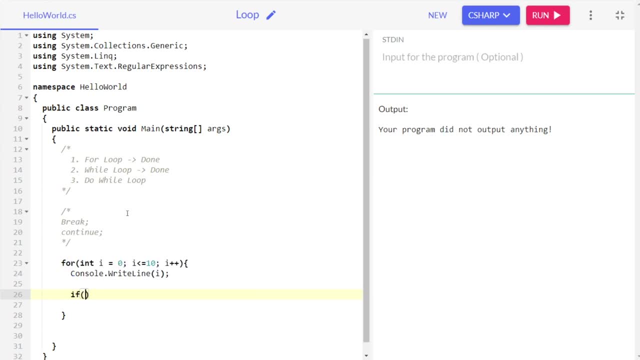 So I'm going to print all the numbers in here And now what I want if? all right, if I. if I reaches to seven, All right, If I reaches to seven. What I'm going to do is if I reaches to seven. 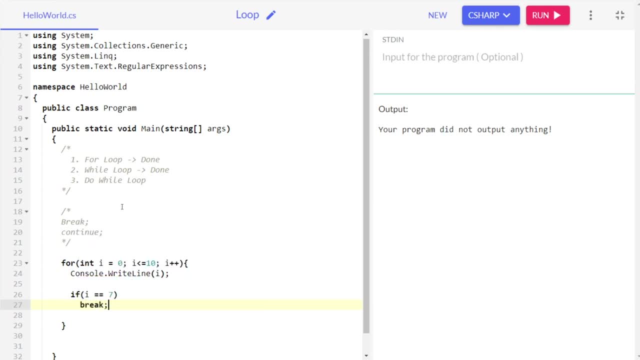 What I'm going to do is I'm going to break. All right, I'm going to break, So let's see if this works or not. See, it didn't print it, It broke. it broke the program, All right. After I reached to seven, it broke the program. 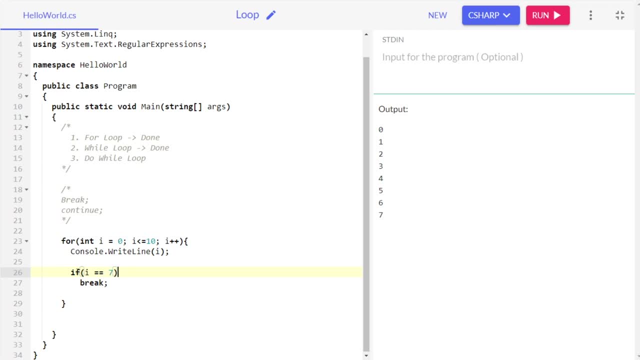 All right. So that's what it is doing now, basically a break statements. now, after reaching some point, a break statement helps us to terminate the whole program. All right, That's the whole point of break. All right, That's the whole point of break statement. 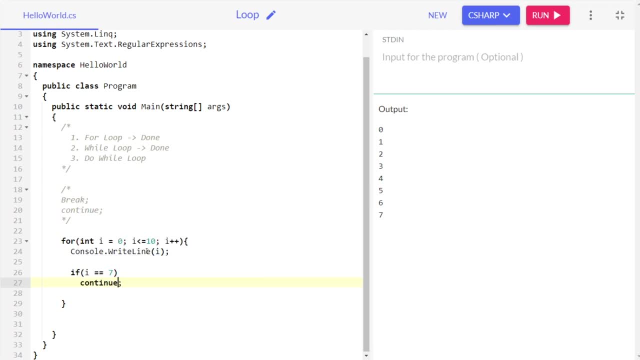 Now here comes continue statement. All right, See, continue statement is a bit different. It will actually keep that particular value and move to the next value. Let me show you. All right, Just give me a second, So you guys might be thinking. 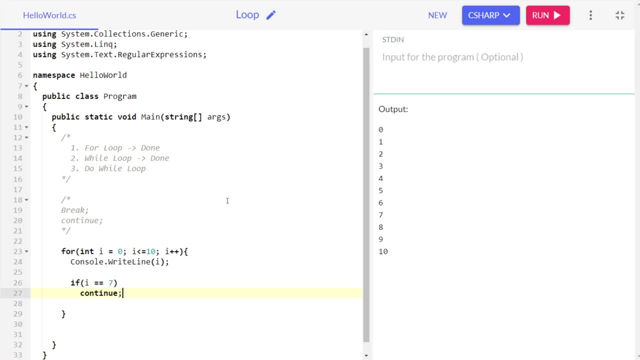 All right That I told you that continue statement skips some part, right. It skips some part and then moves to the next one, All right, But here in the output it didn't happen. Right Because? all right, because here you can see before the if statement: 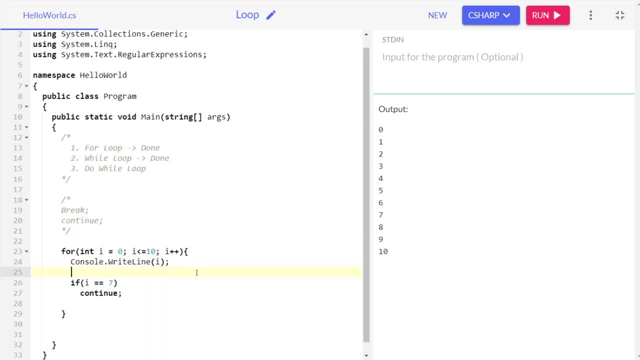 this console dot write line is being executed, So in this case it already had printed seven. Then how is it going to skip If it has already printed it Right? So That's why to actually use the continue statement in this case. 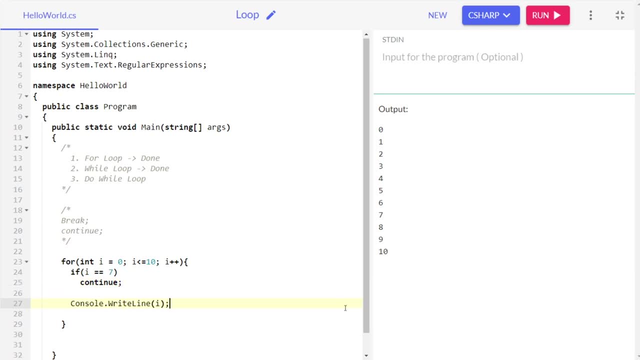 what we do is we, first of all we check for the condition and then We write console, dot, write line. and now, here you can see that we are able to print up to ten by skipping or by skipping, number seven. All right, So that's how this whole looping 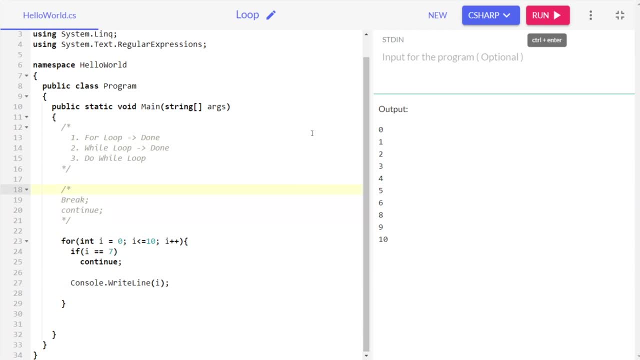 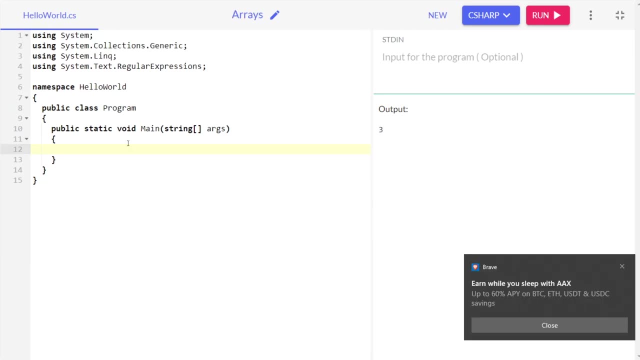 works. All right, And I hope this concept is very clear to you. All right, So yeah, that's it for this lecture, So see you in the next lecture. Thank you, Hey guys, welcome to this lecture, And in today's lecture we are going to learn about arrays. 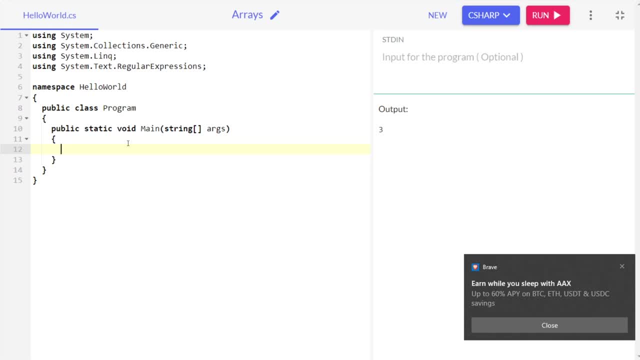 All right, Arrays is a very important concept. All right, It's a very important concept in C-Sharp or any other programming language. So, like, buckle up your belts and see tightly, because It's really important for you To understand the concept of arrays. all right, because when see at this stage, all right. 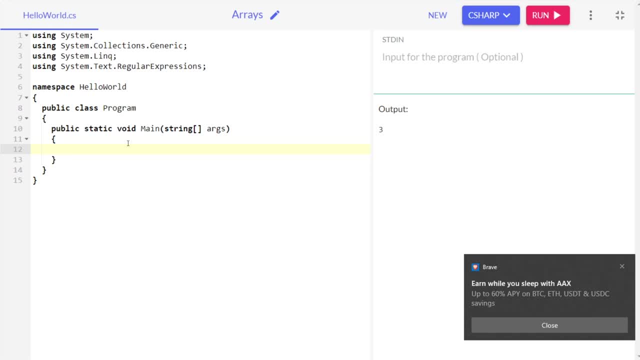 at this stage, in the beginning stage, you might have very less use cases for array. Even actually in the beginning stage also, you'll be using arrays more often than you know. So what I want to say is: let's say, take for an example in augmented reality only. 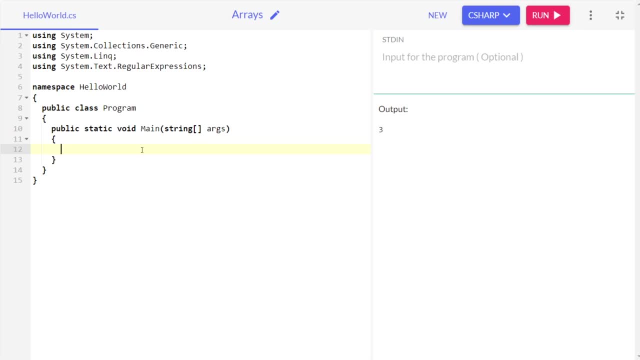 All right, We we use arrays in a lot of things. All right, We can we like in plane detection when we want to, like you know. let's say we want to place all right, place multiple objects into the real world. All right Means in Markerless AR, whenever we want to try to, let's say 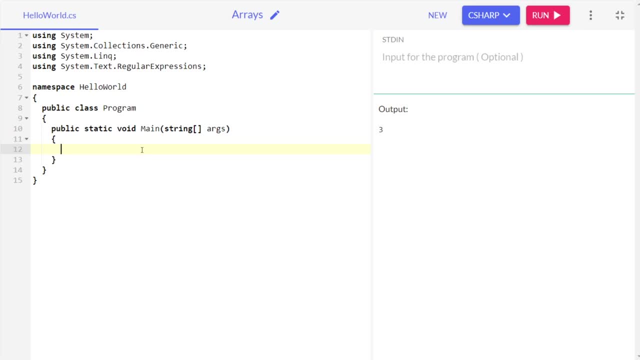 place multiple objects in the real world. we create an array of these objects so that we can, you know, place them in the real world. All right, So you are going to use arrays in Everywhere. All right, So it is one of the very important concept. 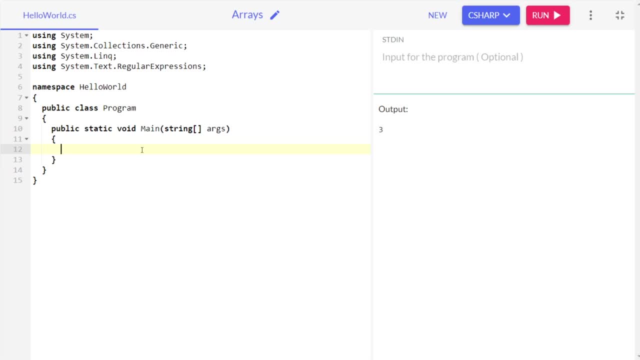 So let's dive into this topic, All right, Without waiting anymore. So see, in general, when we store values, we use a variable, All right, But there's a problem. All right, The problem is. the problem that comes with it is that we can only store one single. 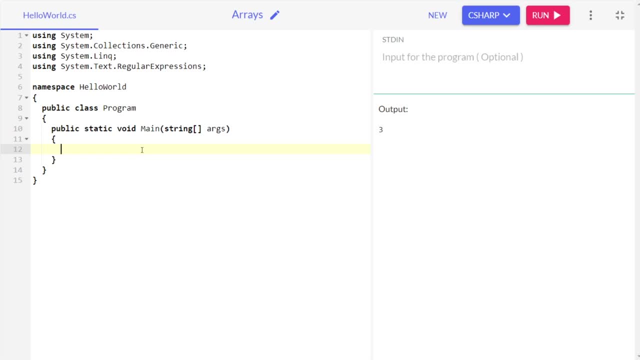 one single value, All right. We can only store one single value. We can't store multiple value, All right, And that's a problem. If arrays, or arrays, or lists, or they, wouldn't have been there now, then we wouldn't have been able to, you know, store multiple values in a variable. 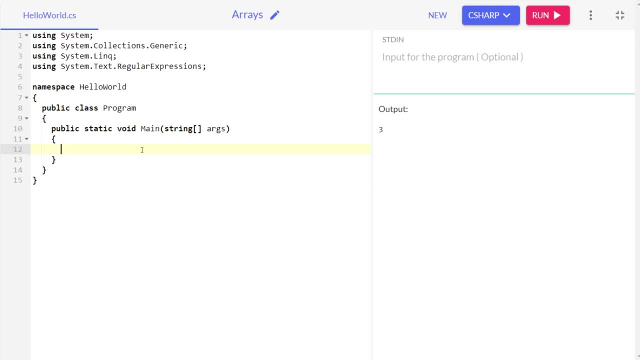 All right. So what arrays does is arrays actually enables us? Arrays actually enables us to store numerous number of value of any data type, or it can be of string, It can be of integer, It can be of double, It can be a float, All right. 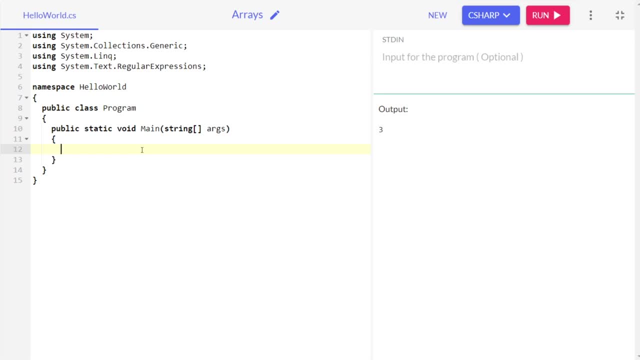 Can you have care So they help us already, provide us a technology so that we could- now we could- store multiple values. All right, We can store multiple values within one single variable, All right. So that's how we use And, sorry, that's what is an array. is an array in simple words? 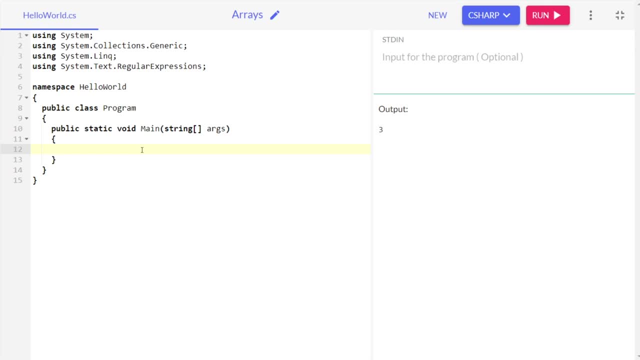 All right, An array is a collection of data. All right, It's simply a collection of data. All right. Now, as we have learned about what actually array is, let me tell you about the agenda of today's lecture. So today we are going to be going to the very basics of array. 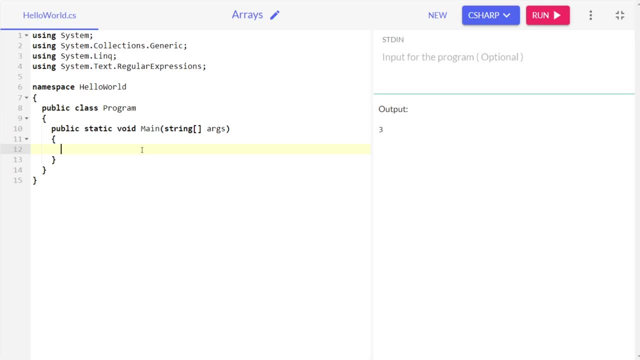 All right, That is, we'll be learning how to initialize an array. Then we'd be learning how to access values within an array. All right, Then we'd be learning about some different, different methods, All right, Available in an array. 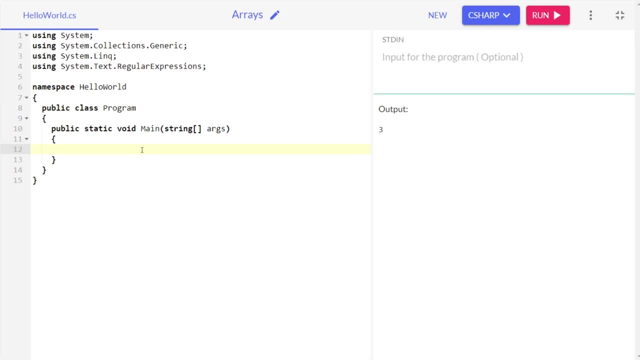 All right, So let's get started. So the very first thing is that we have to understand how to, you know, Implement an array. All right, See, there are two ways of implementing an array. Let me first of all not in common weight. 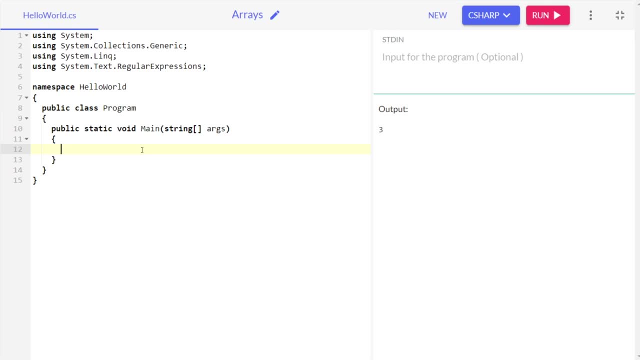 So let me show you. All right, There are two ways. One is a dynamic way and the one is a static way. All right, I would tell you why they are called those. All right, First of all, let's try out the dynamic way. 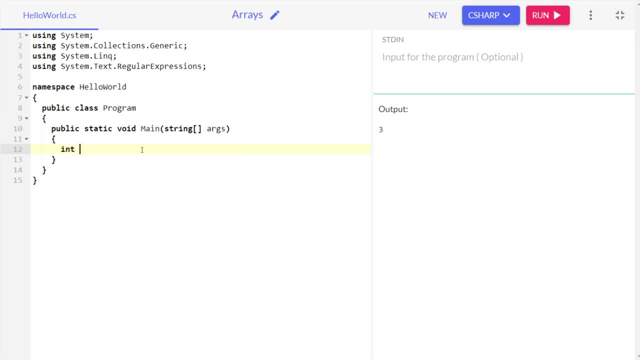 So the first thing, All right. See, whenever you declare a variable, how do you do that? So you can say: int val equals 12.. Right, You declare a variable like that Now when creating an array, or when creating an array. 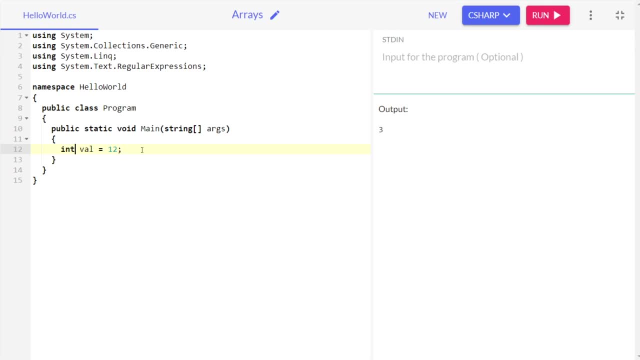 Make sure, All right, That you don't miss the square bracket. way to put the square brackets. You have to put the square brackets after int variable, All right, You have to put the square brackets after int variable. After that, This variable: All right. 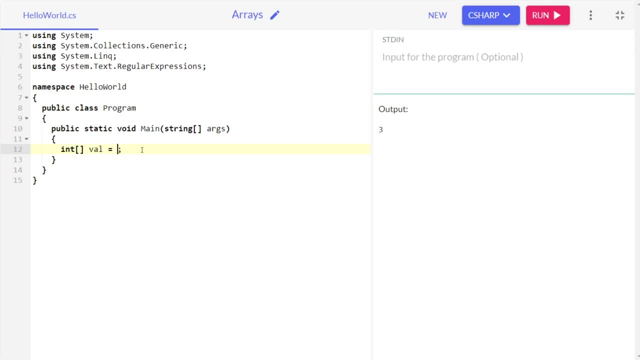 This variable you created would be Considered an array, All right, Will be considered a variable that can store arrays. All right, Now to store arrays, What we have to do is open curly braces, All right, And within that curly braces put some values. 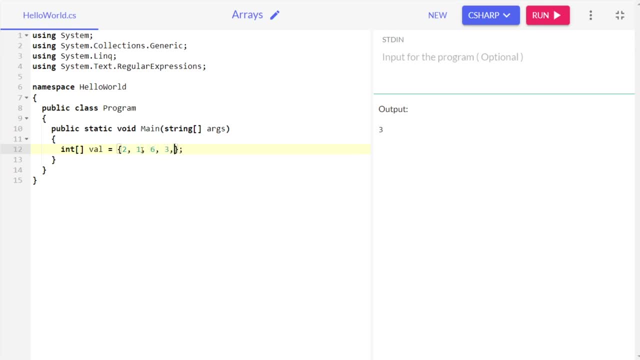 All right, 216,. let's say 3, 4.. All right, So now let's run it and let's check whether it's returning us any error or not. All right, So here you can see it is, It's returning us. your program didn't, did not output anything. 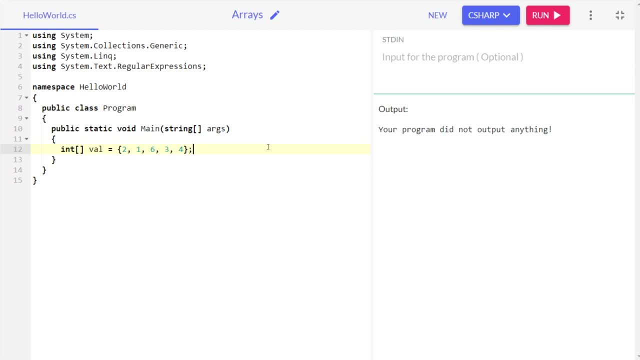 All right, Don't worry about that. All right, Because we actually haven't printed anything. I would show you how to you know how to print each and every value within an array, Right? So don't worry about that. So this is one way. 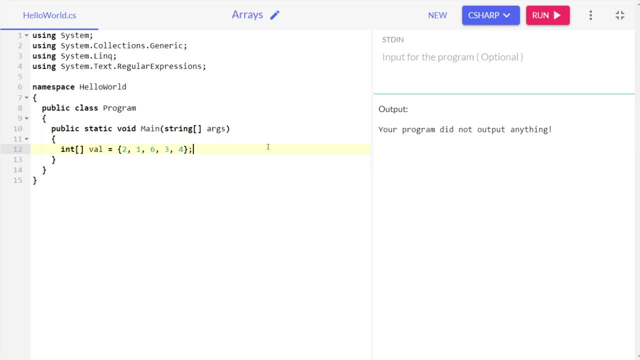 All right, This is one way of you know initializing or creating an array, And this is known as dynamic array. All right, Now The other way around in creating array is you have to again for the same thing, that is, in square brackets, then give the variable name. 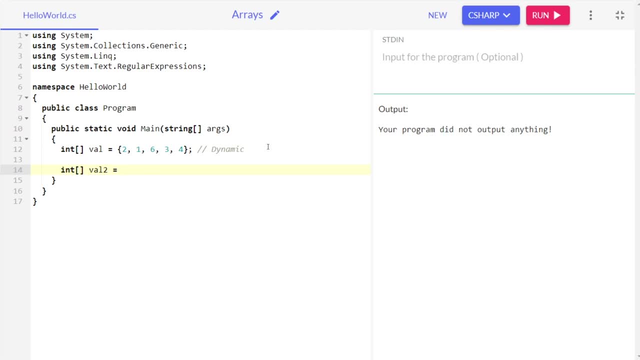 All right After that. All right After that. what you have to do is you have to write a new keyword. All right, Then int, Then again square brackets. Now, this square, this square bracket, has a special meaning. 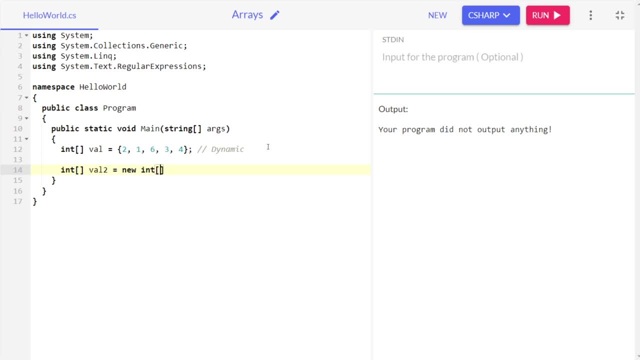 I would. I would tell you All right, So. So what is the meaning? See, there's a reason why we call this type of array and static array. The reason is we already all right from the start, only when we declare the array. 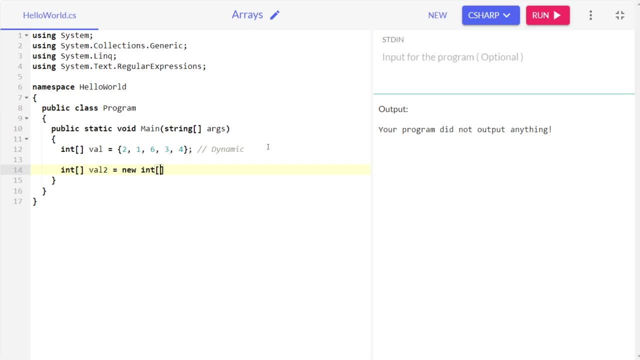 All right From the start. only, we specify the size of an array. That's what we are doing right now. So in this square brackets, we have to give a size of an array. So let's let's give it five, All right. 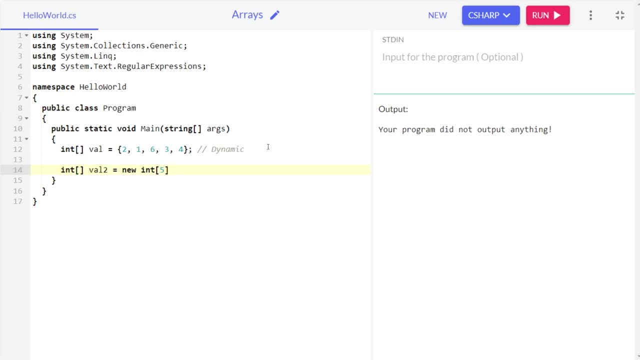 So now, this is a static array. All right, This is a static array, It doesn't have any value in it. It means, of course, it does have. All right, It does have value in it, But, All right, But it is static. 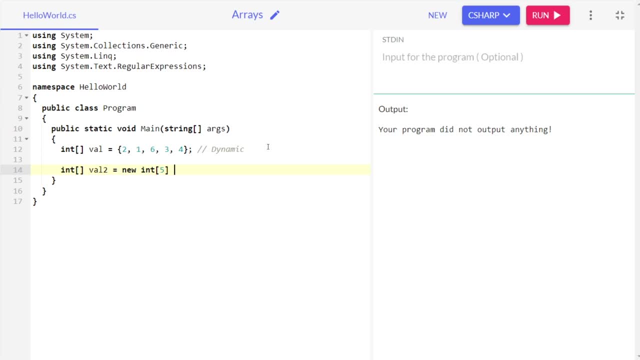 The reason is we have already. all right, We have already initialized this array. All right, We have already initialized the array. And because we have already declared the size of the array, because we have already declared the size of the array in the memory, 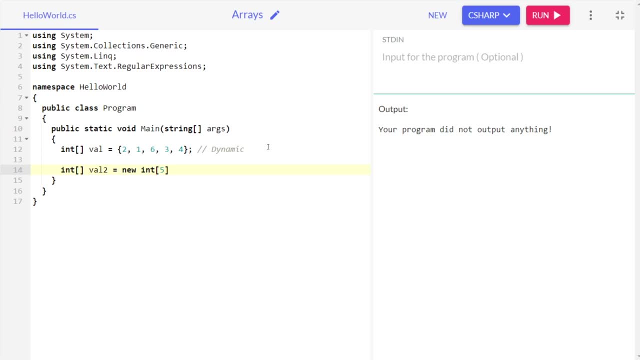 All right. In the memory, it has created a static space, or in the RAM, it has created its own memory that cannot be exceeded. All right, So that is it. Now. after after this whole bracket thing, what you have to do is again open your curly brackets. 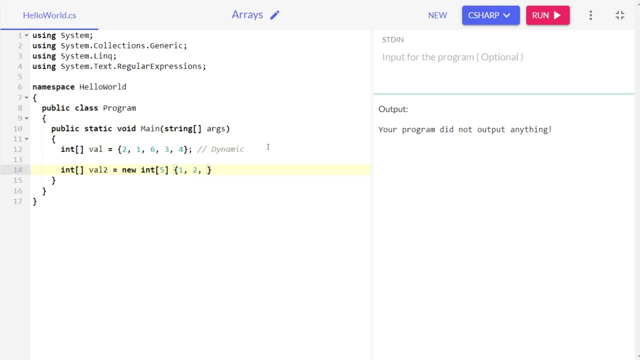 All right, And after that Write the number you want to give. All right, So yeah, that's how we declare a static array. All right, Now let's again, Oh, run it and let's see if it's returning any error. 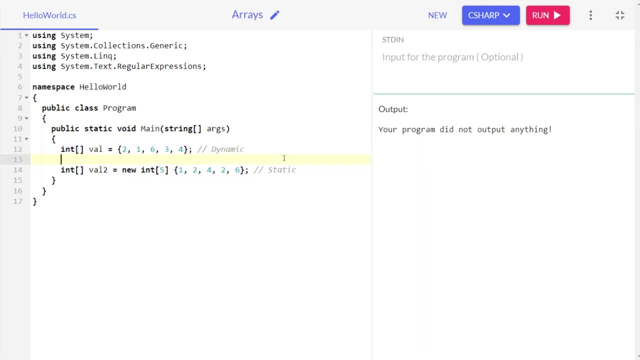 No, it's not returning any error because the syntax is totally correct: All right. Now see The difference. now, the difference between both All right, Both dynamic and static array. All right Is basically. It means: now see. 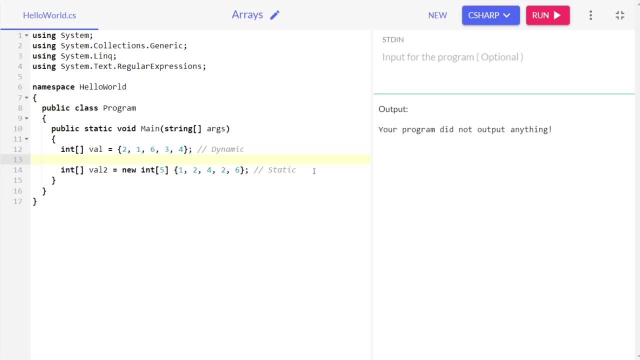 Static. why is it called static? Why Something is called static? Static means which can't be changed afterwards, All right, Which we can't change afterwards. What if it is declared on the start? it is declared declared, All right, We can't actually change it. 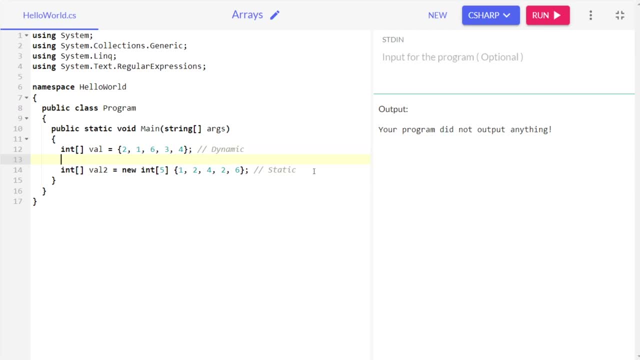 Or we can't actually add something more up to it. All right, We can't exceed that memory, All right. But dynamic means it is. you know what can I say? It is adjustable in the runtime. Dynamic is adjustable in the runtime. 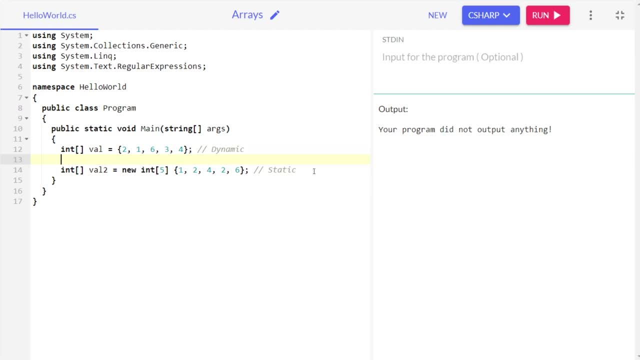 That is what the you know. That is what the difference is Between dynamic and static. All right, I hope you are clear about it, All right? So yeah, so I'm going to keep working with dynamic arrays only, All right. 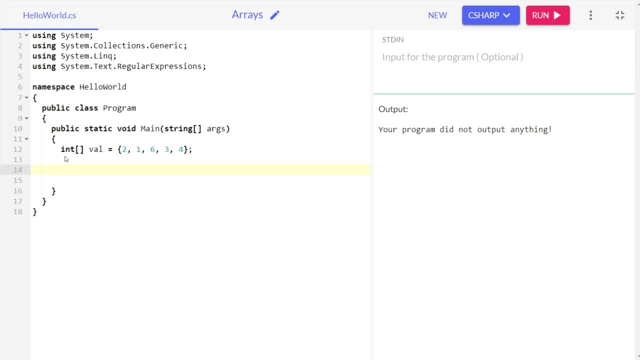 Now, Here's the thing. all right, so we have learned about initializing array. We have learned about what exactly is an array. All right, Now let's learn about accessing values within an array. Do you remember when I taught you about the window in the second lecture? 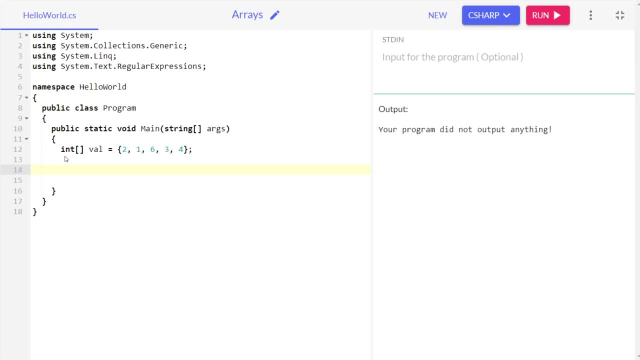 Only I taught you about indexing. All right, I hope you remember the concept, All right. But if you don't, let me tell you indexing Now it defines, all right. Indexing basically defines positions, positional value of some data. All right, In simple terms, it means all right. 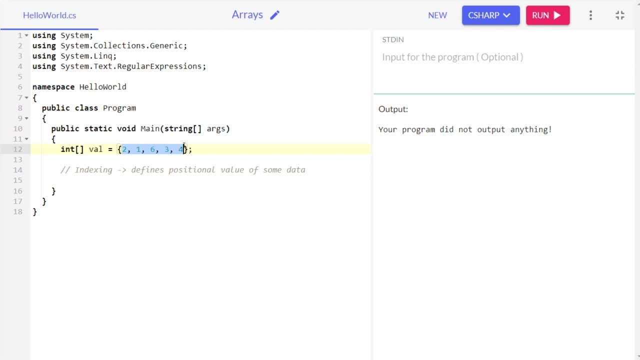 It means, let's say There are how many, how many elements are there in this? you know how many elements are there in this particular array? There are a total five elements, All right, And if we start indexing them, all right. 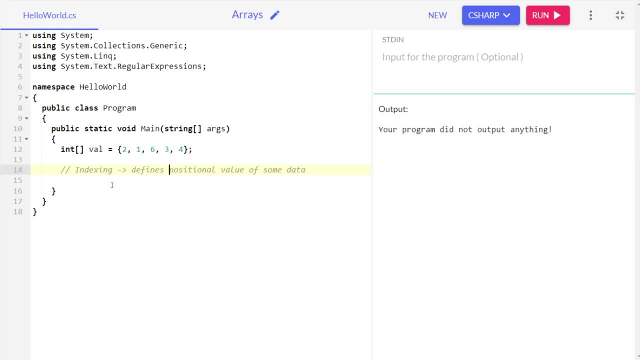 Indexing in in. in simple words, you can, you know, you can understand indexing as basically address, all right means exactly. if we talk about memory address of any variable, it's totally different or it's totally different. I'm just trying to make you understand how, like what is indexing with indexing? 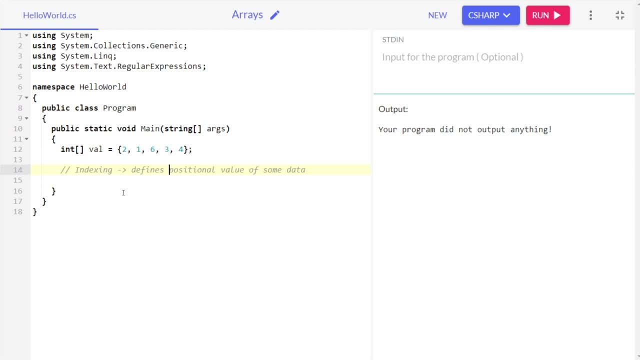 It's a think of it as an address of someone All right, Like, for example, I am Priyanshu, All right. There are two Priyanshu Right And both live, or both live in two different, like two different places. 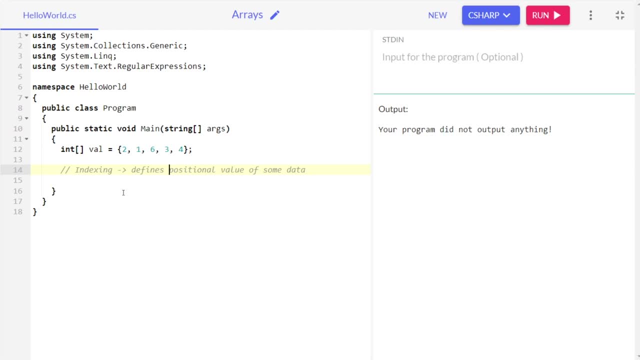 All right, But both are Priyanshu, Both are means whose name and title are totally similar. All right, But how will? how will we know that Priyanshu means the Priyanshu he is finding is the actual one? 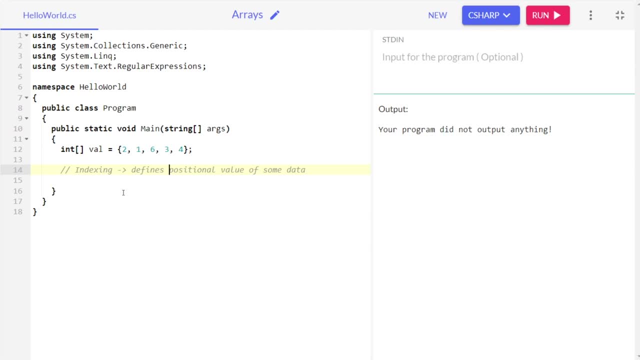 All right. So that's how address comes in. All right, The person will ask for the address and if the address is get to the right, Priyanshu. So basically now, indexing is basically the positional value of some data. It's simple as that. It is the address of some data. 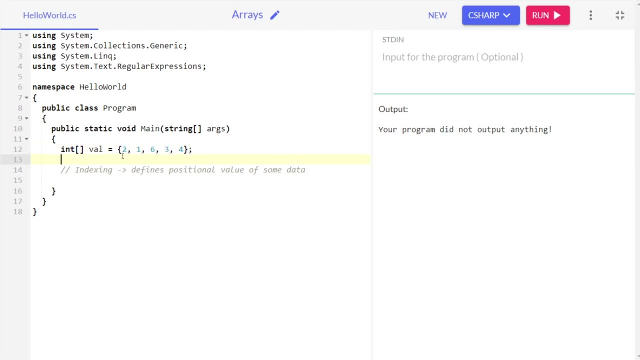 Like see for two. for the first element or the first element of an array, The address is zero Means in the index value of first element is zero, The index value of second element is one, The index value of third element is two, And it goes like this: All right. 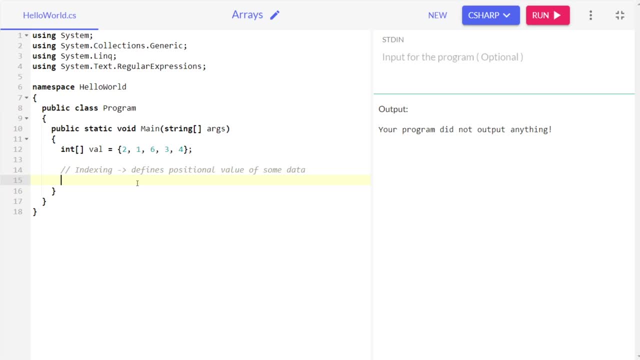 It always goes like this. So that is what indexing is And this is how indexing will help us accessing the value. All right, Now, let me show you. So, let me show you by printing it. All right, So I want to access. 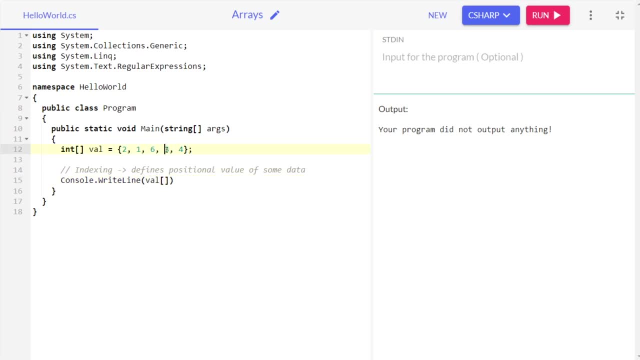 All right, I want to access, Let's say this, All right, Three, Three from the array. So how would I do that? So let's count it. So, as it is starting from zero, Zero, one, two, three, All right. 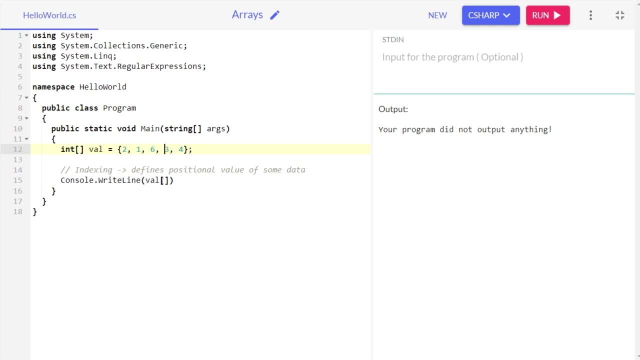 So this is in the. it is in the third position. So what I'm going to do is I'm going to write three in here and let's see if it works. Yeah, we got it Right. We definitely got it, because the positional value of three 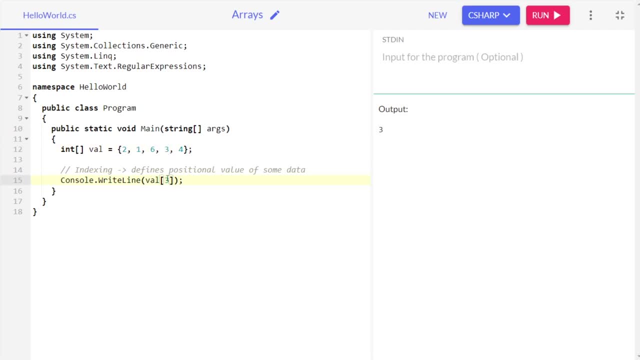 Sorry, the positional value of three is three, Right, So if you are confused, all right, let me. let me give you another way around. All right? So let's say I want to, you know, access this, All right. 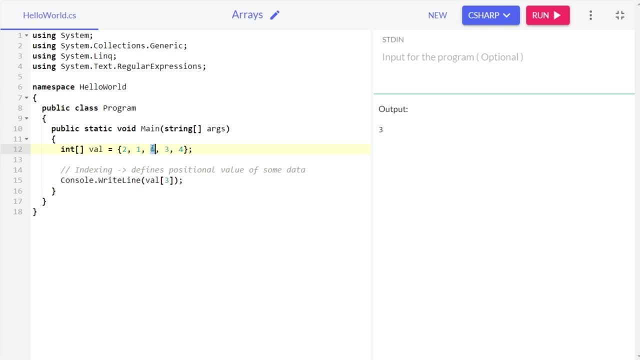 This particular value already means I want to access the six. So how would I do that? So let's count it: zero, one, two, So it is in the second position, Right. So now let's run it. So here you can see we are with the index. 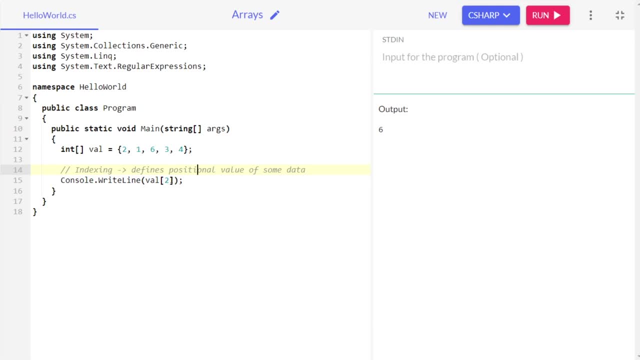 All right, With the help of index value, we are able to access it And always remember. Whenever you want to access index value. now write the variable name, then open square brackets and inside that put the index value. All right, So this is how we access. 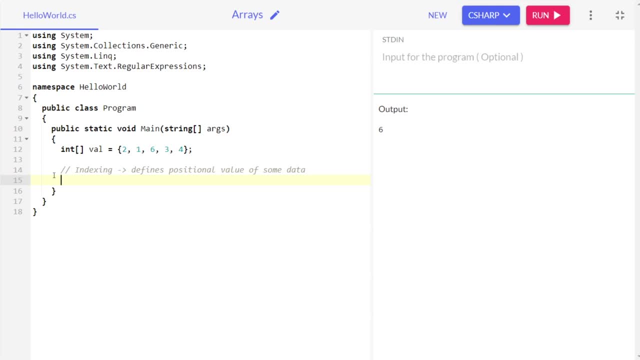 All right, This is how we access values within an array. Now, let's say, if we let's say, I want to print, All right, Each and every element within this array, All right, I want to print each and every element within this array. 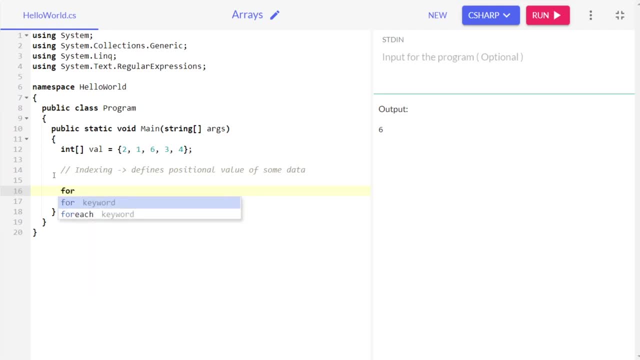 So what I'm going to do is For in type equals zero, I less than equals. All right, How many elements are there? One, two, three, four, five, Right? So what I'm going to do? less than. 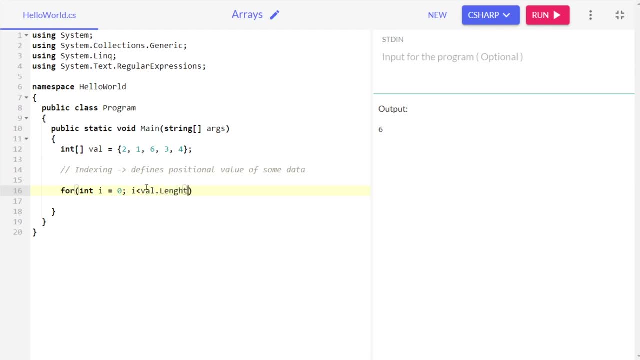 All right, Val dot length. All right, See, this is a method. All right, You already learned your first method. All right, Dot length. All right, See this dot length method. Now this length method returns the total length. 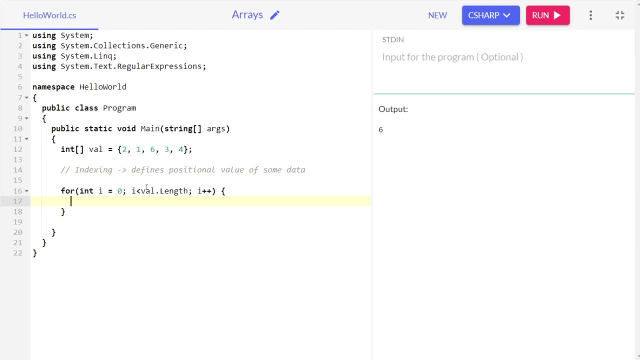 All right, The total length Of your array. All right. So, as our total length is, you know, five, that's why it has returned five. Now, here comes the problem. Here you can see what I've written in type: equals zero. 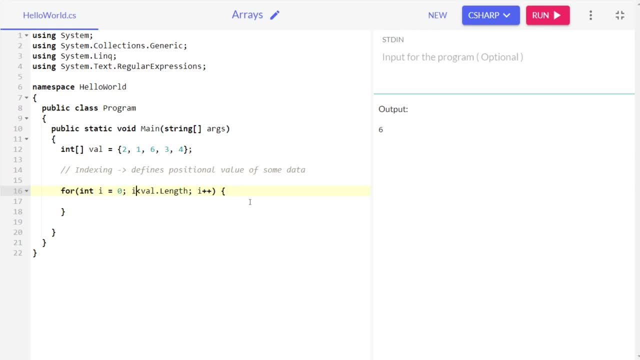 I less than means it will iterate less than five. All right, Do you know why it is ideal and why this solution will work, and why Why not less than equals will work? Actually, it is better to try by yourself. actually Pause this video. All right, Pause the video. 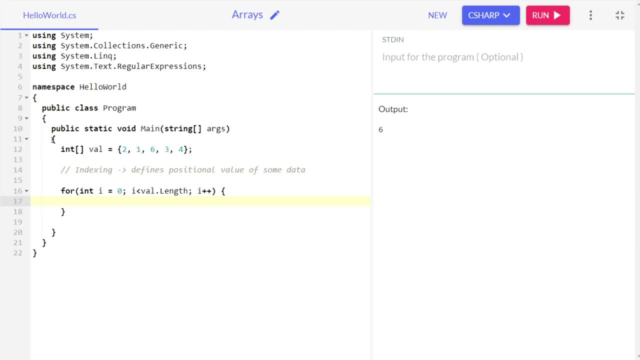 Try both the, both the way. All right, Try both the way and check which one is running. All right, I will show you right in here. Just give me a few seconds. So now, as we have you know, try to access, as we are trying to access the values. 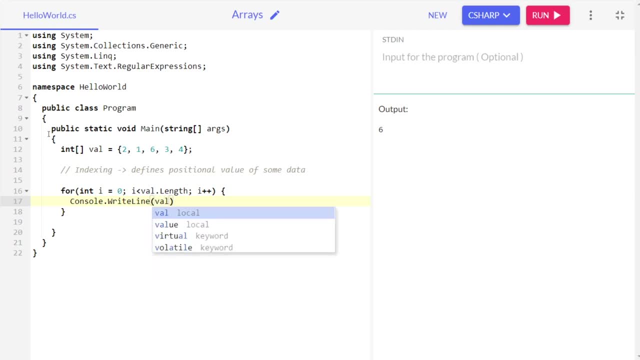 again every value. what I'm going to do is I wrote console dot, write line. Then I'm going to take the variable name, the square brackets, and I'm going to put the I inside it because you know, with every iteration the value of I is increasing. 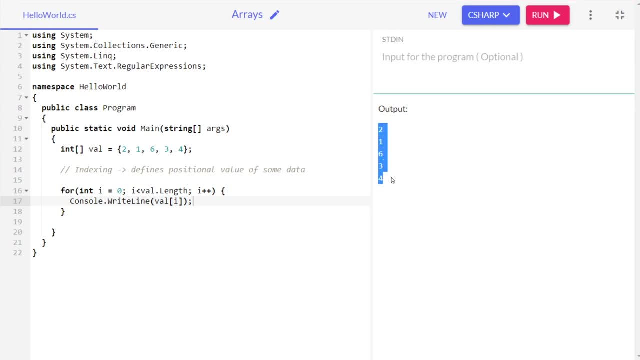 All right. So here you can see, we got all the elements. We got all the elements because we started from zero- Zero is this one, All right- And ended with four- All right. And the fourth positional value is of this one, Right. 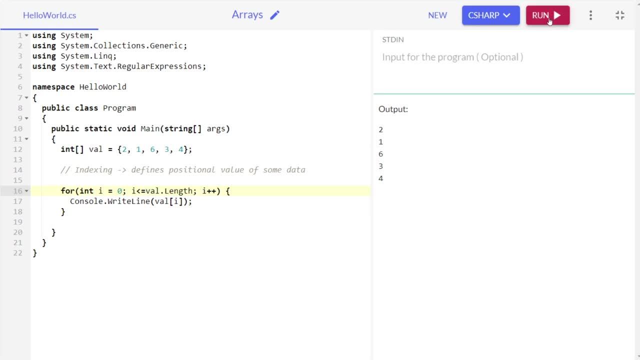 Now let's try out. less than equals one. Let's see what happens. Let's see, See, it has printed, but here you can see it is returning us error. Now what's the error? index was outside the bounds of an array. 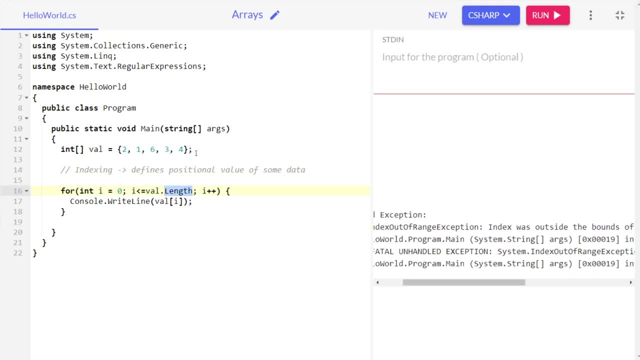 The reason is: the reason is the length of an array, or the length of an array is five, All right, The length of this array is five, But Indexing ends at four, All right, And we are trying to access the elements of. we are trying to access the elements. 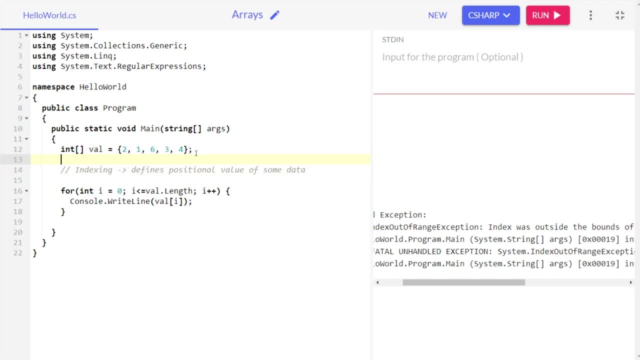 of this array through indexing. So if there is all right. if there is no element present, if there is no element present in the fifth position, all right. if there is no element present in the fifth position, then of course it will return error because it doesn't have any value. 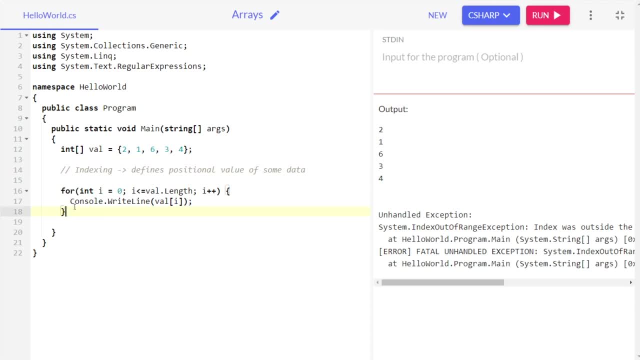 All right, Now here's a fun fact. All right, Here's a fact that you, you must know. All right, Like I guess I forgot to tell you about this, Like when we create this kind of array. now, just wait. 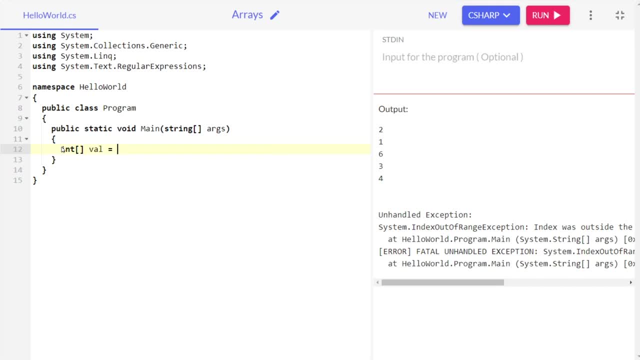 When we create This sort of array. All right, If we, let's say, if we don't assign values in here now, like I assigned previously, if we don't assign those values in here now, it will automatically like automatically zero. All right, Zero will be assigned to each and every position. 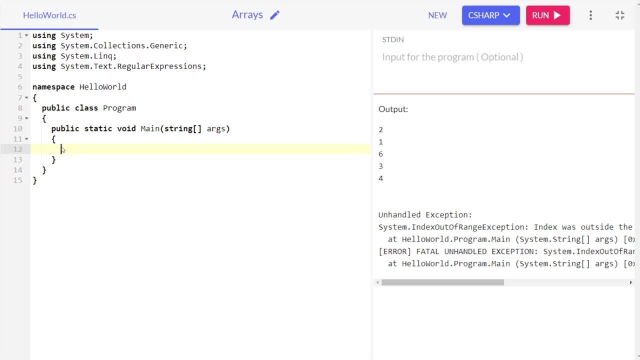 All right. So this is for a fact, And you guys must know it All right. So Now we have learned the very basics of array. All right, We have learned how to access elements in an array, Right. So now it is our time to look into the methods. 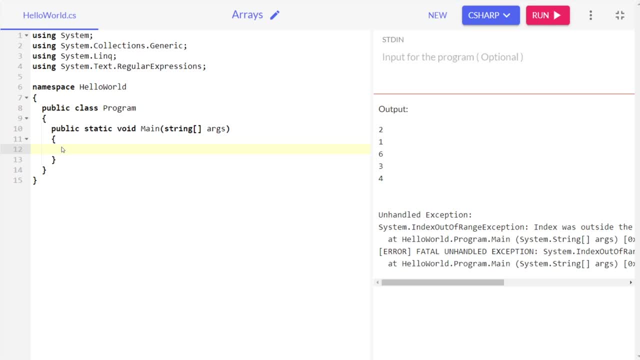 All right, The methods are present in an array. All right, You already saw. All right, You already saw method length. Now let me show it to you again. So here I am, declaring a variable that is int val. All right, 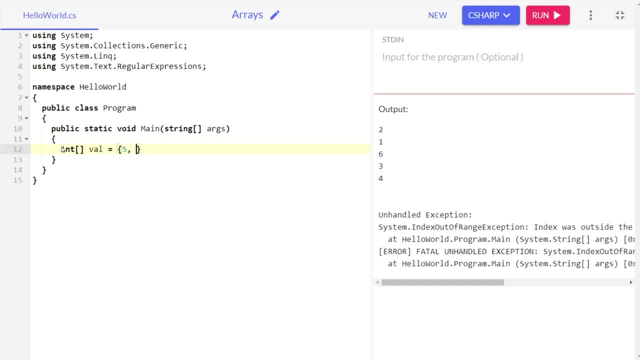 So int val, Then let's give it five to zero, A seven, let's say three, nine, eight. So here you can see: All right, We got, we created our own array. Now the first method we are going to learn about is length method. 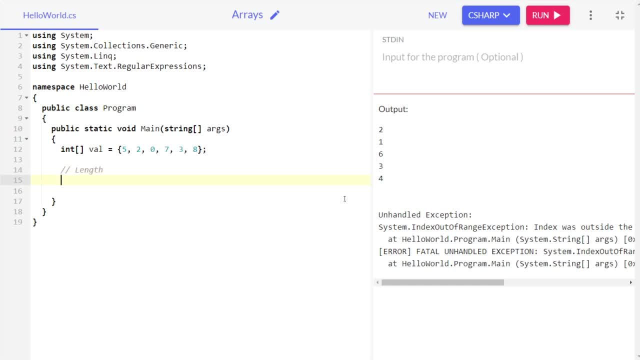 All right, And you, you already know what exactly is length, Right, How length method works. What I'm going to do is console dot right line, All right. So what this will do? it will return. All right, It will return us the total length of the array. 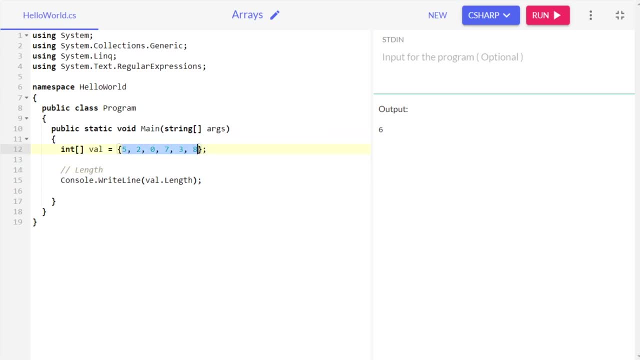 So here it is returning six because there are six elements present in the array. Similarly we have, let's say, we have another variable. All right, We have another variable, Not exactly a variable, Just just so. we have a variable of array. 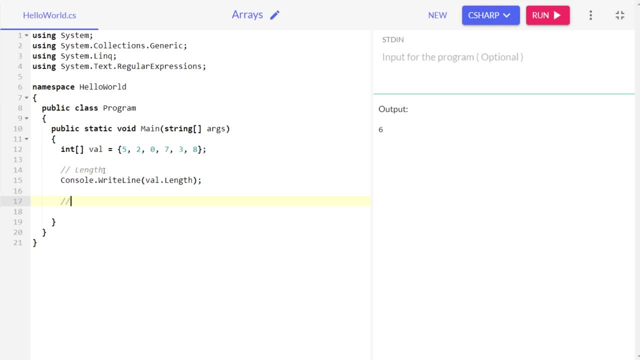 All right, So we have a variable of array. Now what we have To do is: now, what we have to do is we have to learn another function. All right, And that function is basically sort function. All right, See sorting, or sorting is basically rearranging. 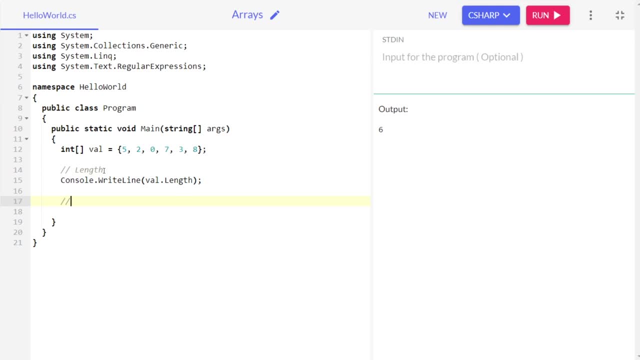 rearranging. rearranging- you know the rearranging, the values, All right, Means the gibberish values in an ascending order or descending order, All right. So that is what you know. sorting is All right. So here comes the function. 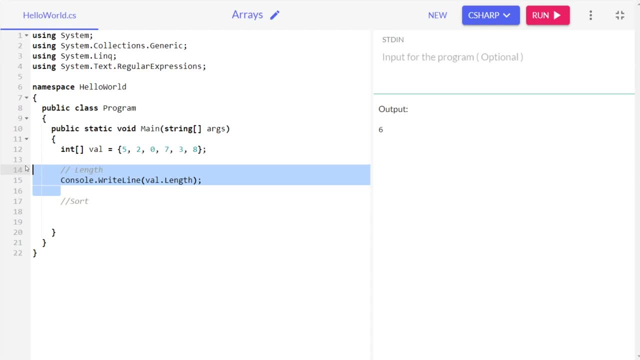 All right, So this is the sort function. First of all, let me remove this. This is the second one, because, of course, we don't need it anymore. Now, what we have to do is let me show you that we have, you know. 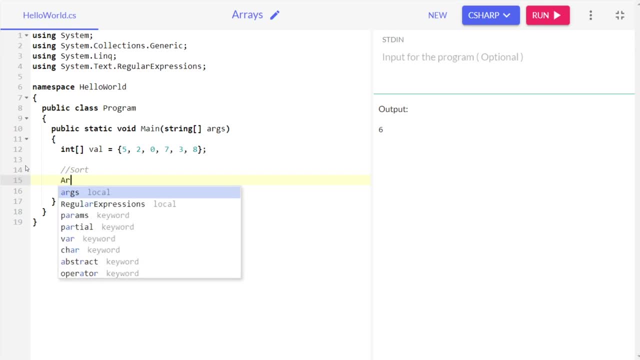 have an array initialized. now what you have to do is you have to write a function: array dot, sort. All right. And inside the sort function we have to pass an argument and that argument will be an array. All right. And now what you can do is for int. 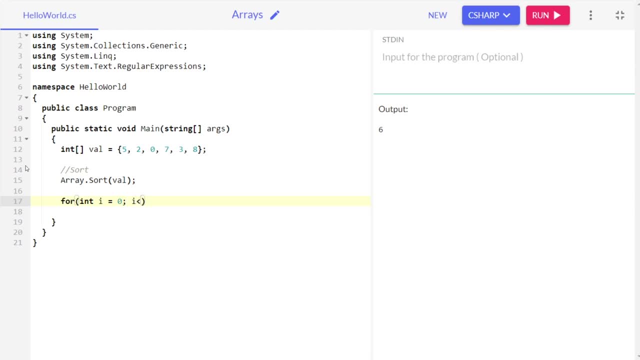 I equals Zero, I less than Array. All right, So not array. val dot length, I plus plus. All right, And let's try to print it. All right, Let's Try to print this value. All right, Let's let's try it out. 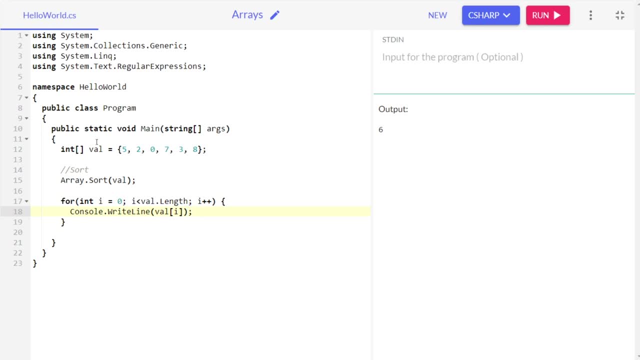 Let's see. Let's see what happens Currently. this is this: This particular array is not ordered. All right. And now to make it ordered, we use the sort function. So here you can see it has arranged. all right, It has arranged all the elements in an ascending order. 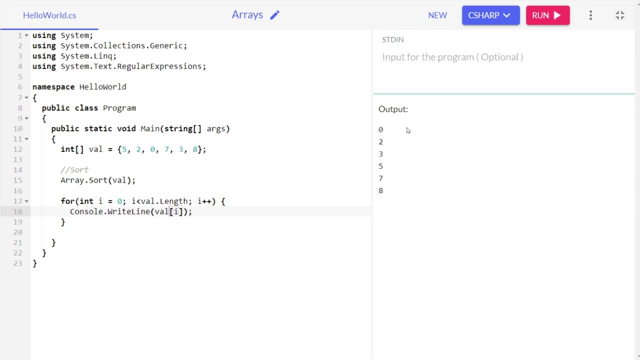 All right, So that's how this thing works. All right, So now we we are going to learn another function. All right, That is index of all right. This is index of function, that is, it will return the index of some value. 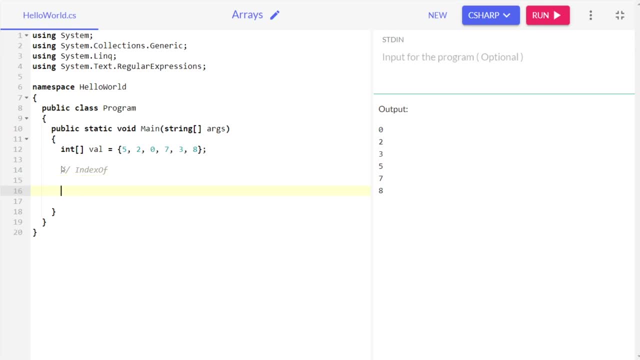 All right. So you already know how this works, Right? I guess I showed you previously. Means not in this and not in case of arrays. So int IDX equals array All right, Dot index of All right, And within that we have to pass two arguments. 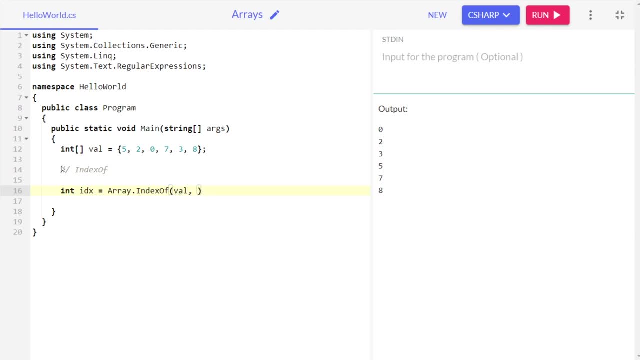 The first one would be the array- All right Means the array from which you are looking for the value, and the second one will be the Value means the value On which you will be taking out the means you have to put, the value of which you want to get all right means, which you want to get, in the sense. 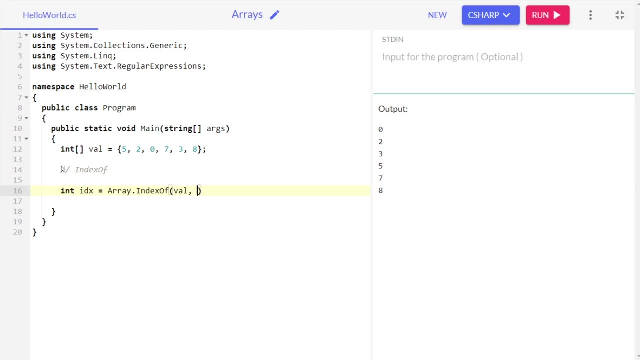 Let's say I want to put a value and I want to get index value Right. So that's what I will be doing. So I'm just going to put a certain value in here. So I'm going to put seven in here. 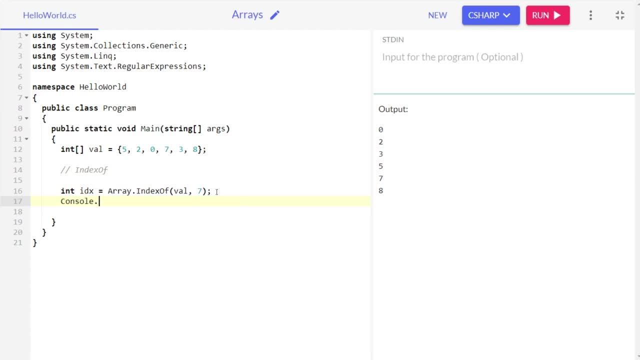 All right, And no, let's, Let's print it. All right. Console dot right line: IDX: All right. So let's run this program and let's see what happened. So here you can see: it is returning three. The reason is zero one, two, three, seven is available in index three. 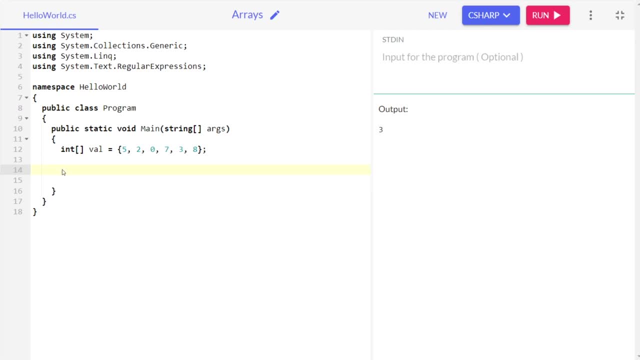 All right, So that's how this whole index of function work. All right. Now here comes three more functions already. that is maximum minimum, that is max min and sum. All right, So the meaning is hidden in their name only. So it's like the max function. 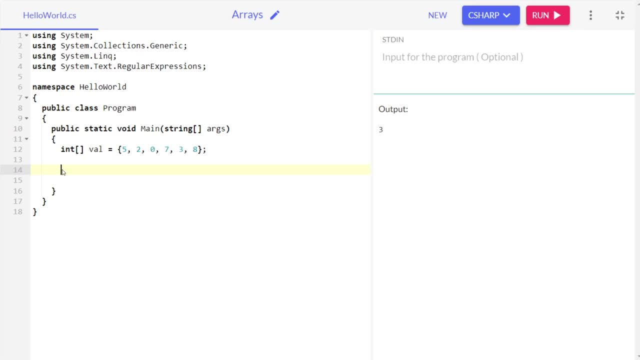 All right, First of all, understand this map function. Max function will return the maximum value available. All right, The maximum value available in an array: The mean. the mean function will return the minimum value available in the array And the sum. 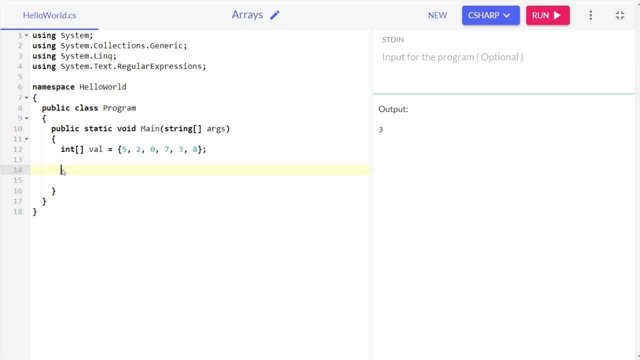 All right, The sum function will return the total sum of elements from the area. All right, So let's try to print it out. All right, So console dot right line All right, And inside this, val dot max and give parenthesis. 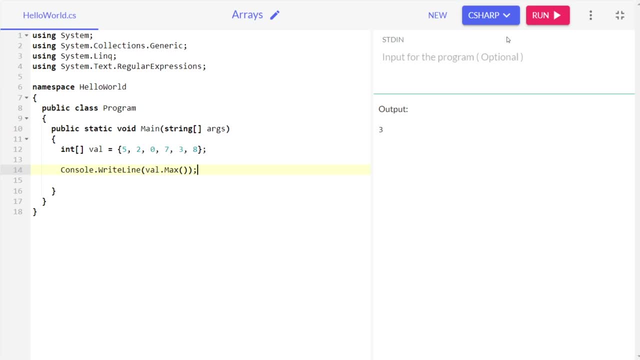 All right. So now let's see what is the maximum value in here. In our case, the maximum value is eight. Now let's see the minimum value. and that's totally right. And let's see the minimum value. The minimum value is zero. 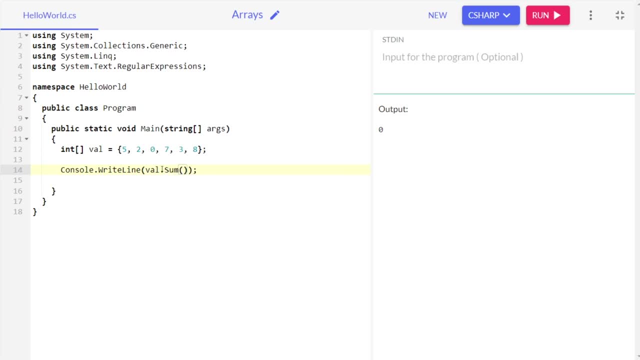 And that's also totally right. Now let's print out the sum of, you know, the sum of total array, So you can, if you want, you can, perform the calculation and you will be surely getting twenty five, All right. So. 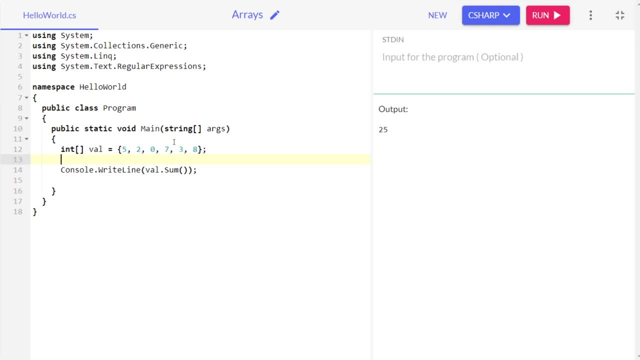 These are the array methods. all right that you must like, you must have an basic idea about all right and I would suggest all right, I would suggest you guys to look more into areas after this session. also All right, Because Array is a very important concept. 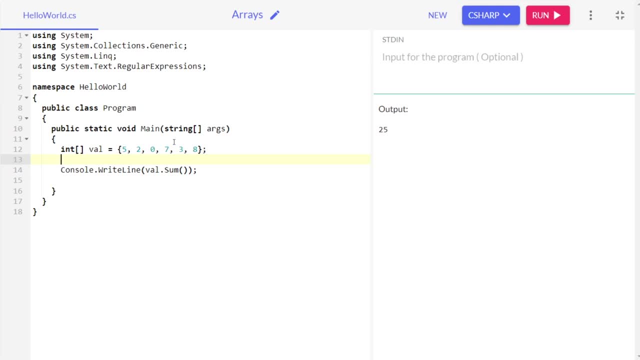 All right, And there are a lot of algorithms that works on arrays, like there are multiple sorting algorithms, searching algorithms- So I want you guys to have a very good idea and understanding of array, All right, So make sure you do that. And so, yeah, that's it for this lecture. 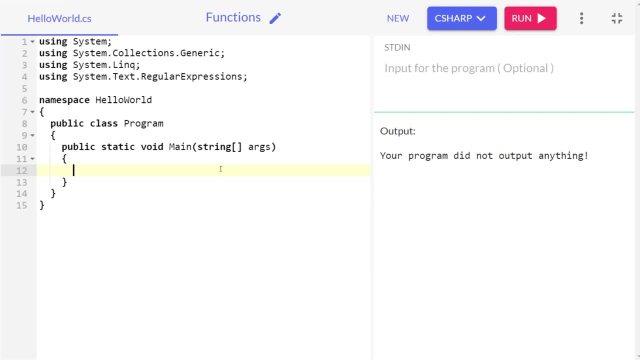 See you in the next lecture. Thank you. We are going to learn about functions in C sharp. All right. See, functions are a very important topic. All right In terms of programming. All right, The reason behind that is because functions helps us to manage our code. 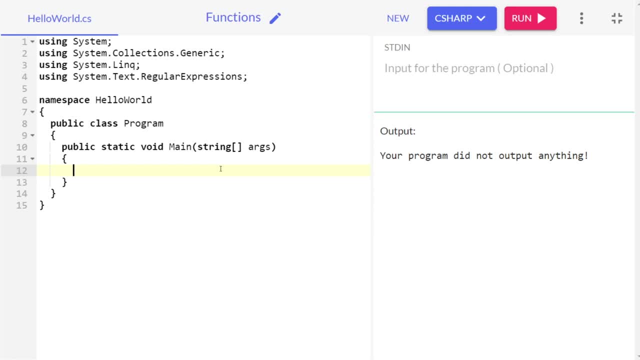 All right. It helps us, to you know, lower the number of codes we write. Function helps our function, helps us to keep our code clean, All right. So function. a function has a lot of use cases, All right. In when you will be developing your AR application, you'll be working with functions. 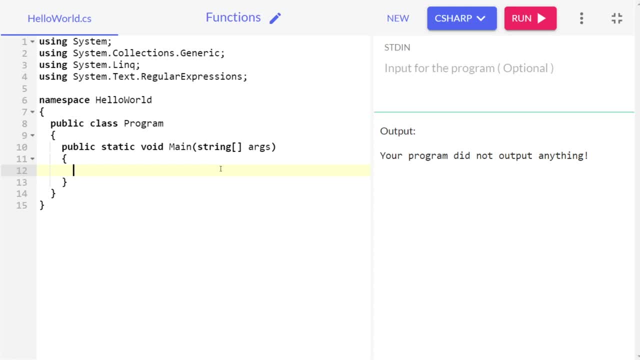 All right, Like update or like the update. method in unity is a function. The start method in a unity is a function, Right? So basically, functions and methods all right are an essential part of programming any software. All right, See whenever we code. 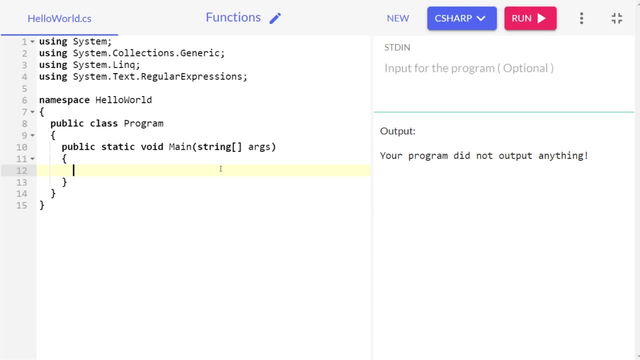 we have to follow a very simple principle of dry. Now, what is dry? Dry means don't repeat yourself. All right, Why? Because it increases the code quality, It saves a lot of time, All right, And functions in simpler terms. functions or methods are basically a block of code. 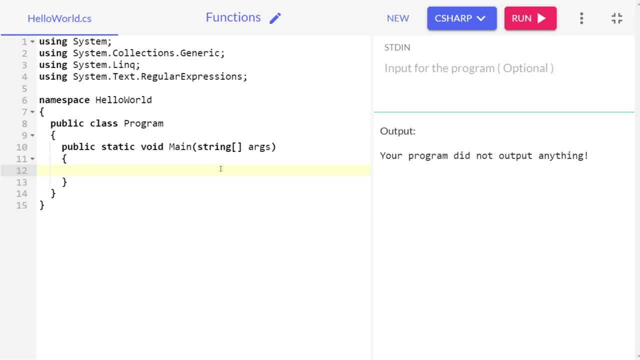 All right, They are basically a block of code which can be used any time we want. All right, Without repeating ourselves. All right, Like, for an example, you have implemented an algorithm. All right, That is a sorting algorithm. Let's say you have implemented. 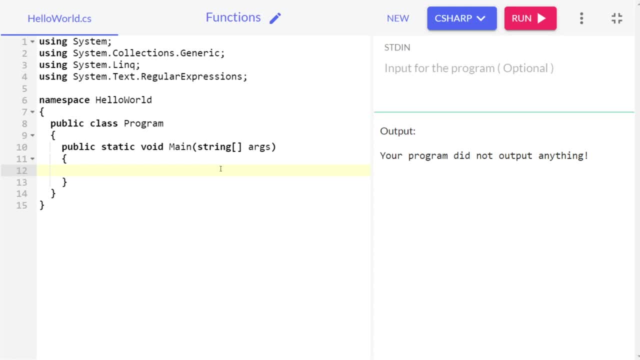 our selection. It's a sort algorithm. All right, Now you have to use that algorithm at multiple places in your program, Right? So let's say the algorithm is of 10 to 20 lines, All right, For example. now the problem would come that if you 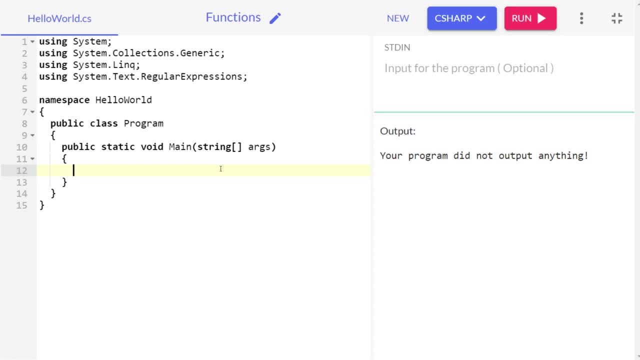 manually write that algorithm in each and every portion. now it will increase the code base, or it will increase the code base, then it will, you know, cost you a lot of your time. All right, And time is money Right. So what function does is we can create a function of that particular sorting. 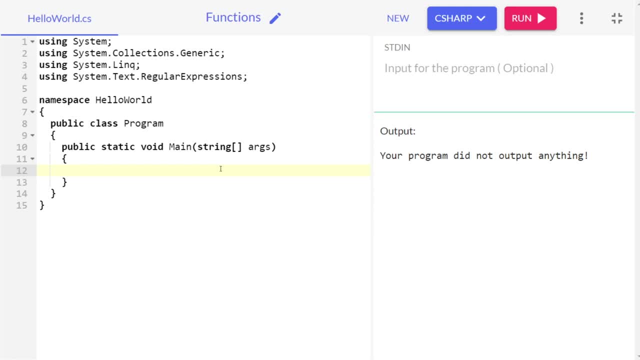 algorithm and use that function everywhere. All right, So that saves a lot of time and makes the code base more optimized. So it is very important to understand the concept of functions, All right. So basically, there are two steps through which we can use a function. 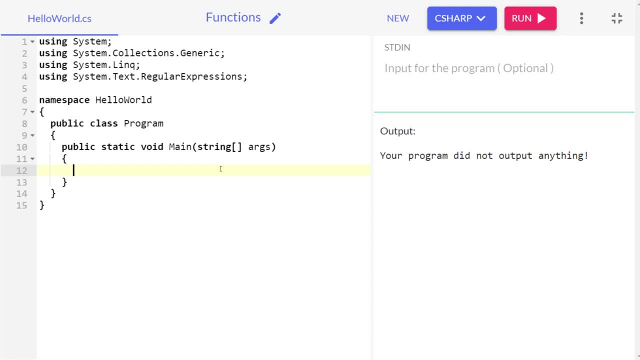 The first is we have to create a function, All right. And the second is we have to call a function, All right. Now see, call. I would show you what. what does calling a function mean? All right, See, for an example, if I had to show you a function right now. 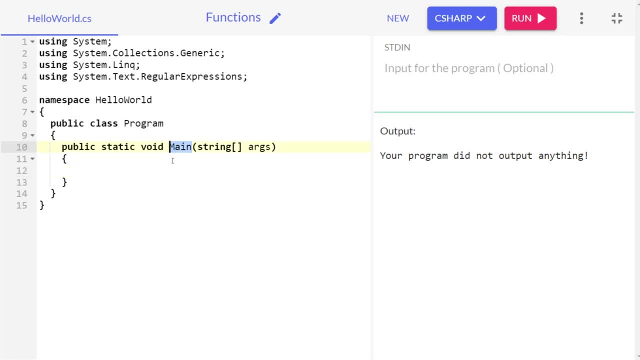 this. you can see this main method right in here, All right. Or main function: right in here is a function, All right. The difference between a regular function and this main function or the main method is that main method calls itself automatically. All right, It is called automatically. 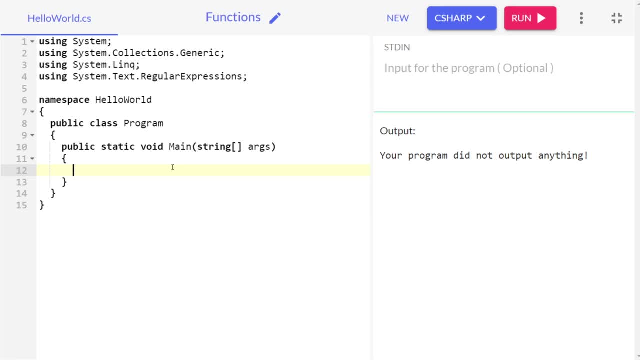 Whereas a regular, regular function has to be called by the user- All right- Or the developer. So this is the major difference between a specified means, this main function, and a regular function. All right, Now, by calling it, we means we have to, you know, call the function. 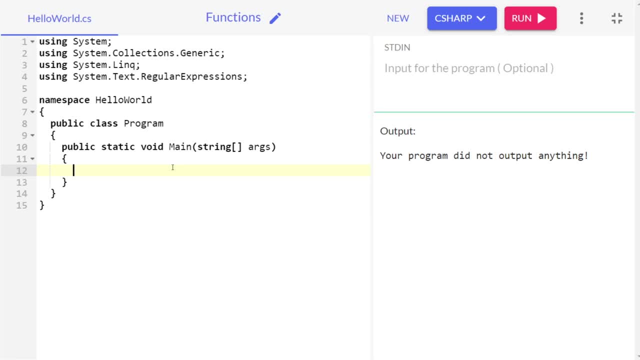 We have to say to the function: that function, do this task for me. Then only the function will work All right. He won't do the task by himself, We have to command him, All right. So that's why we call a function. 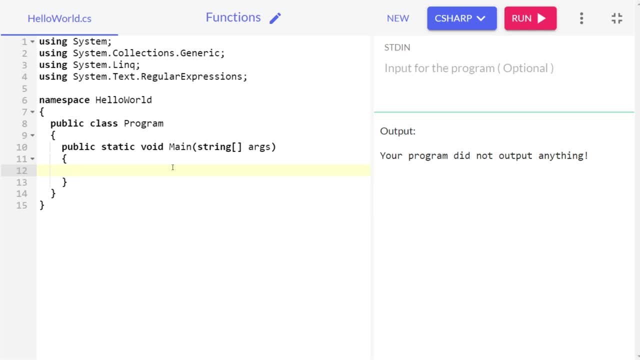 All right Now, as we have discussed about function, one more thing is that you have to keep in mind whenever creating a function- Now you can't write- means create a function inside another function, All right. Always remember that. So whenever we create a function, it should be outside a function. 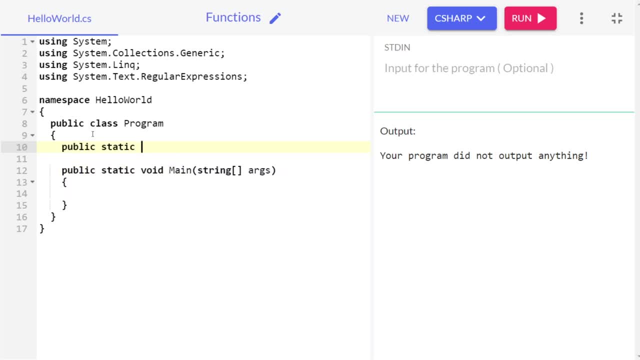 All right. Like this Public static: All right, Void set score: All right. And like this: All right. We create a function like this. Now, I know this might be a bit confusing, All right, So I'm going to explain you each and everything. 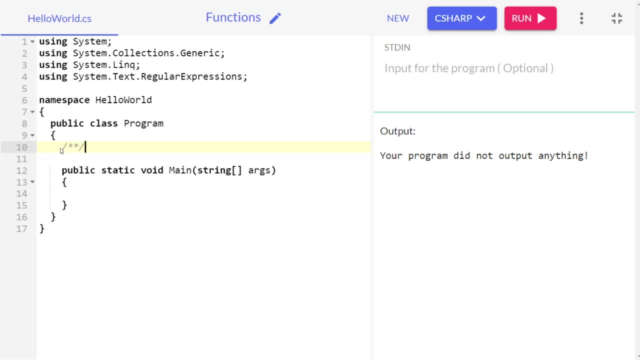 First of all, let's start with the syntax. Let me comment or create a comment line. All right, In this comment line, the first, All right, The first that would come will be an access modifier. All right, The very first thing will be access modifier. 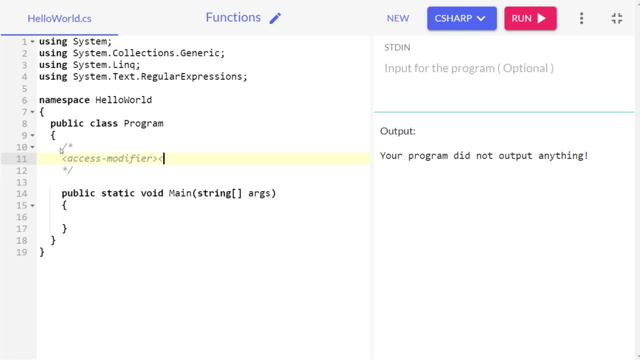 I will tell you what exactly: the access modifier. All right, After that there will come a return type. All right, After the return type, you have to give the function a name. All right. And then you have to give a parenthesis. 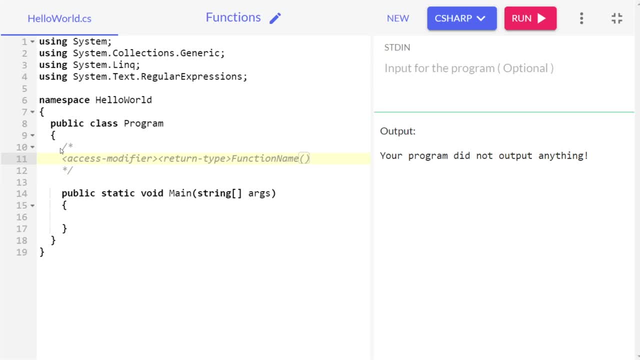 All right. Inside the parenthesis you can add parameters. What are parameters? Parameters basically takes, It is basically a list of arguments, All right, That we provide, like like an array dot sort function that I taught you in the arrays lecture. What happened in there? 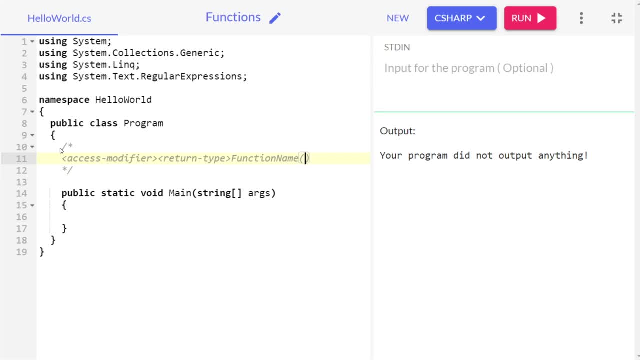 We provided an argument inside that sort function, Right. So that's how. that's why we use parameters. Parameters would come Inside. This function means this: parenthesis, and then you already know what to do: Open and close, curly brackets, All right. And inside this you have to put some code. 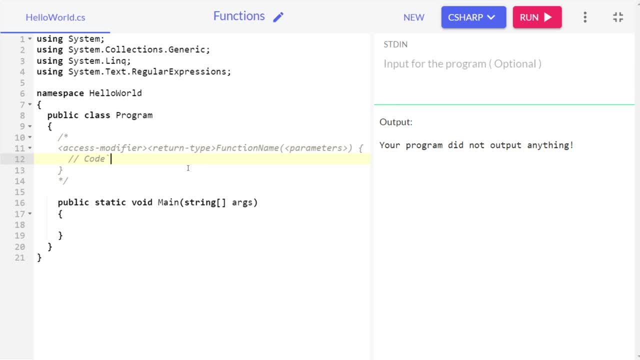 All right, Now you know. let's see the actual code for it First of all. All right, Here you can see we are writing a function. First of all, we are giving access modifier public. All right And All right. 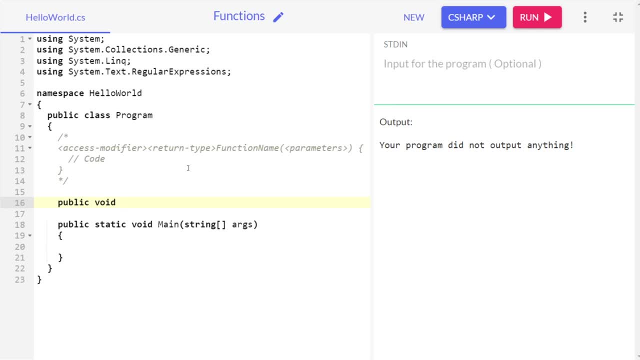 And then what you have to give us a function name. what would be the function name? the function, let's say the function image set score. All right, And now, Inside this function we have to give: all right, some write some code, that is console dot, write line. 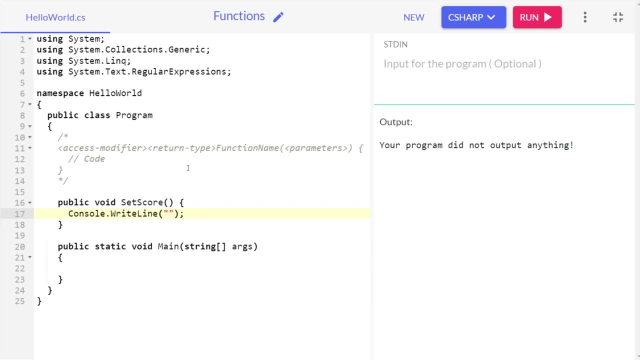 And inside this You have to Print something. Let's print Hello World. Now to call this function. or let's say, let's rename this function to hello world only. All right, So now to call this function. what we have to do is: 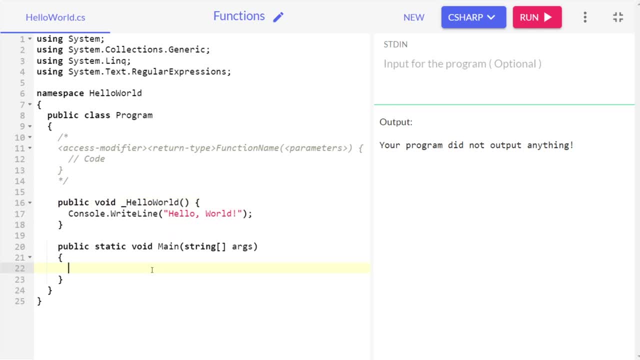 Just wait, Yeah, to call this function. What we have to do is we have to write the function name like this and then add parenthesis into it And let's run it. So here you can see. All right, Here you can see. 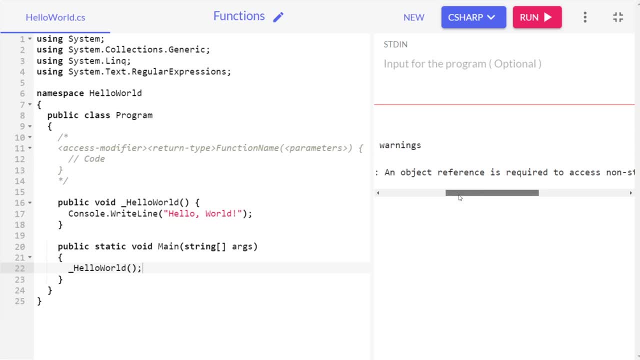 It is giving us an error. What is this error? It is telling us an object reference is required to access non static member. All right, The reason is we didn't give any reference to the object. All right, And currently, as you have not learned about object oriented programming, 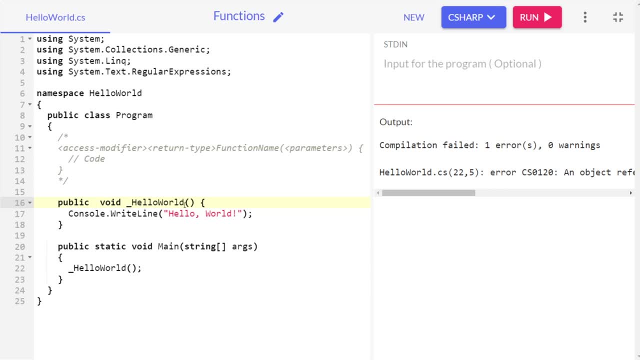 we'll be learning about object oriented programming in the next class. So here's a keyword: All right. Static. All right, Right now, You don't, you know, you don't have to put your mind Into the keyword static and public. 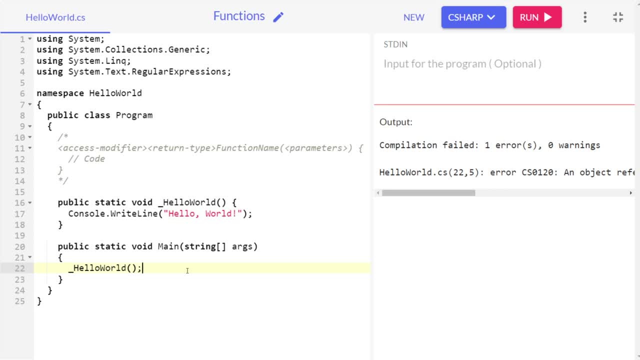 All right, Because these two keywords will make more sense after the next lecture. All right, Because these are these two Basically. these two keywords are mostly used in object oriented programming. All right, So now let's run the program and let's see what happens. 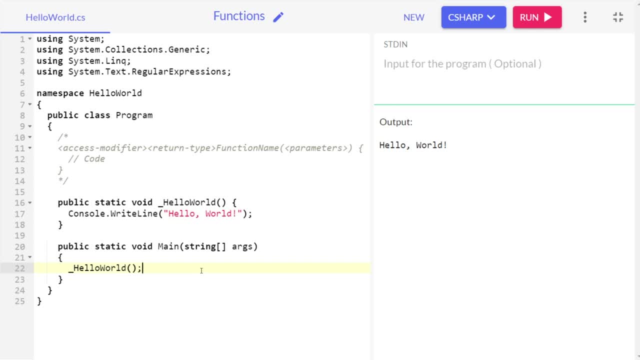 See, we are able to get the output. All right, Now I would explain you. All right, I would explain you this code. All right, What exactly are these? First, you can see we are specifying an access modifier. That is this one. This is access modifier. 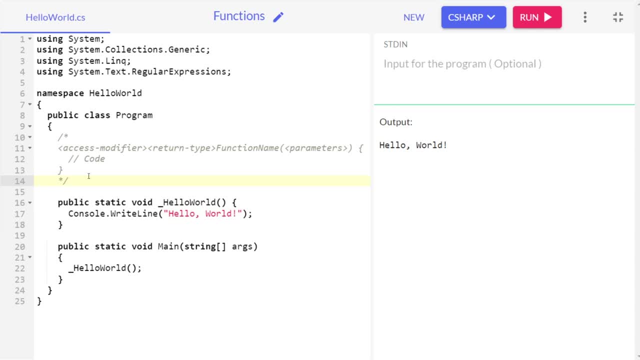 Now, what is? what exactly is an access modifier? Access modifier is like a gatekeeper. All right, Like like. let's say, you have a security guard in your house. All right, You have a guided means. you are told that the security, security guard that you are. 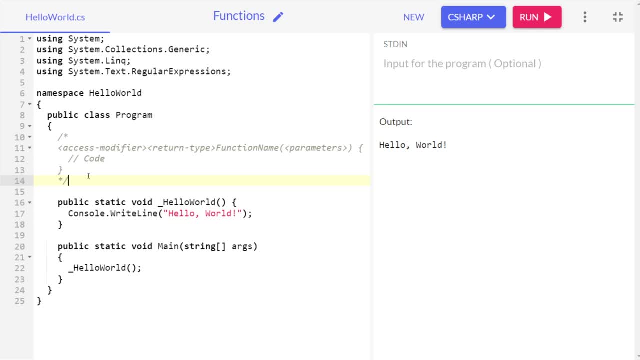 like you don't want any buddy to Disturb you, All right. So at that point of time you have gone private. But if your security guard, if you haven't like, if you have told your security guard that, brother, if anyone comes to meet me, then let him inside. 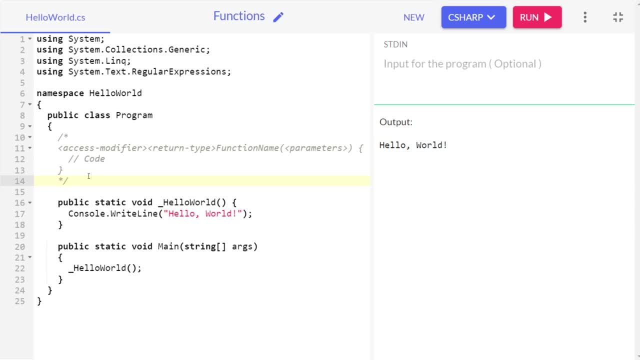 All right, Let him come inside. So then you are public. All right, The security guard will let it go. It's the access modifiers are also something like this: Public and private. public and private Public means you can access that particular thing from any class. 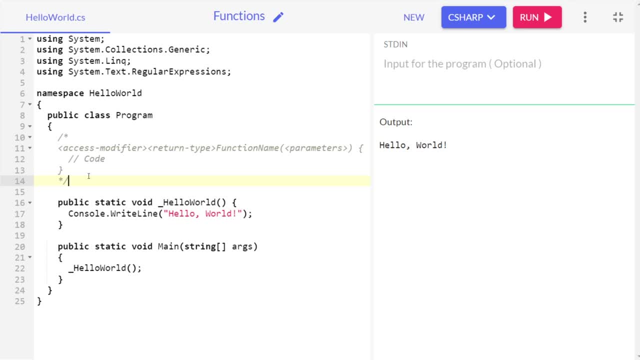 All right, Whereas private means you can't access that particular thing, let it be a variable or method, you can't access it outside of their class. So I know this might be this might seem a bit overwhelming, or maybe it might seem, you know, a bit confusing, but that's totally OK, because all these concepts 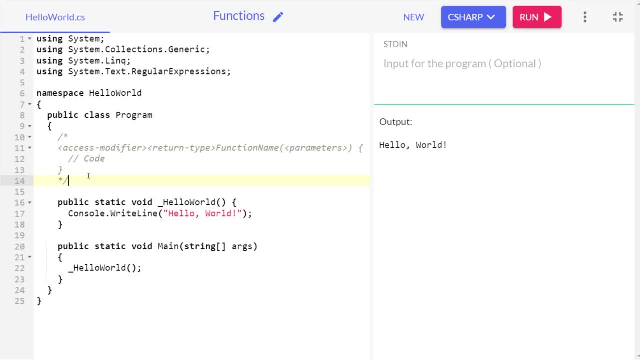 All right, You will get a grip on all these concepts after the next lecture, because in object oriented programming, we are going to learn more about methods. We are going to learn more about access modifiers. We are going to experiment with it, All right. So 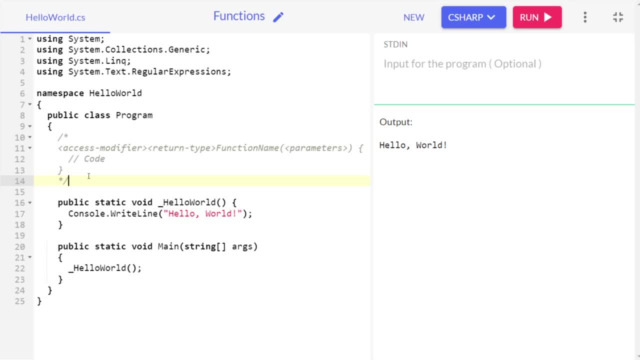 Don't worry, All right Now, as I hope. the basic concept of access modifier is clear. it just: access modifier helps us to modify the access, All right. It helps us to modify, restrict the access of any variable or of any method. 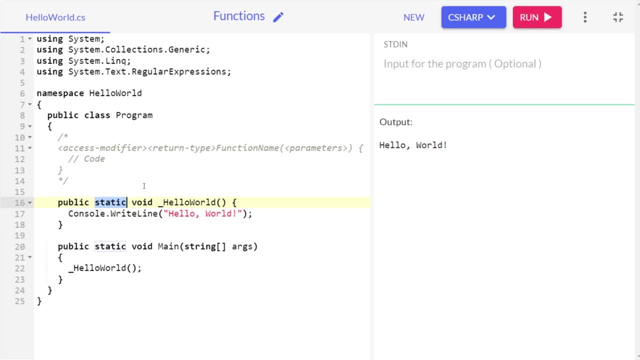 All right. So that's what an access modifier is. Next, here comes the static keyword. All right, Don't worry about that. Don't worry about the static keyword. All right, Let me. I'm going to explain the static keyword in the next lecture, because this static keyword is one. 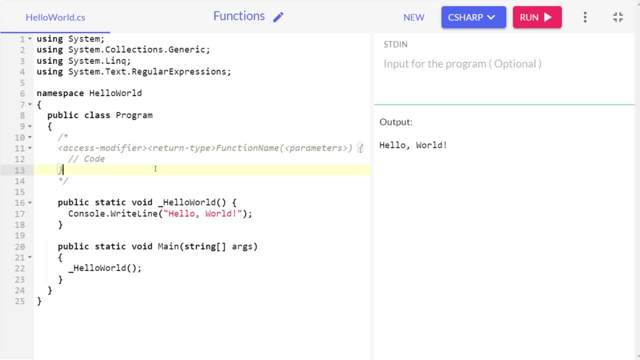 of the very important concept that you should know. All right. After the static keyword comes return type. All right Return type. All right Return type is basically what kind of value we want to return to the function. All right Return type basically defines what value can be returned to the function. 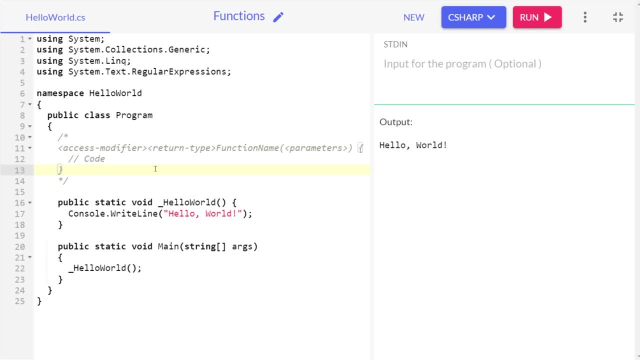 It can be of void, All right. It can be float. It can be string, All right. So now see access modifiers can be of multiple types, All right. It can be boolean, All right. It can be of bool, It can be, you know, of float. 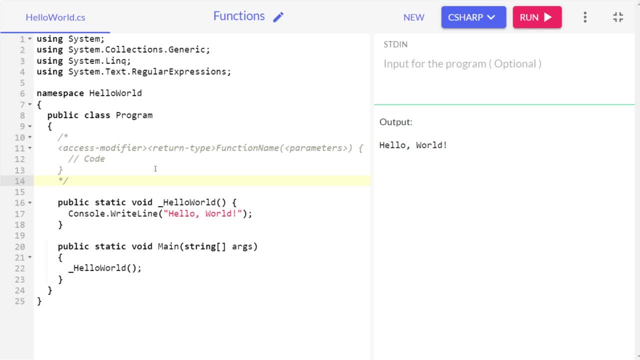 It can be of string, All right. Another type is void in a void, All right. In a void return type. we didn't, we do not need to return, All right, We do not need to return anything in a void, you know, in a void function. 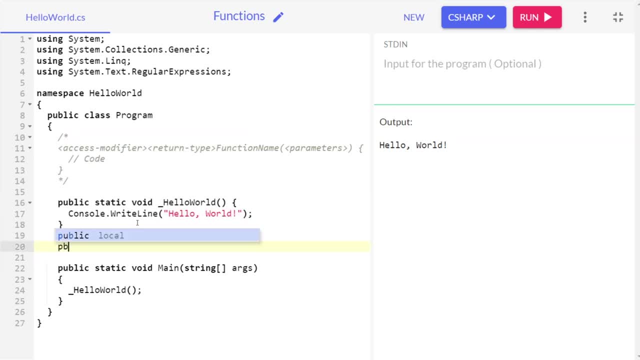 But let's say we create a function with a different return type. let's say int- All right, So public, static, int- All right. Let's say: we are, you know, let's. let's create a function that would you know, give us the square of some number. 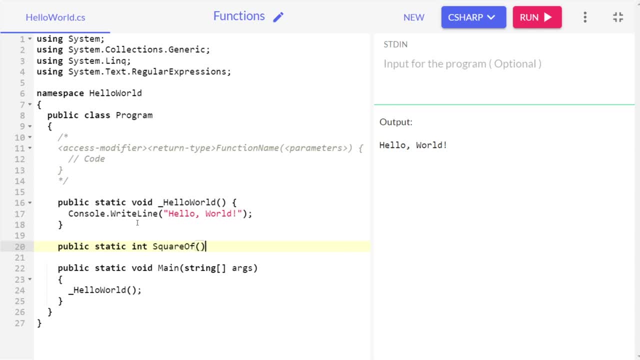 So let's write a function that is square of. All right. Then in here, what I'm going to do is I'm going to create a variable. All right, That is int. Let's say, square Square. All right, Square of. 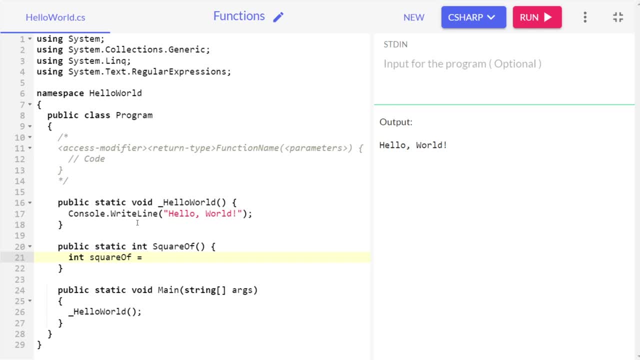 Square of. I'm going to create this variable, All right, In here the S is small and in the function it is in caps. All right, So don't worry. So now what I can do. how to you know? how can we exactly? 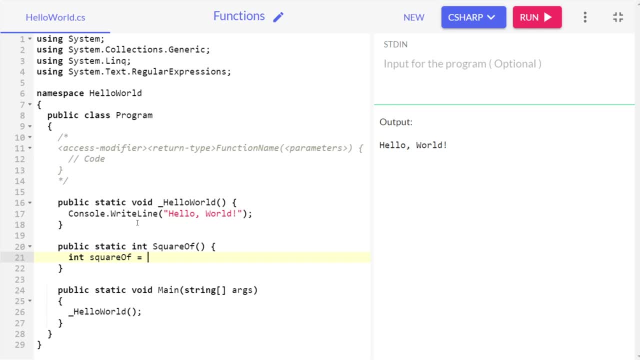 make a square of the number Right. I can multiply that number with the same number Right. So here I'm taking an parameter. All right, So the parameter would be integer n. All right, You can take as many parameters you want. 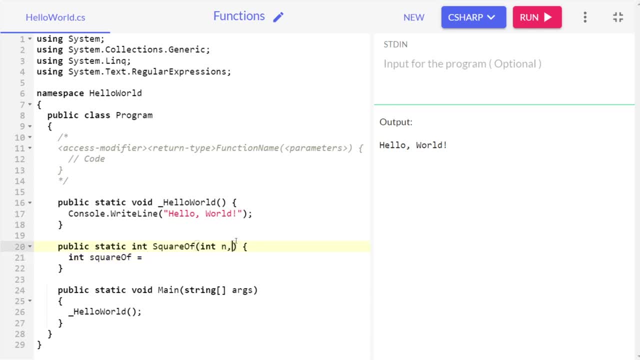 All right, I can even take another parameter, as in float. All right, I can even take that That is float n1.. All right, I can do that. So the thing is, you don't, you don't have to be like the function can only take one parameter. 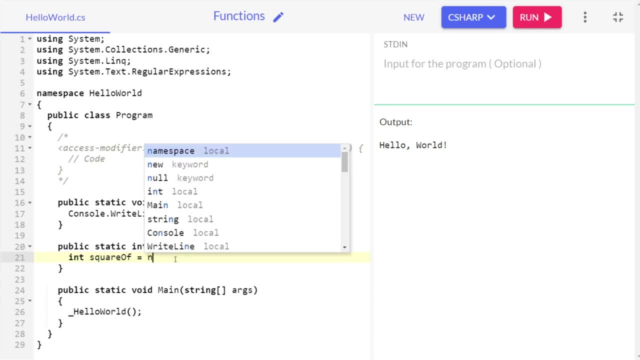 You can give any parameters you want, All right. So now, as we have given the parameter, we are doing it n into n And after that I'm returning. All right, I'm returning, We are. we are using the return keyword. 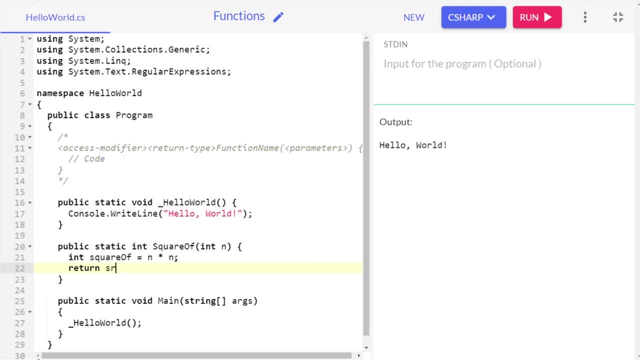 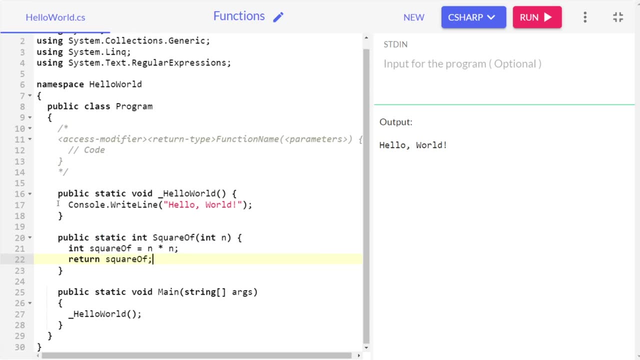 I'm returning this square of. All right, I'm returning this square of variable to the function now in here, as we call this function. It printed us Hello, All right, But to you know, get the value of this function. 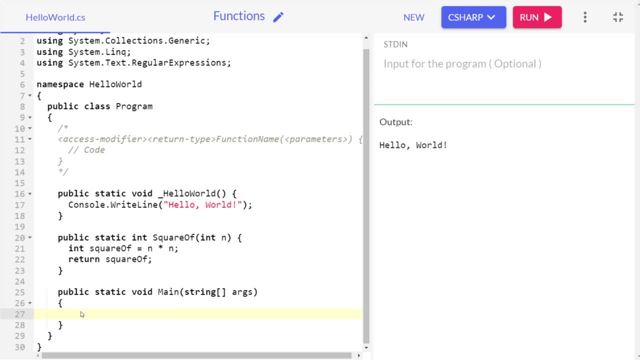 All right, That is the square of function. It would be a bit different How? Let me tell you. Let's try it out. actually, All right, Let's take the square of you know square, square of function and let's put a value. 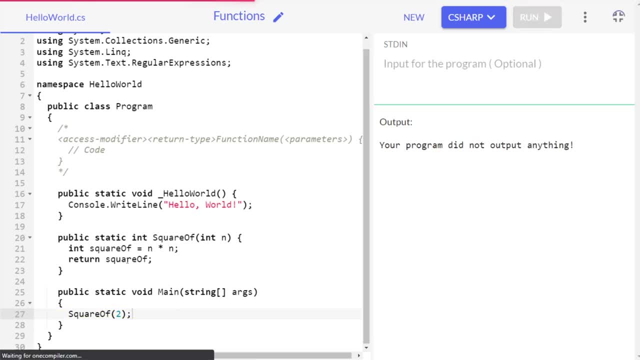 Let's say two. We want square of two. Now let's run it, Let's see. See, here you can see your program did not output anything. The reason behind this: it is not printing anything, It is returning the value to the function. 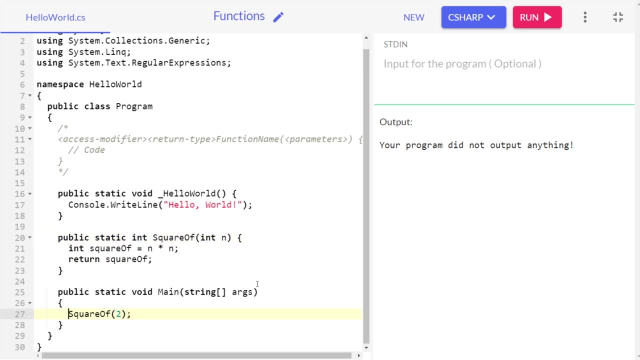 Now to print. all right, now to print the value of the function. What we have to do is we have to store this, I mean store the returned value, into a variable. So how would it? how do we do that? So create a variable that is in final. 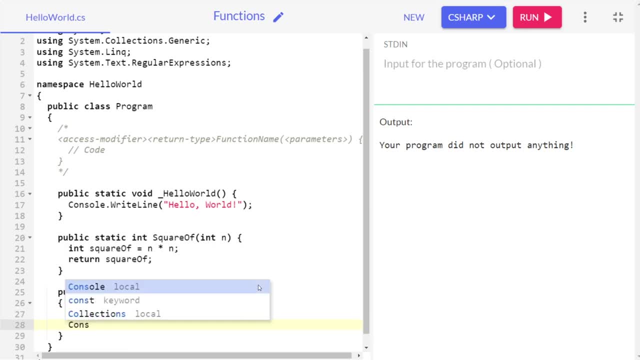 You can name it anything after you have stored it like this, Then you can do console dot Right, line Final, All right. And after that you can simply print anything. All right, I mean simply print it. Now let's try out a square of four. 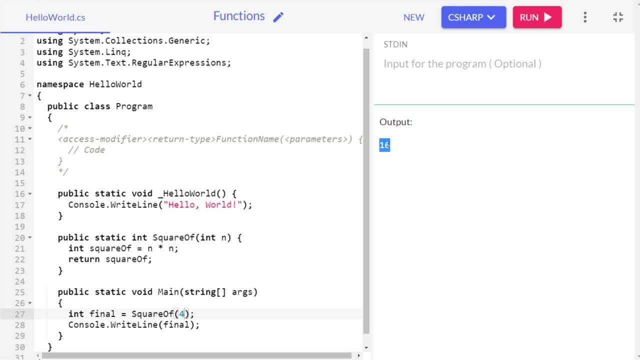 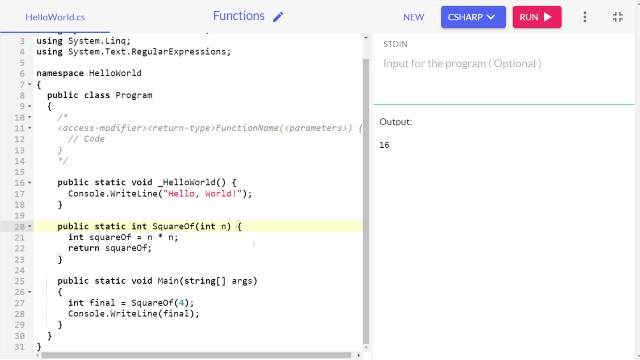 So the square of four will be 16.. Right, So here you can see that it is giving out the output A 16.. Similarly, you can also create your return types as boolean. All right, You can create your return types as string. 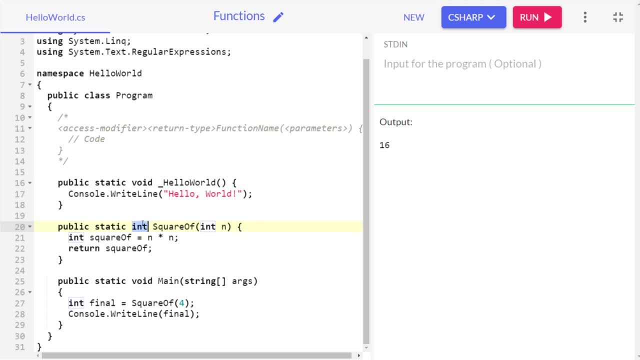 All right. One more thing you have to keep in mind: If you are specifying a return type, like you have to return integer values only. if you try to return float value, floating point or string value, it would give you error, All right, So make sure you practice on this. 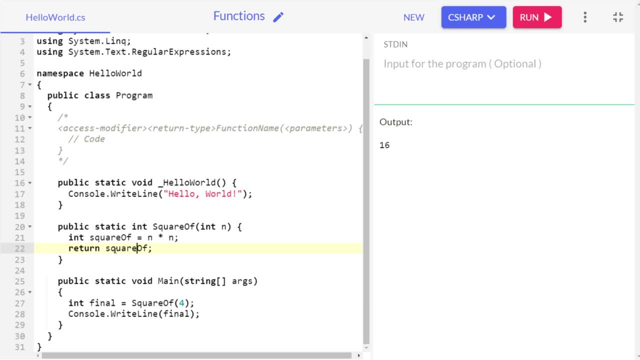 All right, And don't worry about the access modifiers and the static keyword. All right, Because in the next lecture, in the next lecture, that is where we'll be exploring classes and objects, that is a basic of object oriented programming There will be. there you would be learning about the static keyword. 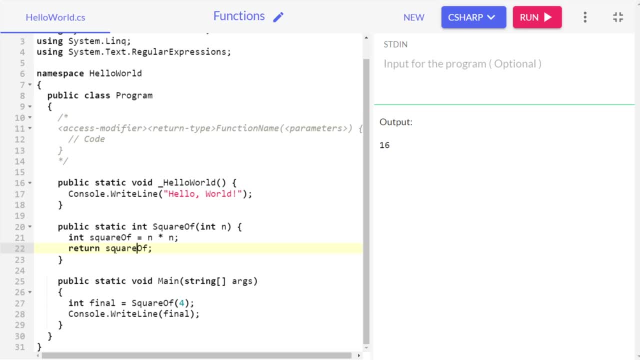 The. you know about static classes to be learning about objects. You will be learning about instances. Then you would also be learning about this access modifier and how we use them Right. So you'll be learning all those things in the next lecture. 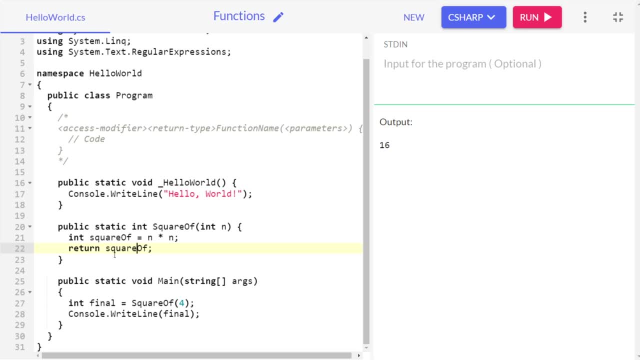 So don't worry. if you are, if you are confused somehow By the next lecture, the function, the topic of functions, will be very clear to you. But if I had to say in a very simple word, functions are just basically a block of. 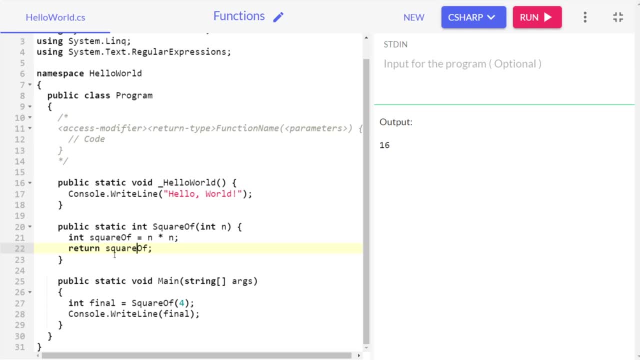 code that help us to reduce the means, to reduce the lines of a code. All right, We can reuse that function And always remember, don't repeat. Always follow the principle of don't repeat yourself. All right, Like, let's say, if you are creating an algorithm. 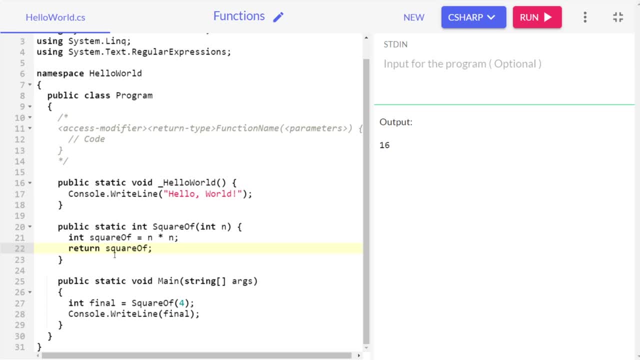 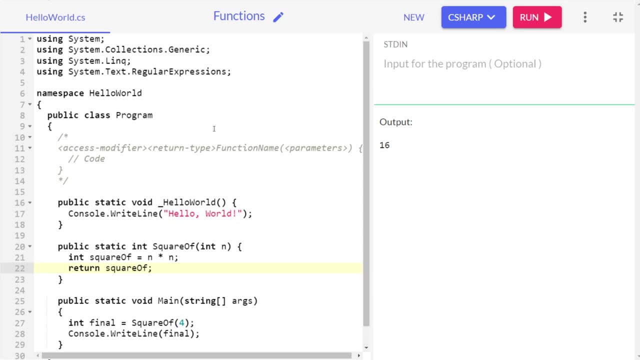 then create a function of that algorithm so that, so that you can use that function anywhere you want, All right, So make sure you Follow the principles of dry, All right. So, yeah, that's it for this lecture. So in the next lecture we are going to learn about classes and objects. 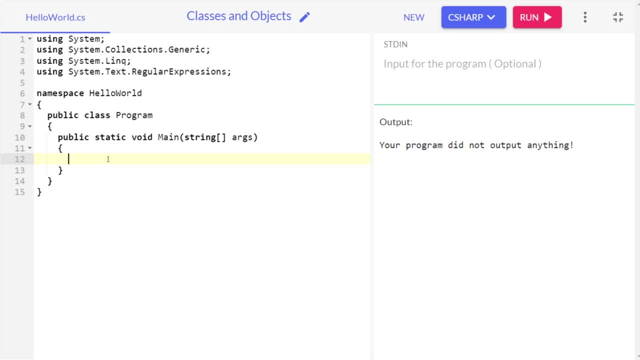 In this lecture we are going to learn about object oriented means, the very basics of object oriented programming. all right, and in that would be learning about classes and objects, All right. So this is the very basic of object oriented programming. There are many other concepts already that you would be needing to learn. 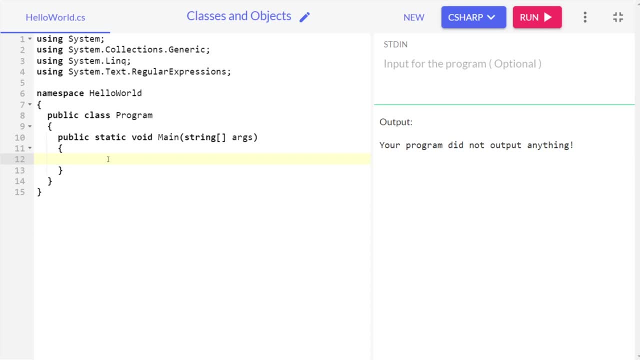 But for now, for the starting, All right, For starting, This is the topic that I'm going to teach you. All right, We'll be learning about classes and objects. We'll be learning about fields. We'll be learning about methods, that is, class members. 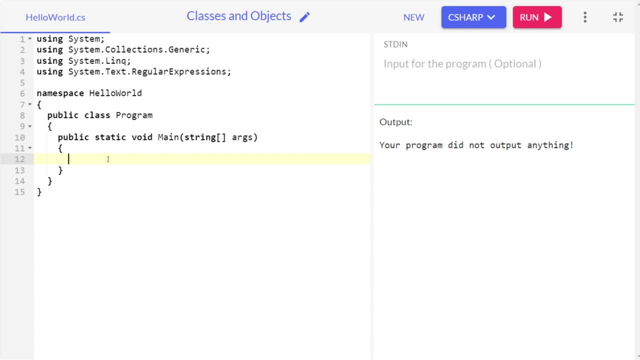 All right, We'll be learning about- you know- constructors- how to create a constructor. We are going to learn about access modifiers, static keyword. We are going to learn about static classes. All right, So without any further ado. All right, Let's start with the lecture. 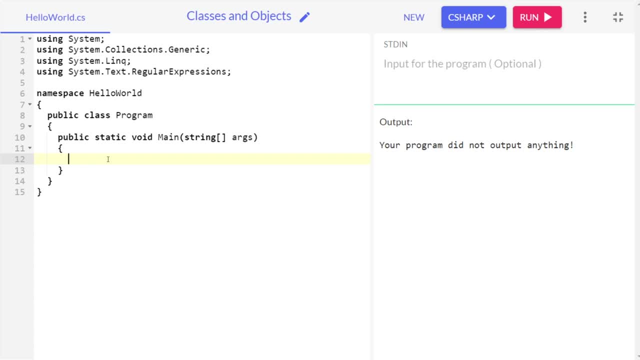 All right, See to understand classes and objects, Now understand this object oriented programming. All right, We have to understand the, A very fundamental concept of object oriented programming. What exactly is it? Object oriented programming is basically an approach. All right, That breaks a programming problem into. 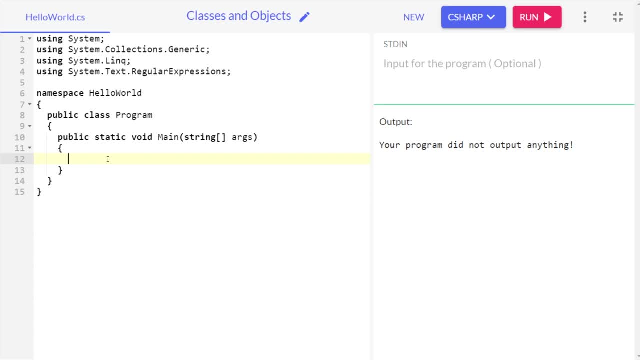 you know objects that interact with each other. All right, Basically, objects are created from. you know templates, and those templates are known as class. All right, You, we, actually, we actually can think class as a blueprint or a class as a blueprint. 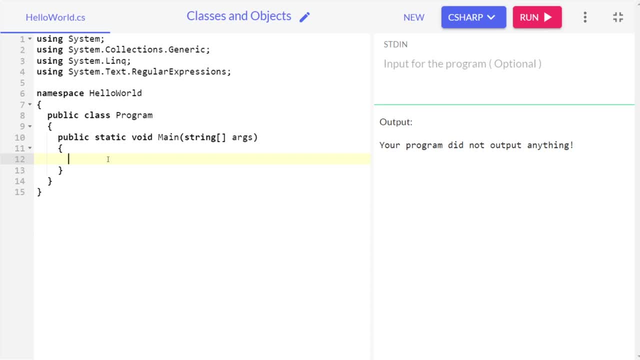 And you know, just like a, you know a blueprint of a building, All right, And from that blueprint of a building we build an object that is the actual building, with bricks and motors and all those things, Right. So that's what object oriented programming is. 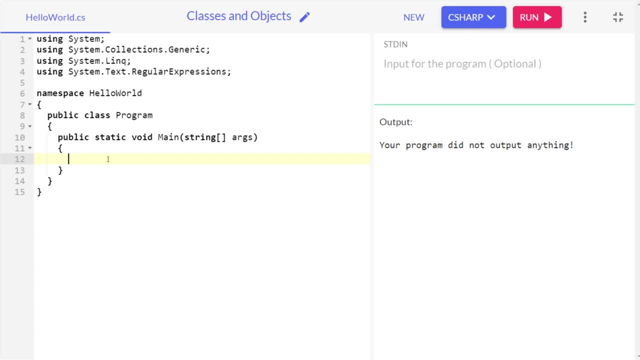 All right. So I hope this- you have understood what exactly object oriented programming is Right Now. as we've understood What exactly object oriented programming is, It is our time to understand about classes. All right, As I told you, class is like a blueprint, Right? 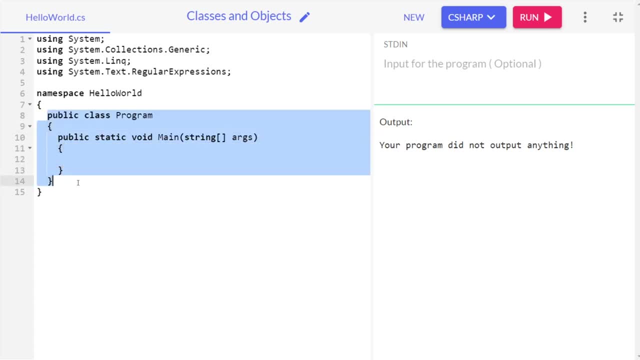 Like here. you can see this is a class public class program. Right Inside there is a method that is the main method, Right, So we can write our own class. now to write our own class, First of all, remember you can't write a class inside another class. 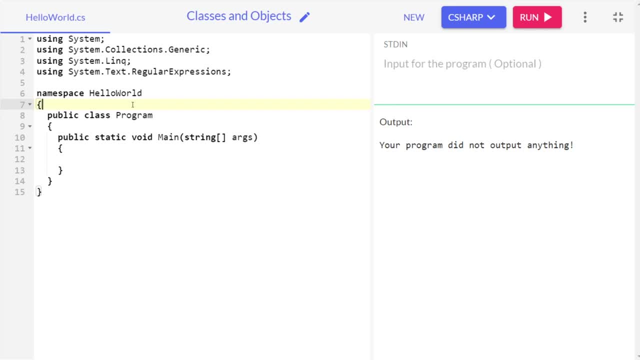 All right, You have to write a new class outside of that class, All right. So what we have to do is write public, All right, Public class, All right. And give the class a name. All right, Give the class a name, and let's give the class a name as person. 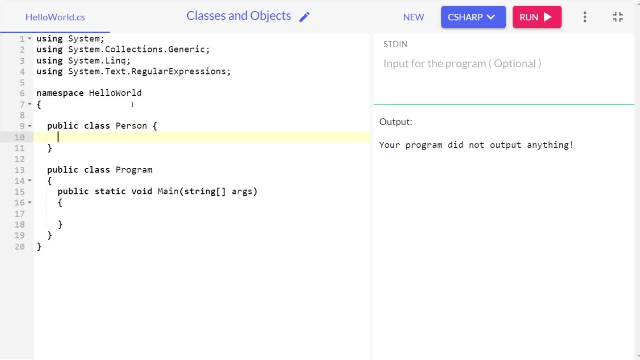 And then what you have to do is you have to open curly braces and close it. So this is how we write a class. All right, This is a public method, This is the class keyword And this is The name of the class. All right, 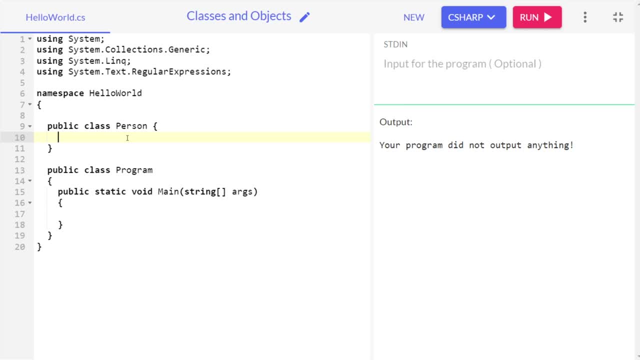 So that's how we create a class. All right, Now there's some. there is another thing called fields. All right, To understand field, you can say: fields are, you know, variables only. All right, They are variables only. 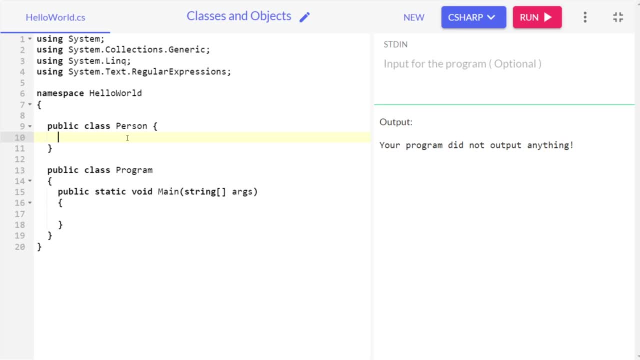 A field is simply a variable. that is we know. we declared. we declare inside a class, All right. Like any other variables, All right. They are used to store data, like here You can see. we can write public, All right, In, or, let's say, public string. 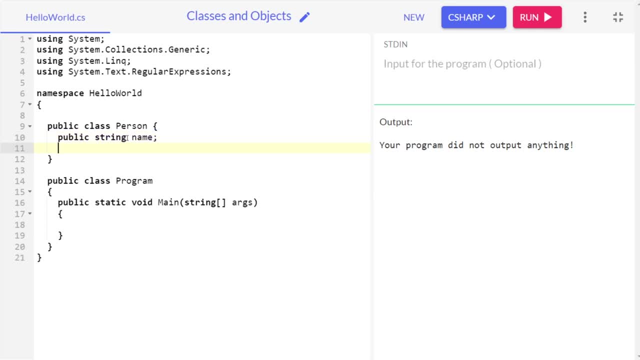 Name of the person. All right, Then we can write public In age Right. So this is how we this. this is called fields, All right, So this is our call. This is called fields, All right. Now, here you can notice that there is public keyword in you know. 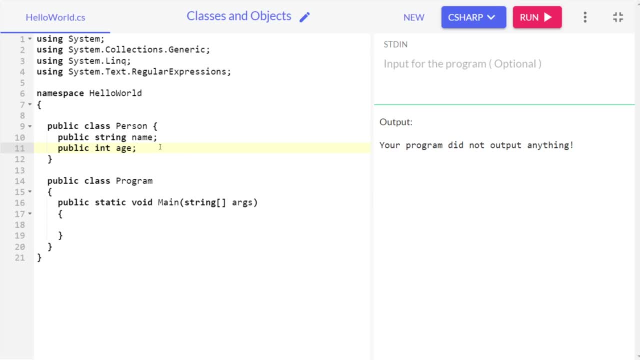 in front of all the variables. All right, So they are. now they are known as access modifiers. They are basically gatekeepers. They, you know, control who has access. All right, Who has access to the fields or methods? Now, the who in this case, is another class. 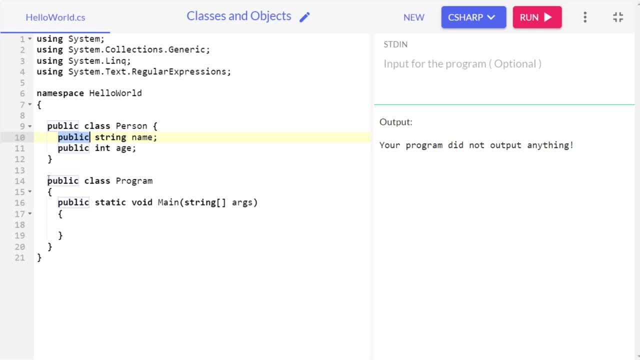 All right Now. if we make this to private now, this program class won't be able to access this variables from this person class. All right, Now. you know, to access this class, we have to create an object of this class. All right. 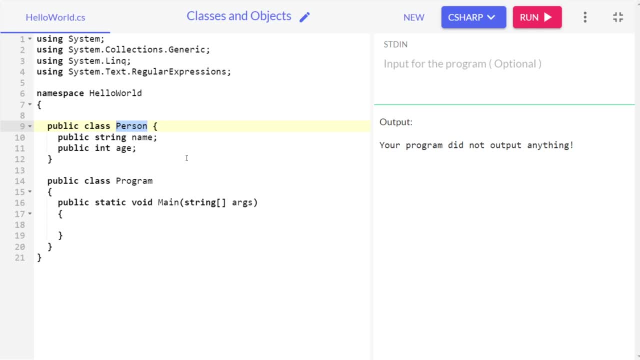 So I'm going to teach you how to do that, But before that, let's learn how to create method. All right, Let's learn how to create methods inside, inside a new class. So it's it's also similar, like this public static void. 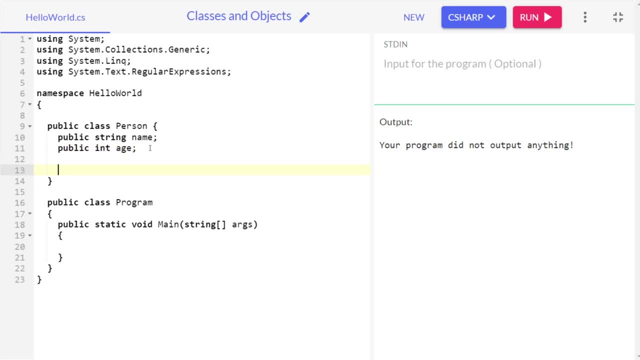 Just like I taught you in previous lecture about function. So what you can do is public, All right, Static Void and let's give it a name. All right, Let's give it a name. That is a get name, All right. 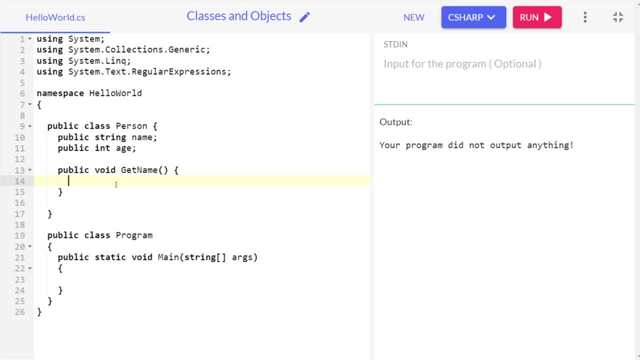 And in here it is not necessary to give the static keyword. All right, I would. There's a reason behind that. You would be learning that reason after you know, after we get into the concept of static keywords. So don't worry, we are going to get in there. 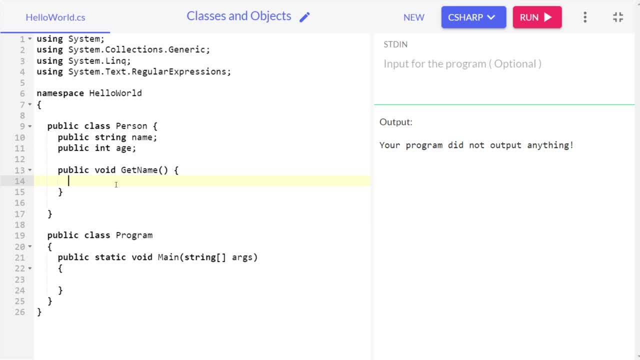 All right For now. remove the static keyword. Remove the static keyword. What you can do is console Dot Right, line All right And write it like: this name is Get the. you know, get the name variable in here. 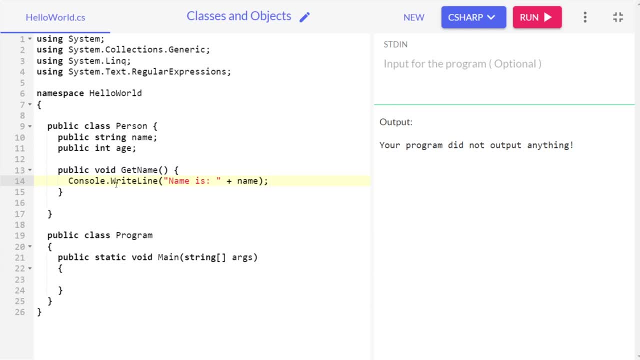 All right, Get the name variable in here And, similarly, do the same thing for the age variable. All right, The age is at all right. So now, what you have to do is now we, as we have created our method, as we have created our method. what we have to do is we have to create. 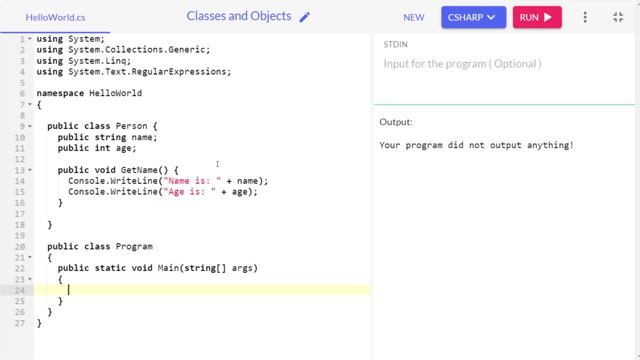 an object of that class, all right, or in simple word, An instance of that class. what does that mean? See, an object is created from a class. All right, We have already created a class named person, So now we can. 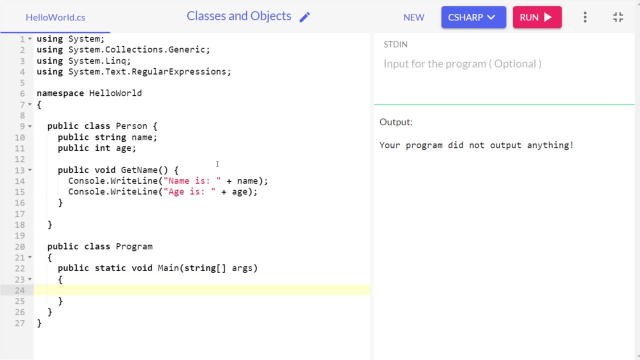 We use this to create objects. The object is basically an instance of a class. All right To you know. to create an object of the class, we use the new keyword. Let me show you how. All right, So it's very simple. 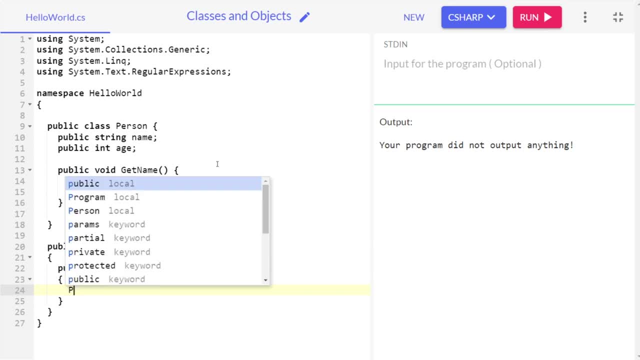 What you have to do is first what you have to do: take the class name, That is, in our case, the class name is person. After that, give you know, give it a name That is I'm going to name. 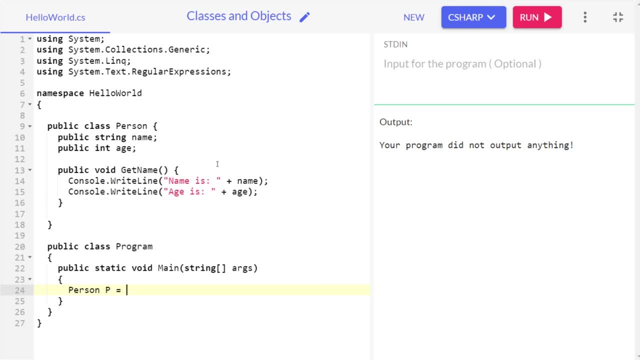 P for now and then Or put equals to in there, then write the keyword new and then again call the class like this: all right, and then Give parenthesis to it after that, if you run it, let's see if you get any errors. 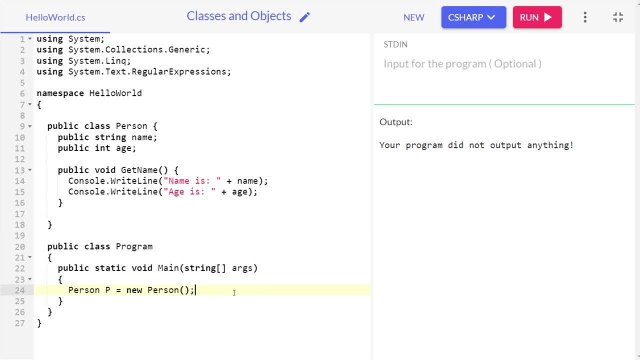 or not. you are not getting any error, so that means we are good to go, All right. So now here, we have created an instance of a class, or you can say an object of a class. All right, We have created an object of a class. 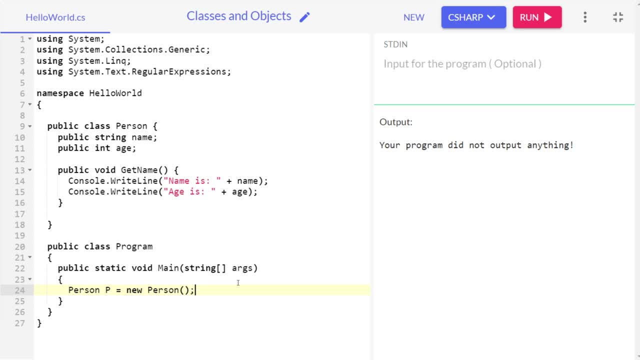 Now, as we have created an instance of the class, we can also access the fields and methods available inside the class from our program class All right- And make modifications to it. All right, Like in here, All right, So what? first, what I can do is P dot. 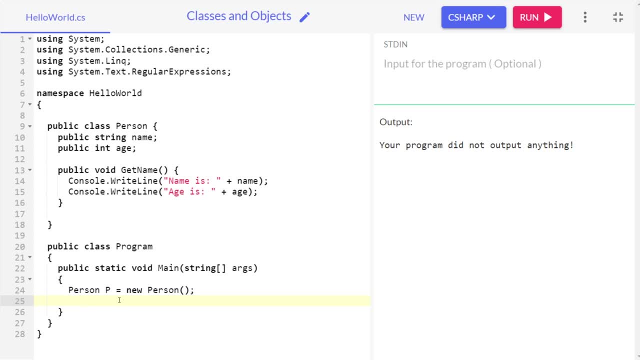 Here, first of all, to access. you know, to access the fields and methods of the class, you have to call that Right. So what you can do is here you have named the class Right, That is, you have named the object as P. 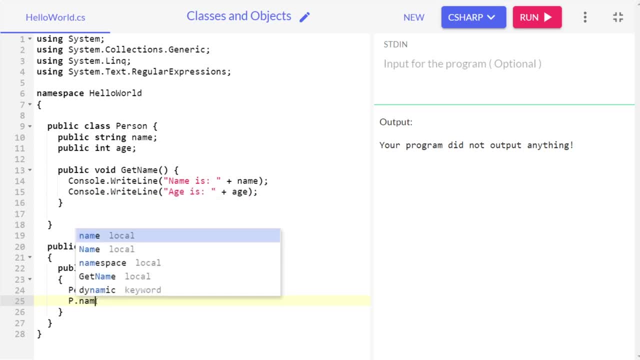 So write P in there, then dot All right. Then give the variable name and set the variable name to you. know anything? you, let's say your name. All right Now. after that set it, set the age value to, let's say my age, currently 17.. 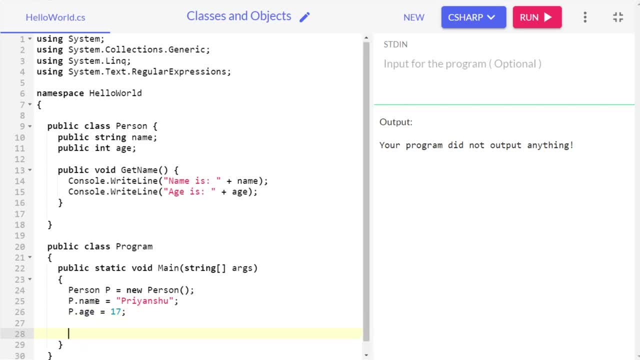 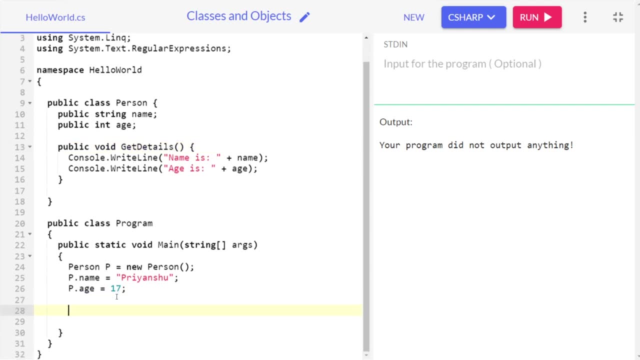 All right, So I'm going to put it like that. after that, All right, Here you can see, Let's change the name to get details. actually, Yeah, that would be better. So now, here you can see, Let's actually try it out. 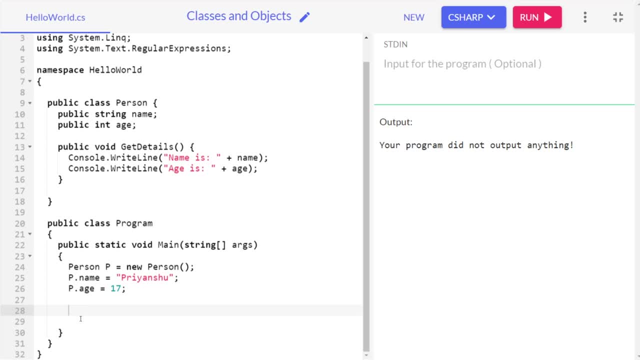 Let's see if any error is coming or not. So here you can see we are not getting any error now. Now let's get the details. Let's see if, like the means in the object, the details we have filled- has been set or not to do that. what if, as a creator of no method, that is, get details? 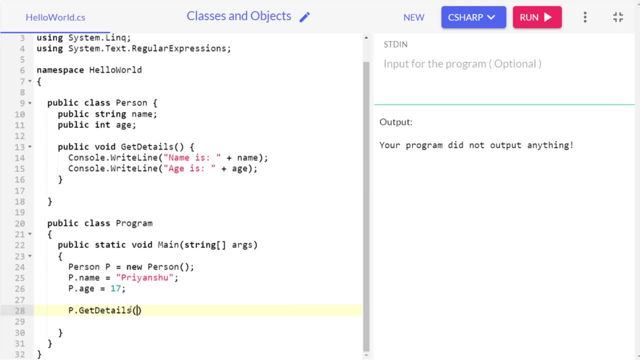 What I can do is P dot, get details And let's see if everything is working or not. So here you can see: all the things in here are working. now You can create all that. you can create multiple objects, All right. You can create as many objects you want. 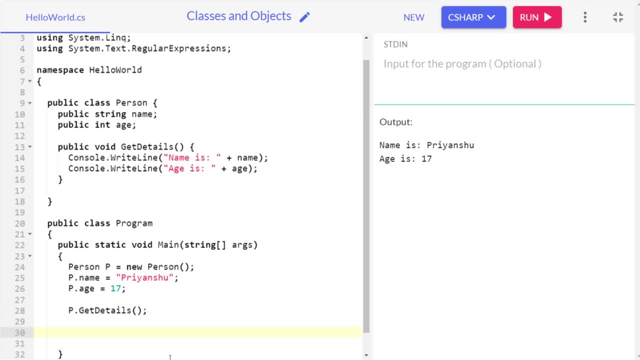 All right, Like this, Let's let's try another one. That is person. P equals new person, And in here what you can do is P, dot, name equals, let's, you know, give it Rohit, All right, And let's give, give its age also, you know 18.. 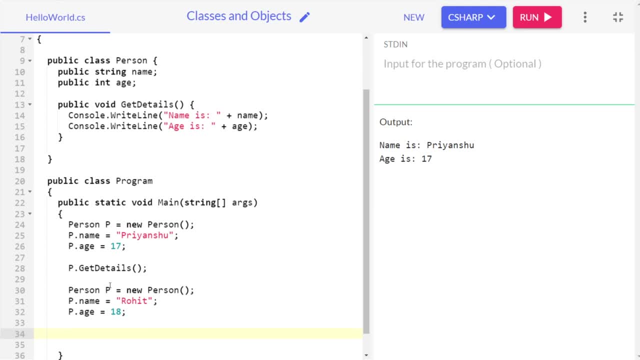 Let's give it. And now let's see. All right, Always I did a mistake. I, you know, name both the means, both the instances with the same name, So don't do that. All right, Change the name in here. 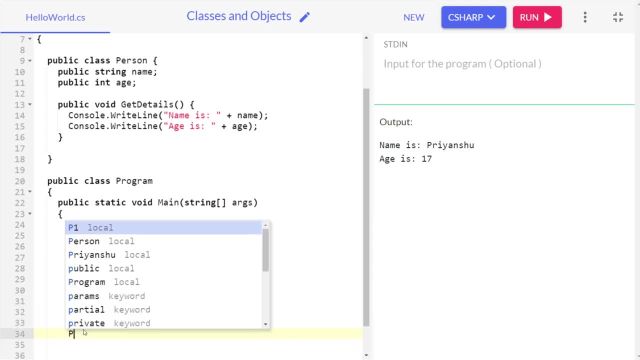 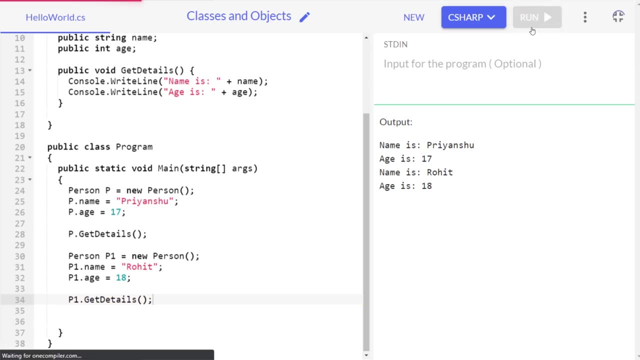 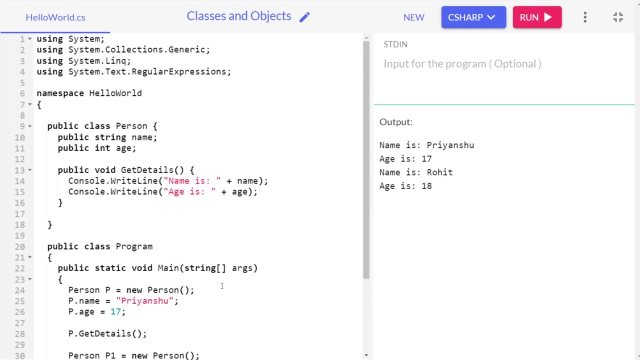 My bad. So now what you can do is: P1 dot, get details. All right, Now let's see if this works or not. So here you can see: both the instances are working. So this is how we create a class and we create an instance of that class. 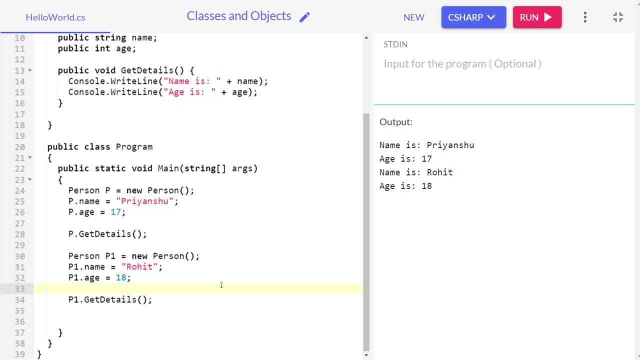 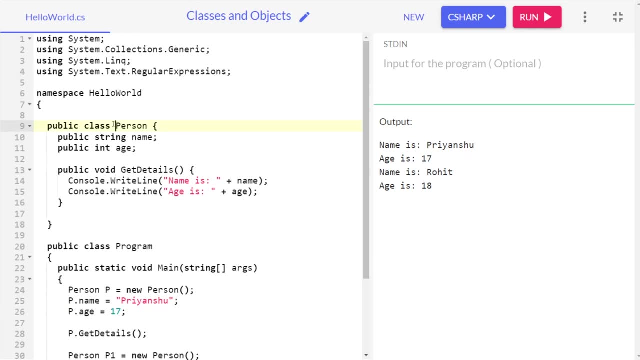 All right, So this is how we do it now. See the fields and methods inside all the fields and methods inside a class. All right, Like this is a field, This variable is a field. This variable is a field And this is a method. 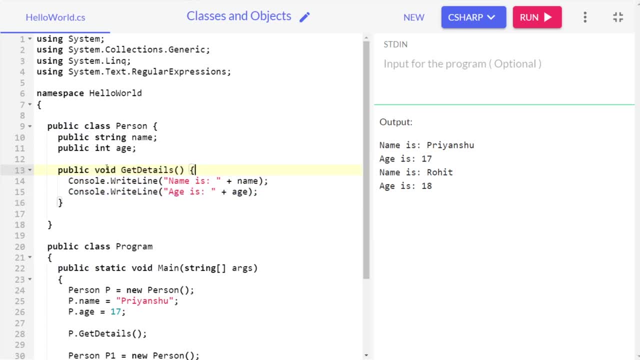 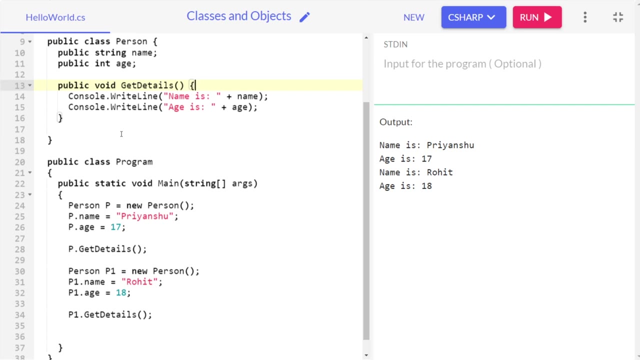 This, this whole thing, is a method, So they are often referred as class members. All right, They are the member of the class called person, All right, So make sure to keep this in mind, All right. So now, as we have learned about, you know classes and objects. 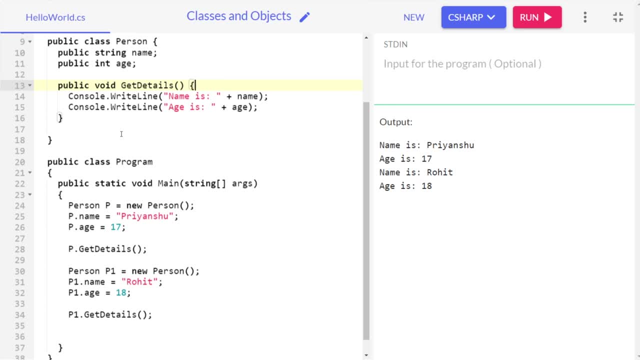 now it is our time to learn about constructors. All right, To learn about constructors. I know it, This, you know this. This might seem a bit, you know, confusing, but don't worry. All right, Don't worry. 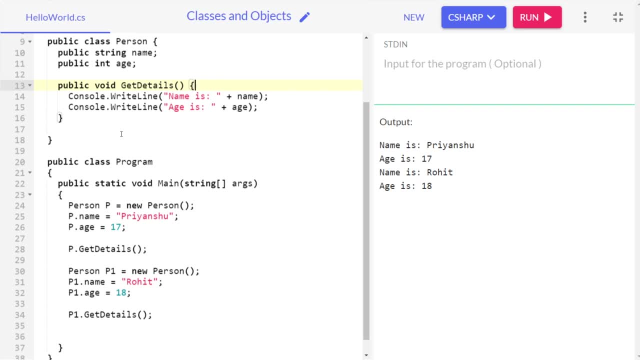 I'm going to tell you how to do it. All right, See what is a constructor? A constructor is basically a special method, All right, That is, you know, used to initialize objects. The advantage of using a constructor is that it is called when an object 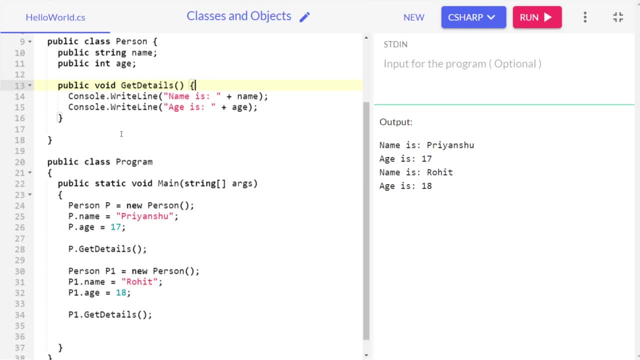 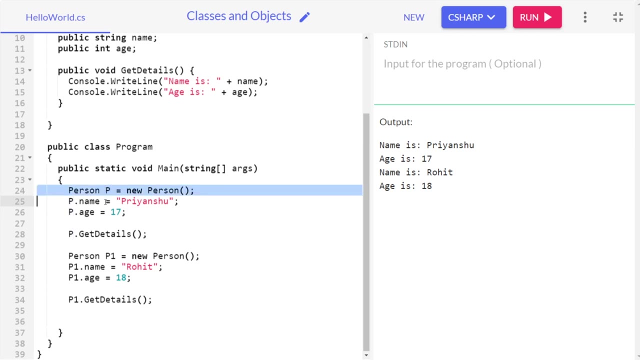 All right. It is called when an object is created. it can be used to set initial values. All right Means right now, whenever we are calling this. you know, whenever you are creating an object of this class, no value is being set by default. 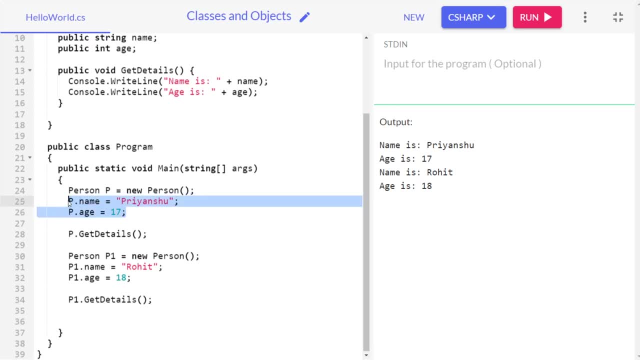 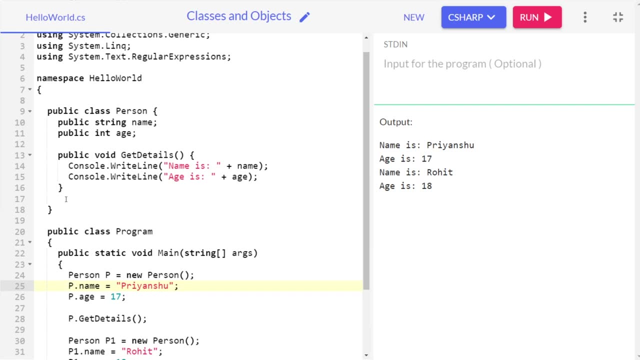 All right, We are not able to set any value by default. We are setting them later on. What constructor does is, whenever we create an instance of a class, a constructor is called. All right, A constructor Is, Is, you know, is called. 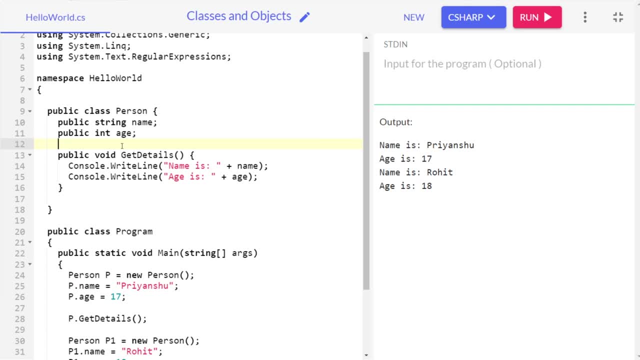 So to you know, to set means to create a constructor. it's very simple. What you have to do is public, All right, Then you have to write the class name. All right, You have to write the class name, then parentheses. 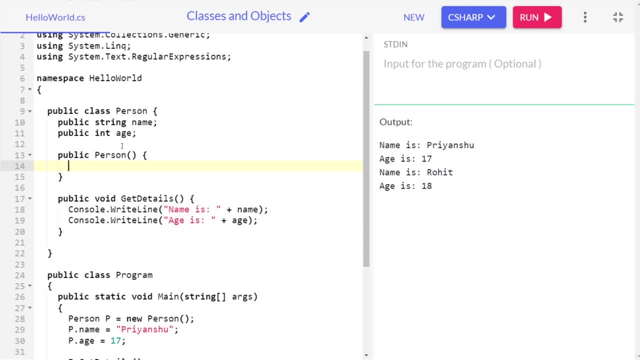 It just looks like the function that you don't have to give the return type. All right, Then, in the person, in the person I'm going to set. All right, I'm going to set the name to, let's say, default human. 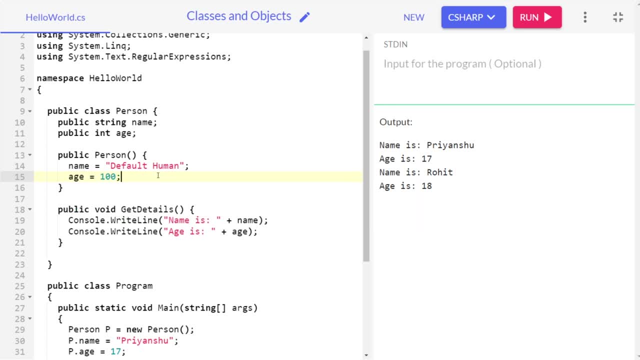 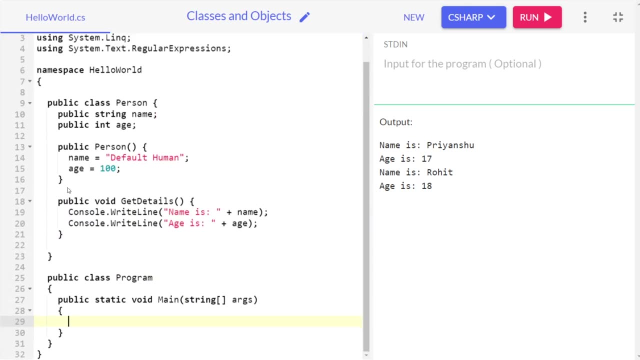 And the age to, Let's say, 100.. All right, Now you know, let's remove the previous code. Let's remove the previous code and let's see how this whole constructor thing is working. Right, See, I won't be setting the name right now. 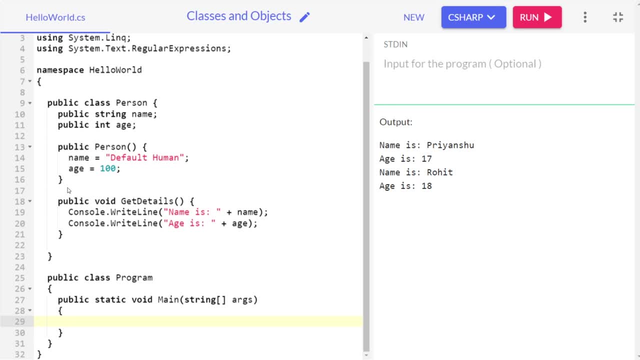 What I'll be doing is I would just, I would just be, you know, creating an instance of the class, and then we'll be calling this method directly. I won't be setting the name right now. You will see what will be the output. All right? 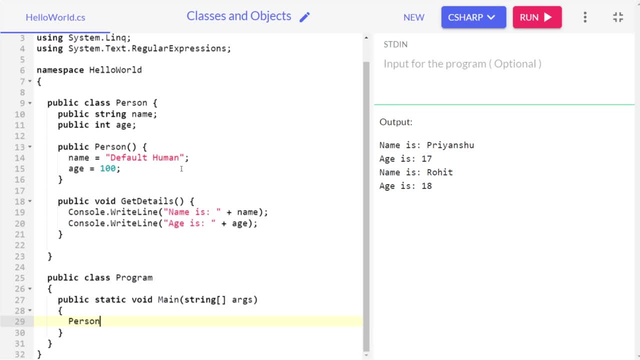 So let me show you. So, first of all, what you have to do is create- create an instance of the class. So how do we do that Person? P equals new person, All right, Semicolon, and then P dot- get details. 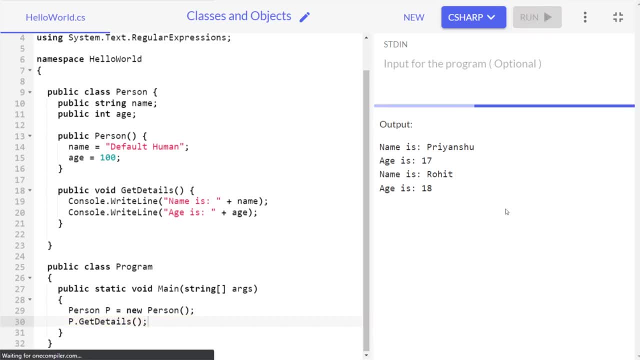 All right, And in here let's see if it works or not. So here you can see, here you can see. we didn't set set the name, or we didn't set the class name in there. We didn't set it explicitly. All right, We didn't set it explicitly. 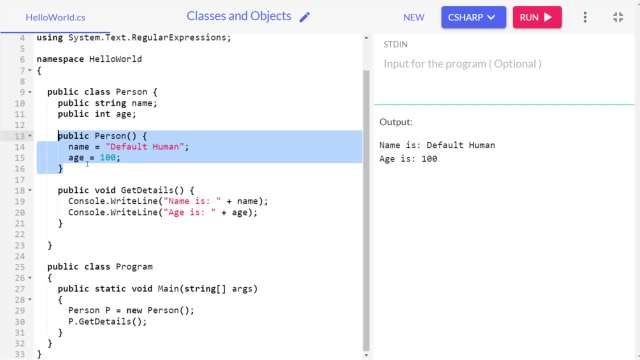 The constructor, or the constructor is called when the object is already created. So that's why, by default or by default, the constructor has set the variable name and age to the specified value And in our case, for the name, the specified value is default human. 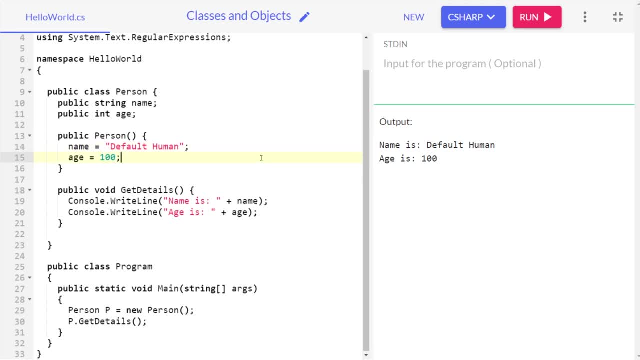 And for the age, the specified values: 100.. All right, I hope you understand that. you know the concept of, you know constructors. Now there are a few pointers that you need to remember. All right, A constructor name must match the class name. 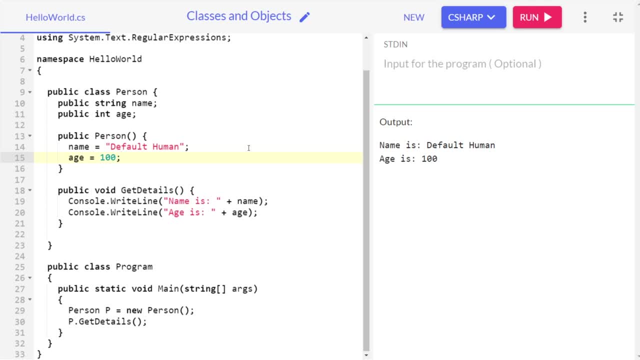 All right, And always remember our constructor cannot. All right, Cannot have a return type. All right, And remember this constructor, All right. A constructor is called whenever, Whenever an object is created or you can say, an instance is created of the class. 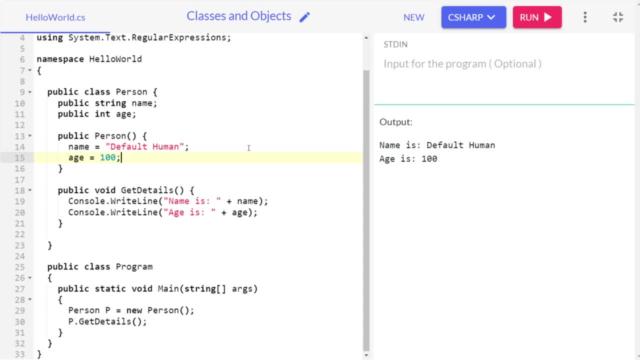 All right And always remember: See, all classes now have constructors by default. All right, All classes have constructors by default. If you don't create a constructor by yourself, the C sharp programming language or any other programming language will create a default constructor for you. 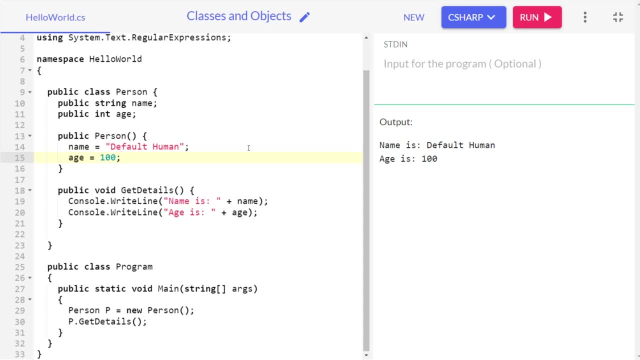 All right, By himself, All right, But the C sharp will create automatically a constructor for you. All right. However, the problem with that comes is that you won't be able to- you know- set the initial values for the fields. 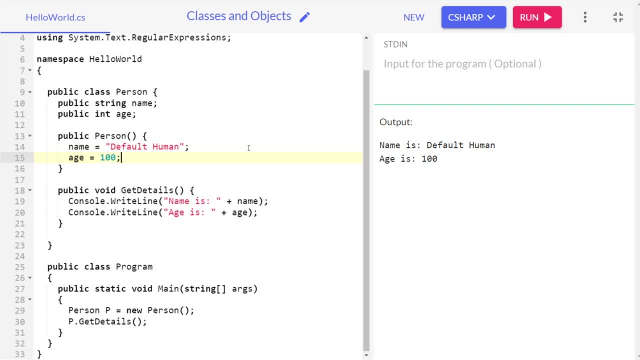 So that's a problem. That's why we can. you know, we define a means, we define a constructor manually, All right, So I hope the concept of constructors And classes and objects are clear. All right, I hope you have understood the concept of classes, objects and constructors. 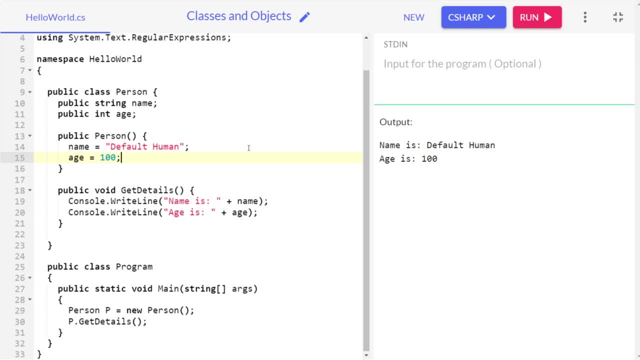 You have understood about. I hope you have understood about fields and methods, about class members. So now our next topic. All right, Our next topic is of Constructor parameters. All right, Like you know, in functions, how I told you about parameters, 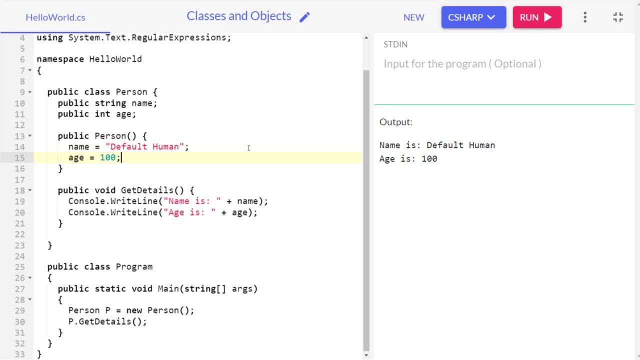 This is also something like that. All right, This is also, you know, same. So to create a parameter, what you can do is, in within the parenthesis, you can create variables, All right, That is, you can create parameters. 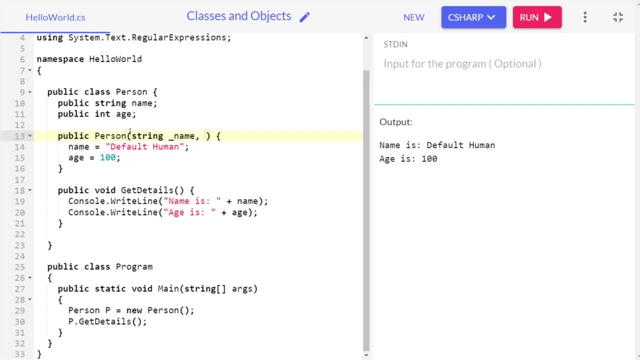 Now let's create a parameter name. All right, Let's create another parameter as age. After that, what we can do is: What we can do is we can remove the default human from name and set it to dash name and again do the same thing for age. 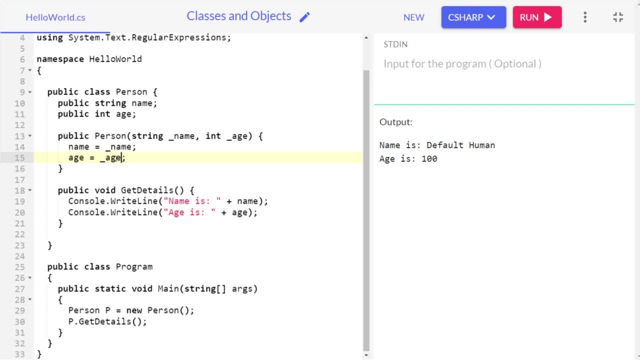 to dash age. All right. Now what is the? you know what's the benefit of it? Let me show you. All right, Let me show you the first of all. this will reduce the lines of code. All right, This would reduce the lines of code by a lot. 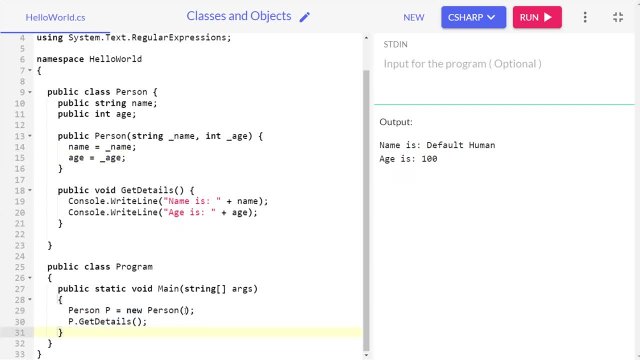 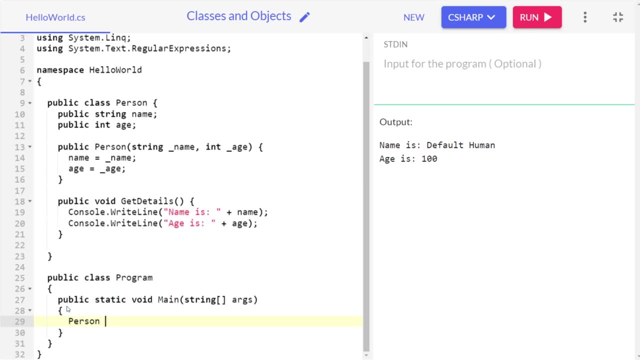 So now, as we have set the parameter, it is very simple. It is very simple, So I'm going to create another object that is, let's say, Person: All right, Person B equals new person All right. And then we don't get details. 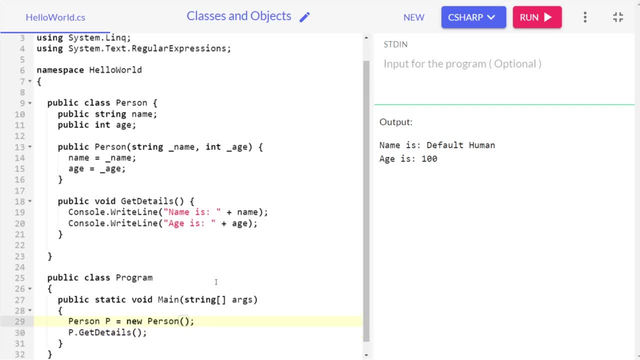 And now in here- here you can see, there are parentheses. Inside of this parenthesis we pass some value. So how do we do that? It's very simple. First of all, the first parameter is a string. So we're going to give it a string, that is Priyanshu. 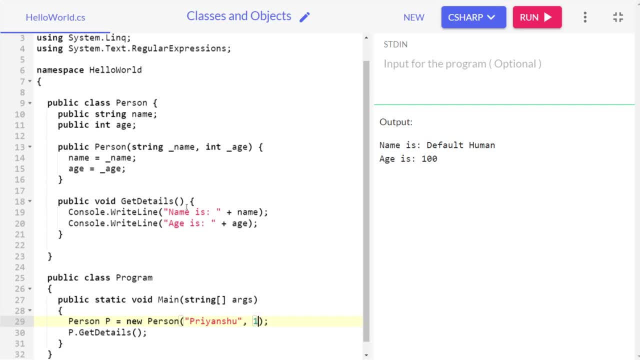 And the next parameter is age, And we are going to give it 70.. Now let's run it, And here you can see, just within two lines. like previously, we were using four lines, Now we have reduced it to two lines. So now, here you can see, we are getting the same output we got previously. 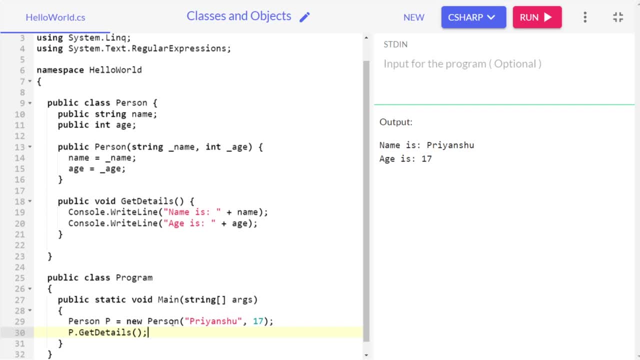 All right. So that's how they save a lot of time. So I hope, constructors, the concept of the concept of constructors, are clear to you. All right, Because the next two topics are going to be very interesting, That is, access modifiers and static keyword. 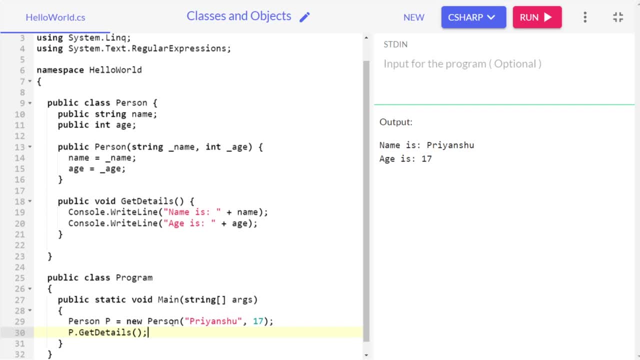 All right. So Let me show you See access modifiers basically defines from where we can access our methods and variables from. So far, there are two access modifiers that you that you should know: That is public and private. Now, public means that you know we can access the class members from outside. 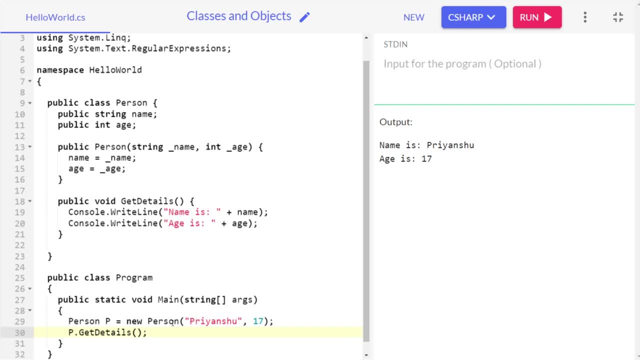 the class, whereas whereas in other side, private doesn't allow us To access the class member outside the class but only can be accessed within the class. All right, So I know it. might you know it might seem a bit overwhelming, or 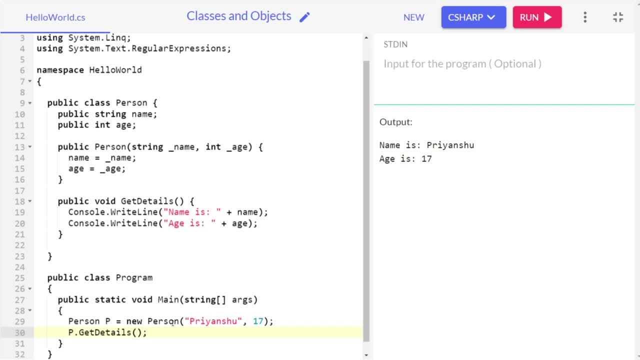 you know it might get a bit confusing, but that's totally fine. All right, That's totally fine. The thing is, I'm going to show you, show it to you, by doing it practically Now. let's remove this constructor, because we don't need it as of now. 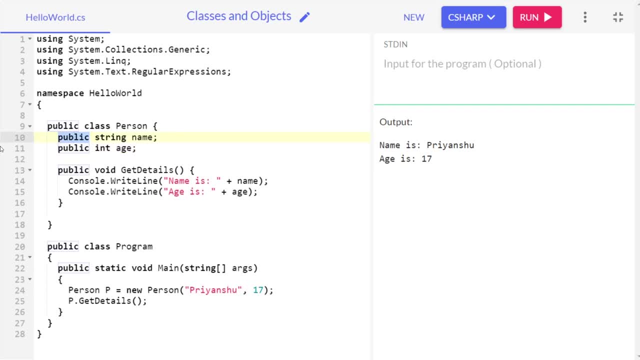 All right, Let's remove this. All right. Now in here, let's change the name. All right, Let's change the public keyword to private. All right, Let's change it to private. Now let's create another instance that is person P equals. 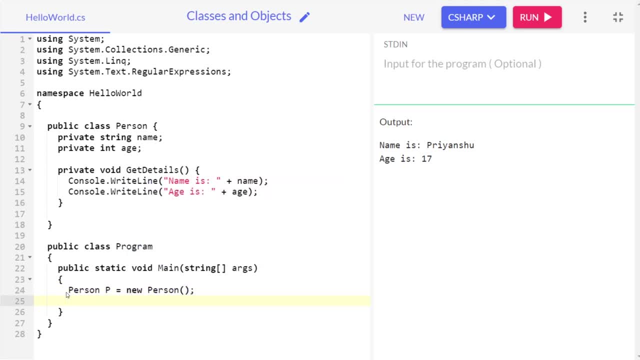 New person Now in here: P dot name equals- let's set it to, you know, Priyanshu. All right, Again let's set it to Priyanshu. And again let's set the age to, let's say 17.. 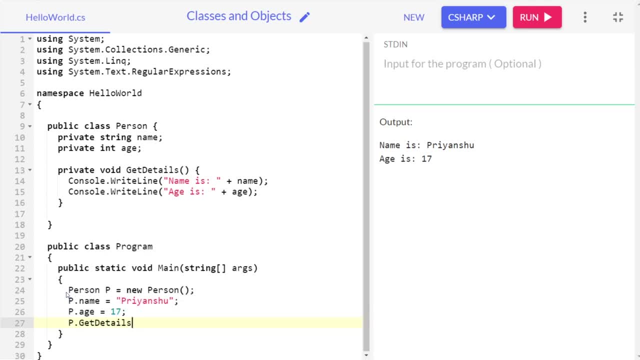 All right, And let's get try to get the details Now. let's see what happens. First of all, let me ask you: will it return an error or will it work? Will it work or return any error? Just give it a thought. 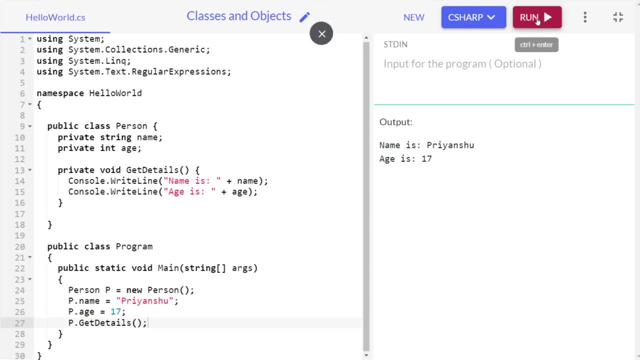 All right, Pause the video, give it a thought and then return. So I'm going to show you Here. you can see there are three errors. The errors are The hello world. All right, That person dot name means this is the name fits- hello world. 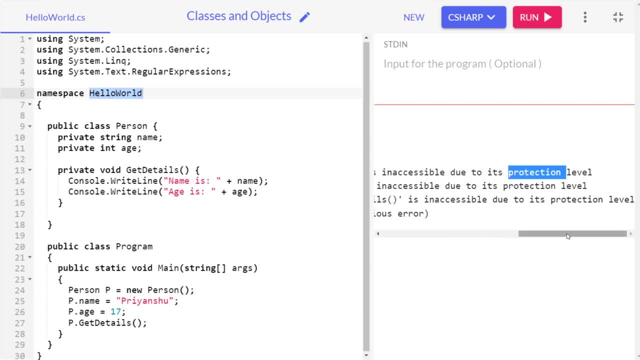 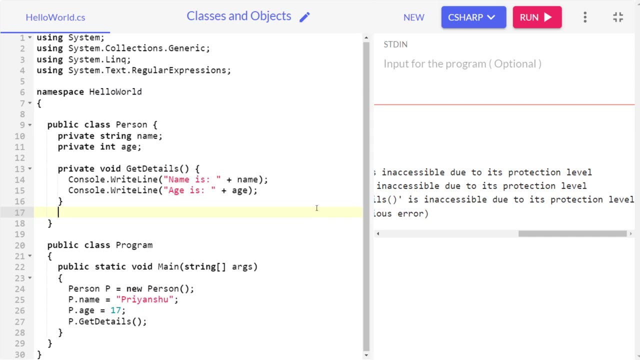 All right, The person dot name is inaccessible due to its protection level. Again, another is person dot age is inaccessible due to its protection level. The same goes for person dot get details is inaccessible due to its protection level. So, because of the private, because of the private, you know this private keyword. 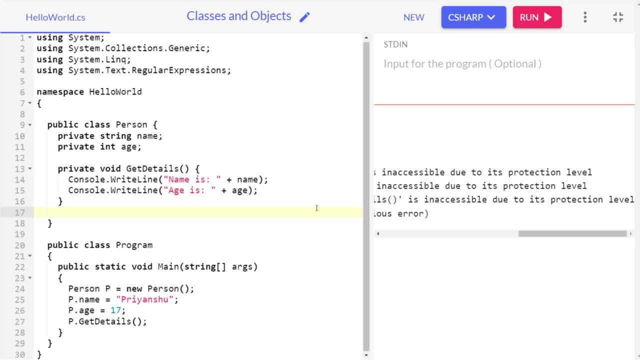 What is happening? It made our fields and methods private, So we can't access the variables and methods outside of the cloud, Whereas with public keyword we can do that Right, And let's say there's another way to you know, make you know field or method. 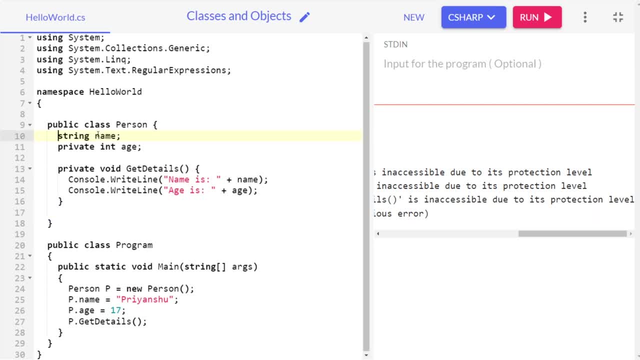 Private is that you can simply, you know, remove the private and it would be go to private by default. But you know, I don't, you know I always like to write private because I don't know, but it seems really good to write. 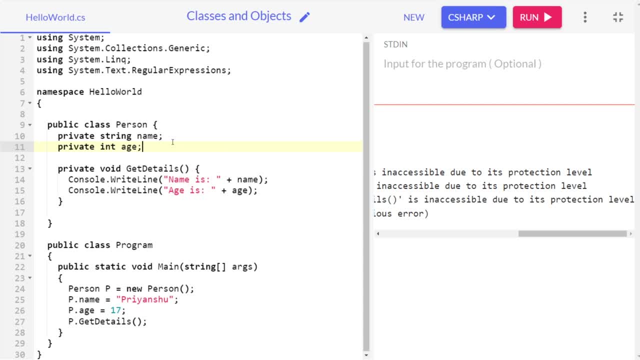 Private at first. So that's why I always write private And I also suggest you for initial stages or for initial stages, write private All right. If you are creating any private method, then for initial stages, write private All right, So that you know, you get it more clearly that what is the use of private. 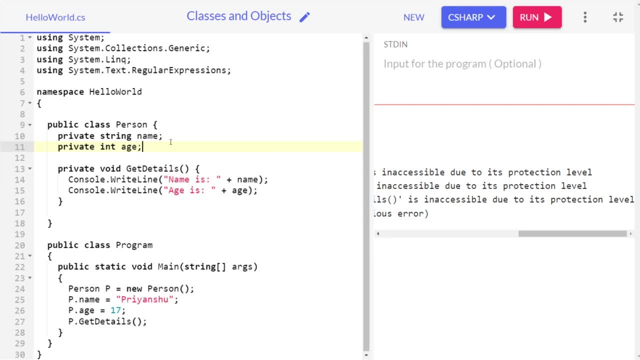 So I hope you are now clear with the concept of access modifiers. What are public and private? All right. Now there are two more access modifiers. What is, you know, protected or protected is there, And so you can, you know, learn more about them. 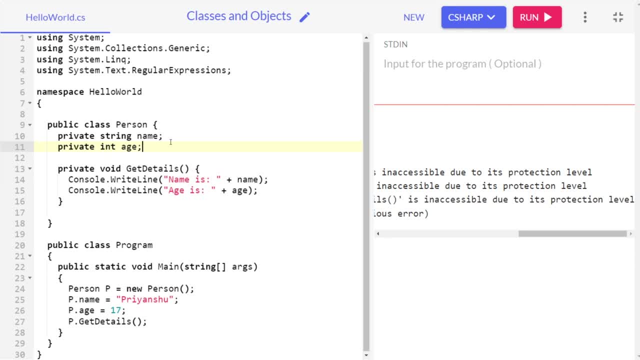 All right, You can learn more about them. You can search about them, You can learn more about all it through Google, So make sure you do that now. Next, the next concept we are going to learn is static keyword and static classes. 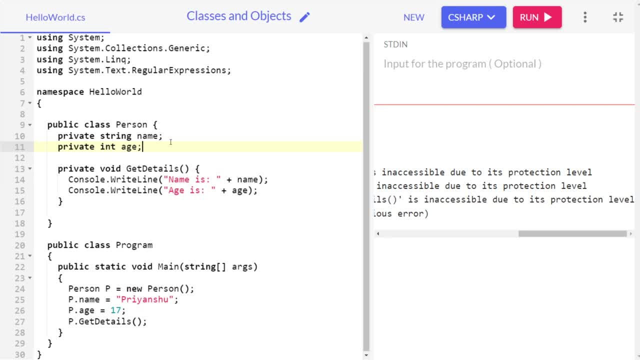 All right. So First of all, let's Understand the concept of static keyword. All right. See, the static keyword actually helps us to get access to the class members, such as variables, methods, et cetera, with it, without needing to create an instance. 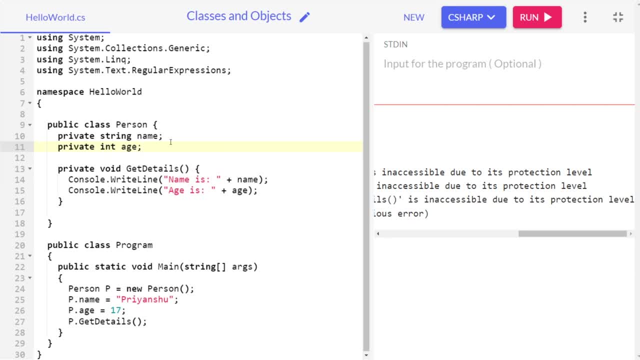 or object of the class, whereas I hope you understood this right Right now. All right, Let's make this, you know, variable to public as of now. Let's make them to public. So now, here you can see, We are creating an instance of the class. 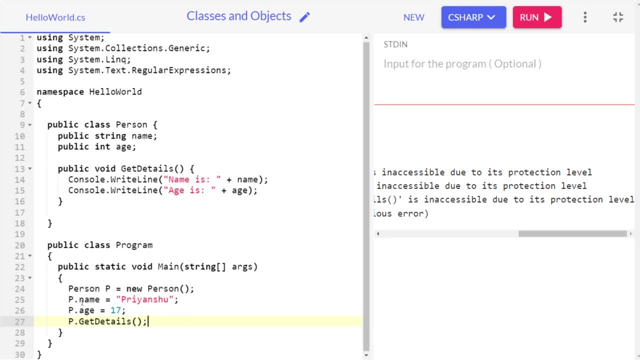 Right, We are creating an instance or object of the class to access these variables. Right, We are creating an instance of the class to access these variables. Now the thing is, if we put a static keyword, if we put a static keyword in front of every variable or field or method, like this static- 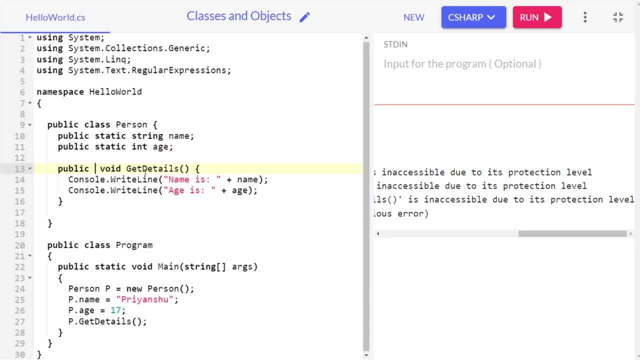 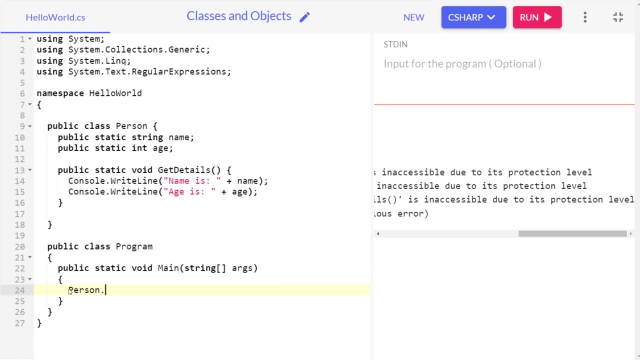 All right, Static, Public, Again public, static, And let's you know, let's not create the object. Now, what we can do is: person dot name equals Priyanshu. Sorry, Then person dot age equals 70.. 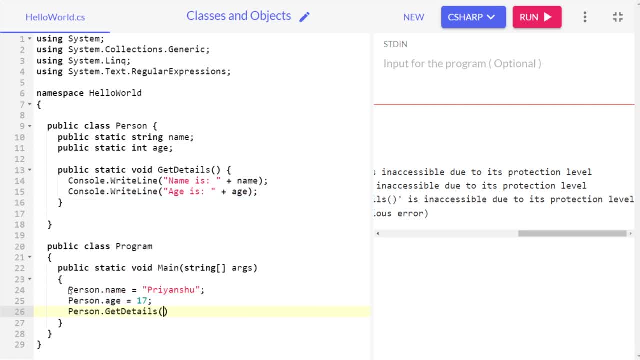 Then person dot get details. Now let's see if this works or not. See, this is working, This is totally working. Now let's again try the same thing without this. you know static keyword. Let's try it out. 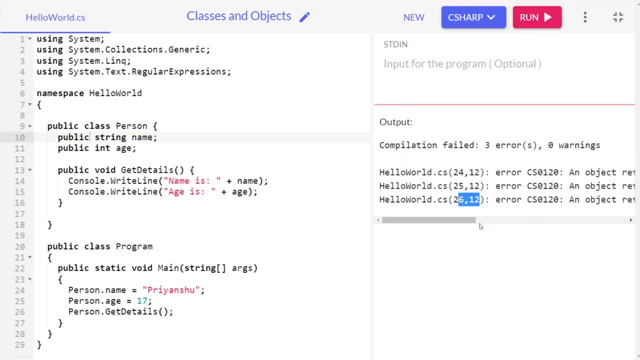 Let's see if that works or not. Here you can see, it is telling us an object reference is required to access static member, So non static member. So here you can see, Always remember, All right, Always remember If we, if we create, if we make something static. now. 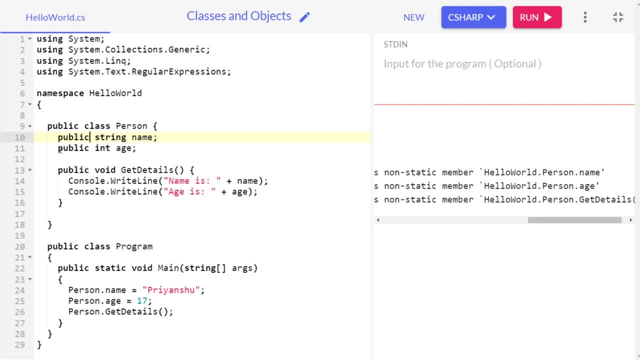 we don't need to create an object of that class to access it. We can access it directly. But if any variable, If our method is non static or like currently this, all these, all these methods and variables right in here are non static. All right, That means they are not static. 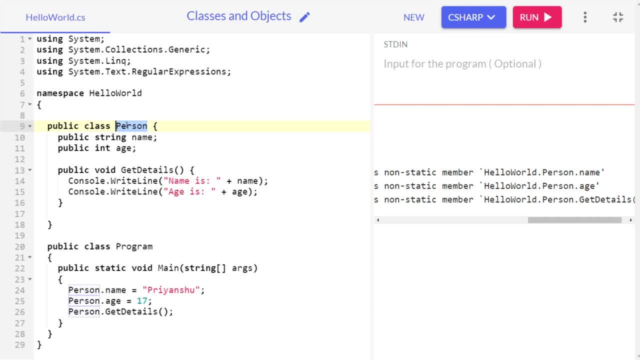 So we have to create an object of of this particular class. To you know, edit, or you can say: access all the fields and methods present inside the class, All right, So I hope you are clear about this. So, basically, what we get, static keyword helps us to get access. 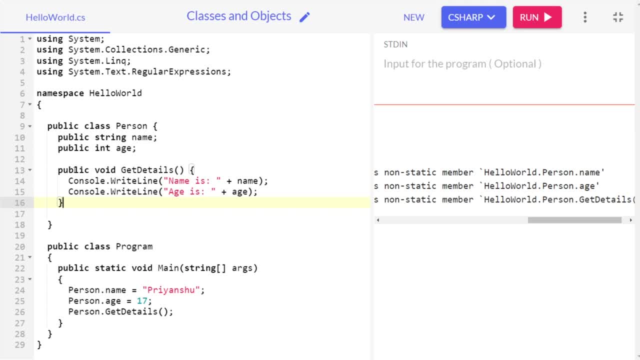 To the class members, All right, Without needing to create an instance or object of the class. All right, So that is how the static keyword helps us. All right, I hope you are clear about the static, The concept of static keywords. 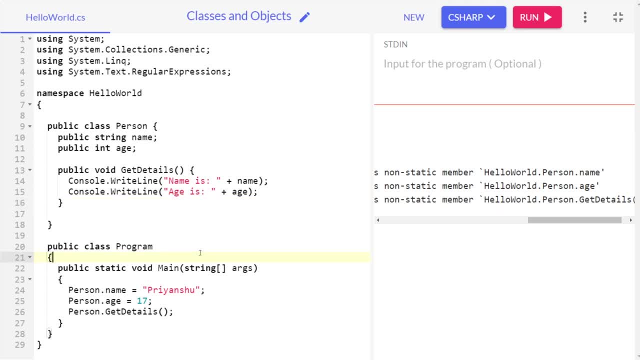 Now What we have to learn. All right, What we have to learn is about static class, And this is the last concept that we are going to learn into today's lecture. See, just like we learned about. you know this. 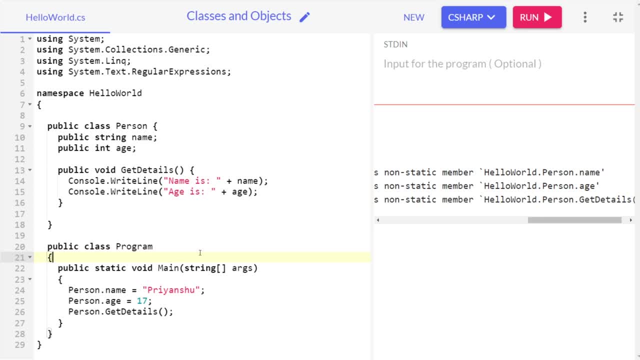 Static, you know variables, Basically, let me tell you. you know, just like having static methods or fields or properties or constructors, we can also have, you know, static classes. You know our static classes can only contain static members. 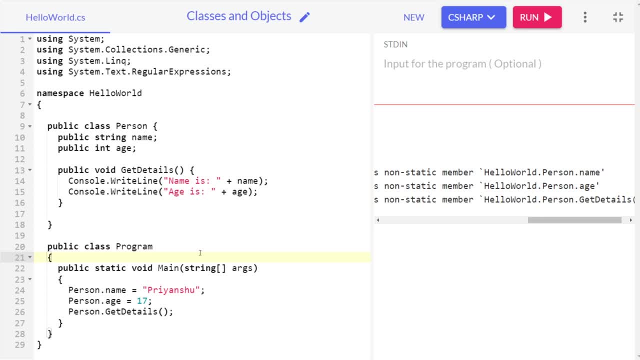 All right, A static class can only contain static members. That means let's say, if I create a static class right now and again, let's, let's, you know, Let's try the old step. What we are doing, like creating an object. 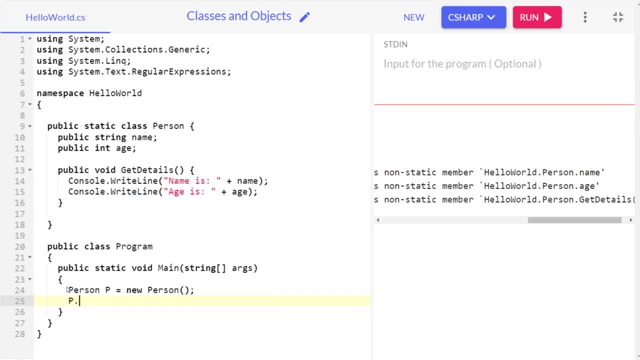 Let's do it now. Let people you know: P dot name equals. let's say the answer: Then P dot, age equals 17.. Then P dot. get details. Now you, you'll be getting an error. All right, The error is. 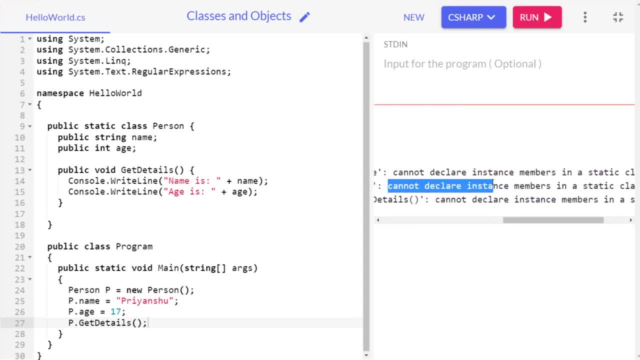 Cannot declare instance members in a static class. Cannot declare instance members in a static class. The reason? the reason is: all the variables and method right in here, All the variables and method right in here, Is non-static and let's, let's turn it to static as of now. 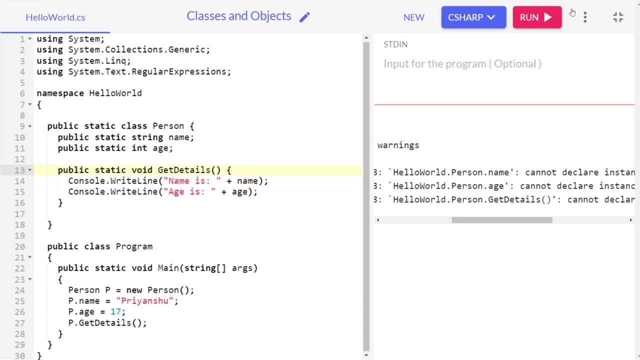 Let's turn it to static and let's see if we are getting any error or not. Here we are getting again an error. The reason is: The reason is not because all the all the variables are in here are static. The reason is because, as the class is static, we are trying to create 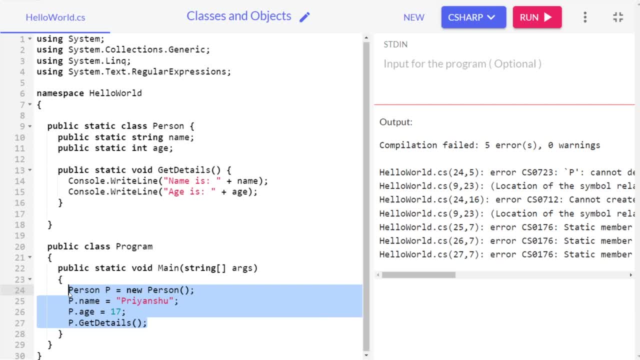 an instance of the class. and that is not possible because stat we cannot create instance of a static class. We have to do it, We have to get direct access to it Right. So for that person- not you know- name equals a. 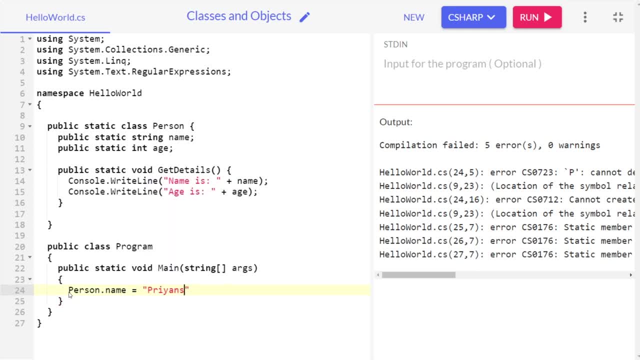 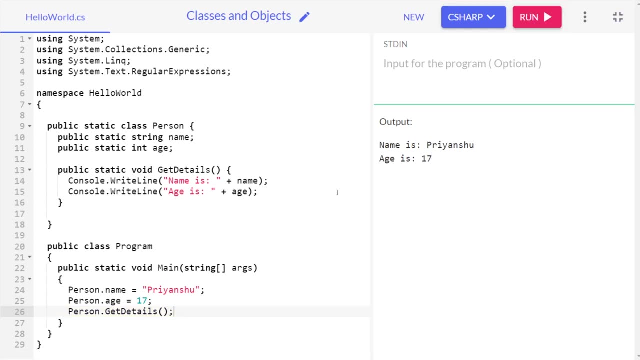 Priyanshu Priyanshu. then person dot- age equals 17.. Now, let's do it. Person dot, you know, get details as Let's see it. now See, it is working like that. So this is what a static class is. 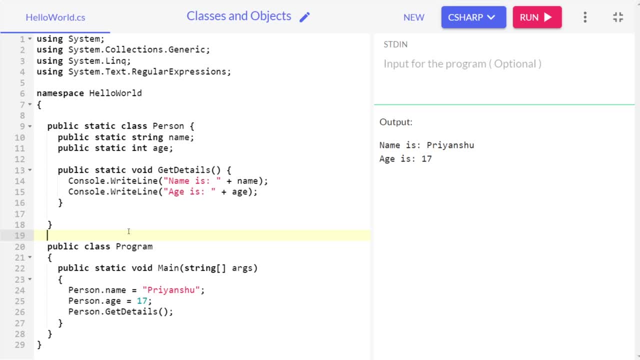 All right. So I hope the concepts of classes, objects, fields, method, class, members, then access modifiers and, you know, static classes, are clear. All right, And this is going to really help you to understand how we, you know, work with C. 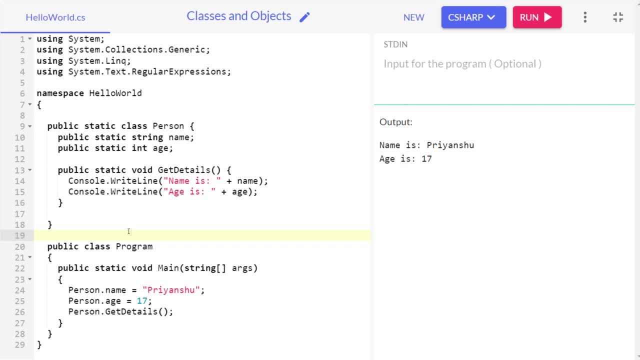 uniti. All right, So as of now, this module: all right. In this module, we have completed our lecture. We have successfully completed this lecture, All right, So next we'll be start creating our own AR application. All right, With Vuforia. 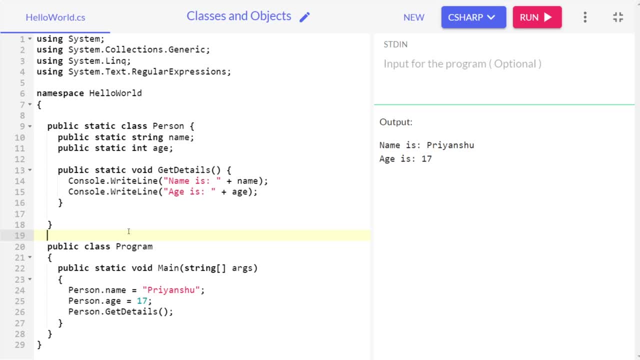 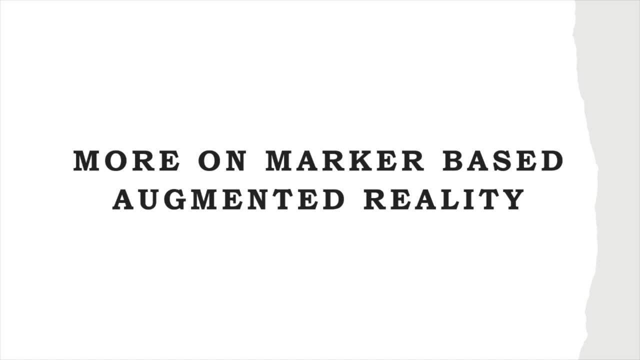 So, yeah, let's get into the next module. Thank you, Hey folks, welcome to module four. and this is the first video Of module four And in this lecture I'm going to explain you. All right, We are going to dig deeper into the concepts of market based augmented reality. 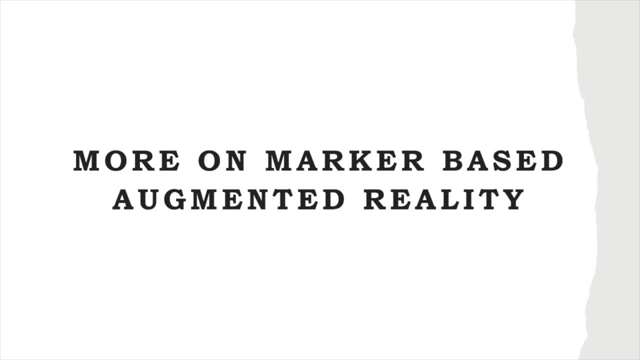 That is, we are going to learn about the architecture, We are going to learn about the available SDK, We are going to learn about how things work in market based augmented reality. All right, And later on I'm also going to tell you what you what means. 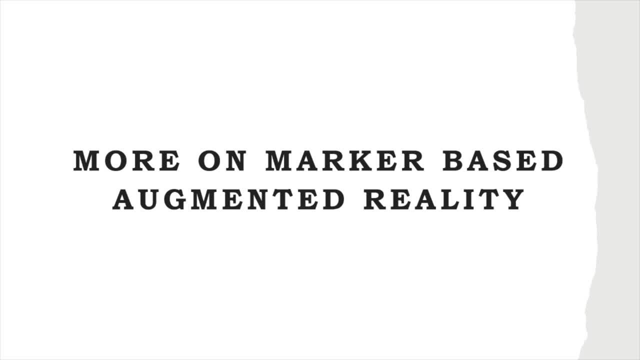 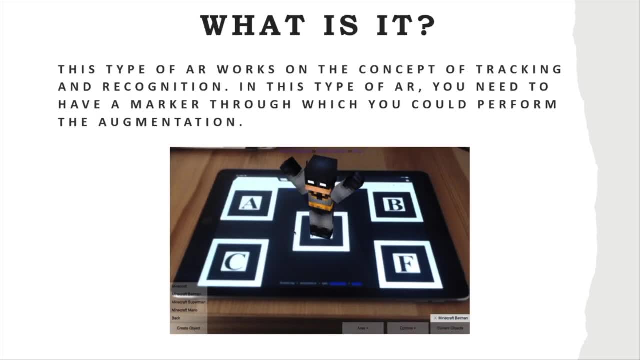 How, like? which tools are we going to use to develop our like AR applications? Right? So For now, let's get started. So what is see? first let's recap, All right. First let's recapitulate our concepts of market based augmented reality. 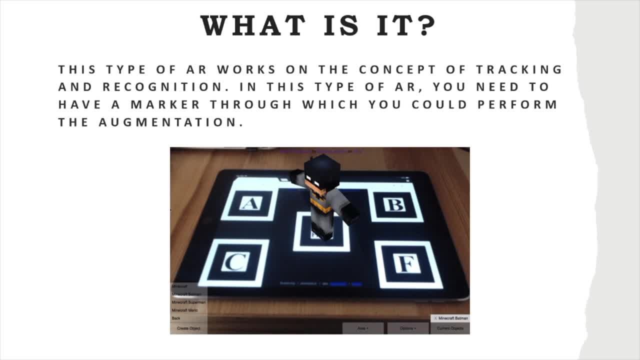 All right, See market based augmented reality. All right, This is a type of augmented reality- All right, That makes uses that, that makes use of recognition and tracking. All right, It is the property of, or you can say it is the feature of computer vision. 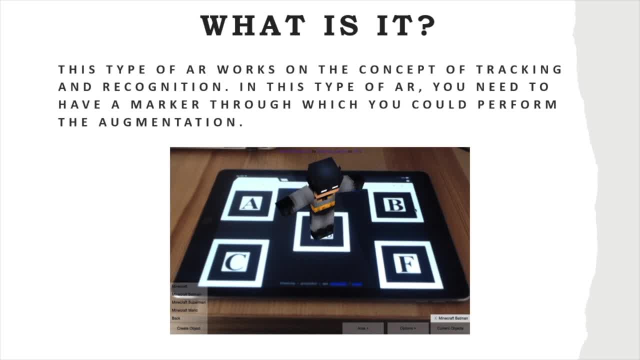 All right. So it make uses the properties of computer vision, that is, tracking and recognition, to to recognize and track a market and put all right And place or augment a 3D object or any kind of digital objects on top of that market. Right, You can even augment a video on top of that market. 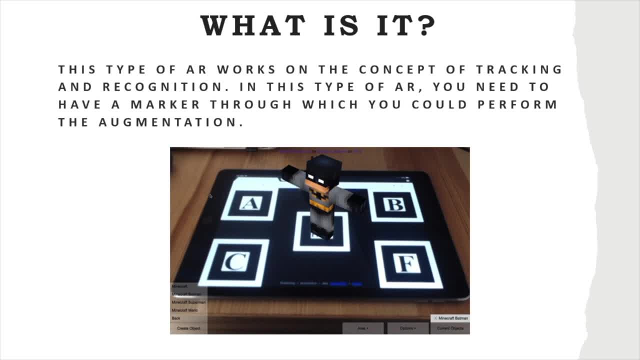 So that is what market based augmented reality is. All right. So, yeah, that is what market based augmented reality is. You can even see that. You can even see that there is a diagram. right, It's not exact diagram, but the GIF. right in here there's a mobile and there are 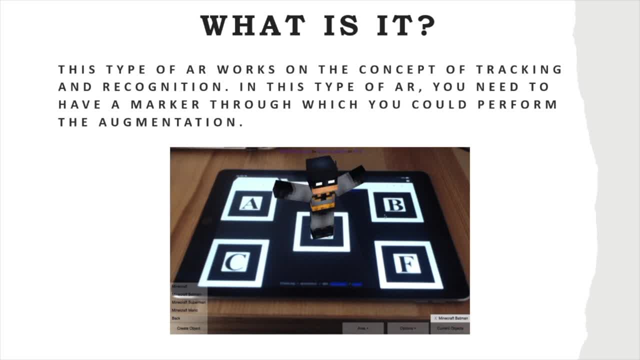 some ABCD are written, some alphabets are written and they are working as a marker. Right In the center marker, the Batman is like the Lego form of Batman is placed. So this is what market based augmented reality is. It basically makes uses of. 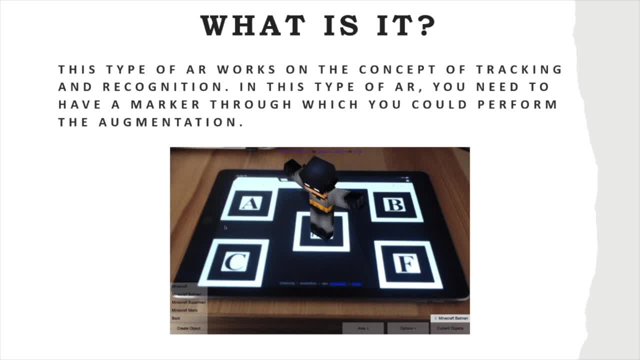 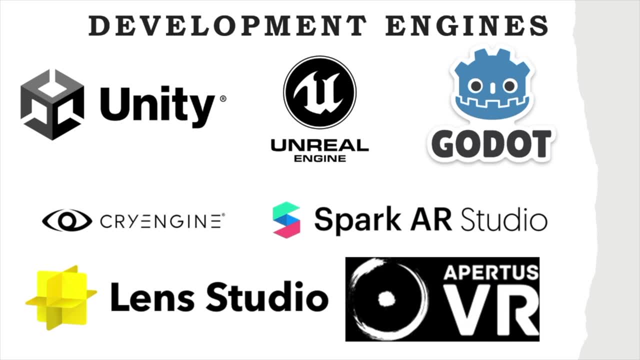 markers to augment, all right, to place digital objects into a real world. That's just it. All right, And see, we already know what a, what a market based augmented reality is. Now it is our, our very time. All right, It is our time to understand or learn about. 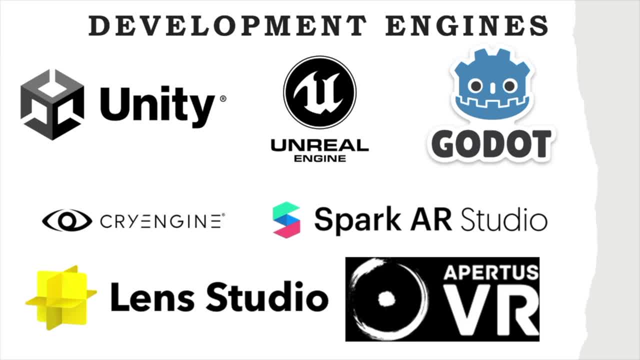 different types of game engines: all right. Different types of development engines available: All right. If we talk about there are multiple available in the market, These are just some of them. Right, I have. I have just listed down some of them. 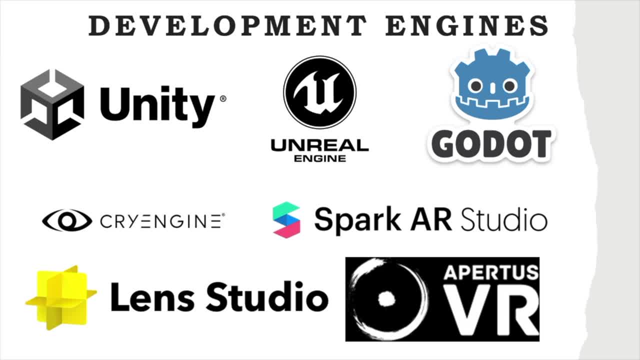 But there are many others available in the market. All right, If we talk about the things that are the engines that are available here- that is, Unity, Unreal, Godot, CryEngine- then if you want to develop your own AR filters, let's say for you want to develop for Instagram or Facebook? 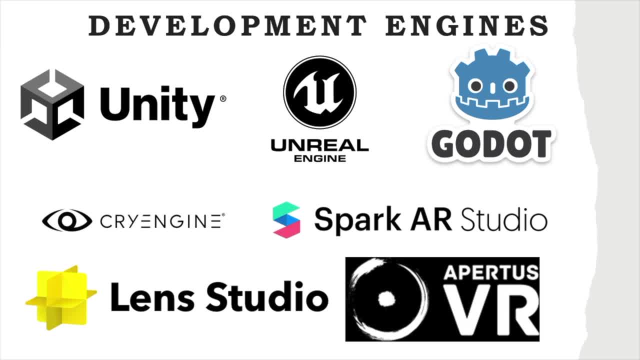 Right, There is Spark AR Studio that I am going to cover in this course also. So this is the bonus section. All right, In the bonus section, I'm going to cover the Spark AR Studio. Similarly, if you, if you are a user of Snapchat and you want to create your, 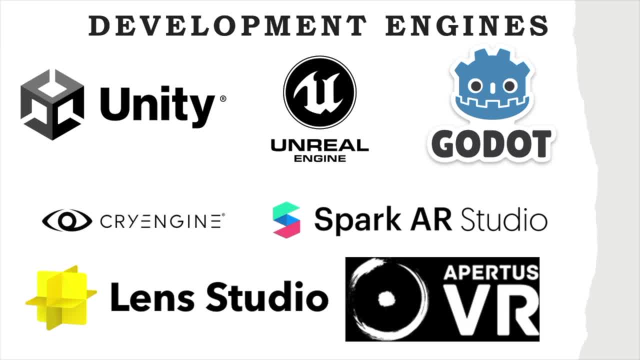 own filters for Snapchat. then there is there is Lens Studio. All right, These are augmented reality technologies, All right. Then then there is Apertus VR. Although I haven't used used Apertus VR, the engines that I have used till now. 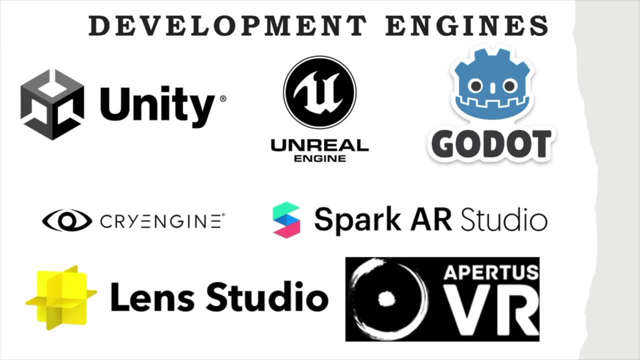 the development tools that I have used till now is Unity, Unreal, Godot. I have tried out CryEngine, but it wasn't suited for me. I didn't like it So, and another I used was Spark AR Studio. All right, I haven't used Lens Studio or Apertus VR. 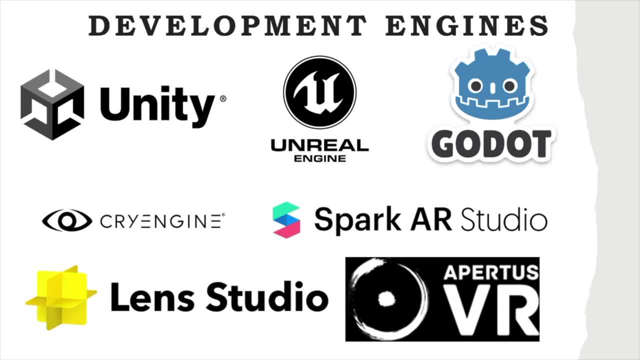 but you guys can try it out, All right. So these are the development engines that are currently available in the market And the most used all right in the. in the field of augmented reality and virtual reality and mixed reality, the most used is Unity. 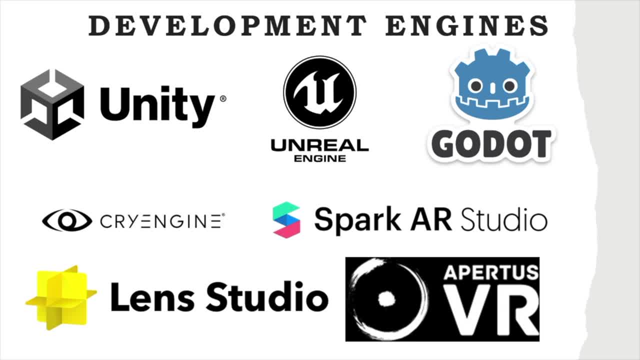 All right. Like the major major companies use as Unity for developing AR VR applications, Unreal Engine also is also used. So these two are the main like major development engines that are used. Even Godot supports AR VR. You can- even you can- try it out. 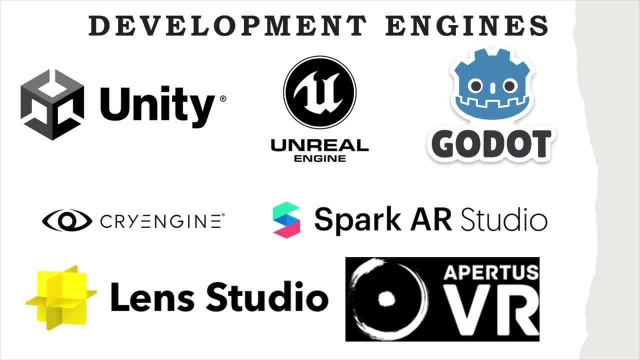 Same does CryEngine. they also support AR, VR- All right, So you can try these out, All right, And in this course, I am going to teach you Unity. All right, And we are going to cover the AR part with Unity. 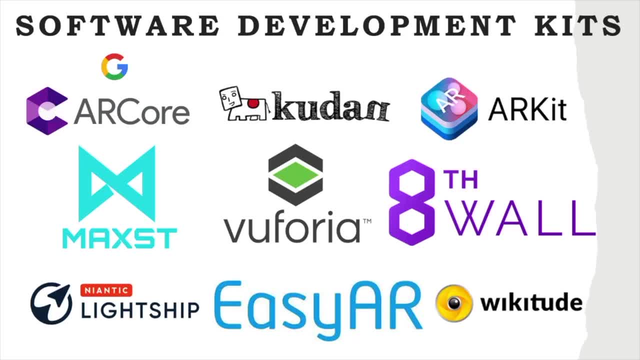 All right. So as we have learned about the development engine, now it's our very time to learn about the software development kits available. All right, Here you can see there are multiple available, like Google's AR code. Then there is Kudan. 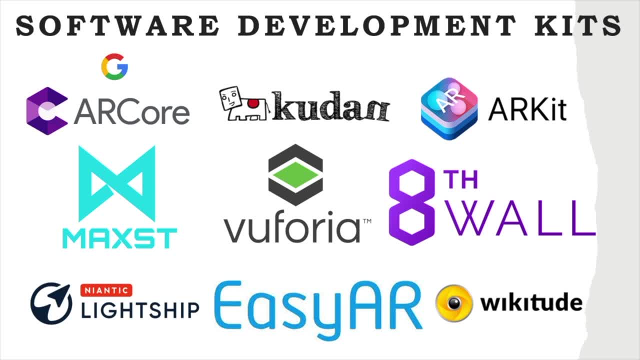 Then there is Apple's AR Kit, Then Maxed is there, Then Vuforia 8th, Wall XR, then Lightship ARDK, then Easy AR is there And Wikitube is there. Right See, these are software development kits, that is SDK. 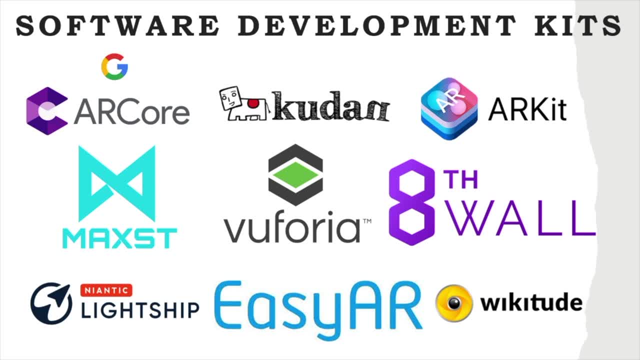 They come in packages. All right, They come in packages, All right. And in this course I'm going to cover the Vuforia. All right, I'm going to cover Vuforia, As Vuforia is very famous and very good for market based AR. 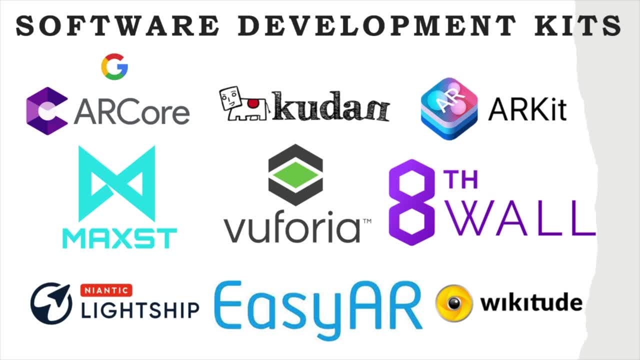 And it is also easy for beginners. So it is better to cover Vuforia in this course. So I'm going to cover Vuforia, All right, And the tracking tracking feature of Vuforia is better than any of these. all right means better than any other. 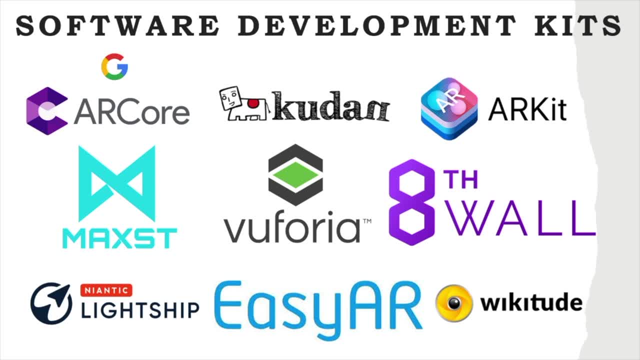 market based AR technologies. All right. So that's why I'm going to cover Vuforia in this course, And also if I tell you which SDKs have I have. I tried, I have tried out AR code. I have developed multiple apps with it. 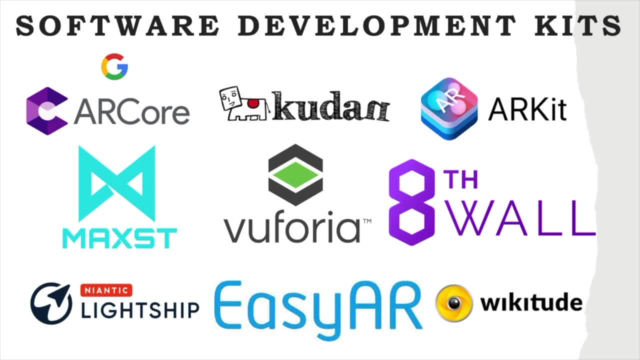 I have tried out AR kit, that is, Apple's. Then I have tried out Vuforia, of course. Then I have tried out Aethual XR, although I didn't like it much, but it's decent enough, All right. Then I have also tried out Niantic Lightship, AR. 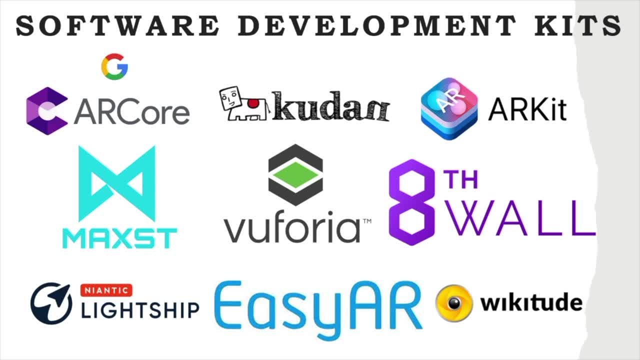 All right, It has just launched, like it has launched on 8th of November. Currently it is in beta. All right, If you want, you can go through the documentation and download the SDK and try it out. All right, So Niantic has launched their 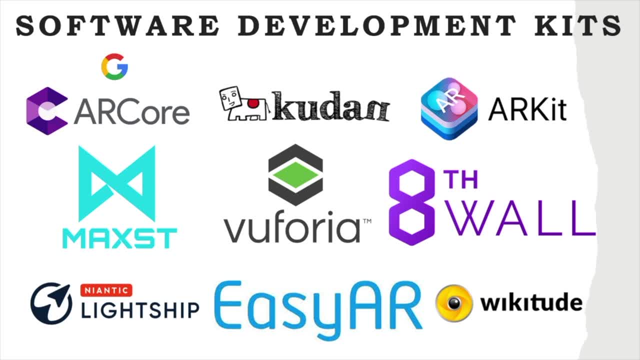 own Lightship SDK. Niantic is the same company who developed Pokemon Go. All right, So they have released their technology behind Pokemon Go on the like publicly. So I would suggest exploring the Lightship AR SDK. All right, And yeah, I have tried these. 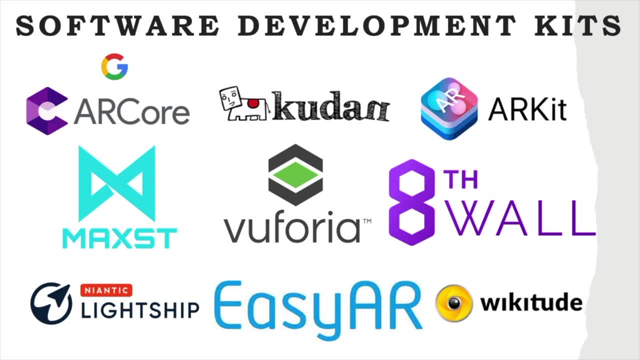 All right, But if you want, you can try the others also, Like you can try out Kudan, You can try out Max, You can try out Easy AR, Wikitude and all these available in here. See, these are not just all right. 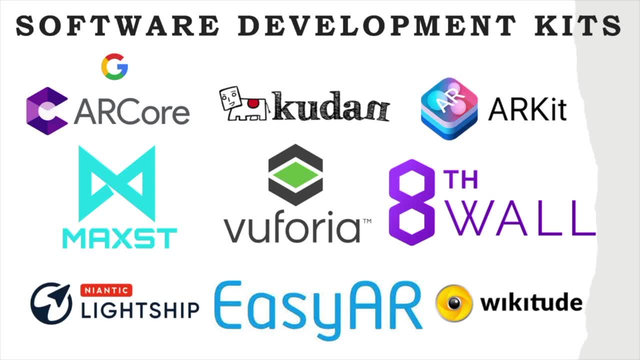 I mean there are many others also, All right, Like I haven't listed all of them, but there are some of them that I have listed, All right. So try to do some research. All right, Do a research by yourself and find out. 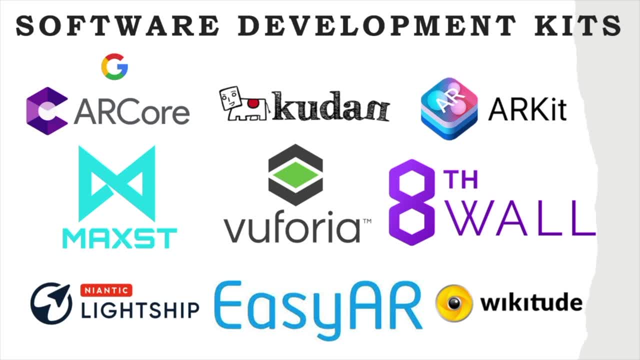 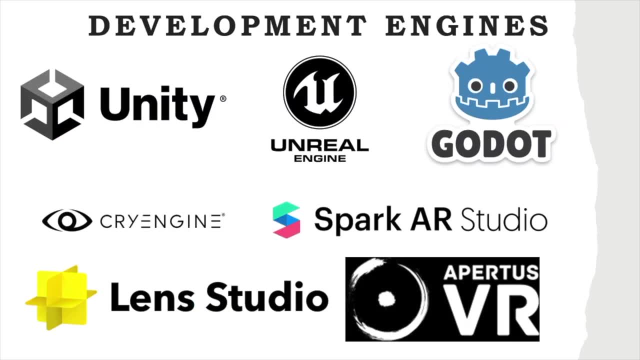 what more SDKs? AR SDKs are available in the market- All right. So yeah, these are the SDKs that are available. And in the development tools? All right, In the development tools I'm going to use Unity. 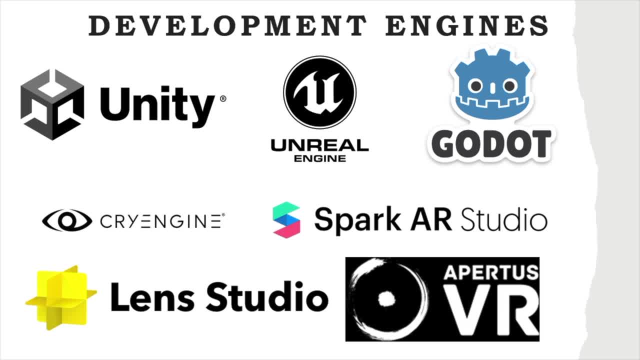 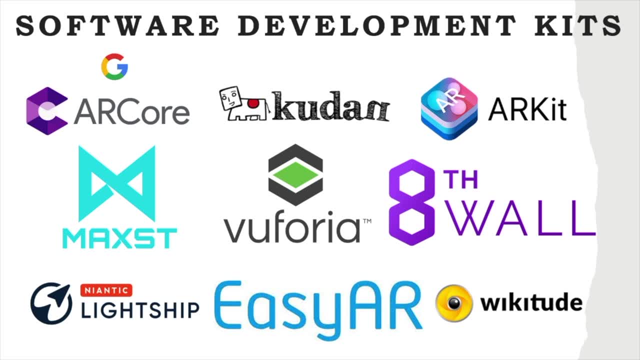 All right, I have already taught Unity, And in module two and in module four, I'm going to teach you Vuforia. All right, So we are going to for this course, we are going to, we are going to cover this whole course in. 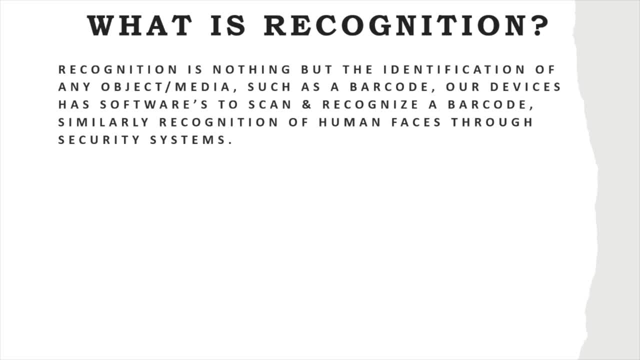 Unity and Vuforia- All right. So yeah, let's get a dive into the concepts. All right, See what is recognition? All right, What is it? Think of in human terms? All right, Just think of in human terms. 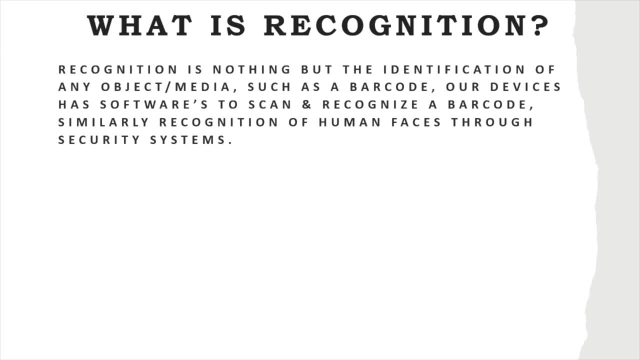 See, a person is coming to you. All right, He is the person, is your relative. All right, You know. you know the face. All right, It is stored in your brain. All right, The face of that person is stored in your brain. 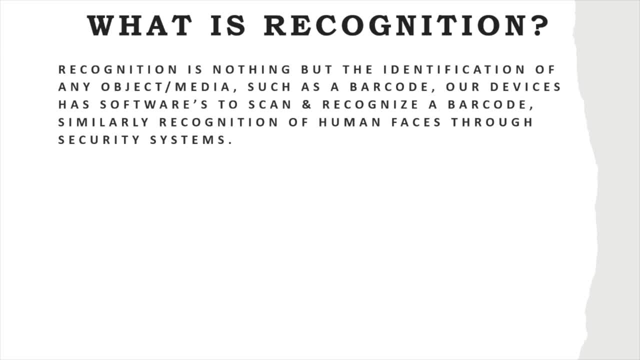 Now you can recognize that person. Right, You already know that. Right, You already know that. So that's how you are recognizing Right. That's how you are recognizing the person. Yeah, This person's name is ABC And he works at this ABC company and this and that. 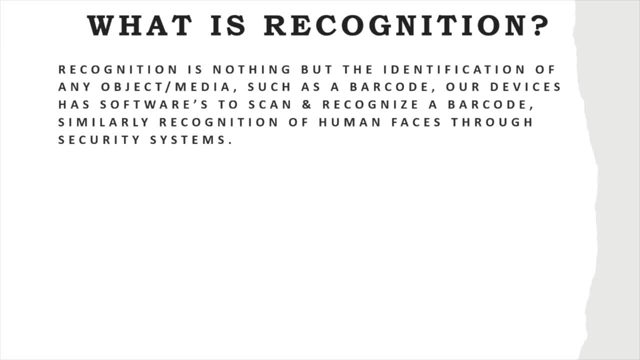 All right, You know that person, You are able to recognize it. Similarly, if you think about devices, All right, Let's say barcode devices. Right See, if you buy any sort of product, All right, Let's say we go in a mall. 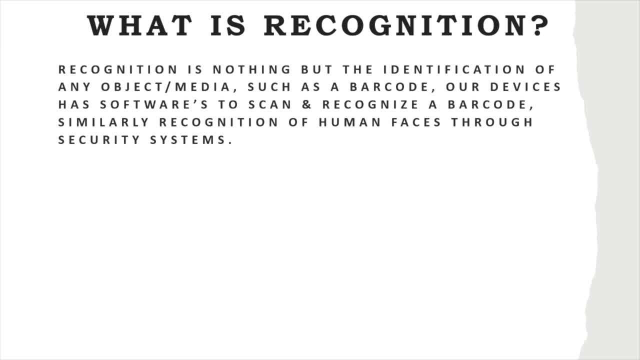 When you buy any sort of product, you submit it in the counter to make the bill. All right, What they do, they have some sort of reader, Right? I exactly don't know the name. I think it is called barcode reader. 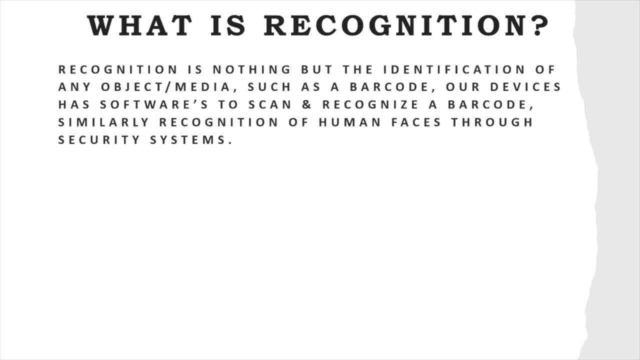 So what they do? They, with the help of the device. they read the barcode, All right, And then push the object or the thing that you are buying forward Right And make the bill. So how, the how the device is recognizing the barcode. 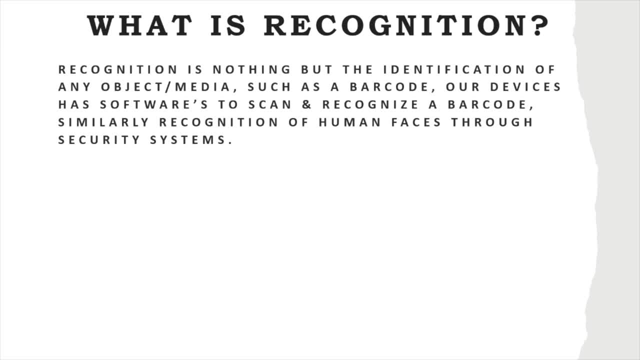 Right, Because the device already knows, like it already has the data about the barcode. Right, It already does have the data, So that's how it is recognizing it. So let's say I have bought some some. Let's say I bought a pair of shoes. 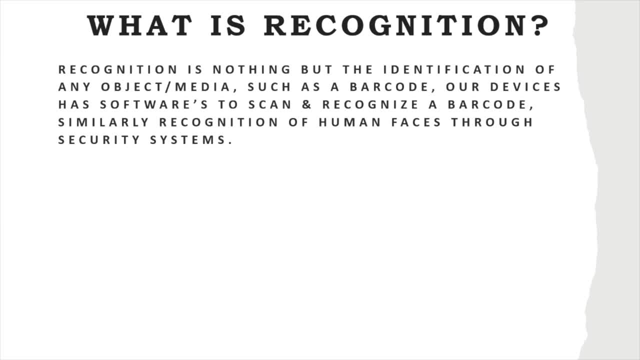 All right, And there is a barcode, The person I have submitted in the counter, the person scanned the barcode and pushed the shoe forward for the billing. All right, So the particular barcode is stored on the database. All right, So that's how the barcode reader recognized it. 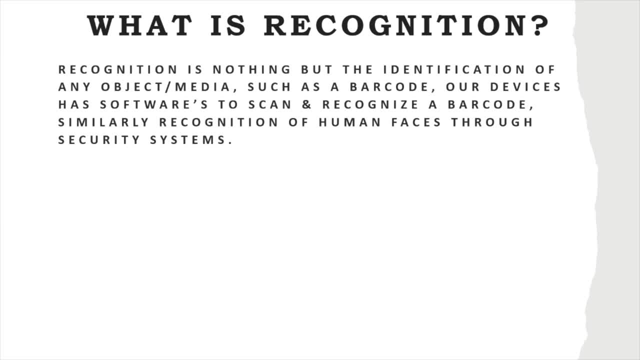 Similarly, if we talk about face recognition system, same thing works, Like in big, big companies. they use face recognitions also Right To verify the employees. Right, They use fingerprint recognition also. So these are stored in the database and some algorithms are there. 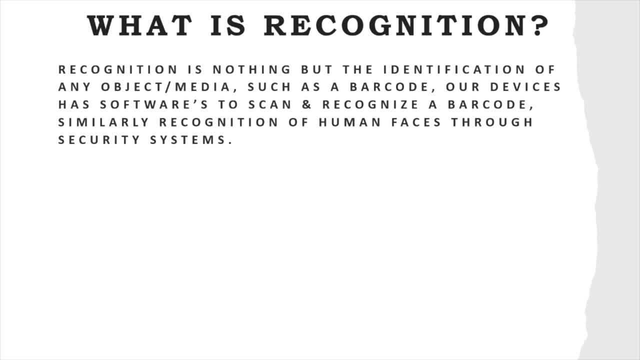 There are some algorithms, some computer vision algorithms which, which are able to recognize the person Right. Similarly, in AR also, there are some sort of databases. All right, In marker based AR there are some sort of databases, Databases in the sense there are markers. 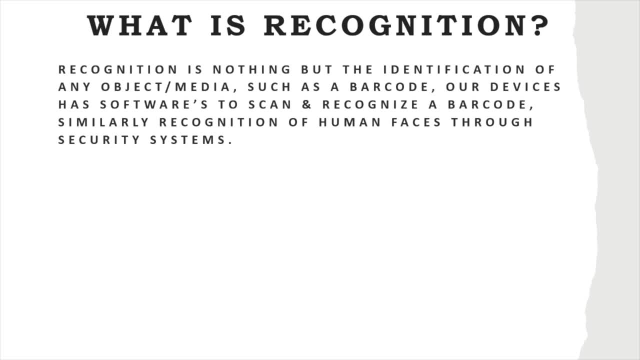 All right, Those markers are stored somewhere. Those markers are stored somewhere And our app- and we design our app in that way. All right, In a way, we design our app in a way so that it can recognize, it can recognize the marker. 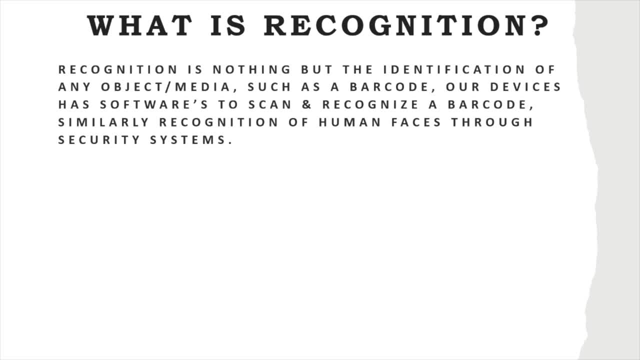 If the marker isn't in our database, then it won't be able to recognize it Right. And if it is not able to recognize it, then how would? then? how will it put the marker like? how will it put the marker on top of that? 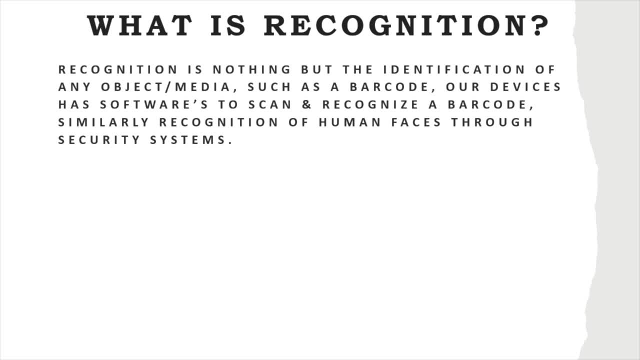 Sorry, put that object on top of that marker, Right? How would he do that? How would the algorithm, how would the SDK do that? So it is always important to, whenever working with marker based AR, we have to put a marker on the marker on the app's database. 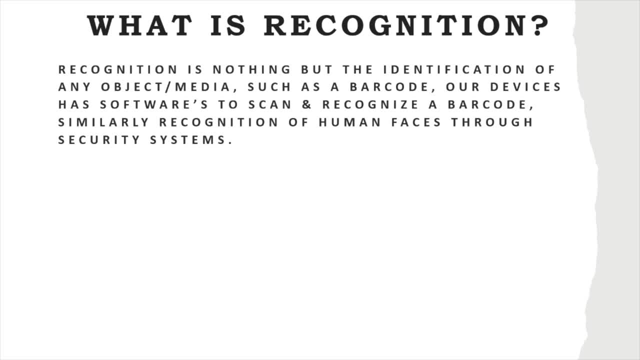 And, don't worry, we are going to see how this is done. All right, There's a very basic of euphoria only. So, yeah, So that's how recognition works in marker based AR, And this, this process, is valid in multiple ways. 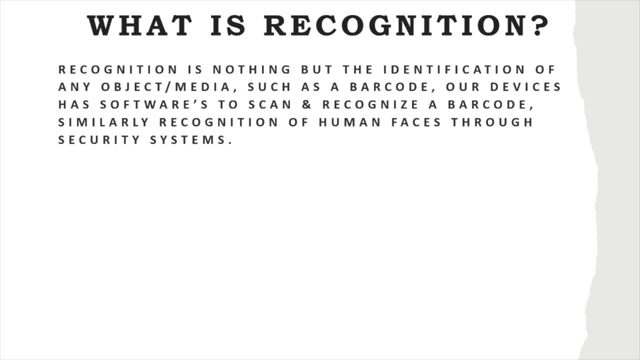 Right. So this is what recognition is. Recognition is basically recognizing something that is in the database, like in our human mind. All right, If I, if I see a person, I, I, I might know the person Right, Like I know my brother. 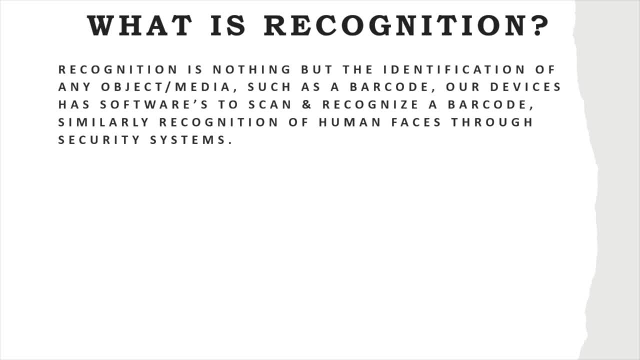 All right, He's a person that is in my brain's database, Right? I know that person, So I will be able to recognize it. All right, Now let's say some new person will come. All right, I won't be able to recognize him. 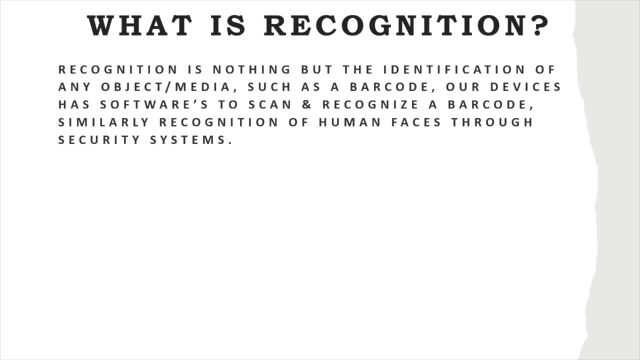 Right, I won't be able to recognize that person if it was a random person, because I don't know the person. his his details aren't stored in my database, Right? So these things work something like this. All right, So this is what recognition is. 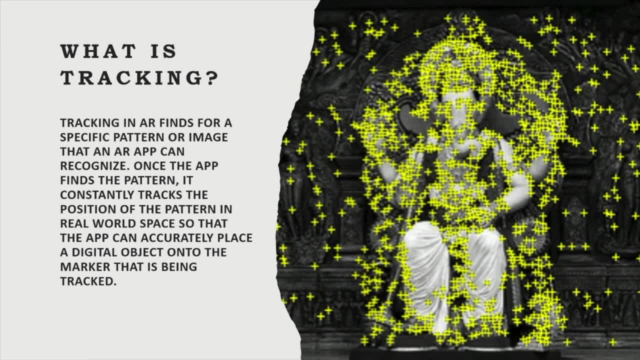 Now, if we talk about tracking, All right, See, this is a, this is an image. All right, This is the image of Ganesha, Lord Ganesha. All right, And you can see multiple plus. Right, You can see multiple plus are there. 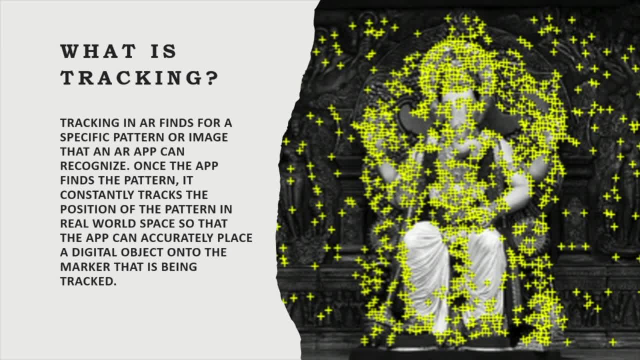 Do you know what is this? These? these are basically the trackers. small, small trackers. These are feature points. you could say, All right, These are feature points of the image that help us tracks. All right, That helps tracking the markers, All right. 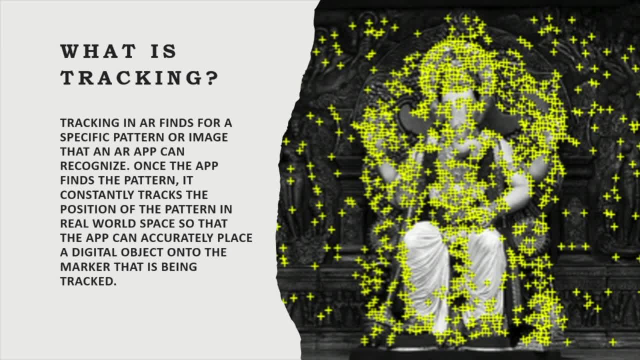 That helps tracking the marker. How does this help See? basically, whenever, whenever we upload a database, all right in our database system, all right in Vuforia, in Vuforia's dashboard, after you have uploaded your image in the database. all right, you can. you can view the tracking points. 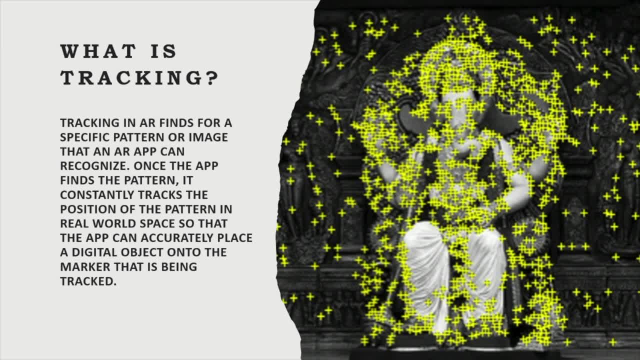 All right, This is an image from Vuforia. only Like I means, I uploaded this image on the database so that I could get the feature points. All right, I can. I will even show you how to get that feature point, how to see the feature points by yourself, Right. 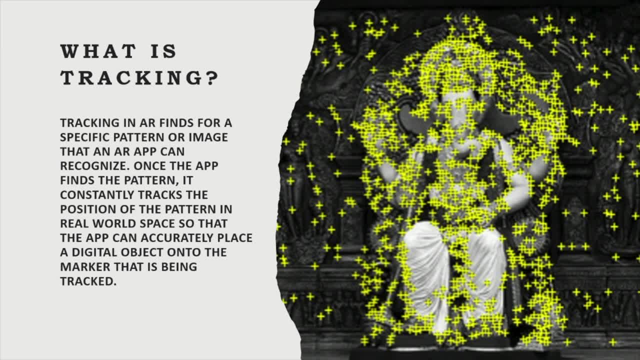 In the next video only. So these feature points: all right, these are some sort of patterns. You could say: all right, see the tracking. all right, the tracking technology, all right. in AR basically finds all right, they try to find some sort of pattern. 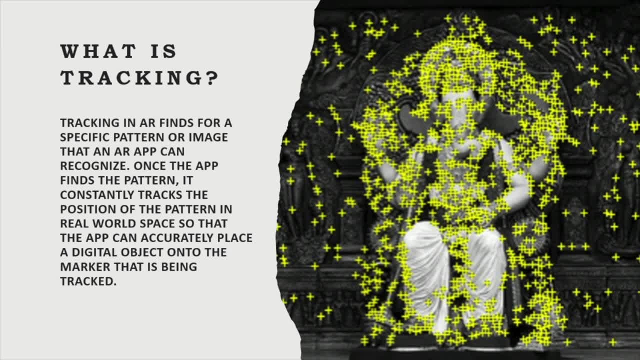 All right, These feature points are useful for tracking and recognition. All right Means see if the how would see if I had to give an example. All right, You, you have created a marker. All right, You have successfully placed all that. you have successfully placed the digital object on top of that marker. 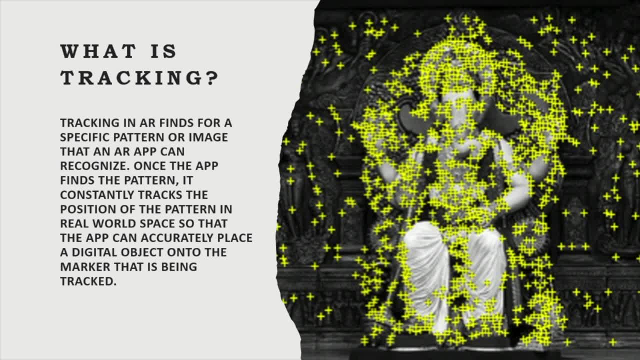 All right, You have successfully placed the digital object on top of the marker. Now how do you think will the like if I, if I move my, move my marker on onto, let's say, 10 units to the left side? All right, 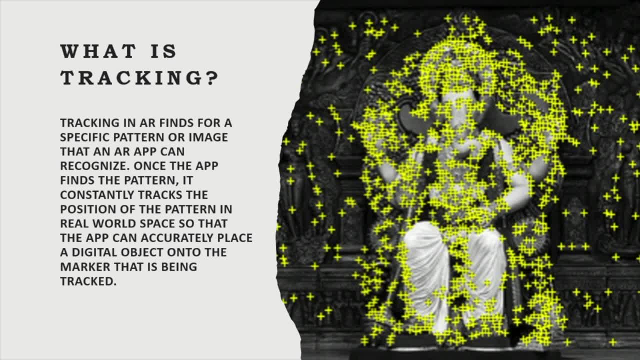 How do you think the object will also move? Because, yeah, yeah, it is recognizing the marker. right, It is recognizing the marker, That part is done and it has been placed on top of that marker. But when we will move our, our marker from one place to another? 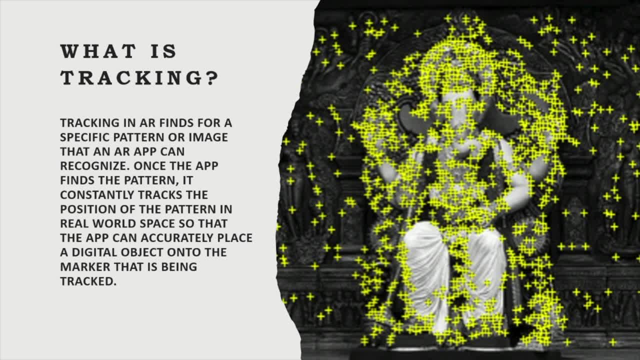 All right, How will, how will the digital object move? Can you think of it? That's where the tracking helps. All right, How it helps. See There, you can see the feature points right. Here are the feature points, All right. 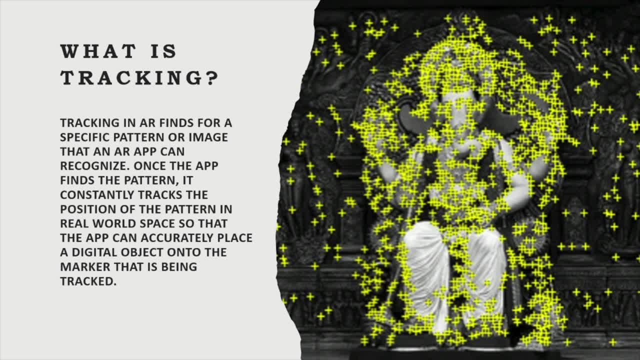 These feature points helps the marker or it helps the app to to track the track the marker or to keep the marker in track and also move, and also move the particular digital object along with the marker If I am moving, or if I am moving the marker to the left. 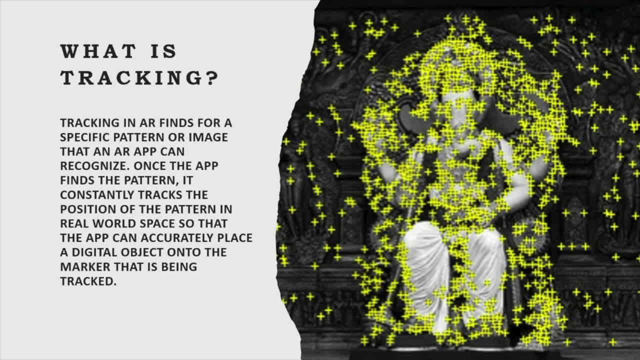 All right. Let's say I have moved 10 units to the left, All right, So the same thing will happen with the object also because the marker has moved All right And our app has tracked that the current position of the marker is 10 units from the center. 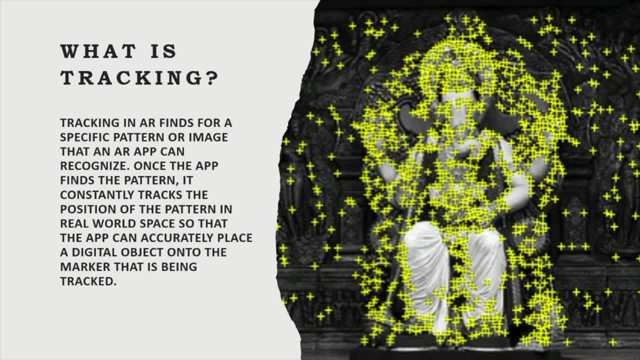 Right. So what our app has done? it has tracked and again placed it in there. All right, Although if you try to move it, the object will also move with itself. It will be a smooth like. it will be really smooth. So that's how tracking is. 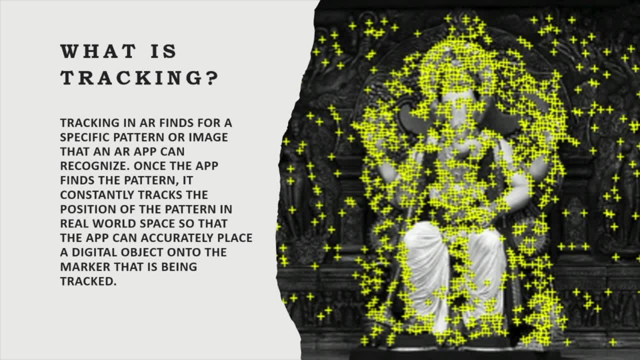 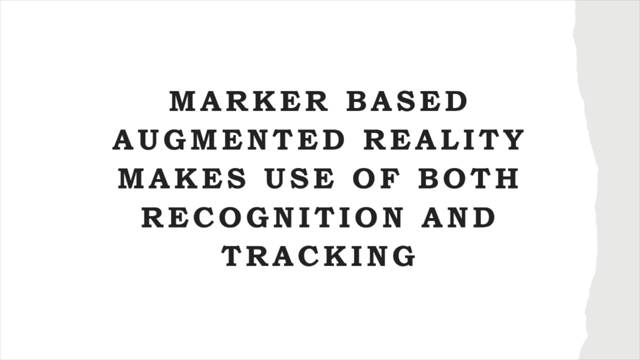 So tracking helps in marker based augmented reality, All right. So tracking and recognition, All right. These two are very fundamental and important technology of marker based augmented reality, All right. So, yeah, I hope you have understood that what is recognition and what is tracking, and how they are helping in a marker based augmented reality. 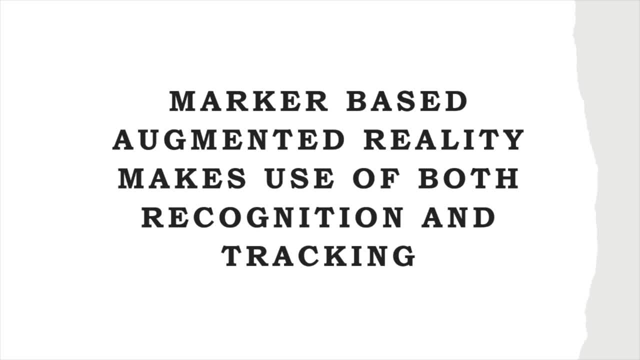 All right. So, yeah, the same thing. it is written here. The augmented reality makes use of both recognition and tracking, All right, And you and now, you know how it makes use of them, Right, Why it makes use of them. 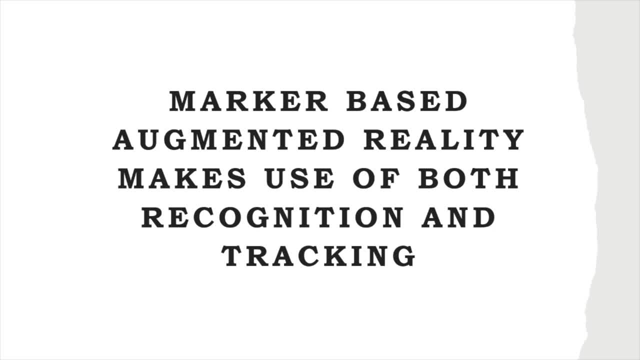 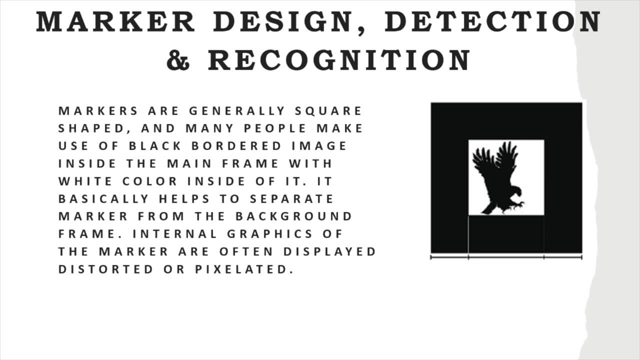 What is the use case of them? Right, You know right now, So also before moving to the next section. All right, So do subscribe my channel, All right, Because it helps me to bring more videos. All right, More courses for you for free, All right. 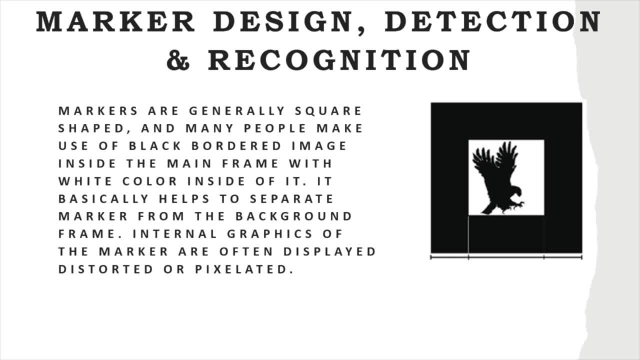 And also join our Discord community, All right. And if you have any doubt, all right. if you have any single doubt, join our Discord community, you can ask. in there We are, we, we will be helping you. in there. There are many like minded people who are, who will, if I'm not available for some. 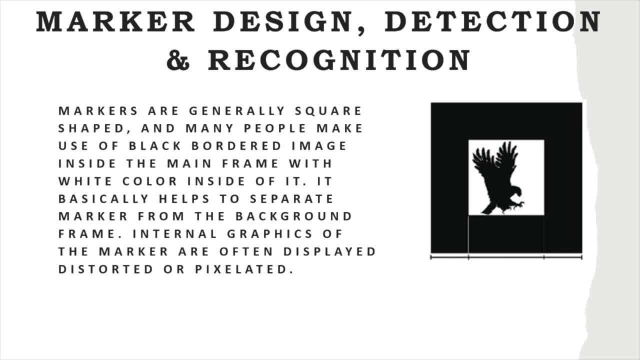 time, then they will help you to figure your doubt. So make sure to join our community And if you have any doubt you can ask in there. All right, I would like to help. And also, if you, you can even comment or comment down in the comment section that 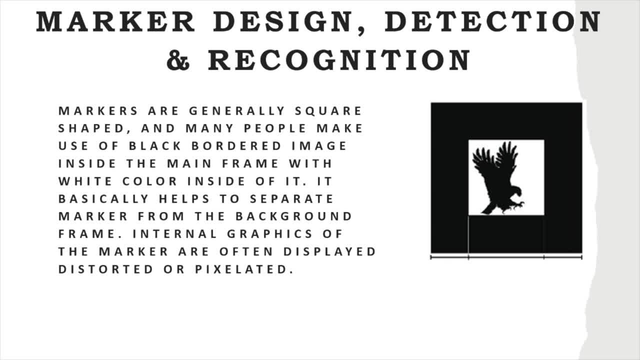 what your doubt is, and I would clear that right in there. All right. So now our here is another topic, that is, market design, detection and recognition. All right, See, this is. this is a very basic, fundamental thing. All right, Now there are colorful markers also. 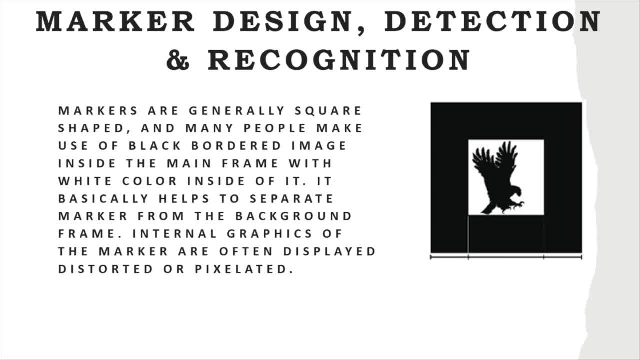 All right, But to make you understand, I have taken example of a black and white marker, All right. See, basically, Majorly many people prefers to use like black and white markers, something like this, All right, Which are basically square shaped and and. 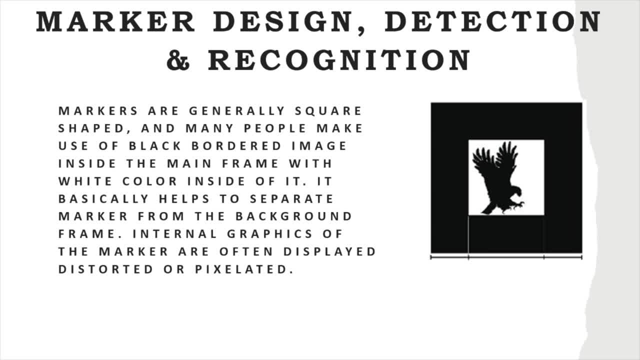 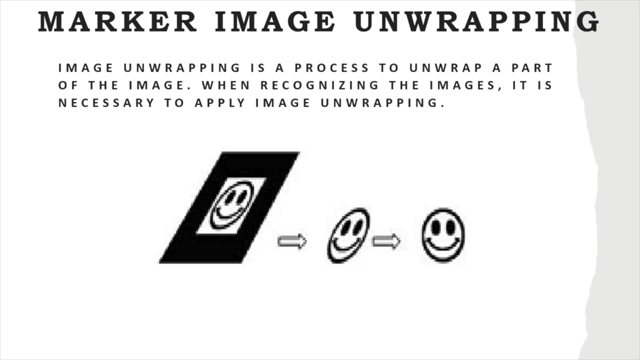 are black and white, like uses black bordered images, and also like the image inside, those black borders are black and other are white. So basically what it does Right, See this: this, this type of images or this type of images, helps in image unwrapping. All right. 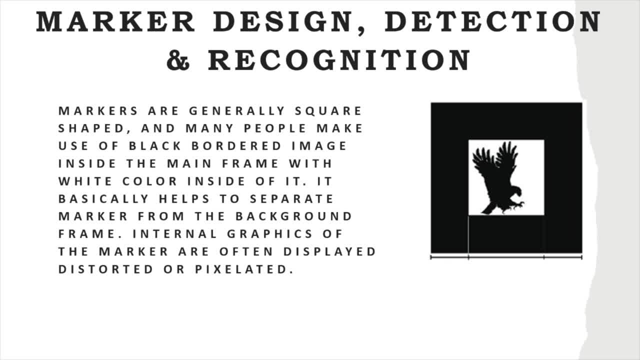 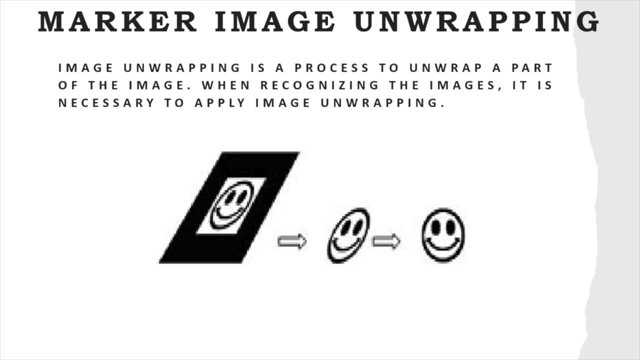 Here you can see that this is a bird. All right, This is a bird All right. After the image unwrapping or after the image unwrapping technology is applied, Here you can see, like in this image or from this image, the face or the white borders are there. 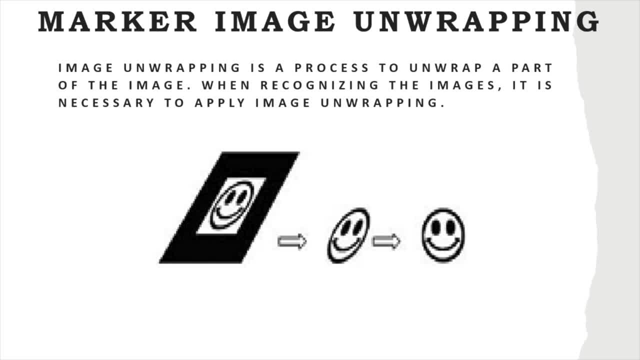 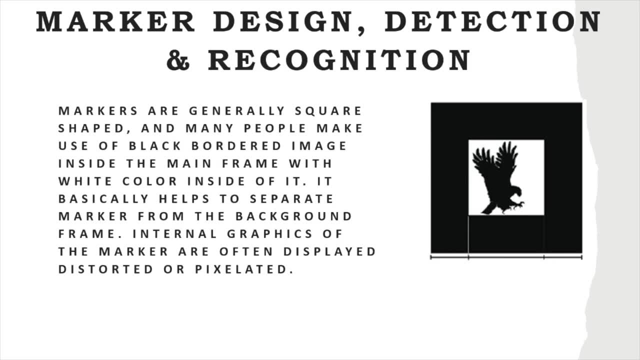 And here is the face. It, the face, has been unwrapped from that whole, Sorry, black borders Right. So here you can see: the face has been unwrapped and it has been positioned like the similar thing will happen with this bird also. 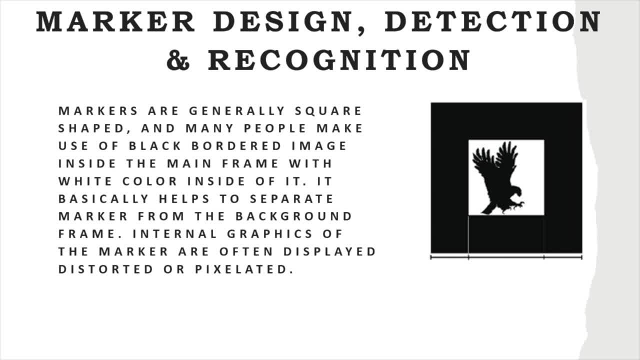 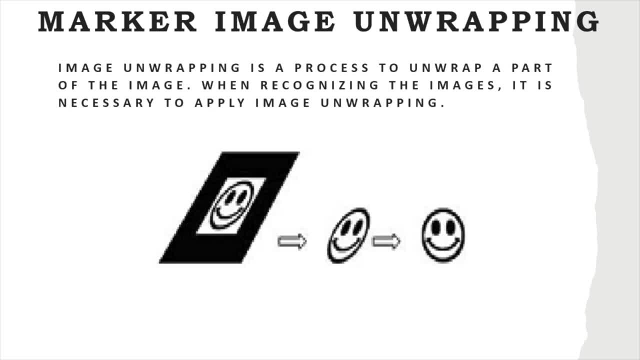 All right, It would be unwrapped. All right, This image would be unwrapped, and then It would be placed like this: All right, This would be the main image. So this is how image unwrapping works, All right. 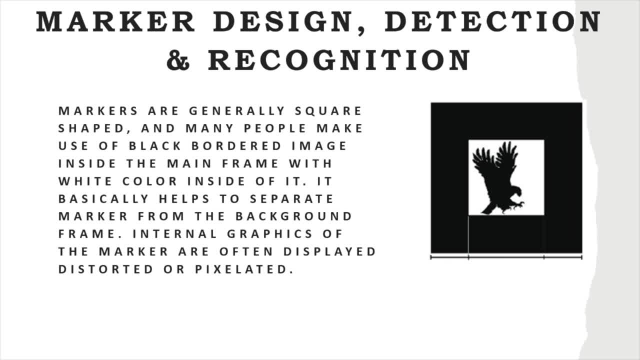 And image unwrapping is also a very, very important concept. Similarly, you can see this is like many people use this. All right, And this black and white image makes it easier for the algorithm. It makes it easier for the algorithm to do the detection to. 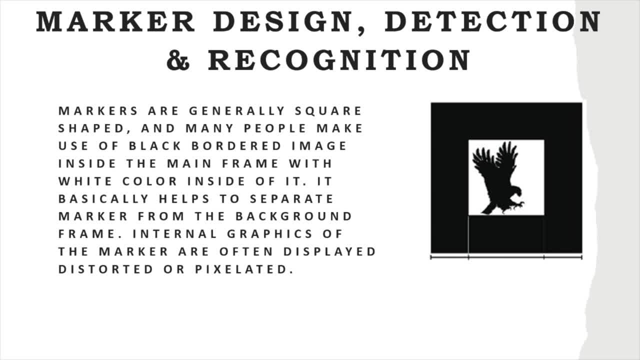 unwrap the image, All right, But there are many powerful algorithms that have been designed and they can efficiently extract, or you could say, unwrap the images of, unwrap the color images also, So that's why we can also use colorful markers too, All right. So yeah, 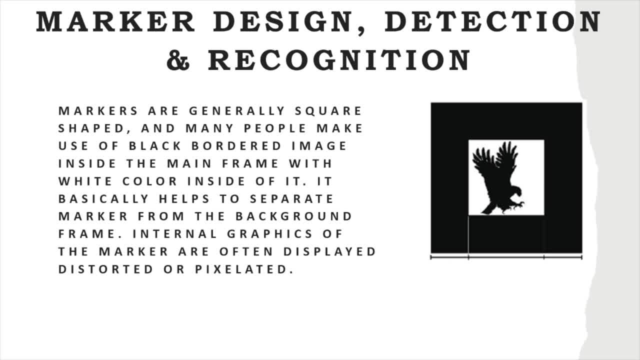 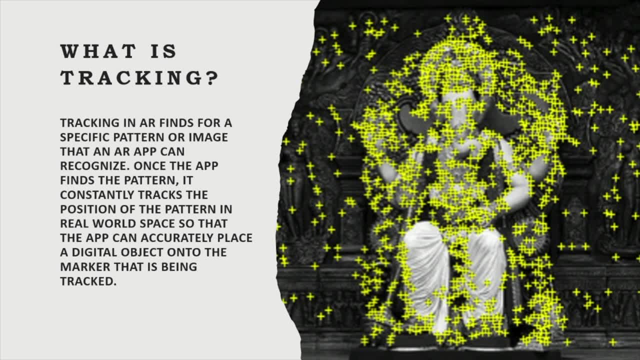 And even if you notice, all right, if you go to let me show you in here also, All right, Here you can see the marker. All right, I have already told you that this is the. this is the marker. This is the image of the marker that I have uploaded on Vuforia's database. 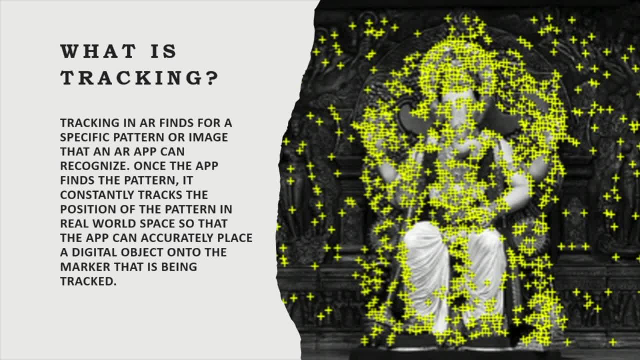 Right For marker based tracking. As you can see, the image has been. like the texture of the image has been is really low, like the quality of the image is really low. It has been pixelated. You can literally count the pixel if you want. 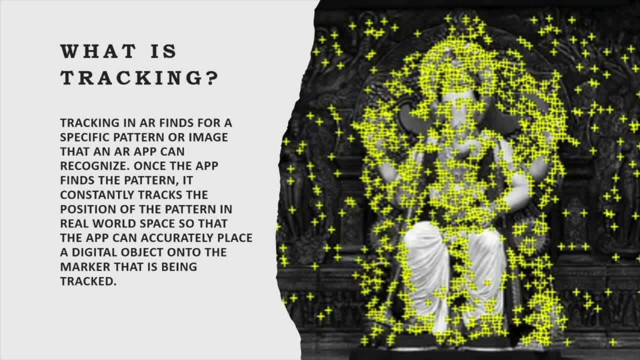 All right, Although it would be hard because there are lots of pixels in there. But here you can see that the image has been pixelated. The quality has been lowered. All right, The image is distorted, All right. That's how it helps to track. 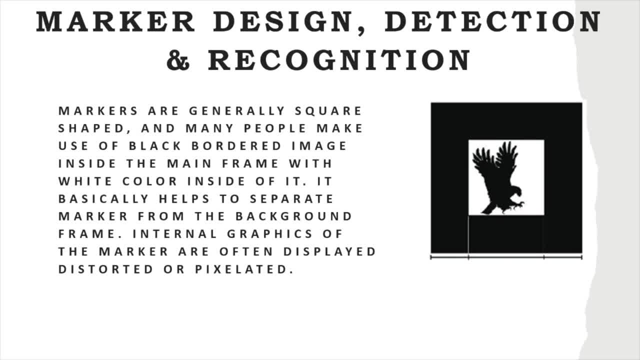 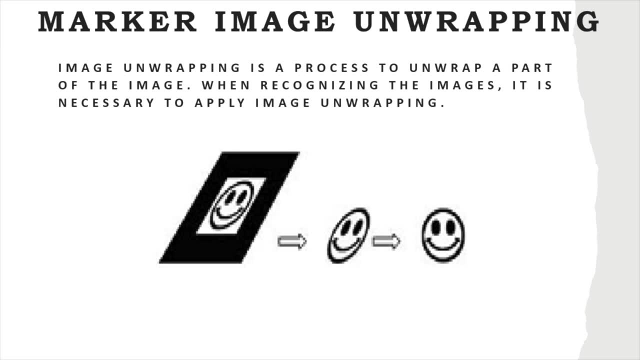 Right, That's how it helps to track. It tracks pixel by pixel. It Helps to unwrap the image also. So that's how marker image unwrapping works. All right, It unwraps the mean particular portion from the whole image. 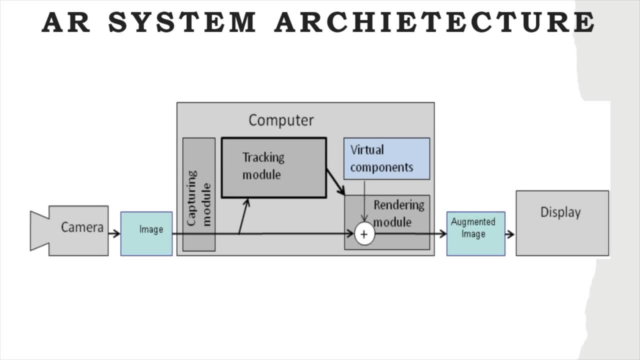 All right. So now it's our time. All right, It's our very time to understand AR system architecture. All right, See, if you understand the architecture, you can even create your own AR SDKs or marker based AR SDKs. 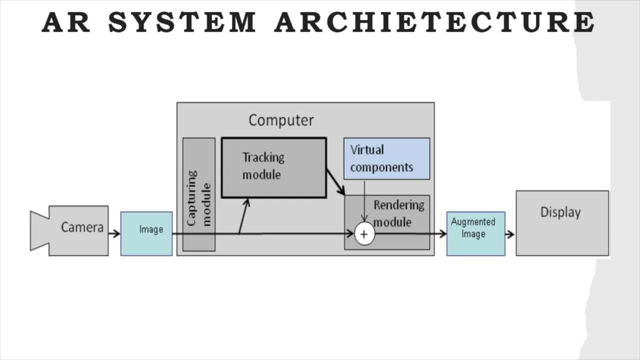 That, of course, won't be easy, because before developing any sort of SDK you need to have a good amount of knowledge of computer vision. All right, Because augmented reality was built upon computer vision only. It is, you could say, a product. 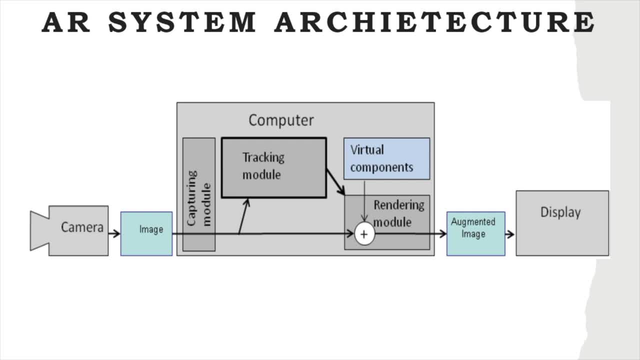 All right, You can say it is a technology of computer vision. only, If computer vision wasn't there, then augmented reality also wouldn't have been possible. So computer vision is the root. All right, It is the root of augmented reality, So it is really important. 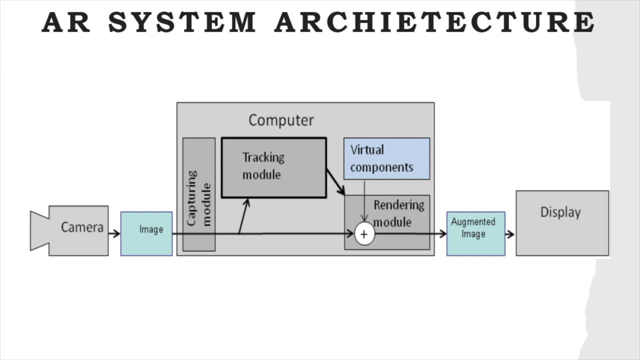 See if you want to create your own AR SDKs. if you want to create your own SDK, you need to have a good knowledge of computer vision. You need to know the algorithms. All right, Even I'm learning computer vision for augmented reality so I can get. 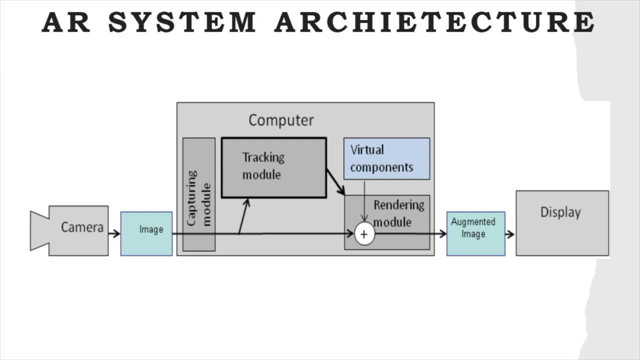 a more deeper understanding of how these things work. All right, I have a decent understanding. All right, I understand how these things work, but I don't know how to develop these things. All right, What algorithms are used? So for that, I need to learn computer vision. 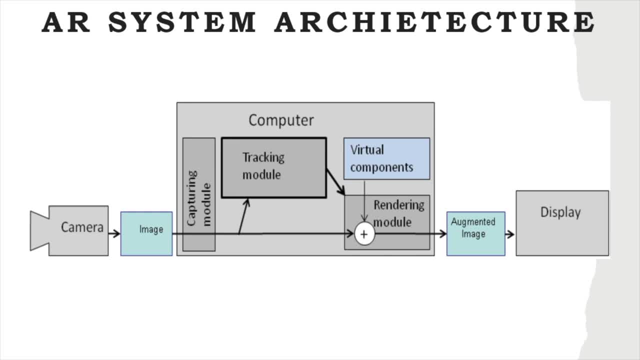 So I'm also learning that, So it is very important for you. All right, If you want to develop your own SDK, you have to learn computer vision. All right? So without any more talk, let's start with understanding the system architecture. 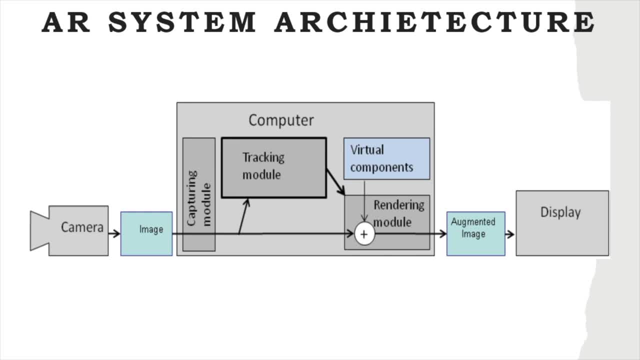 All right, See, in this architecture you can see there is a camera. Then from the camera the image is passed. All right. Image is passed to the tracking module. All right, Some things happen in there. All right, We'll understand what things happen in there. 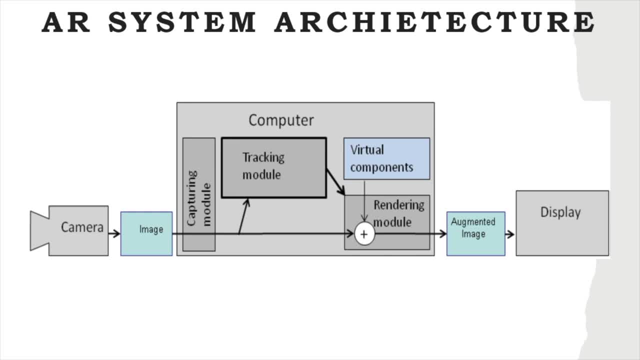 All right. Then it is passed to the rendering module, where the real world and the virtual objects are combined in the rendering module- All right. And the augmented output, All right. The output is passed through the rendering module to the display, All right. 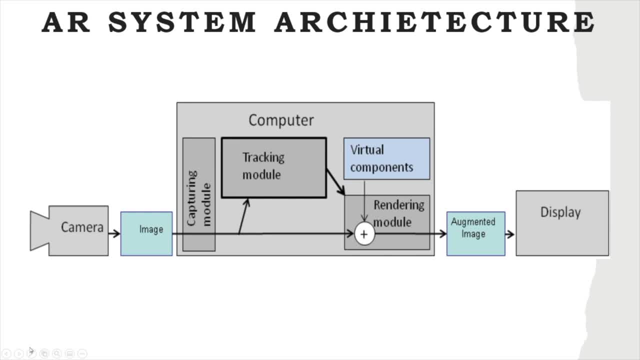 So this is, this is how it works. You can see the diagram. All right, Like like if I, if I had to show you like this, All right, Pen, First of all, it is moving from here and there. Yeah, Then from here it is going to here. 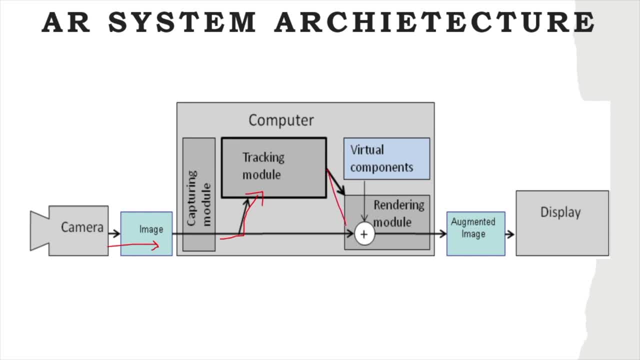 All right, Then from here it is literally going to the rendering module And this, this virtual module, is adding. all right, This virtual module is Adding to the real world component. All right, Sorry for this bad handwriting, But this is RC means real world component. 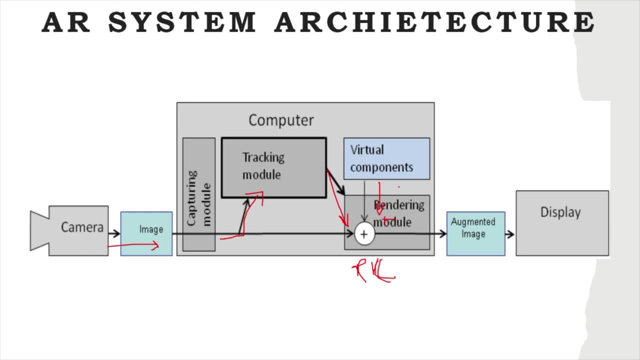 All right, And real world component and real world component. Sorry, Virtual component and real world component are like actually attached. All right, The real world, the virtual component, is attached to the real world. And then the output. All right, Then the output is generated. 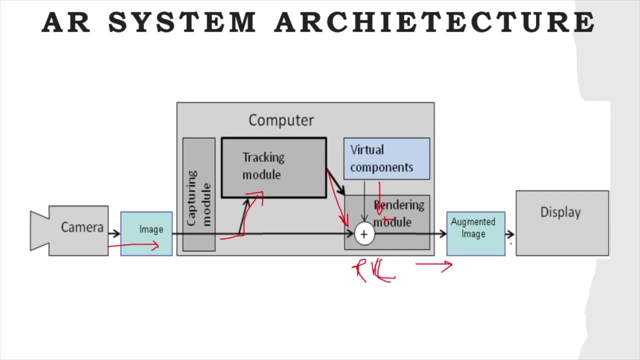 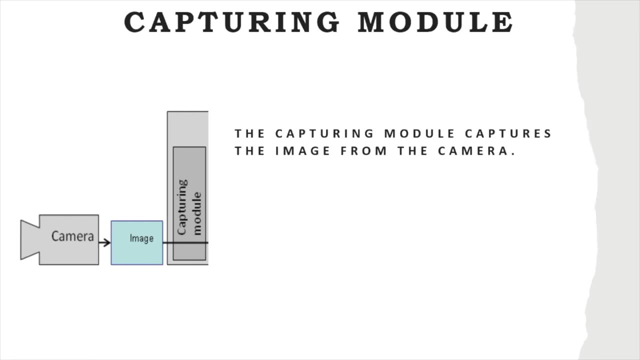 That is the augmented image. All right, it is being displayed in in your system's display, all right. so this is it. that's how it is working. all right, now if we talk about understand the module, all right, see, if we talk about, you already know what is the camera, right? 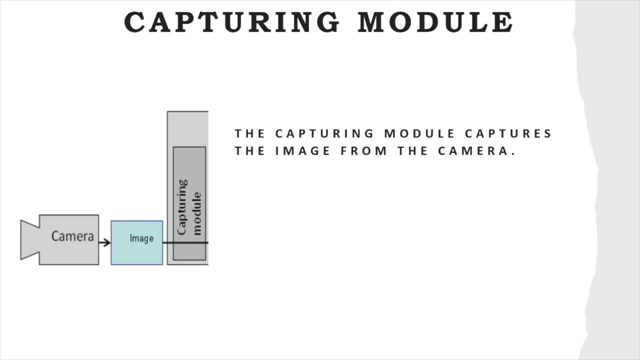 what this camera module does? right, because it it renders like, it renders the image of real world, all right, into your phone. that's what a camera does. but what is a capturing module? all right, see the things that you see from your mobile camera. all right, you can even capture it. right, you can even capture it. 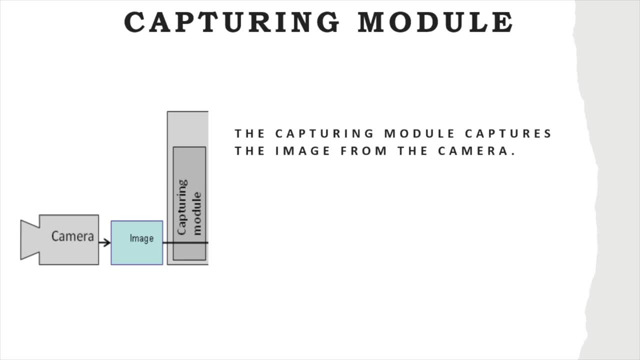 so through the camera, some sort of image is passed to your display, all right. and when you click on that centered button available in your mobile camera software, when you click that, it is captured, right. so the capturing module basically helps to capture the image. all right. basically itか helps to capture. 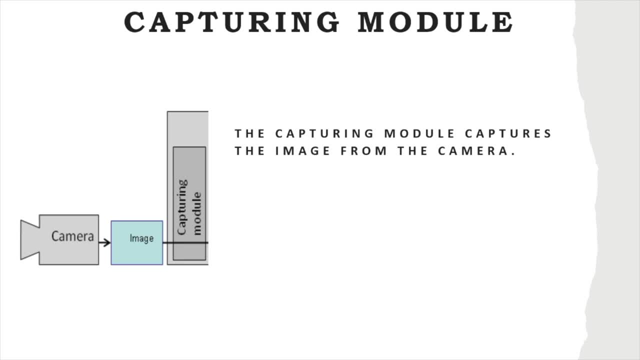 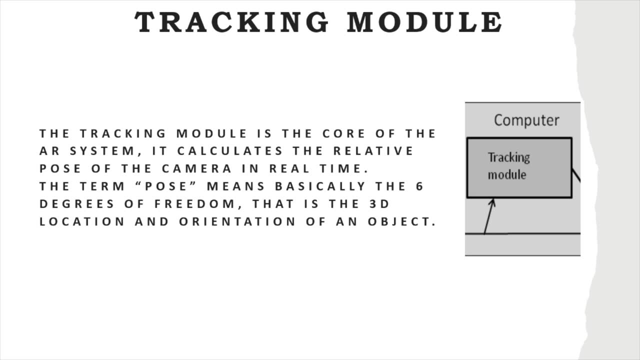 the video or the or the image. all right, so this is what capturing module does. now, if we talk about the tracking module, all right, see, the tracking module is the core. all right, the tracking module, uh, is the code. and if we talk about, uh, see the how tracking module works, now it, it calculates. 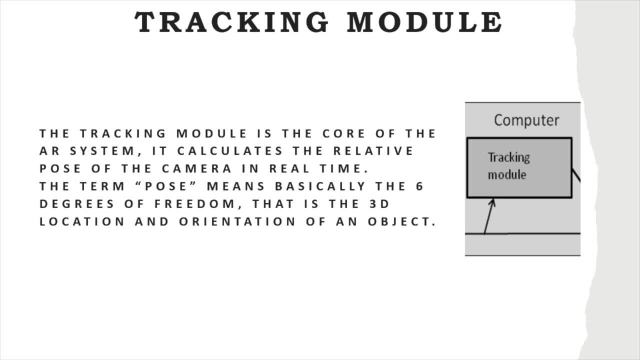 all right, it calculates the pose, all right, of the camera. all right, in the real time, all right, like it will, uh, calculate where your camera is. and if i talk about, uh, fovs, all right, that is six degree of freedom. it means that, uh, you have a freedom of to look anywhere. all right, you could. 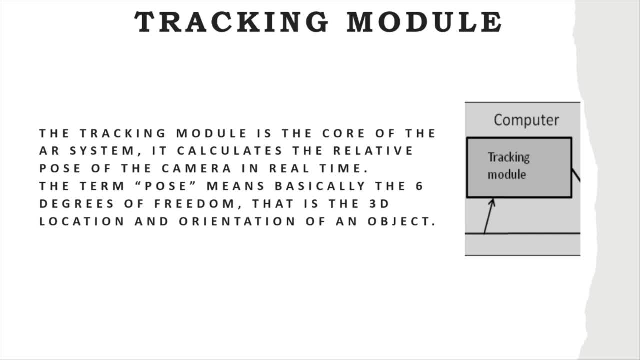 this is a very basic definition of uh six dofs. all right, see what this term pose does. let me tell you uh pose estimation. all right, basically helps. uh helps to get the camera to look anywhere. all right, so this is a very basic definition of uh six dofs. 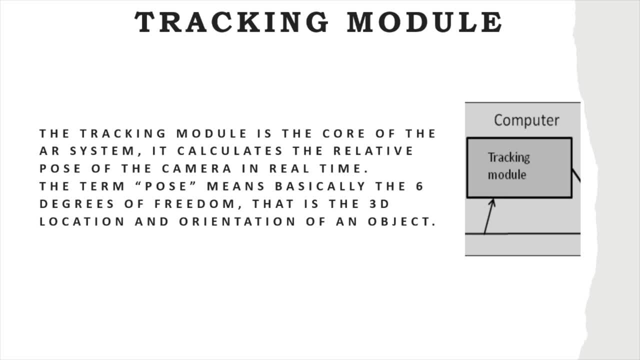 get the orientation and location. all right, get the orientation and location of of a particular object. this is what the tracking module does. all right, it has, it is basically the code. all right, it helps to calculate the pose of the camera. all right, in real time. it's not like. 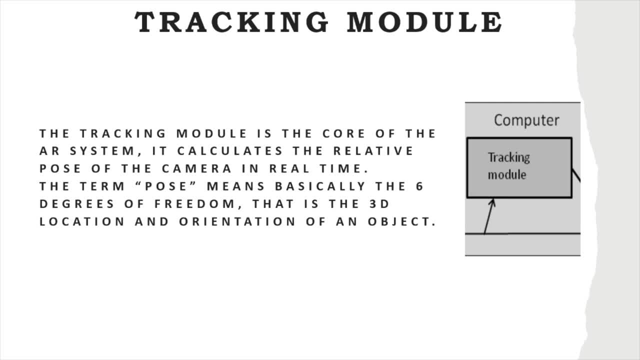 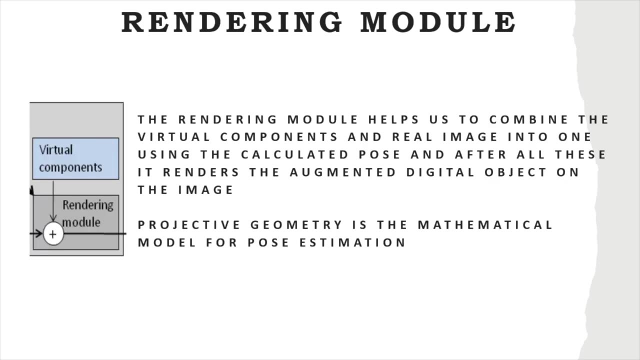 it will, uh, only capture once, then it won't do it again. it happens in loop. so the pose estimation is done and also because of that we get the 3d location, or you can say the orientation of any sort of object. that that is the work of tracking module. all right, if we talk about the 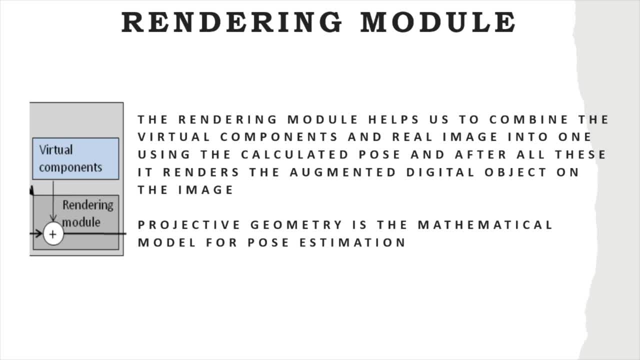 rendering module. all right, see, uh, what this rendering module does is basically it combines- all right, it combines the digital object. all right, it combines the digital object with the real world visual. all right, with the real world image. right, if you, if you have used any sort of augmented reality, you might have seen that, right, that, uh, some 3d object is. 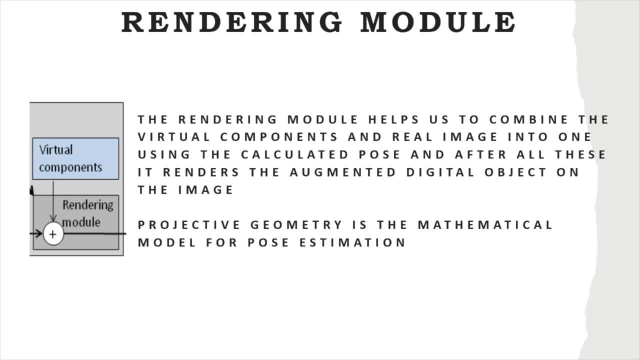 appearing on sort of on any marker right on an image, a 3d object is occurring. so a virtual uh, a virtual, basically a virtual component is being attached with that image and then it is being processed and pushed forward for the display. all right, and if you are confused, all right, if you can. if you are confused about these uh modules, don't worry. 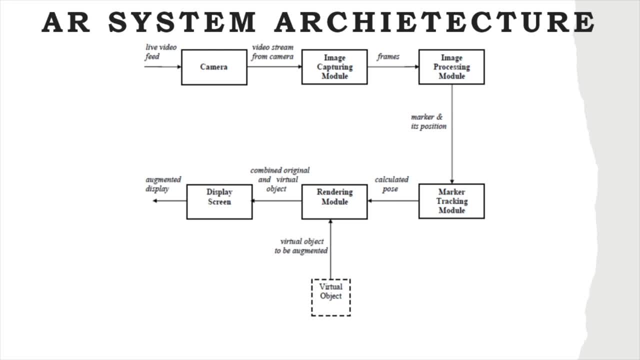 all right, we are again going to look into another. all right, this is a very much more simplified version. all right, this is a much more simplified version of that ar system architecture. i have included this because i thought that for the first, for the first iteration, i think people will get. 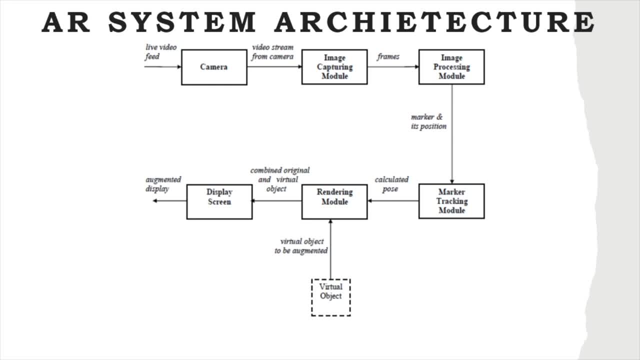 confused that. how this, like what did i explain to you? you might not understand it right, so i have also included another architecture. all right, the same thing happens in here also, but i will re-explain. see in here: all right, a live video feed. all right, is going through the camera. 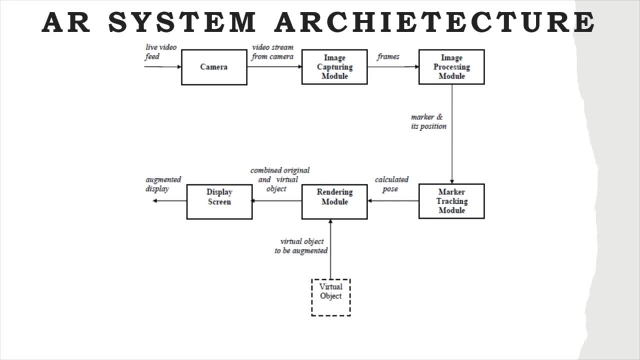 all right to the image capturing module. all right, and it is all right, and it is divided in frames, the the video is divided in frames and then it is going through the image processing model module, all right, and in there, in there, the marker is detected and tracked. all right means? uh, in there, the marker is detected. 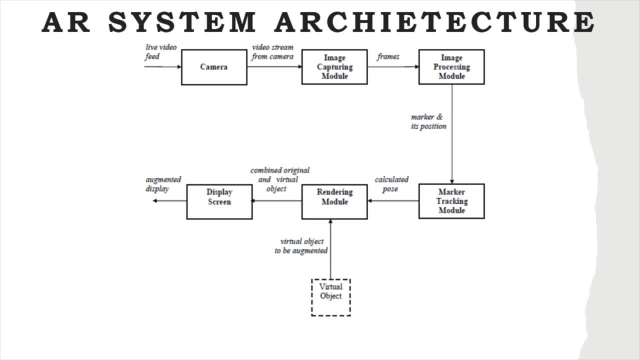 actually all the processing is done, all right, all the post calculation is done, and then we go to the marker tracking module- all right, where the post calculation is generally done and all the tracking stuffs are being done in there only all right, all the uh, what can i say? those are virtual points. 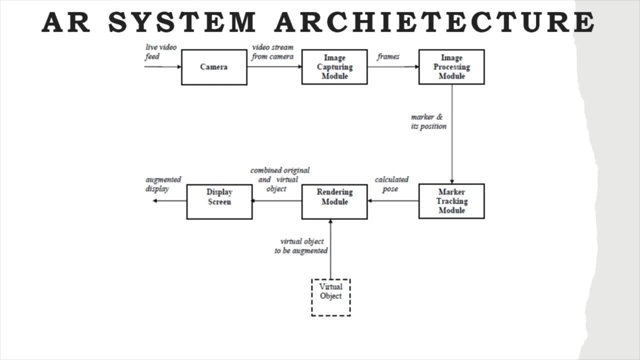 right, those feature points are applied in the image in there, only, uh. and then we go to the. the post calculation is there. only see, if you are confused about post, post calculation, don't worry. all right, uh, let me explain it to you again. see, post calculation is basically it. 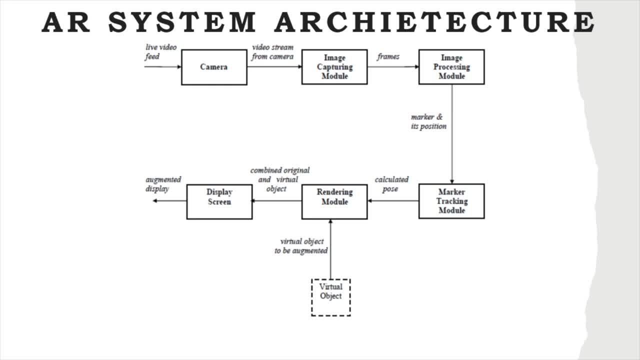 calculates the position, all right. it calculates the position of any object, all right. that's what post calculation is. it calculates the orientation of the object and the location of the object, all right. so that's what post calculation is. and then, after all these processing and tracking is: 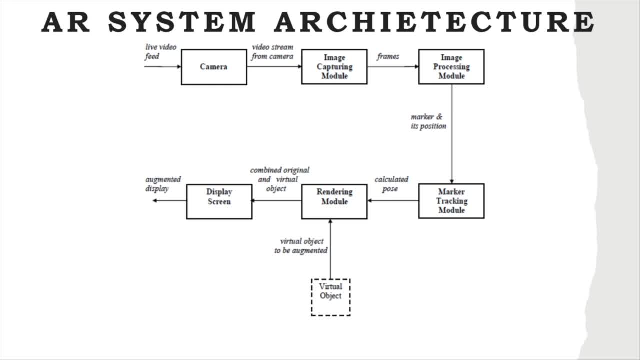 done. it is passed to the rendering module. all right, the virtual object. all right, the that the virtual object that we want to augment- all right, that we want to augment- is combined with the real world image. all right, the virtual object is combined with the real world image. then, then it is passed. 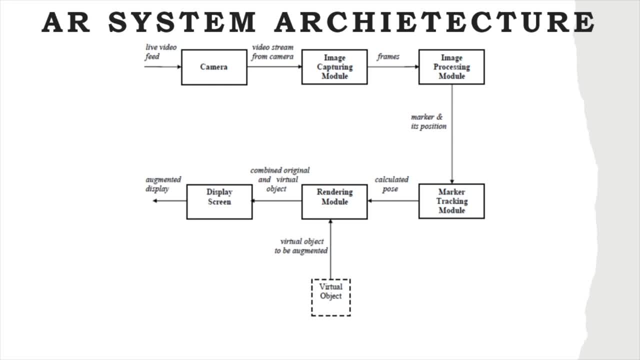 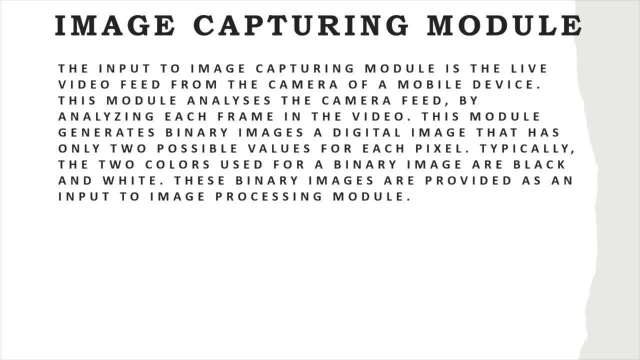 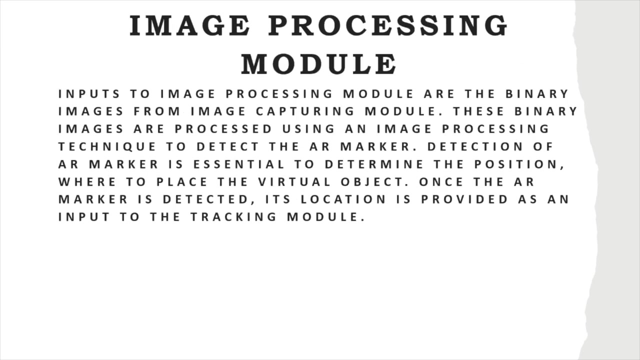 to the display screen and we actually see the output on our displays. so that's how this ar system architecture works. all right, i hope you are clear with the concept. right again the same definitions, all right. the image capturing module that takes the images. it breaks it to frame by frame, then, and all those things are that are being done. then there is 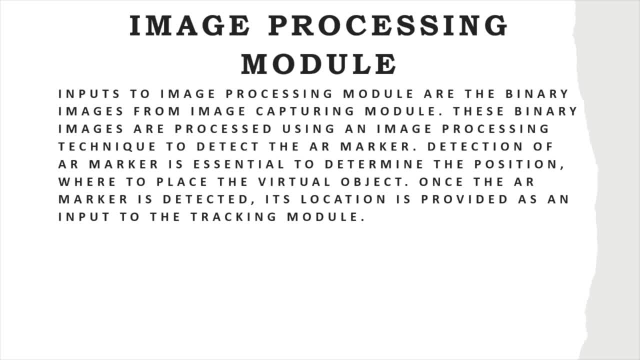 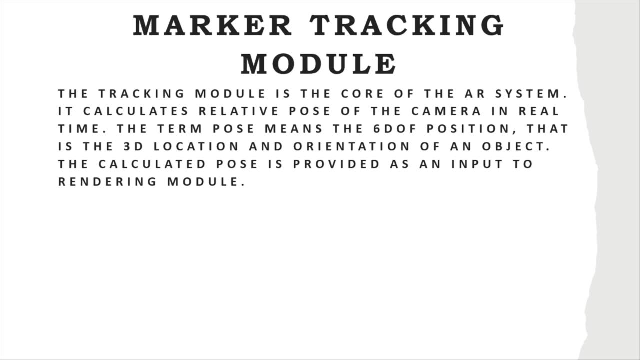 image processing module. already the processing that are being done, all right, means the detection or you could say the recognition techniques are being applied in there. all right, then, if we talk about the marker tracking module, in there the position is being calculated. all right, the position is being calculated, and then feature points are provided. 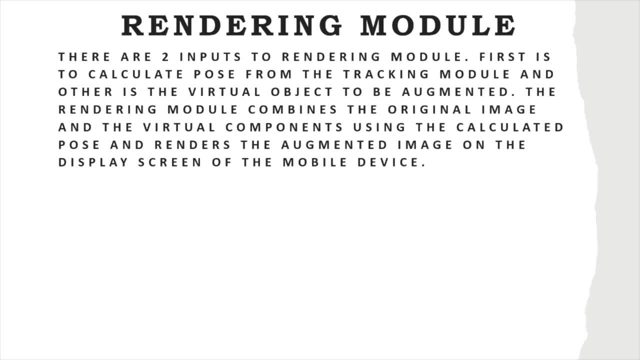 and the rendering module. all right, this rendering, what this rendering module is doing, this rendering module is basically, uh, combining the virtual object to the digital object. this is just it. all right, it is doing that and, yeah, that's it. so that is that's it for our today's lecture, and i hope you have understood. all right, i hope you have understood. 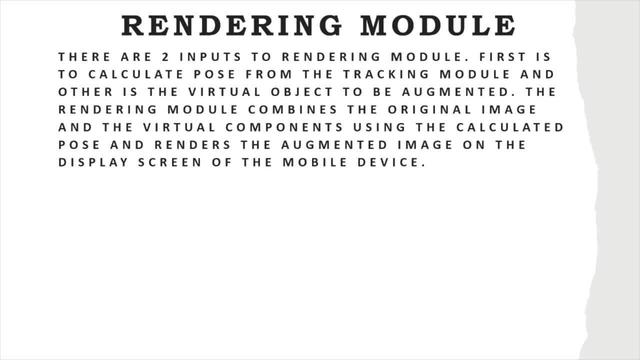 how all these things work. all right, i hope you have understood how the marker-based ar system architecture works, all right. so i don't think now it would be any problem, as you have, as i have cleared all the very basics, all the very basics of marker-based augmented reality. now i don't think. 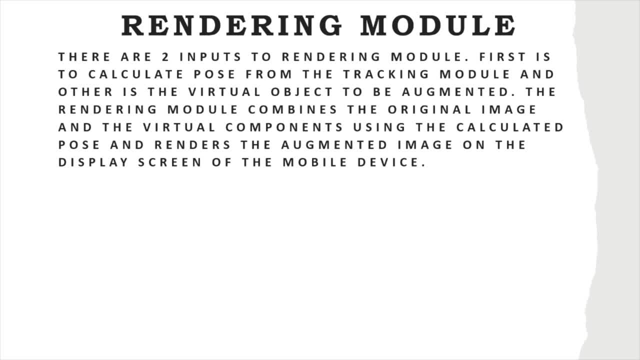 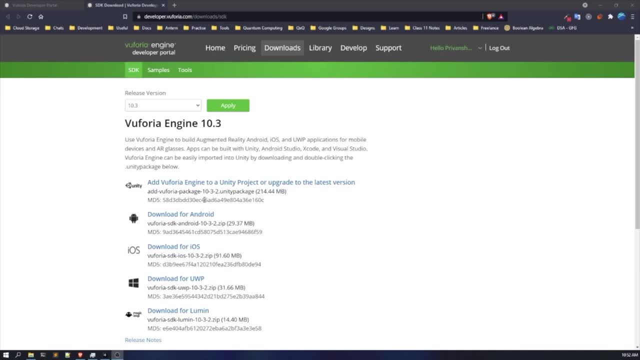 it would would be any problem learning marker-based ar development. in this lecture, i'm going to tell you how to set up your unity and viewphoria engine for developing ar applications, and later on, in this video only, we'll be creating our very first augmented reality application. 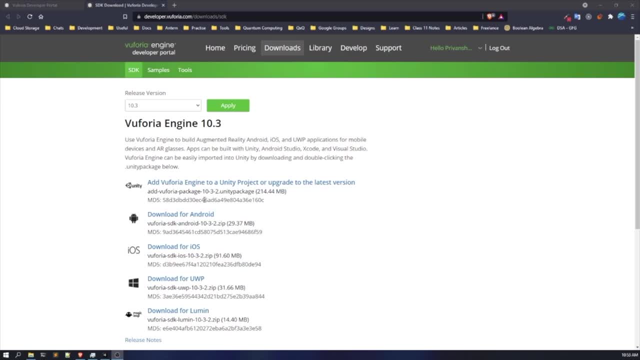 with unity and viewphoria. so yeah, the very first thing you have to do is go to this website, developerviewphoriacom, all right- and in there you have to create your account. after creating your account, all right, you can see right in the top that there's a download section. click on that particular section and you will be redirected. 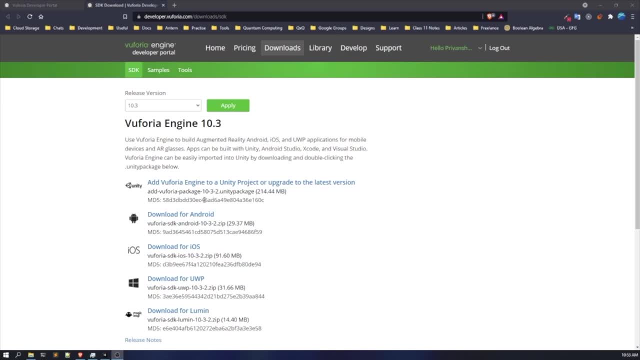 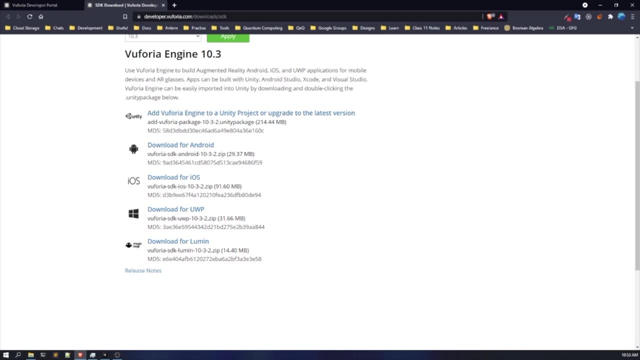 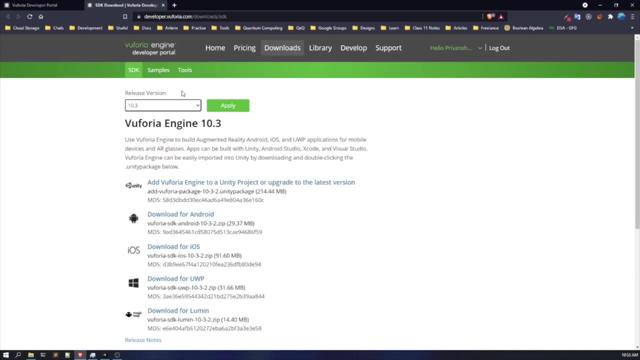 to this page, all right. and in this page, all right, you are seeing multiple option. and yesterday only, like in 15th november, the latest version of viewphoria engine has got released, that is, 10.3. viewphoria engine 10.3- all right. you can even select your particular version right from. 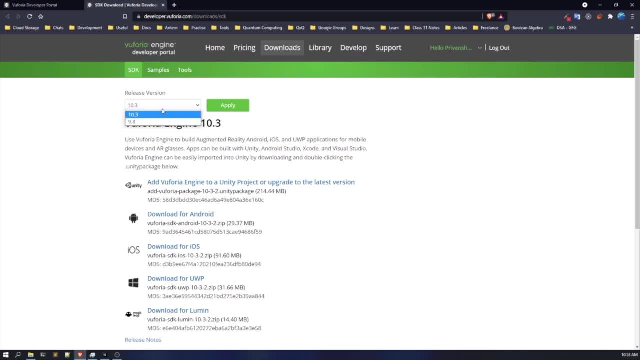 here. all right, that is 9.8 or 8.3. i have seen one problem, that is, when using any version of any 10, like any viewphoria version of 10, i'm facing an error in unity. so i would suggest using 2020 only. all right for this course, because i'm going. 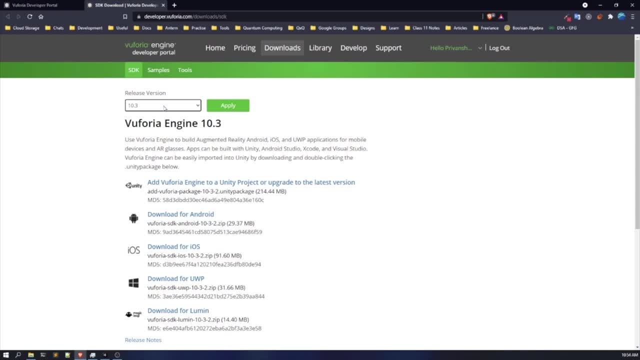 to use the latest version of viewphoria, and now you have to download the sdk. all right, what is an sdk? sdk is the software development kit that will help us to develop for means ar applications with unity and viewphoria right? so we have to download our. 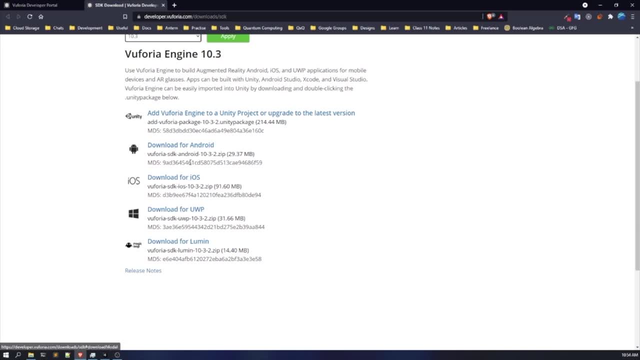 sdk. now here you can see there are multiple options available. all right, let's say, you don't want to develop with unity, all right, you don't want to develop your marker based ar application with unity, you can go for android studio. or, if you want to do it for ios, you can. 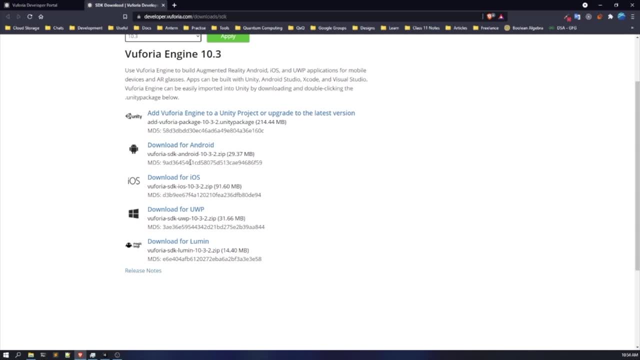 that is xcode you can, you can download for ios. then there is uh uwp, then there is uh lumen. so uwp is a basically universal windows platform. so, uh, you can use that too. so for uh for this course, all right, for this, for the sake of this course, we are going to use um viewphoria. 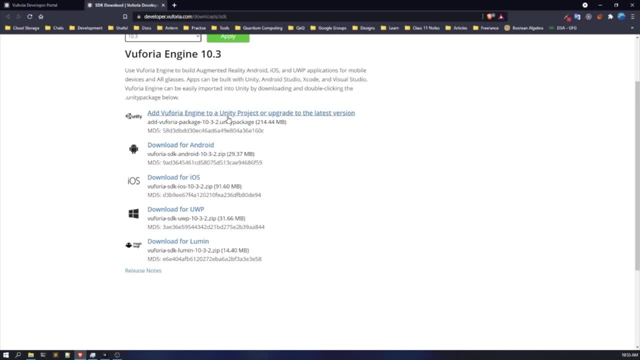 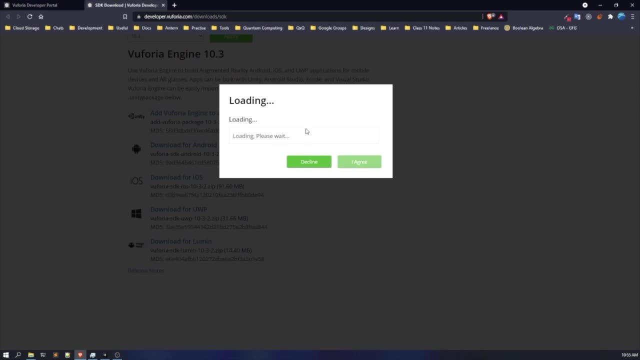 engine. all right, the very first option that you are getting, that add view for the engine to a unity project or upgrade to the latest version. so just simply, uh, click on it, all right, and uh, some things will be loading up in here, all right, and then click on agree, i'm going to decline it. 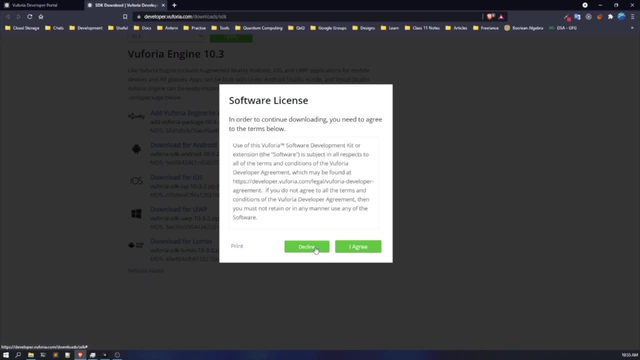 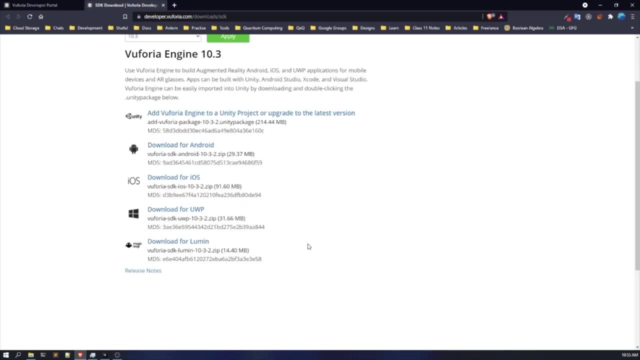 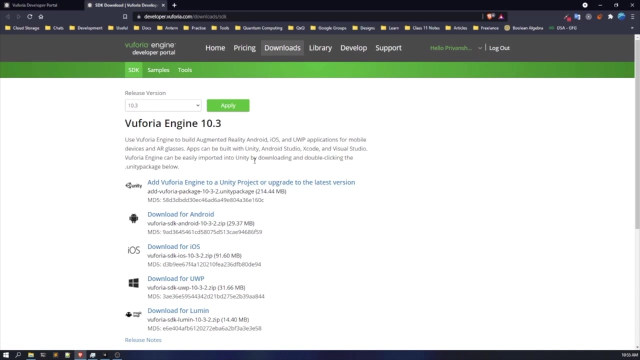 because i have already downloaded, uh, the sdk. but you can, you have to click i agree and then download the sdk, all right, so yeah, after downloading it, all right, uh, after downloading, what i would suggest is first let's set up the web version, all right, like set up all the things from the web side, right, and 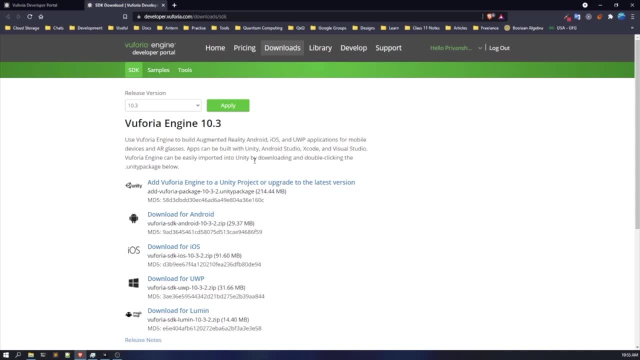 then after that we'll be moving towards unity. so how to do that? right? so now we have to get uh into another page, that is, this develop section. all right, remember, you have to create your account first to uh get all these things. so do create your account. so now click on. 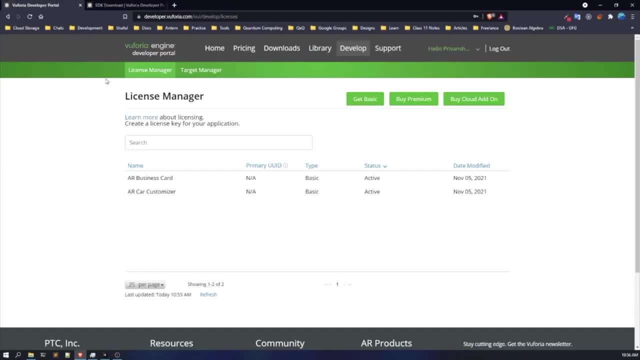 this develop. i've already opened it on my second window and here we go. so here you can see. uh, they are target manager, license manager. so what are these two? uh, the license manager actually helps us to manage the licenses. all right, licenses means there are some particular lines of code. 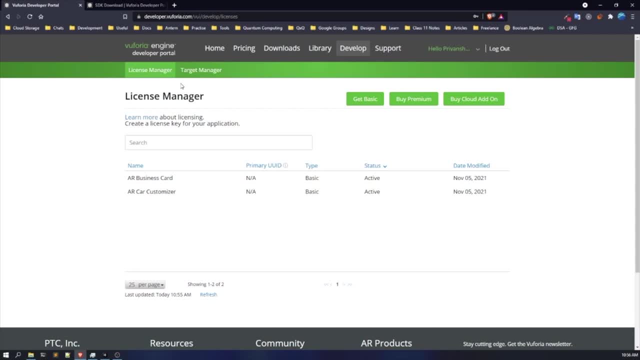 all right, there are some particular uh lines of code code you could say, uh, some special unique code that helps uh view4d to connect with the backend server and verify actually, uh, what kind of uh services are we using? right, like, i'm going to use the basic service of euphoria, that is. 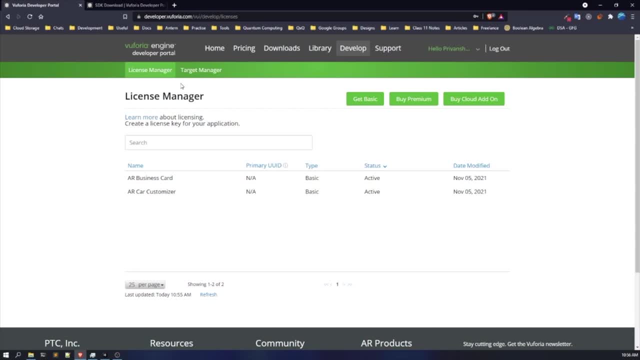 free. so, yeah, all right, so that uh, that, uh, basically, uh particular key actually, uh, we call that a key- that particular, that particular key would help us actually to uh connect to the view4d portal. all right from our unity, all right so that our app can utilize the feature that we 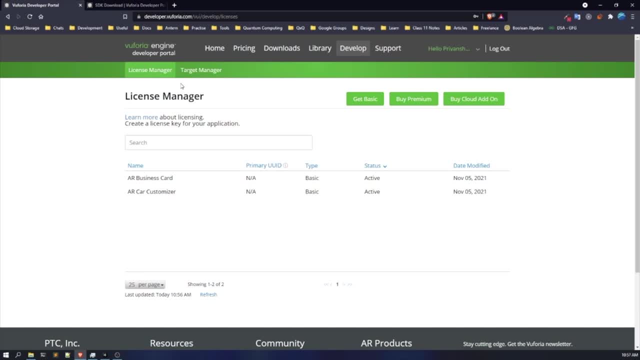 uh, get after, uh, using the different versions of euphoria, that is, basic, premium, all right, any of these two versions. so, yeah, now, uh, the very first thing we have to do is we have to create our license. so how would we do that? see, uh, you can even buy the premium version, but i don't, i don't have the money to. 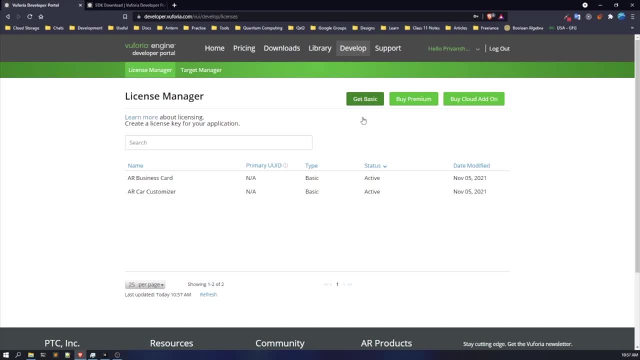 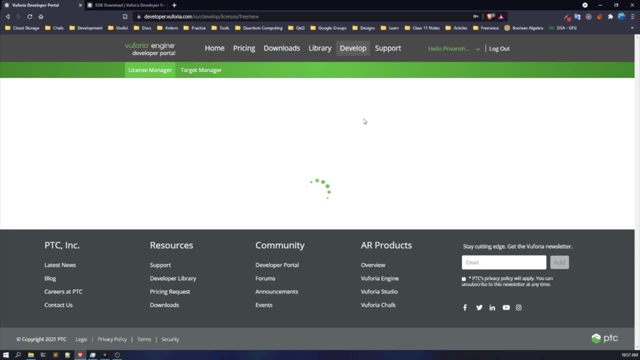 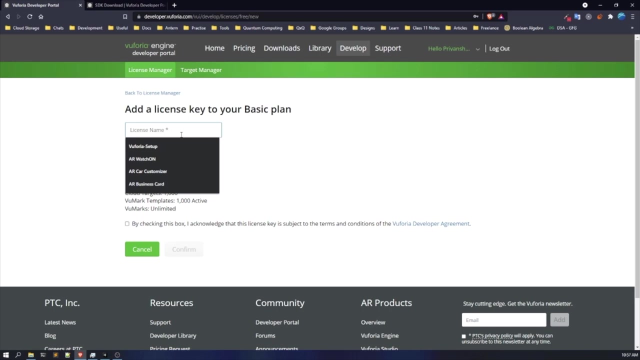 buy it. so i would uh simply get the basic, all right. i would click on the basic, all right, and it would load some sort of page. so, as you can see it right here, it is loading some page and, uh, in that page, all right. uh, keep your license name. all right, let's say i want to 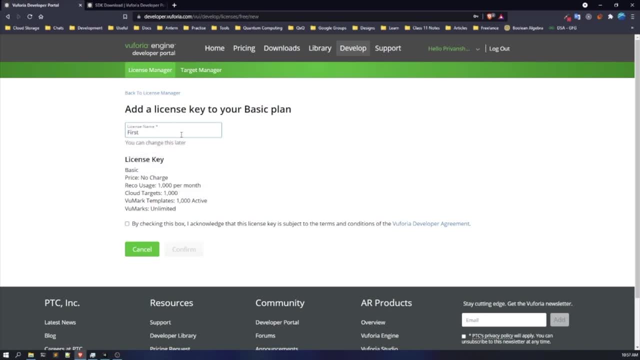 name it: view first. uh, first, ar, uh, app. all right, this should be the name for my license. and here you can see this. these are the things and uh, we have to check this box. all right, we have to check this box, and after that, uh, click on confirm. 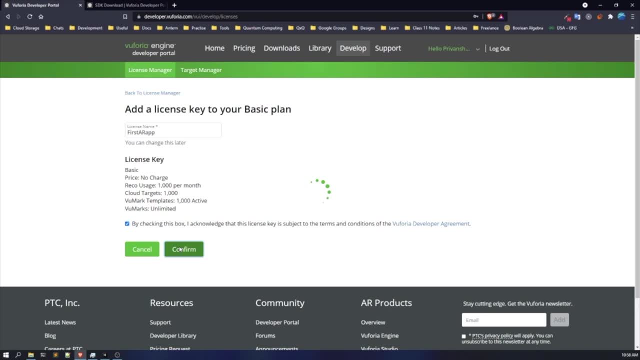 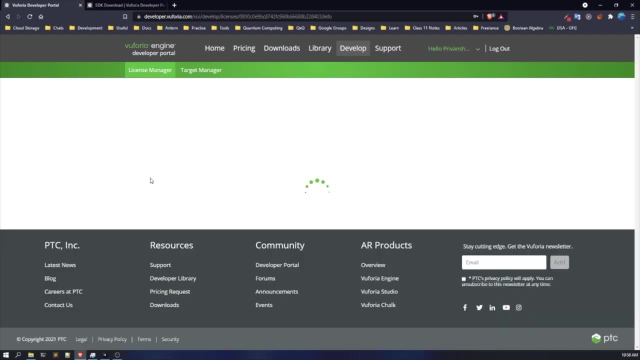 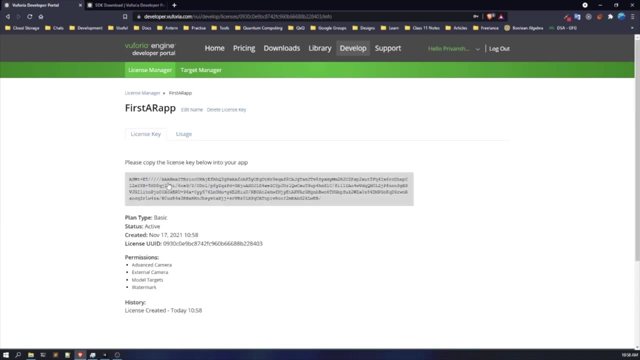 all right, and that would uh, redirect, uh, that would create actually our um license and we can click on that and then simply go, uh, go to that license and copy the license for us, right? so i would simply click on the license, all right, i would simply click on that license and here we go, we got uh. 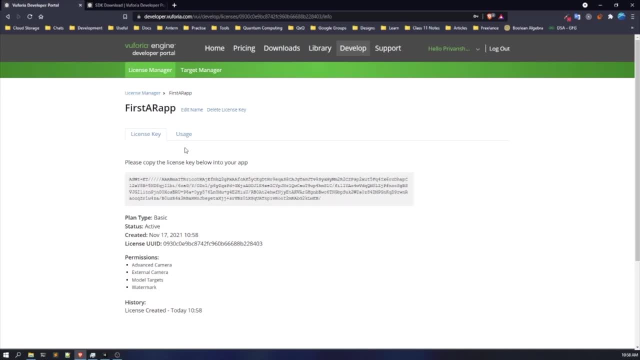 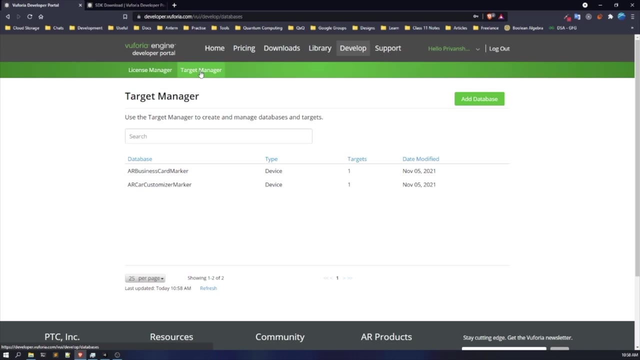 it copied, uh, it got copied in our clipboard. now, another important thing that we have to do is we we have to go to the target manager, right, just click on the target manager. see what, uh this target manager does is. it helps us, uh, keep the markers. all right, see, i have already told you that. 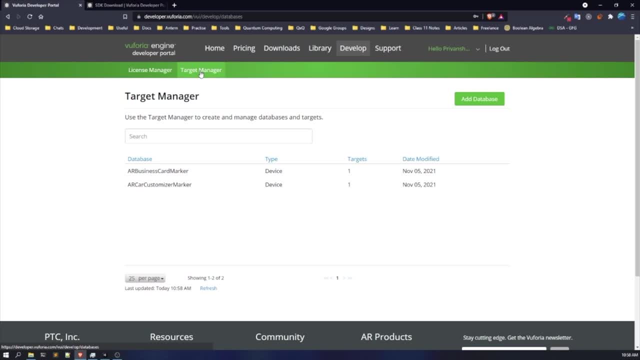 in marker based ar. we need markers and we have to store or like store it somewhere, right. so uh the target manager uh helps uh keep track of the marker on the servers of euphoria, and also we have to download a unity package for that so that we can include it on our. unity means local, uh local. 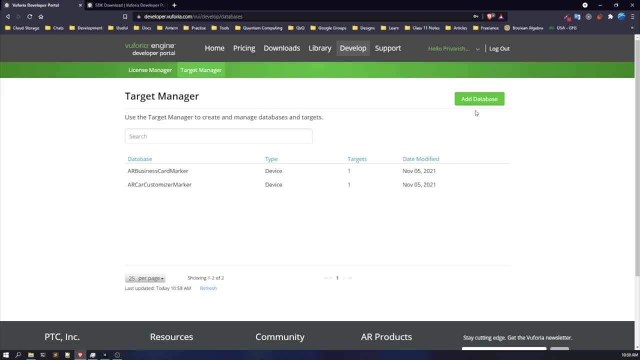 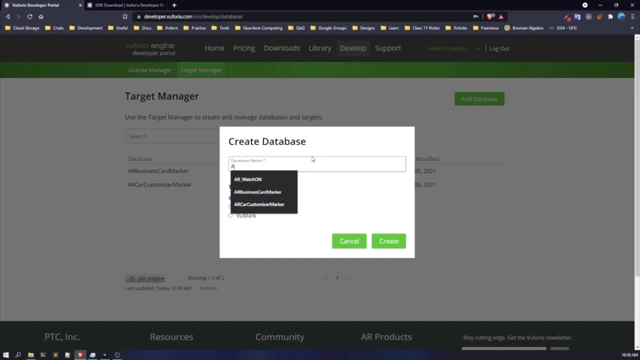 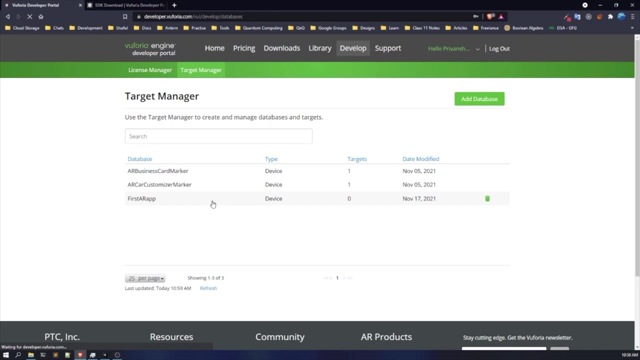 computer, right. so how would you do that? so for this, simply, you have to click on add database, right, and then you have to uh name your database. let's say: uh first ar app, right, first, uh, first ar app. uh. oh, i missed that r, no worries, yeah. so then i have to click create, all right, uh, uh, and uh then uh turn it on. 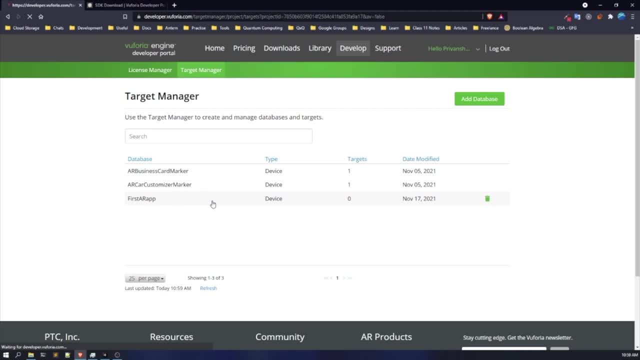 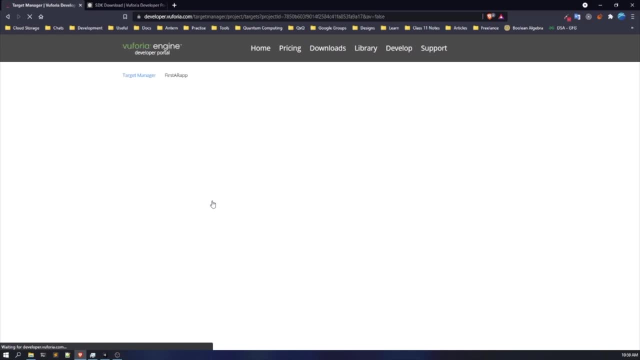 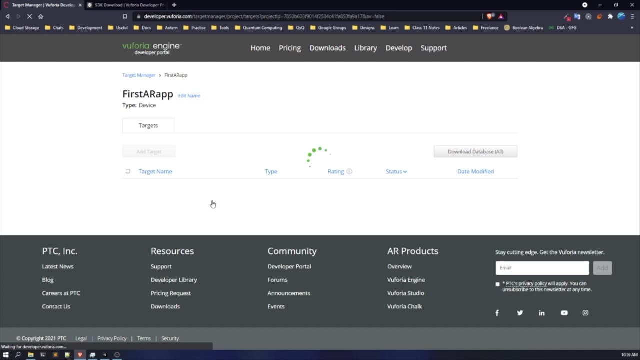 then then go to that particular target and you have to upload your target in there, like means, the marker image, so that, uh, we can use it right. and i would show you some other things also so that you can choose your right marker. all right, uh, choose the right marker for your application. it's really important. 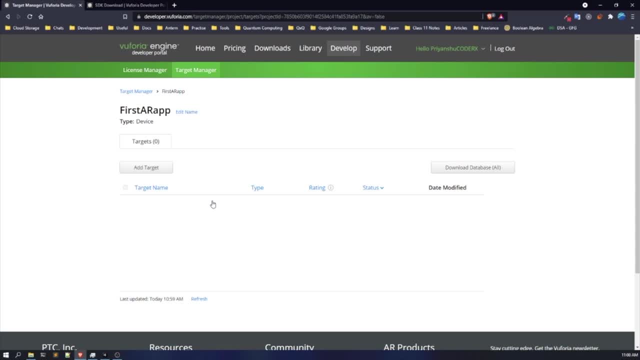 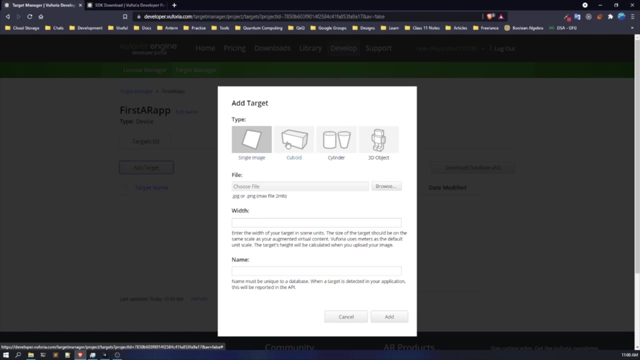 to get the right marker, because if the marker is of low quality, then, uh, marker based ar won't work well, so that's why, right, so click on add target. all right, so i i already have some images, so i'll be choosing from that. now here are three other options. all right? uh, we won't be looking at. 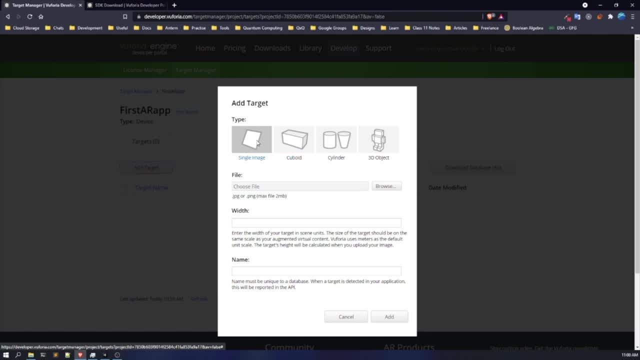 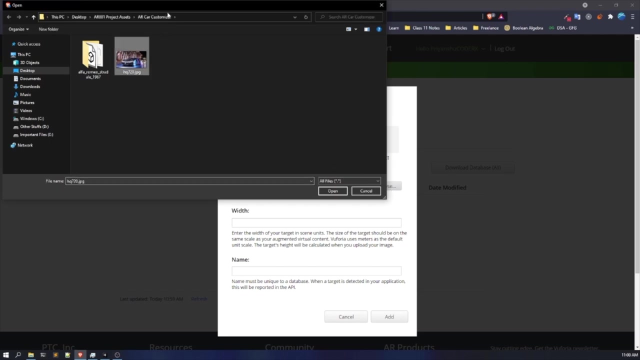 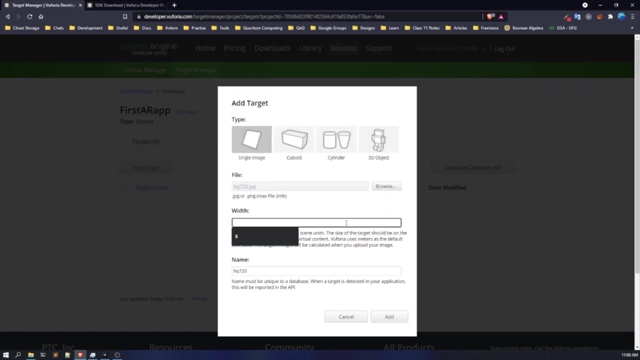 now, all right. so just uh, click on the single image. all right, basically, single image. uh is selected by default, so no worries. but uh, then you have to click on browse. you have to choose an image. all right, you have to choose uh image. so, yeah, here we got an image of a car. all right, uh, i don't have any other image, so i'm gonna use that. 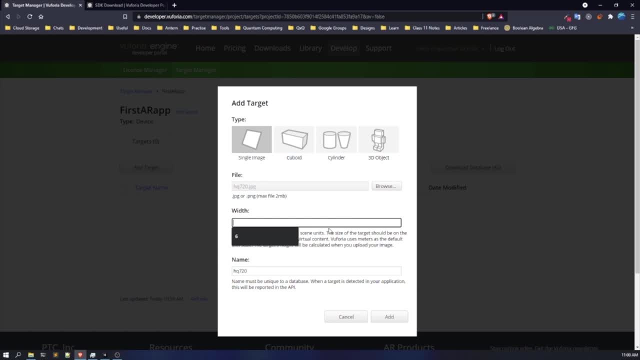 one and you can give any width you want, all right. so my uh, i would like prefer to give six. basically, what would happen now that, uh the width you give, all right, it would uh get that particular units of width and uh the unity engine, right. so uh remember that that won't uh be like. 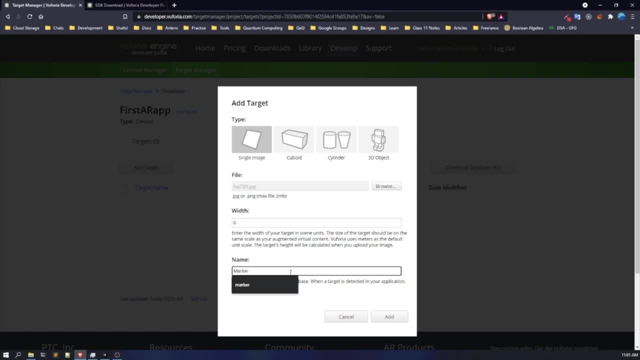 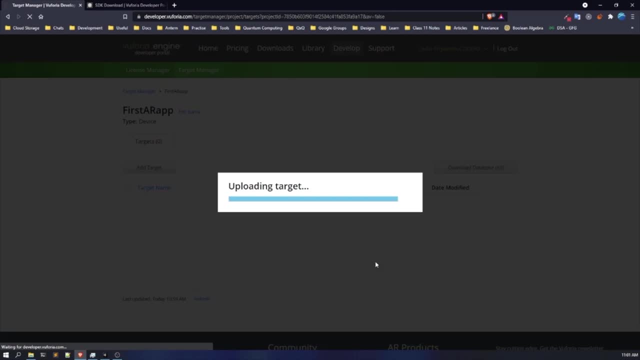 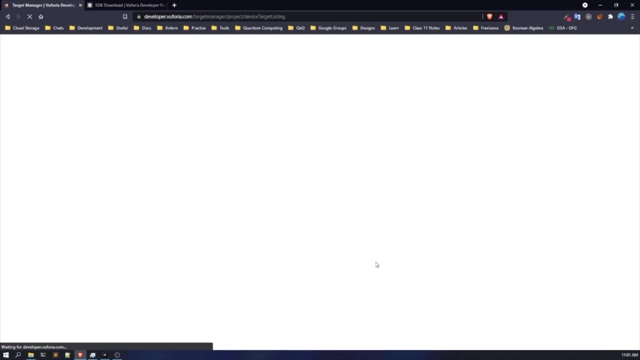 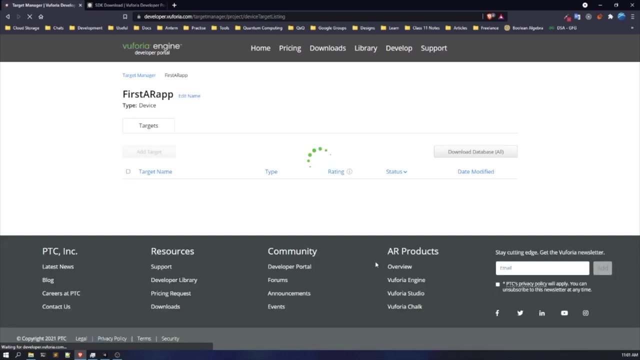 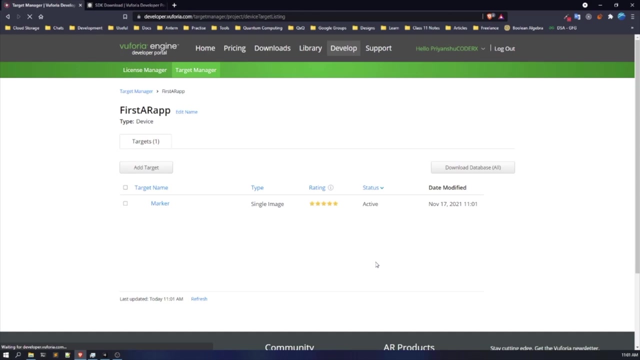 give any sort of difference, so i want to name it marker, all right. so then click on add and now it's, uh, uploading our target. all right, it's uploading our target, and that's really cool, so let it do its job, okay, so how should i do it? um, let's keep our sense. of tips for today. 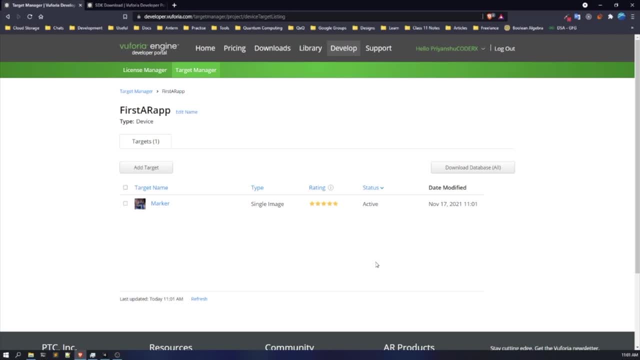 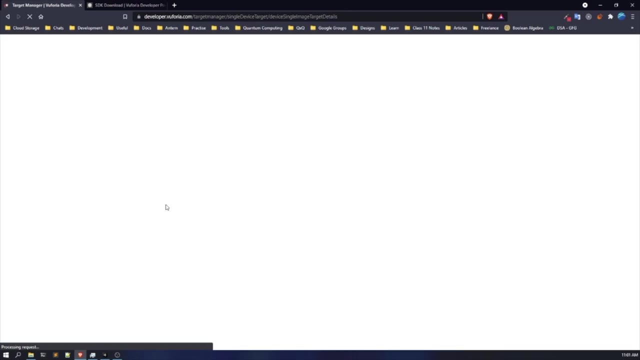 all right, i'm going to take that again'll do that. goodbye, cool. so here's uh, our target. uh means marker has been added. i want to show you some other things also. so to get those things, click on the marker, right click on the on the marker. it would redirect you to the marker properties. you could say that: 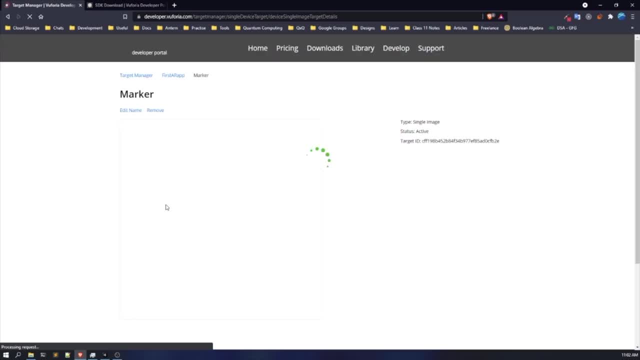 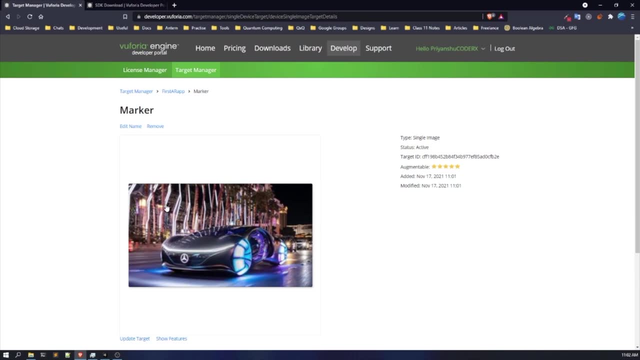 so then i'm going to show you some very important things, all right, and what sort of marker you should not use for your marker based AR applications. alright, so, as you can see here, alright, in the in the, if you can see, in the right side, there are multiple text, right type, single image status: active target. 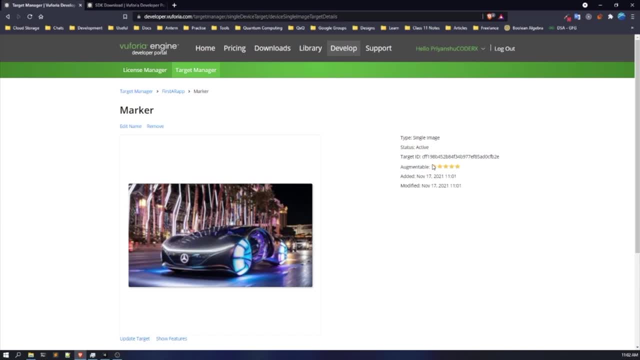 ID augmentable. alright, this is the section that this is the text we want to focus on as of now. what this tells is: five star means this image is very good. alright it, it is going to be superb for tracking. now, see, remember always that three- the range between three to five star- is okay, alright, below, below it. 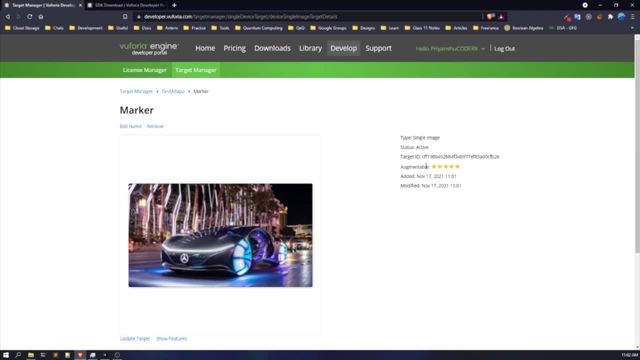 won't give you good results. even three sometimes won't work that great, so always remember to take a picture. alright, always remember to take a picture that is that has got four to five rating. alright, four to five star rating and it's really really really important, alright, so yeah. 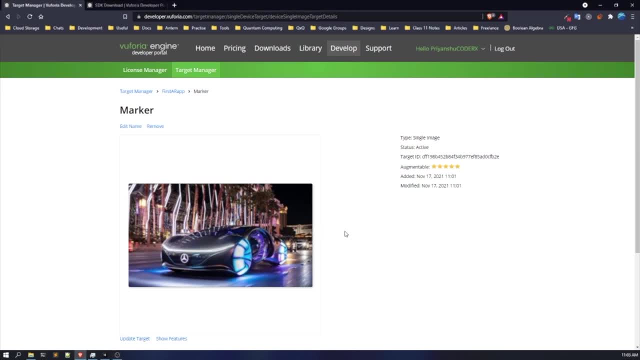 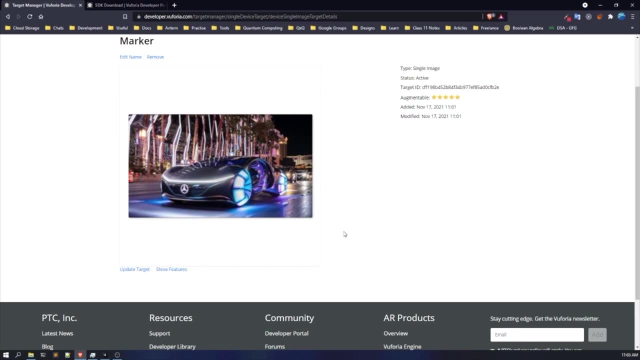 so now, as we have seen that what sort of marker we should use, so we should, you remember, we all, we always should use a marker. that is really good. now you have to click on this show features option. alright, I'm going to see here. you can see that. remember that slide, that are that in that slide there were so 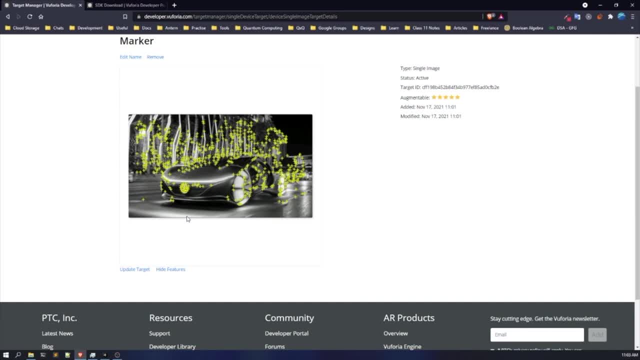 was a ganesha's picture and there were some dots in it, so you can call those as tracking points. all right, those are known as tracking points. with the help of these, the marker actually tracks the marker and helps to put it up on the marker, right? so, uh, yeah, this is. these are the details that you 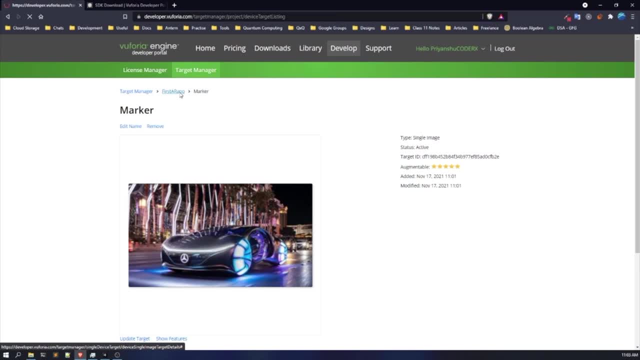 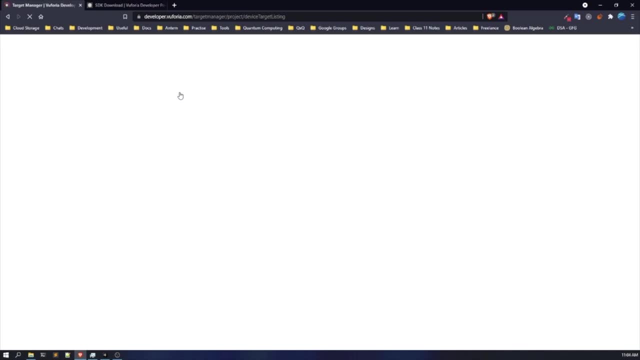 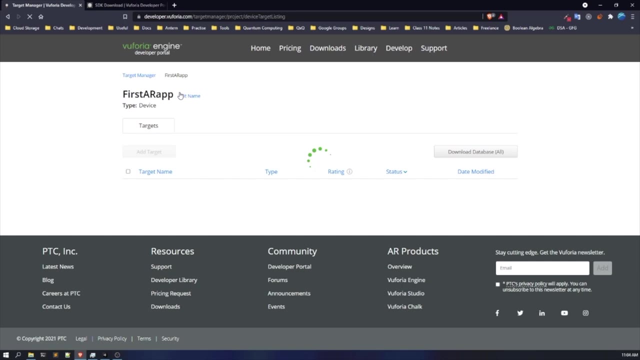 need to know. all right, and now, uh, another thing we have to do. all right, uh, another thing we have to do is to download this database and then, after that, we are going to set up our unity engine. all right, we are going to work on our unity engine, so, first of all, let uh, let the scene load, let the 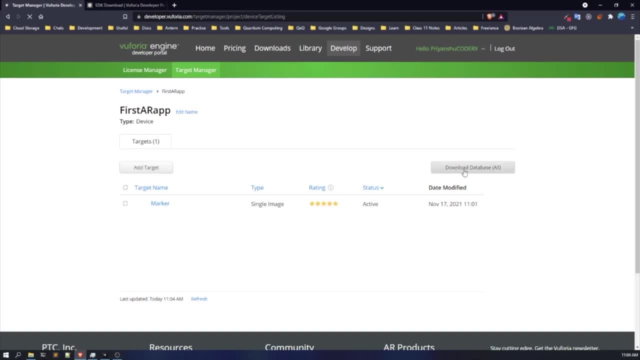 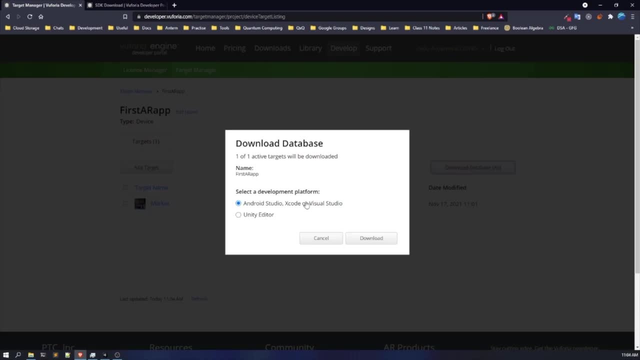 scene load. all right, and then click on this download database. all right. and here you are going to find two options that are android studio, explorer, visual studio, but of course, we aren't working on any of them, so we are going to choose unity editor. right, we are going to choose this unity editor and then simply click on download. so it is. 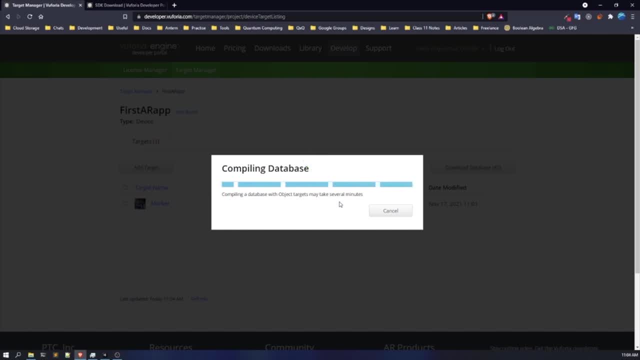 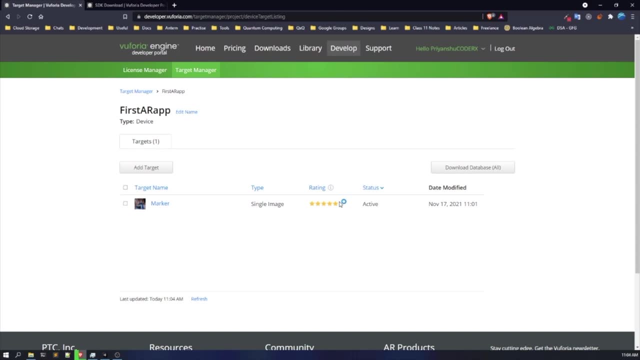 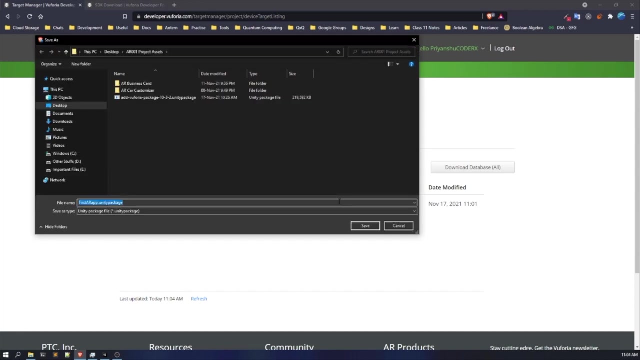 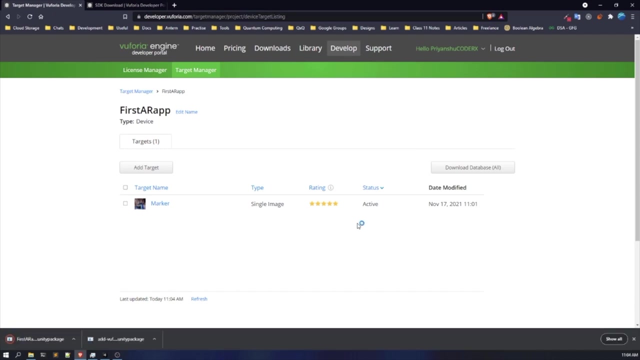 compiling our database as of now, all right, after it is done compiling, uh, we are, we are going to save that file and then we are moving towards unity, right? so, yeah, that's cool. so now just click on save, all right, and our unity package, uh, will be downloaded, just as you can see it. 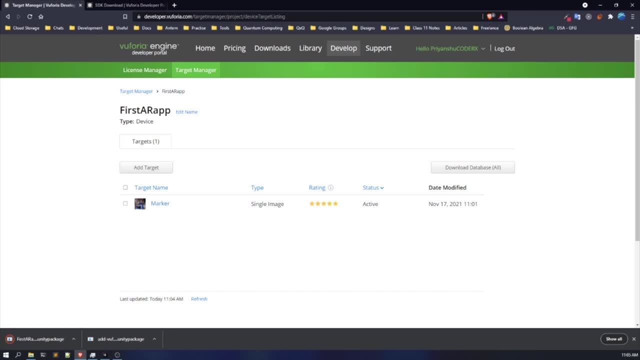 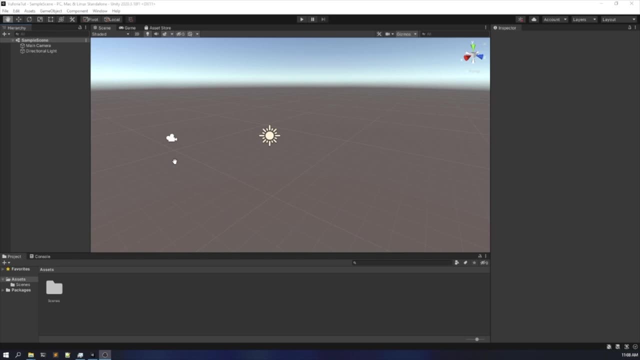 has got downloaded. so let's move towards unity. so, as uh, we have created our viewphoria assets, that is, we have created our marker and set it. uh, set a, i have set a target, so now we have to uh actually change our platform. so how would we do that? right, see, uh, basically we are developing ar application. 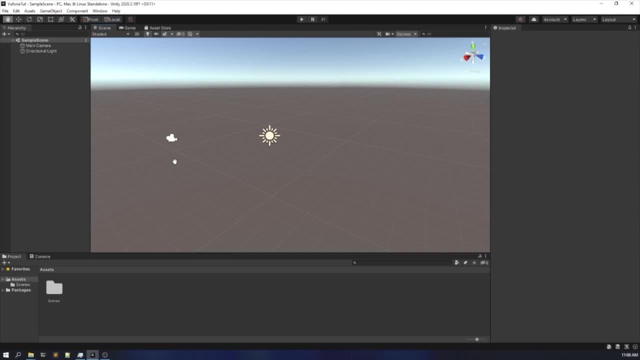 for our mobile right. so we are developing our application for our mobile right. so now we have a mobile right for our mobile devices, that is, android devices. so what are we going to do? see, uh, currently, currently, if i, if i show you, as you can see in the top, the, the currently we can. 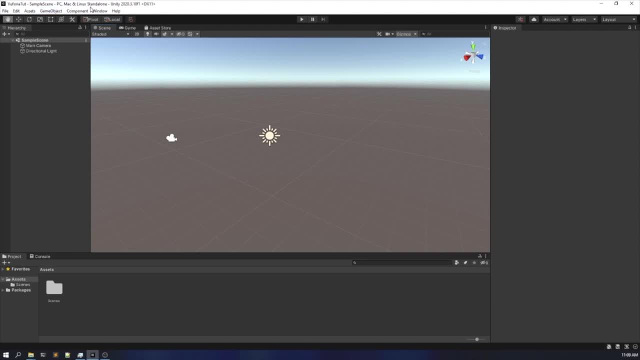 develop for pc, mac and linux standalone. right, that's what we can develop for, but we have to develop it for android. so what we have to do, it's fairly simple. all right, just go to this file. all right, then click on build settings. now, here you are seeing multiple option, that is, pc, mac and. 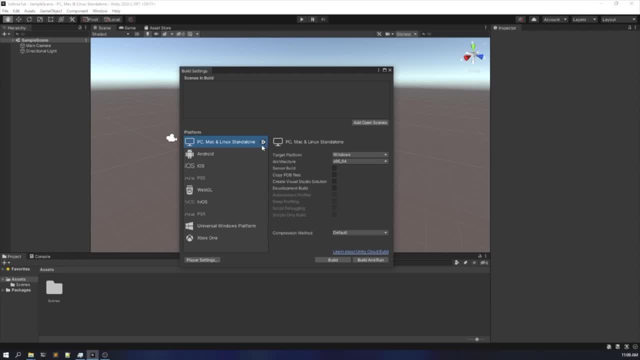 linux standalone and we have to develop for our mobile devices. so what are we going to do is we are going to click on build settings and the unity logo you are seeing here. it means this particular thing is active. all right now, if i click on android, you are getting multiple option. don't look at that. 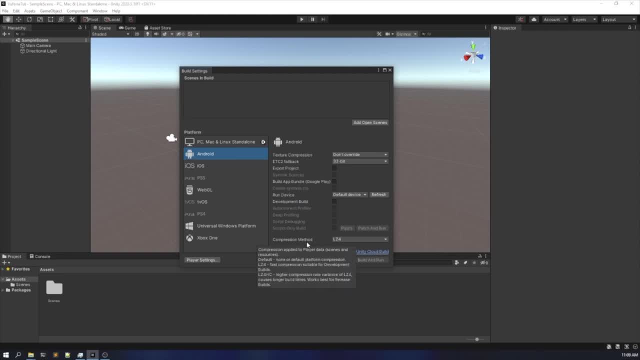 as of now. all right, you can actually take a look at that afterwards, this whole lecture. all right, you can try it out by yourself. but we have. what we have to do is we have to click switch platform. but let's say, you don't want to develop for android, you have an ios device, so you can click on ios. 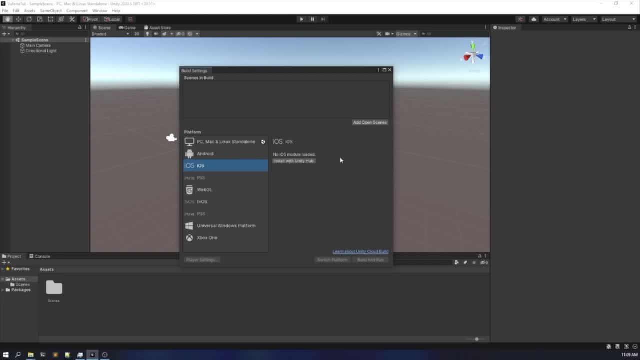 also see. these things won't work if you haven't installed the ios module. all right, i'm on a windows laptop, so it doesn't make any sense to install the basically to install basically ios module in unity. so i haven't done that, but i have android one right. so what i'm going to do is i'm. 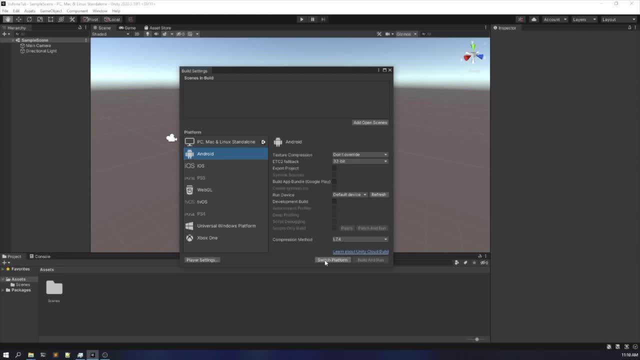 going to click on android and then switch platform. it's simple as that what it will do. it would make our unity uh. that means it would uh give the means, it would give the power to unity to develop for android. so just click on switch platform and it would start doing its work all. 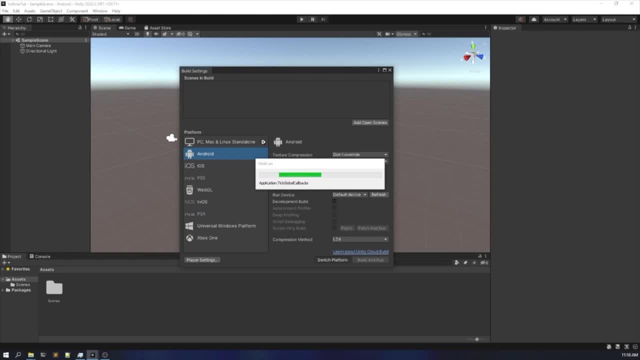 right, and after it gets switched, uh, i will return back with uh, with the next section. so now, uh, basically, our platform has been converted to android, or you could say shifted to android. now we have to import our sdk, and one tip i would like to give you guys is that, before, all right, if you are developing for any 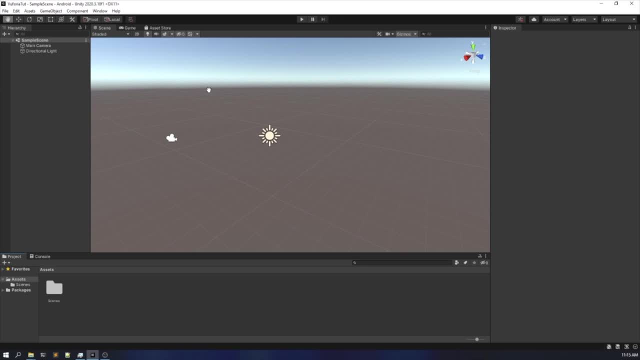 platform. let's say you are developing for android only or ios only. always remember: first change the platform, then import anything you want, because after importing- all right, uh, this happens to me a lot like, still it happens- what happens uh is basically: uh, i do the development. all right, let's. 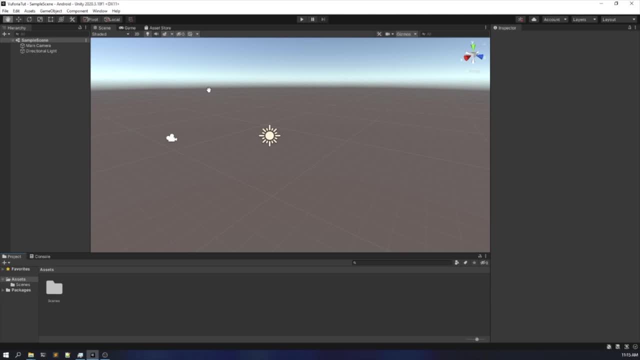 say: i'm doing it for android, all right, i do the development and later on, when uh, i notice that i haven't shifted to android platform, and you know, when uh, after half of the things are done, multiple modules will be there, multiple assets will be there in your unity. 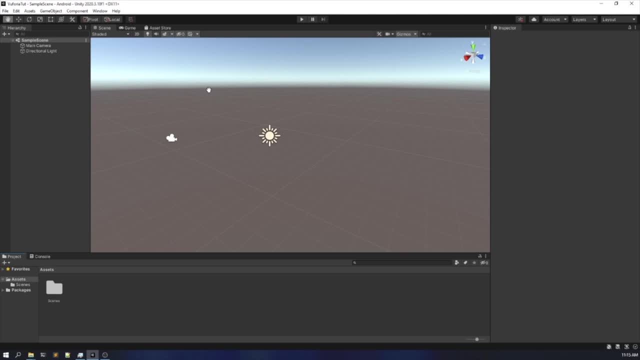 and when you will shift that now it would take a hell lot of time. so remember, whenever starting with unity, if you are going to change platform, do it, do it at the first. then only import any asset module or anything you want. all right, because it would reload all the. 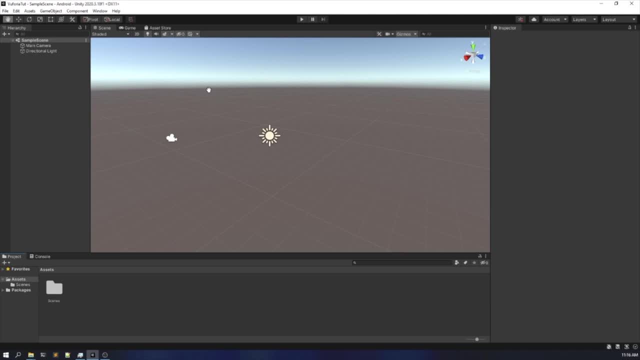 script uh things. it would uh recompile, it would uh make the assets compatible for android and all those things, background processes going on. so always remember to do that right. and now it's our fair time, all right, to import the sdk. so how we do that: two steps means two methods are there. 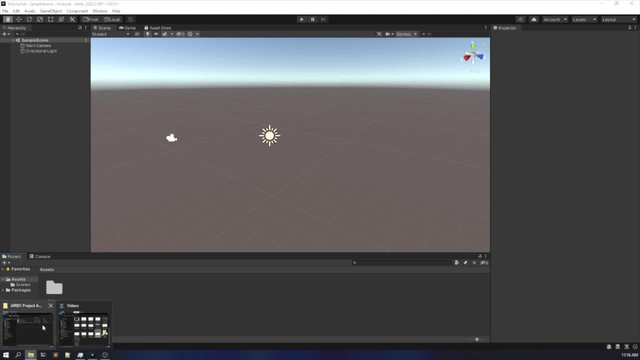 that is, first of all, simply um, open that whole folder. all right, open this folder and simply drag and drop. all right, simply simply drag and drop it in here. all right, one way is this. another way, uh, is to basically right click import package, custom package, then import it. all right, it's uh, simple. 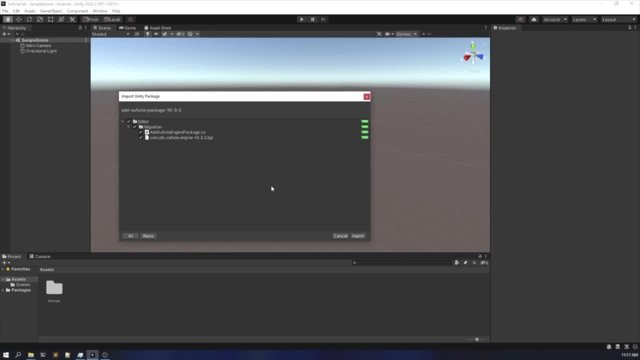 as that. well, so now, uh, as, uh, as that whole processing thing is done, now we have got an another window. all right, basically this is the package window. all right, don't worry about anything here- and just click on import, all right, and it would import your uh view for your. 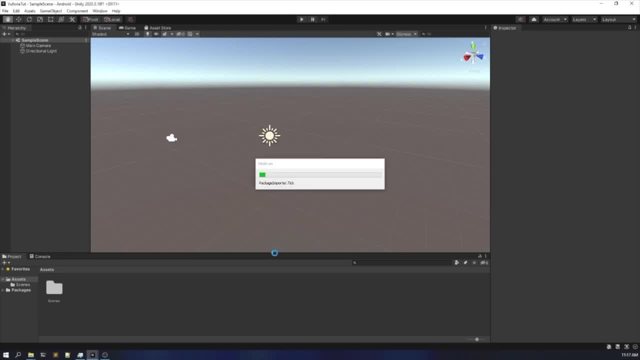 module and into unity, all right, and give it its time so that it can do so, all right. and also, when it says something like this, what you have to do is click on update, all right, and it would again start. uh means resume with the importing uh stuffs. so, guys, now our viewphoria. 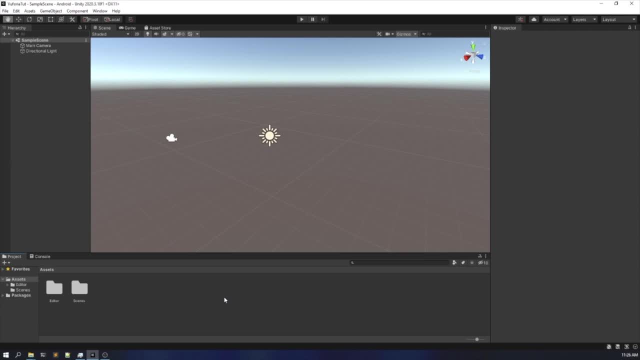 engine has been imported. all right, and one of the uh very good things, all right. actually, uh, there's a problem with sometimes, uh it occurs, or what happens is that uh sometimes, when you import uh view4d right, uh unity fails to compile it or something like that, some sort of like that happens all right, and your uh view4a. 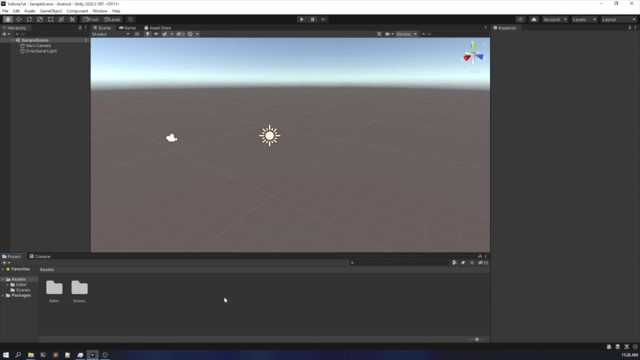 engine doesn't get imported successfully. so how would you check that your view4a engine has been imported successfully, right? so what you can do is click on the hierarchy panel, right click, and out of all these uh default options, you will get a new set of option that is view4a engine, and that's when. 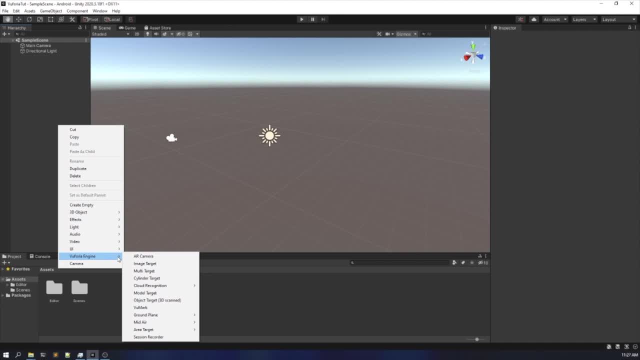 you know that you you have successfully imported view4a engine and if not, all right, maybe due to some problem, you uh, you wasn't, you weren't able to uh import it successfully- what you can do is re-import it. as simple as that, and i'm sure that that would fix your problem. 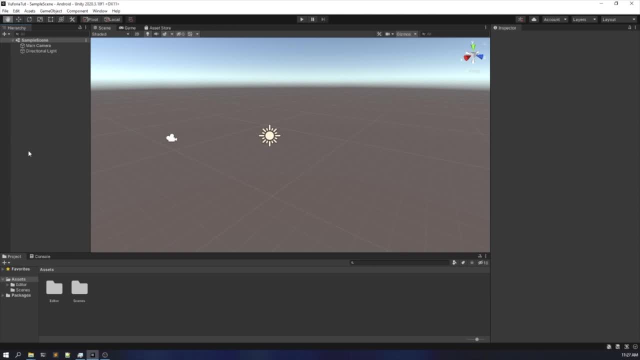 right. another thing, all right, uh. do you remember when we uh create our, create our, our marker database in the target manager in developerv4.com, we downloaded another unity package, all right. so what that? what is that unity package? that unity package contains the markers, all right, and we have to import that unity package, all right. so again, uh, previously i showed you uh. 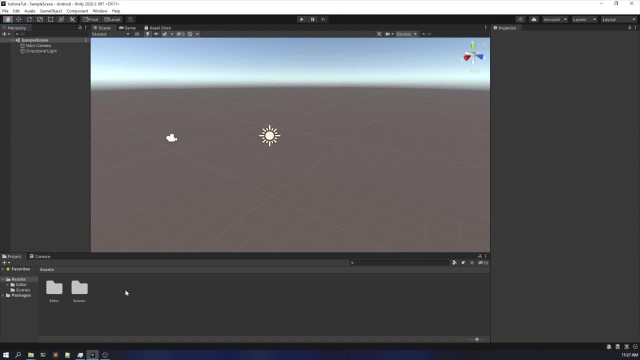 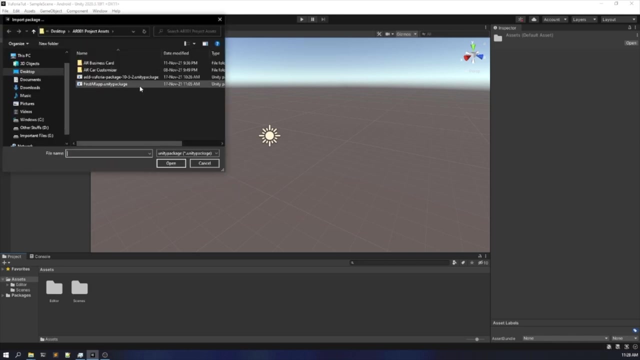 the drag and drop method. now i'm going to show you the right click method. so click on the project panel, right click- all right, all right, uh, simply, uh, simply, just right click. click on import package- custom package: all right, and then get that marker package, the, uh, the. my marker package is named cost ar app. so i'm going to 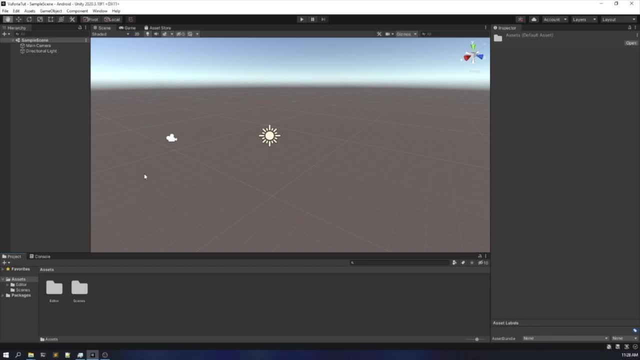 import it. all right. so again the same steps. you will get a window like this and click on import and your files will be imported. so now as we have imported our asset, all right, uh, so now as we have imported our marker database and also the view 4d engine, sdk now. 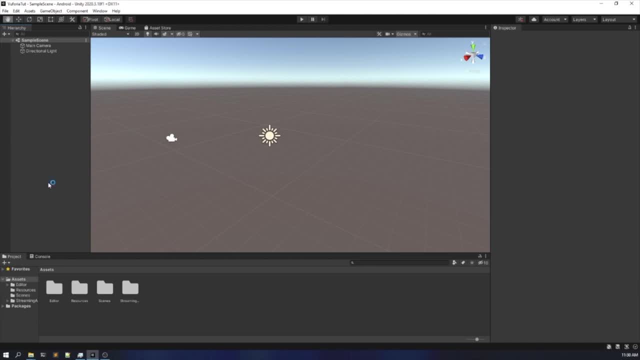 it's time, it's our very time, to develop our own ar application, right? so how do we do that? the very first thing, all right. the very first thing: our view 4d developer does: delete the main camera. we don't need that main camera. all right, because that main camera is meant for, uh, virtual rendering. 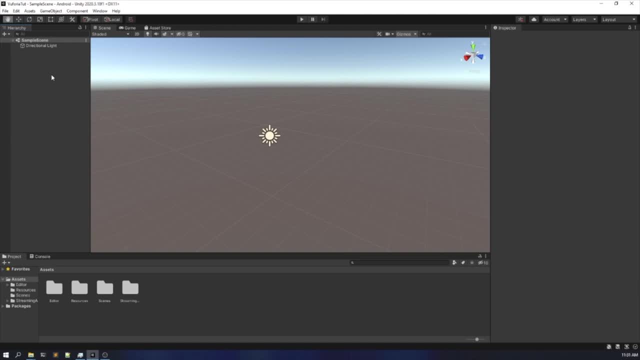 all right, it is only for virtual rendering, not real plus virtual. uh, what view 4d does is: view 4d is really good and he provides us an ar camera built into it. so just right, click in the hierarchy, click on view 4d engine and then click on ar camera. and here we go. you got an ar camera now. 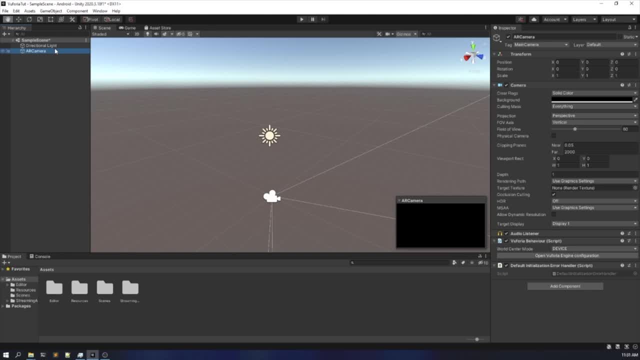 this camera is going to work for augmented reality. so you can see, the ar camera is an ar camera built into this camera. i am adding this camera to the world of the virtual reality. that is, it is going to capture the real world and put the digital object in the real world. all right, and that's what we wanted. now, remember, we copied our license. 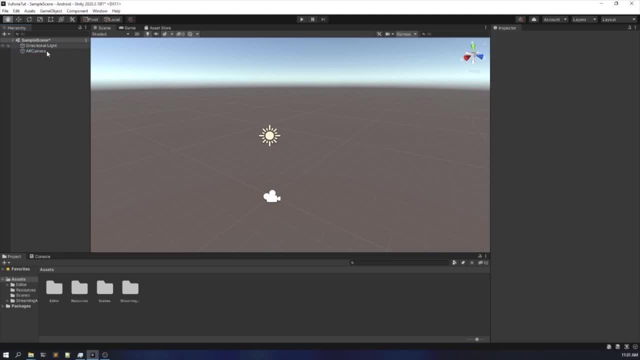 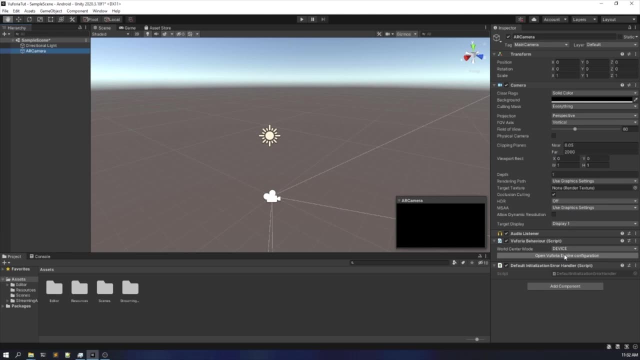 previously, uh, during the web part. all right, when we are covering covering the web part, we are going to need that license. so just click on ar camera in the inspector menu. you are. you are going to get this open view 4d engine configuration. you are going to get this open view 4d engine configuration. 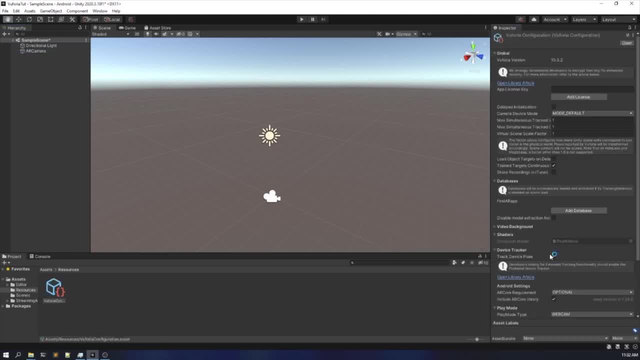 all right in the view 4d vmware. all right in the view 4d vmware script. click on that. you are going to get something like this. all right, and click on uh in this app license key section. right? this is the main section. so what i'm going to do is don't click this button. 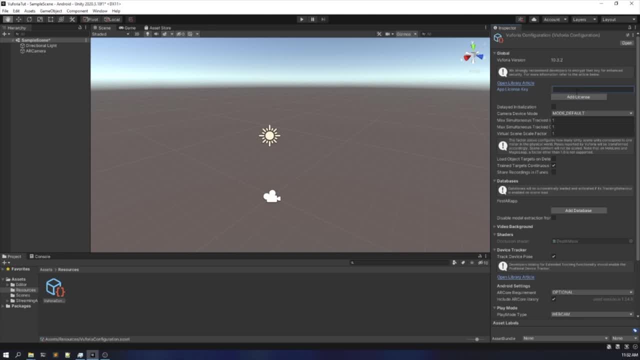 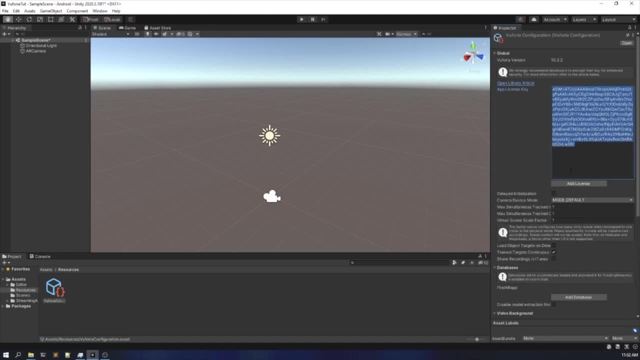 it would redirect you to that website and you have to create another license. but we have already created our license right, so i'm going to just paste that license right and voila, viewfodia got the license right. so, yeah, that's cool now, as we have done the very basic setups. all right, see, uh. 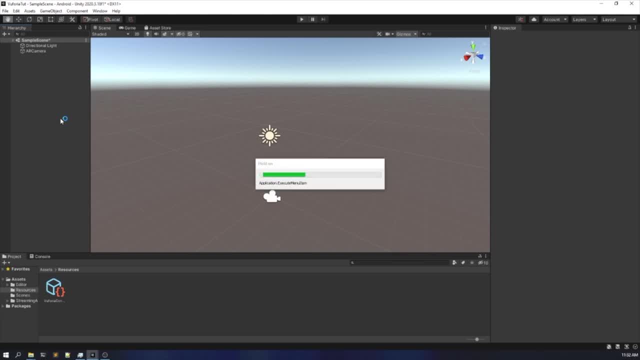 in this. in this one, i'm not going to uh tell you how to create advanced viewfilia app. this is just a setup video. and this is a video of how we set up our viewfodia. and also, uh, we'll be creating our very first ar application. 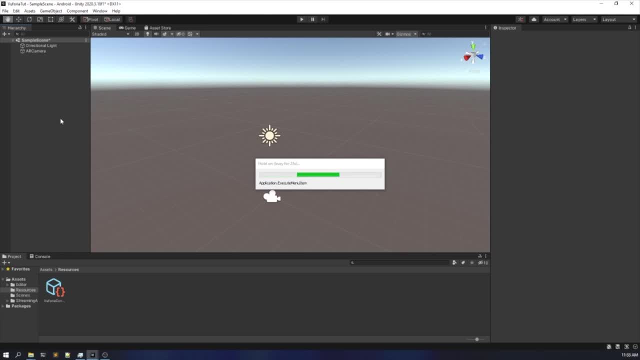 with Vuforia. all right. so unity is doing its processes, so let it do it. it's taking some time, but don't worry, yeah, it's done. now what we have to do is we have to right click again, go to Vuforia engine and now see in marker based: oh, as I 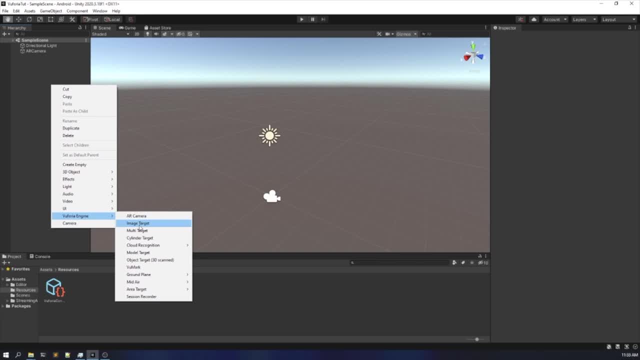 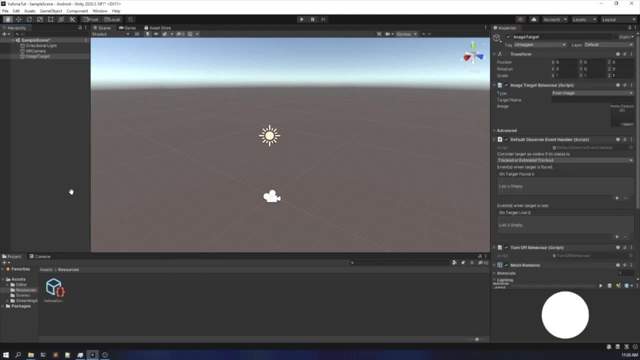 already told that we need markers. so how would we add those markers in unity? so right click Vuforia engine. then there's something known as image target. click on that, all right, and you will get another game object known as image target. right now, I know you might not see if I if I zoom it to you, you will be seeing it. 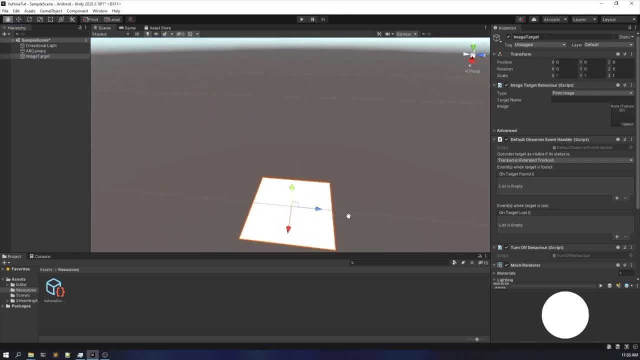 totally white. now, believe me, this one, we have a fix for this, right. see, by default unity uses image type that we have to specify from unity. only this, that is, image uploaded in unity. but as we already have a database, all right, we already remember, we made a. 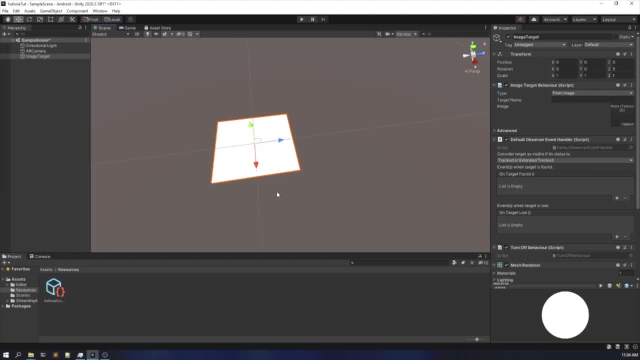 database. we made a target manager database so we are going to use that. so click on the image target. all right, go to this inspector menu and you will find something called image target behavior. all right, don't look into another other options. we are going to explore these options in our next term list, like in: 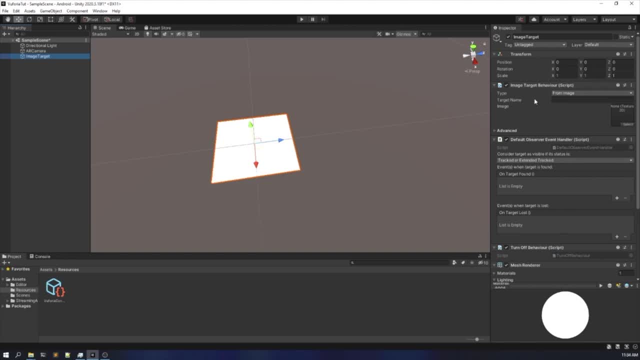 project videos or next videos. so what we are going to do is click on this type of selection menu. all right, and from here you would find multiple things: cloud reco, basically cloud reco. what it does it? it fetches the data from cloud, that is, the images from cloud, and here is from database that we uploaded in our 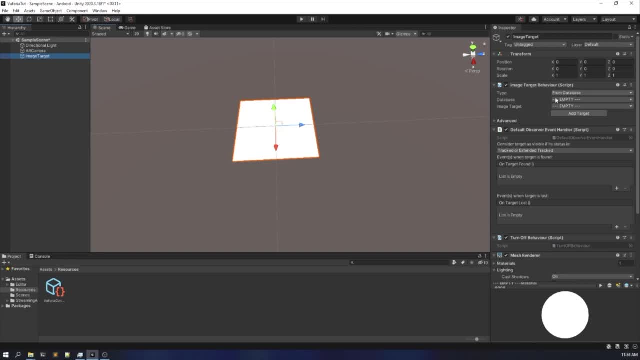 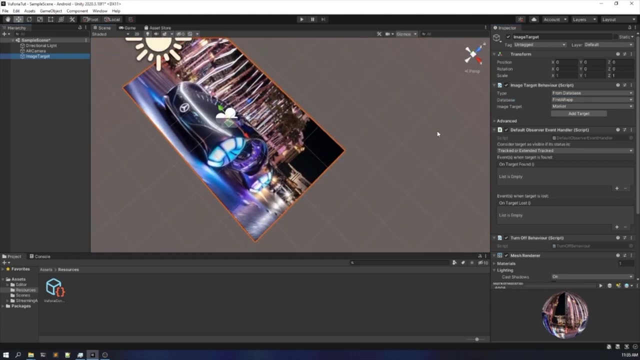 unity. all right, and now we have selected our database. now we have to select which database. all right, maybe we have multiple database in our AR application, so we can. we have to select it. that is our first era. and voila, it will automatically get you the first marker, the very first marker available in the database we have. 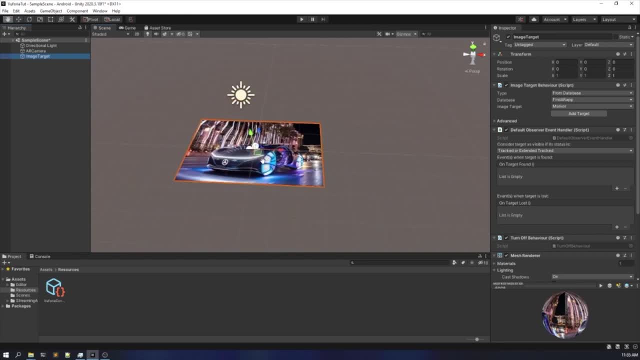 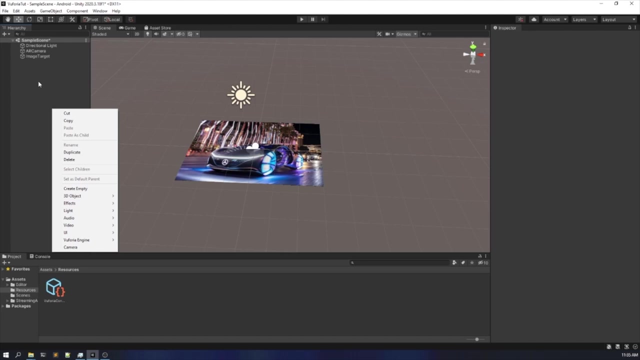 this marker available in the database, right? so as simple as that, nothing too complicated. now, what we have to do is all right. now what we have to do, we have to right-click again. all right, see, I'm not going to include any 3d models, right? 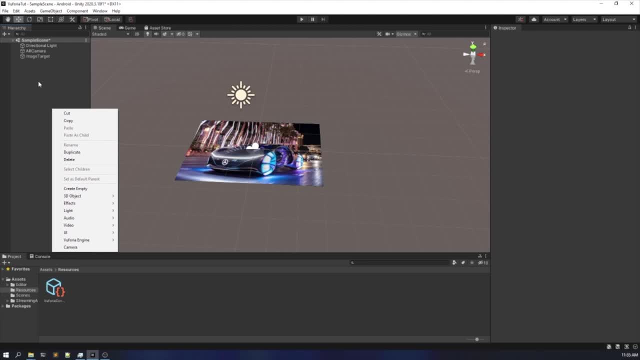 now. all right, yeah, we'll be doing that in our future videos, but as of now, this is on this, only a set of video, so just add a 3d object. all right, add your favorite 3d object. there's no favorite one of mine, so I'm just going to add a cube. yep and voila, a cube got. 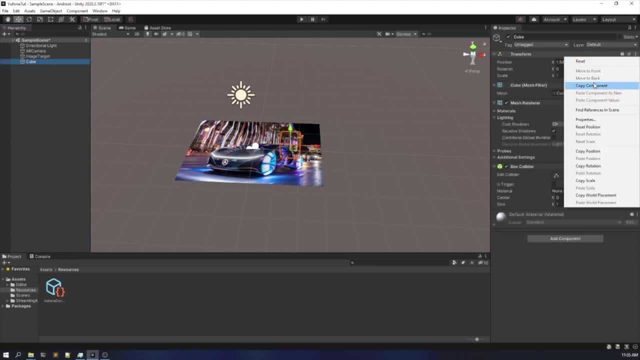 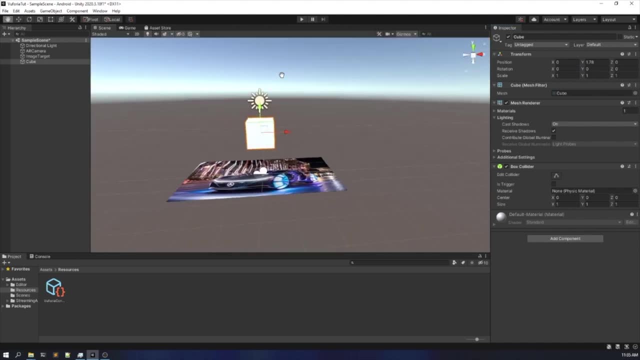 added. now reset it, transform, or a reset: it's transformed, so it's back to zero. all right, and put it up a bit. right. put it up a bit and voila, you got your cube. now if you play this, all right, if you play the scene, the cube will be there. right, the marker won't perform its. 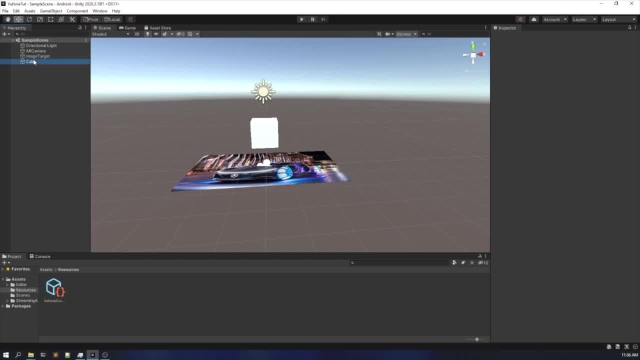 functions. why? because you haven't put this cube inside of this image target. so that's what we have to do. we have to make the 3d model that we are using the child of the image target. all right. so now we are good to go. all right, that's. 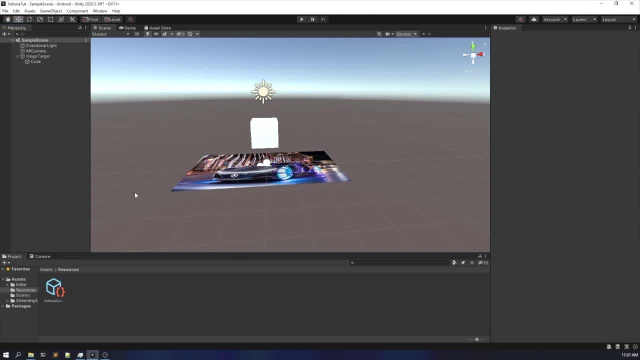 cool right, one of the good things of unity and view for you is that you can test we've on your pc only. so how would we do that? uh, just click on play button, all right, and it would start the camera. all right, nothing too complicated, so let's do that. 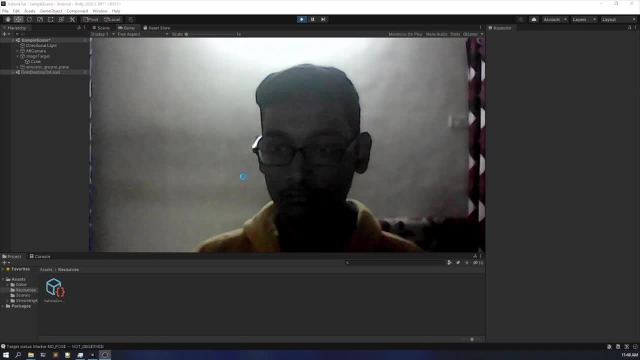 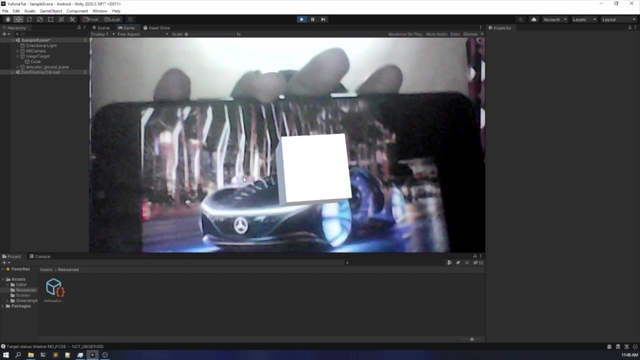 so now, if i put the camera, all right, i mean if i, if i basically put the marker right in front of the camera, right, uh, it would start tracking the cube, it would start showing the cube. all right, just see it in here, right, you can, you can see it clearly right now if i remove it, all right. 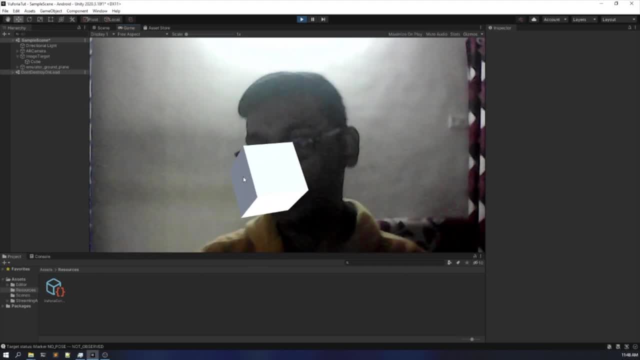 you can see that the cube is staying here. all right, now, this is a feature that called extended tracking of uni, for viewphoria only, but it is useful also, but not in this case, so i'm going to remove it. how would you remove that? all right, just get out of the play mode. all right, uh, so i 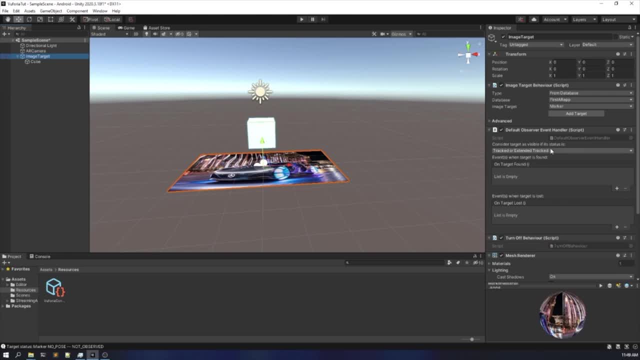 got out of the play mode. uh, click on image target. then here is a. uh in the the different observer event handler. only. here you are seeing multiple or an option that is tracked or extended tracked. so what I want you is to select only tracked, all right, and what would do? what it would do is it would set like it won't. now it. 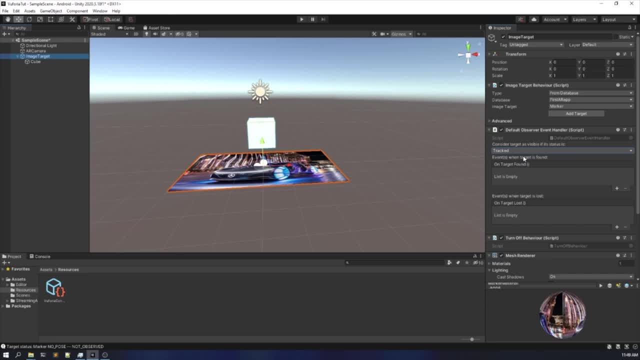 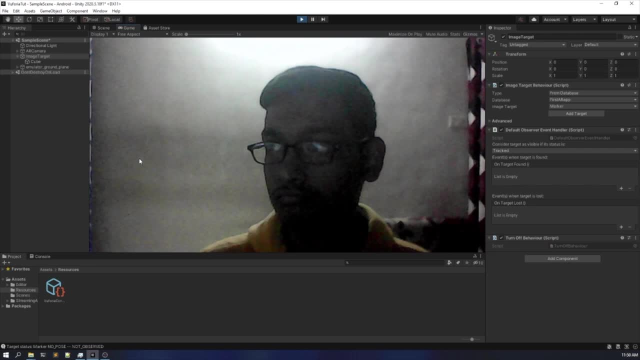 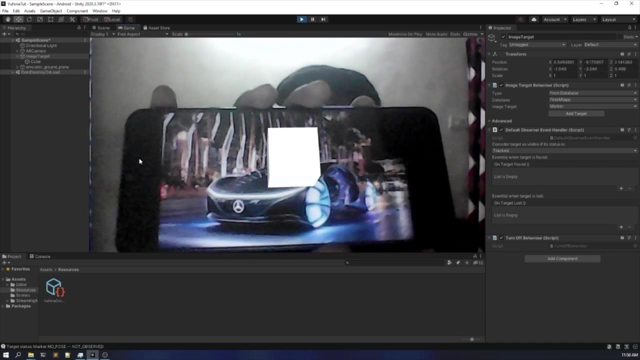 won't have the feature, all right now. it won't have the feature of extended tracking. all right, let me show you by entering the play mode. all right now, if I, if I show you, all right, just just check it out in here. see, the cube is here, right, the cube is here now. as soon as I remove it, all right, as soon as I. 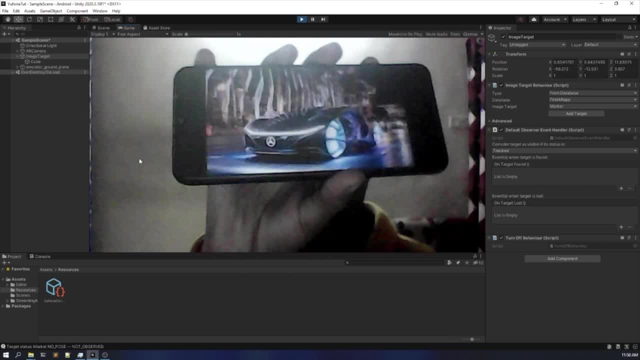 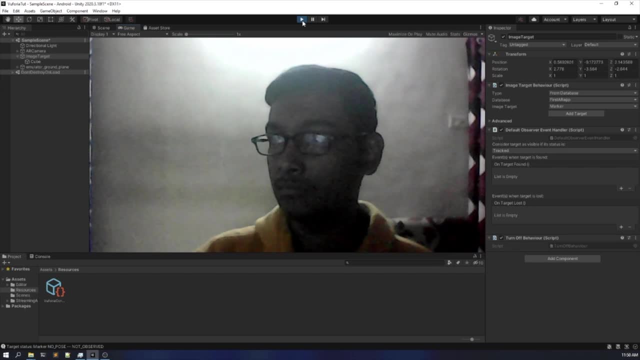 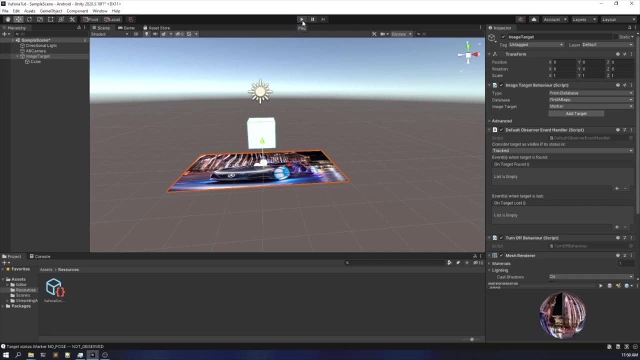 remove it, the cube goes away. right, see, the cube goes away. so this works much better if you try it on Android, all right, so I would recommend you to build that application. I would also show you how to do that. all right, I would recommend you to build that. 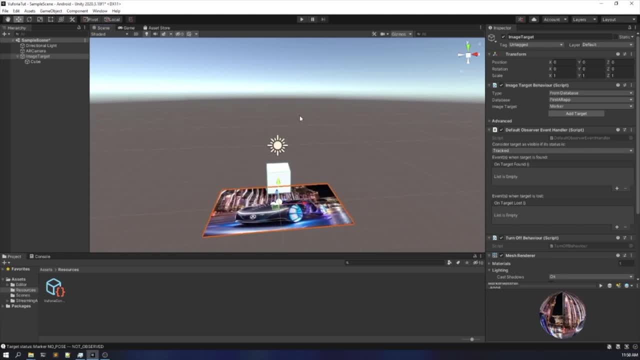 a Sala application and then try to try it out on your Android phone. so- and I guess you all are happy- all right, you created your first AR application. I know that this is a cube, but the project would be doing is going to be really interesting. all right, it is going to be really really really interesting. so now to 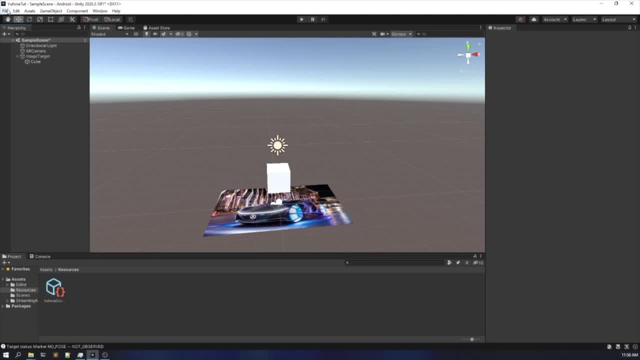 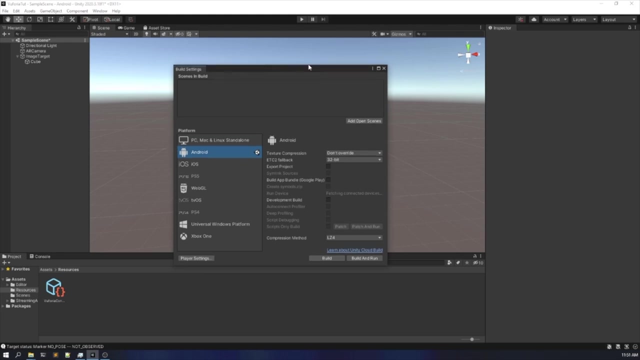 build our view for your application. what do you have to do? see, I already told you in the very first video of installing: you have to have the android module open- jdk, all right, ndk and all those things- so that you can make the things work right, you can build your application right. if you don't have that, then 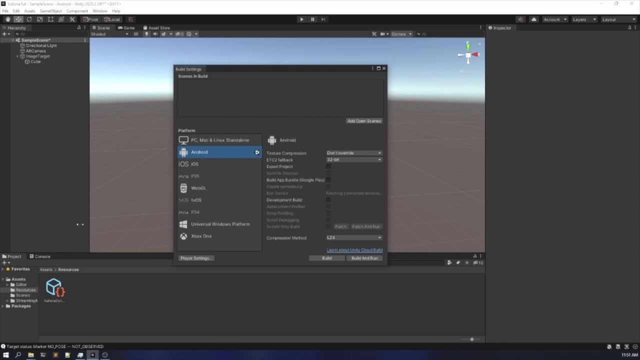 it would be a problem. all right, and now what you have to do is go to asset. all right, now the scene. all right, uh, the scene we are on is known as sample scene. all right, we are using the sample scene and in here in in this particular section, you have to add that scene. all right, you can just. 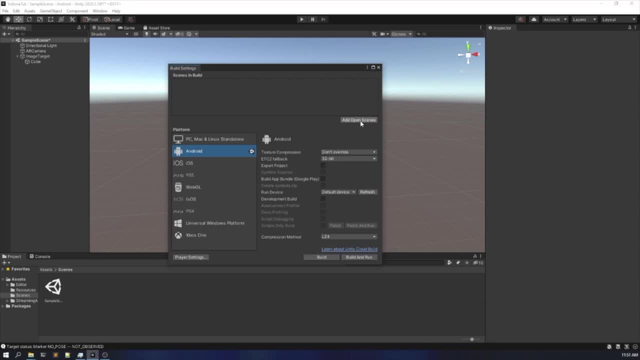 click on add open scenes, like it would add the scenes that are currently open. my sample scene is open. i can simply click add open scenes. you can even add uh it by drag and drop, right, it's as simple as that. but as uh, now we have added, all right, remember, without adding the scene. 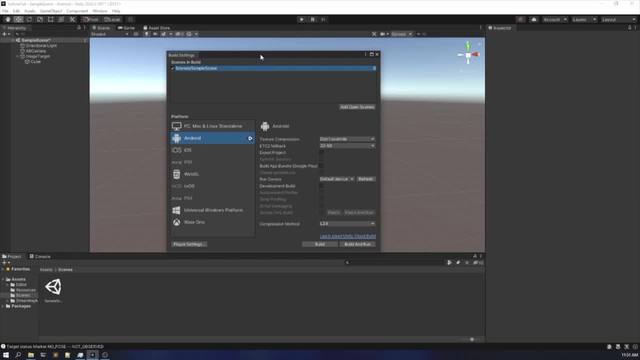 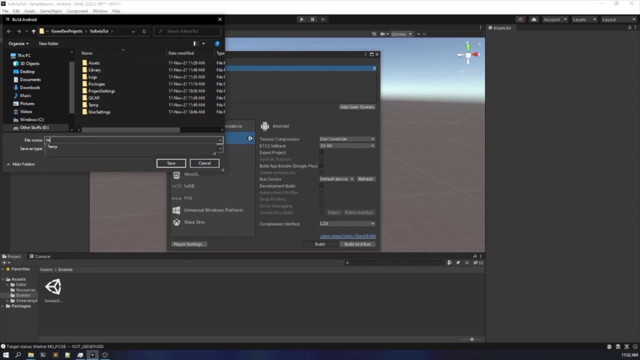 if you build that application, it won't work out right, so it's really important to include the scene you are working on, then click on build, all right. then uh just click on build and then uh name your application. i want to name it test, all right, and then click on save. it would start building, building your application. 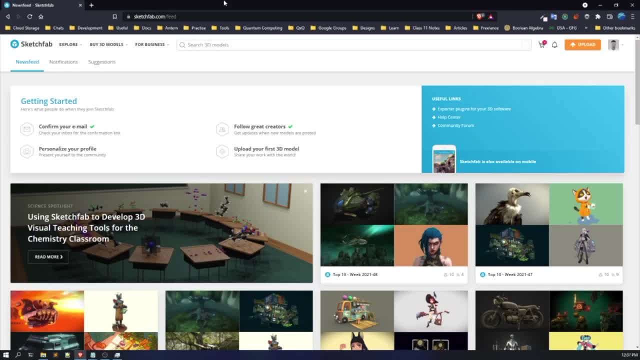 in this particular section of the video, i'm going to tell you about some of the free resources that you can use and how you can use them to build your application. so i'm going to tell you about uh in your development. all right, see, as a exact developer, i need 3d models, animations, all the 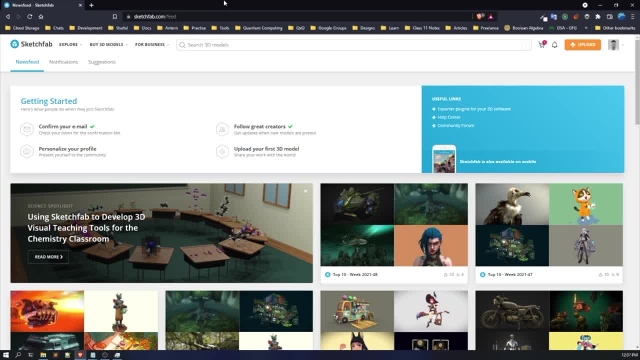 time. all right, and these resources are a lifesaver, believe me, like when i started. see, i am not a 3d modeler, all right, when i started i didn't knew about these things, but i got to new over time and, believe me, these resources have helped me a lot, and one of the resource is sketchfab: see sketchfab. 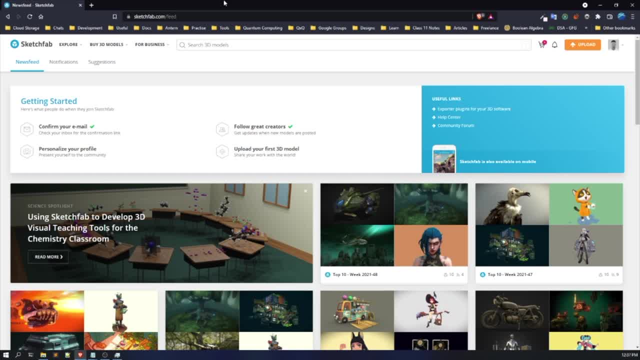 is a really good place to find your 3d model. all right, see if you, if you want a 3d model of a car, you can just search for it. you will get multiple 3d models for free. all right, there will be paid 3d models. free 3d models too. you can get your own, all right. so sketchfab is a really great place. 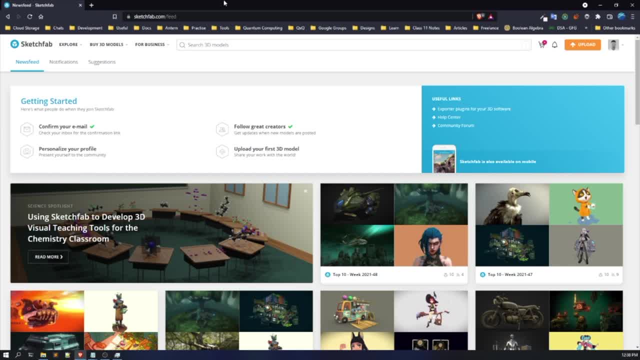 if you want some other options, all right, if you want some other options also, there is, uh, another that is cg cg trader. i guess its name is cg trader. then there is turbo squid. all right, turbo squid, is there? there some some sort of free 3d models are available. 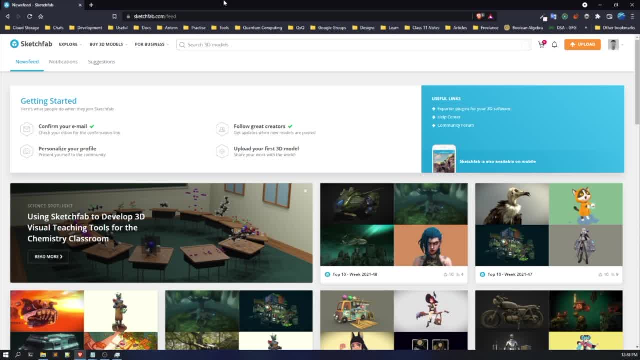 also. there are also available in there, but what i prefer the prefer most is sketchfab. sketchfab has a lot of 3d models available for free, so i'd suggest whenever you're looking for in 3d model, go to sketchfab. this is from where i get my 3d models. all right. 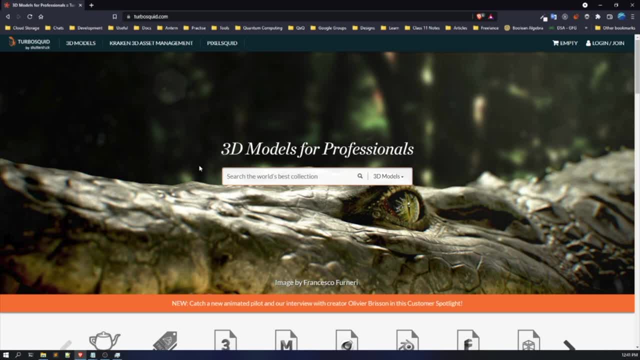 so here's another resource that is known as turbo squid. i already told about it to you, but let me show you see, this is another website from where you can get multiple 3d models for free and also for paid. all right, you can get it from here. it has multiple 3d models of. 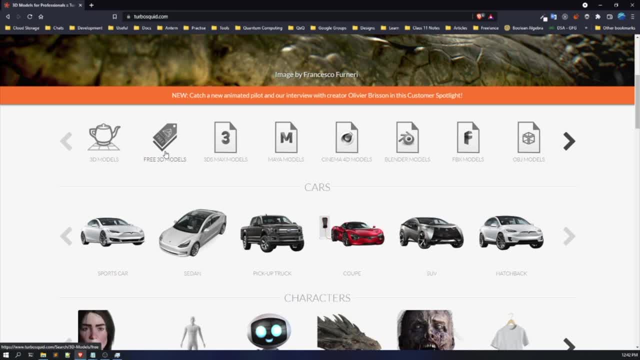 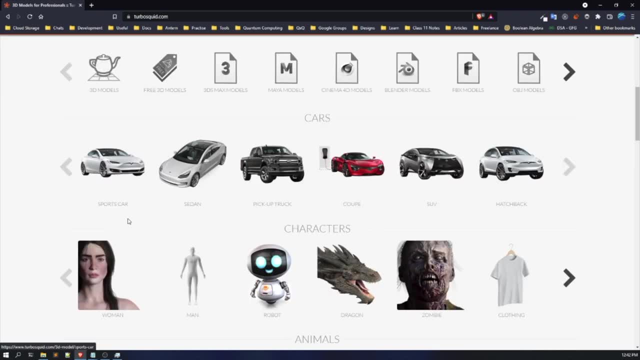 3ds like it. you can get blender 3d models, cinema 4d models, maya models, 3dx models, obj models, all right. similarly, you can get cars, models of multiple cars, you can get models of multiple characters, you can get models of animals. 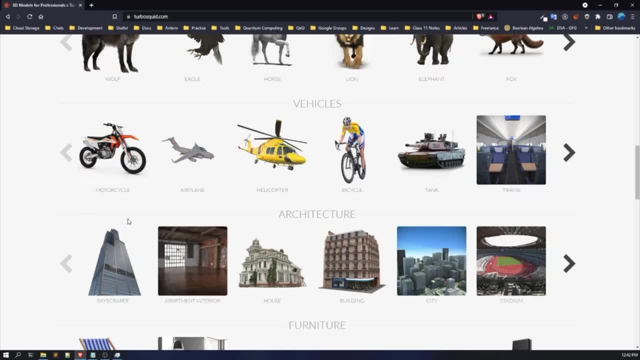 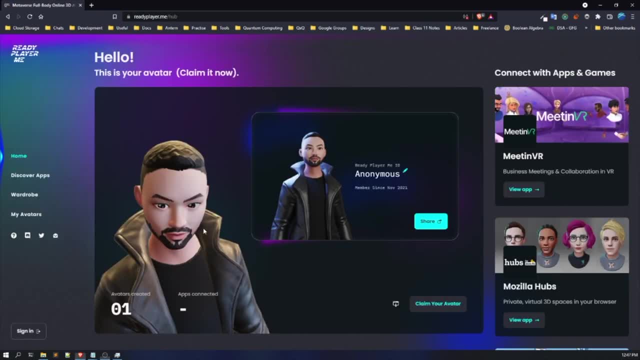 then there is of vehicles. you can search for any model you want, all right. so this is another very useful resource that you should have a note on. this is another resource that you can make use of. this is known as readyplayerme. see, if you want avatars, all right. if you want avatars for your. 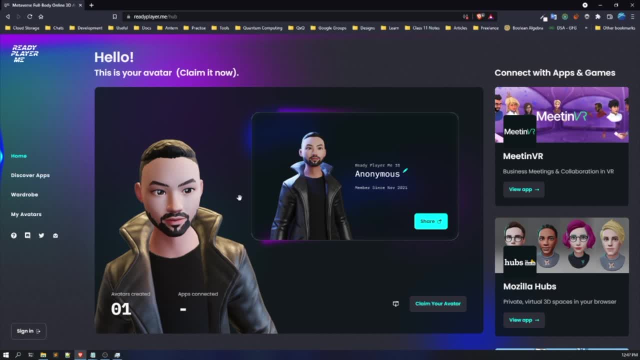 games. let's say you want your own avatar, you can go to this website. uh, go to this website and make your own avatar based on it, you all right. you can make your own playable characters with this readyplayerme- all right, there is a really good avatar creation engine. even if you want to build your own, like if you 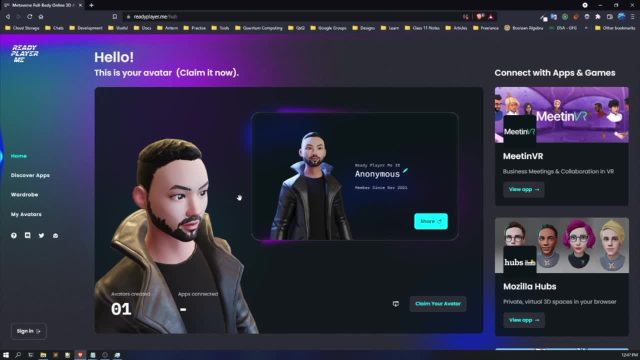 want to implement? all right. if you want to implement this readyplayerme avatar engine, they also have a unity plugin for it, so you can check that out too. all right, the thing that you are currently seeing is a is a output. all right, there is a 3d model that i customized, all right. 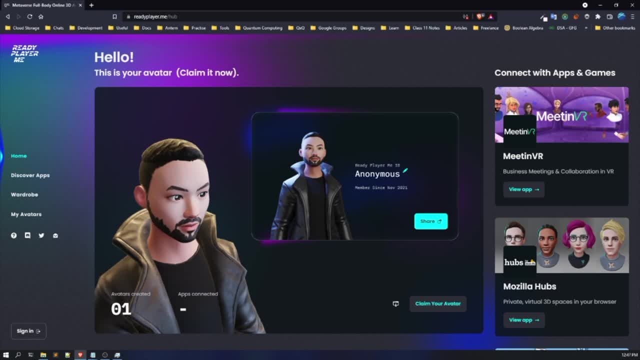 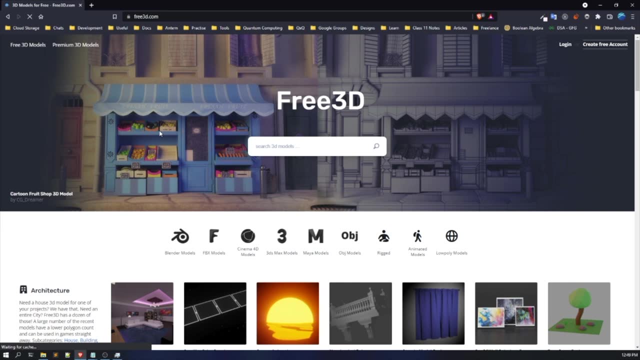 that i customized. so there is a 3d model that i customized, and even you can make your own avatar. so here comes another website, all right, from where you can get a lot of free 3d models. all right, there is a really great website. i prefer this one too. all right, my next uh means after sketchfab, my 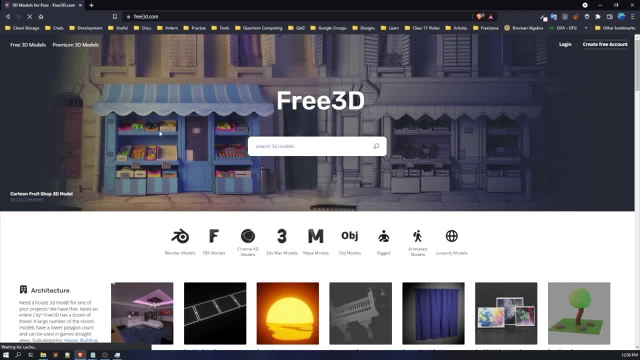 next choice is always free3dcom. you, you can uh, don't worry if if you are, uh, if you want these links, all right, i will provide a link down below. all right, i will provide all the links of the website that i am using down in the. 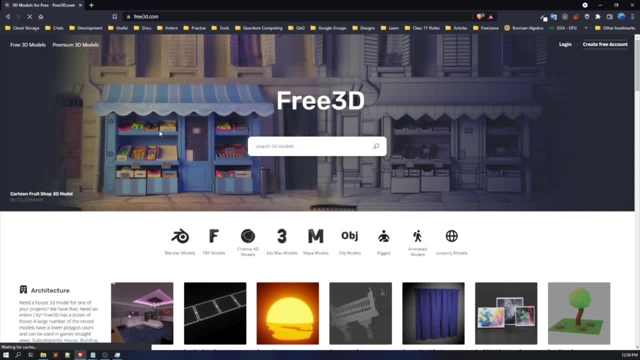 description or description box, and also i would also create a pdf of it and upload it on my course website. all right, so you can check the links from there also. so free3d is also a really great website from where you can get a lot of free 3d models, all right. so if you want to make 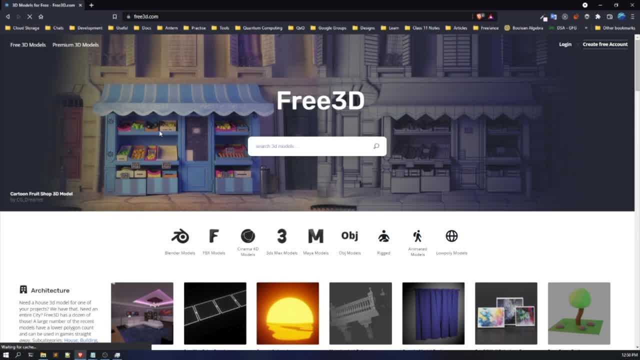 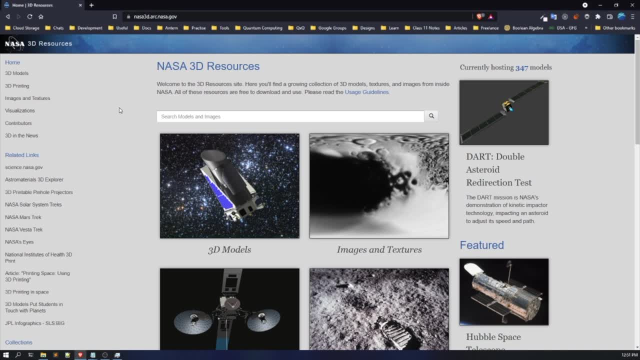 a lot of free 3d models, so this is also one of my choice. here is another website, all right known as nasa 3d. uh, here you can get all the free resources from nasa. all right, the- i guess all the models in here are totally for free. you can get all the. 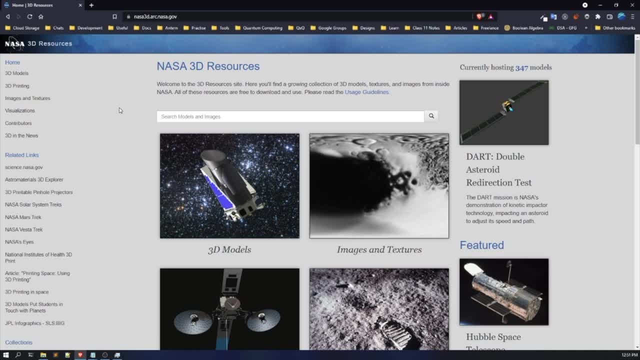 models or free models related to space, all right, related to nasa at this place, all right, i would provide the link down below. so this is another great platform for you to get a lot of free 3d models, where you can get the 3d models. it also provides you textures, all right. so this is a really great 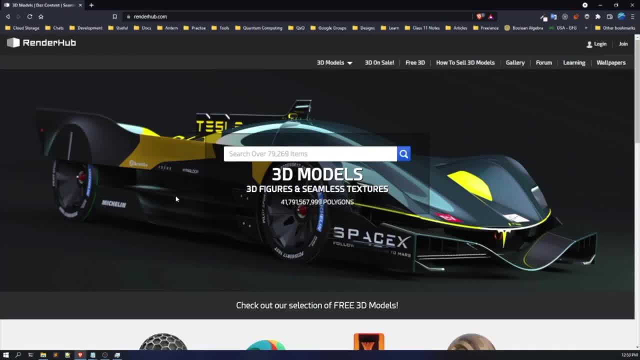 place. so this is another website known as render hub. from here also you can get a lot of 3d models, both paid and free, so you can search any model you want. all right, and i'm pretty sure that you might get those models in here. all right, even sketchfab is also there. i already showed you. 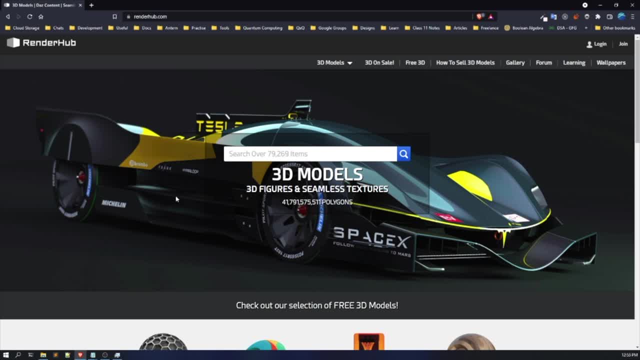 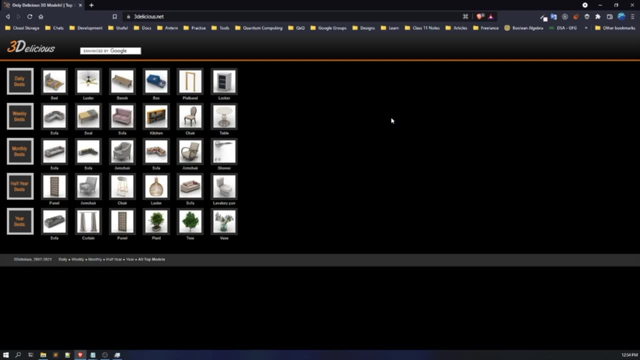 abu squid is there. then there is free 3d. now comes render hub 2. all right, so this is another resource. all right. this is known as 3dlicious, so it can. if you want any sort of low poly household items, you can get all the things from this website, this particular 3d website. so this is a really 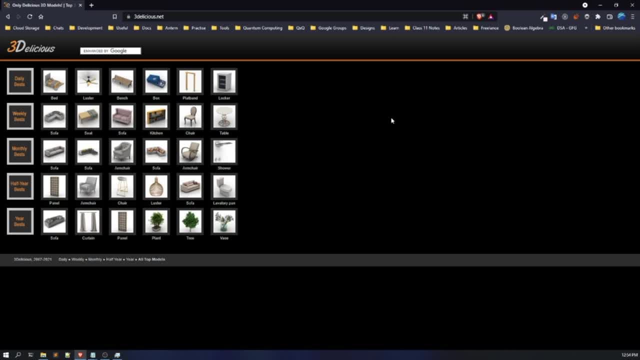 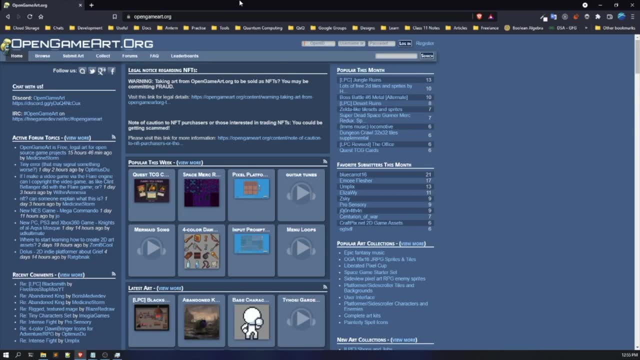 great platform also, so you can simply go into this website and download your 3d model. here's another resource called 3d licious, so this is a really great platform also, so you can simply go. another resource known as open game rorg. this is a really great website if you want to have. 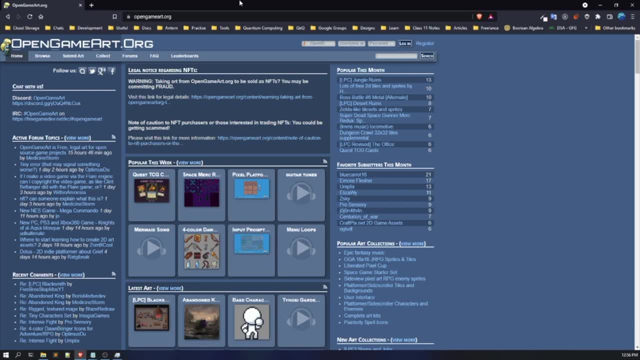 free assets. all right, free ui assets for your application. you can go to this website, all right if you want. if you are making any game, this website is also going to be really helpful for you for getting the ui assets for free. all right, so it contains both paid and free assets. 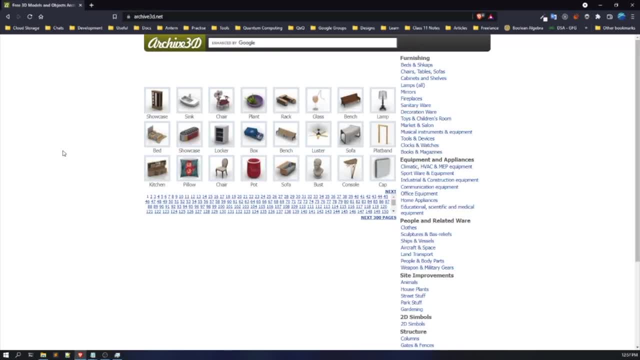 this is another website known as archive3dnet. all right, from this website you can get any 3d model totally for free. all right, none or none of these models available in here are paid. so there are free models means the models that are available in. 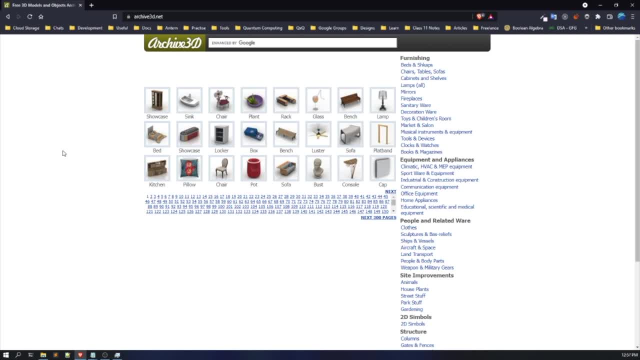 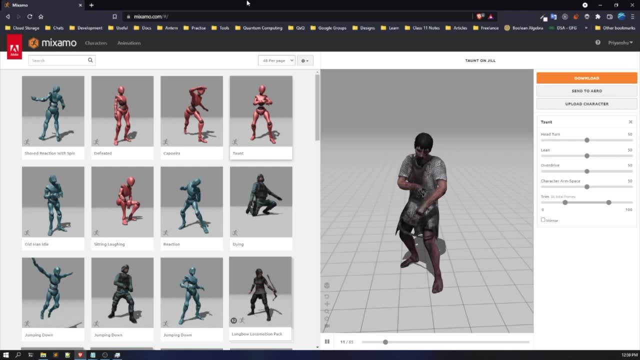 this website are totally for free, so you can also visit this website and search for your models. here comes another free resource known as mixamo. this free resource is provided by adobe. you can add animations to your human animations, and you can also add animations to your human animations, and you can also add animations. 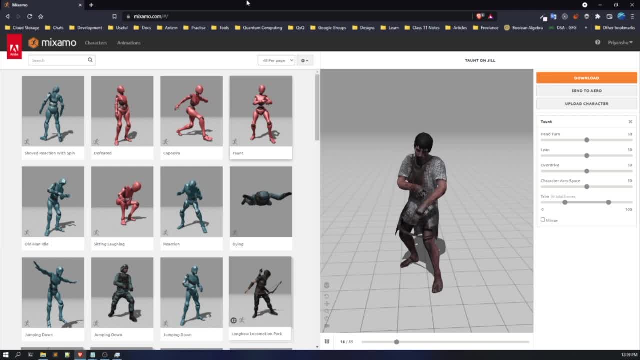 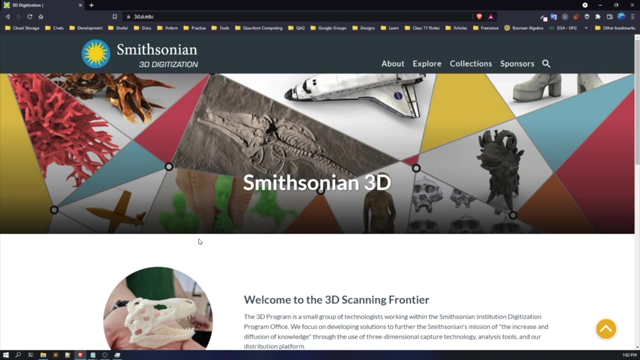 3d models, and there's a really great website that you should look for. yeah, this website lags a bit, all right, but there's a really great website from where I get animations for my 3d models. all right, so here's another resource. all right, this is going to be the last resource of the video that. 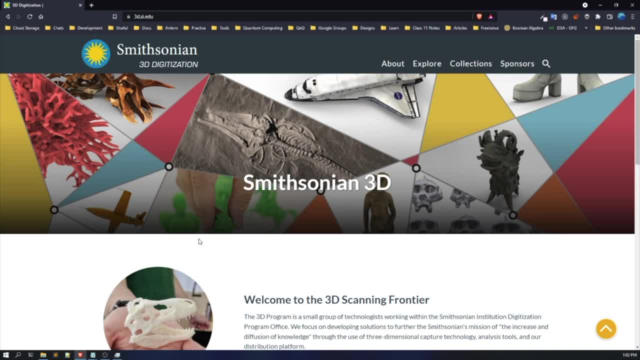 I'm showing, all right, but there are plenty of more resources available over the internet. all right, I would include all the additional resources that you might need also in the. I would also add them in the PDF, all right, that I'm going to share with you. all right, and to get the PDF, you 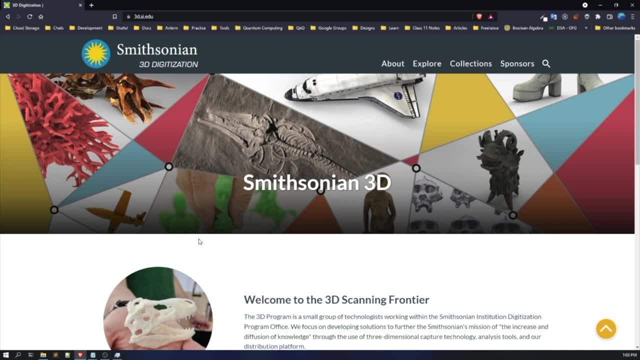 can simply search for it in the description below in the video, and also you can get that from the course website. all right, so this is. this is another website that says Smithsonian 3d digitization. all right, this is also a really good website for getting 3d models, as you can see. 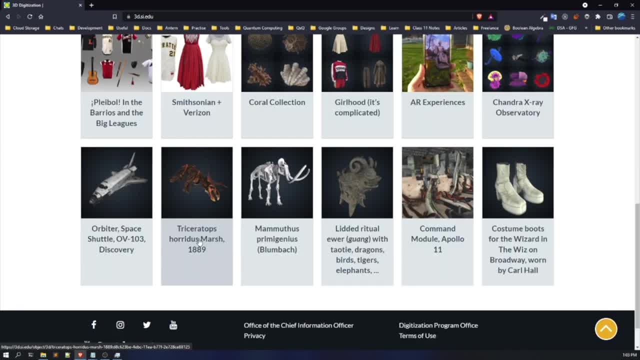 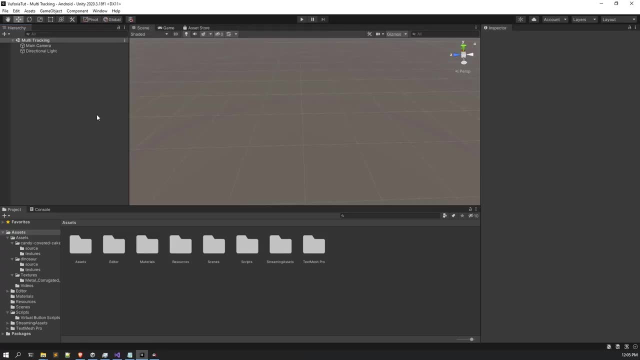 here. there are many models available like of for like, skeleton of triceratops, all right, so this is also a really great resource. all right, so this much for this video. in this lecture, we are going to look into multiple tracking, all right, so this is basically a feature of view for ya, where you 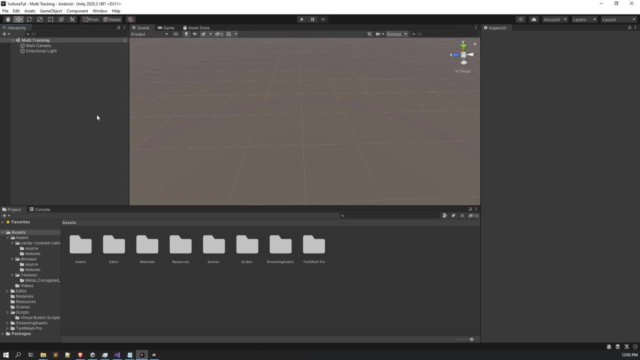 can track multiple markers at the same time. all right, it's, it's a. this one is really useful whenever you are making an AR book. all right, you, whenever you are making games. so these, this feature has a lot all right, like, for example, if you are going to make an AR Pokemon game- right. 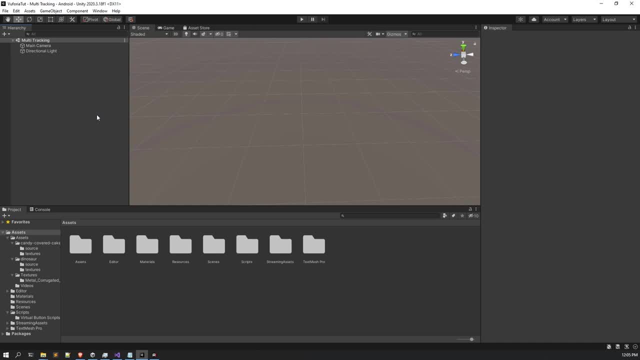 so with within one mobile there will be one, there will be two carts and you would be scanning those car and make, and two Pokemons would appear and you would make those two Pokemons fight each other, all right, so multiple market tracking helps a lot in many ways. all it and in two things. 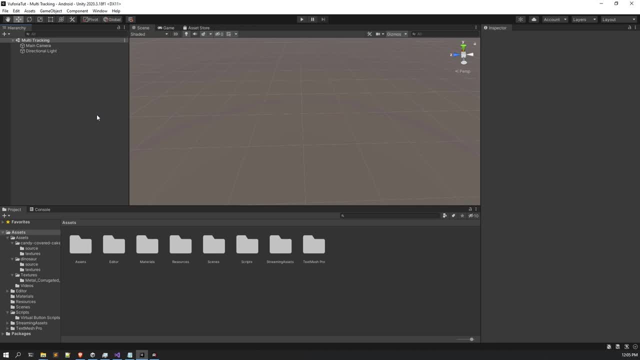 to this lecture only. I am going to show you all right. so first of all, I want you to set up your viewing le classic reenactment site, or multiagara and shot Prophet, and let me implement this for v como account, your sd case. all right, you already know how to do that. i have shown you in my previous. 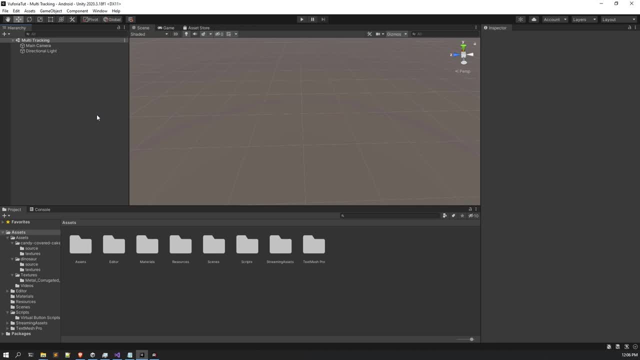 video. so if you are confused you can watch it, watch that particular portion again, and if you have any doubt, you can comment it down in the comment section. all right, so without any further delay, let's get started. the very first thing you have to do is click on this main camera and delete. 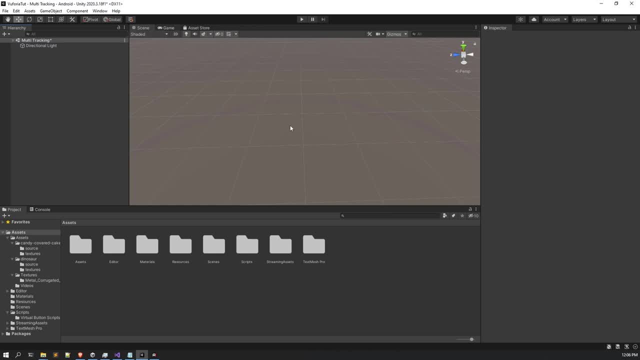 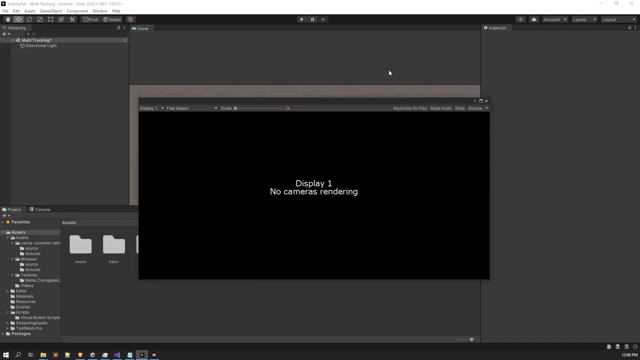 it all right, because of course, we don't want the main camera. and one more thing i would like to do is to stack up, stack this game window, or to the side, all right, to the side of my scene window, so that i can see whatever thing is happening. all right, so, yeah, so just wait a few seconds, all right. 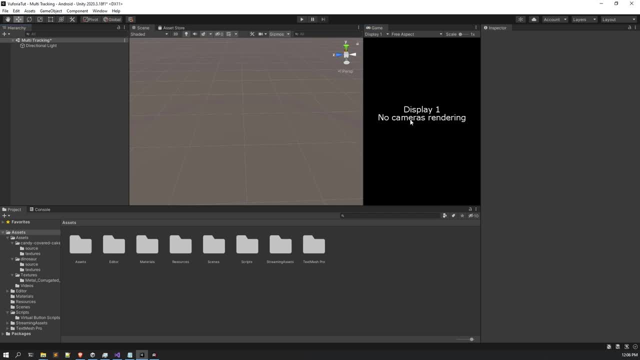 cool. so here you can see that it has been written no cameras rendering. that's because we don't have any camera. so now what you have to do is click on hierarchy, uh, go click on viewphoria engine and select ar camera. all right, uh, so you can keep it like this. 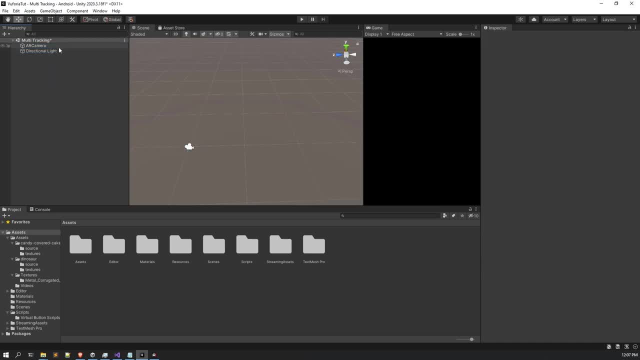 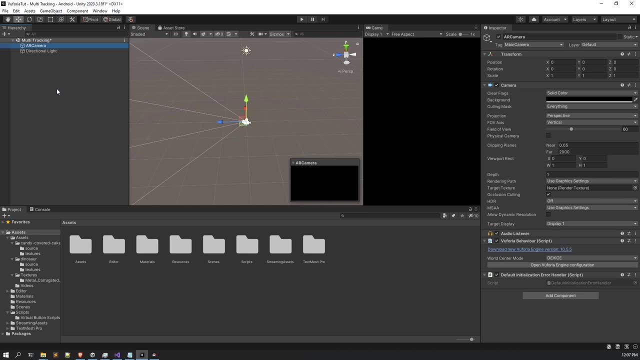 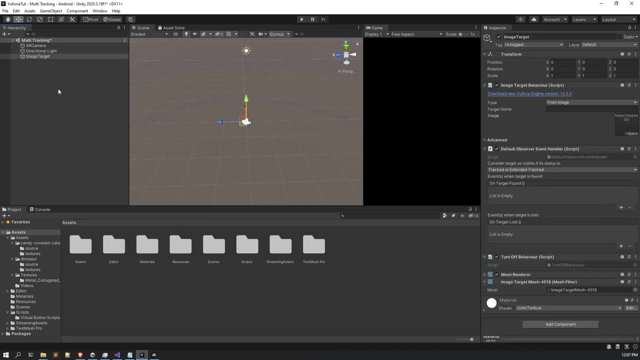 or you can stack it up, uh on top of directional light. i prefer stacking up on uh directional light. it feels better, actually, looks good, actually. so that's why it's just a personal preference, all right. and now what you have to do is uh click on, i mean right click. then again uh click on image. 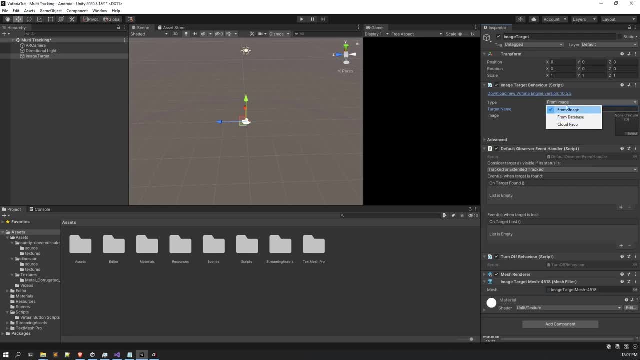 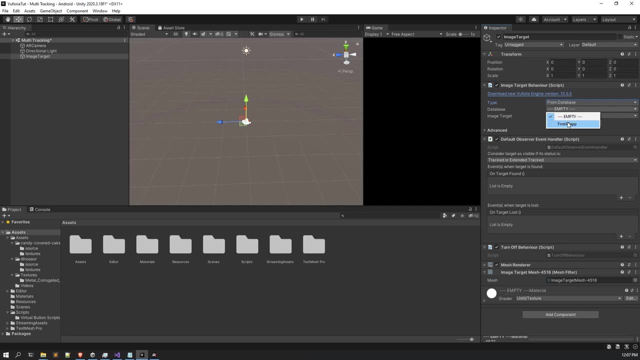 target. all right, select a marker right from here. click uh in the image target behavior, click on from date database and select the database. my day for for my case, the database is first ar app. all right, and the marker i'll be using for this is m1, and let's name the image target as m1, all right? 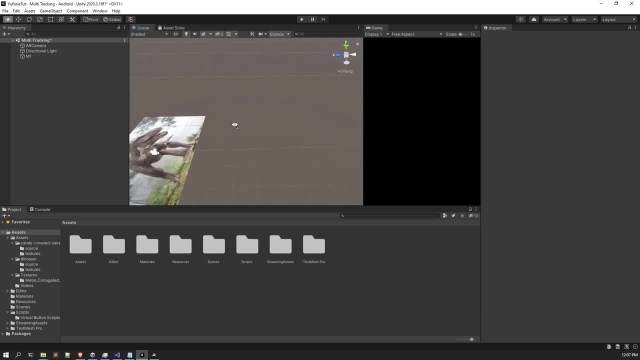 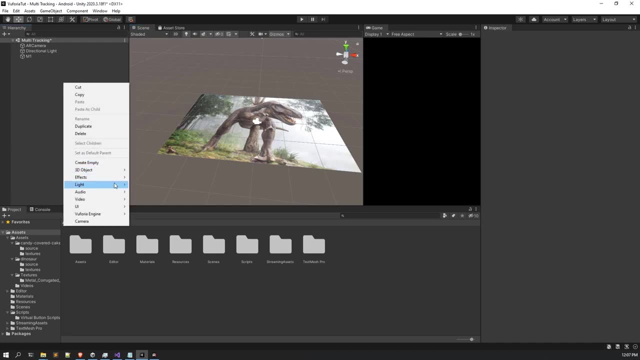 because i'm using, uh, the m1 marker. all right, so yeah, so here we got our very first marker. all right, i would be placing the 3d models later on. first, let's set up our second marker. so, again, right click, click on view for your engine, click on image target. all right, 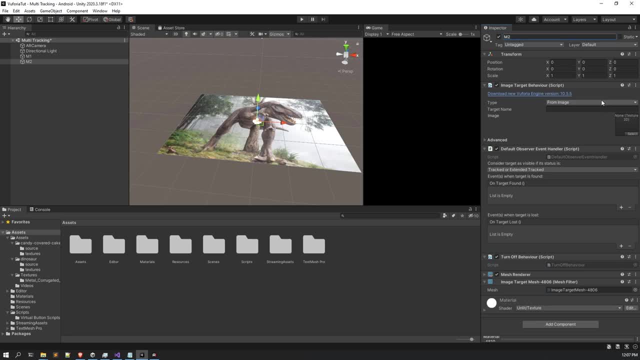 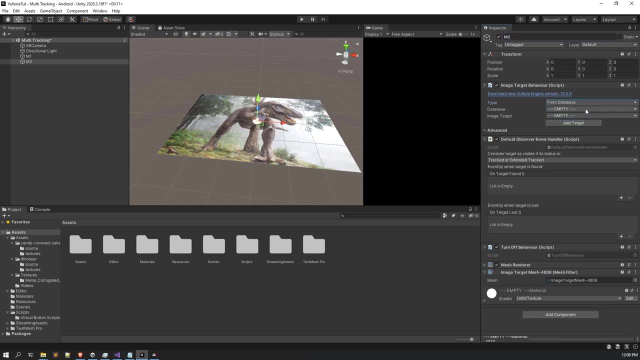 then again name it m2, all right. so then again in the inspector window only you will get uh type. select it from database. then select the database. that is first ar app in my case- and take this m2 marker. that i have all right. so you can uh, you will get the marker, what you have named. 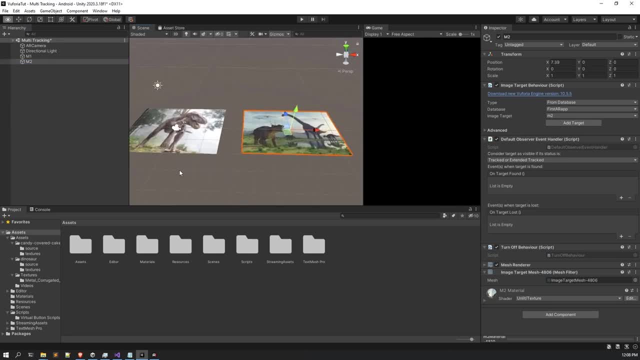 after all right, so make sure you do that. now we have two markers in in place. now the problem with that is: if we, if we try to show one marker, all right. if we try to show one marker at a time, then uh means, uh, let's. let's uh say, for an example: all right, uh, i'm using this app, all right, and now? 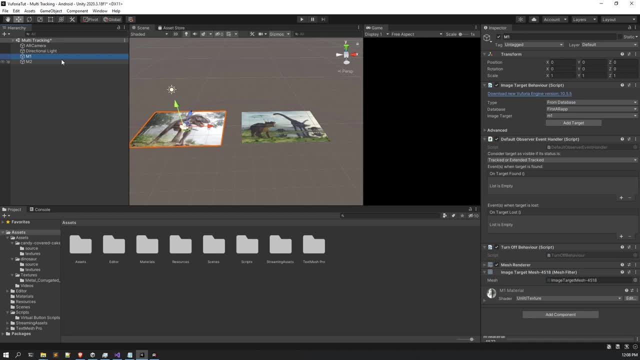 i want to show, uh that total, how many means i i'm trying to uh means, track both the markers at the same time, all right, so i'm trying to do that and uh, of course that wouldn't work, all right. so, to figure out uh this problem, uh, we have a solution, all right. so currently, the problem we are facing 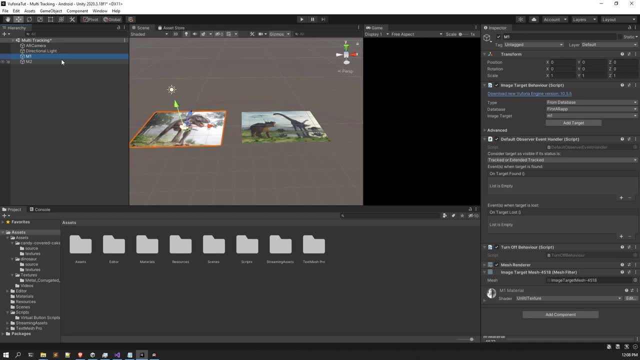 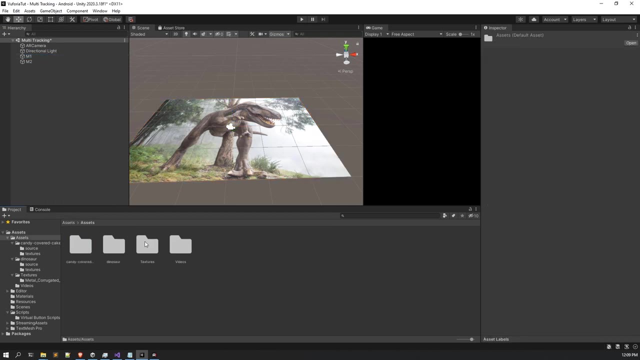 is, uh, it will only track one marker at a time, all right, but we want to track both the markers at a time, all right. so we are going, we are going to go to that feature, but first of all, let's uh set up our 3d models. all right, so, right click and uh, not right click, uh, i, i already have the 3d models all. 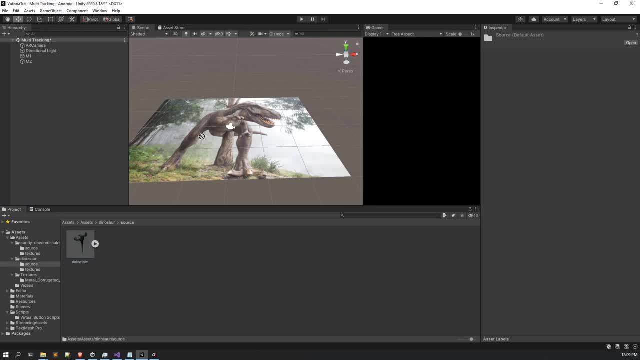 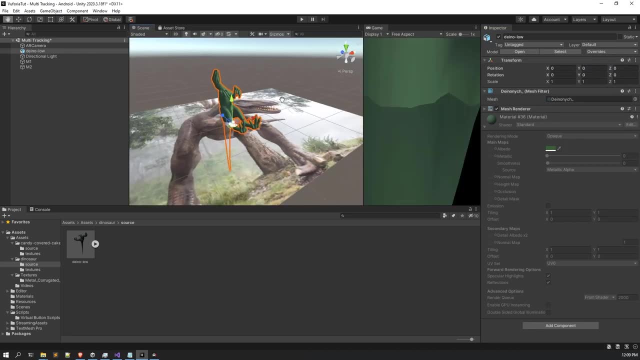 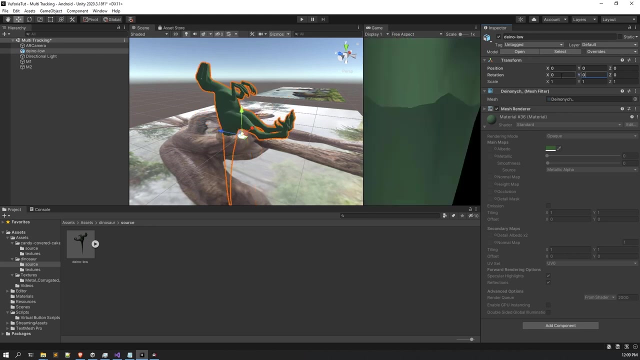 right, i have the. uh, i have one dinosaur 3d model, so i'm just going to import it right in here, all uh, let me reset its uh transform, all right. so here we uh actually got the dinosaur. i know it doesn't look that good, uh, i just uh choose one random from sketchfab. uh, these are objs, uh, and believe me, i 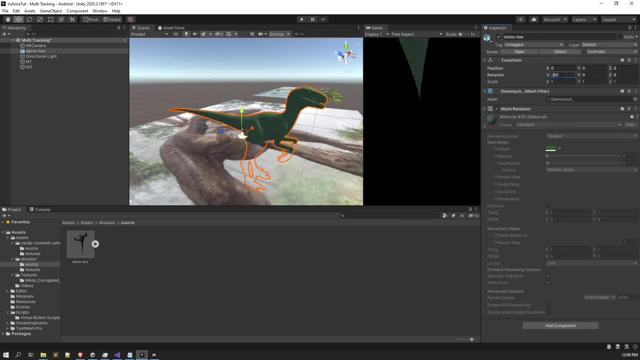 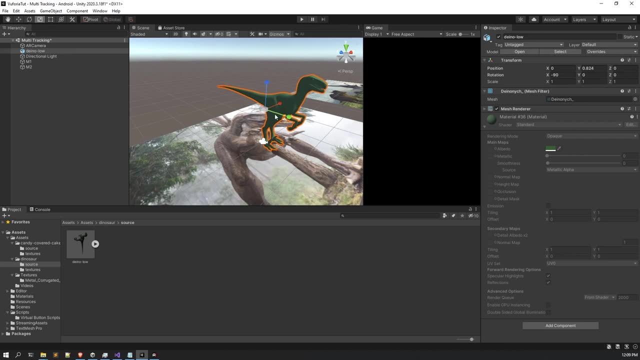 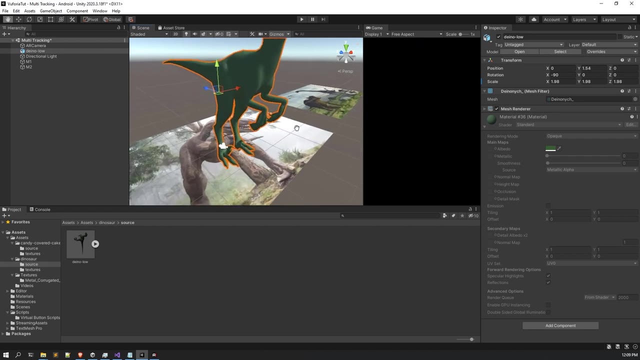 don't uh want you to like use obj files. all right, i i want you to use uh glta files because they have better quality, better texture quality and all those things. all right, uh, that's, that's the major reason. but, uh, for the sake of this tutorial and to make things work first fast, so i go, go, got to go. 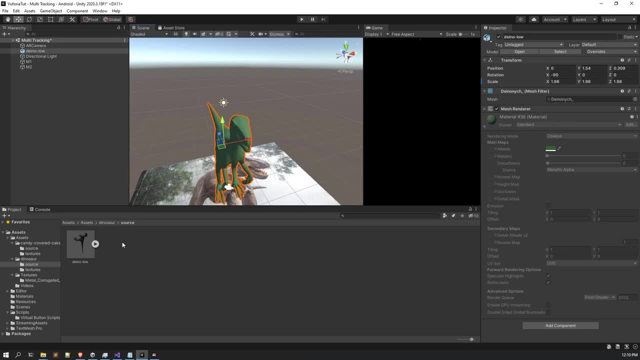 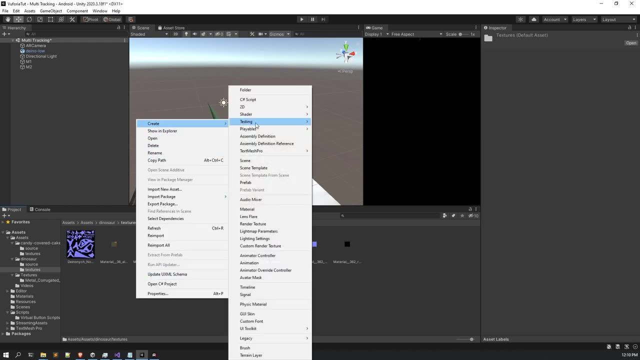 for uh this obj morning. all right, now there are some materials. all right, so i will. i will create the materials. it's uh, it's pretty simple here. you can see there are multiple materials in here, albedo, so what you can do is, uh, right click in the texture section and create a dinosaur material. 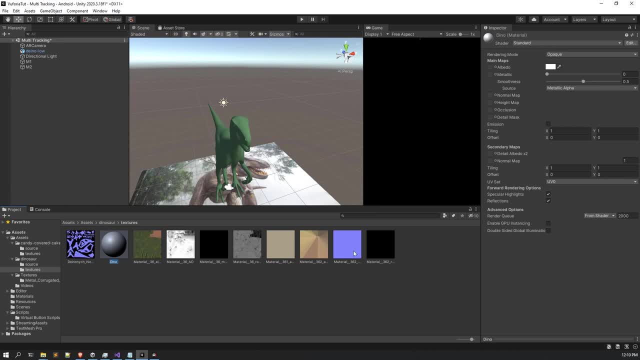 so here i create a dinosaur material. now i try to find where is uh exactly the means? this is the normal map, right? this is uh the albedo one, all right? yeah, so i found the albedo one, drag and drop it in. uh here, all right, and drag this on. 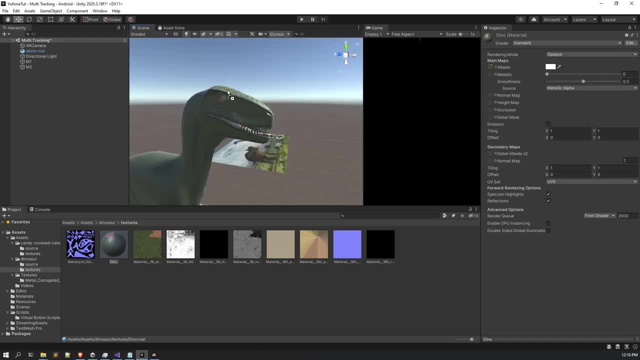 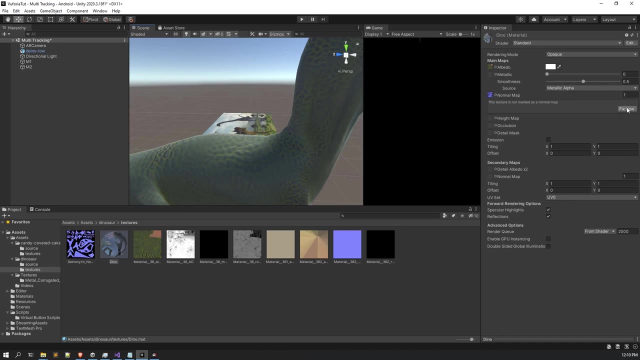 top of this. now, this, this one looks, uh looks pretty good, all right. so now, uh, i need- i also need- to add the normal map so that it uh gives a better look, all right. so, yeah, it's, it's uh looking really, really great. so i uh currently i've click on fixed now because it 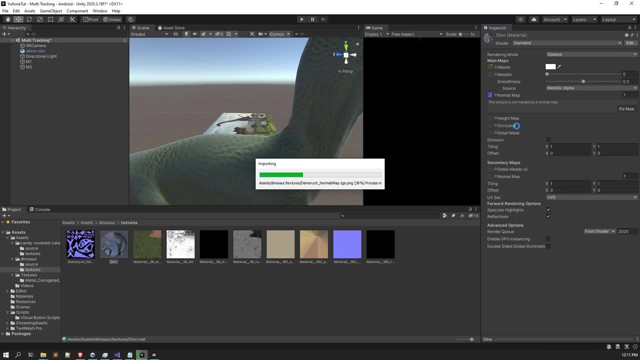 is not being marked as a normal map. so what, uh, what this fixing process would do, is it will uh fix that, uh, uh texture to a normal map. all right, so just just wait for a few seconds and, uh, this process would be done. all right, now, let's, let's see. uh, we have ambient occlusion, we have. 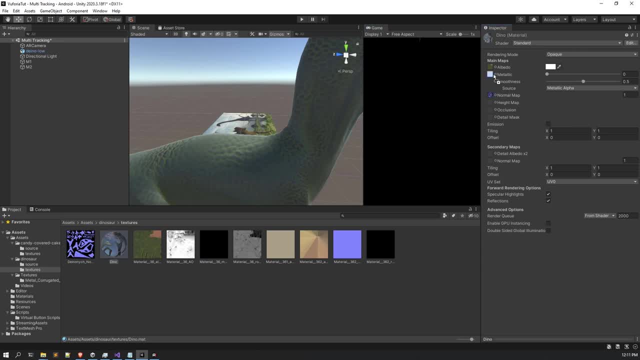 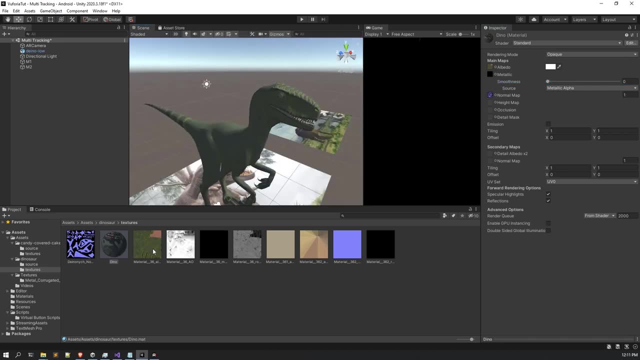 metallic texture. so, uh, let's apply the metallic texture first, all right, so here we got the metallic texture, but uh, actually, let's remove the smoothness, all right. uh, then here we have the roughness, all right, uh, so, and uh, then where is it? yeah, there's another albedo one. 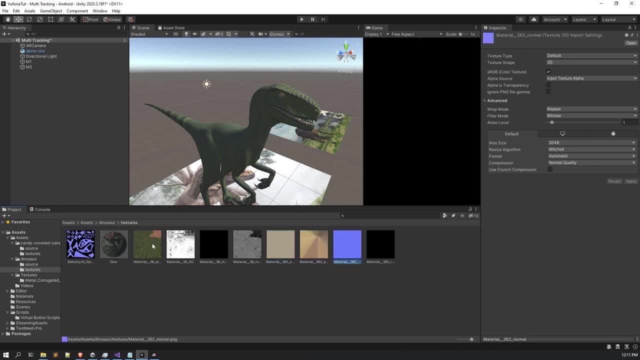 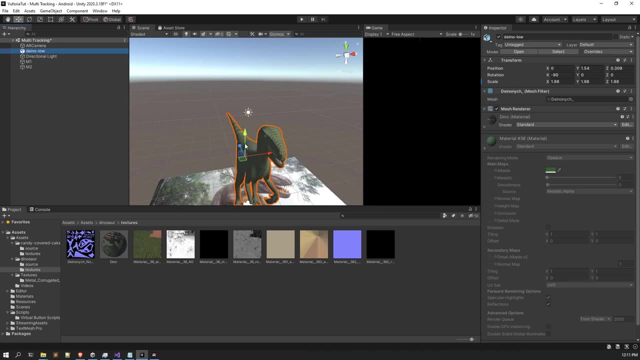 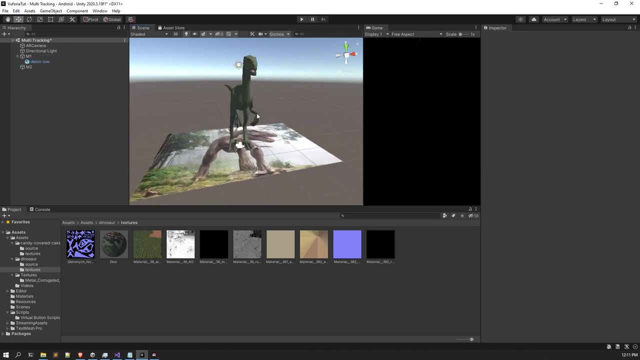 this is, uh, maybe for the eye, so i'm not going to go into that much. so, uh, for now, this this thing looks good, all right, so, just uh, as our model is ready. so what you have to do is, uh, put this model under the hood of m1, that is, make it a game object of m1 marker. all right, so for now, our this, this model. 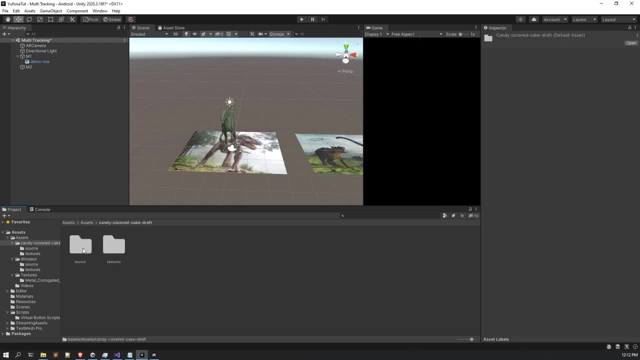 is set up. now, again, we have another uh model, that is of a cake. i uh like i was thinking to take another dinosaur model, but then i thought, let's, let's take a cake. how many dinosaurs would be there? all right, uh. so now i need to bring the scale up, all right, so i'm going to make it 50. 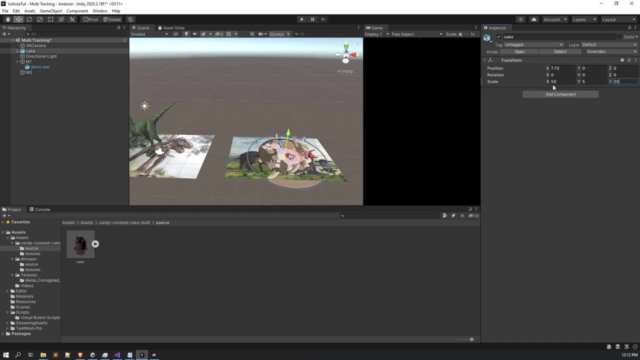 uh 50, sorry 50, and here goes another 50. all right, so this this seems uh pretty big, um, so i would scale it down a bit. so uh, don't worry. okay, this, this, uh, this thing looks good, all right, okay, cool now i wanted to save this. all right, uh, save this and uh simply drag and drop this inside the m2, all right. 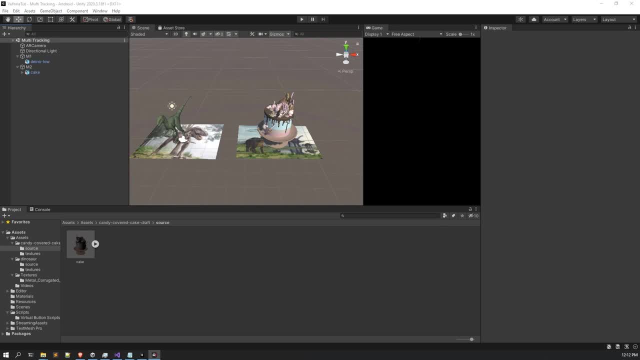 so, yeah, so now, uh, here, uh, one thing we would be seeing is: all right, one problem we'll be seeing is that whenever, all right, whenever we are going to like play, uh, this scene, what would happen is, uh, we only one marker will be detected. all right, if we give, if we feed it two markers, all right, then it will. 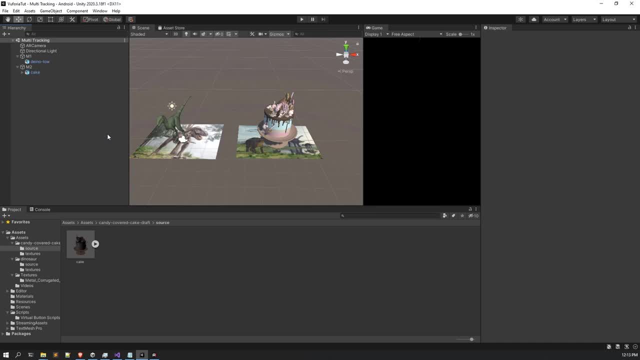 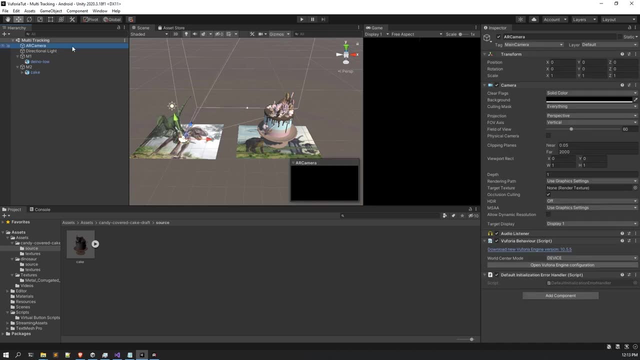 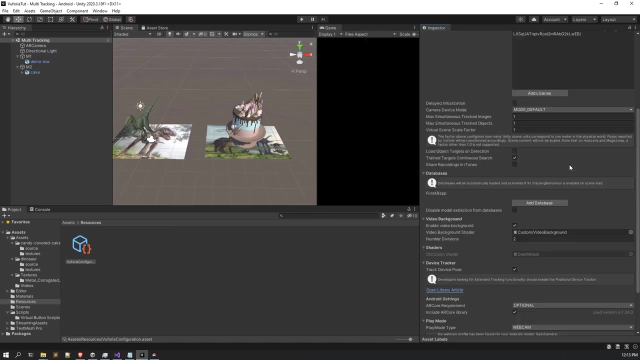 only detect one of it because, uh, we haven't set up the setting that is needed, right, so that's what we have to do. or click on ar camera, all right. then click on open view for your configuration, all right. so here you can see. here are multiple options and the one that would be, uh, our 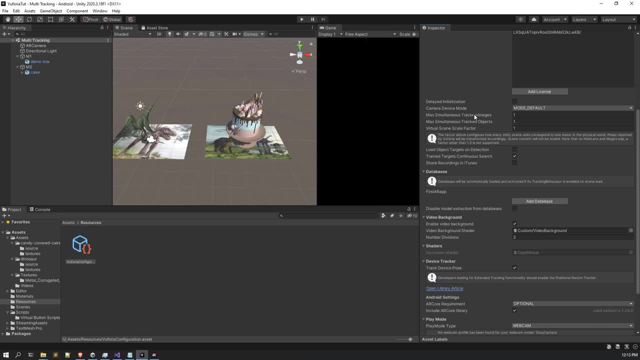 preference is that this one maximum simultaneous tracked images, all right, so, and there's another one maximum simultaneous tracked object. so basically, the the first of all, let me tell you what the this two does basically currently, you can see one is written there, all right, and that means only one marker or only one object would be detected, all right, at a time. so what? 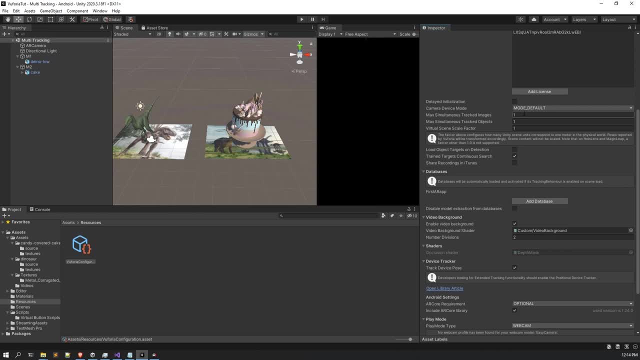 we have to do is, uh, we have to increase it to how many uh like. to home to as many as means as many numbers as we want. all right, like let's say that we can assume that we wanna attack an object free. say, if we want our app to detect four markers at a single time, right, so we can write it four in. 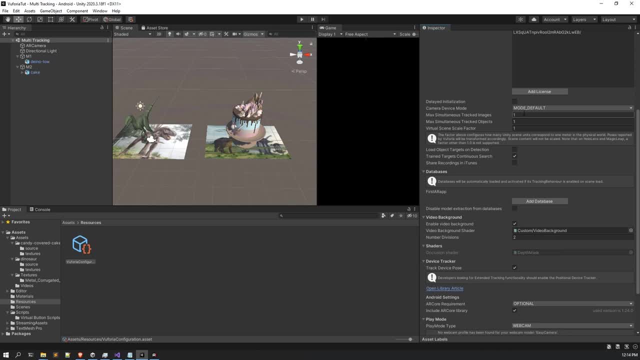 there, all right. or if we want it to track four objects at one time, then we can write uh four in the object section. but for, for, for this course, we are only uh like we aren't uh exploring the tracked objects portion, all right, so we are going to explore the maximum simultaneous track. 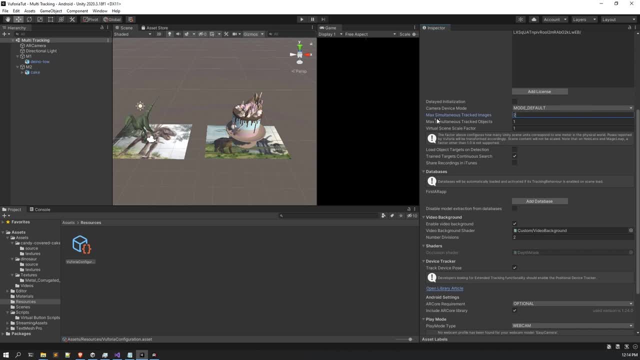 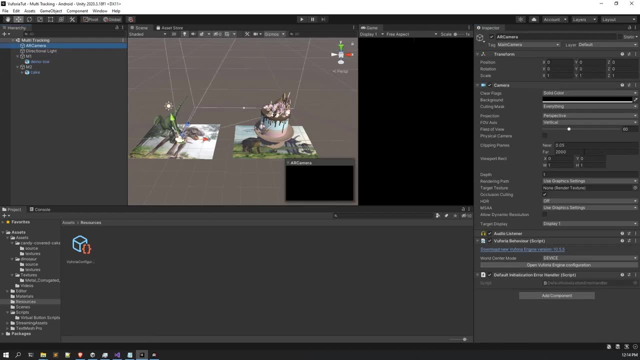 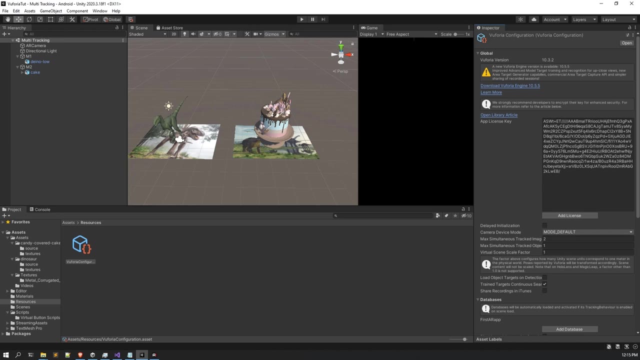 images. so what you can do is calculate is one, just simply change it to two. all right, so that's how it's uh, it's going to work. all right. so it's pretty simple as that. there's nothing much to like, exactly scare about, all right, but yeah, this is uh, this is it right. see, uh, the thing that i. 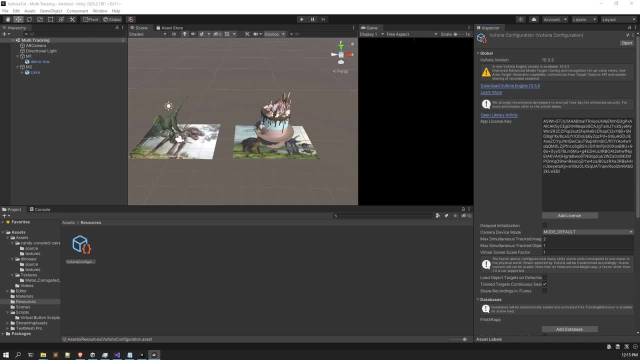 would like to say is whenever, all right. uh, generally, generally, uh, whenever we actually like create ar books. we don't usually, uh, keep mac means, means we don't usually track two to three images at one time. we just track one images at a time. all right, and that's what i would recommend. 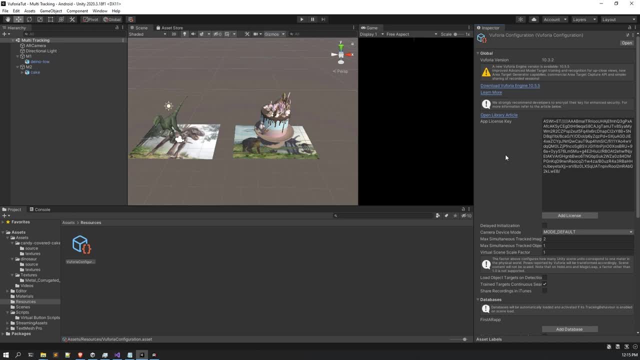 you to track one images at a time, because then that would make it more efficient, all right. or else, uh, the the ui might get cluttery if you, if you don't manage it in that way, all right, and that gets a bit more complicated. so i always recommend people to uh like for. 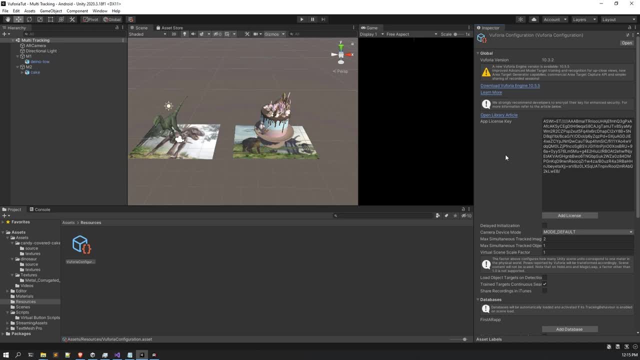 ar books. all right, for specifically ar books. try to use only one marker means set the maximum sample trainers, tracked images to one, because at that point, uh, you guys will want uh to exactly use already, to exactly use one marker at a time, all right, so let me show you. all right, let me show you. 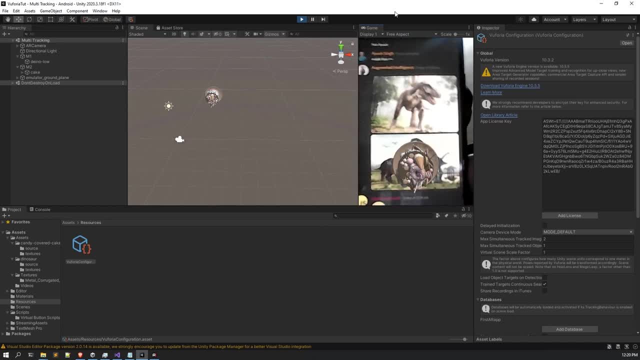 um, just just see this now. all right, so we have uh able to just- uh, yeah, we got it, so we are able to see that uh at at a single time. all right, we are able to detect two markers, all right, so that is what how it works, all right, so i i would recommend. 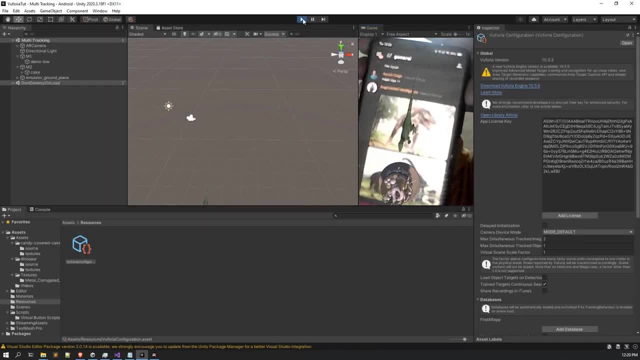 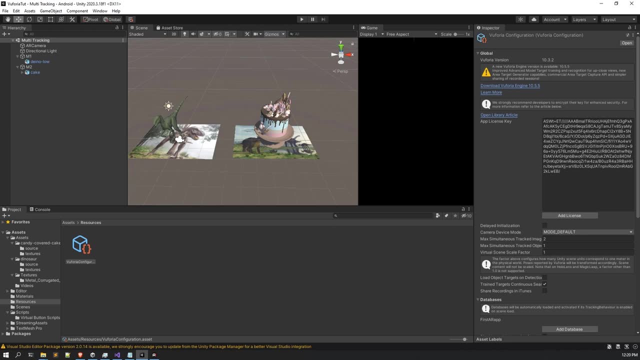 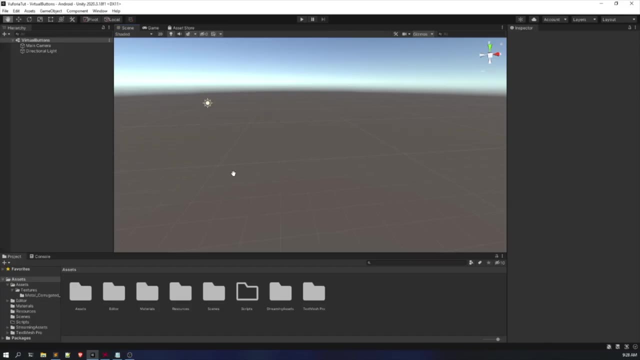 you to try, uh, play with this. this features feature mode, all right, so that, uh, you explore more new things, all right? um, so, yeah, that that's it. so that's it for today's lecture. all right, so see you in the next lecture. thank you. in this particular section of the video, we are going to look into virtual buttons, so virtual. 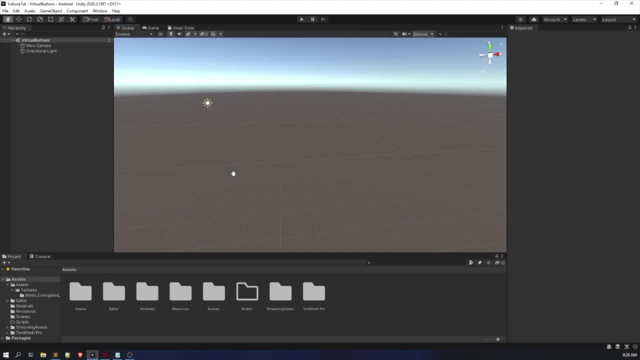 buttons are another way, all right, or another way to add buttons in your view for your application, all right, you. there are two types of buttons that you can add. first of all, ui buttons- all right, like, uh, using simple canvas and those buttons in world space. all right, you can do that. 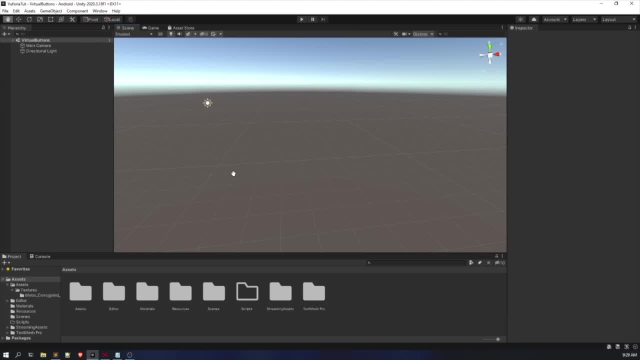 another, uh, another way is, that is, to use virtual buttons. all right, so in this tutorial, we are going to look into the virtual buttons. uh, and before starting- all right, before starting with virtual buttons, there are some rules to be followed. all right, some suggestions, some rules that are needed. 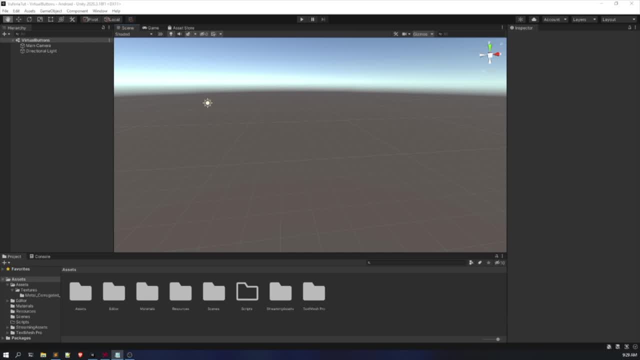 to be followed. the very first thing, all right, the very first thing that should be kept in mind: that the size of the button- all right. the size of the button should be equal or greater than 10- all right- of the overall target area. always remember that the size of the button should be equal or 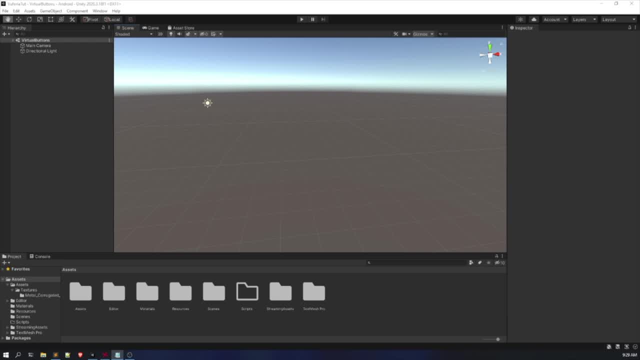 at least. all right, at least 10 percent of the overall target area. all right, now, if the like: if the area is 100, then the 10- uh, the button should be at least the size of 10 of that area. all right, that's it. another thing, all right. another thing. that is always all right, always. 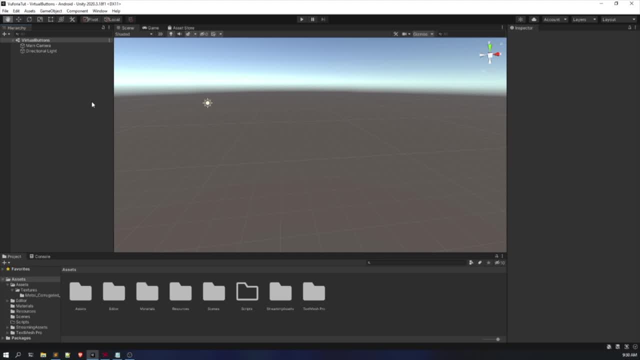 try to place the button. all right, always try to place the button where the place is, where the button is at all right. all right, and also in the introduction video i already showed you how to check for feature points and open the v4d website and look for where the 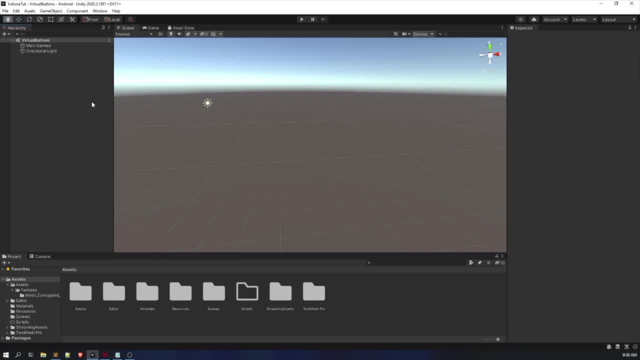 feature point is much greater, all right. where the quantity of feature points is much greater, and always place the button there, all right. another thing is that, uh, insert, insert the buttons, all right. what does that means? that means, uh, is that don't make the buttons touch the image target borders. 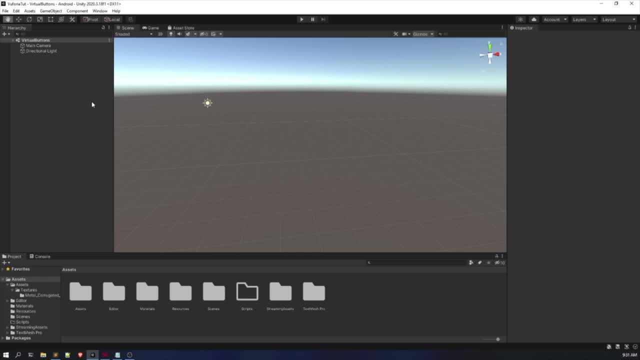 the borders of the image target. so always give some padding in the button from the outer side, margin in the button from the outer side. so always remember that. so always insert the button so that they don't touch the borders of the image target. another and the last point is: don't stack the buttons upon each other. 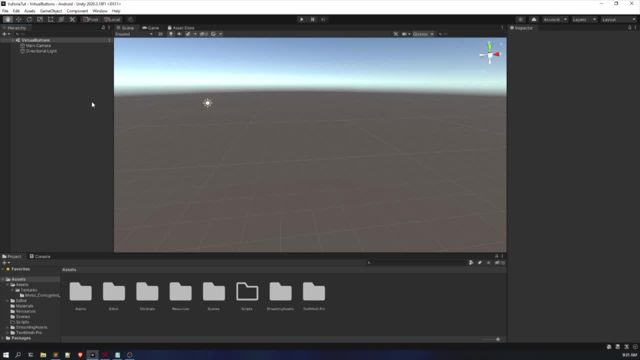 all right. what does that mean? see? when you are viewing, all right. when you are viewing from some point, all right. when you're viewing the image target from a particular point, you would see, all right. you would see that if you place those buttons on top of each other, all right, you won't be able to reach the. 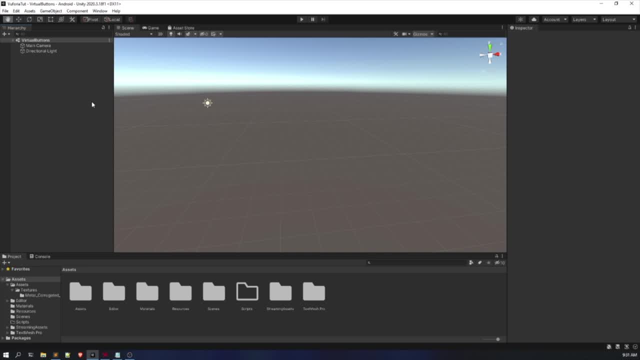 second button. it would be really like it would be really hard to get uh to the second button, so don't ever stack the buttons upon each other. all right, so that's it. so let's start the development of our virtual button. let's implement it, see, uh, i would like to mention is that i'm using the same project. 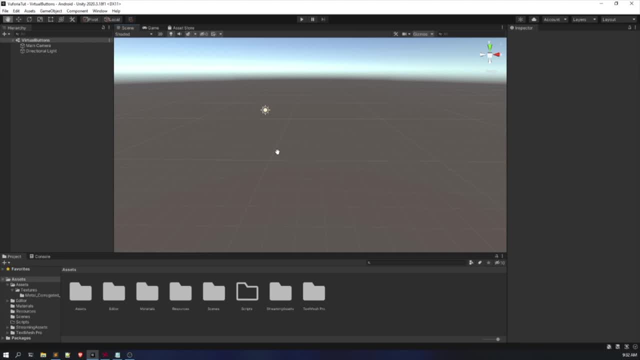 all right, the same previous project that i used to uh develop the work like show you the very initial steps of you can do all right, so i'm using the same project. so i i haven't had changed my license key and my database, although if you want you can do so. all right, it's totally upon you. if you want, you can do. 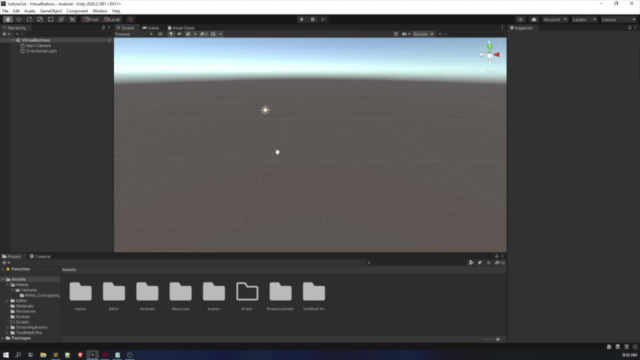 so you can even create a new project for implementing virtual buttons. i am doing this because i want to keep all the source code at one place and provide- uh, provide- it to you all right, so it won't be cluttered up. so yeah, let's get started the very first. 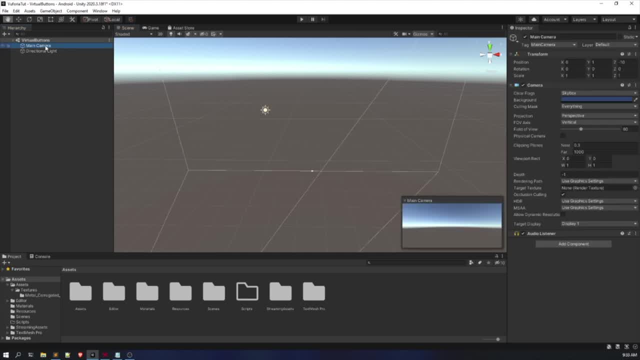 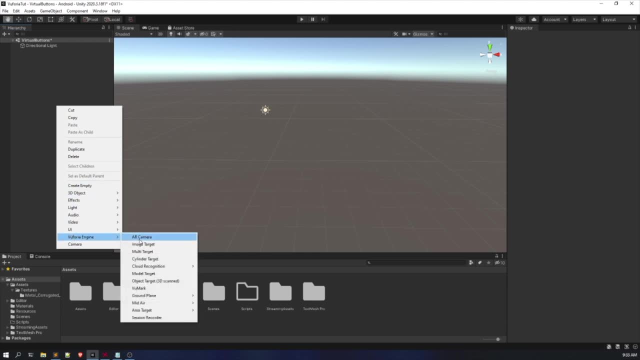 thing all right. the very first thing is you have to delete the main camera and then add a ar camera. so select viewphoria engine and click on ar camera. so, uh, let me uh place it on top of the directional light. uh, don't worry, it won't have any sort of 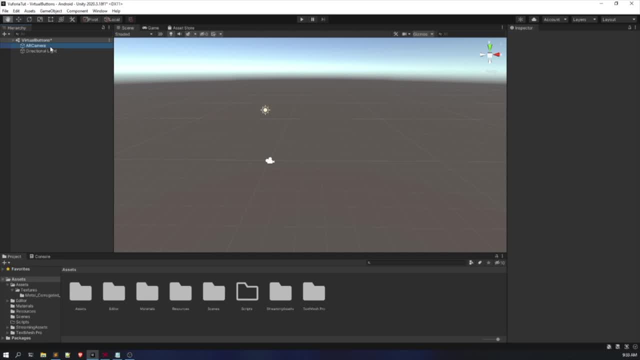 effect. so it is totally upon me now i have placed my ar camera. another thing is to add the image target. now the image target would be same as the previous one, because i haven't changed my image target. but you can do so if you want. all right now, if i click on image target, 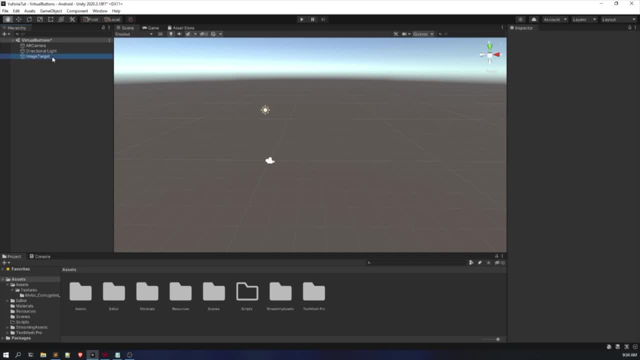 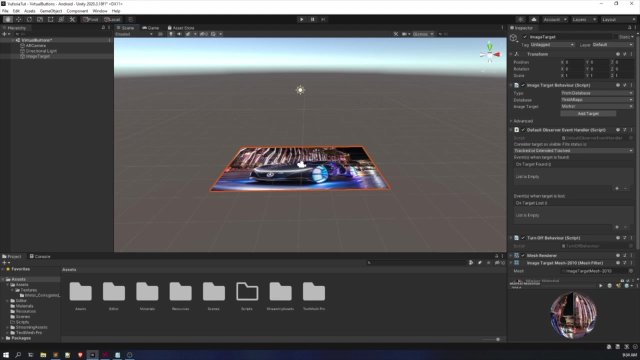 here i get my image target. now let me, uh, select the database. so i'm going to select from database and now i'm going to select the database. that is first, ar. here is the marker, that is selected. all right, now what i want? what i want is to create a 3d cube, all. 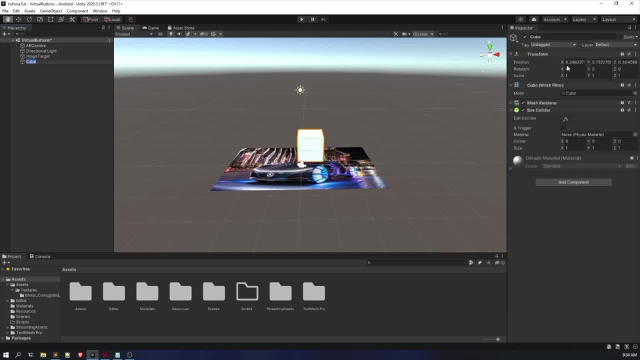 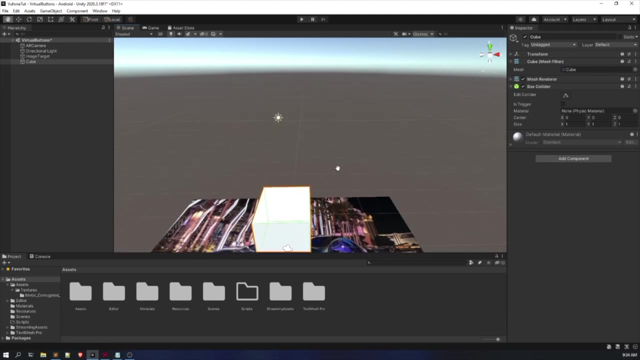 right, i would show you why. just wait for a moment, for a second. let me reset the transform of it. so, as i've reset at the transform, i'm going to uh place it, uh at the back. all right, i'm going to place it at the back. 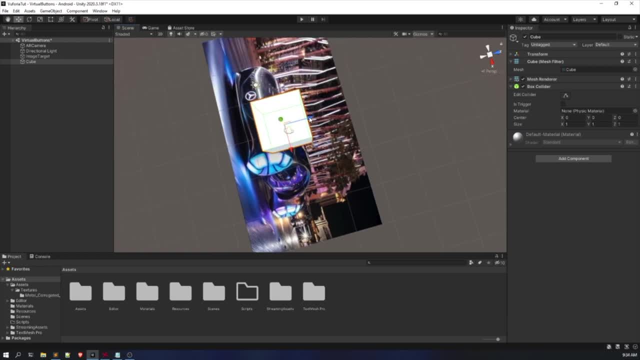 uh. so see, i'm using shortcut keys q, w, e, all right, q for uh, the this hand tool, uh, w for this uh anchor tool and e for the rotational tool and r for the scale tool. all right, so these are some shortcuts. so, uh, i'm using those shortcuts, all right, if you think, how am i getting this? 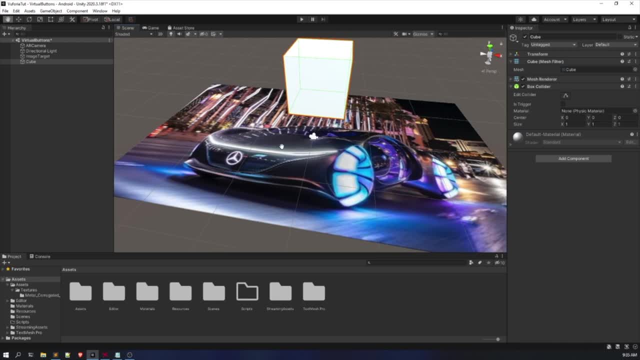 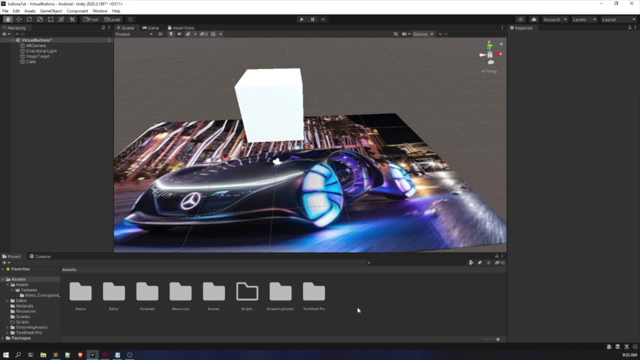 then, yeah, that's how i'm getting it now. uh, this cube looks a bit dull right, like it doesn't have any sort of color. that's totally white, and i don't like it, so let's create a material for it all right now. uh, in this i'm also going to show you how. 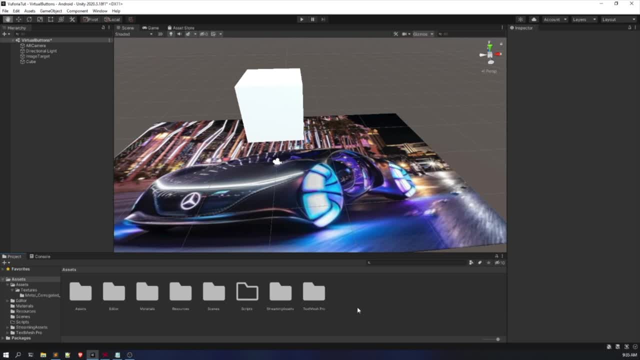 to add textures to your material. all right, and i have already imported a texture i have downloaded, downloaded from 3d texturesme. all right, the links are given in the ar resources file. you can check them out. all right, it is available on my website. now let me show you the 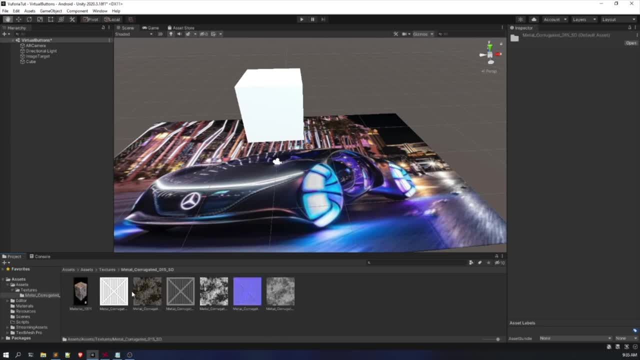 textures. here are the textures, all right, and i'm going to tell you how to implement it. now, this is not a texture, this is just an overview file so you can check how this, how the cube, will look. but i'm directly going to implement it, all right. so, first of all, delete this. 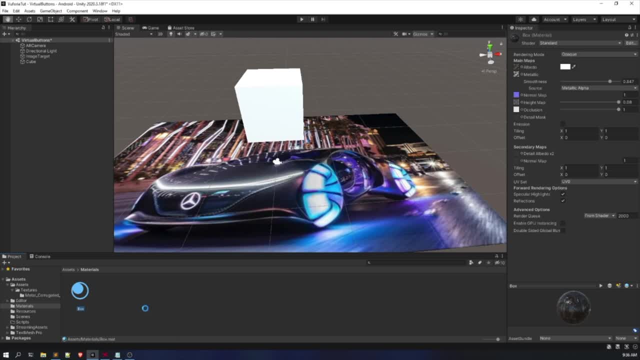 uh, delete this particular material, we don't need it. all right. so, and another thing, all right. another thing is that, first of all, create a material. all right, create a material. let's name it textured, textured box, or let's say cube. all right, this is what i will name it. 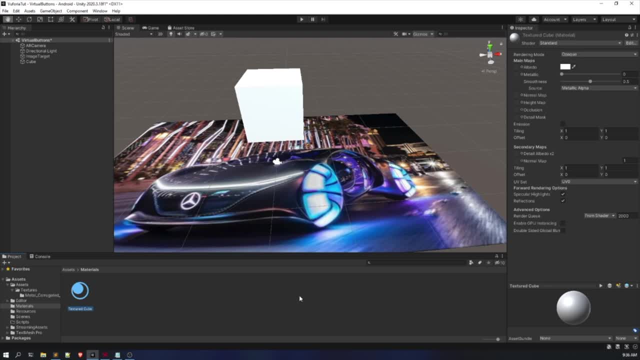 after that, what i want you is to go to the inspector panel. all right, go to the inspector panel and select the textures you want. so what i will simply do is i will click on albedo. it would pop up a panel. now i have to find. all right, i have to find a texture i want. 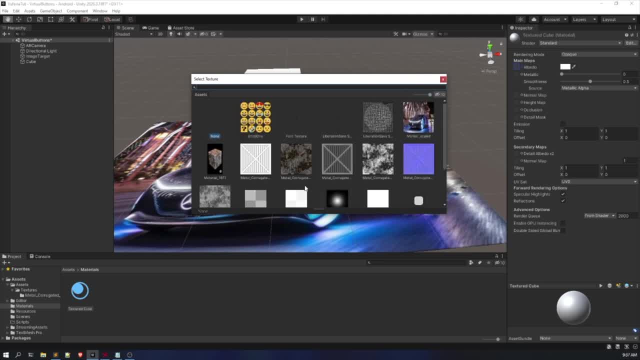 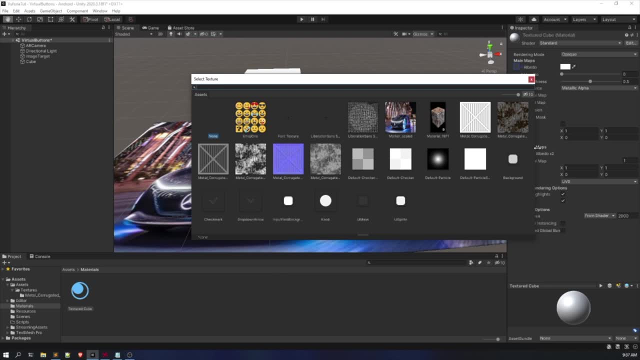 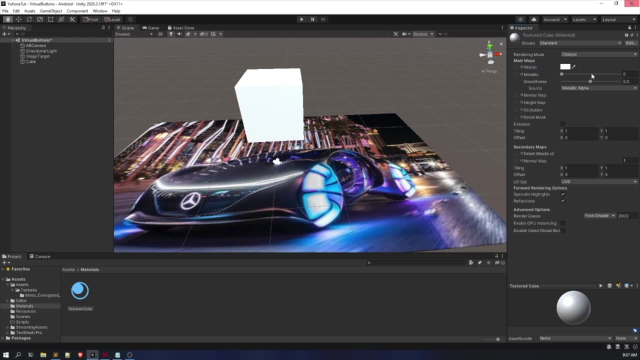 texture. now i'll find a texture that that has been named as baseline. all right, so it's not showing the full name. just wait, let me lock it cool. now from here i can find the what textures I want. So for the very first thing in here, I have to get a base colored texture. 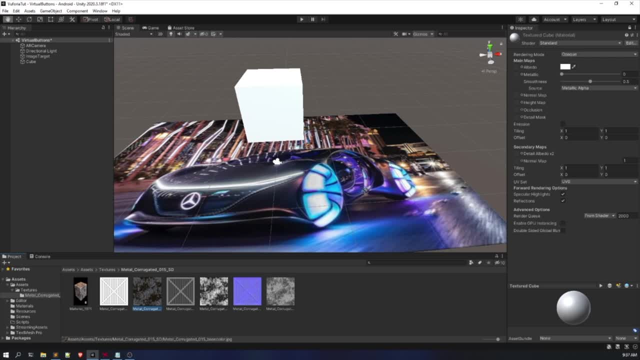 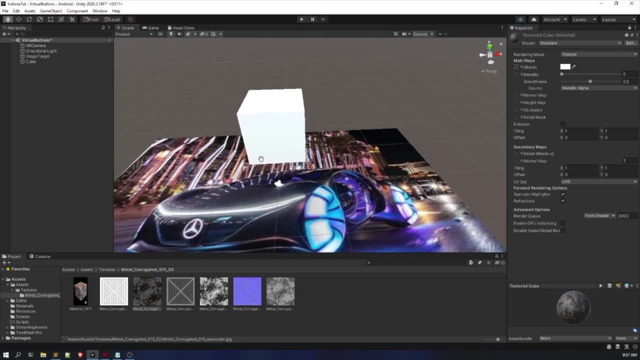 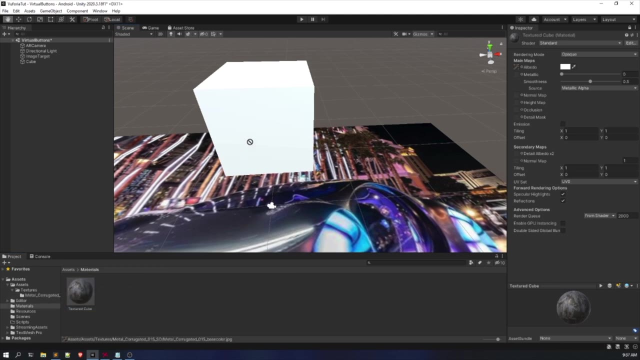 All right, This one, this is. I'm going to put this in the albedo section. All right, Now you might not see the effects in here. All right, You might not see that because we haven't applied the materials. So just drag and drop the material in here and see it has been applied in. 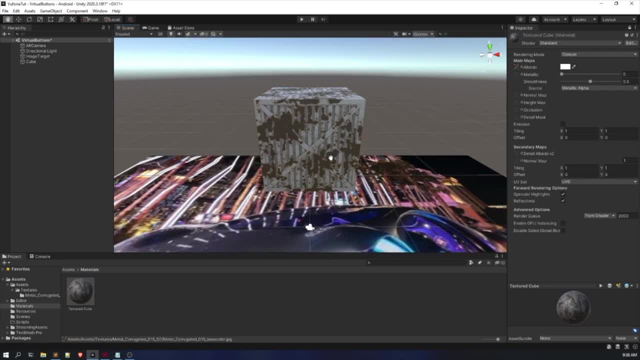 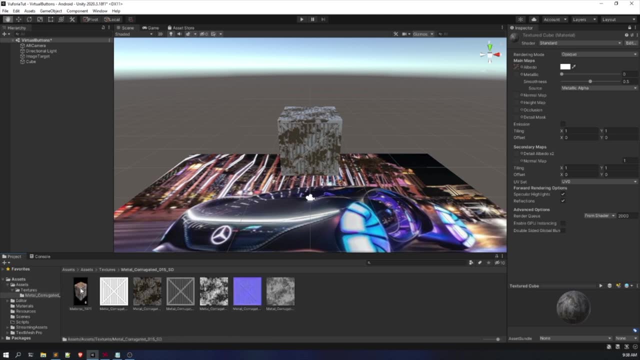 the cube I know it has. the texture has been applied, but it doesn't look good. But you won't say this after watching the whole material applying thing. All right Now. and here's, there is another section that is metallic. Now let's find a metallic texture. So here I got. 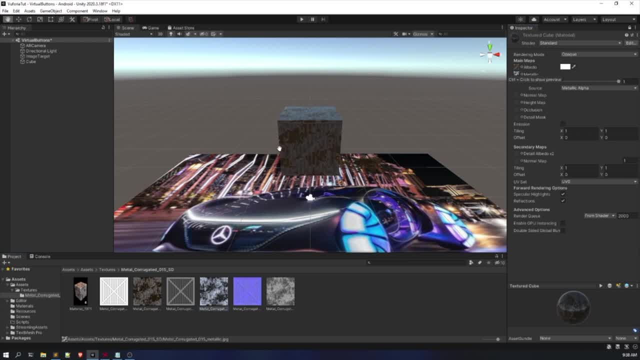 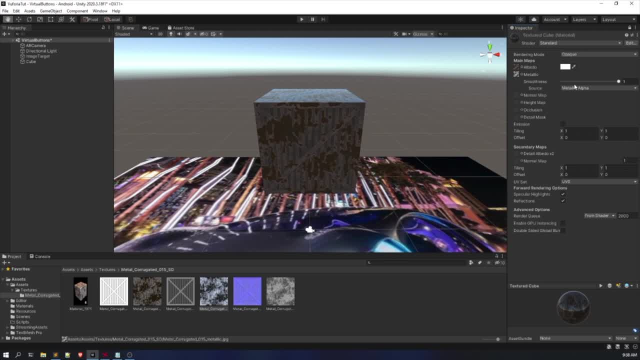 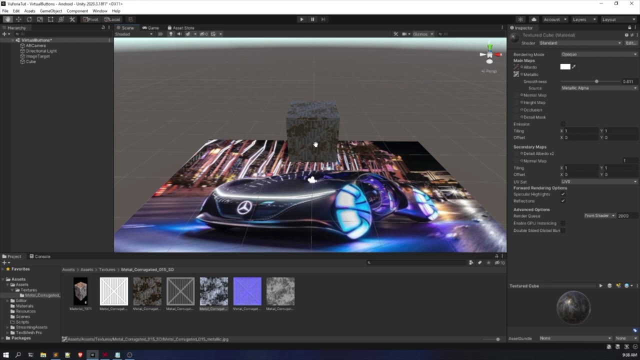 written in the end of the names. Now I would adjust the settings a bit. All right, I would adjust the settings a bit. See, you won't like. you won't like it as of now. The reason is I haven't applied other materials. That's why. that's why it's not looking realistic or good. 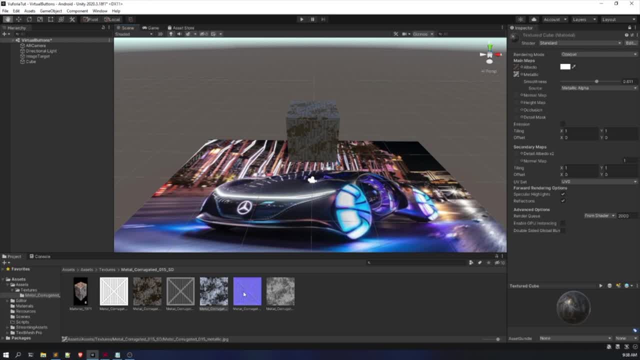 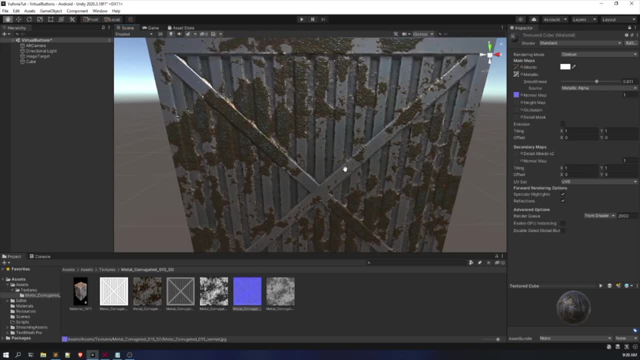 So I'm going to apply those Now. here I have to add a normal map. This is a normal map, So I'm going to apply the normal map And here you can see that, uh, the beds- All right, Here you can see the beds in here are are coming to show up, All right. 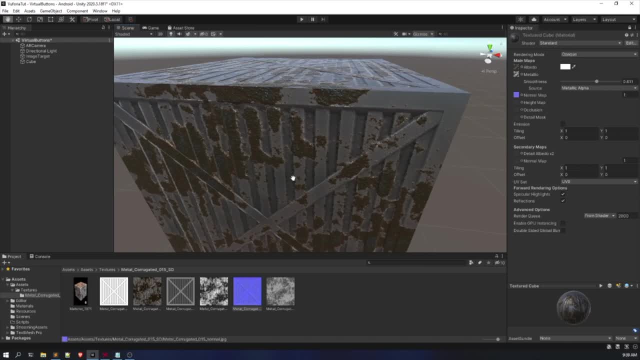 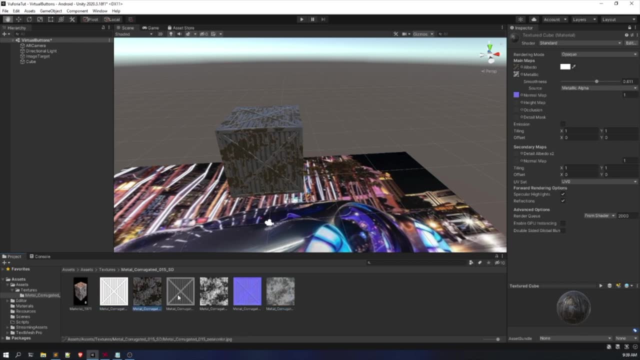 They are putting the 3d aspect in here. You can see it. right now We have to add another thing, that is, a height map. All right, So let me find the height map. Okay, Yeah, Now I have applied the height map, and this, uh, this height map will help me to adjust the height of the like height. 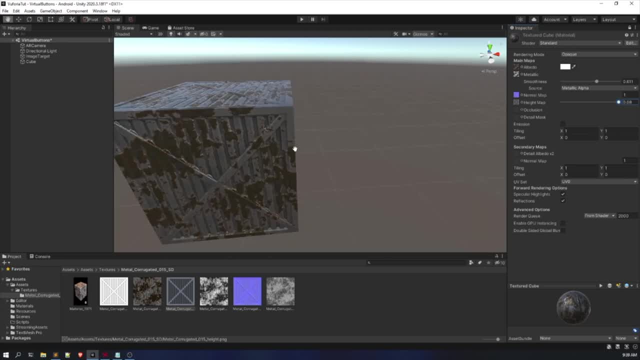 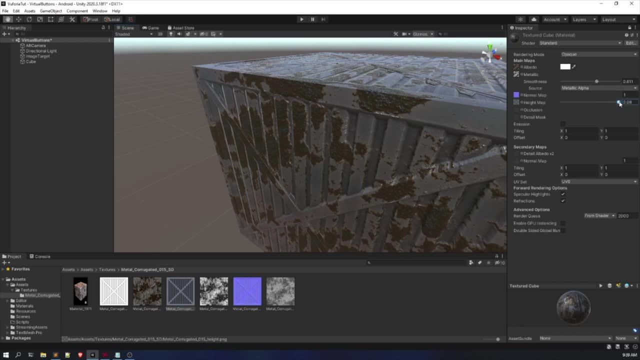 of these uh particular things Right, You can, uh, let me show you from like, from, uh, from nearly All right. So here you can see that it is moving right. It is moving Right. So that's uh, that is what high. 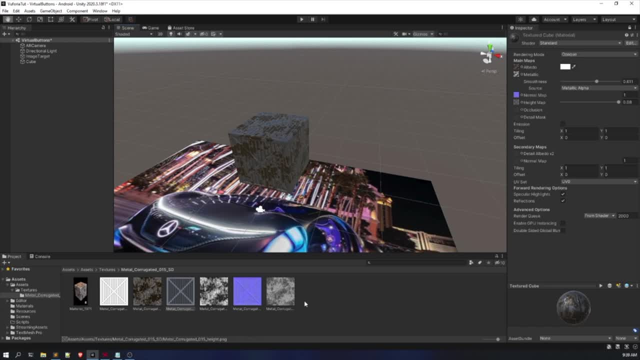 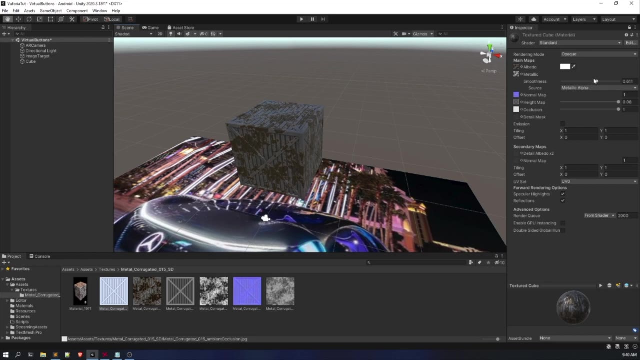 height map does. Now another thing? all right. Another thing is that we have to add an occlusion. Now, this is the ambient occlusion. All right, This is the ambient occlusion mask. So now you can see that, the occlusion mask. Now, if you want to increase the smoothness, you can do so, but I am not. 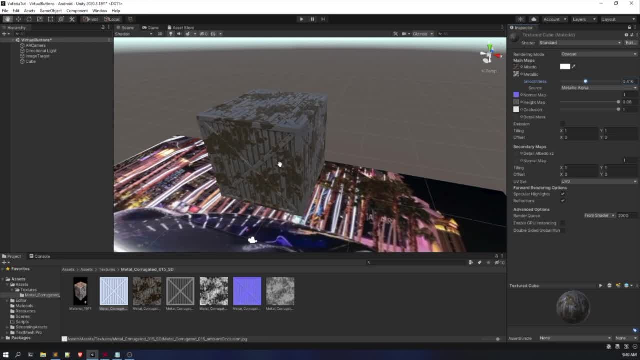 liking the smoothness that much, So it should be something like this: All right, Now let's see. anything is left. Um, roughness, No, Um. all right, Let's see. Okay As of now, all right For us. 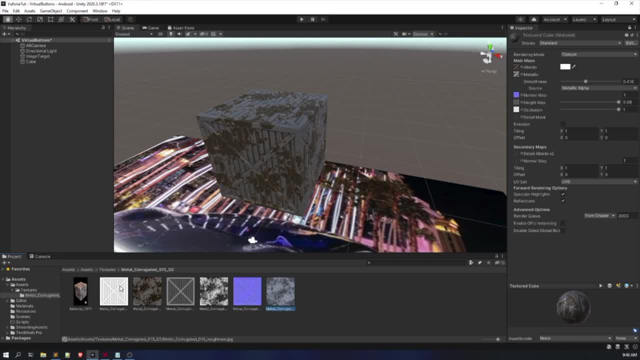 it's: uh, we are good with this cube. All right, This looks realistic too. Now you can get all the textures. All right, There are, uh, really good textures available at 3d texturesme. I would really suggest to go in there and check out the. 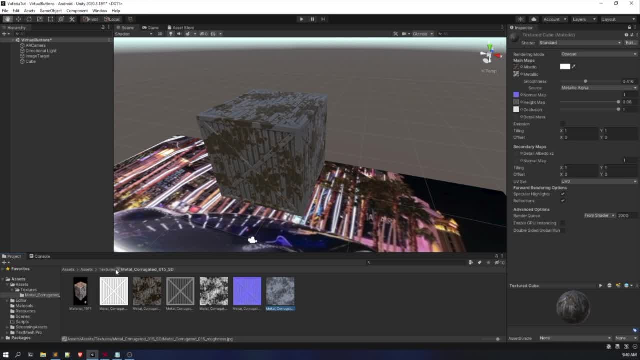 textures. All right, And take the textures that you like. as simple as that, All right. Now another thing: all right, Yes, And the thing is we have to put this cube All right. We have to make this cube a child of image target. All right. We have to make this cube a child of image target. Now click. 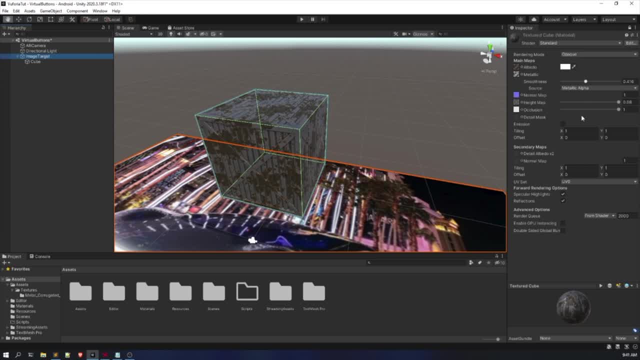 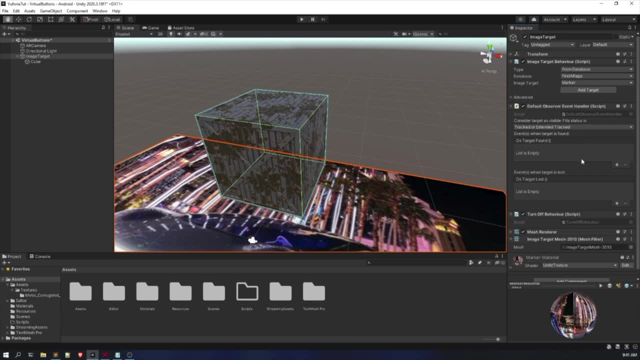 on image target. All right. And another thing that you may. you might see that, uh, the inspector panel is not changing. That's not any sort of bugs, It is basically I have locked the inspector panel, Now I have unlocked it, So I've got all the things All right Now in the image target. 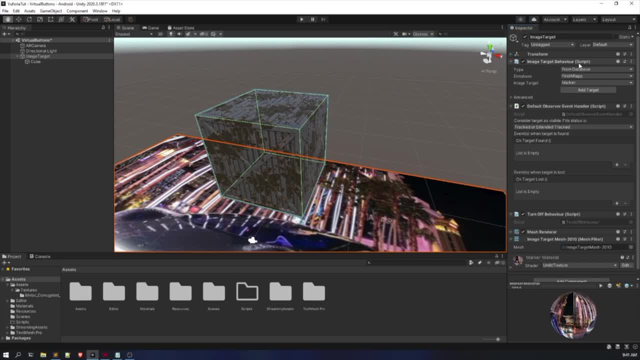 uh, in the image target behavior script under the add target button, you would find something, a dropdown that is advanced. All right, You need not to look into these um properties, but for us the very important thing is this: 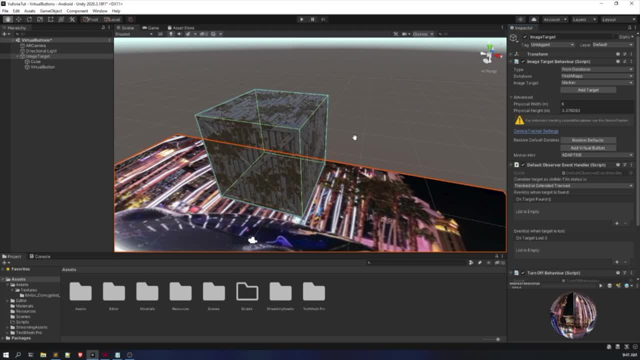 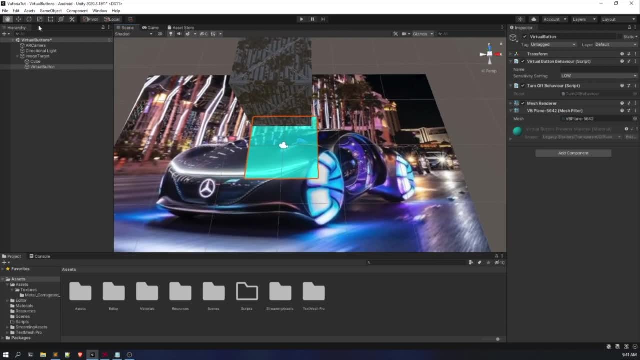 particular button: add virtual button. So click on it. All right, And you can see that it has added a virtual button. Now, if you click on it, the virtual button will be visible to you. All right Now remember the rules, All right. 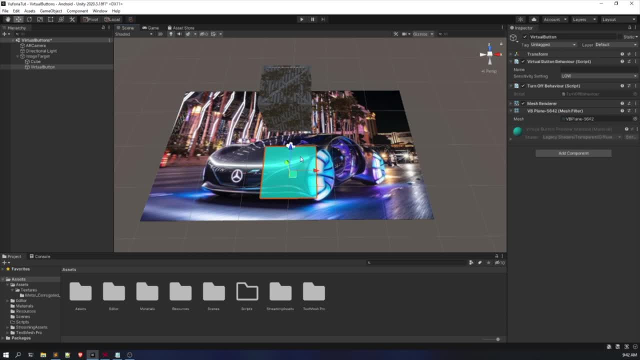 Remember the rules and try to resize it. All right, Now, I'm not sure, All right, And I haven't seen where, uh, where, are the feature points, but I'm, uh, what I'm doing is I'm putting at a 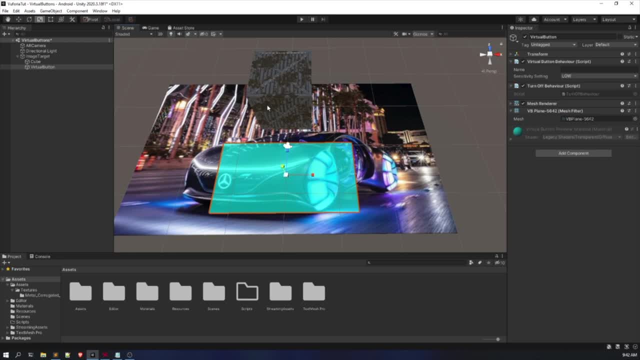 particular place and I'm trying to follow all the instruction, All right, So I would suggest you to follow the instructions too. All right, So we created our virtual button. Now, what See? when you click your virtual button in the inspector panel, you would get some options. 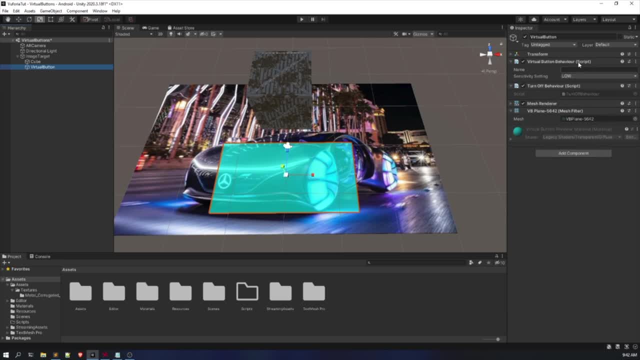 All right, You will get some options. Now the very, the very important thing that we have to see is the virtual button behavior script. All right, In here here's an option: sensitivity setting. That is a dropdown, All right, So in the drop menu you would find high, medium, low. 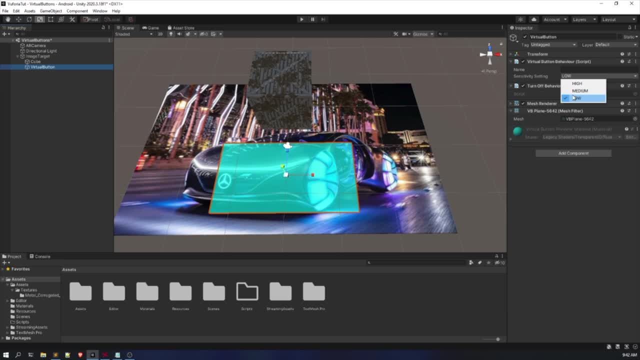 Now, these are the sensitivity settings. What this tells, what this tells us, is that how often? or you can say, um, how exactly are we going to uh like when we uh place, uh, place our hand uh upon, uh, sorry over the particular mark? 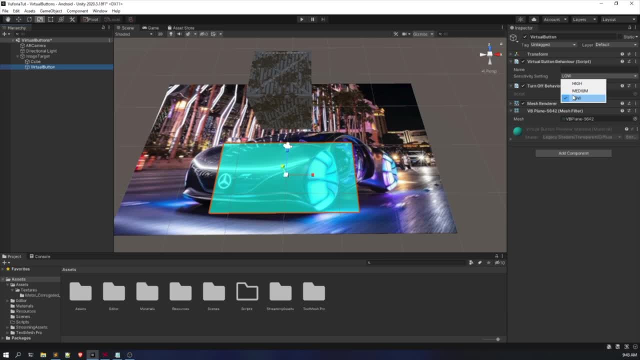 over the particular virtual button, All right. So how? what will be the sensitivity? All right. Or what will be, uh, the rate? All right. When it will like, detect, all right, it would detect and start doing the function. So that's what sensitivity. 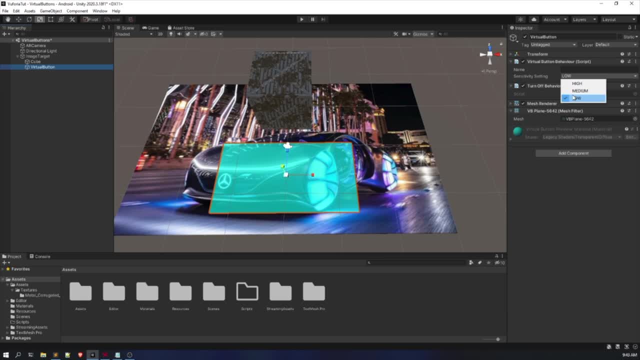 means It tells that how sensitive the particular button is. All right If. if it is low, then it might uh, like it might take some sort of uh hard work to get the button to work. but if it is high then it won't take that much hard work to make the button work. All right, So yeah, Now 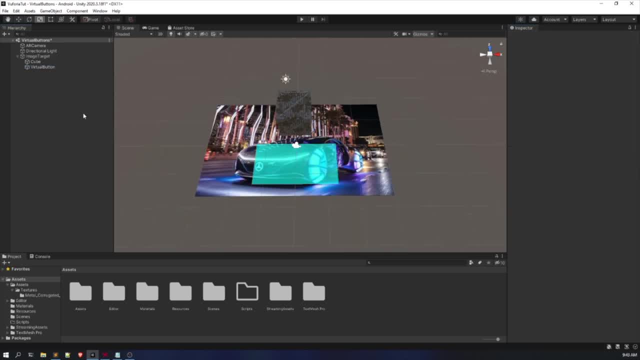 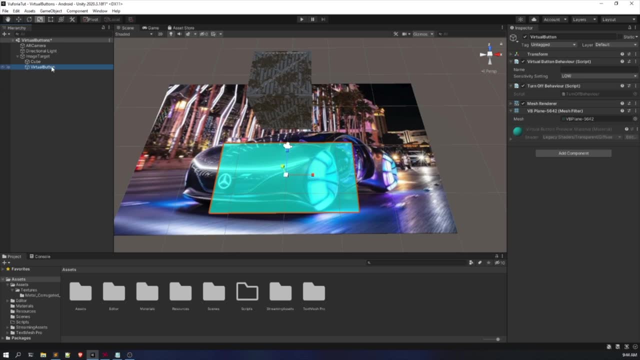 um, now, as we have created our virtual button, all right, we also have to add some functionalities to it. right Now, I'm going to, uh, create a script. All right, Let me tell you first which script I'm going to create on it. 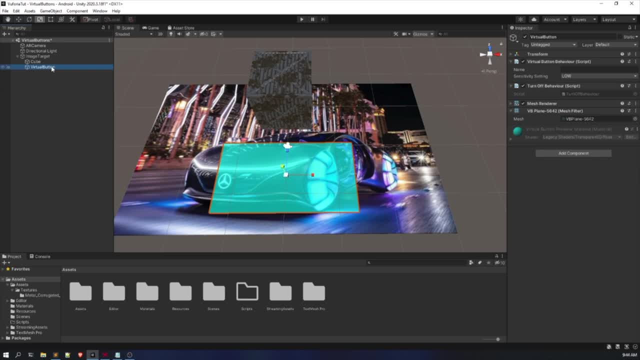 I'm going to create a script that is, that will simply: um, when you hover, all right. when you hover over the virtual button, all right, whenever you hover over the virtual button, what it will do is it will simply disable the cube, or let's say, uh, hide the cube. 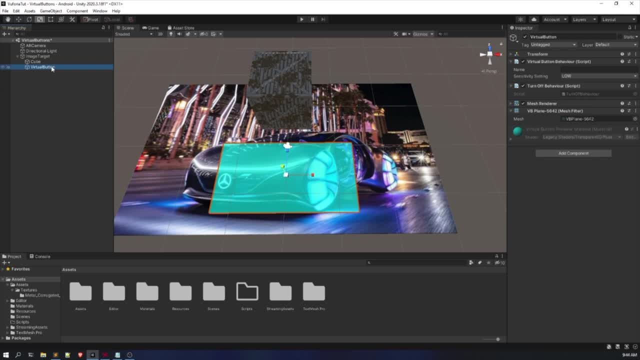 All right, As simple as that, Nothing too complicated, All right. So yeah, let's start coding Now. see, uh, as you can see, I have created uh multiple folders in here, and I would suggest uh: 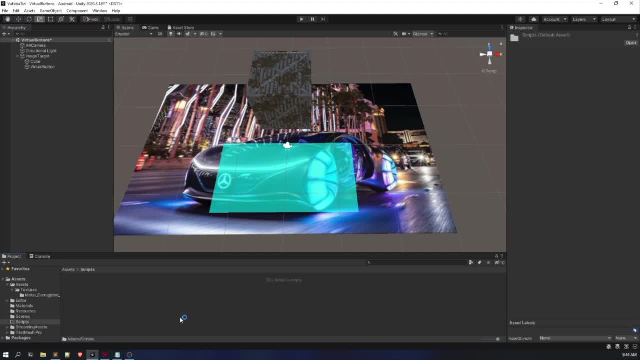 you should also create, because that would help you to structure your projects. Now I would create another folder in here that is: uh watch, uh virtual button Scripts. All right, Now I would uh create different types of folders for different types. 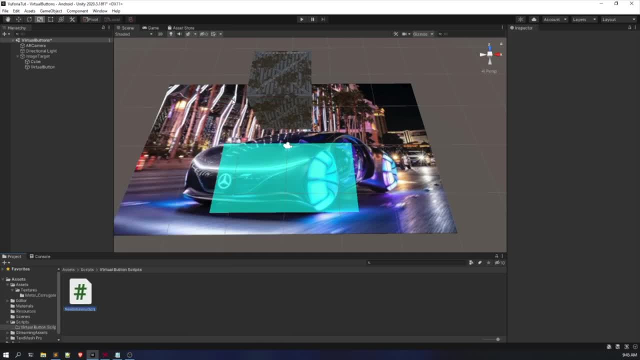 of tutorials. All right, Now in here, create a C-sharp script and I'm going to name it virtual button. All right, Or let's say virtual button, or let's say button behavior, something like this behavior. So it would take some amount. 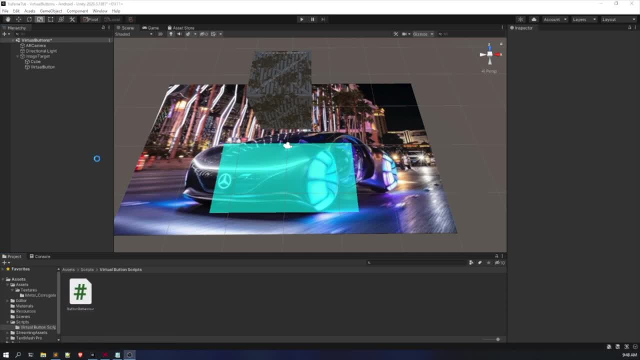 some amount of time to create the script. So now we have created our virtual button behavior script, right now It's our time to code it. All right, And you already know that what we are going to code, All right. So the very first thing, 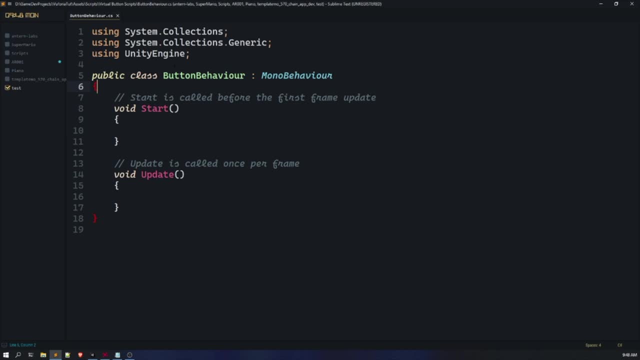 the very first thing is we have to somehow target the cube, and all right. And before that, all right, And before that, we also have to, uh, use a namespace. All right, We also have to use a namespace called view four. Yeah, All right, It's very important to make the virtual button script, virtual button functions, to work, All right. So, yeah, So I remove the comments and make sure that the void start function is there, All right, And if you have forgot what this void start function does, don't worry, I'm going to re-explain it. 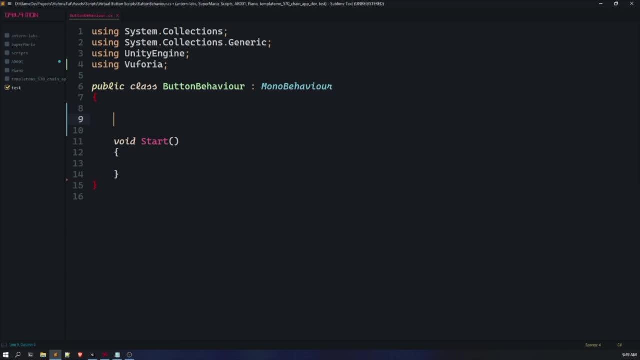 All right, The very first thing all right was to include the namespace view four. Yeah, Now, uh, to like edit the cube, all right, Or do something with the cube. We somehow have to uh grab or, let's say, get the reference to the queue right. We have to somehow store that cube somewhere to be edited Right. So how do we do that? It's fairly simple. We have to create a variable that is public. 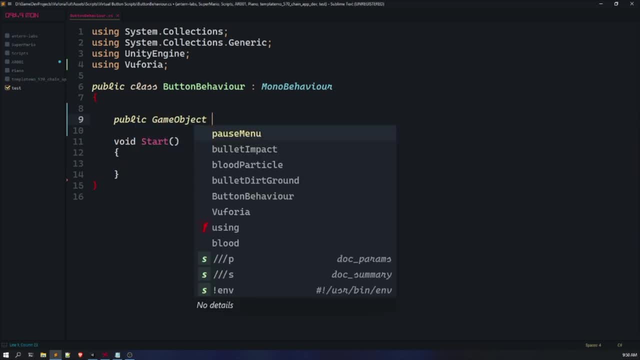 Let me show you, As it is a game object, so the data type. I'm keeping his game object. guys, It's finally the shape we want it. All right, Then, cube. Now one thing you should note: all right, If you, if you don't give public or give private. 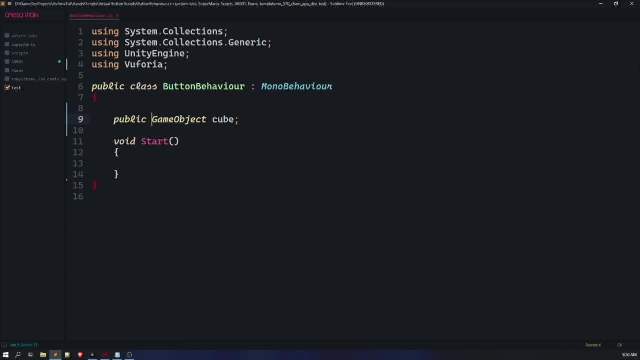 what will happen is: this particular field won't be showed. It won't be shown in the. If I had to show you, just wait, all right, Let me show you. I have created this, uh, particular game object. all right, and let me show you this. 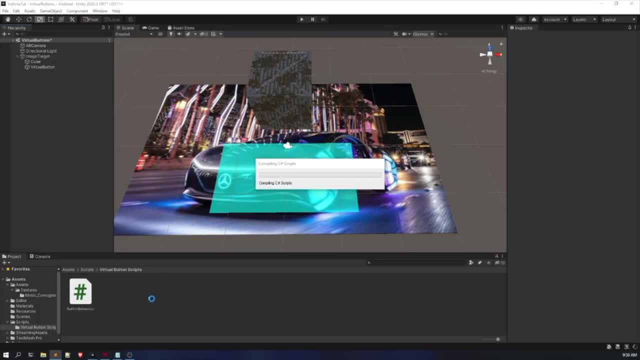 let me show you in: uh, let let the script compile. all right, let the script compile and i will show you that. what will happen if you don't give public? all right? now? see there, there are two ways to reference a variable. all right, i'll be showing you two ways. 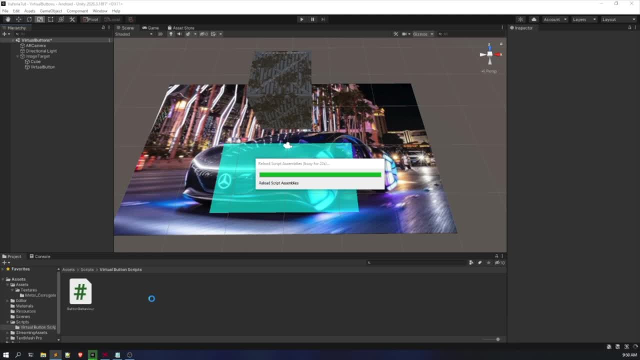 both the ways actually like: the simple drag and drop reference referencing way and another that is using the script to reference. all right, so yeah, now let's attach the cube to our image target. all right, you can create another empty game object and attach it in there, but 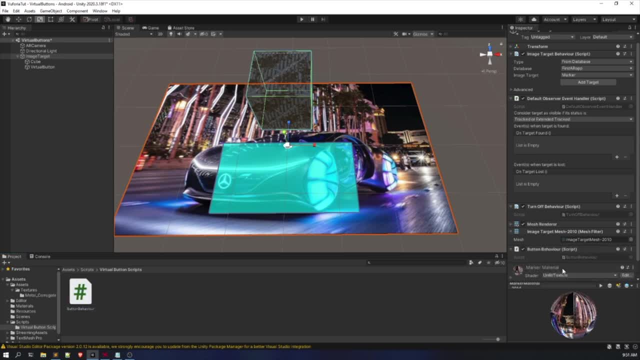 the thing is that the process will be following up. is it requires us to add the script in the image target only, in the image target game object only? there's a reason behind it. i would show you why. all right, it depends on our scripting procedure, and i'll be scripting it in a in that way that 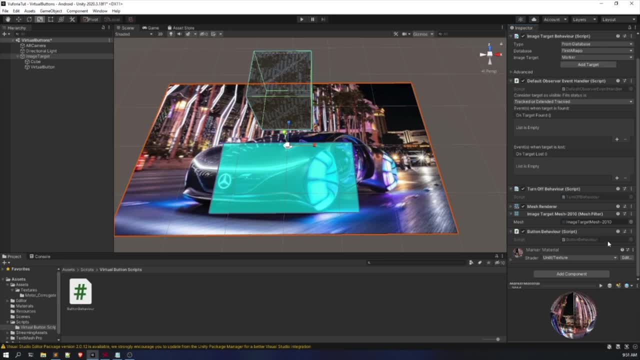 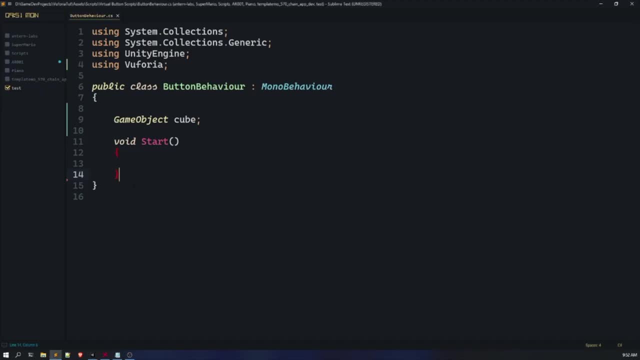 the script should be in the image: target game object only. all right, so you can see that we aren't able to see any sort of uh variable, but we did create one, so let's give public. all right, see by default. all right, by default, whenever you create a game object, all right, or any variable, it is public, it is private. 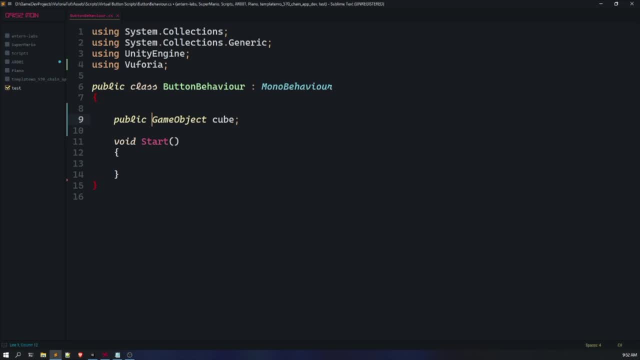 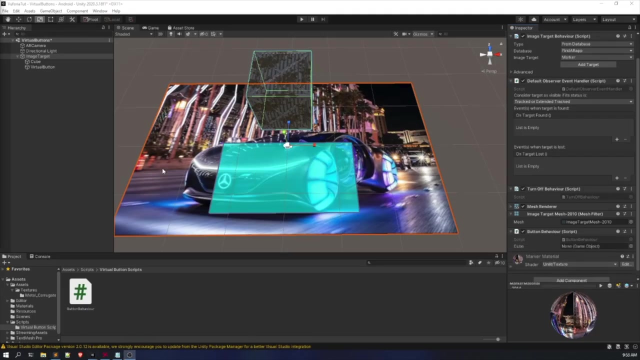 all right, those variables are private by default. so, uh, make sure if you want to make them public. if you want to make those variables public, then you should remember that to add public keyword in front of them. so now let's see if our cube, like if our variable, has appeared. all right, so click on the image. 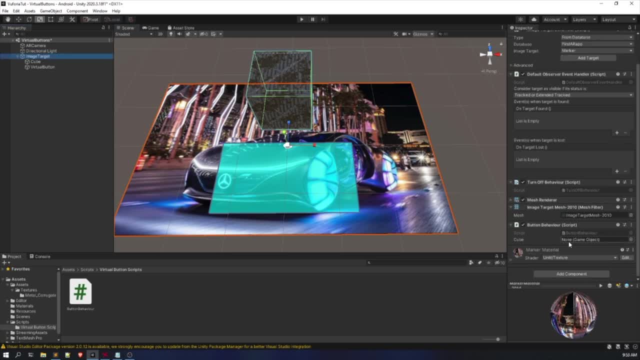 target and then go uh at the last and check in the script- uh, in your script that you created- that the cube is coming or not. all right, so in here our cube variable is coming. now what you have to do is to select the cube. all right, select the cube and drag and drop it in this particular area. all right. 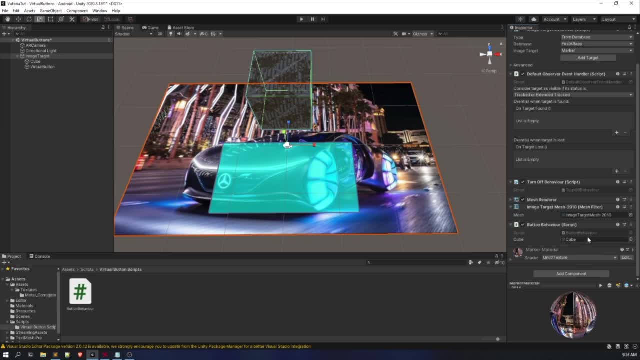 in this particular place. it uh. it is currently taking all the uh game objects that are of type game objects. all right, it is taking all the objects available in the scene that are type of game object, all right. so anything that is game object it will take it in here. it can be stored in. 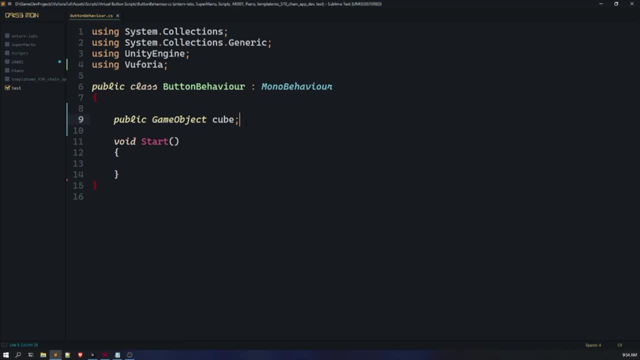 this variable, all right. now another thing is that we have to create a private variable. all right, because i don't any uh want anyone to edit it externally. so we have to give a data type. that is virtual button behavior, and let's name it button, or let's say v button. that is virtual button, all right. 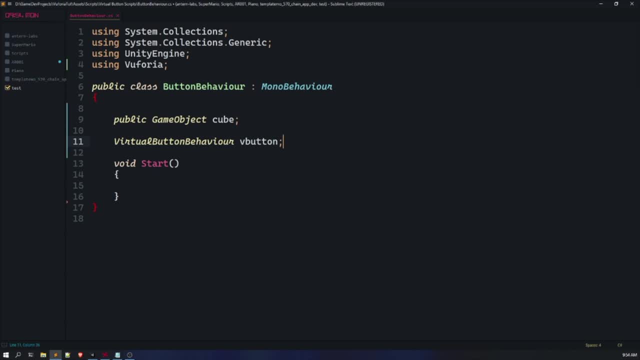 you already know, uh, if you don't give public in front of any sort of variable, what will happen? all right, now, as we have created, all right, as we have created a virtual button, we have to reference it. also right, we also have to refer. so how should we do that? right, it's very simple. all right, there are some, uh. 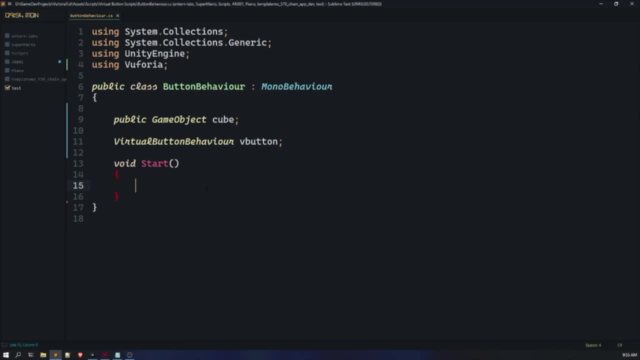 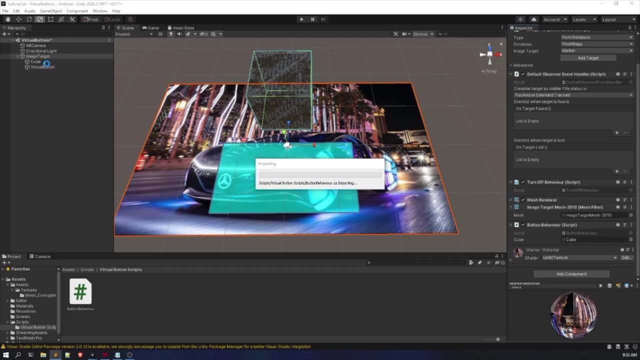 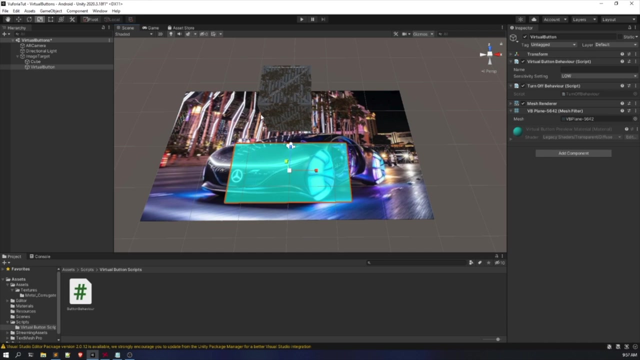 functions, that is, get um, get component, get component in children. we would be using get component in children because we are targeting the like, we are targeting the means. let me show you all right, see, you can see in the unity editor, alright, that this is the image target, alright, this. 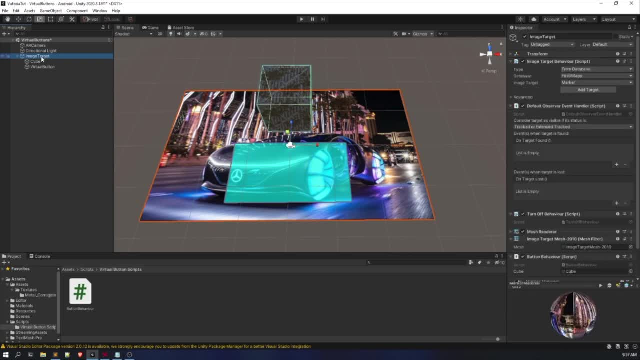 is the mean game object: alright, and the virtual button and the cube. I'll write: the virtual button and the cube are a children, alright, are a children of this main game object: right, so we are attaching the script in this game object: alright, We will be trying to access the VirtualButtonBehaviour script from the VirtualButtonGameObject. 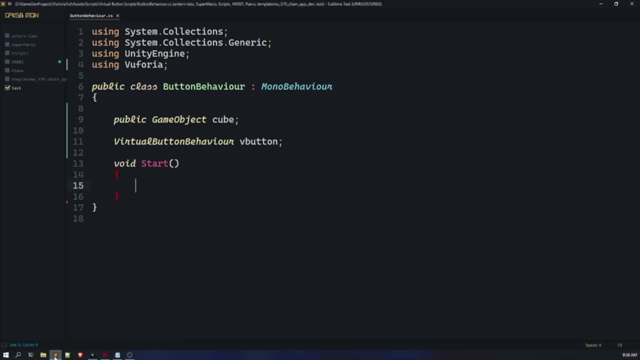 We will be doing this, As I told you that in normal state, the cube should be hidden. When we hover over the VirtualButton, the cube should be visible. That's what I told you. The very first thing is Make the cube invisible, cubesetActive. What will happen with this is: 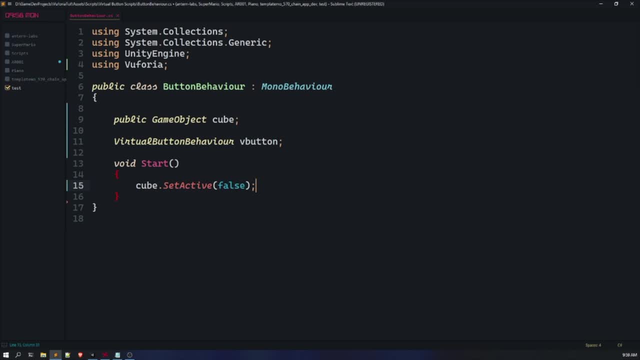 Whenever the game or app is starting At first instance, this cube will be deactivated Or, in simpler terms, It will be hidden. And you know that. what void start is? Void start runs only once, Whenever the application is starting. That's why, whenever the app will start, We will run this particular function. 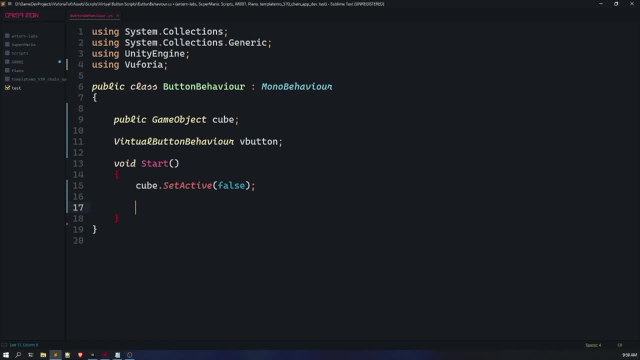 cubesetActiveFalse, So that the cube gets hidden. Another thing is that you can simply hide it from The particular hierarchy panel, from the scene only, But of course that isn't a good idea, So let's do it by script. Now You have to instantiate. You have to contain the VirtualButtonBehaviour script. 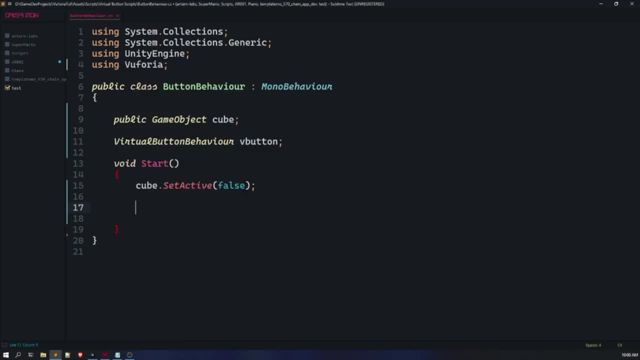 So I am going to name it- Sorry, I have already named it VButton, Sorry, VButton. So yeah, Now let's, Let's sort. What can I say? Let's Add: Alright, Let's reference That particular VirtualButtonBehaviour script. So you have to type this GetComponent And 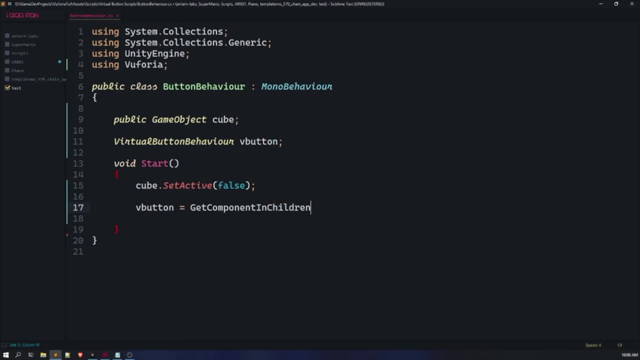 Children. Alright, And inside of this, Inside of this particular greater than and lesser than arrows, You have to write the script name. Alright, That is VirtualButtonBehaviour. Alright, Now We have targeted the VirtualButtonBehaviour script Now. Alright, Now Let's create two functions. Alright, Let's create two. 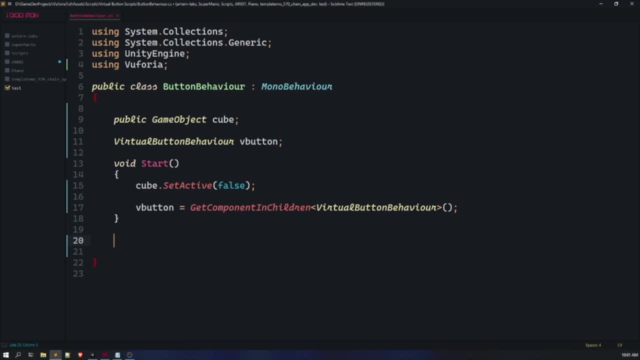 Another two function that will help us To activate and deactivate the script. So Void OnButtonPressed. We have to Take a VirtualButtonBehaviour as a parameter. Sorry, VB, Alright. And then What we have to do is Whenever- Alright, Whenever the button is pressed. Or you can say button is hovered. 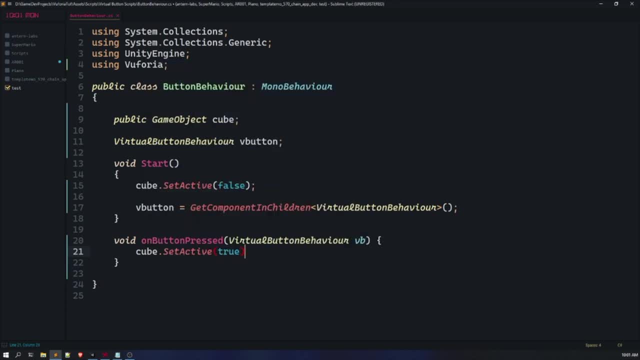 We have to Set the state of the cube to true So that it is visible, Alright. And whenever Button is released, Alright, Released. Whenever the button is Button is released. What we are going to do is We are going to simply deactivate The cube. Alright. So it is as simple as that. 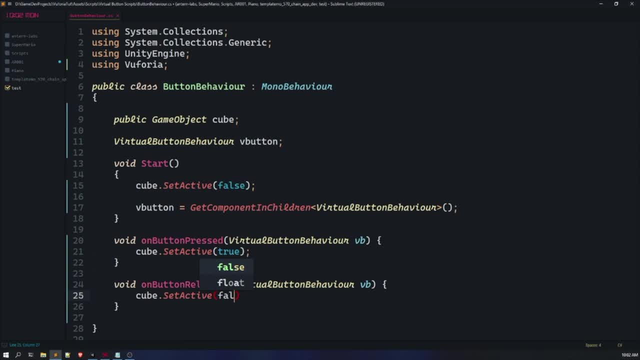 But Alright, But We haven't Like see. Whenever To make any sort of function work Right, Any sort of method work, We have to Call it Right, We have to call that particular Function, But In our case We haven't called it. Can you see That This, This, This. 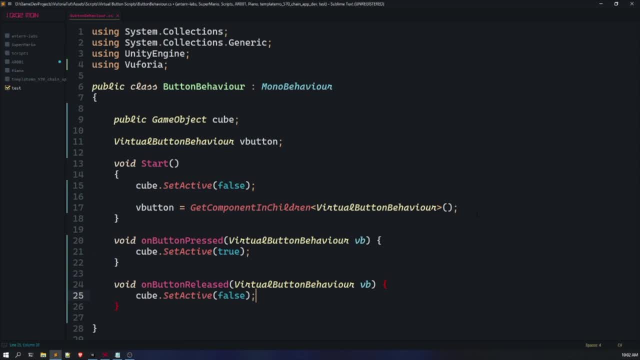 This, This, This, This, That We have called it. Can you see Where we have called it? See Now, Alright, And like When you create normal buttons, Ui buttons, Alright, In Unity There are Some sort of OnClick Functions. Right In the, In the Brton Parameters, There are OnClick. 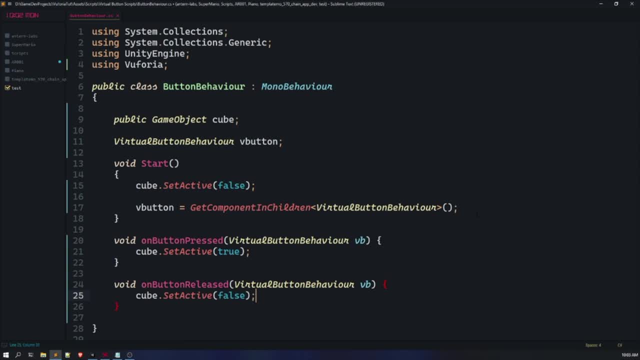 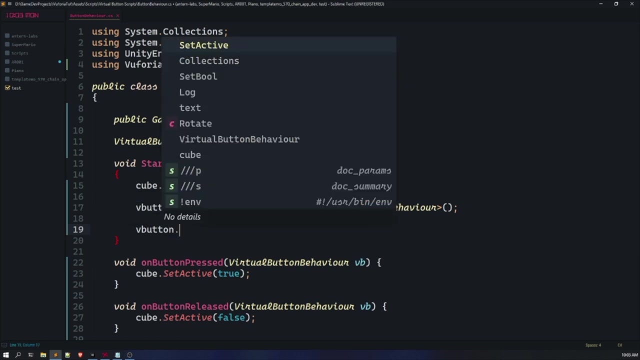 Functions In here. Alright, In here functions in our button. so how do we do so? it's, it is fairly simple. all right, it is fairly simple. so select the button, all right, and then v button dot register on button pressed. all right, and inside the parenthesis, pass the function on button. 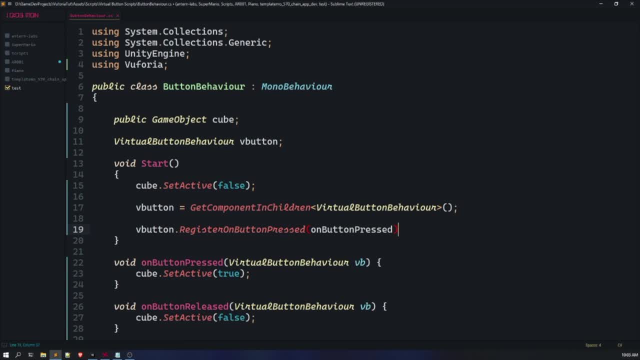 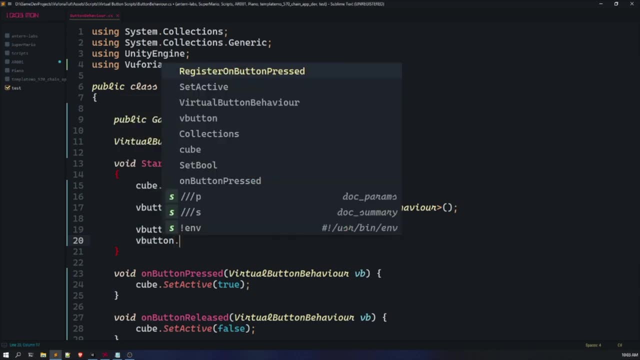 pressed, because whenever the button is pressed we have to run this particular on button pressed function. now v button dot again, we have to do another thing, that is, on button released: all right. so on button released. all right. so yeah, this is it all right. this is it now. 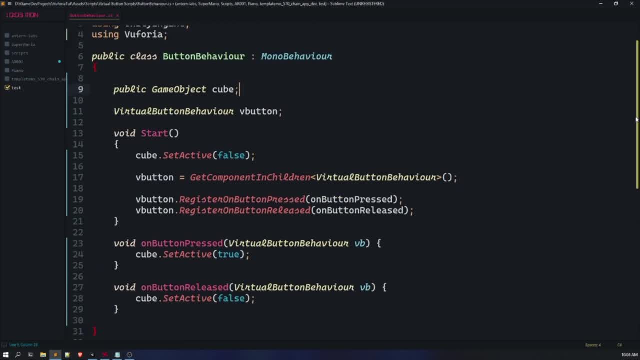 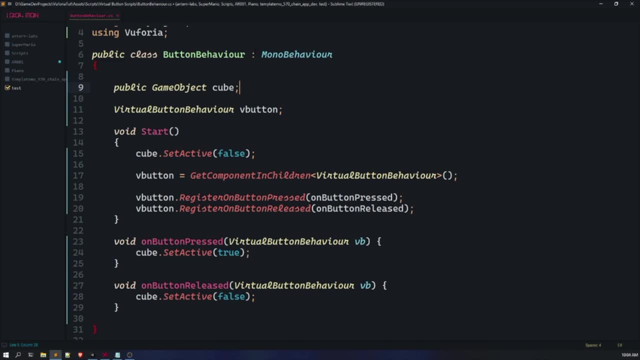 let me recapitulate the whole code to you all right, so that you won't get confused. the very first thing we did is to include the namespace using viewphoria. then what we did? we created a game object- public game object- that is a cube, and referenced the cube to it. then we created a virtual button. 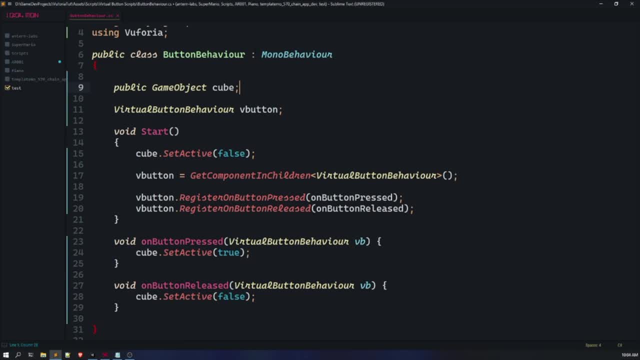 behavior named v button. then in in the start. all right, in the void start what we did we like. in the void start we specifically specified that whenever the application starts, deactivate the cube, all right, the cube should be hidden. then, after doing so, what we? we created two functions. all right, having a virtual button. 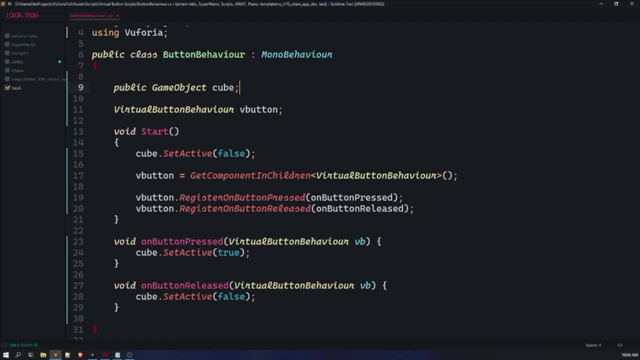 behavior vb as a parameter. so the first function that we created is: on button pressed. what it will do whenever the, when we, whenever we are hovering over the button, or you can say in, whenever we put our hand over the button, that means that we have pressed the button. 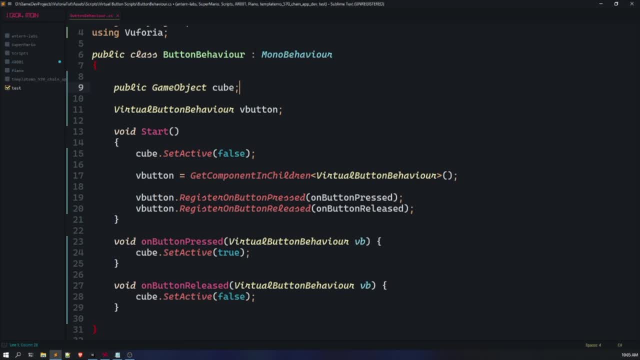 so that's why it is written on button pressed. so basically, we're hovering over it. so, uh, this is what happens now. whenever on button pressed function will be called, the cube will be like will be restored. it won't be hidden anymore, but whenever the hand is released, 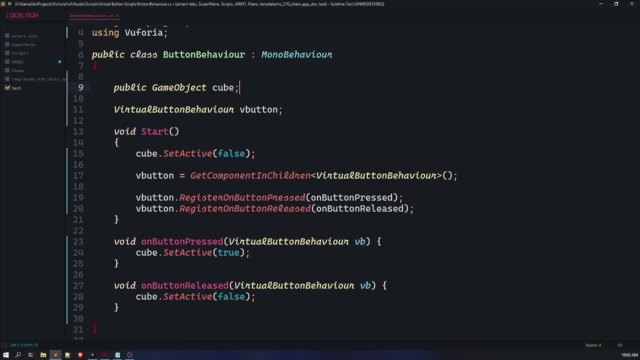 from the button or that whenever the button is released again, the cube will be hidden. after that, what we did is we referenced- all right, we referenced the cube- and we begin integrating everything that was blending in after that, what we did is we referenced and referenced our virtual button behavior script in our v button component and then we used functions. 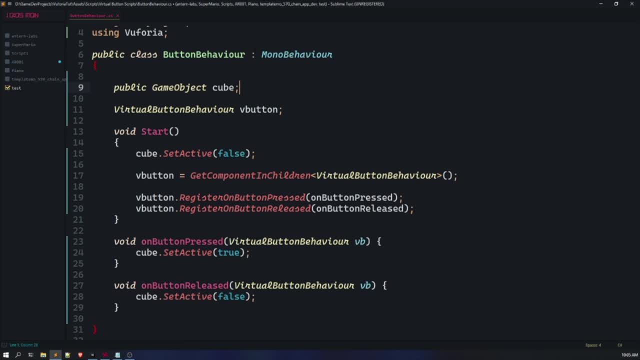 to call our own functions right. like v button, dot, register, on on button pressed. what it will do, is it? these two works like on click, all right, whenever you are pressing the button, it will do some function and we have passed the function, that is, whenever we will press the button. this. 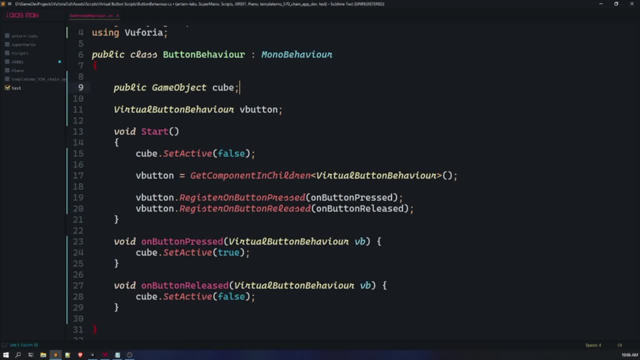 particular on button pressed function should run, and another is that v button dot register on button released. all right, what will? what will it do? whenever the hand is released from the button, it will run the function on button released, all right. so let's save the script, right? let's save the script and try it out in real time. 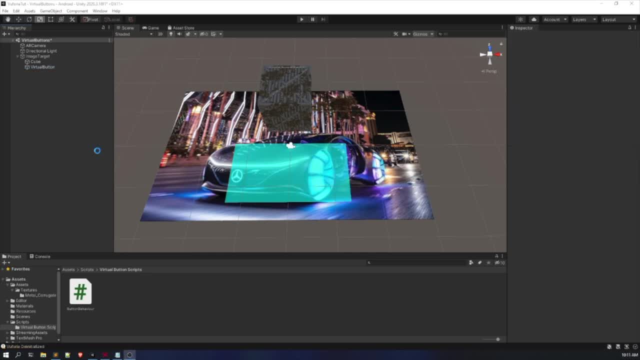 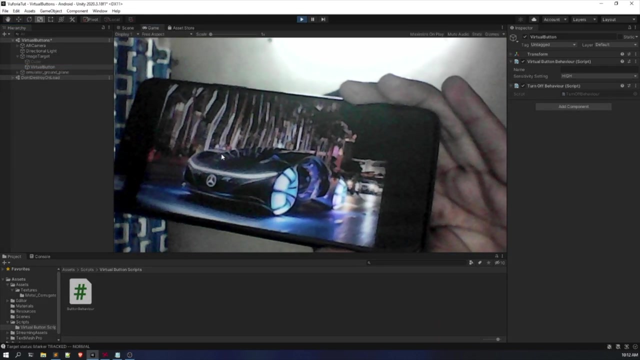 you, let's try it, our basically let's write our application that we created. the very first thing i would suggest you to do is to change the sensitivity setting to high, all right, and then click on play mode, all right, so as you can see it right in here. all right, here is my marker. 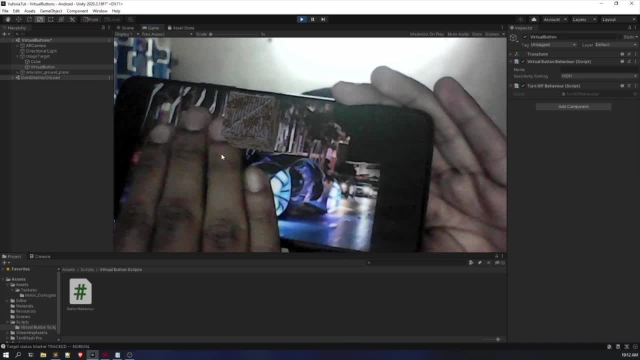 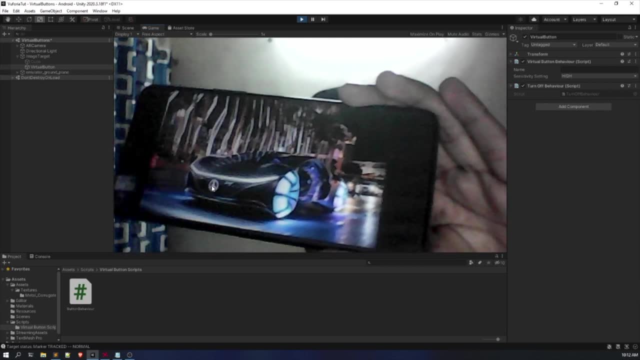 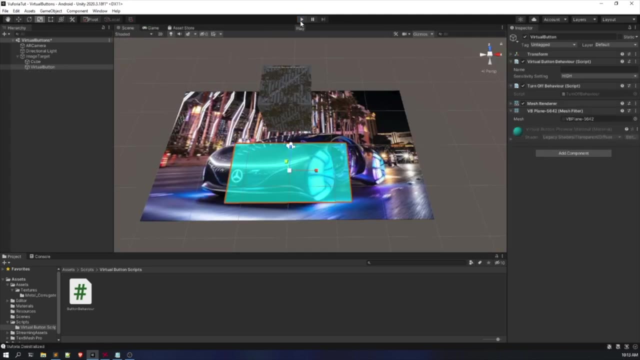 you can see that whenever i am hovering over my uh hand, you can see that the cube is appearing, and whenever i am releasing my hand, the cube is going all right. so this is how it basically works. all right, as simple as that. so, congratulations. you learn to create how, your, how, like how to create virtual buttons, but 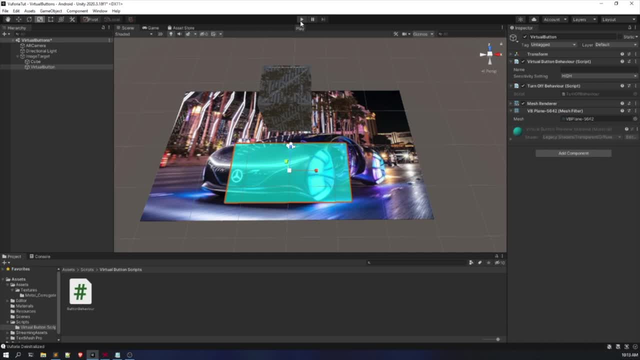 if you, uh, if you ask me what do i suggest- virtual buttons or uh? ui buttons? i will tell you that i am using ui buttons. believe me, ui buttons are far better than these virtual buttons. all right, so i would always recommend you to use uh? ui buttons. yeah, if there is a need to use virtual. 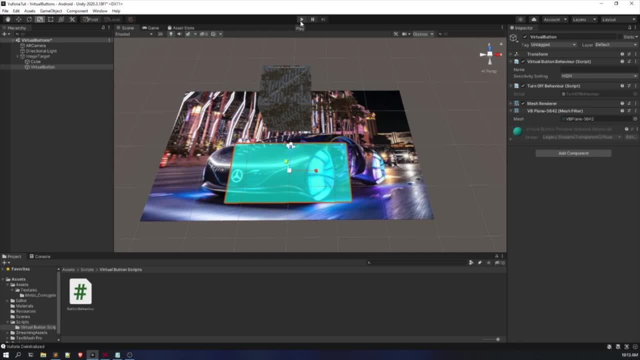 button then only use it all right, because those watch, uh, these virtual buttons sometimes even doesn't tracks the hand, like it's really hard to get them track the hand. maybe it's because of my laptop's camera, but it it is really problematic and, uh, it's really hard to get them track the hand. 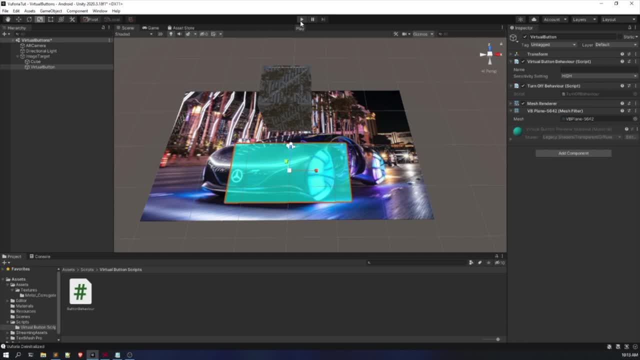 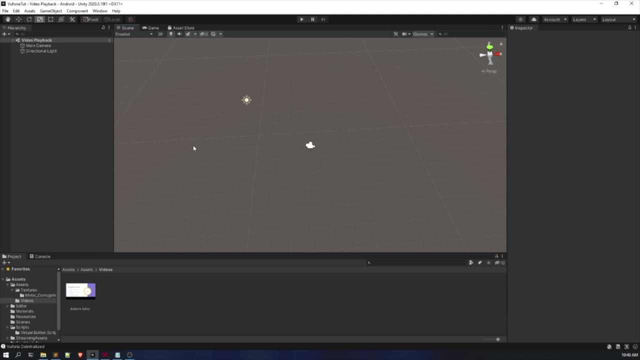 uh creates a lot of problem and also breaks the user experience, so that's why i always recommend uh ui buttons. all right. so yeah, in this lecture we are going to learn how to uh use video playback feature. all right, in our viewphoria project. so the in this video we are going to uh implement. 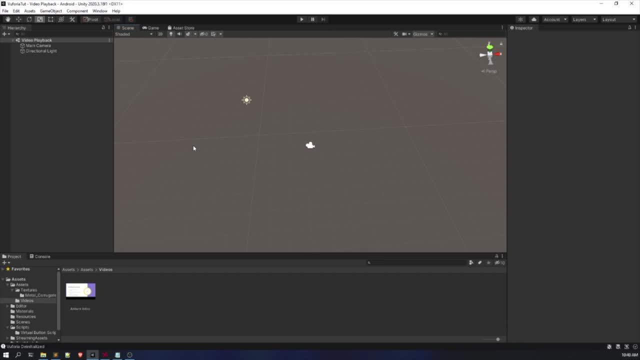 our own video player, you in augmented reality, using viewphoria and unity. after this video, you would learn how to use your videos in your games, all right, in your viewphoria applications. now, in this video, i'm going to show you there are actually two ways to- uh means add. 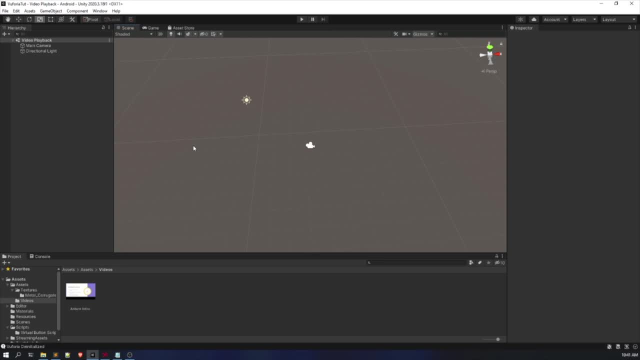 the video playback functionalities, such as play, pause and stop. all right, but there's another way, that is the non-coding way. all right, i'm going to show you the non-coding way. that is, to use the given on-click functions means on-click functions. and then i'm going to show you the non-coding way. 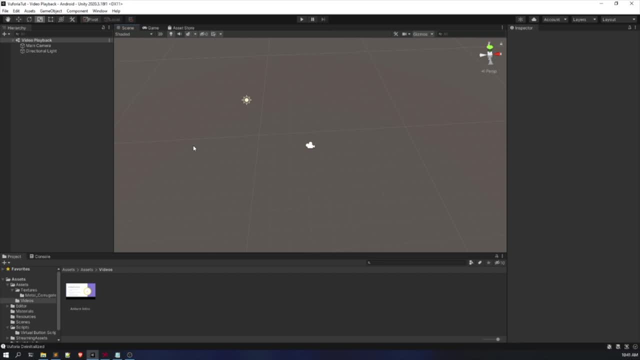 ready-made on-click functions given in unity. all right, even, i'm going to show you how- how to play the video whenever marker is found and stop it whenever marker is lost. all right, this video is going to be the- uh, really is going to be really simple video, so follow along. all right, now, first, 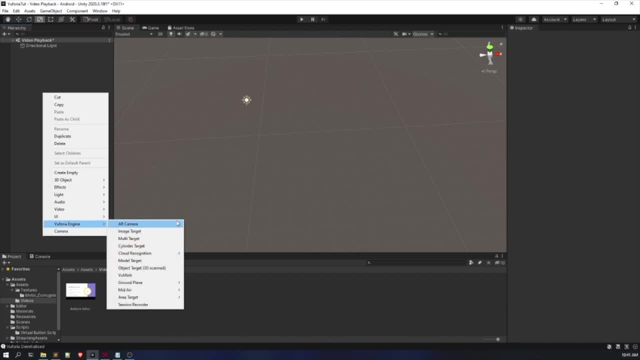 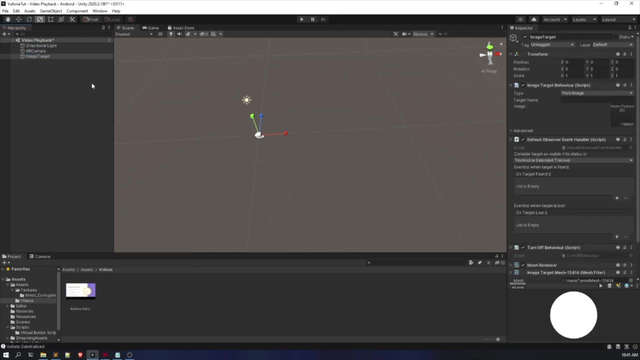 of all, delete the main camera. after deleting it, go to view for your engines- uh, add ar camera. then again right click to view for your engine and then add image target. all right, in the image target, select uh from database. then select the database and the image target, all right. this is the basic process that we follow along. all right, and i am using the. 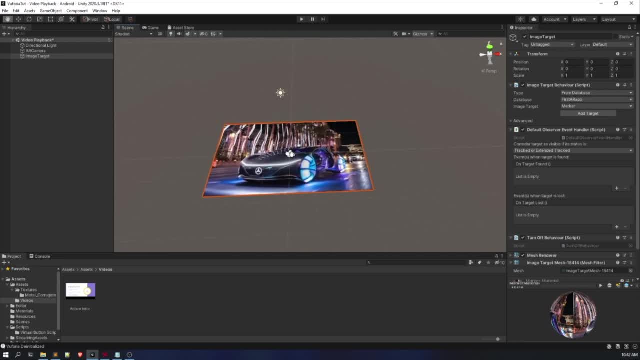 previous project only. so i need- uh, i haven't created any sort of new license or any sort of new database, so i'm using the same marker and all those things, but in different scenes. all right, here's a script: default observer, event handler. in here, the you can see tracked or extended track. 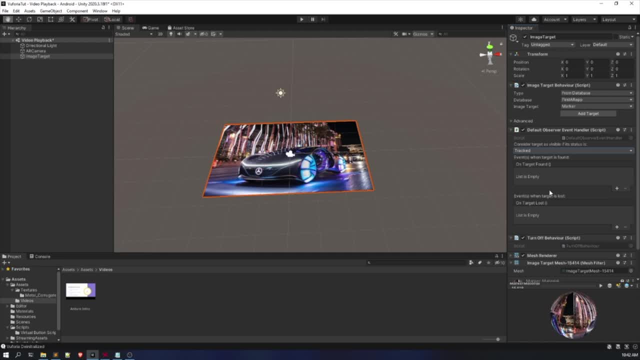 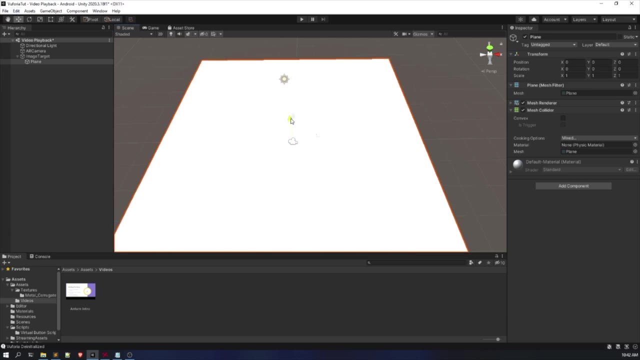 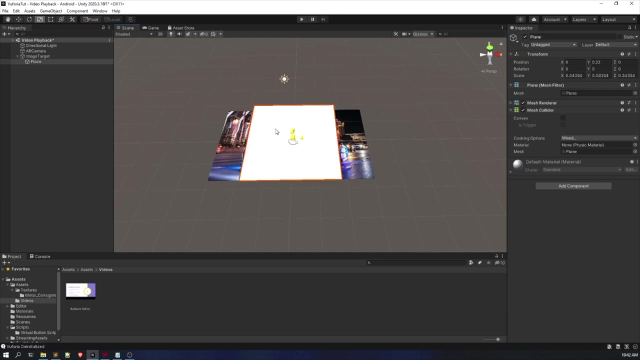 click on tracked- all right. then what you have to do is click on image target- add a plane. all right. go to 3d object- add up plane- all right. here you can see a plane is added. now we have to reposition it. uh, move it upwards a bit, that is, in the y-axis- then resize it, all right, so that it can. 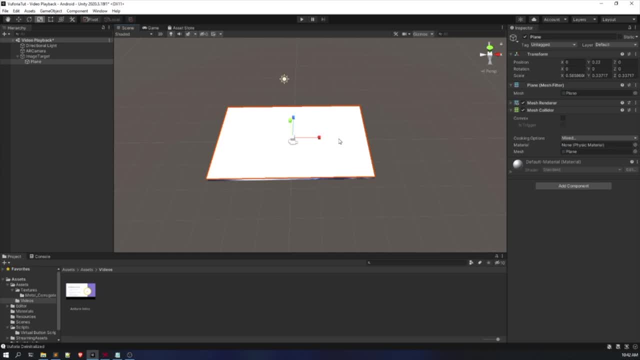 get the markers. all right, you can even create your ar video playback like ar video application or you can say ar video player after watching this video. all right, you can like get all the videos from the file explorer then show it in here. all right, you can create your own application with. 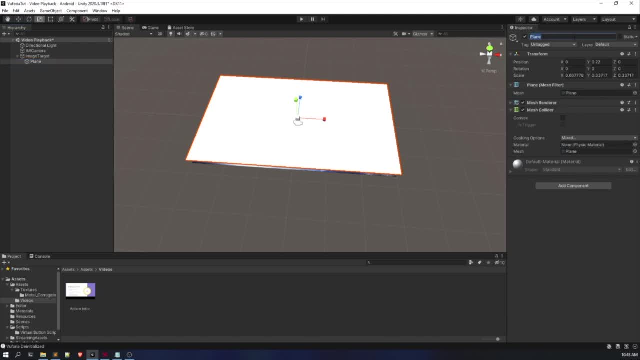 it, but in augmented reality. all right now, let's name the plane to video playback. or let's say: all right now, in here. after that, go to in the inspector panel, only search for video. all right, click on add component, then search for video, and here we'll get a com. here you will get a component. 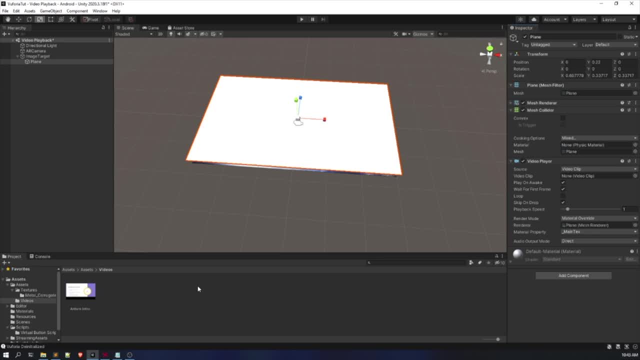 called video player. all right, now, i have already. i already have a video imported. all right, i already have a video imported in my uh assets, so i'm simply, uh, what you have to do is you already know how to import it, right, because you just simply have to download the video and just import it. it. 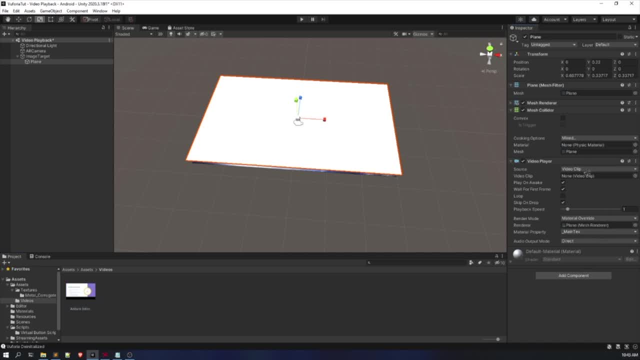 all right now. you have to drag and drop the video inside of the video clip parameter. all right and voila. this is the thing you have to do. all right now. another thing is that whenever you play- all right, whenever you play this, all right- the video will be inverted. all right now. let me show you. 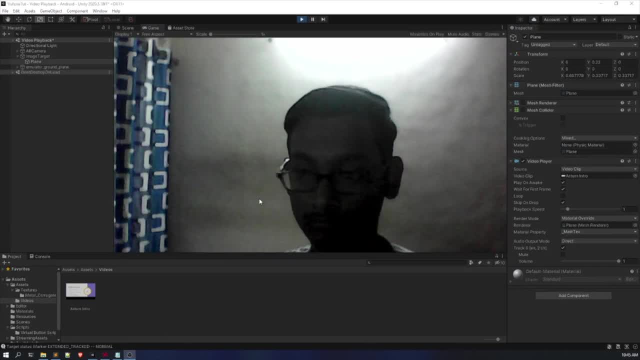 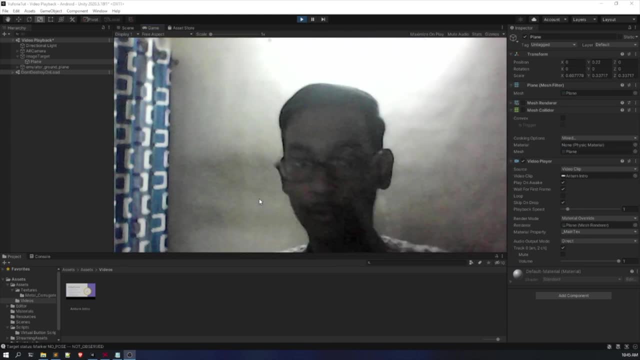 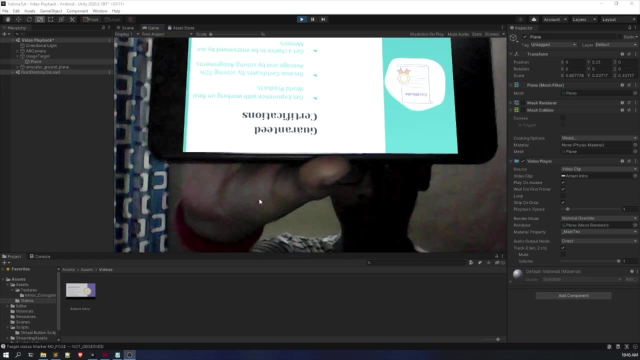 what are the problems that we'll be facing now? so, as you can see in here, all right now. as you can see in here, the problem with the video is all right. it is currently playing. all right, it is currently playing. just wait, the video is currently playing and it is inverted also all. 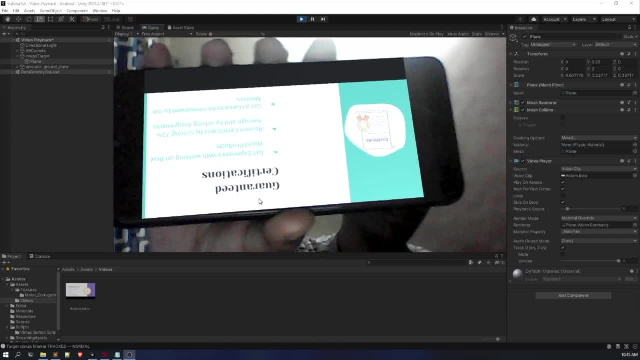 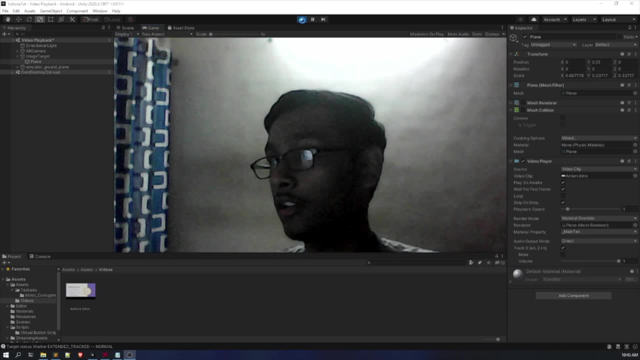 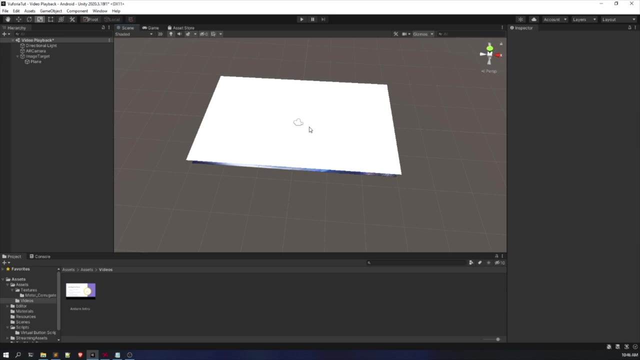 right, you might not be able to hear the audio, but the audio is also playing in the background, all right. so this is the problem we are facing currently. let's, let's fix it. all right, let's fix it. see, the very first thing. all right, the very first thing you have to do is to invert. 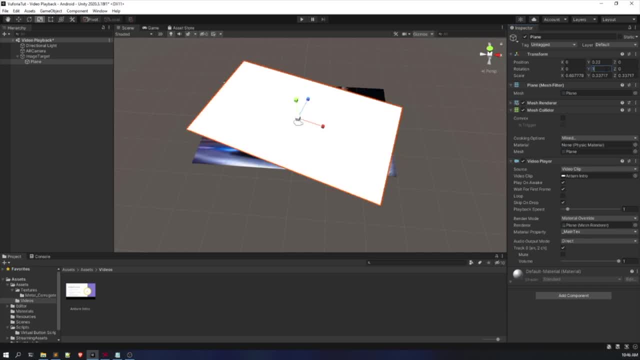 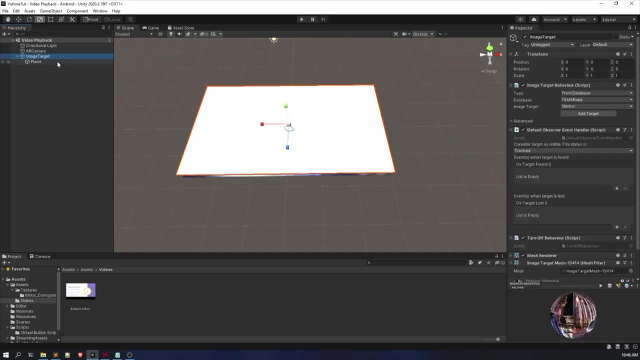 this all right. invert means rotate this in the y-axis, rotate this whole plane in the y-axis so that we get the video straight. all right now. after this, we'll be getting the video straight. another thing: all right. another thing is that click on the plane. all right, in here the video. 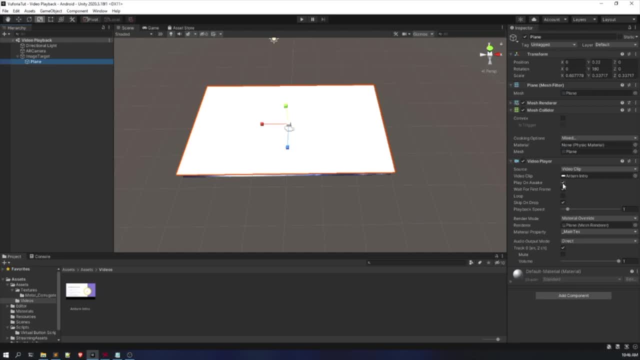 option. there is an option called play on awake. what does this mean? this means whenever you are, uh like whenever the application is starting, it will start playing the video. all right, this is what it means now, uncheck it. all right, uncheck it now. uh, all the problems that we we were facing. 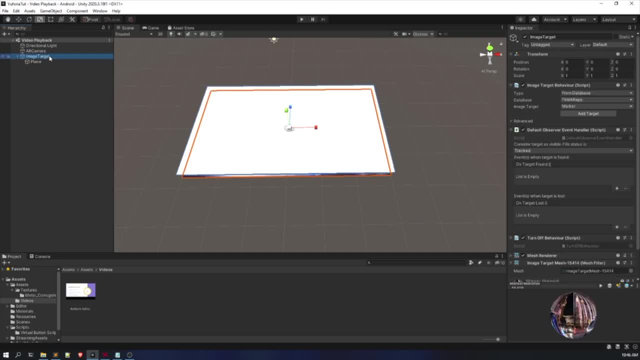 uh is fixed now, so let's implement the features that i told. now, here you can see. here are two options on target found and on target lost- right. what we have to do is in here, uh, click on on target found, click in it, all, right, and then here you can see. this is the video, right? this is the video now. 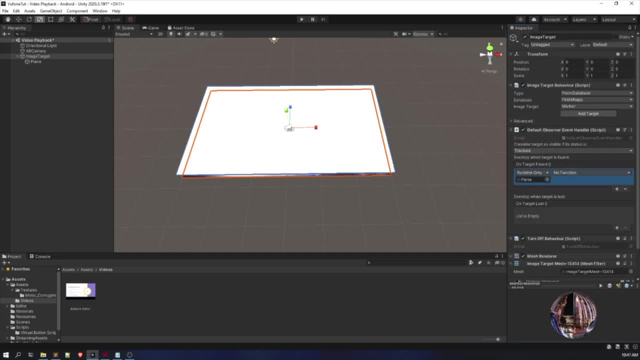 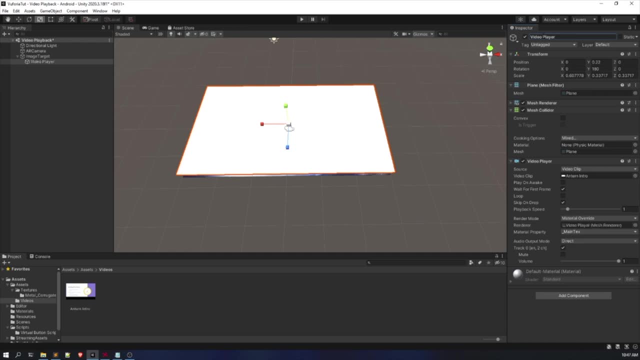 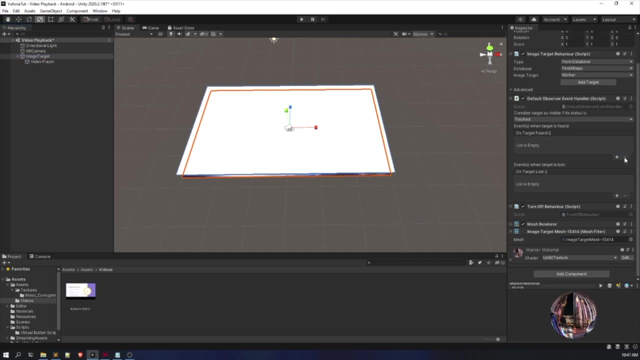 drag and drop it in here. all right, drag and drop this video in here now, uh, i fall. i guess i forgot change the name, so name it video player. all right, name it video player. now what i did. let me show you the process again. all right, click on image target. here are two options on target found on: 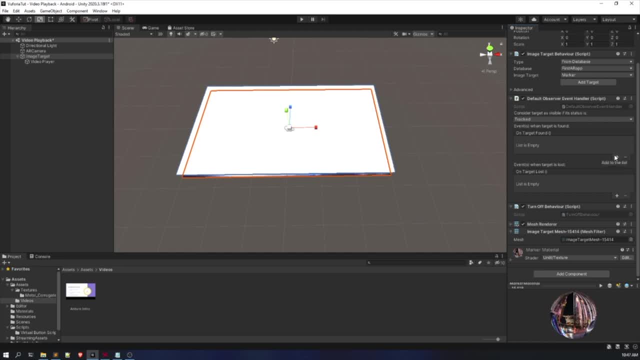 target loss. these are called on target found and on target lost. these are called on target lost events. all right, these events call some sort of function. all right. these type of events are also available in ui buttons also. i'm also going to show you how to create play pause button in ui. 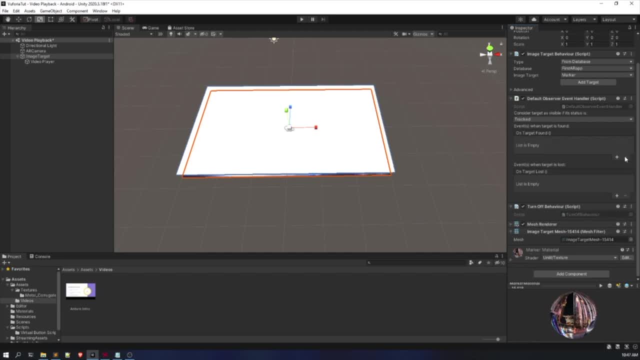 all right, so don't worry. now what you have to do is click on this plus icon in on target found, then drag and drop your video player inside this particular field. then here you can see. here's another. uh, here's a drop down that no function written in here. all right, in here what we have to do? go to the last and you would. 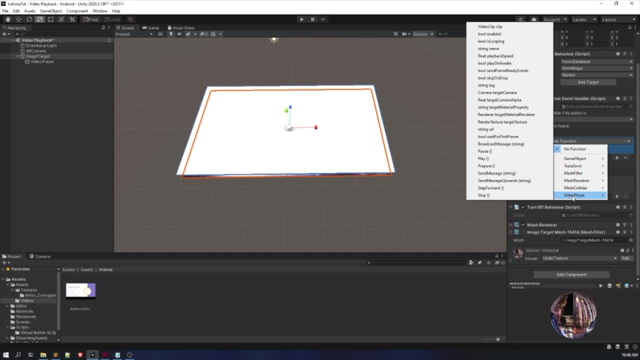 find an option called video player. all right now in here. what you have to do here are multiple options available. from these options, you have to click on means: call the play function. all right. what will happen whenever? all right, whenever you try to play the video, all right, sorry, whenever. 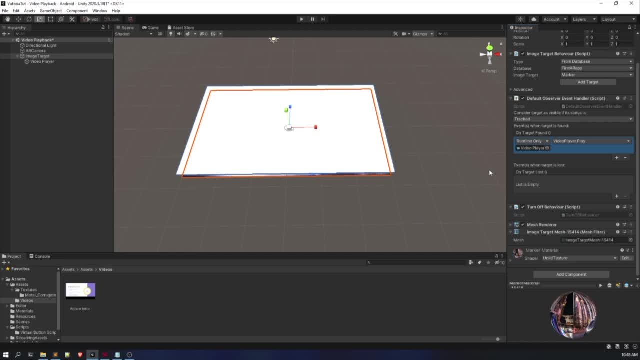 you? uh, whenever the marker is found, all right. whenever the marker is found, it will start playing the video. all right. another thing, all right, another thing is that i want also to integrate whenever- all right, whenever the marker is lost, the video should pause or stop. all right, so for. 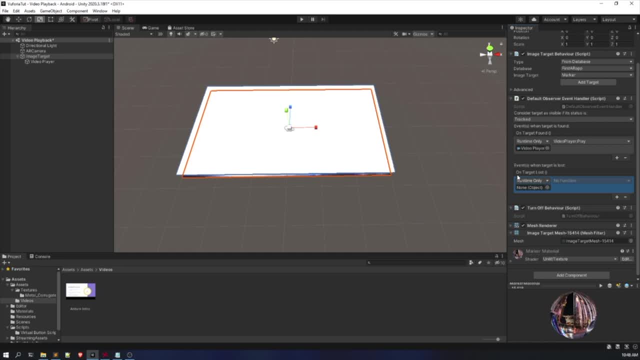 my case, i would like to stop it, so again. uh, in here's an another event parameter that is on target lost. again, do the same thing. drag and drop the video in here. call a particular function inside the video player. i will be calling the video player and i will be calling the video player. 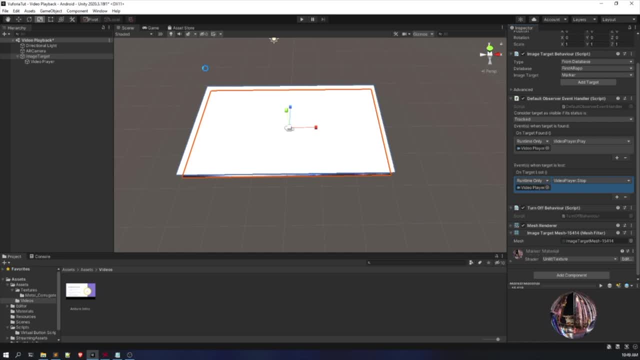 stop function. all right. so yeah, this is how we basically create our own video playback features. all right now, this is the basically uh, this is basically uh, if you want, only to use viewphoria to control the video playbacks. all right, like whenever the marker is found. you want, you want. 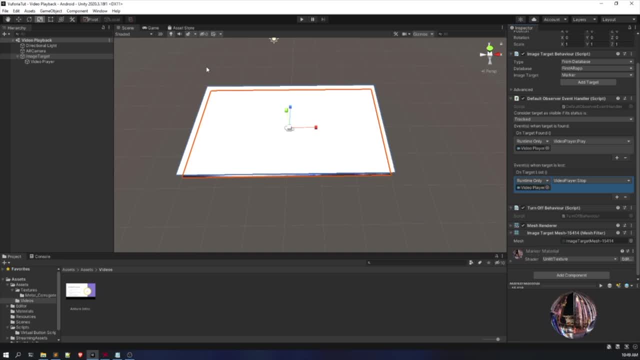 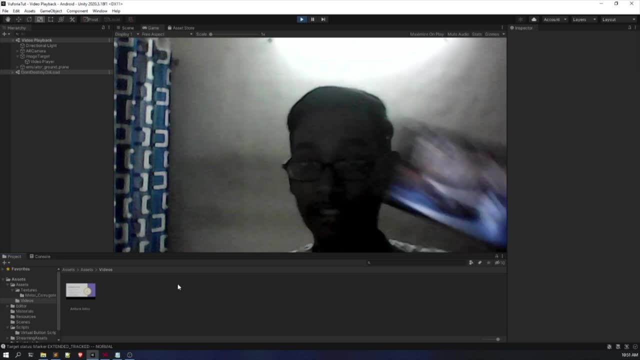 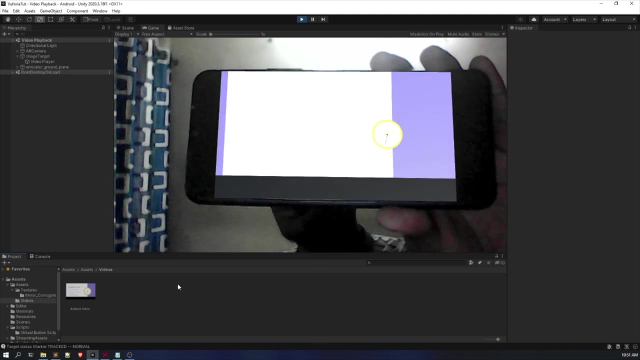 to start the video, and whenever the marker is lost, you want to stop the video. all right, so let's try it. so as you can see in here, all right, here, uh, the marker is found and the video is playing all right. i'm not sure you are able to hear the audio or not, but you can see the video is playing. 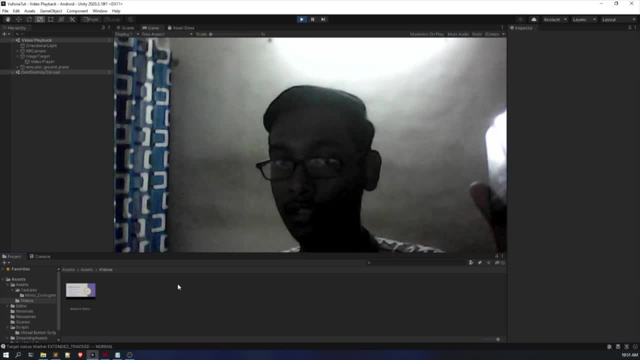 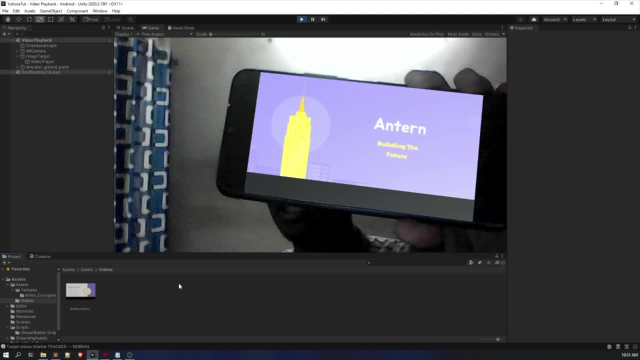 now, if i remove it all right now, if i remove it all, right, uh, the video has stopped. right, you are not able to see anything now. if i again, all right, if i again uh put the marker, you can say: the video is starting all over, right from uh, from the start. the video is starting from the start, all. 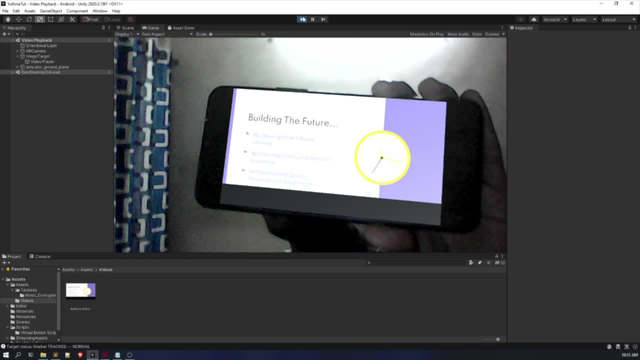 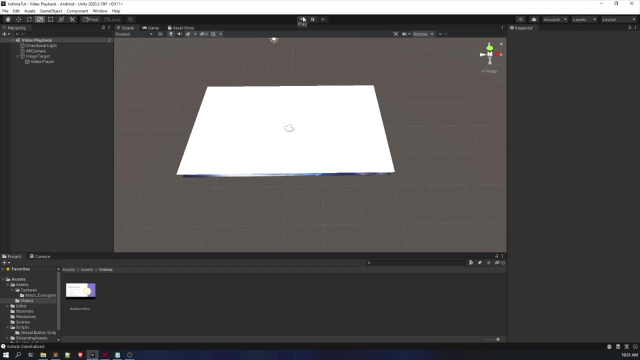 right. so yeah, we successfully created our video playback features. all right, we successfully created our video playback in viewphoria. now it is our time to do the same thing using buttons. all right, that is to implement the play, pause and stop functionality using button. so it is. 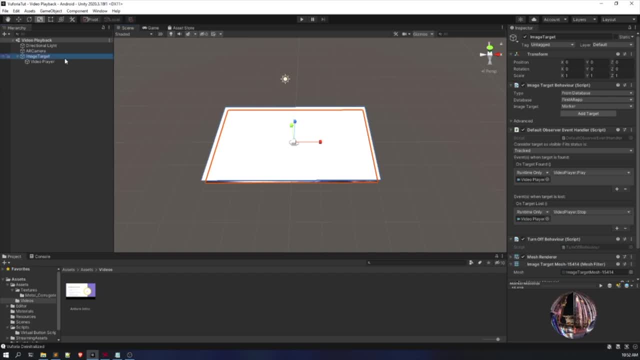 pretty simple, all right, it is not that complicated. what you have to do is see: i'm not going to remove. these are good, all right, because whenever I want key, whenever the marker is found, it, the video should automatically start, and whenever the marker is lost, the video should automatically stop all. 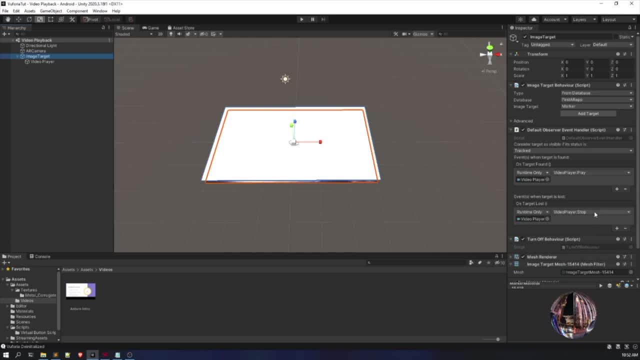 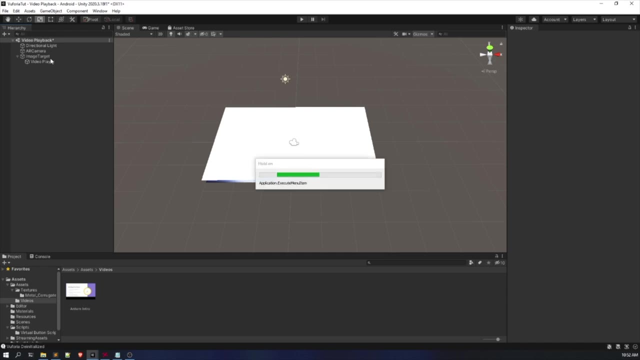 right, or you can. what you can do is: you can like make it pause. all right, just make it pause. let me change it to pause, all right. so whenever the marker is lost, the video will pause, and whenever the marker is again found after being paused, the video will play from the point where it has. 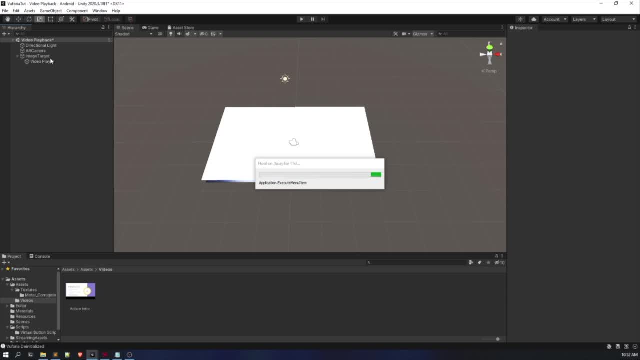 been paused. all right, so it is it. so that's how we implement video playbacks in viewphoria. if we want to do the same thing with markers like marker lost or marker found, all right. now we'll be doing the same thing using UI canvas in viewphoria, all right. 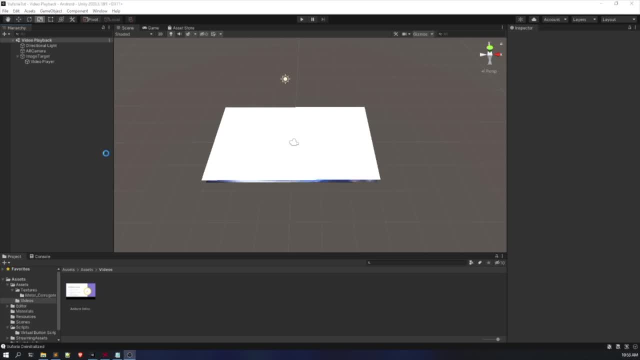 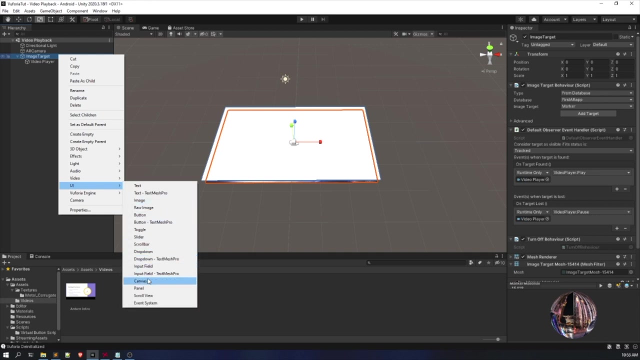 so now, as we have successfully created our video playback, now it is our high time to implement some particular button for it. all right. so how do we do that? the very first thing, click on image target. I'm sorry, yeah, click on image target. then go to UI, all right, and click on canvas. 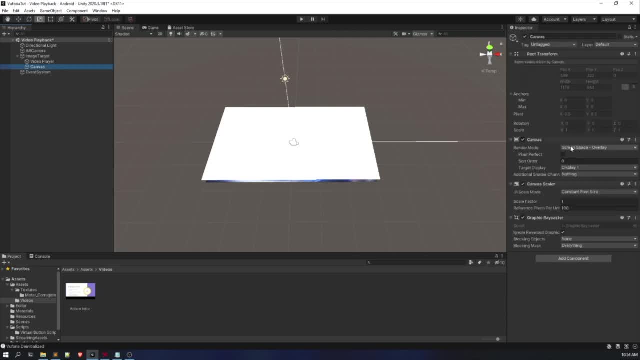 all right. so click on canvas. then in the canvas- here you can see canvas scalar. here it is written constant pixel size changed into scale with screen size. it will help- uh, help- the UI to be more responsive, all right. so, yeah, let me make it first. uh, let me. 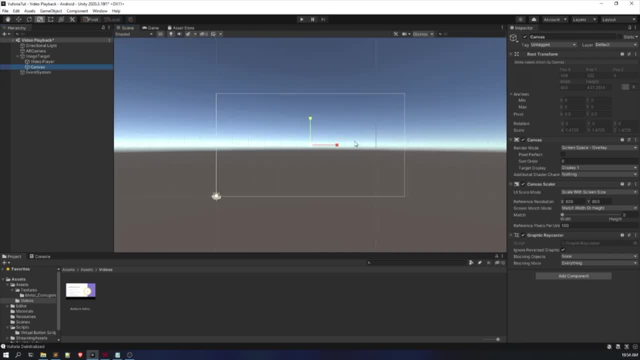 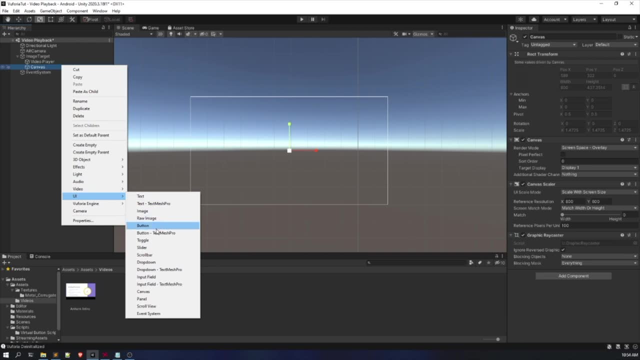 go to the 2d mode for designing the UI. all right now, as I'm 2d mode, as I'm in 2d mode, now I have to implement the buttons. it is fairly simple: just click on UI. then I would like to implement text. 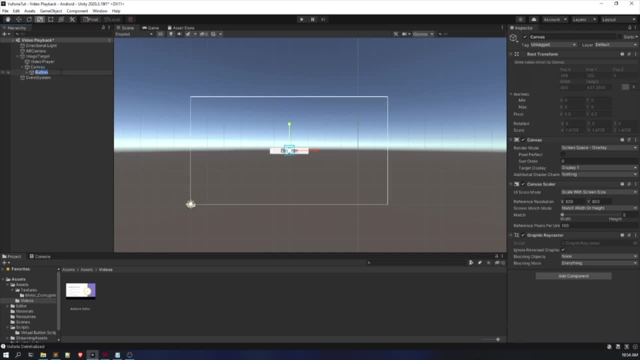 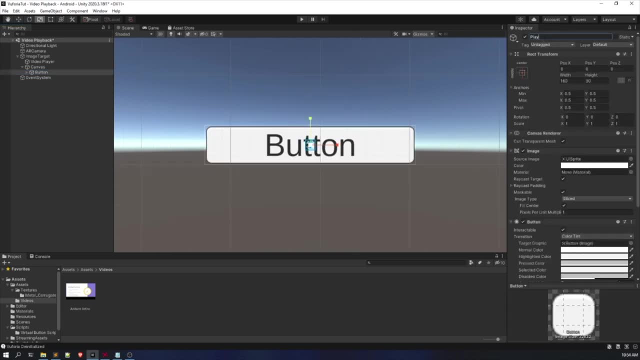 text mesh pro buttons. all right, so I would click on button text mesh pro and it has been imported. all right, the very first button that I have to create is the play button. all right, this is the play button that I want to create. now I have to anchor this button also, all right. so how would I? 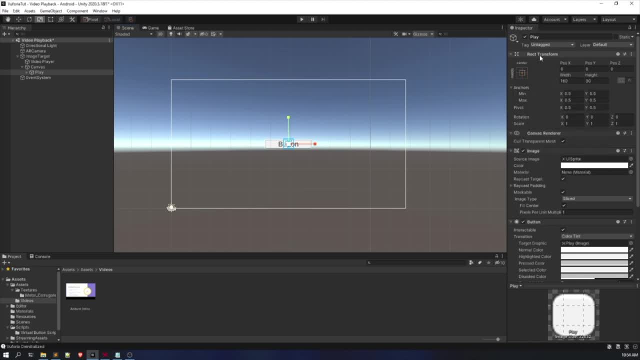 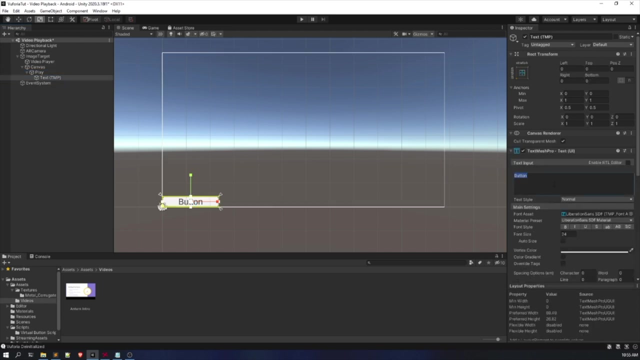 do so, so simply click in here. all right, you can see this rect transform option. click in here and press alt key. after that, click on the. this last, this last one. all right, click on this last one now. I also have to change the text inside it. all right, so that it resembles play button. all right, now, let's make it bold. now. I see I would. 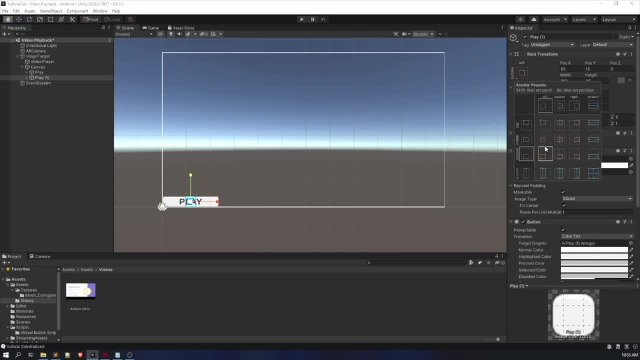 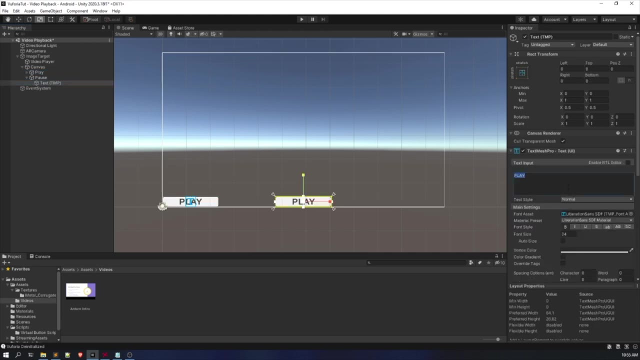 be duplicating this button. all right, so that it becomes more easier for me now. yeah, now, let me change it to pause. all right now. let's change the text of it to: that is to pause. all right now. again the same thing. duplicate it. let's name it: stop. let's change the name to: 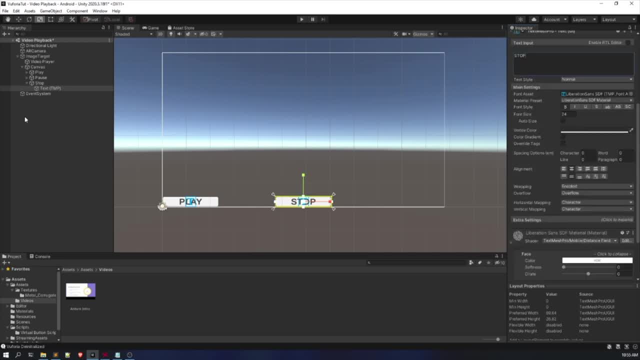 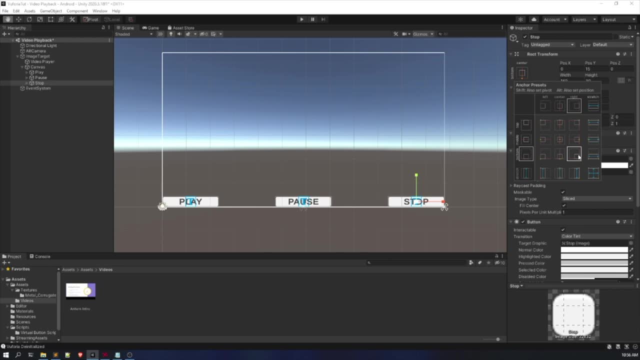 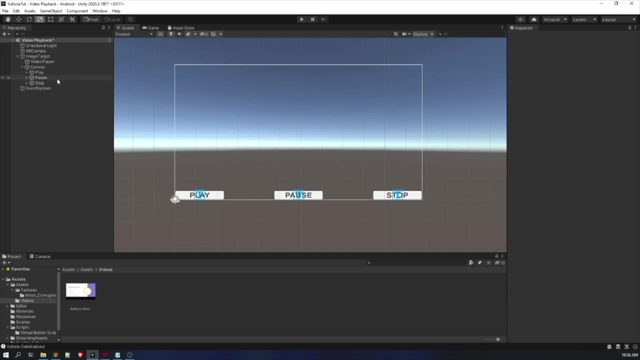 stop and also make it bold. oh, all right, I have already made it bold. now again, go to rect, transform, alt, then the right side. see, our button is anchored, all right, in a great way. now what we have to do is we have to implement the functionalities. so the very first functionality: 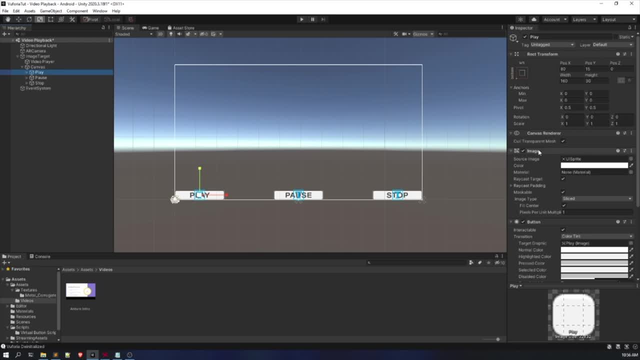 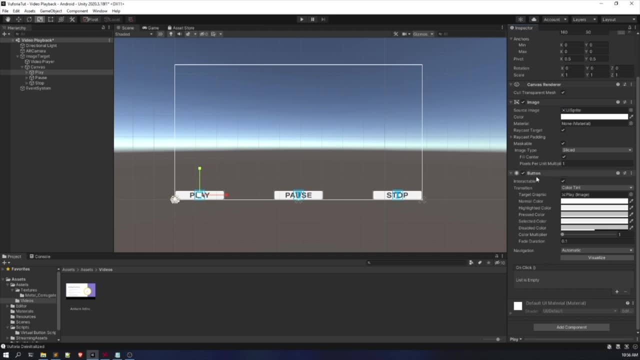 I am going to implement is the play button functionality. so click on the play button, go to go below, all right. go below, like in the in the last, and here we'll find an option called button option, or you can say button component in here. alright, click on that button and then all right, in here there's an option called on click. 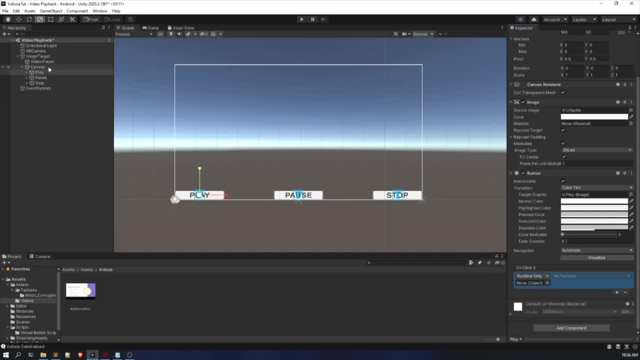 alright, so simply click on the plus button. it's it's. it's similar to the image target on target found. all right, it is similar to that. now again, drag and drop the video player object inside all right. drag and drop the video player object inside the play button. 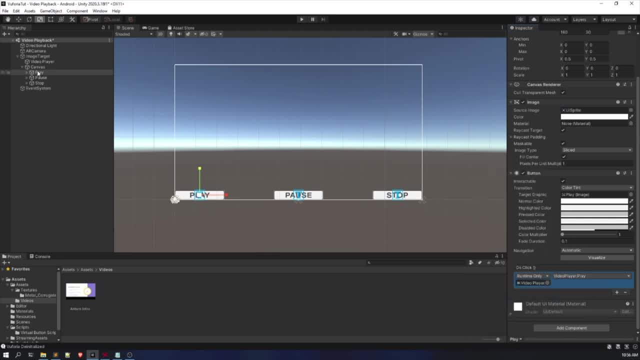 then select video player and then click on play. alright again thing. all right, do the same thing with the other button, but uh, choose different uh set of function based on the uh function functionality you want. all right, so there's the pause button. so i'm going to use the pause function. and there's the stop button, so i'm going to use the stop function. 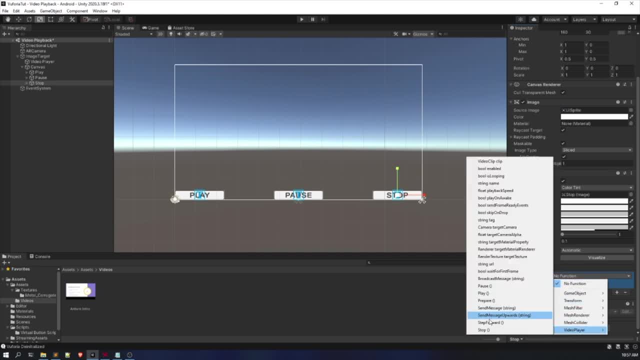 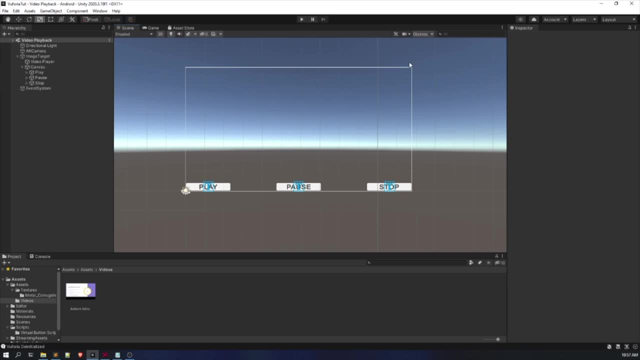 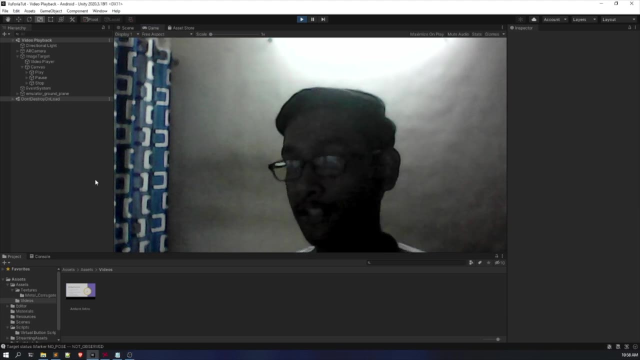 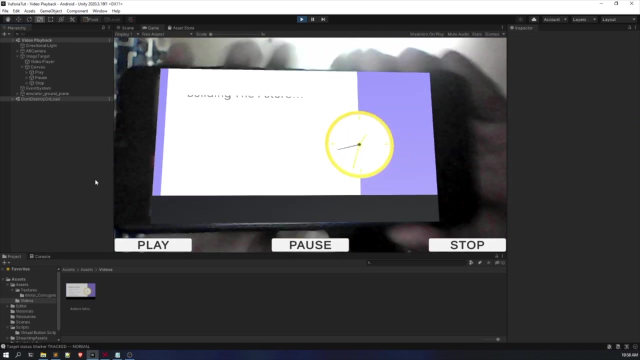 all right, cool, now let's let's test it out by playing it. all right, so, guys, just see what is happening in here. all right, so whenever i you can see the video has started playing. all right, you might heard, uh, some sort of sound, maybe i'm not sure. all right now. 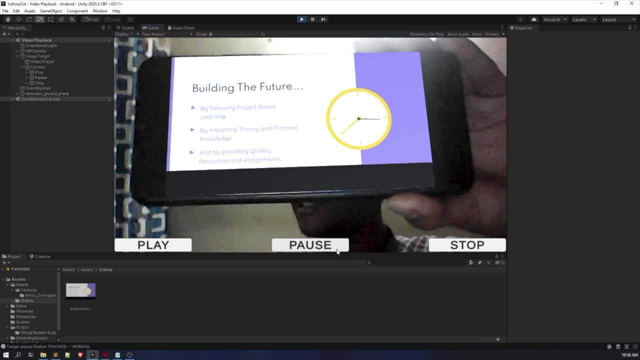 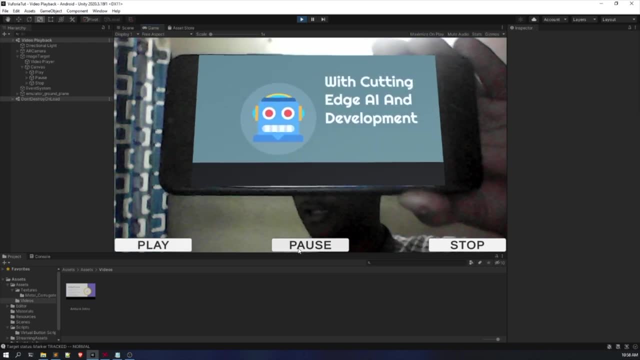 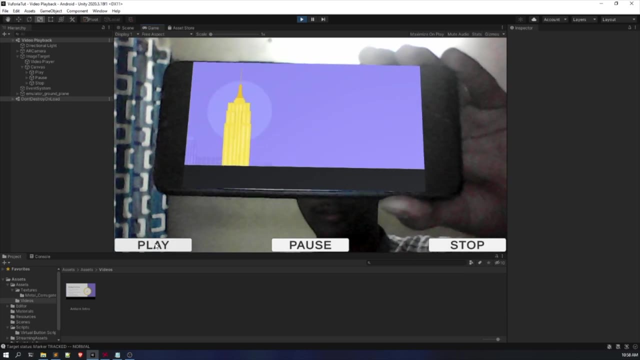 let's? let's pause the video. all right, see, the video is paused now. the video is paused now. let's play it again. the video is playing all right now, let's pause it. the video is paused now. if you want to stop it. the video has stopped now. if we want to play it, the video has started playing, so. 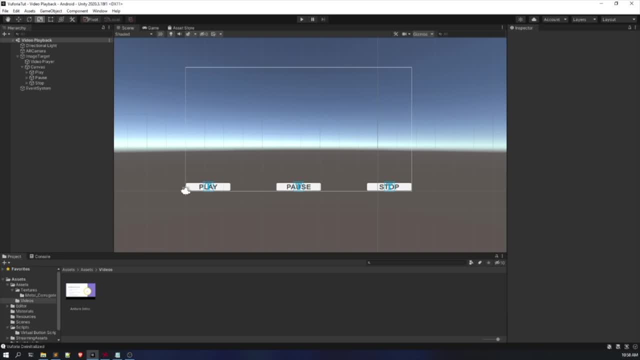 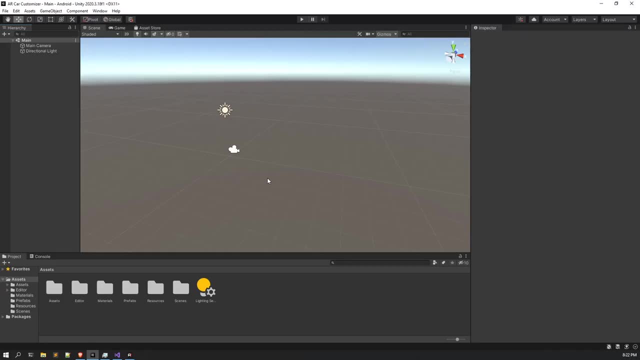 all the functionalities that we implemented is working perfectly fine, all right, all right. in this lecture, we are going to create our own car customizer. so the basic logic or idea behind this car customizer is would would be providing the user three to four different colors. all right, and based on those colors. 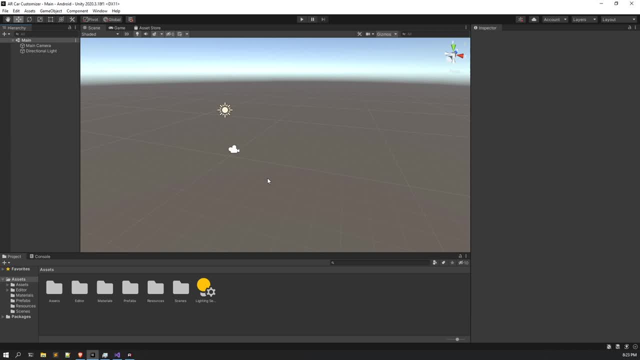 the player would be able to like, select a particular color and paint the car all right or with that color. so this is the basic idea behind today's project: and if you want, all right, if you want, you can like paint the car all right, and then you can paint the car all right, and then 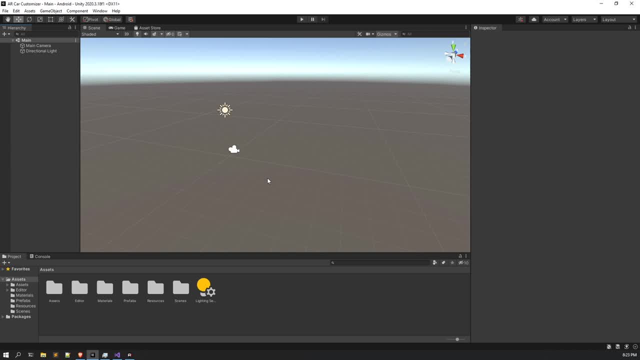 customize this app further. like you can add detachable doors, you can, uh, add numerous numbers of tires that a person could change, right? so, uh, you could, you could do those things also to make this app more, uh like more big, and later on you can launch it on play store. all right, even you can. 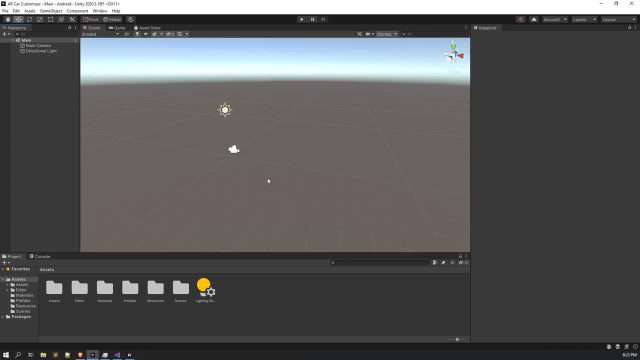 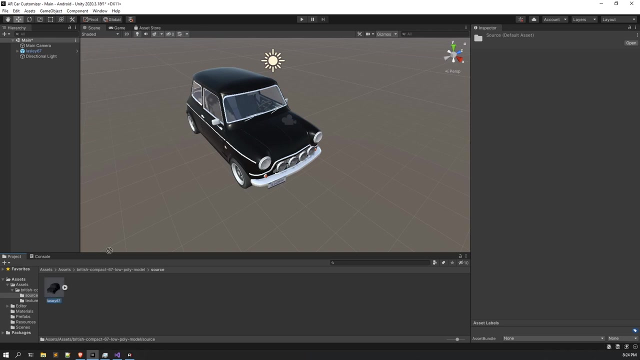 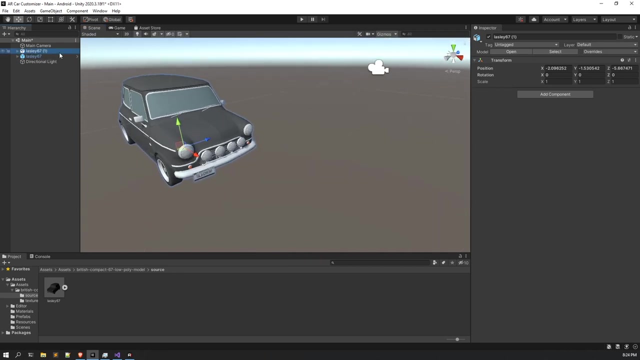 add uh ads into this application? all right, so the uh, let me tell you. so. first of all, i already have a 3d model, all right, inside of my uh unit engine. all right, this is the 3d model. actually, i downloaded it from uh sketch fab. uh, actually, uh, let me show you, this is, uh, the actual model that was there. i edited it later on. this is the actual model. that was a sketch fab uh, so i'll edit it later on. basically, this uh, this kind of color came just because of it's a fbx model, so i'm going to edit it later on. so i'll give you an idea. so this is the 3d model. you can actually see the contrast here, which is the 3d model. uh, all right, now, this is a 3d model and i have moved it to a 3d model, so it's already 3d model. so i'm going to move it to a 3d model and this is the 3d model. so this is what i amazing about sketchfab, but I want to share with you guys. you can see the difference between this three colors. uh, actually, this is my personal favorite color, but i wanted to explain to you guys that, when you know, i 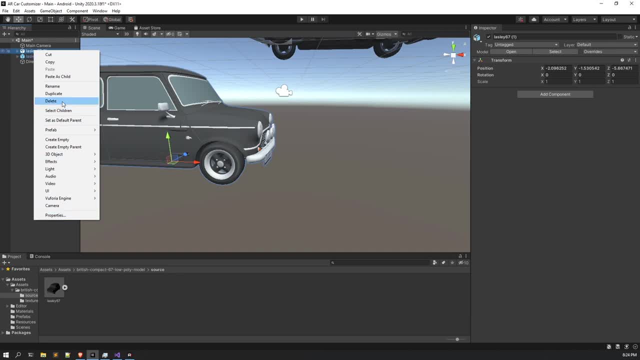 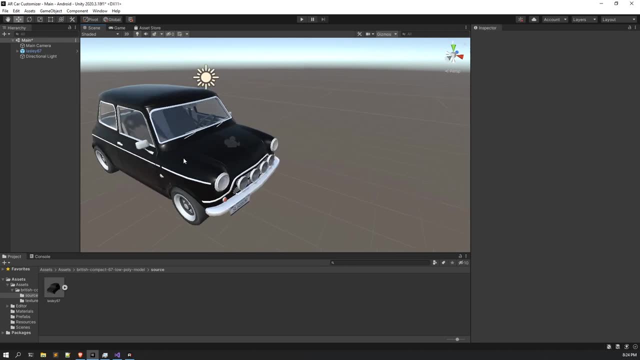 is, uh, it doesn't already have the properties that i want, so i created a new material and applied those materials into the car. all right, so that's what i have done. so, uh, the the better option would be, uh, for you to is, uh, download the gltf models. all right, that is, download the models. 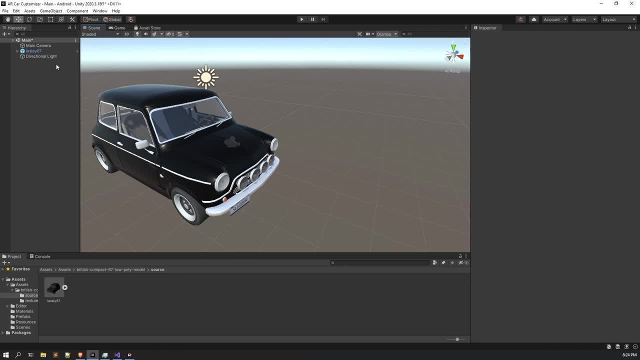 in gltf format, because they are. they comes in much better quality and they have the texture already embedded in it, right, uh, so it would be much better to work with, though. all right, so let me first reset its transform, all right, so, uh. so, yeah, i've resetted its transform and, uh, i'm like 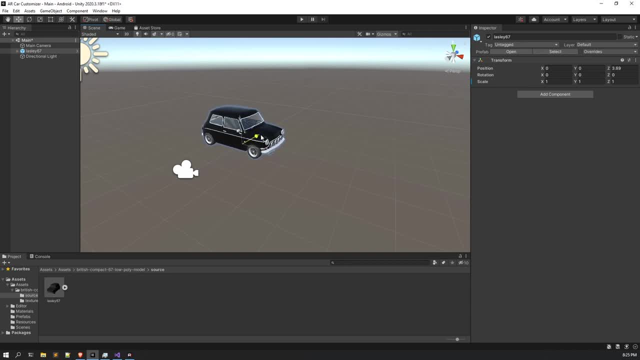 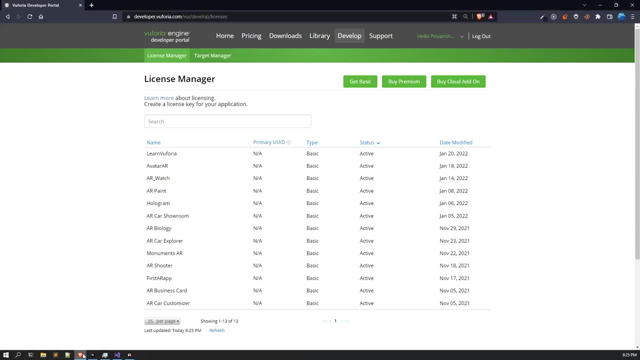 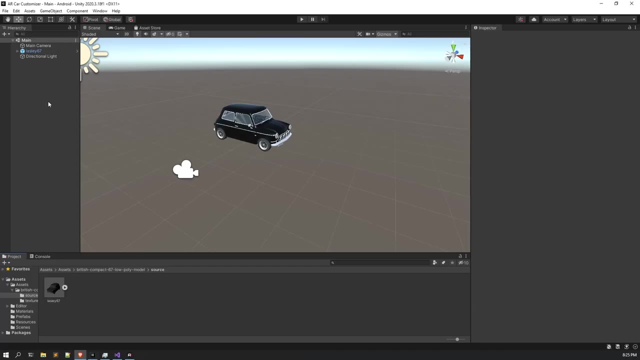 just a bit, moving it uh in the z-axis just a bit. all right, and now what you have to do is, uh, go to your browser. all right, first of all, we have to create a license for our ar application, right, and one more thing: i have already imported the v4ia engine. all right, and 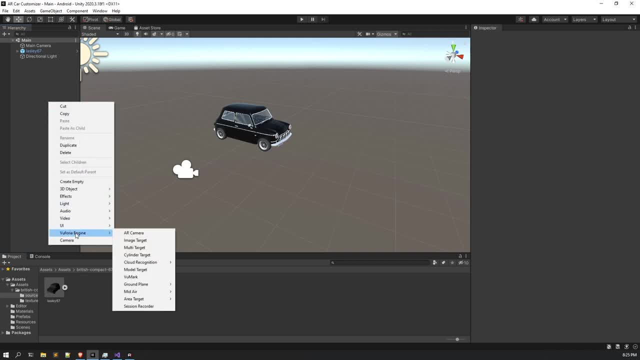 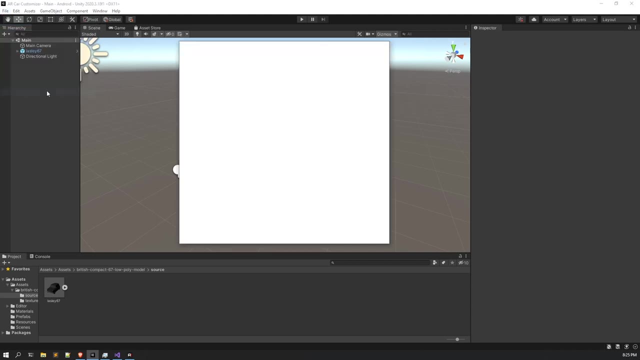 you already know how to do that and you also know that how to check whether it is imported successfully or not. so make sure, uh, you import the v4ia sdk. uh, and before importing, all right, always make sure, before importing, change the uh build platform. all right, because if you 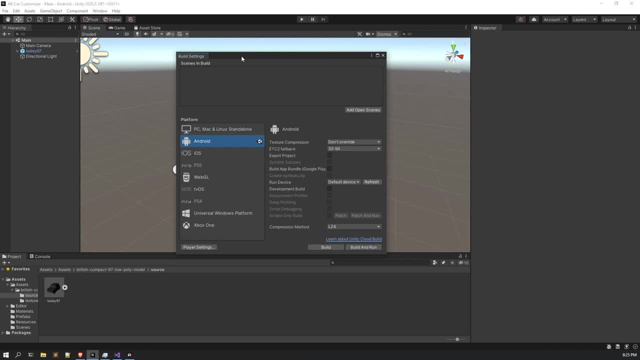 change the build platform later on, that is, after importing the model, the sdks, then it's going to take a lot of time. so what i did is uh, after creating the project, i first shifted uh the build uh platform to android, all right. and then, uh, what i did is i go? i got to the player settings. 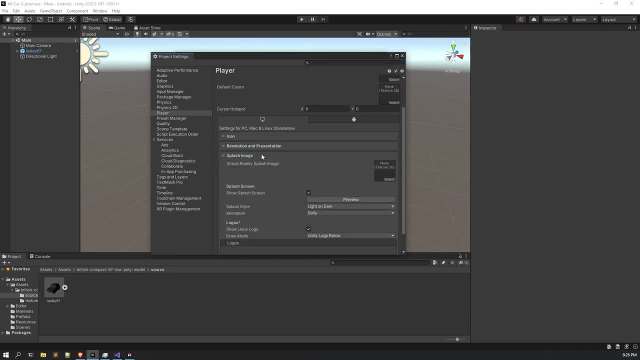 all right. after going to the player settings, what you have to do is, uh, go to resolution and presentation. all right, i'm not sorry, not in the resolution and presentation, just wait okay. yeah, i was actually in the desktop tab. that's why i wasn't getting all the options. so now, as i'm 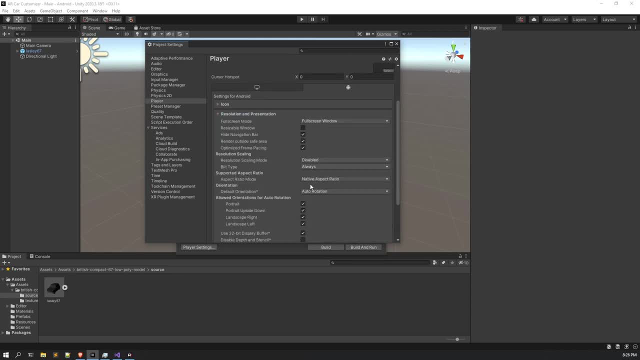 on the android tab. uh, go to the resolution and presentation. you will be getting uh default orientation. change it to landscape left, all right. it's totally based on the camera. you can choose any, uh, any mode you want, all right. but uh, we'll be creating our application in landscape mode only. 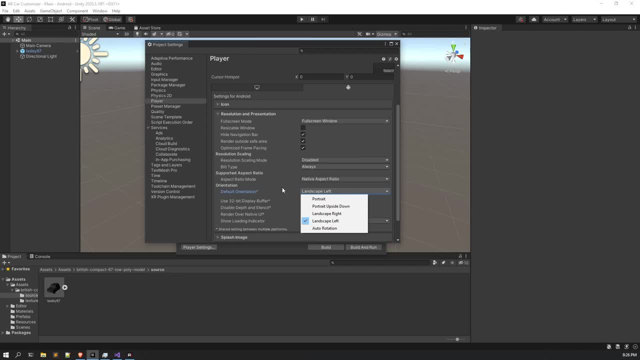 so make sure either to select landscape mode or you can choose any, uh, any mode you want. all right, you can choose landscape right or landscape left. i chose landscape left because of the position of my camera. all right, and uh now go to other settings, all right. here you would find uh android build. 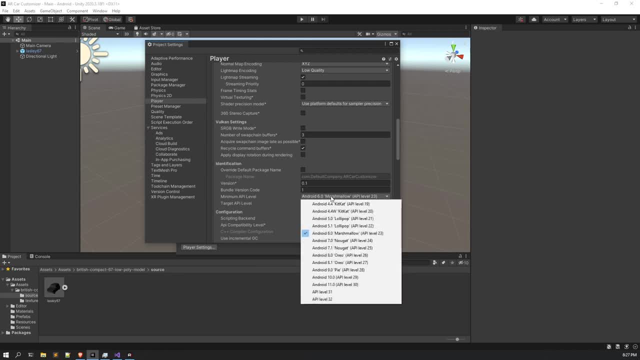 settings right. so what you have to do is uh select, uh android version. all right, that is the lowest standard version you want to support. so for me it's a api level 23, that is android 6.0. you can choose a kitkat. you can choose uh lollipop. anyone would means any. 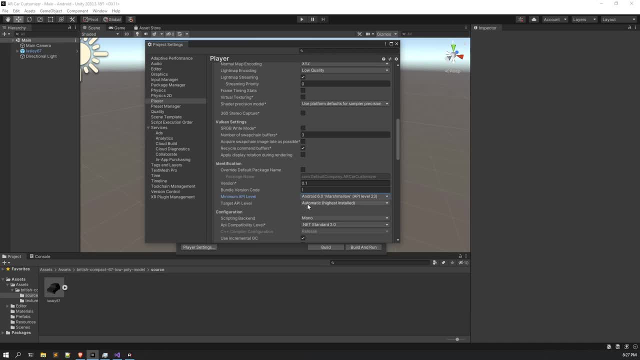 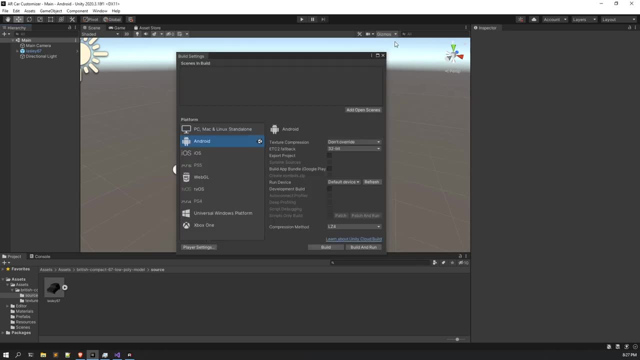 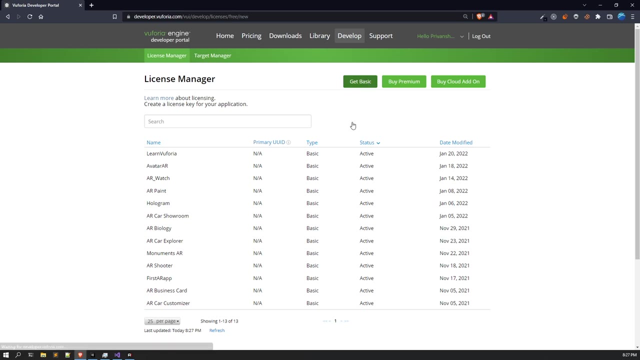 target api level, sorry, minimum api level you want? all right, and leave the target api level to automatic highest input. all right, so, yeah, that's what you have to do. uh, so after this, what you have to do is you got to go to the license manager. all right, click on get basic and create a new license. 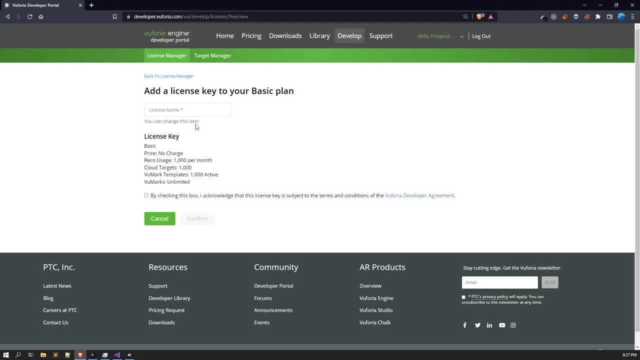 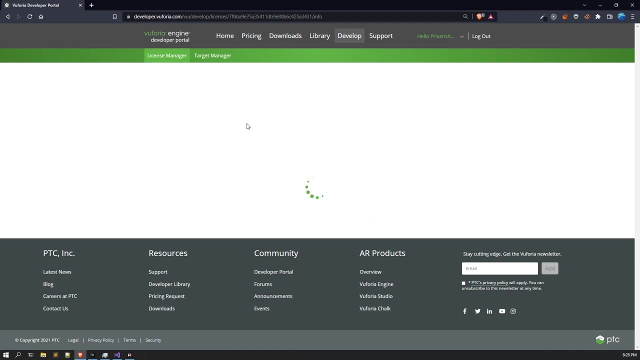 all right, so give this license a new name, that is, i'm going to give it ar car. all right, and click uh, click on the checkbox and click confirm, all right. after that, uh, open this ar car license and what you have to do is you have to copy this license. all right, you have to copy. 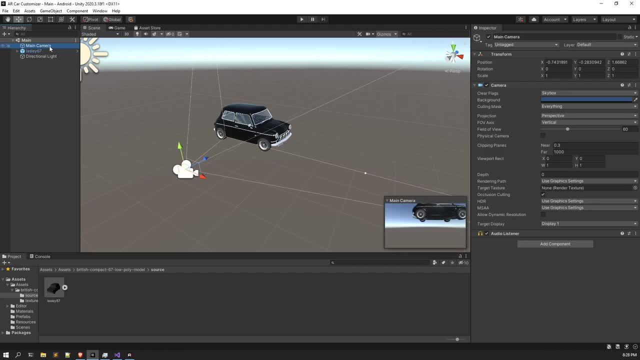 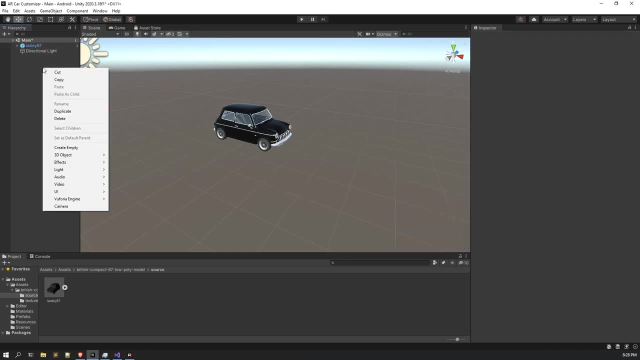 this license and go to a unity editor. then one more thing: delete this main camera, all right, in the unit editor. uh, delete this main camera because we won't be needing it. uh, now, right click view for your engine ar camera, all right. and one thing i prefer the most is: 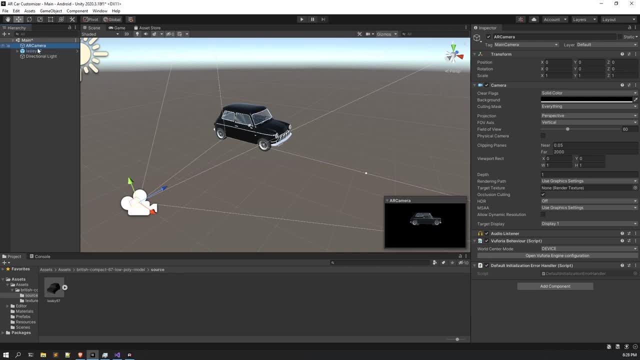 to put the ar camera on top of everything. so after you have done uh setting up the ar camera, what you have to do is uh in the in the inspector tab. only you will get the properties of ar camera, and in the ar camera you'll be finding open view for the engine configuration. 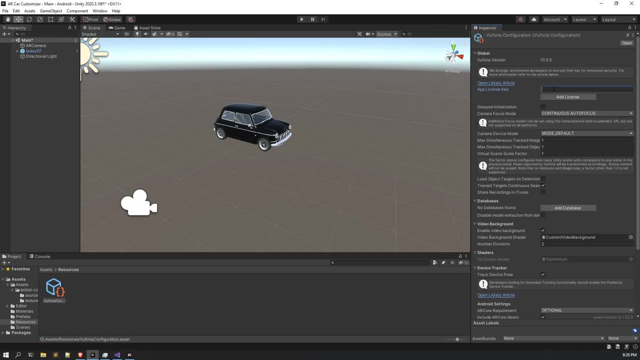 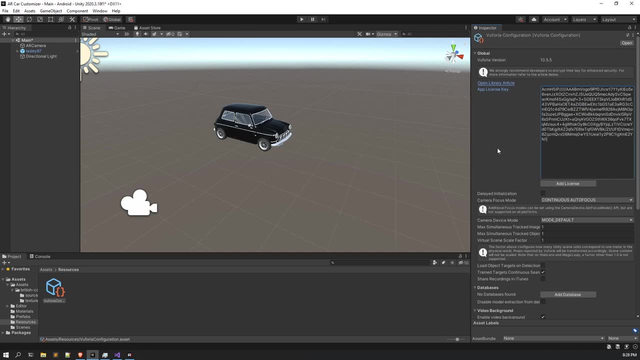 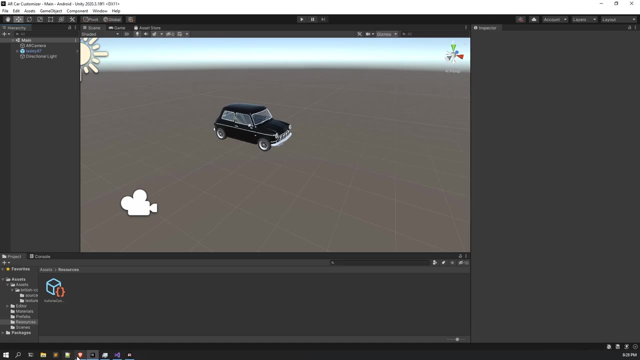 right, and in here you'll be finding app license key. so click on this blank box and just paste the license. all right, just paste the license and you would be good to go right. so, uh, our basic project is set up right now. we have to create a database, so click on target manager. 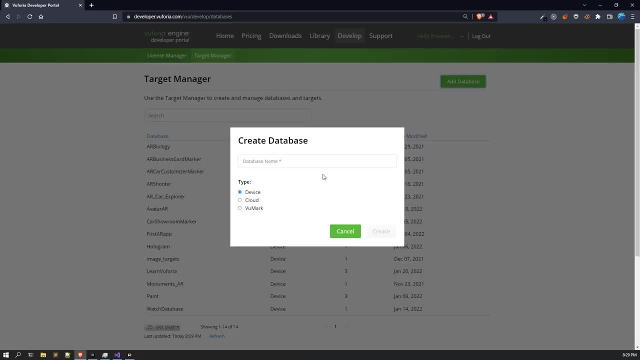 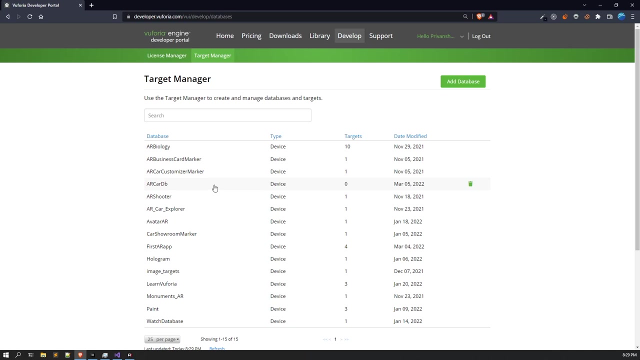 all right, click on add database. give the database a name. so i'm going to give it ar car db, all right? uh, i mean, make sure that the type is device and then click on create. so, after it has created a database, open it. now what you have to do is you have to add a database and then you have to 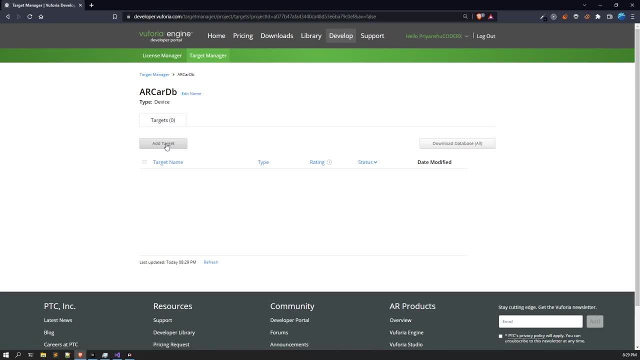 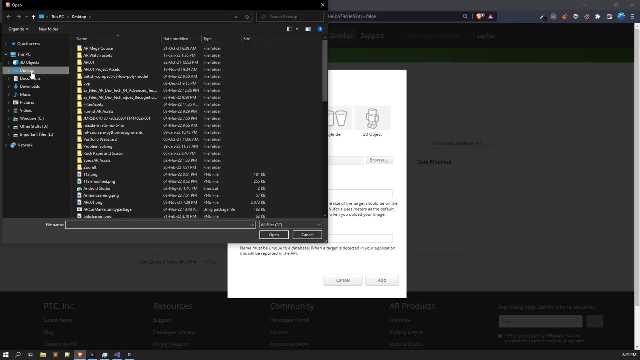 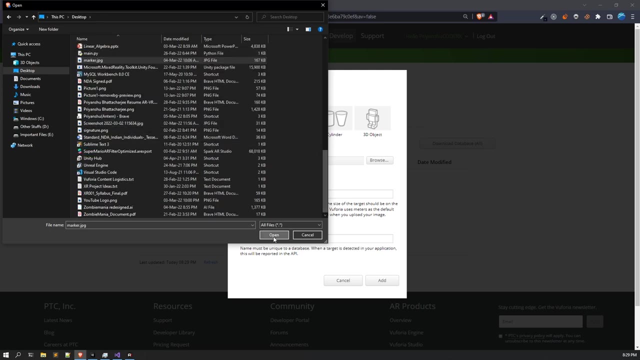 add the target marker. i already have the marker, all right, so you can select any marker you want. so i'm going to select the marker now. let me, uh, find the marker. okay, got it now. give it a. give it a width. i'm going to give it a width of six, all right? 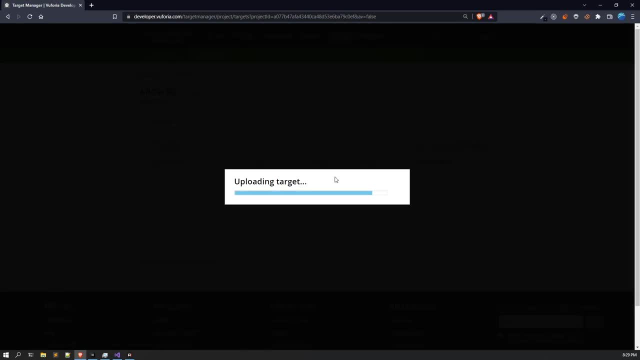 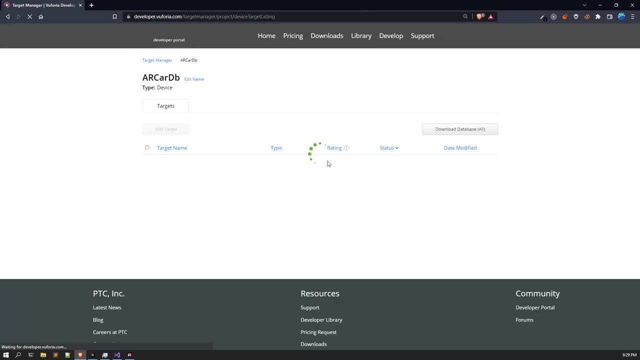 and i will keep the name marker on right, so just let it upload. uh, upload the name and position it. as you see. it's working just fine. so now let's move on to the next step. uh, let's upload that marker, and after that what you have to do is you have to download the marker. 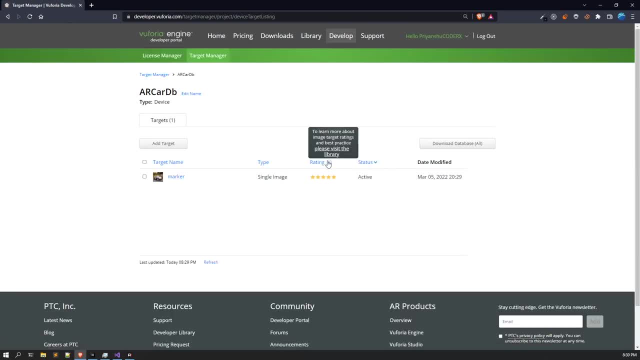 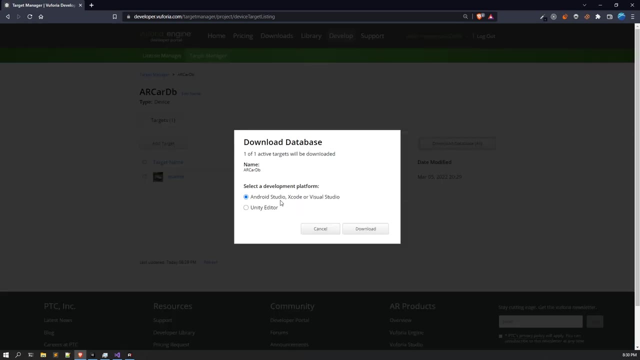 so that we can upload it on our unit engine. and one more thing: always check that. what is the rating, that is, the augmentable rating of your marker, and make sure it has four, minimum four, all right, it should be at least four to five, not less than that. all right now click on download. 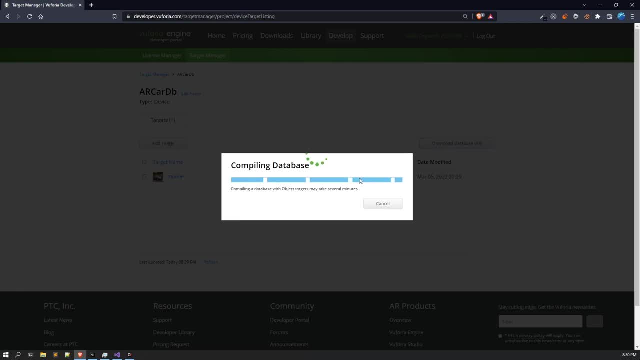 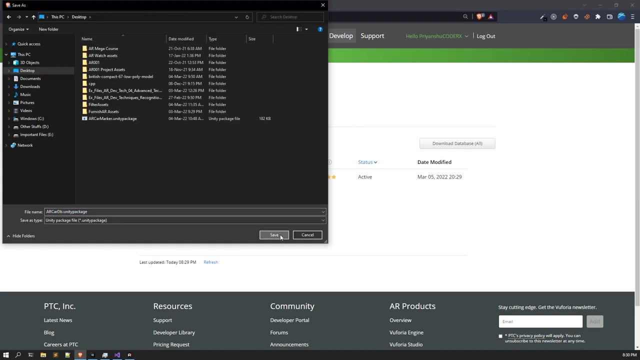 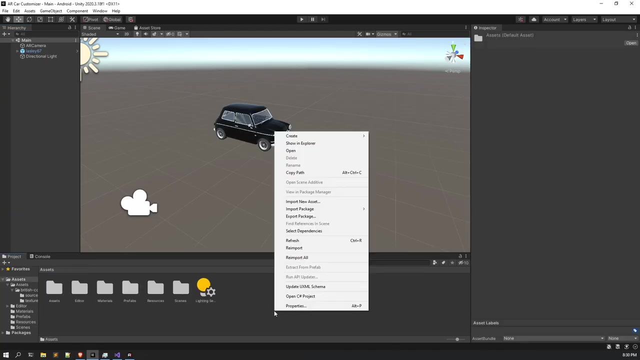 database and select the unity data and click on download. all right, so it would start downloading the database. now save this database somewhere in your desktop and import it. all right, so right click. you can either drag and drop it in here or you can right click import package- custom package. 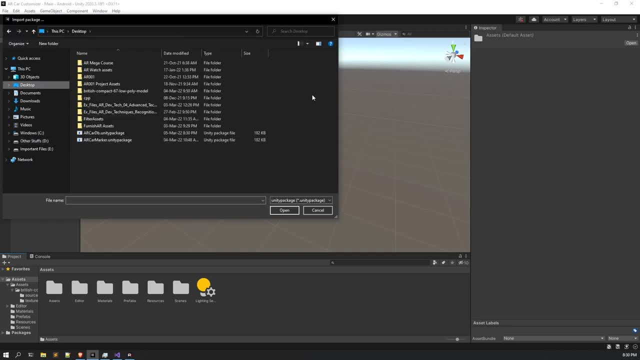 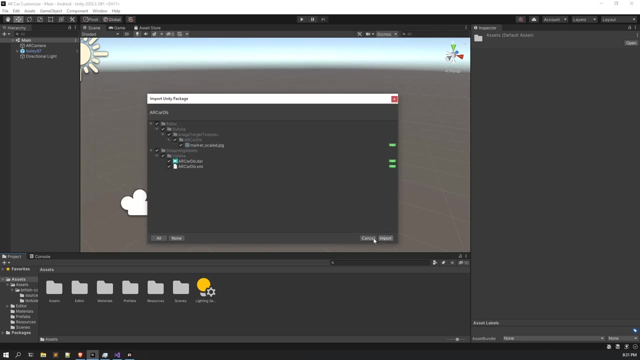 all right, you can do that, so i'm going to follow the second one now. click on ar card db- all right. ar card db- unity package. this is the database i downloaded- and click on open and it's going to take some time to process- and it did the processing- and click on import- all right, so it's going to take. 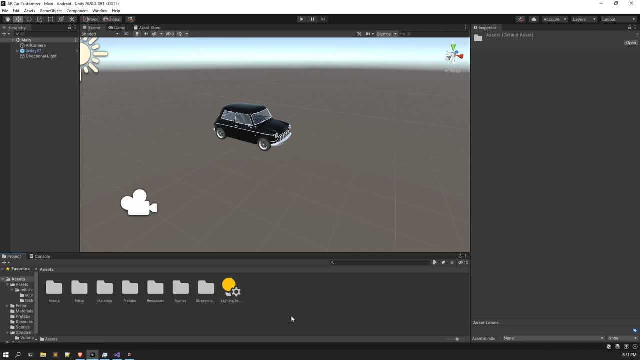 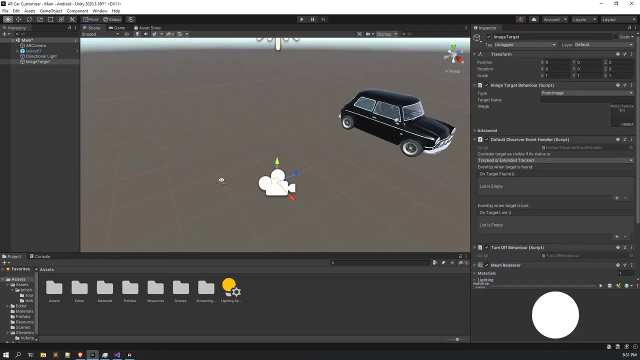 some time to import the assets and wow, cool, so our asset is also imported. right now, what we want to do is, as we already have imported our car model, what i wanted to do is right click before engine image target. all right, and in the image target you will be finding, like in the 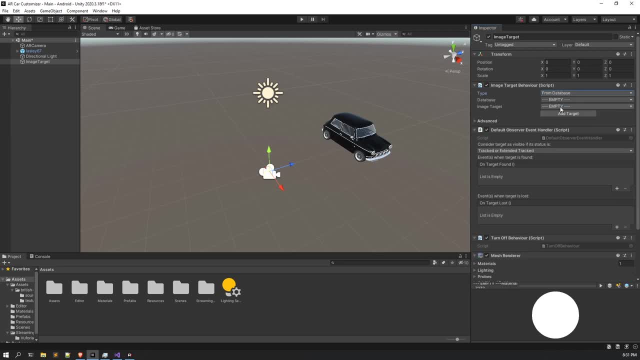 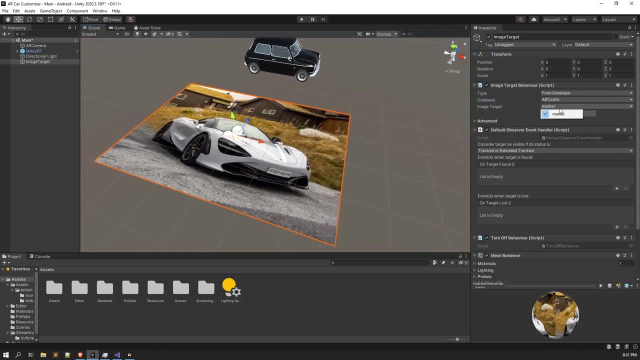 inspector menu you will be finding image target behavior from the type select from database. all right, and in there select the database and your marker will be automatically selected. if you have more than or to mark one marker, that is, two or three markers, then you you can select it from there. 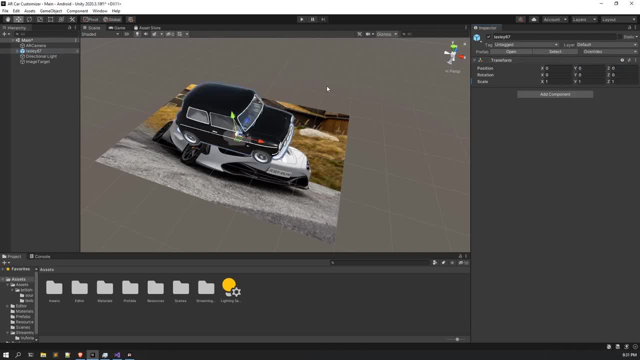 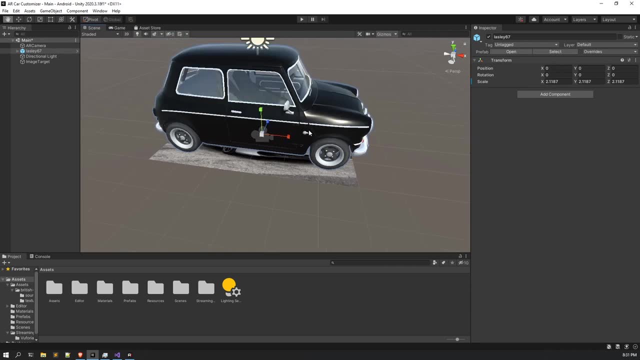 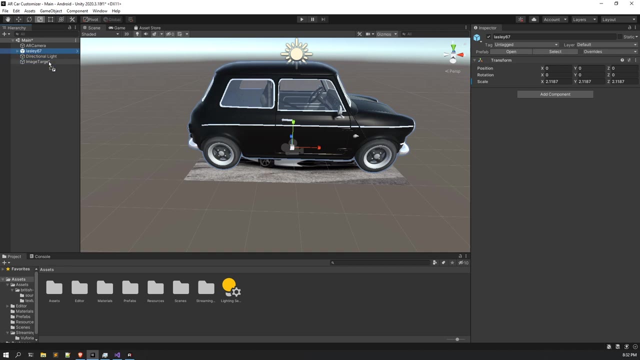 the database. i'm going to like reset the transform again so that i get it in the center of the card. now i'm going to increase the size of the car, all right, so that i could uh match the ratio, all right. now, uh, what i have to do is i have to put this car uh means make this card a child of the image. 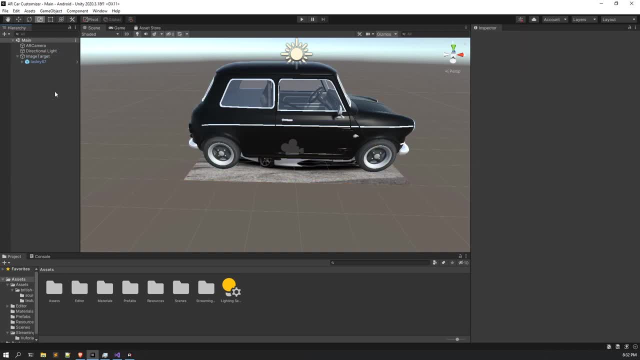 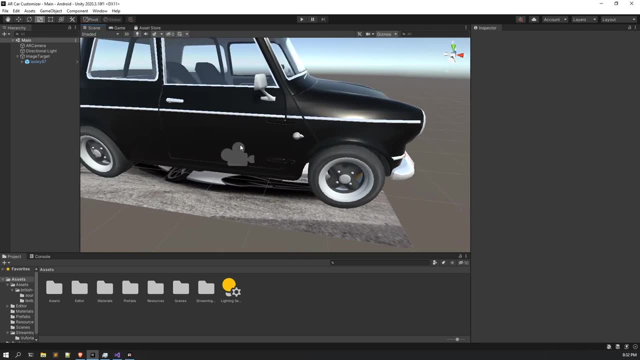 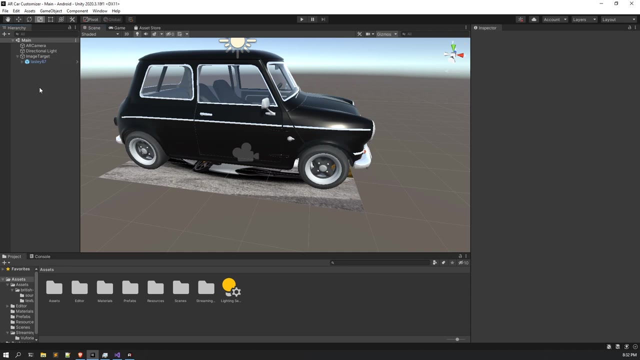 target right and uh, now we are good to go. our markerless- sorry, marker based ar app is set up, all right. now what we have to do is we have to uh code. all right, we have to code our means. we basically have to code what are the functions we want in the app. so for now, we 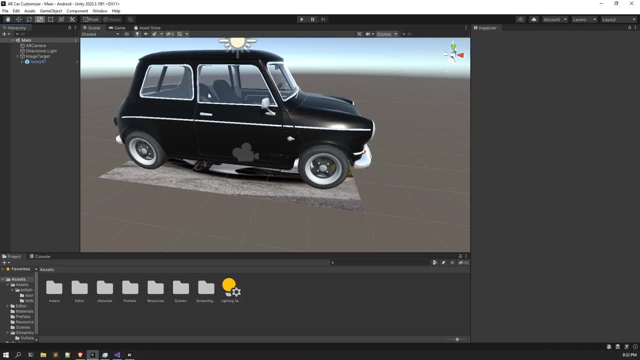 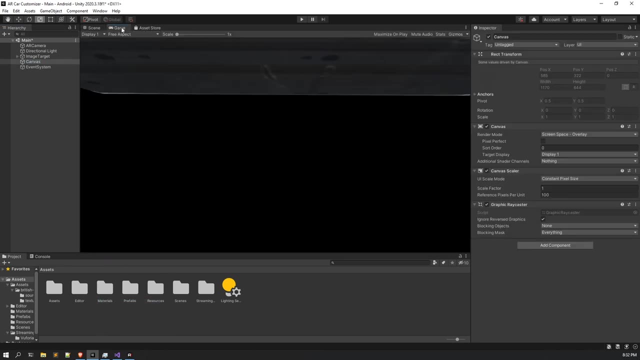 only want to change the color of the car. already that is the material color of the car. so first of all, i want you to create the ui. so how are our going to do that? it's pretty simple: right click ui, um, then canvas. all right as uh. this app is in. 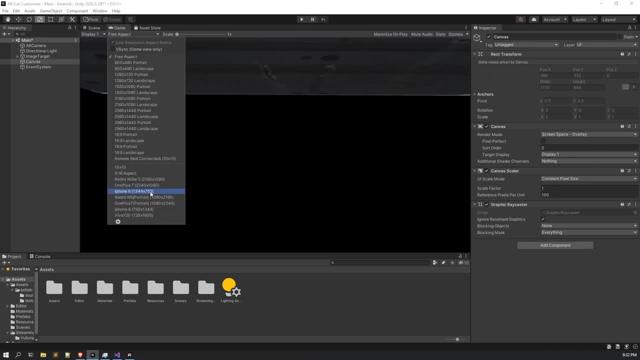 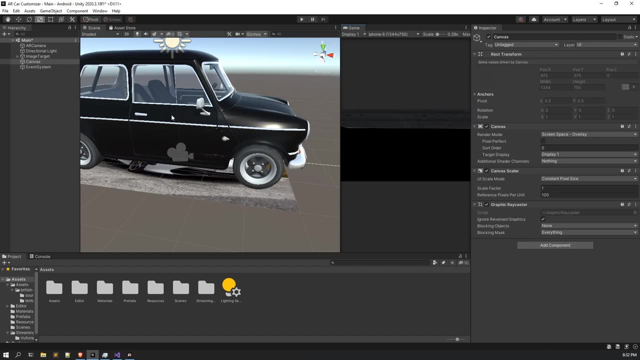 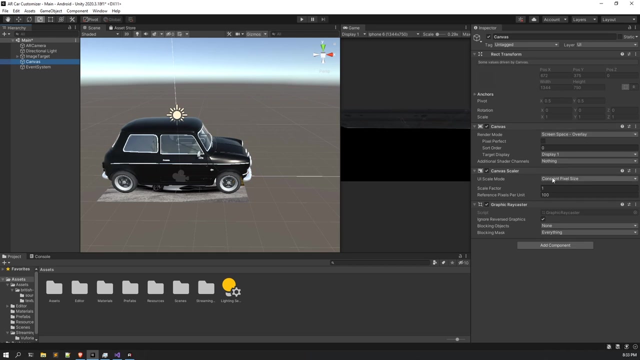 landscape. what i'm going to do is i'm going to choose the medium resolution so that we could, uh like, easily remake our app responsive, all right, and put it right in here. now, after i've created a canvas, you can see that there are multiple options in here. you can say canvas. 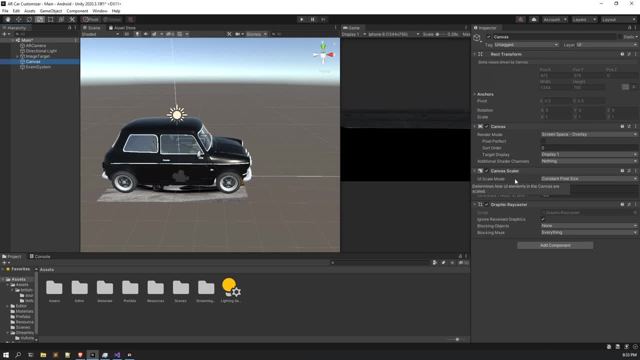 killer option is there in. there in the ui scale mode, uh section, you have to choose. uh choose scale with screen size, all right, and uh leave it there only. all right, because that would actually help us uh to make the ui more responsive, all right. now what you have to do is uh add some buttons, all right. 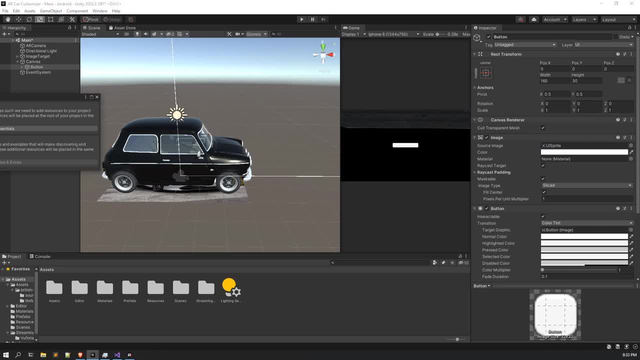 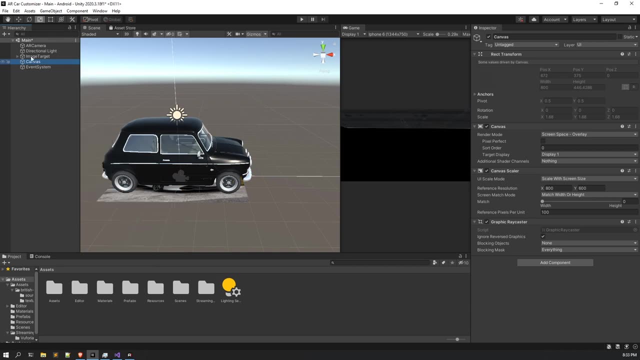 uh, click on button text mesh pro. all right, so it would like prompt the importer. you can import it. i don't want it, so i would be going with the normal buttons only. all right, i would like to go with the normal buttons only. uh, actually we won't be needing the text, so that's why i'm going with. 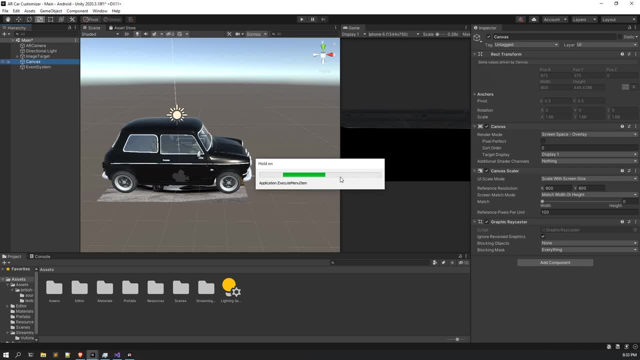 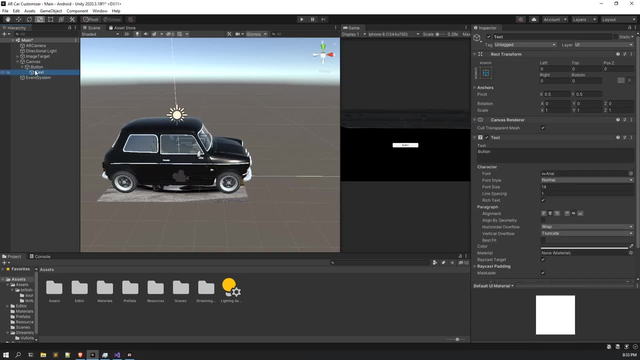 the normal buttons, but what i would suggest you is to: or, if you are going for text based buttons or something like that, all right, or even buttons in general, i would suggest you, or to always go for text mesh pro, because they are thousand times better than you know the other buttons, so give it. 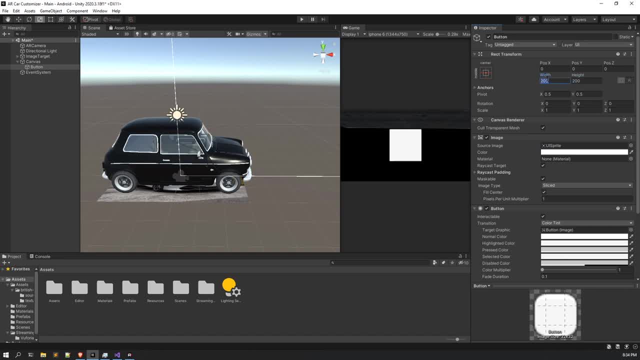 a width of 200, all right, or let's not give 200 search too big, let's give 100 only, all right? uh, yeah, now what you have to do is in the rect transfer mode only in here you'll be seeing a small box. click on it. click, uh, alt, all right, just to wait. 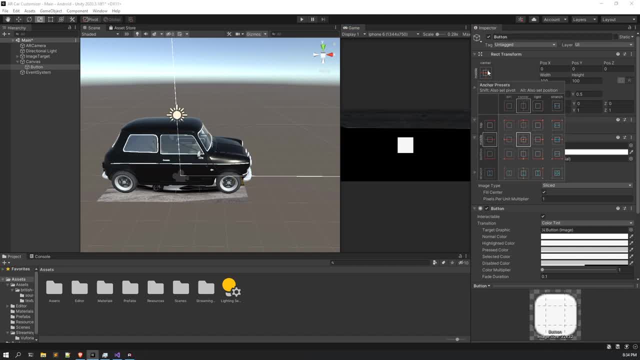 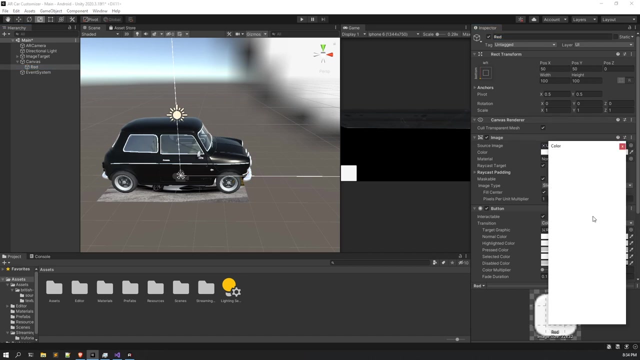 okay, now what you have to do is click alt in here or just do it all right. now what you have to do is, after you have done that, give it a, give it a name. all right, let's give it name. I want to name it red. all right, and let's give it a red color. 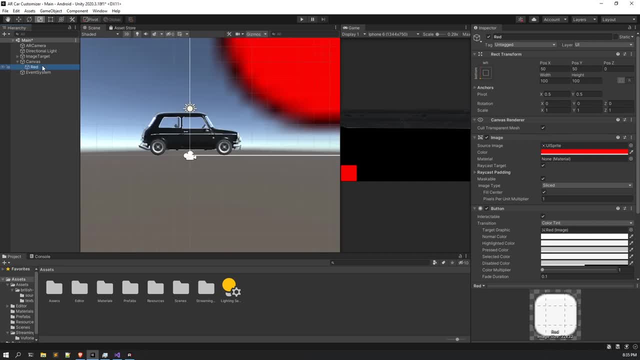 all right, and make sure you are in 2d mode, because we are going to edit this UI. all right, and duplicate this button. all right, duplicate this button and move it right and in here now give it another color. that is, let's say, I want, I want. 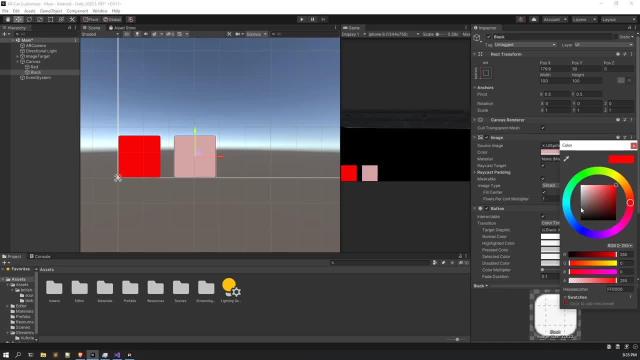 black. right, let's give it another color. that is black. it might not be that visible, so I'm going to make it a bit like this kind of black, so that it becomes visible. all right, now here, give another color. all right, let's let's give it blue. all right, let's make the color blue. okay, now let's give on the color. 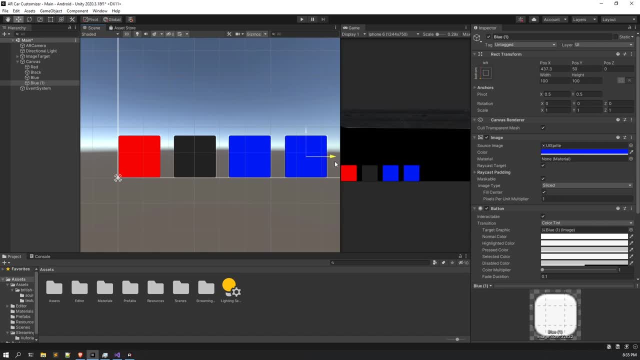 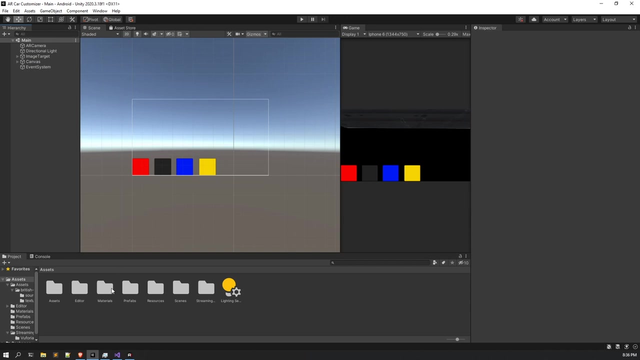 that is yellow. all right, okay, all right. so we have our UI prepared. right, we got our UI prepared. we have all. we have prepared- our buttons. now what we have to do is we have to code right, the very first thing. all right, the very first thing I would like to do is I would be coding a script. 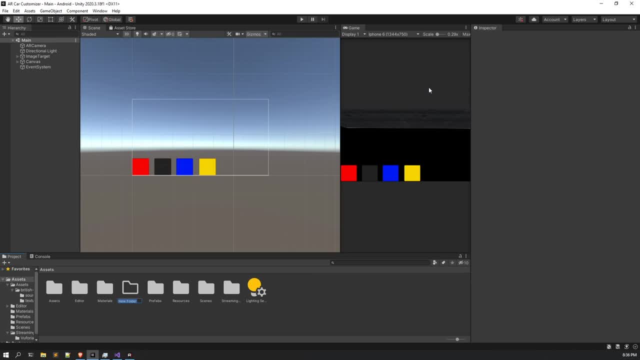 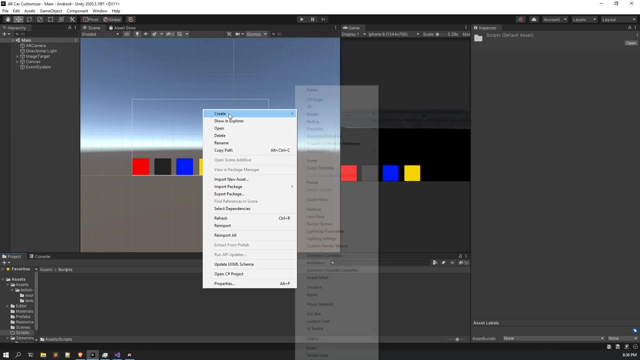 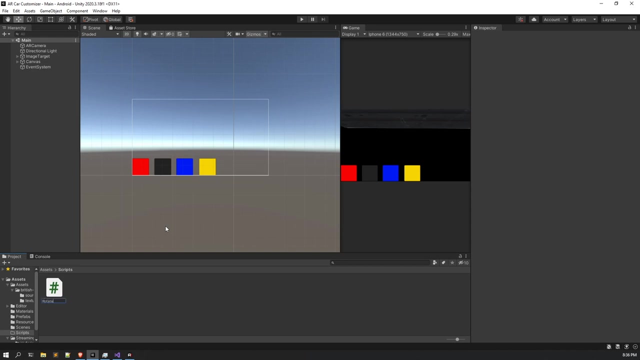 to rotate our car, all right, so that it rotates continuously. and to do that, uh, first of all, what I have to do is I have to just create a folder, scripts folder, all right. and then click on create, then again C, sharp script, and let's give it a name that is: rotate, all right. so I want my car to rotate, actually. 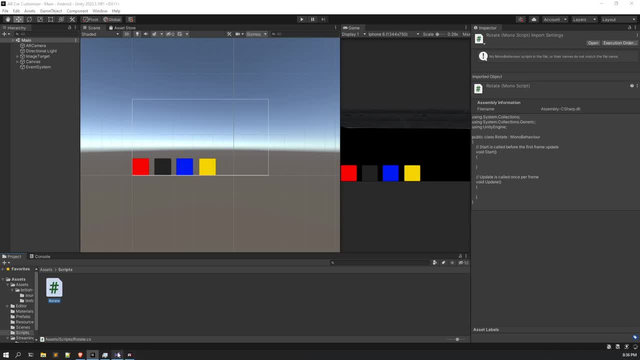 now it's compiling the application, all right, okay, so give it a few seconds, okay, so, all right, it's taking a bit time, so let's give it its time so that it is able to do the processing it needs to do. all right, so our script is, uh, perfectly compiled. now I'm going to open the script in my Visual. 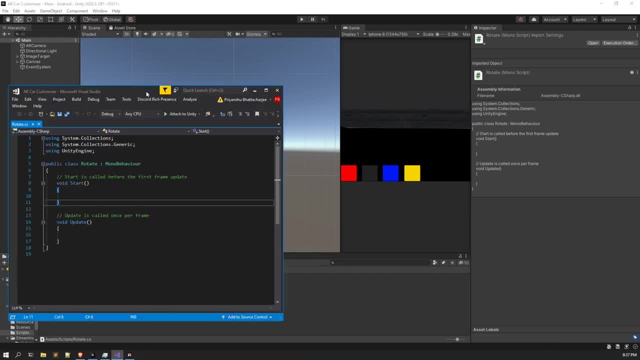 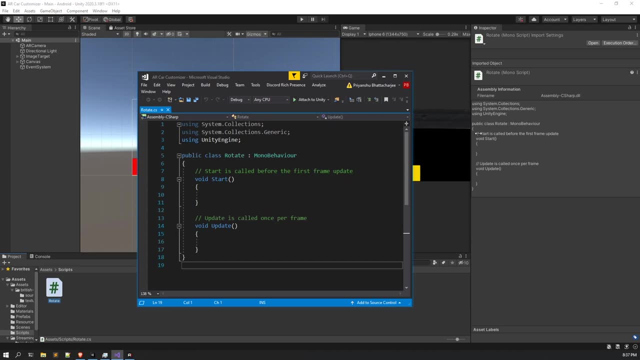 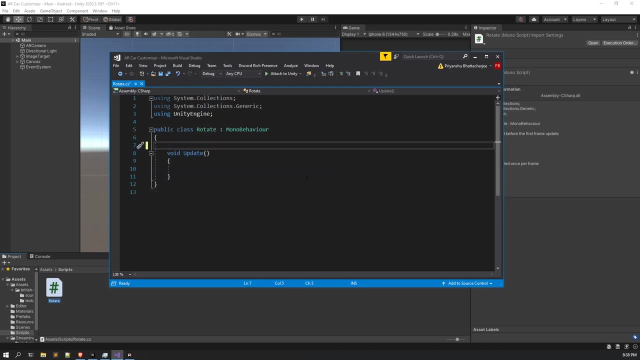 Studio editor. all right now. okay, here we got our editor. all right, I don't want it to be in full screen mode as of now. so, uh, remove the whole start function and comments. all right, we need the update one. so first thing is you have to create a vector 3 variable. all right, vector 3, let's name it rot. all right, and what in the update? 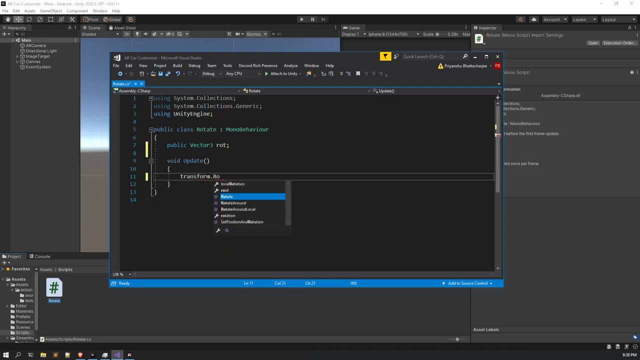 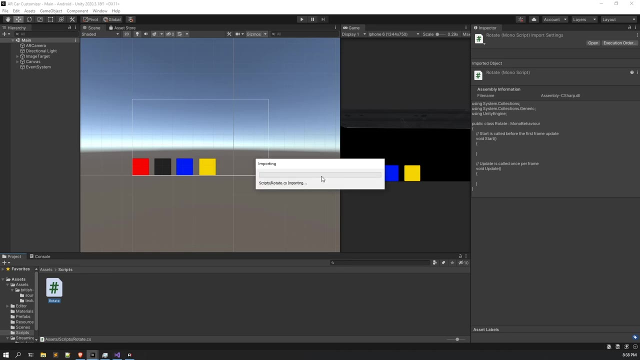 function. only. what you have to do is Transform dot rotate- all right, and pass this roll to variable in there and multiply it with time dot Delta time- all right. now save the script and let it compile in your unity editor- all right. so after it is compiled, what? 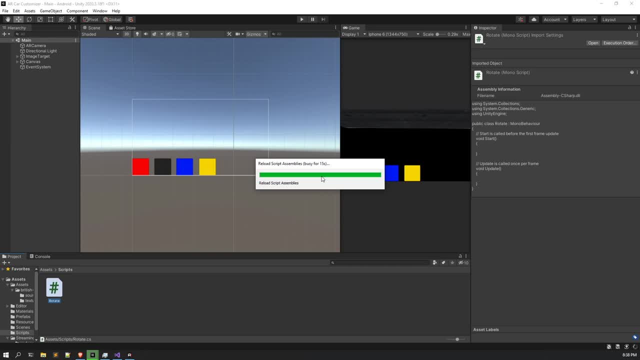 you have. what we have to do is we have to put it in means inside our car model, all right, that is, we have to attach it as a script in our car model, all right, so that we could use it right. and all right, now go to the image target. all. 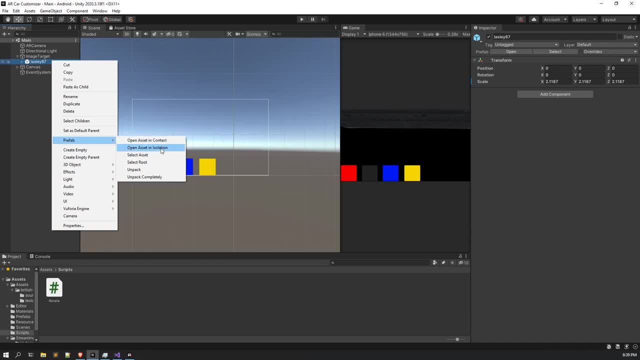 right, and first of all unpack this whole prefab. all right, after unpacking, what you have to do is drag and drop this rotate script in here and in in the rod value. give it a value of 30. all right, it would be like moving and rotating at the speed of 30. all right. now what you have to do is: 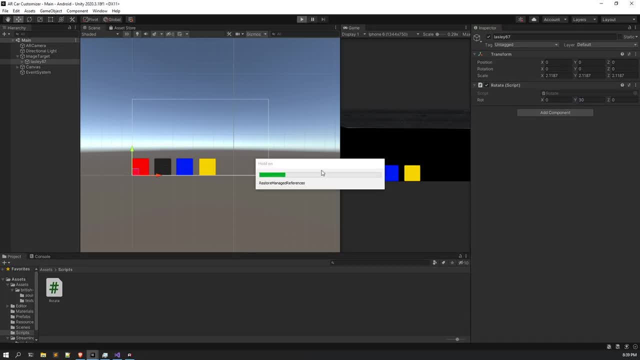 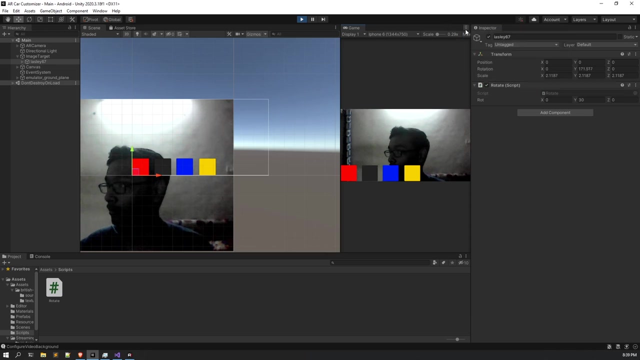 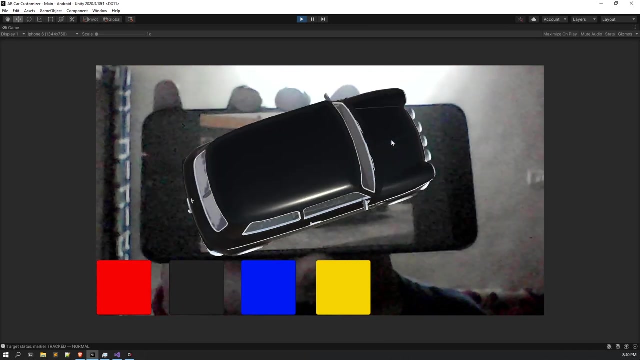 play this? all right, play this particular scene and let's see how all things work. right, so, just give it a few seconds. so just a few seconds, and we would be good to go. all right, okay, cool, let let me maximize it. okay, cool. now see, our car is rotating. 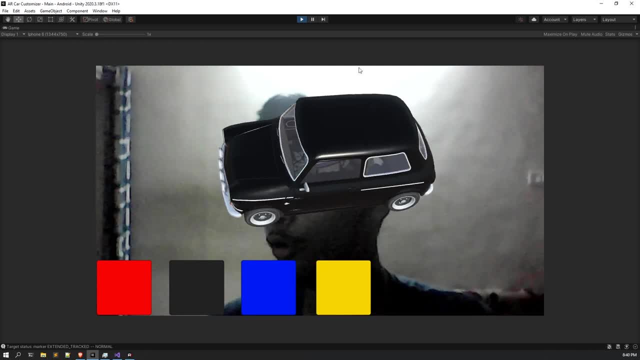 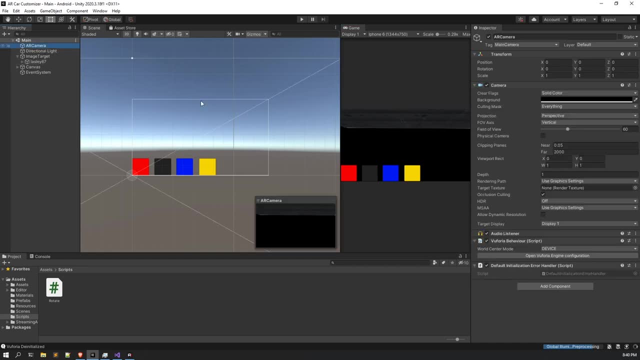 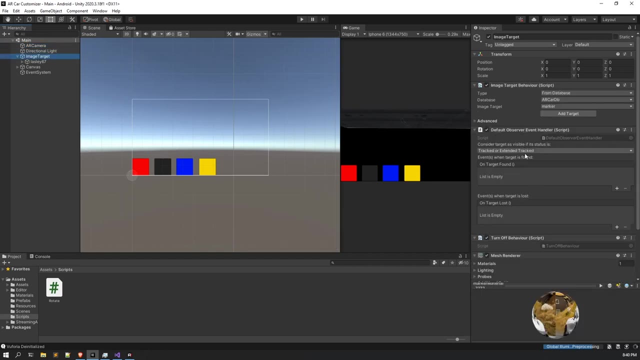 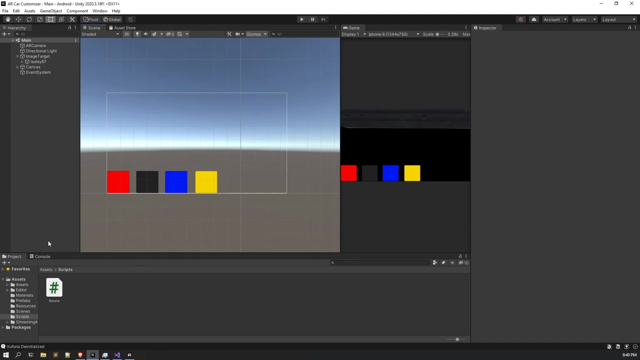 all right, and that's pretty good, all right. oh, one more thing: extended tracking feature is on, and of course we don't want that. go to AR camera- all right, sorry, not AR camera. or click on image target: all right, in here, select tracked, all right, and we'll be good to go right. so now, as our- basically our car means we have 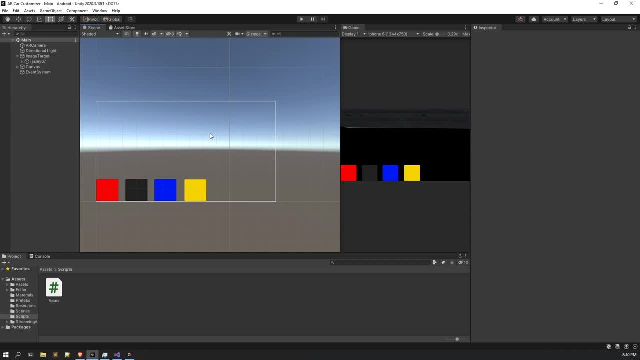 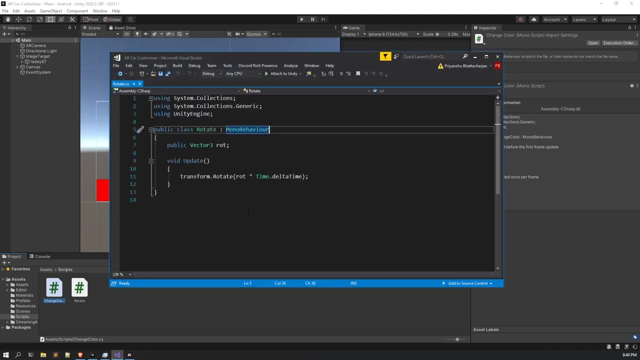 created our car model, right, as we have created our car model. now what we have to do is click on create C sharp script. all right, and let's give it change color. all right, so that's it. we could change color of our car after clicking some particular button. all right, so just wait. 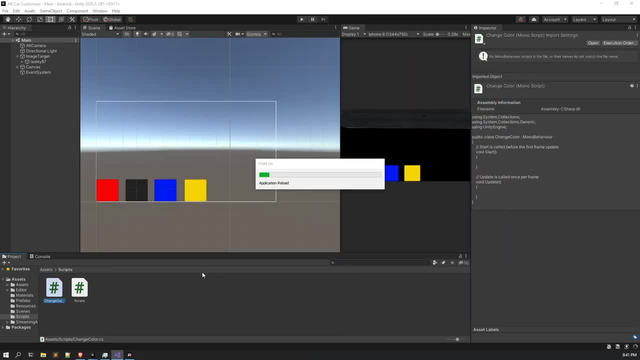 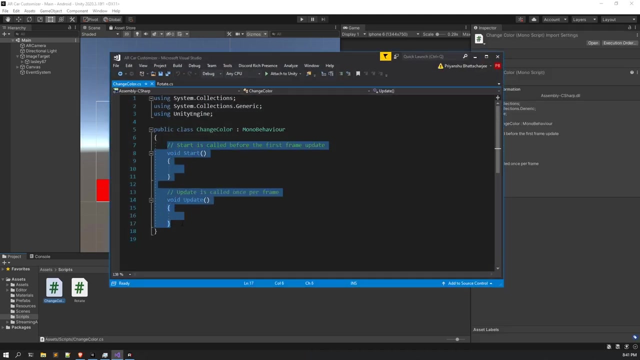 it's compiling the script. all right, just wait a few seconds. all right, let's open the script in our editor. okay, cool. now what I want you to do is create an array. all right, that is a line renderer, so not line render area. just wait, public. just. 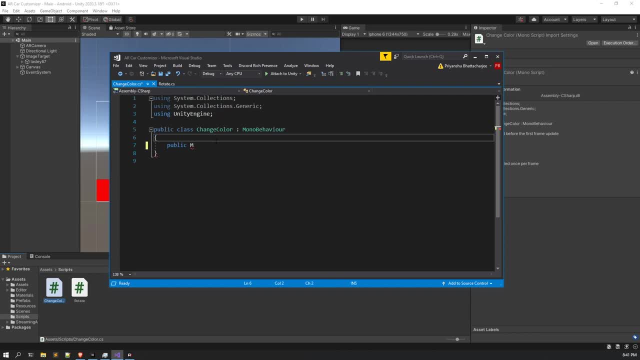 give me a second, all right. so what we have to do is we have to create a array, all right, of, first of all, uh, create an array of colors, all right, so that we can store the colors in here now again. create another array of renderer, that is, it will help us to get the renderer of. 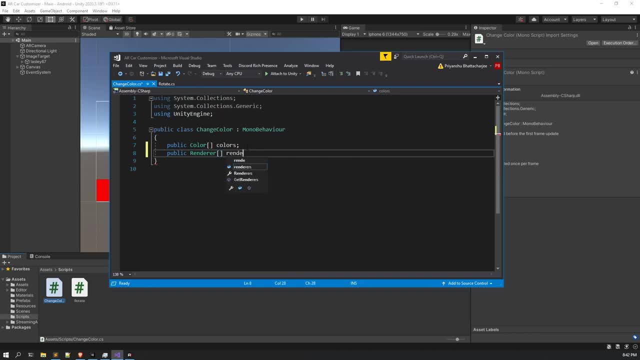 our car material. uh, there's a reason why we are. there's a reason why we are actually creating a renderer, all right, uh, there's a huge reason- means not exactly a renderer- uh- why we are creating an array of renderer. and you know, just wait, let's name it uh, mats. all right, now. there's a reason why we are doing that, because 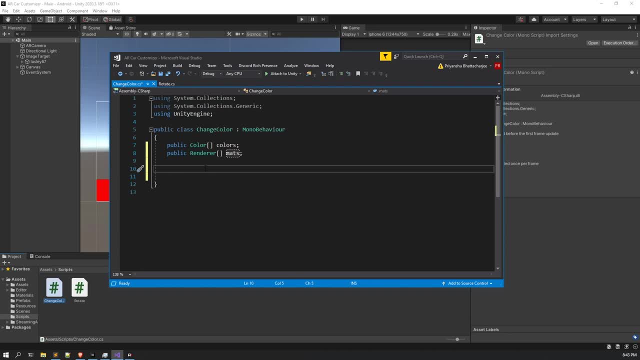 see, a car might have multiple materials in it. all right, that is, a car might have multiple sections in it where there will be different. different materials will be like applied right. so that's why we are creating an array, so that we could include all those uh sections in our, you know, in our model only. 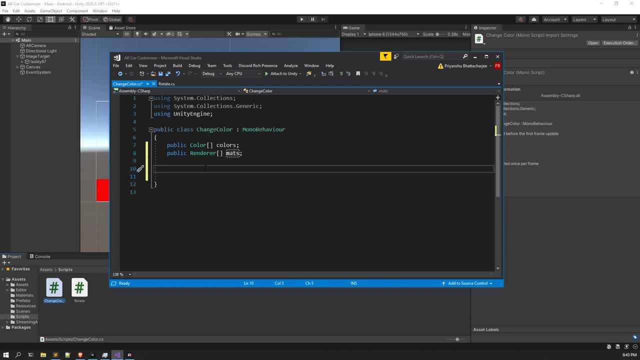 that is in our script. only right now. let me show you. what you have to do is record public void- all right, and write a method or function, all right, called red. now make it public so that we can get it on our inspector menu. right now we have to run a loop, all right, that is. 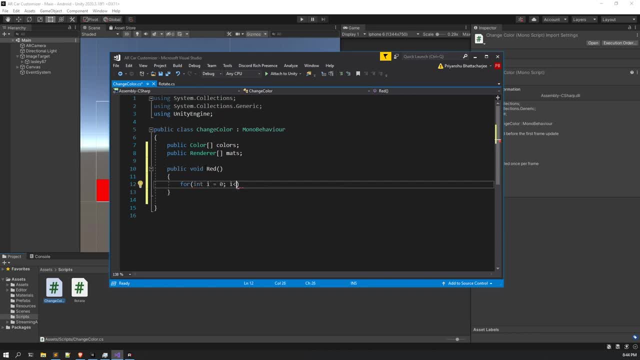 for ntie equals z. let's write some commands so it is running in this way. it's running from zero i less than maps dot length. all right, it would be running from zero to, that is one minus the actual length of the material. all right, and yeah, now you can. you can either open the brackets. 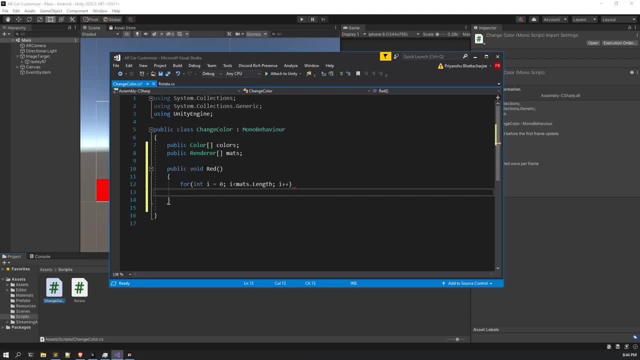 or you can simply write it like this: let me show you all right, because if it's, if it'sa one liner, all right, you don't need a bracket, and currently it's a one-liner. only. now what you have to do is mat, mat of like I we. 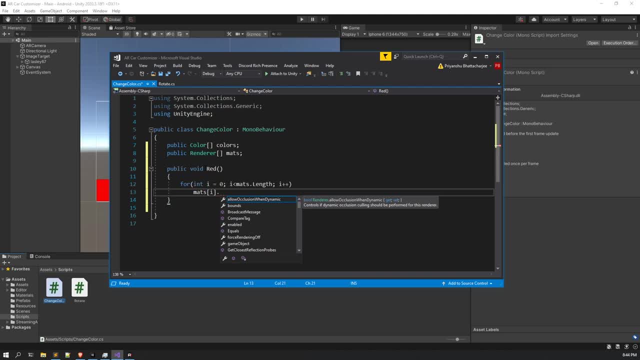 have to give it, take each and every, like each particular material and apply color to it. so mats of I dot material, dot color equals. so you can, what you or what you can do, is just wait. colors: yeah, we got the variable and give it the first, that is the first value of all the colors. alright, now copy and paste. alright. 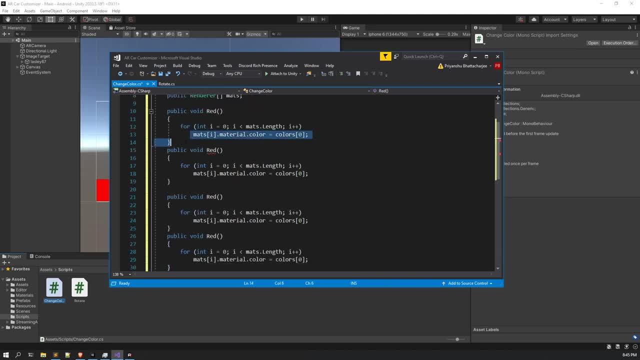 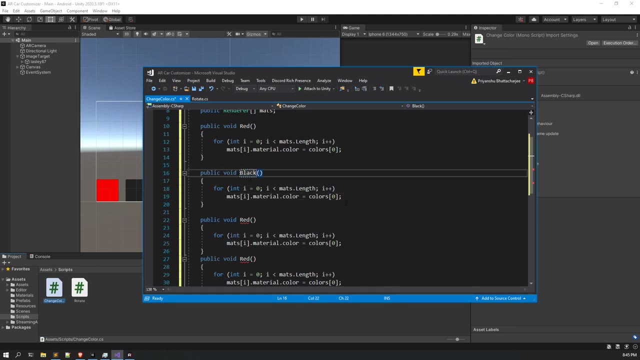 copy and paste it so that we can basically replicate it. alright now, blue, alright. or let's say, which was our second color in here? okay, it was black, right, let's give it black and let's give it one, all right. then in here, let's give it blue, because it was our third, and give it two and yellow. and do you know why we? 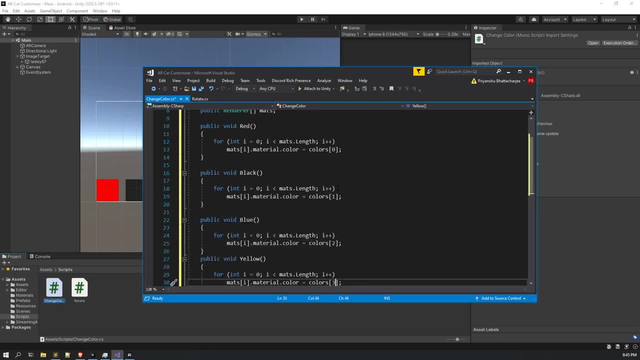 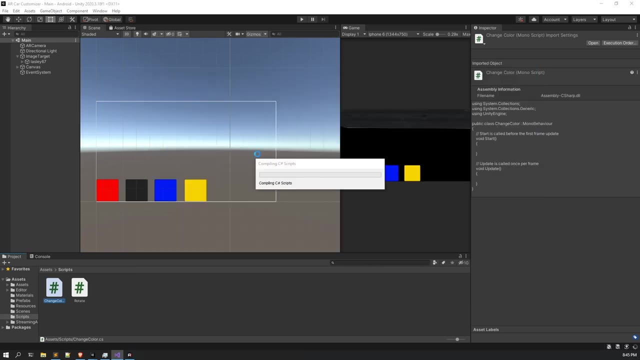 are giving like first index value as zero, then one, then to the second we are giving one, then to a third we are giving two. that's because indexing starts from zero. all right, so we have our script written. all right, i hope you understood. understood the script. now there's nothing else to do, we just 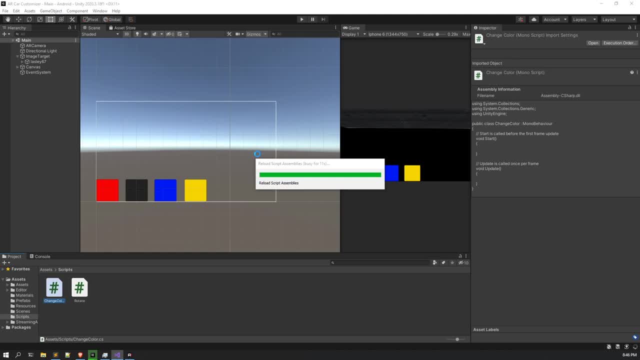 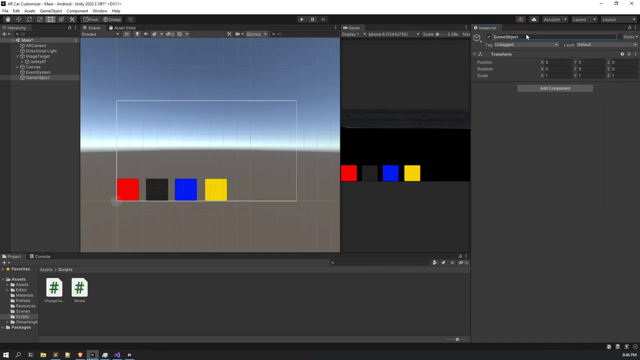 have to apply the script and the functions, all right, we have to apply to the variables, right, so yeah, so now what you have to do is create a empty game object- all right, you can do that- and reset its transform. name it, color changer, all right, and attach the script to the color changer. now what you have to do is you: 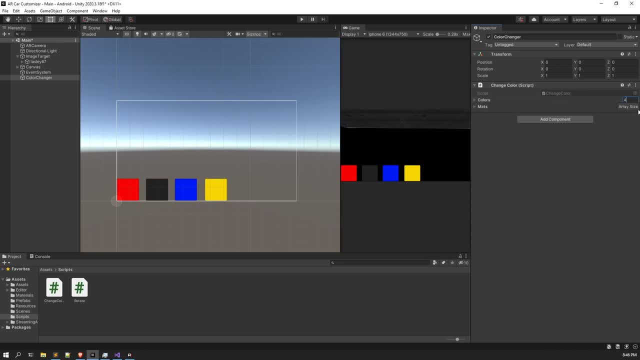 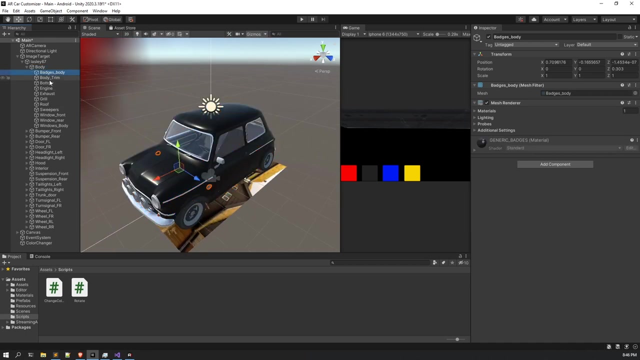 have to give, you know, four colors to it, give the array size four and how. let's see how many materials we have to give in here. all right, so basically, the body is there, all right now. all right, not this one, not this one, this one, this one. 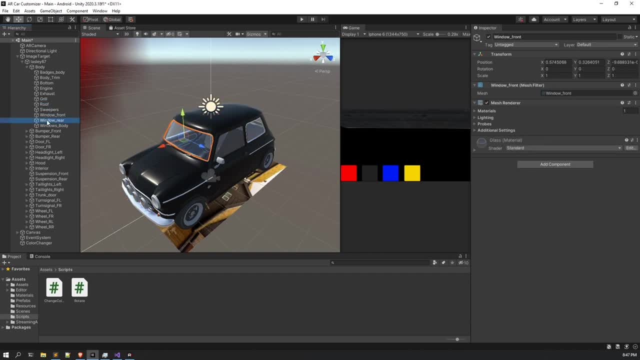 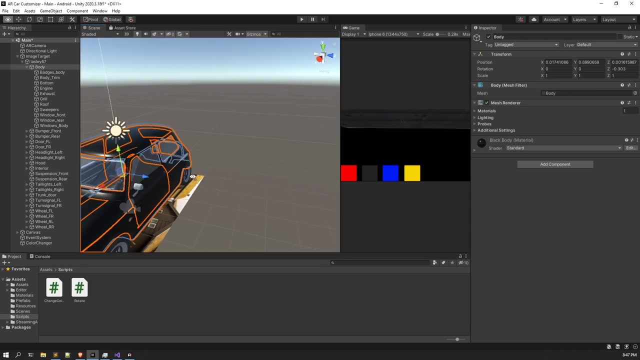 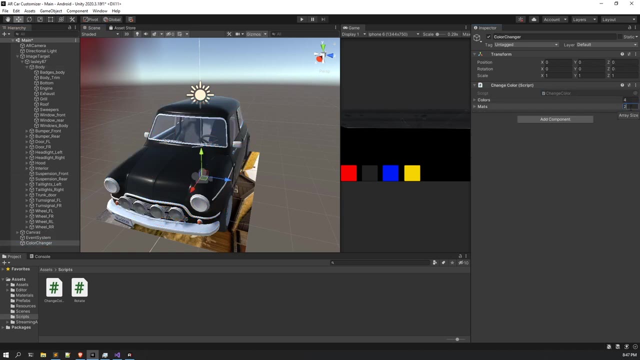 all right, this roof sweep, not sweepers. so window front, not this one, all right. so, uh, okay, all right, i understood, so go to the color change script. all right, and let's give it two as of now. all right, now what you have to do is get the body material in here. all right, the body is for the whole body, right, and 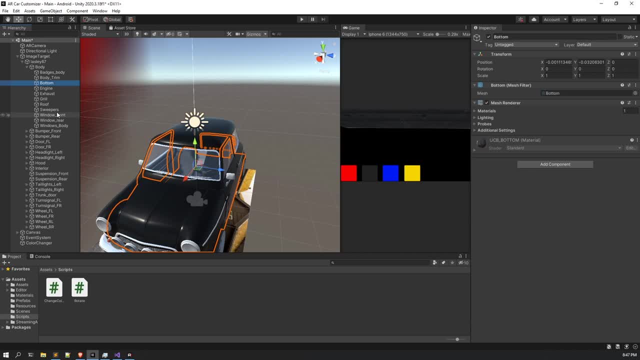 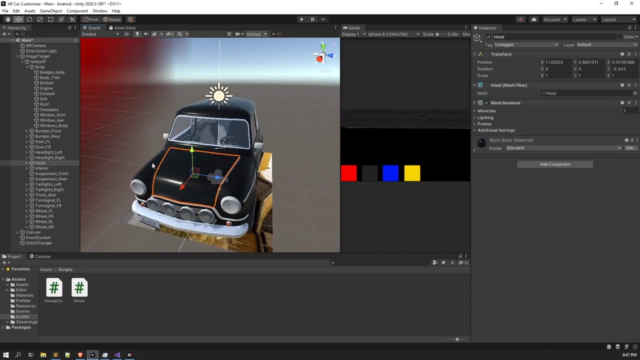 let's get the sweepers. that is no, sorry. the roof one. all right, let's get the. where is the roof? okay, yeah, we got it. so yeah, here we got the hood. all right, actually, there are multiple layers in it, so that's why, uh, that's why i told you to add, like, create an array of those materials right now. let's get the. 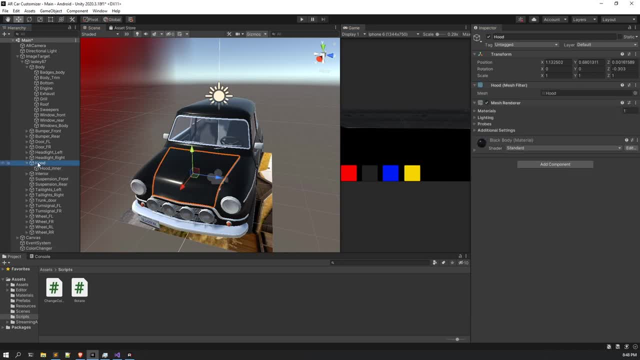 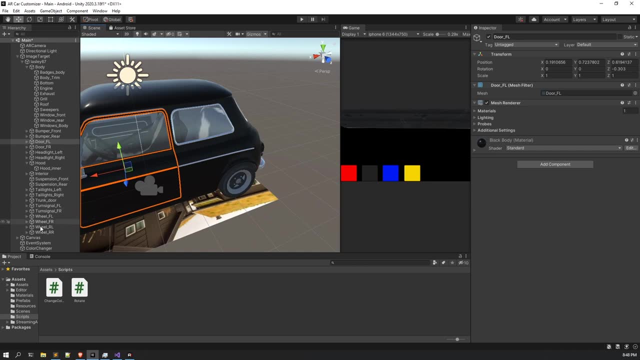 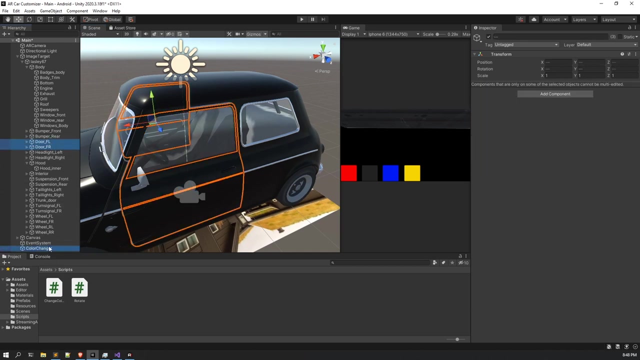 hood in here. okay, so we got the hood now. okay, the body is done, the doors right. uh, yeah, the doors. so go to the color changer. add another section, all right, and uh, let's give it the doors right, take the doors, all right, okay, just to wait. okay, okay, here we go another one, that is door fr. all right, now, now. 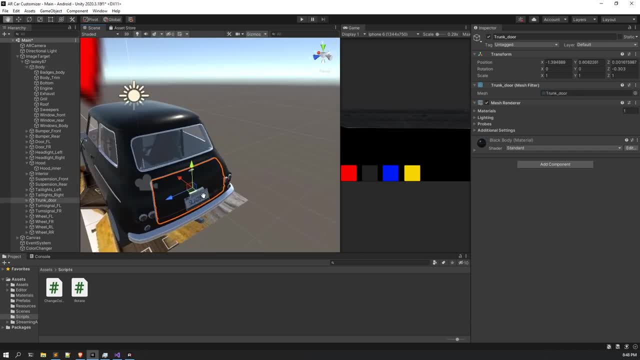 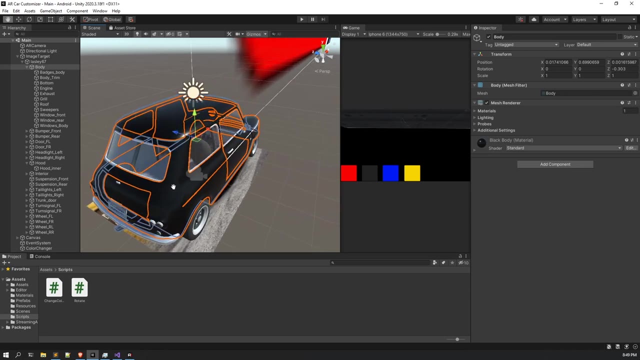 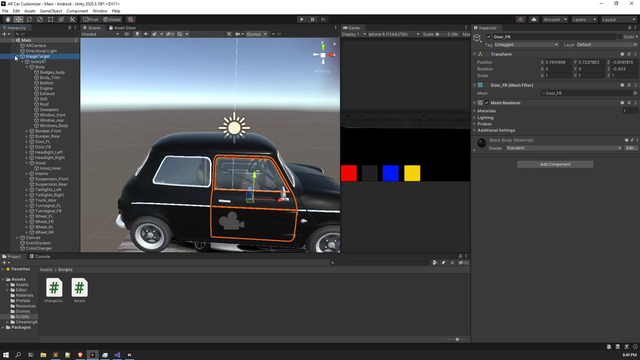 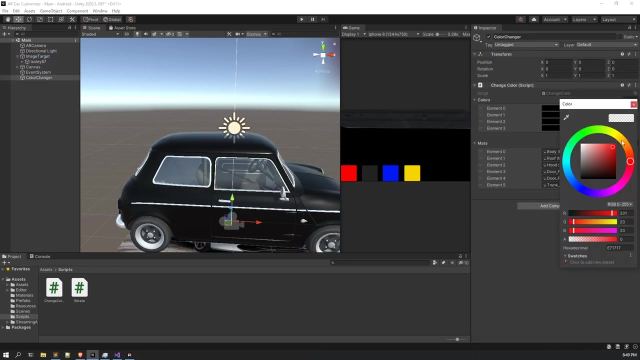 let's see what other things we have to give. okay, trunk door, right, let's give it the trunk door. all right? i hope not, nothing else is left. okay, no, i guess everything seems good, right, yeah, everything seems seems good, now, let's, let's see. let's uh, now let's give those colors. the first element should be red. all right, it should be red. 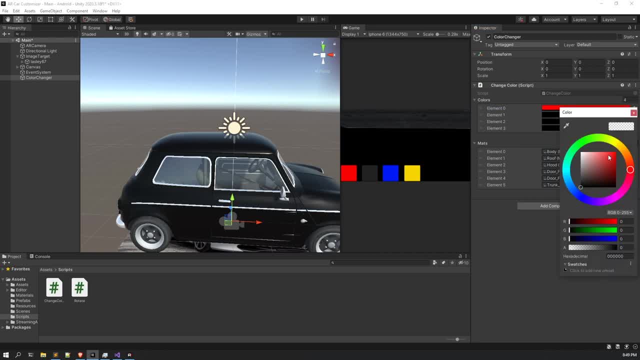 okay, the next, that is, the next one should be, uh, you know, black, all right now. the second one should be, you know, blue, let's give it a more. a bit sky color, all right, it would look good. and the next one would: should be yellow. right now, what we have to do is click on canvas, all right, click on buttons. 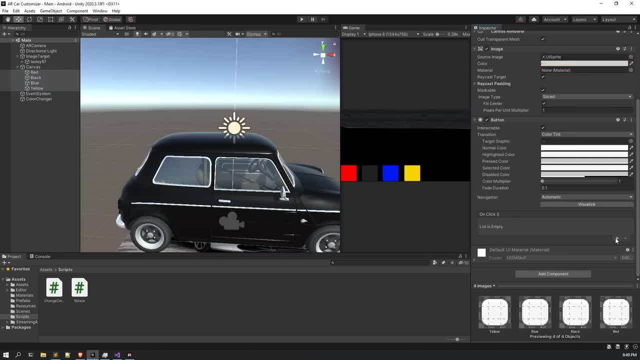 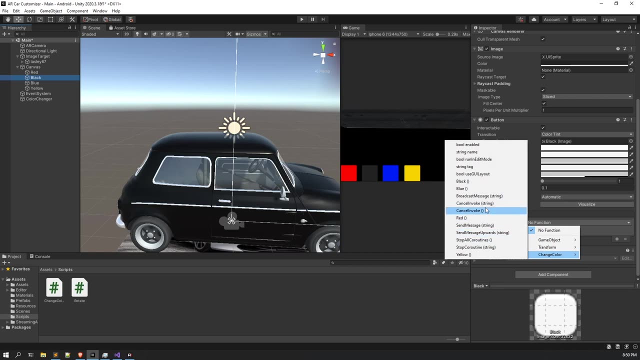 all right, first of all, uh select every button, uh add a plus sign in there and add the color changer script in here. right, what you have to do is uh go to a red button, click on change color, click on red, go to the black button again, or choose from the change color. then select black, then from the blue color, click. 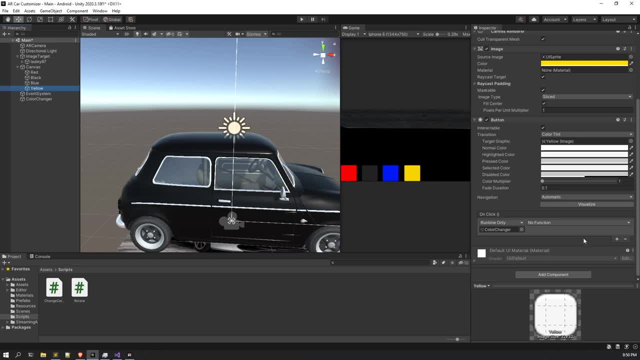 uh, change color, then blue, then from the yellow one, go in here, click on change color and click on yellow. where is it? okay, cool, now let's try our app. so that, uh, let's try our app and let's see, uh, how it performs. all right, let's see. so, give a few seconds and, uh, we would be good to go. 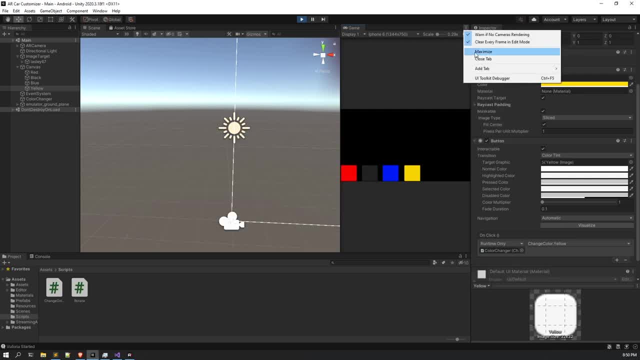 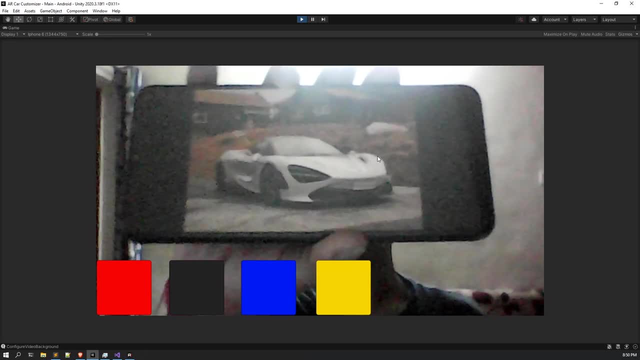 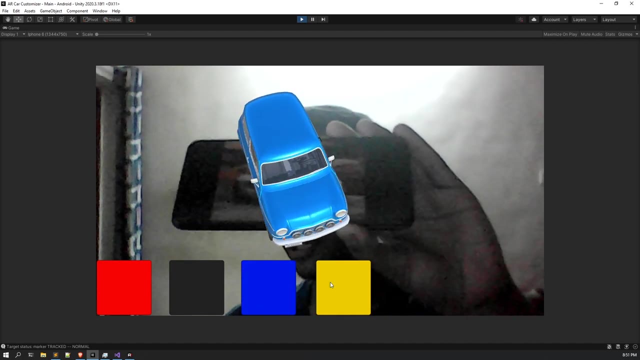 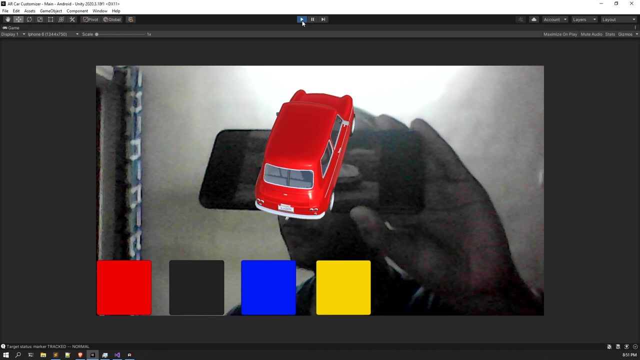 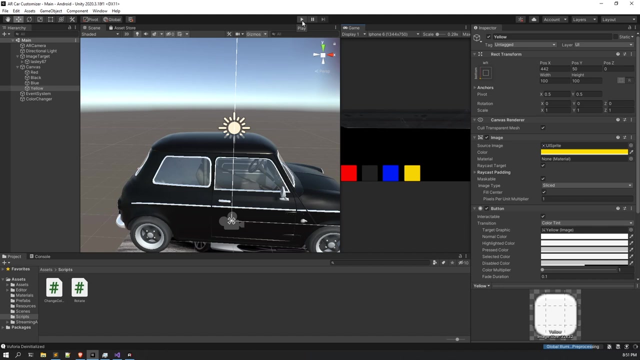 okay, cool, so let me maximize the window. okay, cool, okay, all right, cool, so we are able to see the car right now. let's try the color. wow see, it looks good. right, see, cool, isn't it? yeah, so our first project is done, actually, all right, uh, congratulations. you have created your first full-fledged application with uh viewphoria. 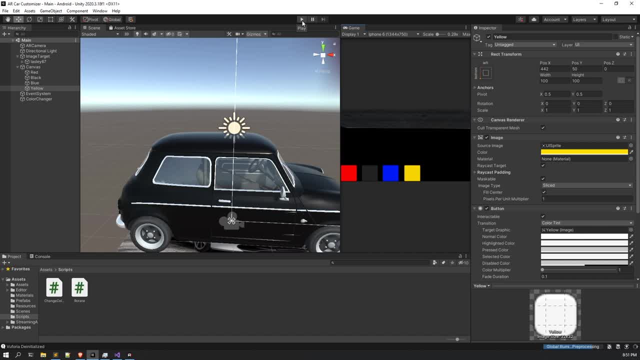 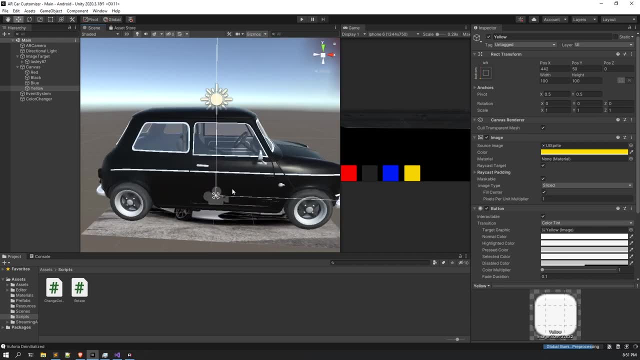 right, uh, let me give you some idea what you can do uh further. you can, let's say, you can add varieties of tires in here. all right, you can add uh numerous varieties of tires. you can add more colors- all right. you can uh like create your own own car model, or you can even like take the door of it. 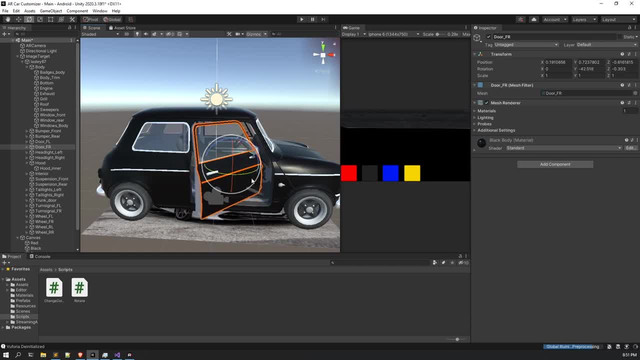 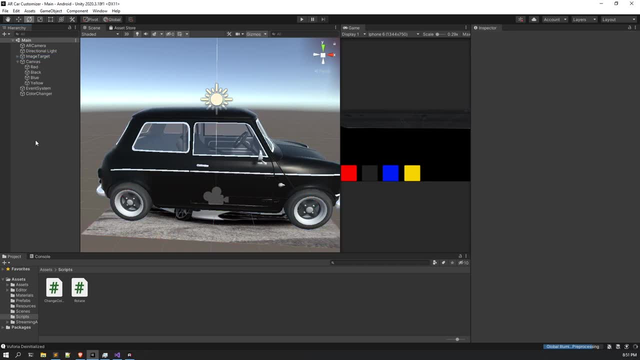 all right, and like rotate it somehow, uh, to get like the opening door animation, sort of thing. right, you can create your own animations like that and add it in there so that the person can actually- you know, the person can actually view the inner parts of the car. right, you can add more. 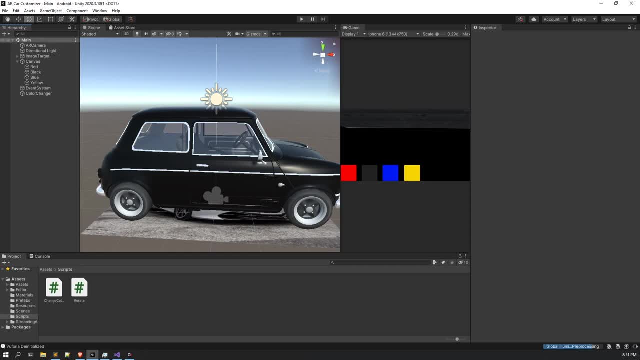 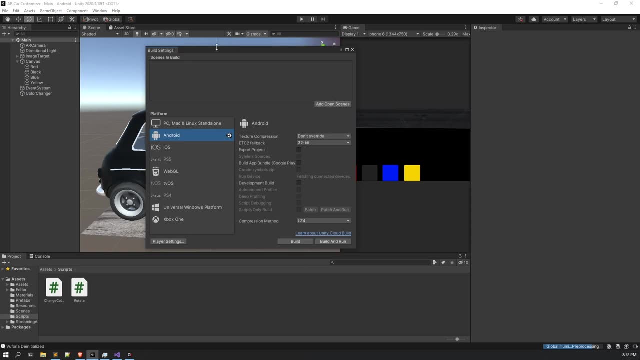 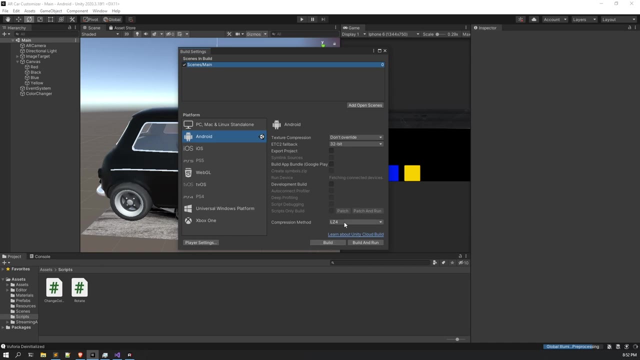 customizations to it. you can add more cars to it right now. the next process for you is to go to build settings- all right, and add, click on add open scenes. all right, that is for our. the scene is main. or you can simply drag and drop the scene and simply click on build and it would start building. 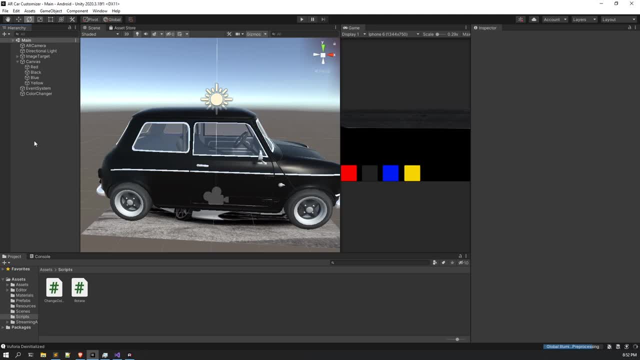 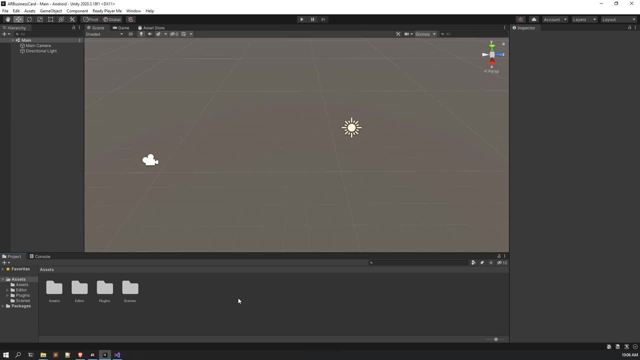 your application. all right. so if you have any doubt regarding this lecture, you can write it down in the comment section. all right, in this lecture we are going to create our second project. all right, that is ar business card. all right, how this project would help you is, let's say you are. 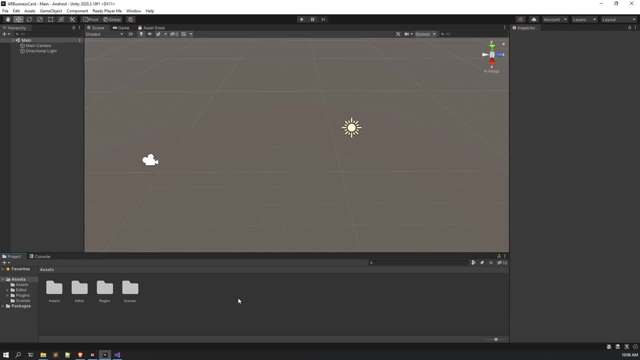 going to some client? all right, and you want to give them your business card? all right, you can share the apk? all right, if, like, of course, you can do this, right, so would we. creating a ar business card: all right, so we are going to create a business card. all right, so we are going to create a. 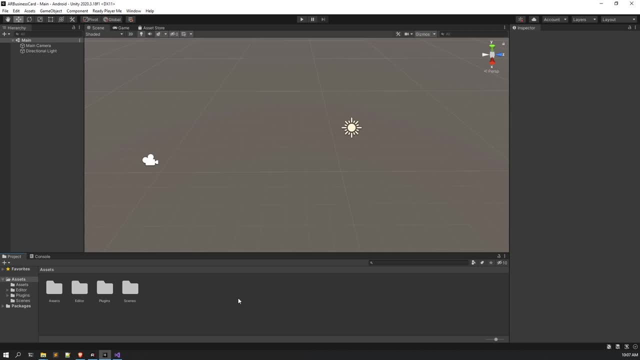 business card today. all right, and in this project, you are going to learn to like, implement your own avatar. all right, and you, you would also learn to apply animations, right? so let's do it. so what you have to do is right now. let me show you. first of all, you have to set up your project, all right. 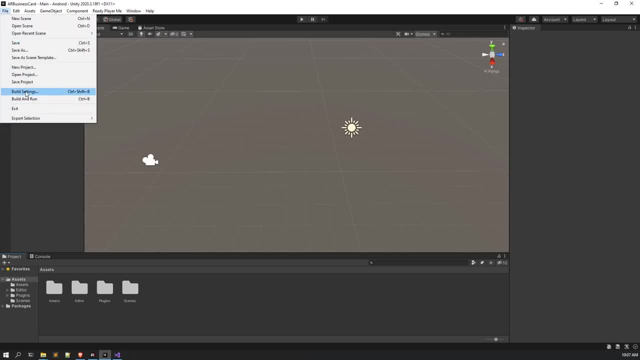 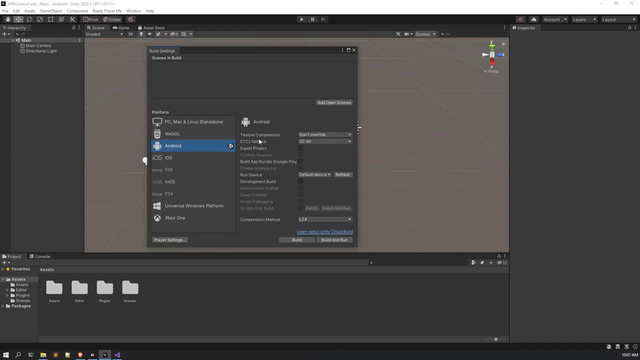 it's very simple: create a new project, go to file- build settings- all right. in the build setting, first of all, switch your platform to android. all right, i have already done that and make sure whenever you are opening a new project, when it's blank. all right, that's totally. 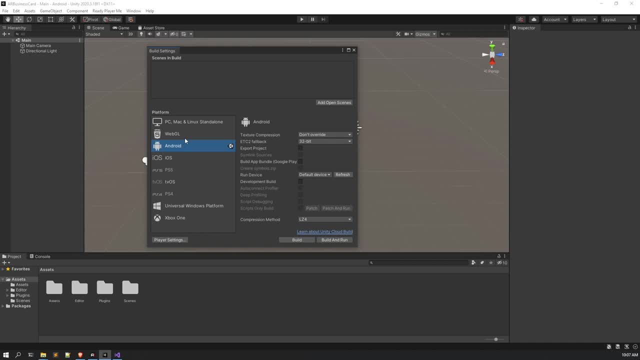 new uh, switch the platform first. all right, because if you do that later on, after multiple things are done in your platform, means uh in your project, then switching the platform would be very tedious because then it is going to take a lot of time if your system is slow. all right, after you have. 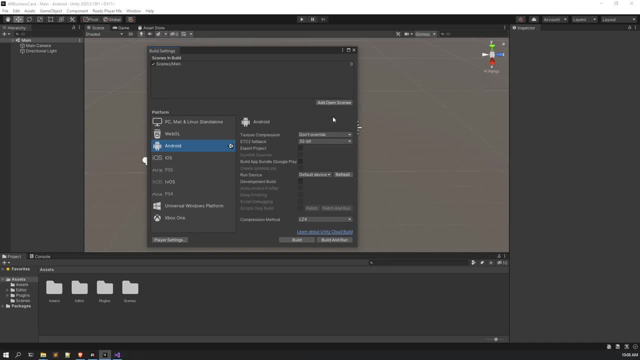 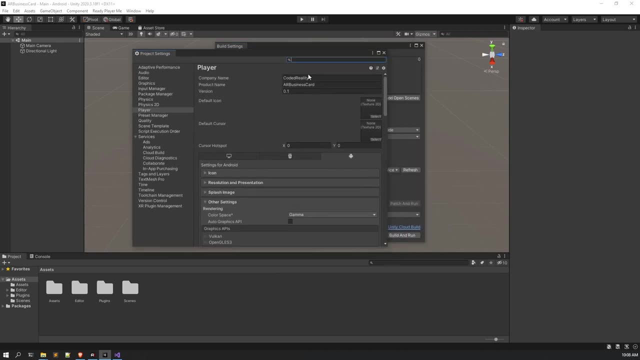 switched the platform to android. all right, you are going to do that, and then you are going to click on add open scenes. it will add a primary scene i am using all right now. all right, and go to player settings. in the player settings, give it a company name. all right, give it a product. 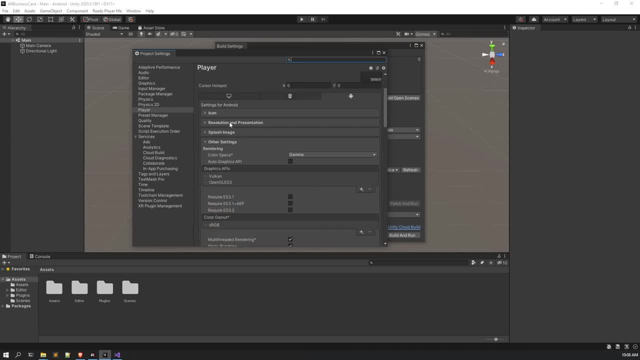 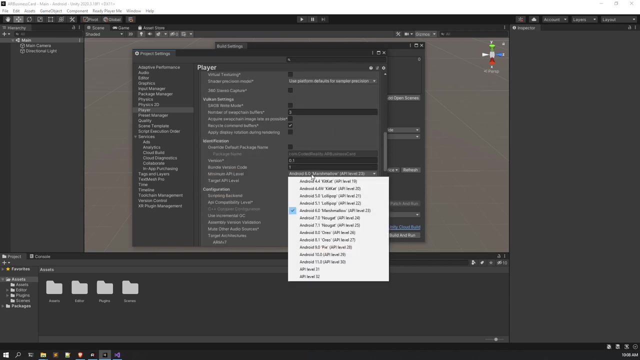 product name. all right, and go to resolution and presentation in the default orientation. select whichever you prefer. all right, i, i prefer landscape left because of my camera position. all right, then in the other settings, uh, select the lowest standard version you want to keep. all right, for me it's marshmallow. all right, and 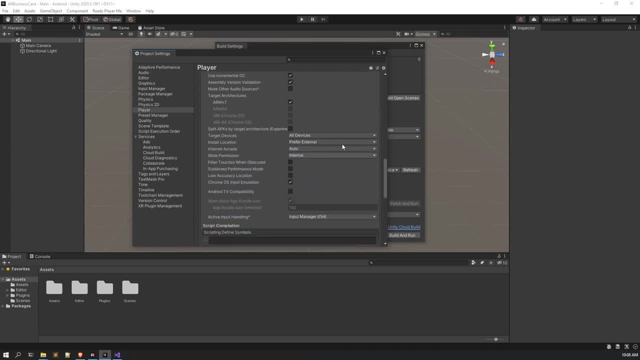 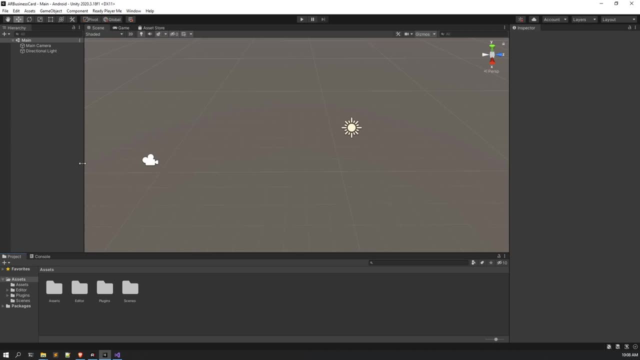 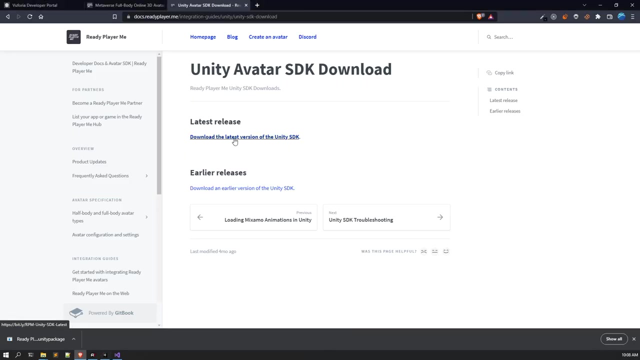 leave the target api level to automatic highest intro, all right, and after that we are done setting up the uh like project, all right. now what you have to do is import view 4d engine- and you already know how to do that, right- and another. you have to import another sdk that is ready player, me sdk. 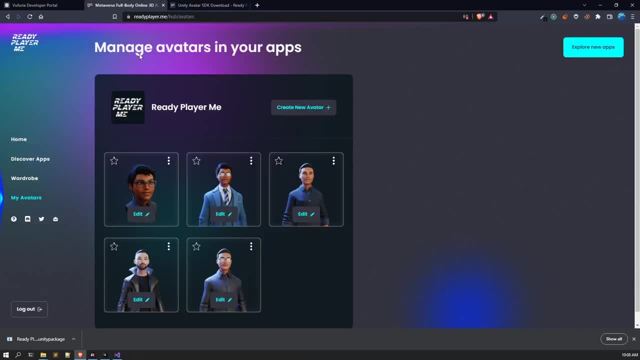 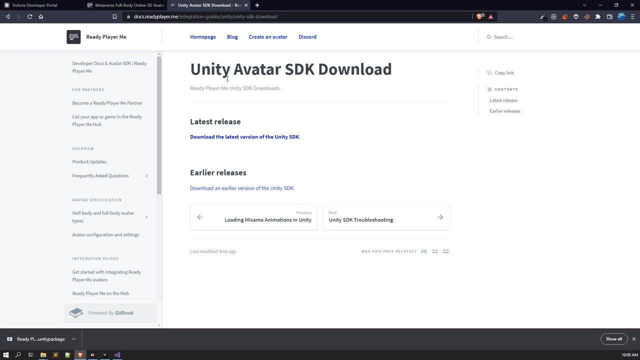 all right, uh it. it will enable us to create uh 3d avatars. all right, i have already. i already have 3d avatars in my uh dashboard. all right, so you can also create yours and uh upload it in unity. all right, and to upload them you you have to use this uh unity avatar sdk. all right, so 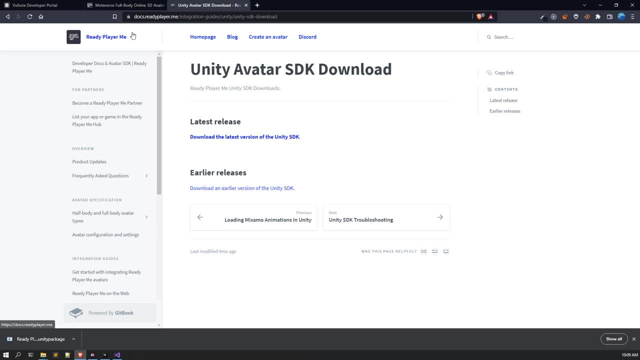 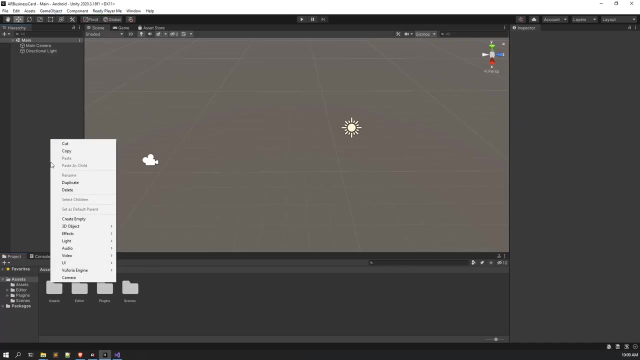 click on this, download the latest version and download your sdk right and then import it. the importing process is totally similar. all right, there isn't much any difference. so, yeah, all the things are there are totally similar. all right, i have already imported both view 4d and ready player me all. right now. what you have to do is 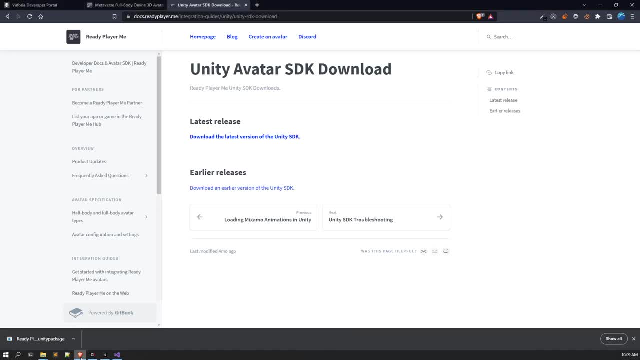 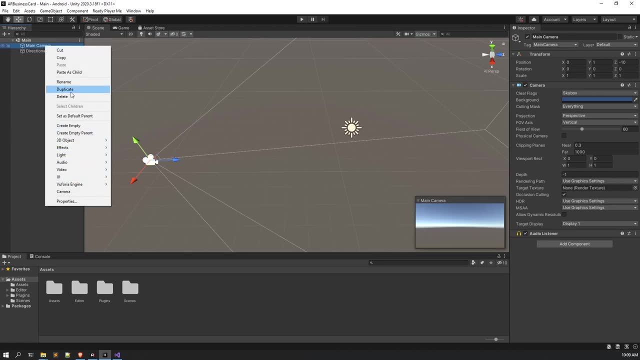 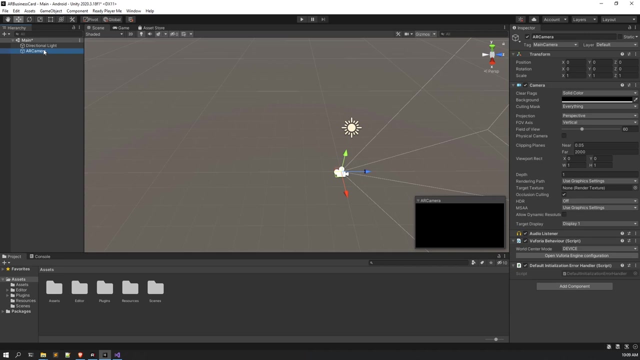 we have to set up our view 4d engine now, all right. so first of all to do that, go click on this main camera. then delete this main camera, all right. then again go right, click view 4d engine, ar camera. all right, you have this ar camera now. put it on top. all right, put it on top. okay now, after this: 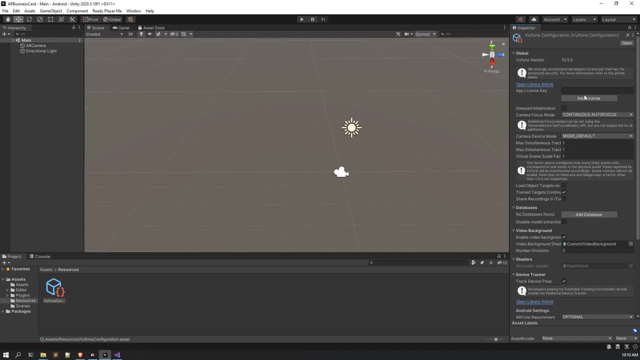 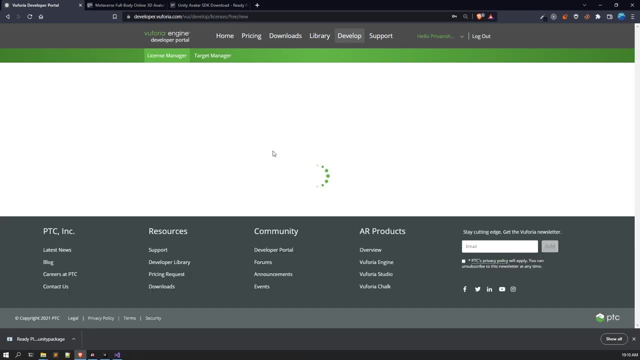 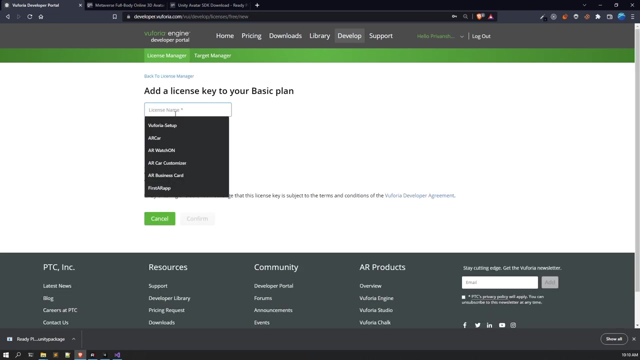 we have to add a license key, all right. so go to open view 4d engine configuration and we have to add a license key in here. so to do that, go to your view 4d developer portal. click on get basic. all right, and then you have to get a new license. all right, give the license name, that is. 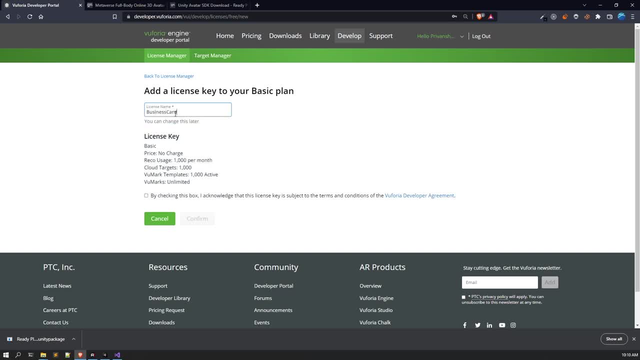 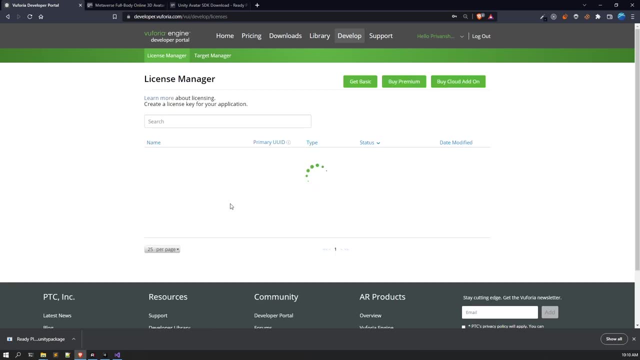 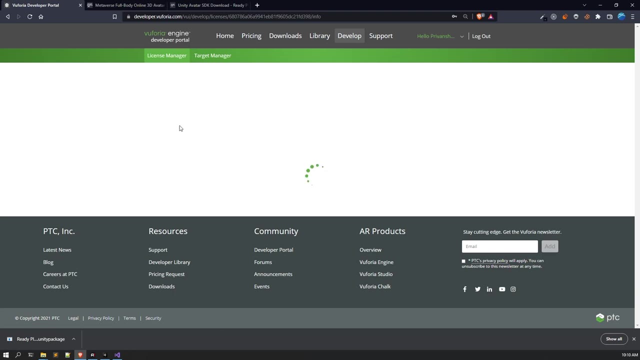 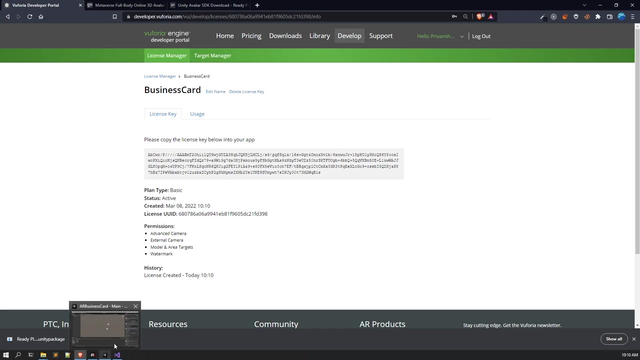 business card, all right, and check, check this box and click on confirm, all right, then you have the license key in here and you only have your business card right and here. all right, that is the license of your business card. so now what you have to do is, uh, click on this particular means. co copy this code. 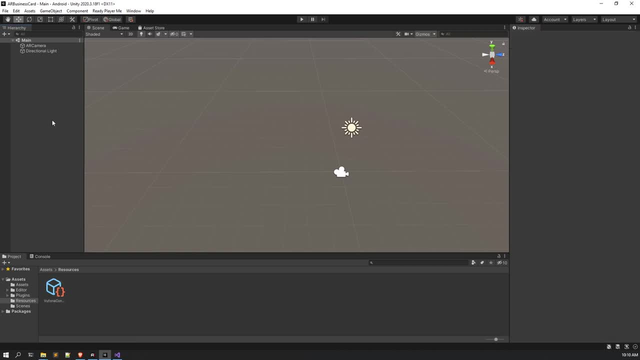 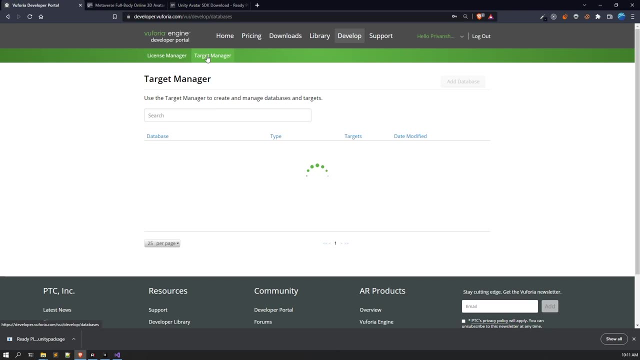 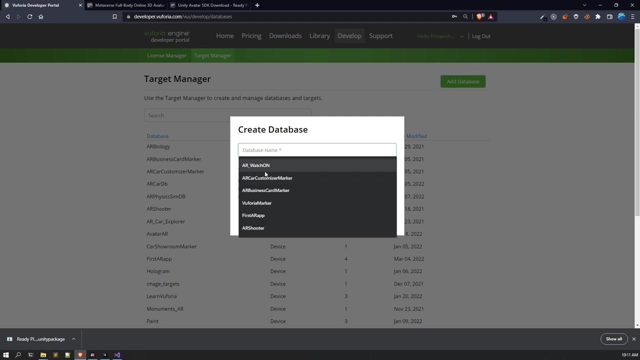 all right, and paste this code in your view4d configuration, that is, in the app license key. all right, and we are good to go. now what you have to do is open this, and we also have to add our own market database. so how do we do that? uh, click on add database. all right, then let's uh. 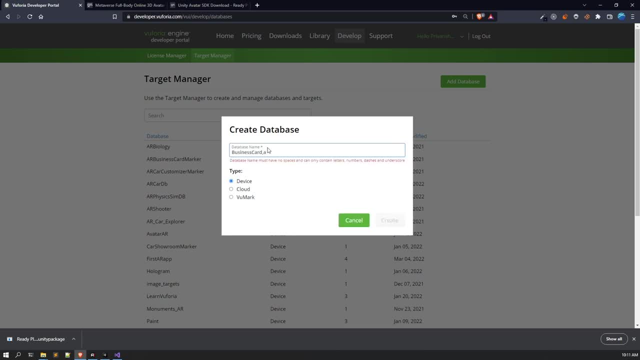 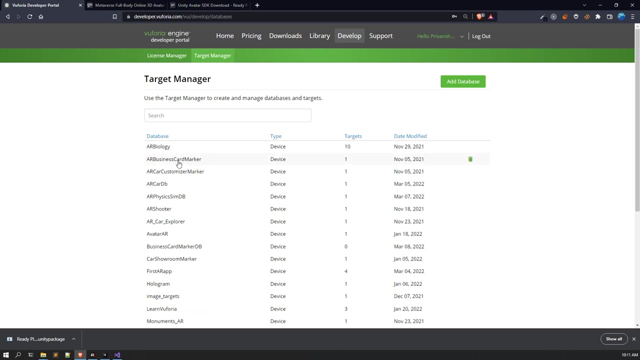 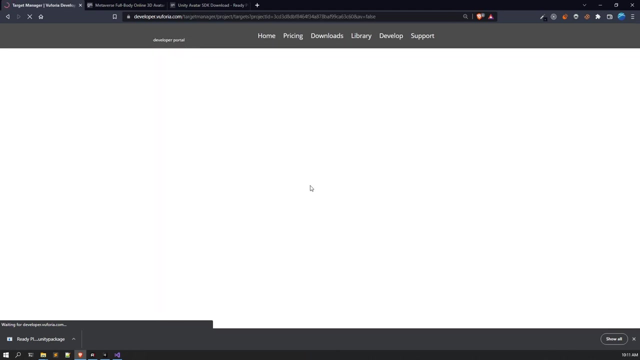 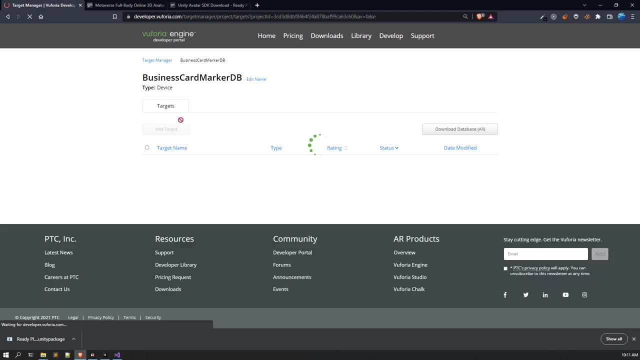 business card marker: all right, card, wait, okay. marker. all right, db. so i create this database, all right, and after you create this database, you are going to find, uh, open this database and add the marker. all right, add the marker that you have created in there. all right, i have my own business card marker, all right, so i i will simply add that in here. 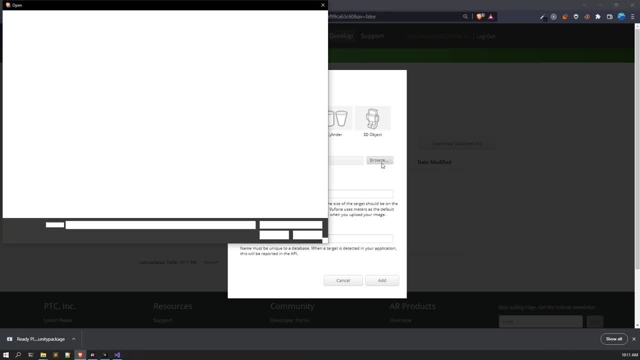 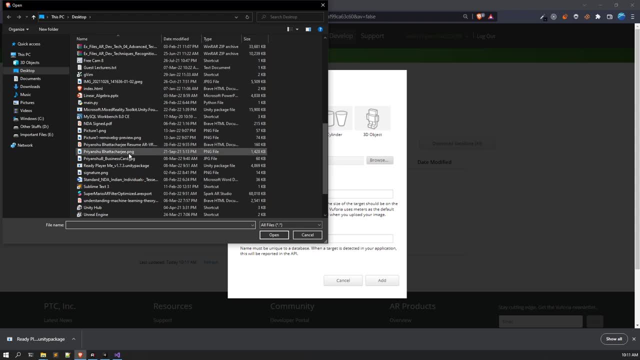 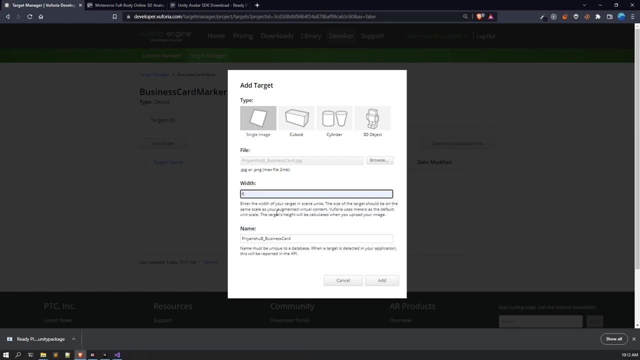 and then download it all right. so just wait, let me find my business card marker. oh yeah, i got it now. import it all right after that. uh, give it a, give it a size, all right, i'm going to keep it to six, all right, and you can. 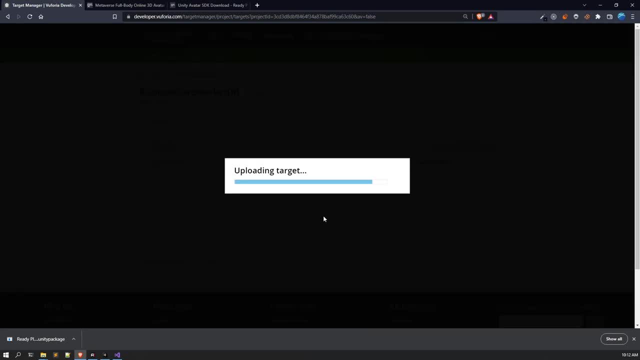 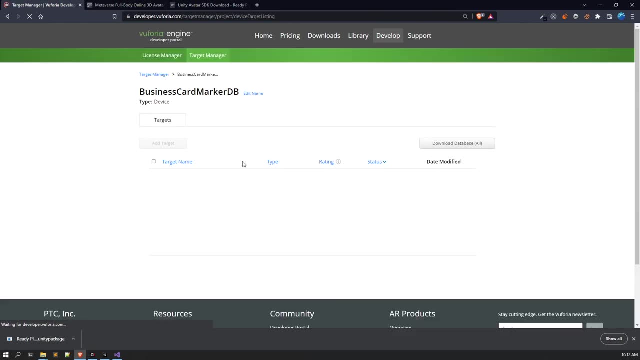 i'm going to keep this name already. you can give any name you want and then click on add target. all right, and it would upload the target in your database. now what you have to do is, after all these, after all these things are done, download the database. all right, click, that is, click on download. 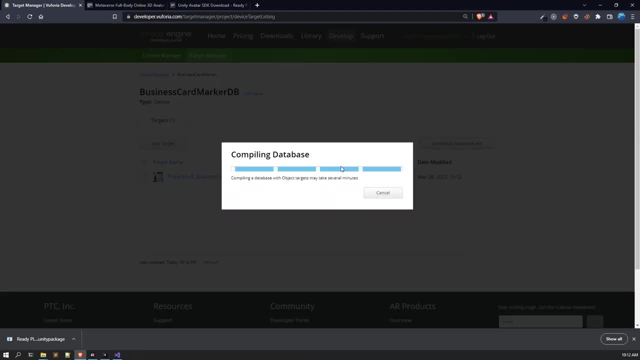 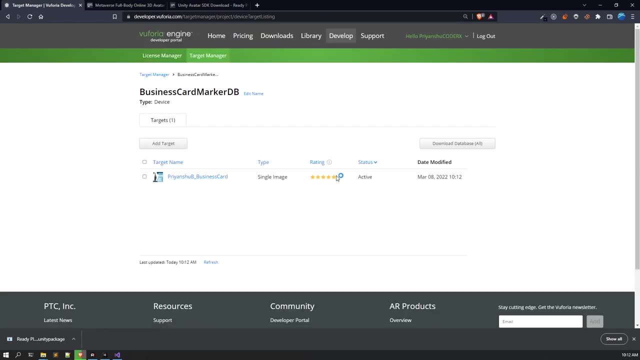 database and then select unity data and click on download. all right, and this would actually start the database. all right, and then what you have to do is you have to import this database in your unity. as simple as that, all right. so now open your unity. all right, open your, uh, unity, drag and drop. 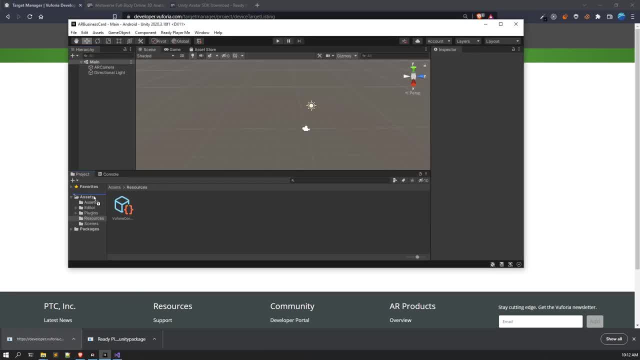 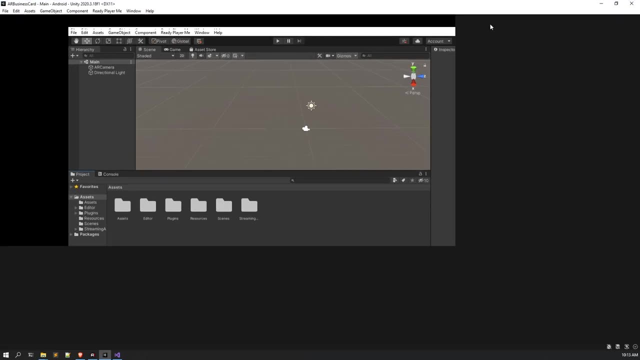 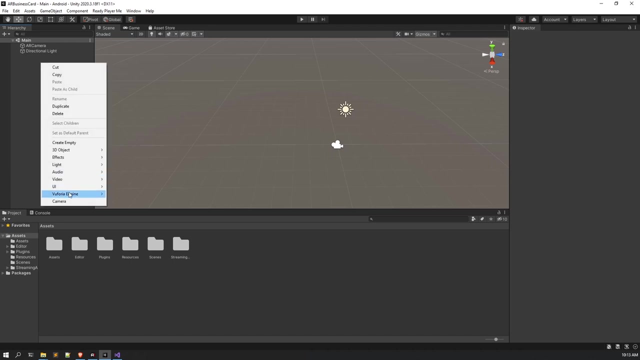 or drag and drop this sdk. all right, drag and drop this sdk into- sorry, not sdk- the database into unity and click on import. all right. so after all this, all right, it would import your sdk and- sorry, not sdk- your database, and we are good to go. all right. now what you have to do is right click in here, click on view for your engine image target. 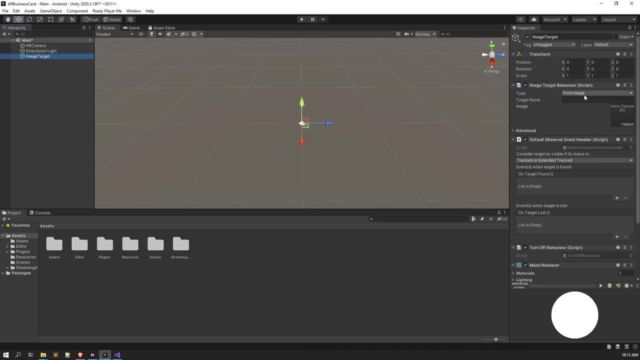 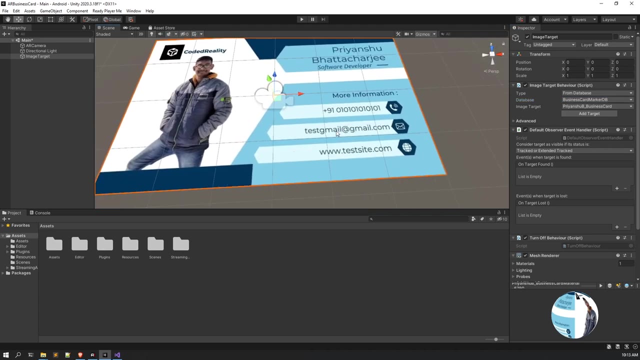 all right. so it would create a image target uh game object in here and in the inspector menu. you'd be finding image target behavior in there. click from database, select the database and voila, you got the marker right. so here you can see we have. i have the business, uh business card right now. 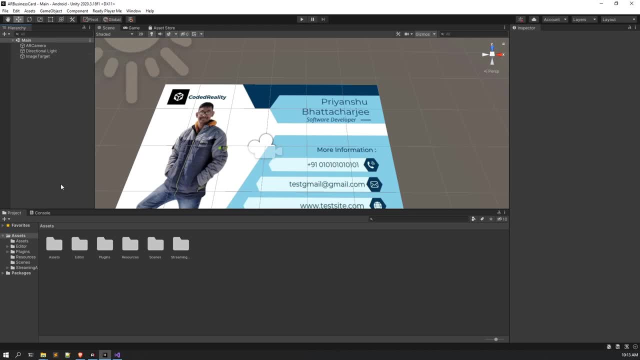 what we will be doing right now is: we have the avatar right. i already have imported the assets, all right. first of all, let me convert the assets, so select all these assets, all right? uh, all all of them are pngs, all right, so set the asset and 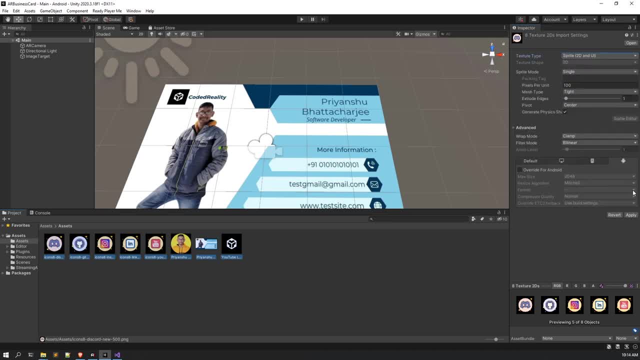 in the texture type, go to sprite 2d and ui and click on apply. all right, so it's going to take some time. it's going to convert all the textures to a certain type, all right, that is this: sprite 2d and ui, all right, and after it is converted, all right, i'll be back. 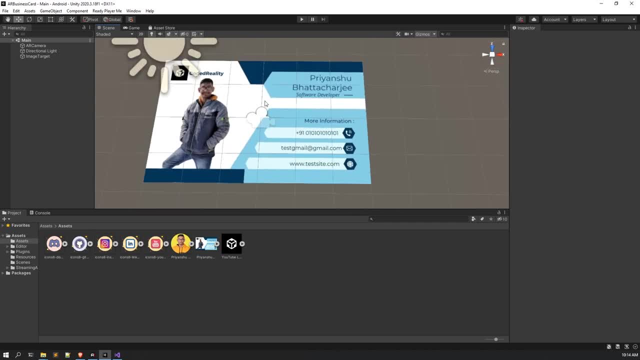 so our assets are converted, all right, and now we are good to go, all right. so now what you have to do is, uh, you have to import the 3d model, all right. so how would you do that? first of all, uh, click on this ready player me. 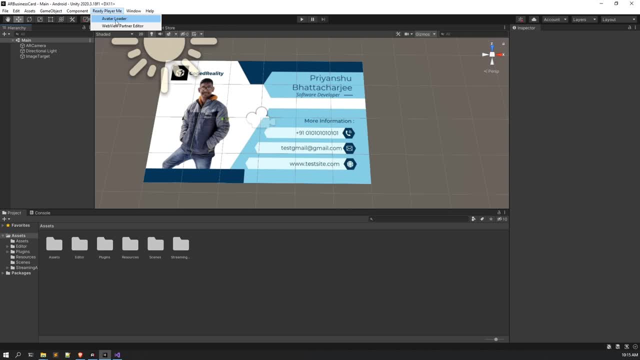 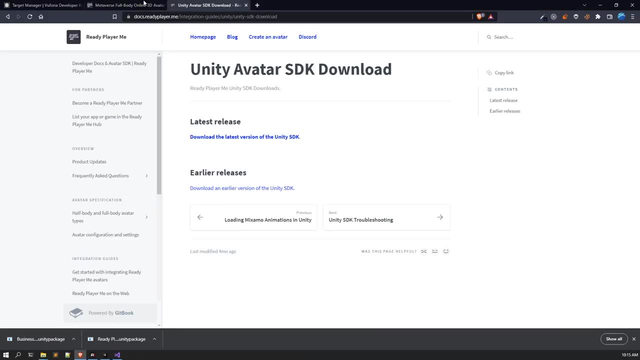 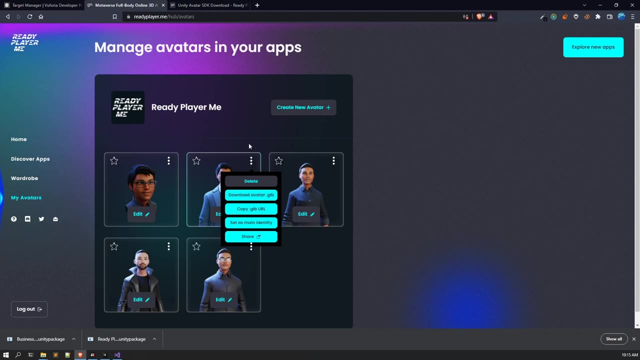 button in here- all right, that is in the head- and click on avatar loader. all right in here. what you can do is uh, create a new avatar for yourself, all right, i i already have them. create a new avatar, all right. it's very simple to to create one and create avatar, and then what you have to do is click on that avatar in the 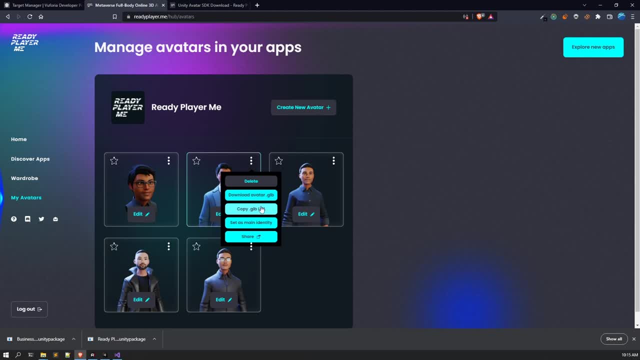 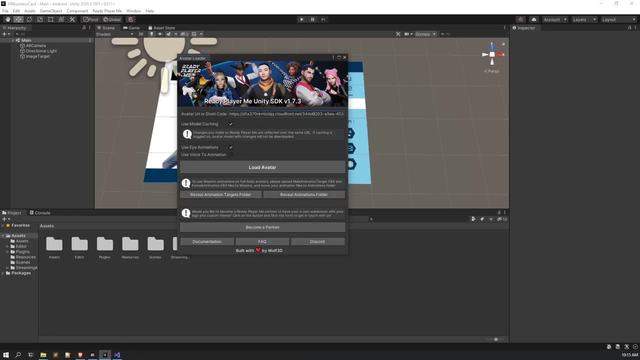 three dots. all right, and copy dot. glb url. all right, copy this or glb url and go to your unity editor. here you can see avatar, url or shortcode. you have to paste that link you copied, all right, okay. so now here are a few options. all right, first of all, uncheck this model caching. why? 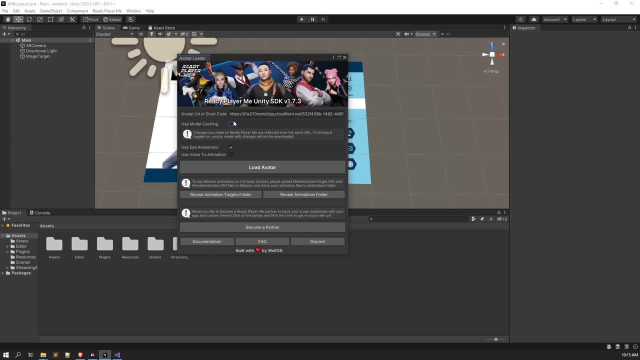 see, this model caching feature is a feature by ready player, me only what happens now? it will cache your model in unity. now, if you don't, all right. let's say, if you, if you uncheck this model caching, what will happen if you make some changes? all right, if you make some changes. 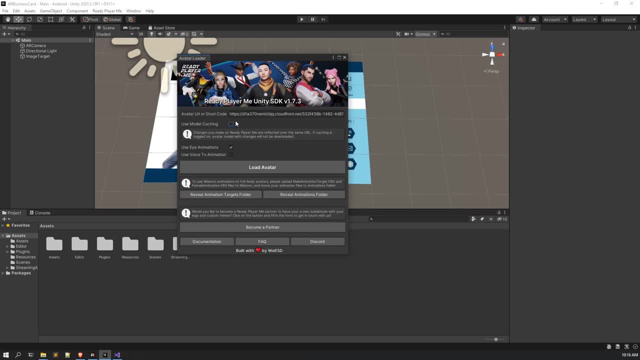 on the ready player me web that those will be cached. all right, so now let's say, if you make some changes on the ready player me web, that those changes of the avatar will automatically get reflected in your unity editor. all right, so for now i don't want uh model caching to be there. 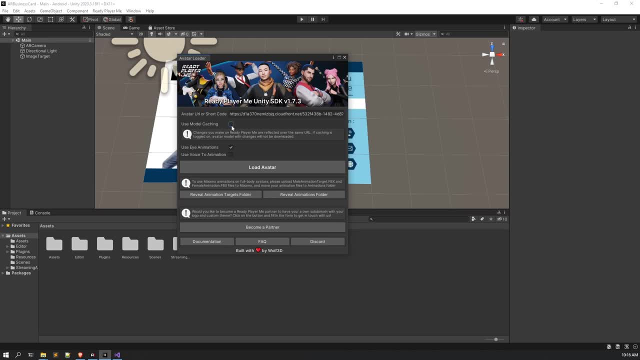 but if you want that, if you want model caching to be there, you can do that, all right. but currently i don't want, uh, my model to be cached, all right. and uh, if, if use i animations is not checked, click on this use i animations, all right, and after that click on load avatar, all right. 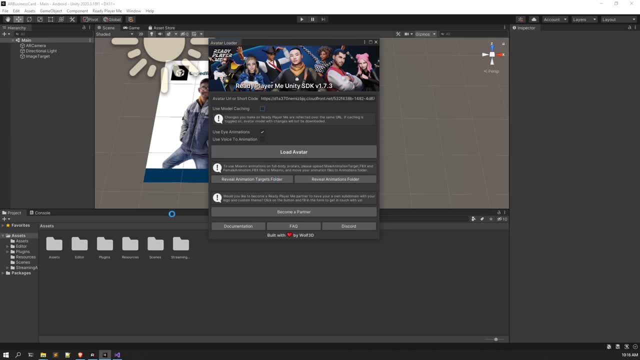 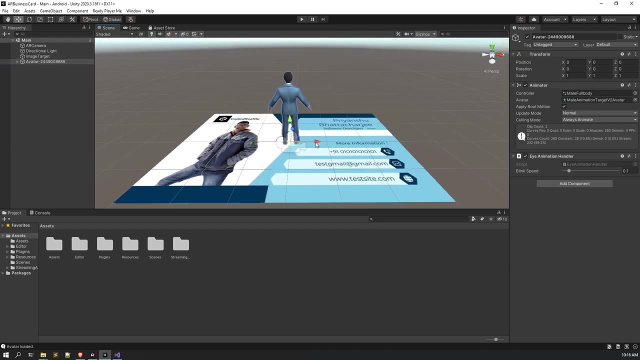 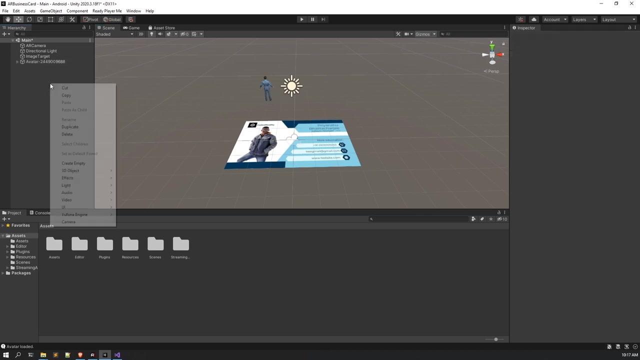 so it would start loading the avatar, all right, so first, first of all, it will download, then simply import your avatar. okay, so our avatar is now loaded, as you can see right in here, all right, so first of all, all right, let me, uh, keep this avatar in a different place, all right, and 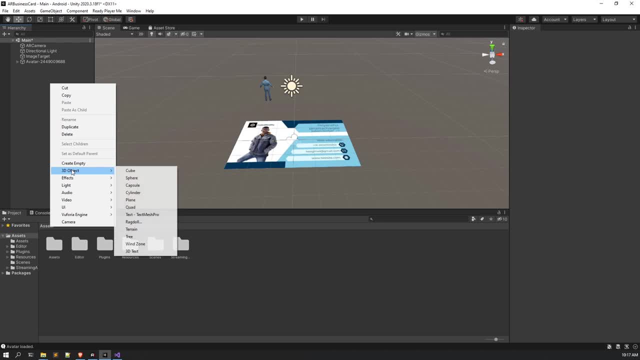 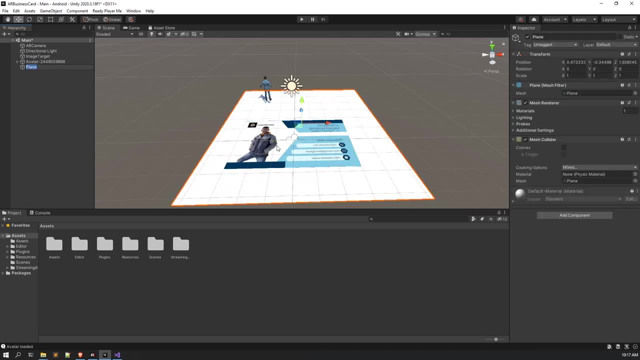 let me add another plane, all right, that is, go to 3d object. in the 3d object, click uh, plane. all right, this plane is, of course, a big. first of all, let me reset the transform, all right, and let me, you know, put it down a bit and let me go. 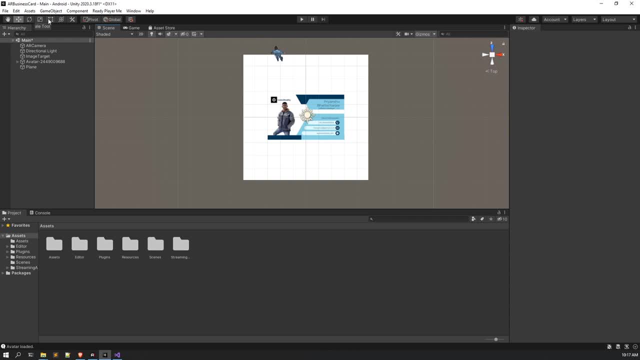 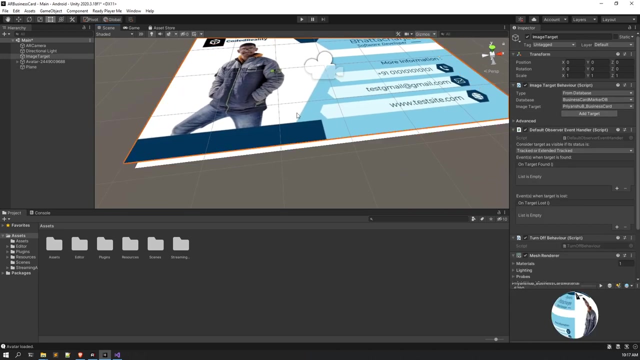 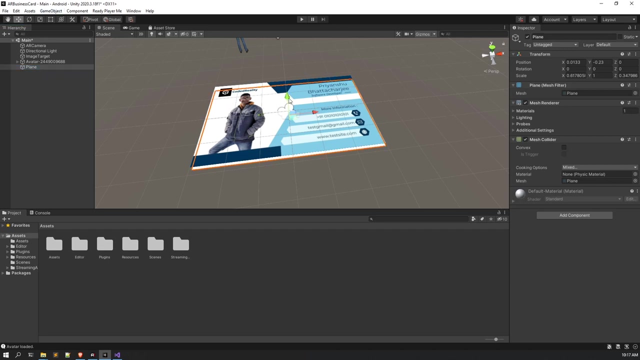 to the top view so that i can, i could adjust. all right, i could adjust this particular plane, okay, cool, okay. all right, okay. so we have adjusted our you know? okay, we have adjusted our plane. all right, now you can, uh simply put it upwards, all right, cool. now, uh, what i want you to do is attach a material into, uh to it. all right so. 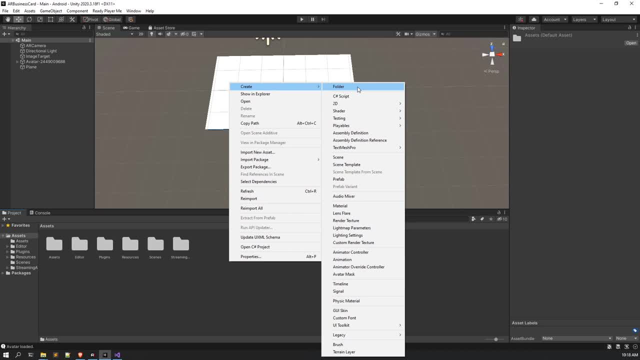 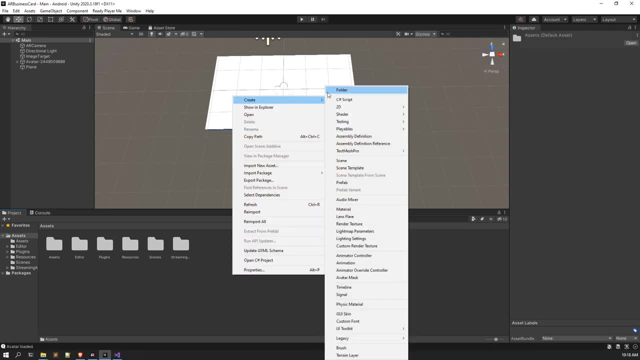 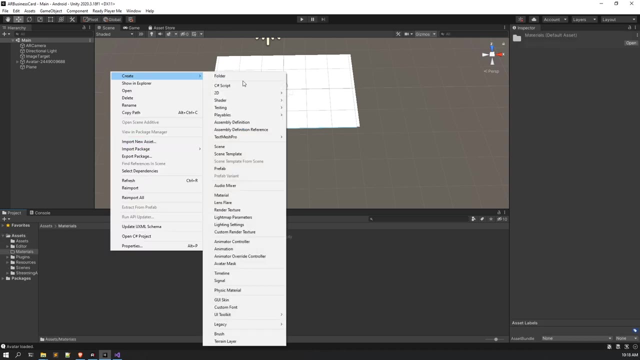 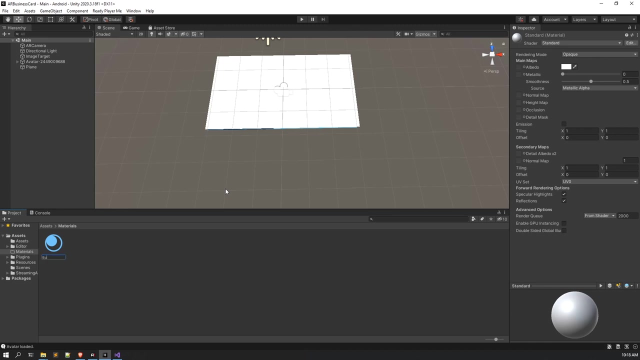 how do you do that? click right click on the project panel. create a folder, all right, uh, uh, create a folder called, you know, material. all right, right click, create folder material. click in here. uh, go to again material and give it a card material- all right, card mat, all right- so that we can add the material in here. 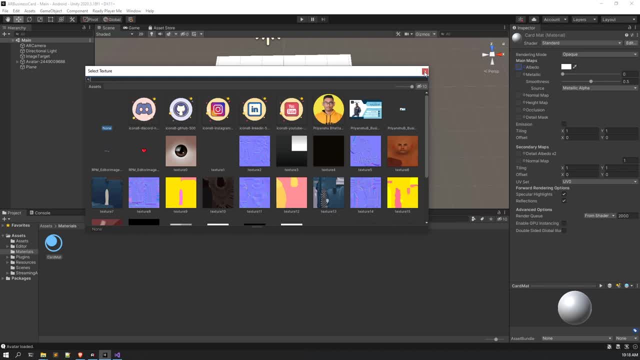 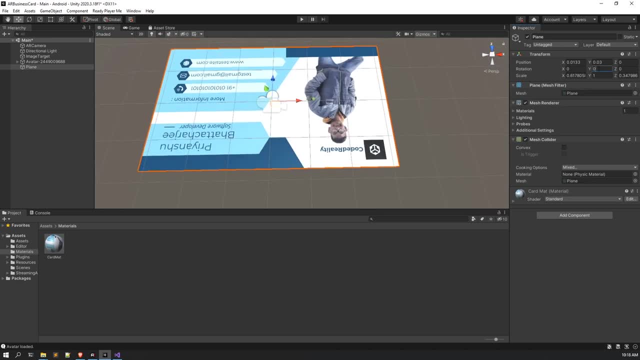 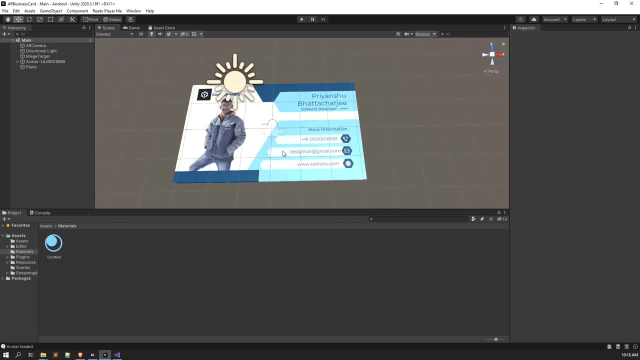 and in this albedo, click on this option all right, and select the card material in here, okay, and then drag and drop it in here. all right, now rotate it. all right, rotate it so that we get the perfect alignment. all right, so now we are good to go. now let's uh, edit this. 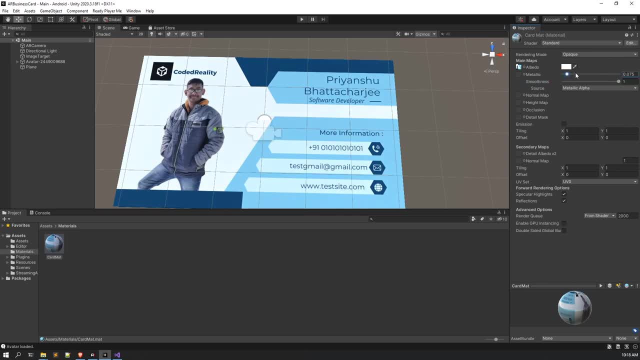 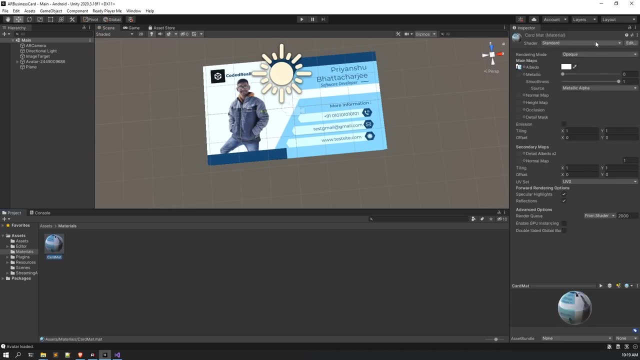 material a bit right. okay, of course, metallic doesn't look good, all right, yeah, let's, let's experiment with this material a bit, all right, okay? so let me first create a material for here. nem allerdings ta. finally. it wasn't readyを wait, so now, as you can see, we have a menu right in here. 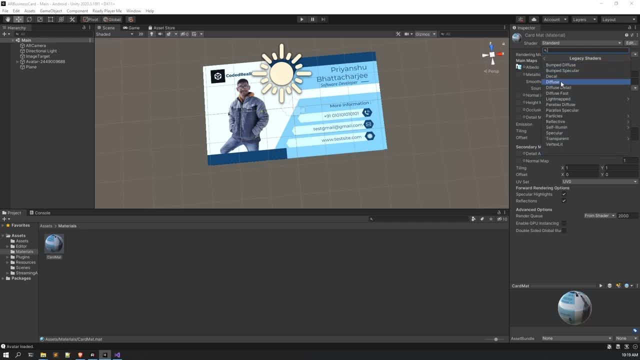 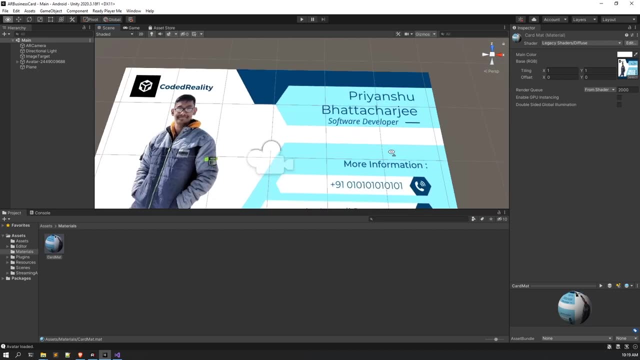 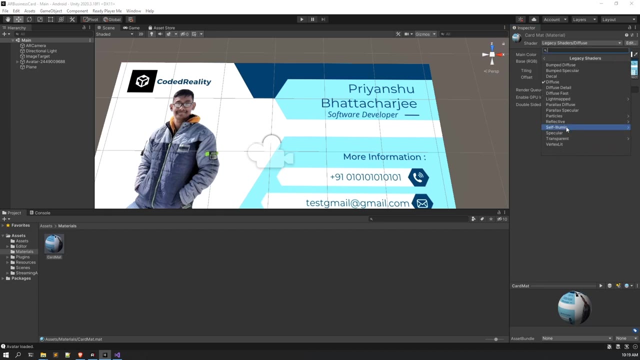 all right, uh, click on legacy shaders and click on diffuse. okay, now it. uh, it does looks good, all right. so let me show you how i did it in the material section, shader option. all right, then go to legacy shaders, then diffuse. all right, so that's how you do it. 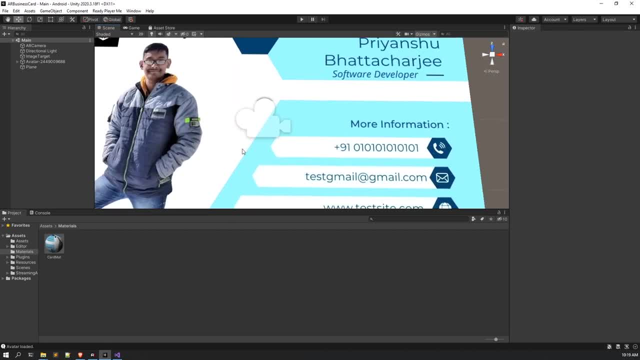 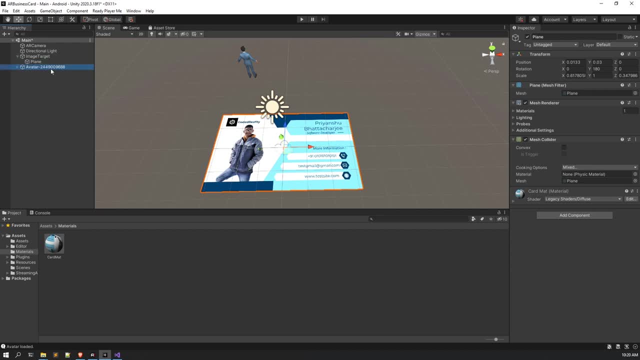 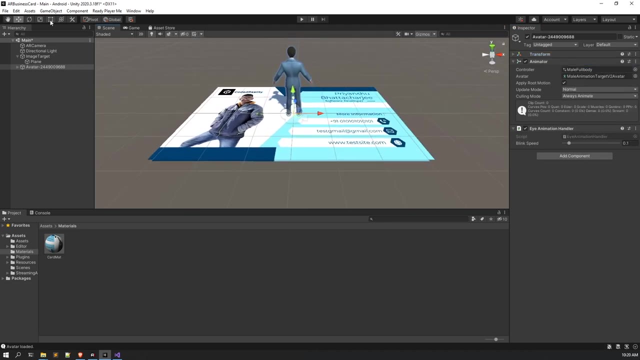 all right. so, yeah, i hope it's clear. now what you can do is, uh, drag and drop this plane all right- inside this image target and you get this avatar right. reset the transform of this avatar. all right, reset the transform of this avatar. scale it all right. scale it a bit. scale this avatar a bit. 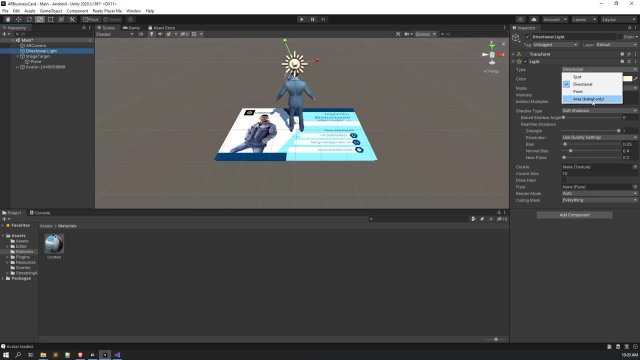 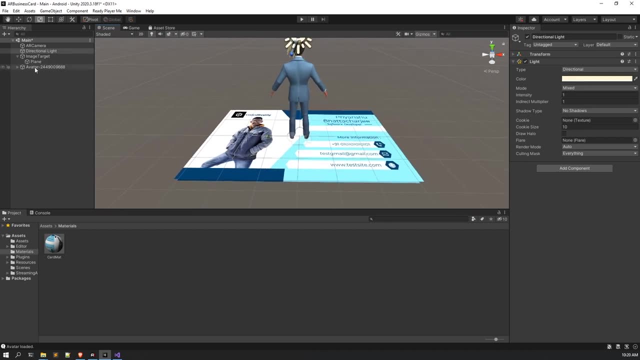 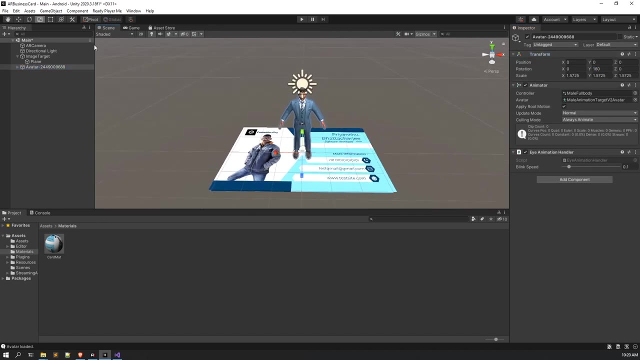 all right. uh, first of all, you remove this directional light. all right, i don't want. this means remove the shadows, not the directional light. of course, after removing the shadows, all right, rotate, rotate this particular avatar. all right, let me rotate it. okay, cool, now put it right in here. all right, on top of the, this blank area, 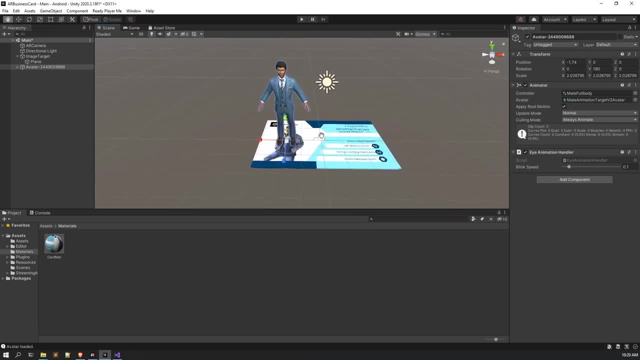 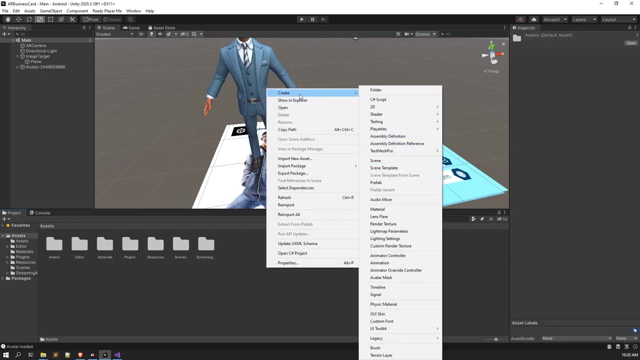 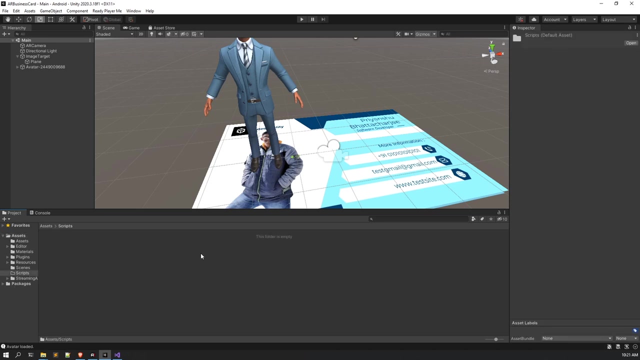 all right, let's make this like this: all right, cool. so now you get a avatar. all right, you can add a rotation script. all right, so let's, let's go to uh, create another folder. all right, let's create a folder called scripts. in the script folder, create a c sharp script- all right- and name it rotate. 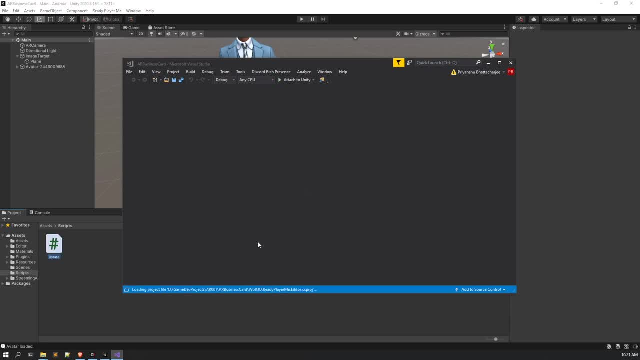 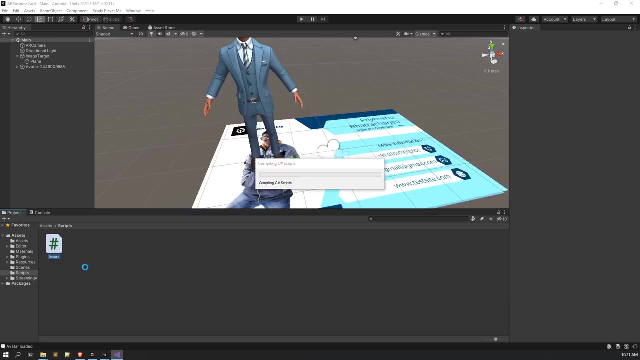 okay, uh, i'm going to hit reload in my visual studio editor. all right, so it's currently compiling and it also reloading my visual studio editor, so just wait a few seconds. so now our script is compiled. all right, now let's open this in our visual studio editor. 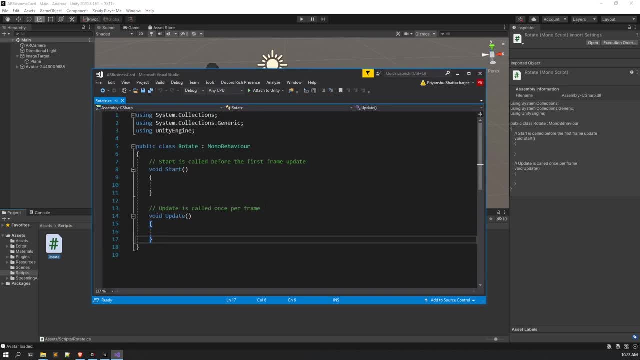 all right, and let's write, uh, some script in it. first of all, remove this task and all those comments, all right, simply create a public vector3, all right, vector3, and give it rot, all right, and then click on transform, transform, dot, uh, rotate. then pass this rod value in uh on the rotate function and multiply it with time, dot, delta, time. 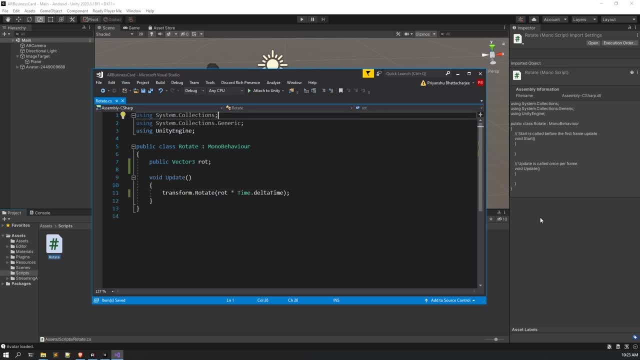 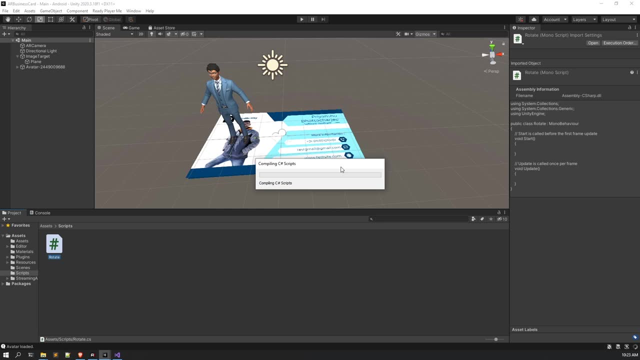 all right. and then, uh, save the lesson for that time. and uh, this is all right, it's ready to go. so now, if you save the script and compile it, all right, after compiling it, we we have to attach the script on the avatar. all right, to make it work. so it's currently compiling the script. 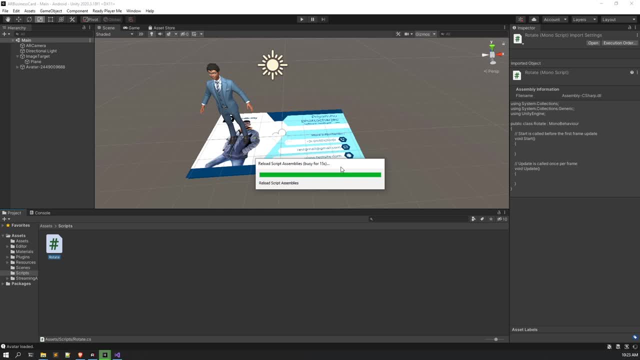 so just wait for a few seconds and you know it would be done, right? so, um, yeah, so our script is compiled. now what we have to do is click on this avatar. all right, add this script right in here. all right, and give it a rotational value of, let's say, 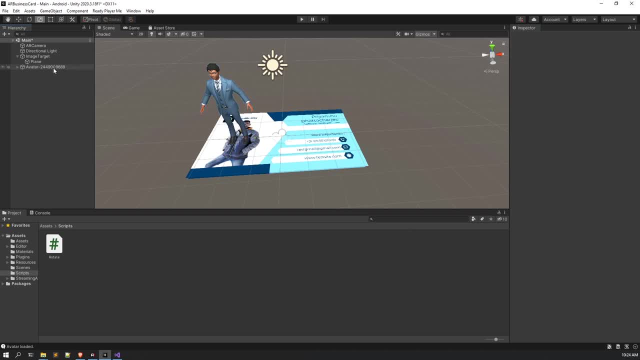 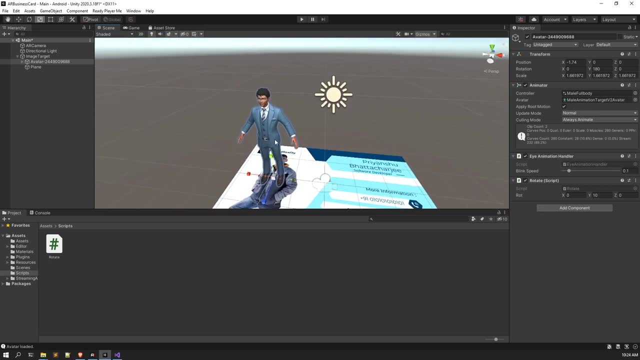 10, all right, and also drag and drop this, a particular avatar, inside the image target, or make it a child of the image target, all right. so now, as we uh, did a lot of things right in here, all right, let's, uh, let's see if everything's working perfectly or not. 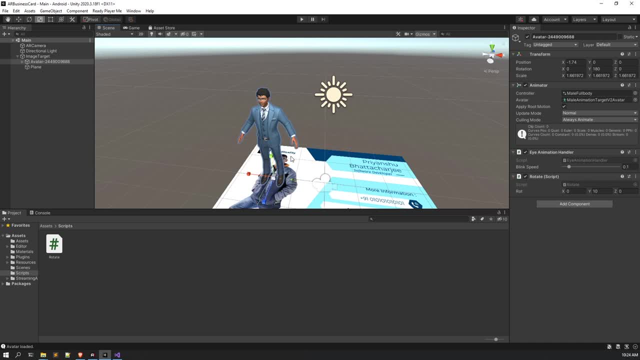 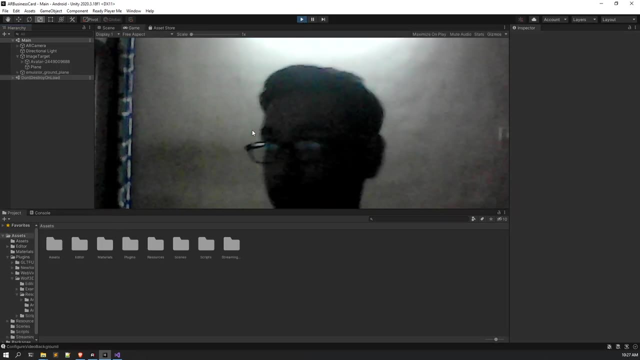 okay, all right, so let me open my uh marker and uh, then hit the play button. all right, hit the play button. all right, so that's what you have to do right now. so click on this play button. so now, as you can see, our camera is open. now let's uh. 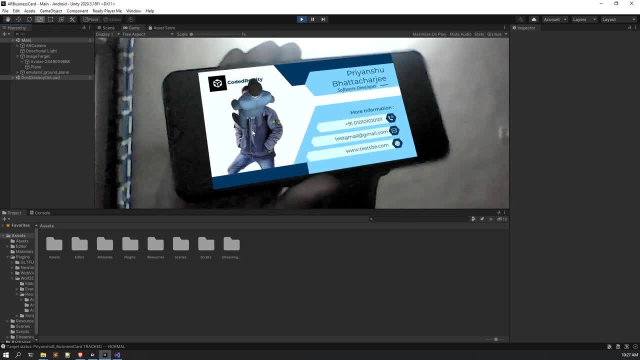 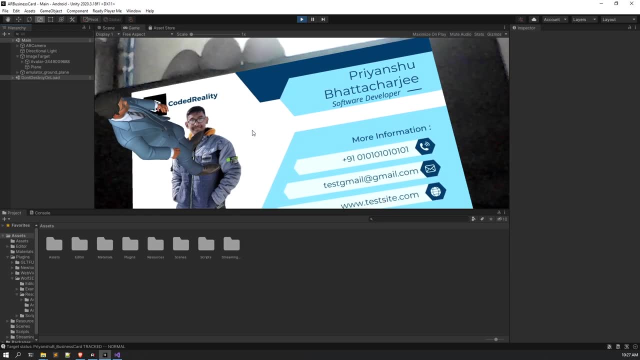 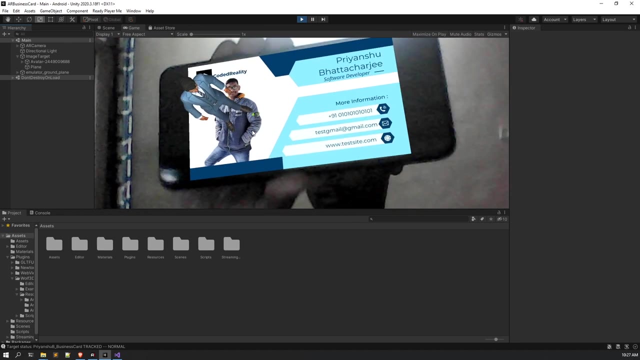 oh, cool, see, uh, all the features that we implemented as of now is perfectly working, but here you can see the uh character animation is being played. right, the character animation is being played, but the problem is that it is sometimes it's also working all right, it's also showing the walk animation and i, of course, i don't want the walk animation. 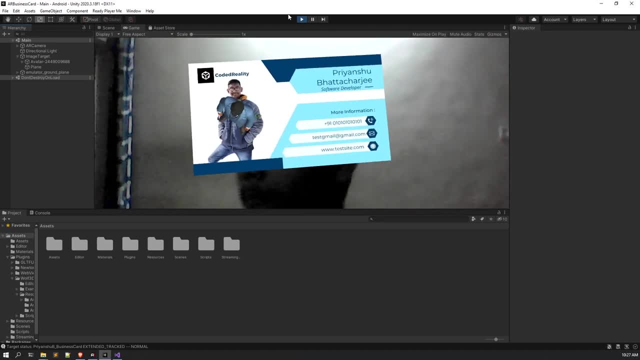 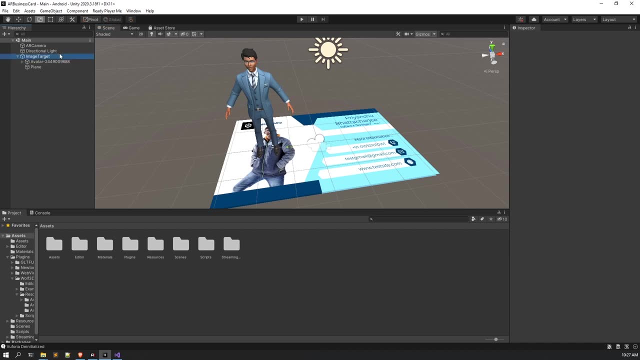 all right. and here comes another problem: that this extended tracking. so we'll be fixing these problems, all right, before moving forward. so how to do that? first of all, uh, let's fix our, or let's let's fix the image target problem. all right, click on this image target, uh. 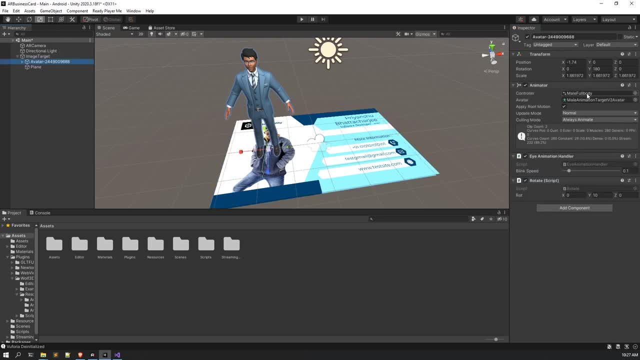 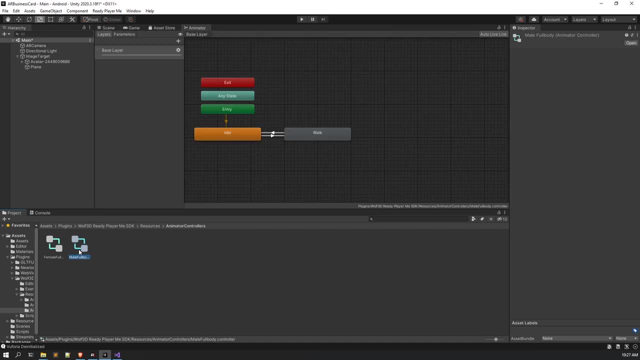 change it to tracked. all right, then in the avatar. what you have to do is, in the you can see in the controller option, click on mail, full ball with body- that is the controller name, and double click on this and it would open an animator window. here you can see that, uh, there there's uh two pathways. 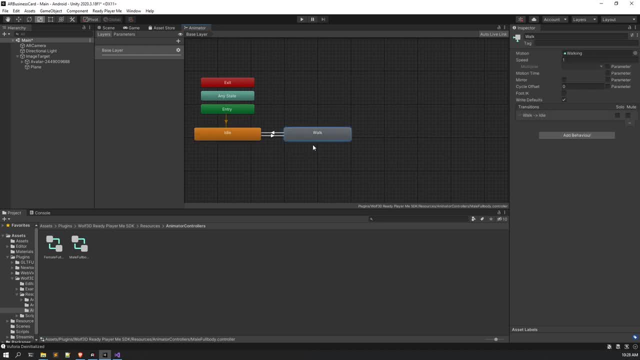 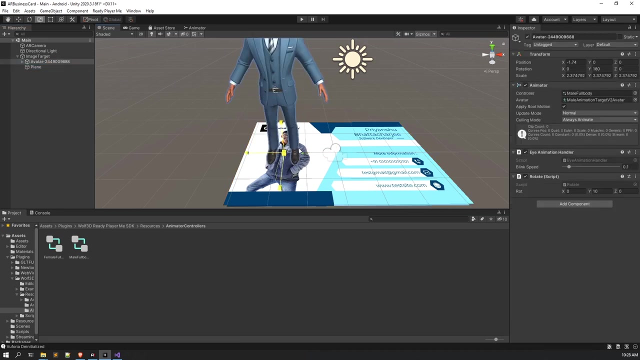 that is, first it is going from idle to walk, then again it is going to walk to idle. all right, so simply delete this. all right. simply delete this particular uh animation, and we would be good to go all right now. also, i want to increase the size of this avatar a bit, all right, so yeah. 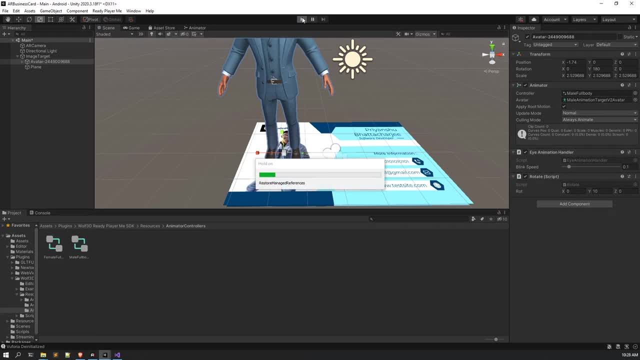 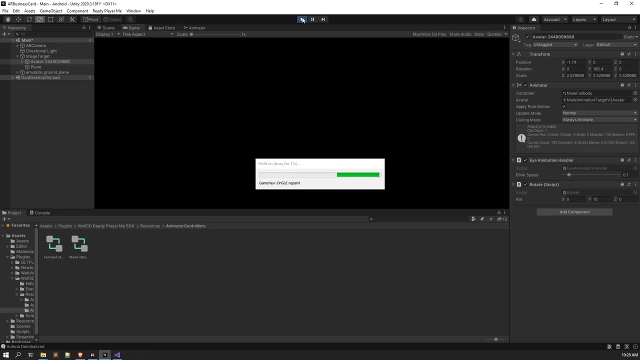 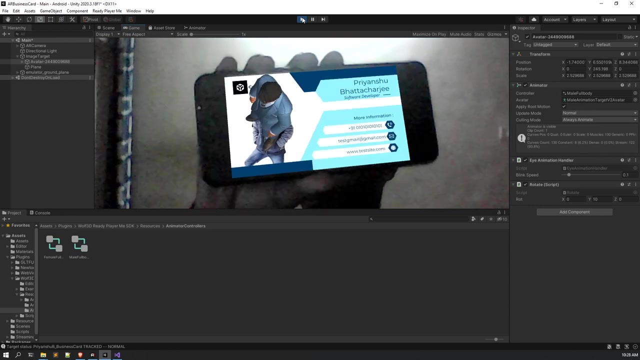 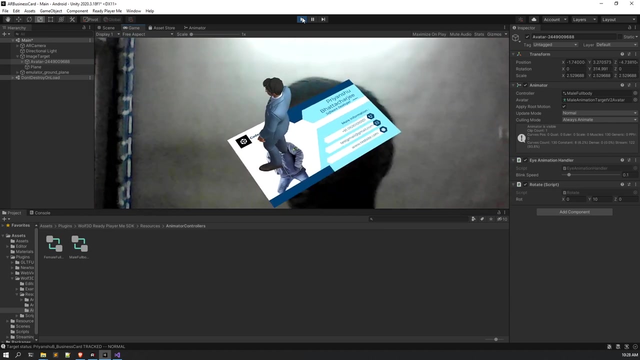 now let's see how everything works right, let's see how, how perfectly uh things are working and if it needs any more changes or not. right, so yeah, just give it a few seconds. okay, cool, okay, yeah, it looks good. it does look good right now. all right, so yeah, and also the tracking thing. 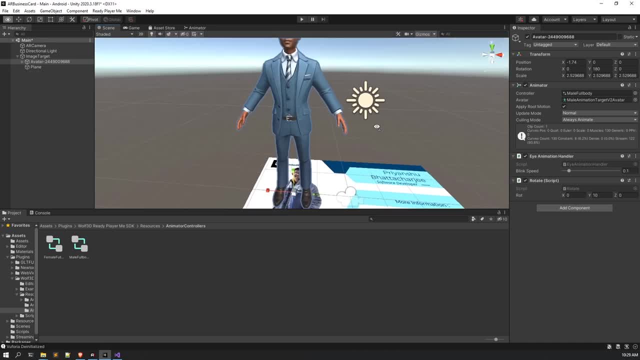 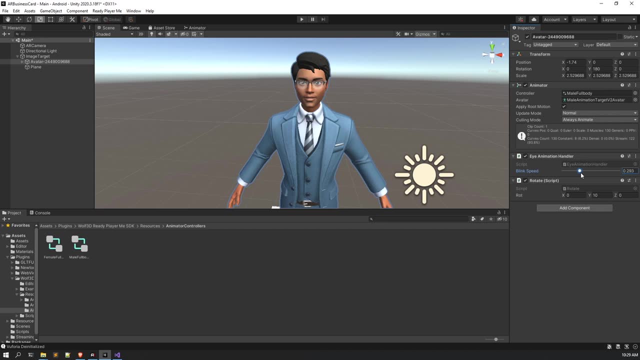 is fixed right and currently you can see the blink speed. all right, the blink, uh. you can increase the blank blink speed. all right. that is where you can make it to like 0.3, maybe. all right, i'm going to increase it to 0.5. it's the ideal value i i find all right, you'm. 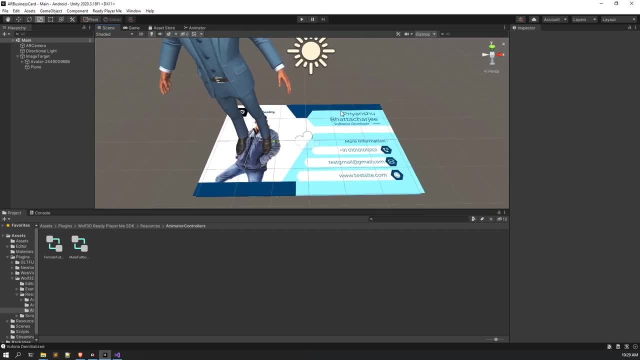 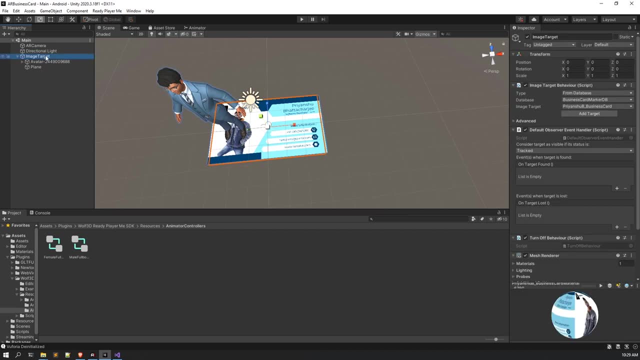 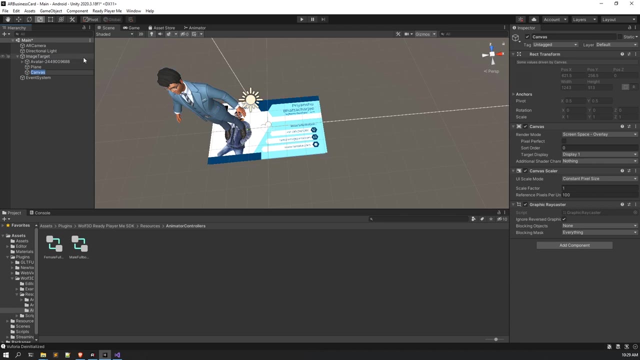 Now, as our avatar is set up, now also set up our UI. now how to do that? This thing is fairly simple: go to image target, click on UI, then select canvas right in here. select canvas, and currently this is a 2D canvas and of course, none of us want 2D canvas. what? 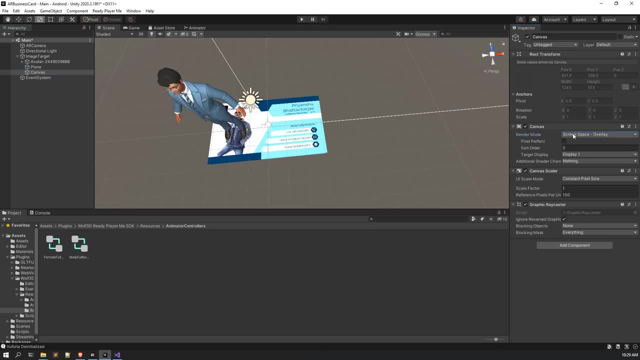 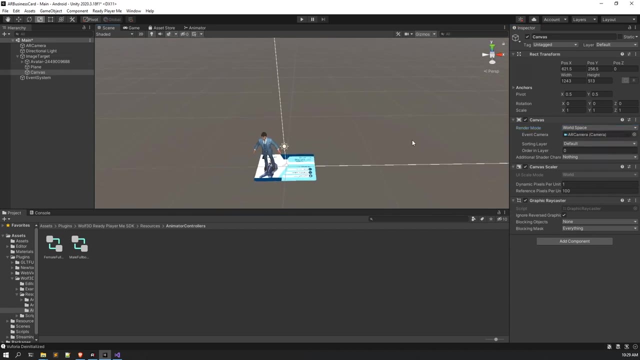 you can do is go to click on this render mode and select world space. select here. you can see, here is an option for event camera. drag and drop this AR camera into this event camera. alright, and here you can see. our canvas is now transformed to 3D mode. alright. 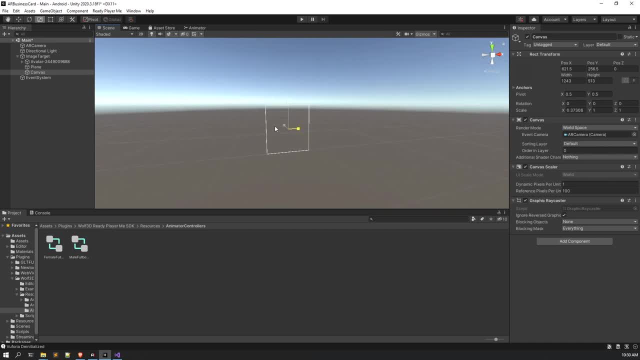 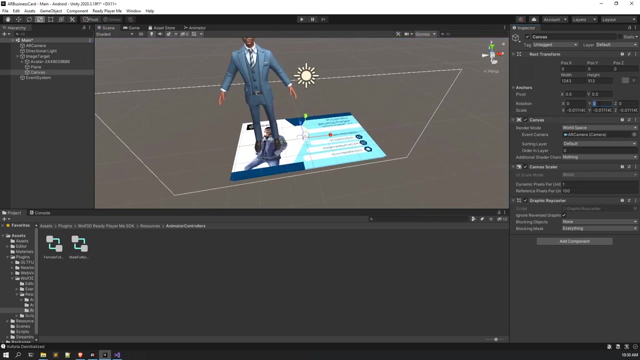 Now let's edit this canvas, alright. let's scale it down. alright, and let's scale it down. let's reset, not reset. let's reset its position. alright. here you can see we also need to scale it down more. okay, now rotate this into Y axis, not Y, sorry, X axis to 90 degree, alright. 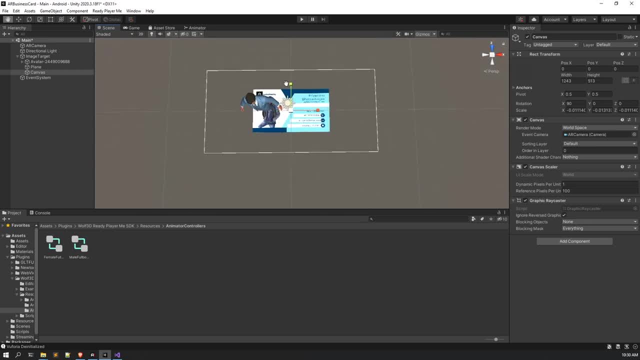 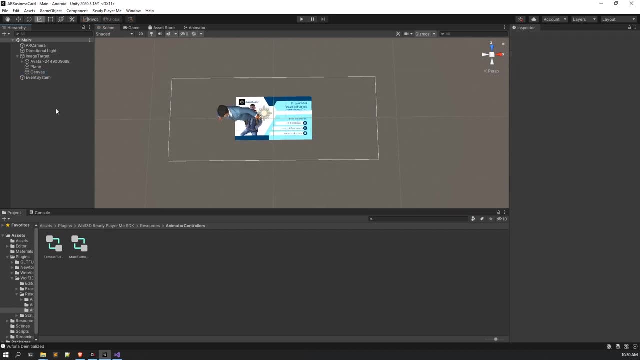 and make sure it is like this: alright, give it a bit space to it so that we can, you know, add our UI into this right Now. what you have to do is you have to add UI to it, right. what you can do is click on. 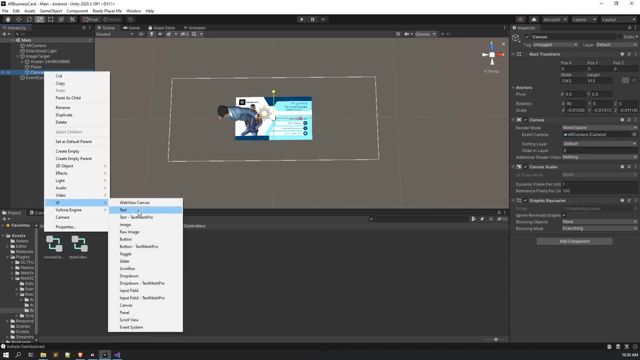 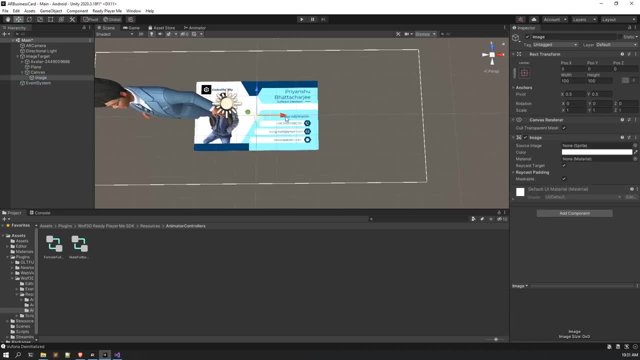 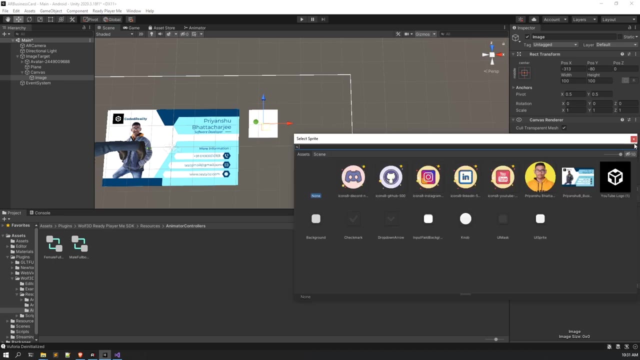 this canvas. alright, then go for. first of all, I want to add an image, so click on this image. alright, and let's drag and drop it in here. alright, So this would be my profile image. alright, and I already have the profile image, so I'm 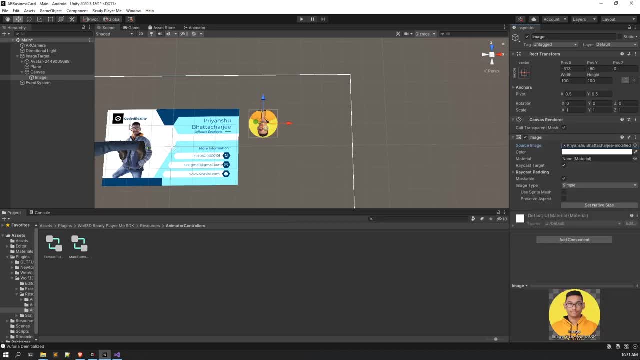 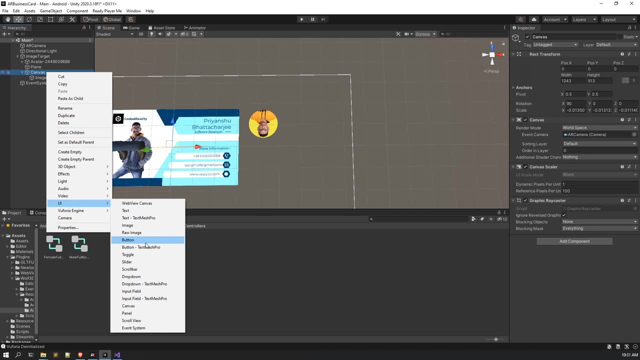 going to add it here, So I'm going to just select it and you can see. first of all, let me actually. I guess the rotation of the canvas is different. let me check. yeah, the rotation of canvas is wrong. just wait, let me fix the rotation. okay, alright, 180. alright, now let's get this particular. 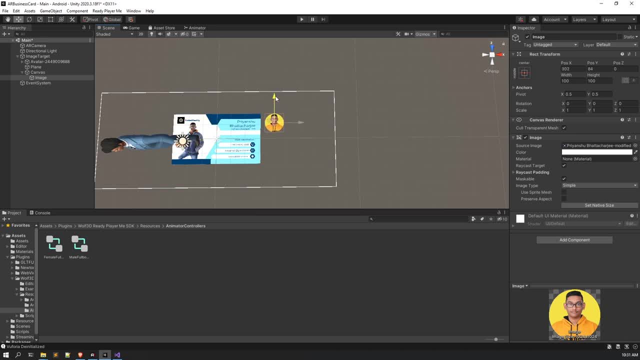 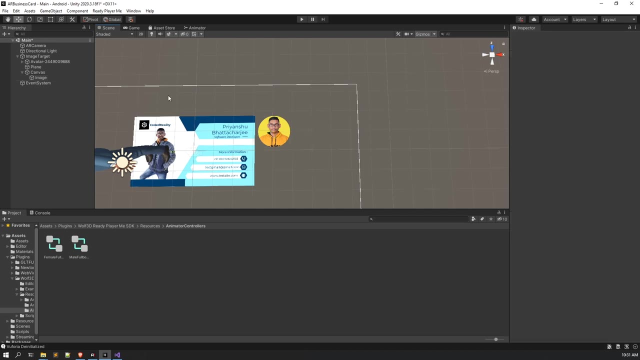 image, So I'm going to drag and drop this image into the right place. okay, cool. So now we got our image right in here, alright, so you can, if you want you can like- increase the size of the image, alright, and let's add a name text on the side of the image. 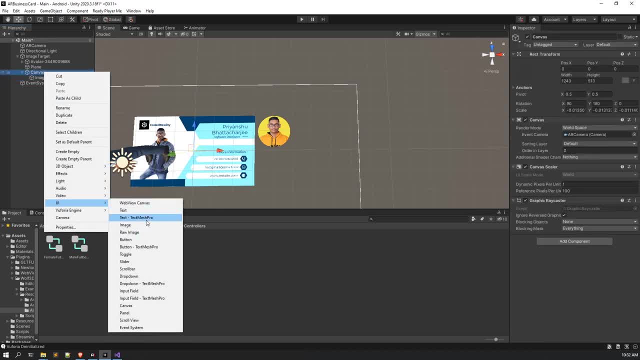 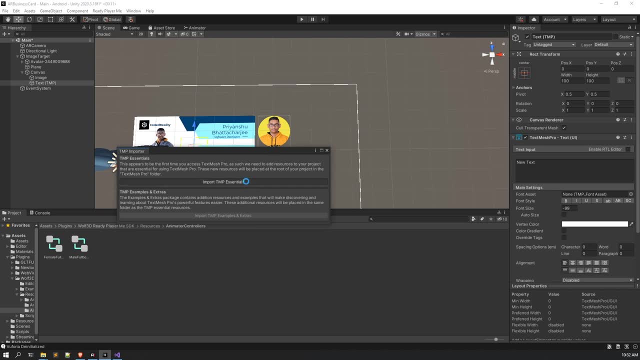 So how do you do that? click on UI, then click on text- mesh pro alright. import the text- mesh pro alright, Because this is the best for button and text, both alright, and it would start importing the assets. so it's going to take some time, so give it some time, alright. 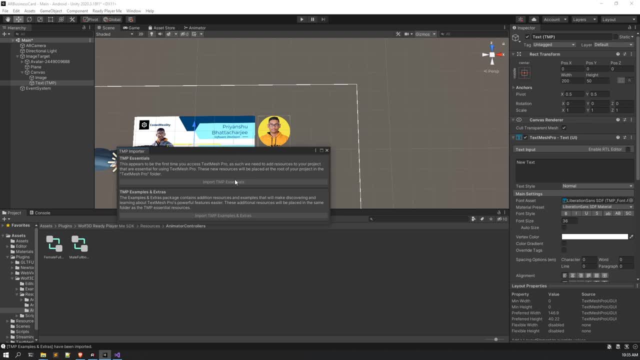 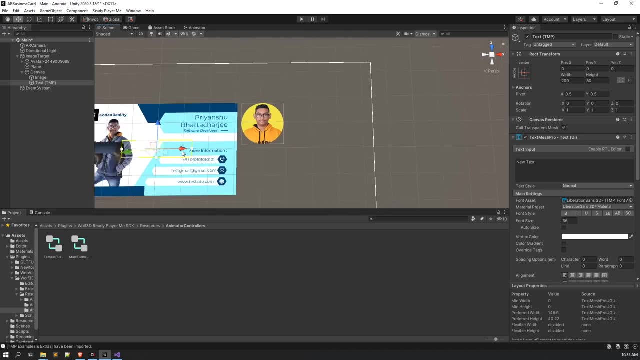 So I have imported the text mesh pro- alright, and also I have also imported the text mesh pro examples and extras alright, because it already provides some really good fonts, so I'm going to use them, alright. Now, as you see, we have, you know, the text in here. 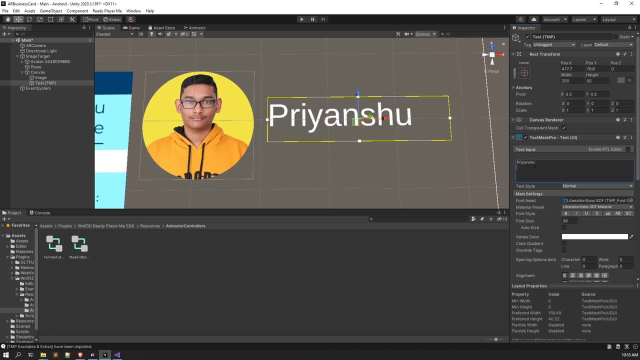 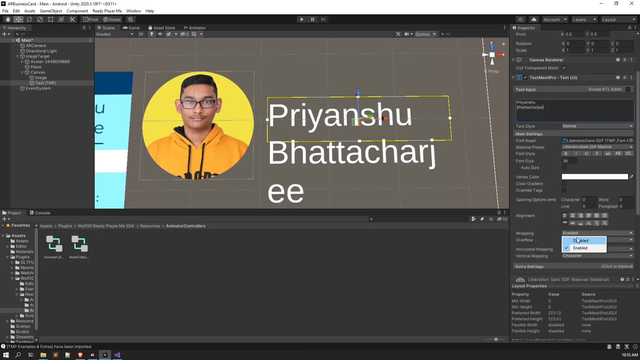 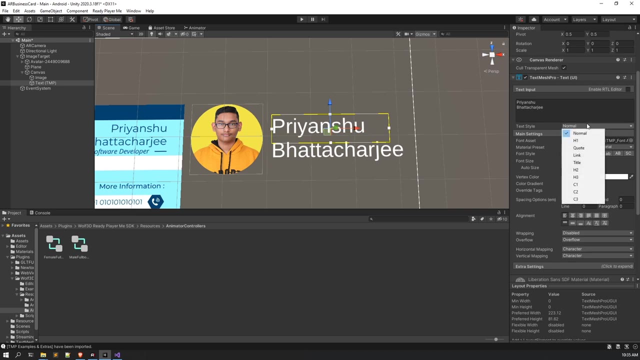 Now write your name in here, so Priyanshu Bhattacharjee. alright, so what I'm going to do is I'm going to like in the wrapping, I'm going to disable the wrapping, alright, because I don't need it now. let's see, let's let's choose a font from the given set. alright, let's see which. 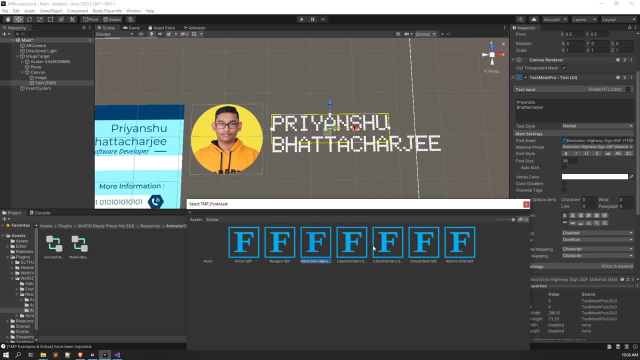 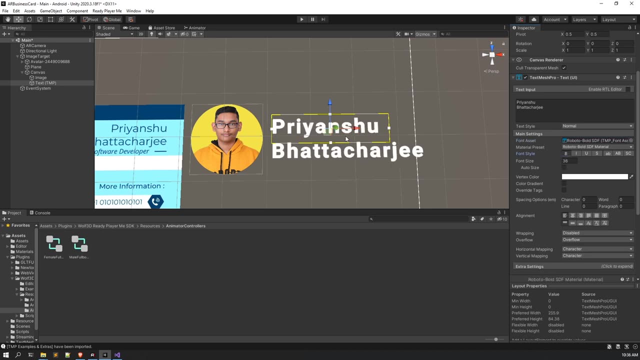 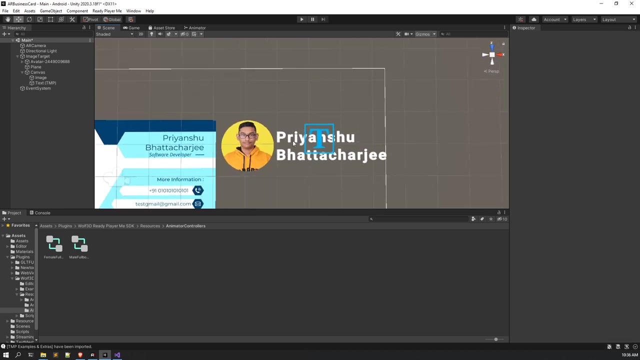 one would be good. okay, not this one, of course, not this one. no, Let's see, Yeah, this, let's check the Anton one. okay, so Roboto looks good. alright, this Roboto one looks pretty good. Now, what you can do is you can adjust it. alright, adjust it more. I think this, this is good, this. 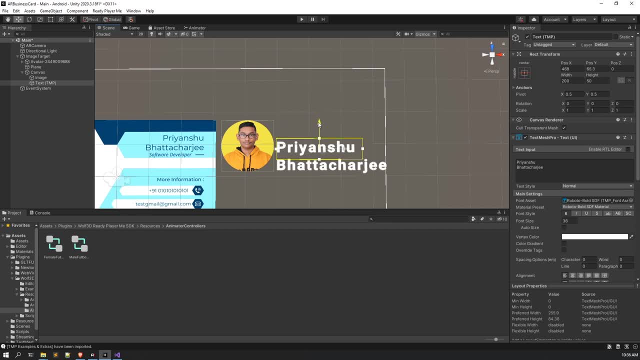 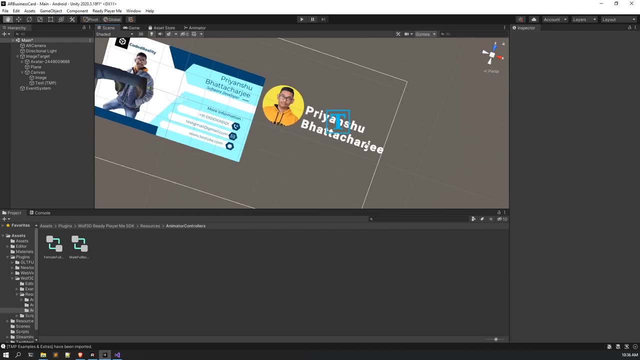 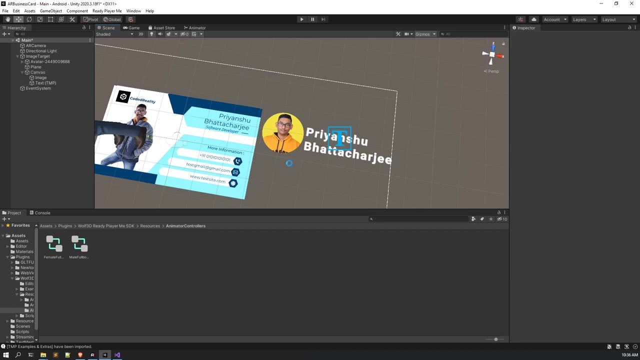 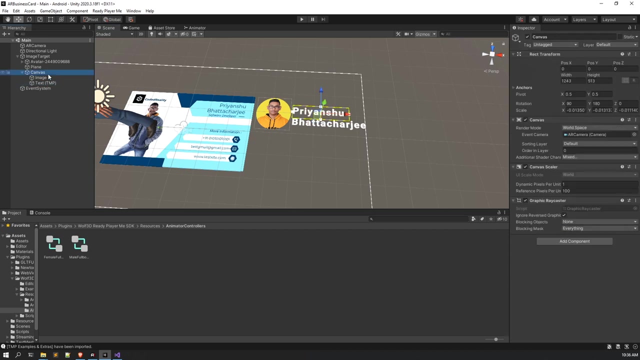 looks. just wait, okay, yeah, no, just wait, let me adjust it a bit, alright, Okay, Okay, Okay, Okay, Yeah, this, this, this is pretty good, this, this looks fine and alright. So now we have set up this particular profile thingy, right now what I want you to create: 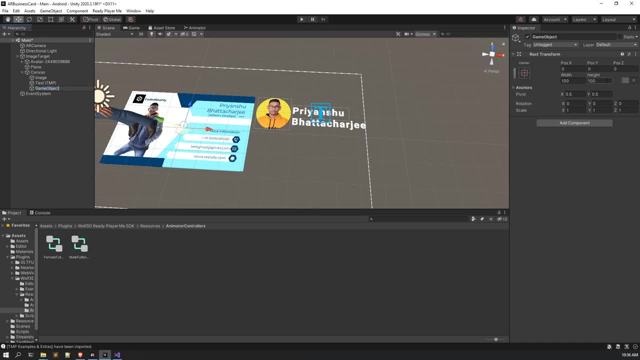 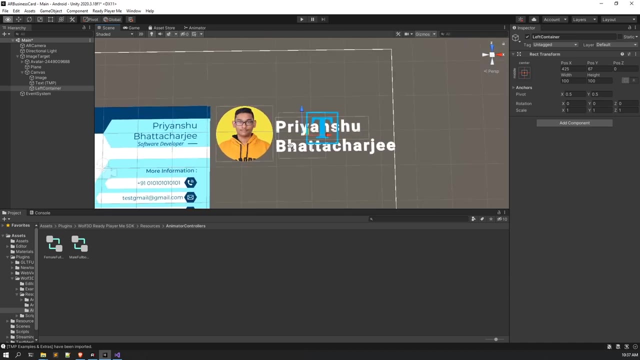 an empty prefab, alright, right in here. alright, create an empty the game object and let's name it left container. alright, because as we are going to add animations to it, alright, So I'm going to position it in, you know, in the center of these two assets. that is the 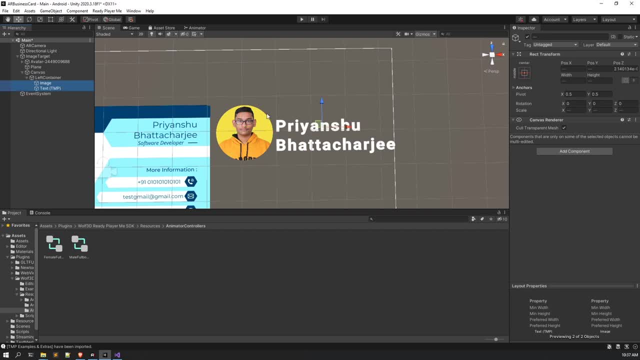 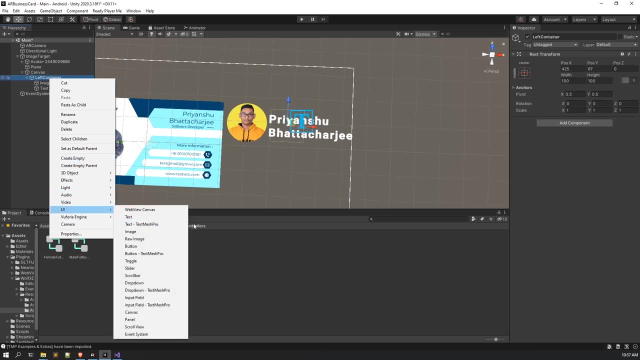 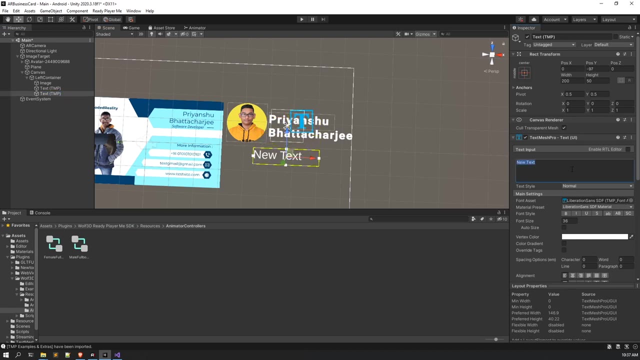 image and the text. put it in the left container, alright, and let's you know, sort of add a bio in here, okay, so this would be a short bio. so I am pretty much, let me write, let me complete the bio, And then I would again resume the video. 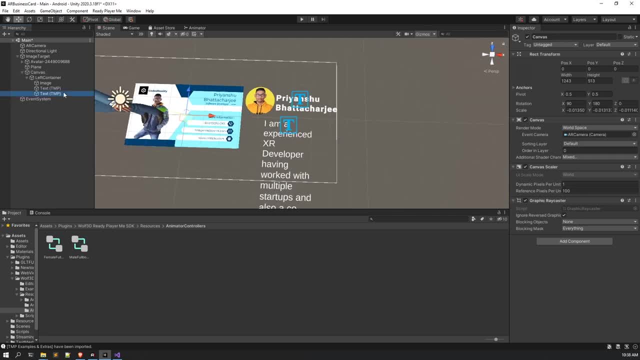 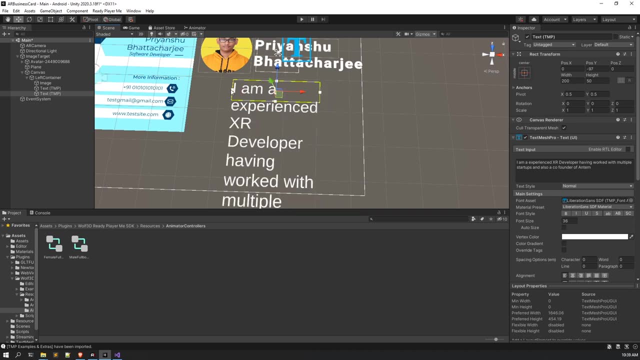 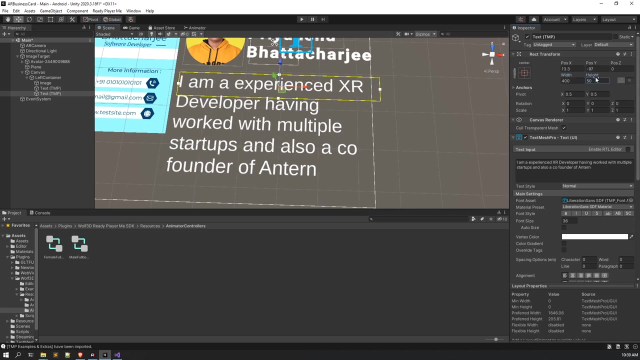 So I wrote the bio. all right, now I have to adjust. let's adjust this bio right in here, alright, so that, like you know, this of course doesn't looks good, and just give a moment, all right, Okay, Okay. So let's give it a height of 400, not 400. let's give it 200, okay, yeah, this, this looks good. 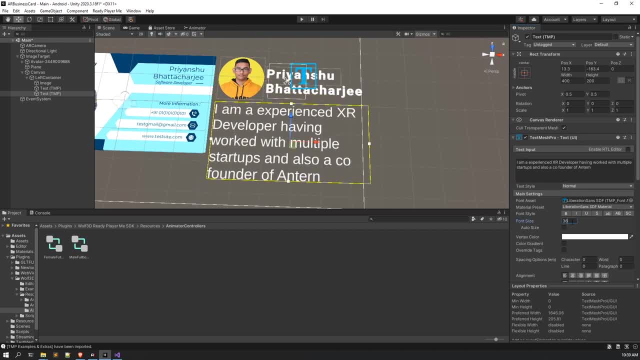 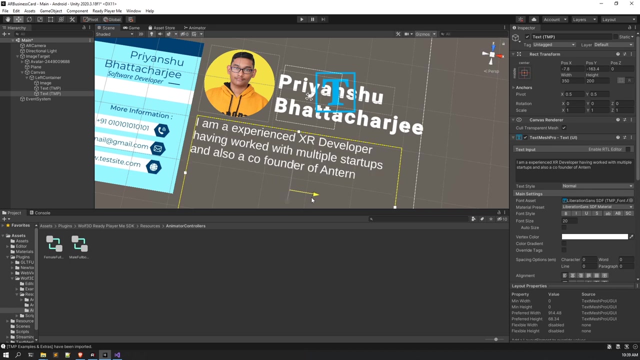 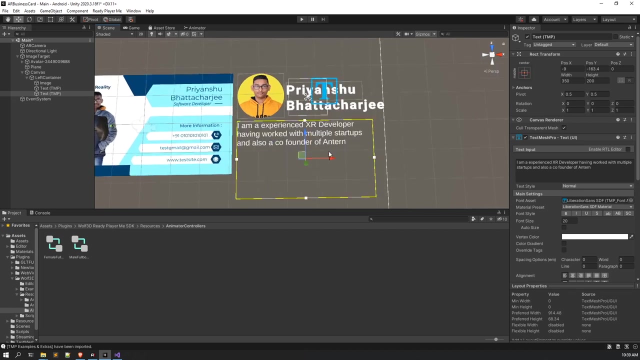 now let's reduce the size. alright, let's make the size 25, maybe, or 20. yeah, I guess, I guess it's fine. let's make it 350, alright. yeah, I guess this is fine, Okay, Okay, This looks fine. now, align it a bit. alright, align this thing a bit, and actually let's 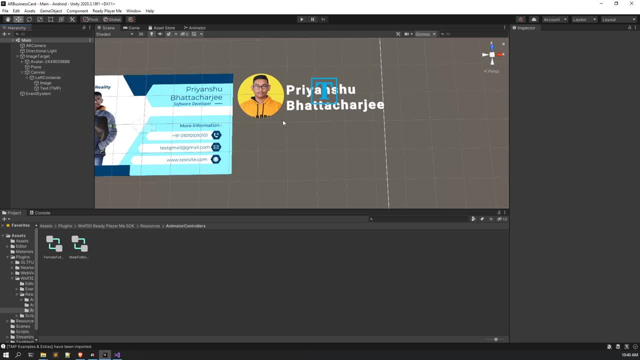 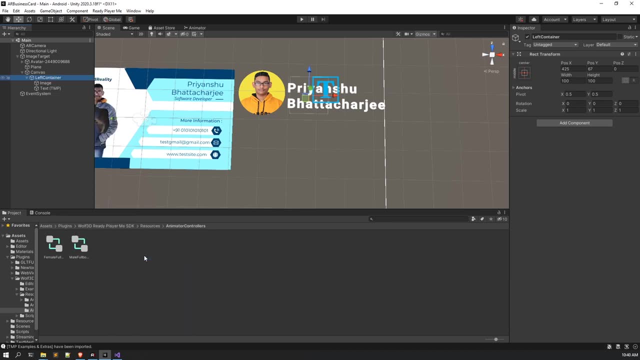 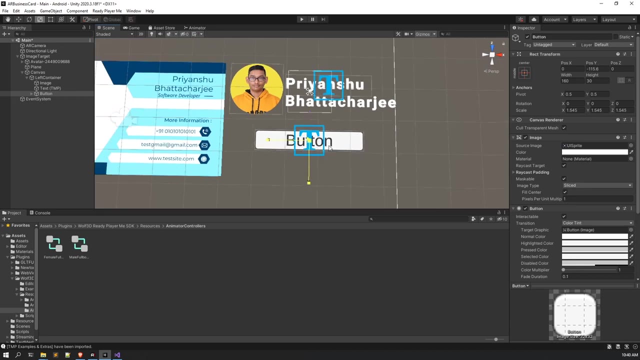 remove this intro thing. alright, let's add two buttons in here. alright, let's add two buttons in here. go to UI. click on button. text match pro. alright, go in here, you know, increase the size of the button. alright, increase the size of the button. put it in the middle, maybe. 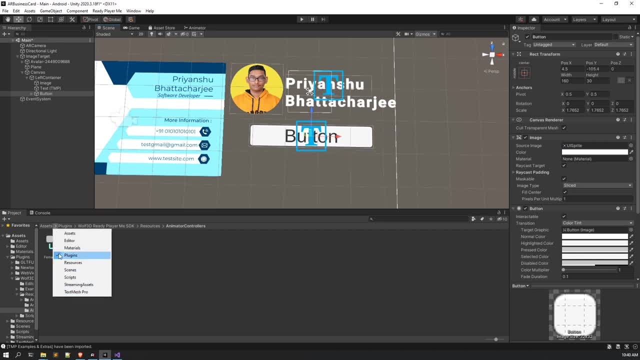 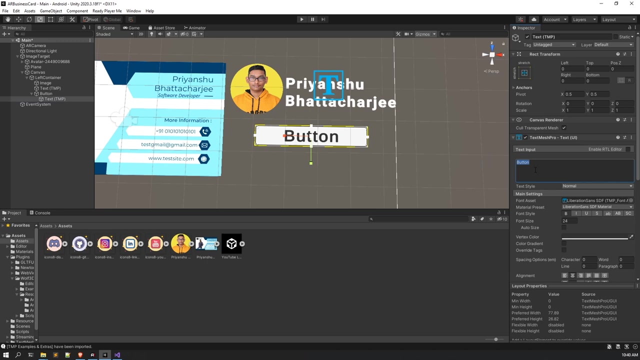 alright, and I have wait. I have the logos right in here. go to assets. okay, let's. let's make two button for our social media, that is, you know this, Instagram and LinkedIn. alright, so I'm not going to remove this particular text, I'm going to make it bold and let's name it linked in, alright, so, and let's reduce the. 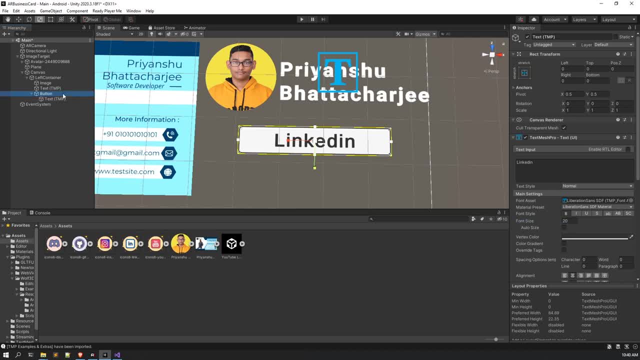 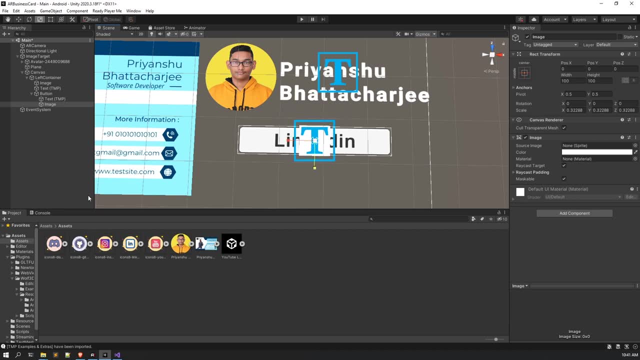 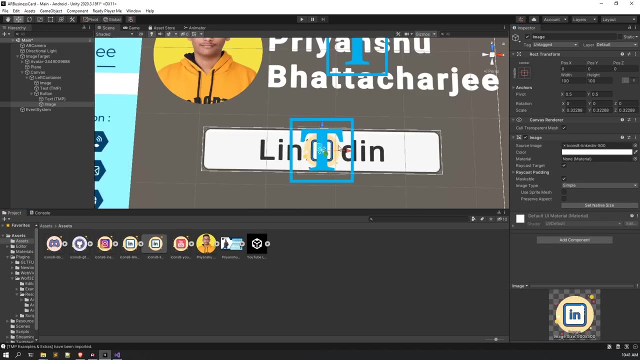 size, that is, make it 20, alright, and in the button only click on UI. then again add an image, alright. reduce the size in the image. add the LinkedIn. you know, link this LinkedIn image in here, alright, and drag and drop it to the side, right, Okay. 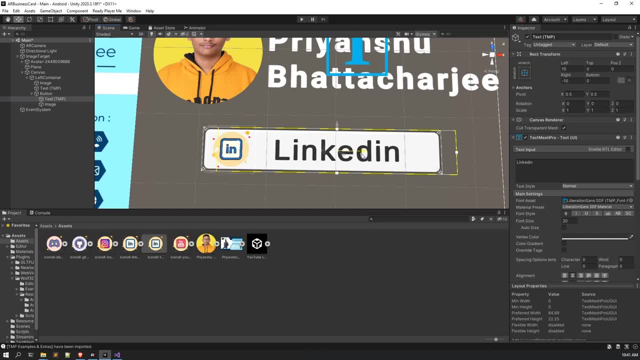 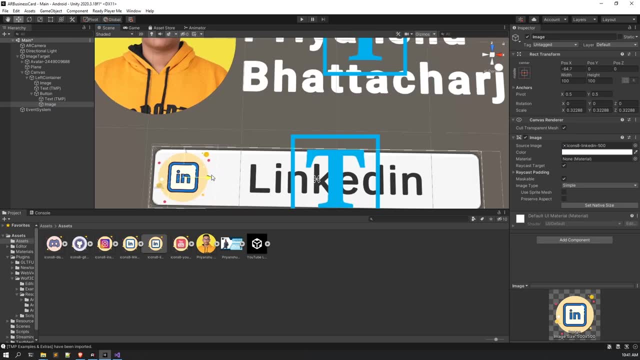 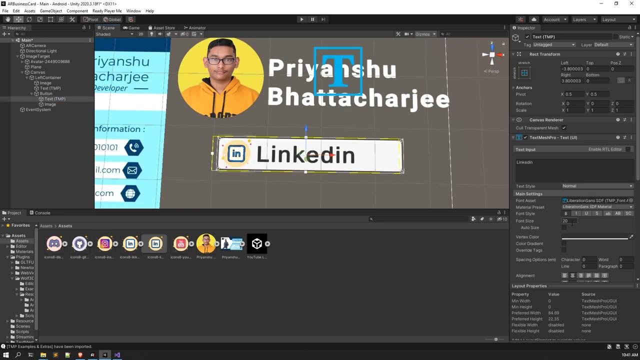 Let's put it in the side, make the text a bit centered, right? okay, let's make it a side. alright, let's just give me a second. let me reduce the size of the text again, that is, let's make it 17, maybe, okay, sorry, 20. I by mistake I give it 27. alright, cool, now I would. 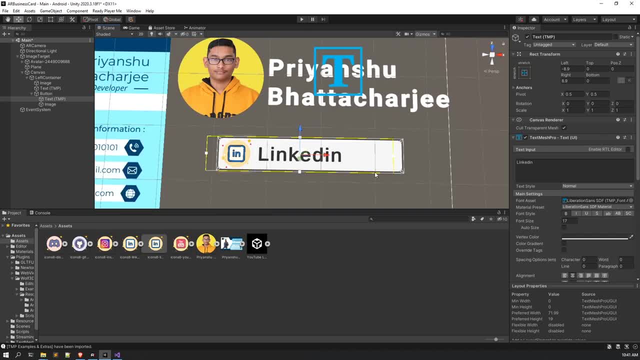 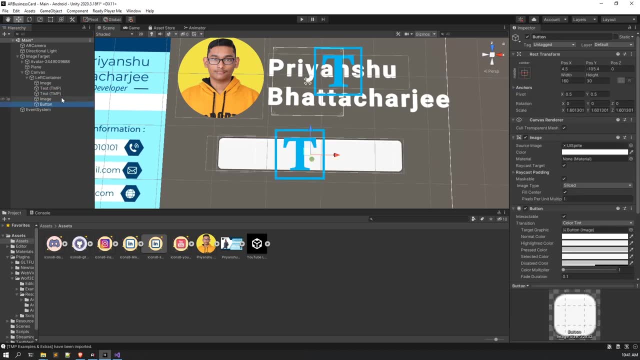 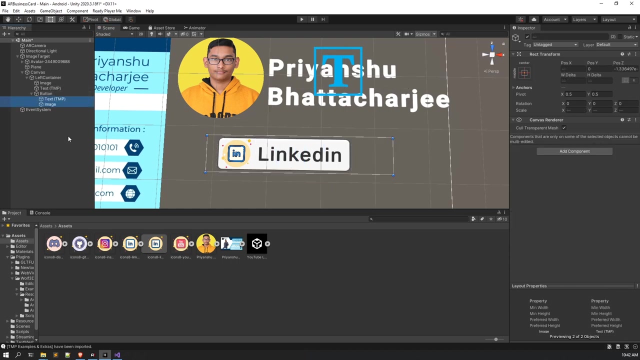 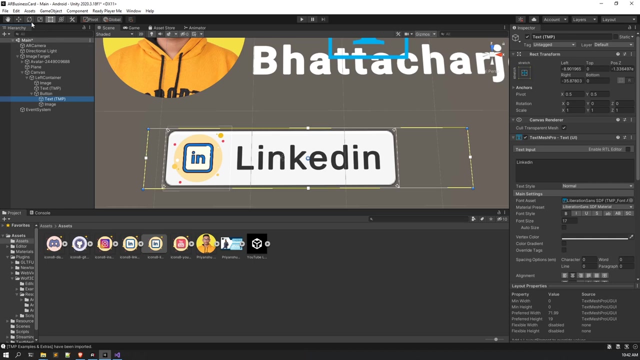 also like like to just wait, Okay, So I would also like to reduce the size of the button. so just simply remove these texts and from there. alright, now just wait, let me reduce the size of the button. okay, good, now again you make those text and images the child of the button, right, so let's adjust it a bit. 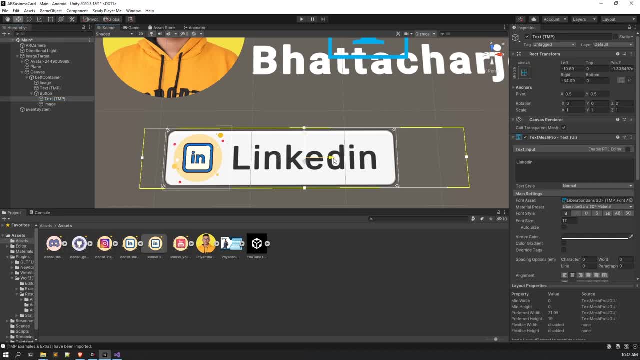 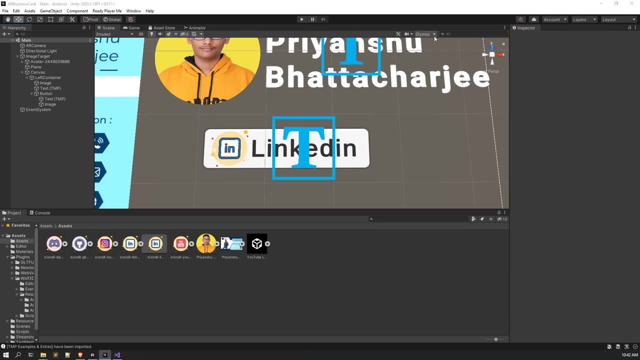 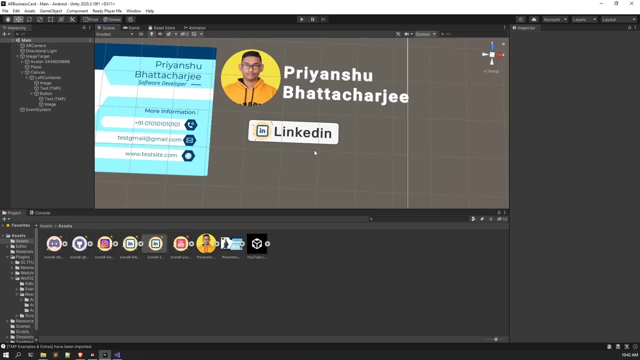 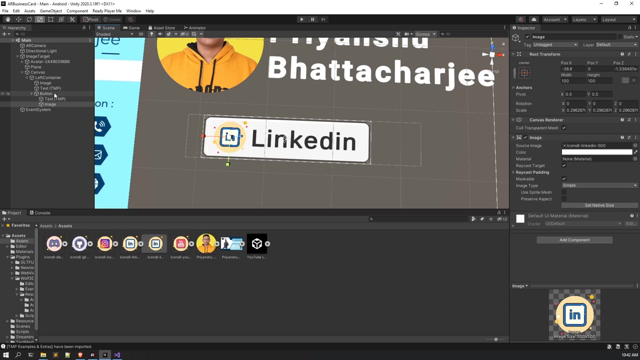 again. all right, yeah, this this looks good. okay, and also, go to gizmos. alright, and go to gizmos and you can see this 3d, 3d icon slider. just make it small, alright, so small that you can't again see those things. alright, and okay now, yeah, this looks cool. so then. 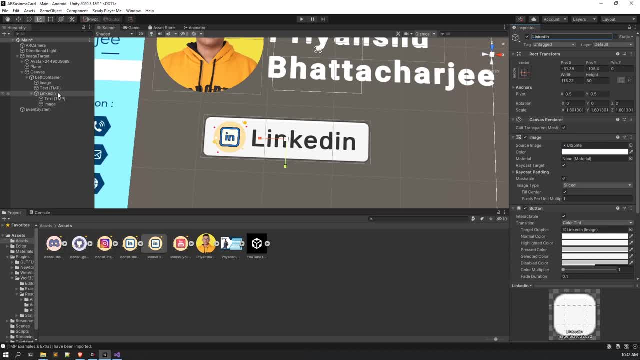 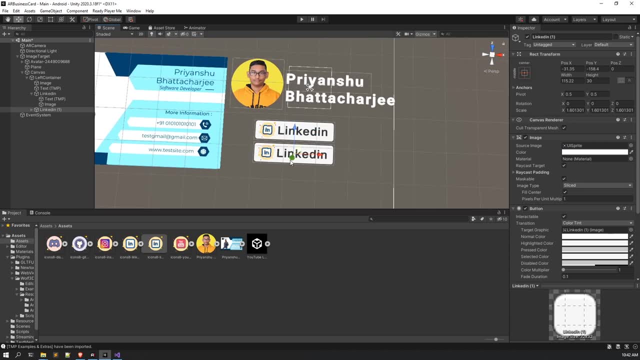 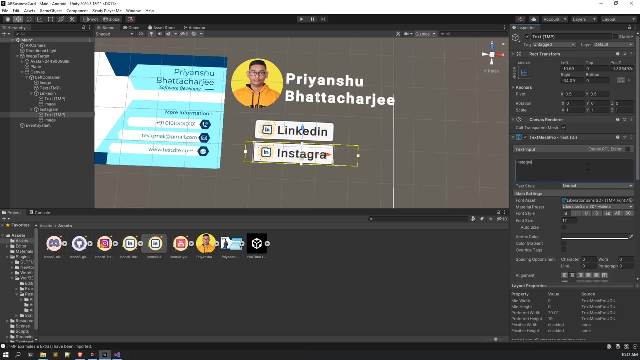 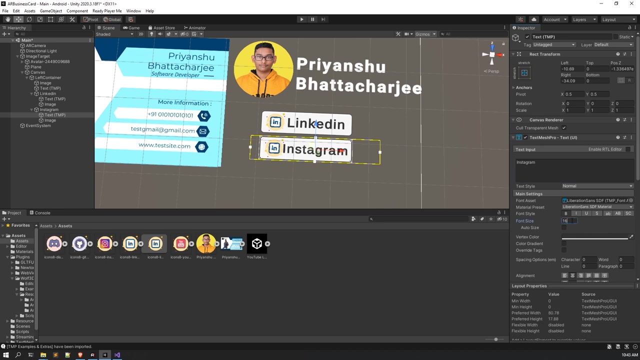 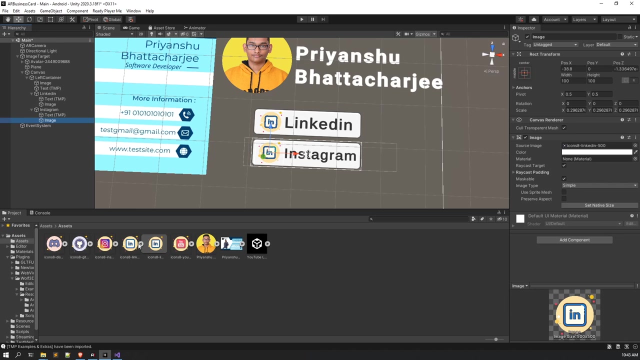 name it linked in. alright, Then again, Then again. you know, duplicate this button. alright, put it in here. alright, and let's name it Instagram. alright, so give the text Instagram. alright, so let me reduce the size a bit for this one, Okay, So I'm going to change it to 15, okay, alright, here we go and change the image to the Instagram. 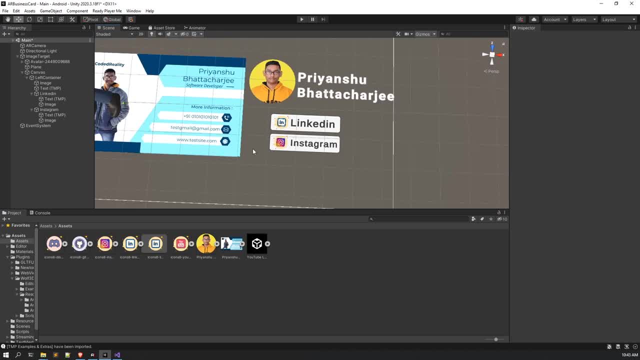 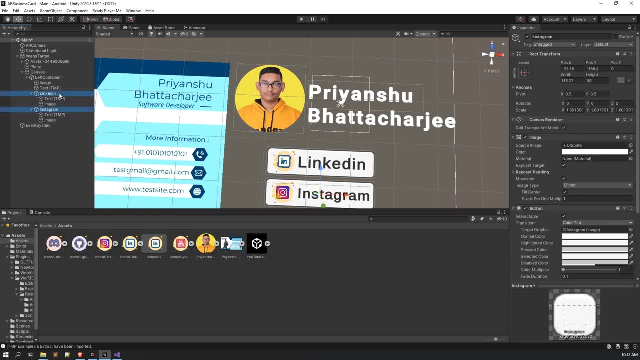 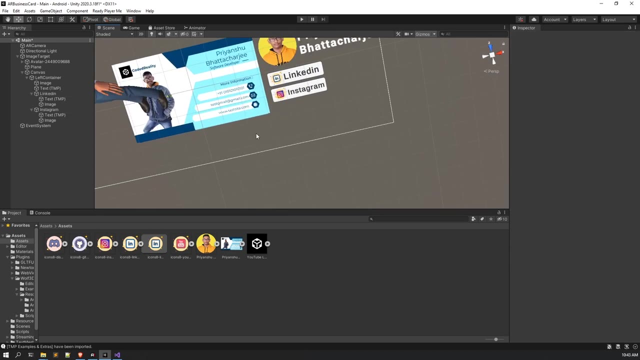 image. alright, and yeah, so we got our buttons in here. so now you, what you can do is you can simply, you know, take these two buttons, alright, take these two buttons and simply put it right in here, alright, or let's try some, let's try making this button. 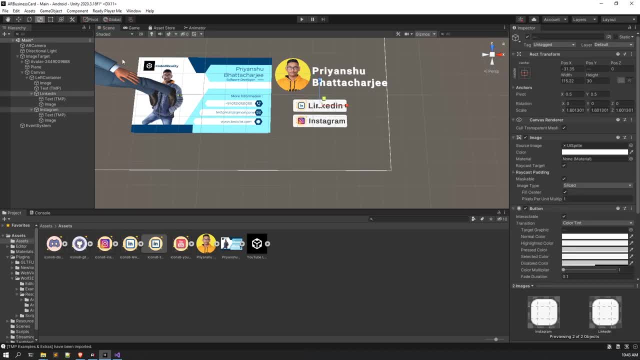 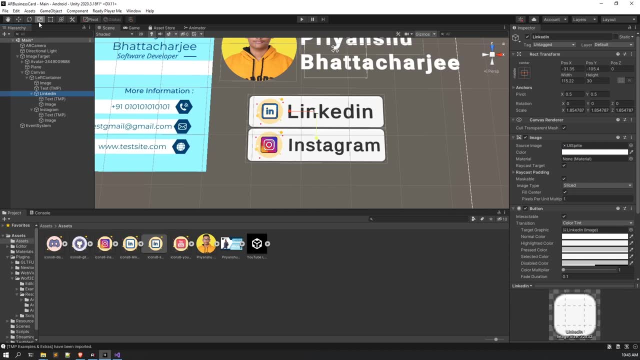 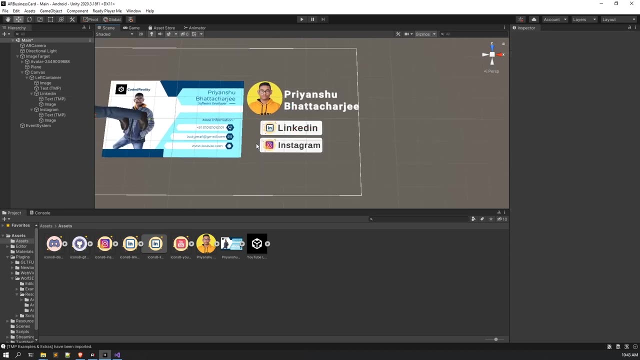 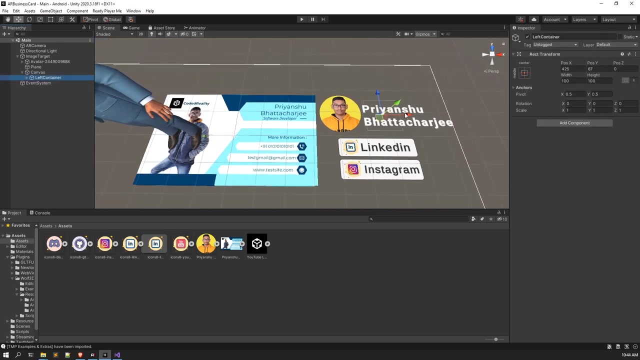 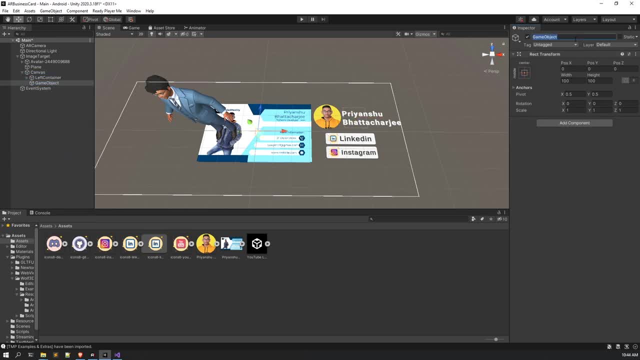 container, alright. Let's create an empty container. Let's give it a bottom, alright, that is, it would be in the bottom container, alright. so bottom container: now in the bottom container again. place that. add an you know UI. that is an image, right, add an image in here. give this image a new you know component that has button. 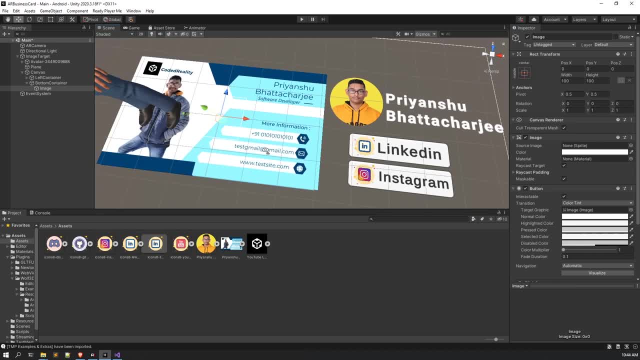 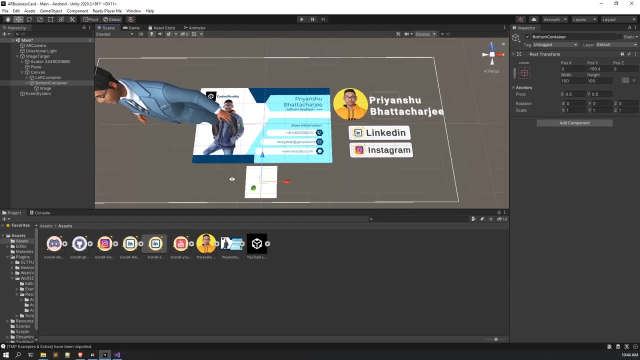 component. alright, because we would be using them as buttons. All right, All right, Now get this container and drag and drop it in here. all right, So get as if you don't get that compact container. all right, now what you have to do is take this. 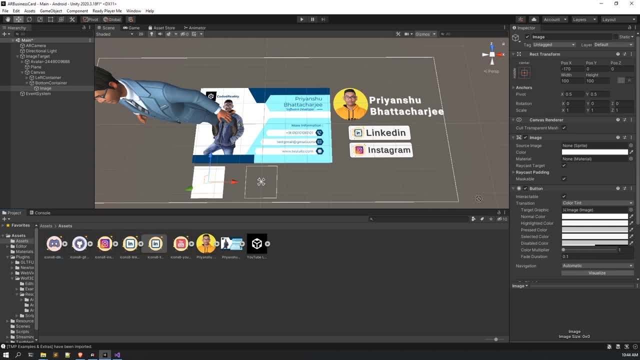 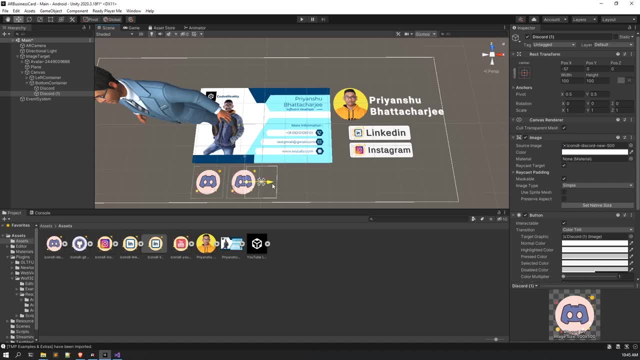 All right. Now I have to put it in some other place and place it in a bit. you know, change the position and place it in the side of it and again drag and drop the github- you know, github logo- and again duplicate it. all right, and now it's the time for, you know, YouTube. 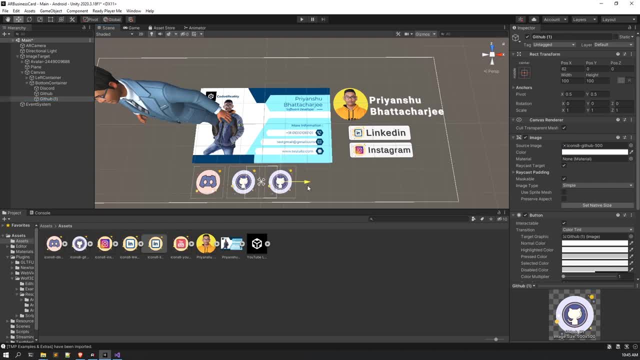 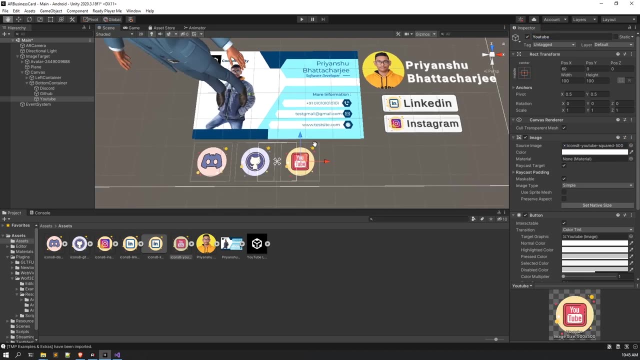 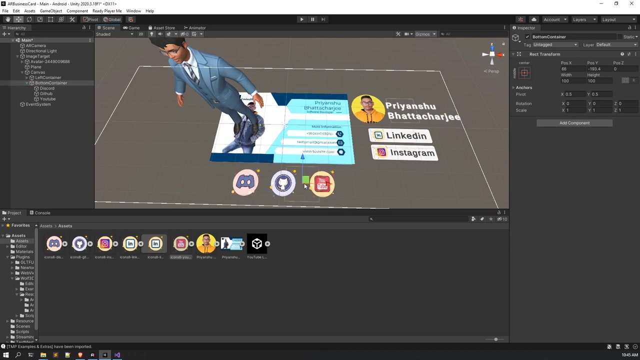 So now rename it to YouTube, All right, Now what you can do is okay, so, yeah, so we got our three button containers, all right, and make sure to place it in the center, all right? um, let me reposition this. you know, the button of. 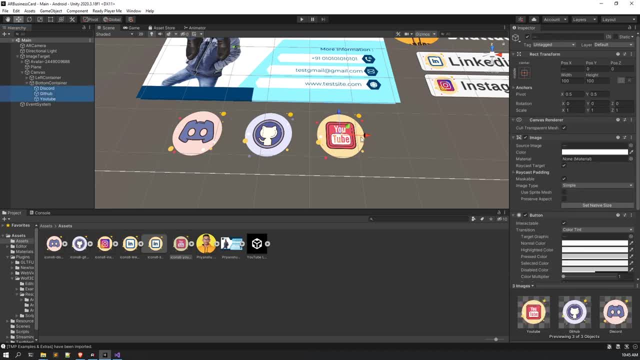 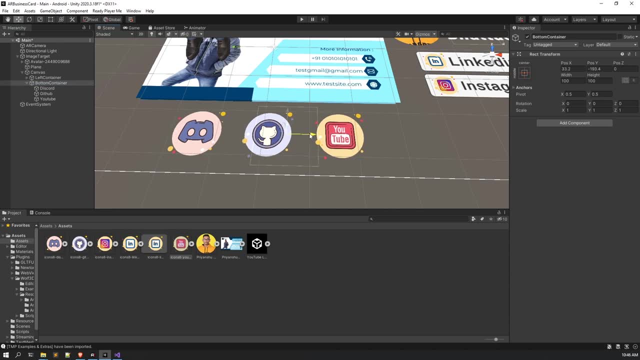 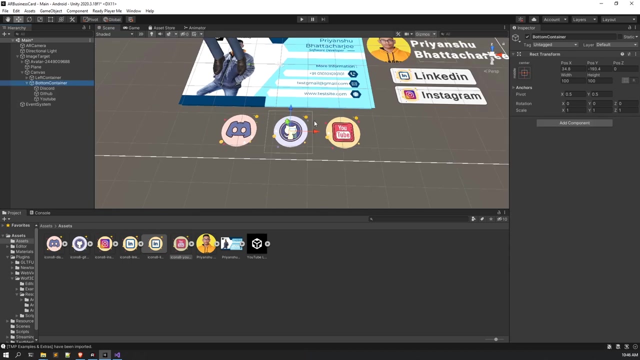 for just wait, let me reposition this. all right, just give me a second. let me make all the things in center. just give me just just a moment, all right, okay, yeah, now i guess everything's fine, right, so now we have the buttons in here, all right? 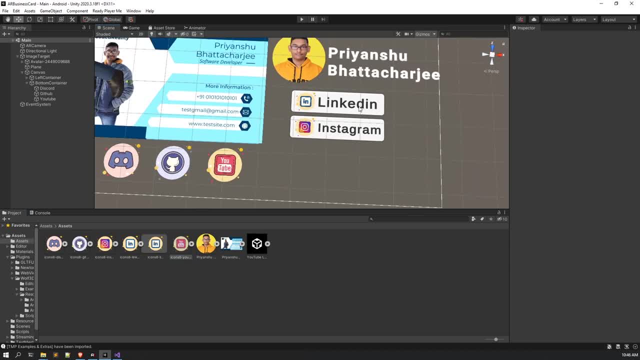 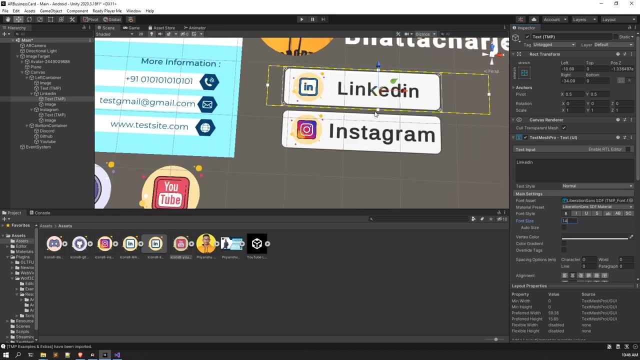 we have all the things that we would be needing. let's uh again. let's reduce the size, all right. so now we have the buttons in here. all right, we have all the things that we would be of this one too. let's make it 14, maybe, all right. 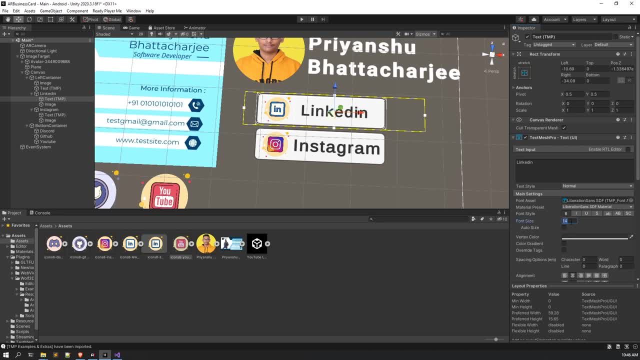 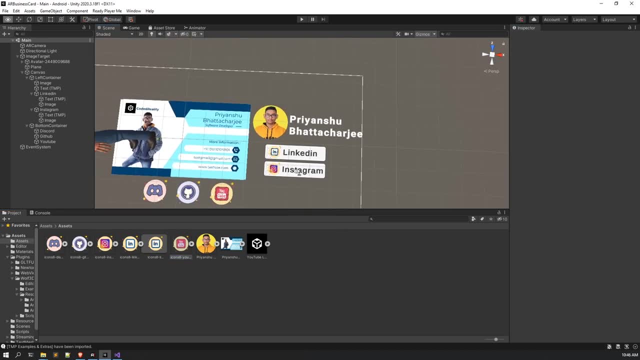 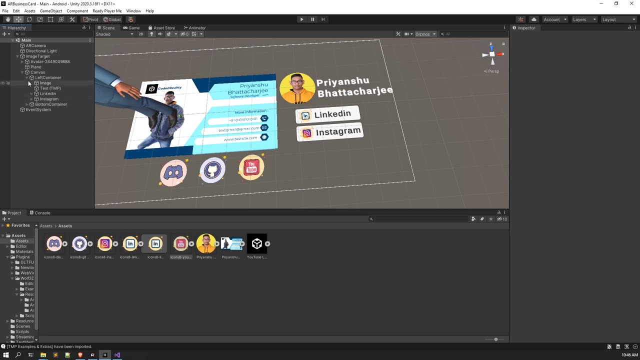 okay, no, let's go for 15.. all right, this looks good. so now, as our buttons are created, right now, what you have to do is we have to create a script. all right, because, of course, these, these buttons have to do something. right, these buttons have to do something. so what? uh, these buttons will. 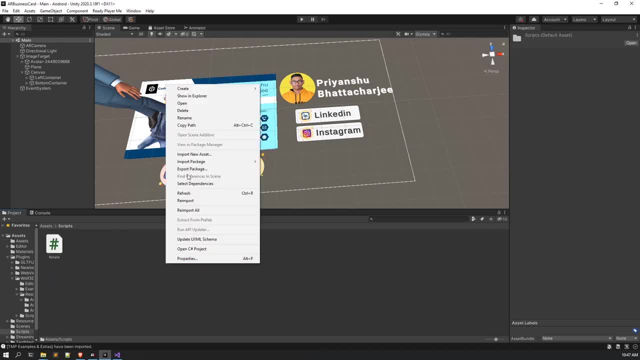 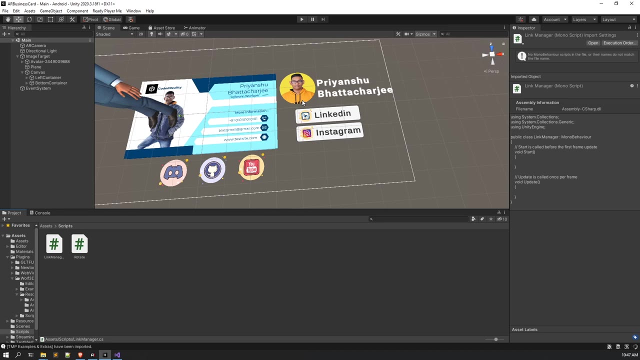 be used to open the links, all right. so how to do that click? or uh, create a new c sharp script, all right. and uh name it link manager, all right, because we would be adding the links in here, all right. and after it gets compiled, open the. open the link, all right. 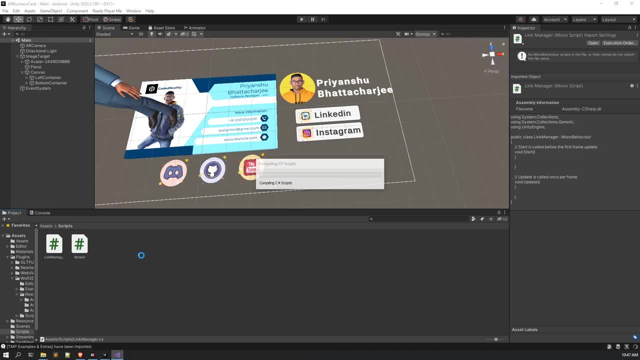 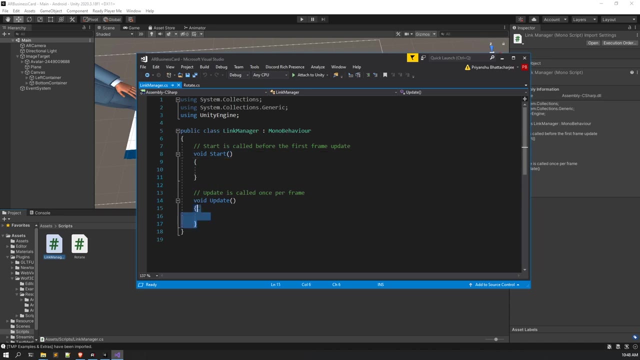 so so we have to write some, you know some functions. all right, to open the links, the. the script is pretty easy. so now, as our script is opened, all right, uh, everything's pretty simple. just remove all this comments and start and update function. we have to write our own function that is public. 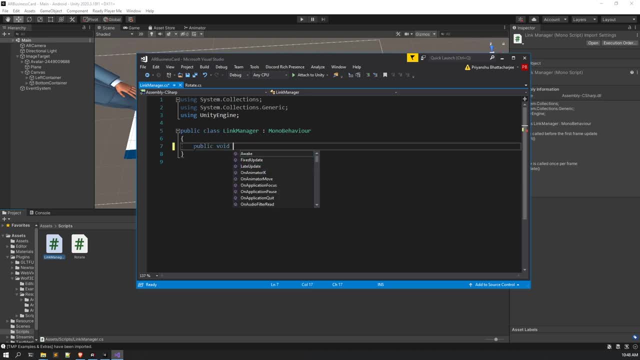 all right, void, i'll say open linkedin. all right, give, give the function name anything you want, right. and now, uh, within that function, we have to write a particular line, that is application dot open url. all right, and in that uh pass your linkedin profiles url, all right. so here i have the 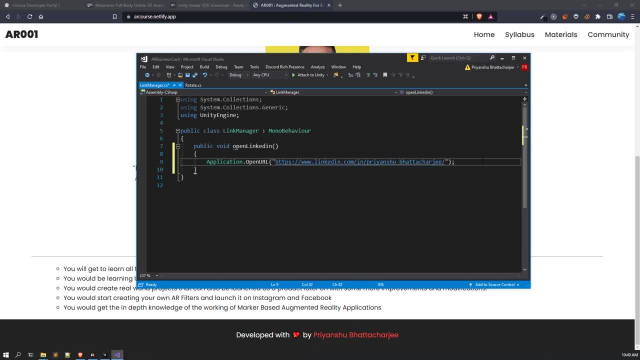 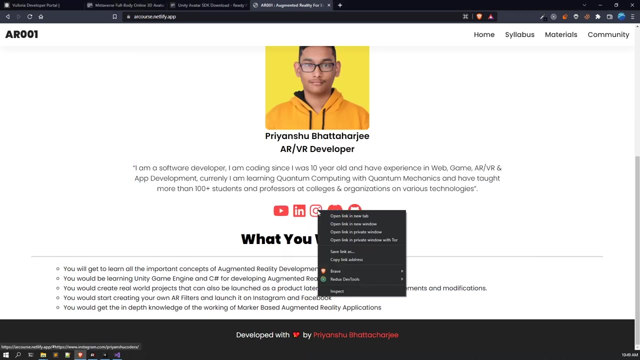 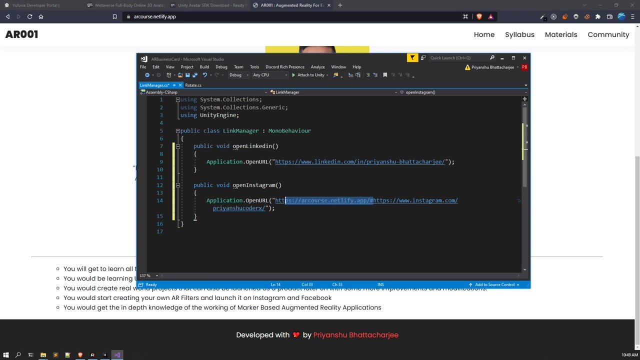 linkedin profiles url. and now i'm going to paste it right in here, all right. similarly, uh, write some other function that is public, void: open instagram. then again application dot open url. then, you know, add the instagram url, copy link address. okay, there's some problem with the link. all right, let's remove this. yeah, we got our. 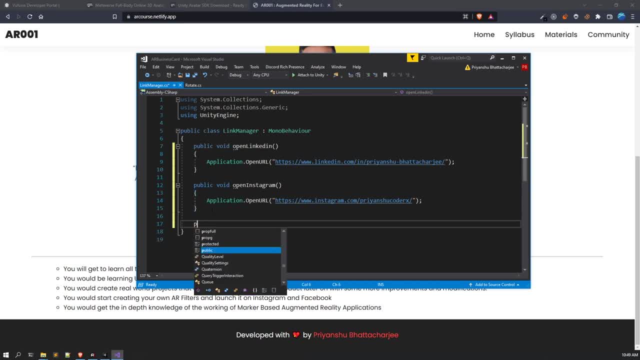 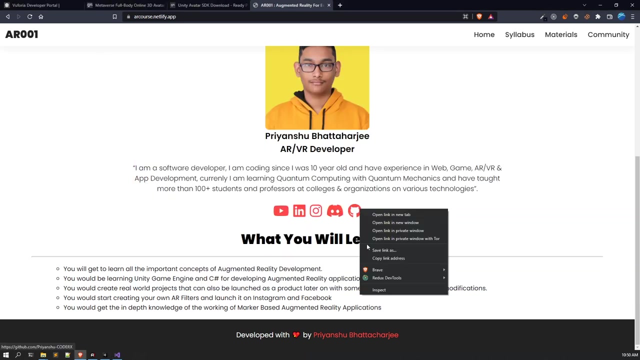 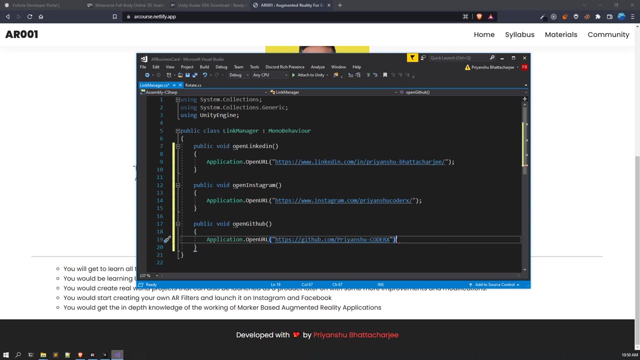 link. that is instagram profile. all right. now again, uh, let's create a another function that is open github. all right, so um application dot open url and let's put our github profile in there. copy link address. all right, so we got our github profile too right, all right. so now let's add: 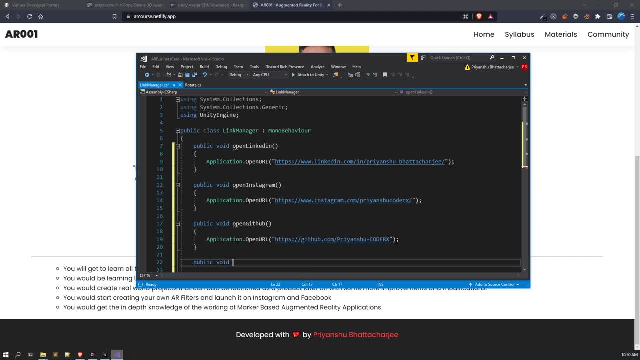 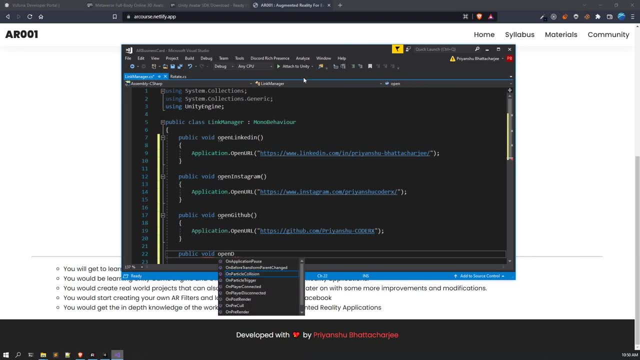 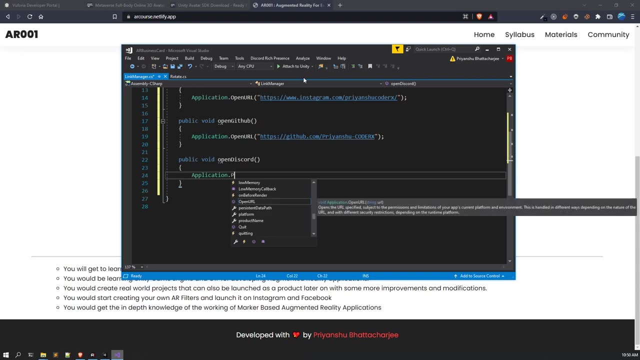 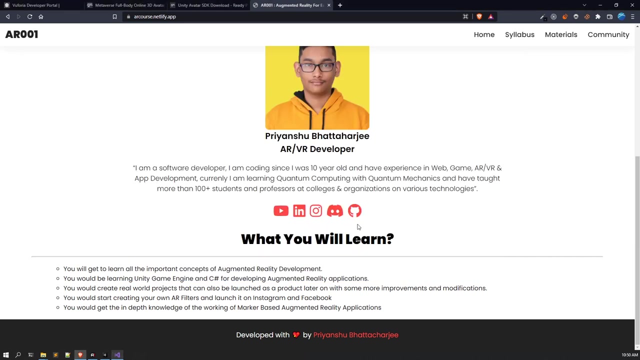 our. you know, uh, which one is left. now let's see discord. yeah, so open discord. so this is the discord server of lantern, so you can join that. so application dot, open url and uh, all right, just wait, let me copy the url. copy link address. all right, so here we have our github profile. 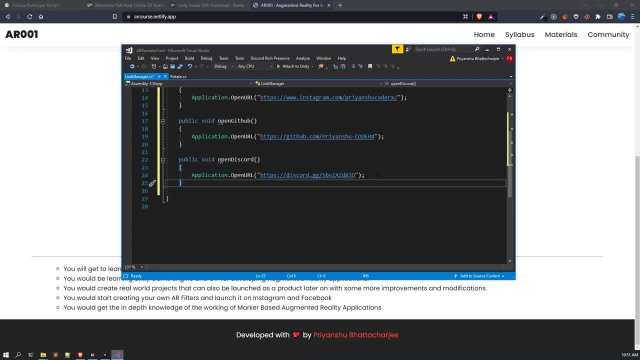 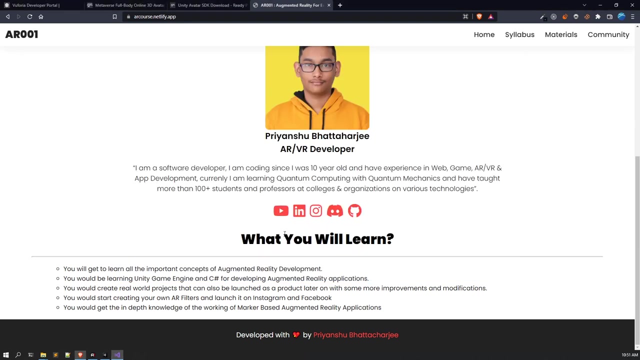 so here we got the url. all right. now another uh was youtube right. public void open youtube. all right, so application dot open url. now again, uh, put youtube in there. this is the. put the link of the youtube in there. all right, so i'm just going to copy the link. 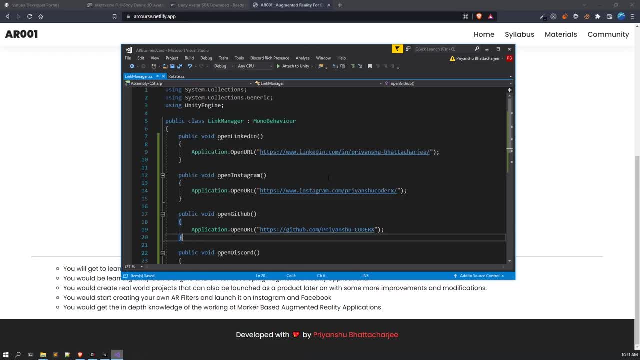 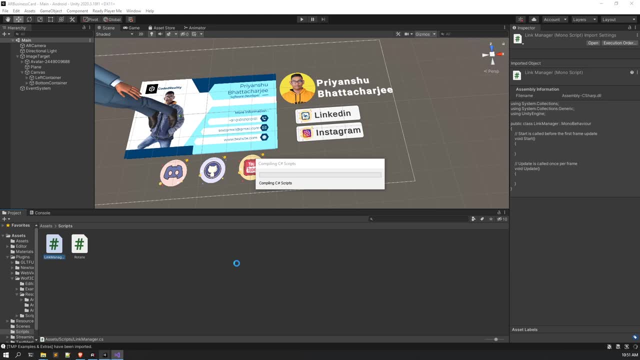 all right, and you know, just paste it in here and let's compile the script. so, uh, so our script is compiled, all right. now what you have to do is create a empty game object. all right, reset its transform. all right, just just do it. oh yeah, so reset. 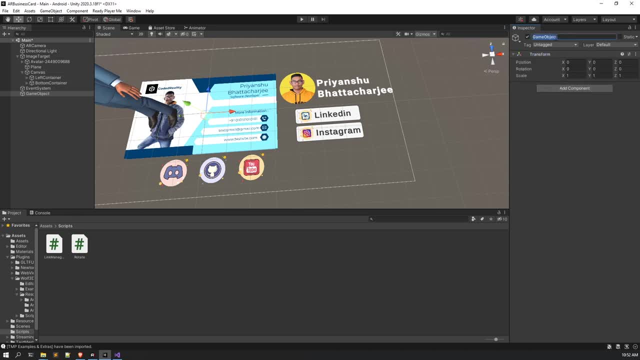 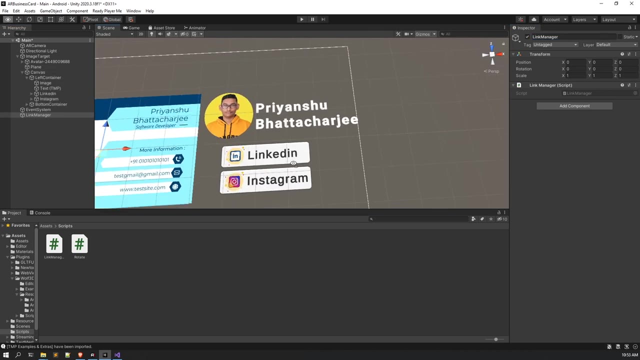 its transform and add this. uh also rename it to link manager. all right, because? uh, let's add: all right, because we'll be attaching our link manager script to it. all right, and attach this link manager script in here. now what you have to do is uh go to the first of all. uh, this is the. 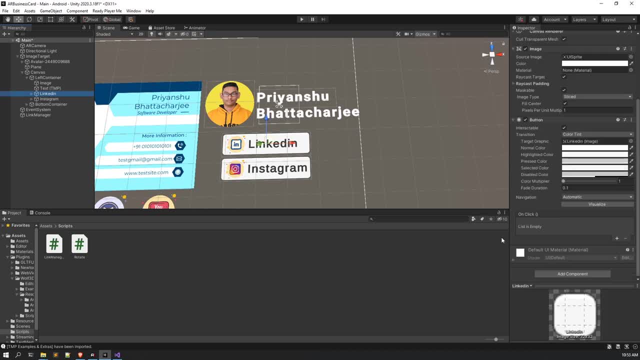 these are the button. all right. so first of all, go to this linkedin button all right in here. you can see on click, click and uh, click on add, then add the link manager, then click on link manager and find open linkedin. all right, so, and we got the open linkedin function. now again go to instagram. 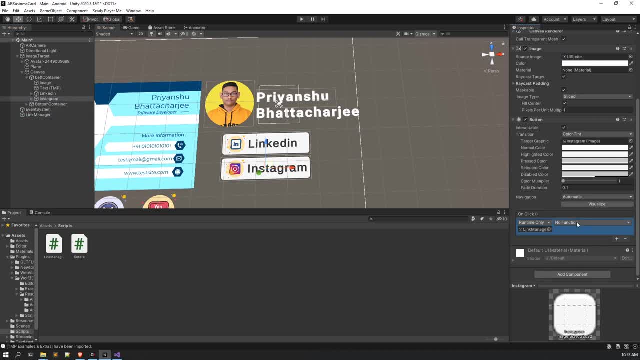 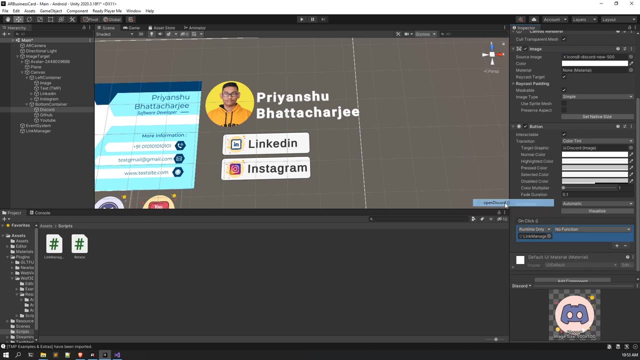 on click link manager: open instagram, okay, and in the bottom container, click on discord, on click link manager and then open discord. and again github- same. do the same thing for github, all right, so add the github one, then click on open github. again. youtube: add the link manager link, uh. then again open youtube. where is youtube? yeah, we got. 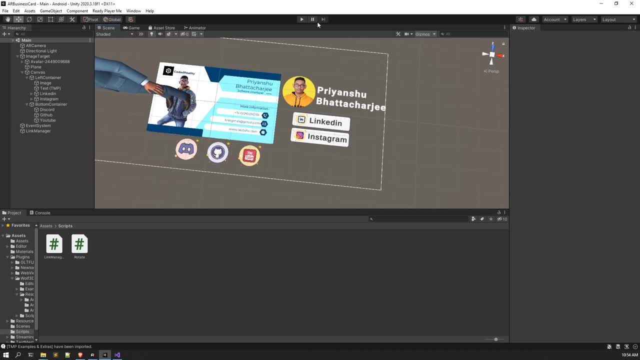 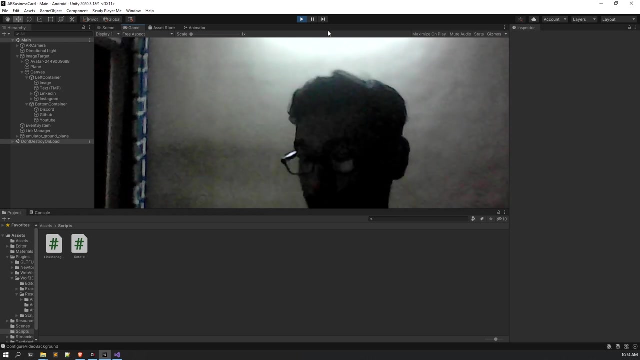 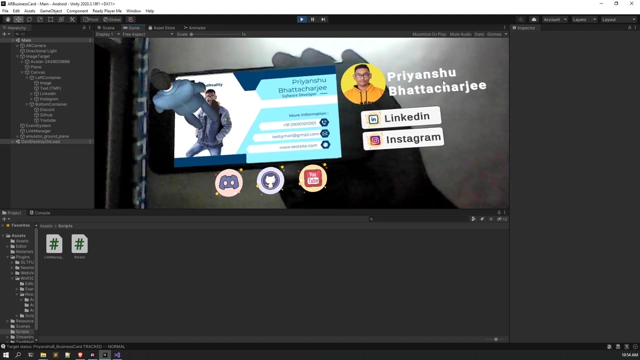 so that's how you do it all. right now, let's test if everything will is working fine or not, right? so just give a few second and let me show you. so here you can see that our business card is created, all right, and click on any button. 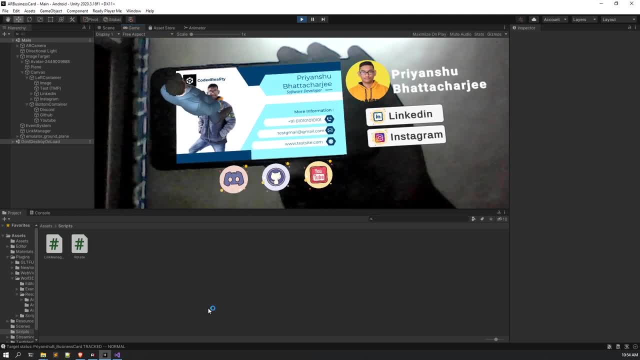 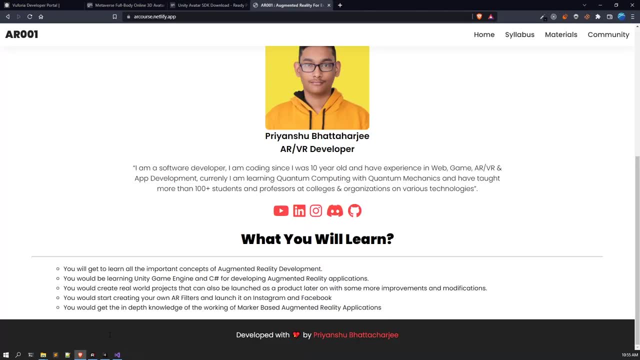 all right, let's say this: this discord button. so what will happen? it would start opening the url in my browser, all right, so here you can see: it has opened the url in my browser and so you can do similar things with that. you can add more features, all right. so let's see how it works. 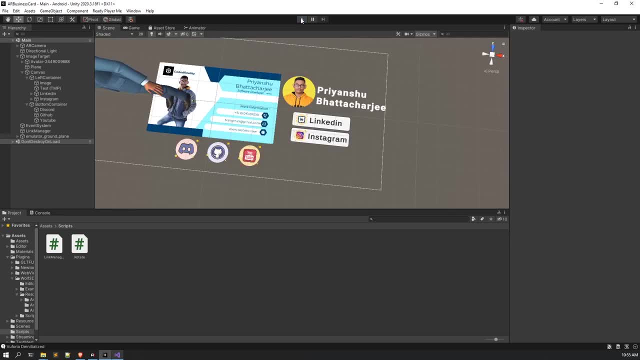 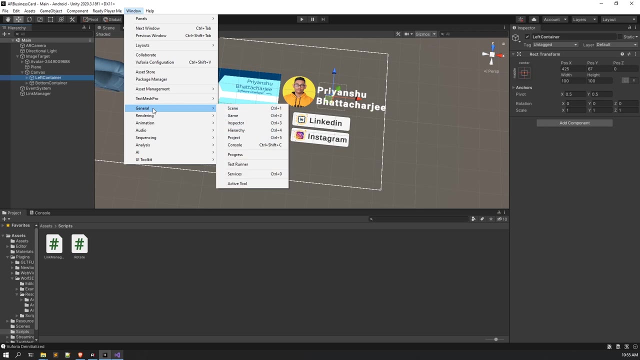 and now it is our time to add the animations to it. all right, so how would we do that? see, uh, adding the animations are very simple. what you have to do is click on this left container. all right, then go to your window. uh, go to- uh, sorry in here- go to this animation section and click on animation. 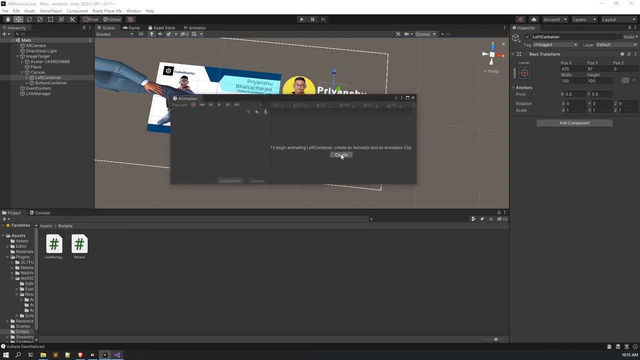 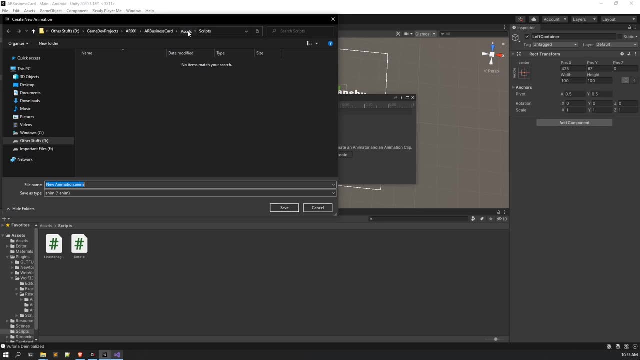 and a window like this would appear. so, uh, create, all right. click on create. then what you have to do is uh create a new folder in here. let's uh name it anims. all right, because we will be storing all our animations in there, all right, and 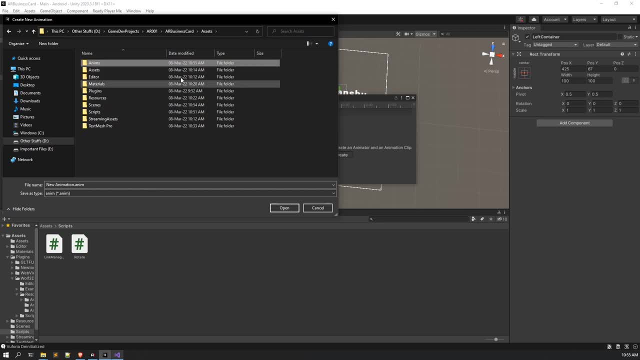 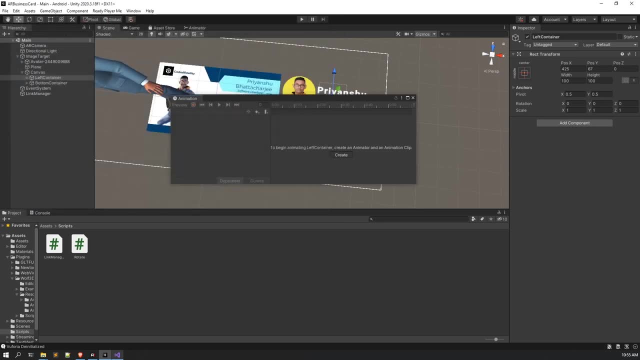 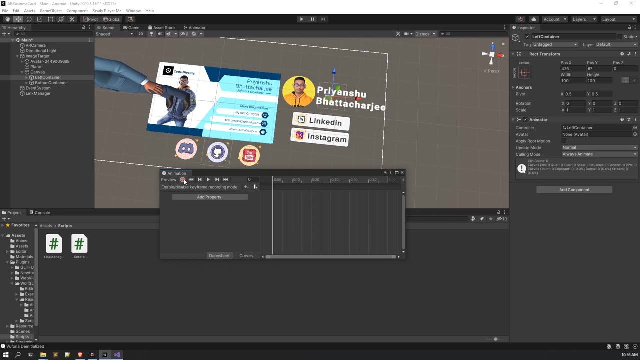 in the anims folder. give it, uh, give it a name called left container, left container, anim. all right, and save the animation. all right, now what you have to do is here you can see. first of all, see here in the record button. click on this record button. 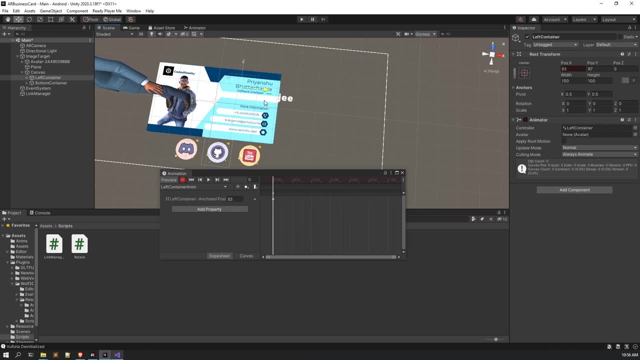 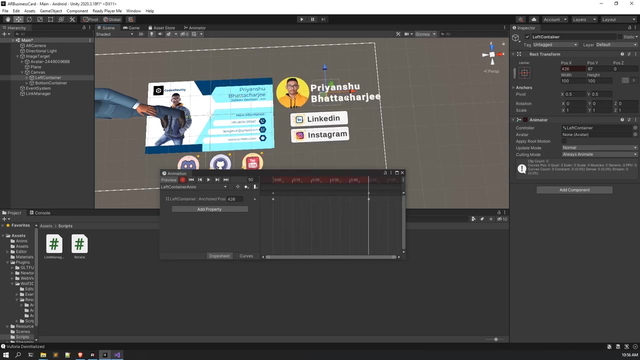 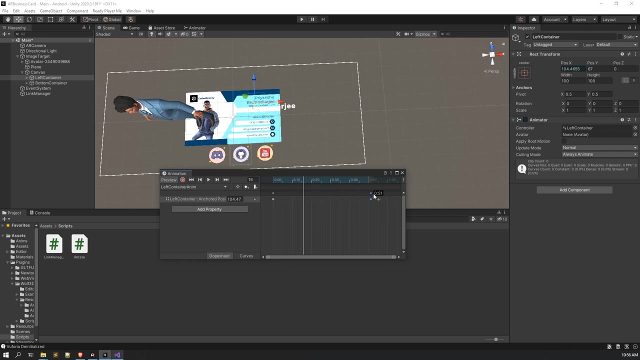 right, and you know, uh, put this inside, all right, put this inside of in here, all right now, uh, let's give it a, let's say, 50 second gap, all right, and again pull it back in here, all right now. let's see, okay, if, if you want, you can make things more slower by dragging it to like uh one. 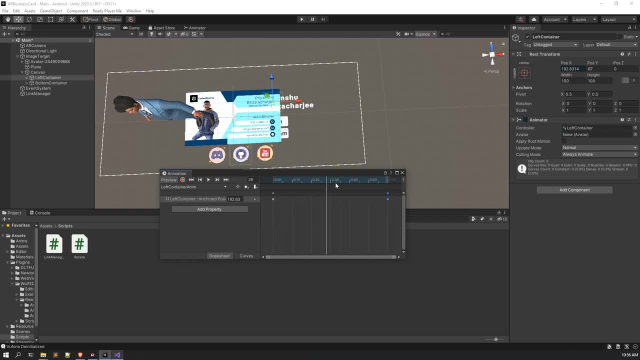 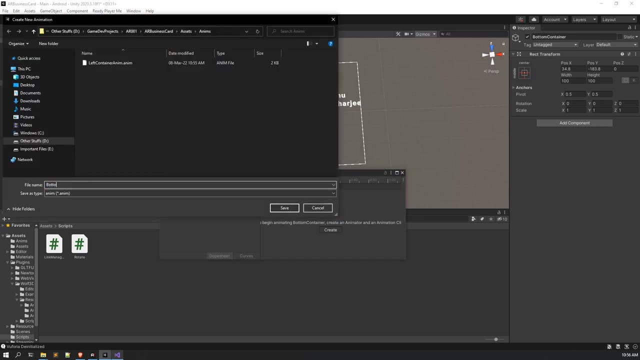 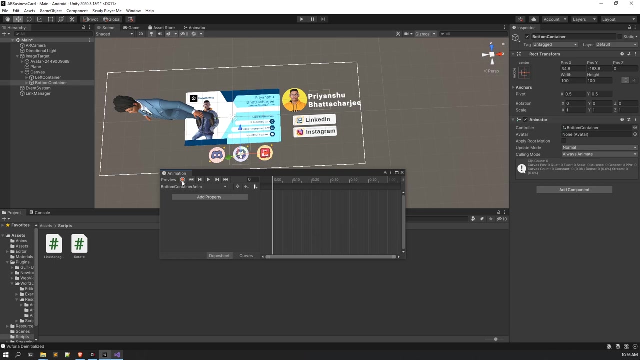 second gap: all right, so now our left controller anim is done. right, so let's make it up to full. all right. and now, in the, the bottom container, what we have to do is again click on create, all right, and let's name it bottom container, anim. all right, and save it. then again click on this red icon. all right, this record button. 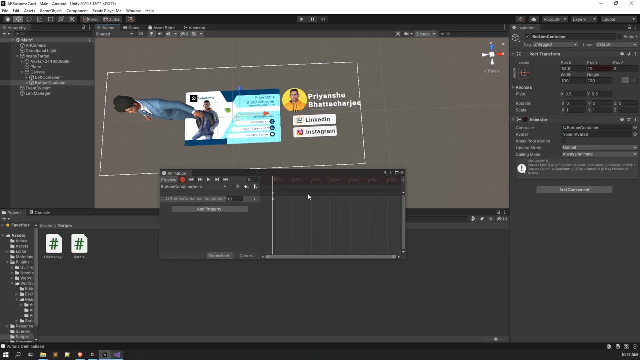 drag, drag it in in here, all right, drag it in here and then again go to one, then again bring it up in here, all right. so that's how we do it right. so that's how everything works, right. so now our animation is recorded. you can play the animation and see. 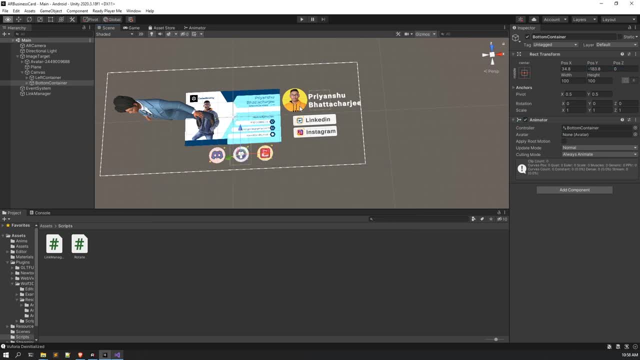 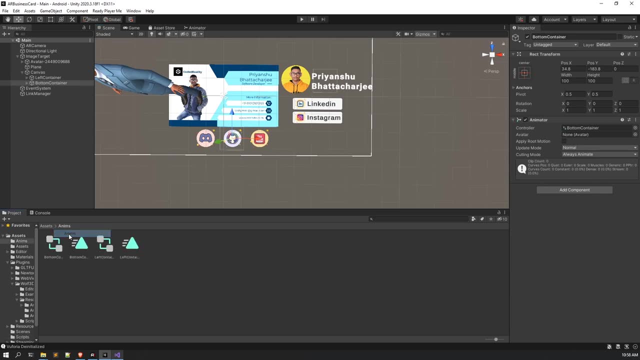 it's working all right. now here's a bit of a problem. all right, this animation. already this animation would be looping all right when, when the animation works right. so to fix that, click on, go to the anim folder. all right, and you can see these triangle icons. 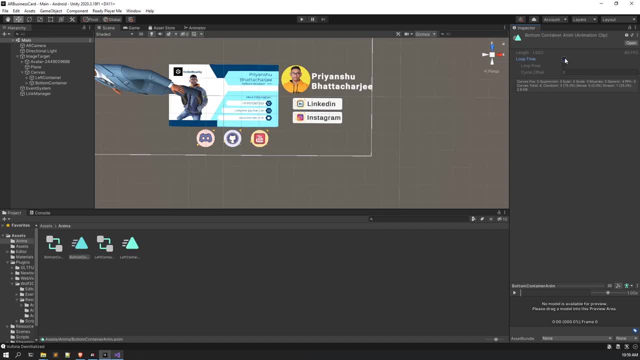 right. so click on them and uncheck the loop time option. all right. and again in the left container, also uncheck the loop time option. all right, now let's see if the animation is working or not. right, let's. let's check that. all right, let's. 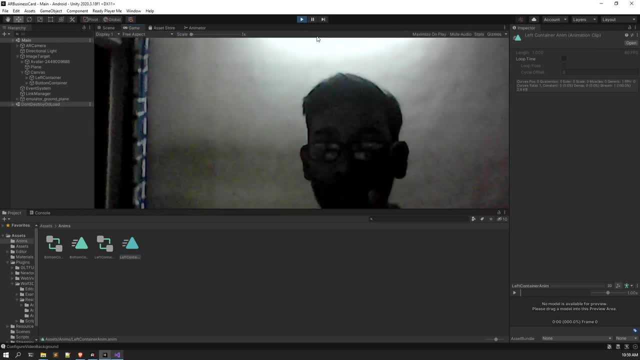 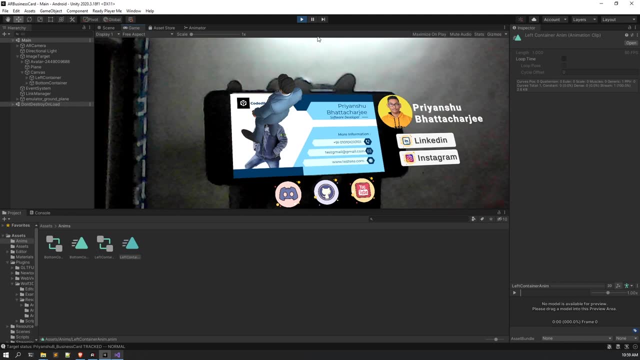 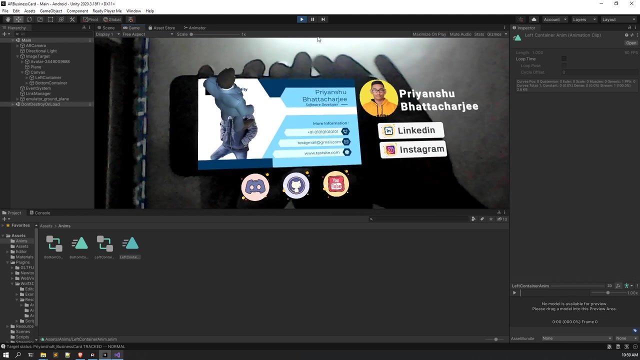 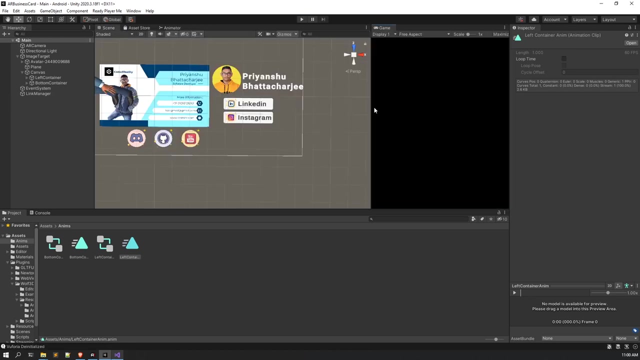 check that. so let's see. oh, our animation didn't worked, but can you tell why? because see, when the scene started now it already played the animation. all right means, let me show you again. all right, let me show you again. let me you know, bring it up in here. all right, and let me show you what is happening in the. 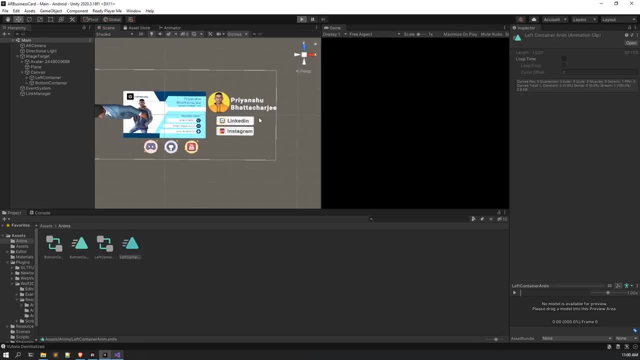 background. okay, so just give me a second. and here you would see that when the scene start, it would already play the animation. now we all we do have a fix for that, and I will show you what is the fix. it's a very simple fix only. all right, I will also make you understand. 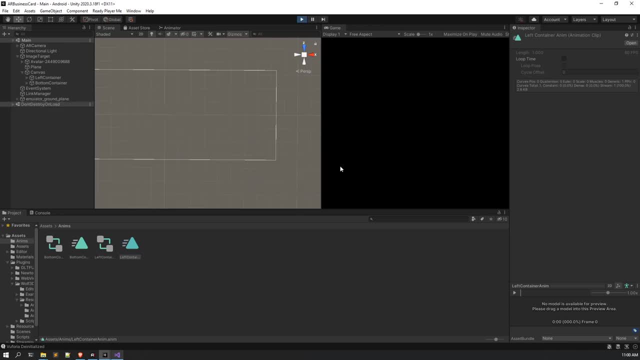 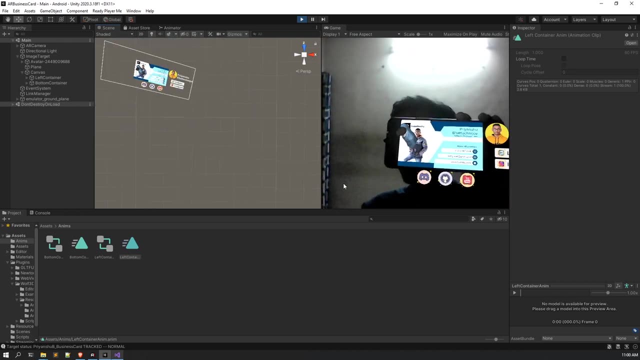 the concept of that. all right, so just give me a second and we'll be good to go right. so here you can see: the animation is actually not playing because it has already been played right. so this is the problem. so how to fix this. so here you can see: the animation is actually not playing because it has already been played right. so this is the problem. so how to fix this. 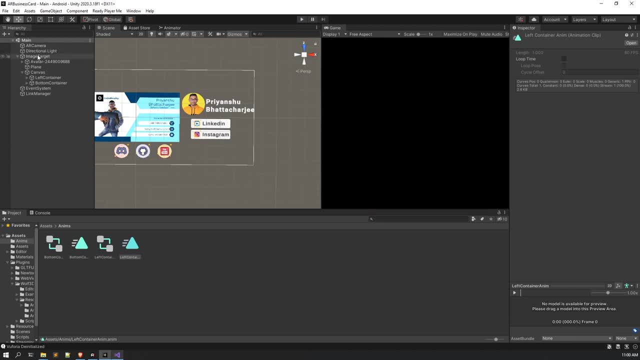 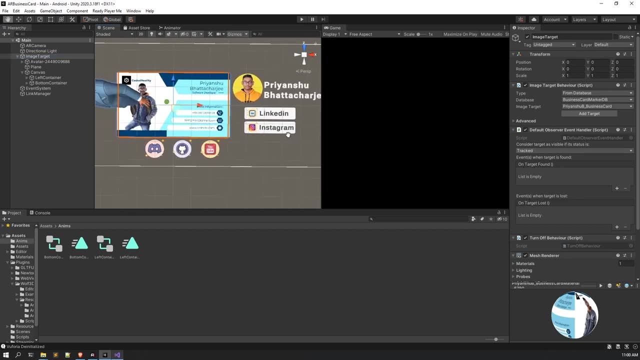 let's, let's see how to fix this, all right. so the very simple way is to go to the image target, all right, and here you can see there's on target found and on target lost, right, and frankly, our work is with this: on target found, right. so 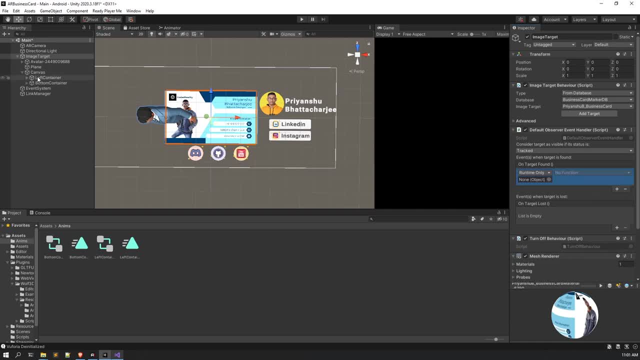 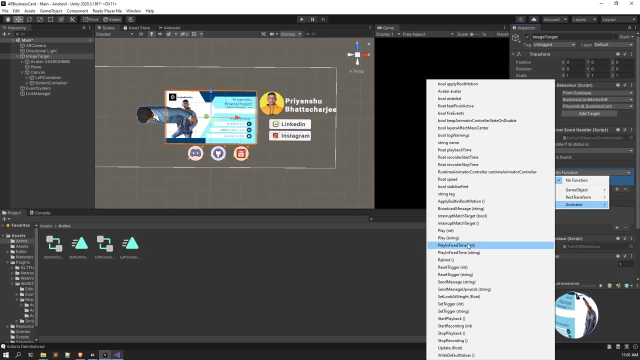 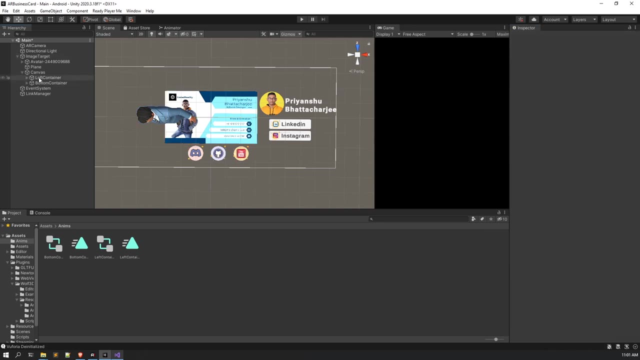 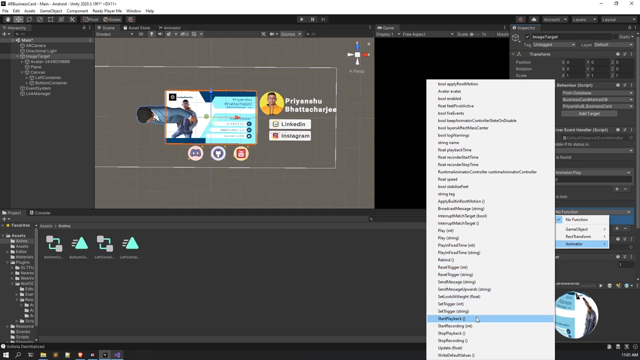 what we will do is click, click on this. get the left container in here, go in here, go in animator, all right, and click on. you know, play right and if on target is lost, all right away. okay, if on target is lost, what you have to do is go to the left container, all right, and just wait. click on stop. 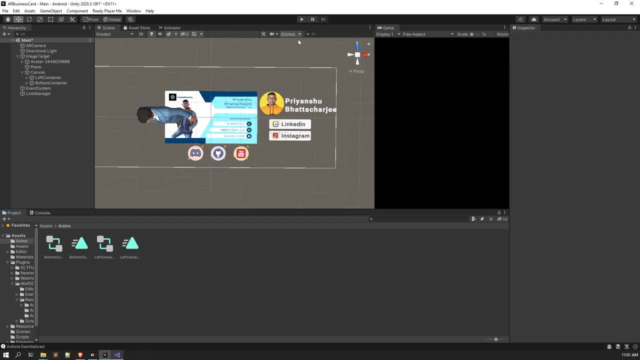 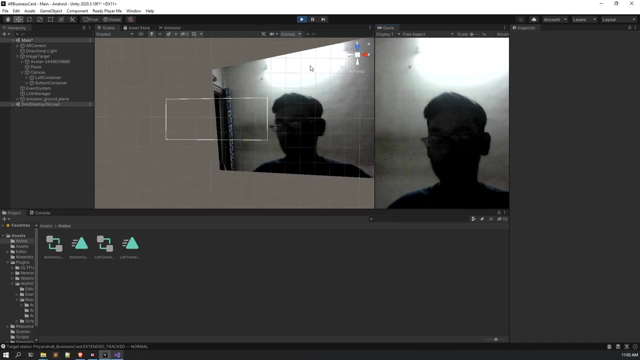 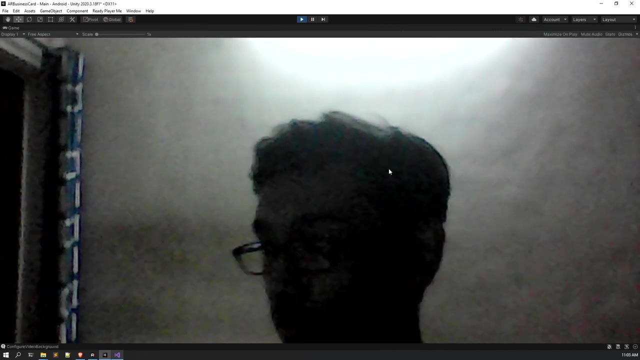 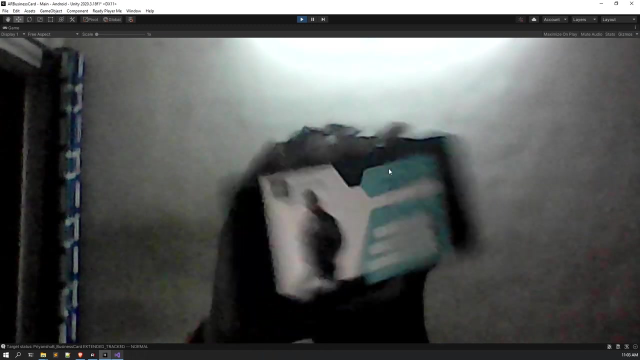 playback: all right now, let's see if if it's working or not. playback: all right now, let's see if it's working or not. alright, so our camera is active. alright, let me maximize the scene. alright, let me maximize this game view: alright, and let's see see. our animation is perfectly. 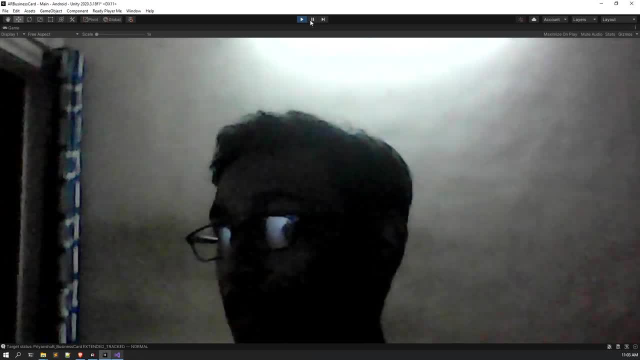 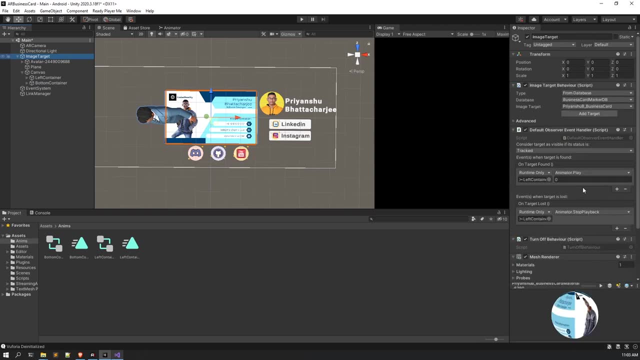 working alright, and let's remove it and then again bring it. see, our animation is the bottom container too. and you know what will happen? our first business card will be created, all right, okay. so drag and drop the bottom container, then again click on play. all right, and then in the on target lost again drag and drop this bottom container and then 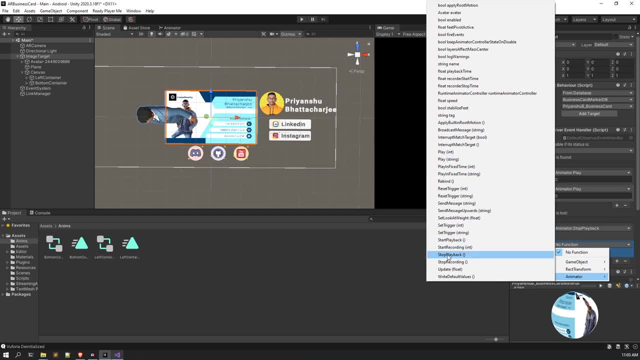 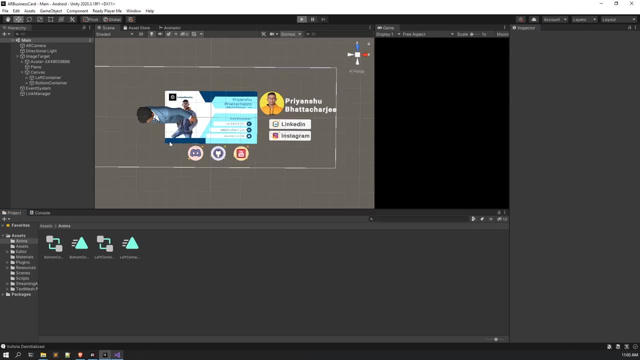 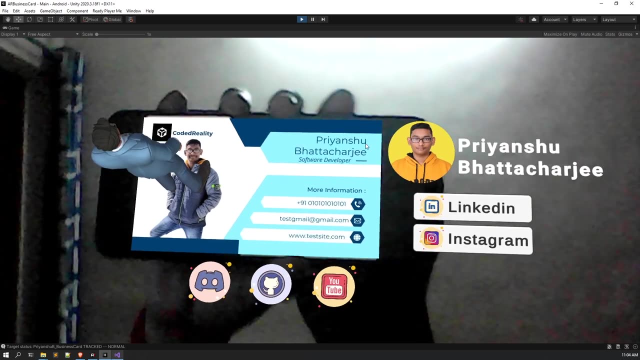 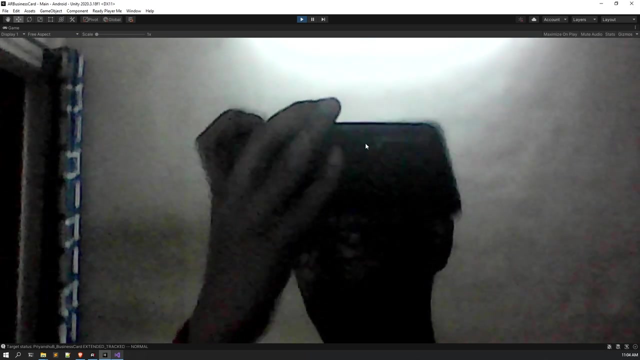 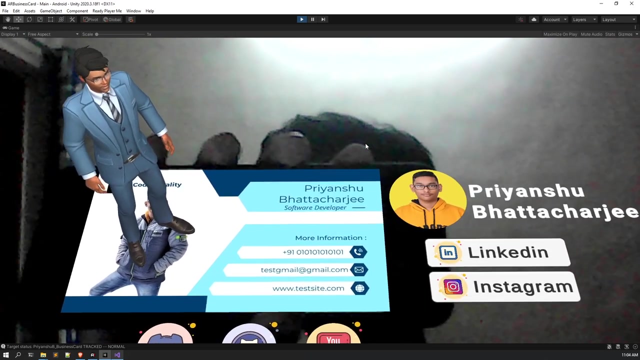 uh, click, stop playback, all right, and uh, let's see. so now let let me show you. all right, see, the animations are perfectly working right, isn't this? uh, great. so, like this, you can create your own avatar. like: see, uh, this, uh means your own business card. see, here, you can see this. there is avatar and it is also. 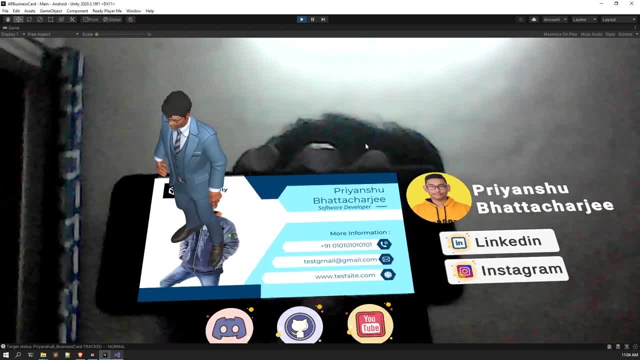 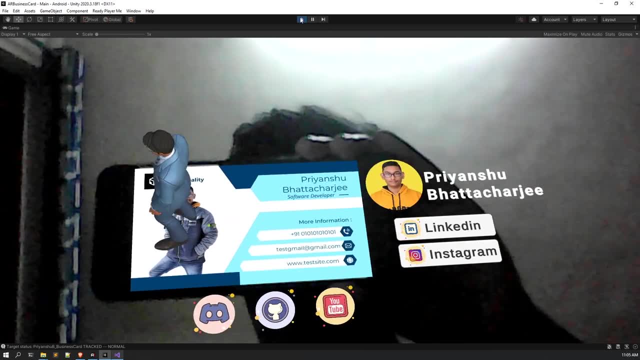 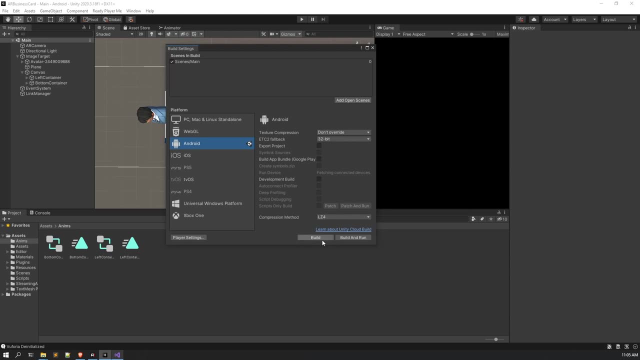 blinking. can you see that? see, it is also blinking. so our, our business card is perfectly created, all right. so now what you have to do is, uh, you have to build this application, and to do that, you simply have to go to file build settings and click on build the application and give. 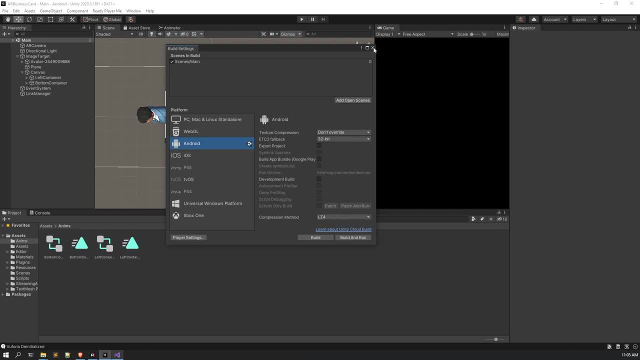 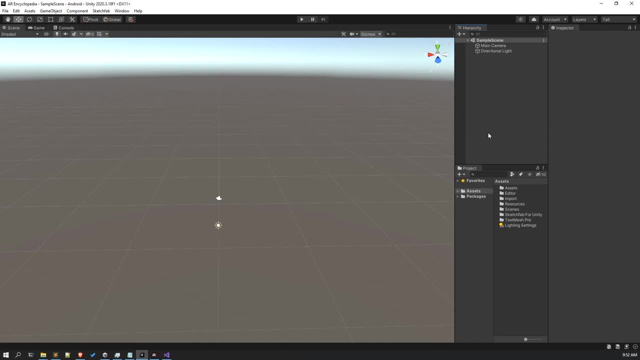 it a name and save it. all right, so that's it. so this is how we create a business card, all right. so, hey guys, in this lecture we are going to create our last project, that is, of view fourier, that is, we are going to create our last augmented reality application in these series. 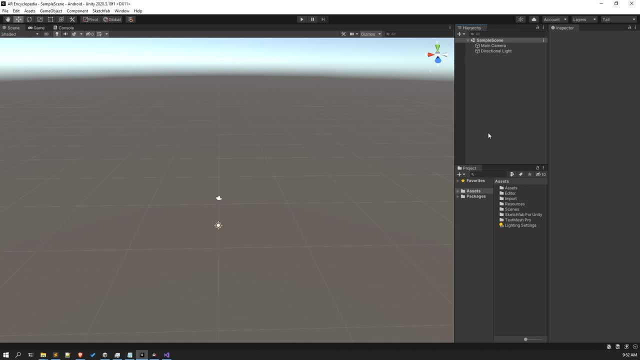 all right, after these, after this uh module, we are going to start with spark ar. so it's also going to be really exciting to work with spark here. so, yeah, without any further ado, let's get started. so the very first thing- all right, i want you to uh- is set up your unity engine. all right is to set. 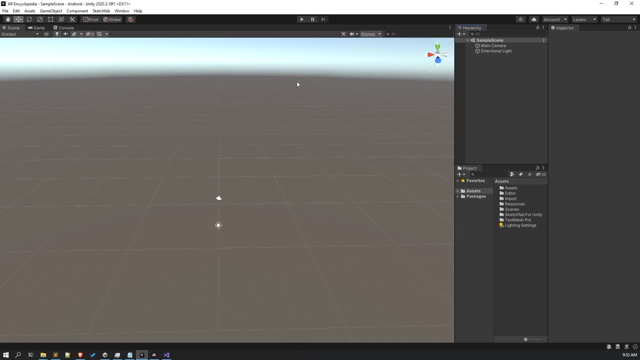 up your view for your engine. you already know how to do that. it's fairly simple. first, the very first step is: go create your unity like unity project, all right. after that, uh, go to your build settings. in the build settings, all right, you would be finding android option. all right, if you don't. 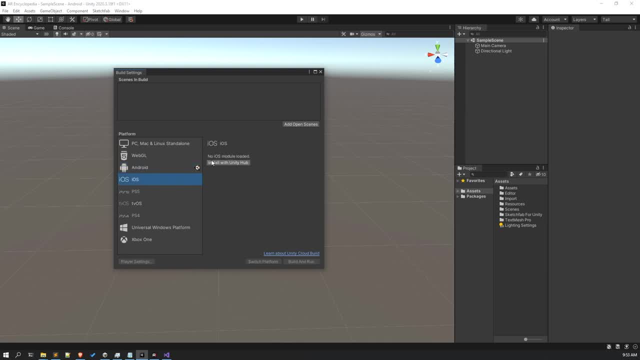 have android option means if. if it is showing something like this: uh, no android module loaded, install it. install with unity. that means you haven't installed your android module, so do that. after that, what you have to do is click on build, so not build. i'm really sorry, you have to uh an. 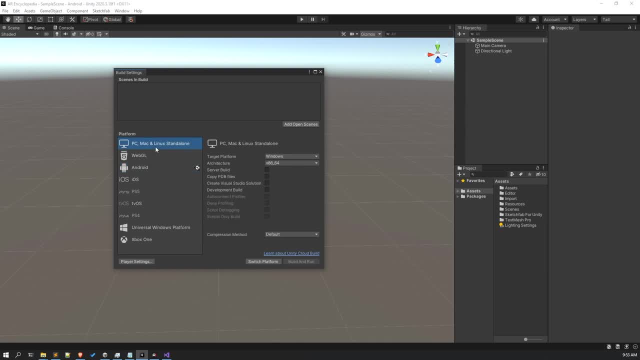 an. an option would be coming, called switch platform. all right, like, uh, like this switch platform. so, as i am already switched to android, it's showing me build, but uh, in your case it will be showing switch platform. so click on switch platform and after you are done, 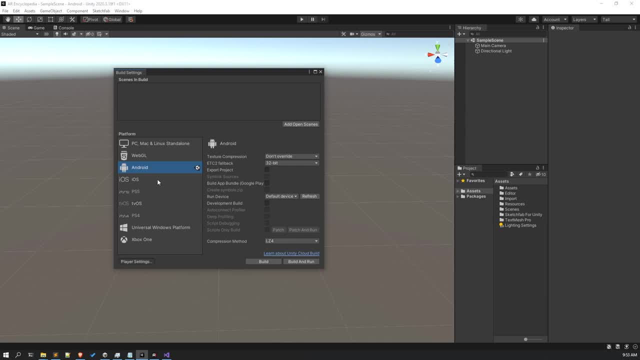 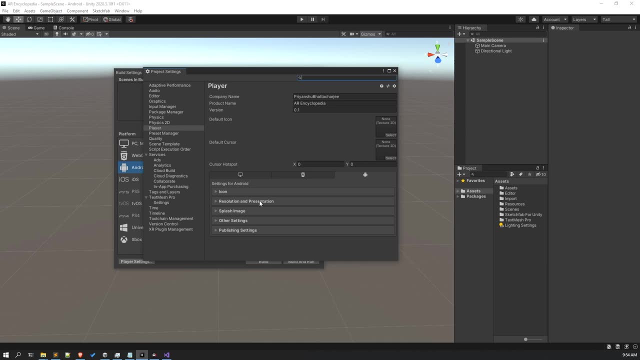 done switching your platform. go to the player settings, all right. go to the player settings in here. add the company name, add the product name, all right. then go to resolution and presentation. in here you would be getting an option of default orientation. i for in my case. all right, in my case. 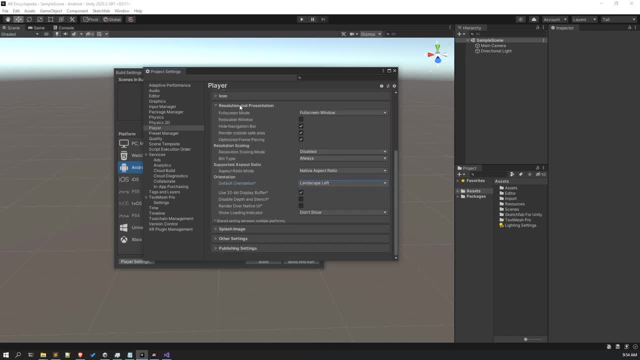 i want it to be landscape lift. uh, i'm adjusting this just because for the camera position of my device, all right, and in the other settings we have to set up our android build version. so currently it is getting all the api level all right. uh, the one i all i means i always go for is android 6.0. 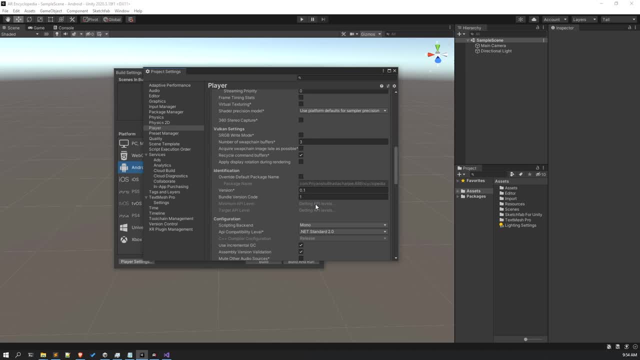 all right, you can even go for android 4.4, all right, it's totally up on you. uh, so i'm again going to go with android 6.0, all right. so here here i have selected android 6.0. there are multiple api levels i have. i have up to 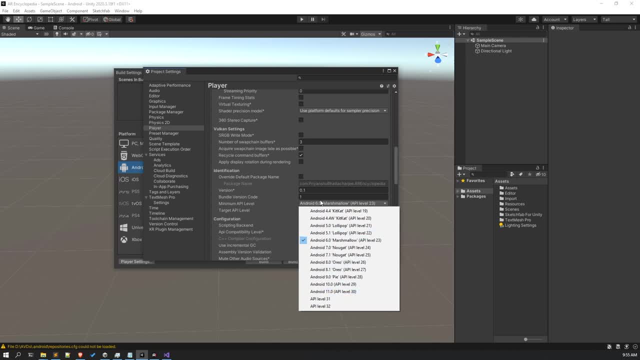 api level 30, that is, android 11. you can choose any one from these and i suggest you not to go above android 6.0. all right, because nowadays most- like most- of our device starts from 6.0. like 4 to 5 year old mobile phones have android 6.0 in them. so uh means, take the api level. 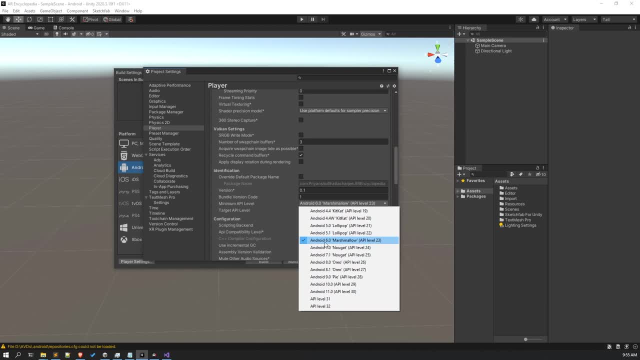 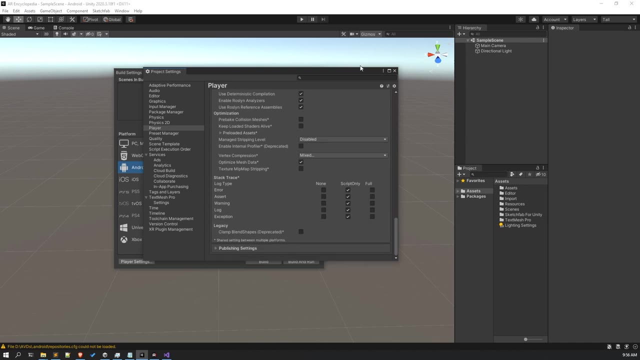 as high as 6.0. all right, don't go above it as of now. now you can even select android 4.4 kitkat- all right, it's totally up on you- and leave the target api level to automatic highest install. all right, just like it is. and uh, yeah, we, uh, our setup is. 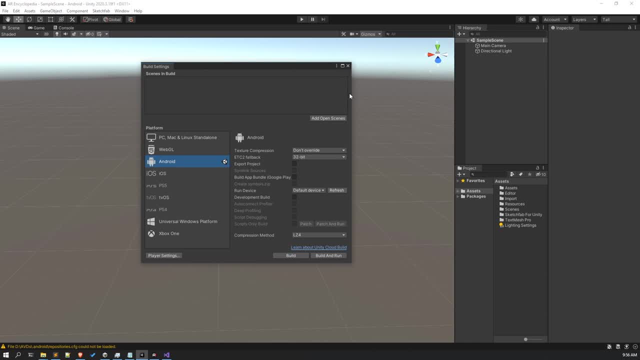 done. all right. now what i want you is to uh import the viewphoria engine. you already know how to do that and i have already imported viewphoria engine, just because, uh, because it's going to take a lot of time to import in my system, all right, if your system is fast, it's. 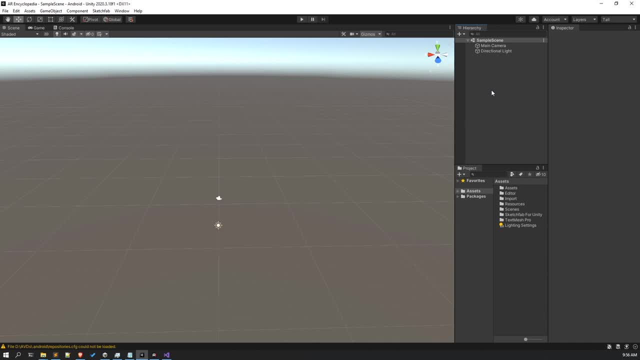 it's not going to take so much time, but uh, in my case it took a lot of time. so i have already imported, and you already know how to import it. all right, so now let's, uh, first create our user interface. all right, that is the main menu. after that we are going to. 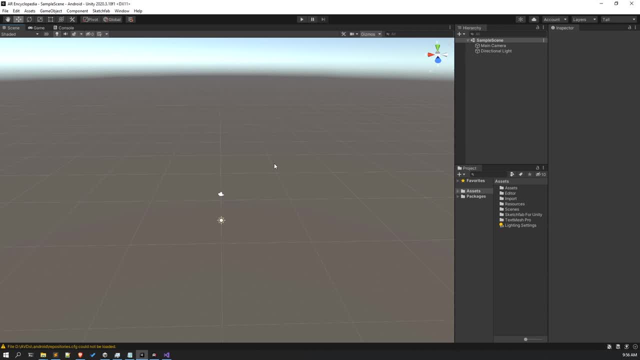 set up our view for the engine, all right. and uh, you see, i'm pretty sure that, uh, you already know how to use the ar camera, how to use the image target, right. how to use, uh means how to use the dashboard, means the website for getting the license for adding the image targets. all right, i'm pretty. 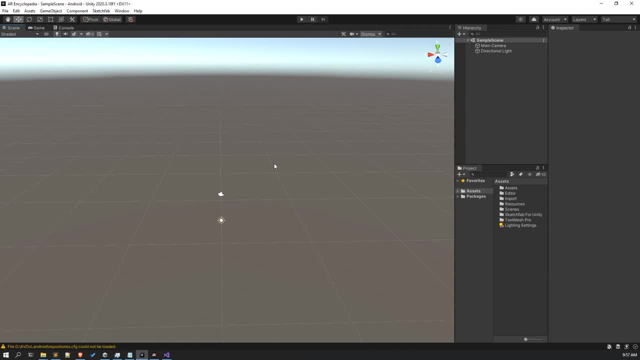 sure you know that. and, uh, i, i want you to try this ar encyclopedia by yourself first, all right. try this one first, by yourself, all right. and then watch the video, all right, because that would be a really good practice for you. so you can do that, or even, uh, watch the video and develop along with it. 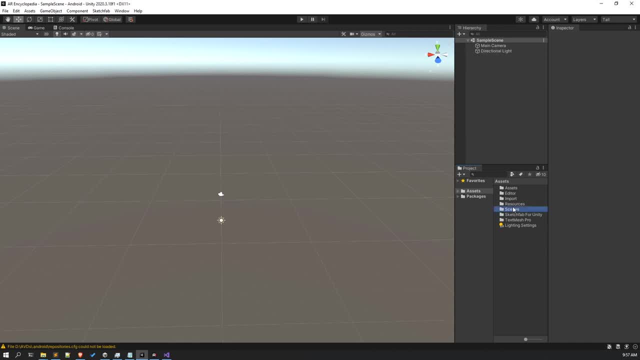 all right now. uh, i, i already have a scene. this is the sample scene. all right, i just want to rename it because this, uh, in here i am going to create the ui, so hit a rename and let's name it main menu. all right, it's asking to reload. okay, cool, so we have basically renamed our main menu. all right now. 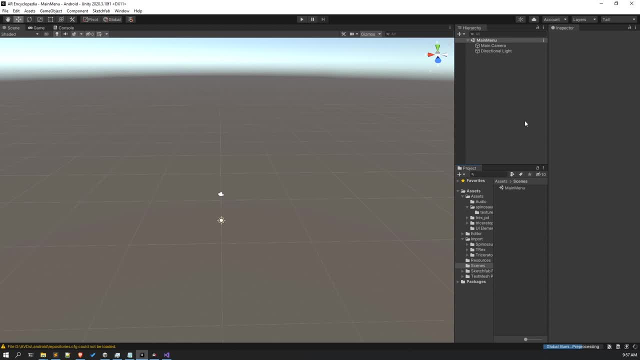 what we have to do is we have to uh provide a canvas to it, right, uh? because, uh, the main menu is here on the screen right now. so if we click the main menu, we will see that it's all right. so i have created an ar project right now. so in the main menu, i have added a ui as well. 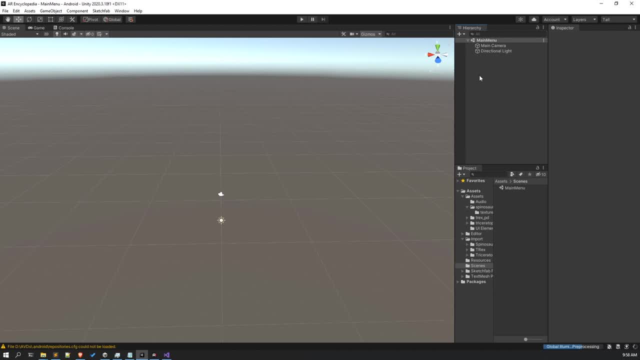 and let's say it's the common ui asset and i also created a ui asset for it. all right, and one more thing: i would like to tell you that this, this ar encyclopedia project, is based on dinosaurs. all right, currently, i have included three dinosaurs. all right, you can add as many as 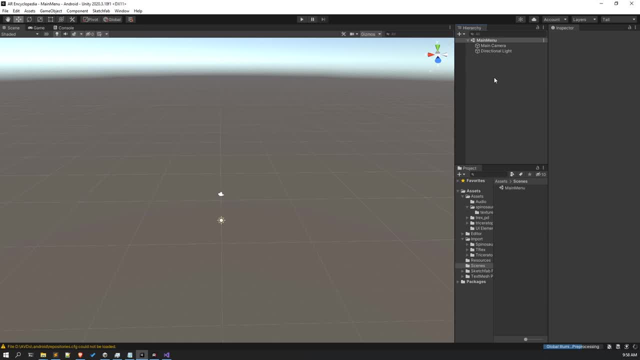 you want. the three are triceratops, uh, t-rex and the spinosaurus. all right, so you can add as many as you want and even launch this product after developing it. all right, and i have also created the uss already. all right, i am also going to show you. here are some of the things that i can do. uh, now i will show you. 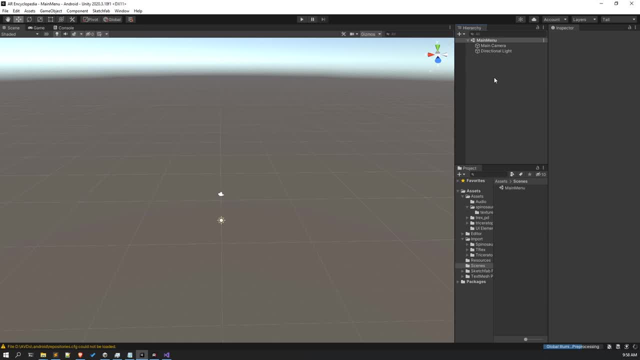 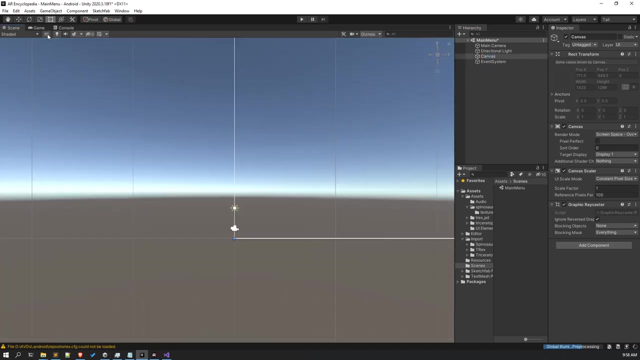 you how to play, pause and stop an audio in this tutorial. so hand tight there and follow the tutorial. so first of all, right, click in here and go to ui and click on canvas. all right, and in here in the top, you would be finding a 2d option. click on the 2d option and then double click on the. 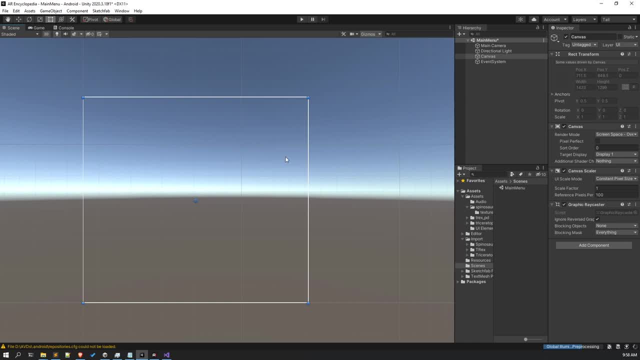 canvas option and it would be focused. all right, so, and the thing go to the game window, all right, and uh choose a resolution. uh see for uh developing a responsive ui. what i generally do is i have three resolution, all right. one one is of iphone 6, that is the medium resolution. one is of uh. 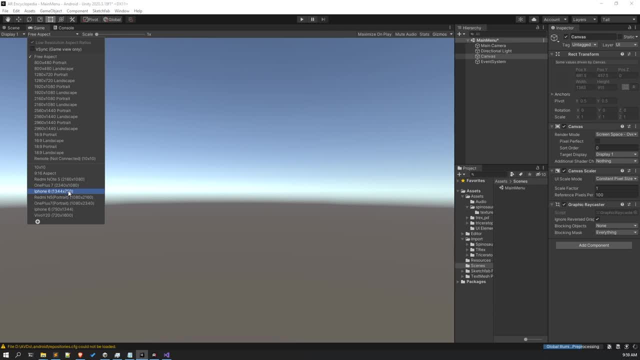 not exactly the medium, all right, but i have iphone 6 that is the lowest resolution. i have one plus seven that has the highest resolution and redmi note 5 that has the medium resolution, all right. so what i want you to do is: uh, you also follow these. uh. three means these three presets. you can create your own by like. uh. 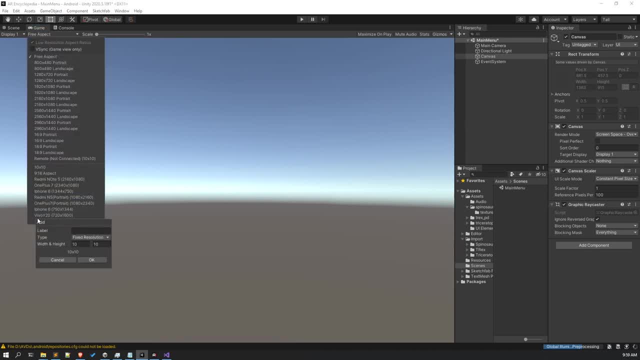 in the game window. here you'll be finding a drop down. go in here and click on this add button. give it a name, uh, give it and width and height, all right so, and click on ok, it would help you create a means, basically a resolution of any phone, all right. so currently i want to go with iphone 6. 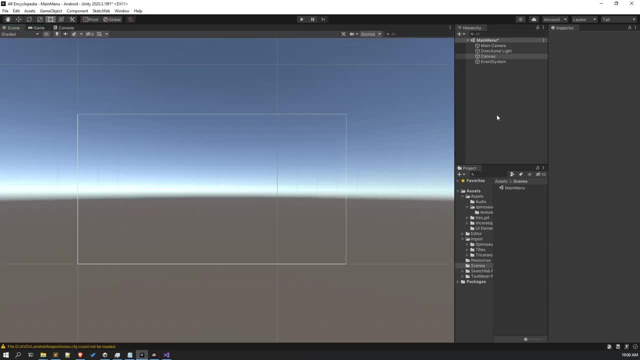 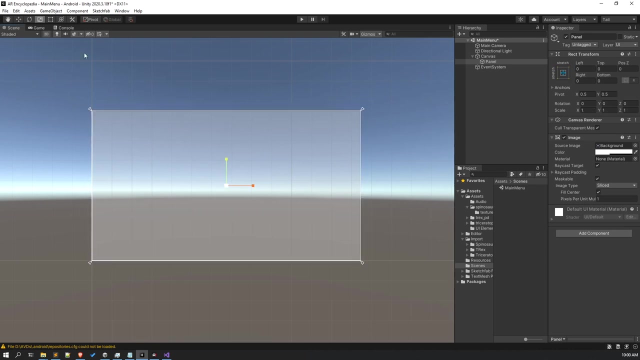 all right, let me just add one more thing here. so let me just add this one and make sure that this looks good. now what i want is: uh, in this canvas i'm going to create- uh, you know, panel, all right for attaching my background image in here. so i i just want to stretch this, uh, you know, stretch this panel out. 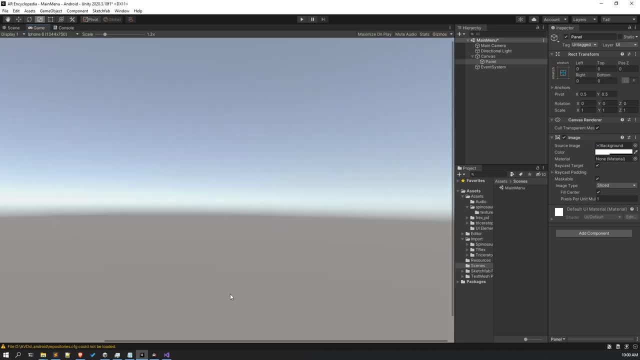 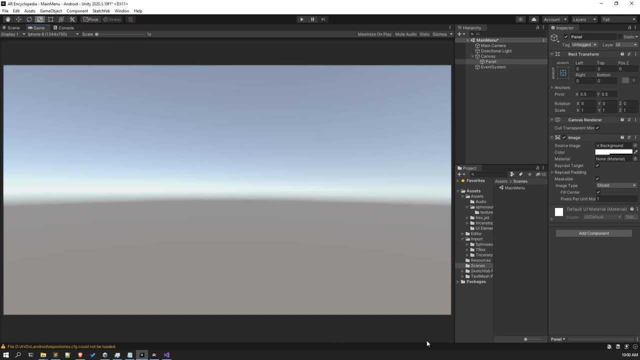 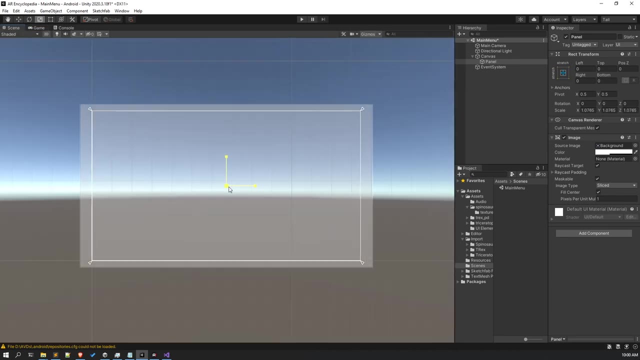 a bit, because let me show you why. uh go to a game window if i'm not sure if it's visible to you or not, but uh, just wait, edge spots, like the panel isn't covering the whole- you know, whole- canvas, so that's creating a problem. so that's why I'm going to, you know, stretch it out a bit. okay, and now what I want. 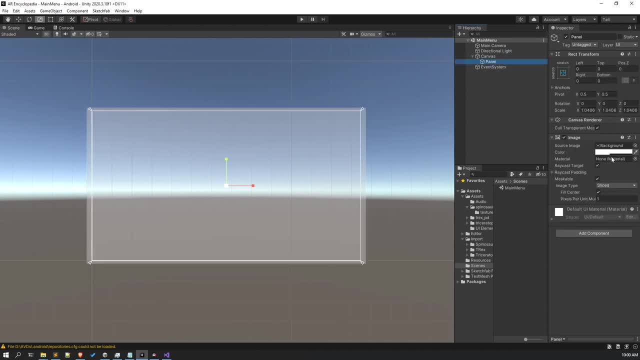 to do is I want to click on the panel, all right. then in the color image here is an option of alpha. I want to increase it, all right, so that it doesn't means it is not transparent, all right, and in the background here you can see source image. I am clicking this button to select the 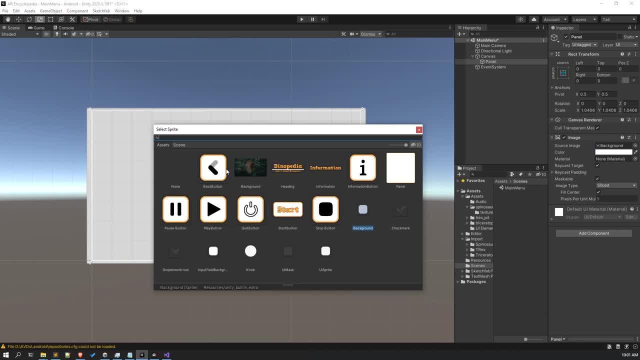 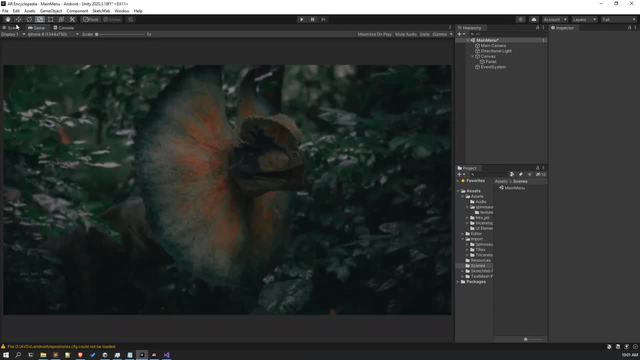 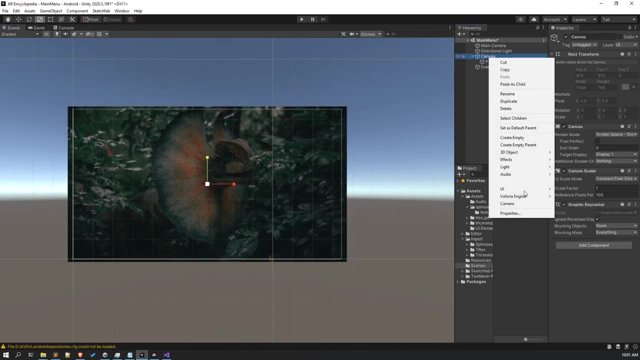 image all right. and in here, let me see: yeah, I got the background image in here, all right. so this is the background image I'm going to use. let's see how it looks. yeah, it looks good, all right. and now what I want to do is I want to give it a heading right, so I have also created an asset for it. so 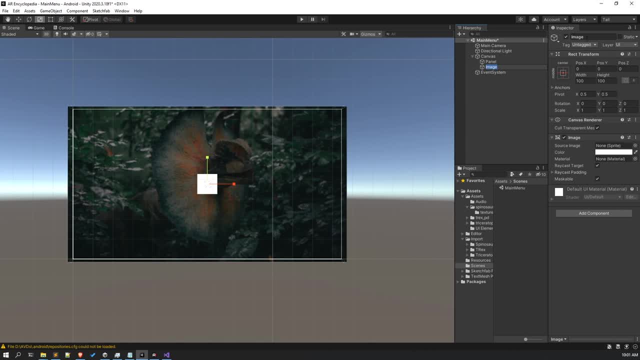 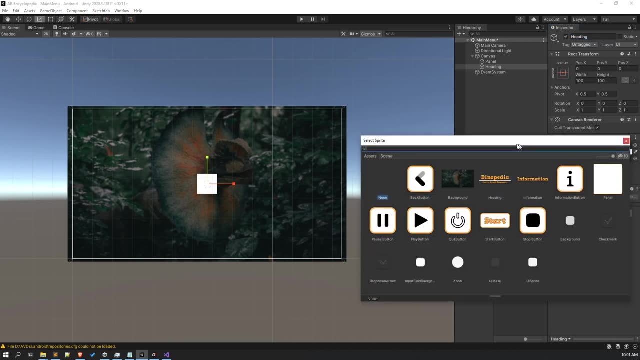 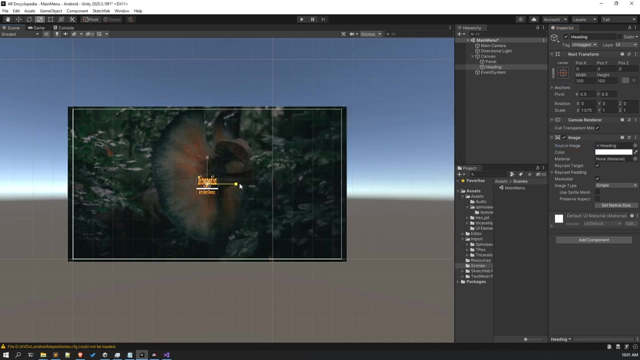 click on this image. all right, click on this image and let's- let's give it a name. that is heading, all right. after you give it a name of heading, what you have to do is you have to choose the title. all right, that this is. I have kept the title as dynopedia, all right, so 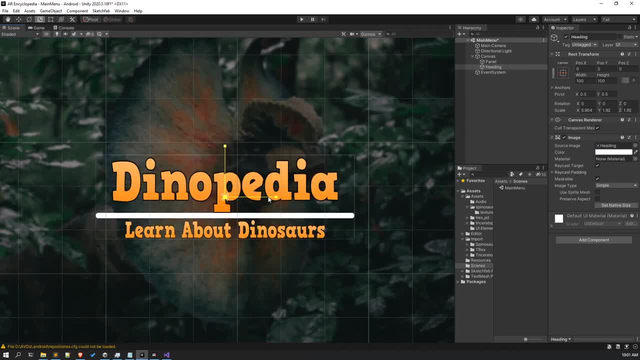 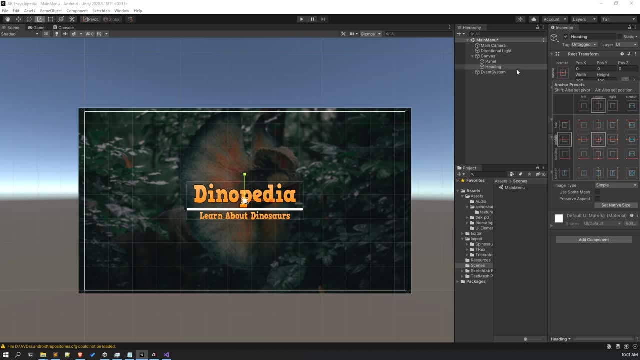 I'm going to adjust this particular asset a bit all right, so that you know it, it fits good to the UI. and well, you have to do one thing, all right, go to this particular red transform alt and you know, then anchor it on the top. all right, now adjust it a bit, all right, and let's see how. 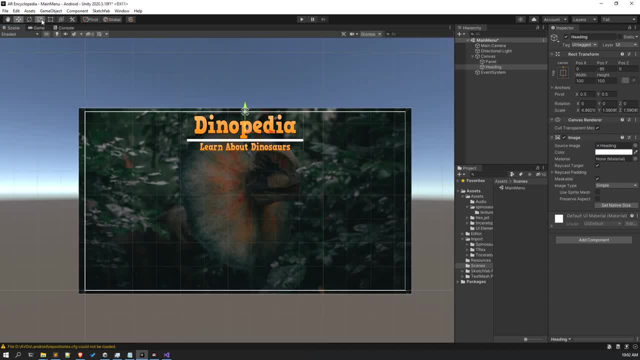 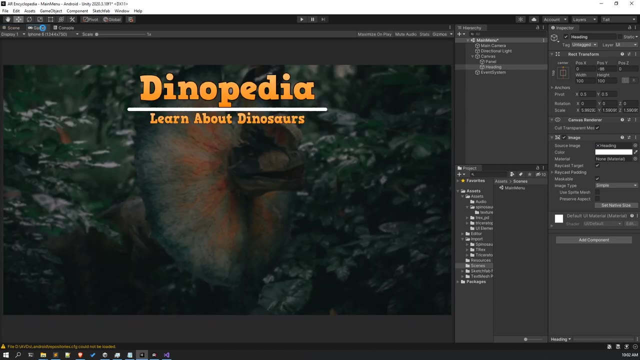 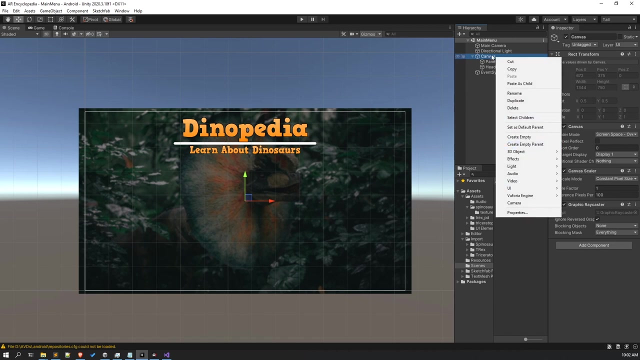 it looks. yeah, it looks good. let's stretch it out a bit. no, let's, let's stretch it out a bit. okay, yeah, all right, now it looks good. now let's drop it down a bit. all right, let's drop it down a bit. okay, cool, now I have to add a button in here that is a start button. all right, so I'm again. there are two. 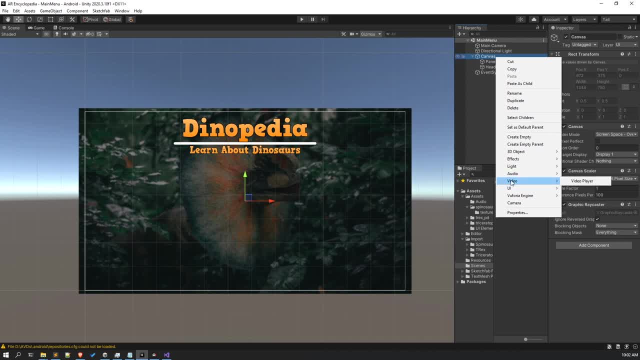 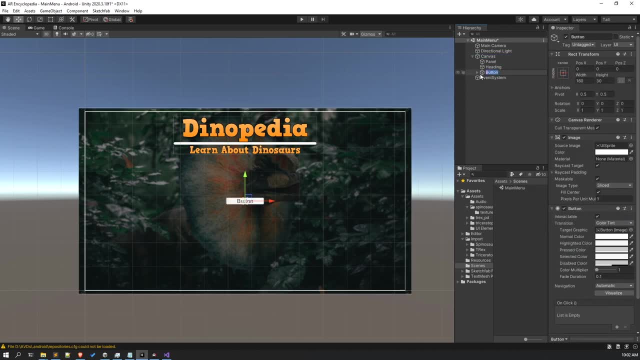 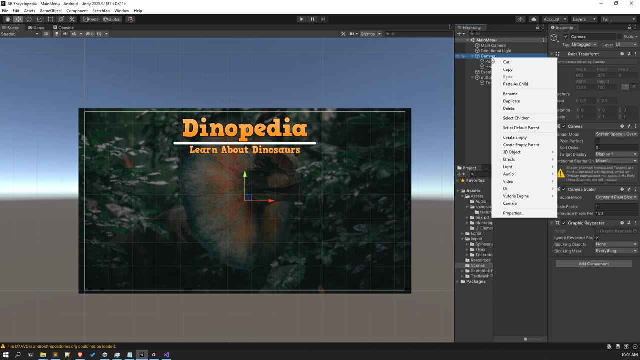 ways you can do that. all right, I'm I'm going for the image one, but let me show you. first of all, go to UI. you can simply select a button. you know, simply select the button and then, from that button, delete the text. all right, but I don't want to do that. I'm going to do a very simple thing, that is. 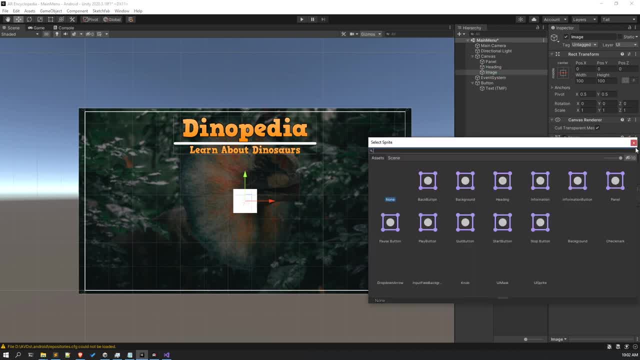 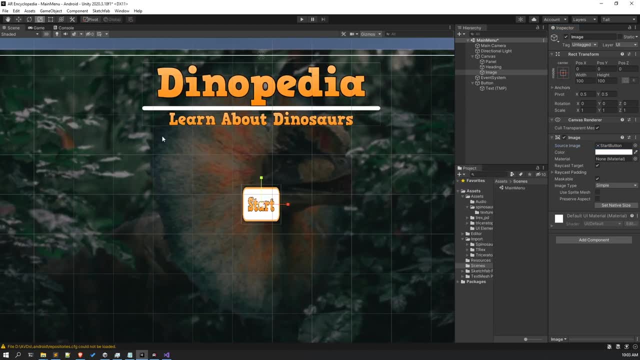 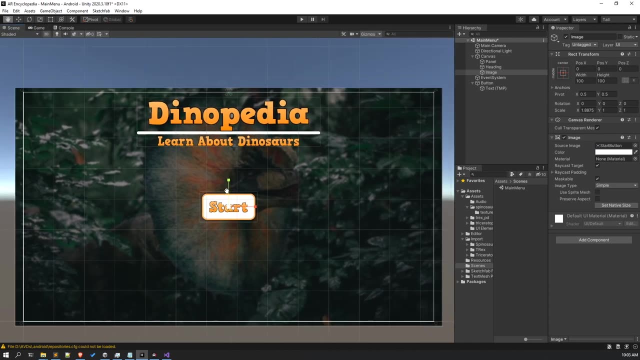 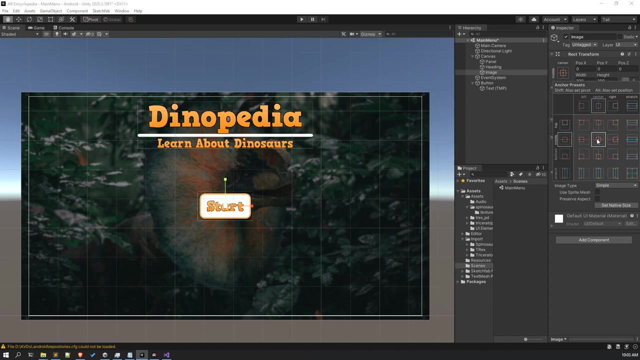 go to UI, select an image- all right. and, you know, select the start button asset- all right. and then again, you know, stretch it out a bit, all right, so that it looks, you know, looks good. all right. now, now that it looks good, what I'm going to do is also anchor it. all right, anchor it. maybe. actually let's anchor it in the center only, let's. 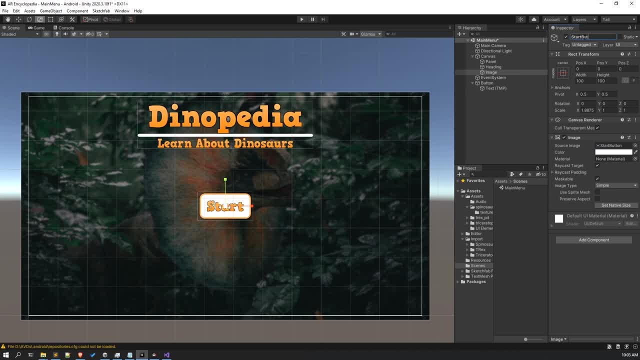 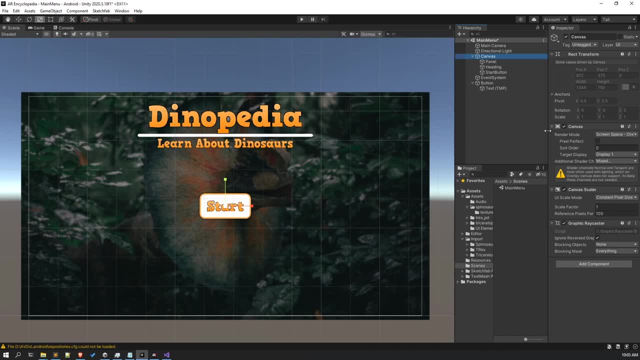 keep it at the center. click on start button. all right, oh, I guess one thing I forgot. yeah, see, I always forget to make this change all right, whenever I'm creator creating a UI and I just it just comes to my mind after many things are done and 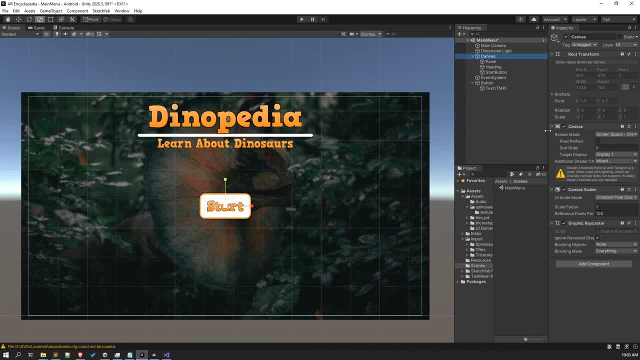 I again forgot to do that. I'm really sorry about that. actually, in the canvas all right click on this canvas here you'll be finding an option of means, a component in the inspector called canvas scalar. in there you would be finding the UI scale mode. what you have to do is you have to change it to scale with screen set and see. 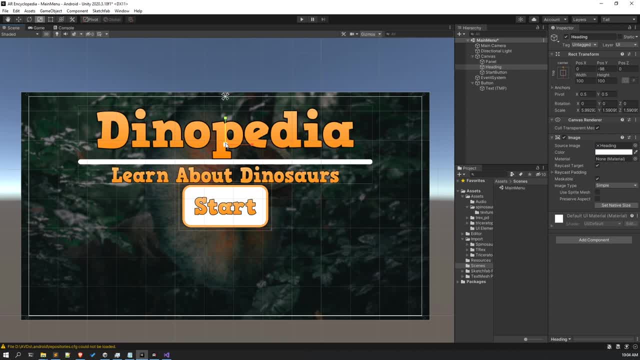 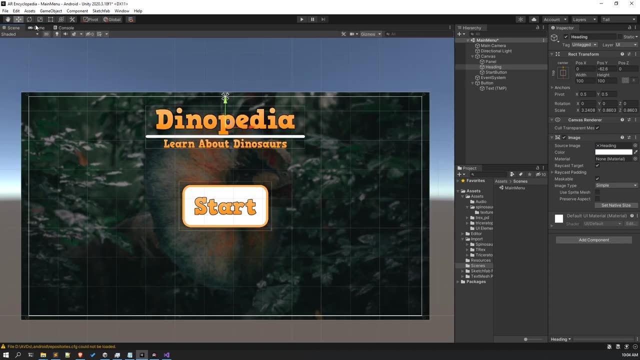 this is why, uh, I like I really hate it when I forget about, you know, uh, setting up all the things in the UI. so it happens with me a lot, all right, so, yeah, forget forgive me about this. but yeah, now, as everything's working, fine, all right. 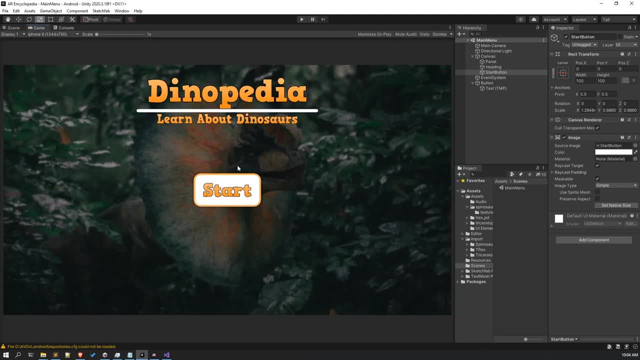 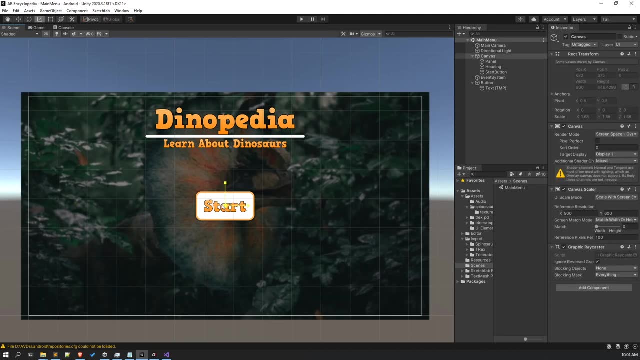 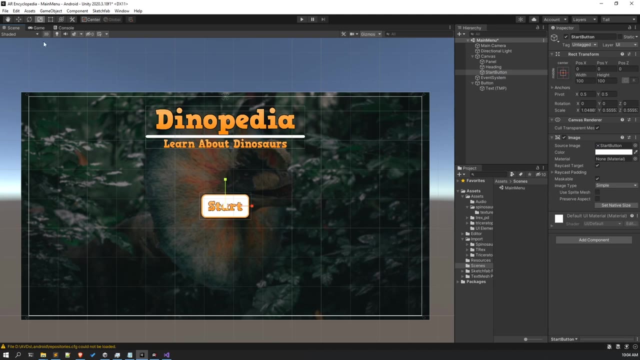 we are good, right, so yeah, let's you know. uh, let's make this button a bit more shorter, just wait. all right, where is the button here? gotcha, all right, yeah, it looks. looks good now in the start button. all right, as it is an image, we won't be able to click this image, or, of course, we. 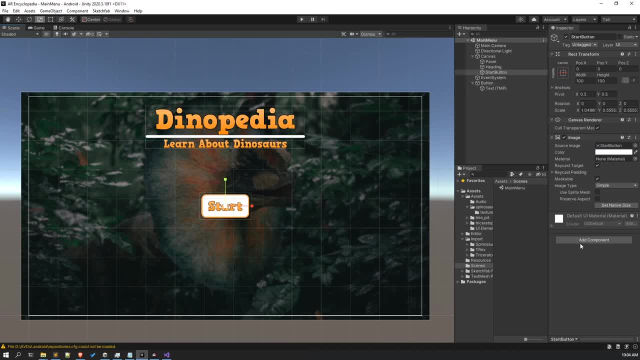 won't do, because it is not a button. right now, to make this image a button, what you have to do is you have to click on add component in here, all right. you have to search for, uh, something called button, all right, and here you would be getting a option for button. all right, and now this image: 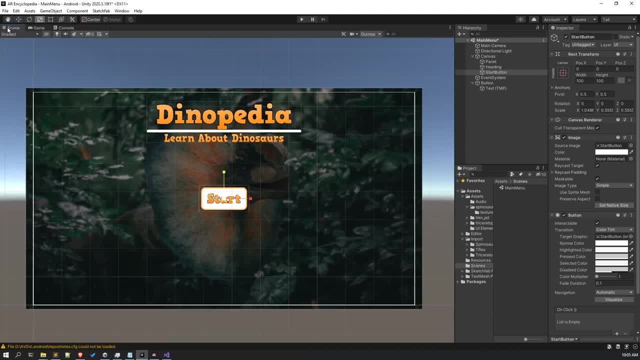 is a button. all right, this image is transformed into a button. right now I want you to create another image, all right, go to the UI. um, then you know, uh, let's, let's give it a size of, let's say, 60, 60.. yeah, I guess that's, that's really cool. then again, select another UI. that is the quit. you to quit. 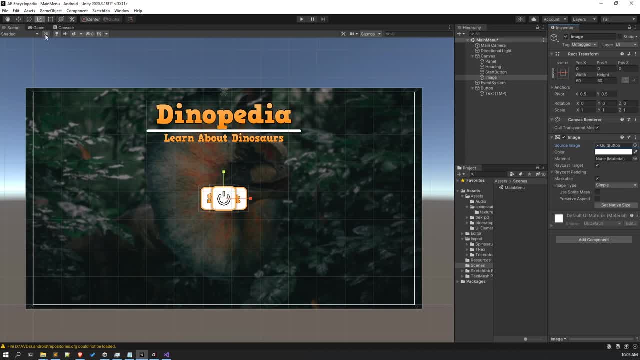 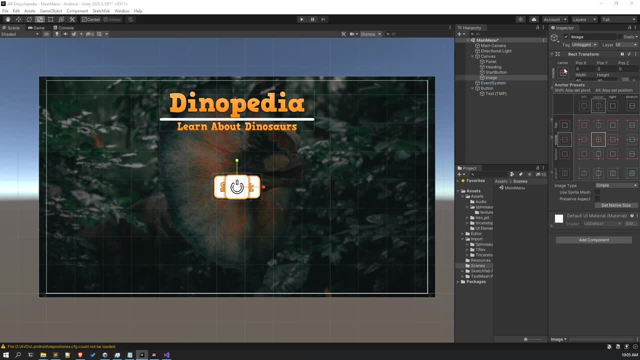 button. all right, of course, you want to give a quit button, right so, so that people can quit from the application right now. what you have to do is again click, uh, click on this rect, transform, click alt and yeah, there you go. we have our button aligned right on the bottom left. all right now. 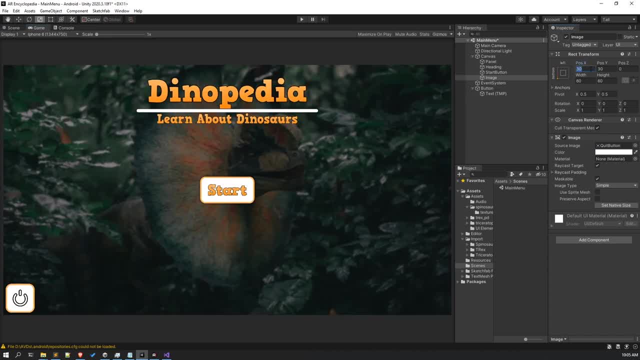 let's see, yeah, it looks good. now, uh, let's just do one thing. let's, you know, uh, shift it on a bit, uh, change the position of it, all right, and let's make the size 50, 50.. yeah, now, now again, let's change it to 40, 40.. yeah, this looks this. 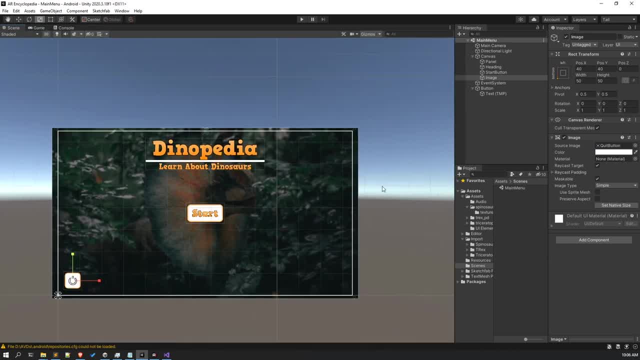 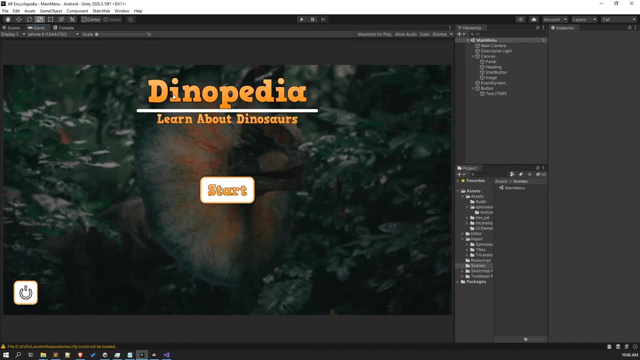 looks really good, right? so we have created our main menu, all right now. as we have created our main menu, now what you have to do is, uh, we have to create our ARC, all right. so let's see how to do that. first of all, as you have created a main menu, 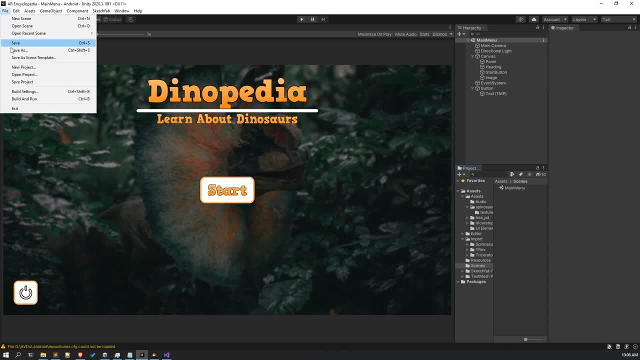 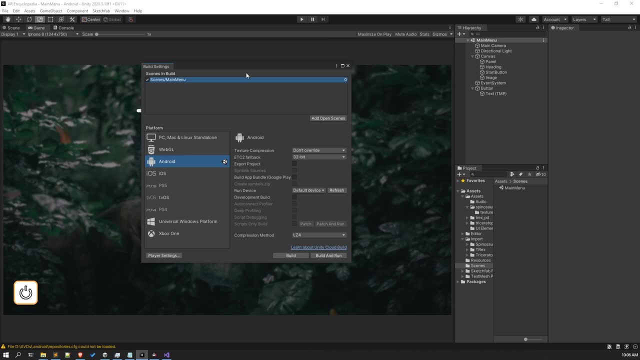 congratulations. and what I want you to do is go to file, click on build settings and add this main menu on the top. all right, and always remember whenever there- uh, let's say there are multiple scenes, all right, three to four scenes- always remember to put the main menu. all right to put. 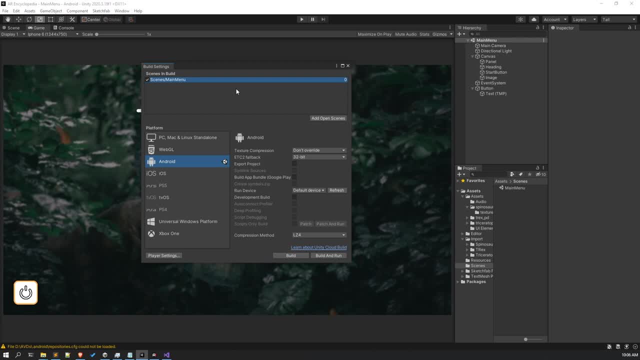 the main menu on top of every scene. all right, because, uh, this would mean the scene in the top. all right, the scene in the top will be the main scene. all right, would be the main scene in the sense that it would, uh means after building the application. 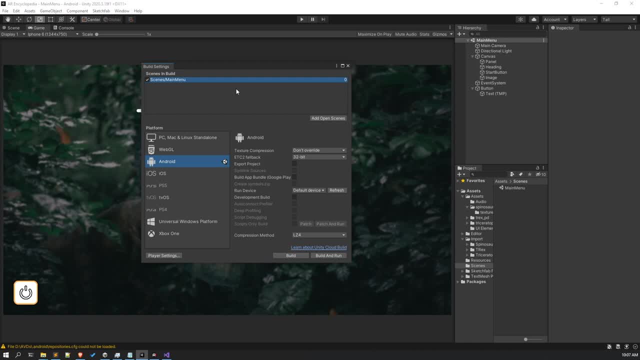 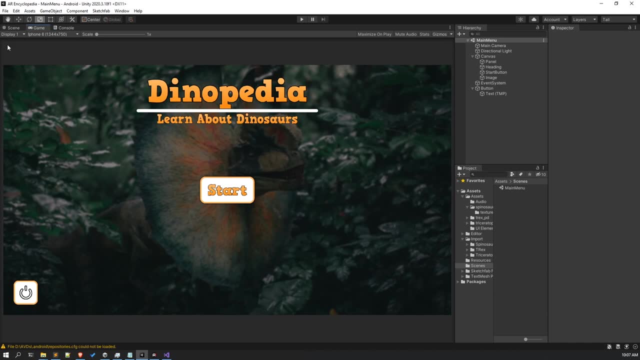 the application would start with the scene that is on the top, all right, so always remember to keep the main menu on the top, all right? so yeah, as our- you know, our- main menu is done. now what we can do is we can create another scene. uh, that would be our ARC. 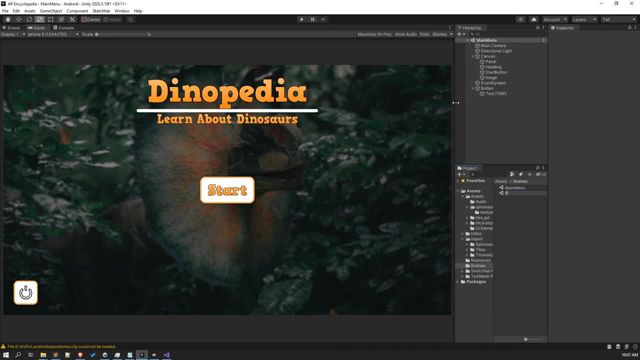 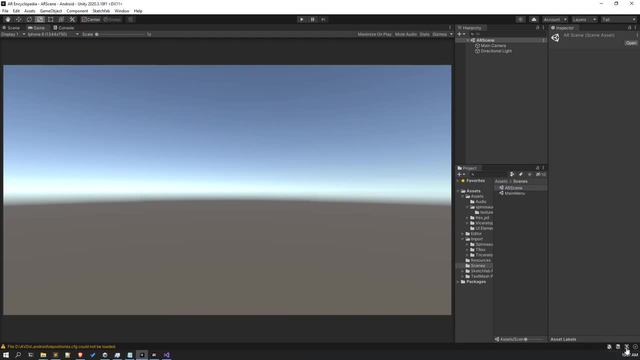 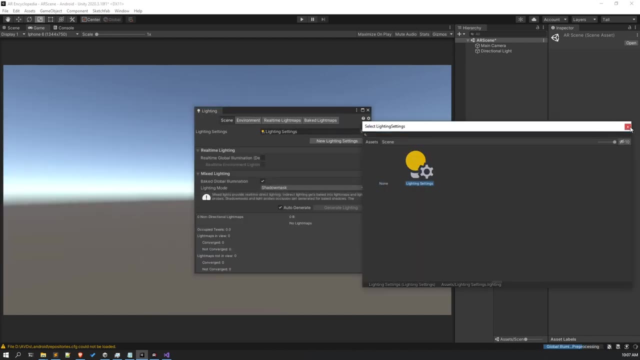 right, so right click, click on scene and let's name it ARC. all right, and let's open it. now. I want to enable the directional light, so let's do it. I'm going to select the common lighting settings. I have all right and yeah, we are good to go. 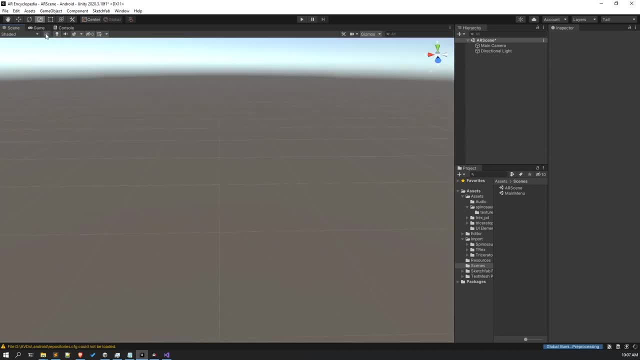 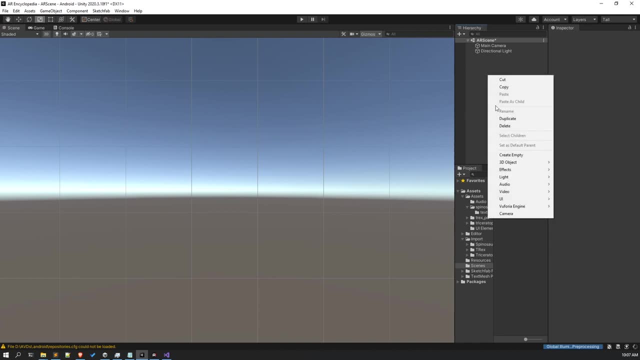 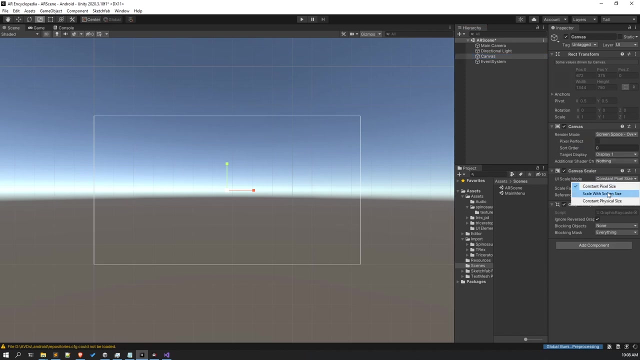 now, what you have to do is: let me show you first of all. uh, first of all, the very first thing is, I think, that the UI would be containing back button, all right, so what you have to do is go to canvas. in the canvas, what you have to do is, uh, change the constant pixel size to scale with screen size. 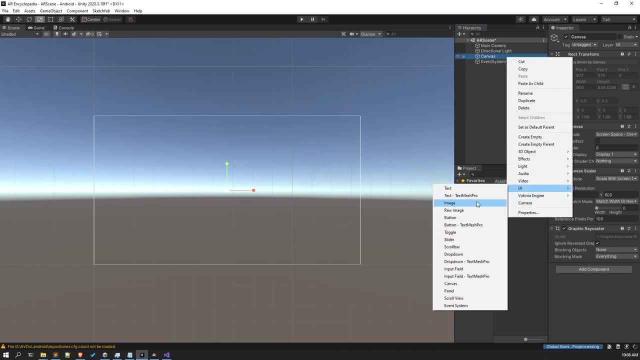 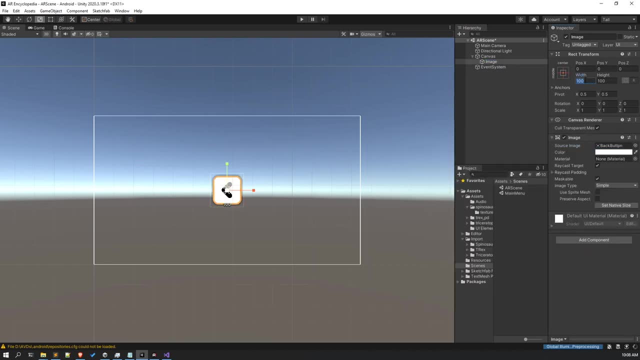 all right, and then in there click on UI, then add an image. all right, then select the back button um, change the width to 50, 50.. all right, and let's you know, anchor it to the top right, so top left. right now let's change the. 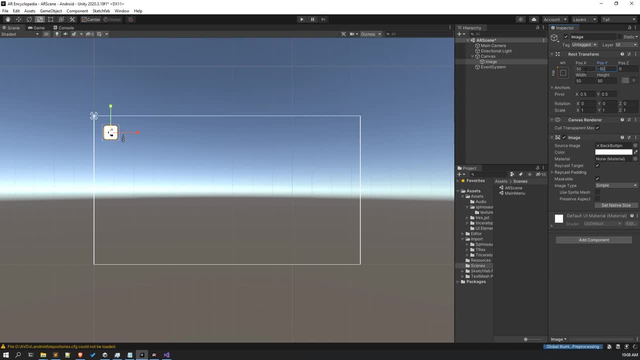 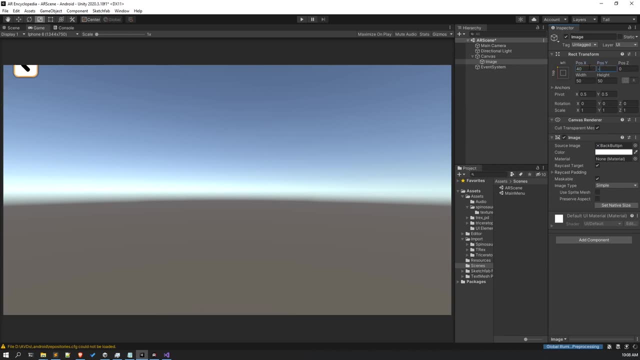 position of it. let's say 50 and minus 50.. all right, so let's see how it looks now. it's uh, it's a bit too much. go for 40 and you know, minus 40.. yeah, this looks good. all right, so this is one of. 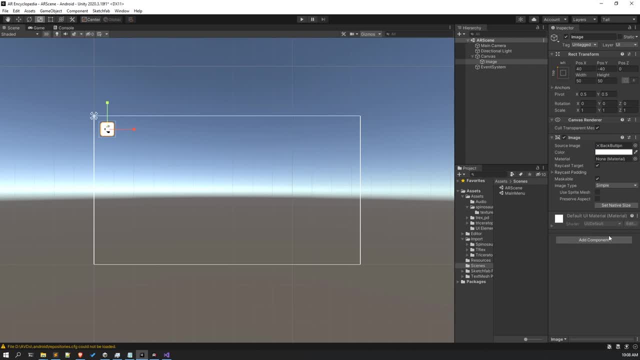 our UI and also add a button component to it. okay, so I I somehow added another component- this is virtual, but button behavior and of course I don't want that just to wait remove. let me remove this whole thing, okay, yeah, just. uh, let me again reconfigure the button. okay, cool, now go go in here and add a button component. 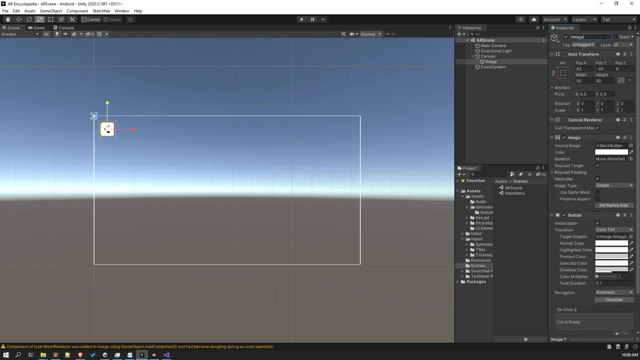 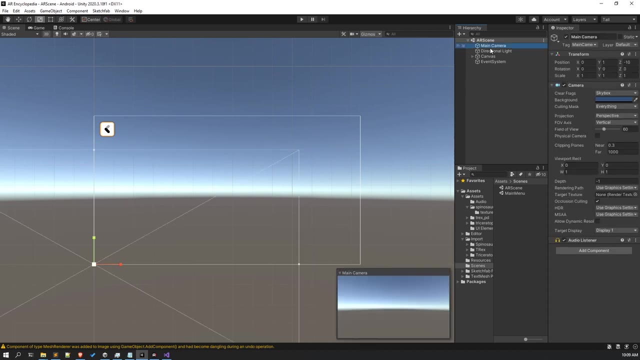 all right, and yeah, our button is created and rename this button to back button. all right, now for uh, further. all right, for further development, we have to set up our view 4d engine. all right, so it's fairly simple. delete the main camera. all right, delete the main. 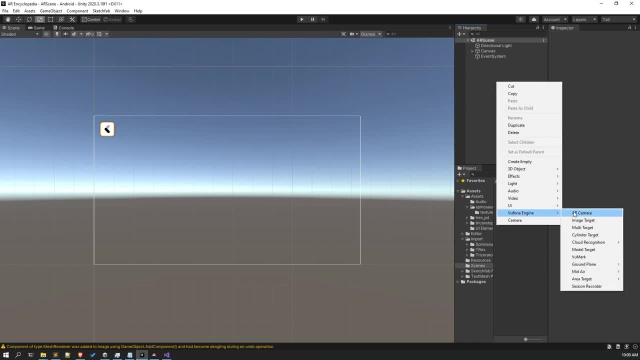 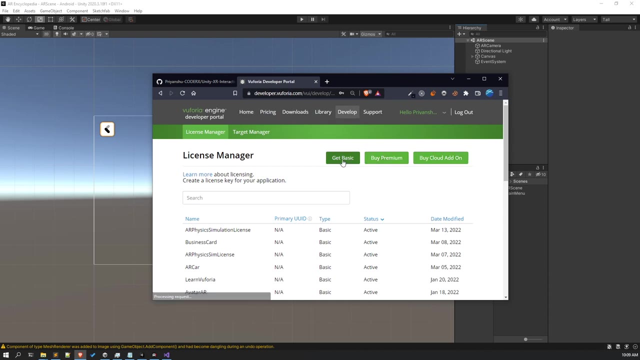 camera. then add a view 4d engine AR camera. all right, and you know, drag it in or drag it to the top. all right, now, as we have the AR camera, we have to, you know, create a license. so what you have to do is click on get basic. 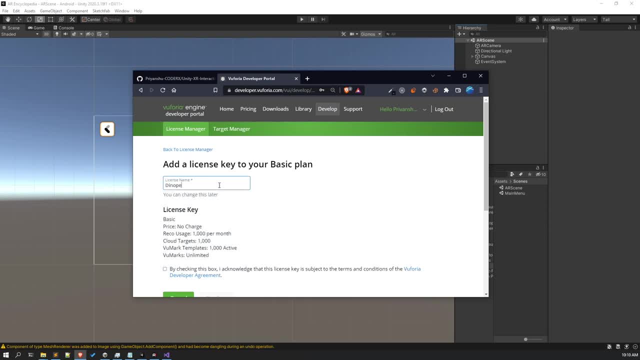 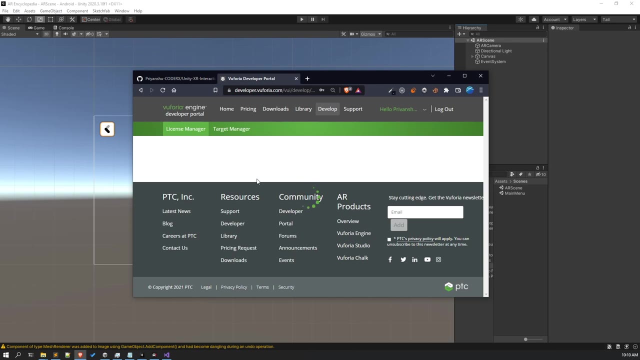 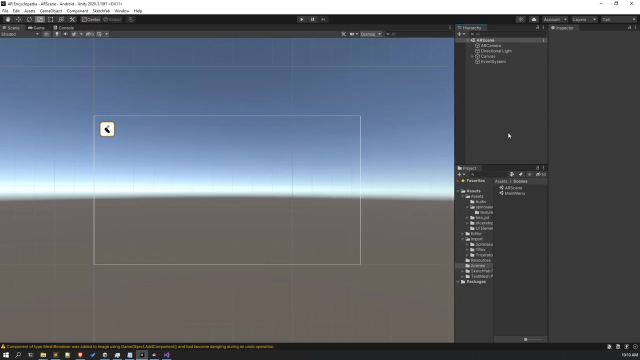 and in here, give a license name. uh, as I want. as my app's name is dynopedia, I'm going to give it a dynopedia license name, all right? and uh, simply, just, uh, you know, copy the license key, create. so, now that we have our license key, go to AR camera. click on open view for your configuration. 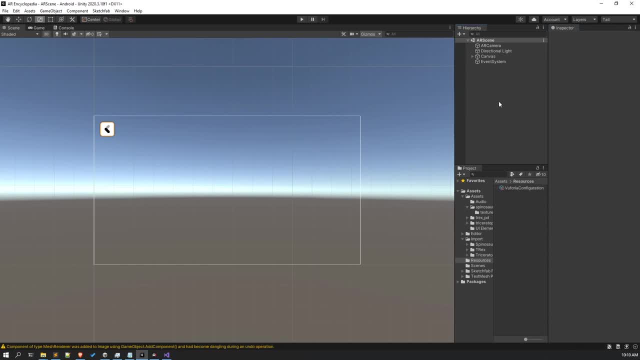 all right, and paste it, okay. so now our license key also set up. now one thing: uh, just give me some time. all right, I'm going to prepare the markers, all right, and then I'm going to come back and show you how to also add the markers, all right, and how to use it in your project. all right. 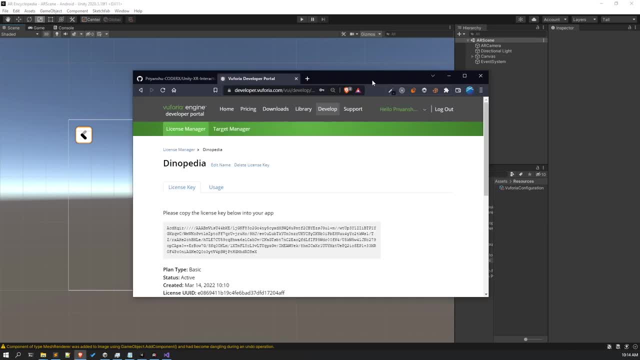 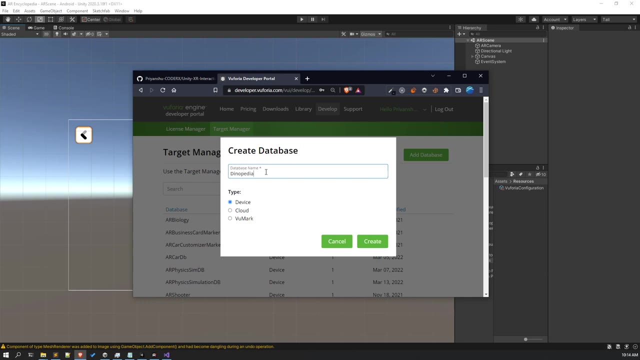 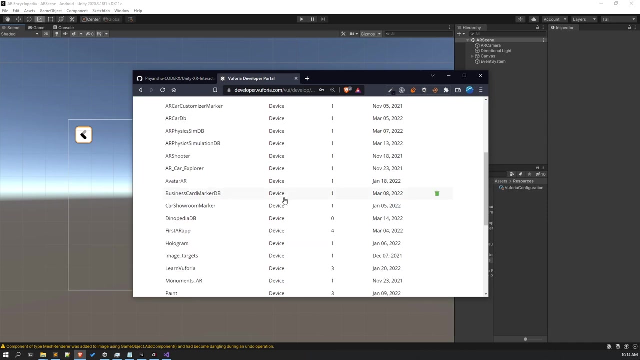 so now we have downloaded all the markers we needed, all right, now what you have to do is go to your target manager, click on add database, then give it. give it give the database a name, let's say dynopedia DB. all right, so then click on create and it's going to create a database for you. so 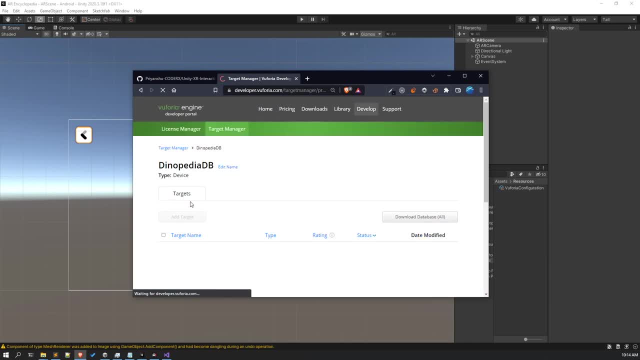 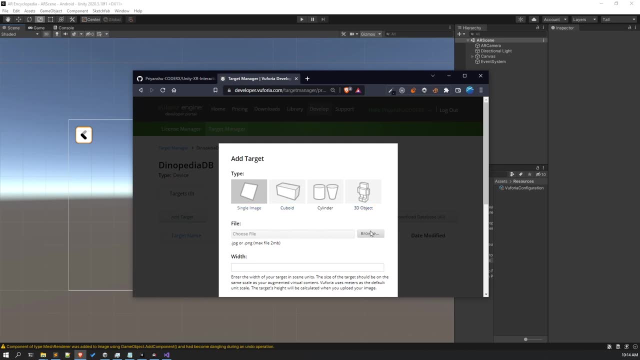 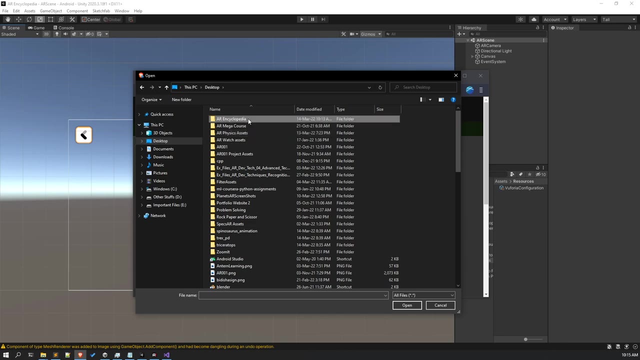 now what you have to do is, after opening the database, you have to add the targets. all right, so click on single image. all right, choose the image file. all right, so this is not the one. just yeah, here I got now. this is the marker one, all right, so let the name be marker one and give it. 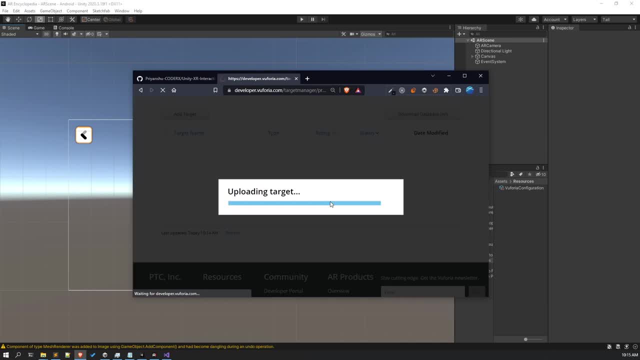 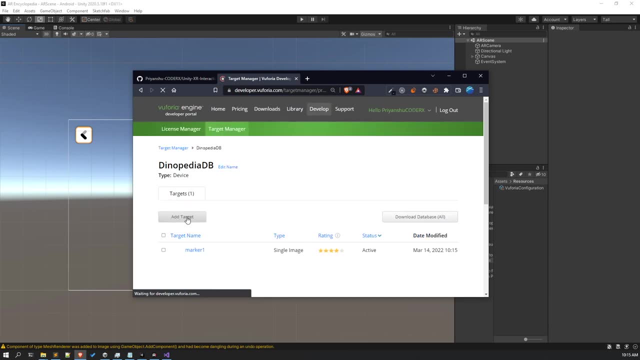 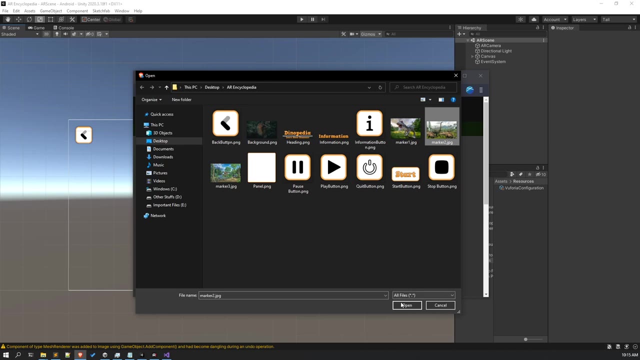 a width of, let's say, six, all right. and uh, wait it for, wait for it to add a new one. so that's it, add the target. and uh, let's add another target, all right, okay, let's again give it a width of six and add it. 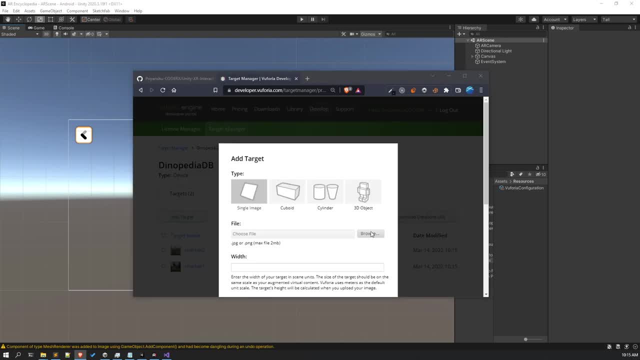 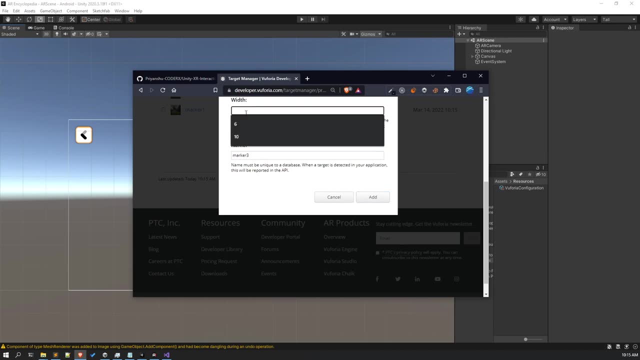 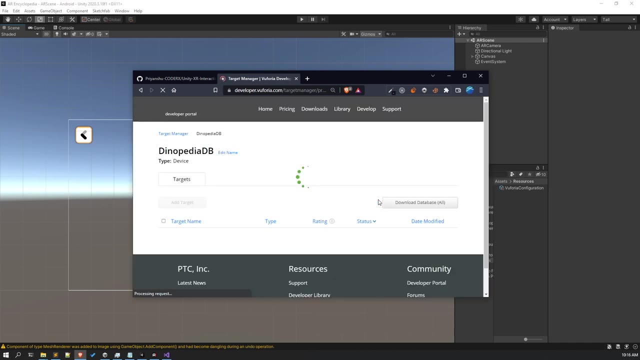 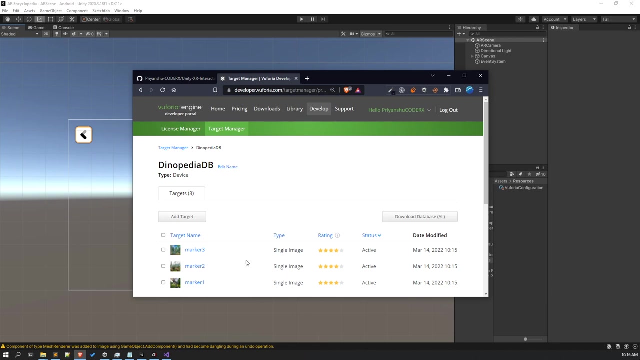 all right, let's add. add another target. all right, see, all these markers are taken from Google. all right, so you can find them on Google. only then click on add. okay, cool, so we have our markers, all right, and all of them are four star markers and that's. 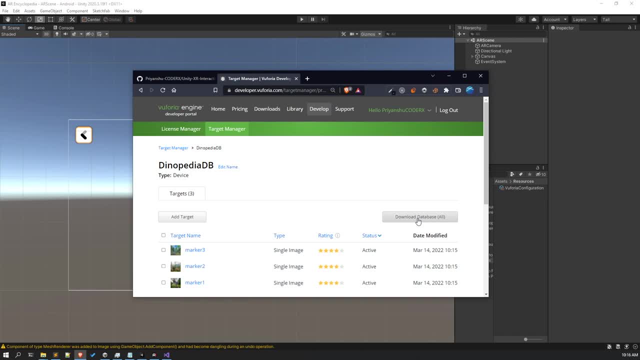 totally fine, anything, uh, between three to five is okay, but less than that don't even like give. uh, don't even work out with those markers, all right. and even I would suggest not to go for three star markers also, because their tracking is also not up to mark, all right. 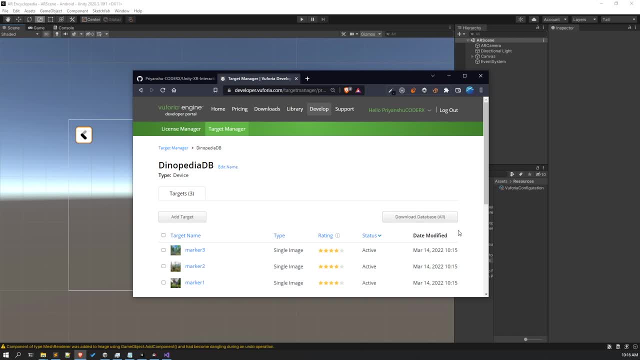 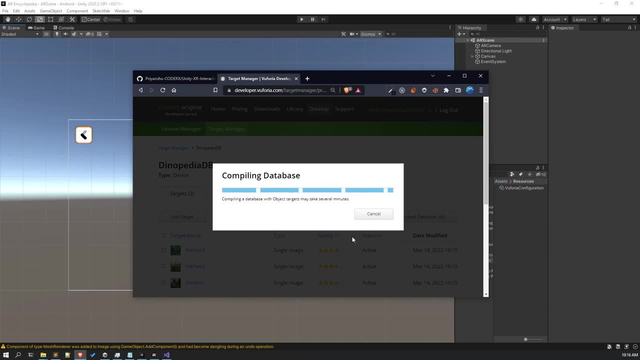 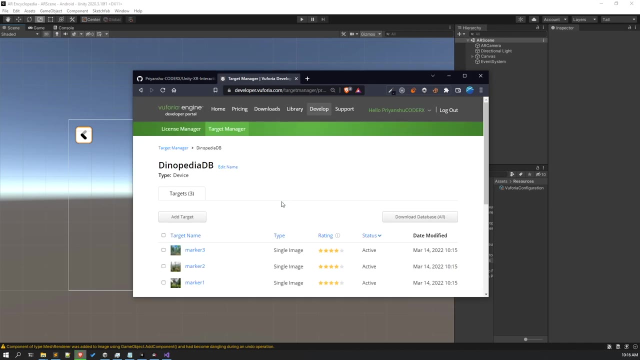 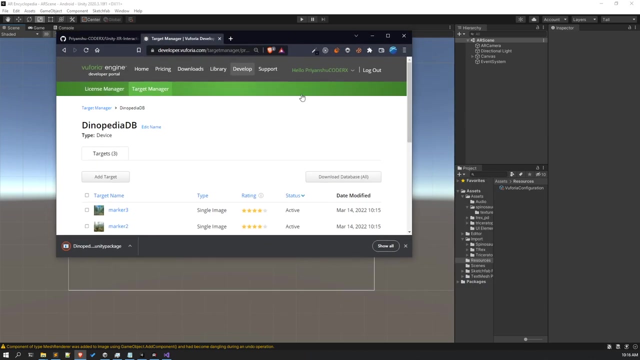 so always have markers having four to five stars, not less than that. now we have to download the database, all right? uh, I'm going to download the database, so it's going to take a few minutes and then it would start downloading. all right, so let me save the dynopedia, you know- package in here and, uh, after it's downloaded, let's. 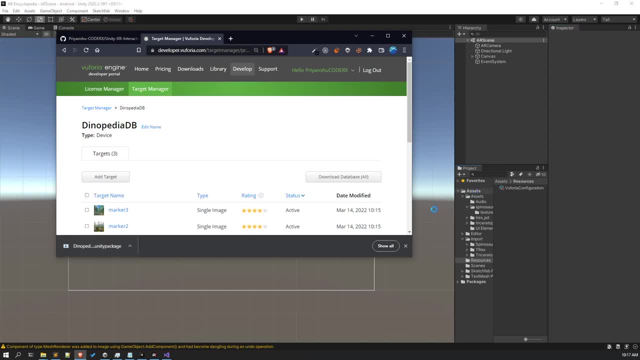 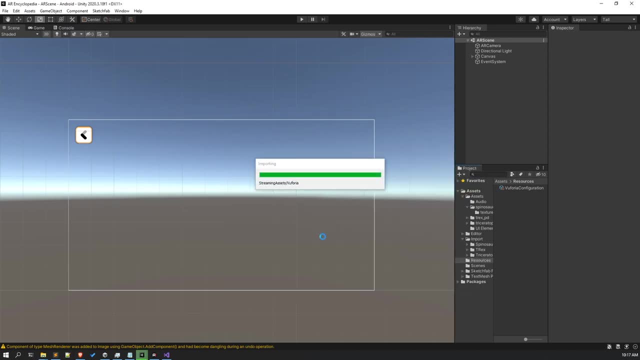 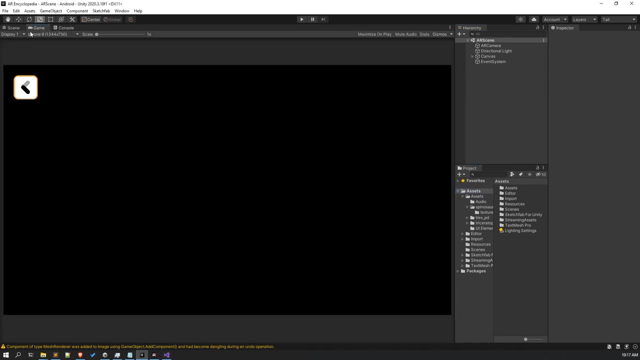 uh, import it all right. so here I got a window pop-up and click on import. so now it has started. importing our assets means our markers all right, and we are good to go now, as everything in here all right is is working pretty fine. our air can, uh, air camera is set up all right. now we have to set up our markers. so 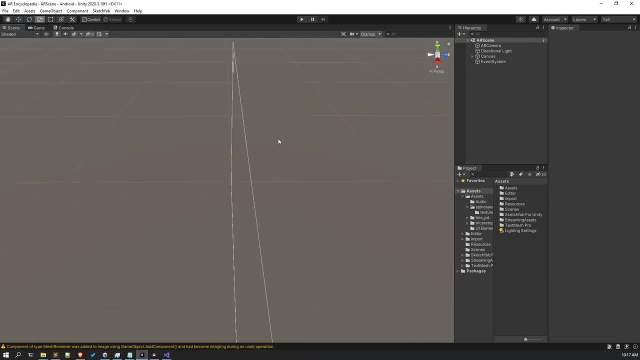 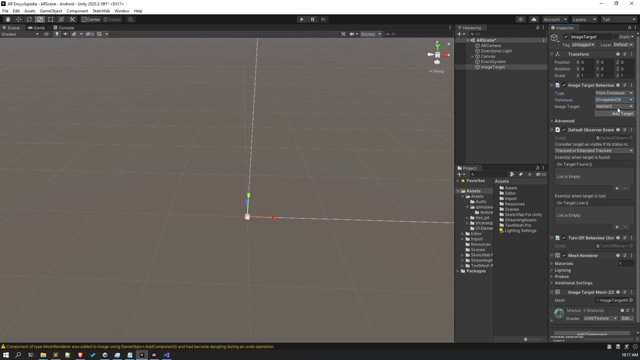 how? how do we do that? first of all, go out of 2D mode. all right, go out of 2D mode and uh click on. uh, there is right click view 4D engine image target. all right, in the image target, uh click on from database, select the database and get one marker. all right, and I'm. 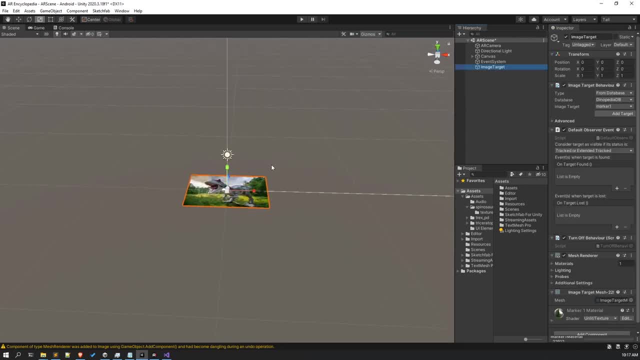 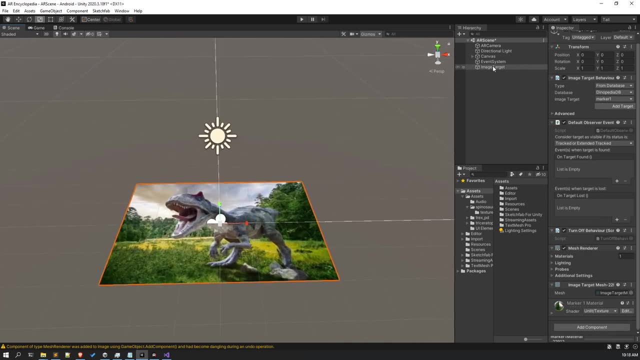 going to get the first marker for the first marker, of course, all right. here is our first marker. now what I want you to do is click on the image target. in here you will be finding an option: tracked or extended trap. click on track, all right, and let's give it a name: marker one or. 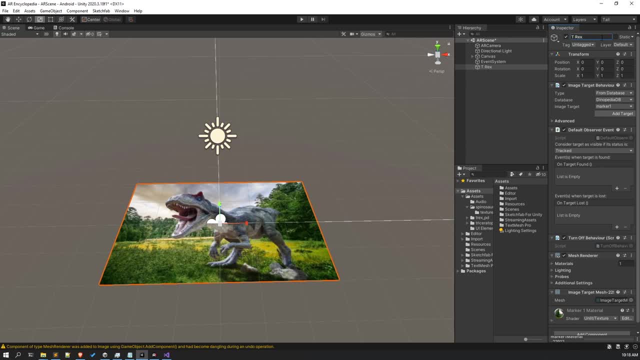 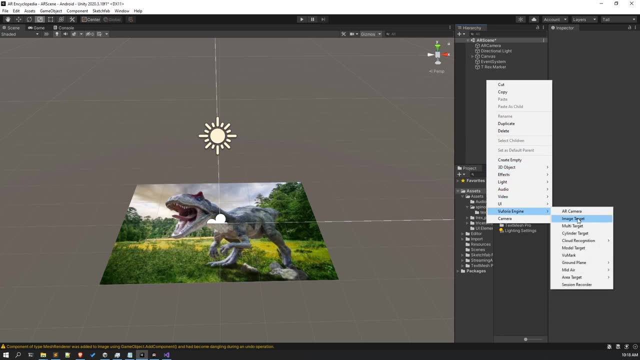 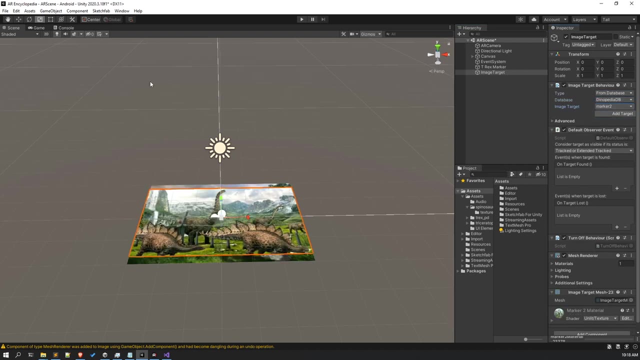 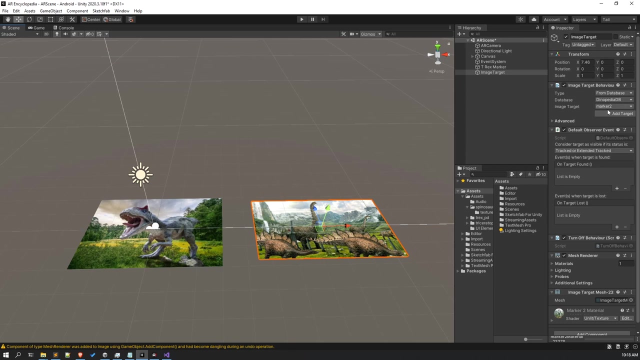 let's uh keep the marker one for the t-rex, all right. or let's name it t-rex marker, all right. let's add, you know another, another marker, and again let's select from the. let's get the marker too, all right, let's shift it, uh, in the side a bit, all right. now, uh name it spinosaurus. 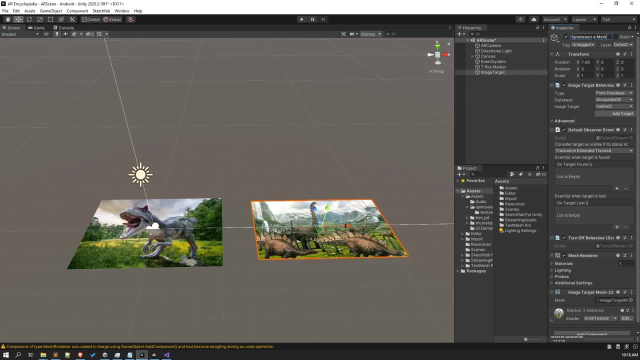 marker. all right. now again view 4a engine, another image target. now name it triceratops. all right, now select from the database. get the database and you know there is our marker three. all right, so we also got our. so we have our three markers right in here. 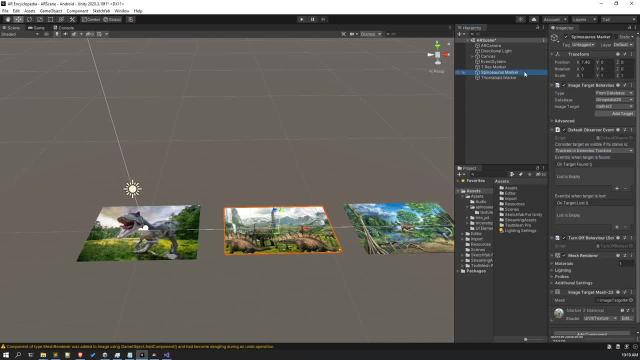 all right, okay, uh, let me uh shift it to tracked only. all right, all right. so let's check if everything is set up correctly or not. yeah, everything is set up perfectly fine. now I have the models imported in here. all right, it is of spinosaurus, t-rex and triceratops. 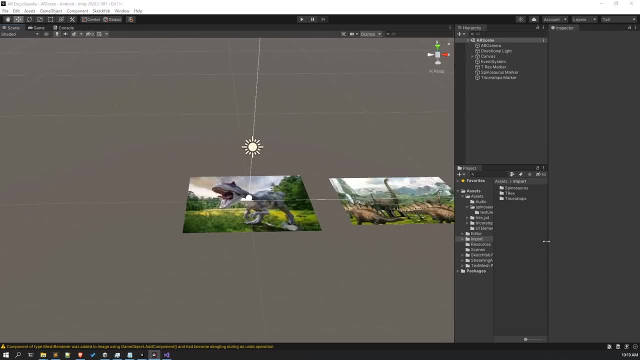 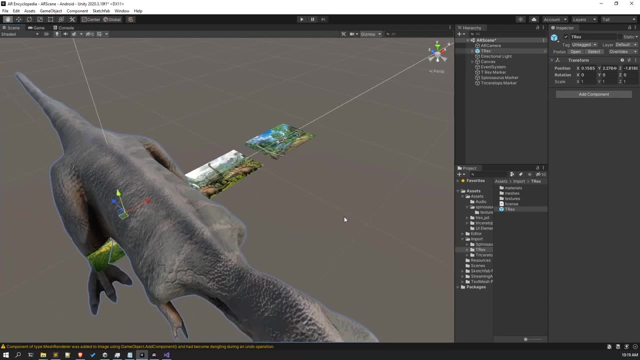 now, what I want you to want to do is I am simply going to add. first of all, I'm going to add the t-rex model in here, all right, here, all right, and you know, it's a, it's really, really big, and I'm going to scale. 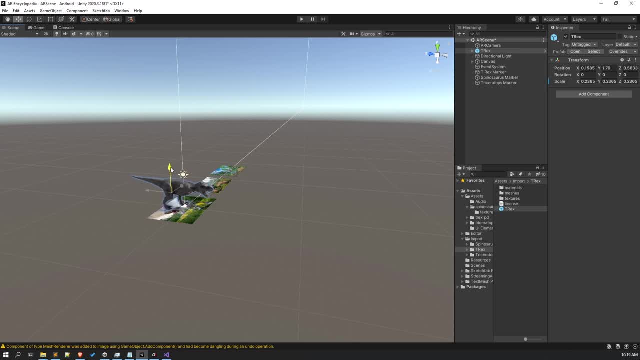 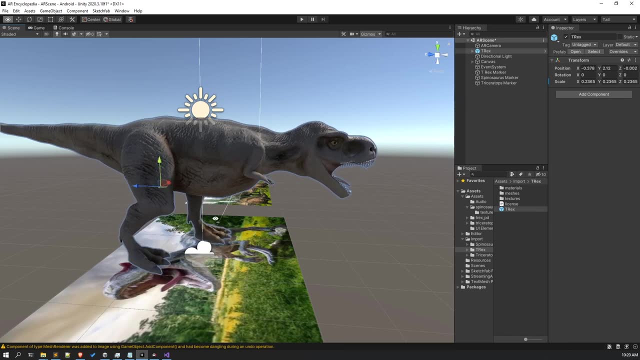 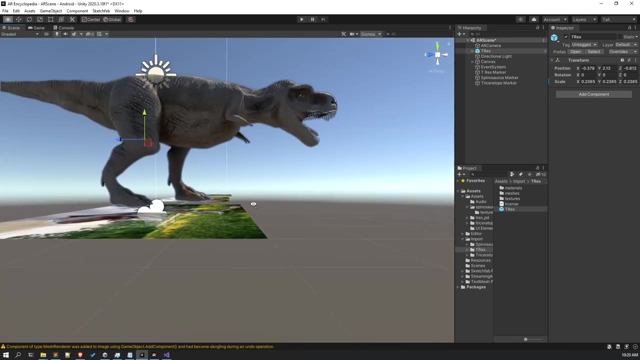 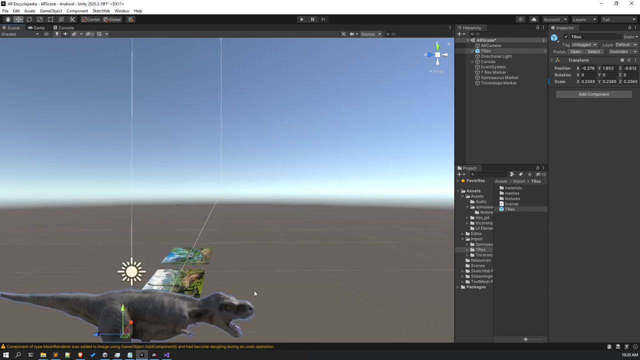 it down a bit, all right, and make it like this: all right, okay, cool. so here we go. we let's, you know, let's make him settle down a bit, all right, okay, cool. so here our first, you know, first model for the marker is ready. I'm just going to drag. 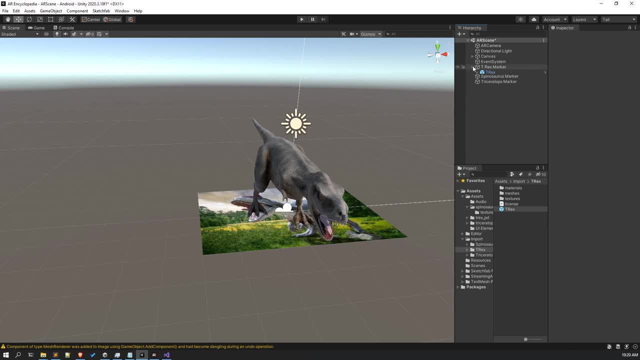 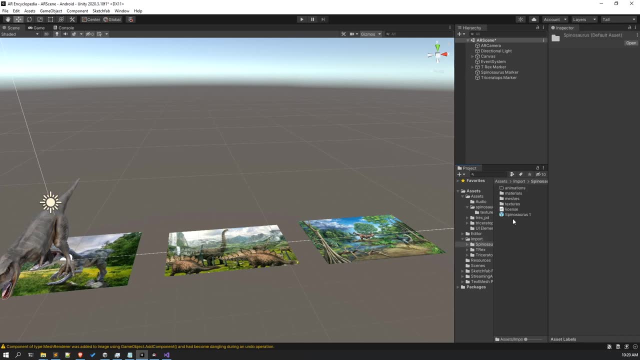 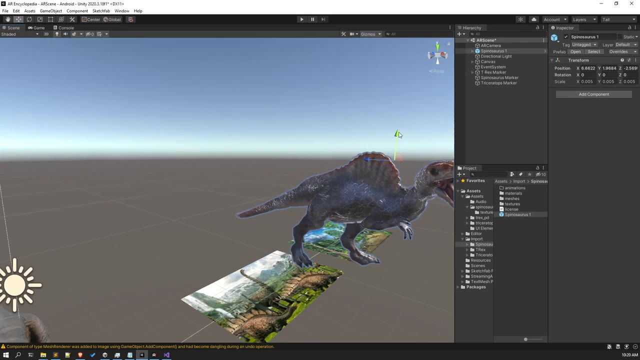 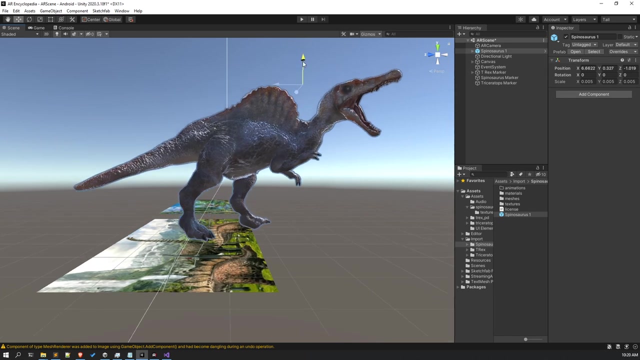 and drop it inside of the t-rex marker. all right, so our first one is ready. let you know. let's get the second one, that is on the spinosaurus. all right, very cool, great one actually. let's set up this one too. all right, if you want, you can add. 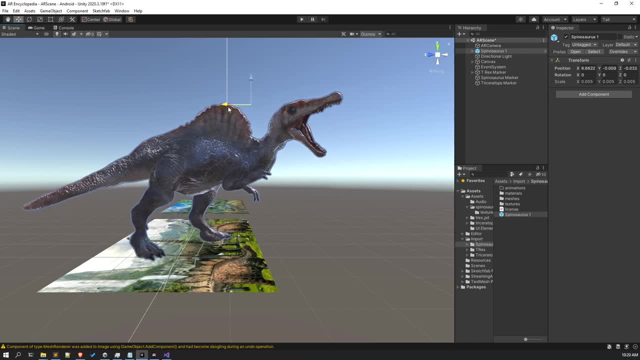 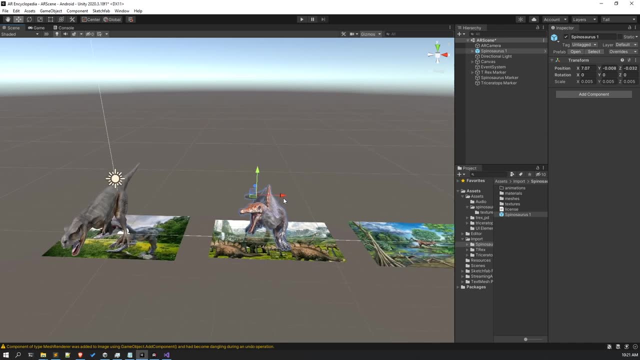 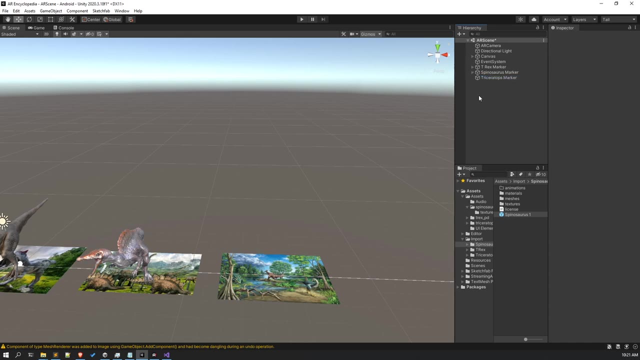 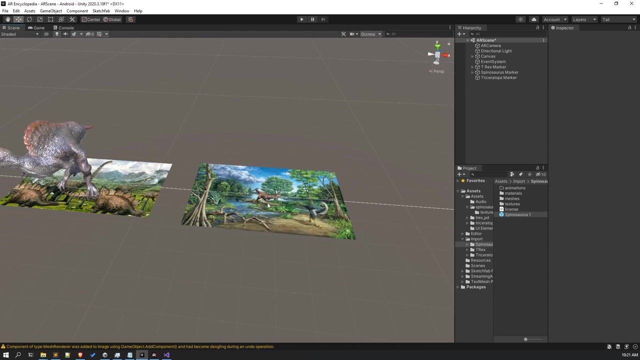 rotations, but for the dinosaurs one I'm going to. I'm not going to add the rotation, all right. I'm not going to add rotations in here, all right. I was actually trying to get animated 3d models for for dinosaurs but actually didn't got any like not in the asset store, not on sketchfab, even I. 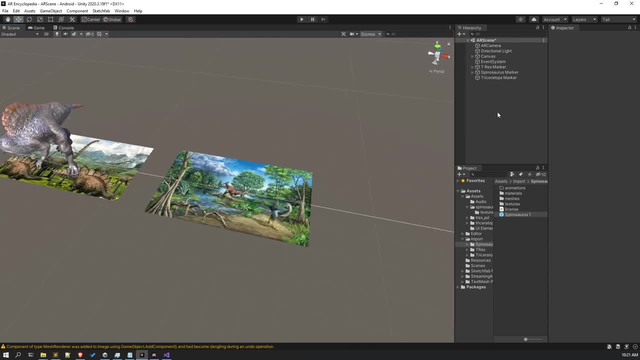 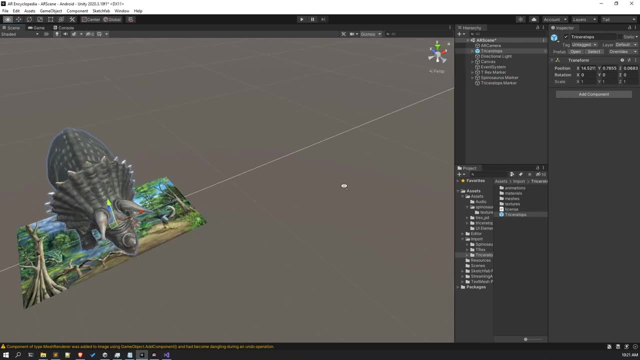 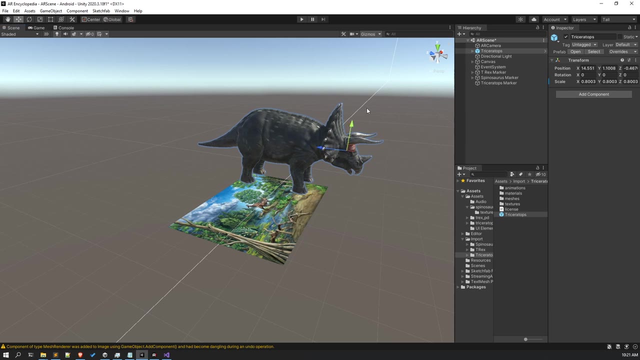 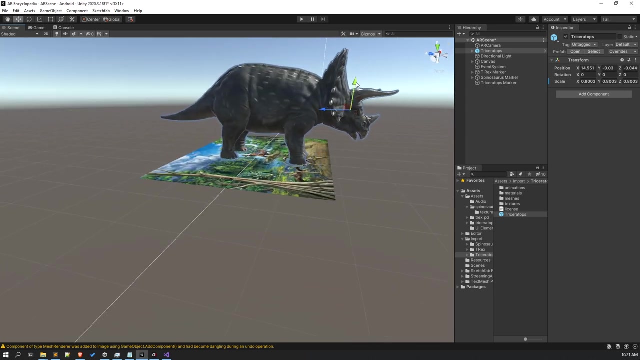 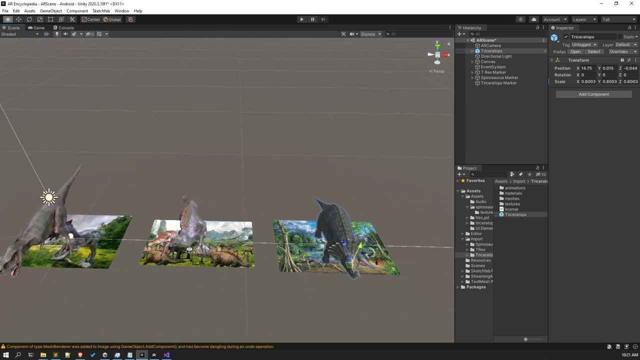 got some of the animated, but the animations were into a working, so you know, that's why I had to get these. now let's again add this one. oh, this is triceratops. all right, let's add this buddy in here. okay, cool, so now we also have our triceratops right in here. all right, okay, where? school? 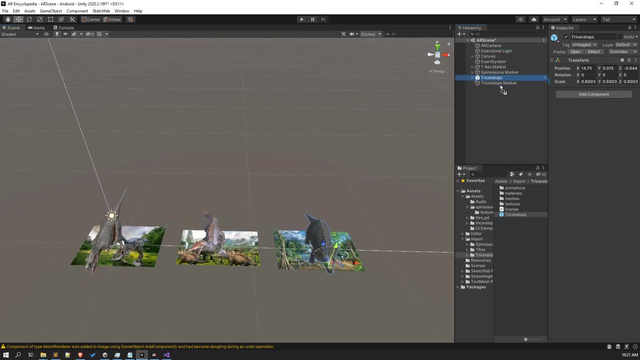 so now, as let's again make it a child of our triceratops marker, alright, so now our 3d models are set up. now you might be thinking, oh, this is it I want third project isn't? no, it's not, because I'm going to show you something more. what see? 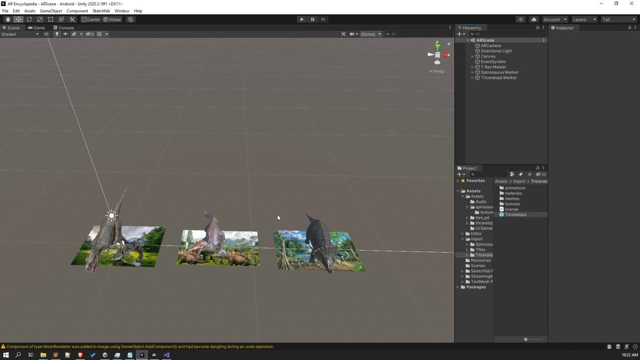 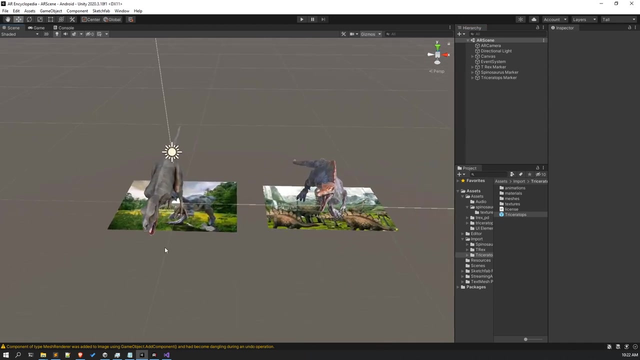 is an encyclopedia, right, there is an AR encyclopedia. how can we call it something an encyclopedia if it doesn't have any information about that particular thing that it is in there, right? so of course, I am going to add some more things to it. alright, as there's an AR book, this is an AR encyclopedia. I'm going to add: 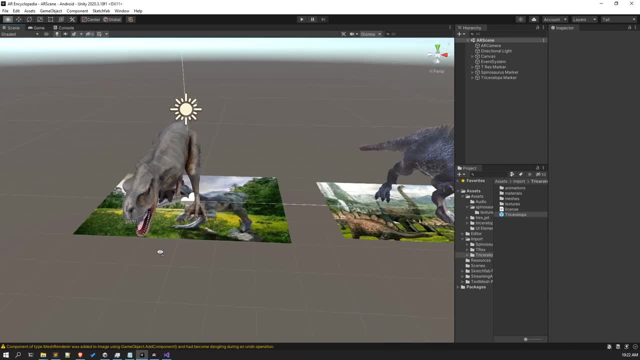 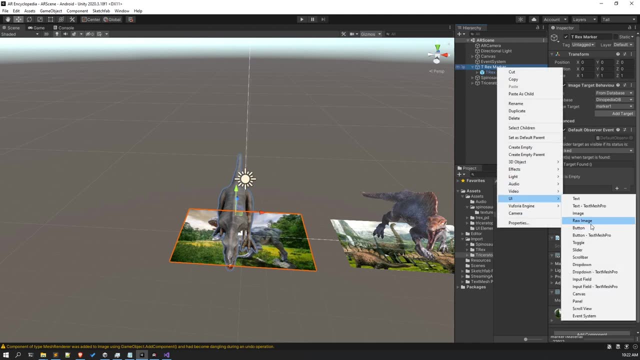 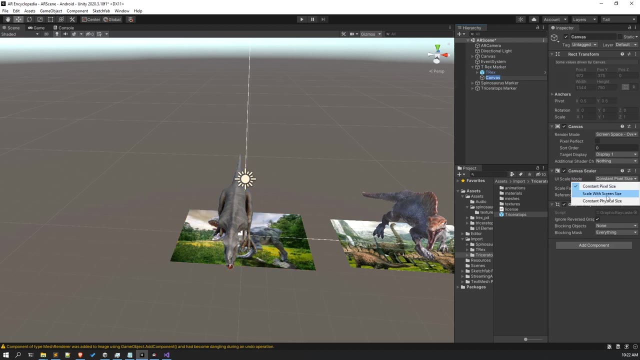 information too. so how would we do that? fairly simple, you need not to worry. first of all, go to the t-rex marker, create a canvas. yeah right, create a canvas. so create a canvas. all right, remove the, remove the constant pixel size and change it to scale with screen size. all right, in here you'll be finding. 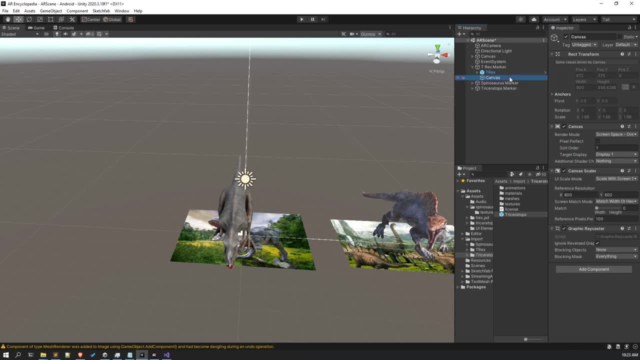 sort order. give the sort order, all right. sort order means it would be, means it would keep this particular dinosaur length layer, means this particular t-rex canvas on top of the main canvas in here. alright, so that's why I give it a sort order of one. all right, so that it. 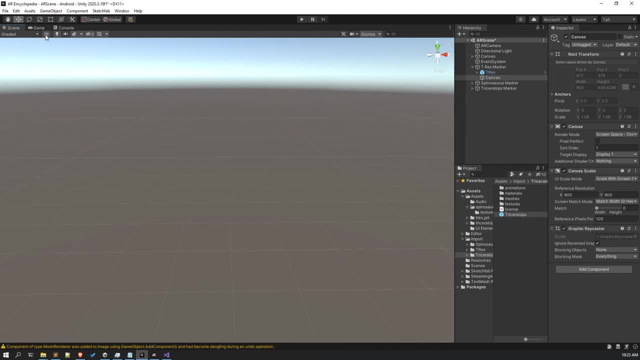 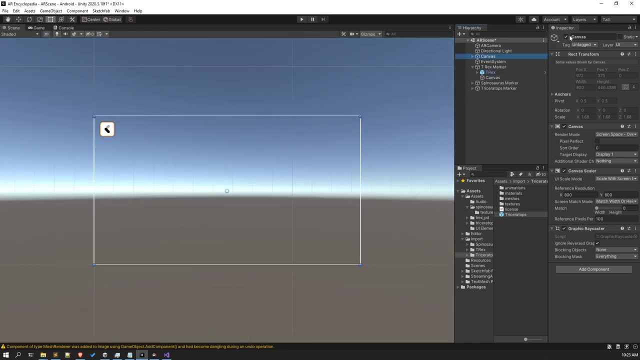 doesn't overlaps or something. right now, go to your 2d mode. all right, go to your 2d mode, select the canvas. first of all, I want to disable this- you know, this main canvas, so that I get the full t-rex canvas in here. now what I want you to do is right click UI image, give it a. 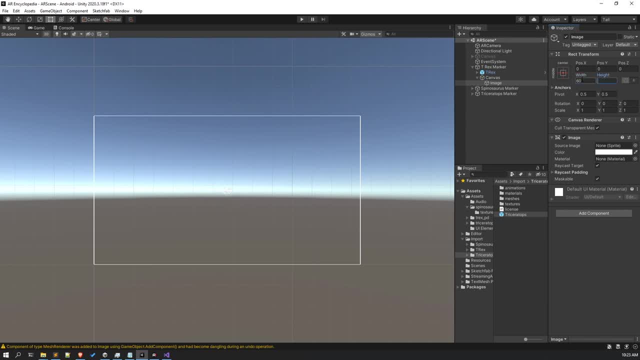 width of, you know, 60. all right, give it a width of 60 and cut it down to the, you know bottom left and, you know, change the portion to 40 and 40 or maybe 50, and so if you actually let's check if it's aligned, okay, so I'll. 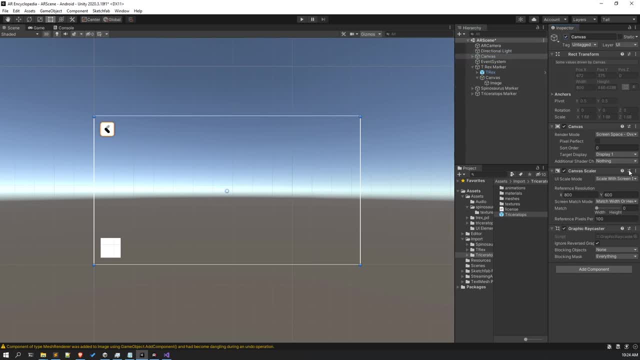 aligning with, uh, you know, this particular canvas, let's check this one, all right. and uh, you know, select this i button. all right, this is going to be our information button and i'm i want size of this button means i want size of this button to be like this, all right, so width and. 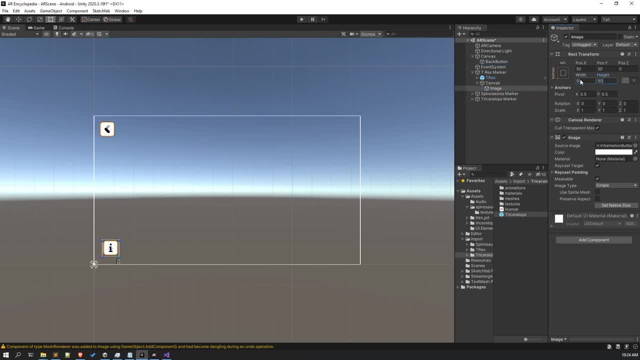 height is 50 and 50, let's give it 50 and 50, all right. and let's make it 40 and 40, all right. very cool, all right. so yeah, one of our canvas is ready now. what i want you to do is you have to add uh. 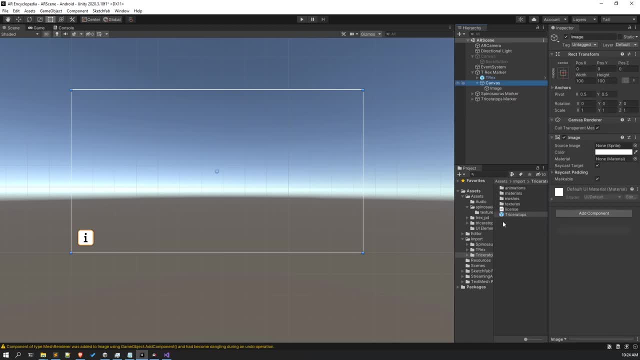 you know another image that is equal to ui image: all right in here. i have a panel right in here, all right, and i want let's say let's scale it up a bit, all right, and uh, let's anchor it down in here and let's reposition it okay. 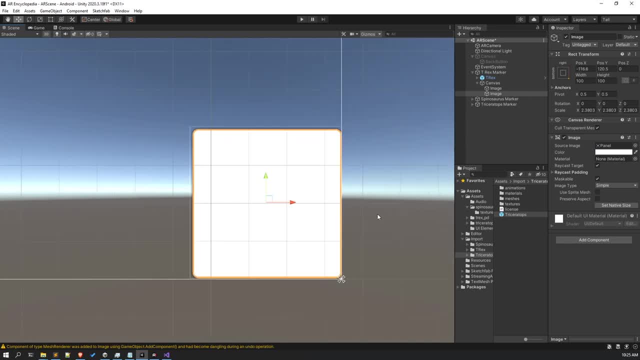 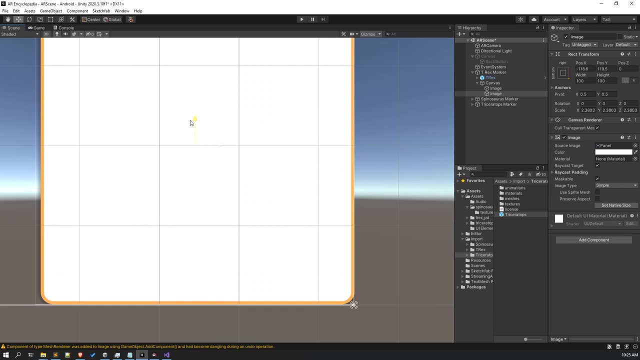 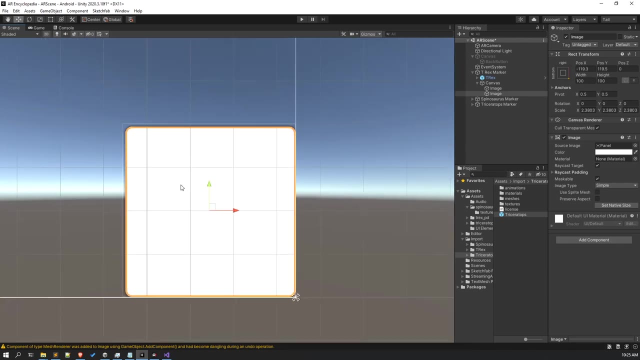 all right, let's see if any spaces are left or not. i don't want any spaces to be left, or all all right, okay, cool, so now let's see in our canvas. all right, let's, you know, let's, let's increase the size of the panel a bit. 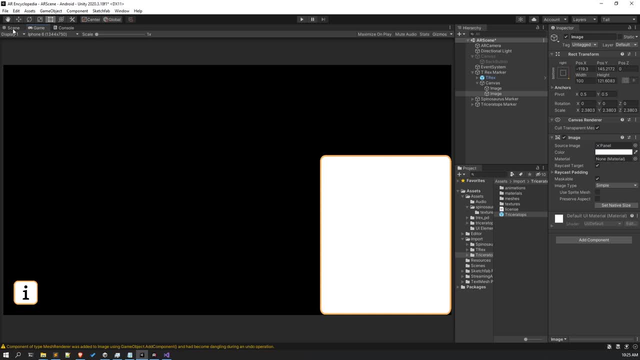 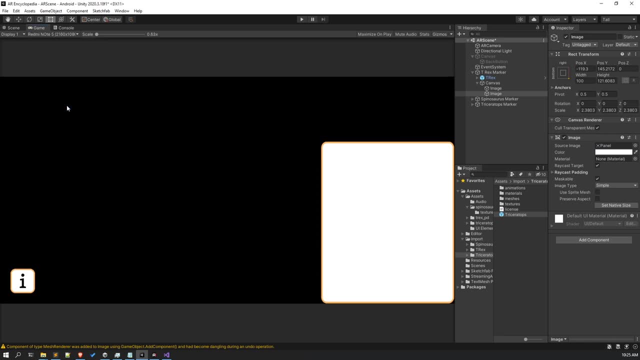 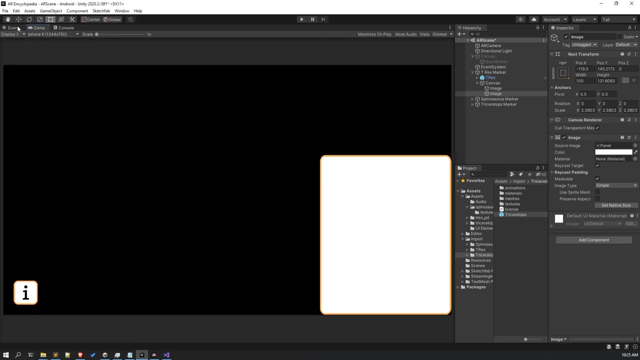 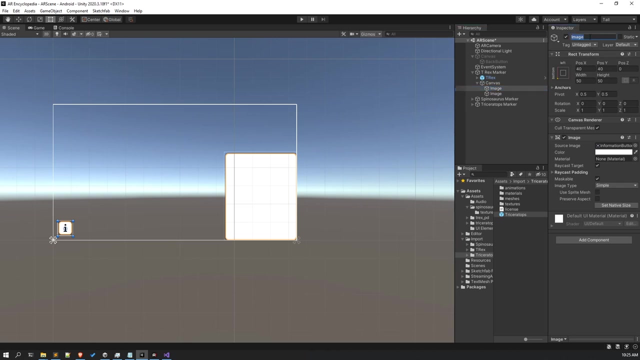 all, right, now it looks, you know, good, right, isn't it? let's, let's check, okay. so, yeah, this, this ui works with. you know all the basic resolutions we have right now. first of all, this, i, this, i is a button, so i'm going to name it information button. all right, and you know what i'm going. 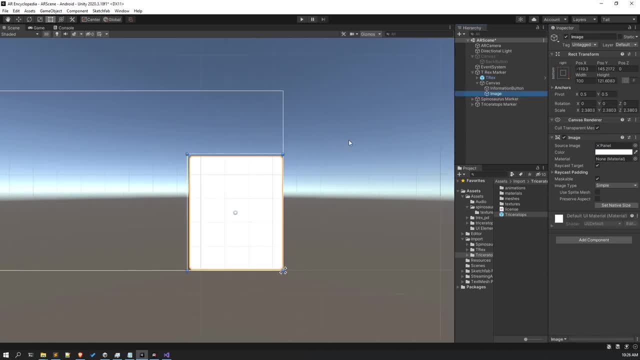 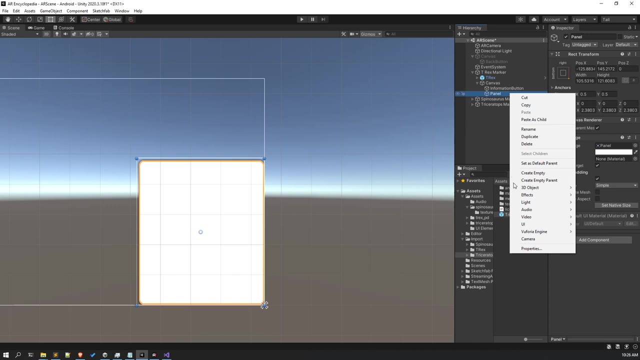 to do? add a button component to it. this image is, you know, a panel, so i'm going to name it panel and all the information, all right would be. all right. all the information would be under this panel. so what i'm going to do is right click. uh, make sure now, all the things i'll be creating all right will be this. 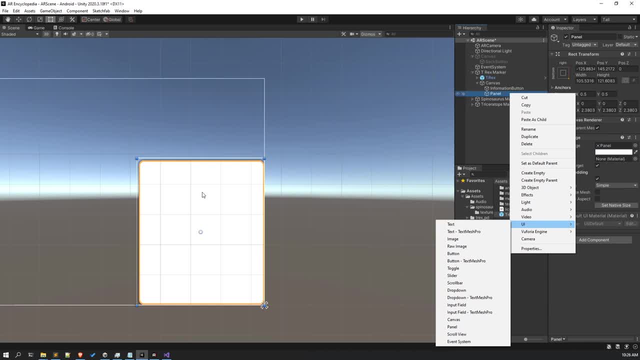 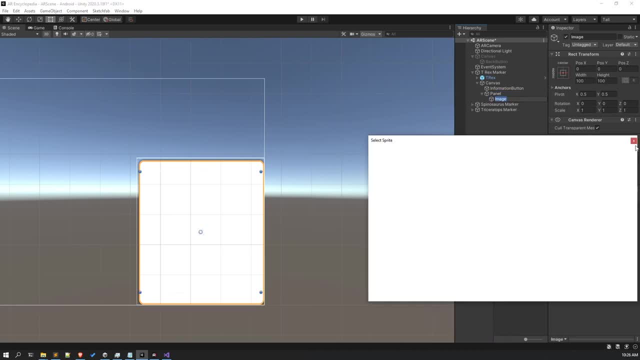 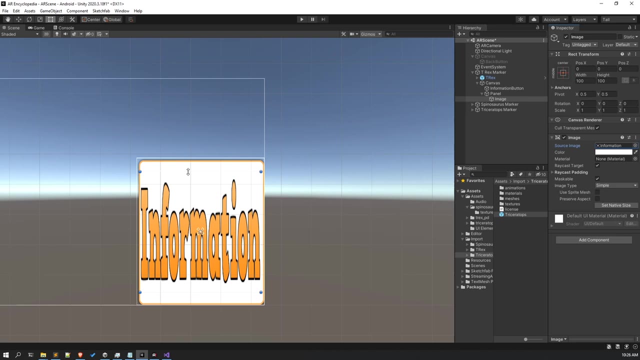 panels child- already the text and all the stuff that i'd be creating with panels child. all right, so what you have to do is ui image. all right, we have an image. select the heading. that is the information heading right now. let's resize this thing a bit. 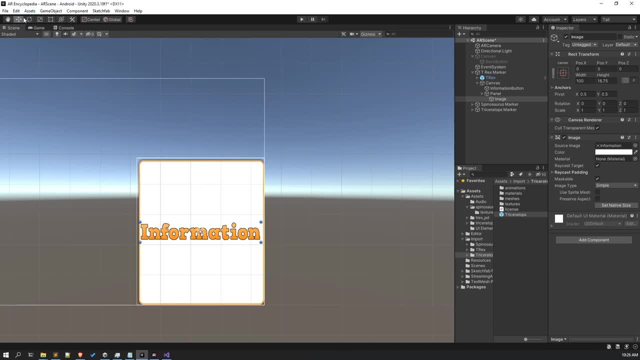 all right, okay cool. now again, rect, transform alt, anchor it in here, reduce, you know, scale it down a bit. okay, cool, we are good to go now. also, one more thing: we have to add a text in here. before adding a text, all right, first of all, let's name the change, the name of it. 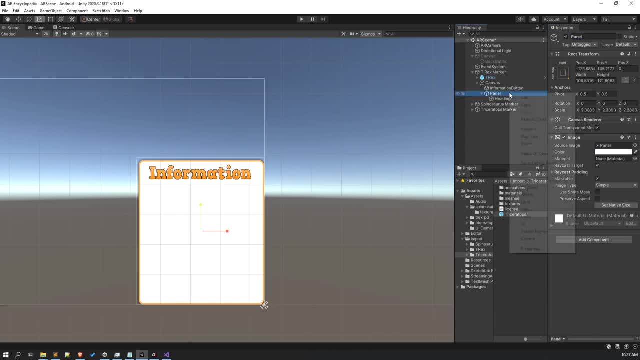 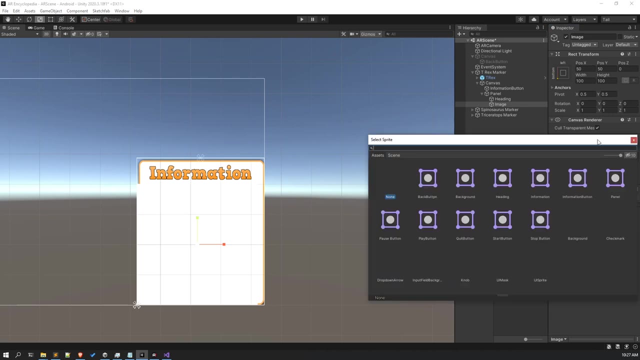 i'm going- i was going to say name the change of it. now we have to add some more buttons, that is play, pause and stop button again. go to you know image and let's anchor it down as of now, all right. and let's, let's get the button, uh size. that is the play and this will be the play button, all right. 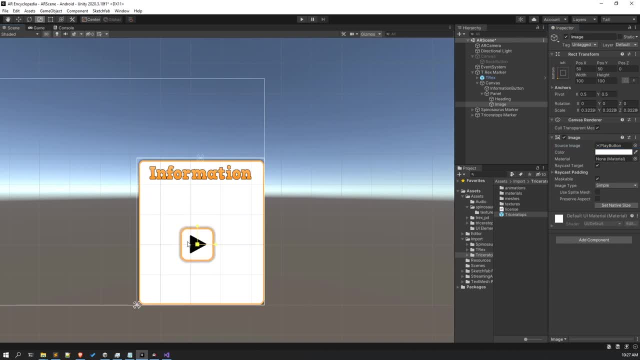 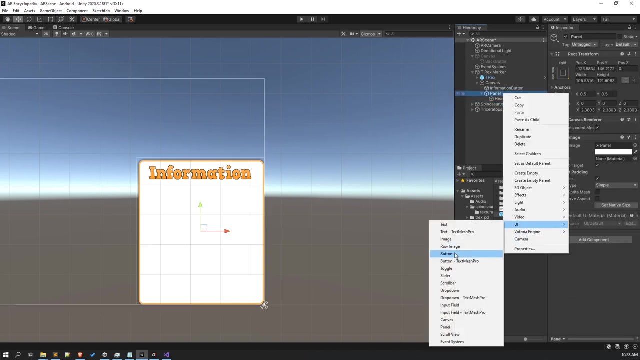 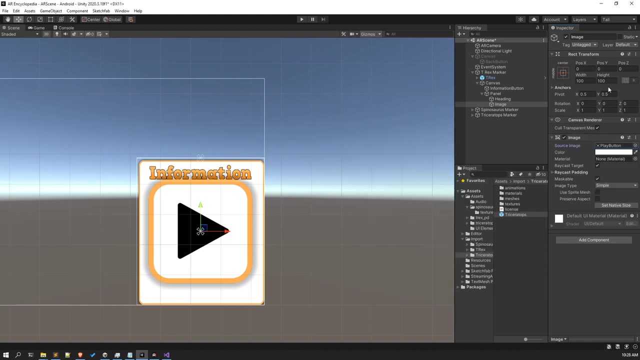 let's say, now drag and no, let's change the size of it. okay, cool, so now just wait. all right, let me. let me start it from again. so again go to you know ui image. no, uh, let's do all this over here thing before anchoring it. alright, let's get the width to be 20, maybe. okay, cool, now anchor. 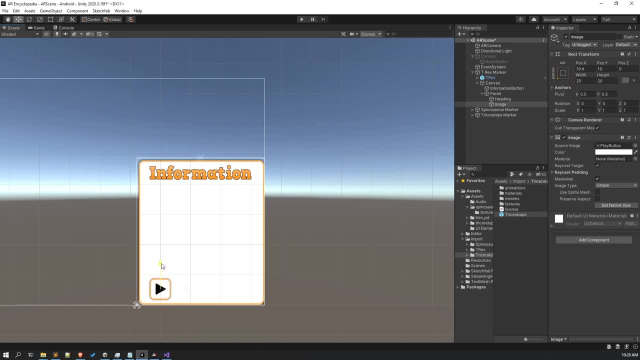 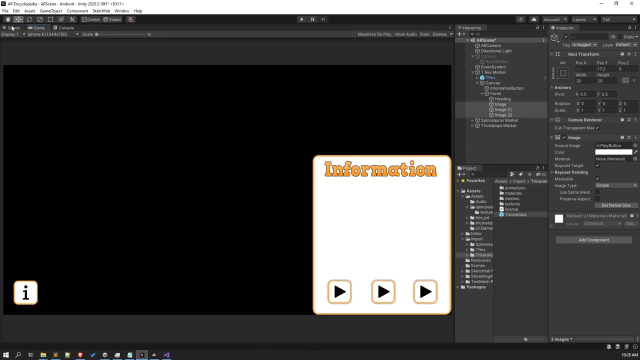 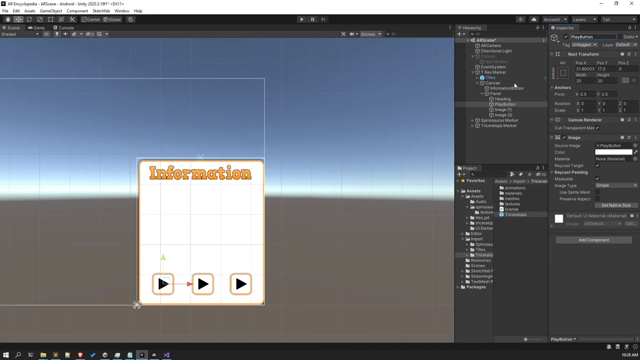 it down. alright, now reposition it so you know it looks good. duplicate it, alright again. duplicate it okay. so now it does look good. alright, make it to the center. alright, so that it looks okay. okay, that's, that's pretty good. change the name to play button. change this one's name to pause. 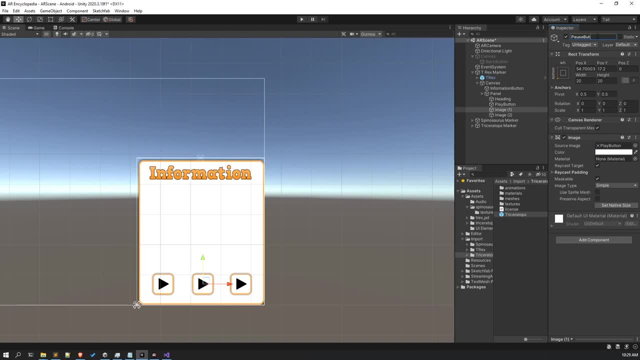 button. all right, just give a moment. all right and change this one's name to stop button. actually, I have the audios. all right, this would be playing the audios in there. so also select all the three buttons. add you know button component in here and we are good to go now. oh, 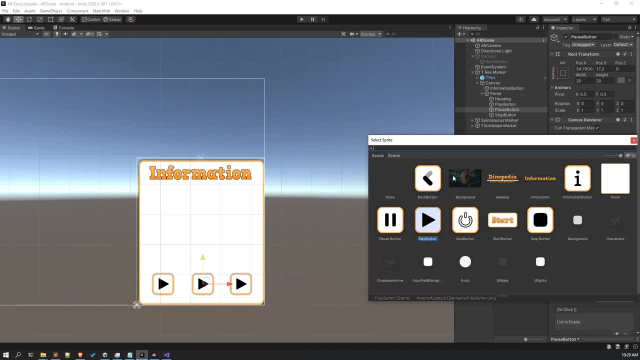 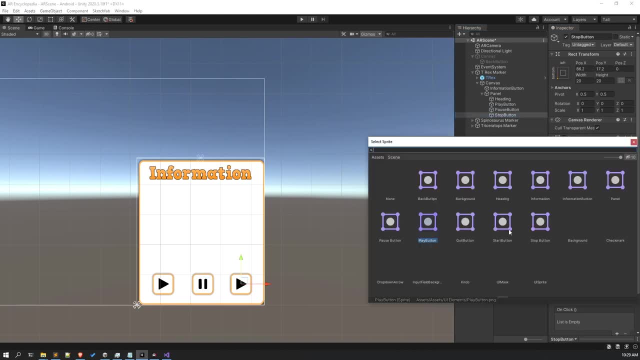 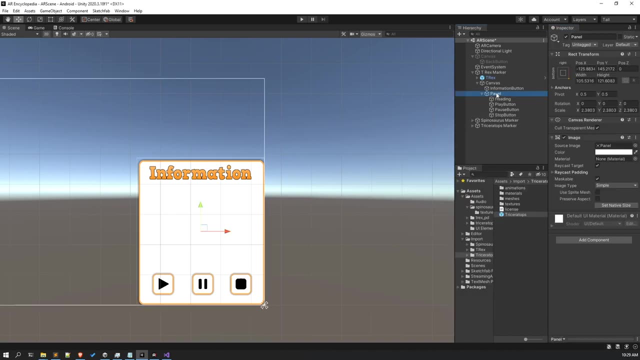 yeah, also I have to change. you know the picture of it right, so I'm going to do that. okay, so pause button- got the pause I can. stop button is going to get the stop in there. oh yeah, you got it all right. it looks good. right now let's add a text in here. all right, so click on UI. always use. 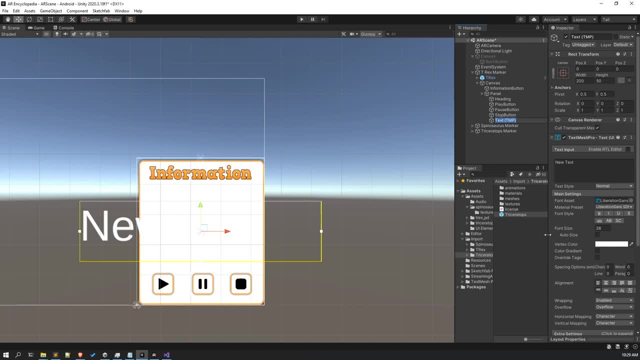 text mesh Pro- all right, use nothing except text mesh Pro. now, first of all, let's change the text color to black, all right, and let's resize it. all right, let's resize it, change the text size to 20 and first of all, we have to create a font asset, because we have a different type of font we have. 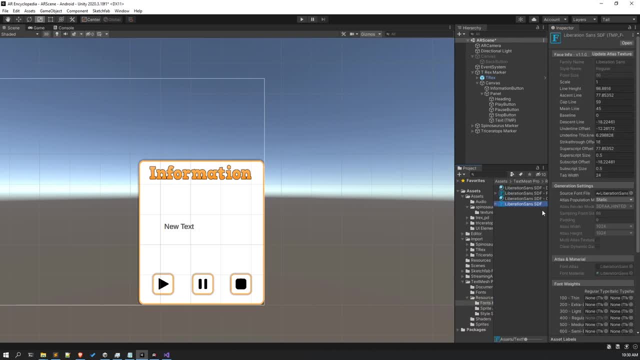 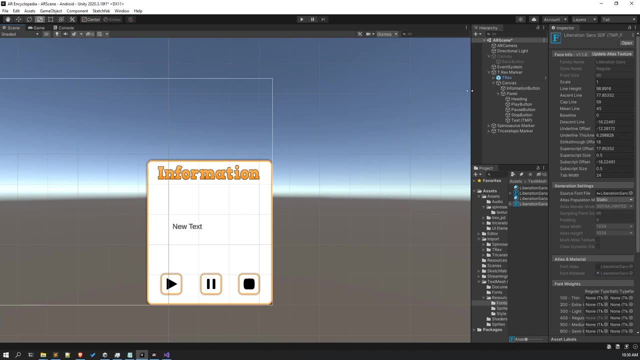 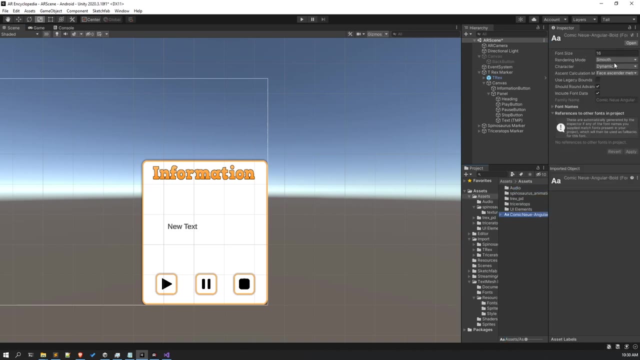 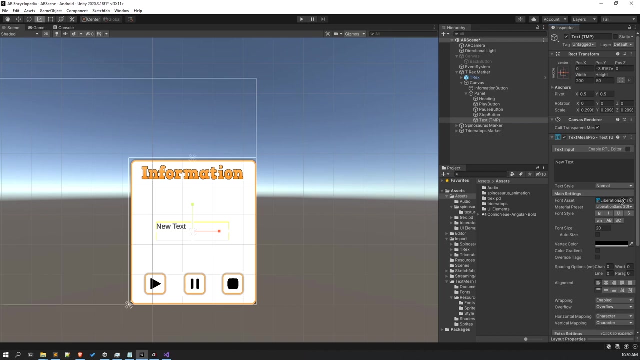 a font and let me show you one thing. this text mesh Pro only, except as the if type font for it. so currently the font, I already have a font called comic new, all right, so this is a comic new bold, so this is a font tolerant, but we won't be able to apply it. let me show you see, we are not able. 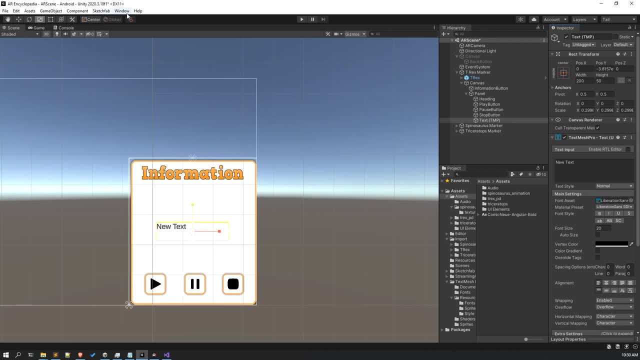 to apply it. so to apply any font for into text mesh Pro. it's very simple. we are going to apply it. click on window: all right, click uh here we'll be finding uh text mesh Pro. click on font asset creator: uh window will be popping up. drag and drop this font asset in here. all right, click on. 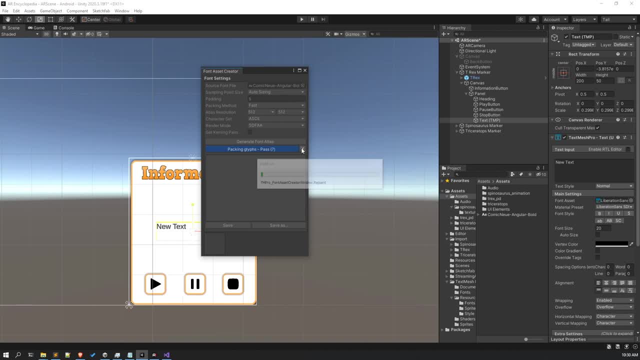 generate font alias. all right, so it's going to take a few seconds and it would be, like you know, creative. create the font asset for you, the, within no time. all right, and click on save. so here we got our font asset right in here. all right, and now what you have to do is click. go to. 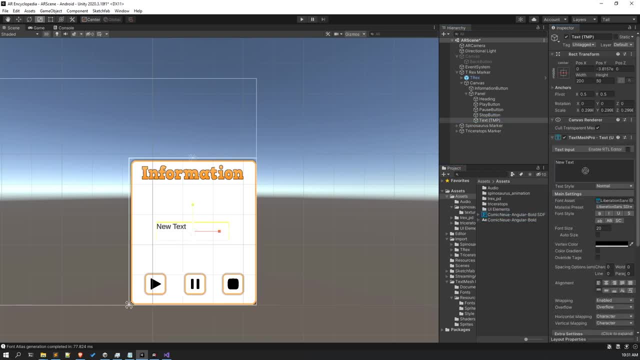 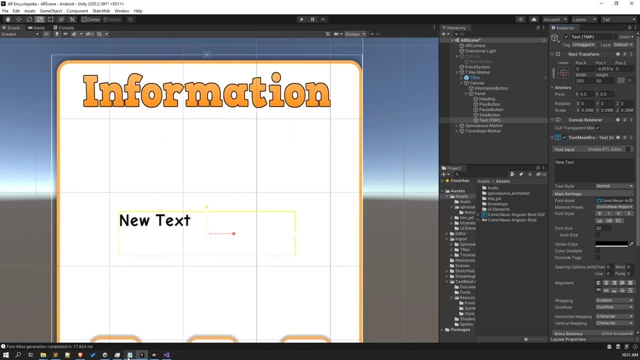 the text. all right, just wait, go to the text and drag and drop this font asset right in here and see we got our description. panel means description text. now I have some text already written in here, all right, so I'm just going to copy it in here and simply paste it in the panel. all right, cool now. 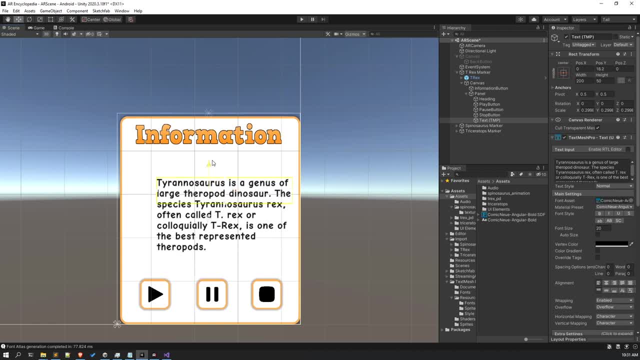 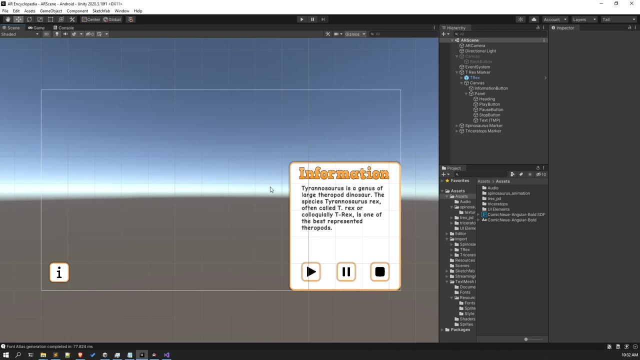 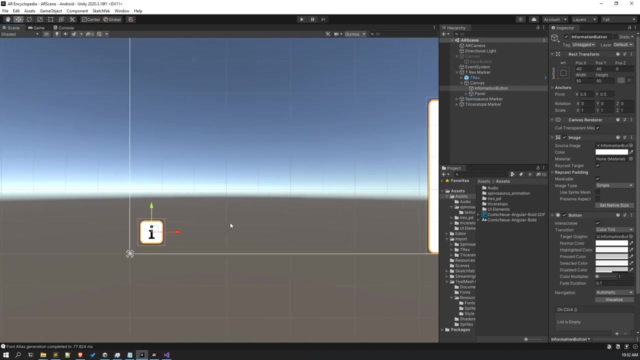 these looks pretty good. all right, doesn't they? and Center them all right like this. okay, cool. now, as we have got our information panel, we have to also code. all right, code is. code means uh, I want to click this button. all right, and enable and disable this particular. 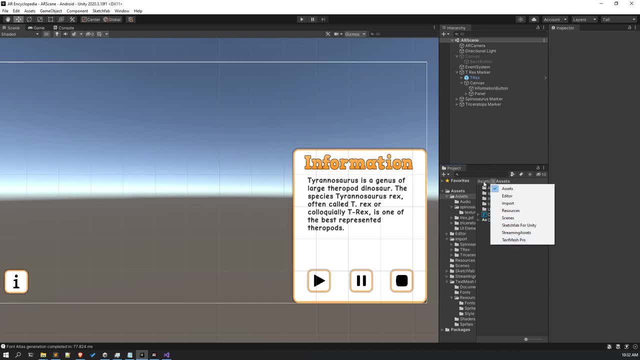 panel and creating the script is fairly simple. what you have to do is go to asset, create a folder of called scripts. all right, okay, the folder didn't got created. all right, okay, scripts- all right. after you create this folder, scripts- all right, you have to create a C sharp script. 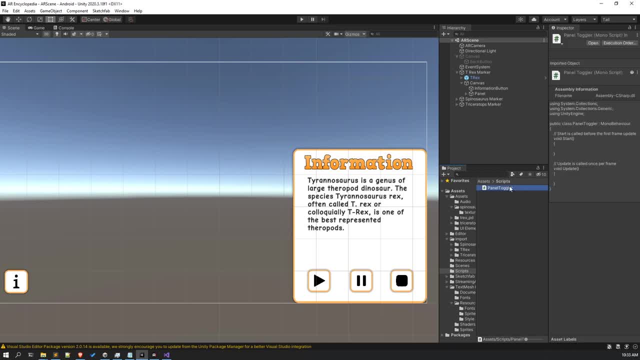 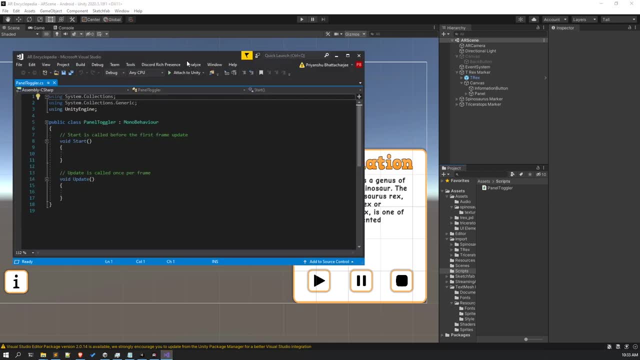 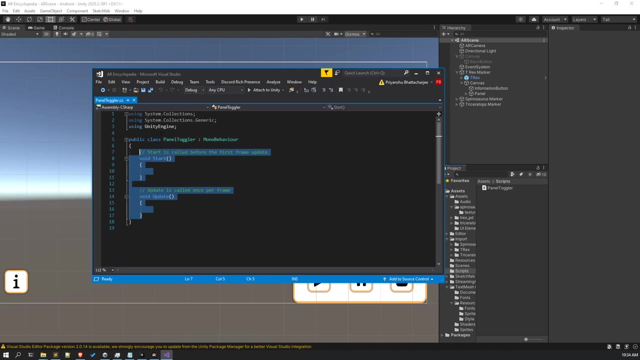 so now our script is created, I'm simply going to open it all right on my Visual Studio. so let's get this thing going in here, all right, great. so first of all, let's start coding it. see, first of all understand the mechanics. all right, you? there are two ways. you. 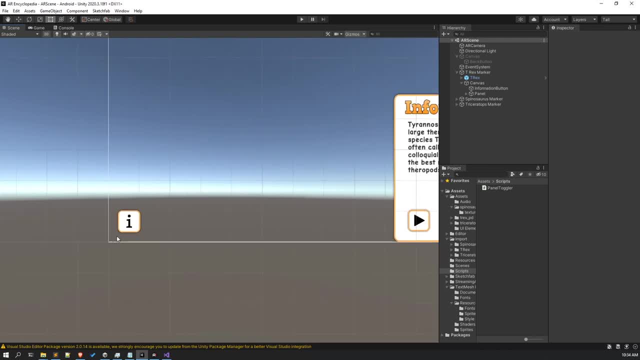 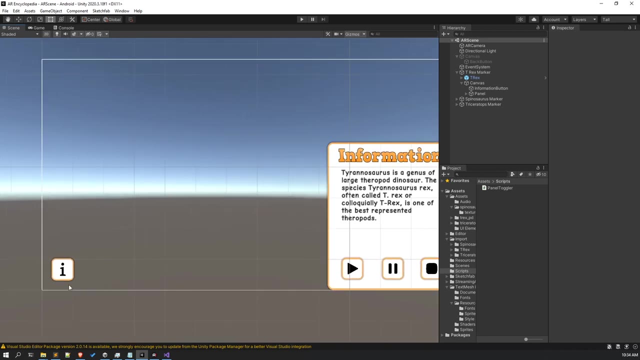 can do that. all right, first of all, uh, let me tell you one way. that is the first way- would a very simple way- actually, both the ways are simple, all right. so the first way would be, uh, adding a set active function to it. all right, set active means, uh, when you will click this button. 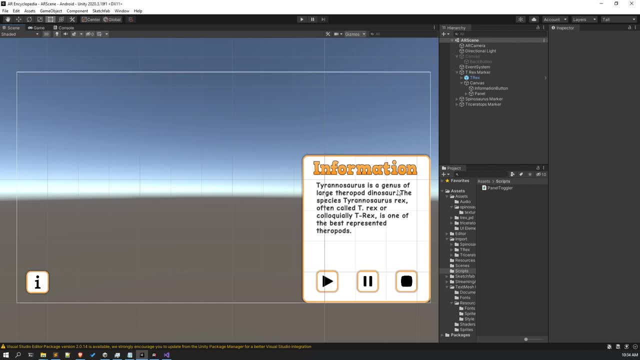 this panel will be deactivated from the first. so set active function would actually activate that and with that, all right. also disable this button and add another button. all right, that is, activate another button that would be less looking similar like this but would be having a different function, that is, it would be setting- uh, it to false. all right, setting the set active to false. 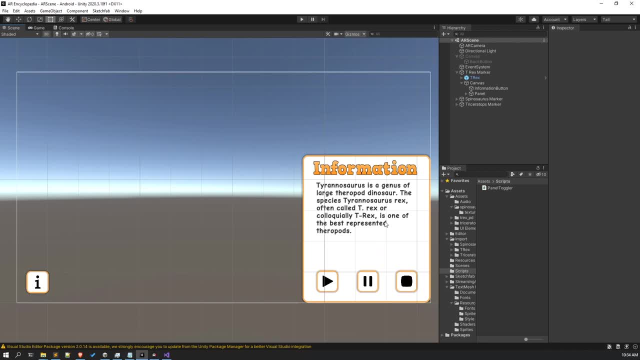 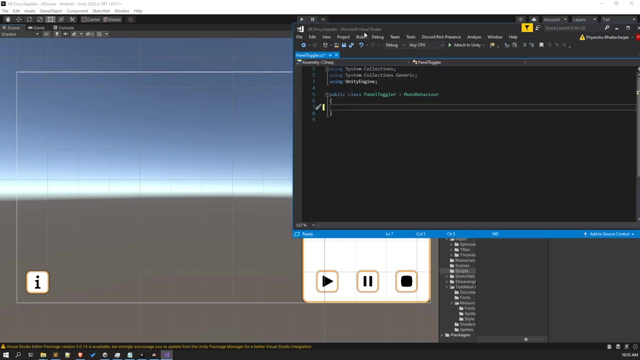 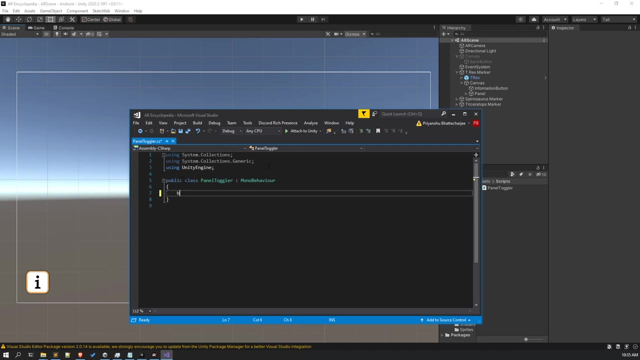 and that would make this particular information panel disappear. right, another way, all right. this way is: uh, i prefer to do it this way. so what you have to do is first of all create a variable. so basically, in this way would be using this single button only to switch on and off the panel, all right, so this is a little. 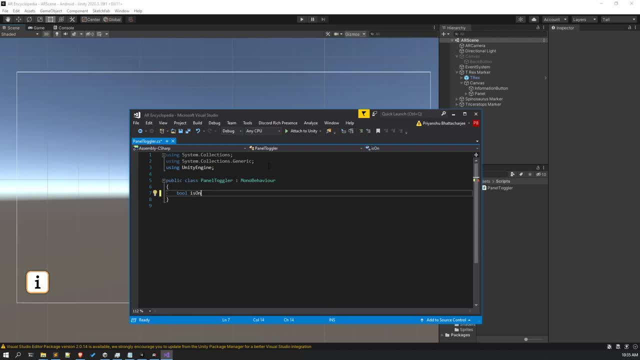 this is less hectic. so first of all, uh, create a boolean variable and set it to false. all right, let me increase the size of this editor a bit now. create a serialized field, all right, and so this is the serialized field, that is. i will tell you. what is it so? game object. 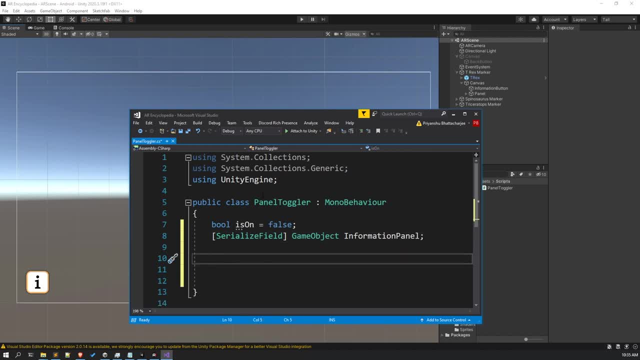 information panel. basically, uh, this serialized field parameter. basically, first of all, uh, understand that this is a private, all right, this is a private variable and, uh, the serialized field helps us to serialize this, that is, show this private variable in the inspector. all right, so that's it. 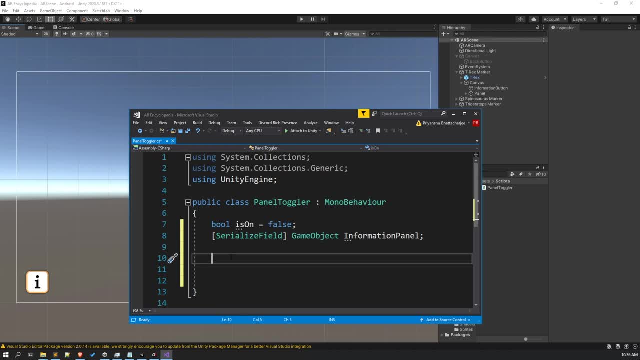 what the serialize field does it. it serializes this particular variable even though it's private in the inspector main. all right now. click on create a function that is public. void on toggle button click or, let's say, toggle panel. all right now. this, this thing is fairly 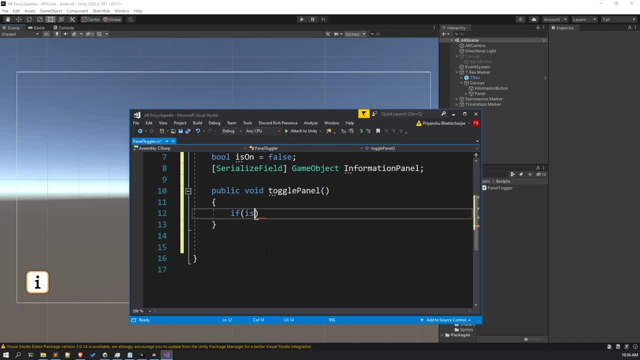 simple click on means right, if. if this is panel is on, what you have to do is you have to set activate to false. all right, you have to disable it and set the is on to false. now in the else block, just copy this, let this two lines and paste it in here and: 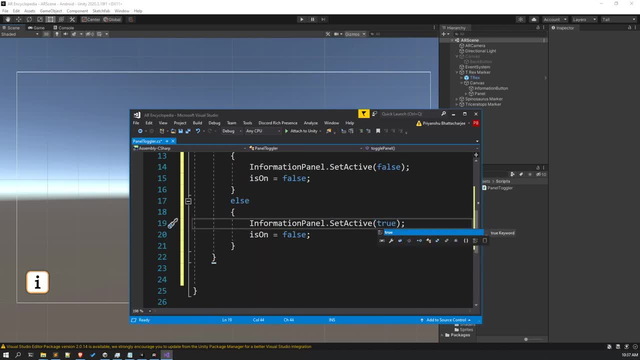 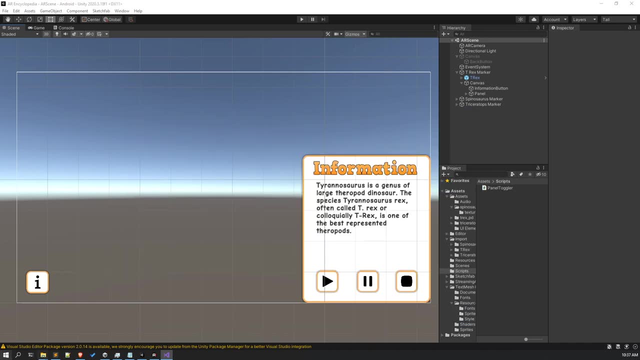 change them to. you know? true, all right, okay, very great. so now let the script compile. all right, so our script is compiled. what you have to do is go to go to this, you know, go to this canvas. all right, add the script in here. all right, add the script in here. go into this. 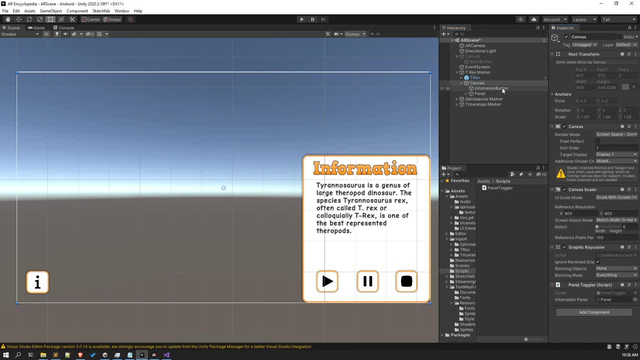 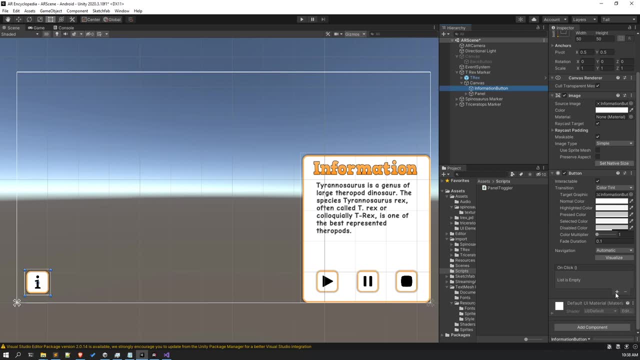 drag and drop this- you know information panel in here and you have the information button right. so in the on click parameter, click on the plus button, drag and drop this canvas in here and you would be finding an option called panel toggler and click on toggle panel. 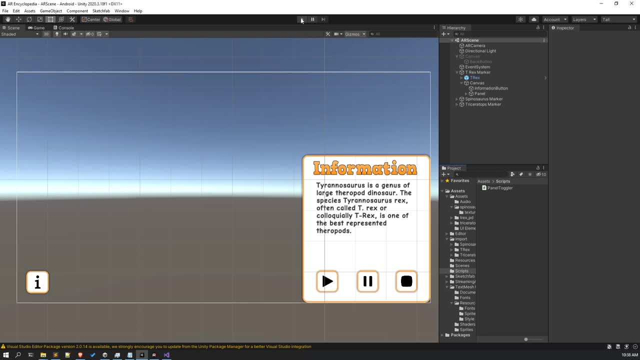 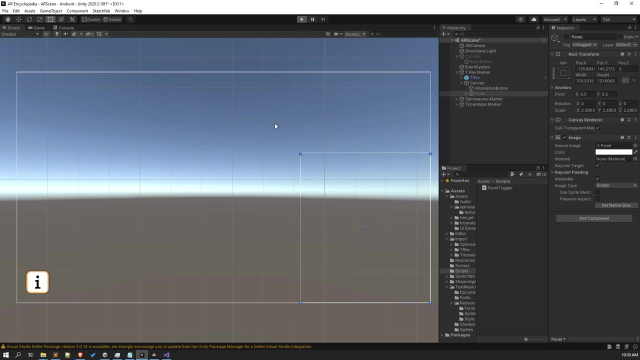 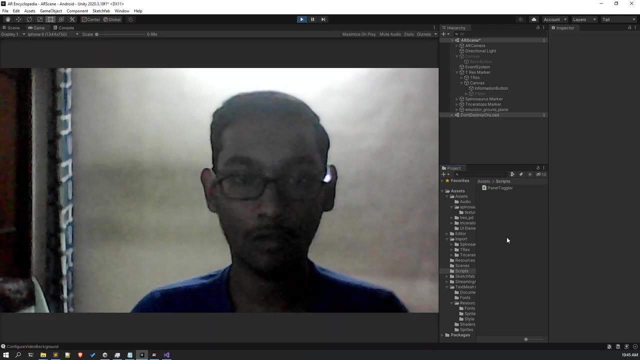 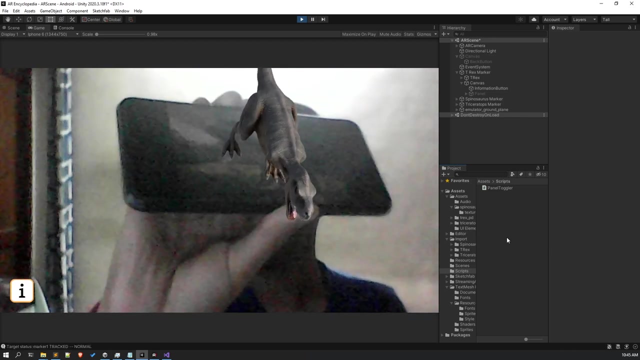 alright, now to test the if, to see if this is working. alright, disable this panel and let's see if you know if this whole thing is working or not. alright, so let's see if everything is working fine or not. okay, so? nope, this is not the one. which one was it? 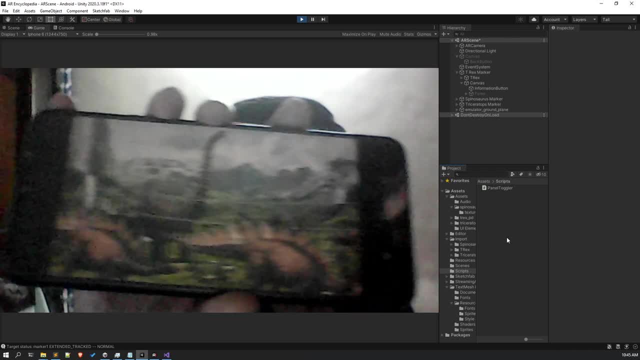 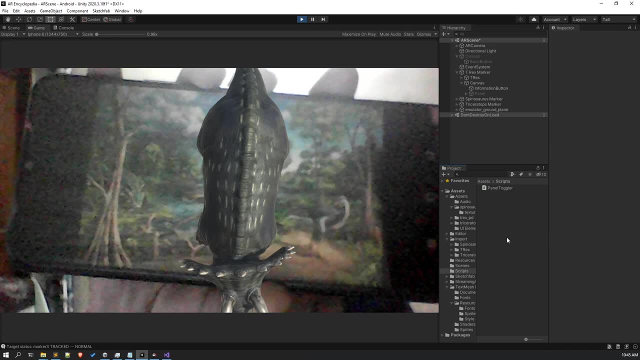 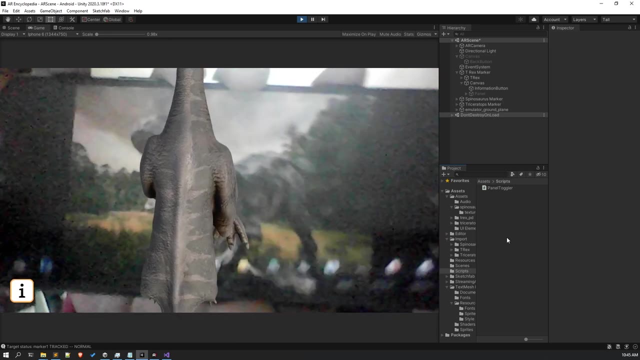 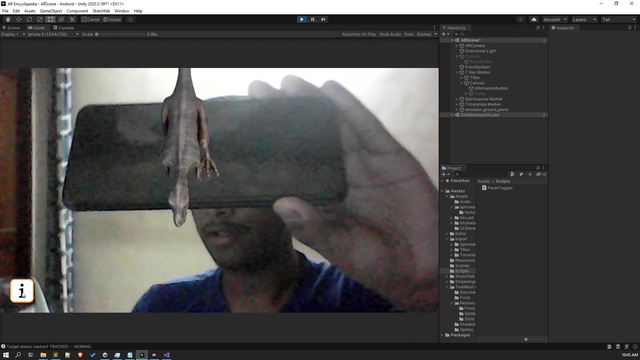 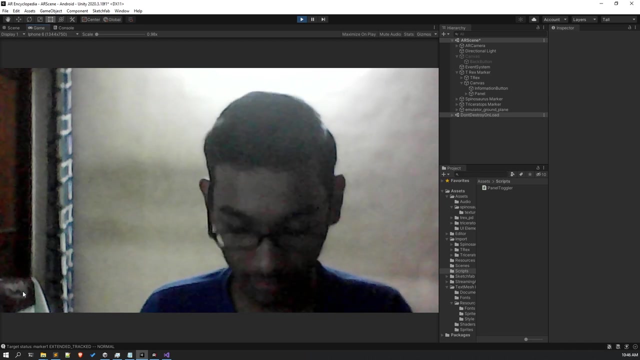 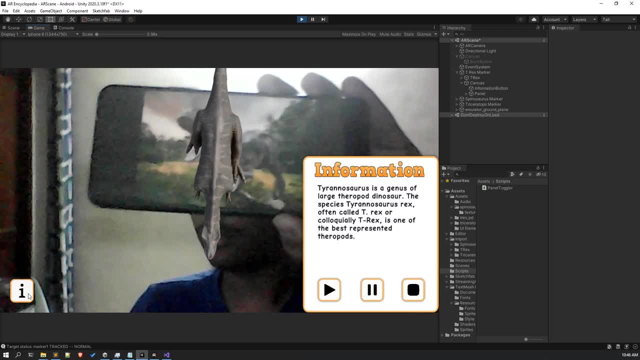 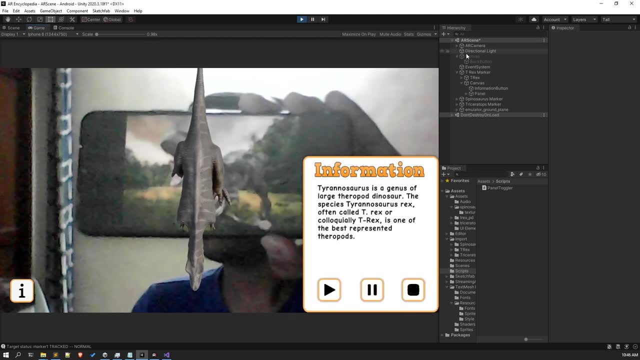 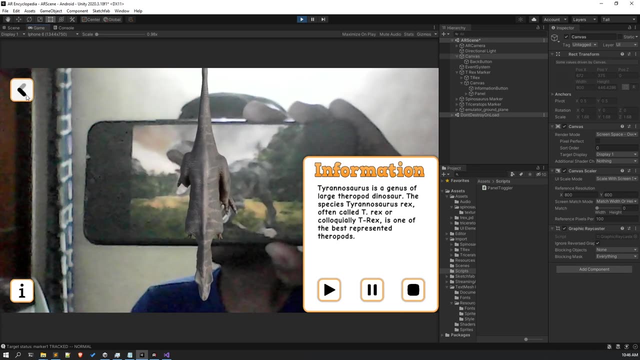 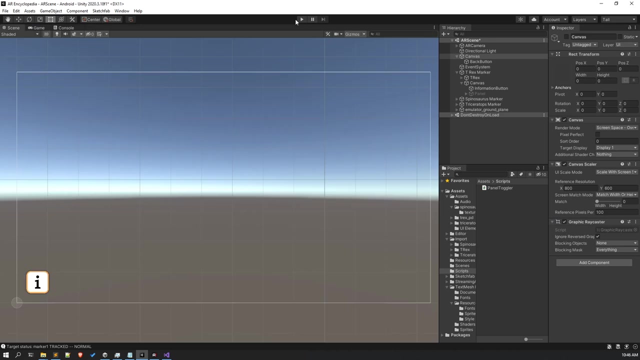 off by itself. alright, okay, cool. so now see, our information button is working pretty fine, all right. and let's see if our main canvas is also okay. so our main canvas is. the button of main canvas is also being clicked, so everything's working fine, all right. so now. now, what we have to do is we have to add the audio. 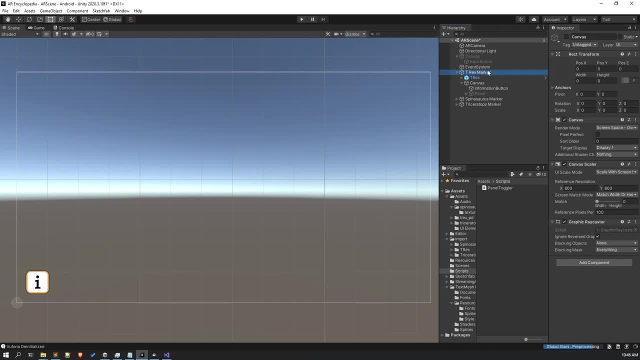 functionality right now. to do that, go to your t-rex marker. create an empty object. name the empty object as t-rex audio. all right, of course this is not the audio of you know, a t-rex, it is the explanation of who he is. right. and now in the t-rex audio game object, add an audio source. 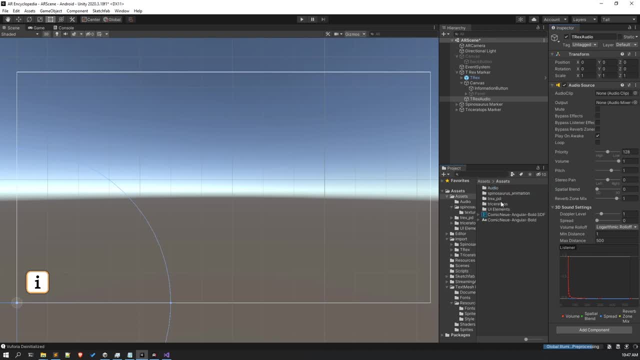 right in the audio source. what you have to do is go to assets. all right, where have i saved audio? yeah, yeah, i got it. so now, in the t-rex audio, add this t-rex description audio in here. all right, and remove this play on awake now, as we have our t-rex audio in here now. what i want you to do is: 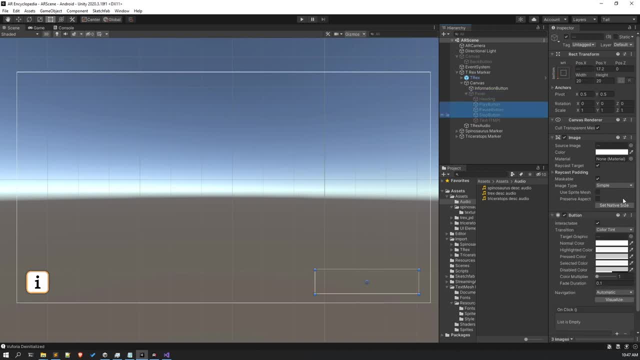 go in here, select the three buttons. click in here means the plus icon, drag and drop this. no, drag and drop this particular audio game object and in the audio source, select the play option. all right, now all the three buttons have the play option. now we have to change one by one. all right, i do this. 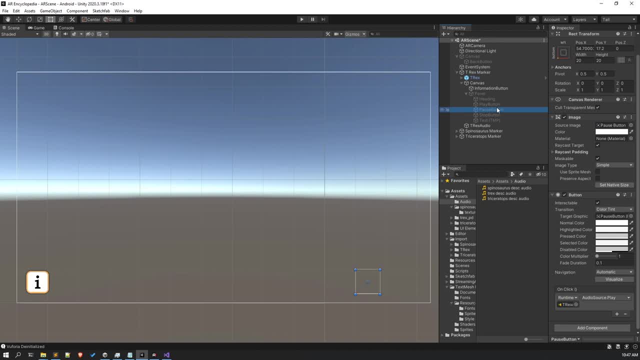 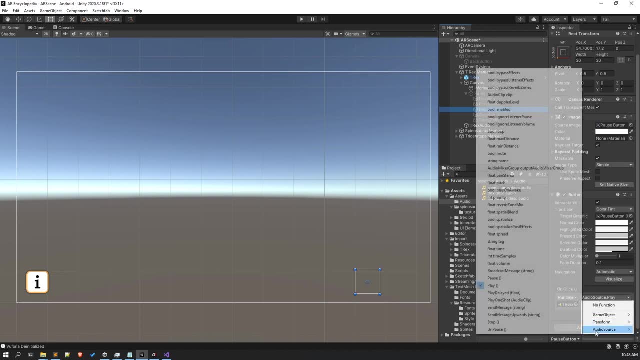 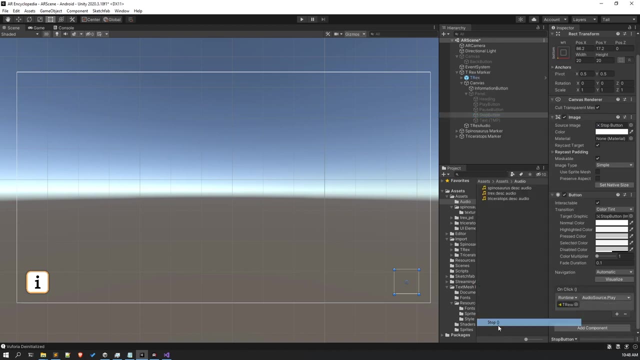 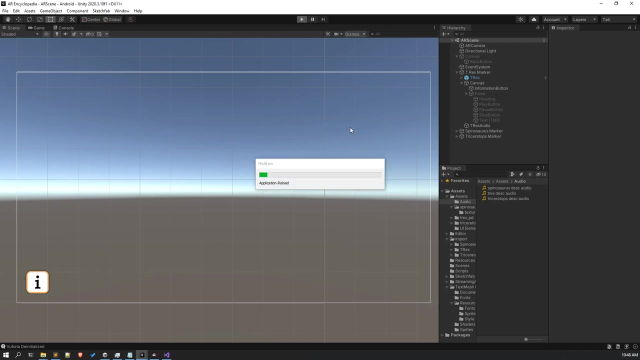 because it it is more faster than the usual, like just selecting one button and adding them one by one. it's much faster now. in the pause button, go to audio source and select the pause, and in the stop button, go to audio source and select the stop. all right, now let's play. play it again and let's see if everything's working fine. 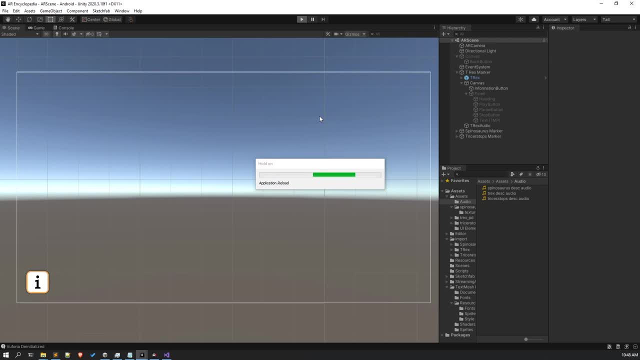 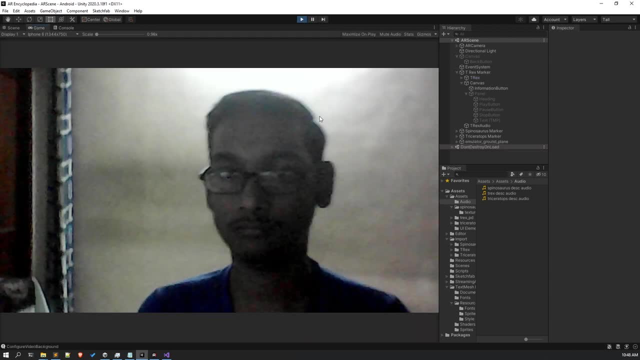 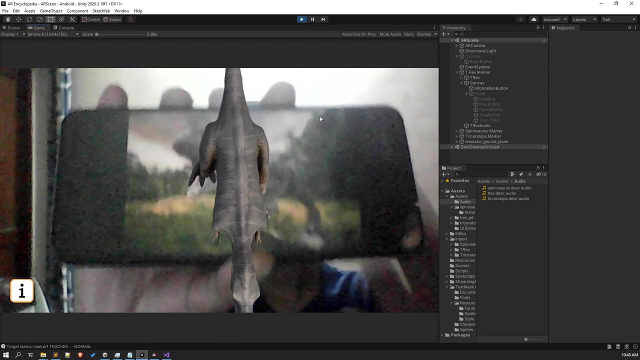 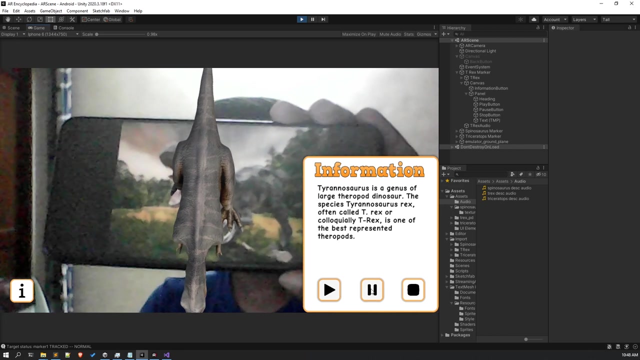 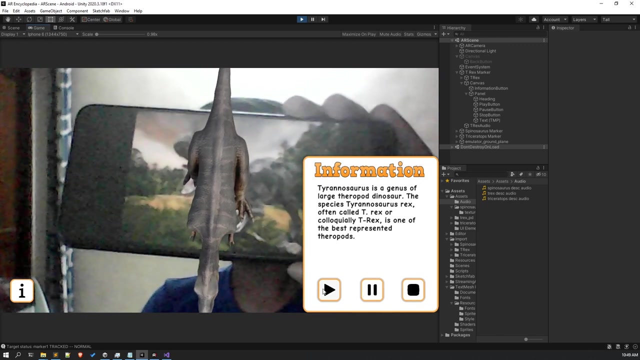 or not. all right, just give it a few seconds and we'll be good to go. all right, so let's see, okay, okay, so all right, let's see. all right, let's see, see, the pause is also working. let's play. all right. so the pause play and stop is working. let's again play. 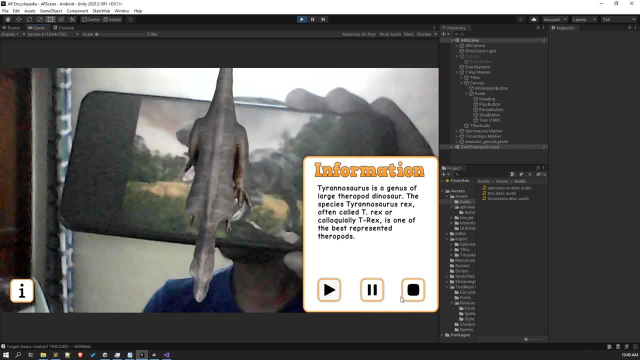 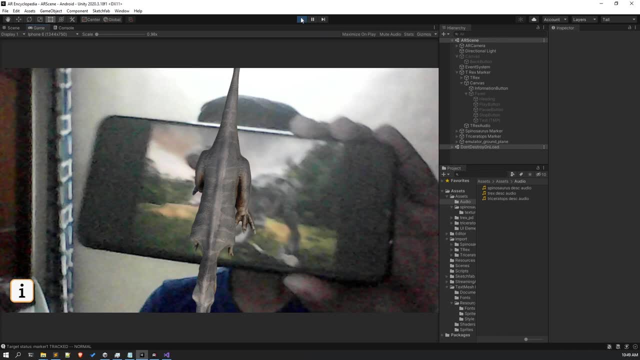 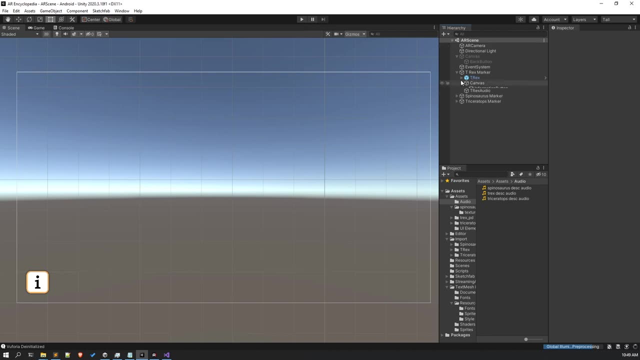 all right. so the pause play and stop is working. let's again play. yeah, pause play, stop. see, this is working pretty fine. so our first marker is totally ready. now we have to do the same thing. now. we have to do the same thing for every marker. so i'm just going to use our red arrow to enter the program. 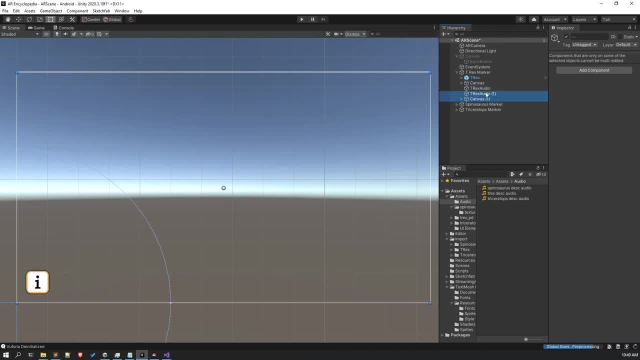 know, duplicate these two game object right and drag and drop it under the Spinosaurus. all right, I'm going to name it s audio. all right, it's too much to write its whole name and this, this canvas. let's put it up in there in the 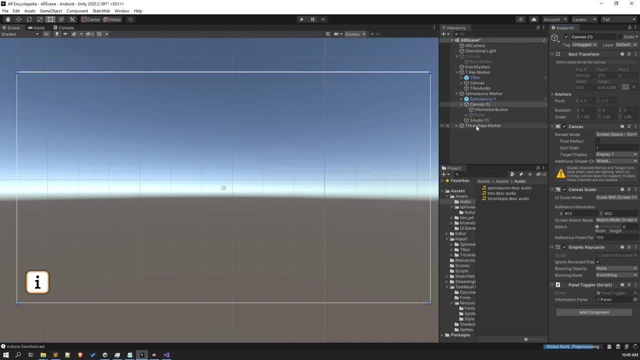 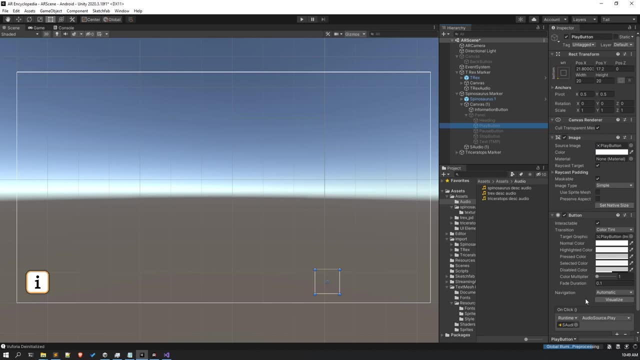 canvas: all right, here's the panel. drag and drop it in here and in the buttons. all right, we already have the s audio. all right means the this audio source, so we don't have to do anything else. also enable this particular button, you know. and in the panel: all right, in the panel. in the text, we have to change the text. 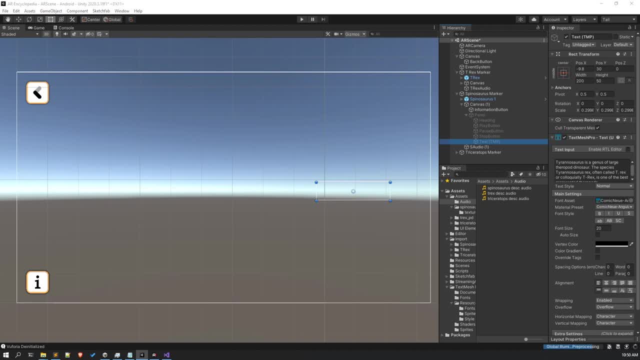 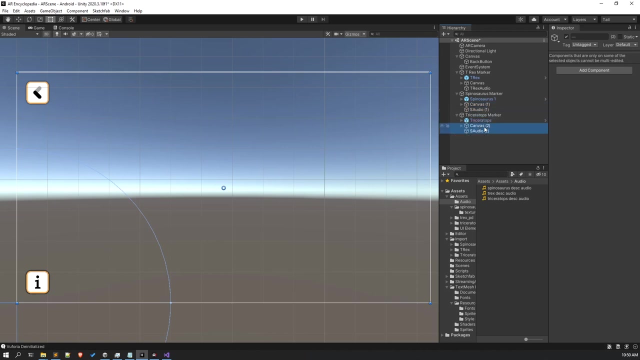 all right in the text. I have got one text. just let me bring it up in here and let's see, let's enable this particular panel and let's see how it looks. oh, it looks really good, right, doesn't it? and again, duplicate it, all right, and drag and drop into T means Tyrannosaurus Rex. all right and not. 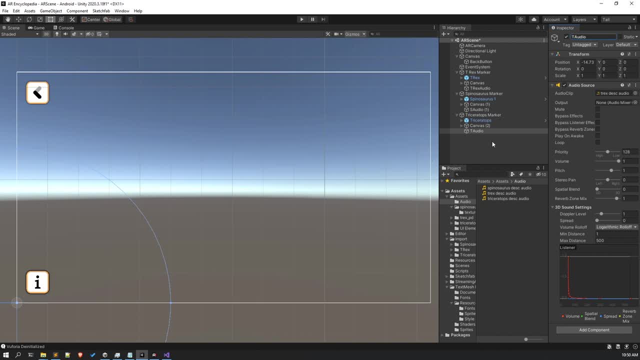 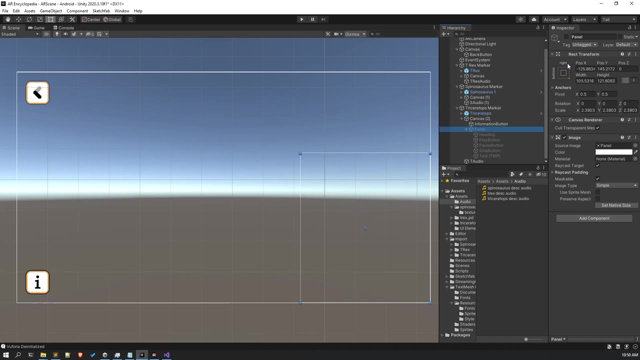 sorry, Triceratops, not Tyrannosaurus Rex. and in the canvas: select the panel. all right, and inside of the panel, let's see if the buttons has the right audio or not. yeah, they do now in the text. all right, enable the panel and we. 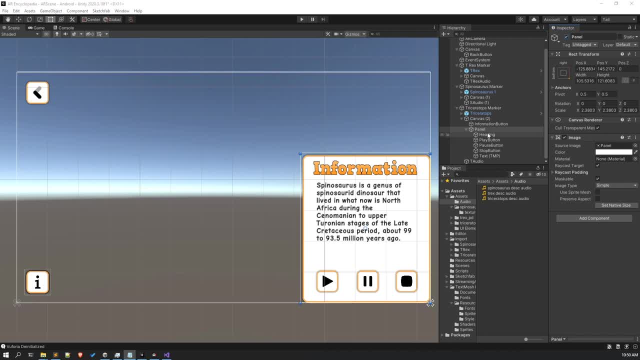 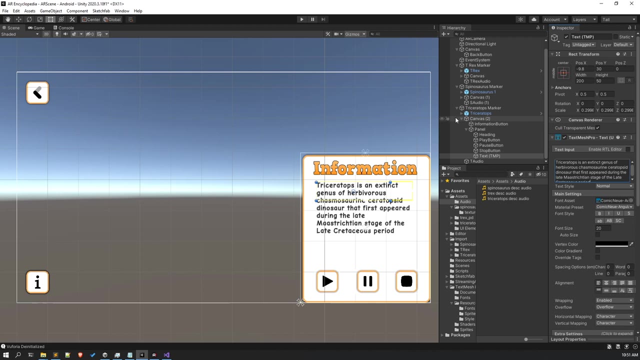 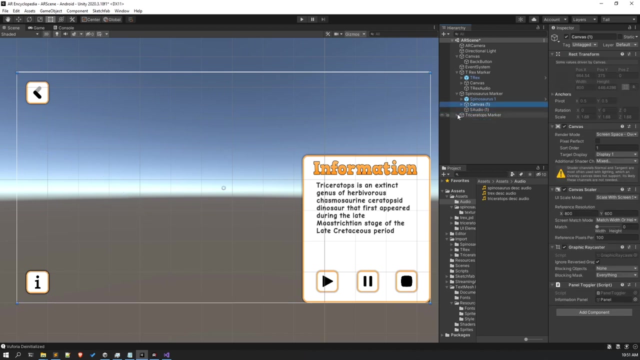 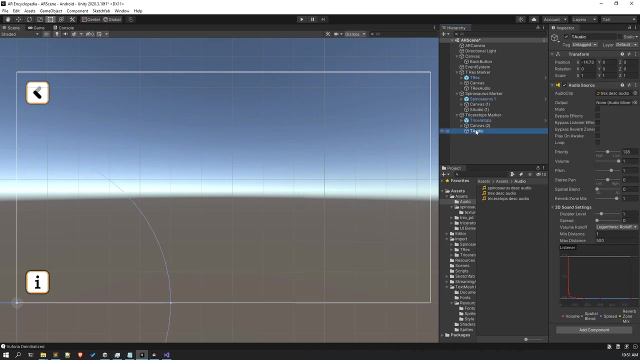 are going to get the actual text. all right, where is the text here? got it now, simply go in there and put it in here, right? okay, cool, now I am going to change the text. all right, just give a few second. all right now. disable this particular panel right in here. all right, so now in the T audio. 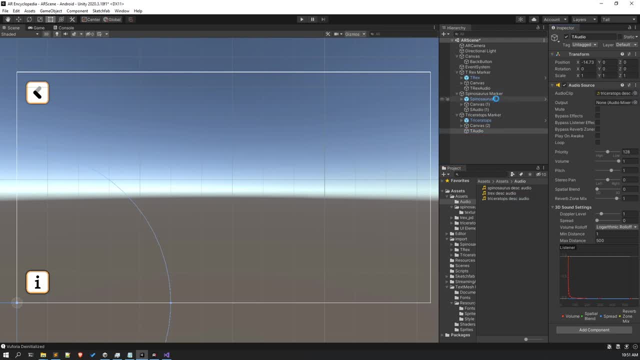 change the audio to Triceratops audio, all right, and in the spinner, Soros Rex audio. change it to Spinosaurus Rex. sorry, Spinosaurus not Rex, not Rick. all right, I'm really sorry. dinosaurs and dinosaur enthusiasts are going to kill me, I guess. so yeah, let's try this out and let's see if. 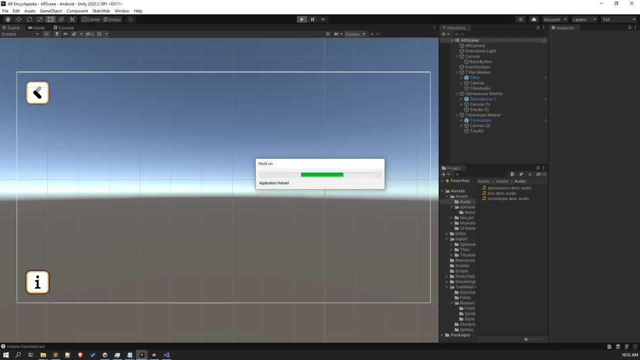 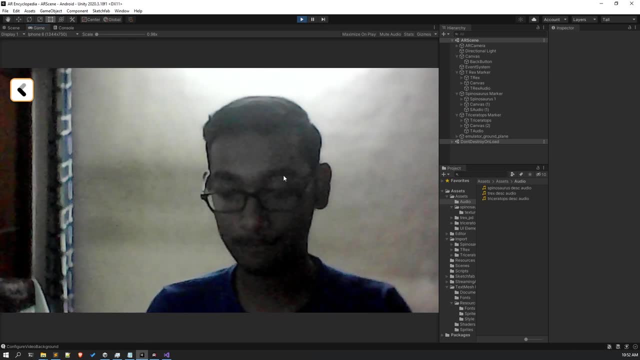 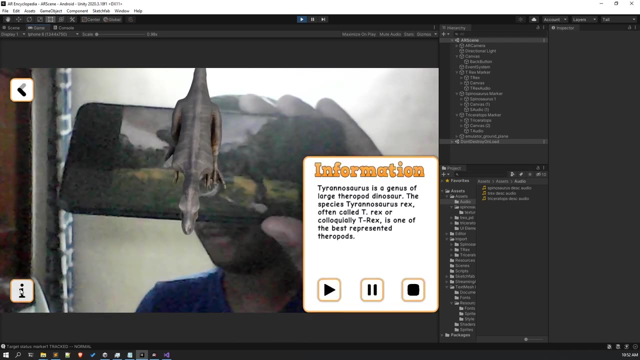 everything's working or not all right. so give it a few seconds to run, all right? so let's see. so there's our first one. all right, this is our special Dinosaur, that is T-Rex. all right, my favorite. so let's see if audio or is all right. so audio, and. 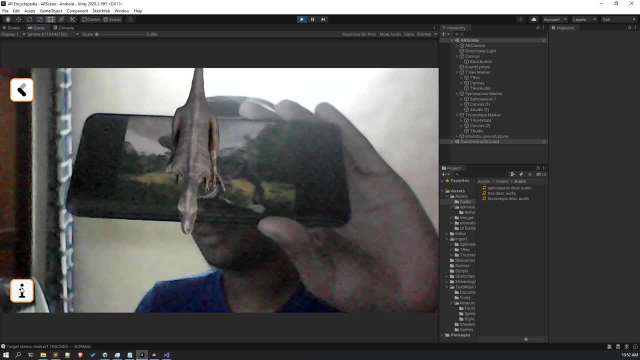 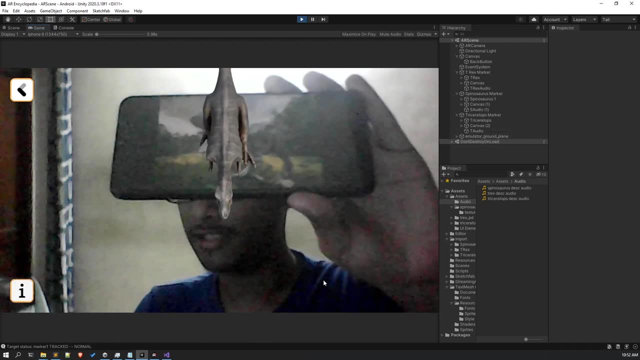 everything. isirenasoras is a genus of perfectly working, I know. so, all right, these species, Tyrannosaurus Rex, often call T-Rex or call: if Christольш is one of the best, let's actually, you know, stop it all right, and if you, let's say a. 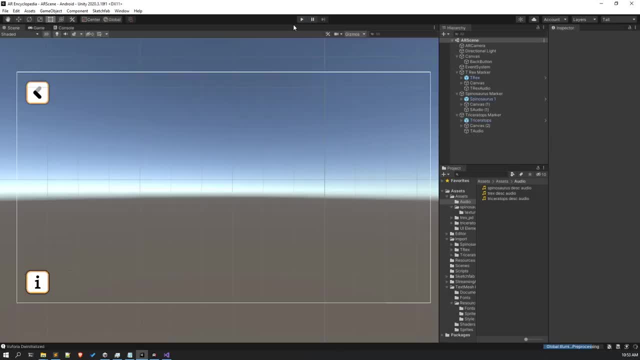 uh, let's say, let's do one thing. let's say if, uh, if, if you want to stop the audio, all right. if you want to stop or pause the audio after the marker is, you know, removed, you can simply do that. so go to t-rex marker. uh, in the on target lost, click on add icon um, get this audio, all right. audio source. 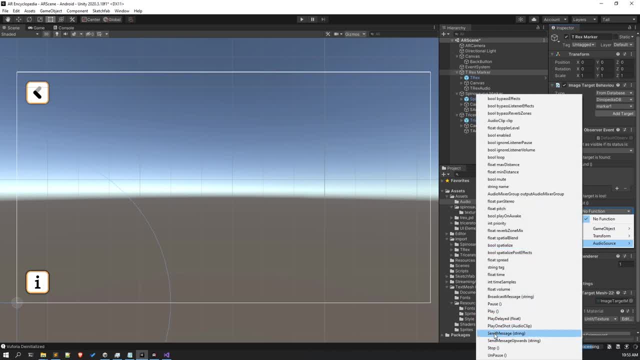 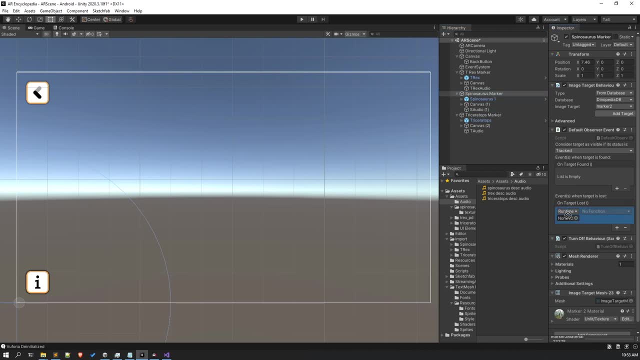 and, uh, i let's say i want to, you know, stop the audio, all right, let's stop the audio, all right. and again, in the spinosaurus marker, do the same thing. all right, do the same thing, and you can do whatever you want. already, when you can pause the audio and even if you want you, 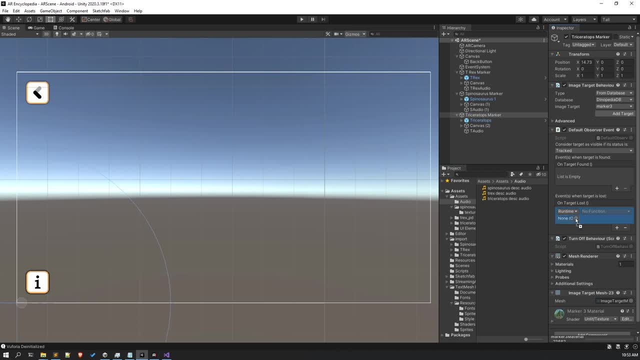 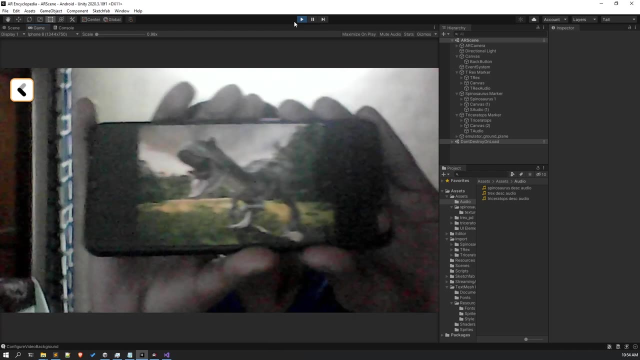 can start playing the audio when the marker is tracked. you know, it's totally up to you, but this is what i'm doing now. yeah, we are good to go right. all righty, let's see, all right. okay, so let's check if everything is playing or not. 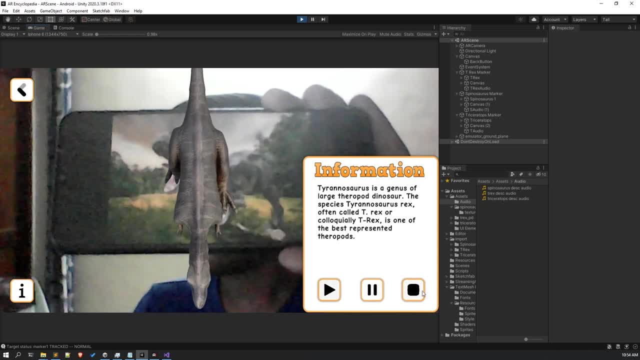 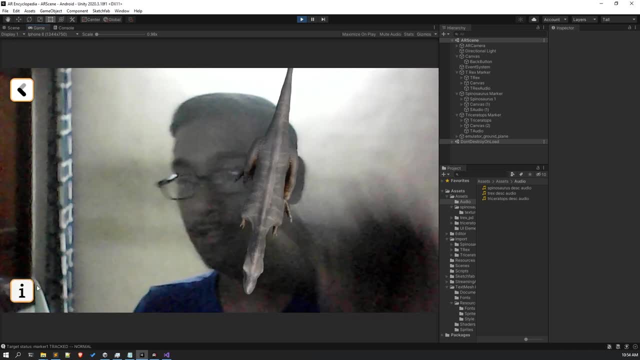 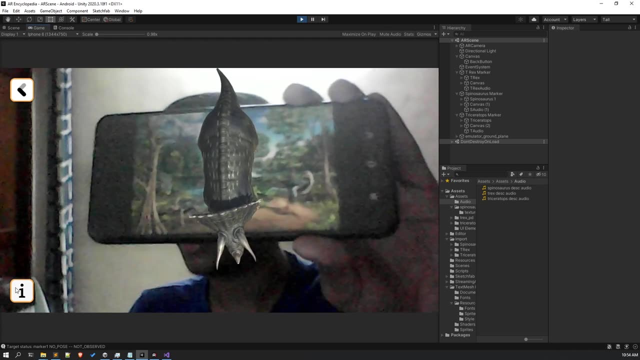 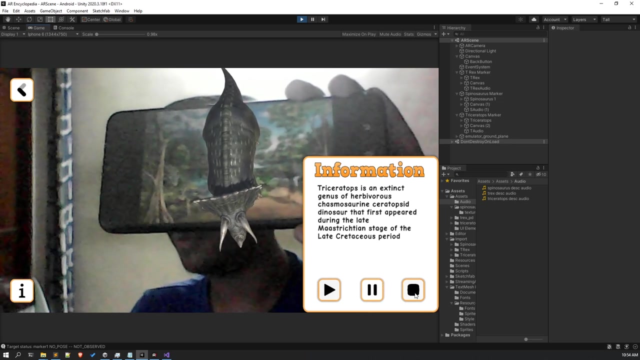 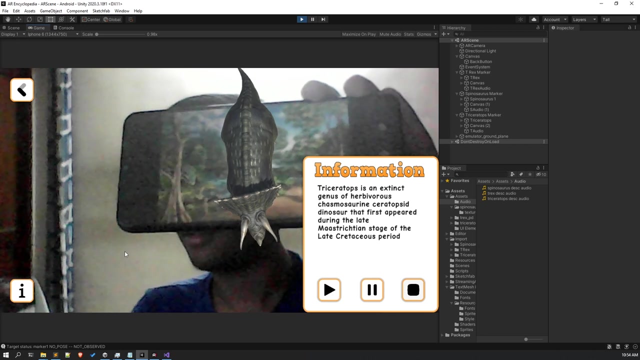 cool, so it's working. now let's, let's select this one. all right, okay? triceratops is an extinct genus of herbivorous. all right, so play pause is also working. stop is also working. triceratops is an extinct genus of triceratops, isn't it all right? good, now let's. triceratops is an extinct genus of herbivorous. 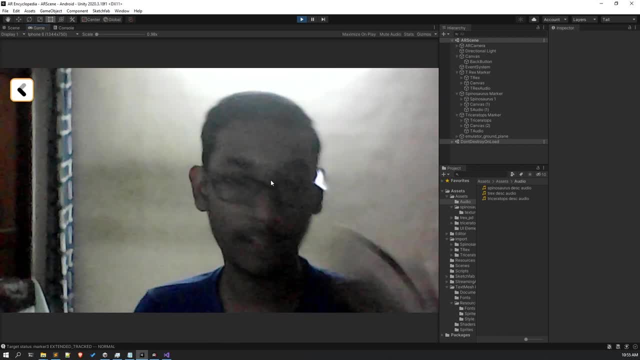 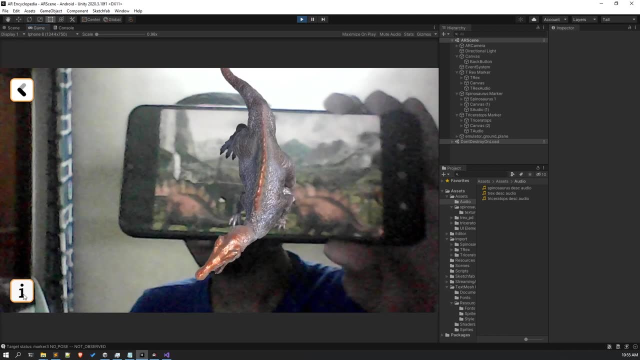 chat, all right. so this one's also working perfectly fine. and let's test this one: our triceratops- sorry, not the triceratops. yeah, spinosaurus. all right, let's play. spinosaurus is a genus of spinosaurus. all right, it's called spinosaurus. 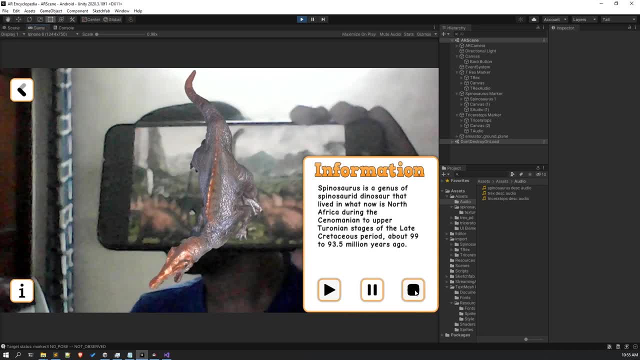 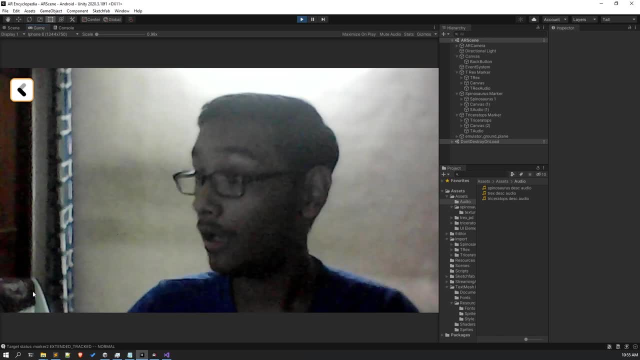 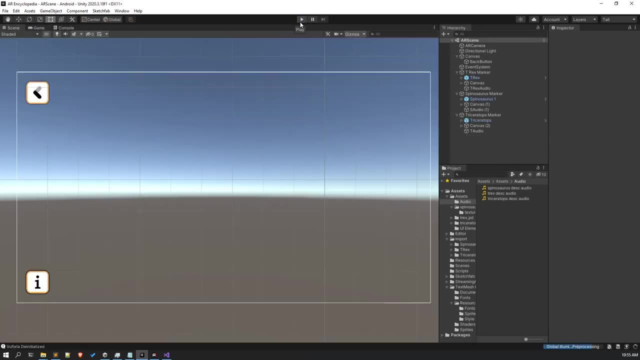 all right, play, play, pause and stop is perfectly working. let's see this one. all right, so our dinosaurs dinosaur encyclopedia is working perfectly fine. now the thing that is left is to code. the back button right means the scene changing script. all right, so what i'm going to do is go to script. all right, uh, first of all. oh yeah, before we go to. 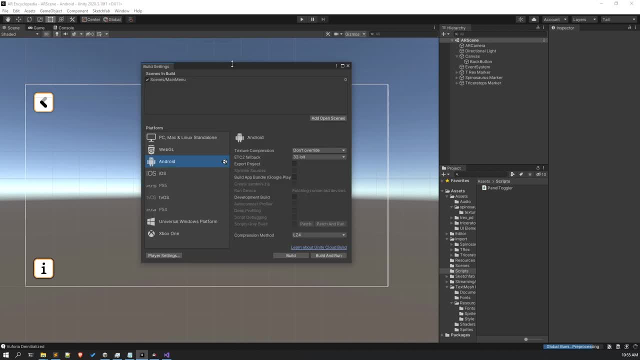 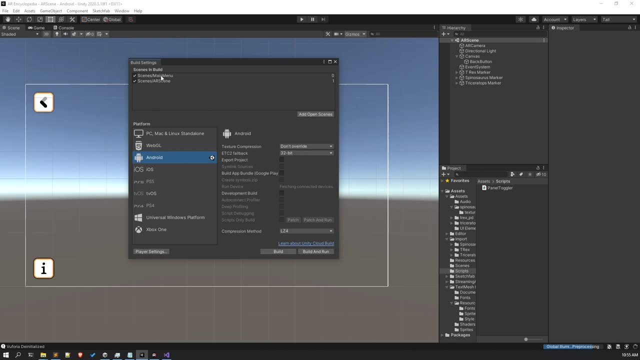 into the script, go to, uh, build settings, all right, and add this ar scene in here. so currently i'm on this ar scene, so i'm just going to click on add open scenes and always remember to keep the main menu on top of every other scene you are putting in the build settings, all right. so make sure you. 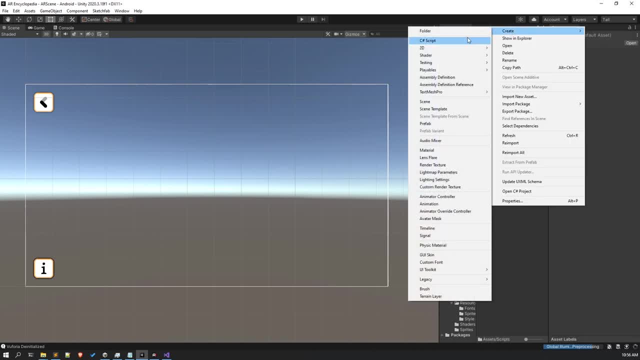 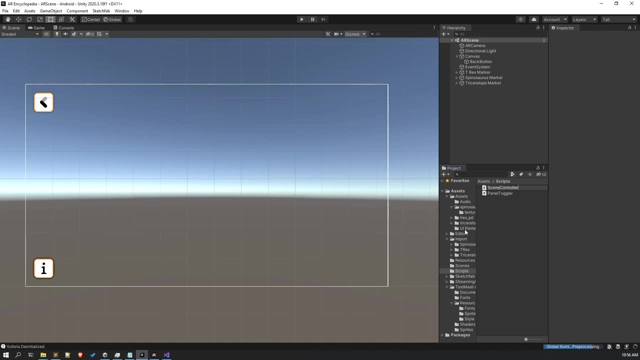 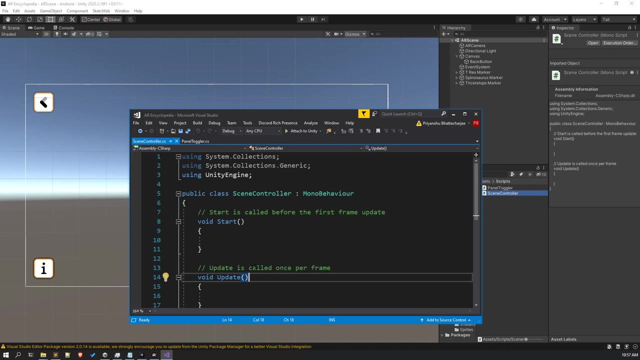 do that now. uh, in the in the scripts, create another script called uh c sharp script called scene uh controller. all right, all right, so now let's code our scene controller. all right, that, uh, that that is. it will be controlling our scene. all right, that means would be we have to navigate through the scenes. 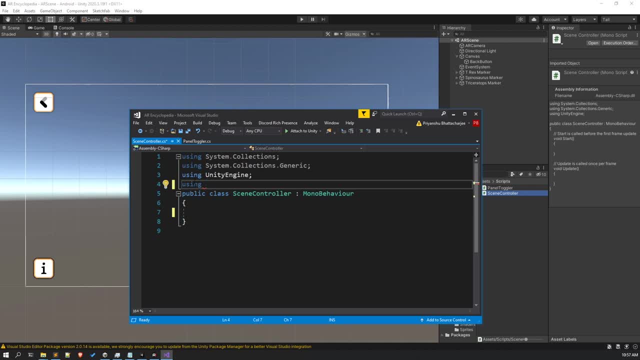 right, so we need that. so what we're going to do is, uh, using unity engine, we have to include that particular library scene management. all right, so here you go. right now, what we have to do is we have to create three functions. first of all, the function would be public void. we are going to call it main menu. this function would be: 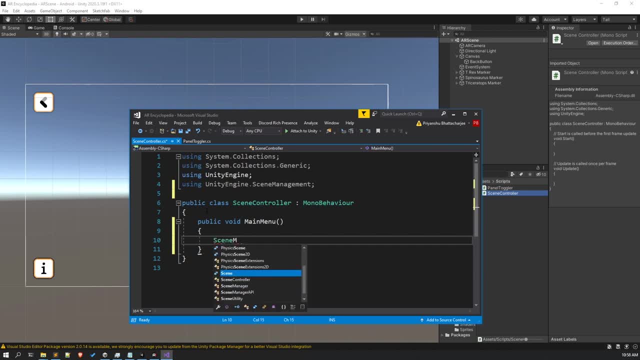 loading the main menu. all right, that is scene manager. dot load scene and give give uh you know. give this uh scene manager and give uh you know, give this uh scene manager and give uh you know in a name. that is main menu. all right. so after you give the scene a name, you have to create. 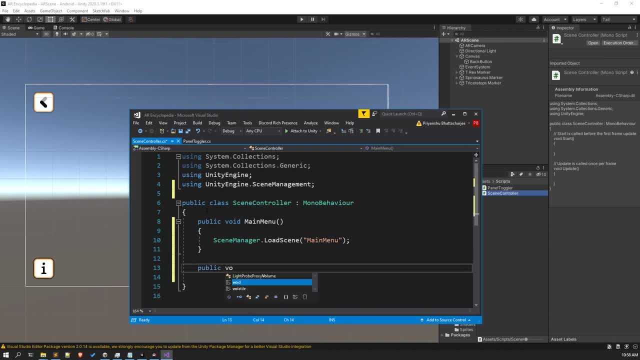 another function, all right. public void. all right, in the public void function, you have to create another. uh, sorry, so now, all right, we have to create another function. all right, that would be for loading our ar scene, right? so public void, let's name it ar scene. right, and again same. 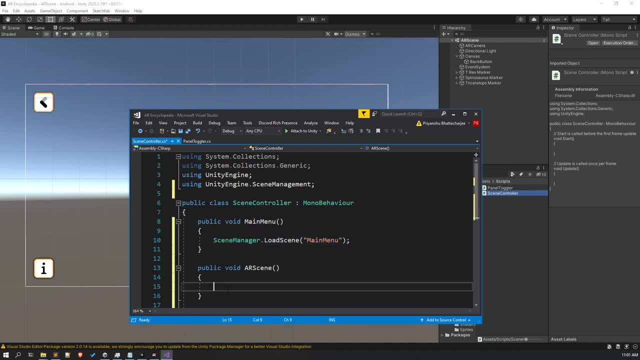 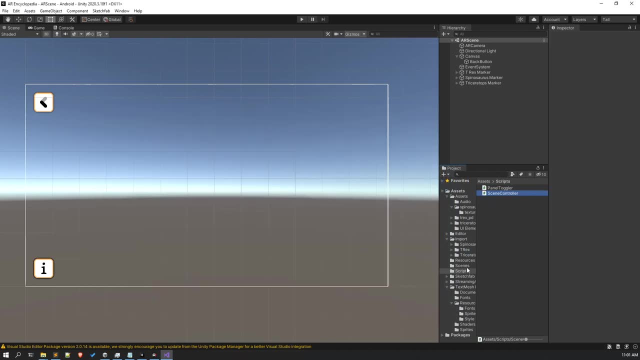 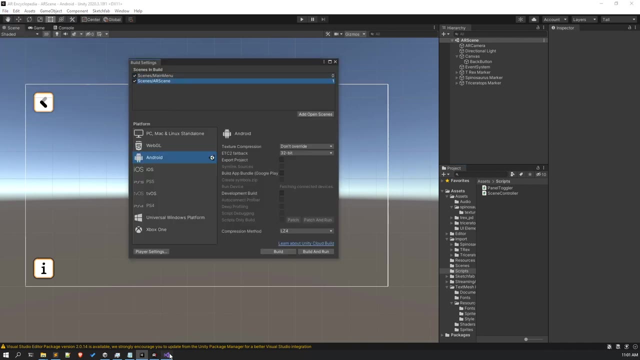 write the same line in here, that is, scene manager dot load scene. all right, and now in here you have to provide AR scene name. see, these are the names. all right, these are the names of the scenes we have. all right, these are the names of the scenes we have. that is the main menu and the AR scene. all right, so make sure to put this. 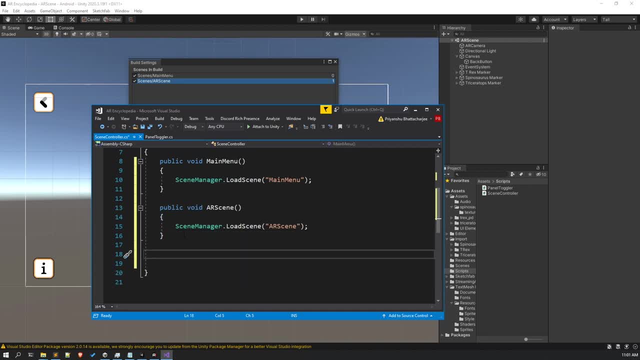 scene name right in here, all right, so make sure to do that. and another is to quit all public void: quit app, quit app. all right now. scene manager dot load scene. and sorry, not loads in what i'm doing. i'm very sorry, okay, just wait. oh yeah, application dot quit, all right so 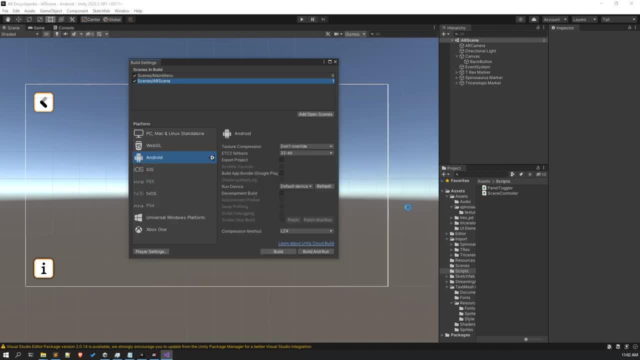 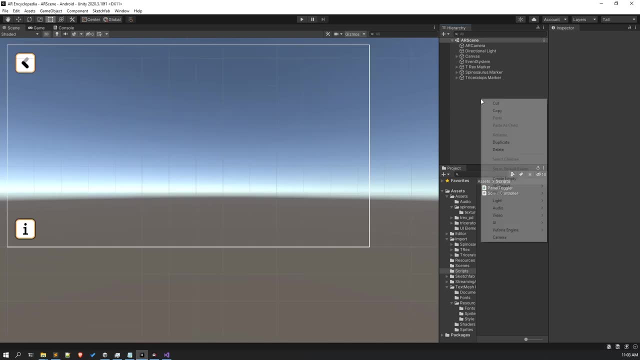 that would help our application to quit. all right, and let's compile the script. so now our script is compiled. what you have to do is create an empty game object, reset its position- all right- and name this empty game object as scene controller. all right, because this empty. 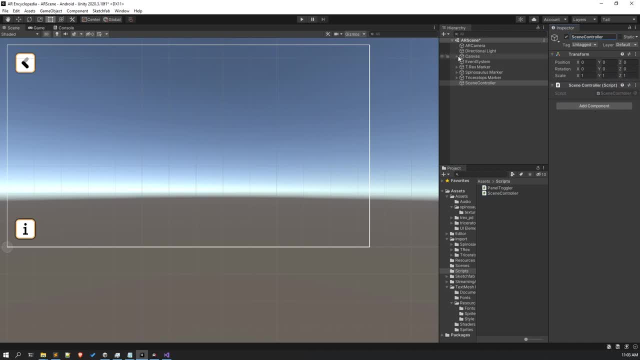 we'll be attaching our scene controller script to this empty game object. now what you have to do is go to canvas, click on the back button in the back button, click on on click. click on the plus icon in the scene. put the scene controller down there and click on scene controller. 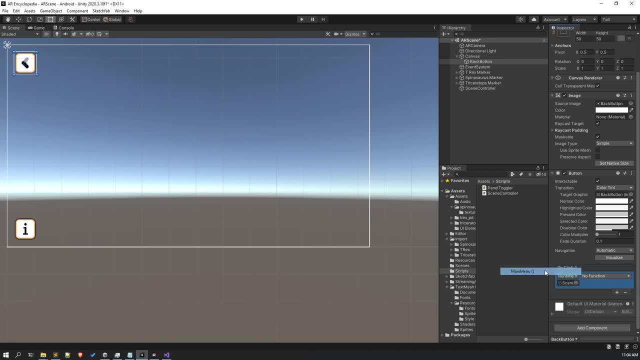 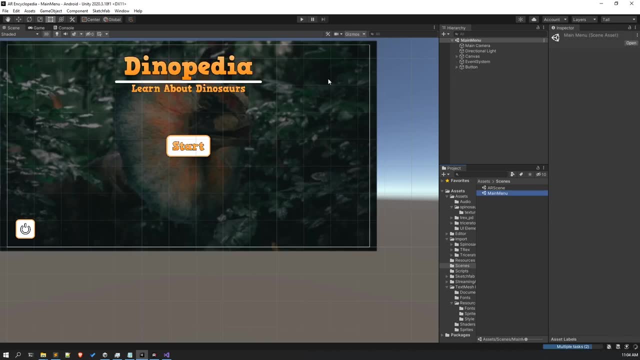 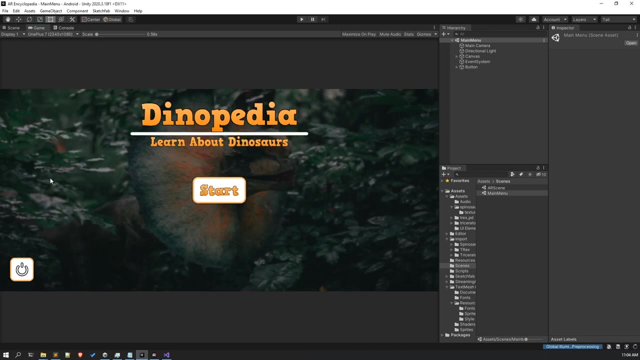 and after clicking the back scene it should load the main menu, all right. now we have to do the same thing with our main menu, all right, and in the meantime we also have to check if everything's responsive or not right. so let's check it, all right, really, really great, yeah, everything's. 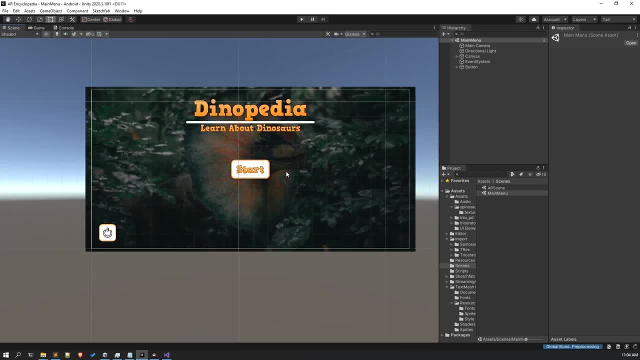 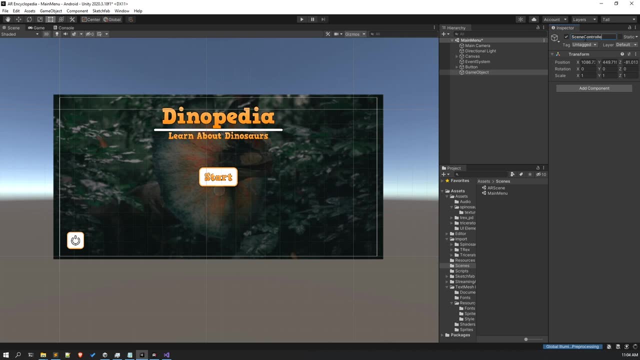 totally fine. right now, again in here, create an empty home object called scene controller, reset its transform. uh, add the you know scene controller script in here. in here you'll be finding: uh okay, this, i forgot to rename this button. let's me rename it. square button, all right. 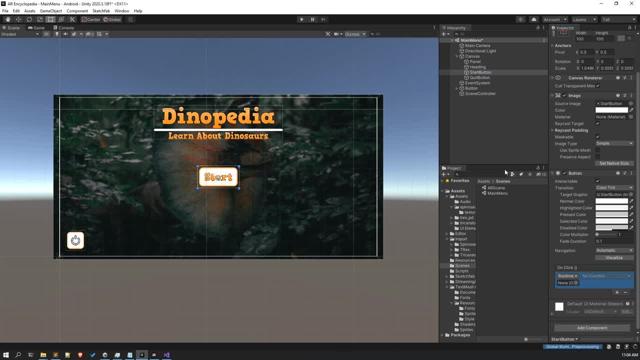 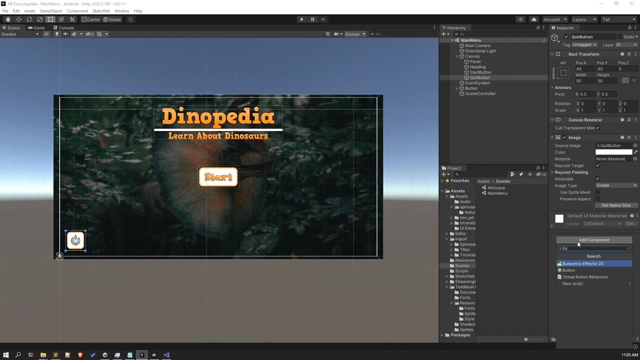 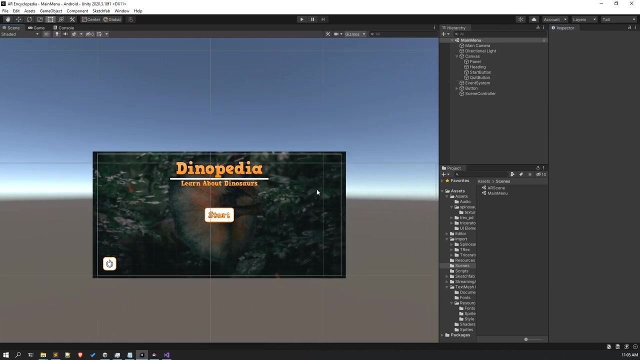 now in the start button. all right, we have an on click function. simply add it in there- scene controller- and click on this arc, because it would be loading our arc. and again, i also forgot to add the a button component to this quit button. click on the plus sign scene controller, scene controller. then again quit app. all right, so now everything's. 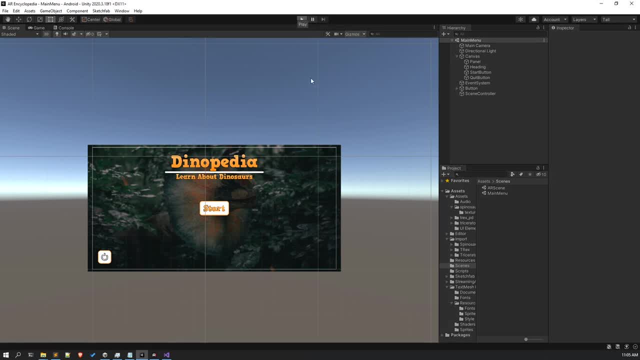 done. now let's play this scene and let's see if everything's working fine or not. all right, and if everything works fine, we are done with our application right, and you can actually launch this application on play store if you want. all right. so, uh, and actually before launching, i would 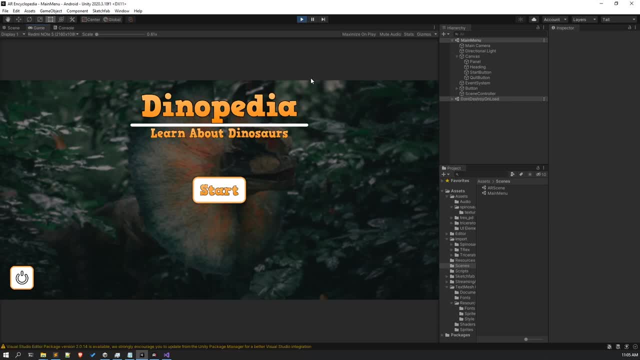 suggest you to add some more information. all right, now let me tell you one thing: this, uh, this quit button is working. all right, this quit button is perfectly working fine, but, uh, you can't see nothing is happening because currently we are not on our phones. so when you, you will be in your phone and pressing this quit button. 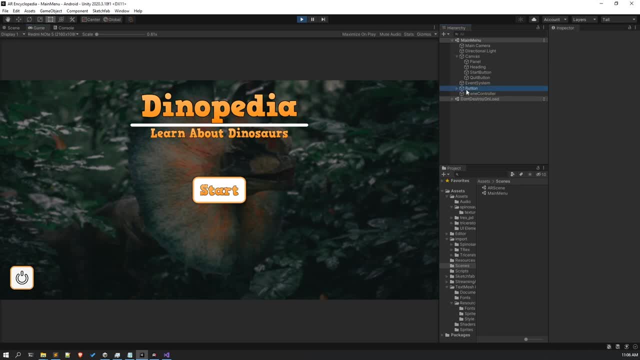 it would be working perfectly fine. all right, and i'm not sure why there's uh. here is one button i have to check. all right, so everything's uh. first of all, let me check if the function is right. right, yeah, quit. the function is right, so quit button will work perfectly fine. now click on the start. 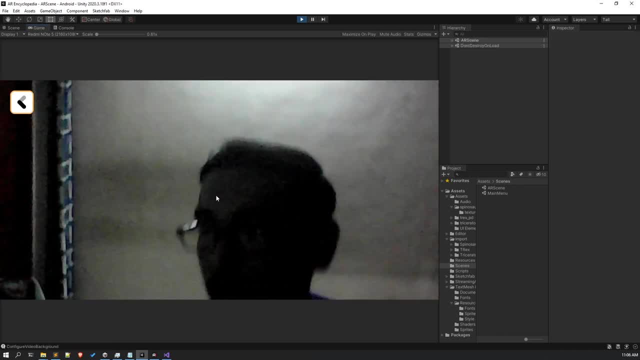 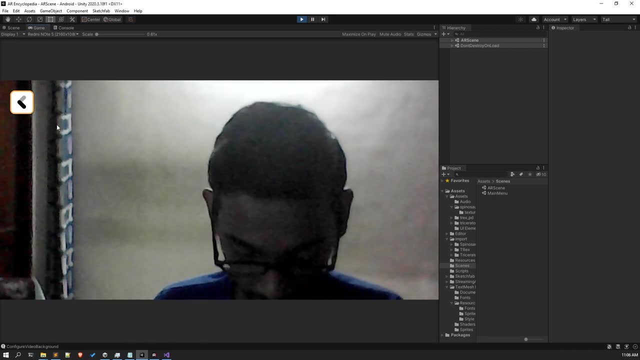 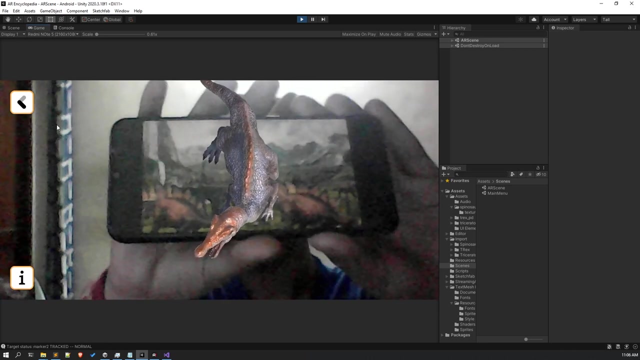 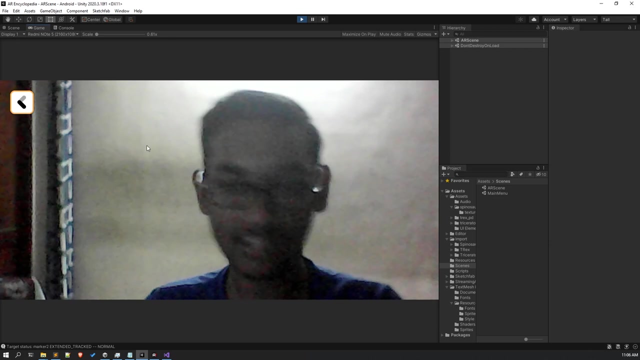 button. all right, and let's let's see it load. all right, cool. now let's try out our markers. just let me open the markers. all right, all right, okay, cool. so now everything's you know working perfectly fine is a genus of: okay, cool, so just like this, every other marker will work and let's click on the back button. yeah, cool so. 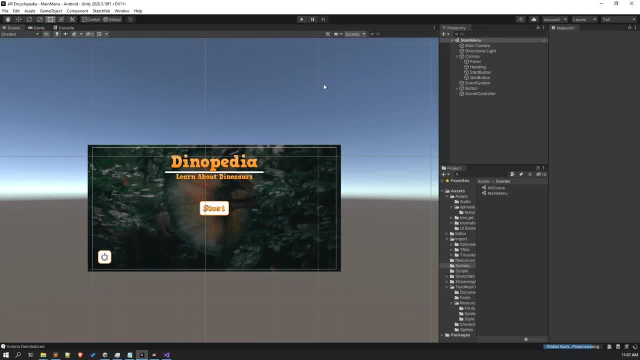 we are able to navigate through our scenes right, so this is working perfectly fine. and which button is this one? all right. also, it's- uh, not inside the canvas, so it's not necessary, so i guess i have added it by mistake. so we are done with this project and hopefully you have. 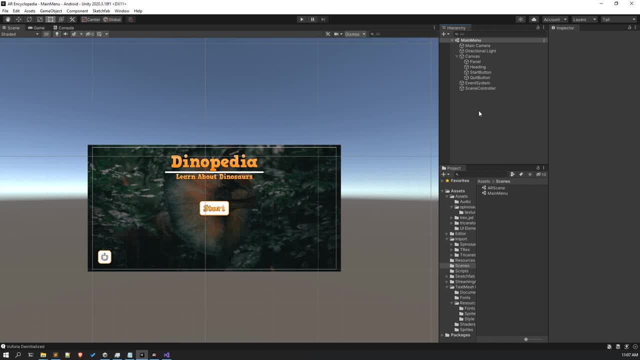 learned uh how to create your own ar books, all right, how to create your own ar encyclopedias, and, if you want, you can launch this application after developing on play store. all right, and also add uh ads to earn money. so yeah, for uh this lecture. this is it, and 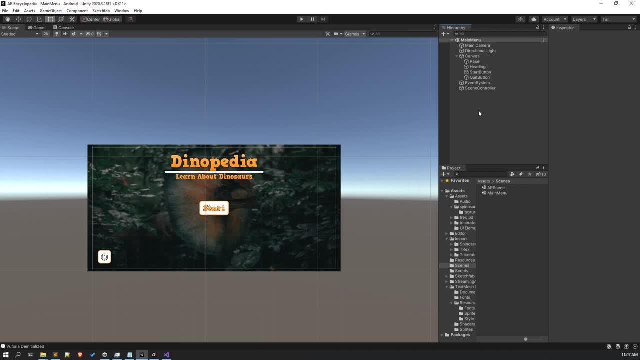 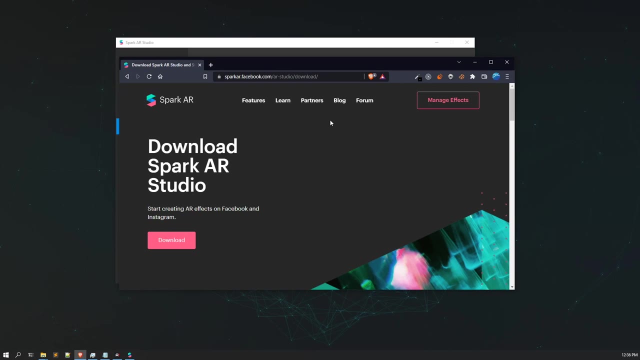 best of luck for, and also create more projects like this. all right, and in the next module of this course we are going to explore spark ar. all right, so yeah, stay tuned. in this lecture we are going to learn about spark ar studio. we'll be getting an overview of the 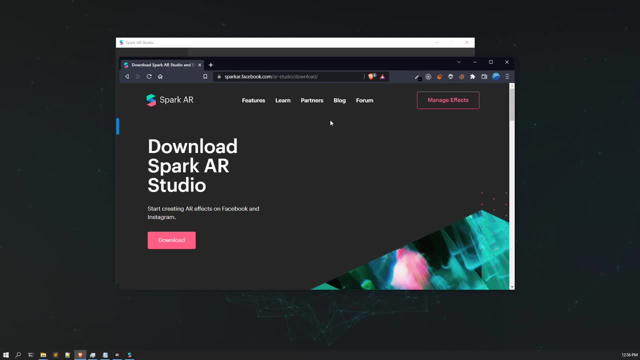 interface. we'll be learning about the spark ar ecosystem, all right, and we'll be doing a lot more things, all right, but before using spark ar studio, you need to download it. so this is the link. all right, spark arfacebookcom. slash ar studio. slash download. all right, so you just need to click on. 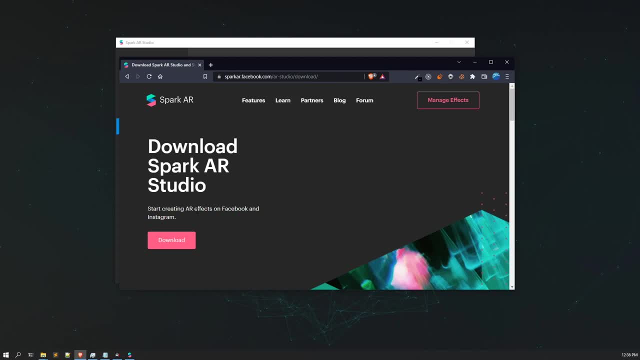 the download, the experience page. the system i just created this is a multi-tool kit and it's all for one person, and the installer would be, uh, downloaded on your system and the process is pretty simple. you just need to install it. all right, it's like any other installation process, all right. so from these, this: 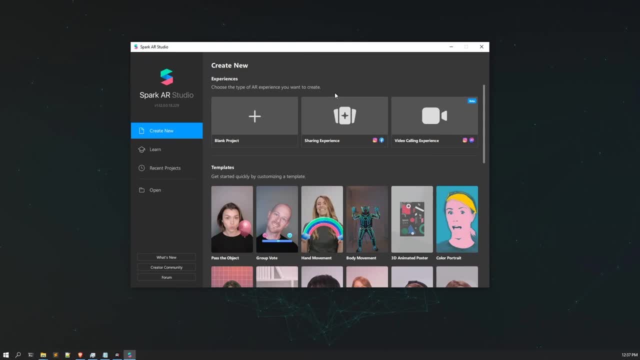 website. you have to download it. all right now. here is the interface. all right, this is a dashboard. all right. now, with this dashboard, we actually manage our projects within uh spark ar. all right, so, first of all, this is the basic interface, the templates. all right, this is the first area that you are going to see. 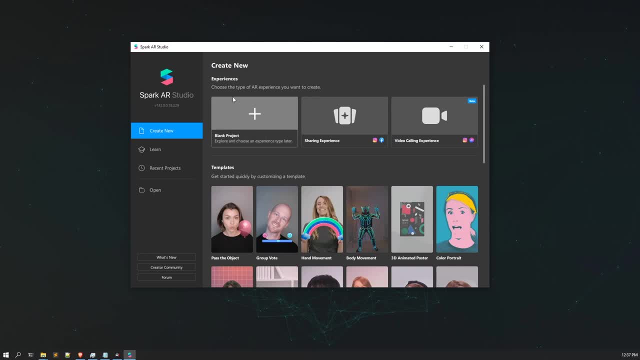 after installing and opening the sparky a studio. here here are three- well, means three, blank templates, all right, that is, oh, one is totally blank, that is blank project. and the sharing experience and video calling experience, all right. and other other than though these three, here are some more. all right, so these are the. 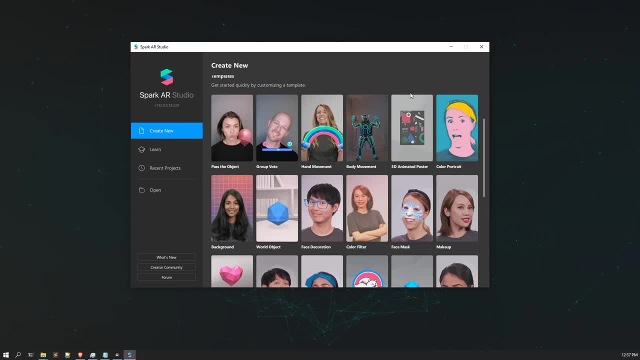 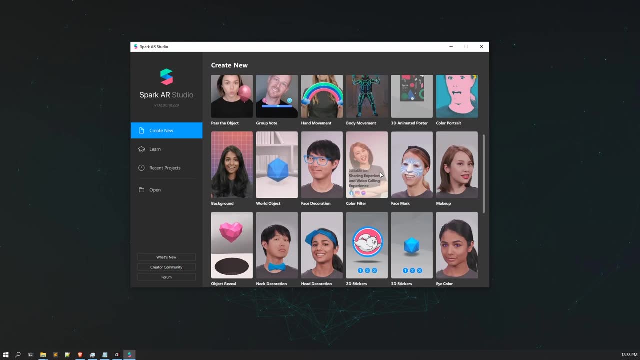 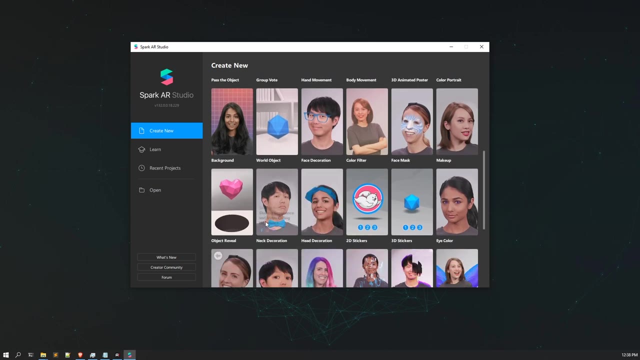 basically templates made by the sparky our team and other creators. all right, so here you can see there are multiple, multiple, multiple templates that you can get this: there is a face decoration, there is face mask, then there is body tracking, then there is neck decoration, then there is head tracking. all right, so 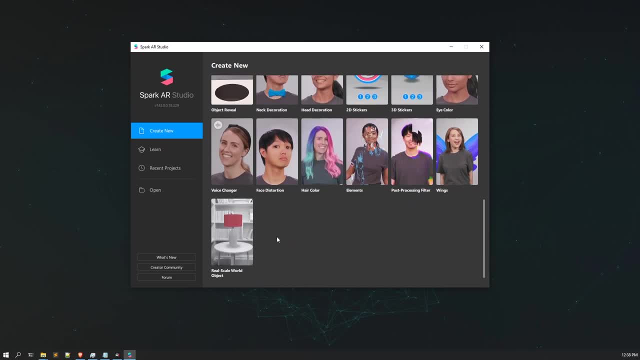 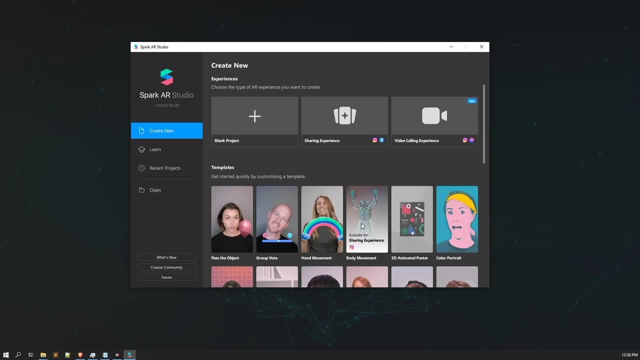 these are the templates that you can explore. all right, there here is a real scale world object tool, that is. that means real world, like real world scanning, markerless scanning. so, uh, you, you can like try to explore all these templates. all right, it would give you a humorous like huge amount of knowledge. all right, 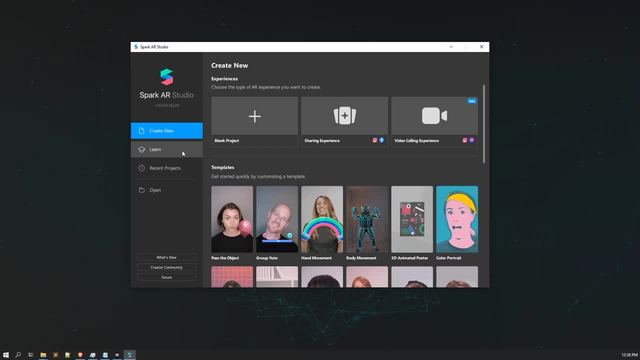 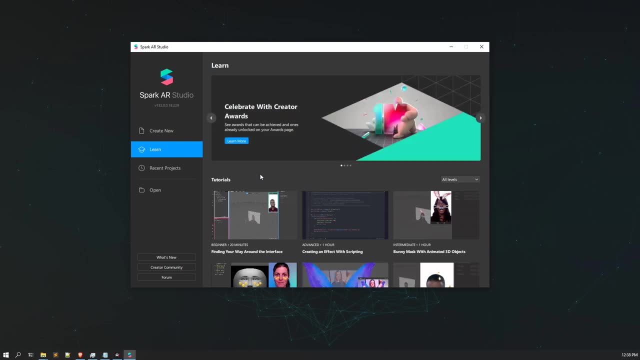 so these are the templates that you can work with now. let's say, uh, after this course, you want to explore, uh, more of spark here? all right, so spark here has their own platform, where they are. there are two to three courses on spark here. that is fundamentals of spark here. then there is 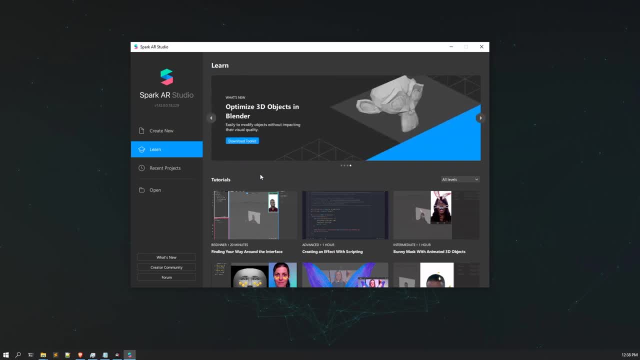 uh, like a totally free means those are totally free, all right then. there is advanced spark here, all right, so you can find it on on the internet. it's by facebook only. it's totally free. you can watch there, all right. and if you want to learn more advanced ar development, all right then. 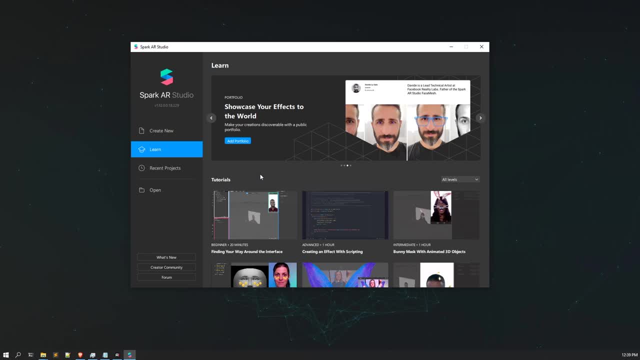 i'm also going to launch one course, all right, uh, it's an. it's called exercise 01- augmented reality for everyone. all right, so it's an augmented reality mastery course. you can get that course. it would be a very low cost course and it would be launching very soon. uh, at my, at my startup. 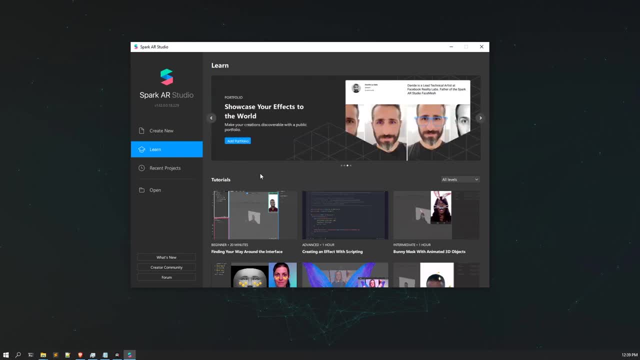 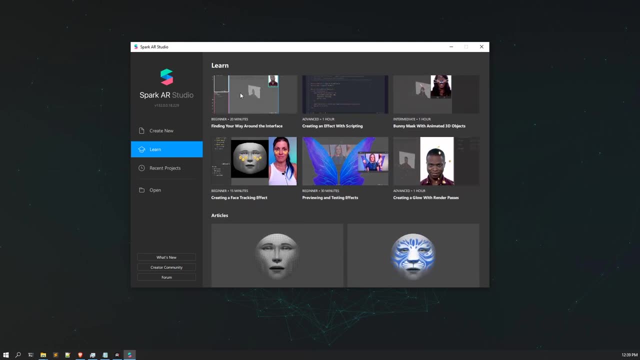 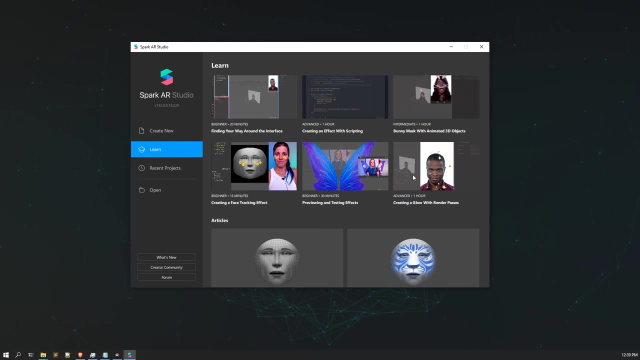 uh and turn all right. so make sure to subscribe my channel to get the updates about it. all right. so here are the tutorials that you can get here. you can see there are multiple tutorials available about the coding. all right about. uh means about creating a glow effect. 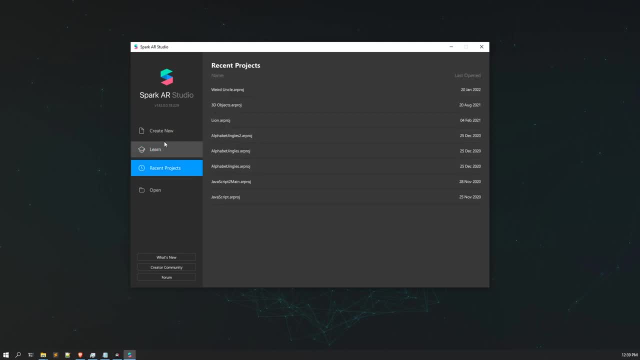 about face tracking. all right, so you can learn it from them. and here are the recent projects. all right, here are the recent projects that you can uh like. if you, if you create some projects, all right, inside of spark ar, you will get those listed down in here. all right, and here is a open option, all. 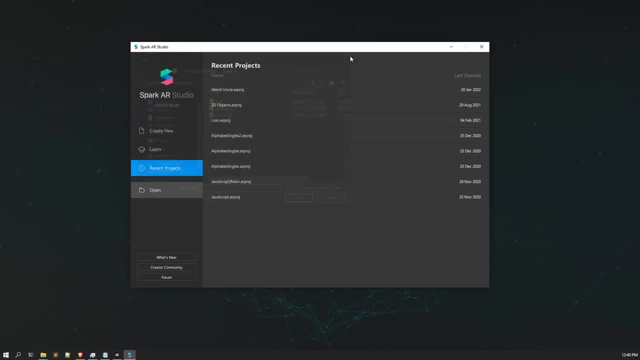 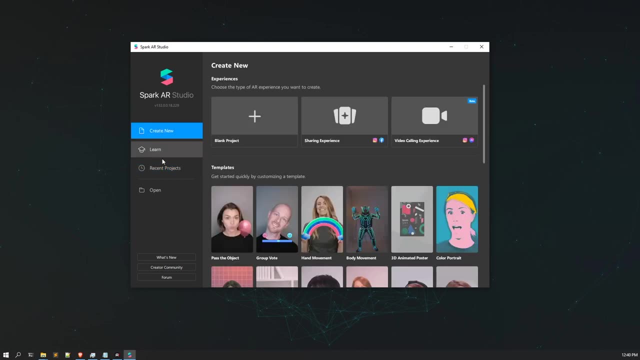 right. so if you, if you have a project file, then you can open that project file from there. all right, and here is the creator: community option, then forum option and what's new option- all right, so this is it all. right. now to create a new project, you have to click on blank project. all right, so we would be choosing. 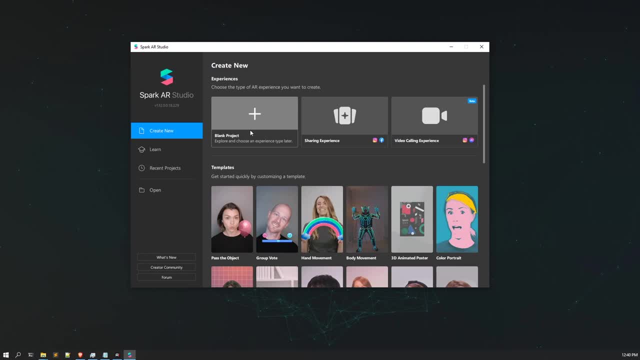 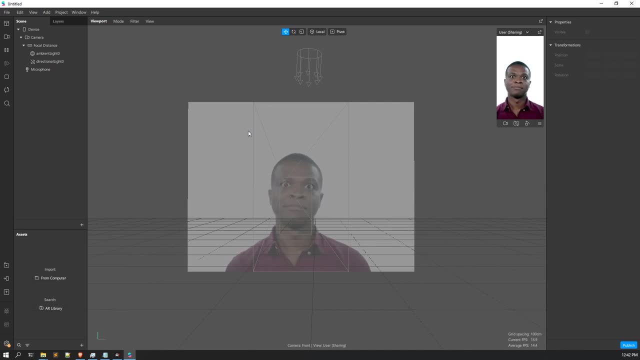 the blank project, and it would start creating the blank project for us, all right, so here you can see that our blank project has opened up. all right, so let's, uh, get a bit comfortable with the interface, all right, so the very first thing. all right, the very first thing. 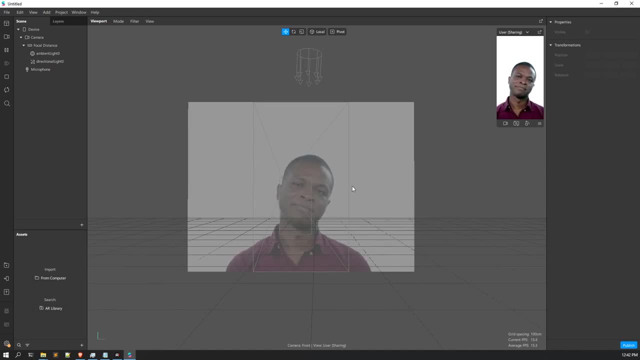 you are going to see is there is a person, all right, here. you can see this. there is a person who is like, rotating its head, all right, and here is a very small mobile like window, all right, here is a very small mobile like window that you can uh see in here. so here are. here is a simulation. 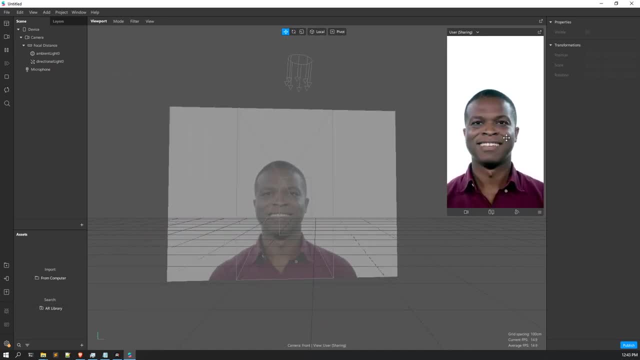 happening. all right, this is the person. so, basically, now, these are test persons. so, whenever we create any sort of marker, all right, whenever we are going to create any sort of marker, these- uh, these are the test persons that we'll be working with. all right, so our we'll be testing our markers. 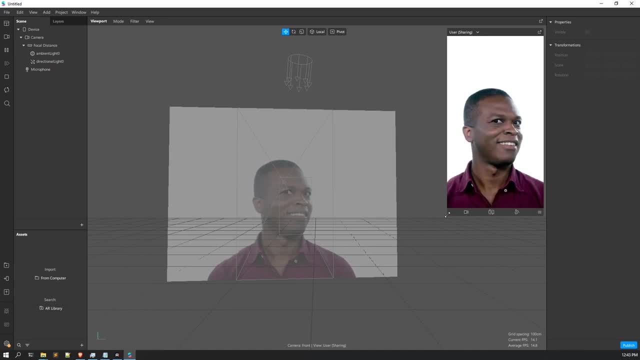 on these test persons. all right, so this is kind of a small phone. you could say, all right, this is kind of a small phone. or you can also say this is a testing window, just like uh in unity. uh, you can even dock and undock it all right, like click on this undock option, then it would be undocked. or simply when 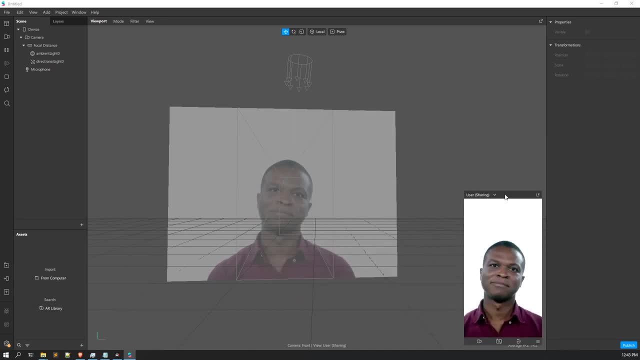 it is docking, you can drag it, drag it down, all right, and you can keep it anywhere you want, all right, but i, i prefer this uh one to be on the top, all right. so that that's where i'm going to keep it. now let me, let me shorten this a little bit. so i'm going to keep it on the top, all right. so 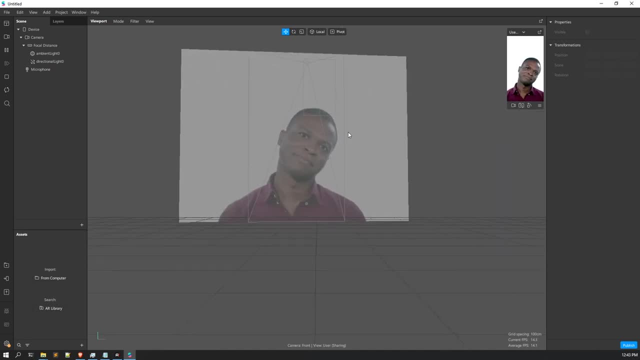 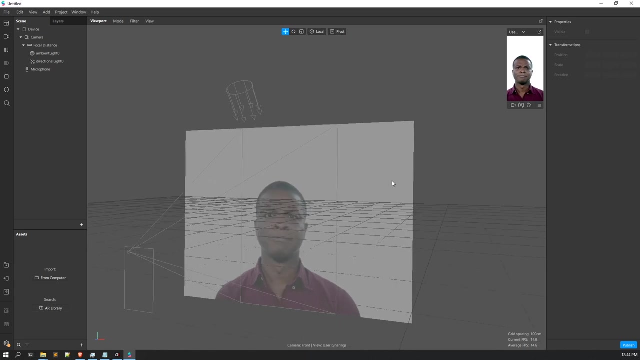 let me make the size small. now. here you can see that we are able to uh see, here's a total new scene where, uh, a camera actually is there, means there's this triangle thing is there and here's a film going on. all right, there's a video, uh, going on. so let me tell you what are these. 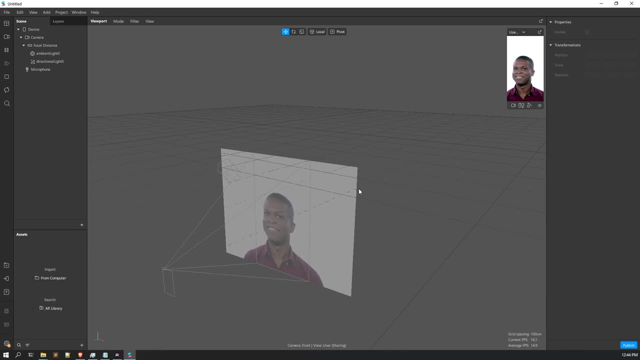 so, first of all, uh in unity- all right, i introduced you to the scene window. right in that scene window we used to add objects. we can, we could manipulate those objects in there, right, similarly in spark, here there is viewport window, all right. so basically this viewport window. what it does is we can add objects from uh in the in the scene panel. 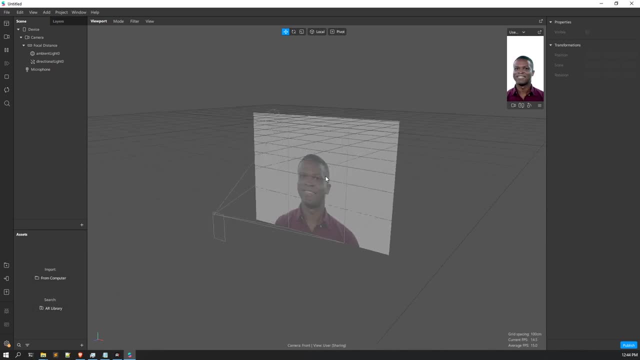 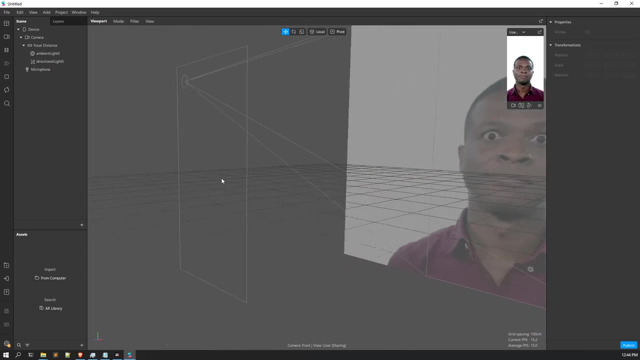 and manipulate those objects from here. all right, so that is it. and here you can see, there is a some kind of like phone, like structure. this one, this one, uh, this this thing have a phone like structure. this is basically a phone. all right, there is a simulated phone there. there's it. 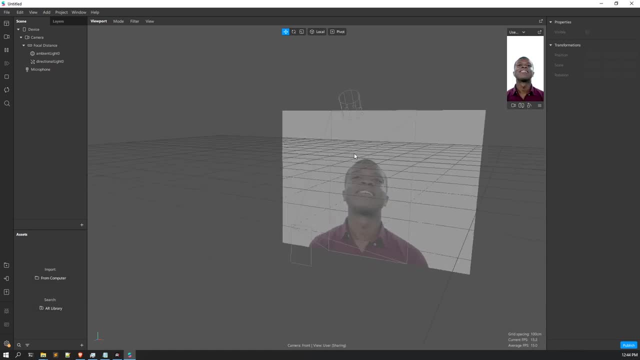 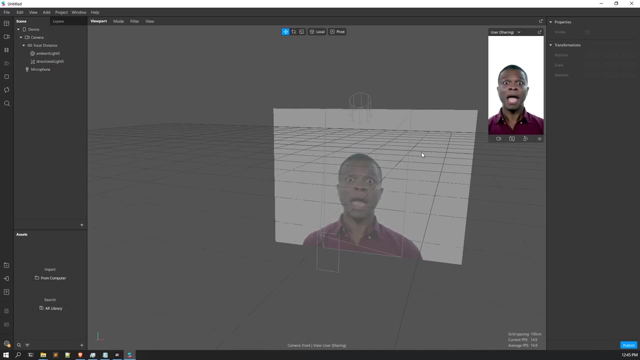 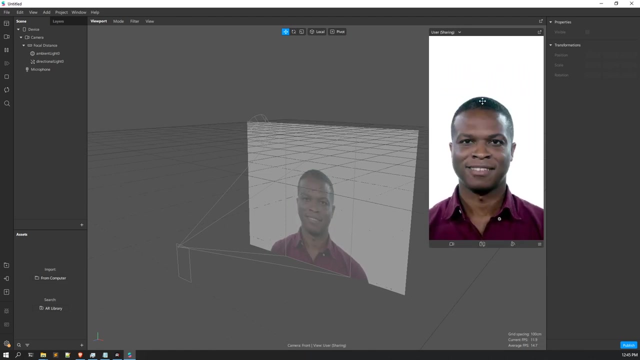 is showing that the phone camera is actually like projecting the filter on top of it. all right, so this is basically the camera, all right, so i hope you understand right now. this is basically, as i told you, this is the scene window, all right, and this one is kind of like the game window in. 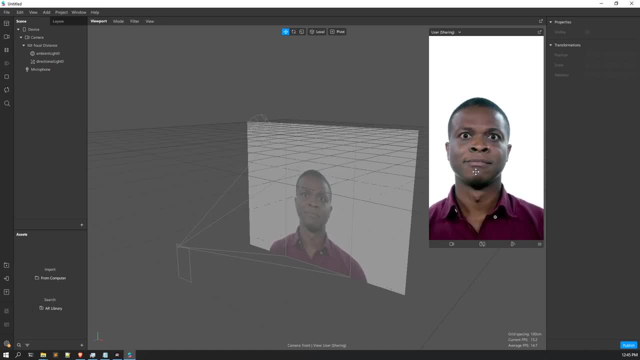 unity, all right, uh, so this game window in spark- here too, all right. so this, this is. you use this one for simulating. all right, now, as we uh learned about hierarchy in unity, right, similarly in spark. here also, there is another panel. this is called scene panel, all right, so what exactly it? 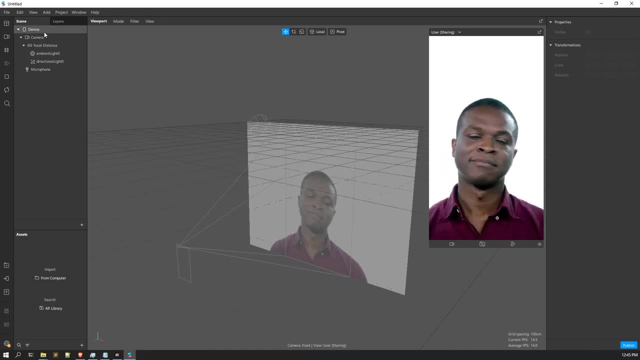 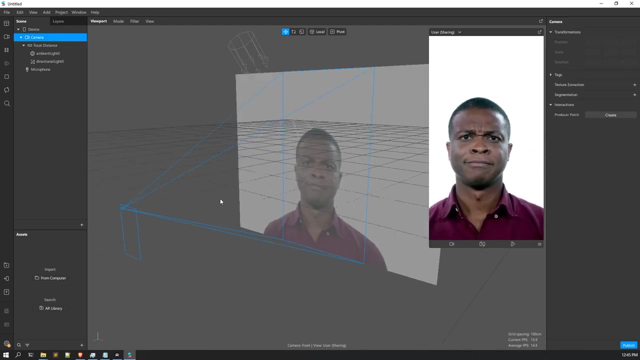 does is it contains all the objects that are present in the scene, right, you can add, add new objects in it. you can manipulate those objects right from here. all right, like: uh, here you can see, here is the camera object right in here. all right, is the camera object right? so this is the hierarchy window from unity. all right, so try to. 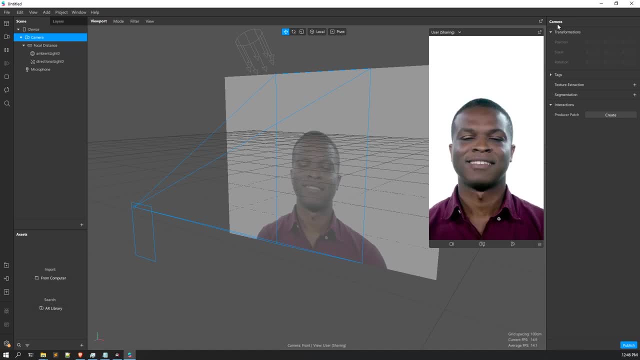 understand it like this. now let's see, uh, the inspector window of you know, spark ar actually in spark here it is called properties window, all right, but if you want, you can even call it. call it inspector window, all right, but it is actually known as properties window. so this uh. 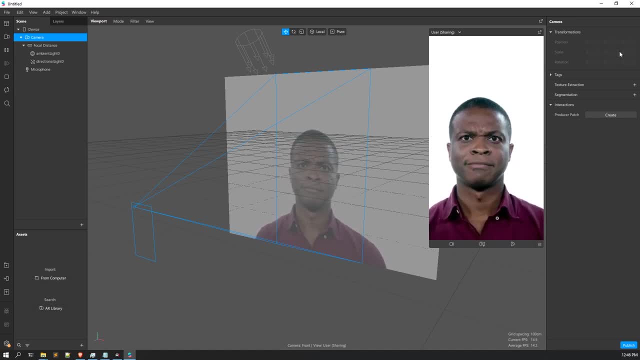 this is also like the unity's inspector window, all right, it also contains all the editable uh properties of a particular object, right like here. you can see that we can see. oh, if we, if we click the camera, we can see its properties right in here. here, uh, here are multiple. 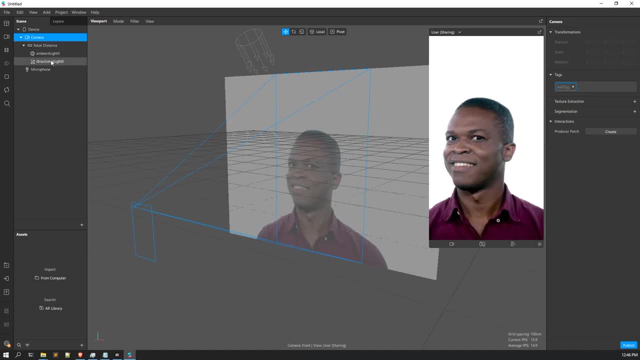 options in there. these are not editable, of course, but uh, let's say, uh, let's, let's try out this directional light. so here you can see that, uh, this directional light is editable. we can decrease and increase the uh means intensity. we can change the positions. uh, we can change the rotations, right, so 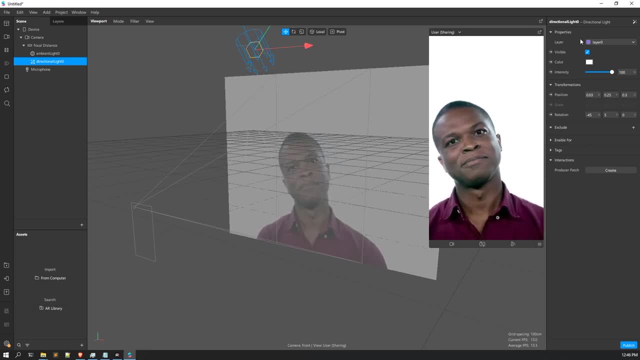 we can edit those. all right, this is kind. this is property window, just like the inspector window from unity. all right, now, in unity there was also something called uh project window, right. similarly, here goes: and uh, here is also one project window called assets window. all right, so this is uh like. 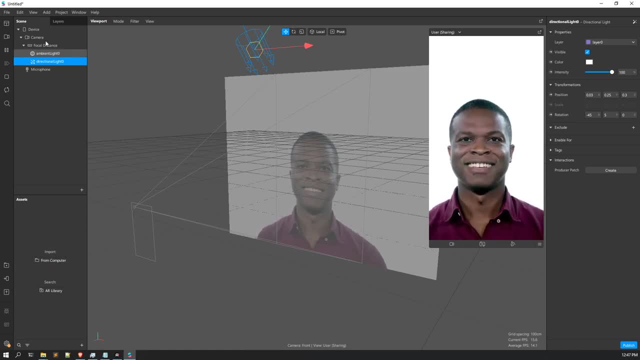 it is true? uh, it is under. it is basically under the scene panel, so you can see it right in here and you can actually drag and drop or import the assets right in here. all right now, this is for the basic interface. all right now, let me show you some more things. all right, like. 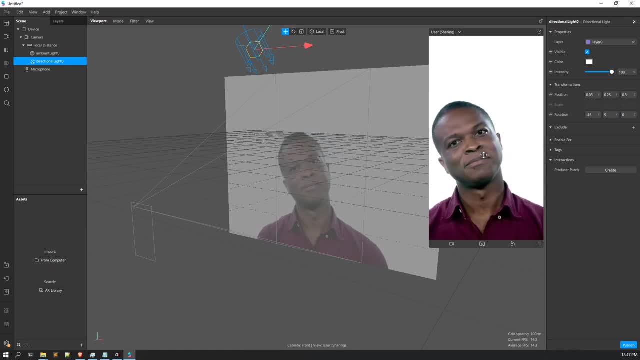 let's say i want to for for for testing my uh filter better, like for adjusting the filter, what i can do. i want to pause this character right. so right in your left. all right, like in the in the left of the interface, you would see a pause button. if you click on that pause button, the 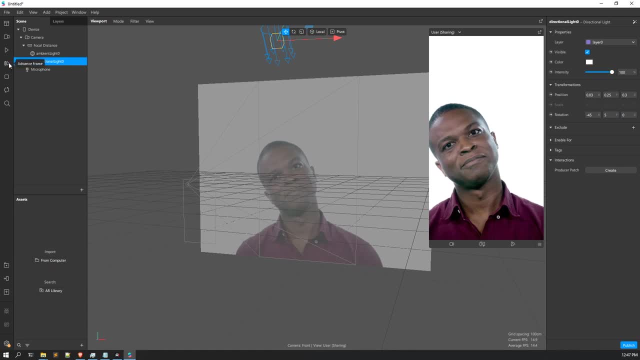 the video. uh, the video playback would be paused right now if you again played, then it would start playing right now. let's say, oh, i don't want that character. all right, i want to uh test with many other characters, there is all right. because, uh, his face, like the shape of his face, is different than others, right, so i want, i also want to adjust. 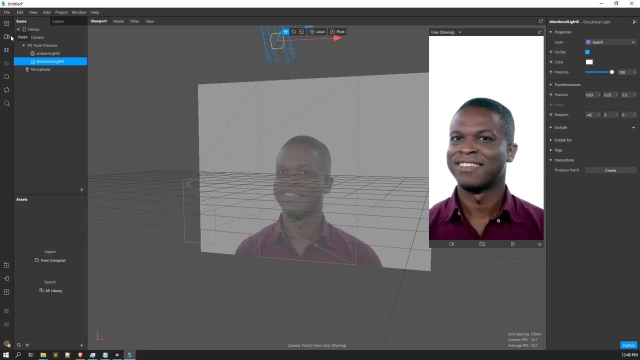 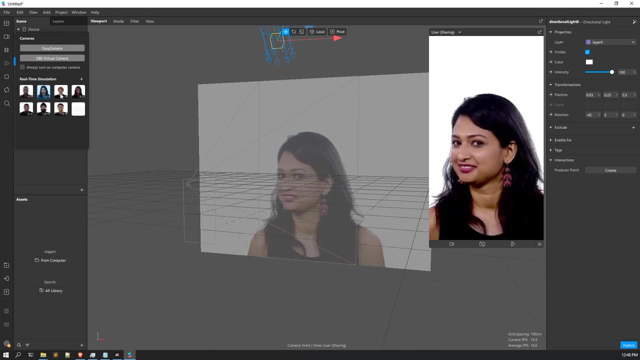 the 3d model. uh, to others, like to others, face shape, right? so what i can do is i can simply get another one in here, right? uh, then there's this thing in here, and if there's another one, then there's another one, then there are many. 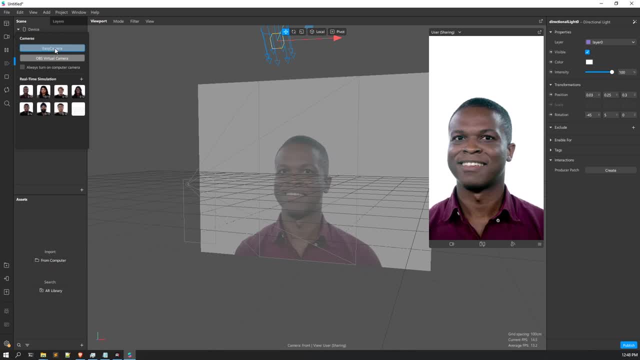 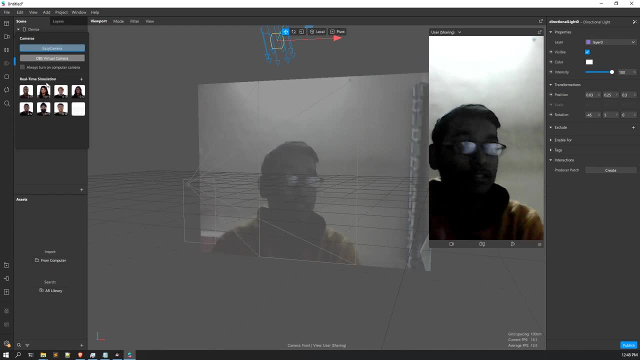 presets available, all right, and if you want to try it on yourselves, then they are like. currently i'm on my laptop, so this is the camera i have all right called easy camera, so i can. i can click on that and get the camera view on here, right, but currently i don't want the camera view, so i'm. 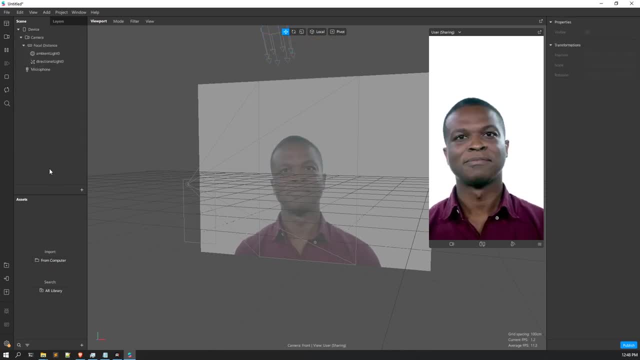 going to keep this person right now, all right, so this is basically would be needing as of now, all right to create the projects, and i'd also be telling you many other things as far as we move right and uh, let me, let me show you all right how you can get, uh, 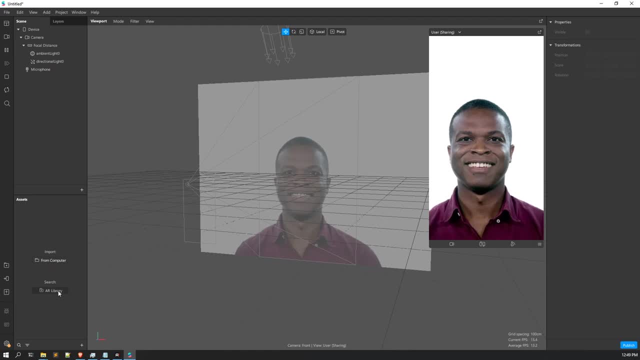 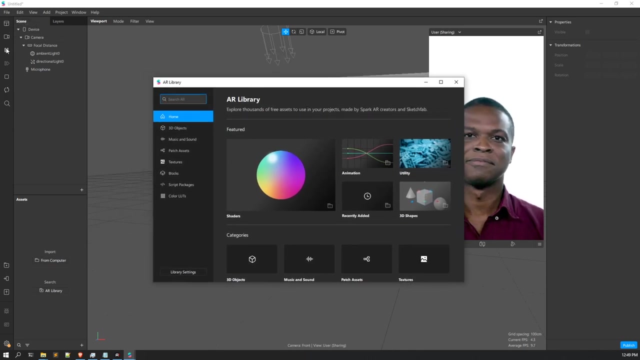 free 3d models. free 3d i mean free patches and all those things from in spark ar. only all right. so just uh, what you have to do is in the, in the assets panel, you have to click on this ar library, all right, and a window will appear, some something like this: all right, so let me pause this character. 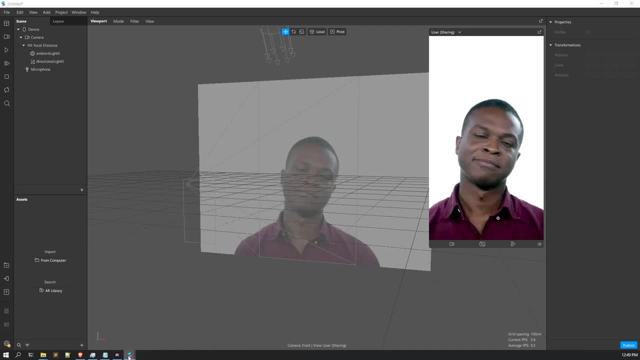 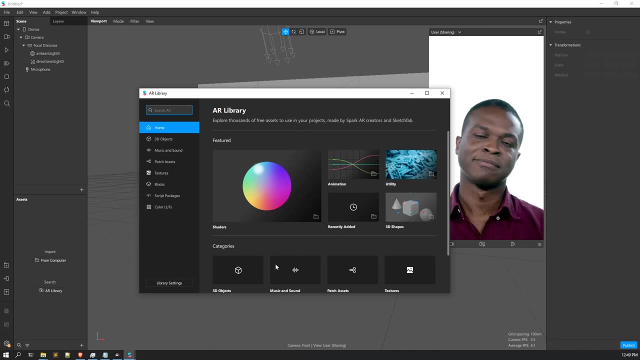 for a minute. all right, let me pause it. all right, and let's get this, this window, all right. so here you can see that there are multiple, uh, multiple options in here there. all right, there are multiple templates available. first of all, let's say, i want a 3d object. right, i can click on 3d objects, or. 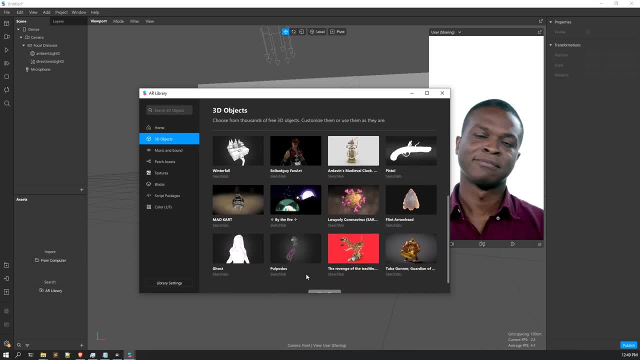 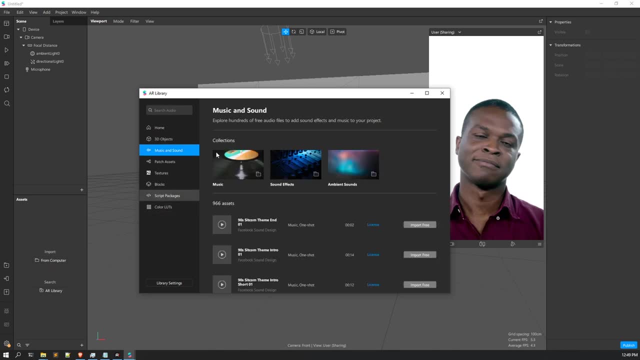 search for any 3d objects i want, all right, so and pick it from there, all right, these, these are 3d models, are free to use, all right. and let's say, i want, uh, any sort of music or sound. i can get that right, i can get. 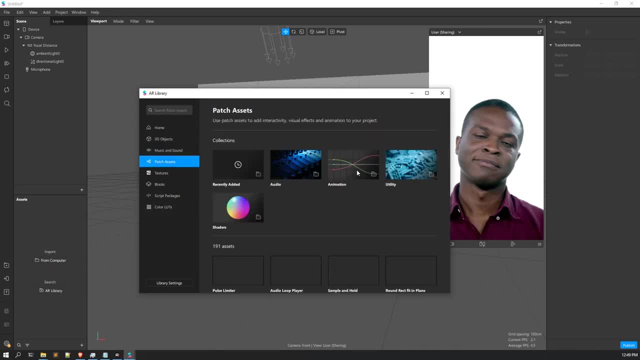 that from spark here. only then there are patch assets, patch are basically there's. there's two ways to uh code in spark here. one is visual scripting, that is the patch editor, where you have to move blocks here and there and connect one block to another to code. and there is that we can. 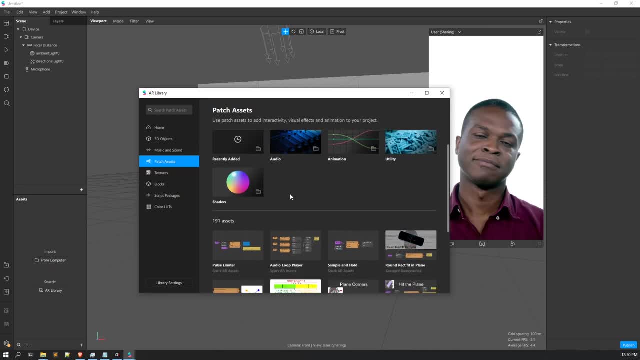 code it through scripting. all right, so there are presets available. you can use those presets. all right, let's say, if we, if we want textures, we can get those textures from here. also. if we want uh blocks, all right, we can also go get those blocks from here. if we want the script packages, 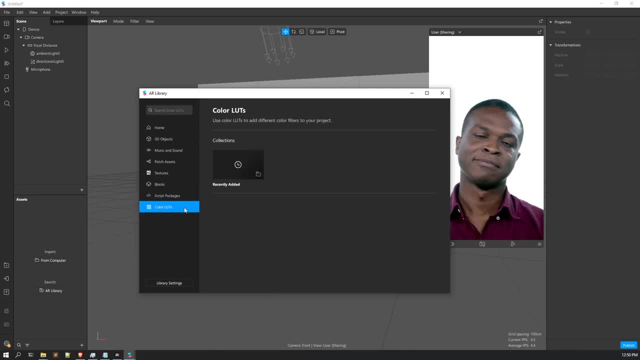 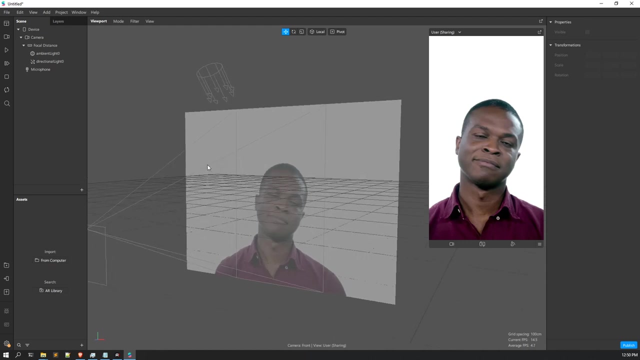 all right, we can also get these script packages from here, if you want. if we want color lut's, we can even get these from here, all right. so spark here has a pretty good ecosystem for its creators, all right, and uh, if you talk about how to launch our own filters, 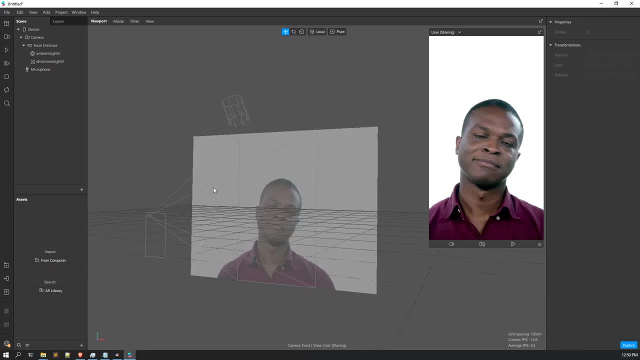 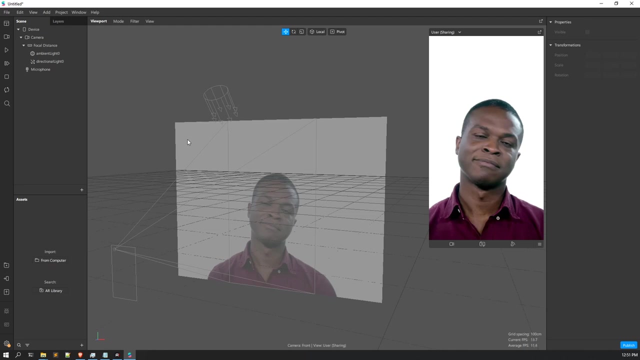 all right, so to launch our own filters. what you, what you would be needing, is a facebook account, all right, and an instagram account to launch your uh ar filters on instagram, all right. so make sure you have a facebook account at least, all right, and uh, of course, uh to upload it on instagram. you also. 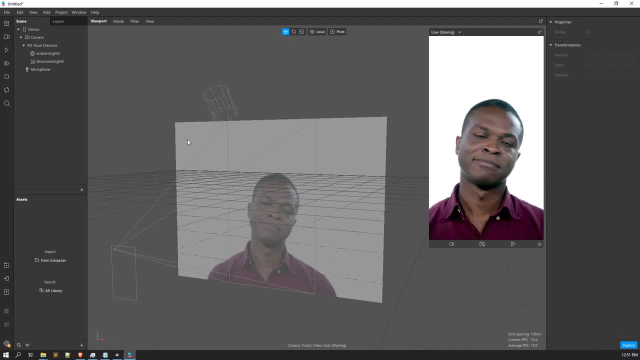 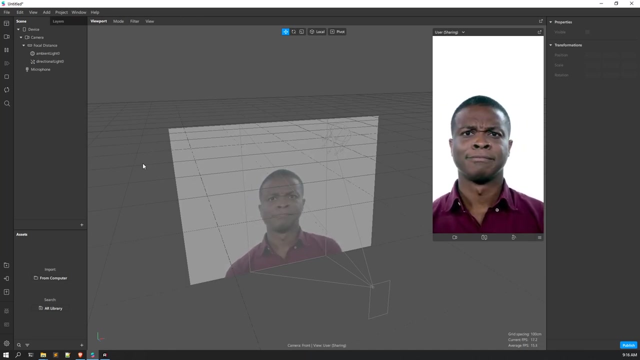 need a instagram account, right, so, yeah, cool, great. so this is it for, uh, this lecture, all right, see you in the next lecture, thank you. in this lecture, we are going to learn about face tracking- face mesh, all right, and and we will also be creating our first filter based on face mesh- all right, so make sure. 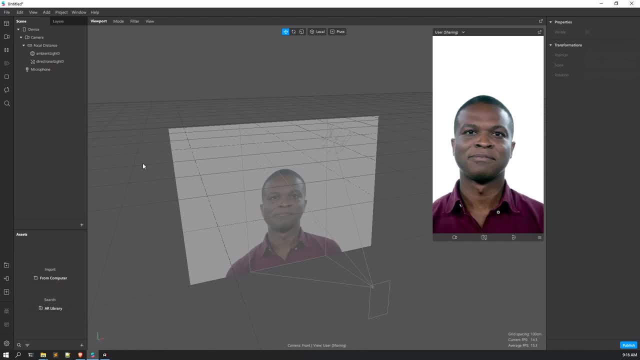 to watch this video till the end. so we are talking about face tracking, right. what is face tracking all right? what exactly it is it all right? see, face tracking is a concept, right. face tracking is an algorithm that actually helps us to track our face right, like, for example, 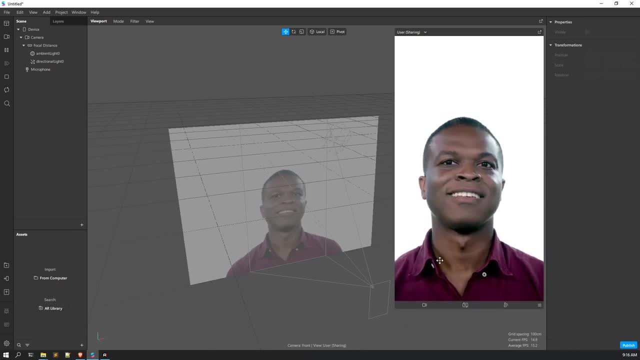 you can see this person right in here. all right, he is moving his head left and right, up and down, right. if we attach an face tracking algorithm on module, what will happen if it would? it would track this person's face like, for example: see this person is moving his head upward. then also the 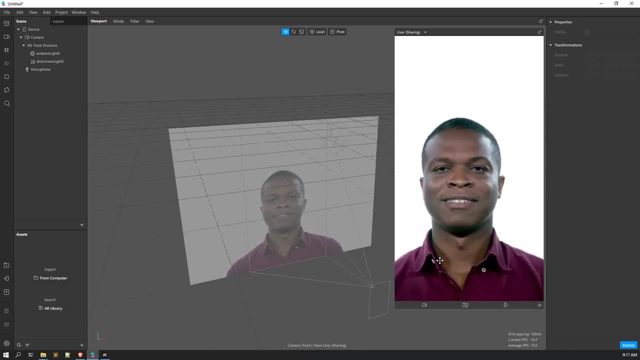 face tracker will also put a face tracking algorithm on the face tracking algorithm and we will also point upward. all right. so that's how a face tracker would work. it would track the person's face, right, it would, it will, it will take, all right, it would actually take the person's head rotation. 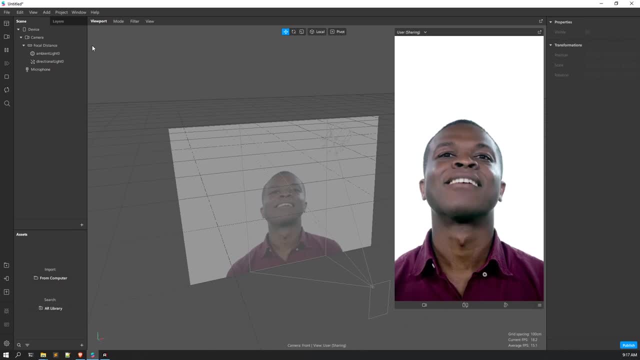 and uh, movement from the real world and uh, put those values inside of the editor, all right, so that it can perform other tasks. that's, that is, what a face tracker is. all right now, a face tracker is very simple, all right. what you have to do is you have to go to the your 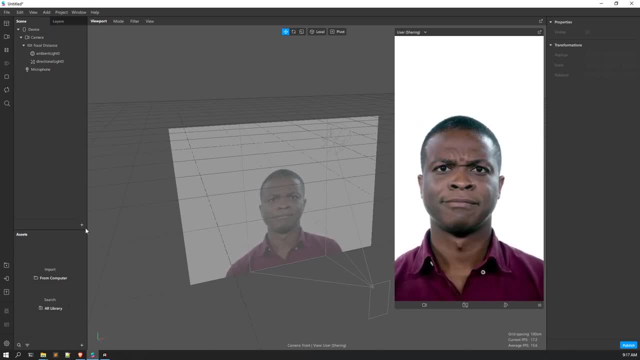 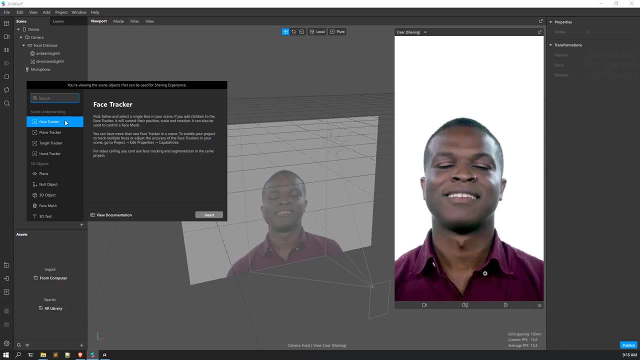 scene panel. in the scene panel. there you would be finding uh addition, uh, plus button. you have to click on the plus button. all right, and in here. in the first option, you will be there. face tracker- right now. if you are not able to find the face tracker, you can simply search it in here. 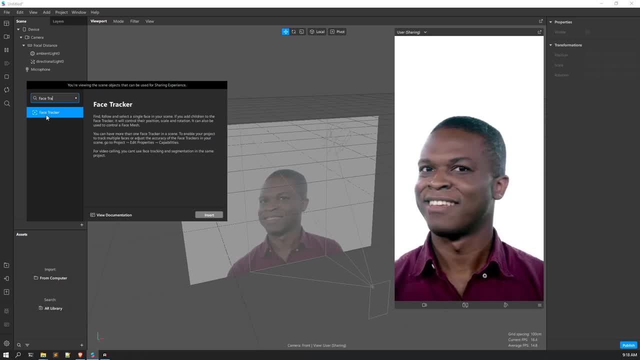 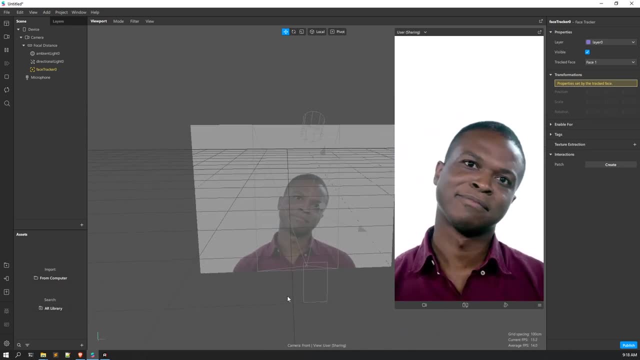 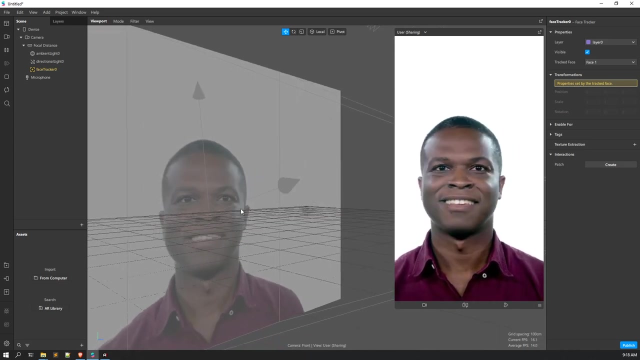 that is face tracker. and after you do that, uh, click on the face tracker and click on insert right. so here you can see, here you can see the anchors right. you are able to see the anchors right, the you can see that, with the face all right, with the rotation and movement of the face, the anchors. 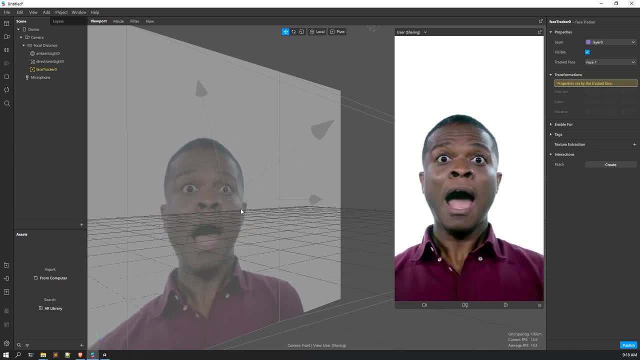 are also moving right. so that's how face tracking works. all right, that is what face tracker does right now. as you have learned about face trackers and spark ar, now there's left face mesh, right to make your see, face mesh now is a sort of a layer on your face. 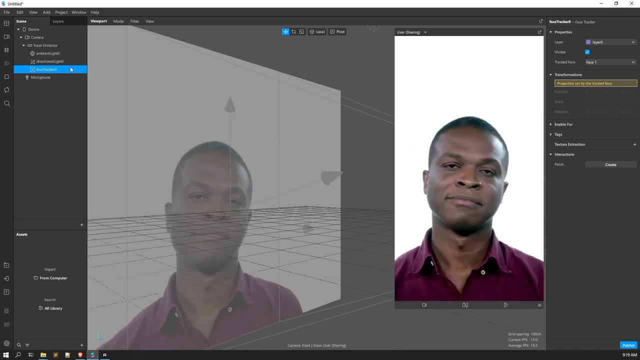 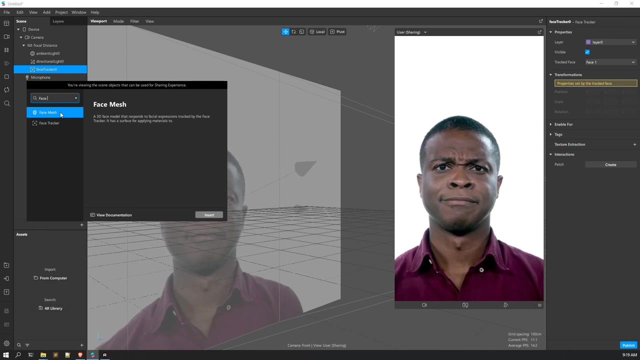 all right, it's, it's kind of another, another object on your face. all right, you can understand the face meshes just like this. all right, now to add a face mesh, click on this face tracker. all right, then click on add and write face mesh and you would find the face mesh. all right, and click on. 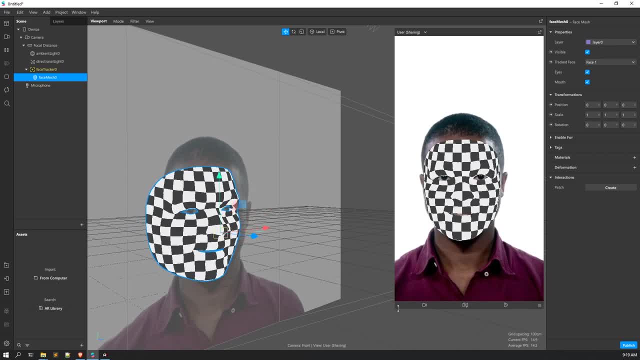 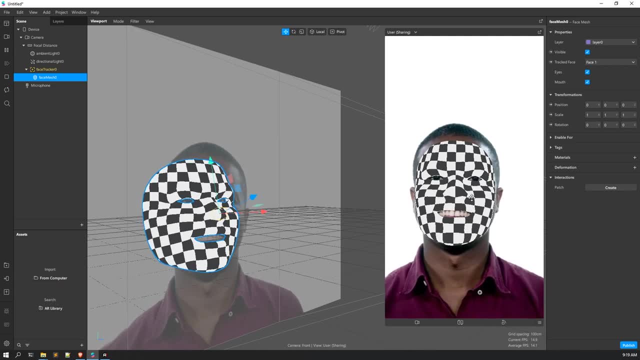 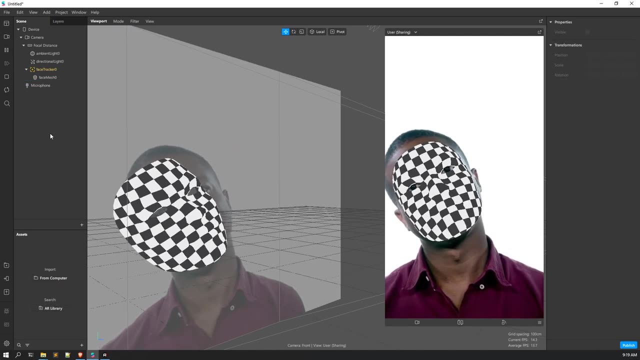 so here you can see that we added our face mesh, right it. it looks like checkers board, right? sorry, not checkers board, but uh, chess board, right. so one more thing you have to remember, all right that whenever, if you want to make like if you are attaching the object, which can totally work with. 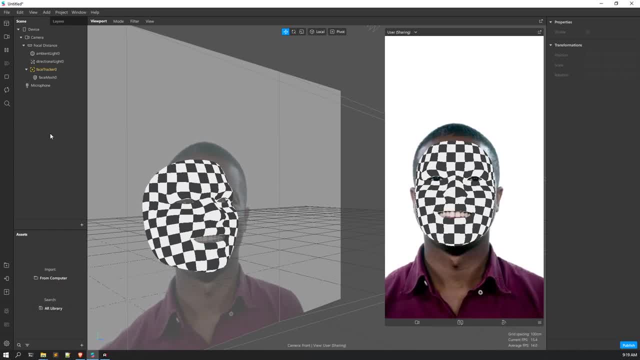 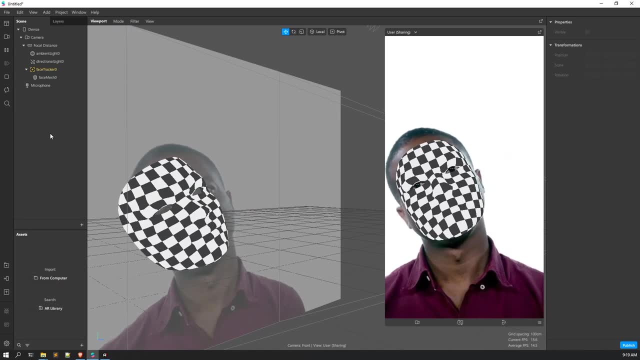 your face tracker. all right. that is, uh, use face tracker for tracking the face. then make sure all the objects that you are putting in your scene, all right, you have to make it a child of the face tracker object. all right, why? because, uh, here you can see. 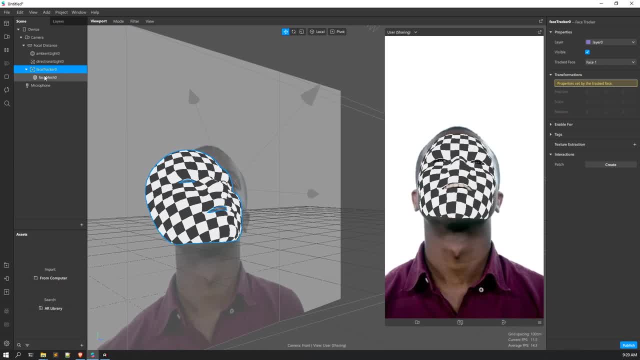 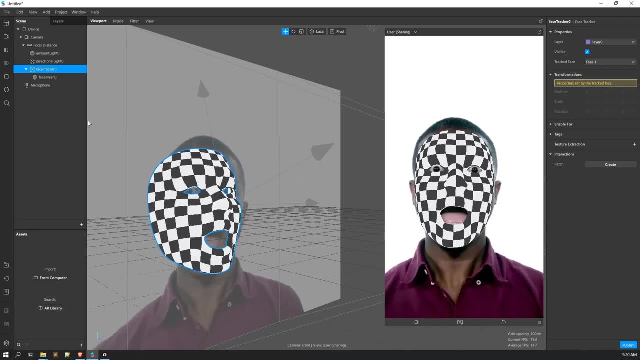 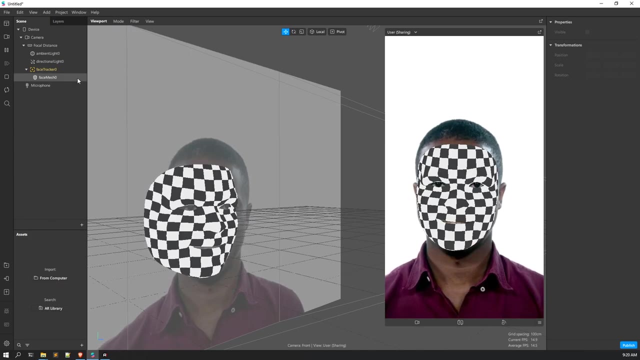 that, uh, as the person is moving its head, this particular face mesh is also moving. all right, moving and rotating, that's how it is working, right. so that's why i told you to make the objects of face uh, uh, like a child of the face tracker. only, if you want uh to like, you know uh, make it rotate. 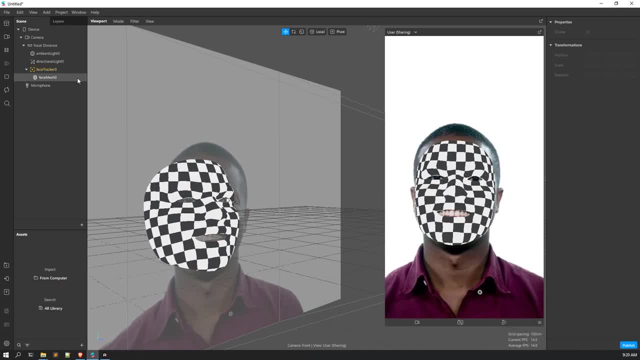 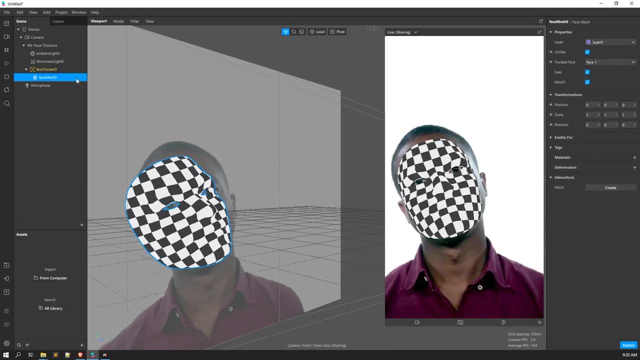 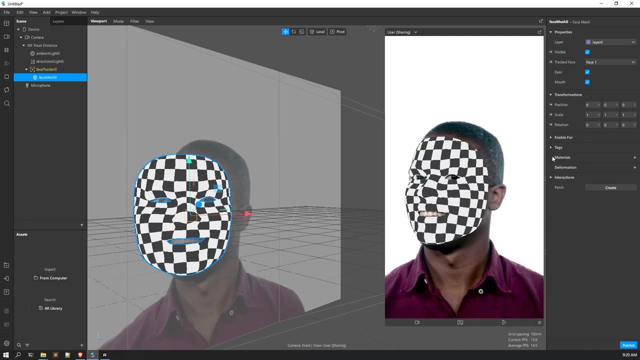 and move on the player's head movement and rotation right. so that's how it all works right now. as we have added a face mesh, we can also add a material to it. all right. so what you can do is click on face mesh in here in the properties panel, you'll be finding a material section and here 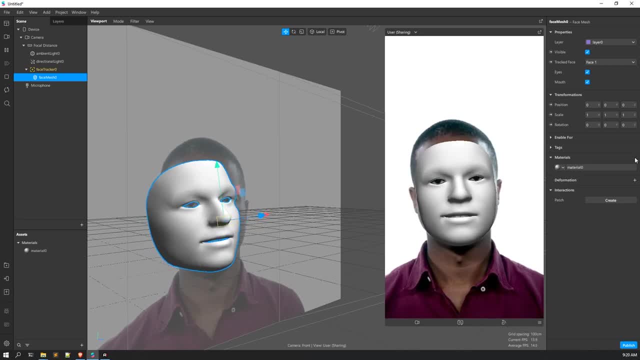 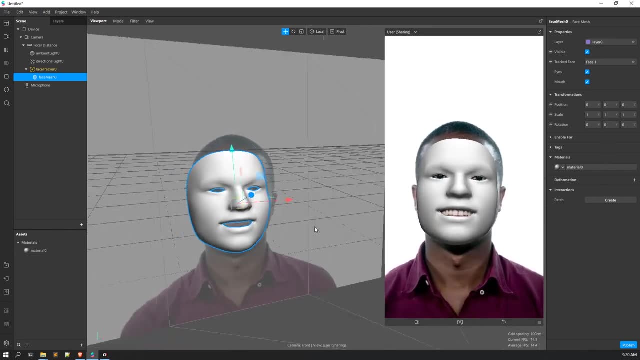 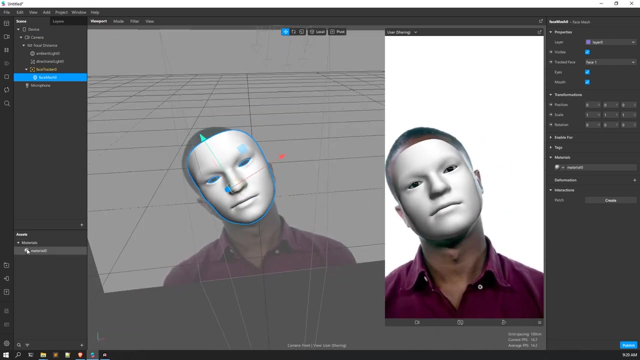 you'll be finding a plus button, so click on this plus icon and here you'll be. a material would be created in your assets panel. and see, a material is also added. right now, if you want, you can- uh, like you know- change the colors. color of the material. all right, so simply select the material, go to its 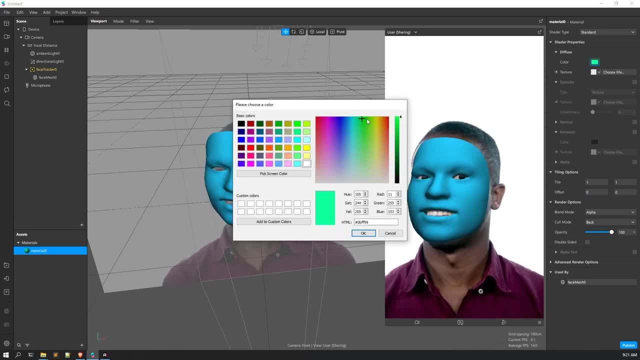 properties and change the color. all right, change the color to whatever you want, all right. you can keep it red, you can keep it, you know. uh, green, you can keep it yellow, uh, you can keep it blue, anything you want, all right, but for for now, i want to keep it. uh, you know. 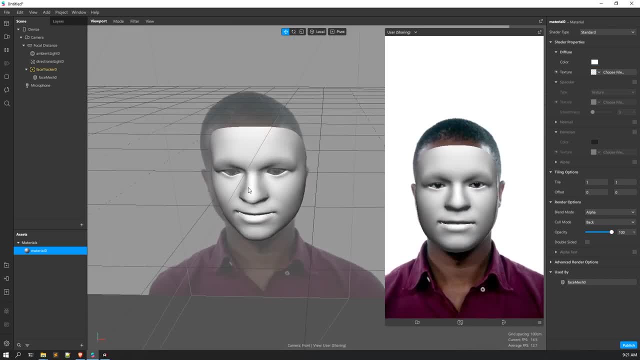 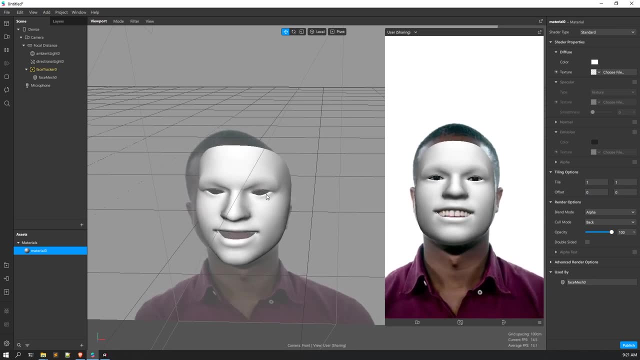 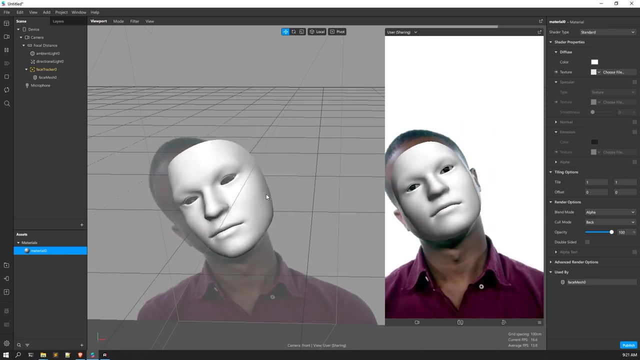 white right. so now, as we have learned to create our own face tracker and our own face mesh, right now, what we have we, what we can do, is we can add textures to it all. right now. this is a bit tricky part. all right, if you are familiar with photoshop, uh, then this would be a bit helpful to 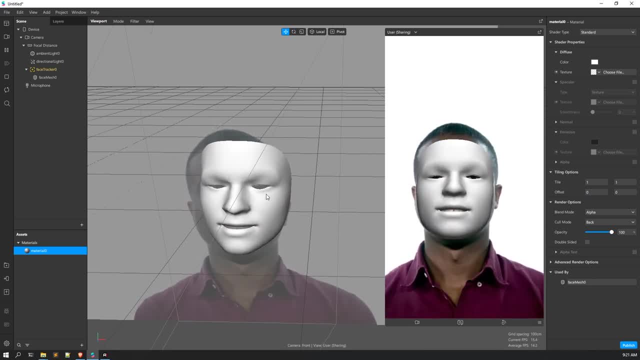 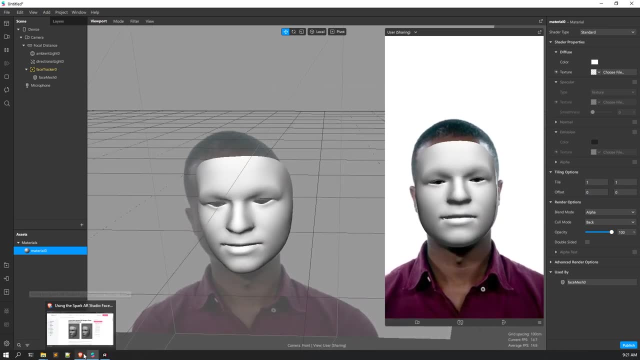 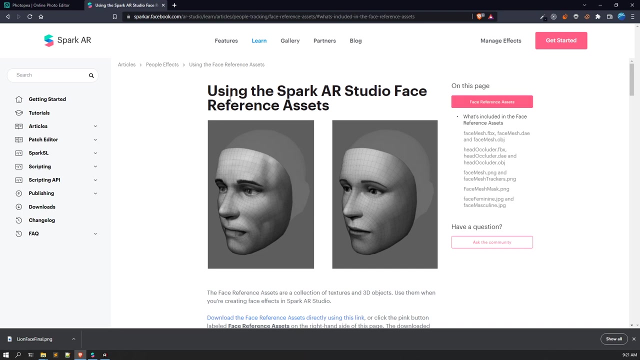 you like you. helpful means easy to you, all right, so let me show you. go to your browser first. all right, download these face reference assets. all right, because these, these face reference assets are going to be really, really useful to us. all right, so, just uh, go to. 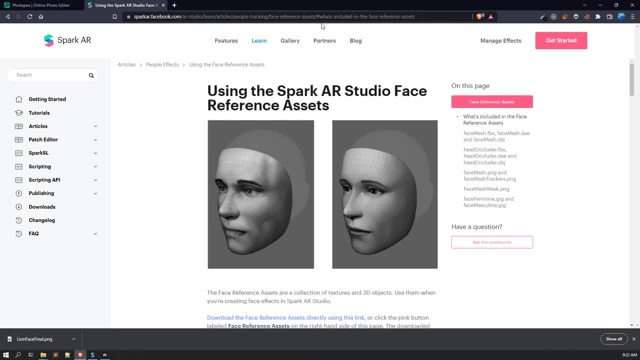 this particular website. you can, you can simply write on the internet: uh, sparky, our face reference assets, all right, you would get. get them in there. now what you can do is you can click on this face reference assets and it would start downloading- downloading a zip file. after you extract it all. 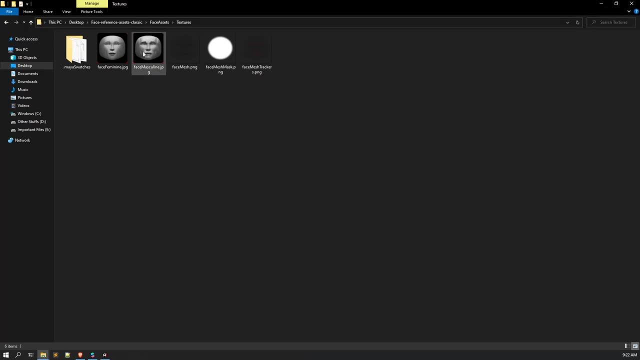 right, go to the textures folder and you will be finding, uh, two textures, all right, one is face feminine and one is face masculine. these are basically face reference assets. all right, to create the textures for our face. okay, so i'm for this. for this example, i have used means. for this tutorial, i have used face masculine. 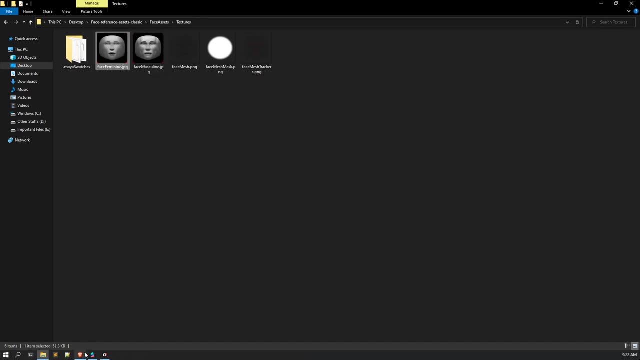 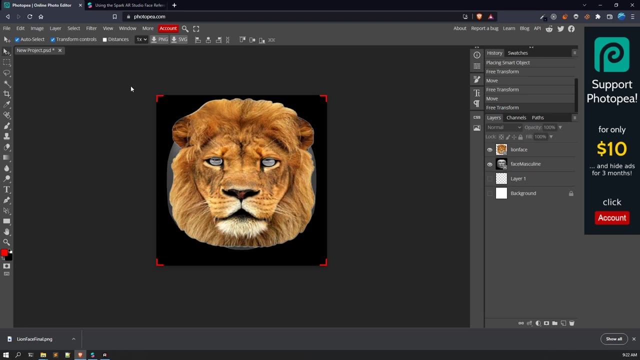 you can even use face feminine if you want. all right, now what you have to do is uh, open photo p your system. you can open that. all right, i have used photo page, so it's like photoshop button online. so now what you can do is, uh, first of all, import this face masculine in here. all right, import this. 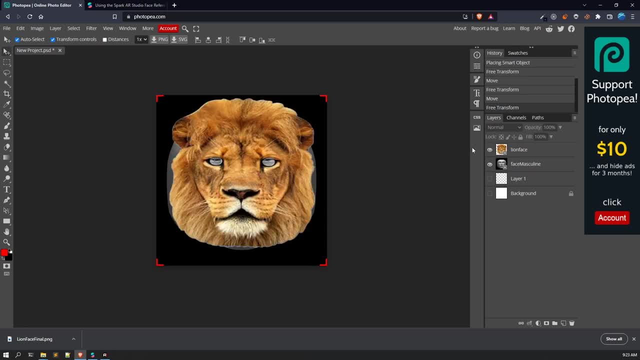 face masculine in here and import your lion face texture- uh, for me it's a lion face texture. you can use any texture if you want. all right now, what i did is i pressed control in my uh. you know, i pressed control in my keyboard and uh mapped it like this: just wait, okay, here you can see that i uh. 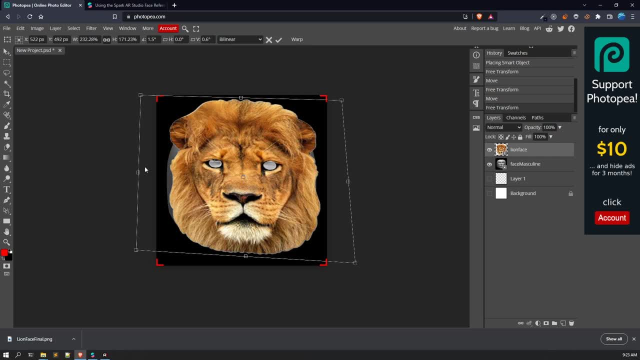 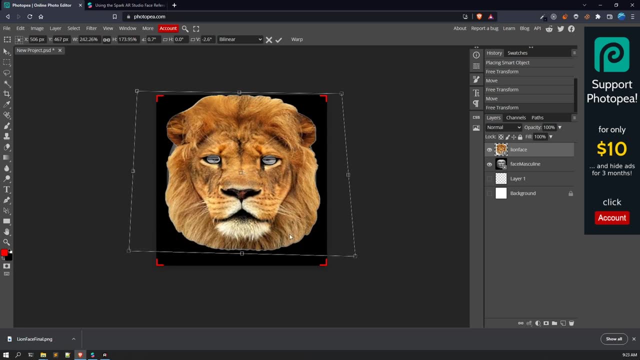 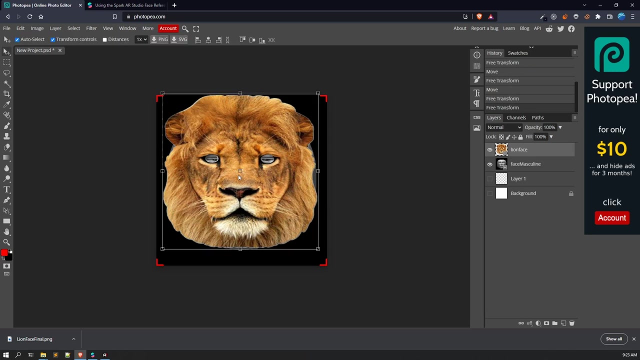 mapped it to the proportions of, uh, the face, all right, to the proportions of the face of the this particular reference picture. all right, and here you can see, you can like. you just have to press uh control, right, you just have to play to press, control and edit the transforms. all right, and you will be good to go and always make sure that. 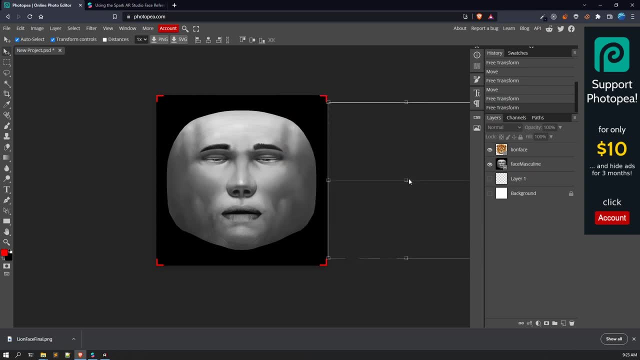 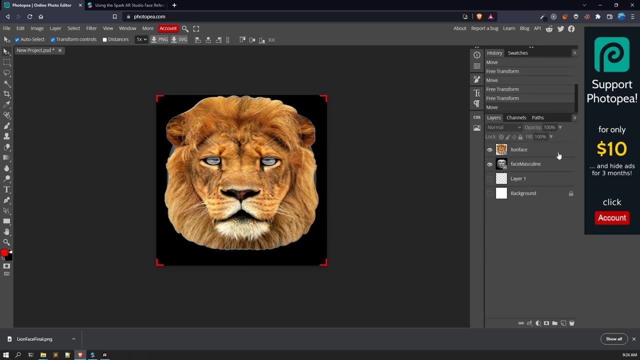 these eye holes, all right, are in place of, uh, this, uh, reference assets eyes, all right. so make sure you do that, okay, and this is it. and then what you can do is you can simply, like you know, uh, turn off this background layer and add another transparent layer and you can simply, uh, go to file, uh, 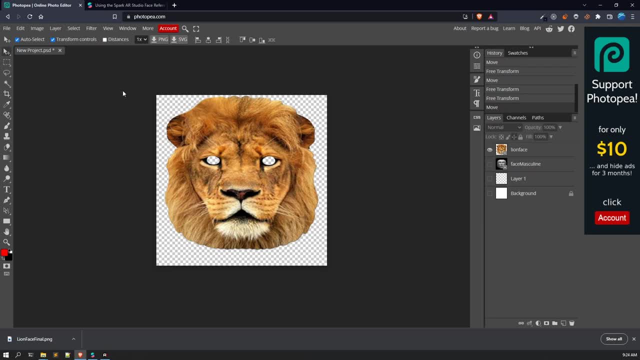 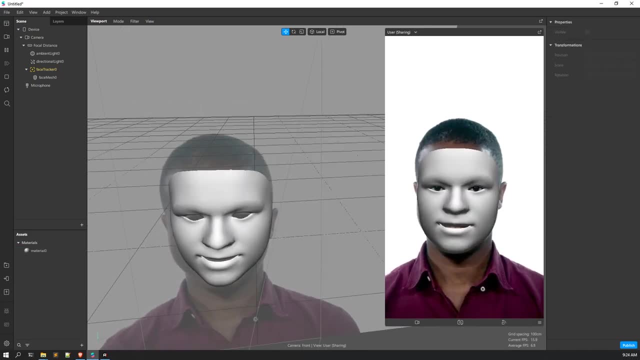 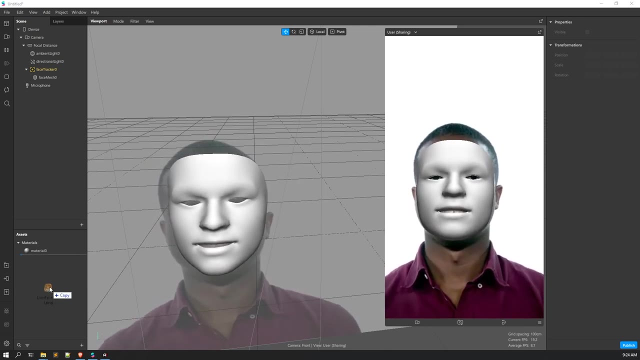 explain as png and your you know your texture would be exported, right? i have already done that. now what you can do is simply drag and drop it, uh, inside your asset. all right, that is inside your editor, so i'm just going to drag and drop it in here, all right? 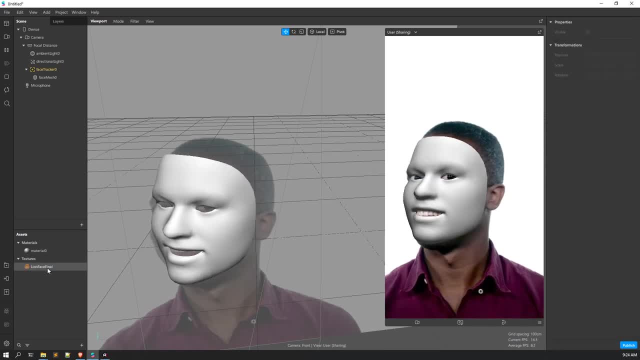 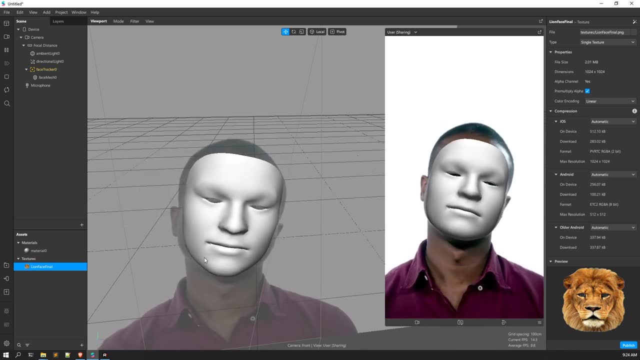 so, yeah, now is it is uh, you know, uploaded on within the. it is uploaded within our spark ar studio. all right now what you can do is sometimes what happens in your uh, it would uh start- actually not sometimes every time it happens- that it would start uh compressing it. 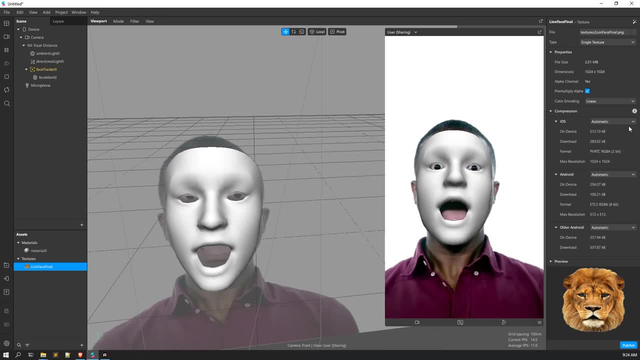 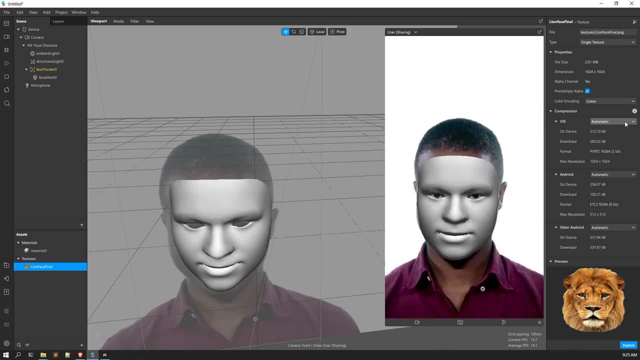 all right, and mine is already compressed. it's. it was so fast, so what you can do is all right, it makes uh, makes the editor slow already. it makes park ar slow for for the moment. all right, for the moment you can uh select it to uh means uh the data, so you can make your, your, uh, your, your, uh, your. 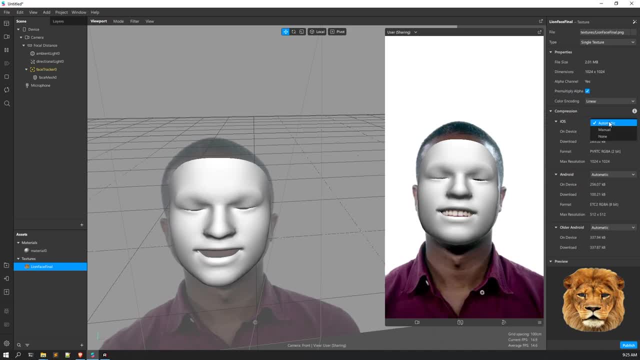 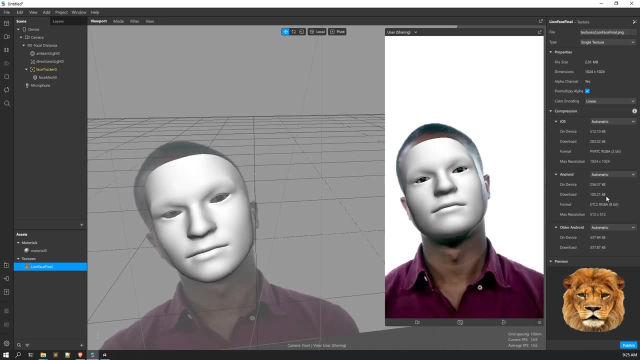 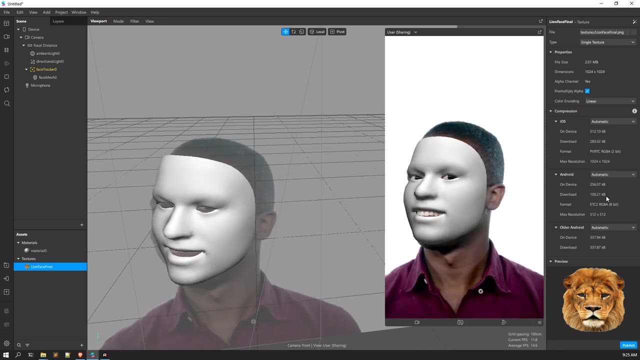 in the ios section make it to none. then in the android and older, or android also make it to none. so it would stop the compression for a moment and whenever you, whenever you will be publishing a filter that is exporting it and then publishing it, it would start the compression. it will compress. 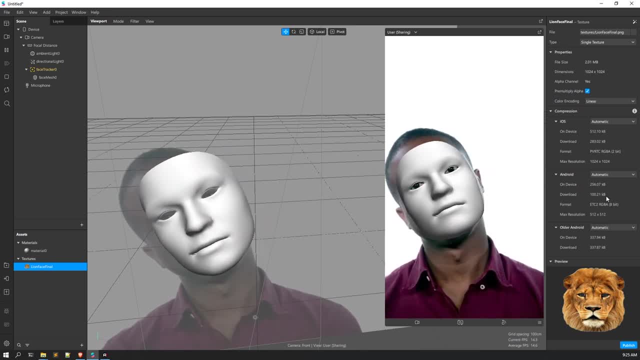 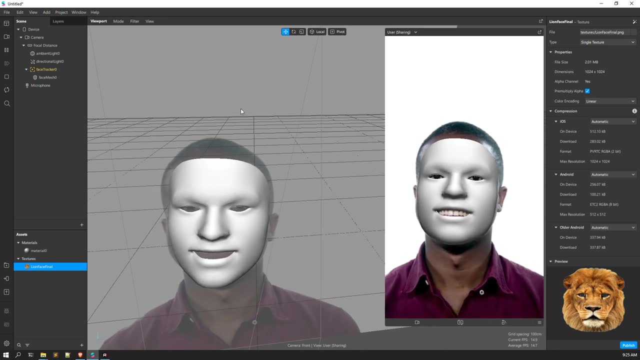 your filter and then you can upload it. now, always remember to compress your filter before uploading it to spark- sorry, to instagram or facebook, all right, so make sure you do that. now, as we have learned to create our face tracker, our face mesh, let's add a texture to the face mesh, all right? 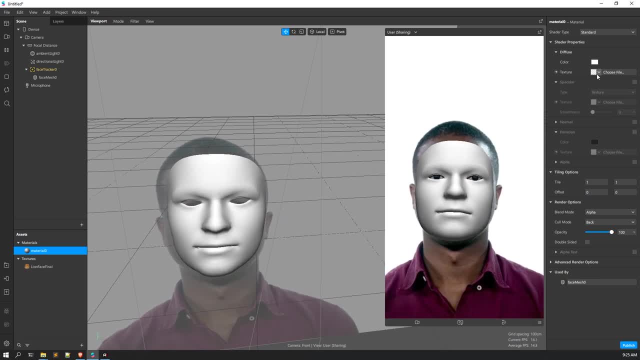 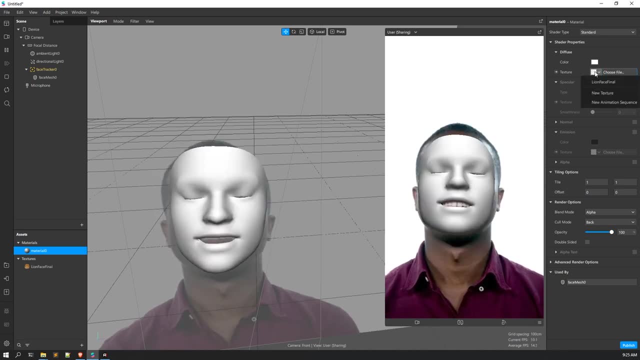 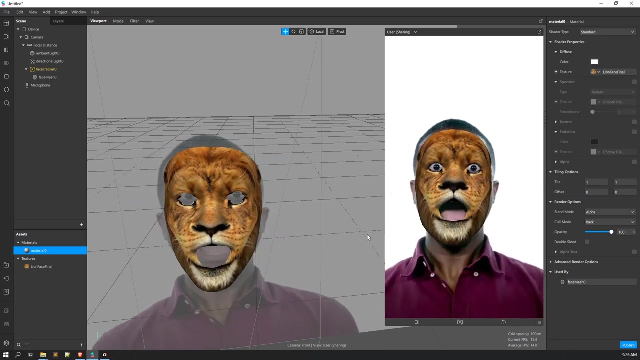 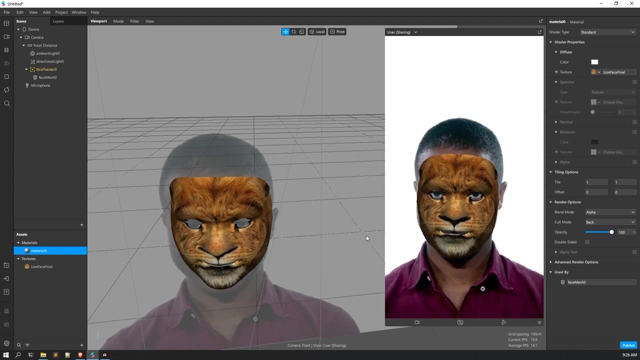 this is also very simple. we already have our lion face, which is mapped to the reference image. select the material in here you'd be finding a texture section. click on this image thing and select the texture. all right, and here you go. you got the texture in your spark here, right? so that's how we work with face meshes. all right you. 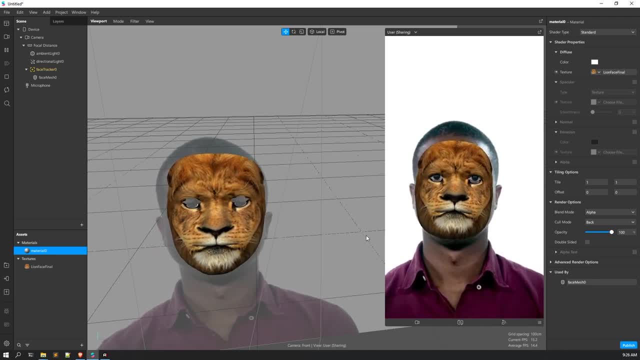 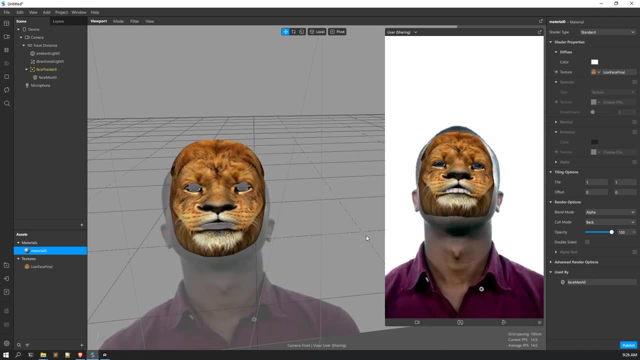 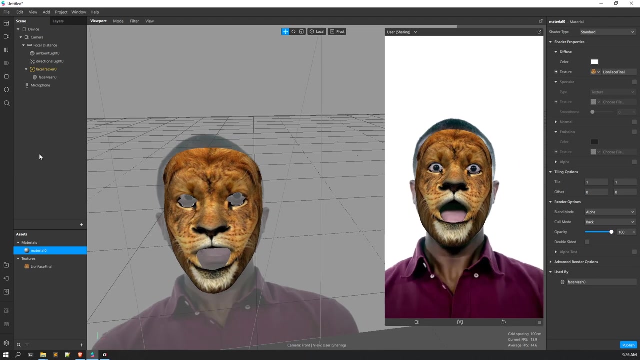 can also like add, you know, occlusion effect in this face mesh. in the next lecture only we will be learning about occlusion because we are implementing our own 3d model, spark here. all right, but for this lecture this is it. and we learned about face tracker, we learned about face meshes and also created our 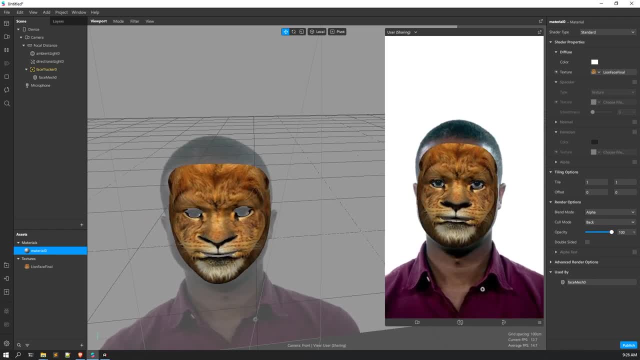 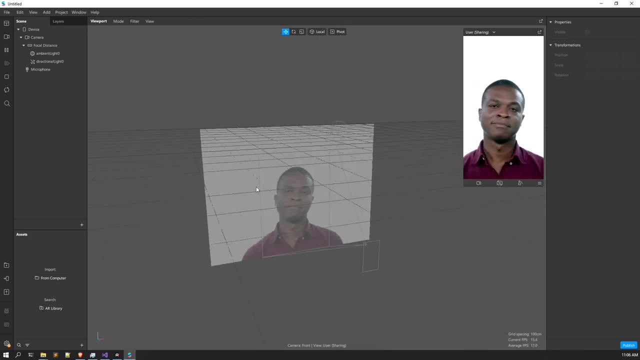 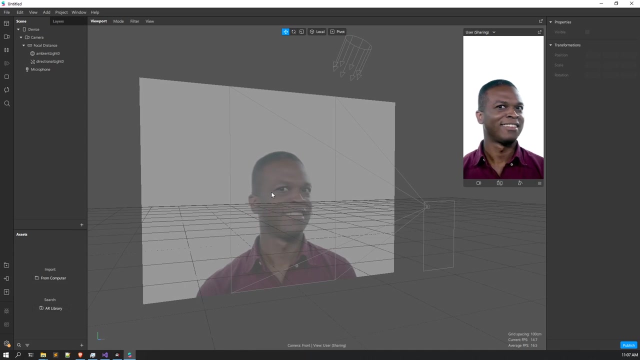 first phase filter, right, so yeah, so, as you are already aware of spark here, all right, and you already know how to create 2d filters with spark here, right now, it is of a very high time to learn how to create 3d filters. all right, that. 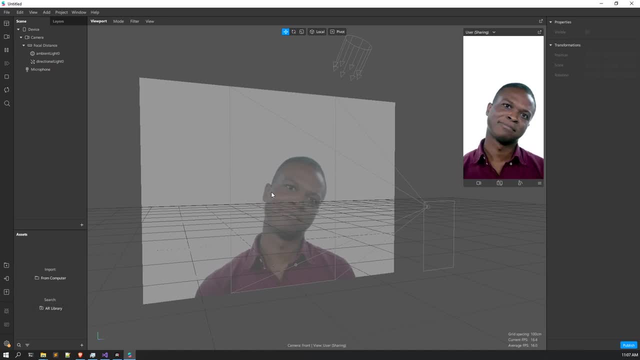 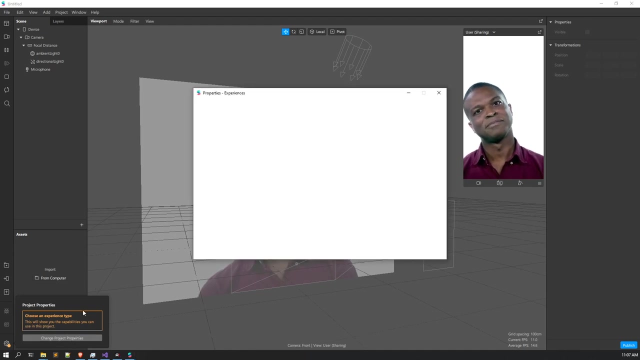 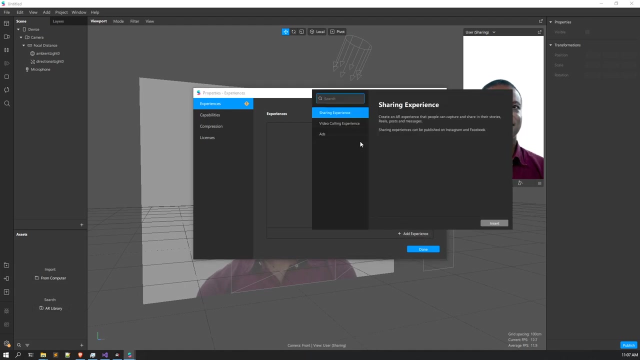 is: use 3d models with I'm with another filter, all right, so the first thing, all right. what you, what I want you to do, is or click on or go to settings, and that is project properties. click on change project properties, all right. here you will see a tab experiences. so click on add experience and where select. 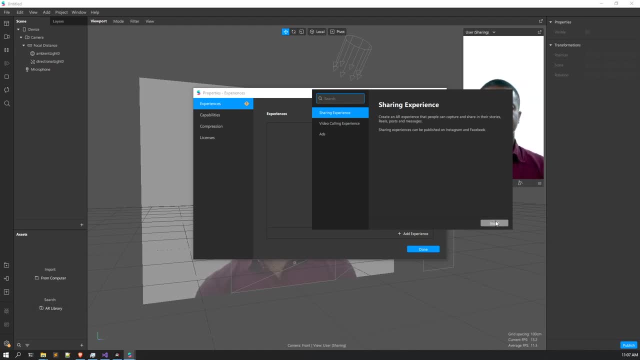 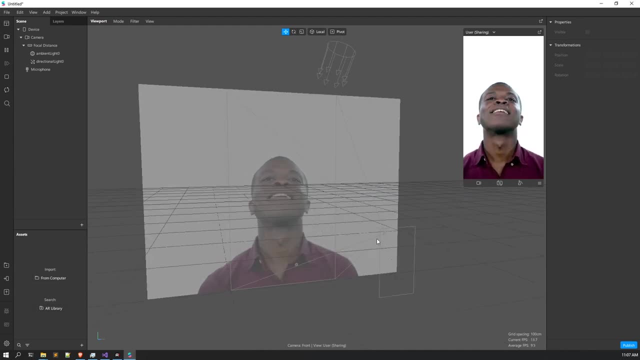 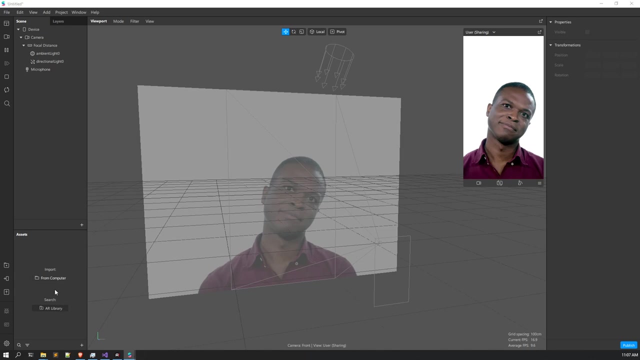 this sharing experience and click on insert. all right. so after you have done that, we are good to go with the project. now what you have to do is add a 3d model, the first of all. add a 3d model of it. well, I click on air library and find 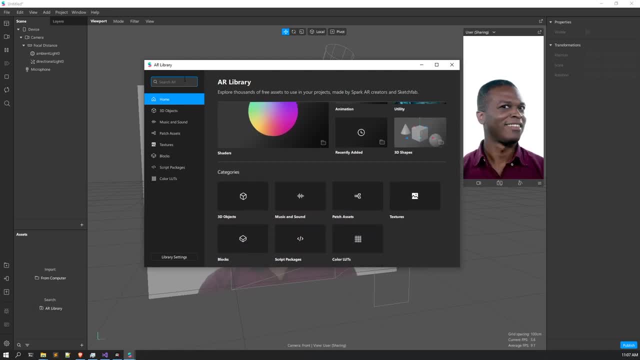 for a 3d model you want. all right. so let's say: let's get our cap. all right, let's get a cap. it's actually a 3d cap right now. let's get this Pokemon's masters cap. right click on import. it will start downloading the model and 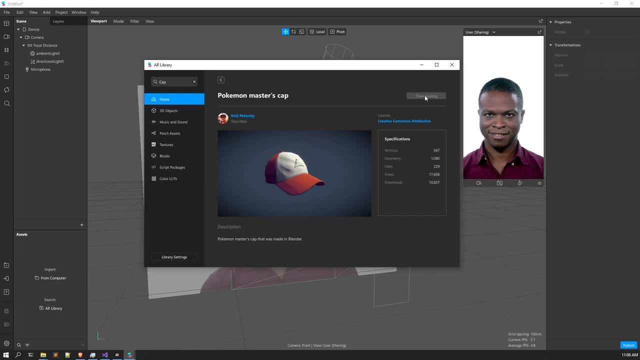 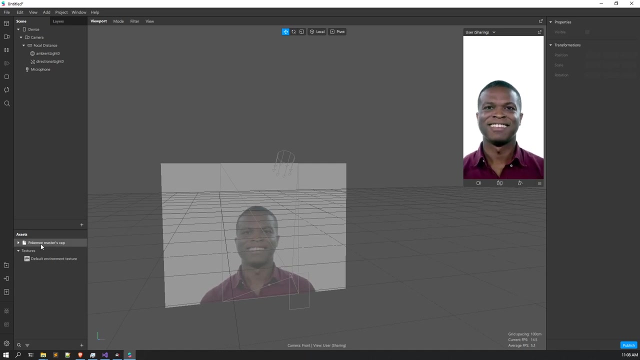 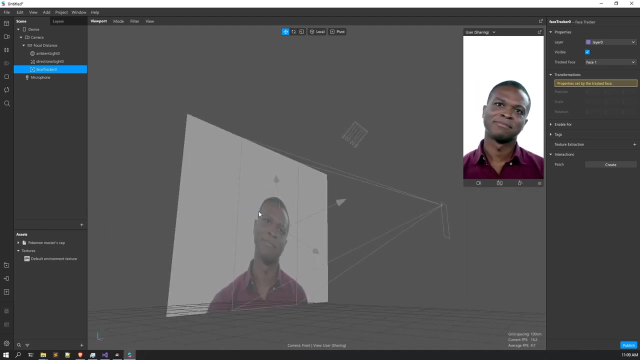 all right, so it has completed downloading the model. now close this window and cool, so we are good to go. now click on this focal distance or camera, oh, all right. then click on add- that is this plus sign and add a face tracker. all right, select the face tracker and insert it. all right now. here you can see that our face tracker is in place. the 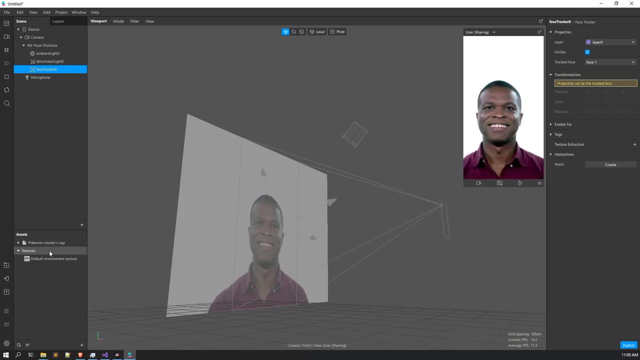 gizmos are working for, perfectly fine. now what i want you to do is click on this default texture environment. so not, not this one, just wait. yeah, this one. material all these textures, all right. what i want you to is remove the compression, all right, because that would slow the when. that would. 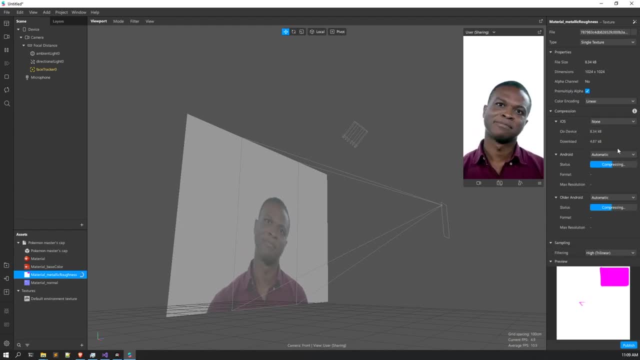 basically slow spark ar for me and i currently don't want that. yeah, of course, when, whenever you are publishing, all right that you will, uh, when you will publish your filter, make sure that, uh, you compress them all right, because, uh, compressing the filters are really necessary in. 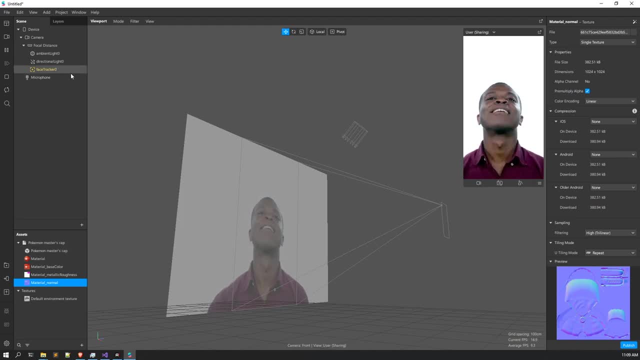 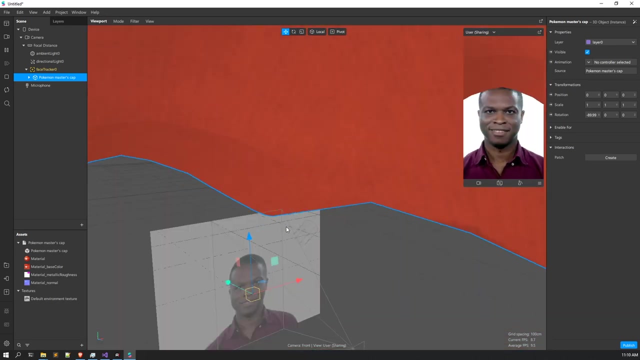 case of uh uh publishing it uh on instagram or facebook. all right now, what you have to do is uh get this pokemon masters cap, that is, this 3d model, and uh drag it inside the pokemon face tracker. right now you can see it. so it's uh like really, really, really big. now let's scale it. 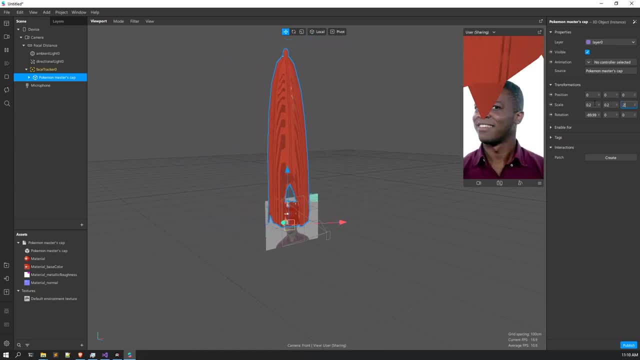 down, that is, give it a 0.2 scale. okay, just wait. okay, cool. uh, still it big. uh, let's give it 0.00. let's say: eight point zero. eight point zero, eight. all right, that's, that's too small. okay, point zero, actually zero eight. i, i think by mistake i give 0.8 to 0.00. sorry, 0.08, okay. 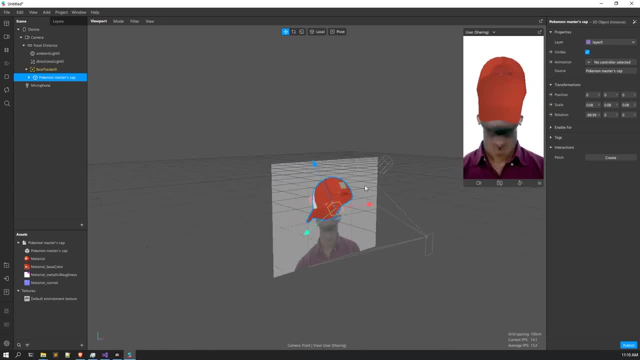 all right, it's, it's uh. now the size look good, but here you can see. all right, one more thing: let's uh remove its uh rotation actually. okay, not, not this one uh. let's give it um rotation like this. okay, it does have some rotational problems. 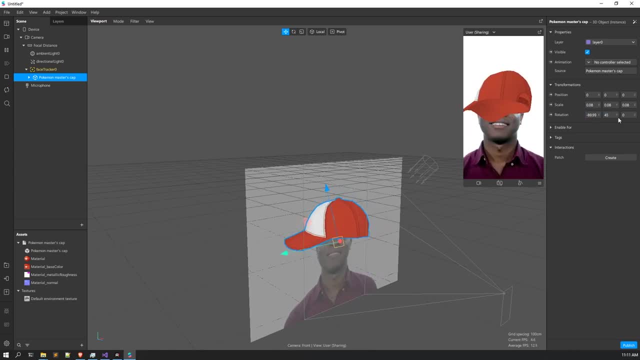 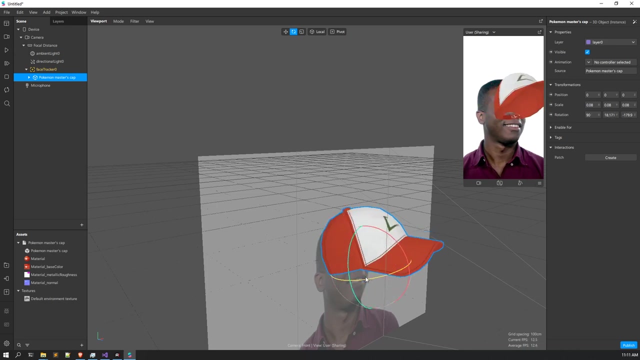 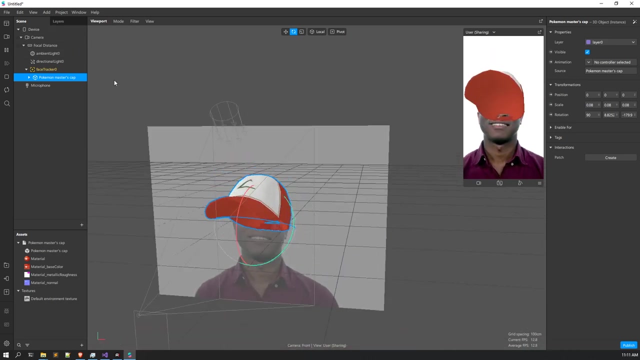 just wait. okay, minus 90.. actually, let's uh, first of all, let's pause the play, all right, and yeah, this, this is better. now, here you can see, we can't adjust, uh this cap on the person right like it's. it's not being adjusted like it, it is not fitting. it's just on top of his uh head and of. 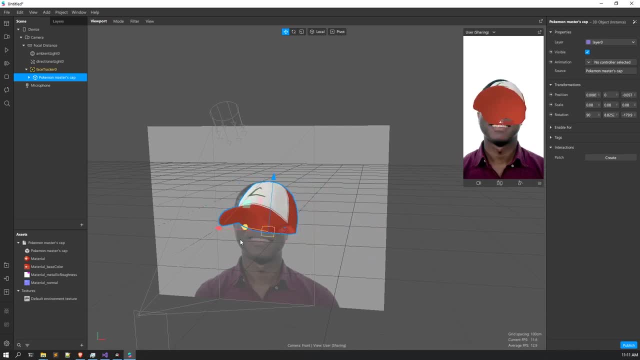 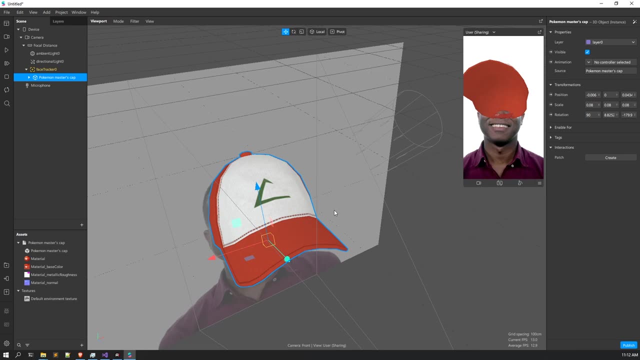 course we don't want that, right, we don't want it. just just see, it can't even go on its face. so now here comes a concept of occlusion. all right, see, occlusion is basically now uh, like in real world, when you put uh, let's say: uh see, you have two hands. right, you have two hands. 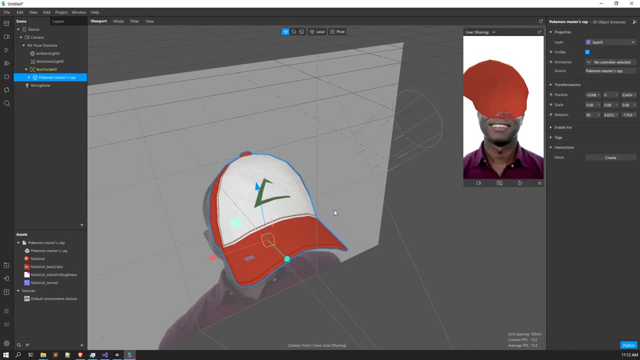 let uh put one hand on top of the other hand. right, would you be able to see your other hand? that is, let's say, if i take one of my hand, all right, let's say i take the right hand and put the left hand on top of it, so, after putting it, would i be able to see, uh, the portion that i covered up with uh? 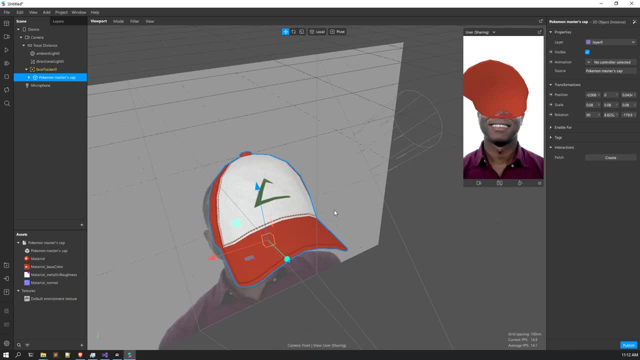 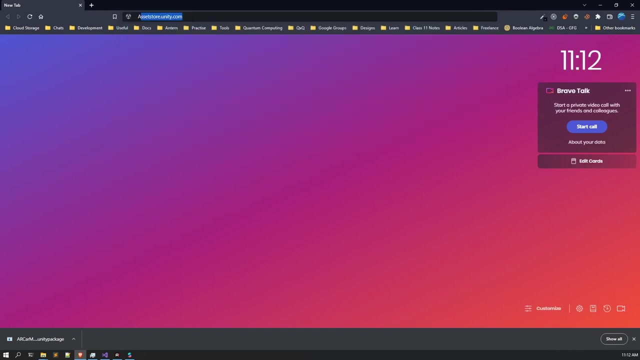 my left hand. we won't all right. that, uh, that is what i can say- is a occlusion. occlusion basically gives a more immersive experience. all right, to uh make it easier for you. all right, let's uh ar uh search for ar occlusion. let me uh get some image to uh make you understand. all right, 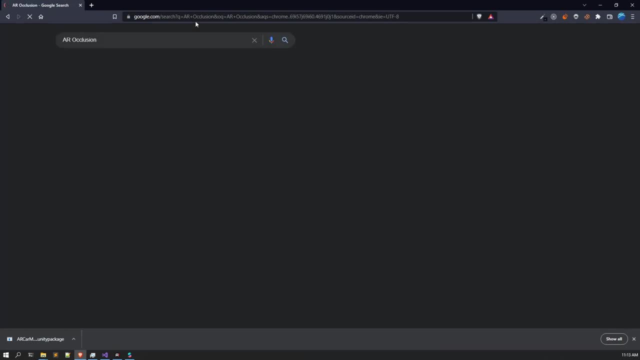 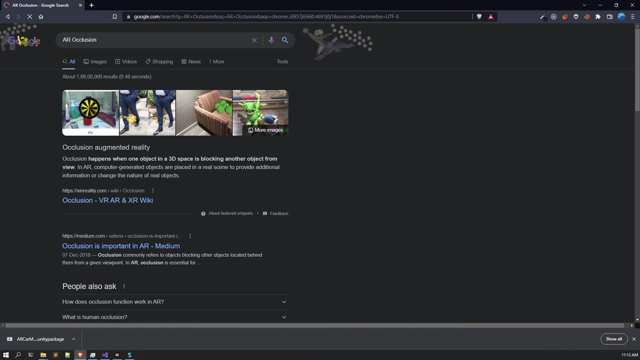 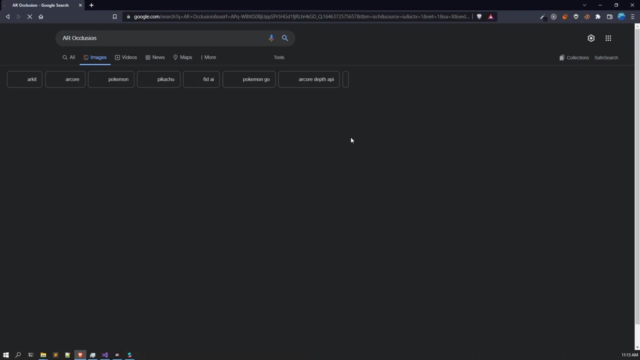 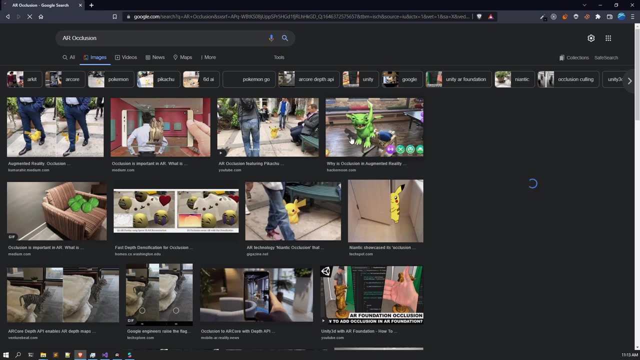 okay. so all right, yeah, here we go. we got, uh, one really good image. just give a few seconds. so here you can see in this image that, first of all, uh, the first, that that is the left side of the image, is non-occ, doesn't have any occlusion, all right, and you can see that the pikachu is like. 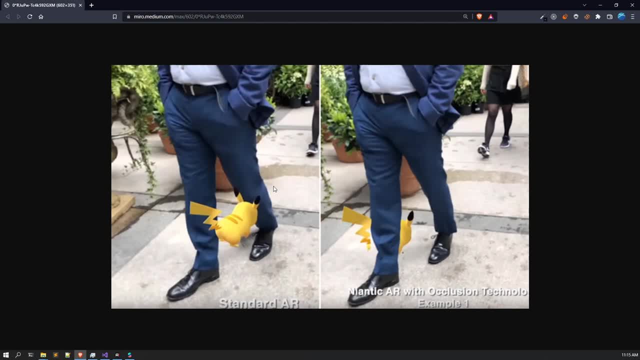 on top of, uh, his legs, so you can see that the pikachu is on top of his legs. so here you can see that the pikachu is, uh like, on top of his legs right, and that is not giving us a sense of immersion, or also it is not feeling realistic. 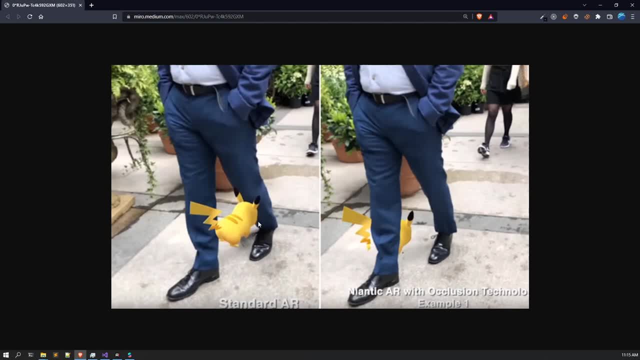 all right. but if we look at the second image, you would see, all right that the pikachu is behind his leg. all right, it's. it's not like overlapping the leg, it's behind the leg and that is what occlusion. is the person or the car in this in the first case? all right, this person doesn't have any. 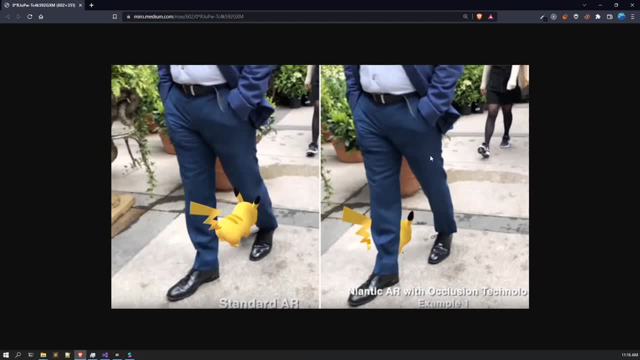 occlusion. but in the second case, the person, the person has an occluder all right on on his leg, so that's why he's able to hide this particular pikachu, all right. so i guess, uh, occlusion, the concept of occlusion is clear, all right. and if you're still confused about that, that's totally. 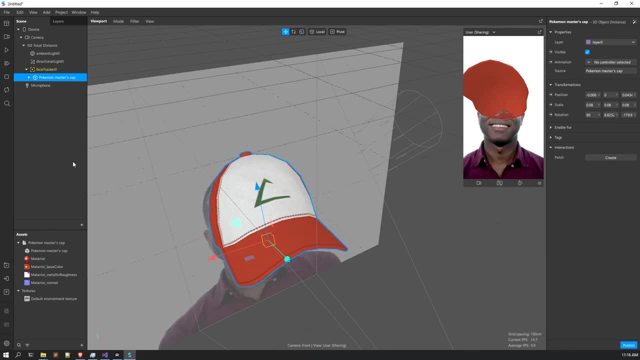 fine, uh, you can ask it in the comment section and if, even if you want, i can make a separate video on explaining occlusion. all right, you now, how would we achieve occlusion in uh spark here, right? so, first of all, there's uh, there's an. 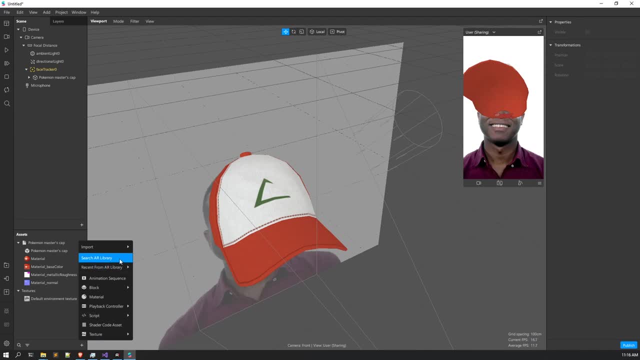 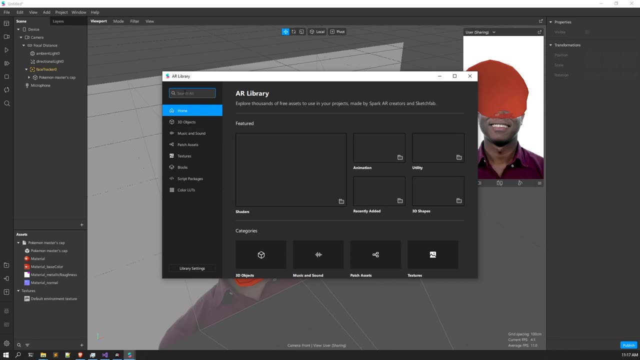 object actually called, uh uh, head occluder. all right, so what you have to do is, uh, go to the ar library and search for occluder it's, but it's given by spark ar only. uh, you would see that in the block section that is this second one, head occluder. click on it. all right, it's. 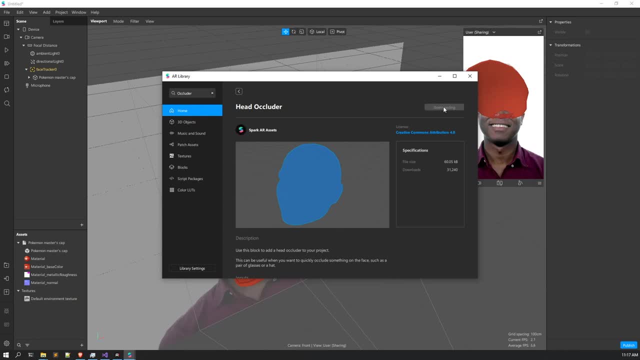 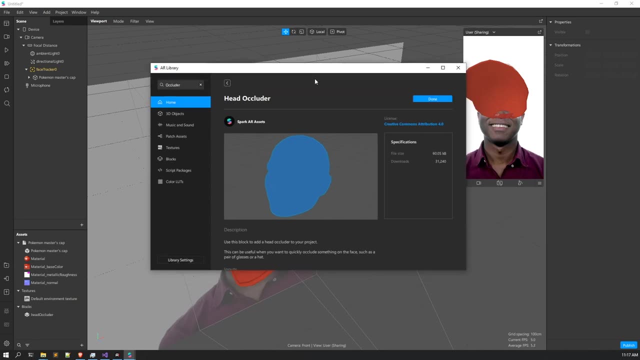 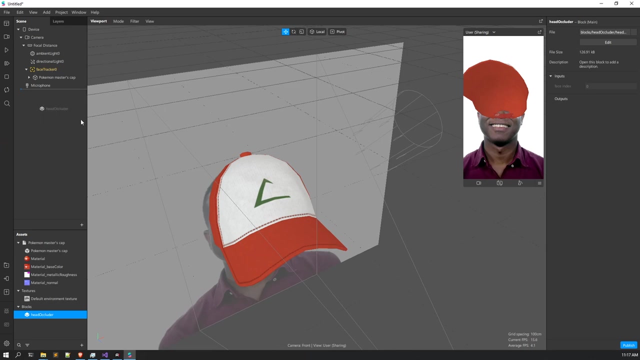 back to the block section and you can see that it's back to the block section and you can see by it's given by spark ar team. so click on import free and it will start downloading it and import it after it's downloaded. cool, so we have imported the head occluder. now what i want you to do is put this head occluder. 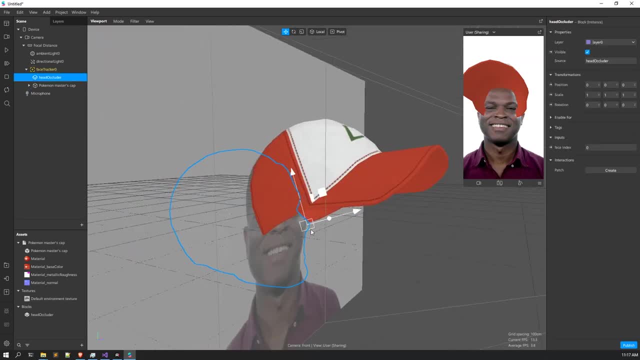 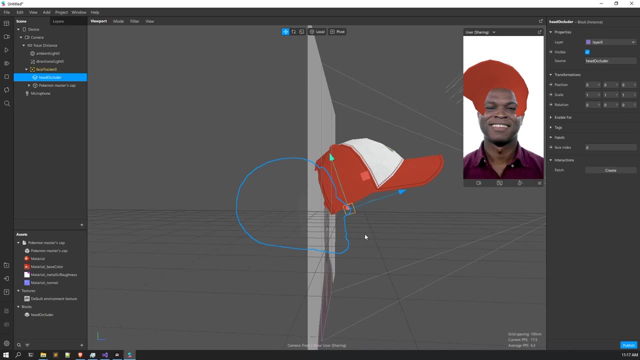 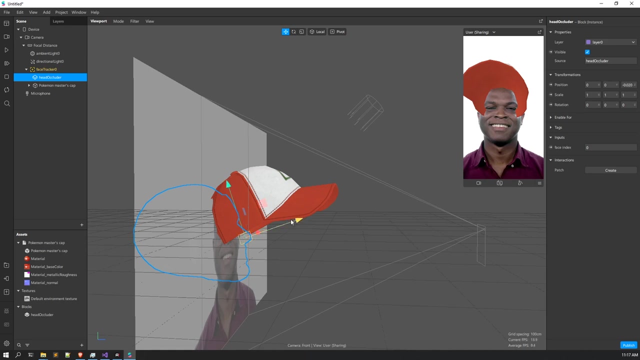 inside this head right means inside this face tracker. now you can see that the head occluder is, uh, the the means some portion of the cap is hidden right, and of course this is good. we are able to see the occlusion all right. now, uh, we have to adjust the cap right, so how would we do that? um, 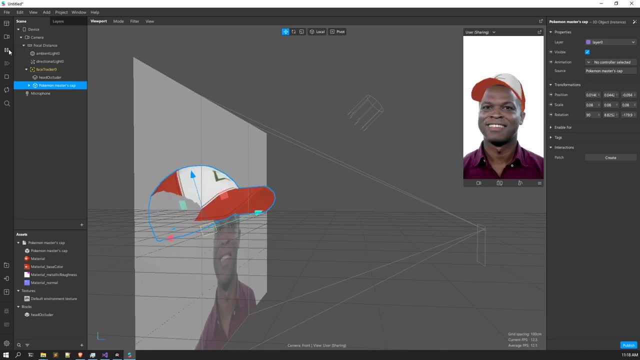 let's see: okay, cool. so can you see that uh occlusion is perfectly working. we are getting the uh occlusion is perfectly working. we are getting the uh occlusion is perfectly working. we are getting the 3d effect we wanted, right, isn't it? so uh occlusion is working perfectly fine now. 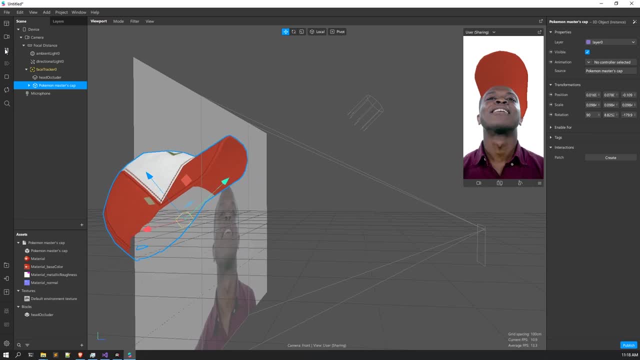 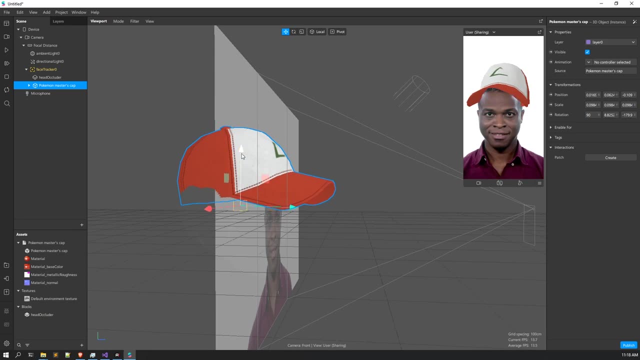 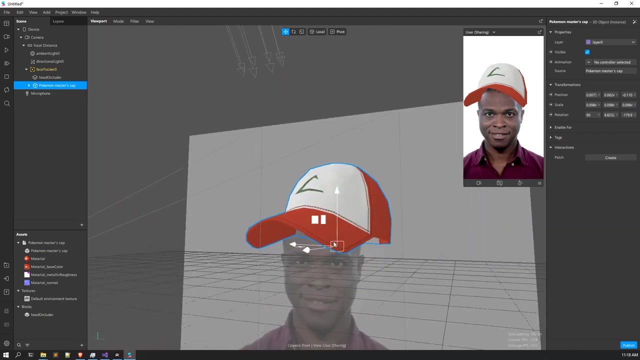 uh, you have to adjust the 3d model accordingly, all right, so that, uh, it fits the head. so that it fits. uh, actually it fits the head and you don't face any uh issues, right, so that's what i'm currently doing. it's a bit tedious process actually, but, uh, the results are going to be. 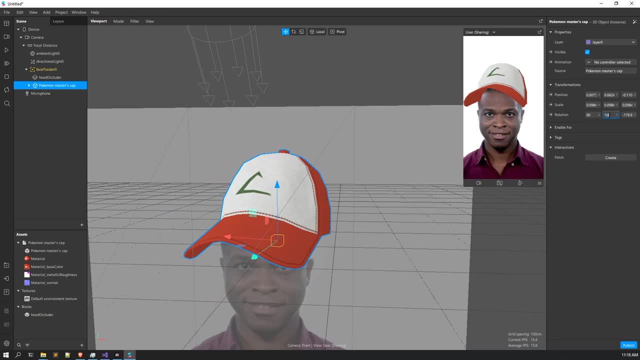 i'm currently doing. it's a bit tedious process actually, but uh, the results are going to be. you, the end result you would be getting is pretty good. you, the end result you would be getting is pretty good, just me. just let me get this cap straightened up. 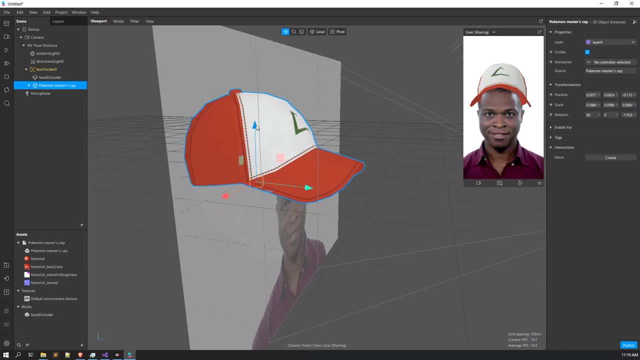 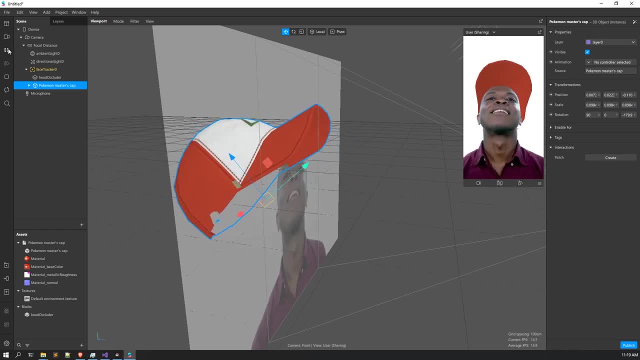 all right, a bit of gap on on the head. all right, a bit of gap on on the head. now just adjust it all right now. uh, now, just adjust it all right now. uh, now, just adjust it all right now. uh, this looks good. this looks pretty good. 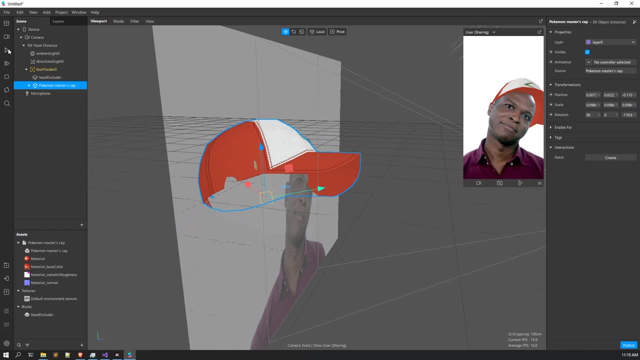 this looks good. this looks pretty good. this looks good, this looks pretty good. then it was previously, so you have to. then it was previously, so you have to. then it was previously, so you have to play. with all the play, with all the play, with all the 3d models. all right, all the occlusion. 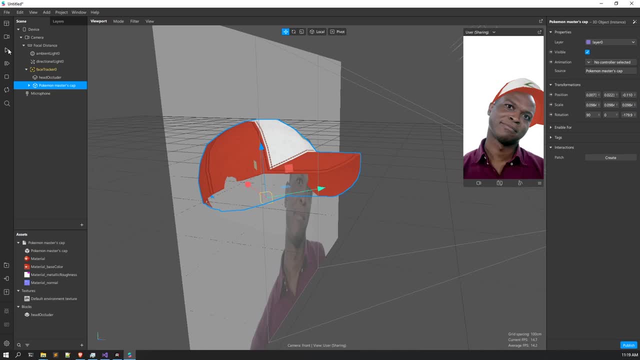 3d models. all right. all the occlusion 3d models all right. all the occlusion effects to effects, to effects, to get uh to the point you want, right to get. get uh to the point you want, right to get. get uh to the point you want, right to get to the final result you want. so it's a 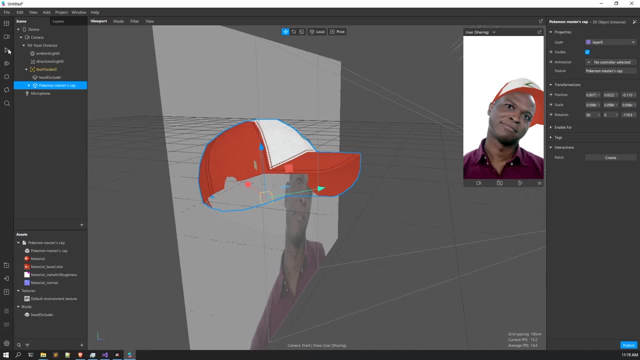 to the final result you want. so it's a to the final result you want. so it's a bit tedious process, but bit tedious process, but bit tedious process. but after you adjust it a bit, the outcomes, after you adjust it a bit, the outcomes, after you adjust it a bit, the outcomes looks really, really great. all right so. 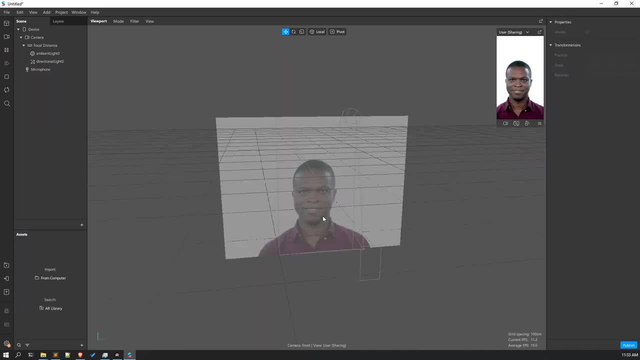 looks really really great, all right. so looks really really great, all right. so, uh, yeah, hey guys, so this is our last lecture. all hey guys, so this is our last lecture. all hey guys, so this is our last lecture, all right, right, right, in this lecture we are going to create a. 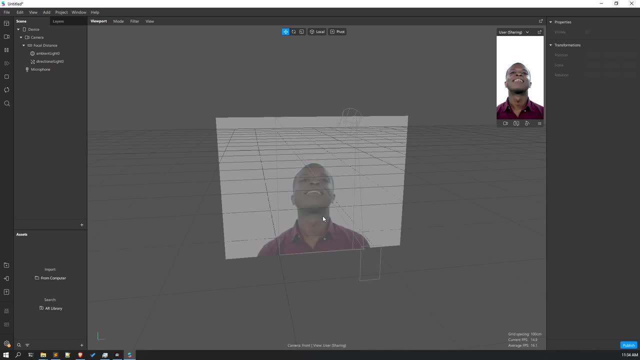 in this lecture, we are going to create a. in this lecture, we are going to create a very simple project, very simple project, very simple project: basic skills: we learned about spark, basic skills. we learned about spark, basic skills. we learned about spark here. all right see. here, all right see. 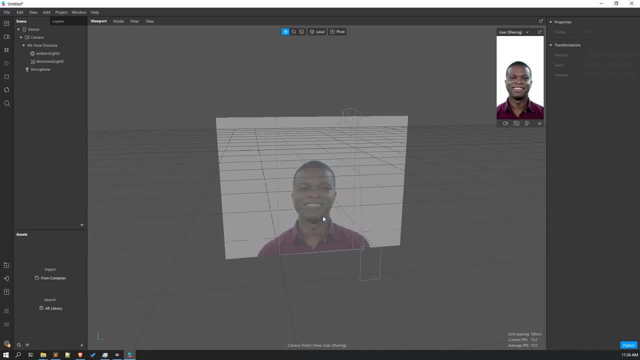 here. all right, see, i i'm going to admit that, uh, i haven't. i i'm going to admit that, uh, i haven't. i i'm going to admit that, uh, i haven't taught, taught, taught. uh, sparky are in much depth, all right. uh, sparky are in much depth, all right. 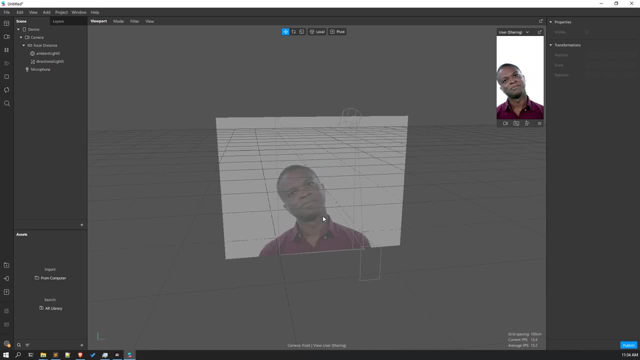 uh, sparky are in much depth. all right, because, because because i'm going to bring out another series, i'm going to bring out another series, i'm going to bring out another series. all right, totally on. sparky are all right. all right, totally on, sparky are all right. 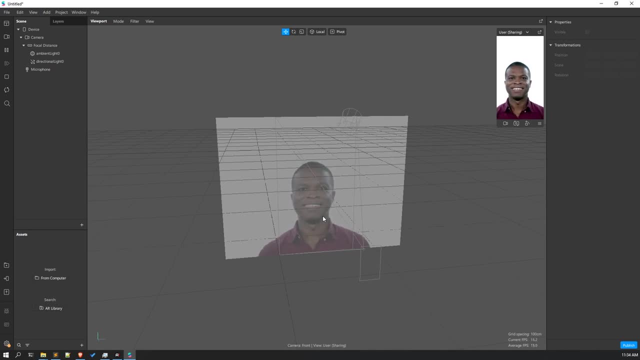 all right, totally on. sparky are all right. which will be? which will be? which will be covering sparky are in depth. the main idea covering sparky are in depth. the main idea covering sparky are in depth. the main idea already, the main motivation behind. already the main motivation behind. 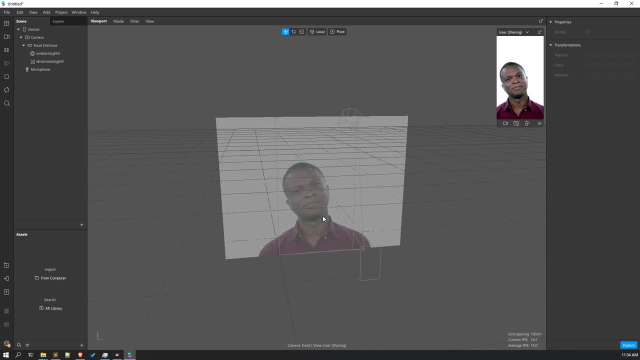 already. the main motivation behind putting sparky are the basics of sparky putting sparky are the basics of sparky putting sparky are the basics of sparky, are in the syllabus, are in the syllabus. are in the syllabus. the reason behind it was that i wanted i. 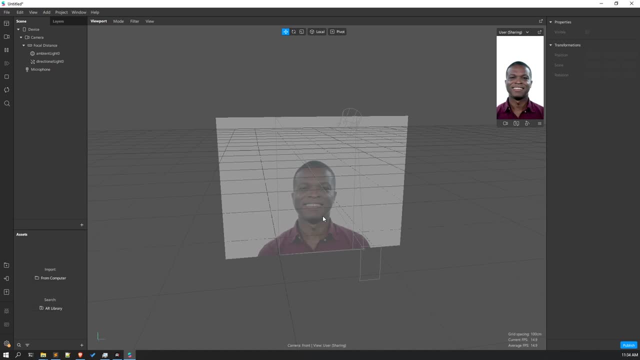 the reason behind it was that i wanted i. the reason behind it was that i wanted i wanted you guys to get wanted, you guys to get wanted, you guys to get excited about augmented reality, all excited about augmented reality, all excited about augmented reality. all right, uh, and. 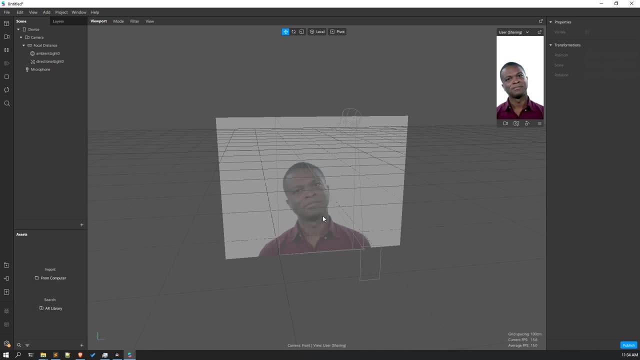 right uh and right uh, and i know many of you are active active on. i know many of you are active active on. i know many of you are active active on instagram, instagram, instagram. all right, i know many of you and you. all right, i know many of you and you. 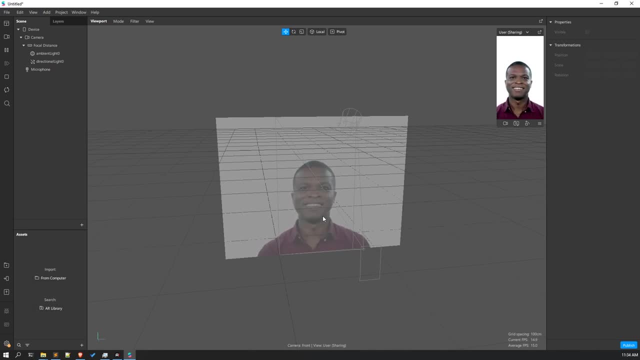 all right, i know many of you and you guys uh enjoy instagram. so why not guys uh enjoy instagram? so why not guys uh enjoy instagram? so why not make uh one filter for instagram, right? make uh one filter for instagram right? make uh one filter for instagram, right? so i i was, i was thinking that uh, it's. 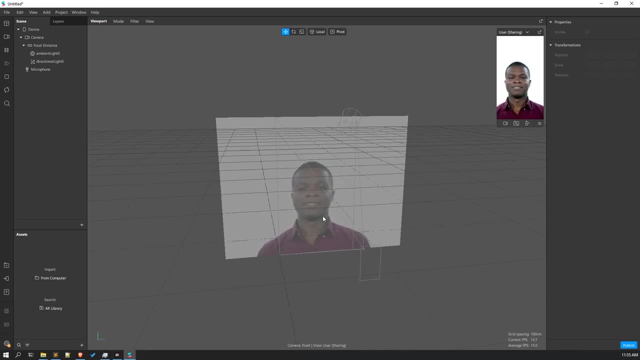 so i, i was. i was thinking that, uh, it's. so i, i was. i was thinking that, uh, it's going to excite you, and uh going to excite you, and uh going to excite you, and uh, i guess it did. so let's jump into the video and develop. 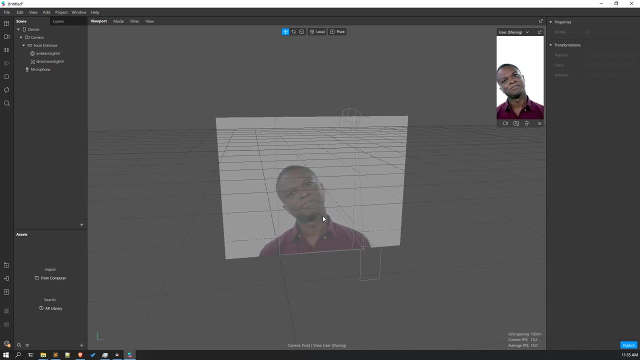 let's jump into the video and develop. let's jump into the video and develop our last project right and our last project right and our last project right. and i promise you all right one thing: i'm. i promise you all right one thing. i'm. i promise you all right one thing. i'm going to promise you that. 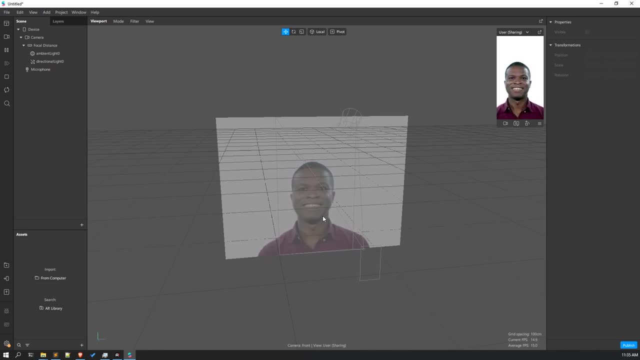 going to promise you that. going to promise you that more series like this, all right, more more series like this, all right, more more series like this, all right, more better than this, are going to come in better than this are going to come in, better than this are going to come in near future. all right, i'm improving. 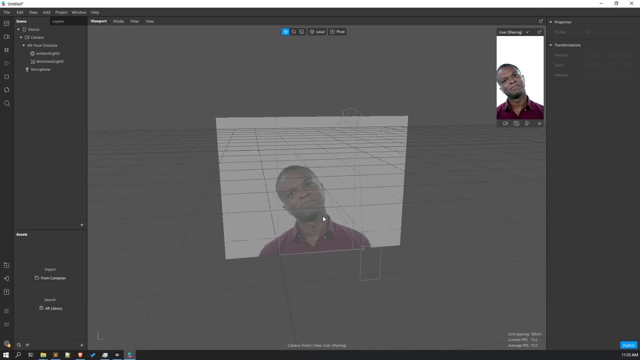 near future. all right, i'm improving near future. all right, i'm improving myself every day. all right, i'm going to myself every day. all right, i'm going to myself every day. all right, i'm going to bring out videos on virtual reality. i'm bring out videos on virtual reality. i'm 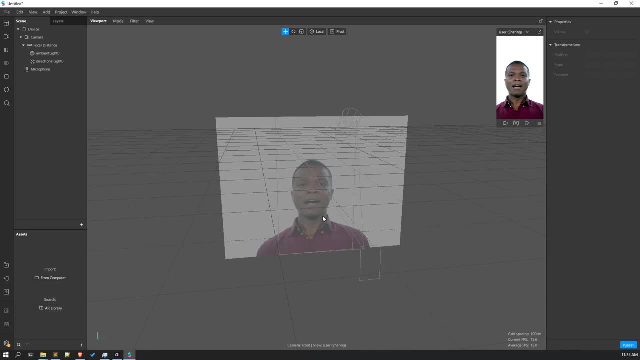 bring out videos on virtual reality. i'm going to bring videos on augmented and going to bring videos on augmented and going to bring videos on augmented and mixed reality. all right, so make sure to mixed reality. all right, so make sure to mixed reality. all right, so make sure to subscribe this channel. 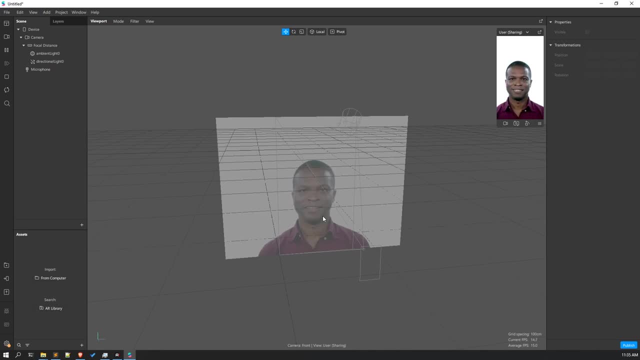 subscribe this channel. subscribe this channel, all right. so make sure to subscribe this. all right, so make sure to subscribe this channel so you don't miss any videos channel. so you don't miss any videos channel. so you don't miss any videos. all right, and uh, very soon i'm going to 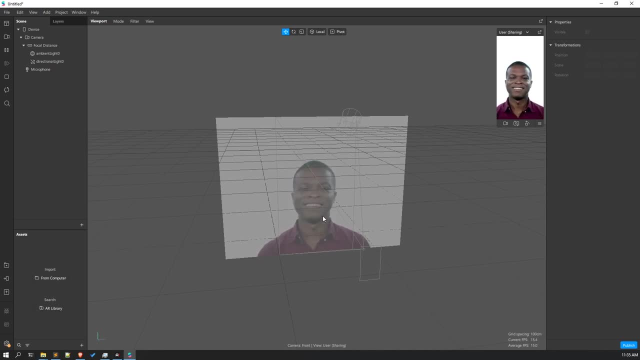 all right and uh, very soon i'm going to. all right and uh, very soon i'm going to launch. all right, uh, most probably in the launch. all right, uh, most probably in the launch. all right, uh, most probably in the month of april i'm going to launch a. 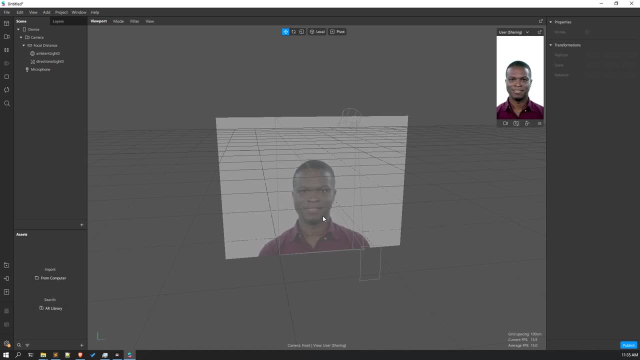 month of april i'm going to launch. a month of april i'm going to launch a course called exhaust 01. all right, it course called exhaust 01, all right. it course called exhaust 01. all right, it would be a paid course, all right. so the 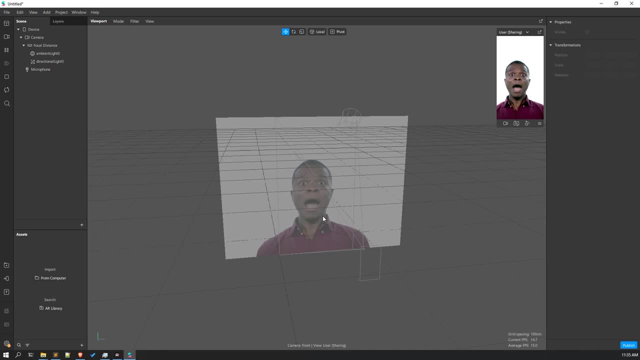 would be a paid course, all right. so the would be a paid course, all right. so the course would be very affordable. all course would be very affordable. all course would be very affordable. all right for, so that everyone can right for, so that everyone can right for, so that everyone can learn from that course. and uh, 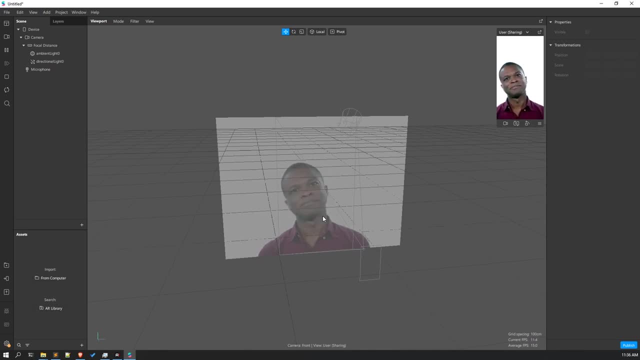 learn from that course and uh, learn from that course. and uh, the course would be launching at my. the course would be launching at my. the course would be launching at my startup. that is startup. that is startup that is entered. all right. so if you want, you can. 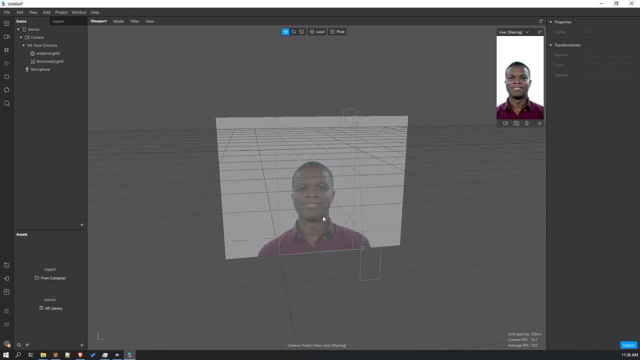 entered, all right. so if you want, you can entered, all right. so if you want, you can, and you, you guys, can enroll in that, and you, you guys, can enroll in that, and you, you guys, can enroll in that course. and, uh, i'm going to announce that. 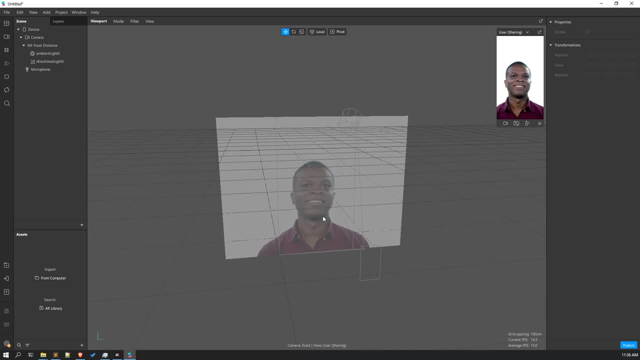 course. and uh, i'm going to announce that course. and uh, i'm going to announce that i have announced that uh course in this. i have announced that uh course in this. i have announced that uh course in this video. so video, so video. so make sure, all right, if you want to learn. 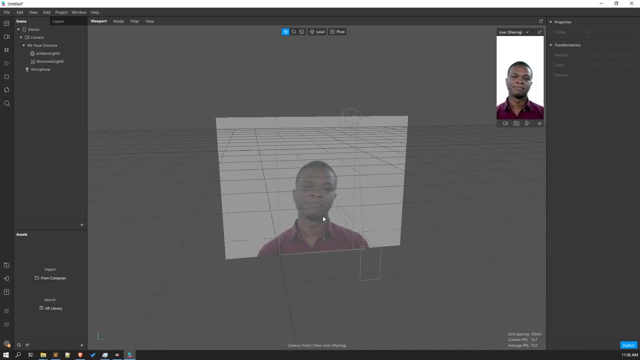 make sure. all right. if you want to learn, make sure all right. if you want to learn more in depth, all right. i have covered more in depth. all right, i have covered more in depth. all right, i have covered very, very, very, very in-depth concepts of augmented virtual. 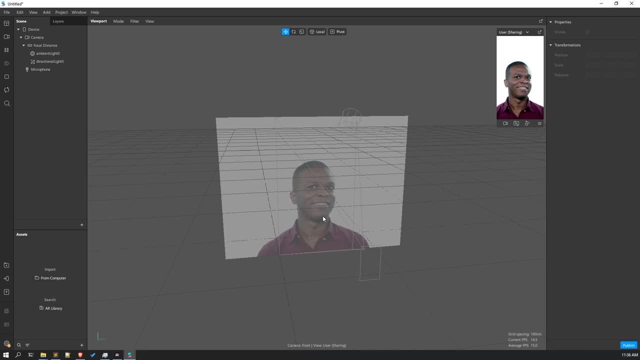 in-depth concepts of augmented virtual. in-depth concepts of augmented virtual and mixed reality in that and mixed reality in that and mixed reality in that course all right. there are concepts- that course all right. there are concepts- that course all right. there are concepts that no one going to teach you. 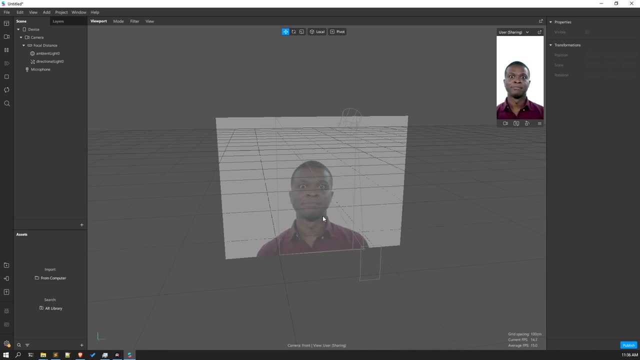 no one going to teach you. no one going to teach you in any of the course around, all right, no, in any of the course around, all right. no, in any of the course around, all right. no one is going to. one is going to. one is going to teach you those concepts i have included. 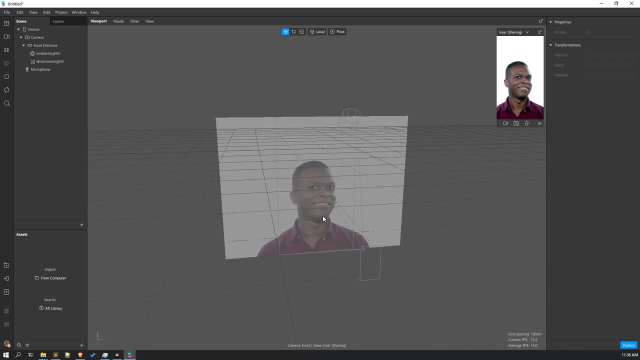 teach you those concepts i have included. teach you those concepts. i have included those concepts because they are very those concepts, because they are very those concepts, because they are very important. all right, i have included important. all right, i have included important. all right, i have included maths required for uh, ar and vr: all. 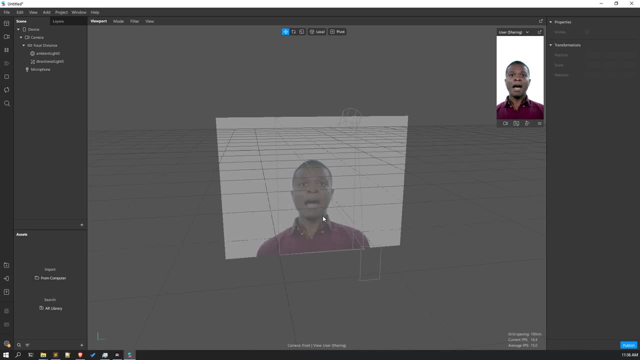 maths required for uh, ar and vr. all maths required for uh, ar and vr. all right, that is 3d maths. so right, that is 3d maths. so right, that is 3d maths. so make sure all right to make sure, all right. to make sure all right to visit that course at least once, all right. 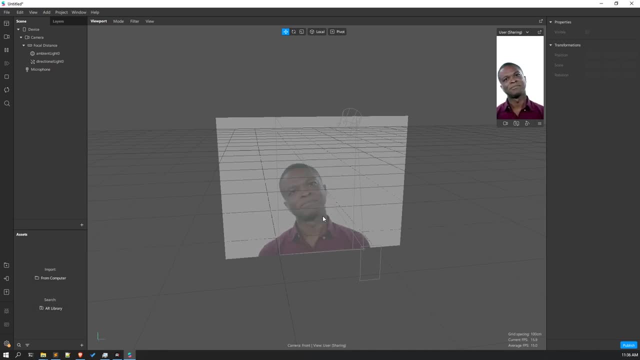 visit that course at least once, all right. visit that course at least once, all right. and if you feel like joining the course, and if you feel like joining the course, and if you feel like joining the course, if you want to pursue uh, augmented, if you want to pursue uh, augmented. 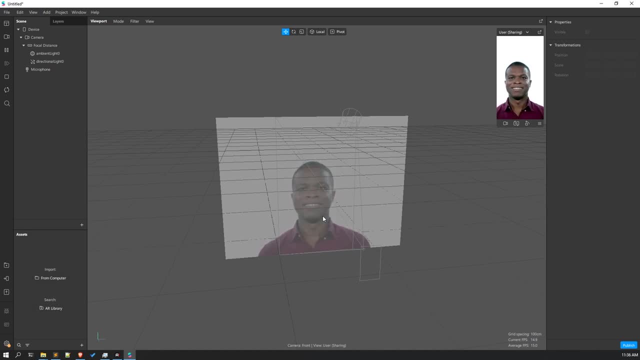 if you want to pursue, uh, augmented reality, virtual reality and mixed reality, virtual reality and mixed reality, virtual reality and mixed reality- as a career, then you can surely reality as a career, then you can. surely reality as a career, then you can surely join that course we are going to. 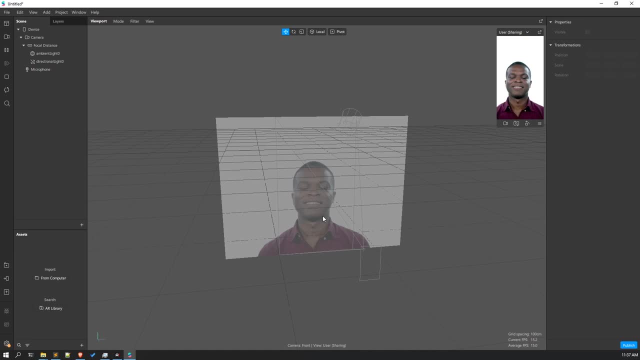 join that course. we are going to join that course. we are going to develop multiple projects. we are going to develop multiple projects. we are going to develop multiple projects. we are going to get in depth of the sdks- all right, we get in depth of the sdks, all right, we. 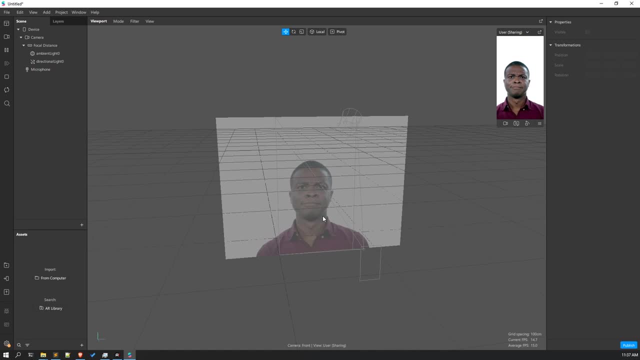 get in depth of the sdks. all right, we are going to get in-depth knowledge of. are going to get in-depth knowledge of. are going to get in-depth knowledge of those sdks, like those sdks, like those sdks like reforias or ar code, that is, ar. 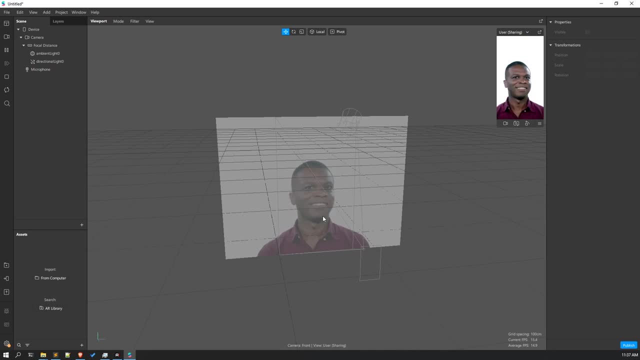 reforias or ar code, that is ar reforias or ar code that is ar foundation, foundation, foundation. then of course spark ar we are going to, then of course spark ar we are going to, then of course spark ar we are going to going to go into the. 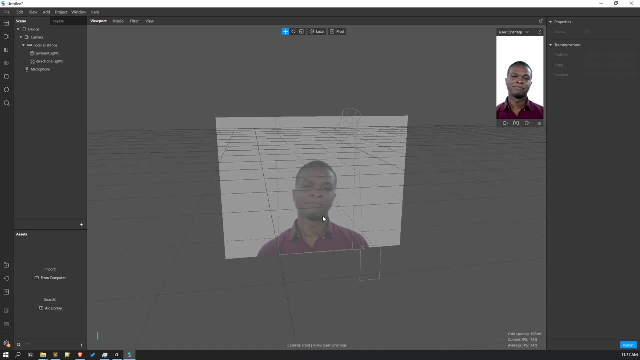 going to go into the, going to go into the depth of spark here, depth of spark here, depth of spark here would be exploring how to code in spark, would be exploring how to code in spark, would be exploring how to code in spark and all those and all those. 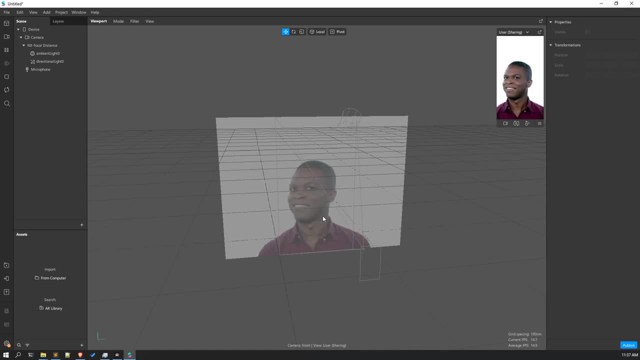 and all those very important things, all right. so if you very important things, all right. so if you very important things, all right. so if you want, you can enroll in that course, want you can enroll in that course, want you can enroll in that course. so, so, so also one more thing, all right. 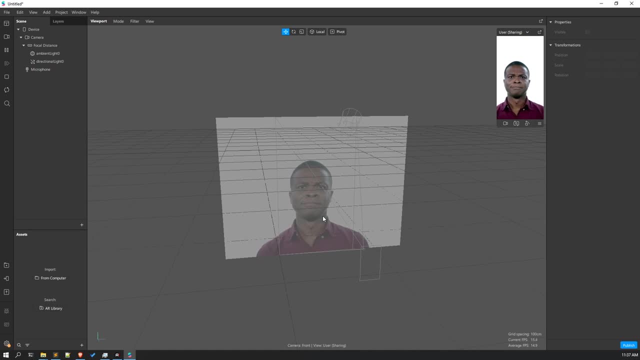 also one more thing. all right, also one more thing. all right, join our discord server. all right, join. join our discord server. all right, join. join our discord server. all right, join anton's discord server. there are many anton's discord server. there are many anton's discord server. there are many experts in there. all right, who can help? 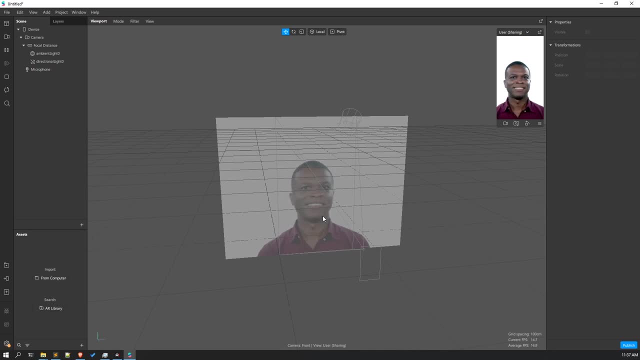 experts in there, all right. who can help? experts in there, all right. who can help you? i am in there, all right. so if you you, i am in there all right. so if you you, i am in there, all right. so if you have any doubt in near future, you can. 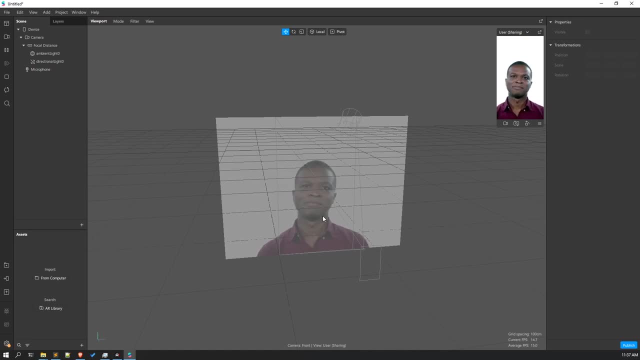 have any doubt in near future. you can have any doubt in near future. you can ask me in there, all right, and also you ask me in there, all right, and also you ask me in there, all right. and also you can connect with me on linkedin all. 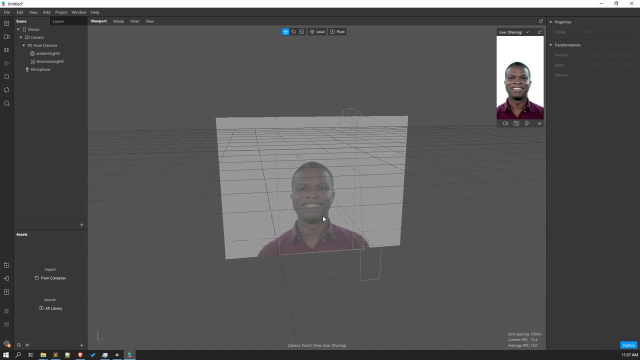 can connect with me on linkedin. all can connect with me on linkedin. all right, you can follow me on instagram. so right, you can follow me on instagram. so right, you can follow me on instagram. so here, all the links will be down below. here, all the links will be down below. 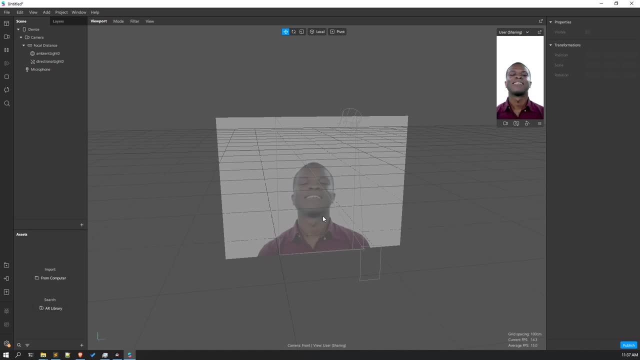 here. all the links will be down below in the description and all the materials in the description and all the materials in the description and all the materials all right that i have used during the all right that i have used during the all right that i have used during the course, all the project assets. 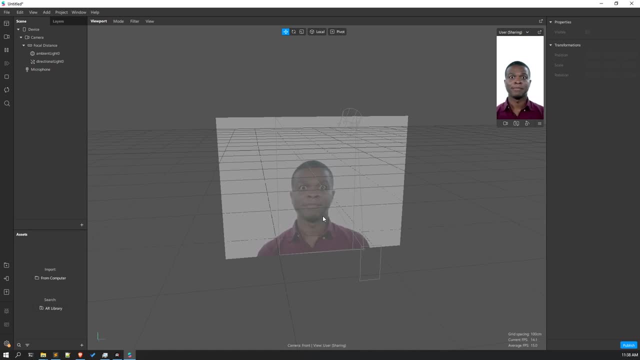 course, all the project assets. course, all the project assets. all those things will be available. uh, on, all those things will be available. uh, on, all those things will be available. uh, on the website. all right, that is ar course the website. all right, that is ar course the website. all right, that is ar course dot or netify dot app. all right, it would. 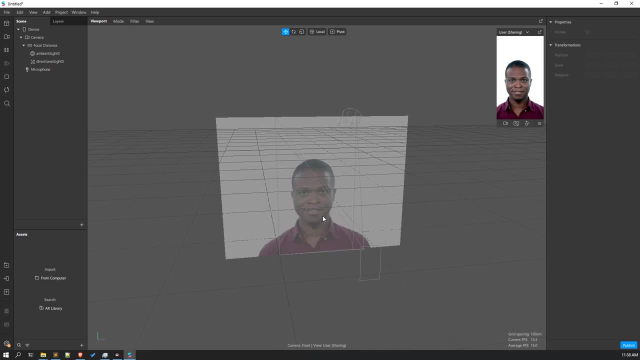 dot or netify dot app. all right, it would dot or netify dot app. all right, it would be available in be available in be available in the website so you can get all the assets. the website so you can get all the assets. the website so you can get all the assets from there. all right, and the spark. 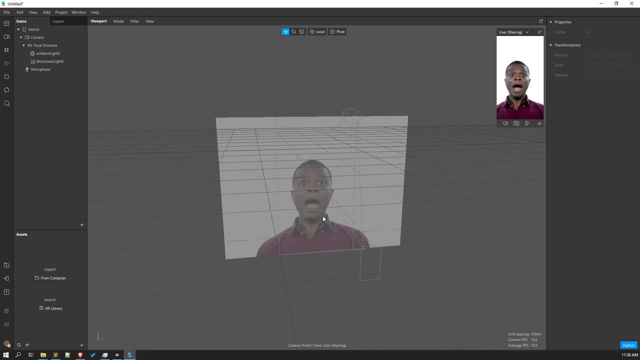 from there, all right, and the spark from there, all right. and the spark air assets you can get from air assets you can get from air assets you can get from the air library on all right. so the air library on all right, so the air library on all right. so yeah, without any further ado. 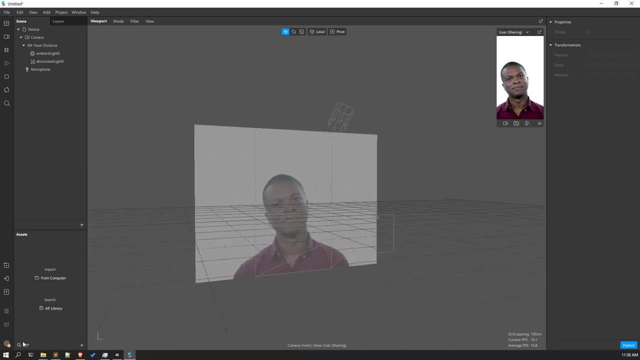 yeah, without any further ado, yeah, without any further ado, let's get going, let's get going, let's get going right. so the very first thing is uh click right. so the very first thing is uh click right. so the very first thing is uh click on this project properties. 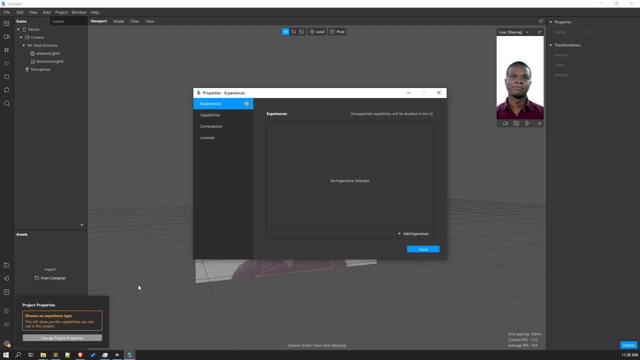 on this project properties. on this project properties. click on change project properties. click on change project properties. click on change project properties. all right, make sure you do that. and in all right, make sure you do that. and in all right, make sure you do that. and in that, click on add experience. all right. 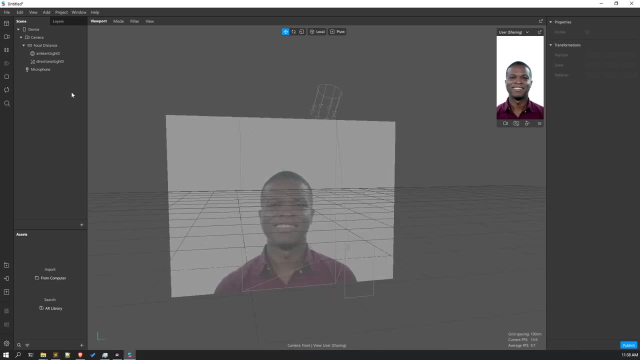 that click on add experience, all right. that click on add experience all right on our mobile and all those on our mobile and all those on our mobile and all those like on our instagram, uh, like on our instagram, uh, like on our instagram, uh, and all those portions, right. 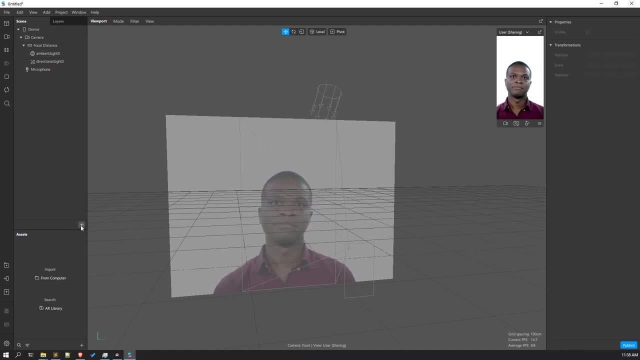 and all those portions right and all those portions right. so now the very first thing is: i want so now, the very first thing is: i want. so now, the very first thing is: i want you to add a head tracker, you to add a head tracker, you to add a head tracker- oh sorry, face tracker, all right. so 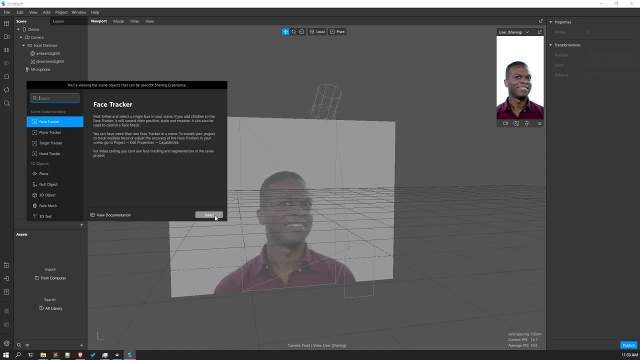 oh sorry, face tracker all right. so, oh sorry, face tracker all right. so click on this plus icon all right and click on this plus icon all right. and click on this plus icon all right and click on this face tracker and click on. click on this face tracker and click on. 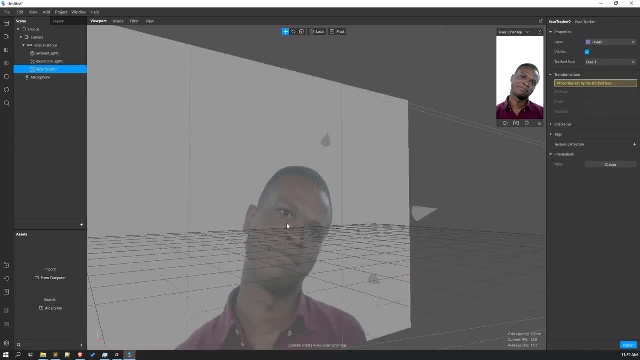 click on this face tracker and click on insert all right, insert, all right, insert all right. so here you can see our anchor has. so here you can see our anchor has. so here you can see our anchor has appeared and that anchor is moving with. appeared and that anchor is moving with. 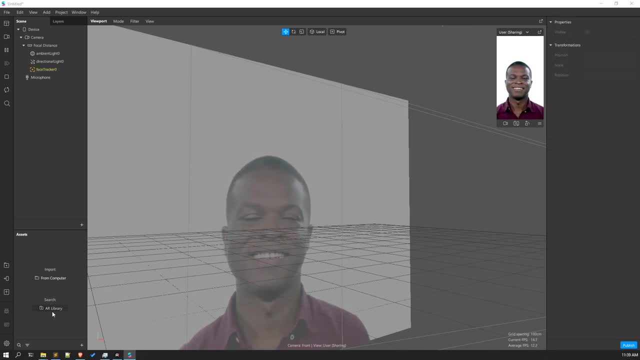 appeared and that anchor is moving with the face, the face, the face. now i want you to add some assets, all now. i want you to add some assets, all now. i want you to add some assets. all right, i want you to add some assets. the right. i want you to add some assets, the. 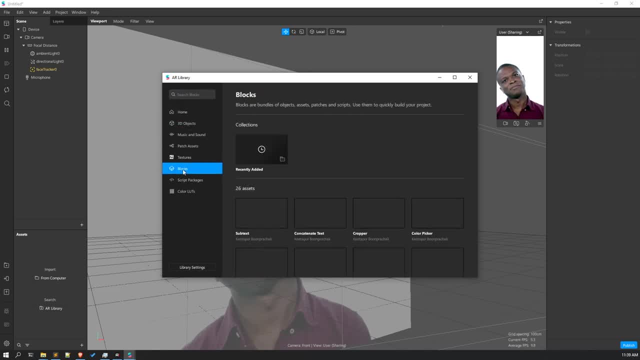 right, i want you to add some assets. the very first asset is very first asset is very first asset is: uh go to the blocks. all right, i guess it uh go to the blocks. all right, i guess it uh go to the blocks all right. i guess it was in the blocks only, right. 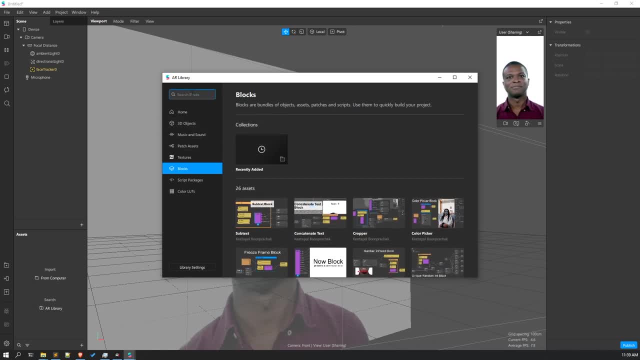 was in the blocks, only right was in the blocks, only right. i don't exactly remember. actually let's. i don't exactly remember, actually let's. i don't exactly remember, actually let's. let's search for it. let's search for it, let's search for it. head occluder. 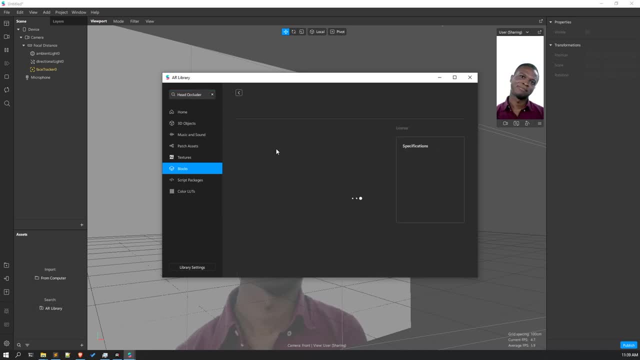 all right. oh uh okay, yeah, all right. oh uh okay, yeah, all right. oh uh okay, yeah, here we got it all right. so make sure to here we got it all right. so make sure to here we got it all right. so make sure to get the head occluder, that is. 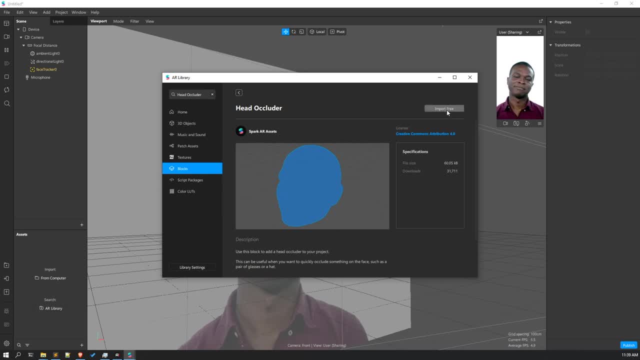 get the head occluder. that is, get the head occluder that is provided by the sparky assets, only all provided by the sparky assets, only all provided by the sparky assets, only all right and right and right and click on import it will dump, it will. 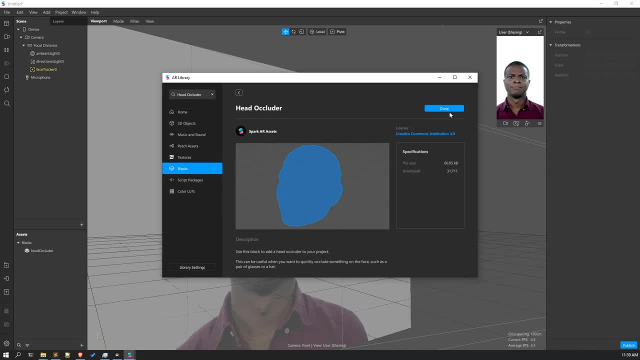 click on import, it will dump it. will click on import, it will dump. it will start downloading it. start downloading it. start downloading it all right. and after it's downloaded, all right. and after it's downloaded all right, and after it's downloaded, click on done. click on done. 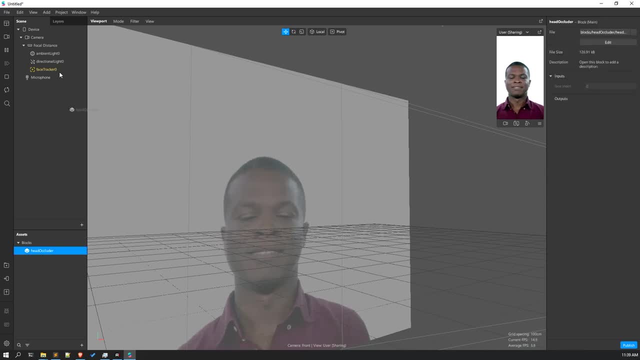 click on done and you know what to do. you just, and you know what to do. you just and you know what to do. you just place this head occluder inside of place, this head occluder inside of place, this head occluder inside of the face tracker. 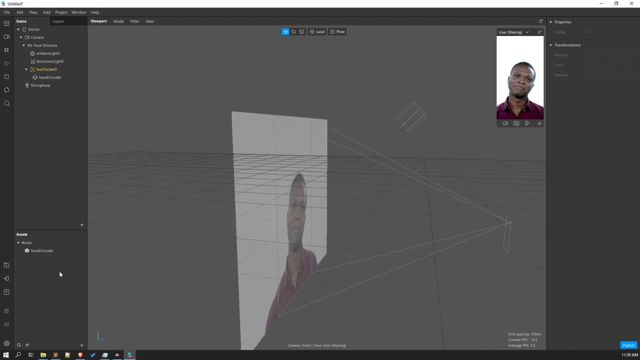 the face tracker. the face tracker- all right. so here we got our head all right. so here we got our head all right. so here we got our head. occluder. now we have to add some more occluder. now we have to add some more occluder. now we have to add some more asset, that is. 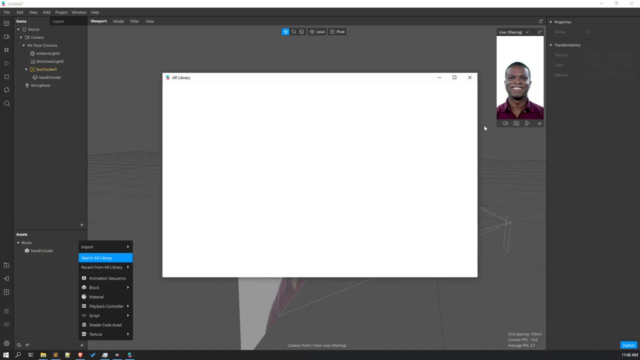 asset. that is asset. that is plus. click on this plus icon, then click plus. click on this plus icon, then click plus. click on this plus icon. then click on search ar library, on search ar library, on search ar library. all right, and here we'll be adding our. 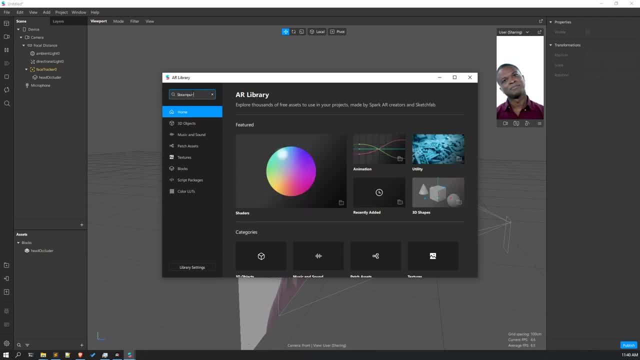 all right, and here we'll be adding our all right, and here we'll be adding our glasses. that is search for steam punk glasses. that is search for steam punk glasses. that is search for steam punk glasses, glasses, glasses. all right, so all right, so all right. so here you will be, getting this. uh. 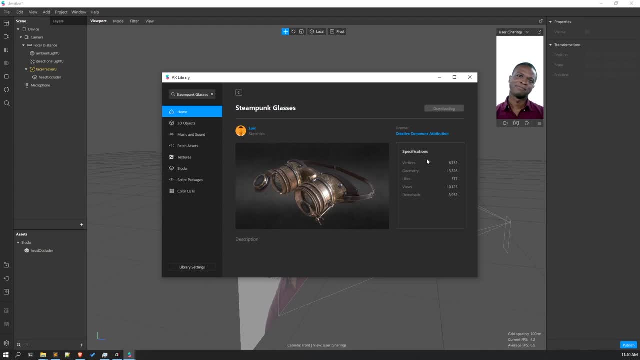 here you will be getting this, uh. here you will be getting this, uh, particular glass. so i'm just going to particular glass. so i'm just going to particular glass, so i'm just going to import it, import it, import it, all right. so it's going to take some. 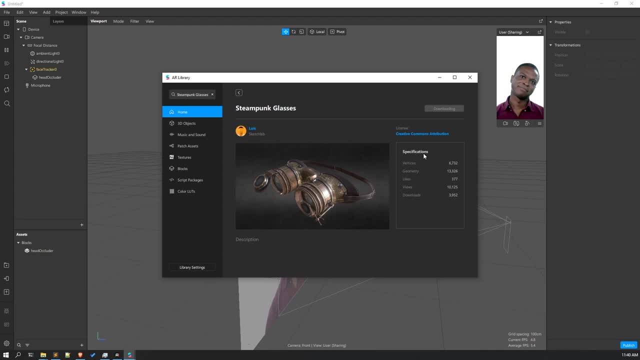 all right, so it's going to take some. all right, so it's going to take some amount of time to download and import. amount of time to download and import. amount of time to download and import the model, the model, the model, uh model. till then, all right, make sure. 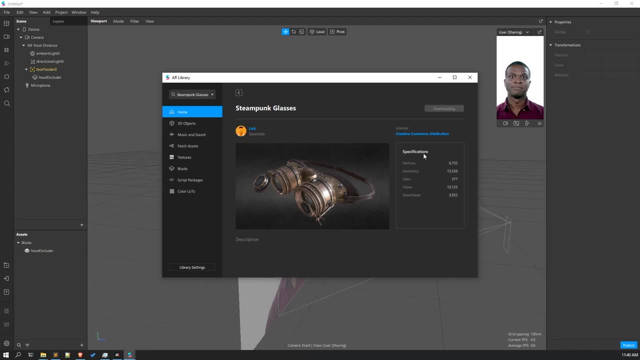 uh, model till then. all right, make sure, uh, model till then. all right, make sure, uh, you subscribe the channel. all right, uh, you subscribe the channel. all right. uh, you subscribe the channel. all right, make sure you subscribe the channel for. make sure you subscribe the channel for. 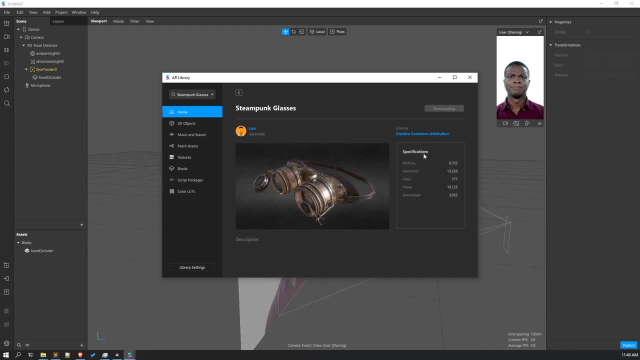 make sure you subscribe the channel for more, more, more uh videos. all right on augmented uh videos. all right on augmented uh videos. all right on augmented virtual and mixed reality. if you virtual and mixed reality, if you virtual and mixed reality, if you want to make a career in in this domain. want to make a career in in this domain, want to make a career in in this domain, and i'm going, i'm sure you're going to, and i'm going, i'm sure you're going to and i'm going, i'm sure you're going to, like. 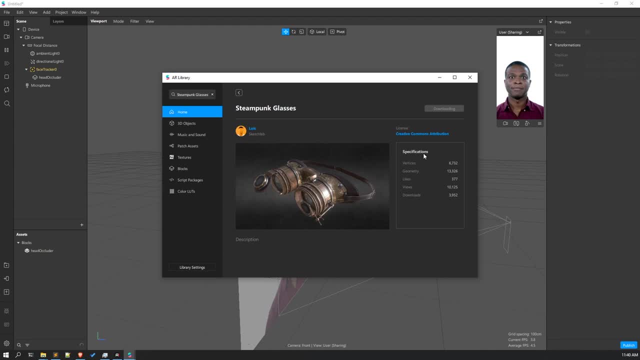 like. like how this domain is like. i love this how this domain is like. i love this how this domain is like. i love this domain for domain for domain for. truly like this is one of my favorite. truly like this is one of my favorite. truly like this is one of my favorite domain in computer science. 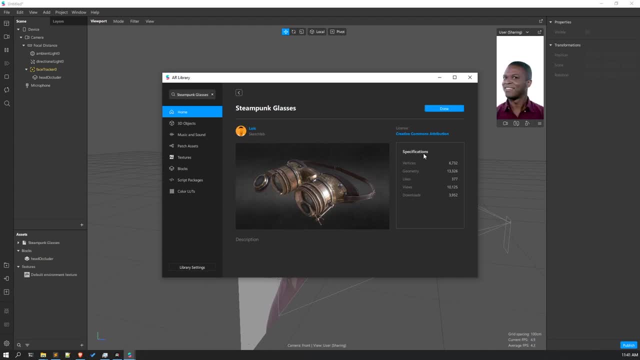 domain in computer science. domain in computer science. so just wait for a few seconds, and it so just wait for a few seconds, and it so just wait for a few seconds and it would be downloaded, would be downloaded, would be downloaded. so now our asset is. so now our asset is. 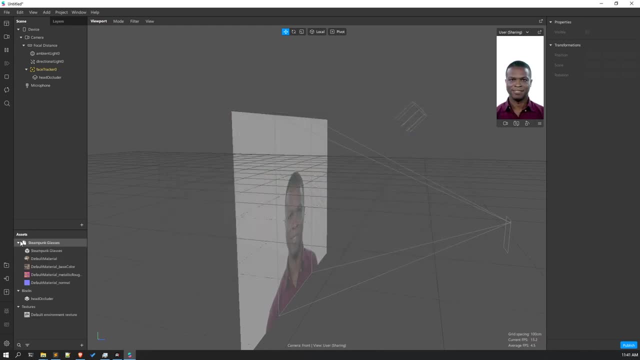 so now our asset is loaded right now. the very first thing i loaded right now, the very first thing i loaded right now, the very first thing i want you to do is want you to do. is want you to do is because this thing will make our you. 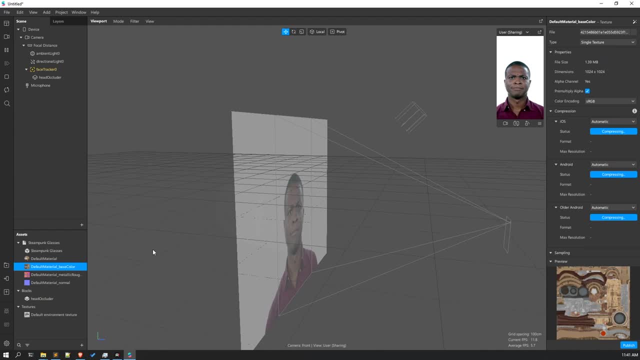 because this thing will make our you, because this thing will make our you, know sparky or slow, know sparky or slow, know sparky or slow, all right. so what i want you to do is go, all right, so what i want you to do is go. 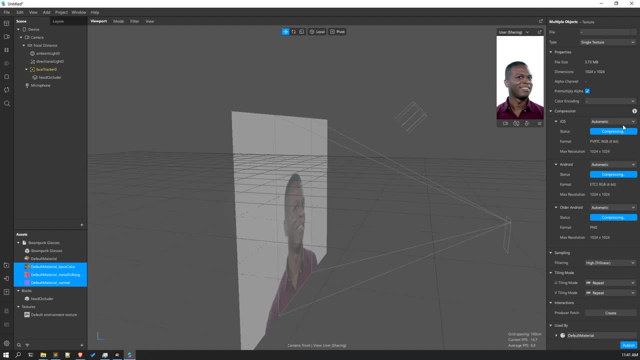 all right. so what i want you to do is go in there, all right, select all the assets in there. all right, select all the assets in there. all right, select all the assets right in here, right in here, right in here, and uh and uh and uh. make sure that the compression is set to. 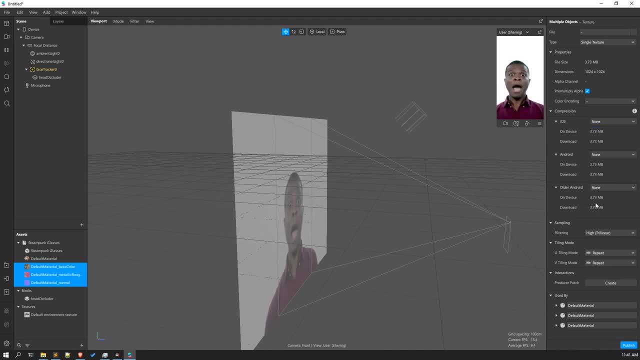 make sure that the compression is set, to make sure that the compression is set to none as of now. none as of now, none as of now. all right, all right, all right. why? see here, you can see the size is. why see here, you can see the size is. 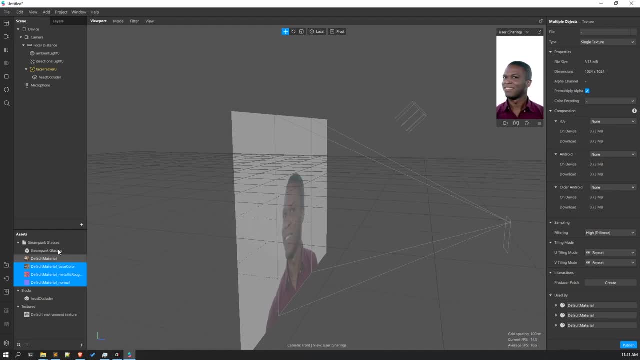 why see? here you can see the size is really big, all right, and really big, all right, and really big, all right. and of course, uh, spark, uh when you will be of course, uh, spark, uh, when you will be of course, uh, spark, uh when you will be launching this filter. 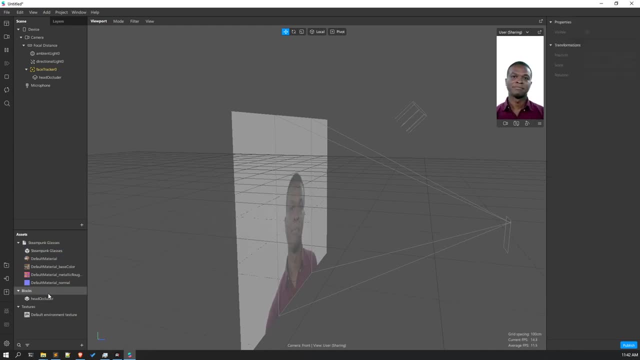 launching this filter. launching this filter, sparkkr won't be accepting it. so that's sparkkr won't be accepting it. so that's sparkkr won't be accepting it. so that's why- why? why you have to compress this filter after. you have to compress this filter after. 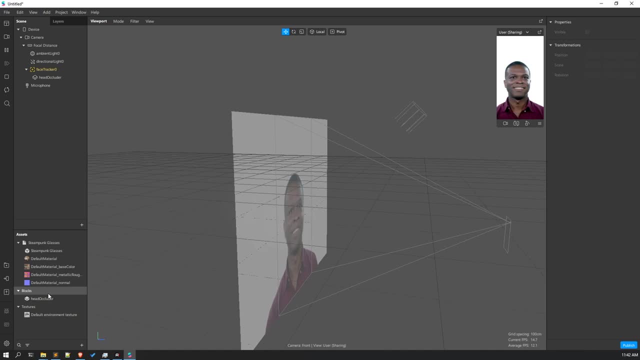 you have to compress this filter after you are done with all the you know. you are done with all the you know. you are done with all the you know. done with all the spark means development. done with all the spark means development. done with all the spark means development of your filter. all right, uh, i always. 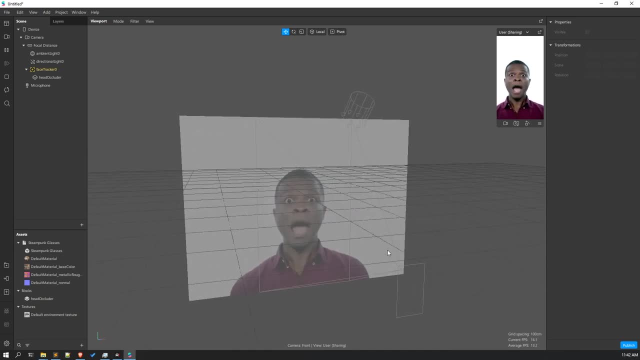 of your filter. all right, uh, i always of your filter, all right, uh, i always do this, so it, it do this, so it, it do this, so it it. like i compress these all the materials, like i compress these, all the materials, like i compress these all the materials after the development is done, because 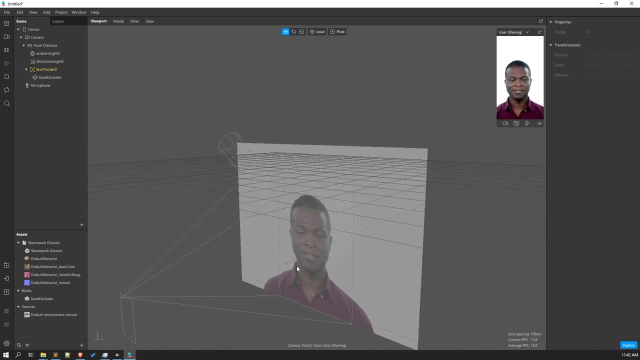 after the development is done, because, after the development is done, because that saves a lot of time for me, that saves a lot of time for me. that saves a lot of time for me, uh, like it doesn't interrupt my, uh, like it doesn't interrupt my, uh, like it doesn't interrupt my development. all right, the development of 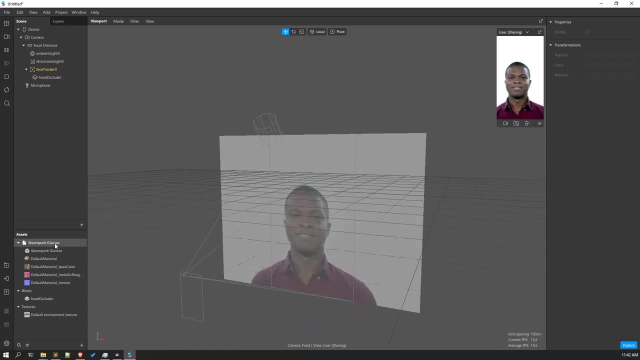 development, all right, the development of development, all right. the development of the filters, the filters, the filters. right now, what you have to do is fairly right now. what you have to do is fairly right now. what you have to do is fairly simple, simple, simple. drag and drop this object. all right, make. 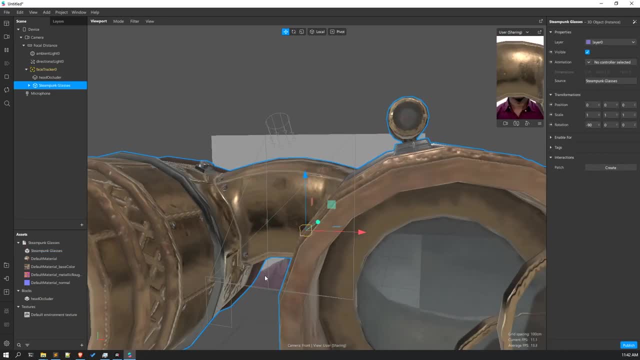 drag and drop this object all right. make drag and drop this object all right. make it a child of the face tracker. so here you can see it's. you know really so. here you can see it's. you know really. so here you can see it's. you know, really big. 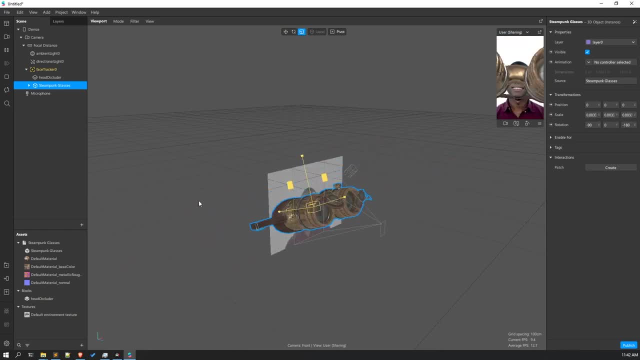 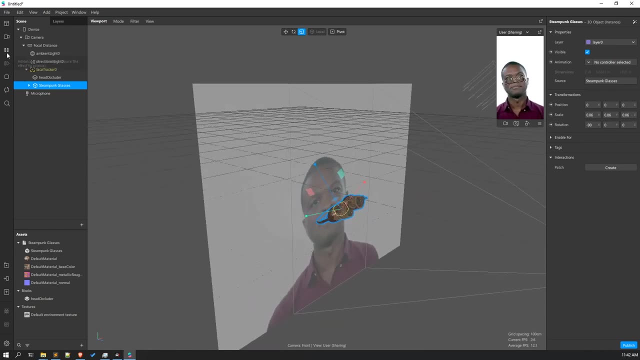 big, big, right. so it's time for us to make it small, make it small, make it small, okay, okay, okay. first of all, you know he's moving really. first of all, you know he's moving really. first of all, you know he's moving really fast. so i, of course, don't want that. so fast. so i of course don't want that so fast. so i of course don't want that. so now, what i'm going to do is i'm going. now, what i'm going to do is i'm going. now, what i'm going to do is i'm going to. you know. 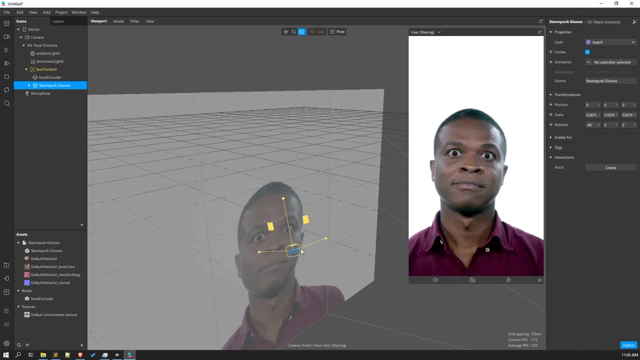 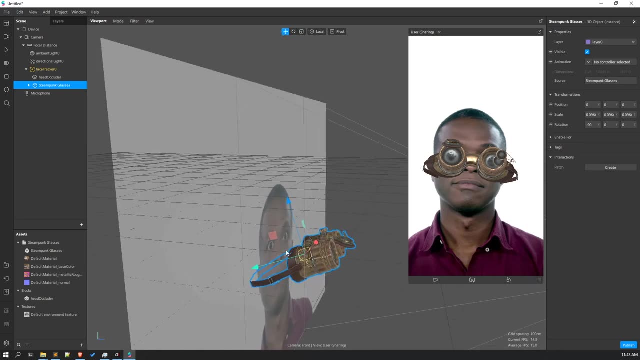 to you know, to you know: all right, okay, all right, okay, all right, okay. big mistake now. big mistake now. big mistake now. all right, okay, cool, all right, okay, cool. all right, okay, cool, very cool now. very cool now, very cool now. uh, you have to adjust this, you know. 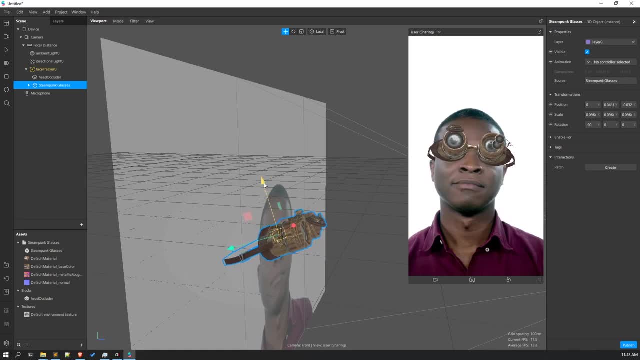 uh, you have to adjust this, you know. uh, you have to adjust this, you know, adjust, adjust this to his face right now. let's see: uh-huh, uh-huh, uh-huh. yeah, this this looks pretty good. yeah, this, this definitely looks uh good. yeah, this this definitely looks uh good. 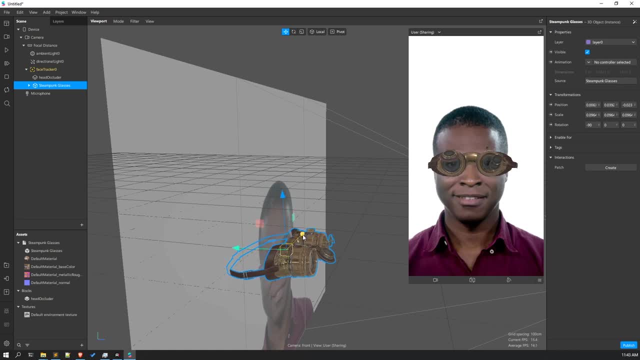 yeah, this, this definitely looks uh good, let's, uh, let's, uh, let's, uh, all right, all right, all right. okay, see, we can see his eyes also. so, okay, see, we can see his eyes also. so okay, see, we can see his eyes also. so now, now. 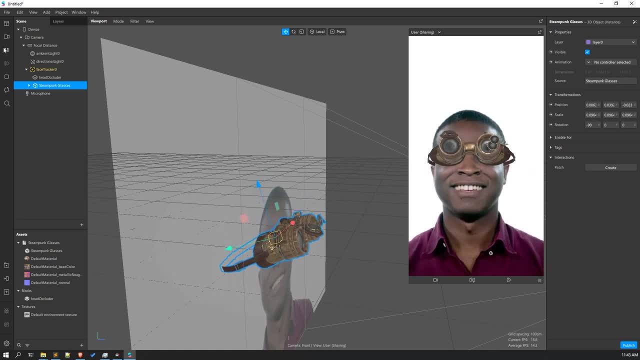 now this, this, this glasses are looking very good and we glasses are looking very good, and we glasses are looking very good and we actually have you know, actually have you know, actually have you know, set up, set up. set up means perfectly set up written there, means perfectly set up written there. 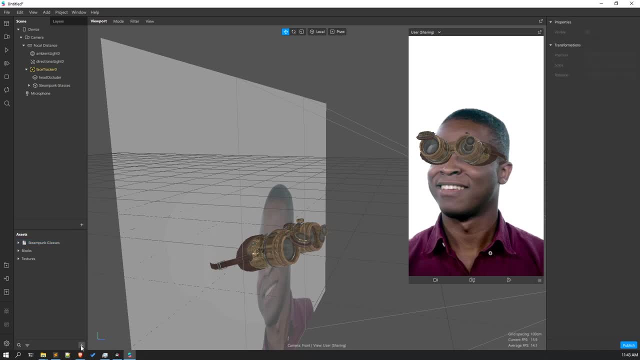 means perfectly set up written there, now, now. now, what i want you to do is add another. what i want you to do is add another. what i want you to do is add another asset that is going to be asset, that is going to be asset, that is going to be, you know, uh, a hat. 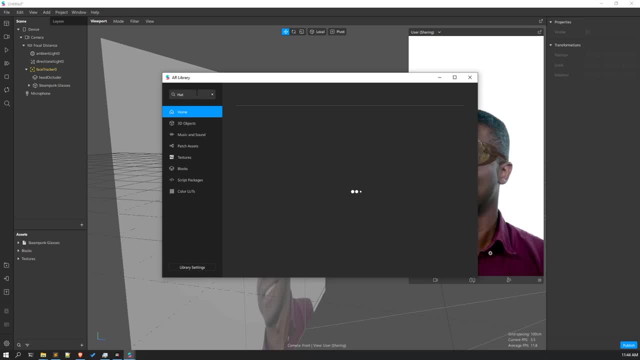 you know uh a hat. you know uh a hat, right or a cap, maybe right or a cap, maybe right, or a cap, maybe so, so, so, add any asset you want, all right, so so, so, let's go for this one, let's go for this one, let's go for this one. this seems a nice fit for this. 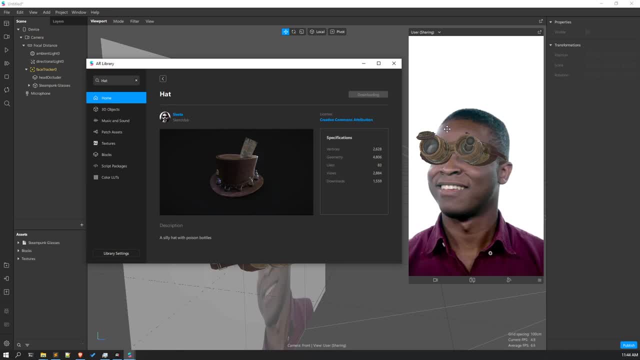 this seems a nice fit for this. this seems a nice fit for this. head right means for head right means for head right means for this. this, this, uh, uh, uh, what can i say? this particular glass, what can i say? this particular glass? what can i say? this particular glass, not head. 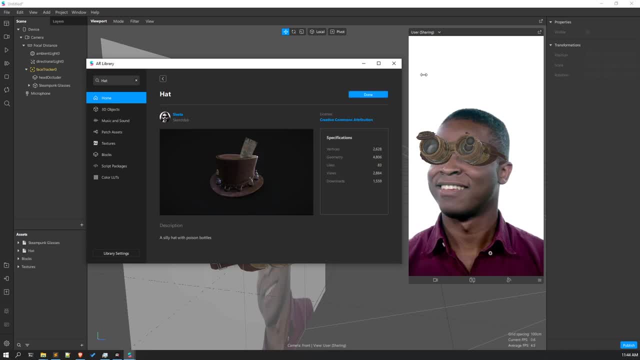 not head, not head. so just wait for it to download all. so just wait for it to download all. so just wait for it to download all right and right and right and cool. you got it now simply drag and cool. you got it now simply drag and cool. you got it now simply drag and drop it in here. 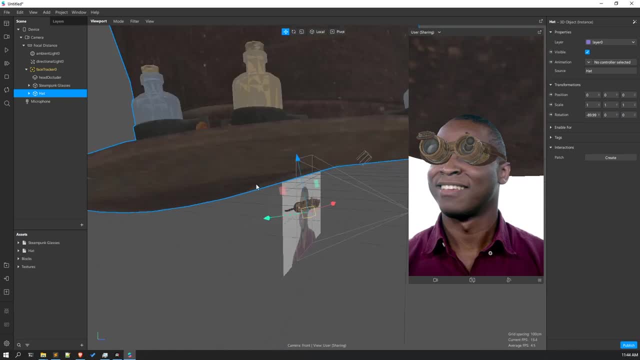 drop it in here. drop it in here, all right, all right, all right. make it a child of our favorite face. make it a child of our favorite face, make it a child of our favorite face: tracker, tracker, tracker, and. and now you know what to do. and and now you know what to do. 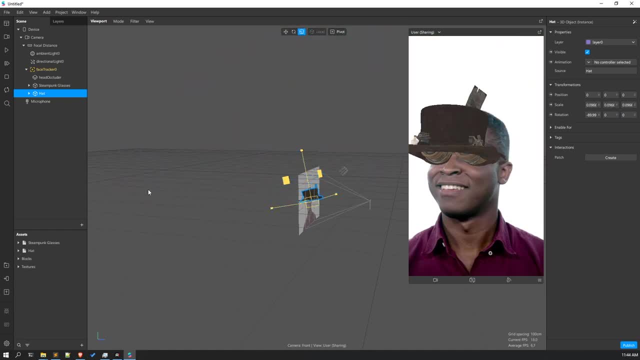 and and now you know what to do. scale it down, scale it down, scale it down, all right, scale it down cool. scale it down, cool. scale it down, cool. now move it a bit so that you know it. now move it a bit so that you know it. 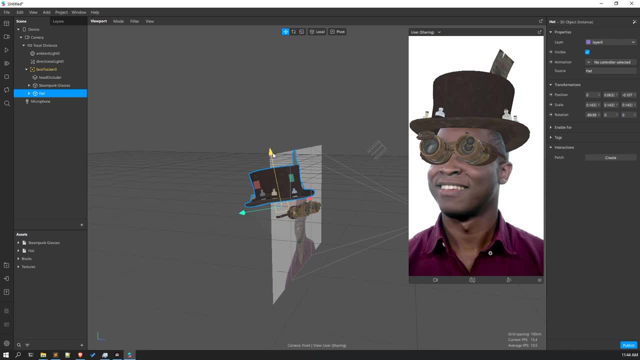 now move it a bit so that you know it gets adjusted on. okay, okay, okay, let's see now, let's see now, let's see now, yeah, this looks good, yeah, this looks good. yeah, this looks good, doesn't it doesn't it, doesn't it? yeah, it definitely looks good. 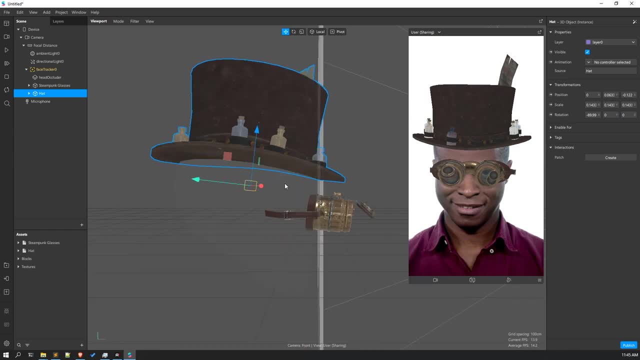 yeah, it definitely looks good. yeah, it definitely looks good now, um, now, um, now, um, just give me a few seconds. i guess, just give me a few seconds. i guess, just give me a few seconds. i guess, all right, so i need to make it a bit. all right, so i need to make it a bit. 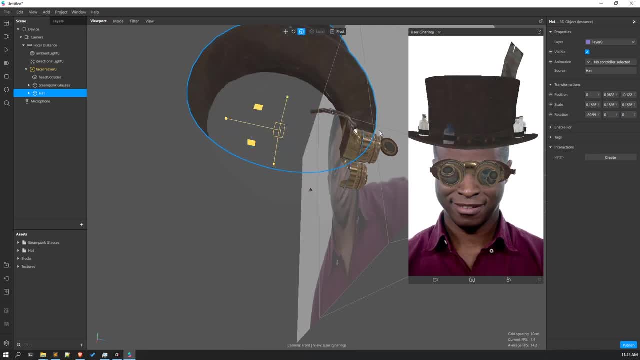 all right. so i need to make it a bit more, more, more. more bigger so that you know it. this cap bigger so that you know it. this cap bigger so that you know it. this cap fits this particular occluded face, fits this particular occluded face, fits this particular occluded face. all right, so 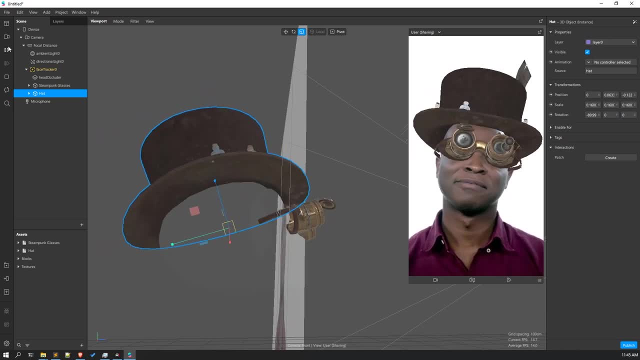 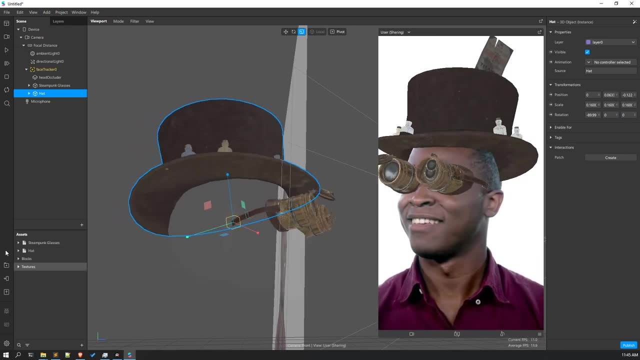 let's see now. let's see now. let's see now. okay, this looks, this looks very good. okay, this looks, this looks very good. okay, this looks, this looks very good. right, doesn't it right, doesn't it right? doesn't it all? right now let's see? all right. 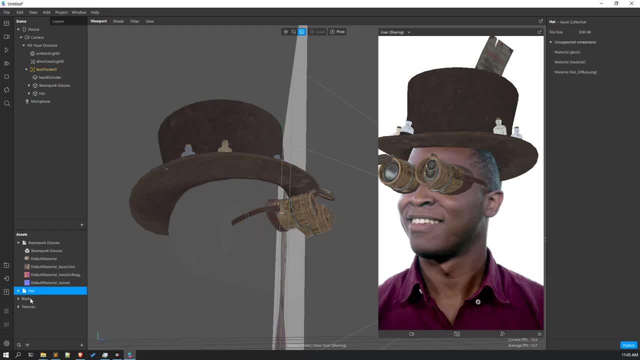 all right now, let's see: all right. all right now, let's see. all right, let's see if, uh, let's see if uh, let's see if uh, everything's working fine or not, everything's working fine or not, everything's working fine or not, all right, 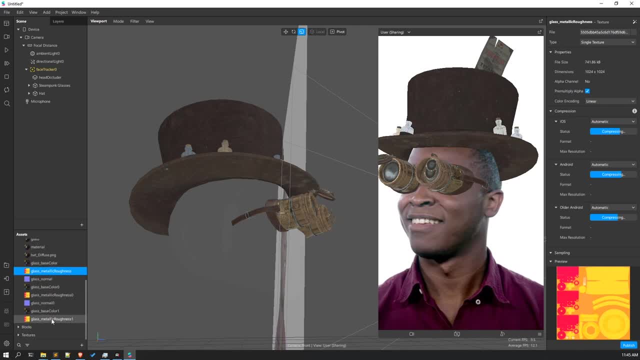 all right, all right, just okay, it's compressing. just okay, it's compressing. just okay, it's compressing. so i'm just going to you know, so i'm just going to you know, so i'm just going to you know, as of now, remove the whole compression. 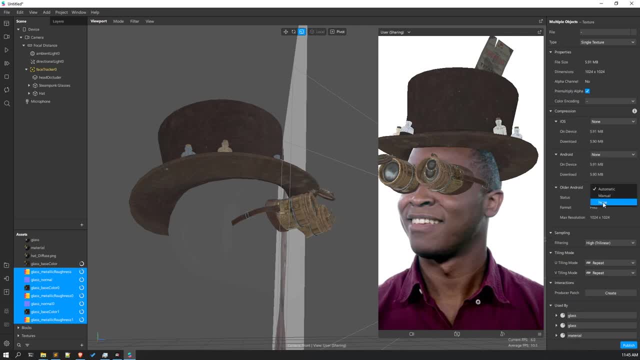 as of now, remove the whole compression. as of now, remove the whole compression thingy, thingy, thingy. of course it's. this thing is of. of course it's. this thing is of. of course it's. this thing is of 6mb and that is of. you know. 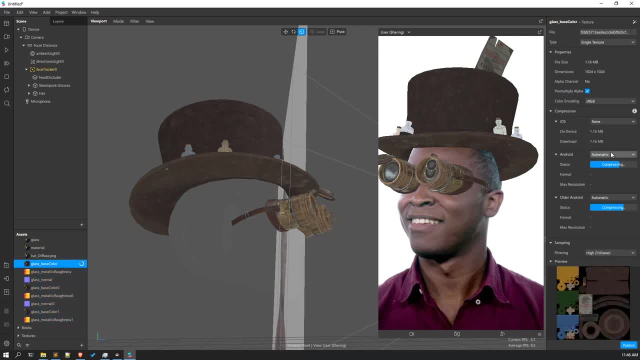 6mb and that is of you know 6mb and that is of you know four or four. i guess it was a 4mb, four or four. i guess it was a 4mb, four or four. i guess it was a 4mb right. so. 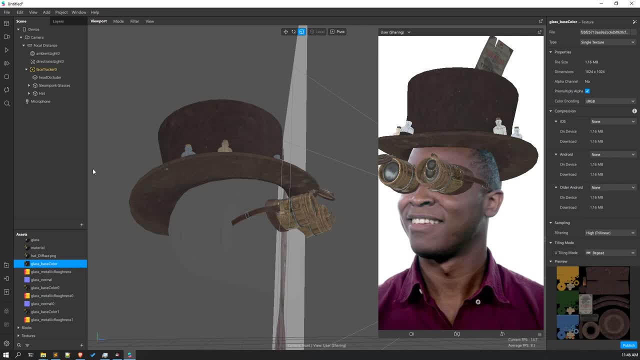 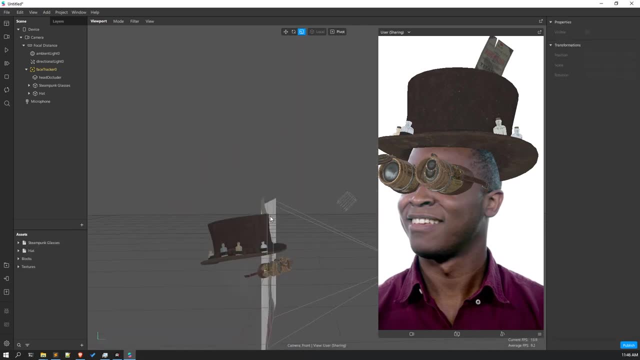 right, so right. so okay, it's of seven and we guaranteed so okay, it's of seven and we guaranteed so okay, it's of seven, and we guaranteed so means this one is of seven and b. so means this one is of seven and b. so means this one is of seven and b. so you know this, uh, particular model. so 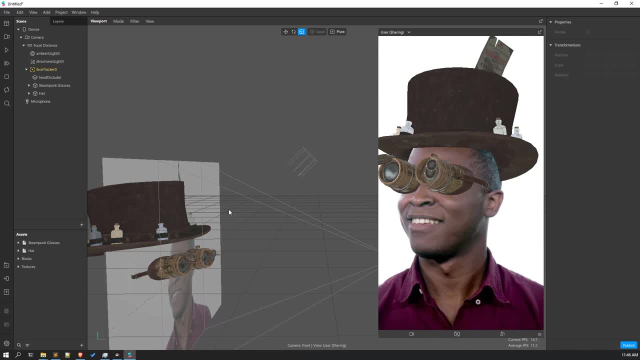 you know this uh particular model. so you know this uh particular model. so the to fix that problem is to compress the. to fix that problem is to compress the to fix that problem is to compress all right to let spark here compress. all right to let spark here compress. 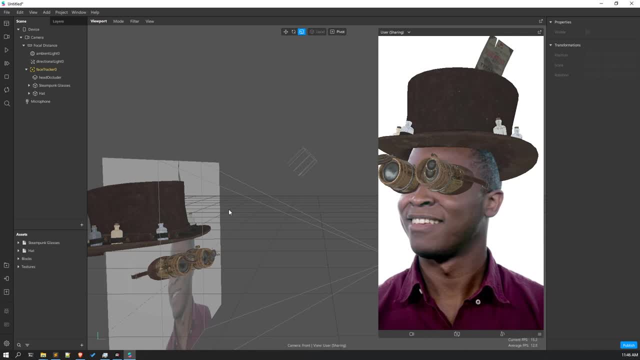 all right to let spark here, compress these particular. you know these particular. you know these particular. you know textures and models, and after that you textures and models, and after that you textures and models, and after that you can simply publish. it can simply publish, it can simply publish it right, and let's try this out and on. 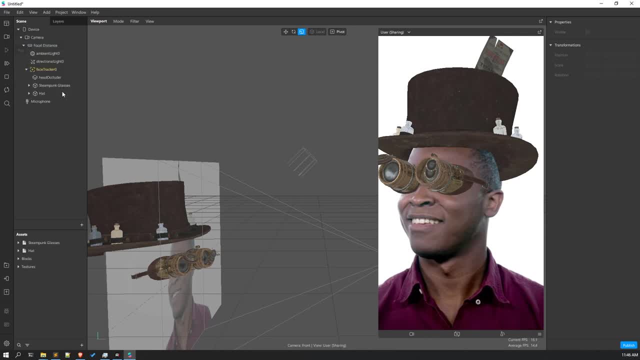 right, and let's try this out and on right, and let's try this out and on myself. all right, let's see myself. all right, let's see myself all right. let's see if it's if it's working or not. if it's if it's working or not. 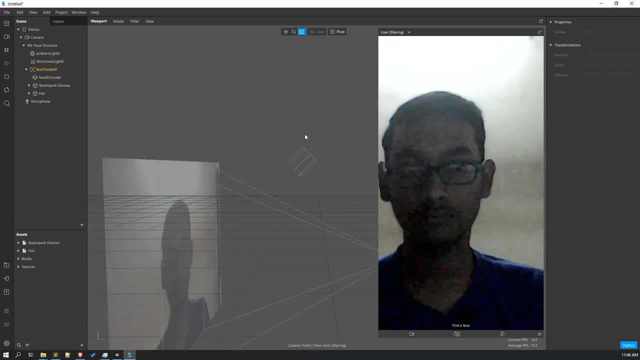 if it's, if it's working or not. all right, just let me you know. all right, all right, all right it's. i guess. because of the all right it's, i guess because of the all right it's, i guess because of the background light, it's not able to track. 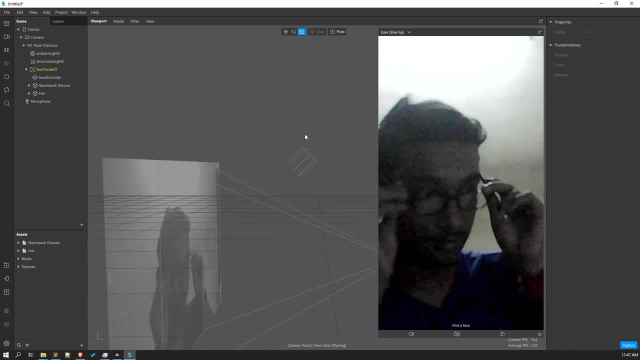 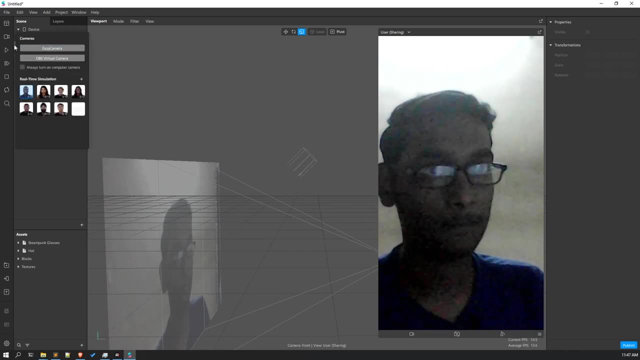 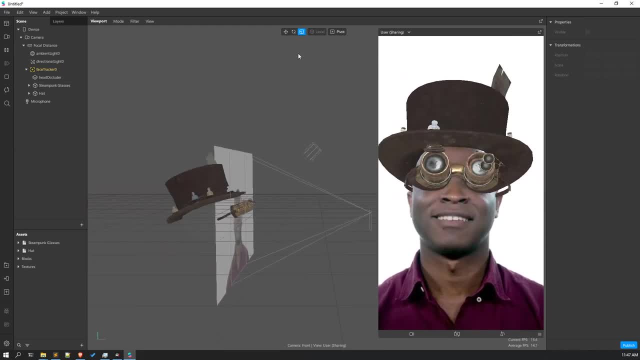 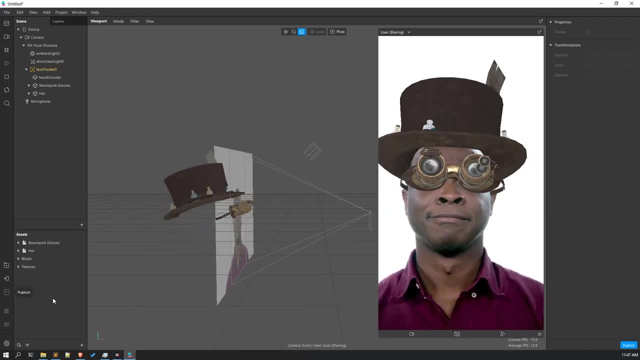 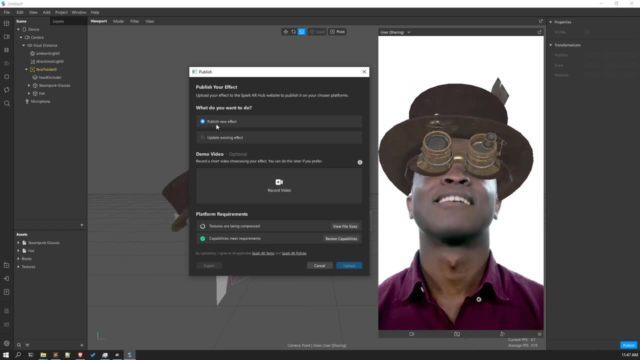 so now, if you want to publish it, what you have to do is have to do. is have to do is you have to click on this publish button. you have to click on this publish button. you have to click on this publish button. all right, then you know, click on this publish new. 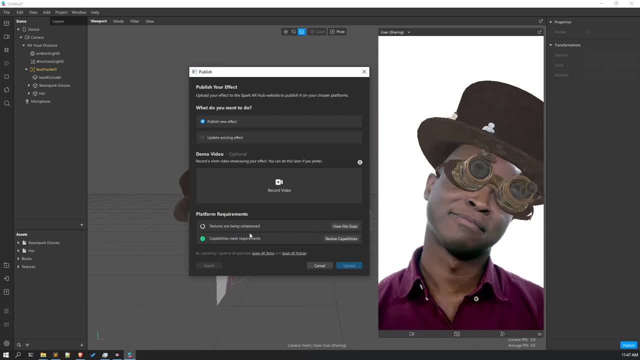 then you know, click on this, publish new. then you know, click on this, publish new effect. all right effect. all right effect, all right. and currently the text. you can see the. and currently the text. you can see the. and currently the text. you can see the textures are being compressed and 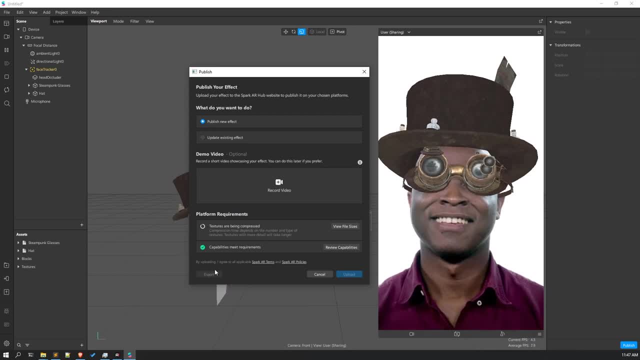 textures are being compressed and textures are being compressed and after the compression completes all. after the compression completes all, after the compression completes all. right, right, right. here an option you are finding that is here an option. you are finding that is here an option. you are finding that is called export. 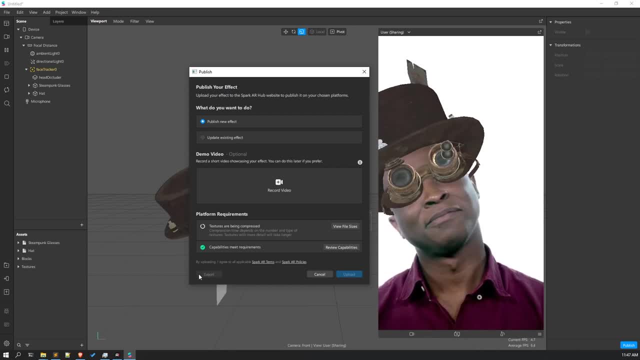 called export, called export. all right, you have to export this. all right, you have to export this. all right, you have to export this particular particular, particular file into one file. the extension will file into one file. the extension will file into one file. the extension will dot ar export after it is exported, all. 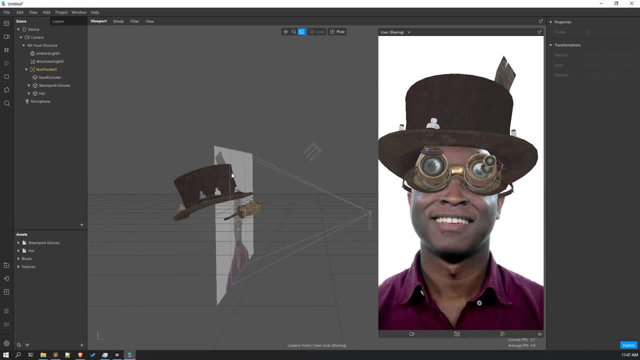 dot ar export after it is exported. all dot ar export after it is exported. all right, you have to go to a dashboard. all right, you have to go to a dashboard. all right, you have to go to a dashboard. all right, let me show you the dashboard. right, let me show you the dashboard. 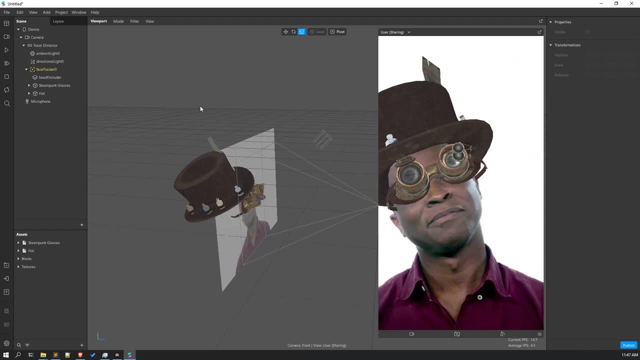 right, let me show you the dashboard. just give me a few seconds, let me pause. just give me a few seconds, let me pause. just give me a few seconds, let me pause this simulation. so this is the dashboard you can simply. so this is the dashboard you can simply. 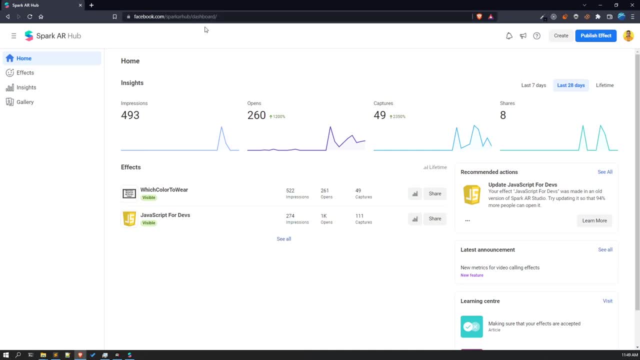 so this is the dashboard. you can simply go in there. facebookcom slash parker. go in there. facebookcom slash parker. go in there. facebookcom slash parker hub slash dashboard. so these are the two hub slash dashboard. so these are the two hub slash dashboard. so these are the two filters i made already. uh, this one was. 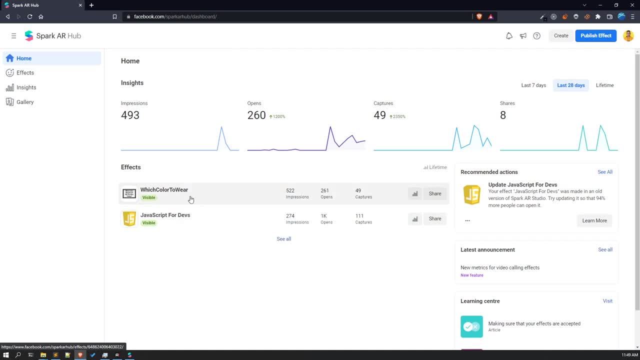 filters i made already. uh, this one was filters i made already. uh, this one was like, like like a long time ago. all right, i had some a long time ago. all right, i had some a long time ago. all right, i had some other filters also, but i deleted them. 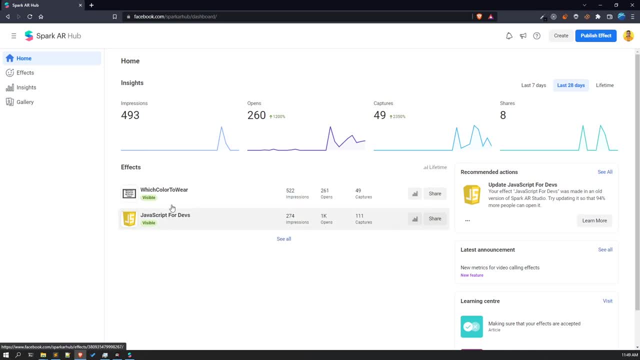 other filters also, but i deleted them. other filters also, but i deleted them. uh, so they are not here as of now. so, uh, so they are not here as of now. so, uh, so they are not here as of now. so these two are there, but, uh, this. 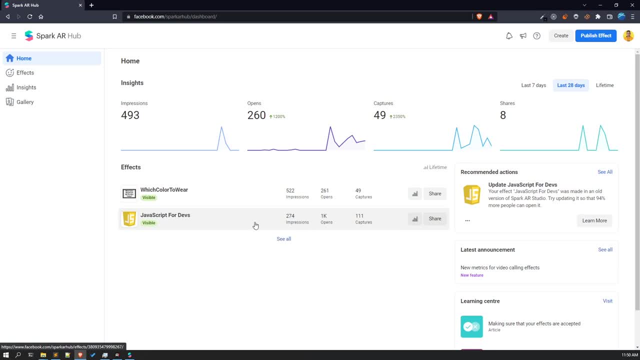 these two are there, but uh, this, these two are there, but uh, this javascript for diff doesn't really work. javascript for diff doesn't really work. javascript for diff doesn't really work because i haven't updated as of now. because i haven't updated as of now. 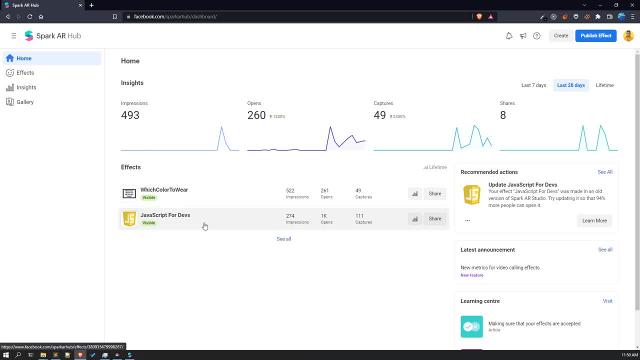 because i haven't updated as of now, because i i guess it's been almost one, because i i guess it's been almost one, because i i guess it's been almost one year. this was my very first filter all year. this was my very first filter all. 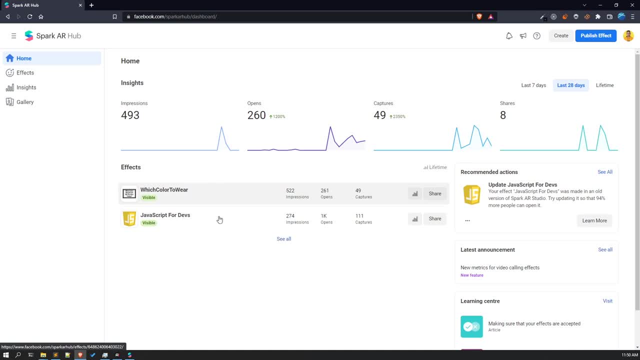 year. this was my very first filter. all right and this right and this right and this and this was. this was the one i and this was. this was the one i and this was. this was the one i recently made. this was a very old one. recently made. this was a very old one. 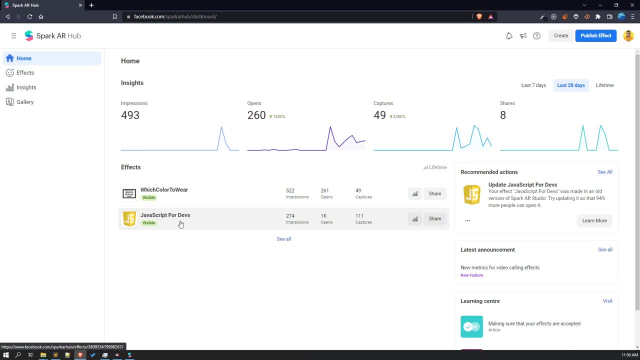 recently made. this was a very old one, like i haven't updated since. i guess it's like i haven't updated since. i guess it's like i haven't updated, since i guess it's been more than one year. yeah, been more than one year. yeah, been more than one year. yeah, so. 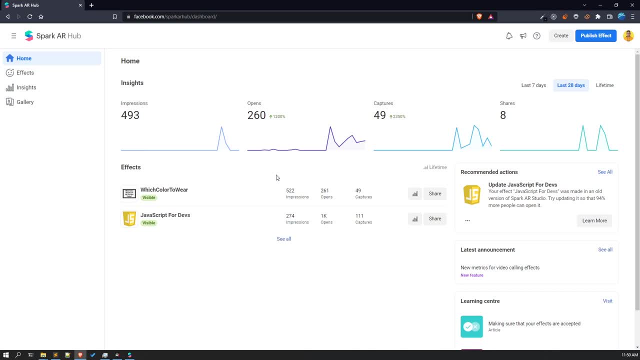 so. so i had other filters too, so i removed them. i had other filters too, so i removed them. i had other filters too, so i removed them. so i'm going to like i'm currently working, so i'm going to like i'm currently working, so i'm going to like i'm currently working on creating a whole new setup portfolio. 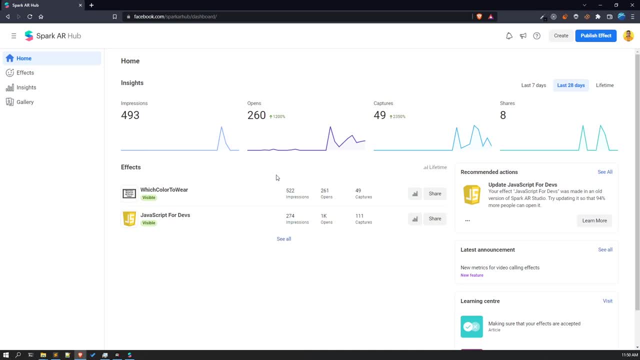 on creating a whole new setup portfolio, on creating a whole new setup portfolio of spark and ar application: so yeah, of spark and ar application. so yeah, of spark and ar application. so yeah. that's why i removed the previous ones. that's why i removed the previous ones. 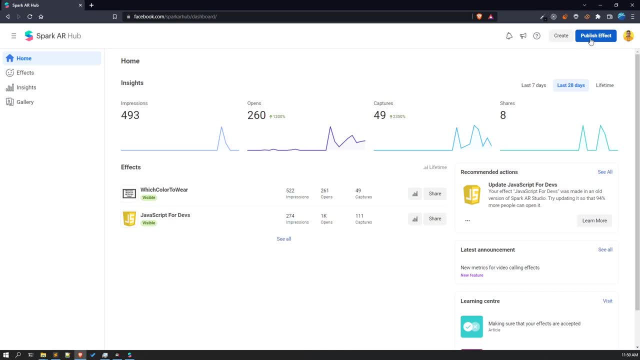 that's why i removed the previous ones. right, so now. what you have to do is right, so now. what you have to do is right, so now what you have to do is click on uh, you know, after you are. click on uh, you know, after you are. 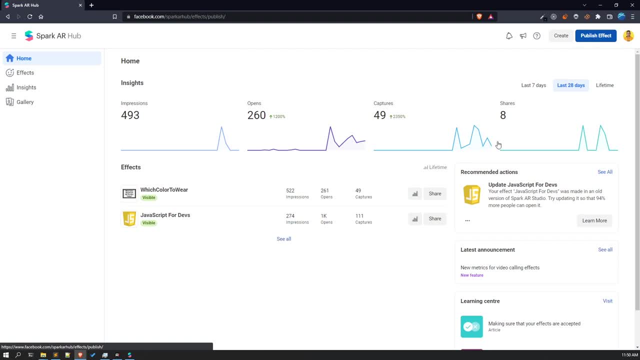 click on. uh, you know, after you are on the hub, you have to click on publish on the hub. you have to click on publish on the hub. you have to click on publish effect. all right effect. all right effect. all right, and a new window will appear. all right. 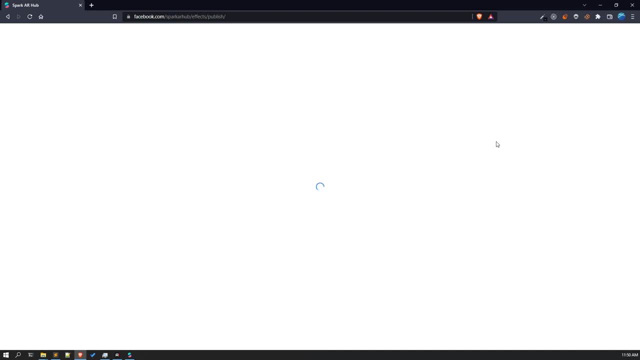 and a new window will appear all right, and a new window will appear all right. so just give it a few moments, all right. so just give it a few moments, all right. so just give it a few moments, all right, just give it a few seconds. and just give it a few seconds, and 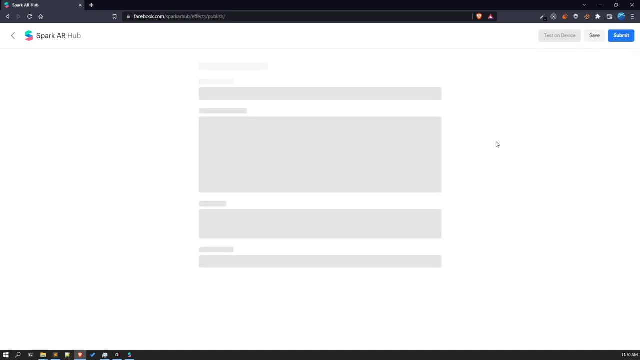 just give it a few seconds and it will open the window for you. it will open the window for you. it will open the window for you, all right, all right, all right, see. uh, make sure you export the see. uh, make sure you export the see. uh, make sure you export the. you know the filter asset. all right. 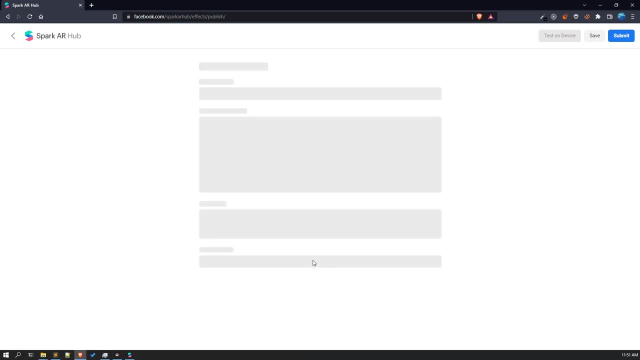 you know the filter asset, all right. you know the filter asset all right, because without that you won't be able, because without that you won't be able, because without that you won't be able to publish- to publish. to publish your filter, all right. okay, cool, see, first of all, uh. 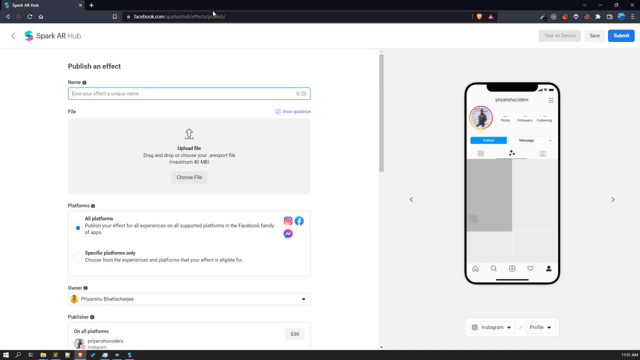 okay, cool, see first of all. uh, okay, cool, see first of all. uh, you have to give a name to your filter. you have to give a name to your filter. you have to give a name to your filter. all right, so you can give any name to a. 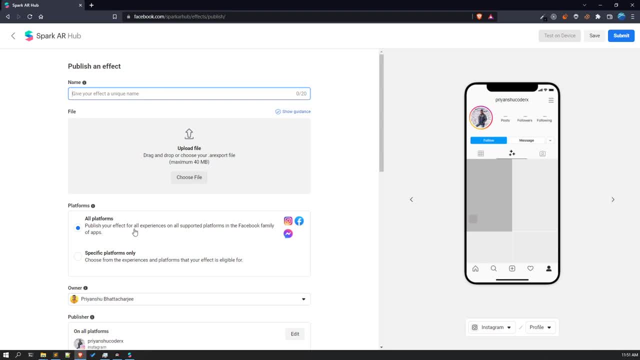 all right, so you can give any name to a. all right, so you can give any name to a filter. if you are filter, if you are filter, if you are going to upload the filter that i showed, going to upload the filter that i showed, going to upload the filter that i showed you in the 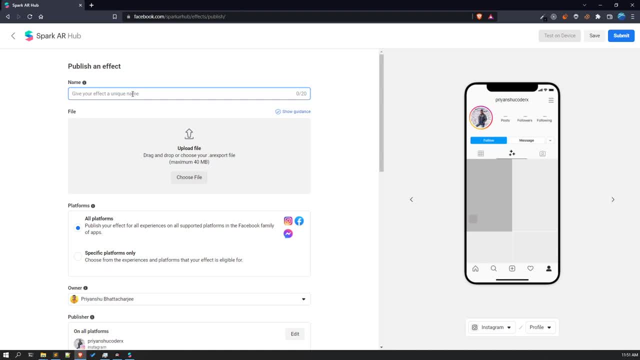 you in the, you in the project, what you can do is you can. i would project what you can do, is you can. i would project what you can do, is you can. i would like to name it weird. like to name it weird. like to name it weird, uncle, maybe i'm not sure, i'm not really. 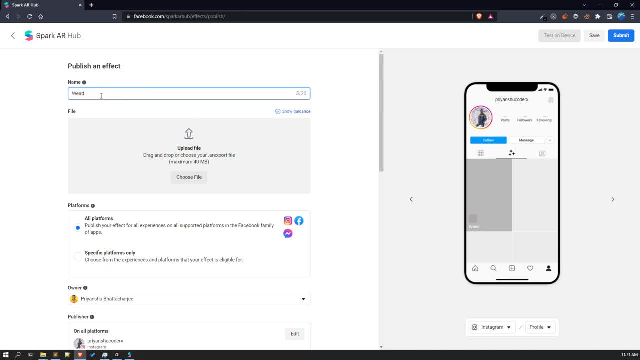 uncle, maybe i'm not sure i'm not really uncle, maybe i'm not sure i'm not really good at good at good at naming. all right, i'm, i might name it uh naming. all right, i'm, i might name it uh naming. all right, i'm, i might name it uh weird uncle. 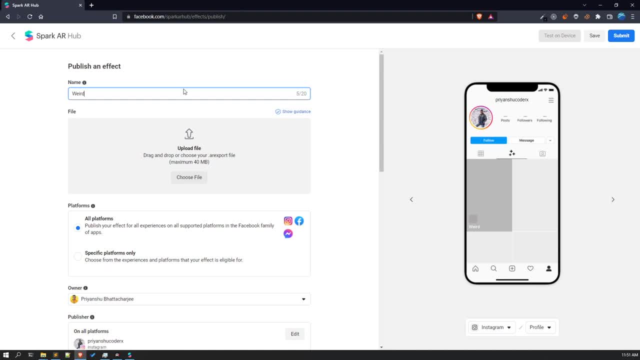 weird uncle. weird uncle, all right, i might name it. all right, i might name it. all right, i might name it weird uncle, you can. you can name it weird uncle, you can. you can name it weird uncle, you can, you can name it anything you want. right after that, when 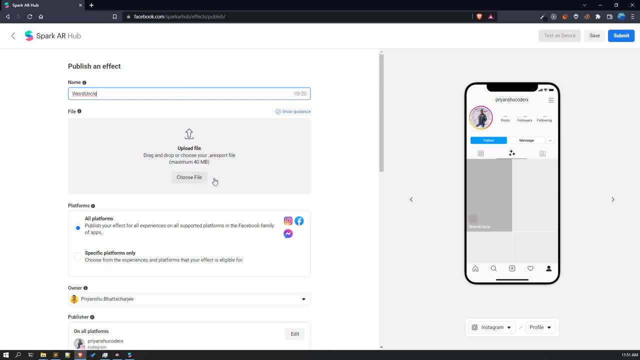 anything you want right after that, when anything you want right after that, when you uh after exporting: all right, you, you uh after exporting, all right, you. you uh after exporting, all right, you will be getting a filear export file. will be getting a filear export file. 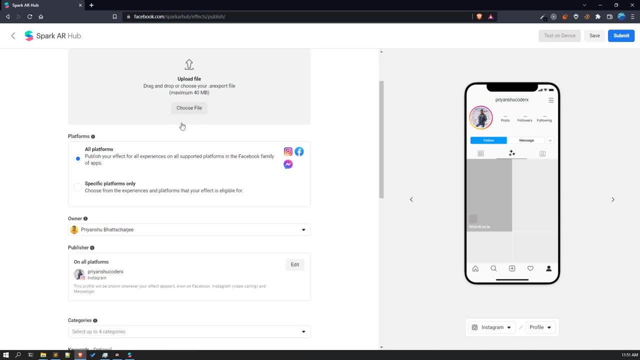 will be getting a filear export file. all right, simply drag and drop that file. all right, simply drag and drop that file. all right, simply drag and drop that file in here and make sure the file in here and make sure the file in here and make sure the file is less than 40 mb. all right, the size of. 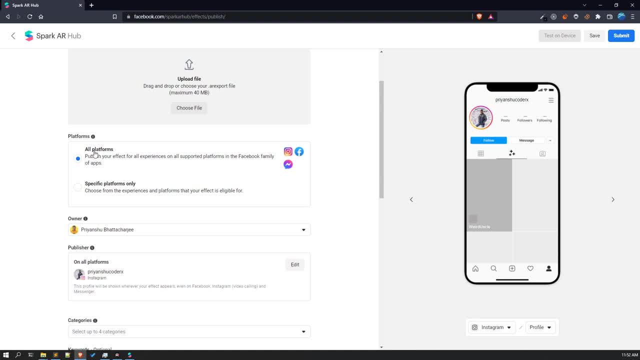 is less than 40 mb, all right. the size of is less than 40 mb, all right. the size of the file is less. the file is less. the file is less 40 mb and i would suggest you to choose 40 mb and i would suggest you to choose. 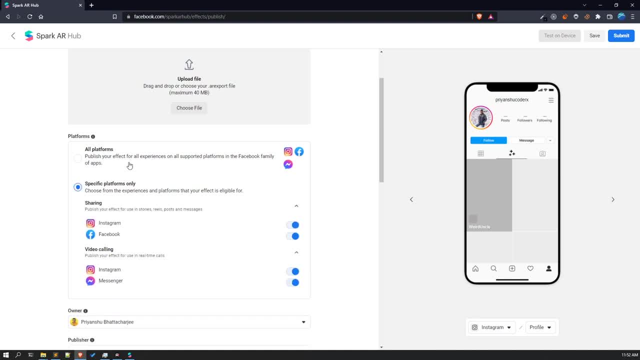 40 mb and i would suggest you to choose all platforms, or if you just want to all platforms, or if you just want to all platforms, or if you just want to, like you know, upload or the filter only like you know, upload or the filter only like you know. upload or the filter only on. 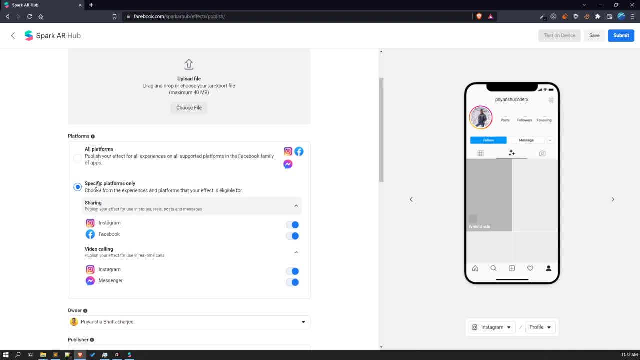 on on instagram. you can disable the facebook instagram. you can disable the facebook instagram. you can disable the facebook messenger and all the things from here messenger and all the things from here messenger and all the things from here. all right, but currently i wanted to. all right, but currently i wanted to. 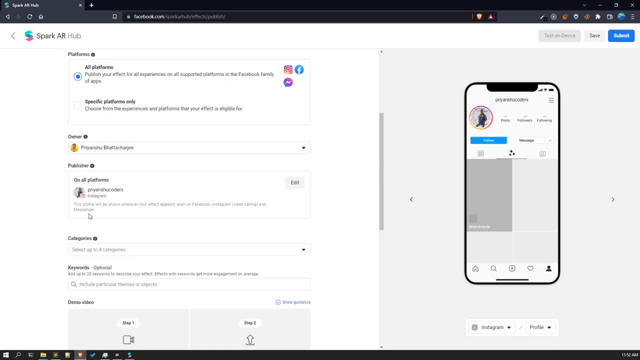 all right, but currently i wanted to publish it on all platforms. publish it on all platforms. publish it on all platforms. the owner is Priyanshu Bhattacharjee. the owner is Priyanshu Bhattacharjee. the owner is Priyanshu Bhattacharjee. right, uh, this is the publisher. that is. 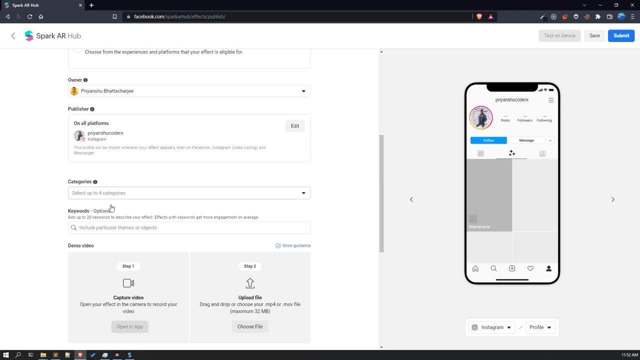 right. uh, this is the publisher. that is right. uh, this is the publisher, that is. the publisher is on my instagram account. the publisher is on my instagram account. the publisher is on my instagram account. here are the categories you can select. here are the categories you can select. 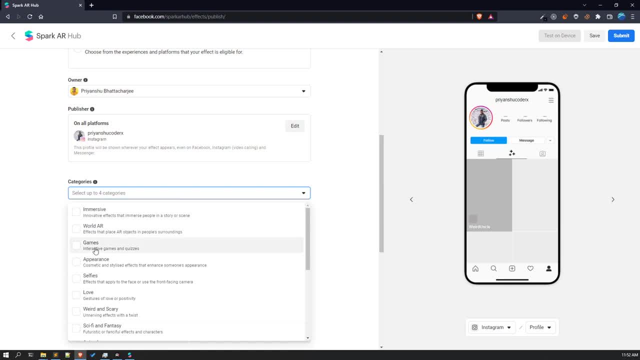 here are the categories. you can select the categories: all right, the categories: all right. the categories: all right. like it? what kind of uh like it? what kind of uh like it? what kind of uh is it? it can uh, it is of sci-fi, and is it? it can uh? it is of sci-fi, and 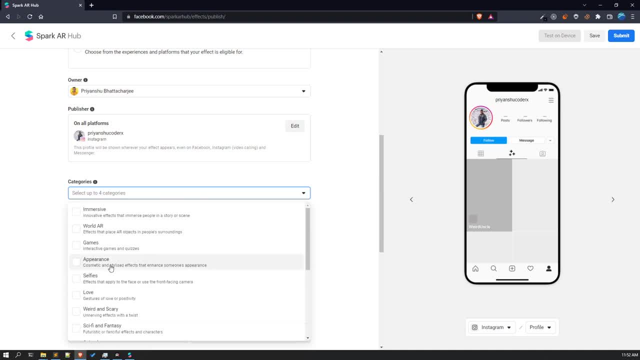 is it? it can? uh, it is of sci-fi and fantasy. of course it looks like fantasy. of course it looks like fantasy. of course it looks like something from fantasy. right, it can be something from fantasy? right, it can be something from fantasy? right, it can be of selfies. 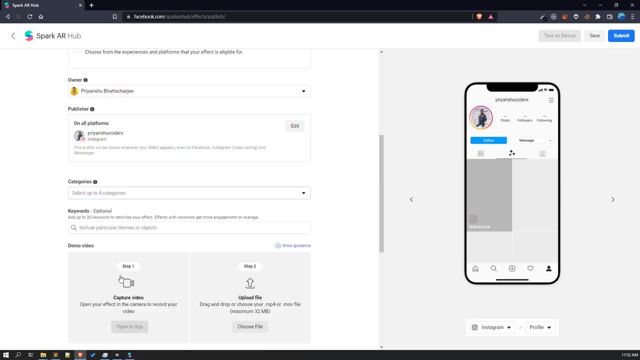 of selfies, of selfies. all right so. and also, you can, all right so. and also, you can, all right so. and also you can like select the weird and scale because, like select the weird and scale, because, like select the weird and scale, because weird is, in its name, only right and 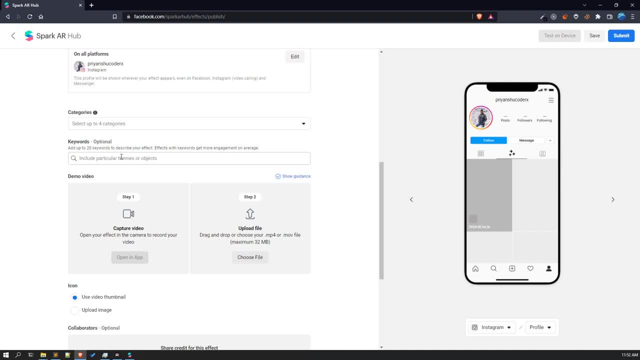 weird is in its name only right, and weird is in its name only right. and after that, you uh. after that, you uh, after that, you uh, for you know, for, you know, for you know, for enhancing the search you, you have to, for enhancing the search you, you have to. 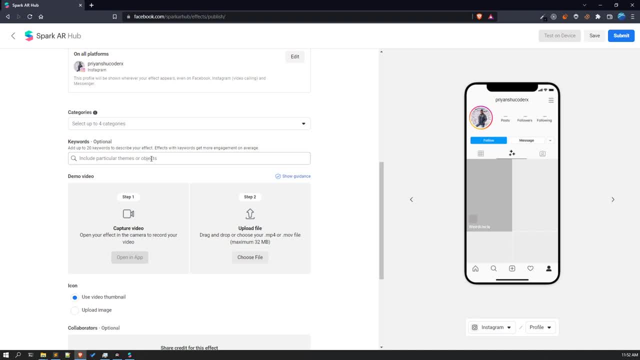 for enhancing the search. you you have to add some, add some, add some. you should actually add some uh keywords. you should actually add some uh keywords. you should actually add some uh keywords in there, all right and uh in there, all right and uh in there, all right and uh. also one thing: 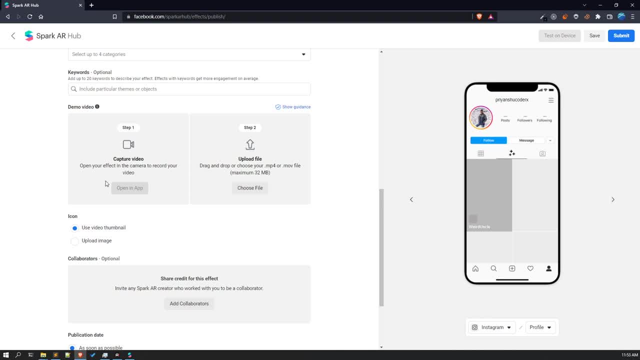 also one thing. also one thing: what you have to do is you have to record. what you have to do is you have to record. what you have to do is you have to record: all right, you have to record the all right, you have to record the all right, you have to record the filter. 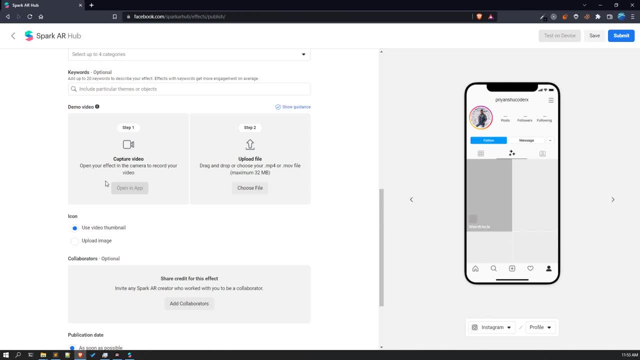 filter filter. all right, you have to record the filter on. all right, you have to record the filter on. all right, you have to record the filter on your phone, your phone, your phone, uh, and upload the uh uh. and upload the uh uh. and upload the uh means 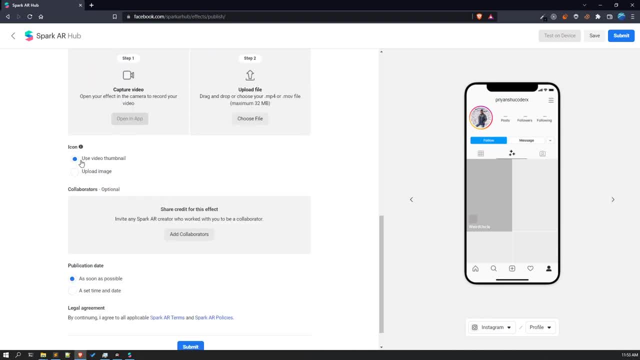 means means the video in here- all right and up after the video in here- all right and up. after the video in here- all right and up. after that, you can use the. that you can use the. that you can use the video thumbnail- all right, and video thumbnail: all right and. 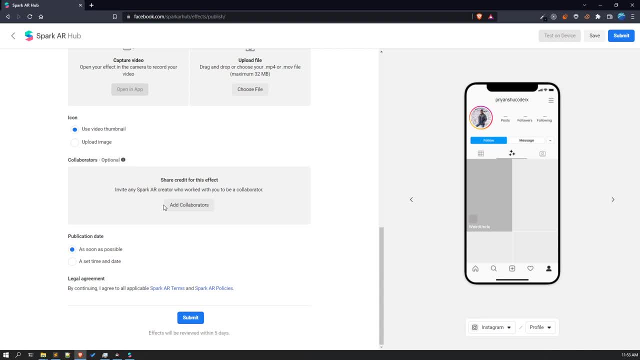 video thumbnail. all right, and if you, if, if you have collaborated with, if you, if, if you have collaborated with, if you, if, if you have collaborated with some other people also during the, some other people also during the, some other people also during the possible and as uh asset, time and date. 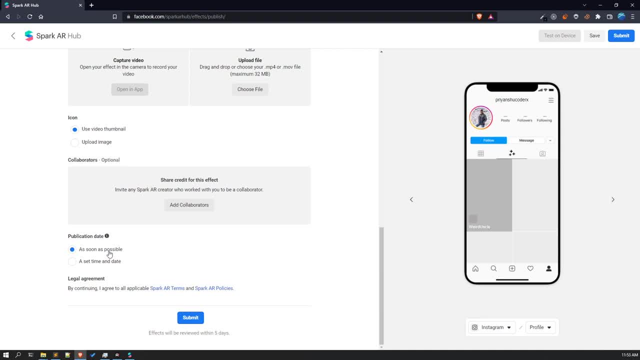 possible and as uh asset time and date possible and as uh asset time and date, so you can't do any of this. all right, so you can't do any of this. all right, so you can't do any of this. all right. as soon as possible means uh, i generally. 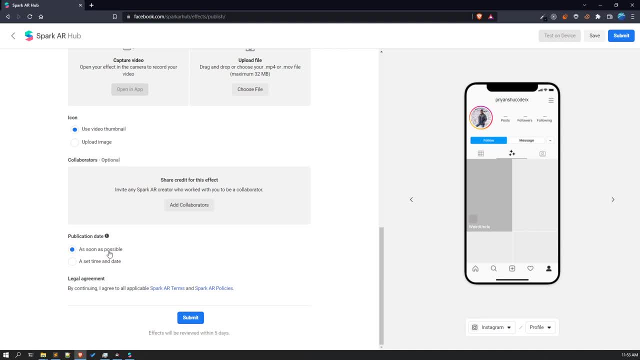 it is. it gets like it takes around three to four hours, or i think it may be even to four hours, or i think it may be even to four hours, or i think it may be even less than that. they publish that filter. less than that, they publish that filter. 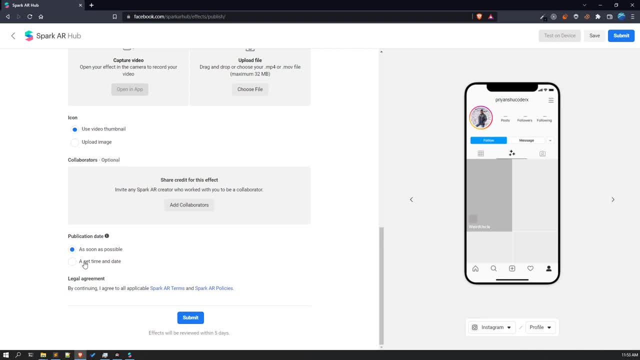 less than that, they publish that filter instantly. so that is one way, and instantly so that is one way, and instantly so that is one way, and otherwise you can simply set a particular. otherwise you can simply set a particular. otherwise you can simply set a particular date and time when you want your filter. 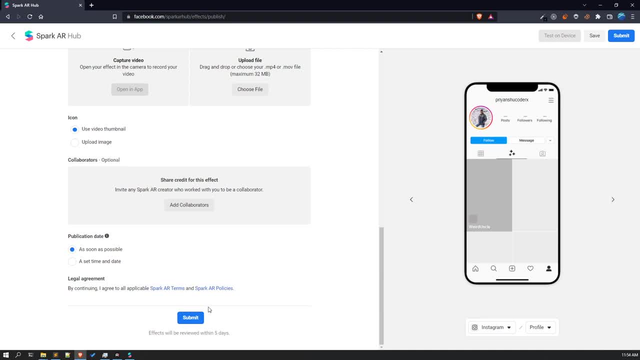 date and time when you want your filter. date and time when you want your filter to be published- all right. and they don't to be published, all right. and they don't to be published, all right. and they don't take a lot of time to verify the filter. 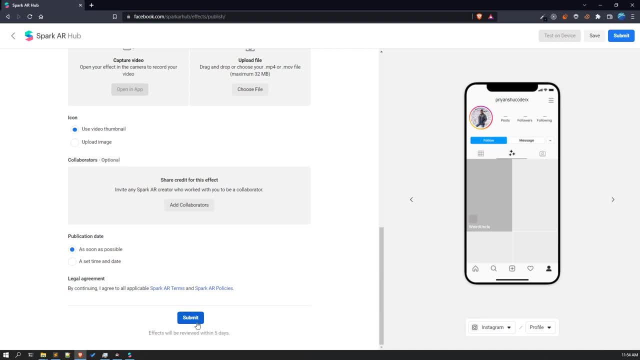 take a lot of time to verify the filter. take a lot of time to verify the filter, all right, and then click on submit and all right, and then click on submit and all right, and then click on submit and your filter will be out for review and your filter will be out for review. and. 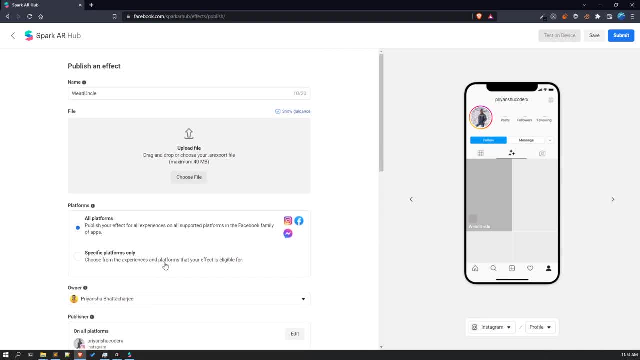 your filter will be out for review and after it is reviewed, after it is reviewed, after it is reviewed, if everything success, if everything is, if everything success, if everything is, if everything success, if everything is successful, successful, successful. you will be able to. you know, you will be able to, you know. 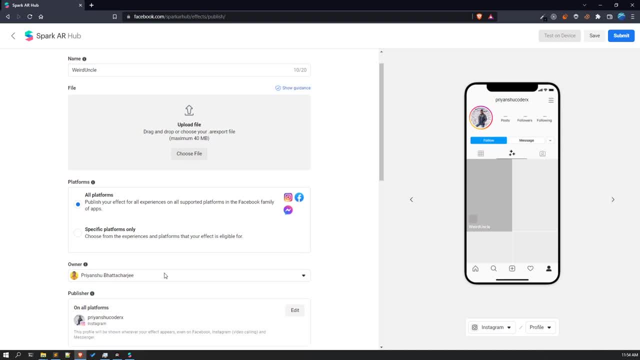 you will be able to. you know, user means distributor filters on all. user means distributor filters on all. user means distributor filters on all the platforms right. and one more thing: the platforms right. and one more thing: the platforms right. and one more thing: while recording the video, make sure the 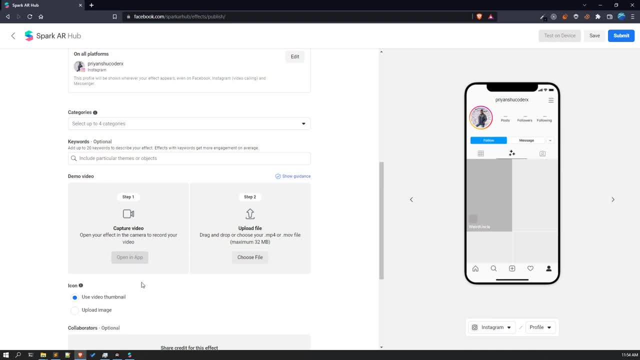 while recording the video, make sure the. while recording the video, make sure the video of uh, video of uh, video of uh. you are recording. you are recording. you are recording the video of yourself only because uh the video of yourself, only because uh the video of yourself, only because uh spark. 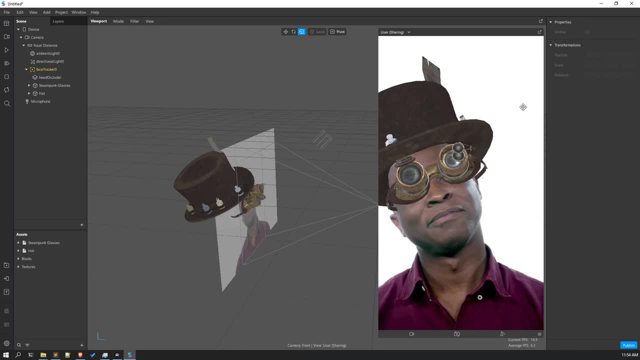 spark, spark, spark. here has a policy of not using their. spark here has a policy of not using their. spark here has a policy of not using their. you know their presets means you can't use. you know their presets means you can't use. you know their presets means you can't use these presets. all right, the presets. 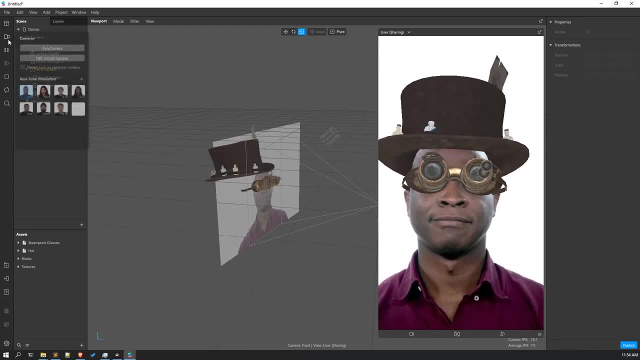 these presets. all right, the presets. these presets, all right, the presets. like this uncle. uh is like this uncle. uh is like this uncle. uh is you, you, you, like you. you can't record this uncle. like you, you can't record this uncle. like you. you can't record this uncle using your filter, right, you can. 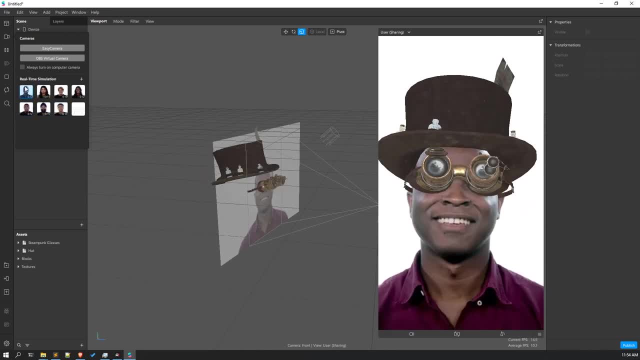 using your filter, right you can. using your filter, right you can. you can't record any of them, any of the. you can't record any of them, any of the. you can't record any of them. any of the filters in here to record it. filters in here to record it. 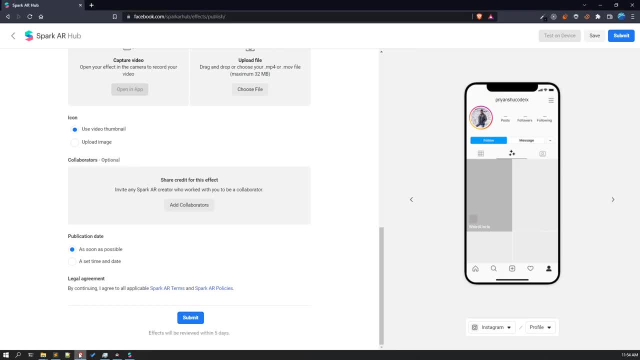 filters in here to record it right, so you have to record all the right. so you have to record all the right. so you have to record all the assets by yourself, assets by yourself, assets by yourself. right, so you have to record the video by right. so you have to record the video by. 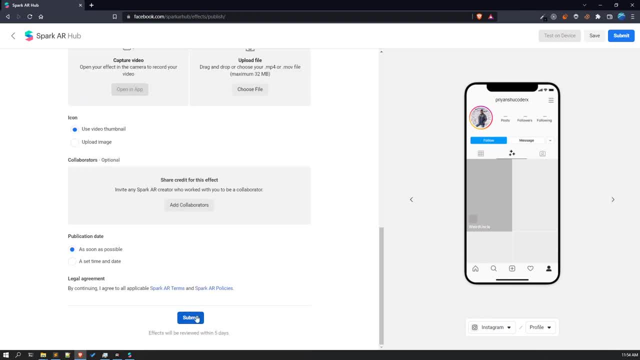 right, so you have to record the video by yourself. all right, so make sure you do yourself. all right, so make sure you do yourself. all right, so make sure you do that and that and that and great, and also one more thing don't use. great, and also one more thing don't use. 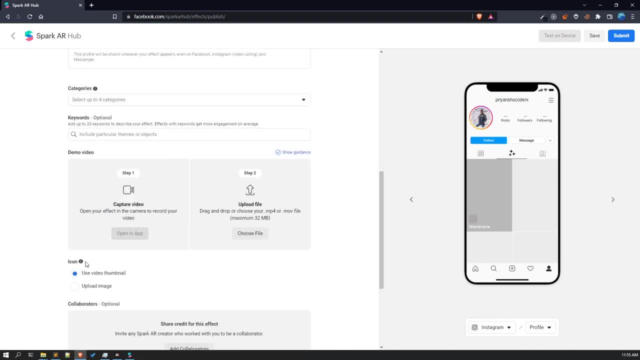 great. and also one more thing: don't use face- all right, your face, as uh you know. face, all right, your face, as uh you know. face, all right, your face, as uh you know- as the icon of or logo of this particular, as the icon of or logo of this particular.